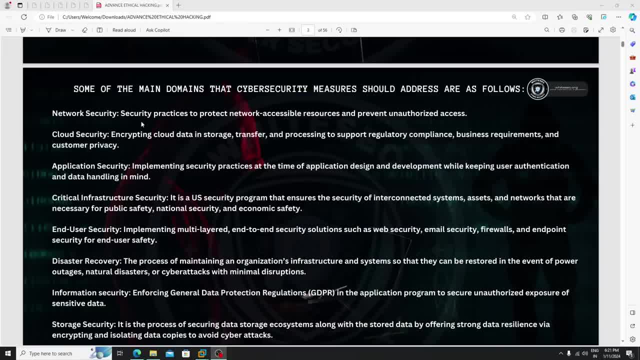 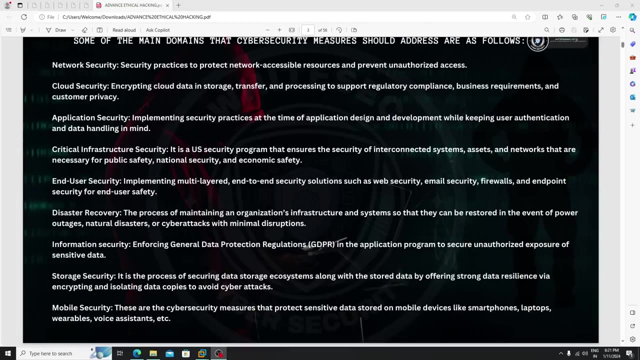 address are as follows: network security: security practice to protect network accessible resources and prevent unauthorized assets. cloud security: encrypting cloud data in storage, transfer and processing to support regulatory compliance, business requirements and customer privacy. and here, application security: implementing security practice at the time of application design and development, while keeping user authentication. 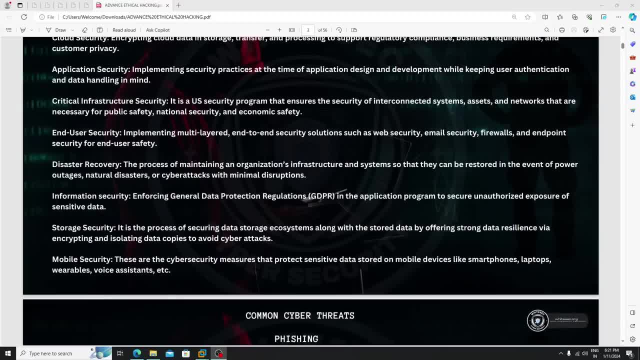 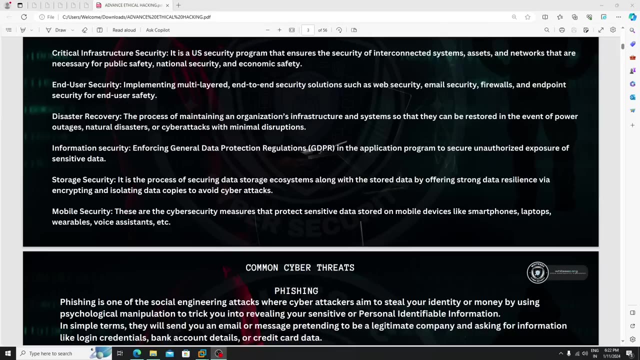 and data handling in mind. now there is a critical infrastructure security. it is a us security program that ensure the security of interconnected systems, assets and networks that are necessary for public safety, national security and economic safety safety. and there is a end user security, implementing multi-layered end-to-end security solutions such 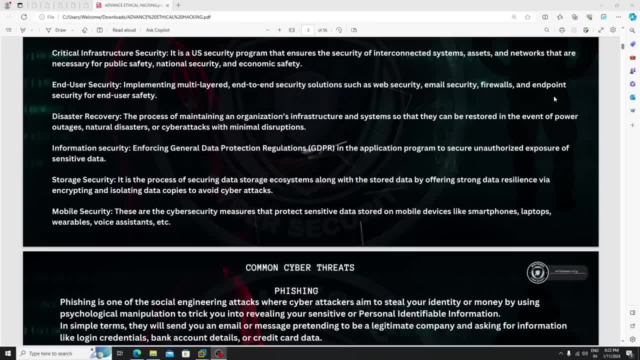 as web security, email security, firewalls and endpoint security for end user safety. what is the end user safety? just take an example of whatsapp. you are using the whatsapp, right? you are a end user here. okay, now there is a disaster recovery: the process of maintaining and maintaining an. 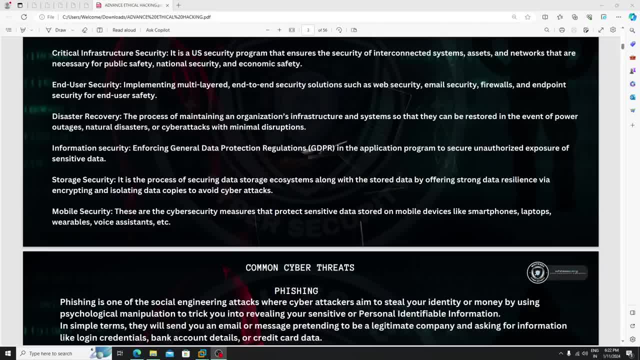 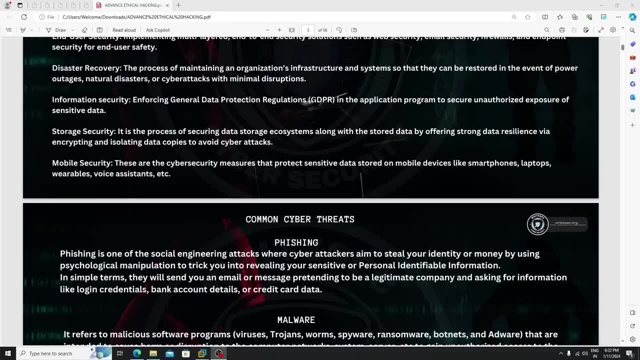 organization, infrastructure and system so that they can be restored in the event of power outage, natural disaster or cyber attacks with minimal disruption. information security: enforcing general data protection regulations, which is known as a gdpr in the application program to secure unauthorized exposure of sensitive data. see everything. 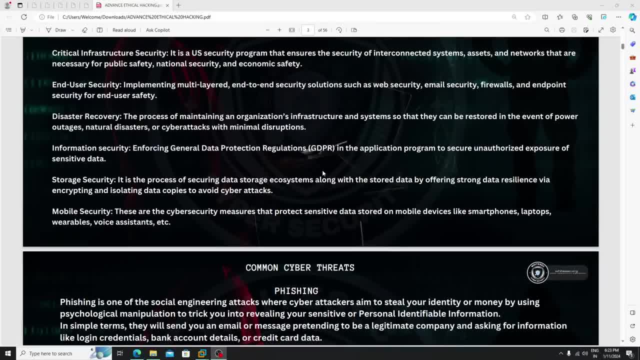 here is a huge topic, right. so the thing is, we are just learning the starting things here. that's it. if you do cissp or cc or cism, at the time, you will learn these things here. okay, uh, it's a complete see in cyber security. what will happen means: 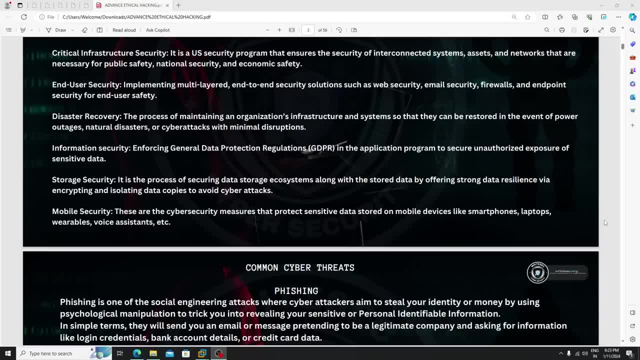 cyber security mostly focus on theory, part right, how to secure it, how to, how to think it. okay, like uh, like simple, how uh, here in the pentesting and hacking what we do, we work as an attacker here, right, but in cyber security, what we do, we think. 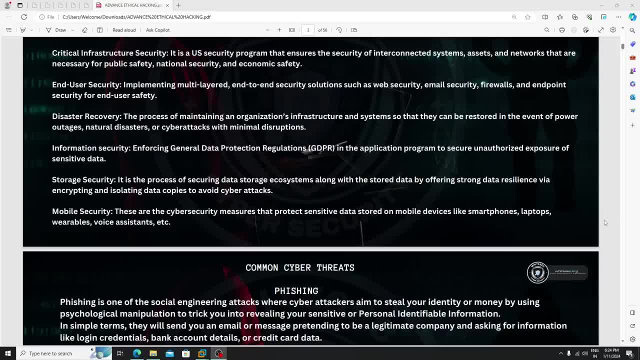 okay, how to uh if the attack will happen, how we need to react. okay, this is the thing which we do. we also perform some kind uh this uh firewall installation. this kind of serves, but mostly here uh only the editing. okay, that's it. now there is a storage security. it is a process of securing data. 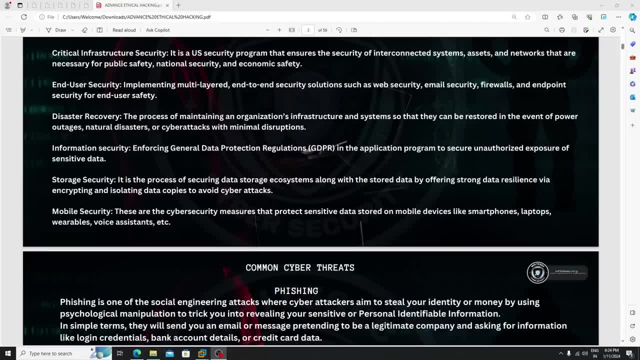 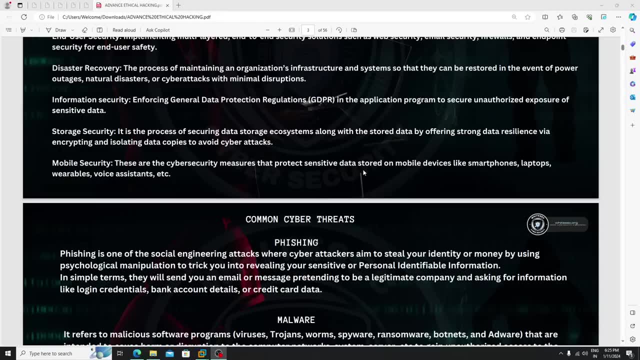 storage ecosystem, along with the stored data, by offering store uh strong data resilience via encrypt, encrypting and isolating data copies to avoid cyber attacks. now there is a mobile system security. these are the cyber security measures that protect sensitive data stored on mobile device like smartphones, laptops, variable like watches, voice assistants, etc. 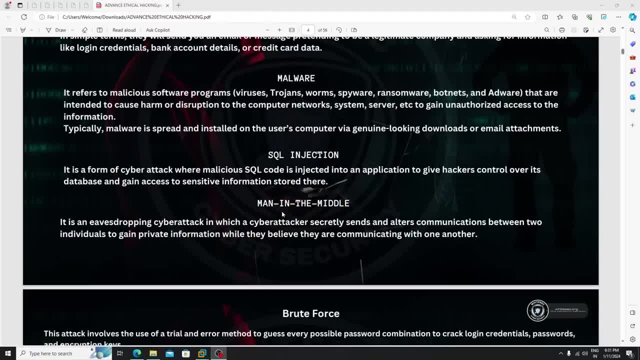 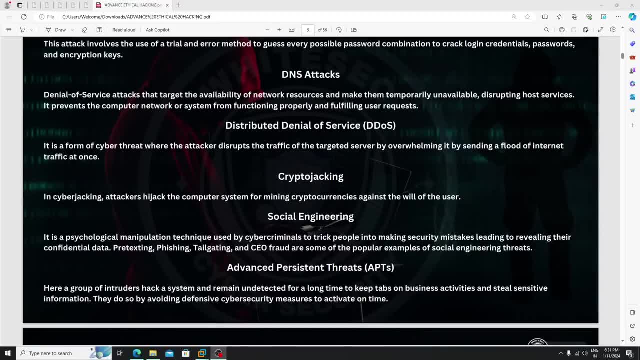 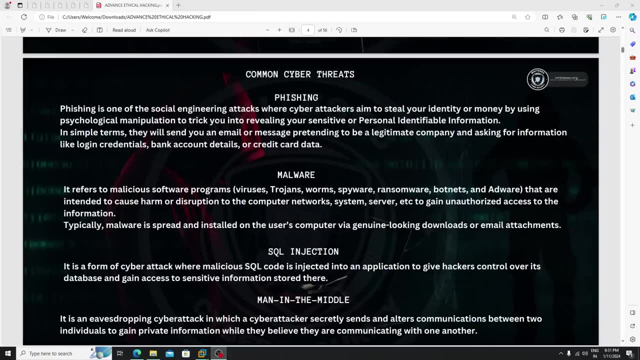 there is a common cyber threats, which is phishing, marvel, sql injection, man in the middle, brute force, dns attack, distributed denial of service, crypto jacking, social engineering, advanced persistent threats, which is apts. see, we just covered. this all serves in ethical just. uh, with practical as well. okay, just try to watch the training, which is around 16 hours. i. 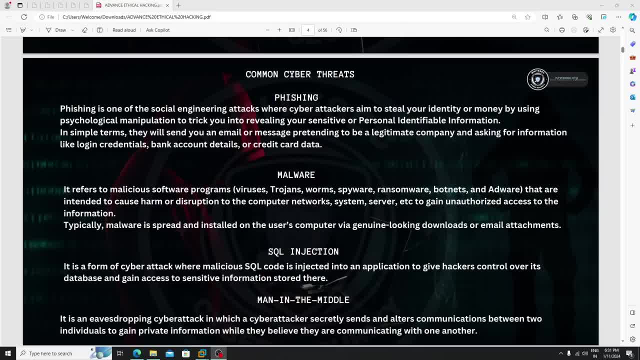 think, just watch it and just do the practice. see here phishing. you know the definition, what is phishing, what phishing can able to do. and also you need to do the practical as well. just do create a lab, uh, perform the attack on your own, on your own email. do the things and see that things as well. ok, 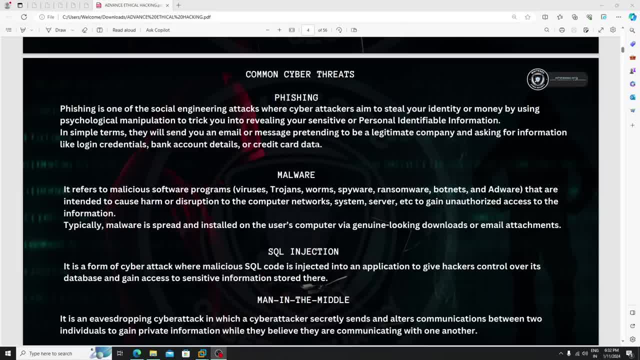 don't go with definition, only just try to do the things practically as well in your own lab. don't, uh, do this process in real world, okay. if you don't have permission, then don't do it. in ethical hacking training, we just learn the rules. what are the rules? okay, each and everything and also watch it. 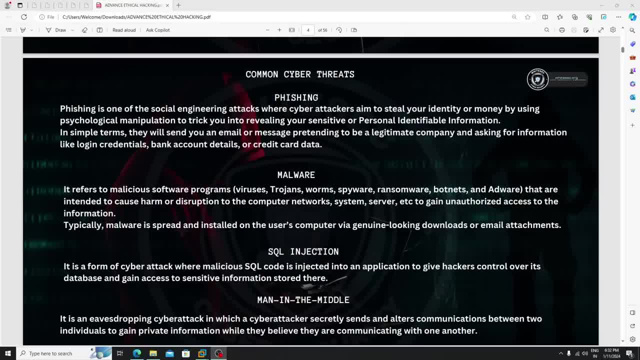 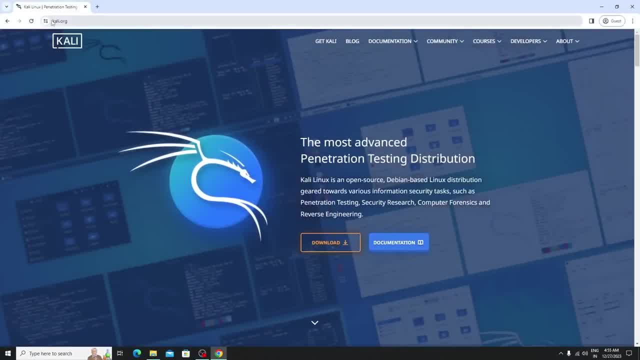 okay, right, hope you guys enjoy this classes. thank you, have a nice day. hello everyone. hope you are fine. in this classes we are learning how we can able to set up the attacker machine. to set up the attacker machine, you just need to visit this url: khalidorg. 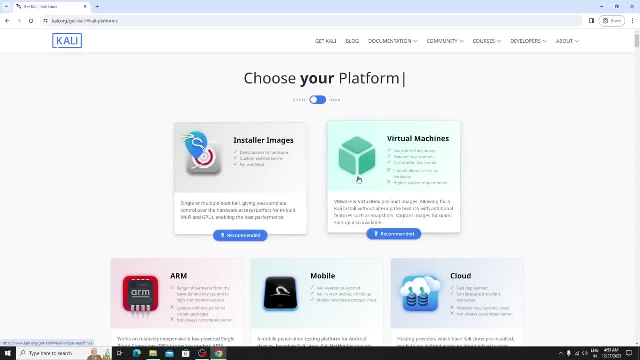 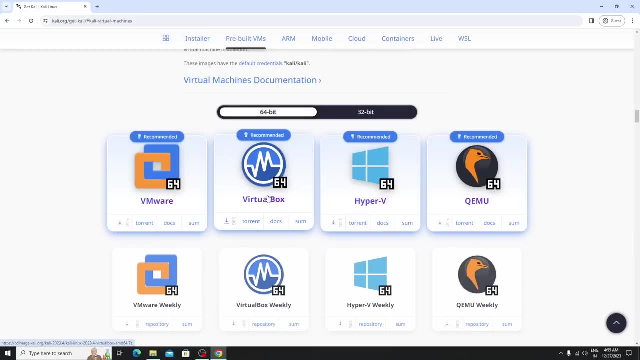 visit this url: khalidorg. simple click on download, just select this virtual machines and here download for vmware. if you want to use a virtual box, you can also use it. okay, if you don't know about virtual box, what you need to do means in this youtube channel, okay, you guys can able to see one training, okay, one course, which. 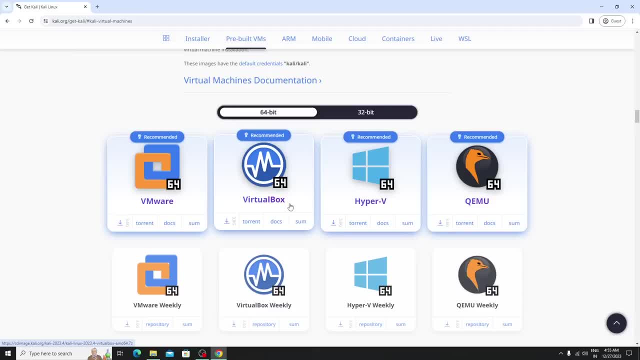 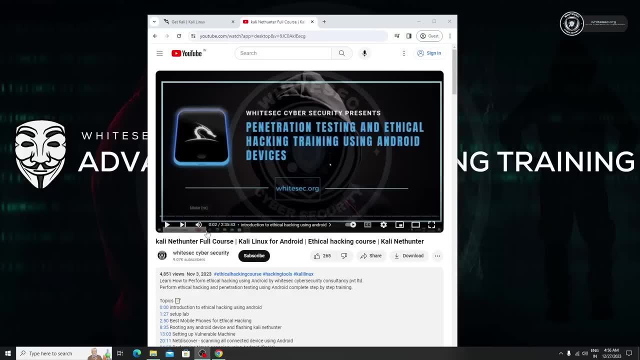 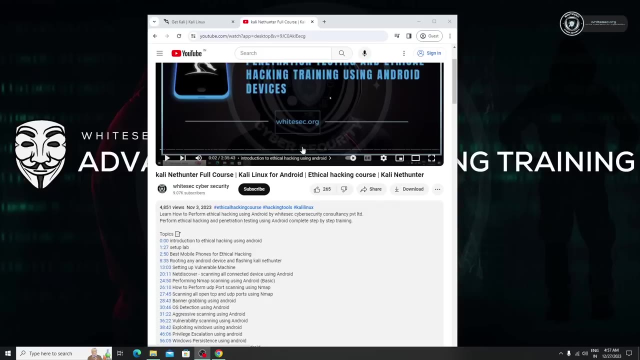 which is a nethunter course: hacking using nethunter. i don't know the title, just wait. just watch this course, which is kali nethunter- full, full course. here you can able to see setup lab. just watch this section. okay, so you will learn how you can able to. 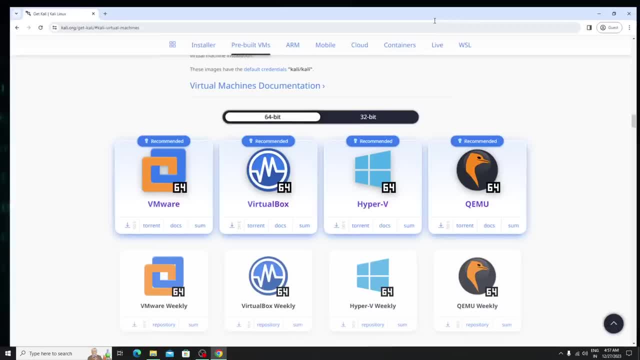 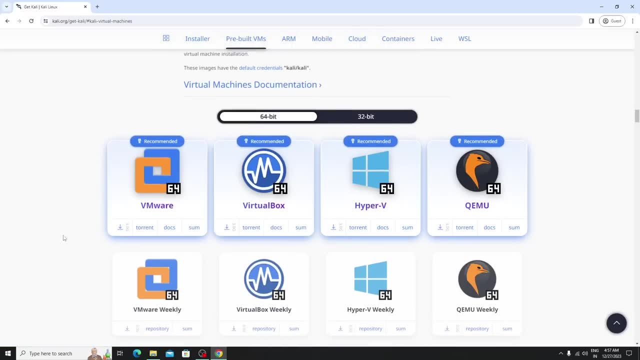 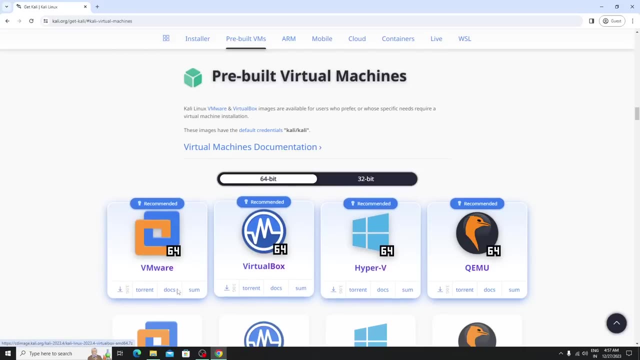 set up the virtual machines. okay, sorry, virtual box, how you can able to use a kali linux in virtual box, right? so simple thing is what you need to do. click on right now i am using the- uh, the vmware one. simple, just download it. it's around 3 gb. just download it and also see here. just focus right now. 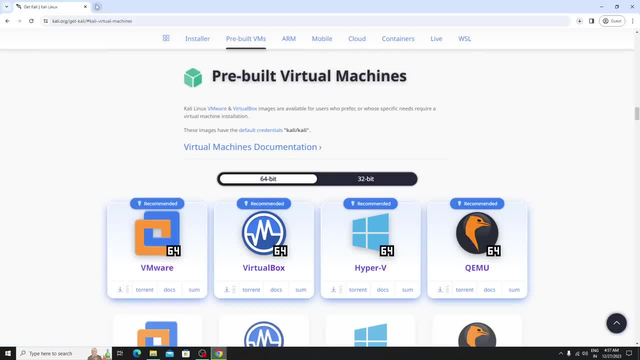 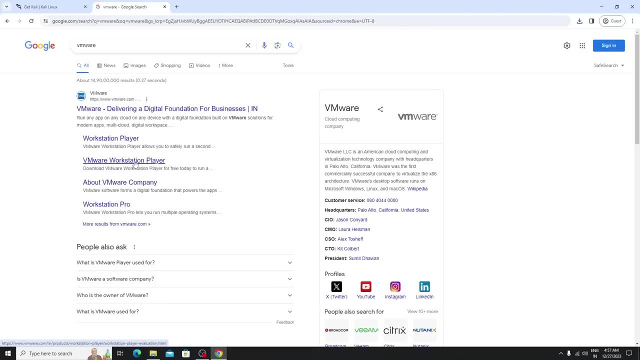 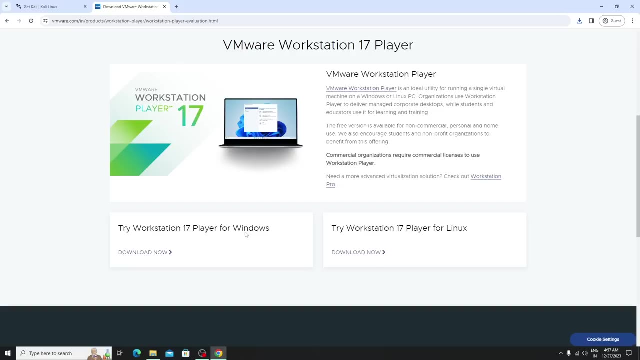 i am using for vmware. right, you need to download the vmware here. simple, just search for vmware and here you guys can able to see vmware workstation player. simple, open this link and from here you need to download it. okay, it's a try. workstation 17 player for windows. 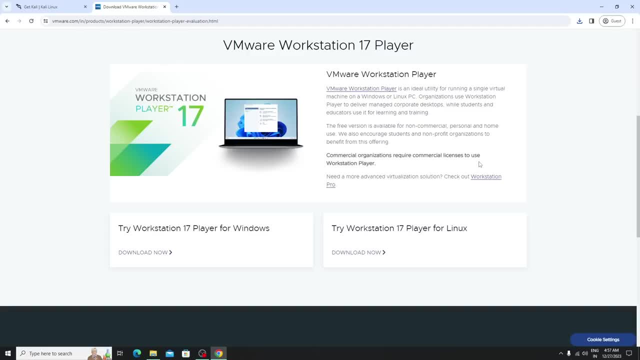 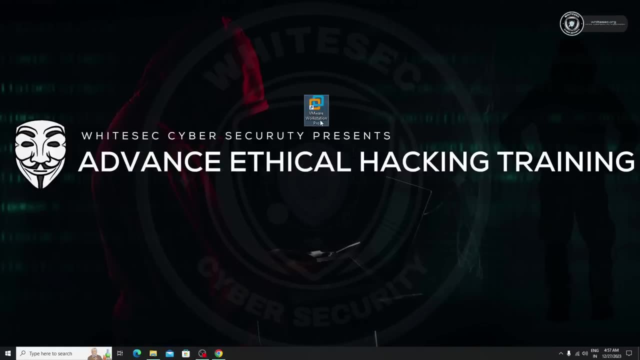 simple: download it and just install it. it's a normal setup, just simple. just type next, next, next and install it. okay, it's not a big deal. now, here see, i already installed, uh, the vmware workstation pro. uh, majority of people will think that it's need any kind of key or something like that. no, 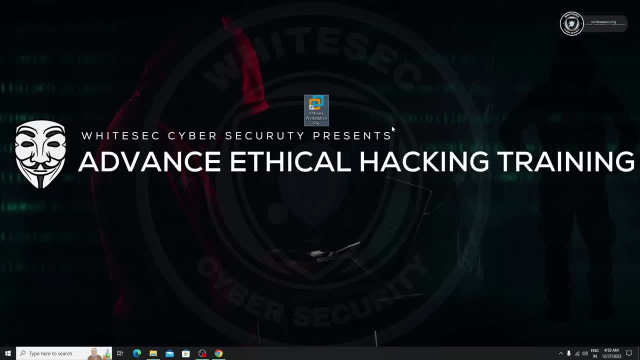 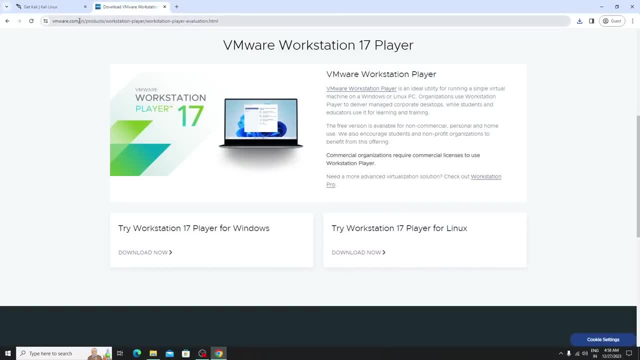 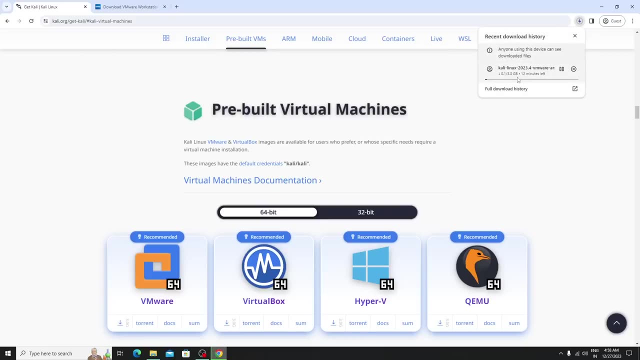 it doesn't require, okay, uh, you can go with a free one as well. okay, it's not a big deal now here, i already installed the vmware workstation. now let's wait for this one to download. just wait, see, i just told you right, it's around 3 gb. 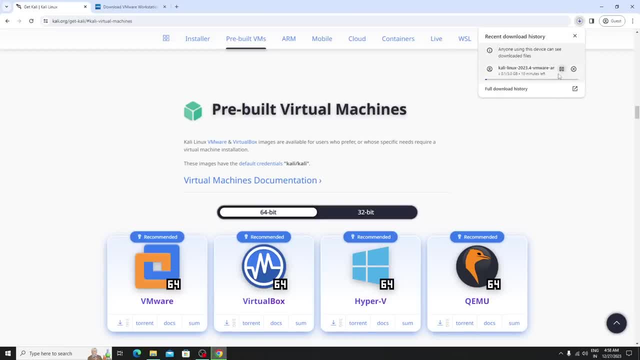 it will take around 10 minutes or something like that. just let me connect with my vpn. it might be fast, just wait. it will take around 10 minutes or something like that. just let me connect with my vpn, it might be fast, just wait. so here it is. 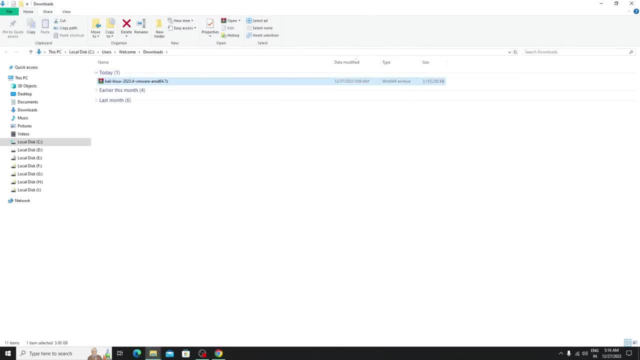 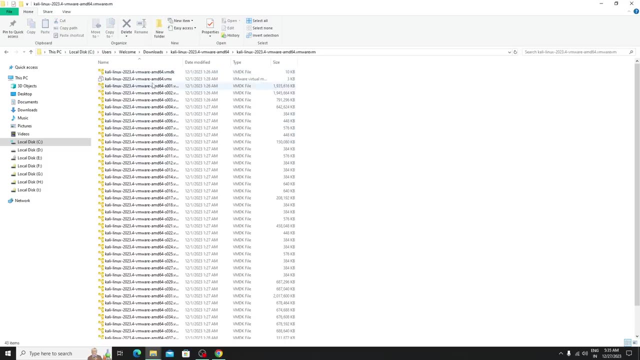 let me extract it. so here it is now simple. let me uh, first of all, the thing is just simple: click on view here and check, uh, check this one file name extension, okay, and here you guys can able to see the file extensions you need to double click. 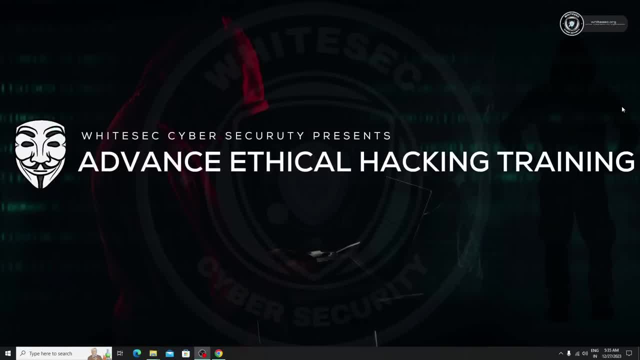 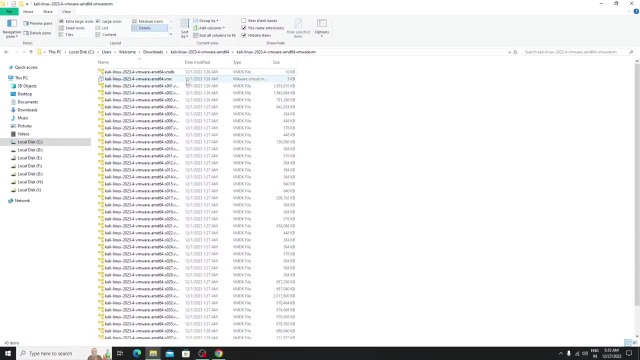 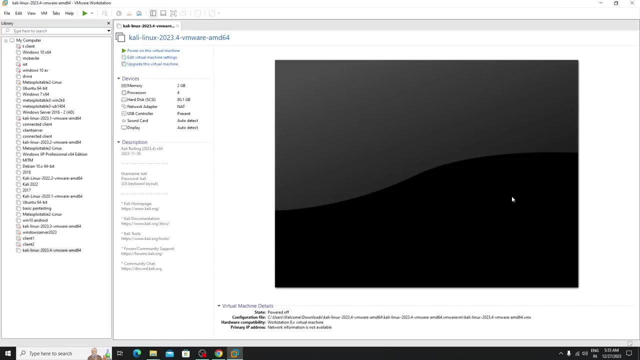 the vmx. okay, before double clicking the vmx, you need to install the vmware workstation so it can able to detect it, and it gonna open it on vmware. okay, this is the thing. double click it, see atom, or you guys automatically, uh, the vmware workstation will open and it will detect the kali. 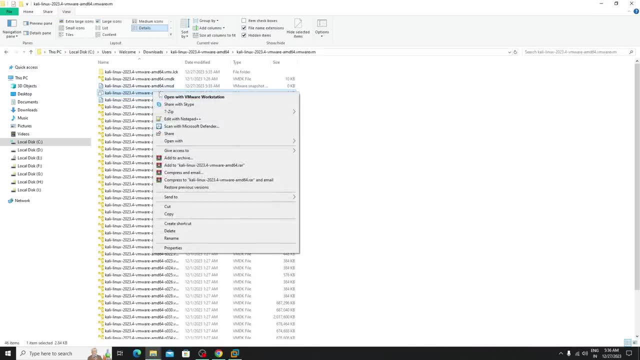 linux here and you can see that the vmware workstation will open and it will detect the kali linux here. if it's not working in your case, simply click on open here. it is open with and choose the vmware workstation here. don't choose a vmware player, choose a vmware workstation, okay. 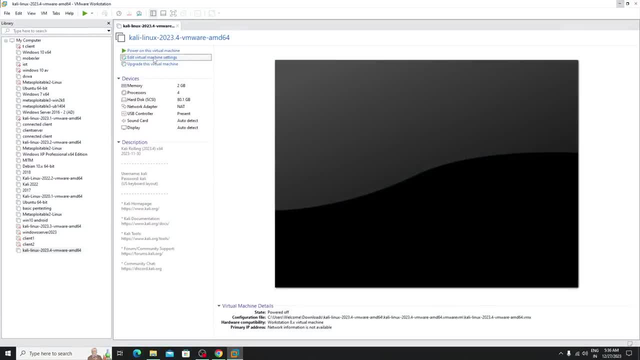 this is how it's gonna work, and here, if you want to edit anything, just try to edit it. okay, uh, the memory, it's enough2 gb ram is enough. processor- that's not: uh, it's just one and one. processor. that's not: uh, it's not just one and one. 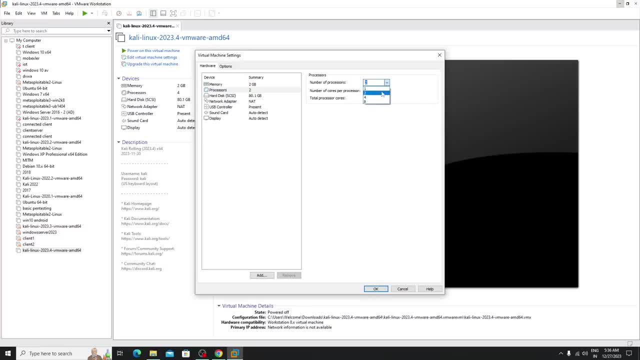 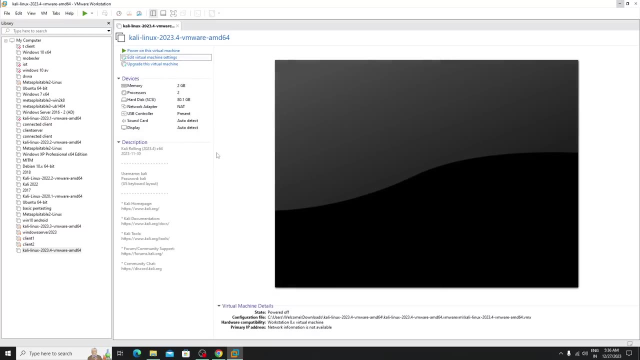 processor that's not uh, it's not just f1. for example, processor that's not uh, it's not just f1. for example, change it to 2. okay, I am gonna give the number of core is 1 and the number of processes to them. okay, that's it, because these things are enough for this thing, this kali linux, a simple. 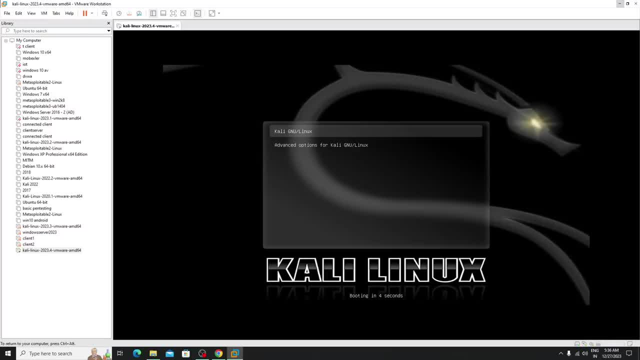 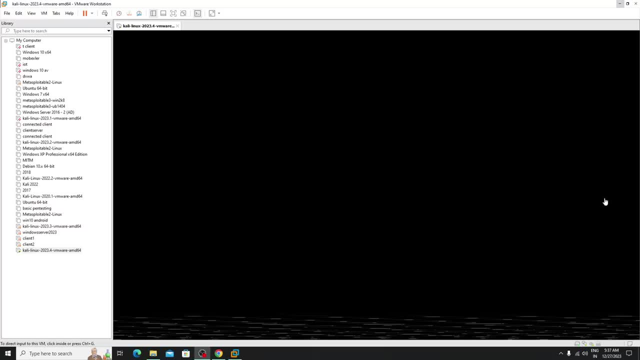 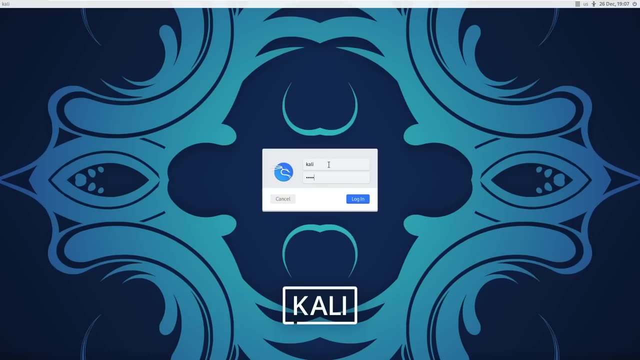 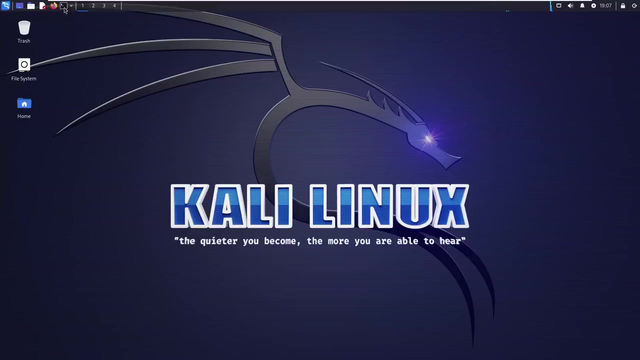 power on this virtual machine. simple: the username is Kali and the password is Kali. okay, this is the default thing. if you want to change it, you can also change it. you can also change the password. how to change it? simple, the thing is, you just need to execute this command. let me write okay. let me type okay. pseudo PAS. 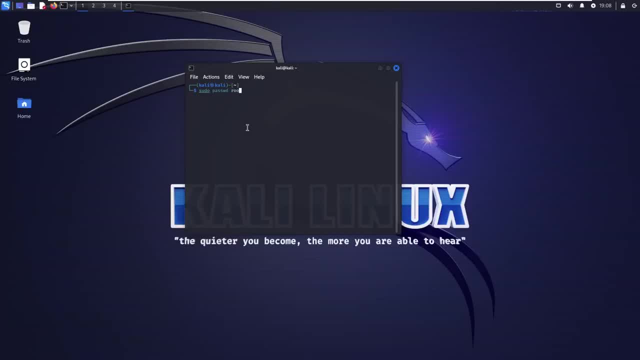 SWD and just type root here. okay, now just type your default password, which is, in my case, a Kali, and what, which password you need to set up. remember this thing: the password must be: you guys need to remember this password. okay, this is a very important thing. so the thing is, let me set. 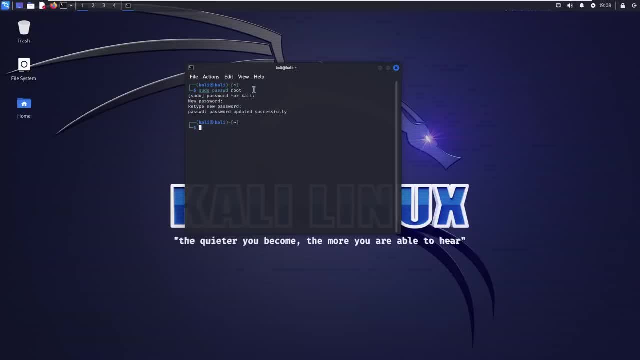 the new password as a Kali okay, because I don't want to change it. simply, in your case, you need to change the password. this is the thing now. this is how we can able to set up the Kali linux right, and you also need to change some preferences here, such as just open terminal and. 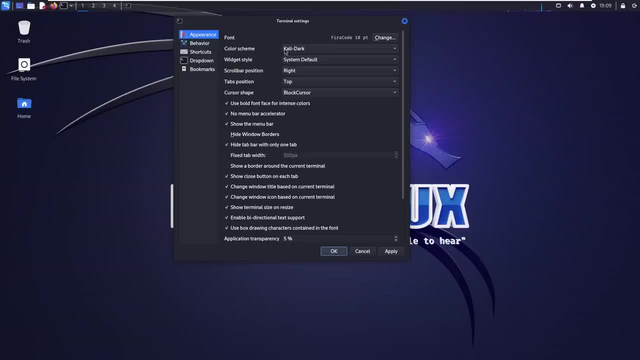 right click and click on preference and there is a color schema and here you just need to change the color to green on black. okay, because this, this color is very excellent. okay, you guys can easily figure out the errors there. okay, you can able to see the errors once you see once. 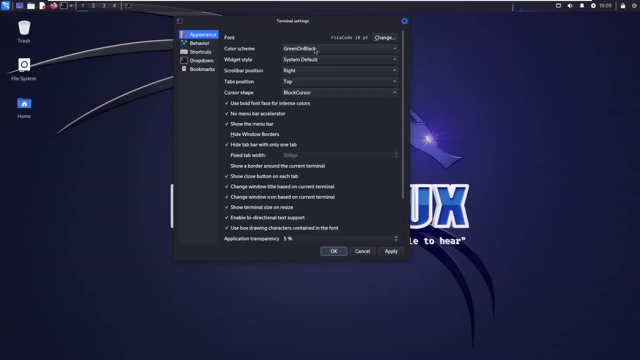 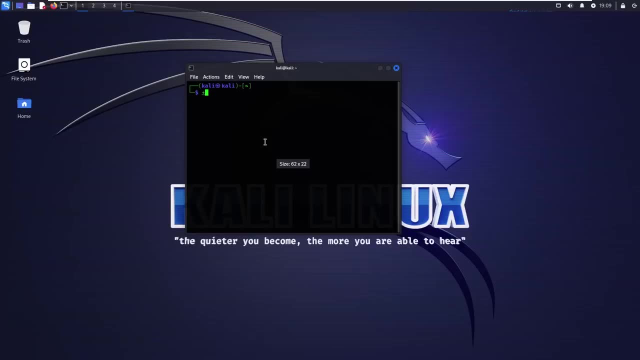 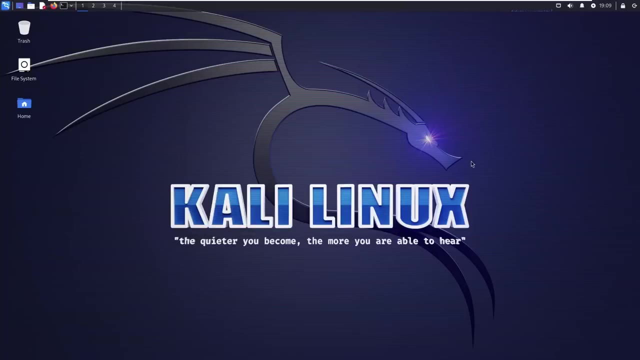 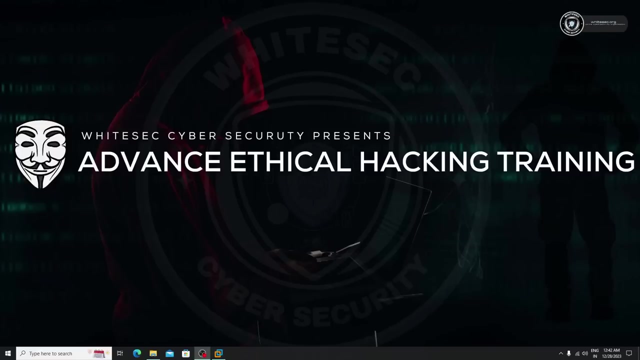 you get any kind of errors. it is easy to see the things there. okay, because it is very reflective. just apply and click OK. now here you guys can able to see. the text color will change to green or something like that. okay, hope you guys get it right. in the next classes we will set up the victim machine as well. hello, guys, hope you. 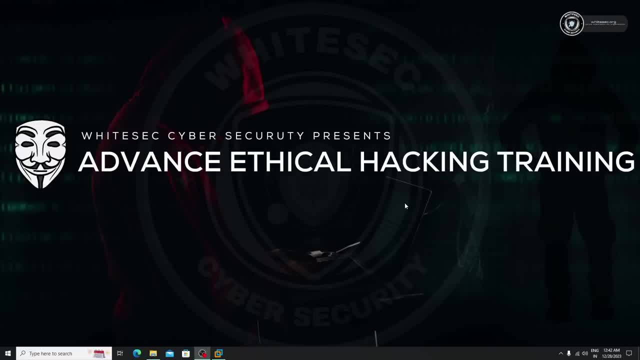 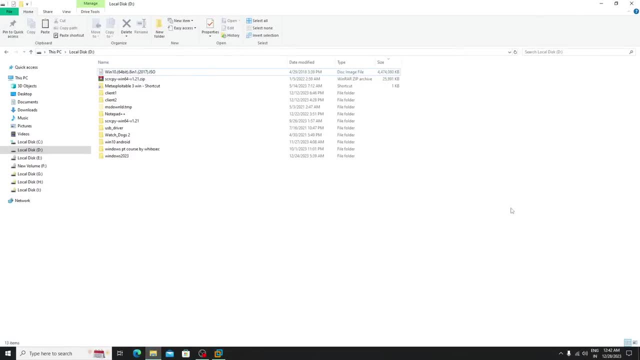 have won. in this classes we are learning how we can able to set up our Target machine. right now are using the windows 10 machine. okay, you will get this iso file on our telegram channel. just visit the telegram channel. they'll there. you guys can able to see the iso file. okay, simple download it. 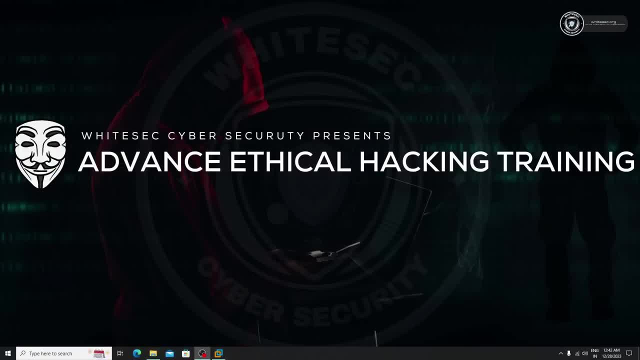 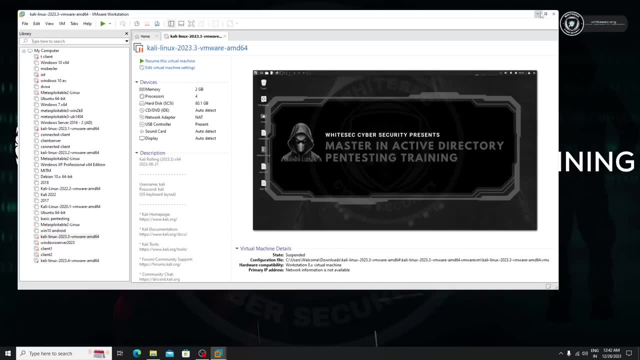 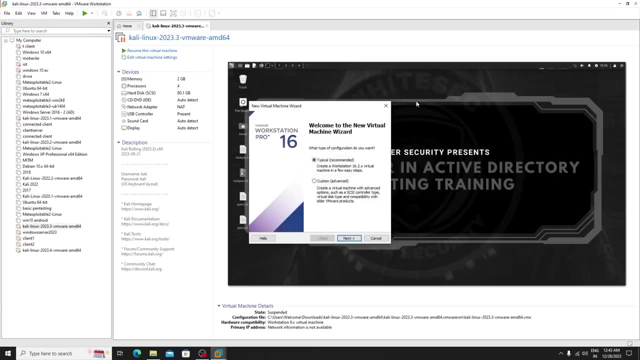 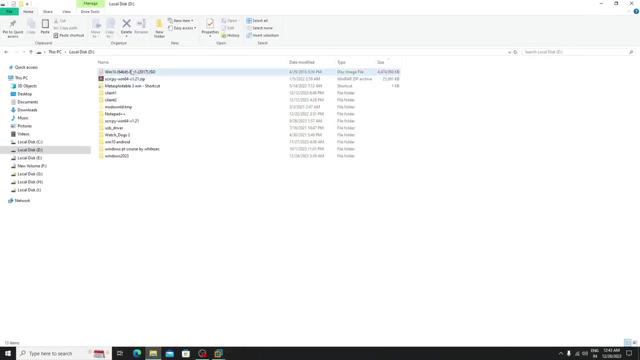 after downloading the iso file, what you need to do means open your vmware workstation. just wait, just open your vmware workstation, then click on files, click on new virtual machine here and click on typical, select typical and from here, just browse your windows 10 iso file. okay, which is in d drive. uh, in my case the iso file is in d drive, so let me. 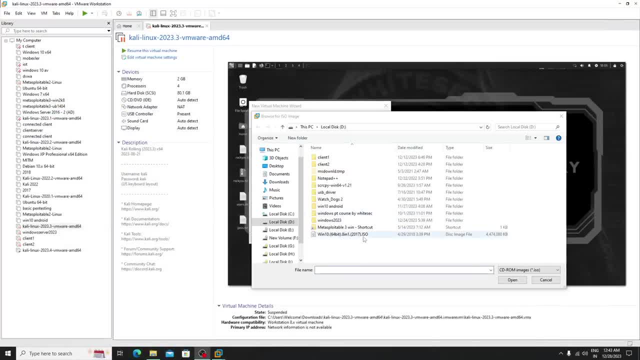 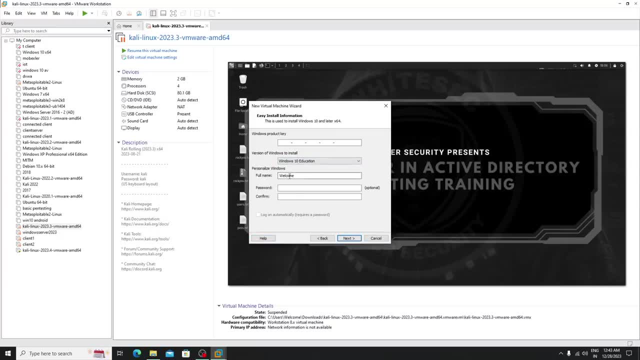 browse it just right. so here you guys can able to see it. just select it. okay now simple click on next. if you want to give the full name, like in my case, let me give the full full name as advanced ethical hacking. all right, and let me give the password as well. let me give the password as uh. 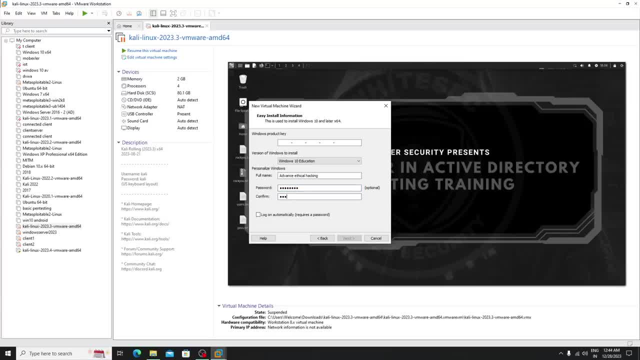 word set right. click on yes, click on yes. and here. simple, uh, just browse the location here where you want to save this file, switch and everything. let me give the virtual name as http: yeah, okay, okay, now let me save this in d drive. let's make a new folder here, the name of: 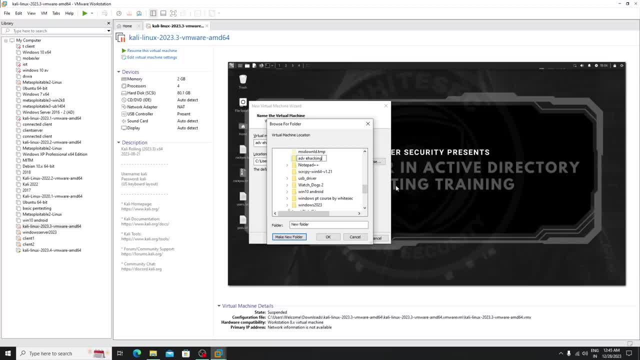 adv ehack: simple click on. just select that folder and click on: okay, there. okay, right now you need to uh like this: you need to save it. okay, because the thing is by default it will save the location in the c drive. okay, you can save it. okay, by default, you can save the location in d c drive. okay, you can. 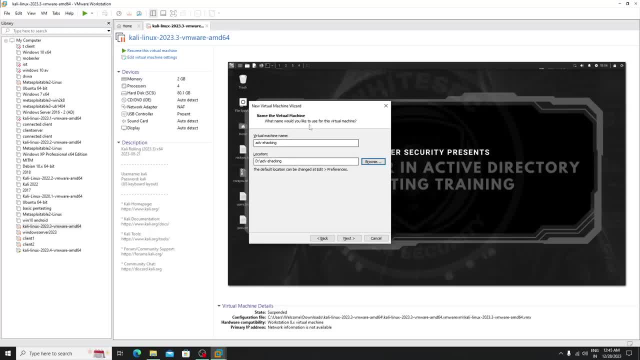 also use a by default one. it's not a big deal if you have a storage in c- mostly we. i don't recommend you to do this process in c drive. okay, simple, just select other drives. simple, just type here. next, just give around 30 gb is enough, and store a virtual disk as a single. 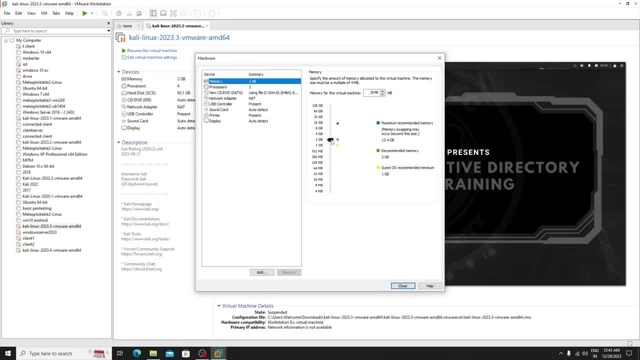 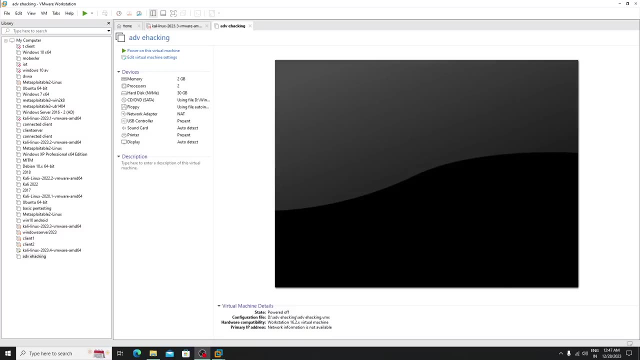 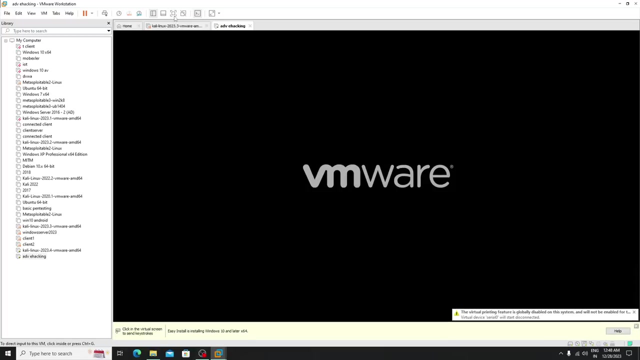 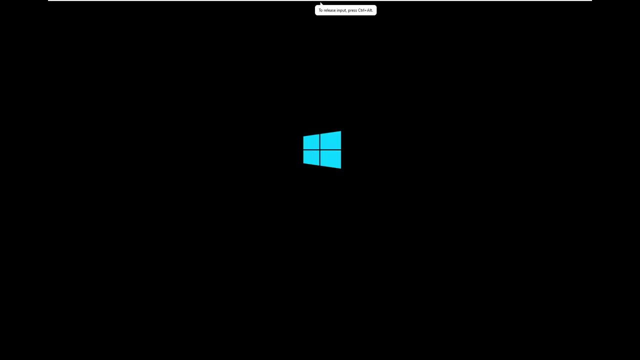 file. next, you can go go with 2 gb ram. okay, it's not a big deal, let me give around. 2 gb is enough. right, close and click on finish. it will take some time, just wait. so here it is now simple click on power on this virtual machine. 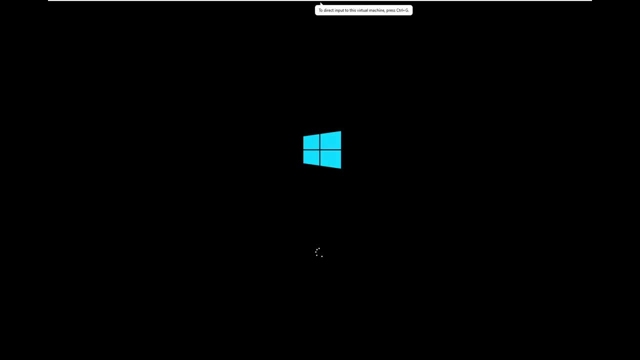 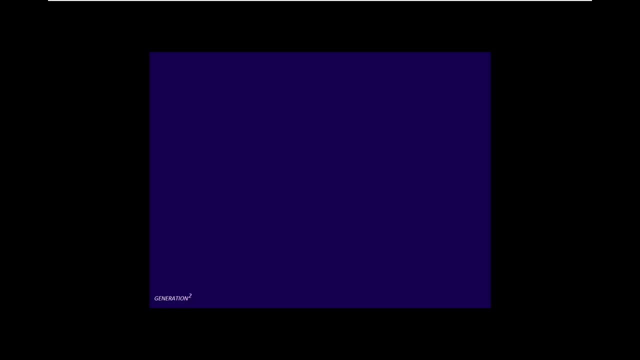 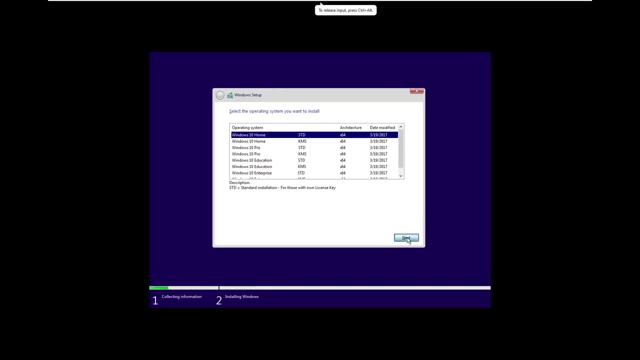 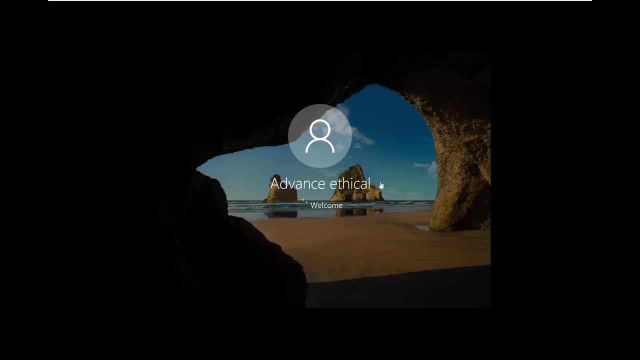 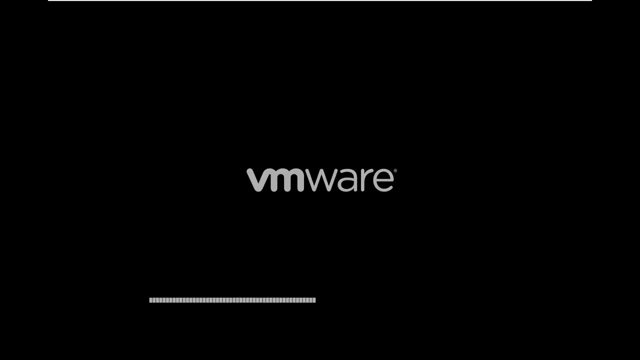 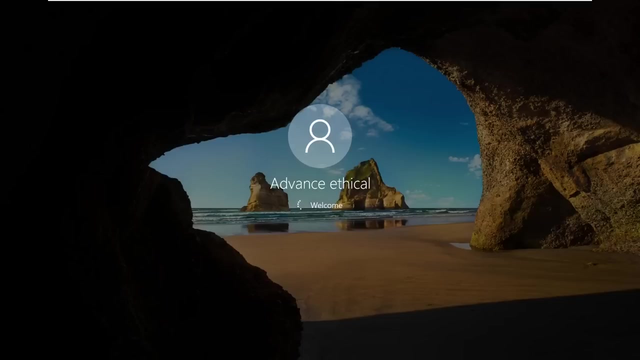 so it will take some time. just wait, let me tell you. you no need to do anything. the process is completely automation, right simple. just select this one. okay, let me select the Windows 10 home. click next there. now you just need to wait, you? oh, here it is. 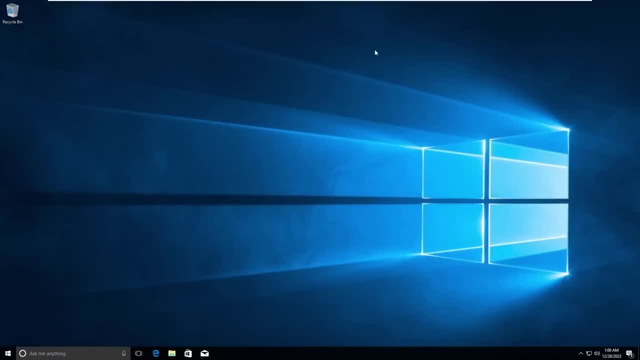 so this is how we can able to set up the Windows 10 machine. simple, just see. if you can't able to see the windows 10 machine, then you can't able to see the full screen here at the time. simple here, click click on install VM tools in my. 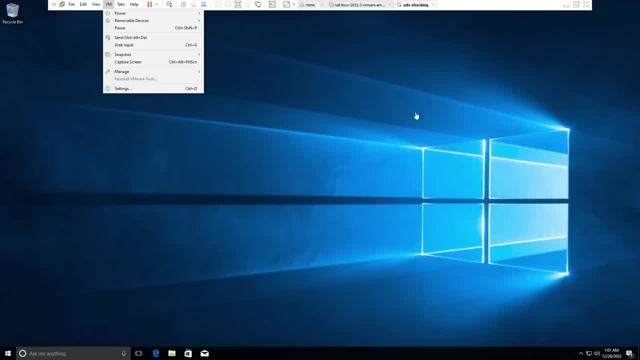 case it's already installed by default, it will install it and it gonna set up it. okay, but in your case, if it doesn't work, then you need to do the process manually. just simple click here, install VM tools- simple, you just need to set up it. right, hope you guys get it. but thank you, have a nice day. hello guys, hope you. 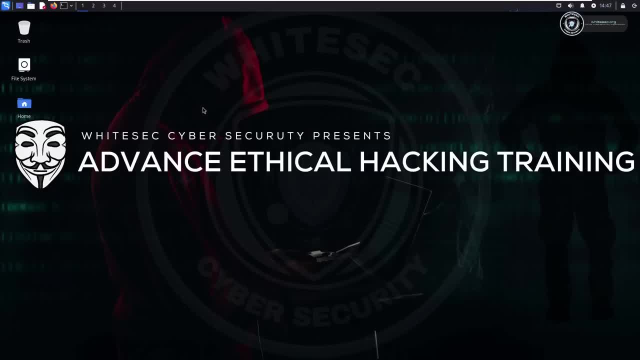 are fine. in this classes we are learning about Kali Linux, right, the basics of Kali Linux. here the thing is, first of all, what we use here. mostly we use a terminal, right, see, you can open the terminal from any folder. this is a thing. see, right now this. 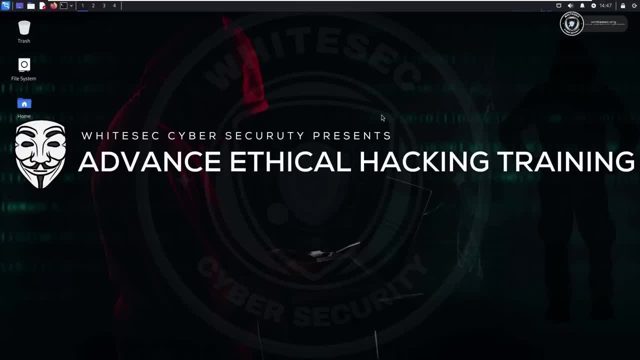 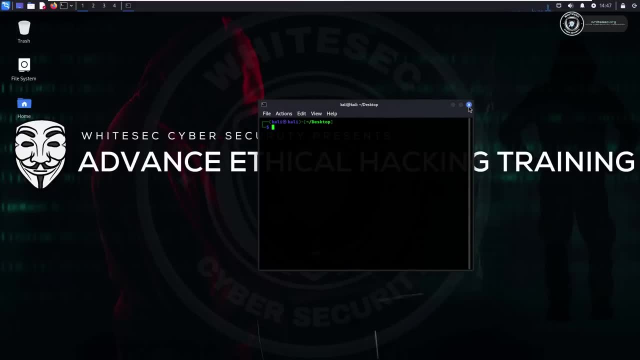 is a desktop. okay, now I want to open the terminal from desktop. simple right click: open terminal. open here. okay, open terminal here you guys can able to see it. right, see open terminal here. if you open this thing then you can able to see that terminal. okay, just see here there is a kali. what is this kali? kali is nothing but our username. okay, this is the. 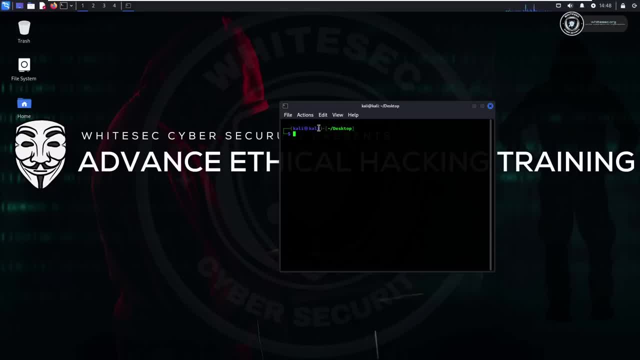 thing right here. just ignore this part. okay, you need to focus on these things. okay, right now, here you can able to see desktop is there. that means i just open the terminal from desktop. okay, i am doing. the whole process will affect on desktop. okay, if i create any kind of folder, if i create. 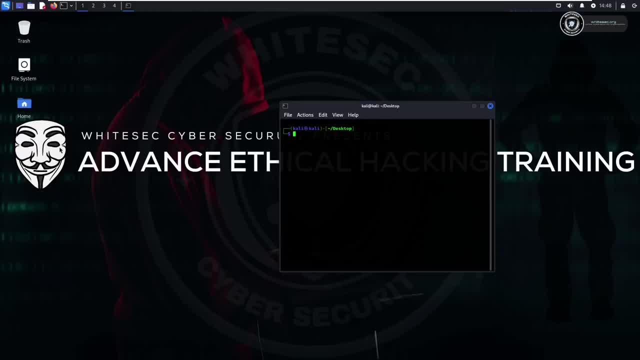 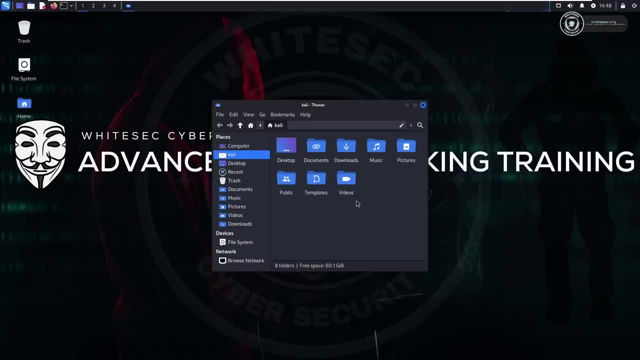 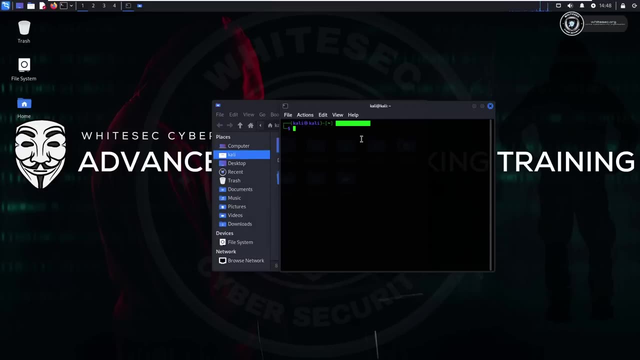 any kind of file it will affect on desktop. okay, this is a thing. see if i there is a home folder, is there? if i open the home folder? right, if i open the terminal from here, see what will happen. you can't see anything. okay, that means you are in home folder there, right? if i type ls, you guys, 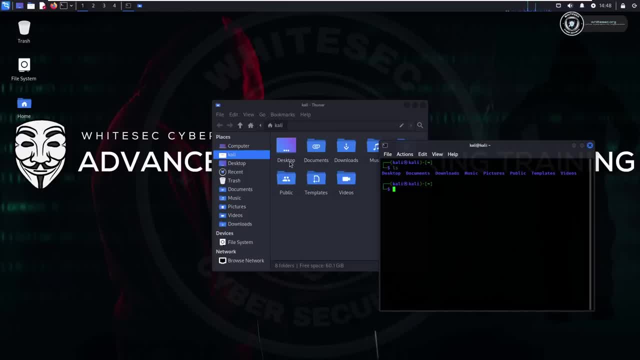 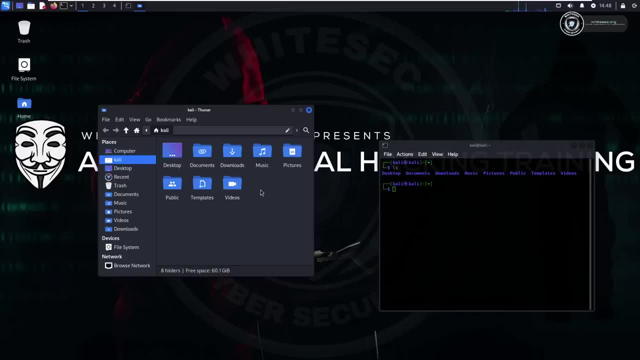 can able to see the whole folders are there? okay, in kali linux we say folders as a direct tree. okay, this is the thing. whenever i say the folder, that means it's a directory. okay, whenever i say the directory, that means it's a folder. this is the thing. it's not a big deal. okay, right now. 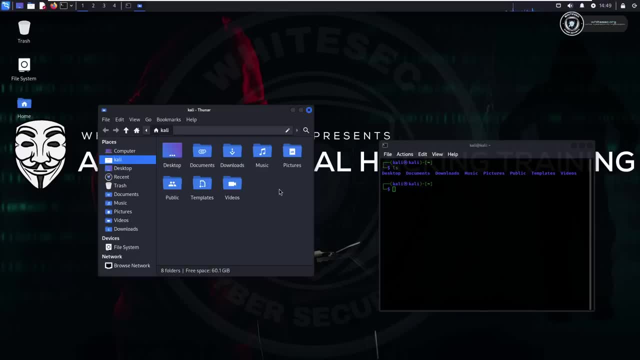 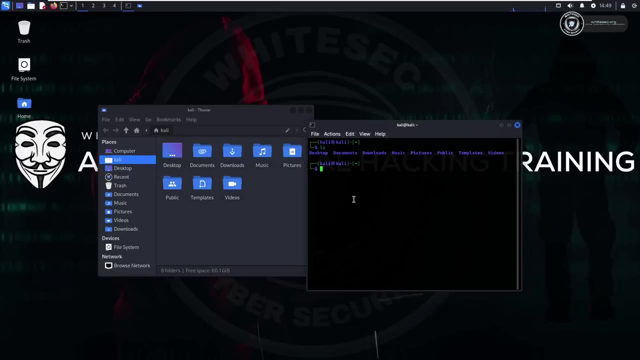 the linux is very easy. previously it is a kind of hard thing. majority of beginners can't able to get it. okay. right now the things has been completely changed. okay, this is the thing. it is very easy now here. if if i want to zoom this terminal at the time, what i need to do? simple control plus okay. 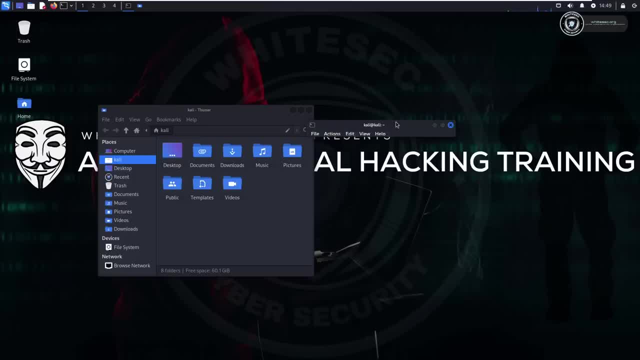 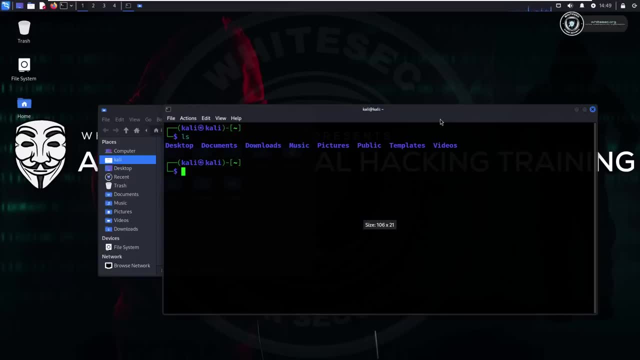 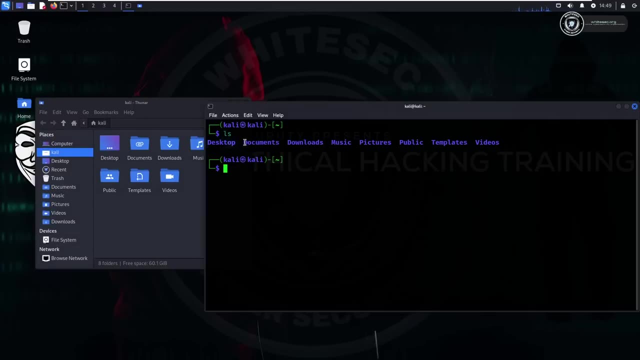 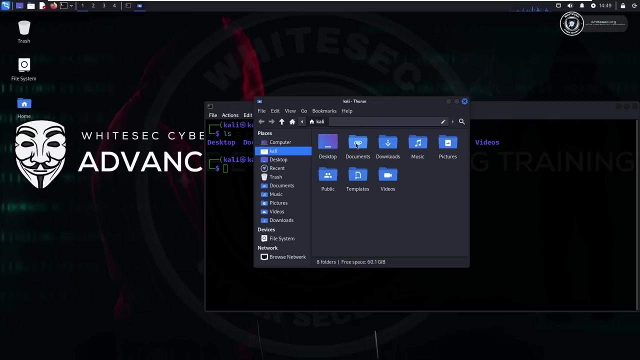 i can able to zoom it right so you can also adjust like this as well. okay, so here is a thing: right, if i want to uh open this document folder, like this in windows, what we do, basically, if i want to open any kind of folder, what i do, simple: i go to that folder and double click it. i can able to open that. 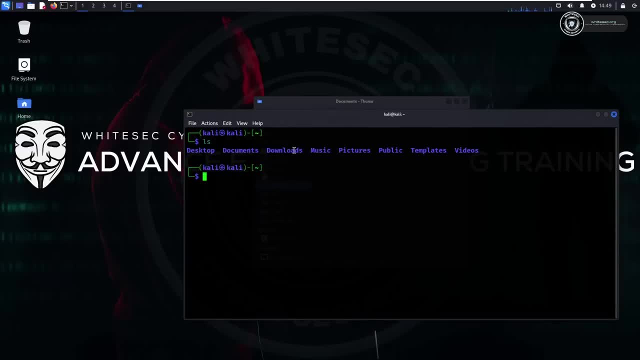 folder. right simple. in linux, what we do means by using terminal also, we guys can able to do this process. okay, we can now let me move to document folder. simple, just type here: cd. cd is nothing, but change directory. change directory to where: uh, which folder you want to open? 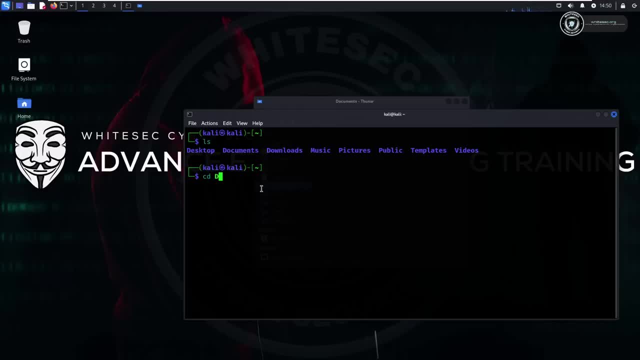 i want to open the document folder. simple: just type d there see, and just type tab. now here, tab is a nothing but the tab button. okay, in your car, in your window, uh, this keyboard, you're guys can able to see tab button right if you click the tab button. it is very handy, guys, okay. 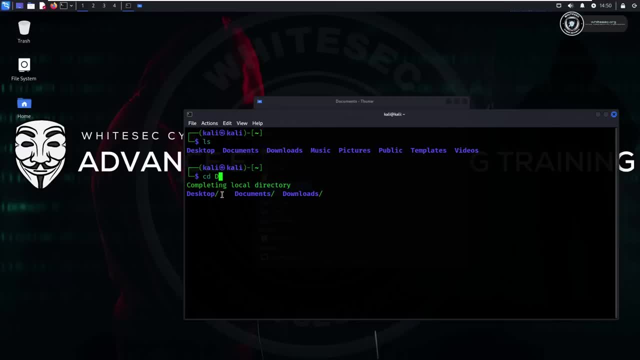 in real world scenarios, the tab button will be very handy because it will auto complete the name there. okay, see right now why it's can't able to auto complete it: because there is a. if i type d there, there are different folders are there with that's. uh, the starting letter is d. okay, see. 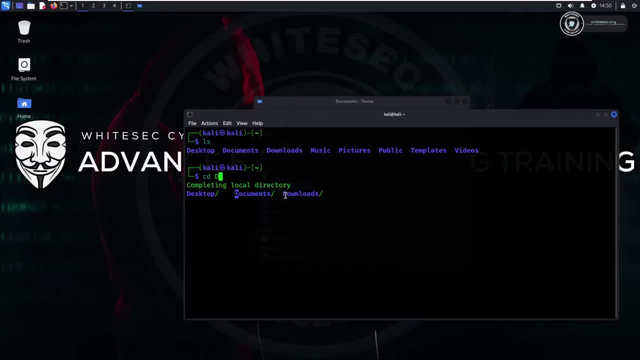 d. it's starting from desktop. document is also d. okay, uh, download is having the d there. okay, if i? uh, i just told you right. i want to move to document folder. if i type d uh o there and if i click on tab right now, it's a two folders. okay, i can able to see two suggestions here. there is a. 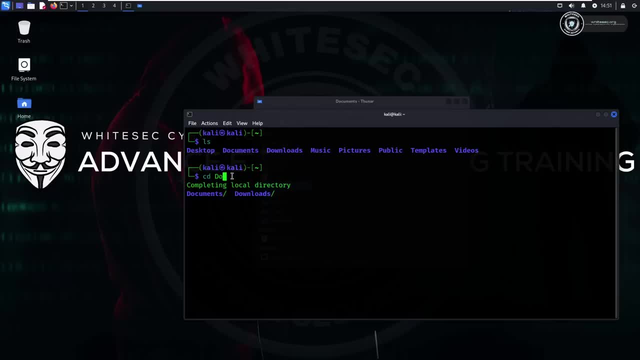 document is there. there is a downloads. if i type another letter doc and if i type tab there, then it will auto complete it. okay, so this is the thing. if i type enter there, right now i am in document folder. right, hope you guys can able to see. right, i just told you this thing. well, i just opened the 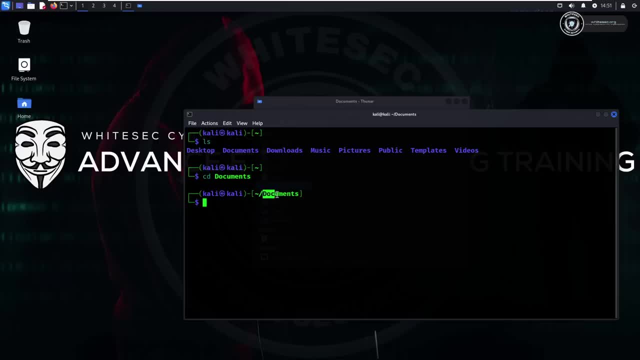 terminal from desktop right right now. i am in what document folder? you can also recheck it if you type pwd- present working directory. okay, where you are working now, simple. if i hit enter here you guys can able to see there is a home folder. in home there is a kali. kali is a nothing. 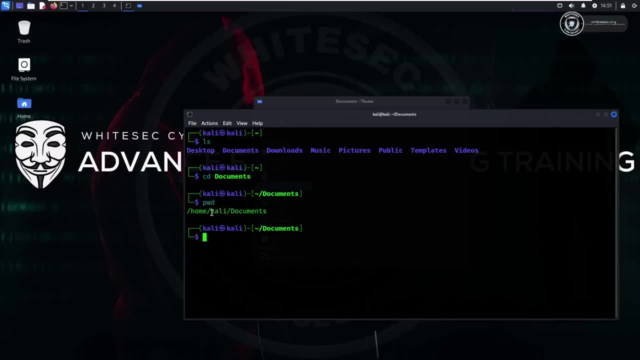 but this is a your. it's based on your username. okay, in windows, uh, we set the username right once we boot the windows system, a new windows system at the time we set. we set the username there okay, such as: mostly people use the welcome in windows. okay, mostly the people use their windows system username, such as windows or their names as well. 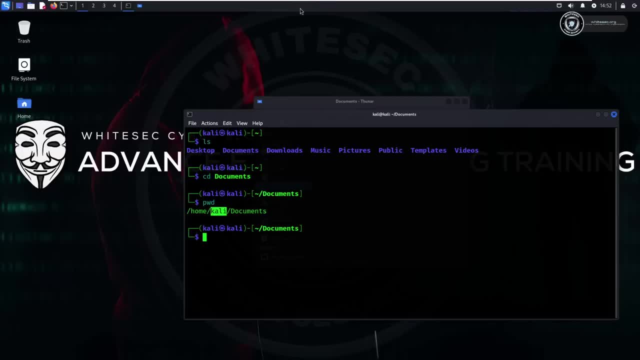 okay, simple, this is your name. okay, here we just use a virtual machine, right, virtual machine. have the by default username as a kali. if you boot the iso file of kali linux, at that time you can able to set up the name there. okay, here you guys can able to see. 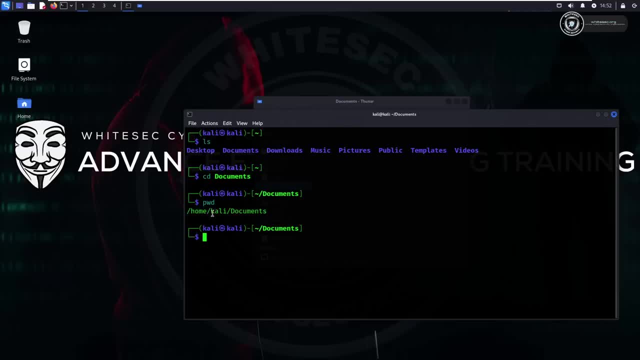 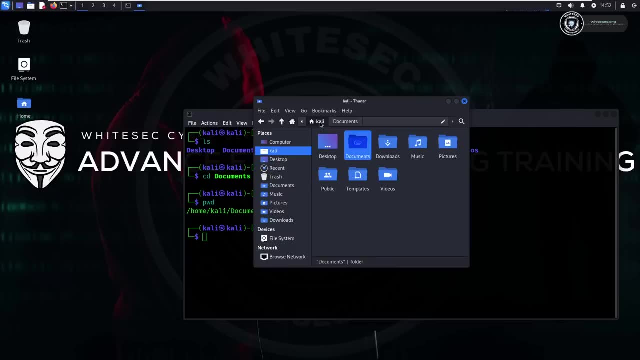 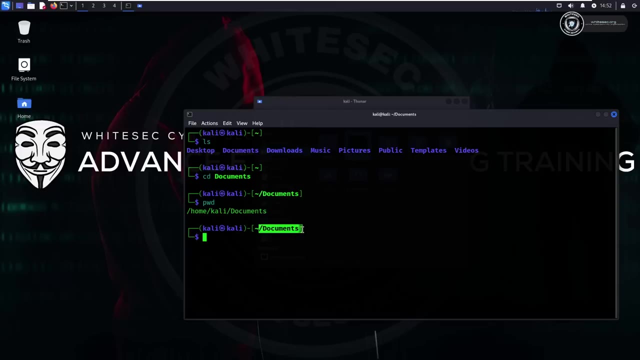 username: okay, that means in home folder. there is a kali in kali. okay, this is a kali folder. okay, see here home. uh, hope you guys can able to see here kali in kali. there is a documents. okay, right now i am in document folder from here also, you guys can able to check. 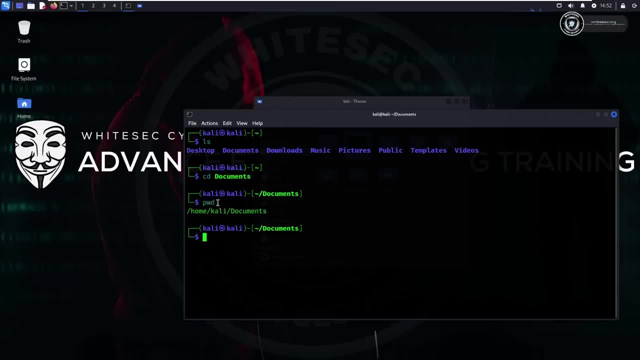 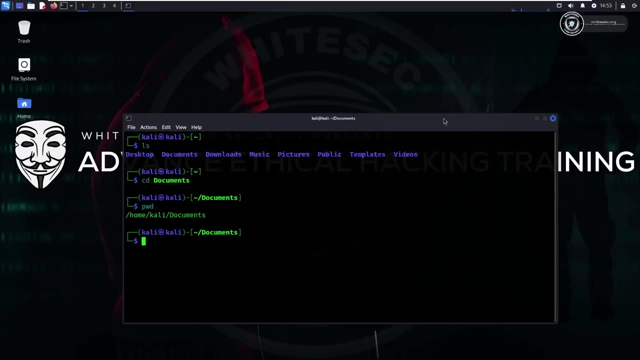 that, but simple. sometimes you also need this thing. okay, once you are performing the pen testing, if the server is linux based, at that time this pwd commands will help you. okay, this is the pwd command. is a thing you will see that in pentesting in window in web hacking section right now here. 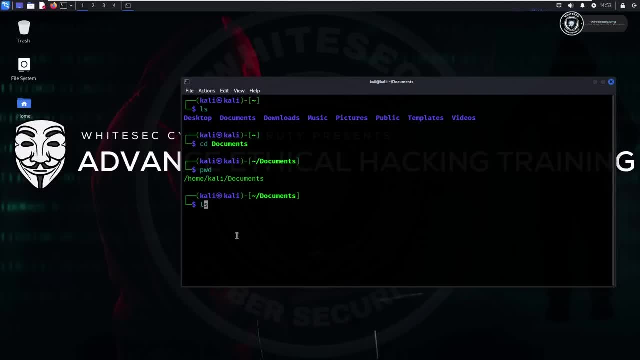 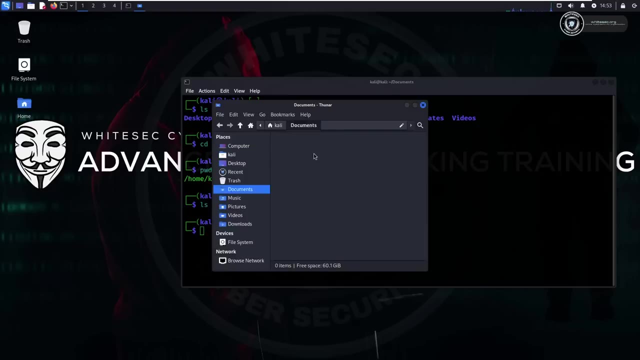 right now. if i type ls, ls is a nothing but list. okay, there is a nothing. okay, you can't able to see any fold, any files or folder in this document folder. okay, because it's empty. let me show you from here as well. if i open the documents folder, there is a nothing here at that time. assume that. 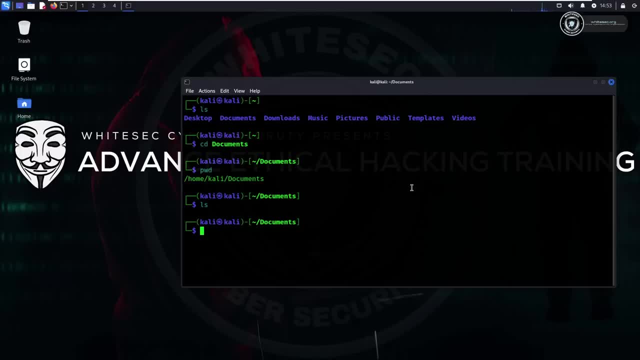 if you want to create any subfolder there in document folder, you need to create another folder in it. simple, just type mkdir to create the folder. okay, let me name it as a test. okay, if i type ls now here, you guys can able to see there is a test folder in document folder. if i open this, 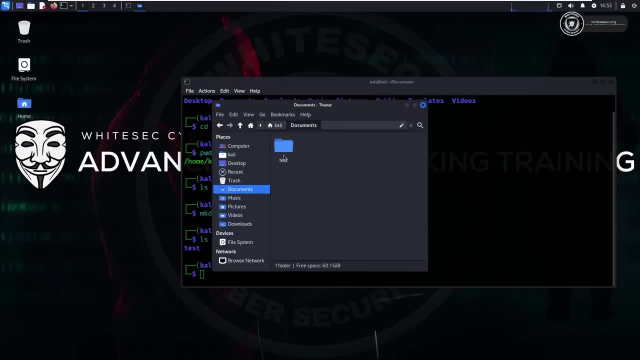 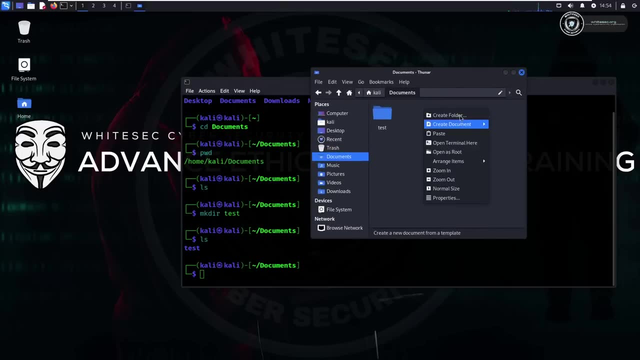 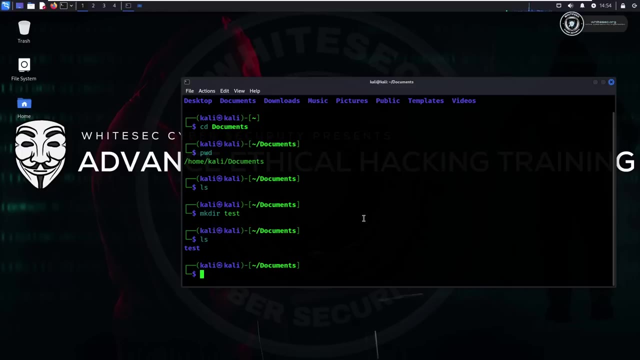 document folder. here you guys can able to see the test folder has been created. simple, you can also create from here as well. okay, right click create folder and from here also you guys can able to create it. okay, it's not a big deal. okay, now i want to remove this folder. i want to delete this one. 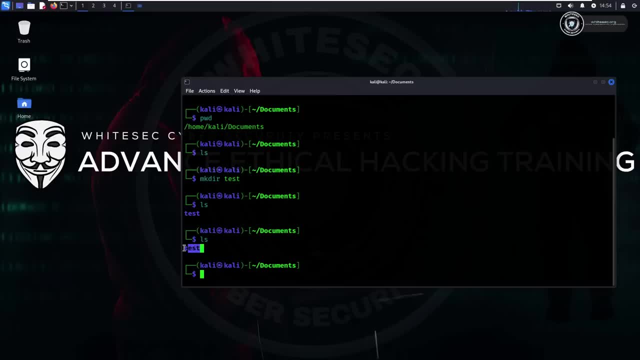 how to delete it simple. first of all, just type ls. just see the name of that folder which which you want to delete. okay, now here there is a test. simple, simple, just type here: rm. that means remove. just type dar. i just told you. uh, in linux we say folders as a directory. okay, this is a short form. 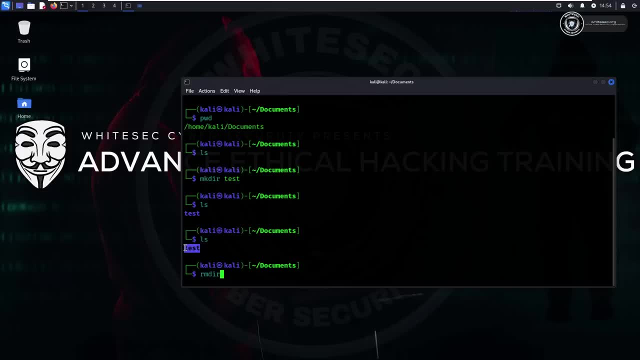 of directory. okay, dir now. simple. i want to remove this. remove is nothing but delete, right. this is a thing. now here. i want to remove this test folder from here. simple, just type rmdir, just type the name which you want to delete, just type enter and again just type ls. here see the the test directory has. 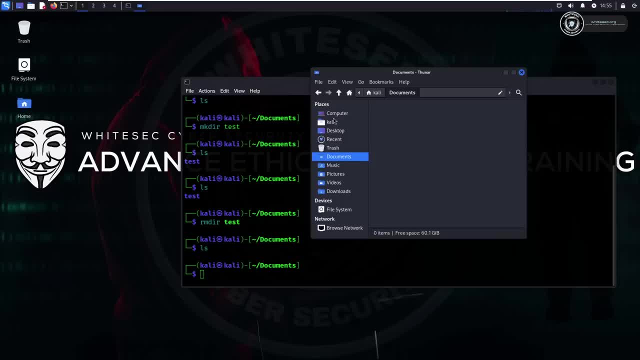 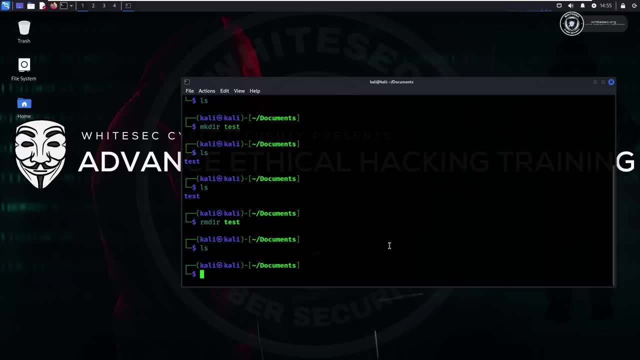 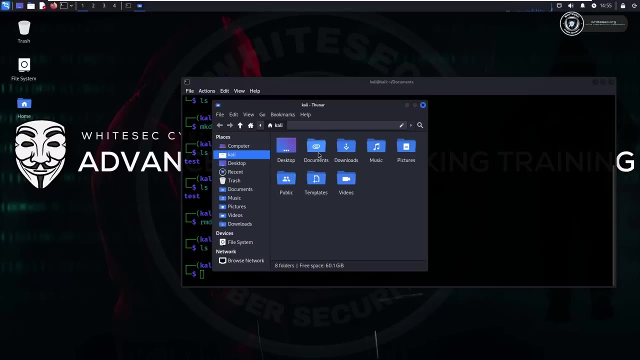 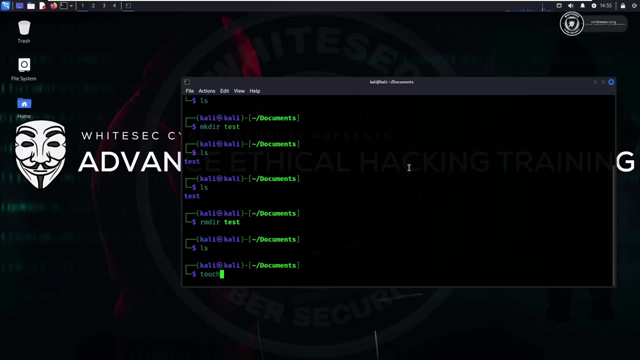 been deleted. let me open. i'll show you from here as well. see, the test directory has been deleted. right now, if i want to create any kind of document, simple, in this document folder, i want to create some, some, some file here. at that time, what you need to do just type here, touch okay, and let me create one text file with the name of white sick. 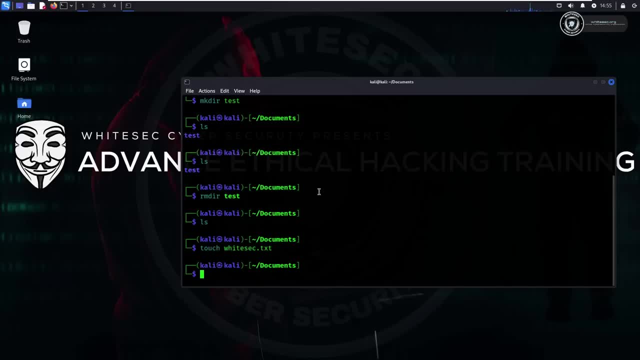 dot txt. just type enter here. if i type ls, you guys can able to see there is a white sec dot txt. the file has been created. if i open this one here, you guys can able to see white sec dot txt. file has been created. if you want to remove this, what you need to type simple rm, that's it okay. if you want to delete any kind, 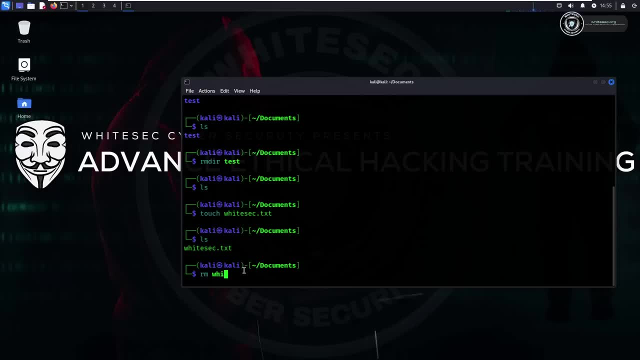 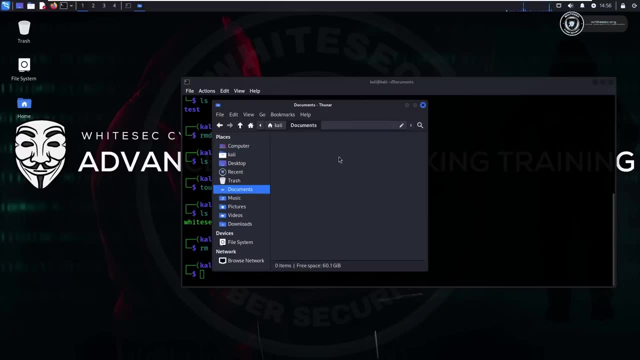 of file. at that time you need to use the rm right. simple, just type white sec dot txt and enter. now the file has been deleted. so see, the file has been deleted from here. this is the thing. it's a very easy, simple, uh. if you are having 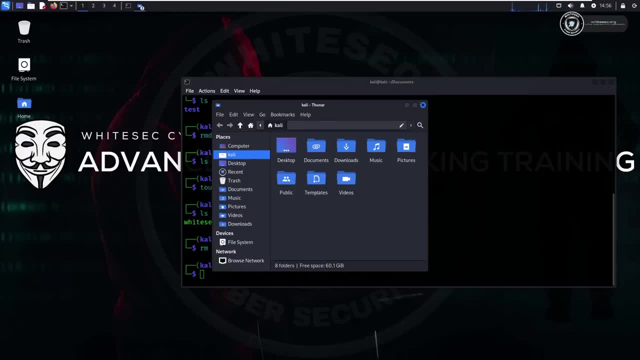 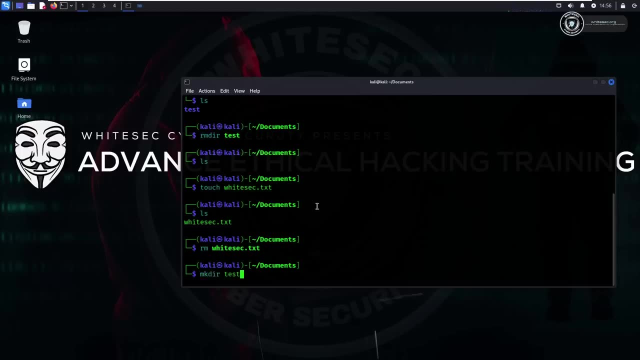 some kind of issue, then practice it. that's it. it's not a big deal. again i am saying now see here, let's create some more directory: mkdir. let me create test. okay, now ls. there is a test. let me go with this directory. just type here: cd test. i am entering in test directory there. 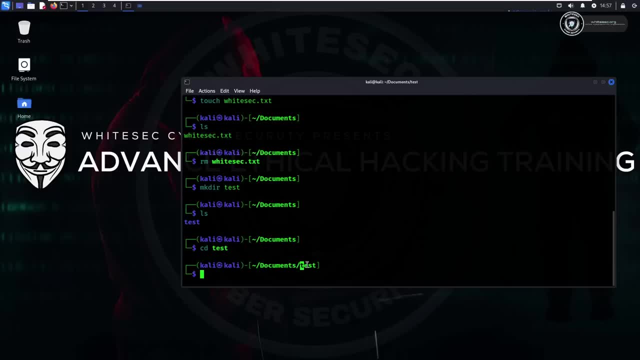 okay, see, right now i am in documents. in documents, there is test folder. okay, i am right now in test folder. okay, this is the thing. now let me create another directory here: mkdir- test2. okay now, simple, just type ls. there is a test2 is here right now. let me go with test2. 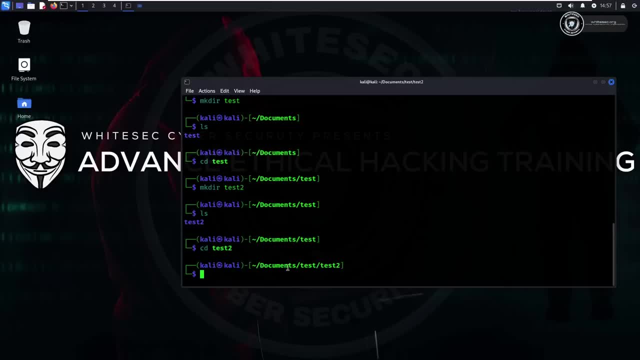 see, right now i am in document folder. in document, there is a test in test. there is another test2 folder is here. okay, right now, my uh, i am working with uh from this folder. okay, this is a thing. now, see, the task is i want to. i want to go back to uh this test for uh, this test folder. okay, this is a thing. 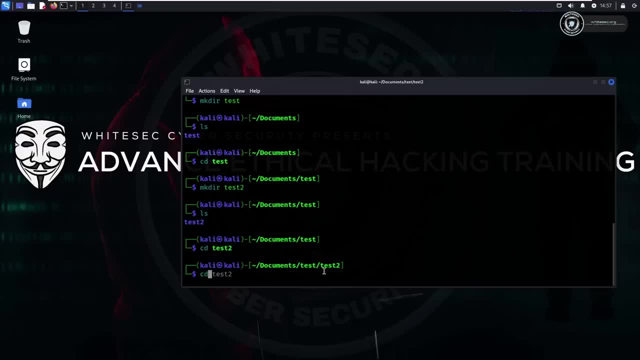 okay, how to do that simple. if i type cd here, then what will happen means i will go directly to the home folder. this is a thing. okay. if i type pwd here, you guys can able to see. right now i am in home kali. this is a by default location of kali linux. 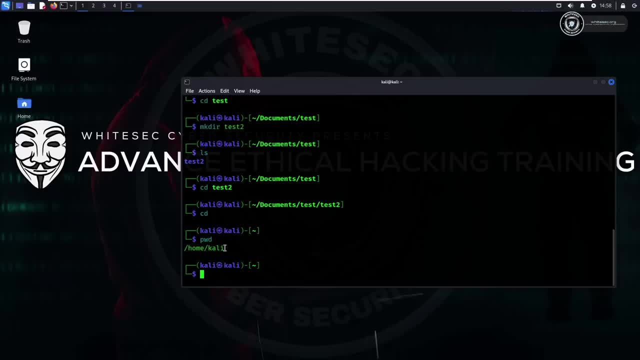 okay, right now i'm uh, i just go back to the uh, this default location. okay, the thing is, i want to go back to test folder, not to uh by default one. okay, this is a thing now let me do it again. just type here cd documents, right documents, and let me go to uh. just let me type ls again. 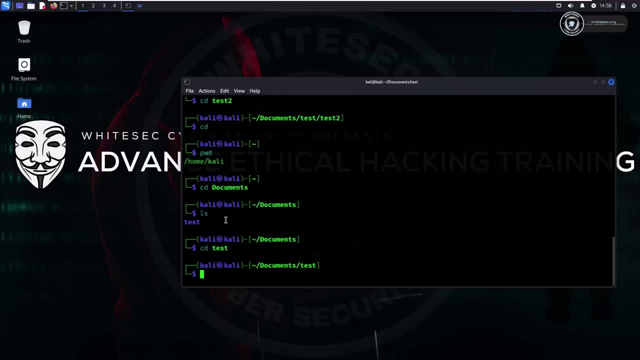 cd test. okay, again, let me uh. there is a test2, there is a test to just type it: cd test to. okay, right now i'm test to folder, right, so the thing is, let's go back to test folder, okay, instead of, uh, default one. okay, so to to do that simple just. 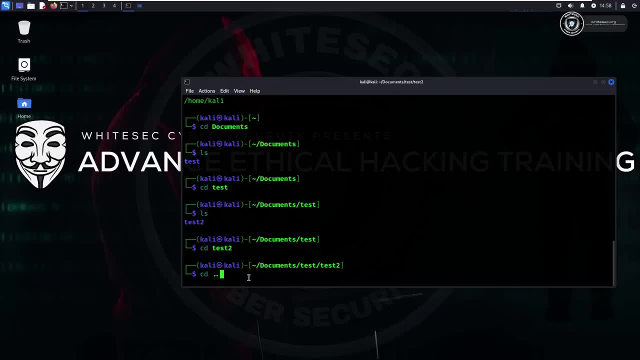 type cd, dot, dot. okay, see what will happen now i just move back to one directory. okay, it's simple. right now i'm in test directory. okay, this is the thing. if i type pwd here, you guys can able to see: right now i'm in test directory. so this is how you can able to go back to spec, uh, the directory. 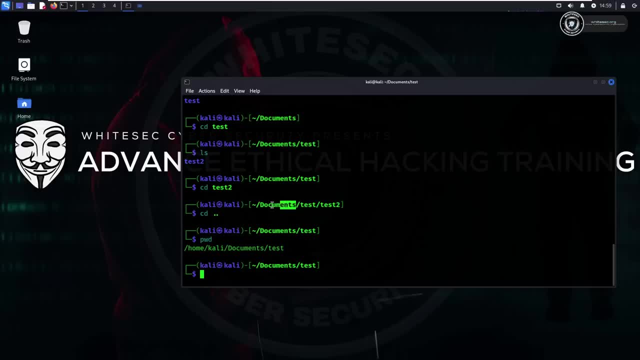 one by one. okay, assume that i want to go back direct to the document folder. okay, let me go back to again test two. now that the task is, i want to go back to document folder. at that time, what i need to do? simple: just type here: cd, dot, dot, forward, slash. okay, that means i'm going back. 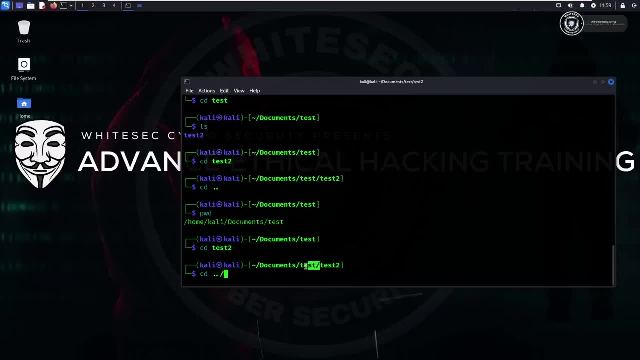 to one directory. okay, now i am in test directory. okay, once i type this one, then right now i am just: you do not have, you do not have beiquer dash, dash, slash, dash f cyber. right now you To test and jumping back from test to test. okay, this is a thing. now the task is: i want to go back. 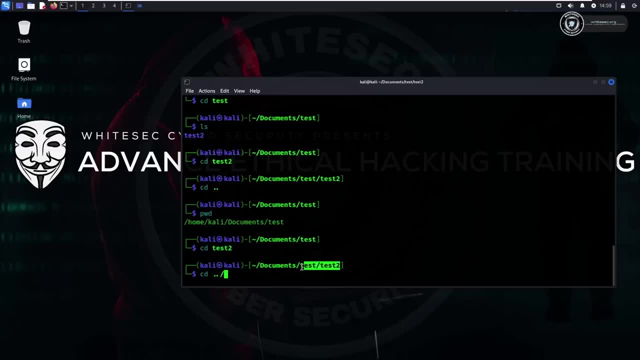 to the document folder. at that time there are two folders i need to go back. okay, this is a thing. now let's go. let's type two times here, okay, like this: one is for test two, one is for test. if i type enter, then right now i'm in document folder, documents folder, this. 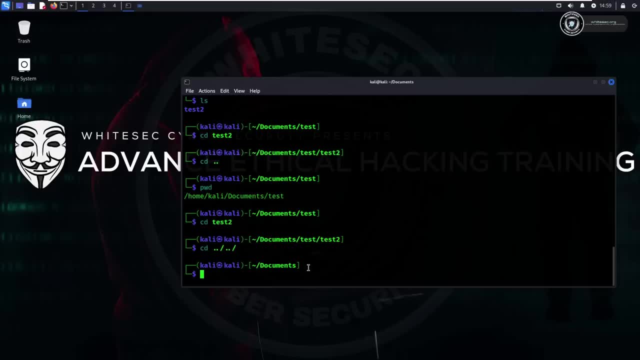 is the thing. okay, this is how you guys can able to go back from the directory. okay, one by one. hope you guys get it. this is very necessary. you uh very important. you need to learn these things. okay, just practice it. that's it. it's not a big deal, okay. now, again, i'm saying: if 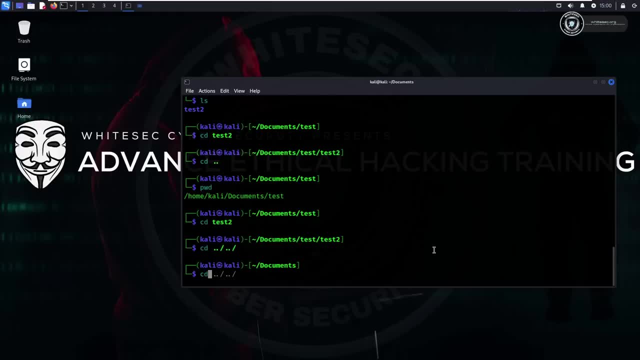 i go back, uh, to home folder. simple, just, i'm gonna type cd there, that's it right. if you type pwd, right now i'm in home folder, right, okay, now let's go back to cd documents again. now let's delete this test test folder. okay, let me delete this one. just type rm dir, just type test. see, now it's throwing. 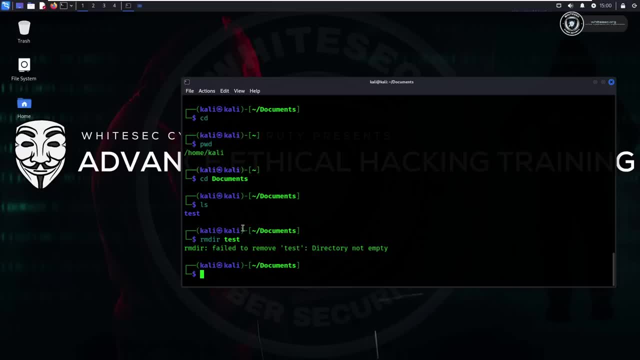 an error, fail to remove test directory not empty. see here in linux, if you want to, if i want to delete the directory, that the directory must be empty there. okay, this is a thing. so how to delete this kind of directory? because in this test direct, in this test directory, 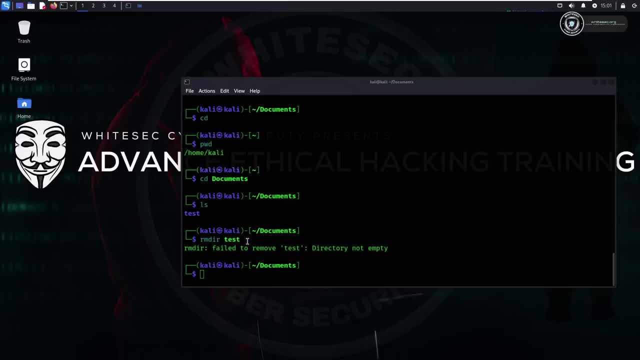 there is another directory, is there subfolder? is there? okay, that's simple. how to delete it? simple: just type here: rm dir. okay, sorry, rm dash r. okay, now just type here: test now. it's successfully deleted. just type ls. see the file. the folder has been deleted, so this. 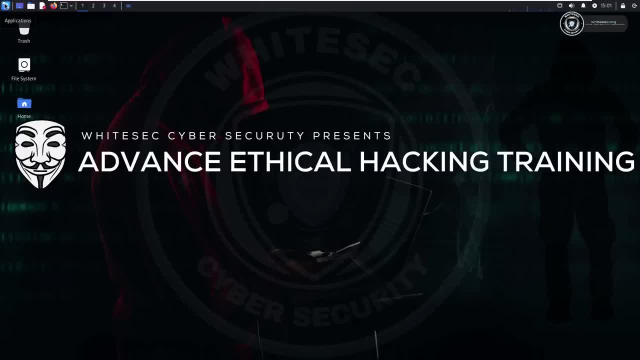 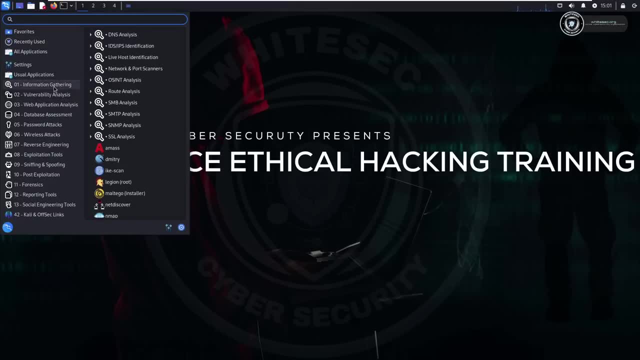 is the thing, it's not a big deal. okay, now let's go for sorry guys- tools as well. see here, every tool is having one folder. okay, if you want to gather the information you okay about your target, then there is a information section is there, the folder is there, okay. 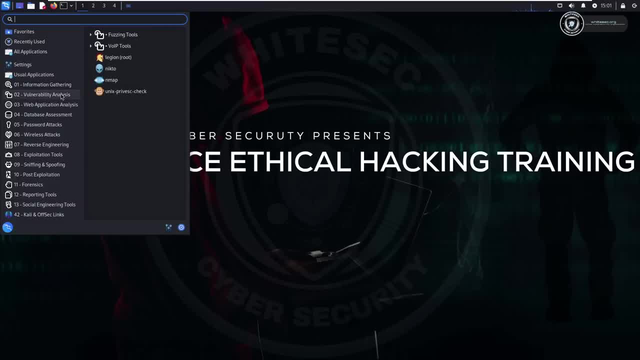 here you guys can able to see all the tools soon. we gonna- i'm gonna- create a course on this, all tools. okay, like about this hacking tools. right, it's not a big deal, it is very easy. okay, but still let me create if i have time. okay, now there is a for vulnerability. 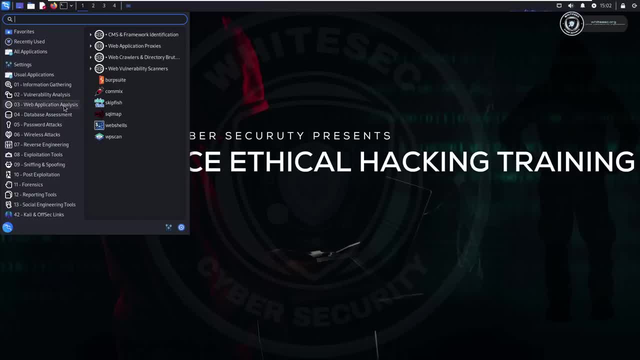 analysis: we have these tools. and web application analysis: we have these tools. okay, for database assessment: we have these tools. okay, don't depend upon these tools only. there are lot of tools on github. okay, you guys can also use it. okay, it's not a big deal, mostly beginners. 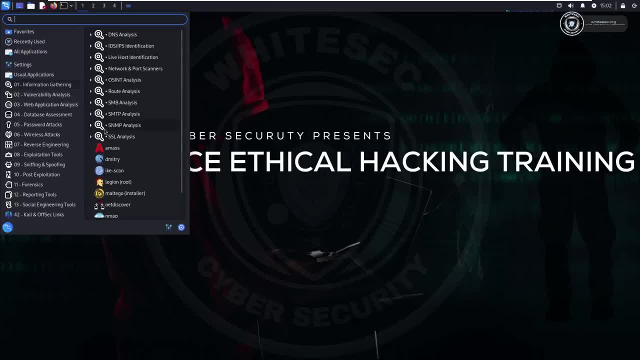 will think that, okay, here, these are the only tools are useful for hacking purpose. okay, no, for hacking or for pentesting purpose. no, there are lot of tools are there? okay, you can also use it. you can also install those tools. okay, we will see that one as well in. 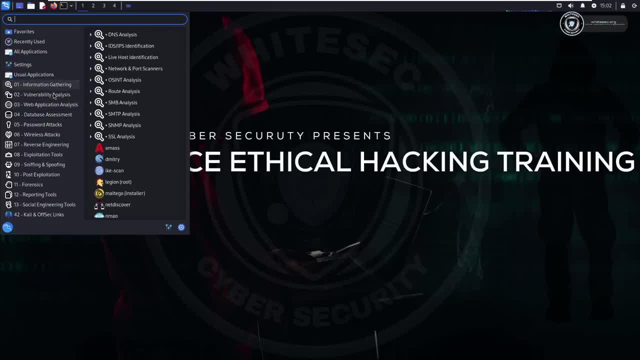 this course we, we are learning here almost exploitation, sniffing, post exploitation, this stuffs okay, you no need to worry, but still okay, it's, it's very easy to use. okay, once you complete this training, you will get a complete idea about how you guys can able to- sorry guys- perform the hacking or pentesting. 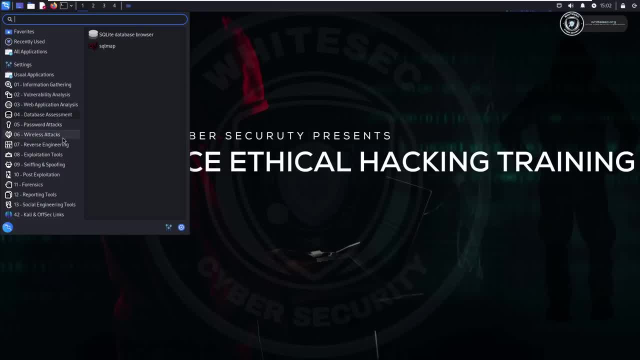 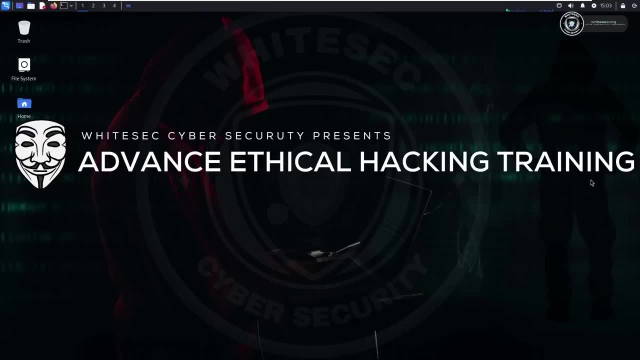 using this tools. okay, so this is a thing. they they just added a one excellent folders where you guys can able to see the tools here. right for pentesting tools. okay, so this is a thing which then we will learn that ok. okay, here also we have a training. did not explain OK. 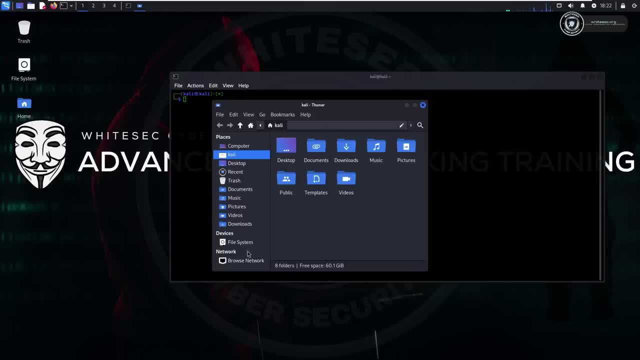 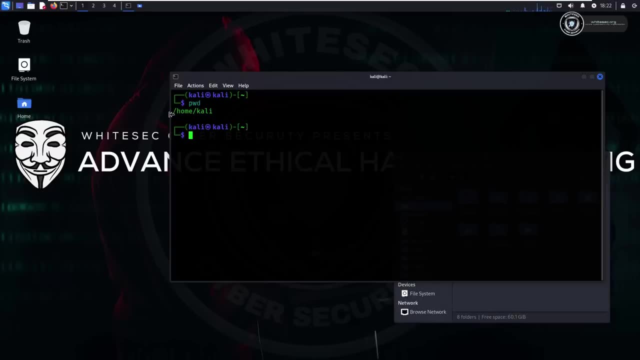 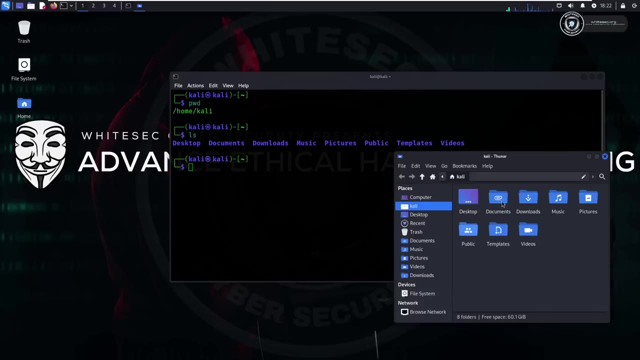 which tools for making their own android default G конце Library up to here left hand corner, right here software. so actually same thing as before when I discuss gUs: where to do. you guys can able to do your t ps4 and we need to, for example, 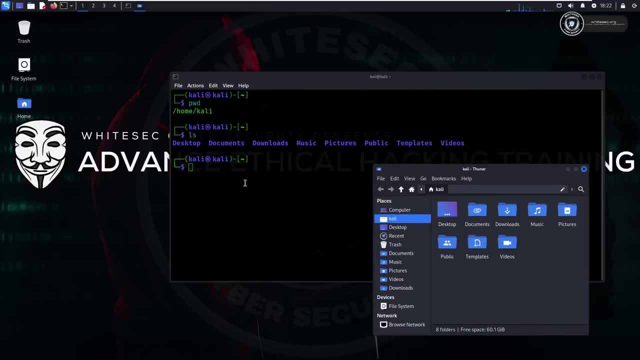 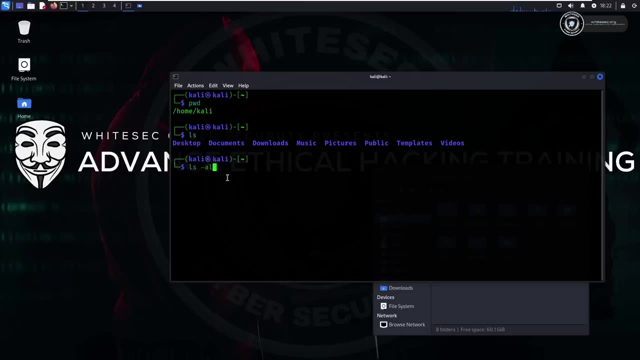 downloads? okay, music pictures, something like that. the same thing. what if i? okay, just type ls dash al. that means list out all hidden files. if i type enter, then you guys can able to see a lot of files which are in hidden mode. okay, just see, i also created one test file here. okay, how i just 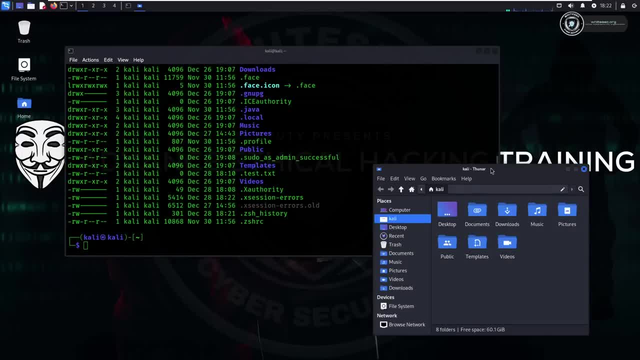 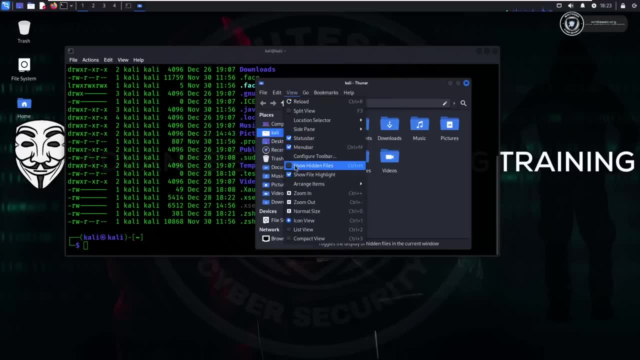 did the this thing. simple thing is you can also list this hidden files from the file manager as well. how simple. click on view and here there is a show. hidden files are there. simple. from here you guys can able to see the hidden files, but during the pen testing you can't able to do these things. 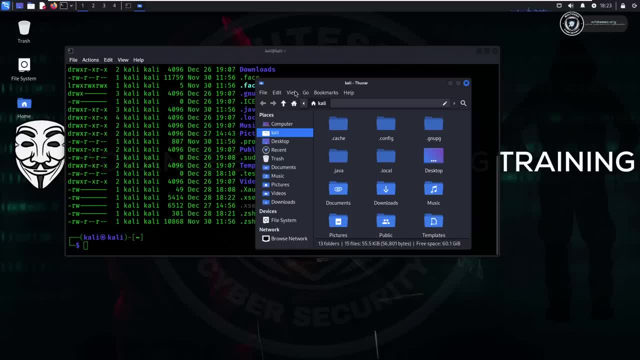 okay, assume that you got the shell. it's a linux server. at that time. you need to remember this command, which is ls dash al. mostly in cdf challenges. you guys can able to see a lot of things now here. let me uncheck it now, how i can able to create the hidden file here, the simple. 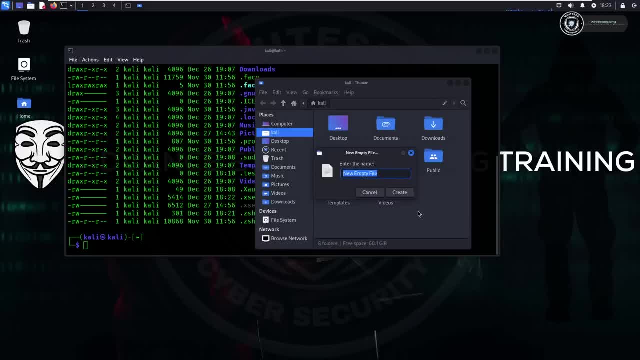 thing is, you can able to see the hidden files as well. how simple- click on view- and here there is a simple thing- is create one document, just a empty document. just let me type here: test2.txt. now it's a normal. okay, it's a normal document if i rename it and let me add a dot in front of that name, okay. 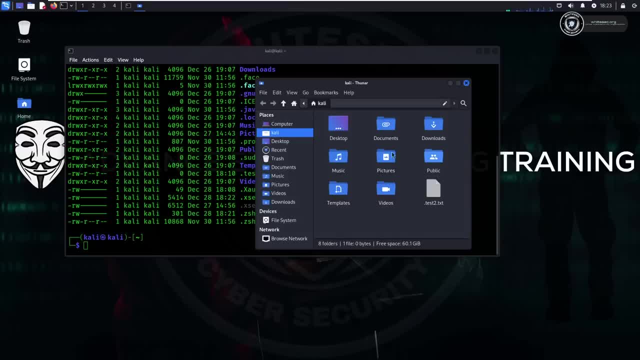 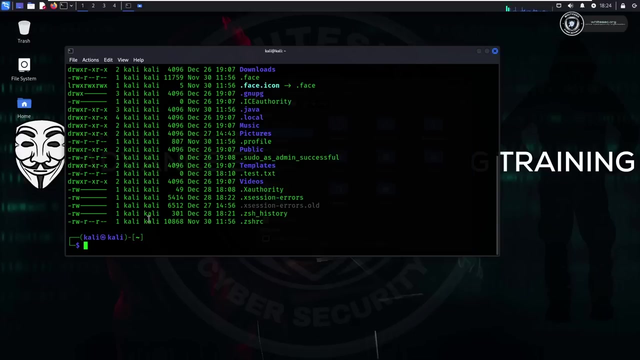 like this: just rename it, okay, just if i click on view and let me type here: show hidden files, let me uncheck it. now the file has been hidden. okay, this is the thing. if you close it and reopen it, then also the file will be hidden mode. okay, this is the thing. if i want to see it, how, what i need to do. 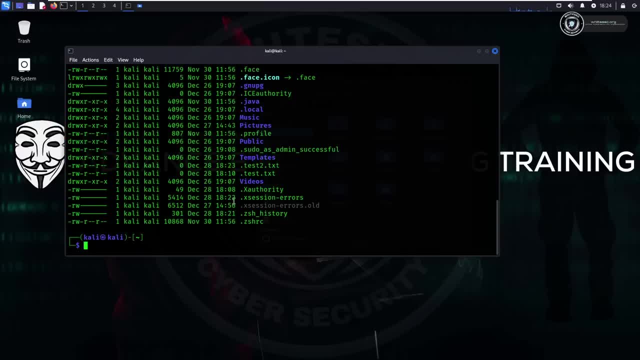 simply ls dash al. if i type this thing then i can able to see those hidden files. okay, here see test2.txt. is there right? okay, now just focus these points, which is checky profile, so it may be like clay and kali. okay, what is this basically see? first thing is: 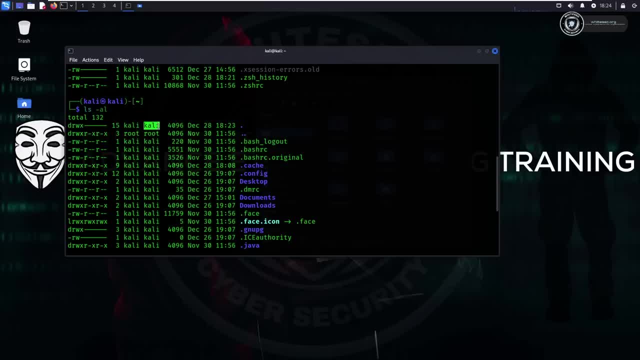 nothing, but it's a user, okay. and the second thing is a group. here in the next class i'm gonna explain you about the what is users and groups. you no need to worry. see. remember one thing here: if you create any new user in kali linux at the time what will happen means it will automatically create new. 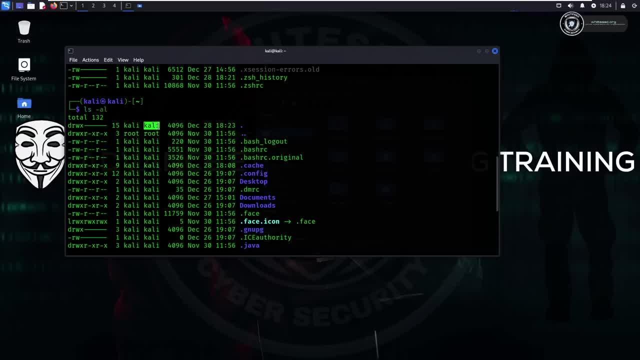 group with the same name. okay, this is one important thing which you need to remember. this is a by. you can't able to change it. you can also copy and delete that folder and you can able to do the integration, you can do the subjet, but by default, what in kali linux, what happen means? 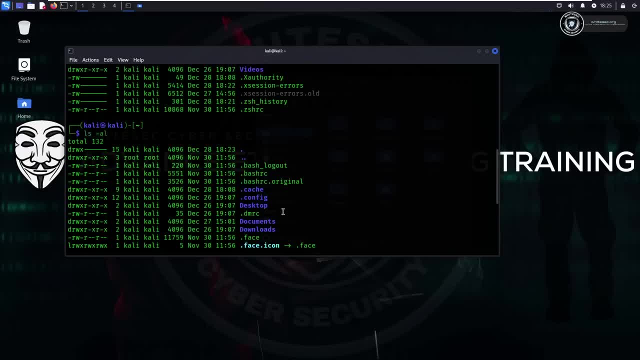 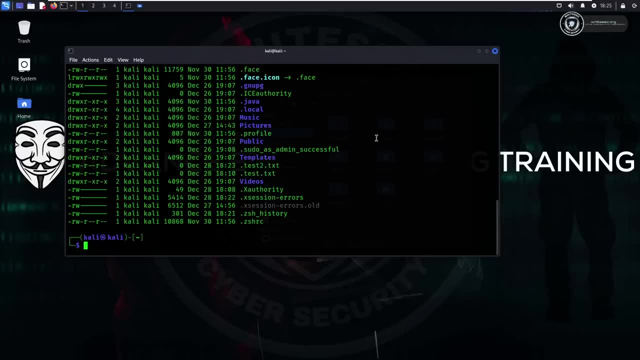 assume that i want to create one username. okay, one user in this account, in this, in this system, in this kali linux. at that time, what i need to do? uh, in the i can able to create it. okay, once i create the user, that kali linux will automatically create one group for it with the. 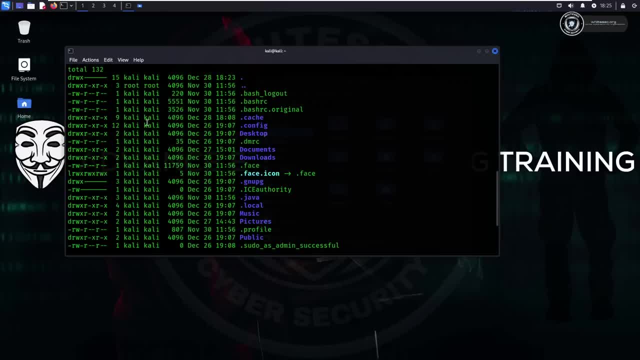 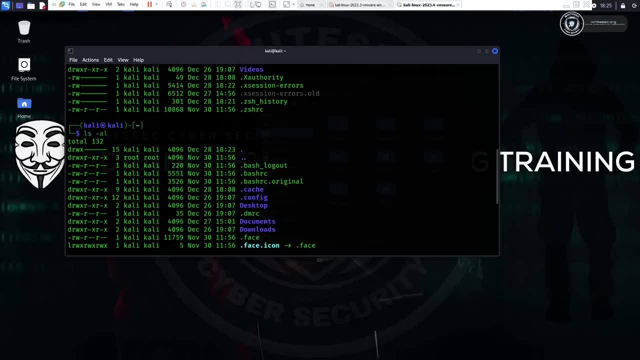 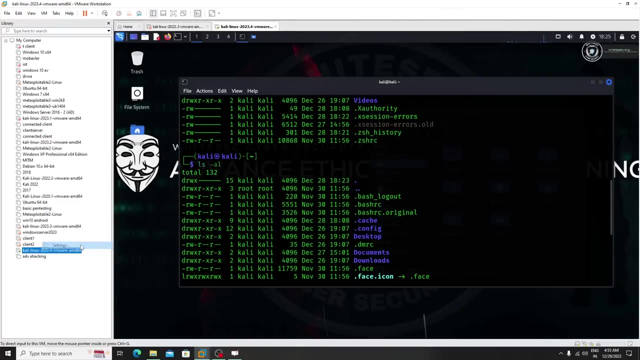 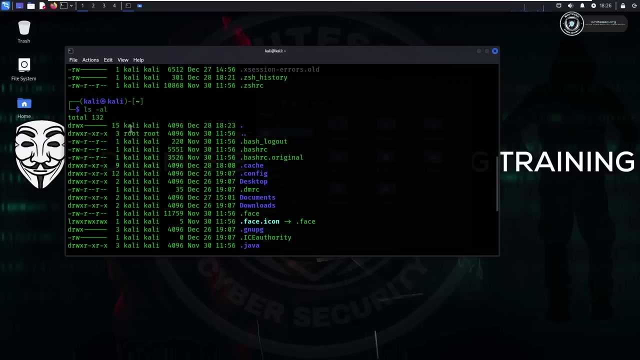 same name. okay, so this is the thing right now we are. uh, the by default user is what? here it's a kali, right, it's a by default user. let me show you, okay, where it is. man like: uh, it's a by default username and the password, right, we just saw in. 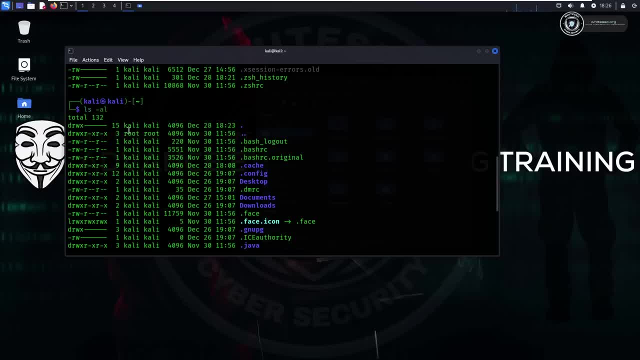 the description of the vmware. so the thing is, it's a by default accounts, uh it uh. the simple thing is what i am trying to say. the first thing is user and the second thing is group here, okay, hope you guys get it. this is also one user is there with the name of root and there is a one 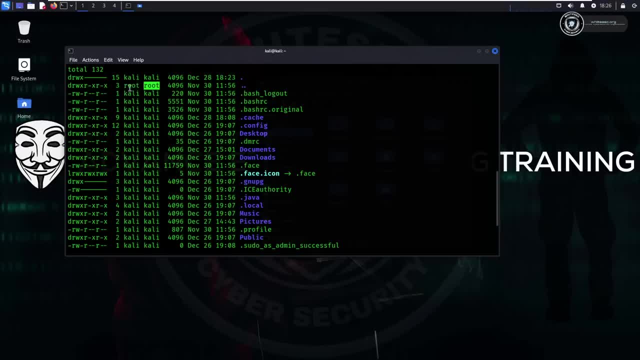 group with the name of the same thing, with the same username as a root. okay, i just told you, once you create any new user, automatically kali linux will create one group for it and it will, uh, name name the same name as a user. okay, now let's focus on this thing. what is this? dr wx, something like that. now, just 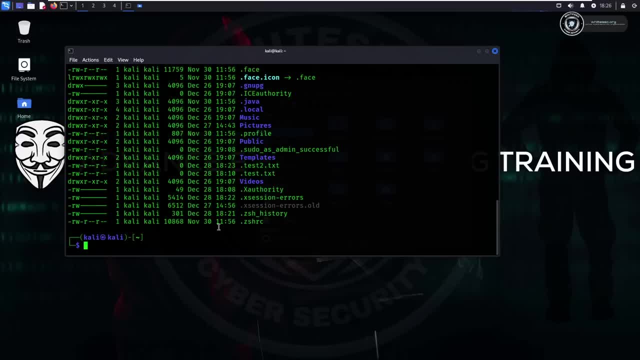 focus here. let me create one new file again. let me type here touch, for it's like dot txt. if i type here touch, for it's like dot txt, type ls. okay, let me type c ls. if you type dash l, also you guys can able to see the things here. 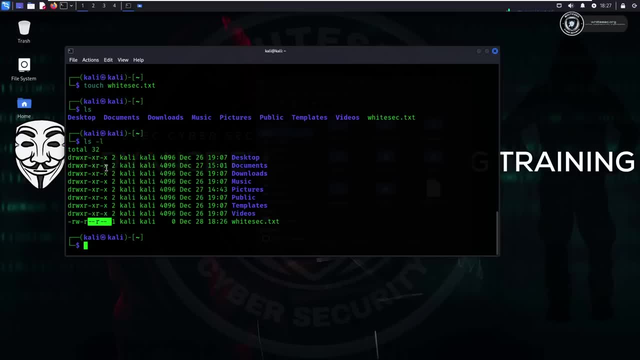 you won't see any kind of hidden uh files, the simple the, the key is here a. okay, if you add the a, then you can able to list out all the hidden files. if i type normal, like this, ls, space, dash, l, then you will see like groups, okay, like the date each and everything like uh, the execution things. 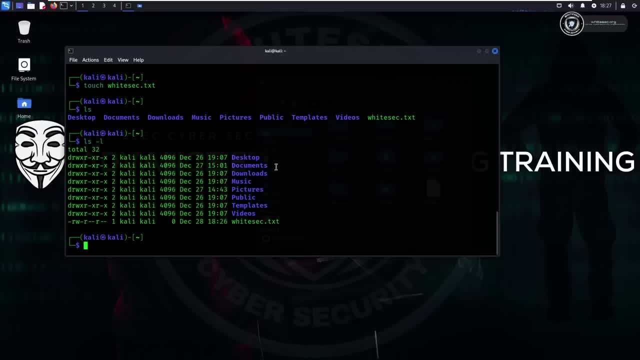 the permissions, something like that. now here, just focus, there is a drw. uh sorry, drwxr is there? okay, see, always remember. i just told you right in the last class as well. in linux we say folder as a directory. okay, folder is a nothing but this. 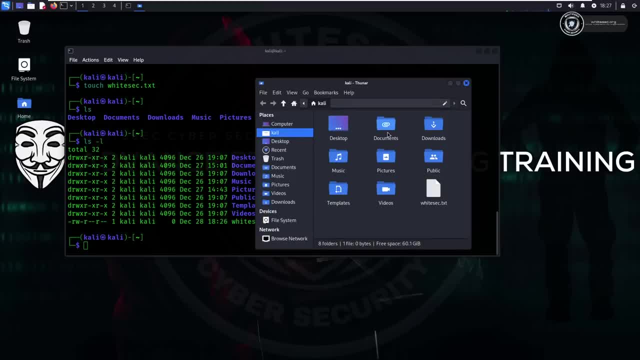 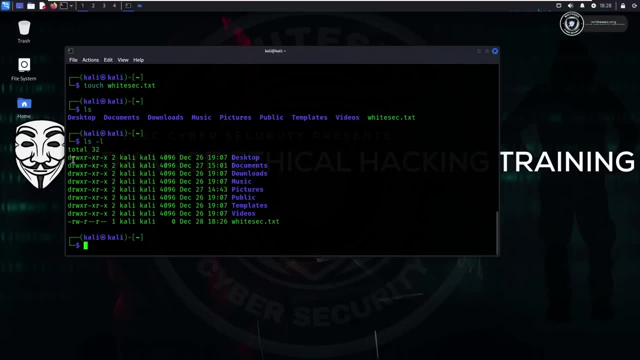 folders. i am talking about these folders. okay, these folders are nothing. but what is this? in linux, we say it as a directory. okay, this is the thing which you need to do. okay, so remember. so that's why here in starting, you guys can able to see d here. okay, that means it's a. 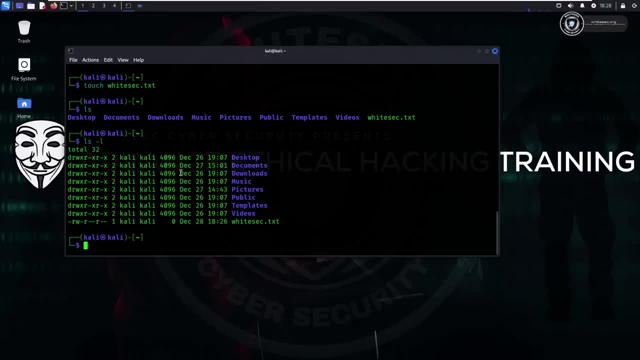 directory. that means it's a folder. this is the thing. and here, just see, i just created one text file right wide sec dot txt. here at starting you guys can able to see dash here. that means it's a file okay once. if you see the dash here, then what is that? it's a nothing, but it's a file okay now. 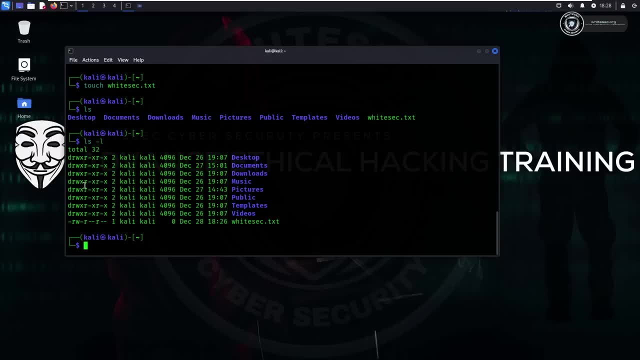 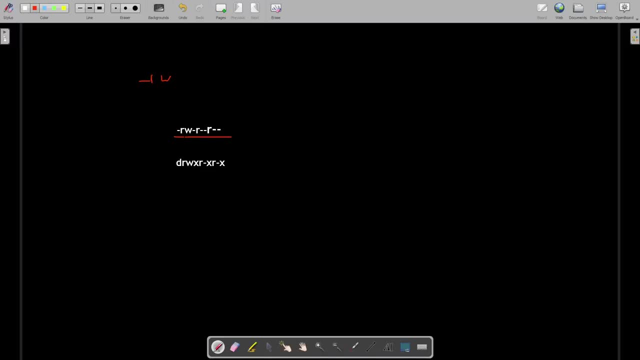 let's see that this things. okay, what is rwxr? okay, right, here i just added something. okay, uh, here you guys can able to see dash rw, dash, r, dash, dash, r, dash, dash, something like that. okay, now, here we. i just told you right. once you see dash at starting, that means it's a file, any txt file or something like that. 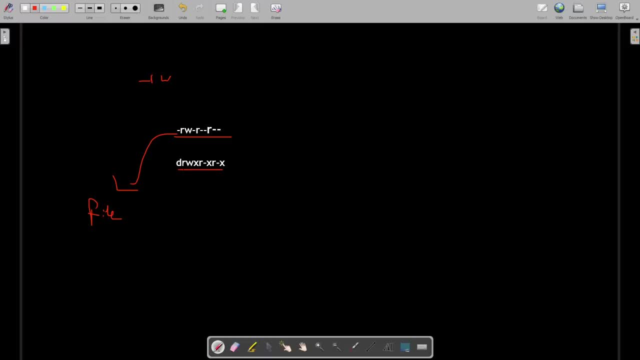 any document. if i see, see, see see d in starting, that means it's a directory, it's a folder. okay, now what you need to do, see simple. there are some stuffs out there which is same, such as: r is here, w is here, x, x is not there here. okay, let me uh write the definition of this thing. 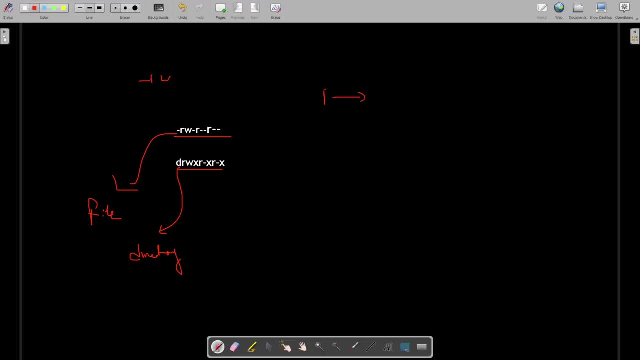 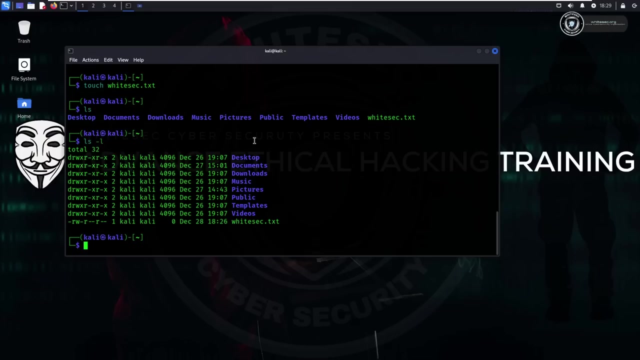 r is a nothing but a read. okay, r is nothing but what read. w is nothing but right. okay, there is a x is there. x is nothing but execute. you will learn. you will see in privilege escalation these things are very important. okay, see here what is read. see, read is a nothing but simple. 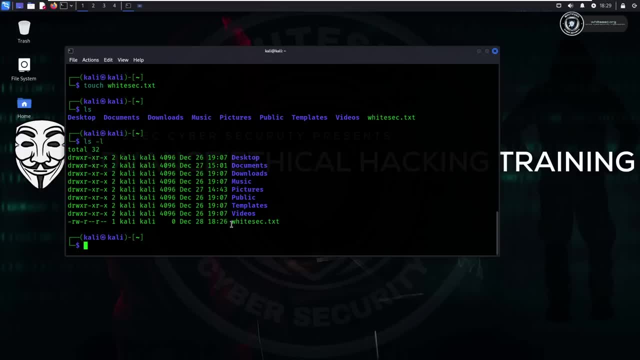 i can. anyone in the system can able to open this file and he can able to read it. okay. okay, what is a right? right is a nothing. but after opening this file, he can also modify it. okay, he can able to edit the text here. anything. it means it's a right. assume that. 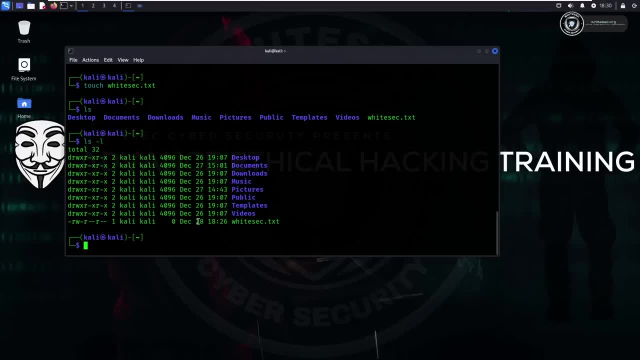 there is a kind of any python file. okay, if there is x there, okay, he can able to execute it. see, in file you can't see the x. okay, this is a kind of security, you can't able to execute it. okay, you can able to open the windows videos, templates or something like that, but you can't able to. 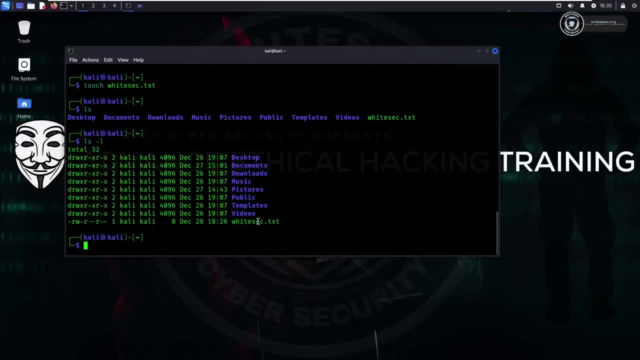 see the x here. okay, in files. this is the thing now. just see if i type here ch mode plus x. okay, let me give all permissions to this thing. just let me show you to this file. okay, now let me execute. let me type ls, dash, l. here you guys can able to see the permissions. 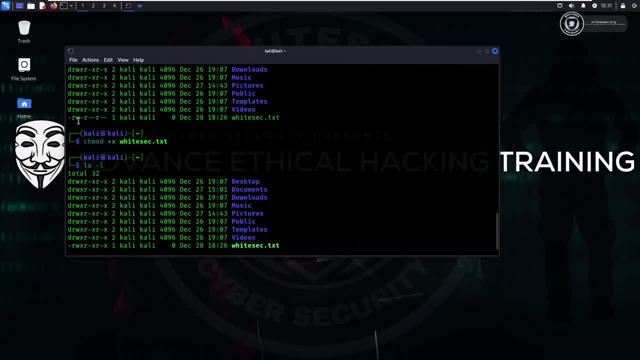 has been changed previously. it's simple: read, write okay. now here you guys can able to see. it's a read, write okay, execute. hope you guys can able to see it right. so this is how the things will change, right, by executing the ch mode plus x. yeah, you can also see that ch mode triple seven is also is there. mostly people use this. 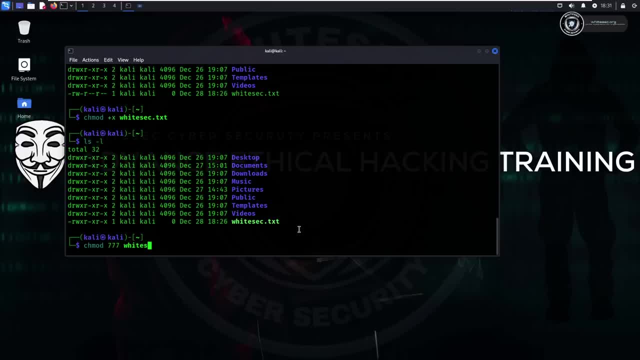 thing, okay, uh, in hacking in term marks, something like that, we use a ch, ch, mode, triple x. what is this thing? okay, uh, let me explain you this thing as well. it's a kind of automation tech, uh, like a addition thing. okay, let me explain you those things as well. first of all, let's focus on this. 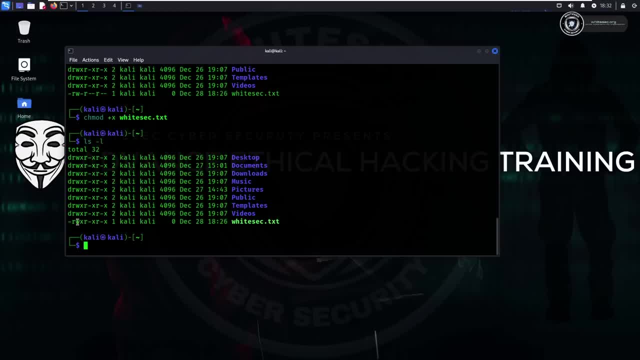 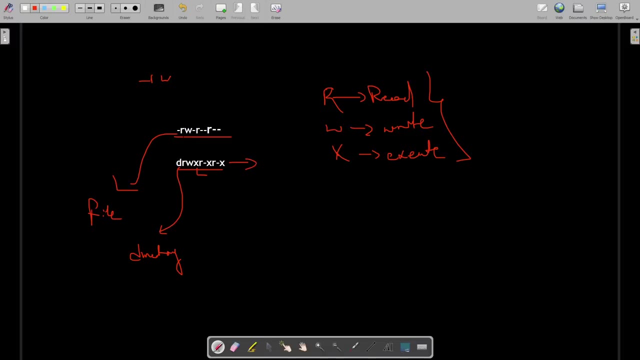 thing. okay, uh, now this will be differentiate in three things. okay, here in between there are some dashes, are there? what is this? now let me explain you here. see here, let's take this example because dash r. see, just just explain you by using this one. see here, dr w is there right and x is here and r is here and dash is here, and then xr. 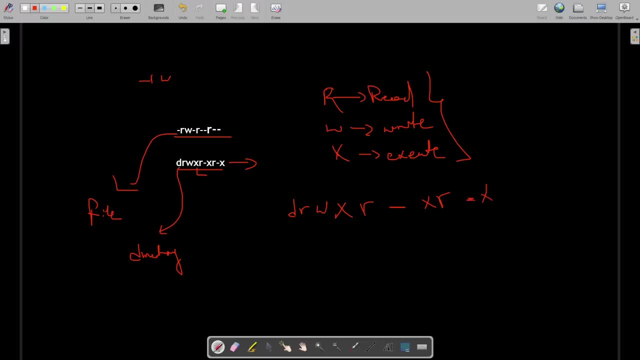 and dash x, something like this. now it will be d differentiate in three things, okay. one, see, just just ignore this part, just start from here. one, two, three, just close this one. it's differentiate in one thing and there is a one, two, three. this differentiate in one thing, one thing, okay, and there is another thing like. this is how it's. 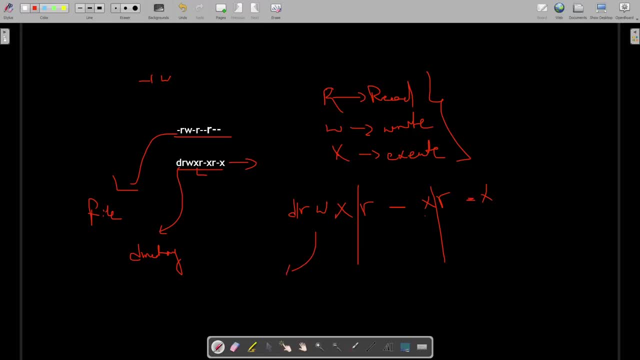 gonna work okay. now, first thing is a known as user- okay, and second thing is a known as a group. you will learn this all steps in the next class, right in the third class, is known as a- anyone who is in that computer like any user or group. assume that you just created a lot of user. 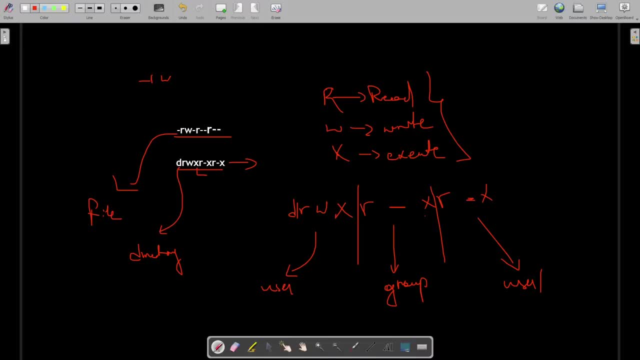 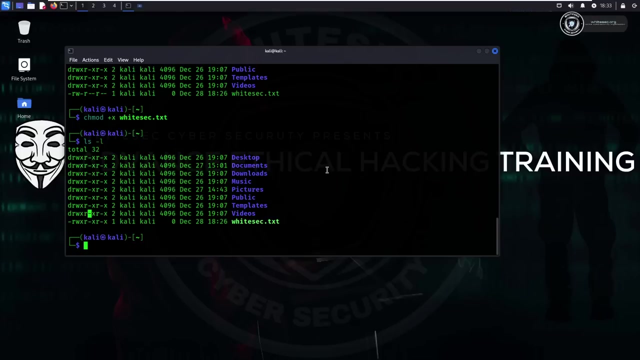 there. yeah, if there is a read write, execute permission is there. that means anyone can able to execute it. execute that file. okay. now here in the group, assume that in in kali linux, what will happen means the specific user can able to run as administrator. okay, which is known as a root user. we, uh, once we just type sudo su there. hope you guys can able. 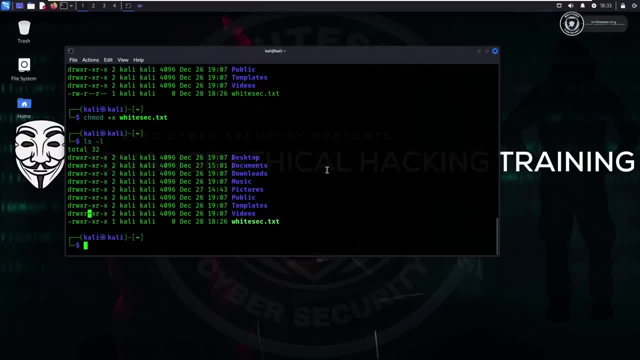 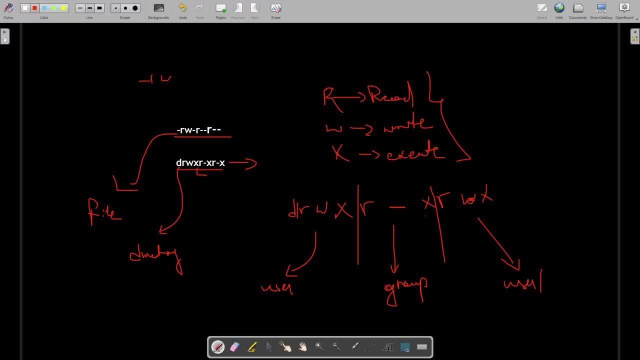 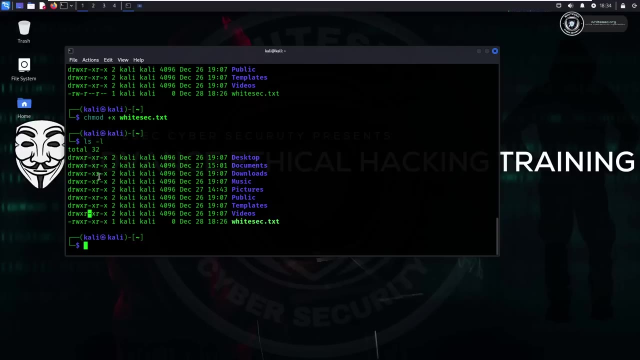 to see. we will become the root user there, the simple thing. the second thing is a known as a group user. okay, like, uh, the root guy can able to do the steps and here there is a user. okay, user is a nothing but the by default user or any kind of root user, okay and able to execute as a that. 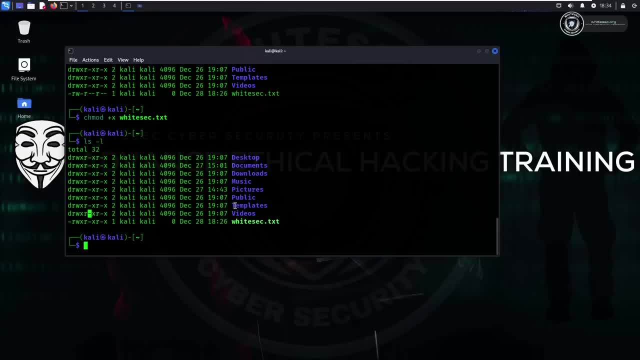 file as a uh, as he can able to execute it, he can able to write it or something like that. because the thing is basically it's totally depend upon the restrictions. okay, specific user can't able to do the all steps. one user can can able to do that all steps there. assume that he's a local administrator in that system. he can able. 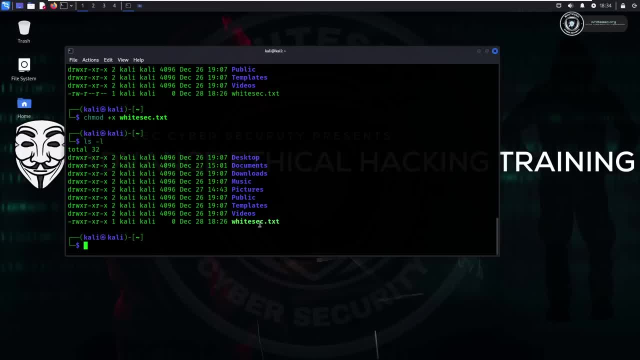 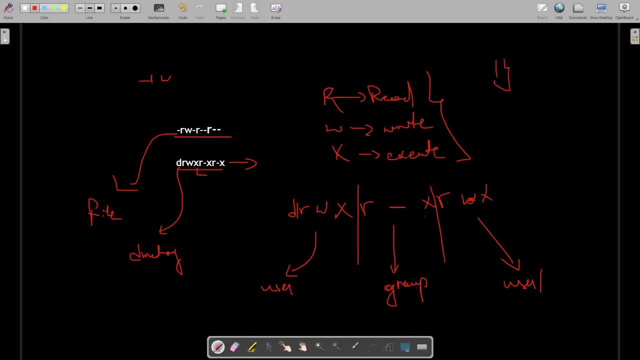 to do anything, right? the simple thing: uh, you just need to take this scenario here. okay, now there is a? uh, there is a. uh, there is a kali linux. okay, in kali linux you just created some normal user so you they can able to access your system. okay, and you want to add the restrictions there, such as: 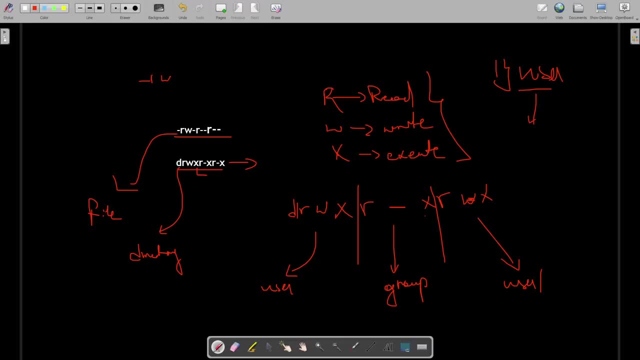 they won't. they can't able to delete the files, okay. they can't able to open the images- okay. uh, they can't able to execute any files there. okay now, see here. assume that this user is known as a, something like: uh, just let me name it as a harry, okay now. 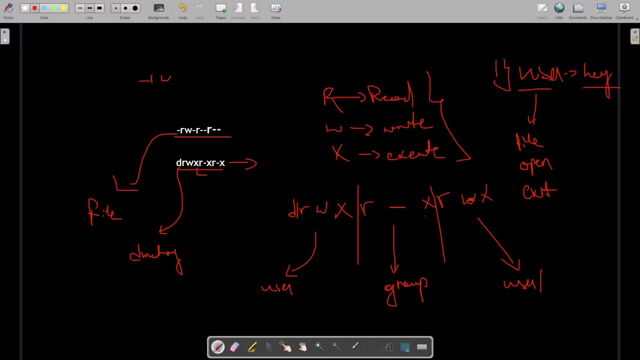 this is a one user. okay, harry, in your kali linux, what he did means: uh, you just added some restrictions to his account. simple, he can't able to access the files. okay, simple, he can't able to edit or open the files there. simple, what will happen means this: once you 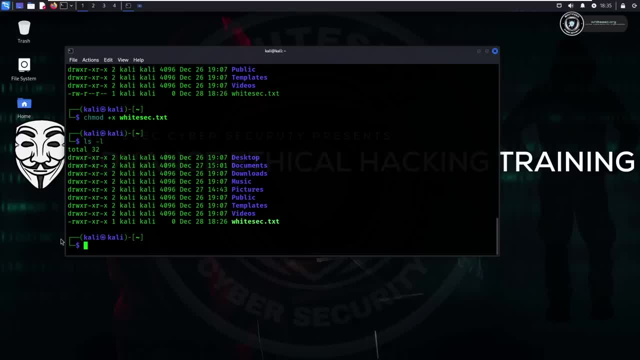 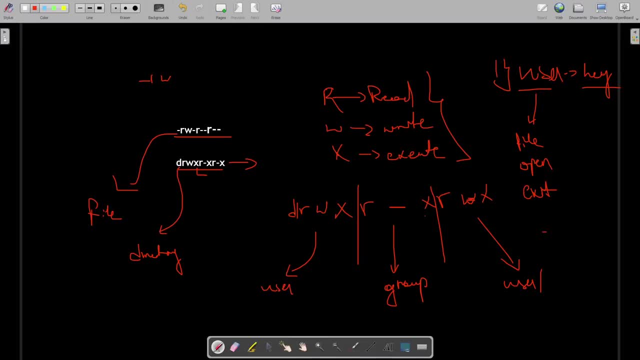 add the restrictions, then you can able to see the dashes there instead of rwx or something like that. okay, the harry will look like this one. okay, something like dash, dash, dash. okay, then again, dash, dash, dash again. okay, that means he can't able to do anything there. he can't able. 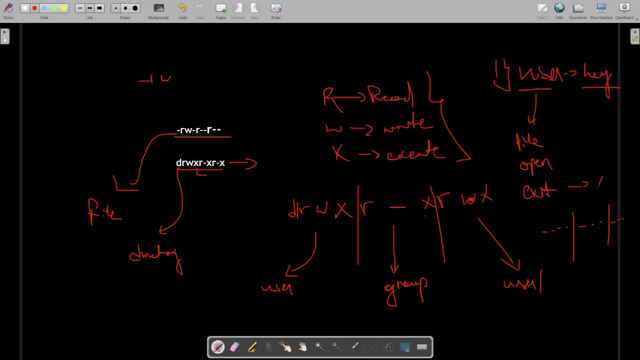 to execute. execute is in what? here, it's a nothing but x, right, this thing where it is x? okay, just let me take this one x right now here. uh, what is your open? open is a nothing but read, right. and what is w here, right? uh, the file i? i simplify, just edit, okay, if you want to. 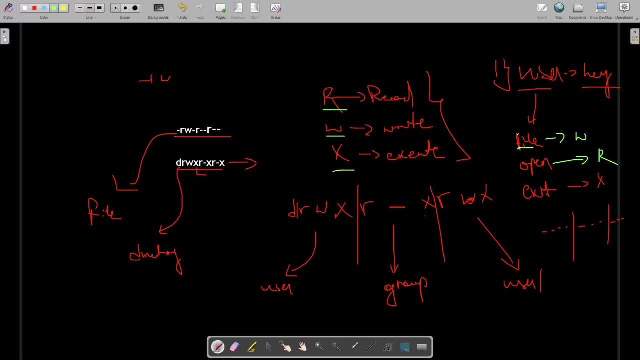 edit any file, then it's a w, so this is the thing he can't. you can also say it as a. he can't even download the files there. okay, from internet or some from using github or something like that. okay, if you remove the restrictions, the simple thing is this will be look like: 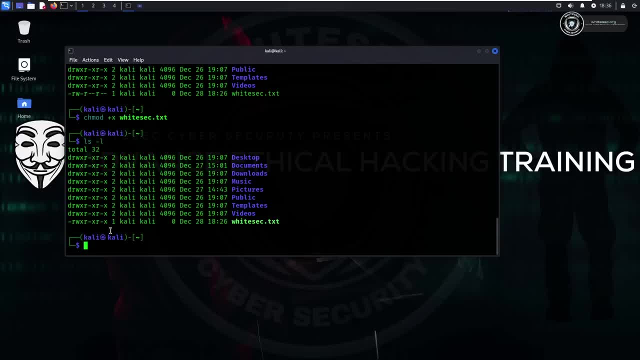 dash, dash, dash or something like that. okay, this is the thing. in the next classes we will cover more about these things. okay, now let's learn about this one. okay, why we use a ch mode 777? okay, something like that. what is this 777? and you, you will give the permission here. 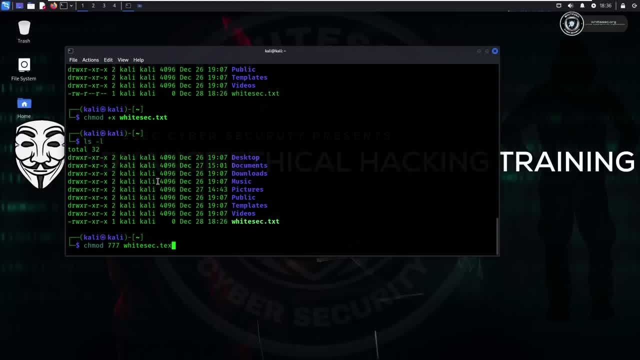 let me give the wide set dot txt for type ls, dash l. here you can able to see more things. okay, he can. he can do anything now. okay, any, any user in this kali linux can able to execute this thing. okay, he can able to. uh, anyone can able to open the file. okay, because i just 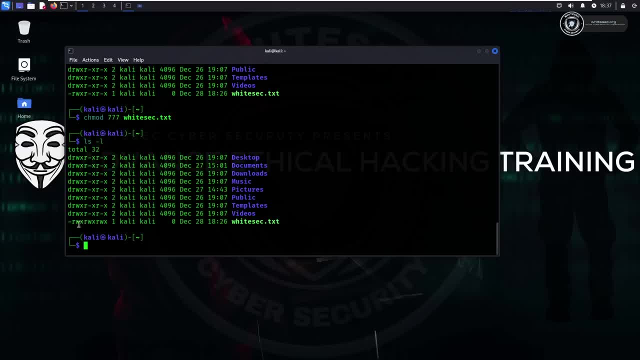 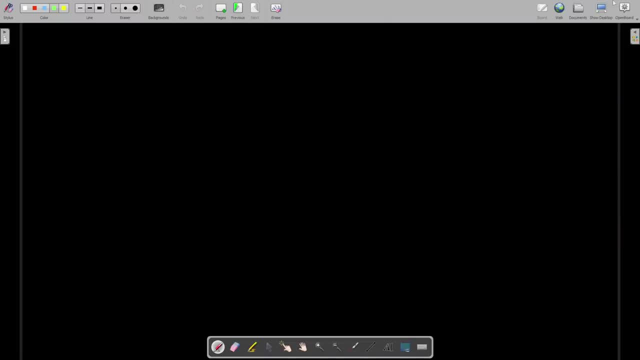 told you this file is open. okay, so you can open the file. okay, because i just told you this will be differentiate in three things. one is user group or anyone. now let's learn about this thing. okay. what is this? ch more triple seven, or something like that. 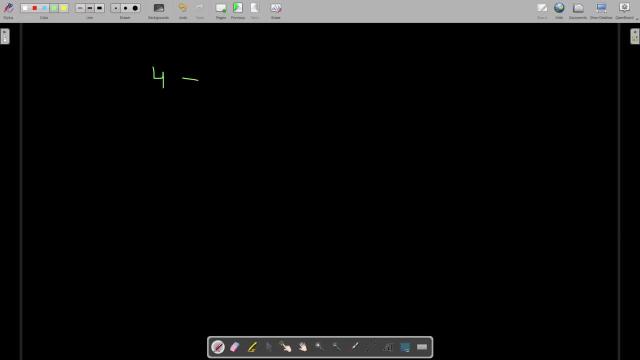 see here there are numbers. okay, four is a nothing but read permission. we use this four to give the read permission. okay, like anyone can able to read that file and there is a one. okay, one is for execute permission. if you add one there, that means the user can able to execute the file there. okay, permission. see if you. 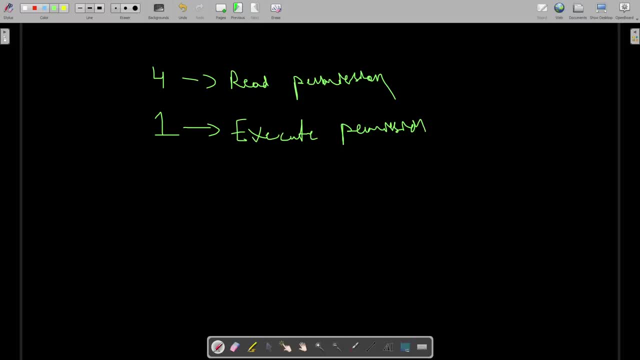 are familiar with kali linux, then you guys can able to get it. if you are not, then it is little bit hard for you. this is the thing now here there is a two. two is for to write the permission. sorry, write permission. he can able to edit it. okay, write permission. and there is a zero, zero. 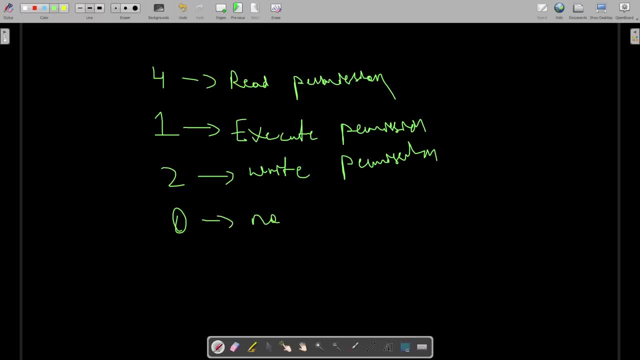 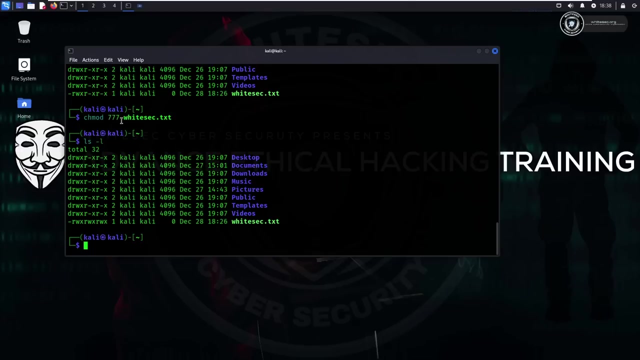 is a nothing but no permission. if you want to add any kind of restrictions, then we use a zero here. okay, to remove the permissions, or something like that. now see here why we are giving the ch mode triple seven. what is this? okay, see here. i just told you right, it's a. 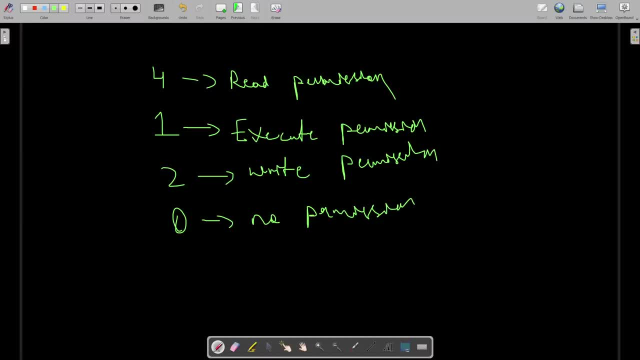 kind of a thing that we are giving the ch mode triple seven. what is this? okay, see here, i just told you right, it's a kind of uh addition. okay, not not kind, it's a addition, basically. okay, see here, what is a seven? we can't able to see the seven right here. we can't able to see seven here. 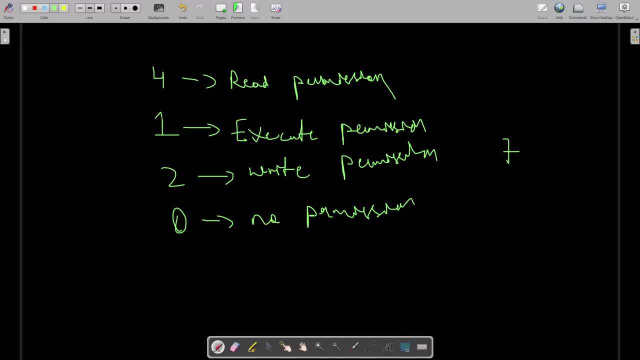 now see, seven is a nothing but four plus one. what is that? five, okay, five plus two. what is it? seven, right, simple seven. okay, i just told you previously it will be denoted with three groups, okay, one is you user. sorry, it will differentiate in three things, right? one is user, one is group and 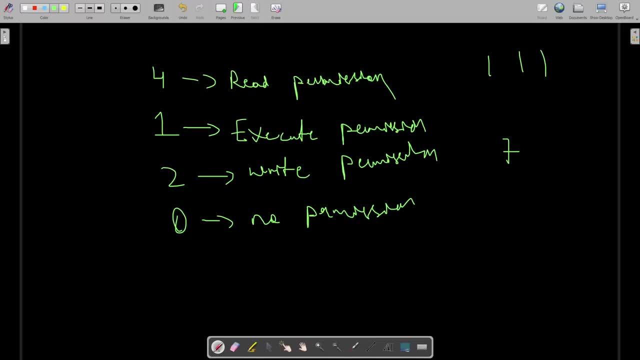 there is another stuff, so other guys, okay, like you just created any user, it will affect on them. okay, now, here there is a user, there is a group. okay, there is a others, anyone you just created one user, okay, who is using those that kali linux? okay, right now, this will first. 7 is 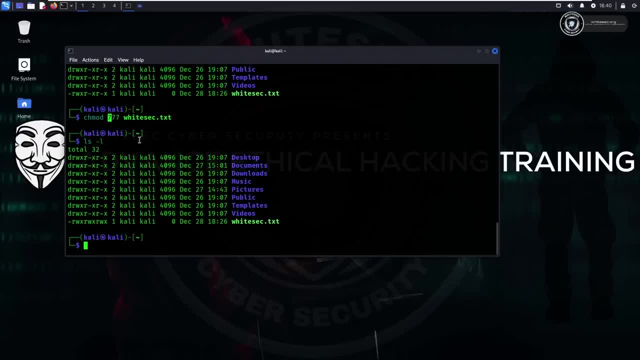 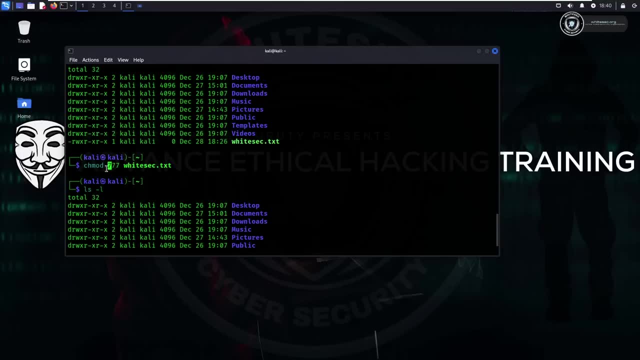 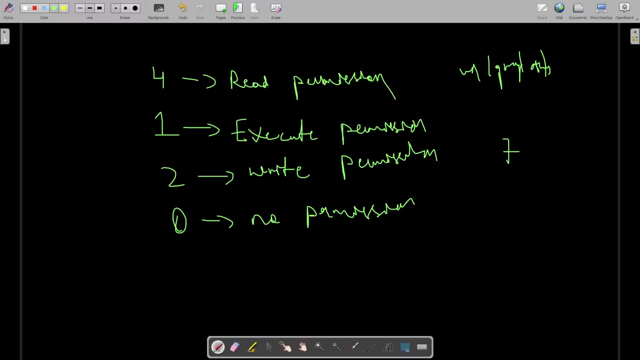 effect on user. okay, this first seven will effect on where? on effect on user. okay, like kali user, root user is there, it will uh he, that user can able to execute that file. okay, now the second thing will be: execute on. the second seven will execute on what it will execute on the groups: okay, 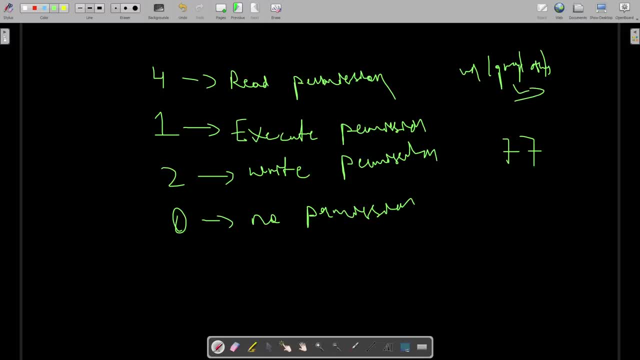 i just told you what our groups are. and the third thing: will execute on anyone who are using the kali linux. if is there any kind of user- normal guy, administrator, local administrator- it doesn't matter, it will execute on the normal guys as well. okay, like he can also execute that file as well. okay, now here. so that's why we add the three triple seven here. 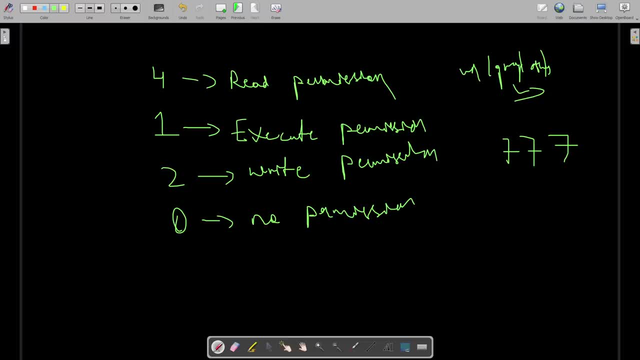 okay, what is the uh, triple seven here? triple. mostly the people will say that during the giving the permission they will say that you need to be focused when you execute this command. okay, when you add something like ch mode triple seven, at that time you need to be focused okay. 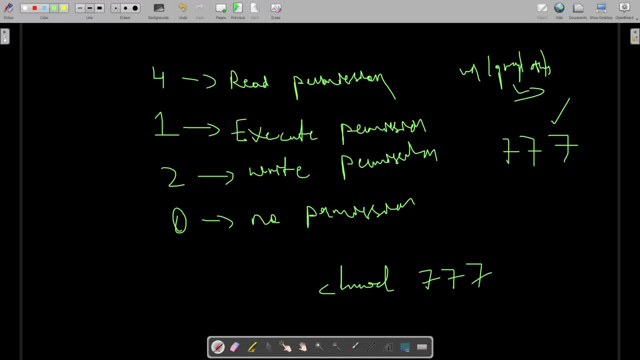 don't give this permission to any file, because anyone in that system can able to execute that file or anyone can able to read it. okay, it doesn't have any kind of restrictions or something like that. any user can able to read it. okay. so this thing will give you a complete unlock. okay, to any. 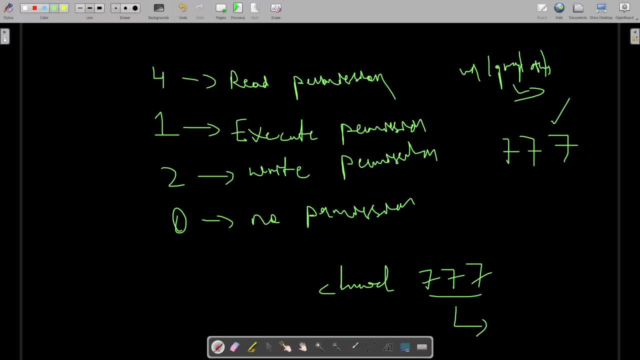 user. so that's why see why it's giving the unlock. the simple thing is: four is for what read permission, right? one is for what execute permission, right? second is for two is for what write permission? now, simple how it's gonna look like. okay, uh, simple, it's look like this: uh, read, read, write r and execute. 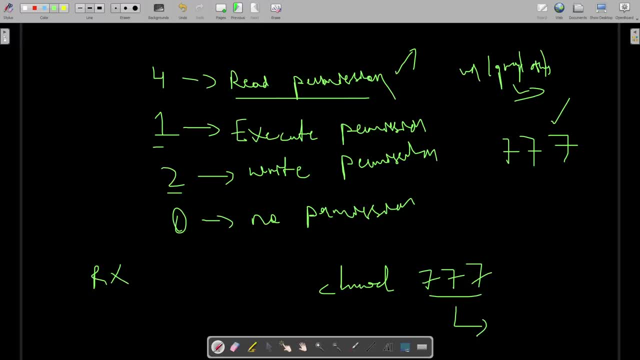 is x. okay, and right is what w. this is how it's look like. okay, not okay. it's use a small r: okay, this is how it's look like. okay, so anyone can able to read it, anyone can able to delete it. anyone can able to see it. okay, you can also see the uh ch mode 444. okay, something. 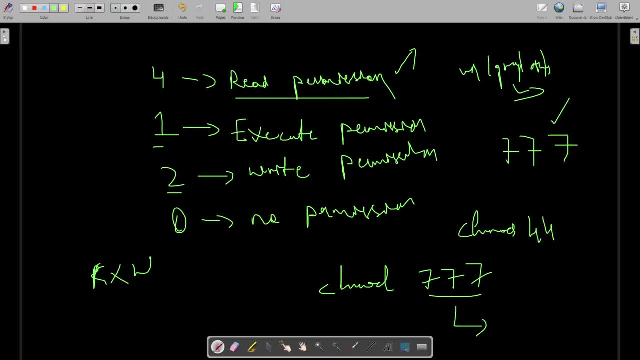 like ch mode 444, something like that. what is this? the simple thing is you are giving the read permissions to them. okay, simple, he can able to read it. he can't able to execute it. okay, something like that. it will look like this: okay, if you are giving the permission to any file, at that time it. 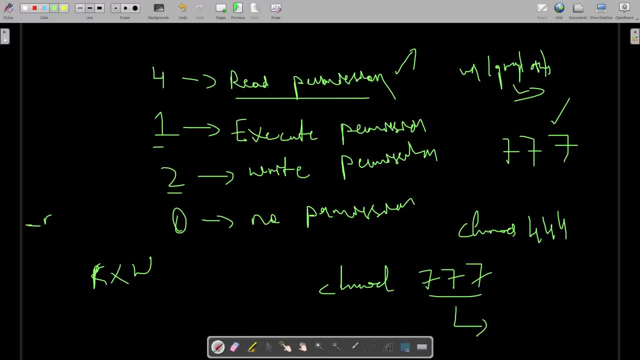 will look like this: okay r, okay, something like that. r dash, dash, r dash r, something like that. okay, hope you guys get it now. uh, assume that if you are not getting this class, what you need to do is just do some research on it. okay, about kali linux: if you know the simple basic linux and 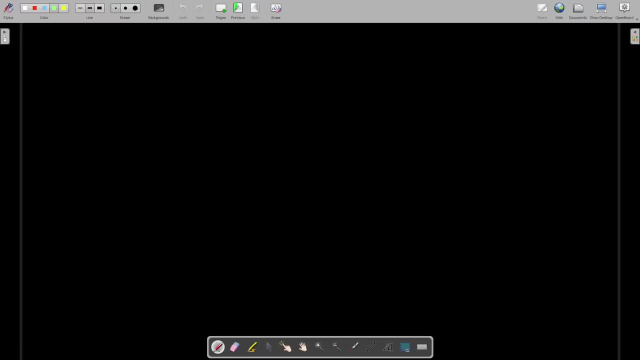 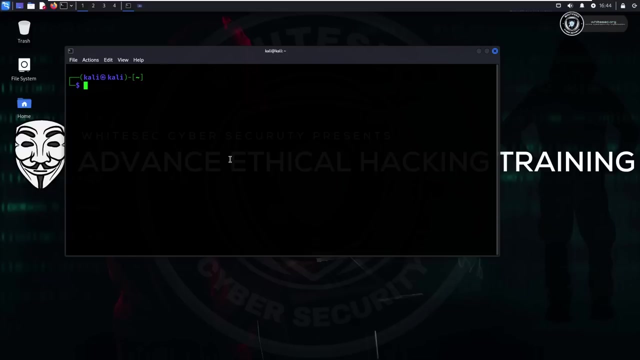 you guys will get it. okay, it's not a big deal. okay, it's a very easy and excellent things which you need to know right now. in the next class, the things will be here, right right now, here. see, if i want to add any user here, then simple, just i'm gonna execute. 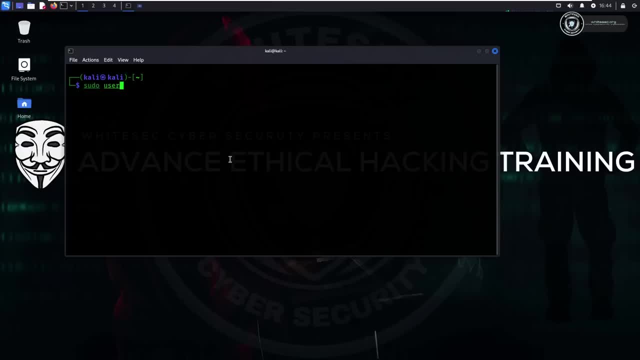 this command. okay, sudo user add. i'm adding a new user in my linux machine. okay, simple, just let me add a user with the name of test. okay, now the user has been added with the name of test. okay, now here, just see if i want to delete this user. uh, then simple. what i'm gonna do? simple, just type sudo user. 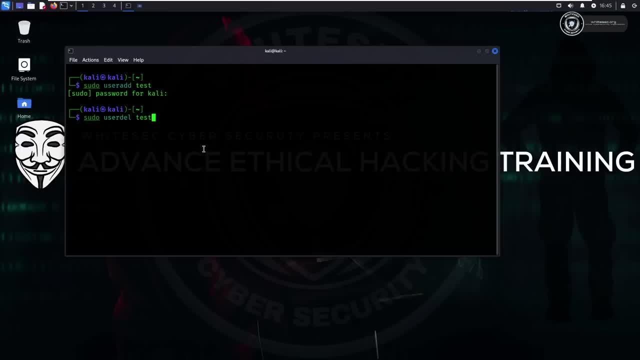 delete. okay, del, and just type the username simple. the user has been deleted there, okay, this is how it's gonna work in the last class also, i just told you, once you create any user, assume that i just created the user with the name of test, automatically the user, uh, this. 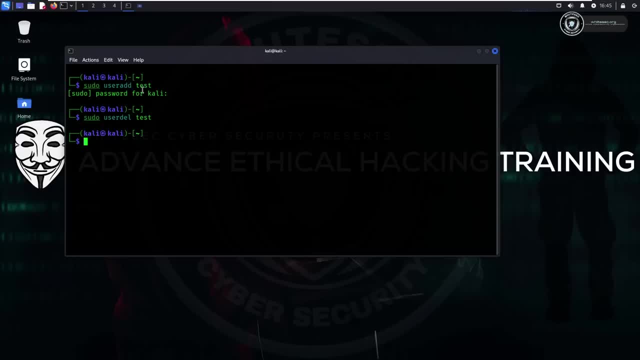 group will be created in the kali system. the group has been created with the same name of test. okay, this is the thing now. sorry guys, now let me, let me create again. okay, let me create the user with the name of test2. okay, now i want to set the password for test2. okay, how to set that simple? 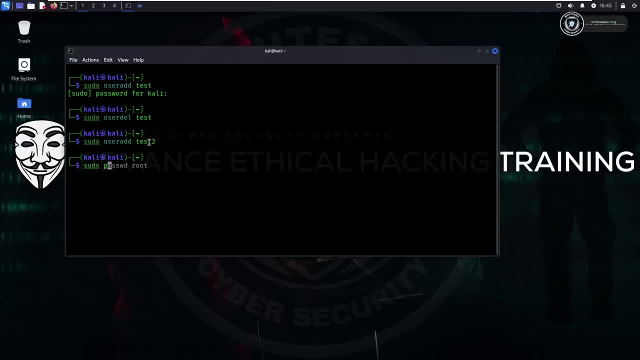 just type here: sudo, which command we just used. uh, once we just changed the password of root user. the same command you need to use, sudo p-a-s-s-w-d password. just add the username there. okay, which you want for which user you want to add the password? simple, in my case, the path i want to. 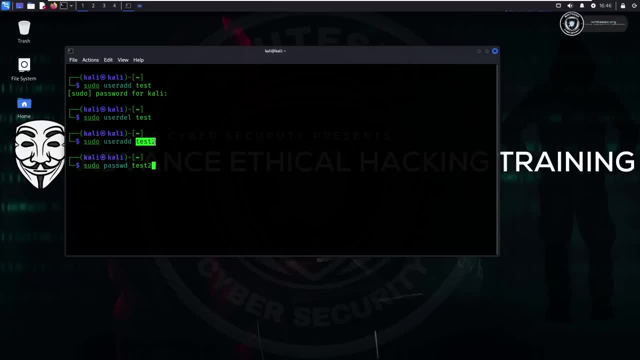 change the. i want to add password for this test to user. simple, just type enter. now, here you can able to select the password for this guy. let me type the password as test. okay, see, password successfully updated. right, this is how we can able to create the password here. now let's do. 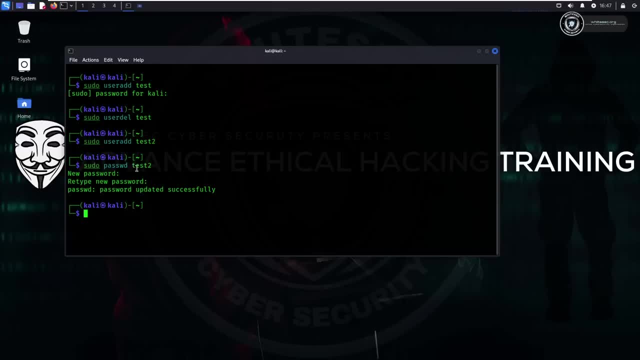 one thing, let me connect, let me interact as a test to here. okay, simple to do that: just type su. test the username of that guy. okay, which i just created. test to just type enter. now it's asking for the password. it's a nothing, but it's a kind of change user here. okay, i am changing the user. 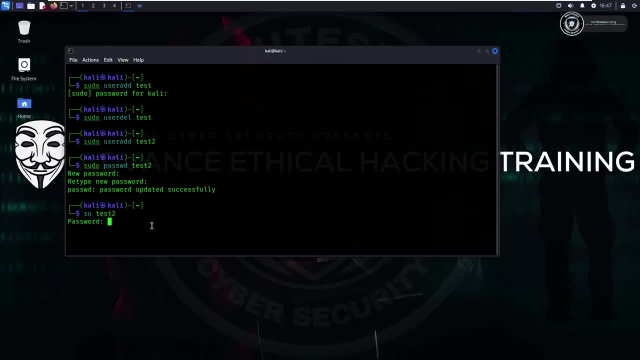 to test to. right now i am kali. just see here, right now, let me type the password. if i type password, then here you guys can able to see i got the dollar sign. basically, it's not a bin bash, simple, if you want. if you want to get a proper shell, just type here: bash now. here you got the shell here. okay, right now, see, i am a. 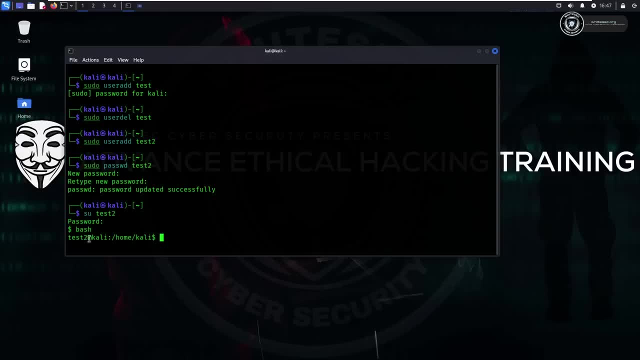 test to. okay, i am interacting with this machine as a test to user. okay, if i type here who am i, you can able to see: i am test to. okay, i am interacting with this machine as a test to user. right now i am a test to. these. things are very important during the pen test. now simple, just see. 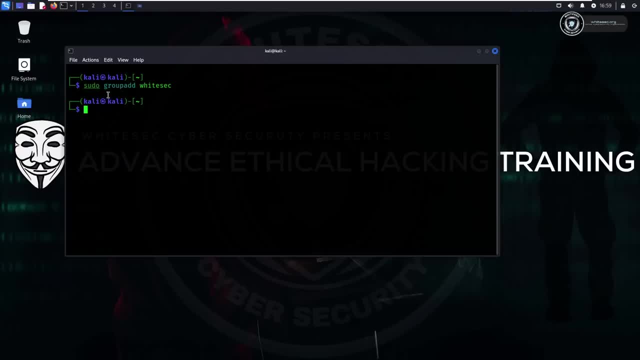 if you want to create group, just type sudo space, group, add space and your group name- any name- you can add any name and also you can add the user to this group as well. okay, see, basically everything which we are doing is totally depend upon the groups and users, because, see we, we just learn. 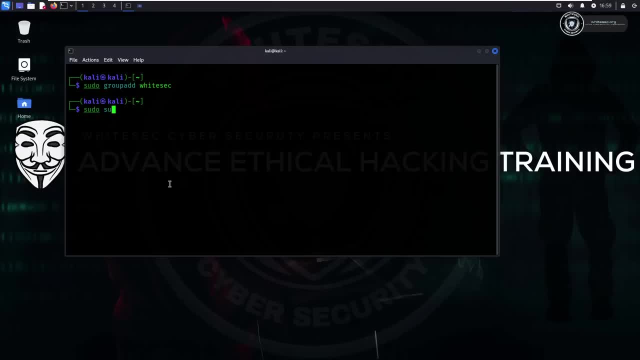 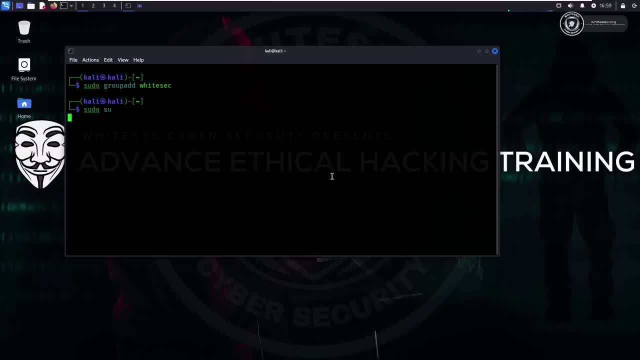 now i uh. right now i'm gonna interact as a root user. just wait, see basically what is root here. root is also one guy. okay, previously, uh, before typing this sudo su, it's a kali. okay, after typing sudo su, it will be: uh, the kali is changed to root. okay, basically, these are the two different users. 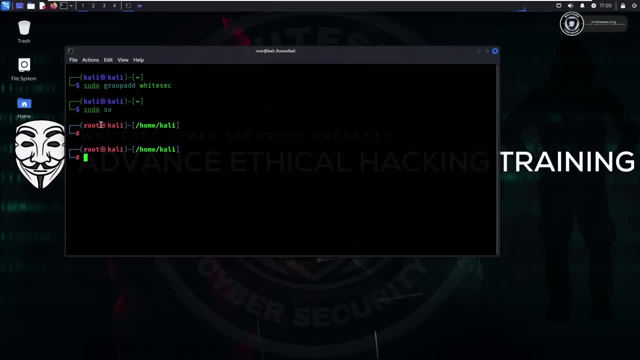 you need to understand this thing. okay, and it's having the groups as well. if you see, you assume that if you there is a kali user, okay, if i add this user to this root group, then kali user also do the same stuff which root do. okay, this is uh, sorry, man. which route do, right? so this is the 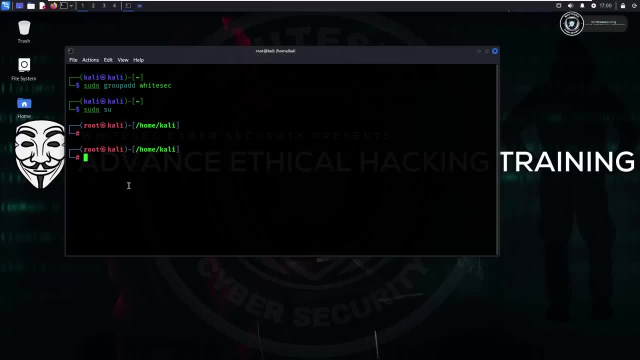 thing which you need to understand. okay, if you are not getting this as well, you no need to worry. just, first of all, just try to learn pen testing or hacking. just do some privilege escalations, then just do some kind of hacking things there, you will get it. okay, mostly the thing is: uh, what i 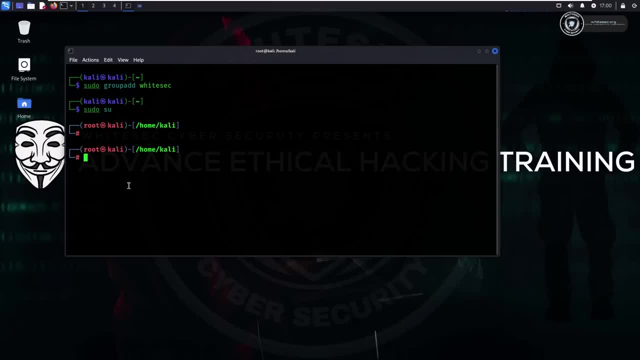 uh, what i'm gonna trying to say. uh, there is no rush. okay, you can just give time, you will get it. okay, this is the thing. and here, assume that i want to add some users to this group. how to do that? okay, we just in the last classes, we just created test user. okay, test to user, simple, i want to add the. 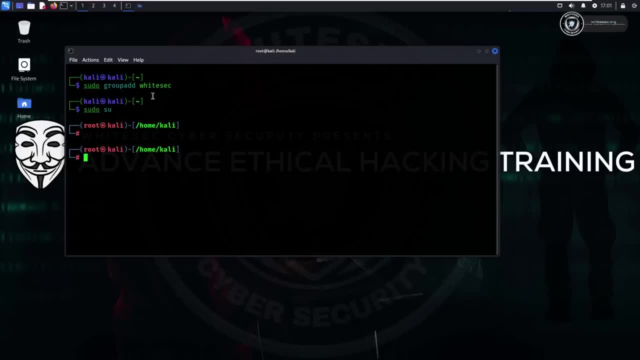 test user to this group, to wide sec group. okay, how to do that? simple: you can use this command: sudo. let me exit from here. okay, just type here sudo without typing sudo. you can't do that. okay, if i type normal, something like that user mode: okay, dash a to add. okay, dash capital g. 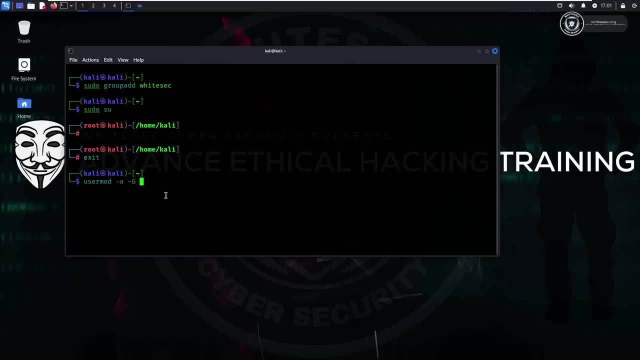 like, if you you are specifying the group here in which, in which group you want to add that thing, okay, that user, your target user, simple, see, i'm gonna target this group, which is sec. okay, in this group i want to add the user test to. okay, if i see it's saying that permission. 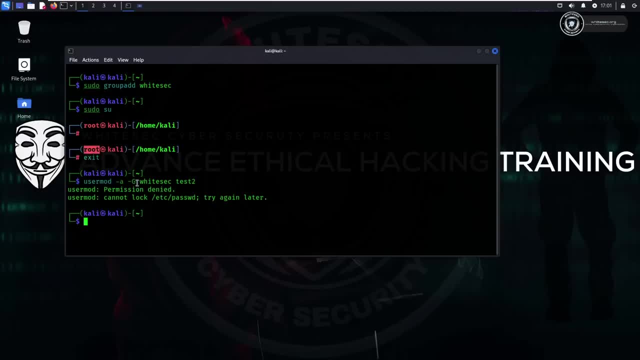 denied. you need to run this as a root user. this is the thing. if you want to execute this, then in front of user mode you need to add sudo. this is the thing. now it's successfully executed. now the in wide sec group. there is a test to user. is there? okay, this is how the things are working. 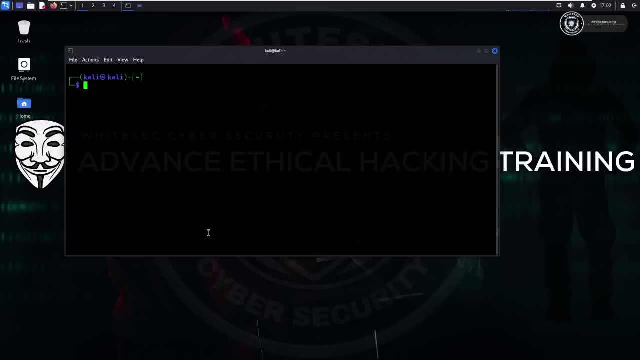 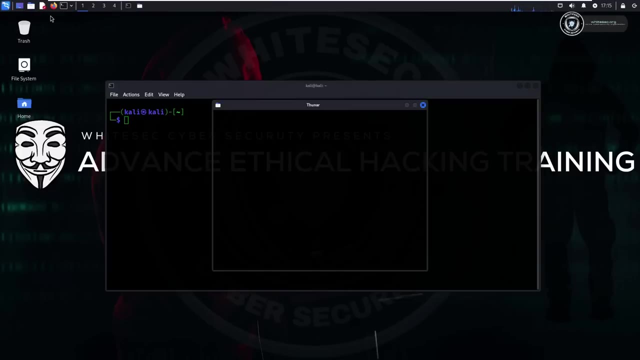 right, hope you guys get it now. in the next classes we are learning about, uh, the shadow file and the password file, which are very important. okay, right in this class, we are learning about uh, password and shadow file. right before learning about that password and shadow file, you need to know about. 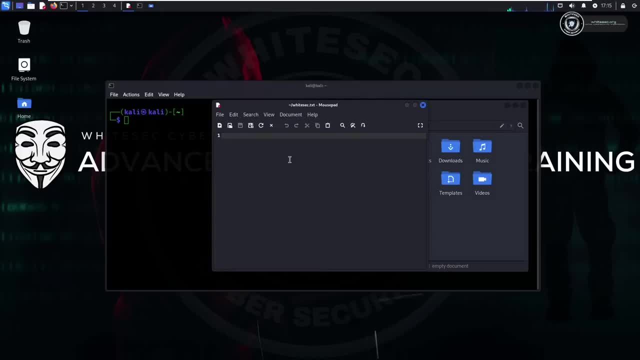 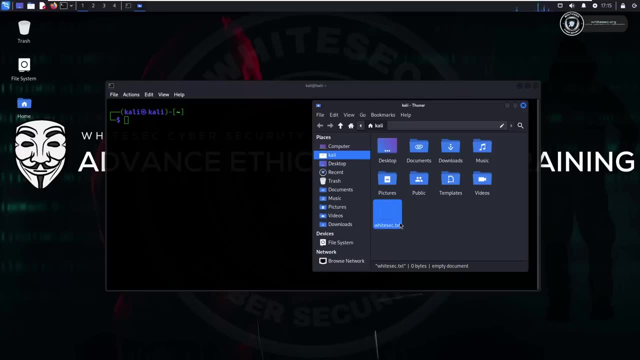 cat command as well. okay, see, cat is a nothing. but let me show you practically. see, this is one uh file. is here, right document file or any txt file? i want to open this file using the terminal. okay, how to do that. the simple thing is: let me do one thing just. let me write something here. 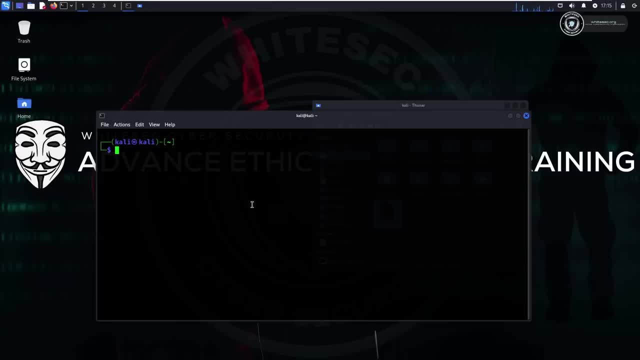 now i want to open this file. okay, just type here, cat. first of all, let me type ls, you guys will get it. see, here there is a text file, is there? now i want to open this through terminal. simple, just type here, cat and just type the file name. okay, now see, i can able to. 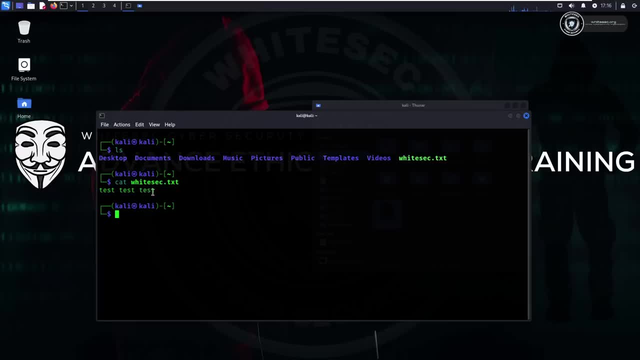 i can able to read the thing using the- uh, this terminal only. okay, it doesn't open any kind of mouse pad or something like that. this is a thing which is very important during pen testing. you also. you need to remember these things. okay, i'm just making this as much as easier for beginners. 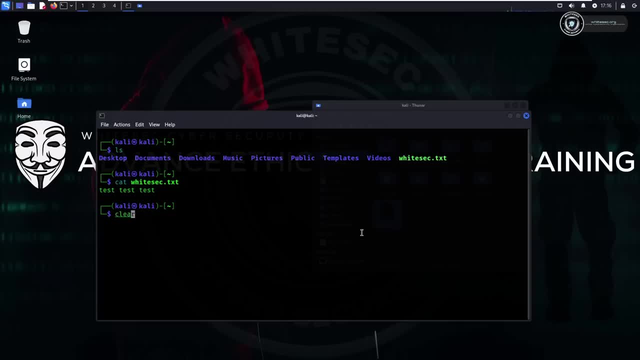 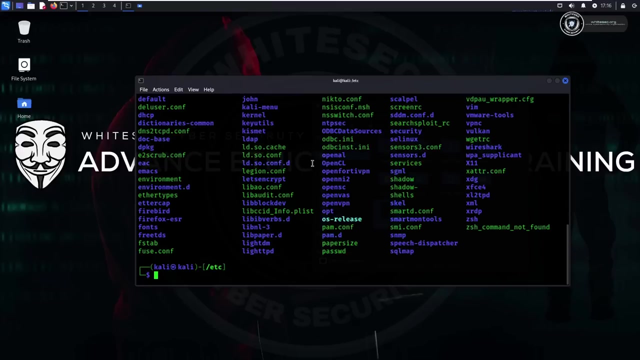 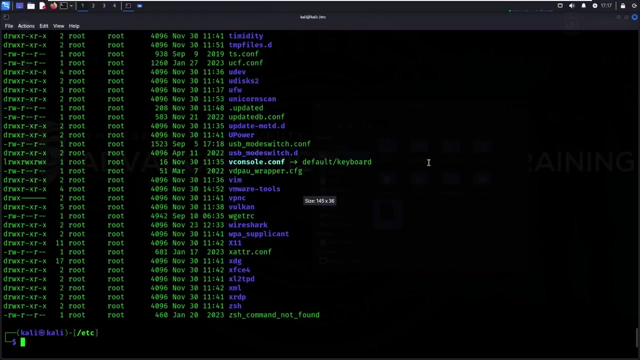 okay, right now, just let me clear it. now let's navigate to etc folder. just type here: cd, etc. sorry, just type something like that. okay, right now i'm in etc folder. if i type ls here, you can let me type something like ls, dash, al, okay, let me full size it right here. there are two important files which you need to focus. first is 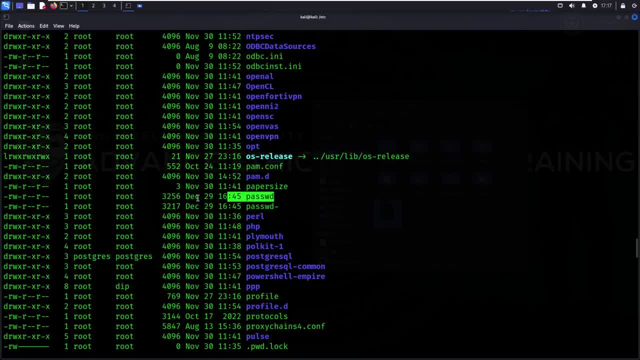 password file: okay, see here, just see the permission. it's a document file. okay, because we are seeing dash here. so that's why in the starting classes i told you about uh, these things, okay, in in documents, in these things you will see uh, dash in starting. okay, dash, we have the read write permission to root user. 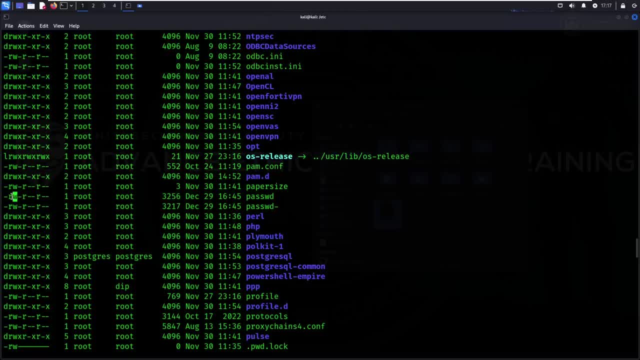 let me tell you it's only giving the rate and permission. read and write permission to root user: okay. and read permission to a root group: okay. and read permission to normal guys: okay, like us, okay, anyone who is in this system. he can able to read it. he can't able to modify it or he can't able to edit it or something. 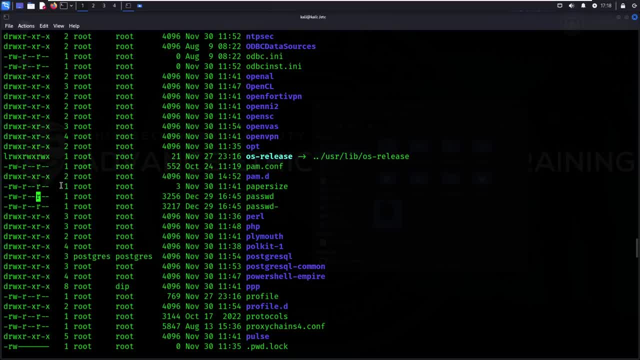 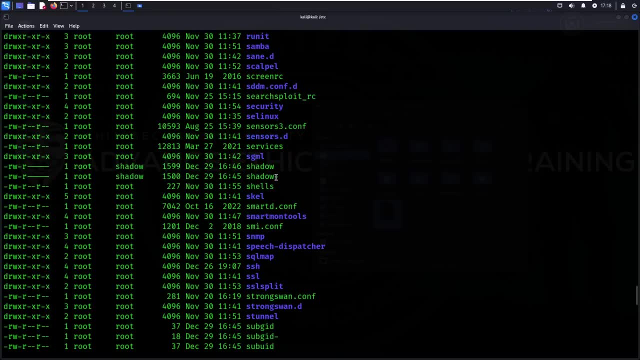 like that. okay, and this is the file right now. there is a one another file which, with the name of shadow, which is very important during pen testing. see, here there is a shadow file. now, by comparing to password and shadow file, can able to see a lot of restrictions here, see, simple, the root user only can able to read and 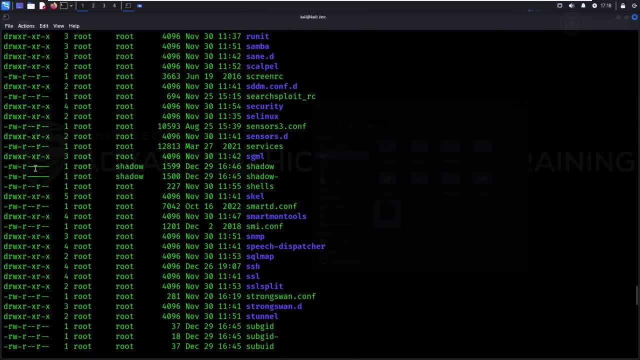 write this file? okay, and also the group. the group is there, which is shadow group. okay, this guy see, user is different here and the group is different. okay, group is shadow here. the group can able to read it. that's it okay. you can't able to modify it or execute it, or something like that simple. 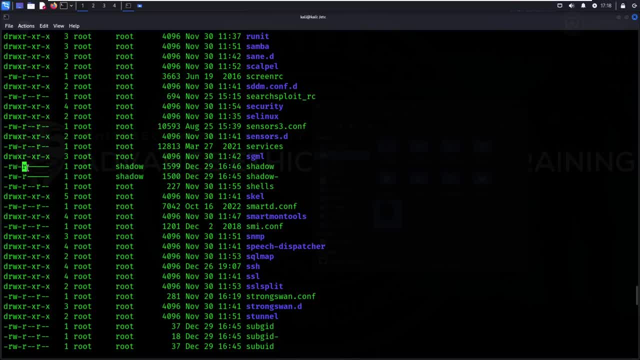 here you can only see the read and write permission. and the second thing i just told you, it's will- uh, it will- divide it in three parts. uh, three parts okay. first is one, first three is okay, just ignore the starting one. okay, if there is a d as well, you need to ignore the starting one. 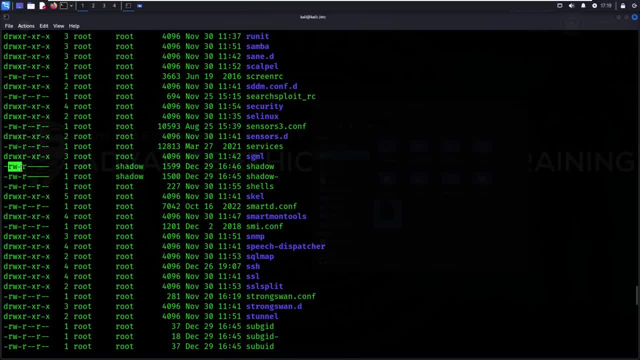 okay, just see, by comparing: from here to here, it's a three, and the second, from here to here, it's a three. uh, okay, it's a one part. this is the second part and this is a third one. okay, this is how it's going to be okay. so, the second one. okay, the third one. i'm just going to use the last one for. 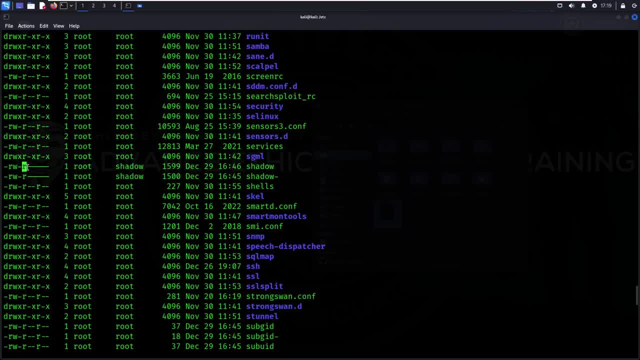 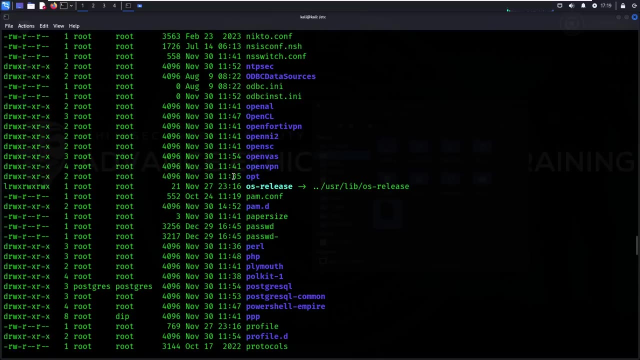 it's gonna work. first is for user, second is for sorry. first is for user, second is for group. okay, third is for the, the normal user who are in the system. okay, anyone right? so here the thing is. but comparing to password and shadow file, the things are very different here. the password file, 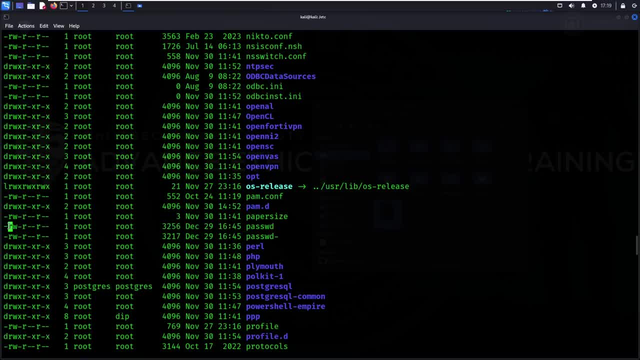 can able to see by anyone. okay, in the simple words there is a read: is there for three group, uh for three user, like uh for user for group for anyone they can able to read the password file. okay, even if you are not administrator there, simply you can able to read the password user. 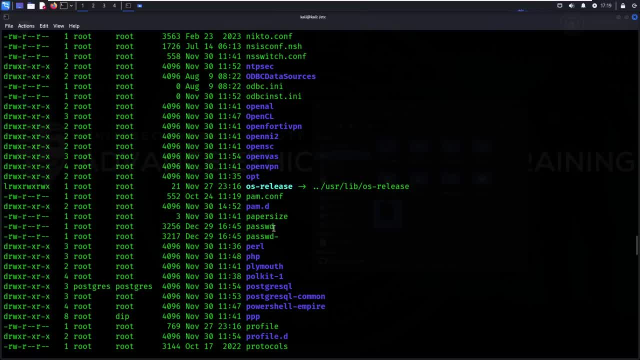 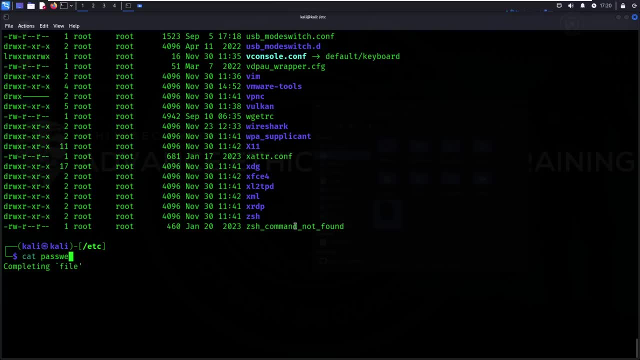 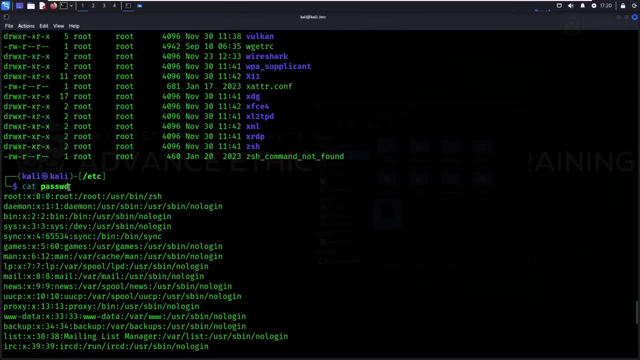 password file. sorry, see what is in this password file. simple i, if i want to open the password file, just type here: cat password. okay, all right, just type: enter there. it see, once i execute this cat password file, it doesn't ask me the any kind of password, just you need to enter the password to see this. 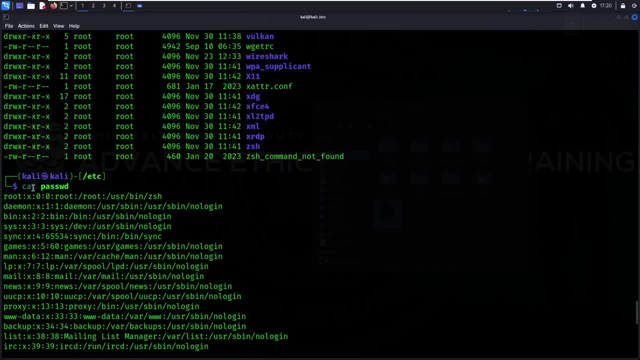 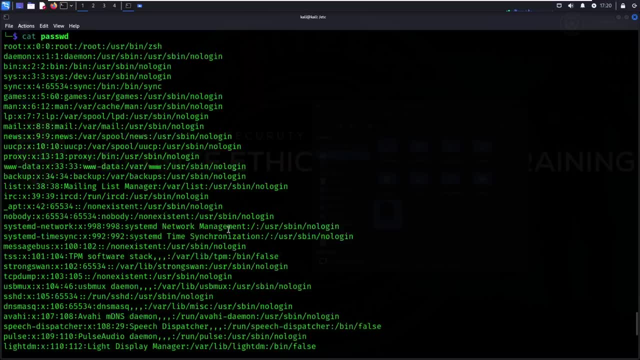 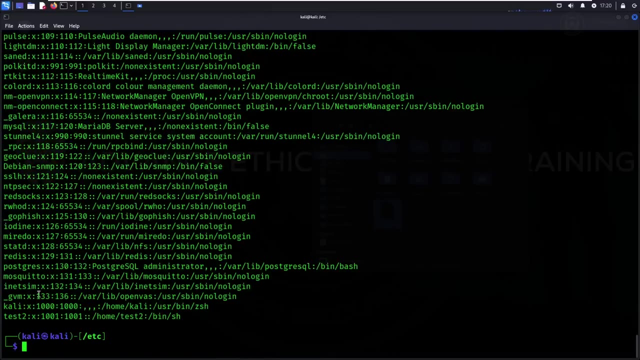 thing. it doesn't ask anything. simple, the uh, it successfully executed it. we all know that there is a kali user. he is a normal guy. okay, now just see, by using this password file, you, you guys, can able to figure out how many users are there. simple, see, there is a kali user, is there? 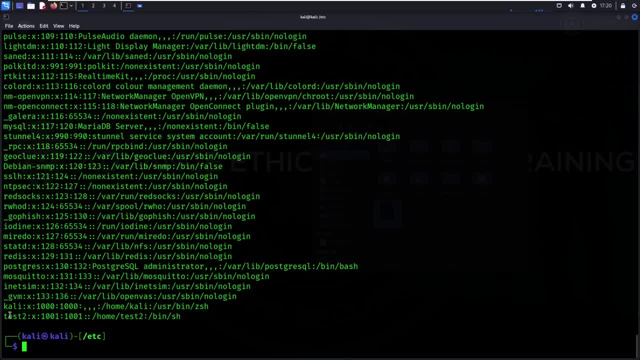 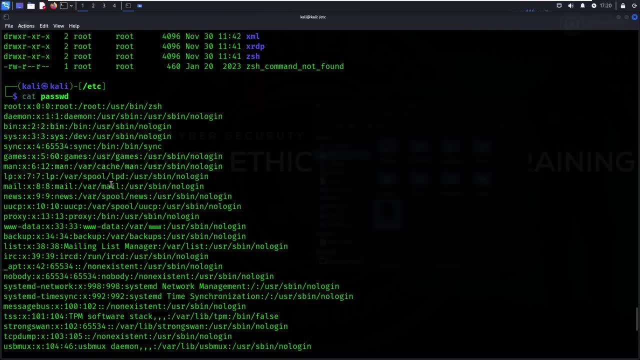 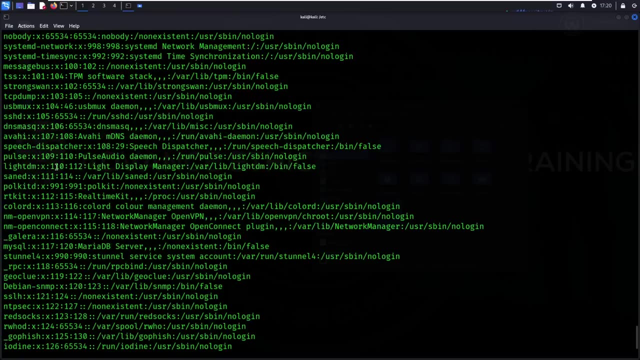 the test user which we test to user is there, which we just created. okay, these are the users which you can able to see. the main user is root here. okay, root is a user and you can also see the shadow user here. just wait, no, no, no, no, no shadow. you can't see the shadow here because shadow is a 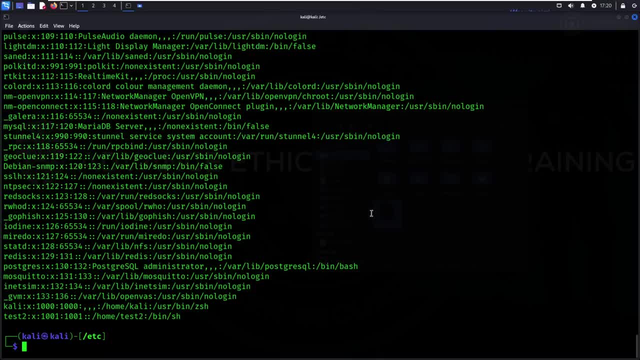 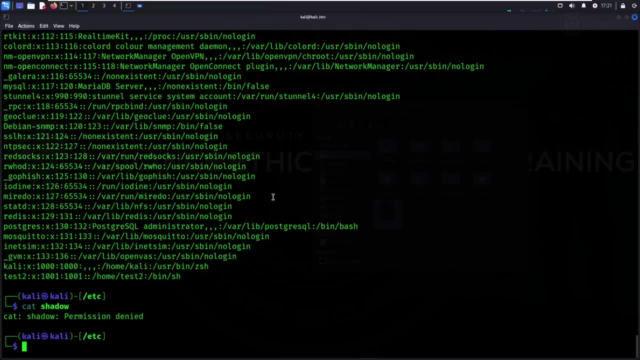 group. okay. now the thing is, if i want to open the shadow file, just simple. let me type here: cat shadow. okay, see, it's saying that permission denied. if i want to open this shadow file, then it won't execute, it won't open. okay, this is the thing. if i want to open it, then i must be a root user here. 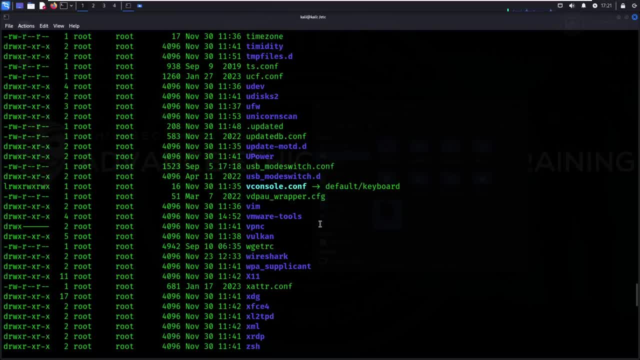 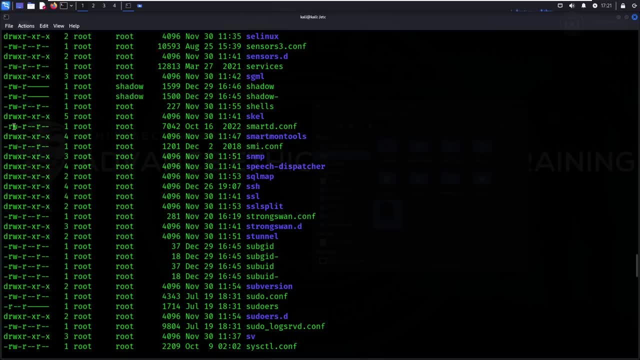 because the shadow files need a permissions. see, see, the shadow file needs a permission. only root user can able to read: right, okay, he can able to read it or he can able to modify it. this is the thing. the other users- the shadow group, okay- can able to only see it. okay, if you are a shadow, if you 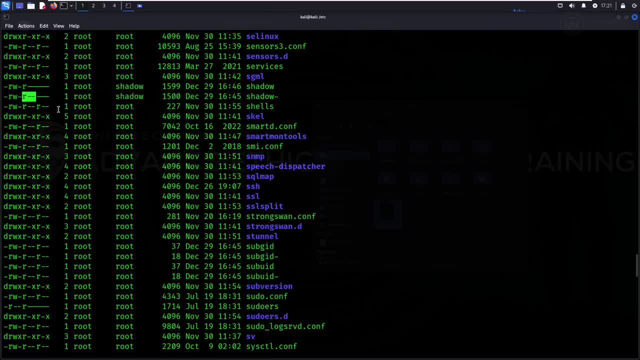 are user in is in shadow group, at that time you can able to read it. simple, you can able to see it. okay, assume that if you are a kali user, okay, right now i am a kali, right. that's why i can't able to see it, because the user- the other other users- won't have any kind of permission here. i. 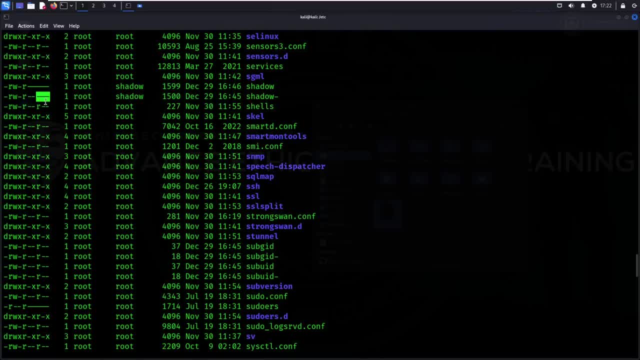 just told you dash. dash means nothing, but you won't have any kind of permissions here. okay, this is the thing. now, if i want to see this shadow file- sorry, here the same thing. okay, the permissions are same- if i want to see the shadow file, what i need to do? i need to execute as a 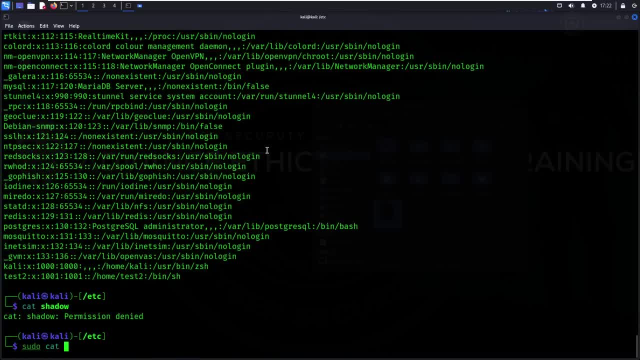 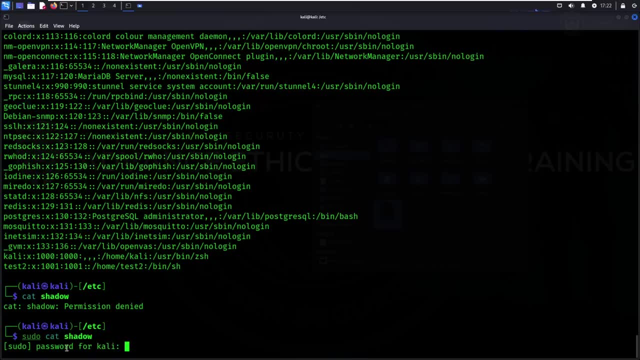 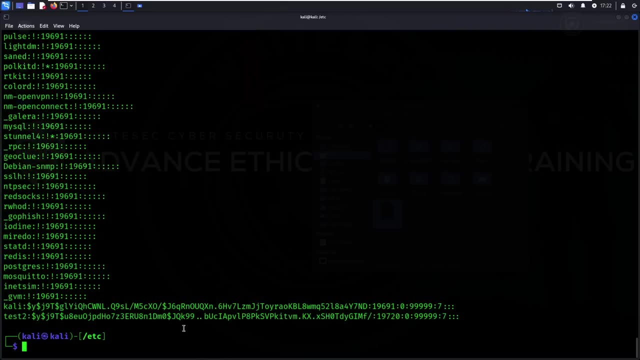 sudo. okay, sudo- cat shadow. if i type execute, then it will ask for the password. okay, see, it's asking for the password here. what you need to do means you need to type your password there. okay, at the time you can able to see the hashes here you can able to see the users and the hashes hash. 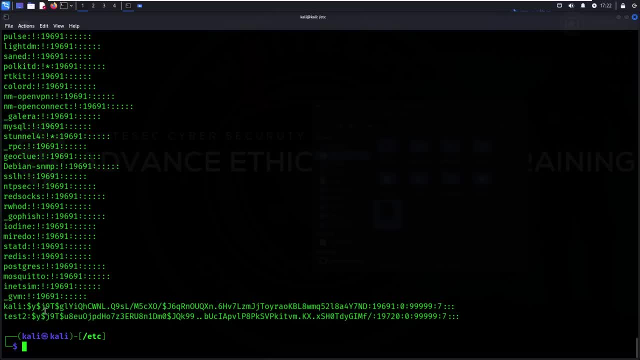 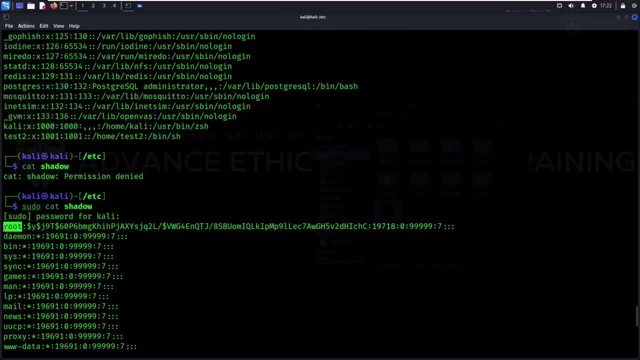 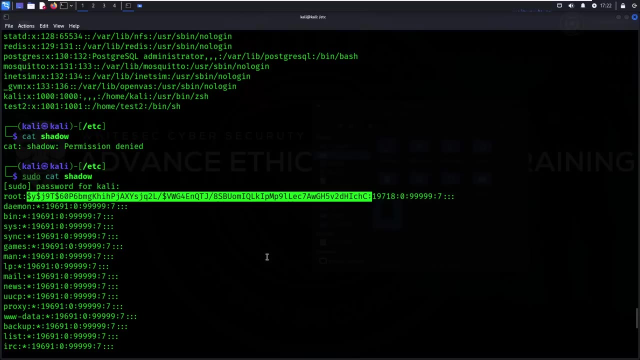 file right. this, uh, we can able to crack it by using the john the reaper which we just learn in a ethical hacking section. right here, there is a root user is there and this is a root password. okay, if you compromise these things, then that's it you. you own this machine. okay, that's it. 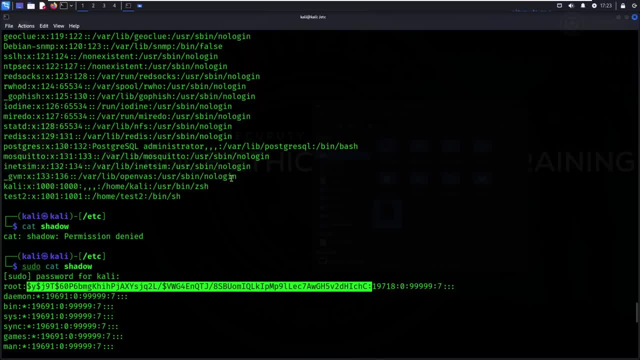 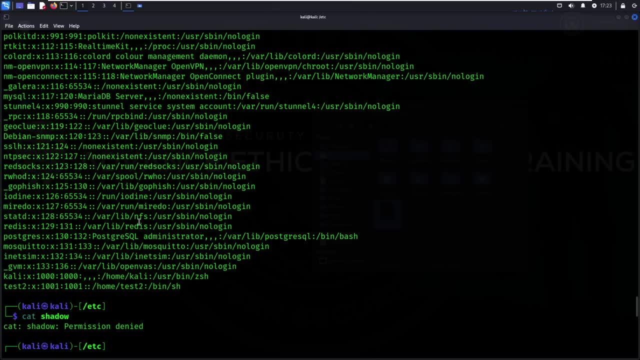 now, here the thing is in pentesting what we do. we just perform the privilege escalation, we check for the vulnerable decision. we just perform the privilege escalation, we check for the vulnerable decision if there any kind of vulnerabilities in the in this system, so we can able to uh, bypass this. 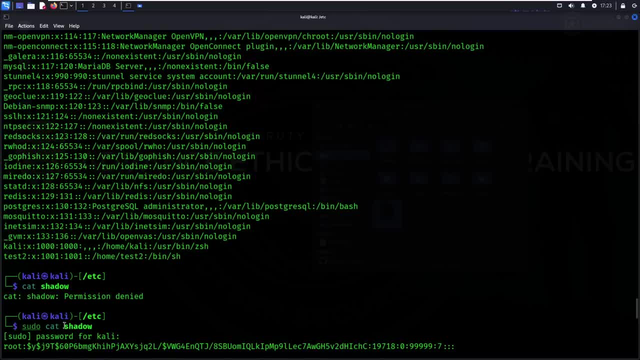 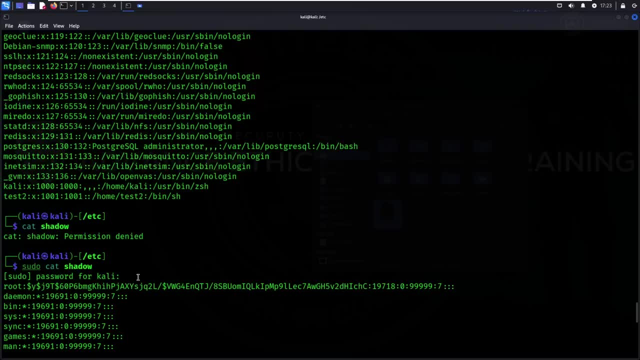 restrictions. okay, right now. if i want to access this shadow uh file, at that time i need to type the password, right? is there any way that i can able to avoid this password and i can able to read this file? so simple in pentesting. we check these things. okay, right. 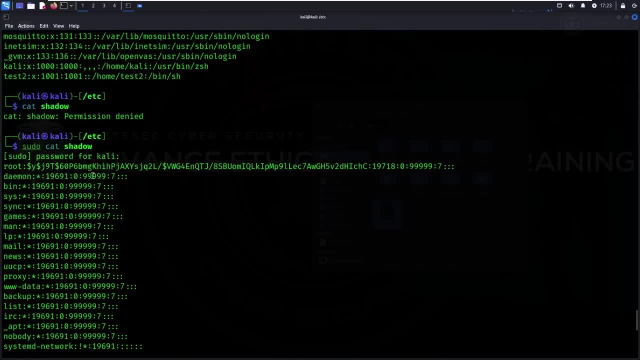 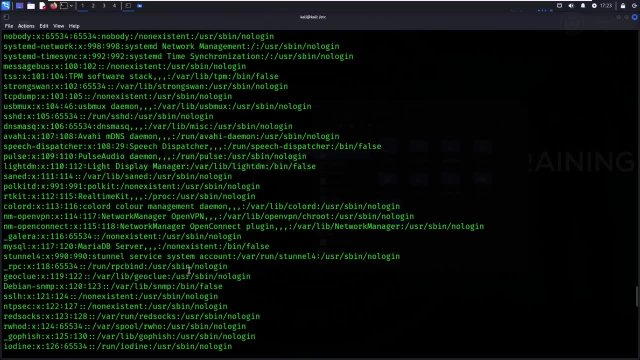 like: is there any kind of vulnerability to bypass this restrictions and we can able to read the password? it's this file or something like that. hope you guys get it. about the shadow file. it's all about the permissions. okay, there is nothing. there is no different. uh, difficulties. okay, it's a very easy. 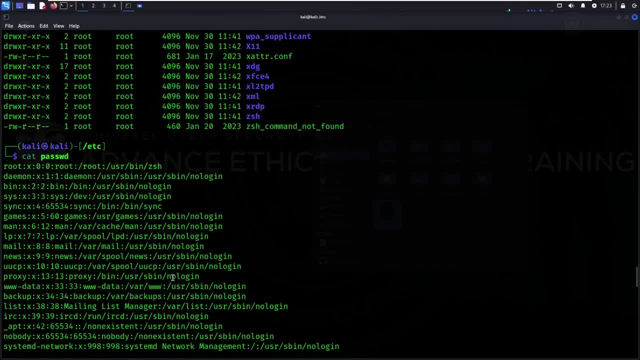 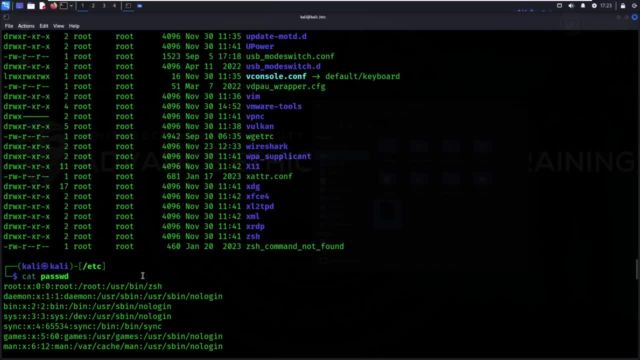 things again. i am saying: once you jump in, uh, practical stuffs, just try to practice it. okay, you will get each and everything. okay, there is a no rush. simple, just watch one by one. okay, it's not a big deal, right, simple, just don't focus on if you are not getting it, just first what you need to do. 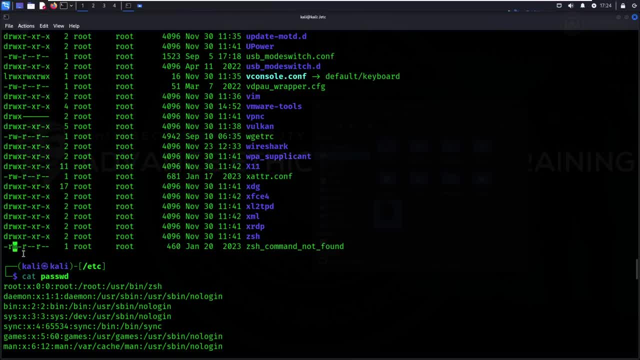 means you need to learn about the full application of pentesting. you need to learn about the full forms: what is r, what is w or something like that. then you need to uh give the. you need to differentiate in three things, okay, like, as i told you, group. the second one is user, that one. 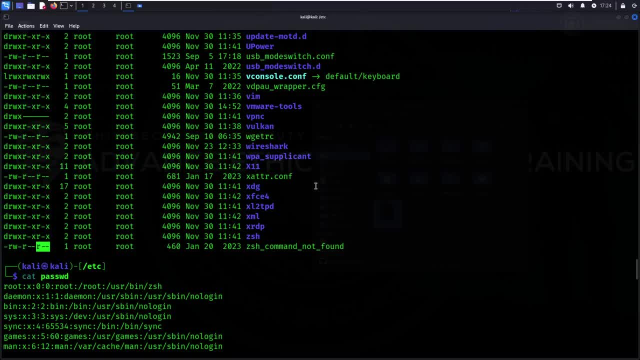 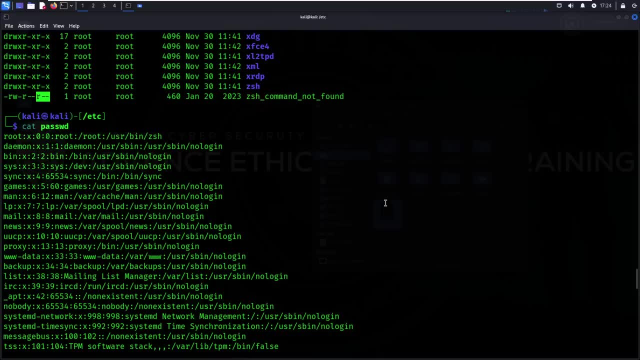 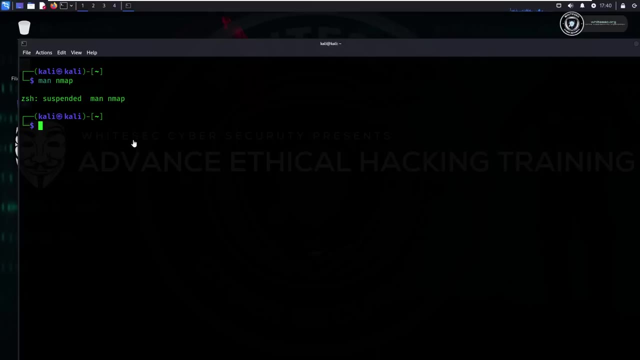 is other users which which are in this machine. okay, this is the thing for anyone here. if not the users, anyone. okay, this is the thing if any user, any group. okay, all right, hope you guys get it right. thank you, have a nice day. in this class we are learning. 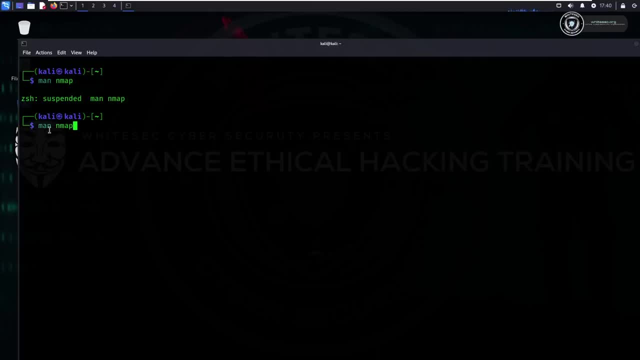 man. this is a one tool which is very useful for you guys. okay, because if you want to learn about any tool, assume that i want to learn about nmap. simple, just type man and just type the tool name, nmap. so simple, just enter, you guys can able to see the description, you can able to see the example. 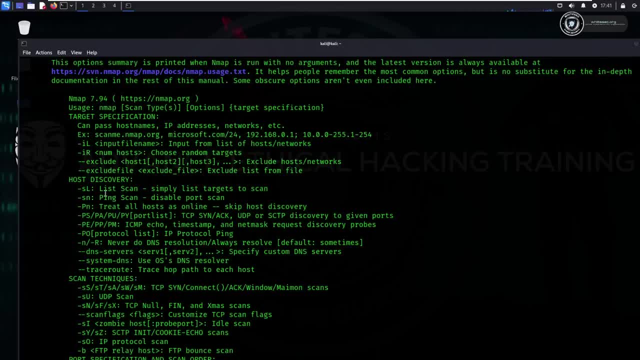 okay, you can able to see the options as well. you can see the details. okay, why the option is why we are using that option. assume that if i am using the sl, then what is this sl? okay, list scan. simple list target to scan. i need to provide the list there. okay, this is the thing. now there is a su. 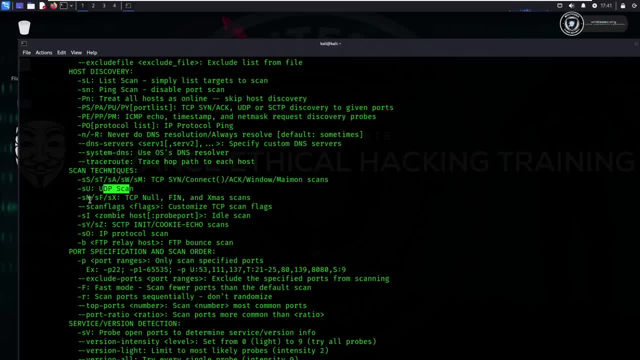 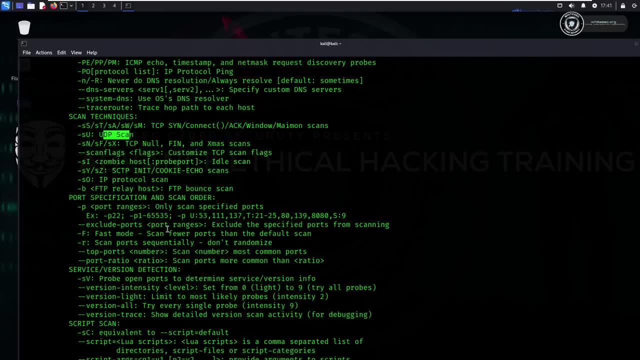 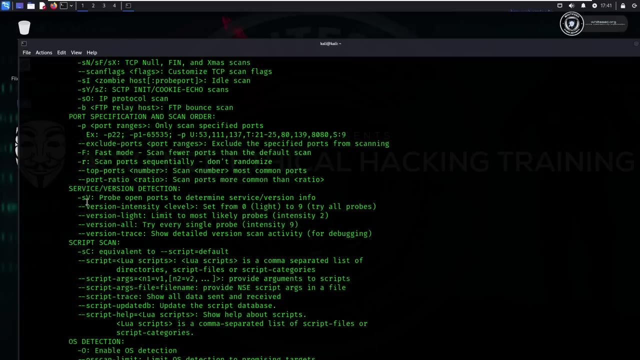 scan. su scan is for what? udb scan? sn is for what? tcp null fin xml scan. okay, so this is a thing. if you want to learn about the tools, simply you need to use a man there. okay, that's it. see, there is a sv. we just learn about sv in ethical hacking section and in the in the windows. 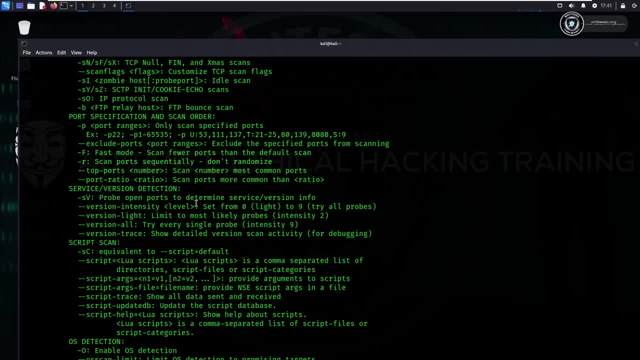 penetration testing training as well. okay, probe open ports to determine the list target to scan. i need to provide the list there. okay, this is the thing. now there is a su, the service and version info. if you want to know the port version info, at the time we use this one. 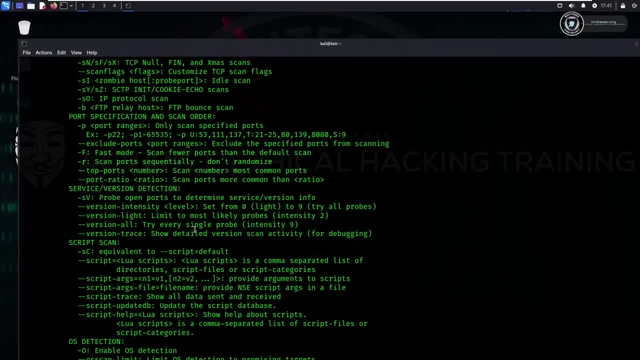 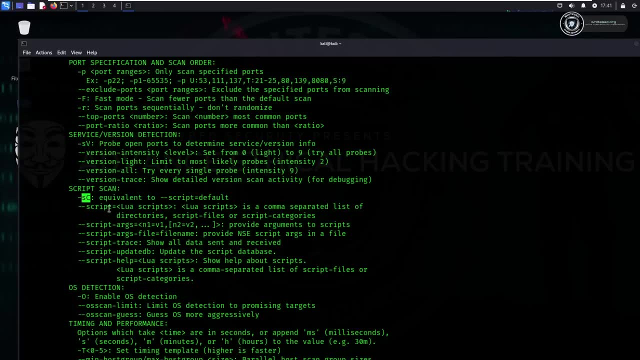 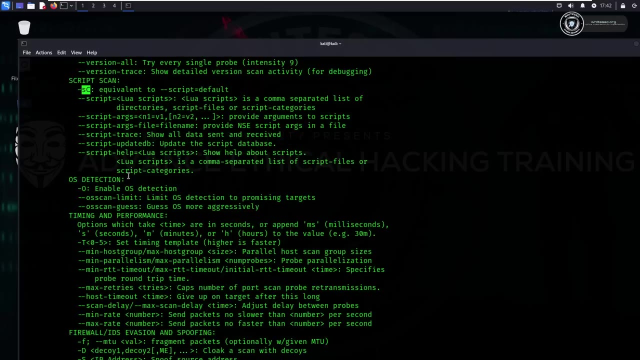 service version detection. see, right, if you want to perform the script scan, at the time we use this thing. okay, dash sc, right, you can also we, we also learn how we can able to provide perform the specific script scan as well. okay, if you are, don't worry, we will learn more. uh, we will learn. 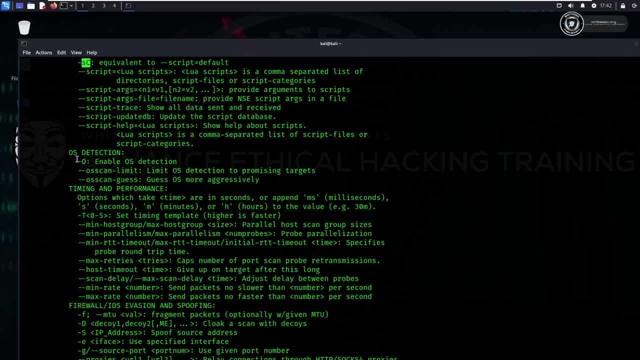 here as well, in this section, in this training right, there is a os detection scanning is here, see dash capital. o is for to perform the os uh detection scan. assume that i want to identify which operating system is my target using at the time. i'm gonna use this one. okay, this flag dash o. 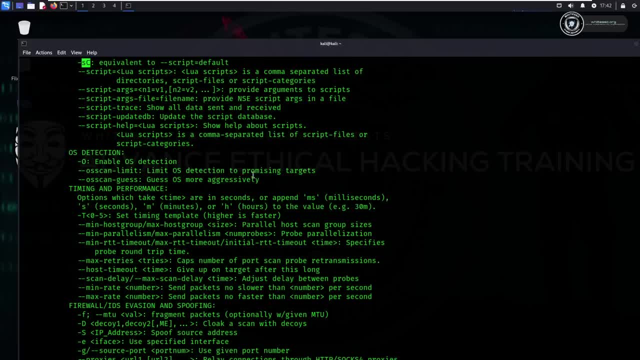 os. os can limit is a limit: os detection to promising target guess os more aggressively. if you perform this scan at that time, assume that sometimes what will happen means if you perform dash o, o there, you won't get the os details at that time. we use this thing, okay. so this is how you guys can. 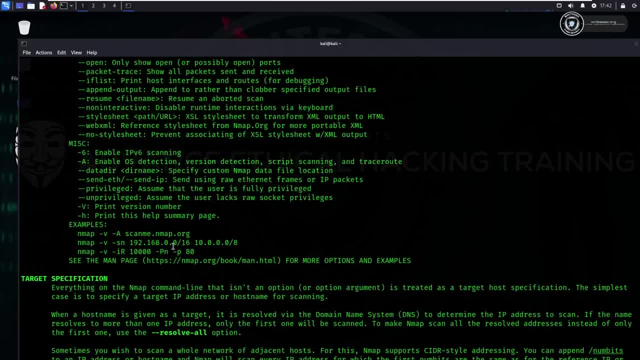 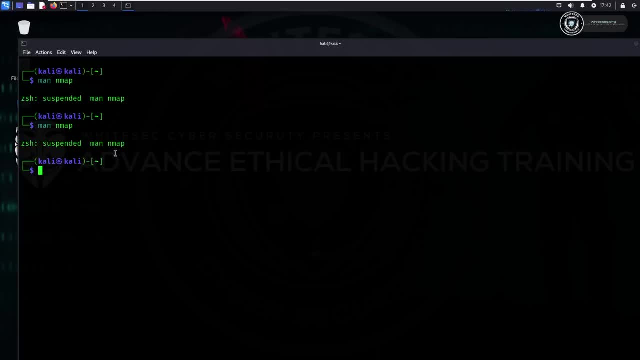 able to know about any tool by using man. if you want to close this simple, just type control plus z, that's it. you can able to suspend it and you can able to close it. this is how you can able to use the man. if i, let me type man, let me search for, uh, let me use a nectar. this is going to beían. 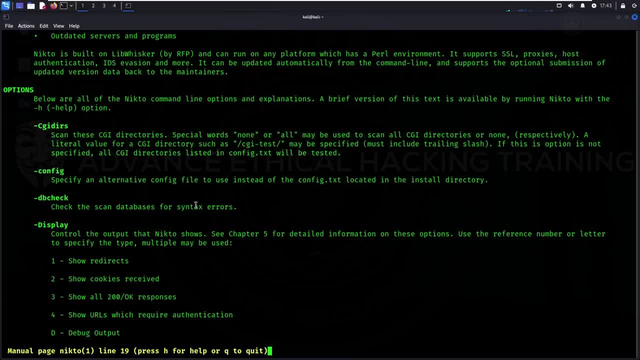 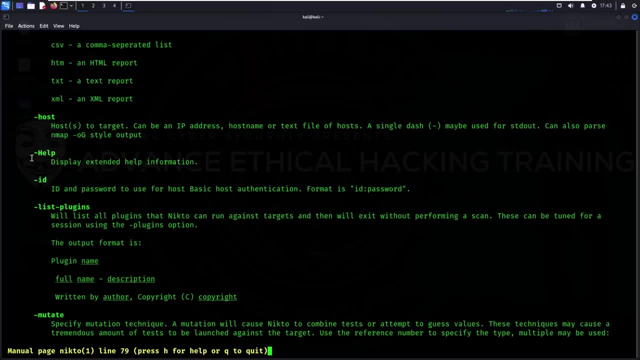 ué yí se b, also same like nmap. so this is how you can able to learn about necto. okay, there is a dash efficient flag. okay, format: host, a help id. this is how. okay, this is excellent, right, if you want to learn about. 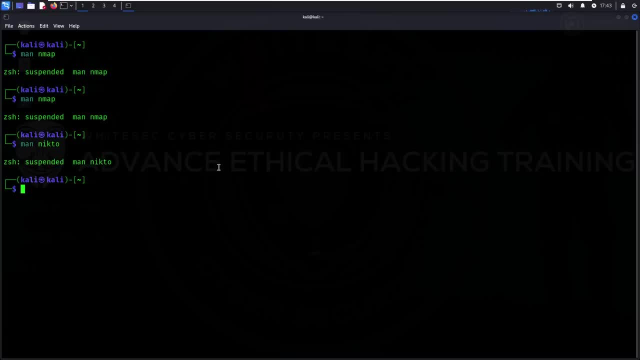 any tool. simple, just execute, type man there and you can able to see the options. you can able to see the description, each and everything. right, hope you guys enjoy this class in the next classes. we are learning about like a basic thing. mostly you guys know how to install the uh scripts in. 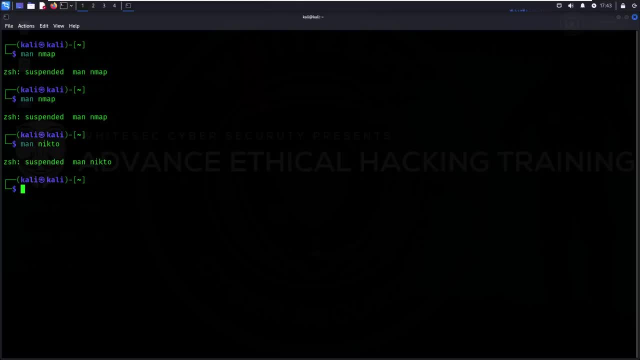 linux simple. let's learn that one as well. okay, right, thank you, have a nice day. in this class, we are learning about how we can able to install the packages, or how we can able to update, upgrade. okay, the simple thing for, after starting the linux machine, what you need to do, or after. 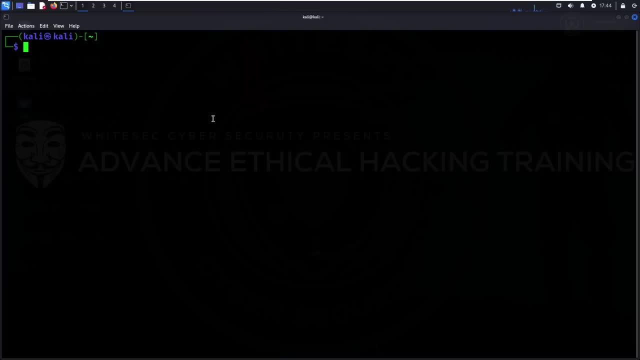 installing any kind of tool. okay, what you need to do simple: just type apt dash, get update. just update it. okay, see, you can't able to execute. you can't execute this command by using kali user. at that time you need to change it to root. just type sudo. okay, now what i am doing. 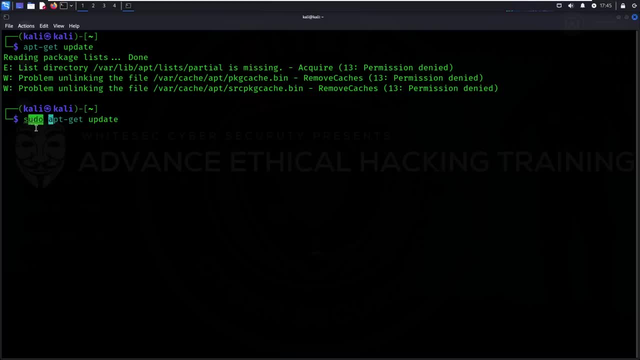 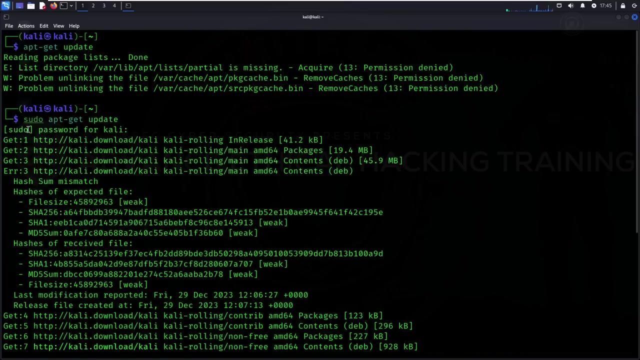 means i am executing this command as a root user. that's it. just type enter. now it will update the packages here. okay, see, uh, assume that you are installing any kind of scripts. it will throw some errors here before installing any scripts. what you need to do just execute this command. okay, sudo, apt, get update and then install. 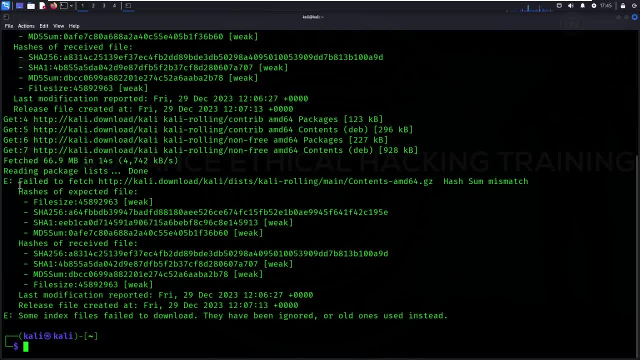 the scripts here or any kind of tool. now i got any uh error. mostly this error is due to the network. okay, assume that you, if your ip has been banned, at that time you will see the error, this kind of fail to fetch or something like that. so at that time, what you need to do if you have a 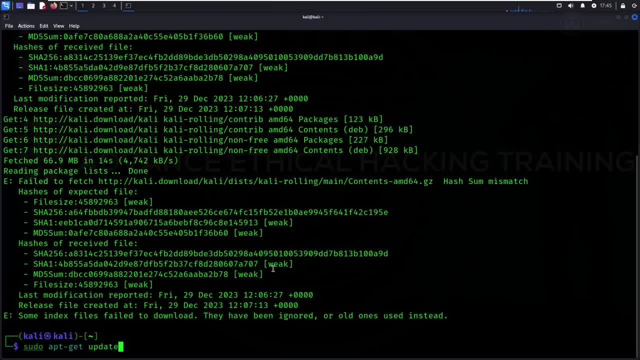 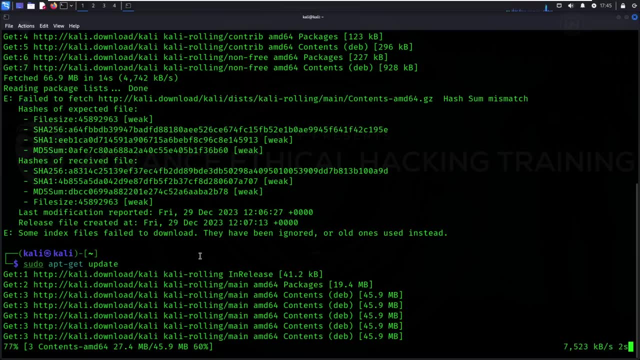 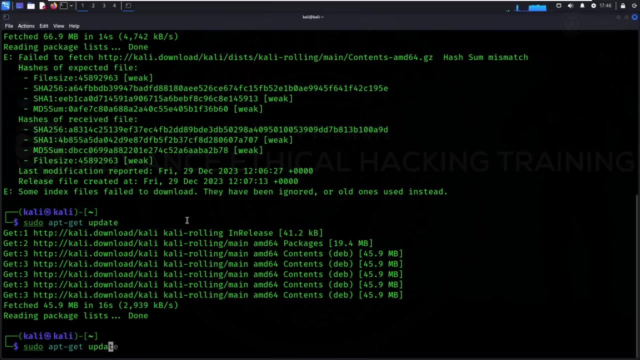 vpn, then connect, and then you will get the error. okay, so you need to do: if you have a vpn, then connect. if you don't have the vpn, simple execute the command again. okay, see, simple, it's done. now there is a one another command. most assume that in your linux machine you are seeing a huge amount of errors. other time we use 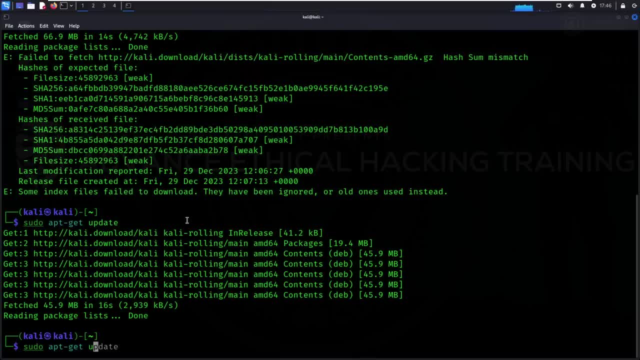 this one: apt get upgrade. mostly i use this to avoid the errors: okay once. if i see any kind of errors during the execution of any command. if i see any kind of error at that time i use this one: okay, apt get upgrade. see once you install linux newly. at that time, what you need to do means: 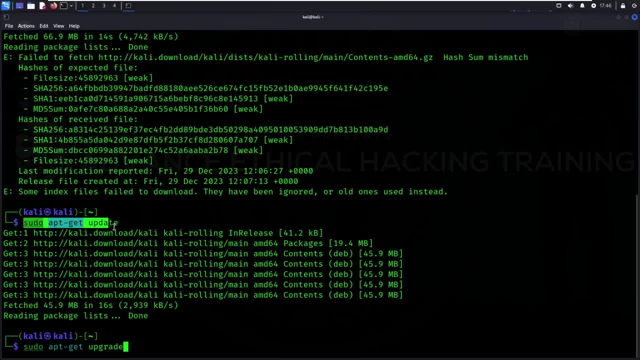 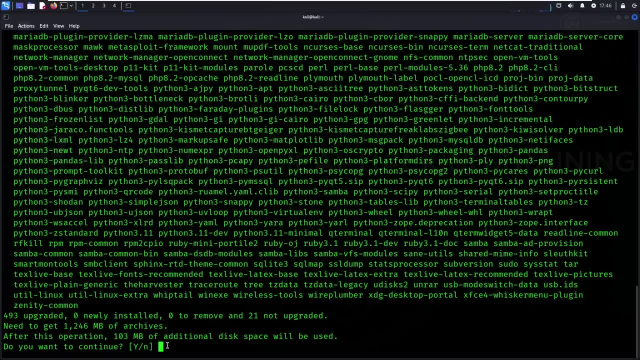 just execute this two commands: okay, apt- get update. then, after doing update, just type apt- get upgrade. okay, it will take a huge time to upgrade. okay, it's a very long process. it will take a huge time. so simple. what you need to do means just type y there and that's it. it will 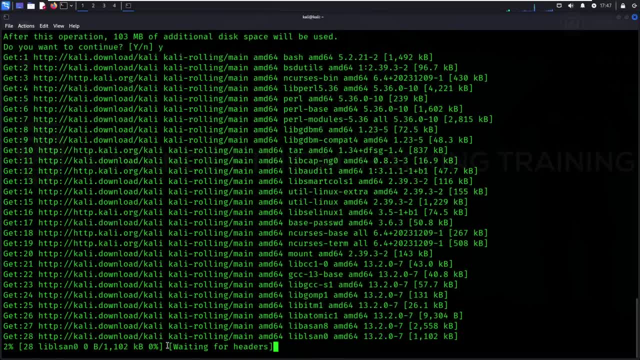 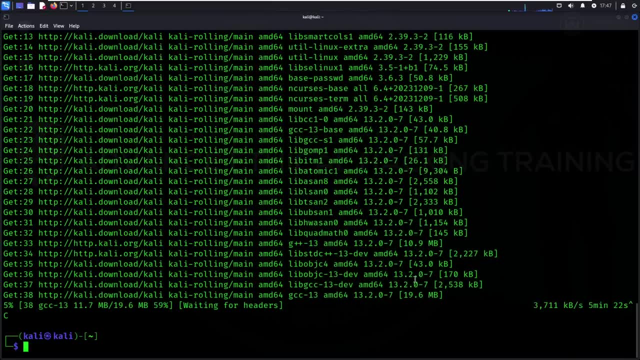 start to update it. it will. i think it will take a huge time. it will. in my case, it it will be five minutes, okay, but i, i i'm gonna stop it. okay, this is a thing, but you need to continue or just continue it, just wait for it. okay, this is the thing. 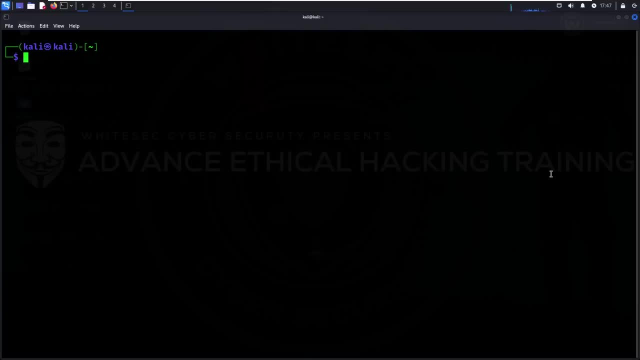 and the second thing is: assume that i want to download any kind of repositories. at that time, what i need to do means see simple, there is two ways to download. okay, from github. also, assume that there is a host. apd is a one tool. okay, there is a one tool. 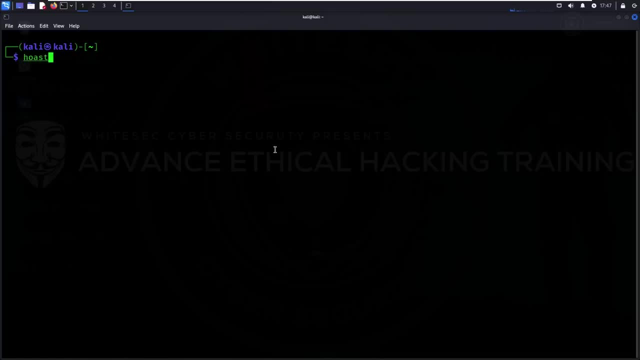 in linux with the name of host apd. basically, this tool is useful to create the hearts hotspot. okay, basically, in my machine, in my linux machine, host apd is not there. okay, after executing host apd i can't able to see automatically. linux will say that in your 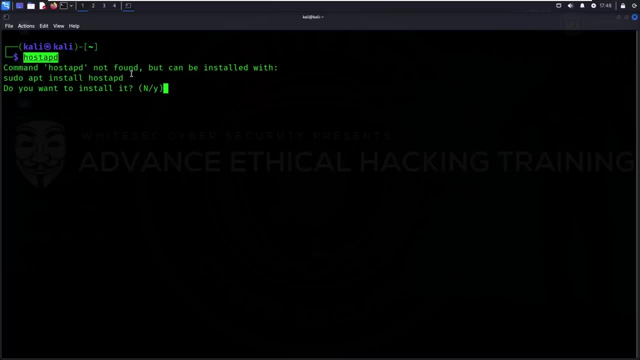 system, the host apd is not there. if you want to install that host apd, you can use this command: sudo apt- install host apd simple. do you want to install it? no need to execute this command. simple by just typing y there, it will automatically install the tool for you, okay. so that's why i 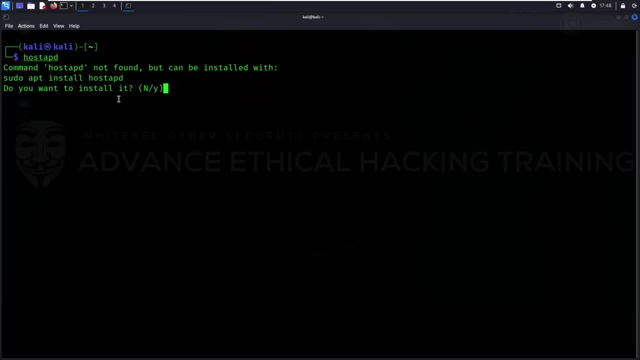 just said in the first classes, right now linux is very easy to use. okay, previously it it is very it difficult. okay, this is the thing. like to fix the issues, to fix the errors, it will take a huge time. right now the things are like a butter. okay, this is the thing. now, this is how you guys it will. 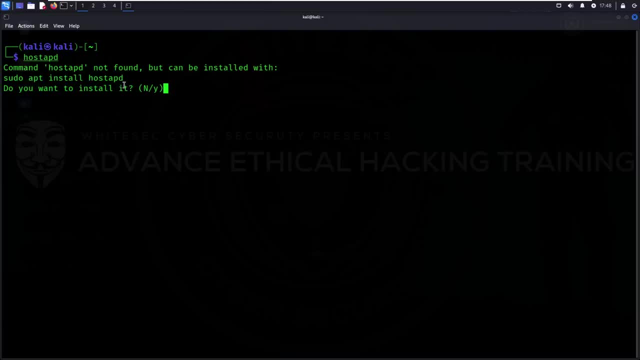 automatically install it for you. if there is any kind of packages or uh, it's missing. assume that you just executed uh, you just any uh. type any command, at that time it will automatically detect it and install it. if you type y there, then it will install it for you. okay, this is the thing. 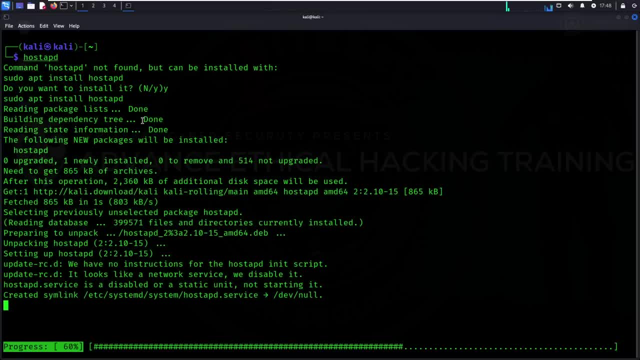 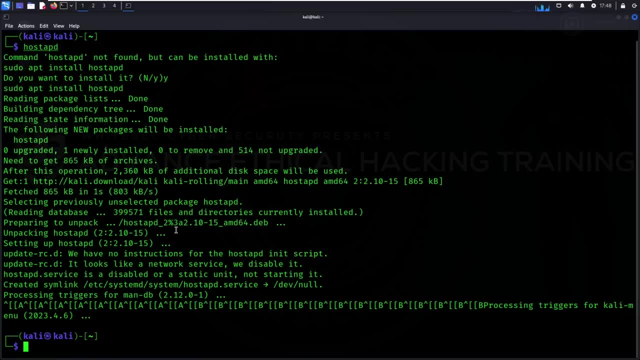 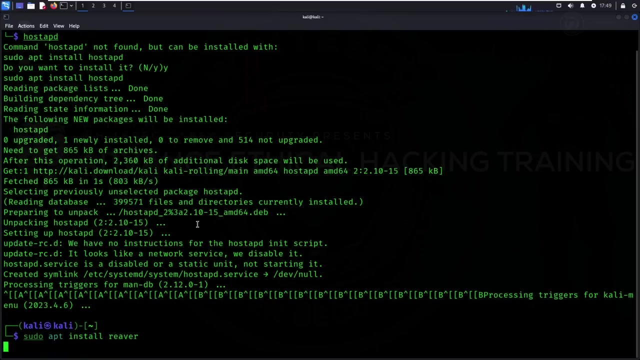 so it's successfully installed this way, right? so if you want to install any other packages, simple, just see sudo. just execute this command: sudo- apt- install and the package name. assume that if you want to install reaver, simple just type: uh, sudo, apt, install reaver. reaver is a tool which is useful for wi-fi hacking purpose. okay. 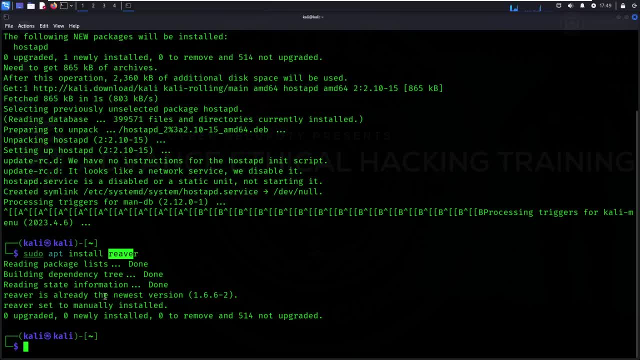 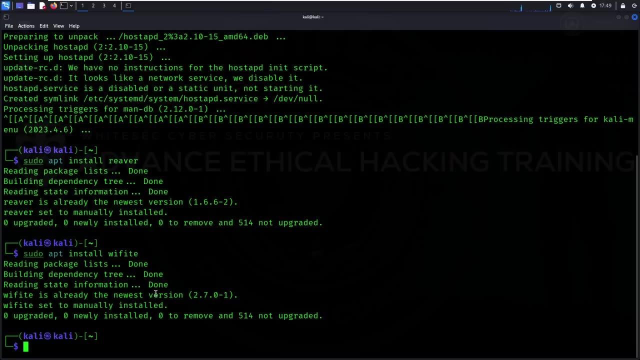 see, reaver is already there. okay, reaver is already. the newest version is available in this linux machine. okay, so that's why it's not installing it. okay, assume that if i want to install the wi-fi te, just type wi-fi te, just simple insert by default. wi-fi te is there in my linux machine, so this is. 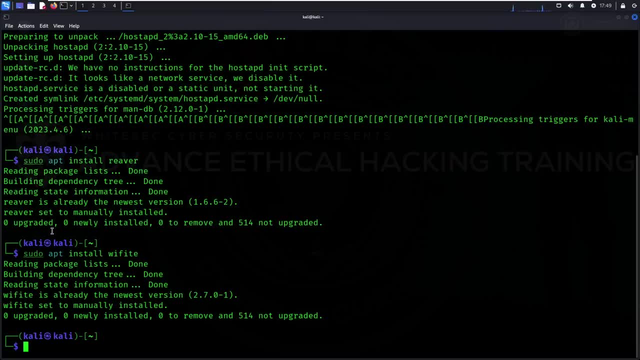 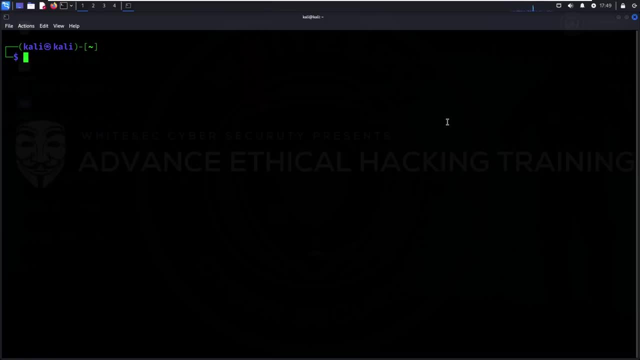 the thing: okay, this is the one way to install the tools. but, uh, if you want to install those tools, okay, like there are some other tools by using same slash, ok, but this was one way to install the tools by using by executing this kind of commands, you can't able to download it. you need to download the. 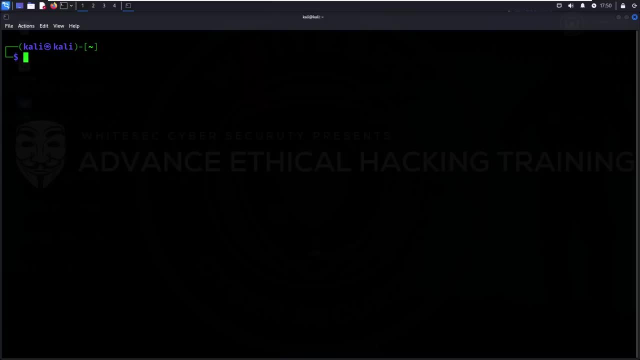 just let me show you first. just just let me show you one example. see, there is a one tool with the name of zfisher. zfisher is a tool. by using the tool, you guys can able to perform phishing attacks. okay, see, if i type here: sudo apt install, okay, zfisher, hope it will it? it won't work, okay, see. 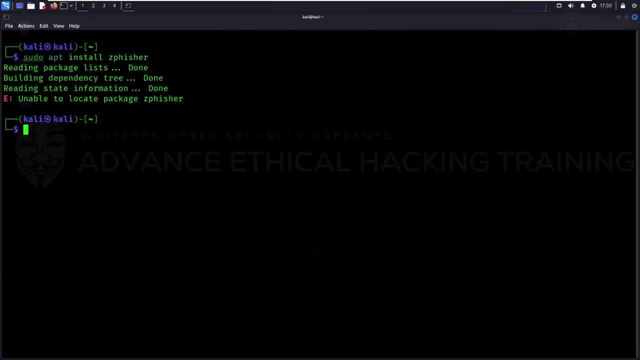 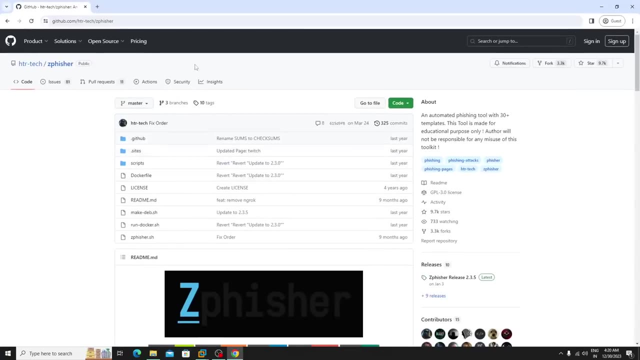 it won't work at that time. what we need to do means we need to use git clone. okay, simple, just visit the github url, like zfisher. first of all, you need to search for the tool uh on google. you will see the github url there. okay, but starting, only you guys can able to see the github url just. 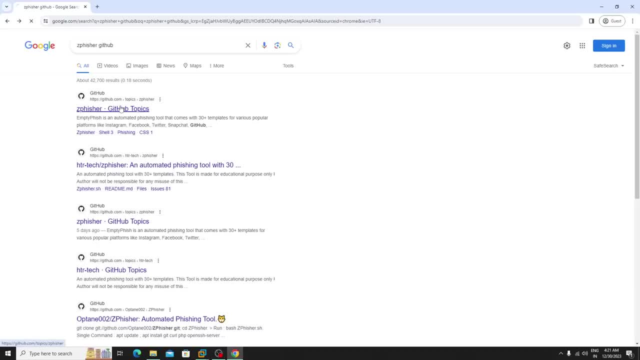 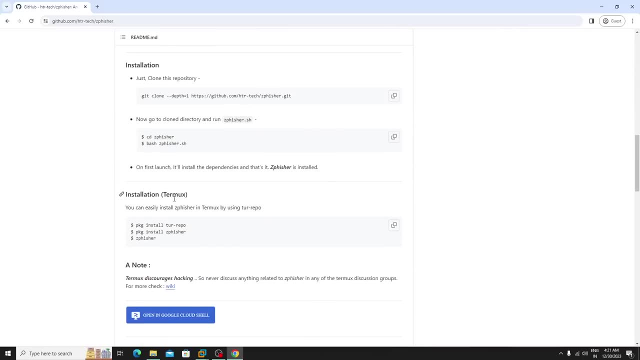 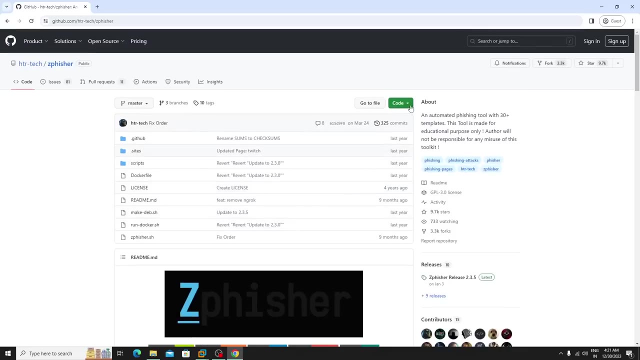 let me show you. see, i just type zfisher here. there is a link. all right, select this one. now how to install this tool? simple, there are installation methods, are there? okay, installation process: just copy this repository. or you guys can also do it from here. just copy this url. okay, just type git clone here. 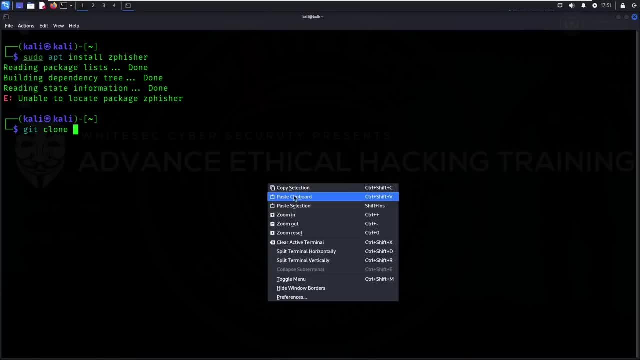 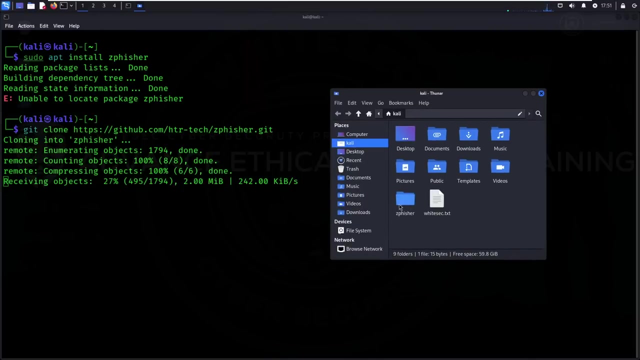 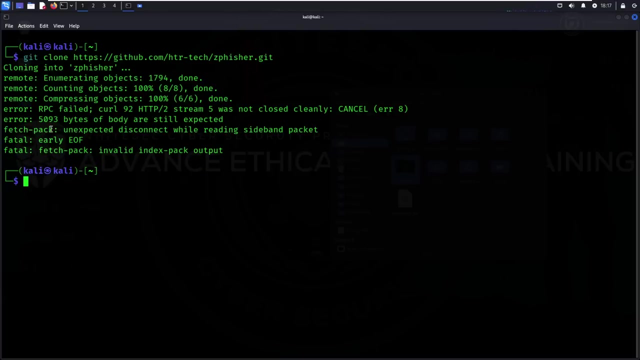 basically, i am downloading this file to my system, okay, by using git clone. see what will happen if i open the file manager. you won't see any kind of zfisher here. right now it's downloading. okay, see, it's downloading in my linux machine. basically, this issue is, uh, due to the internet, okay, or due to your ip has been banned, or? 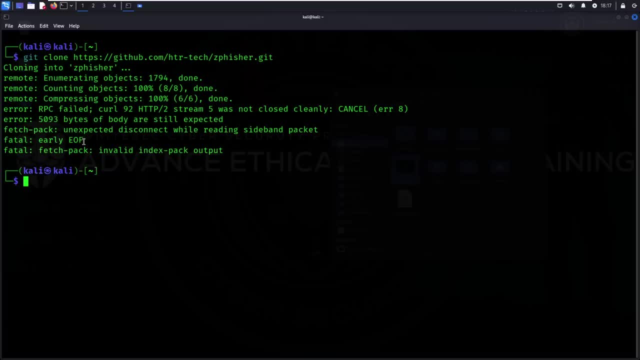 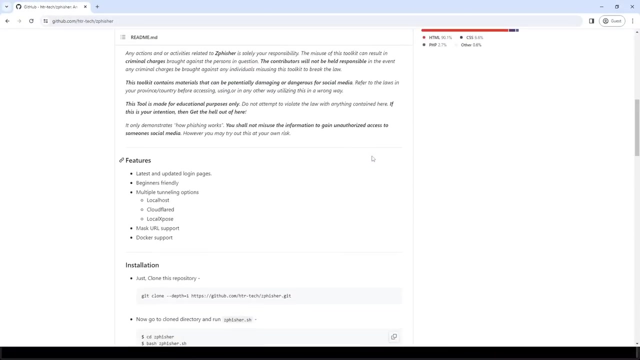 something like that. okay at that time. so that's why i just told you to do, uh, to use vpn. okay, maybe it's a rpc field. uh, okay, it's rpc. but at the time what you need to do means see here only there is a one command. let me use this one: depth is equal one. 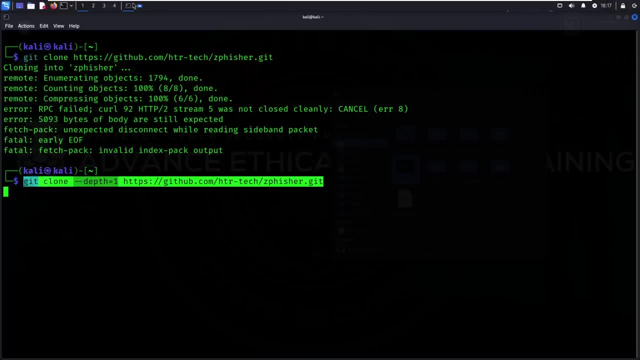 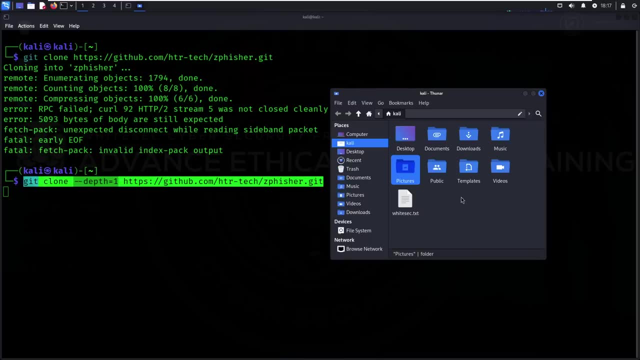 see the folder has been automatically deleted. okay, once the process has been stopped, the folder will get deleted. okay, now let me type enter. just see, the folder has been created. now we will see the thing you need to do. if it consists of something like this, and lets us type it: zfisher. 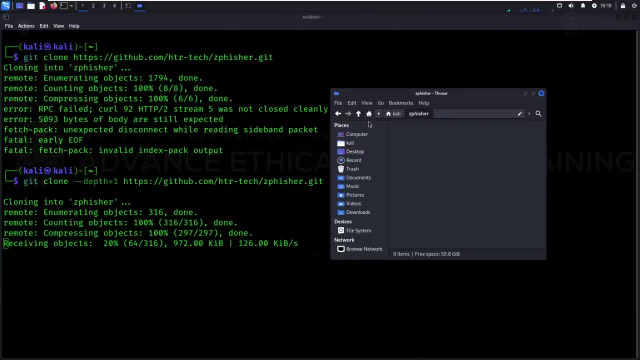 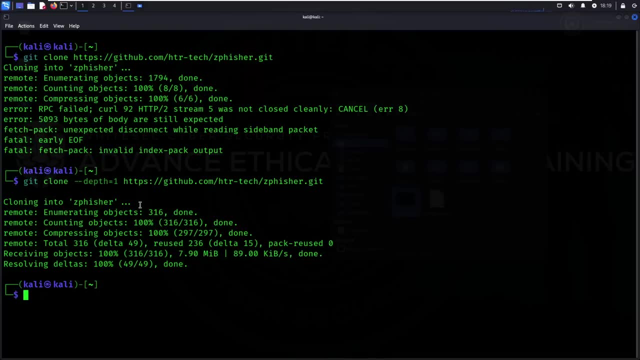 let's write it: zfisher. let's pass this, it justけど. okay. now see, we successfully downloaded it. okay, the folder is here now. the simple thing is: we simply just downloaded it, okay, we didn't install this, uh, zfisher or something like that. okay, again, i am saying: we simply downloaded the zfisher in our system. if i want to install this, what i need to do- there are the steps. 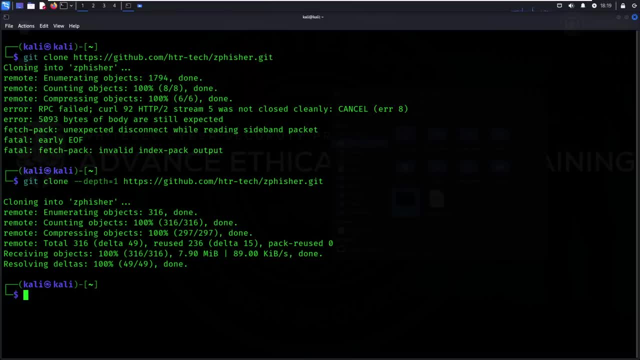 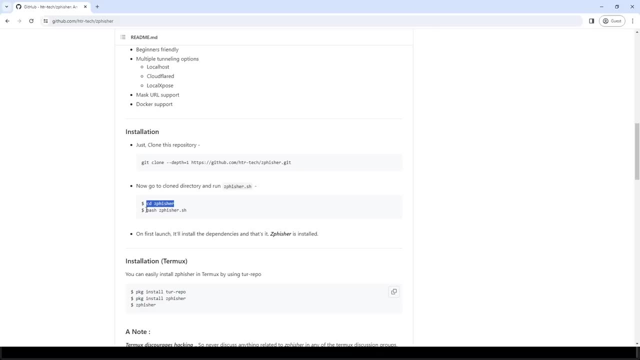 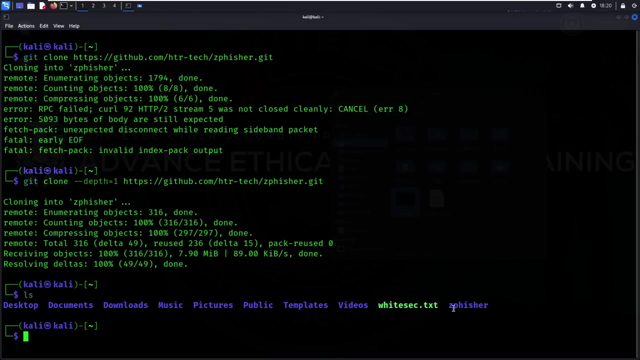 catching up with the tests. steps to install it: okay, cd zfisher and there is a bash zfisher dot sh. now the thing is now go to the clone directory and run this file. simple how to go to the clone directory. if i type ls, there is a zfisher. okay, if i want to go to the directory, what i need to? 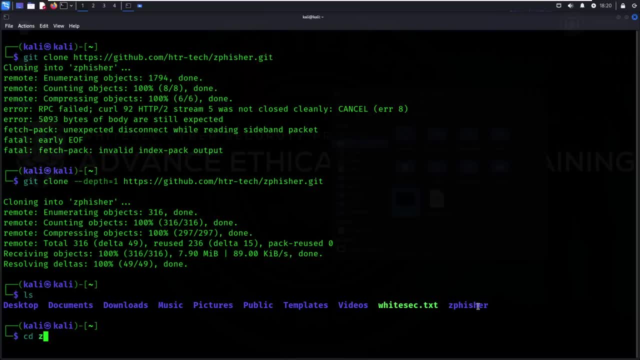 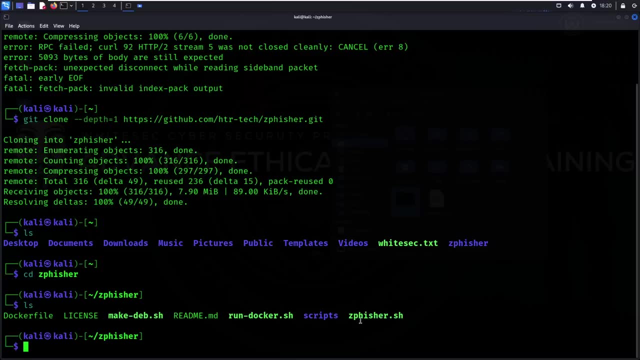 do is just type cd the directory name zfisher. now just type ls. here you guys can able to see zfisher dot sh. see here. dot sh is there right? basically it will run through bash. okay, like here also you guys can able to see. if you want to install this, then you need to. 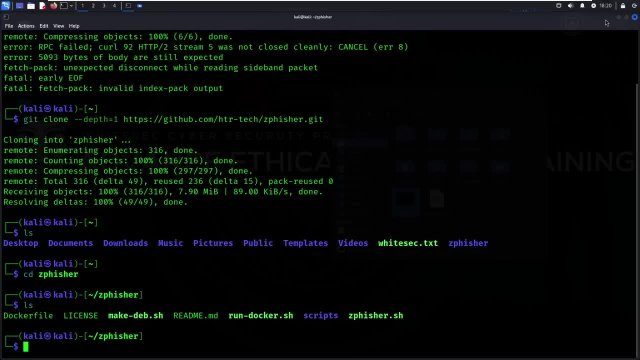 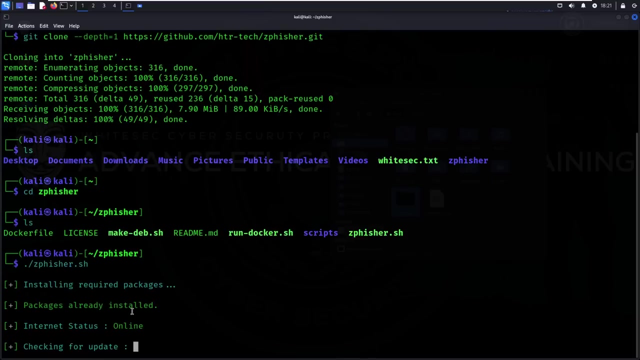 run bash space zfisher, dot sh. okay, assume that there is a dot py. at that time you need to use python, something like that: python, zfisher, dot py, something like that. okay, now, instead of bash, you can also type dot forward slash and just type zfisher. just type enter. it will install this. right, i am gonna install that. 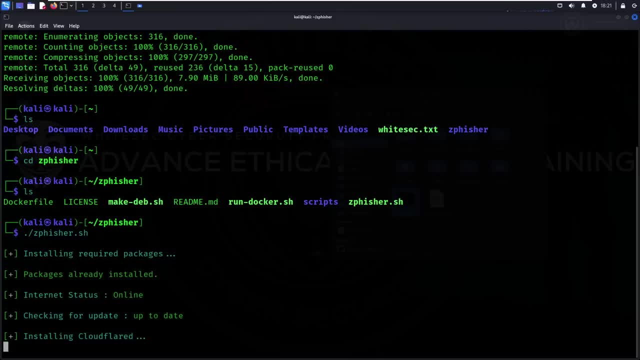 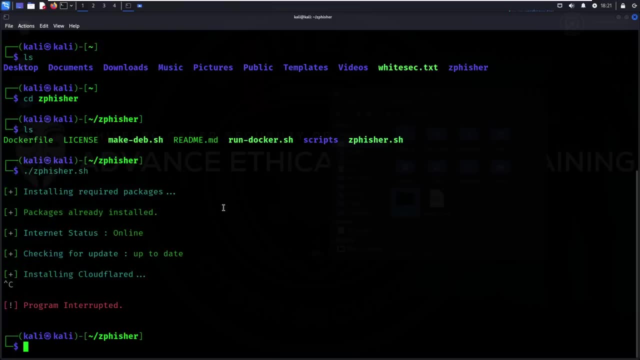 zfisher here, so this is how you can able to install the tools from github. right, let me stop it. i don't want to install the zfisher. hope you guys get it. in the next classes we will learn about networking. hello guys, hope you are fine in this classes and i will see. 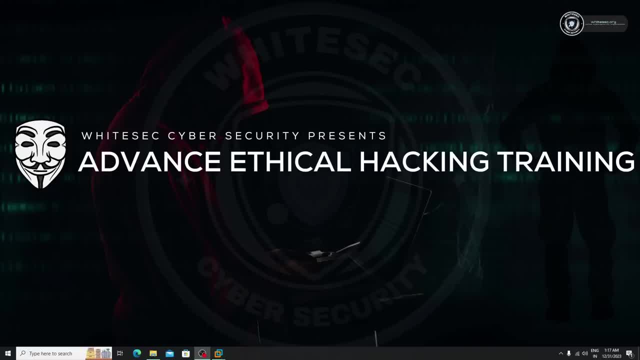 you in the next class. bye, bye. we are learning about networking. okay, it's a very basic training. this is a very basic section which is necessary for you. if you don't know about networking, okay, then just watch this section. if you know about these things which i am covering here, then you can able to skip it. okay, it's not. 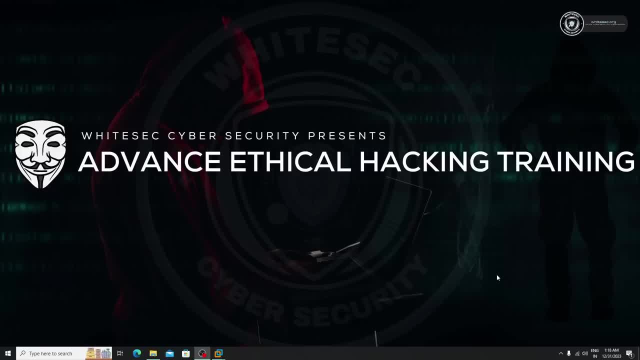 a big deal. and also, again i am saying: this section is enough for you guys. okay, to come, if you want, if you want to implement these things, these attacks in real world, at that time this things are enough for you. this, this section is enough for you see, networking is a very wide 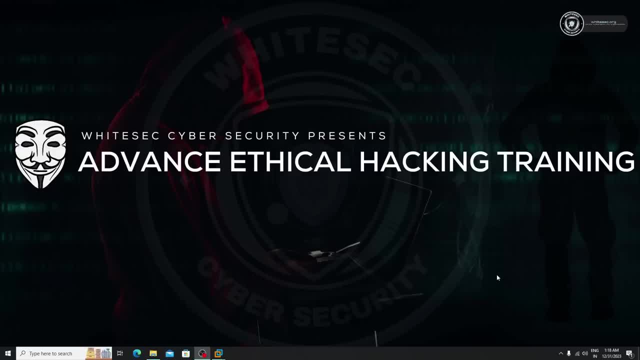 okay, like it's a very huge thing. okay, we can't learn each and everything about networking because we are not a network engineers. all right, we are a pentesters. but we need, we must need- a knowledge about networking, how the things are working. simple, you need to learn that much only, which is necessary. 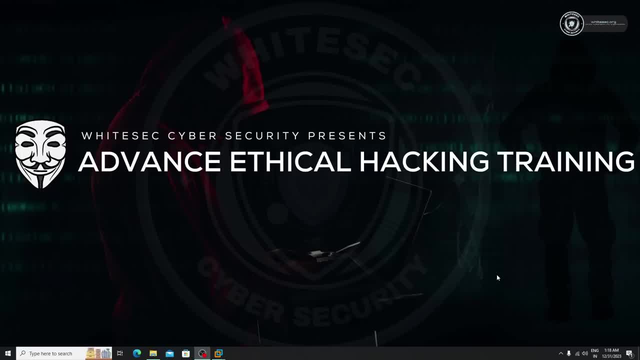 for you in this training. we need this much only so. that's why we are learning this much only. okay, this is the thing. assume that you got some big project at that time. do your own research. okay. google is your friend. okay simple if you type the things. 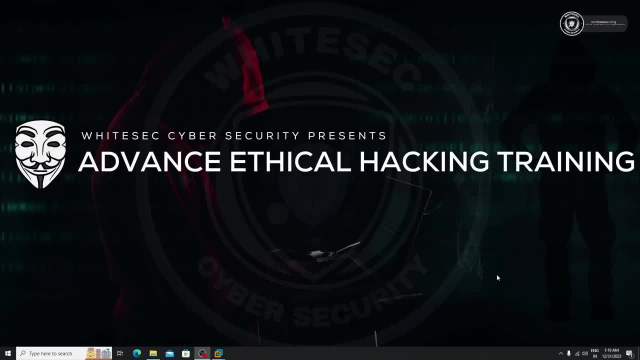 then you will see the results here. and also the second thing is there is a chat gpt. it's excellent. everyone is using that one, okay, even the programmer, even the pentest cyber security professional. everyone is using this thing. okay, just use it. it's not a big deal if you, if you type in your own, uh, 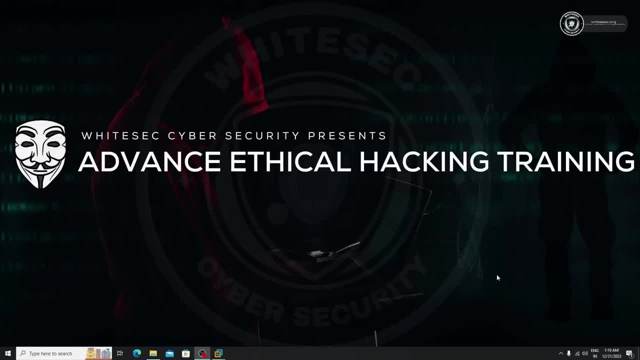 this language as well. if you don't know that much grammar, then simple i. i also type the same things. okay, normal, uh, i don't type any kind of query queries here or something like that. i just type the simple letters. it will show me the results. okay, it's not a big deal. now, here again i am. 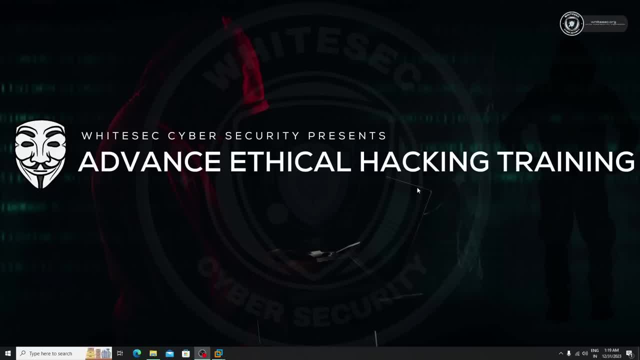 saying: don't be panic here. okay, mostly the people will think that, okay, first let's learn the complete networking, then let's move to the ethical hacking. don't do that. first complete the ethical hacking. then if you want to learn about more about networking, then go for it. okay, first complete. 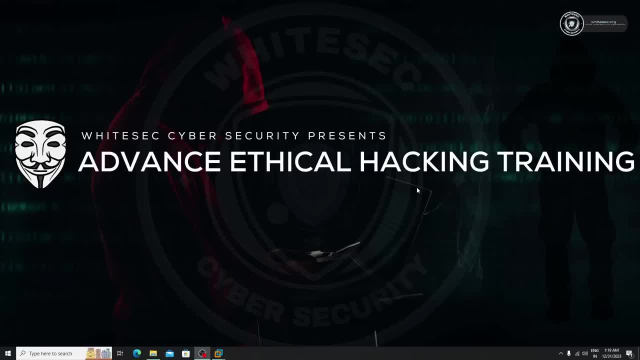 your goal this? uh, if you want to learn ethical hacking, just first complete it, then go for this things. okay, because if you jump, assume that you just was a half section of this ethical hacking training and you are jumping to networking. okay, at that time you will suffer, okay, you won't learn. 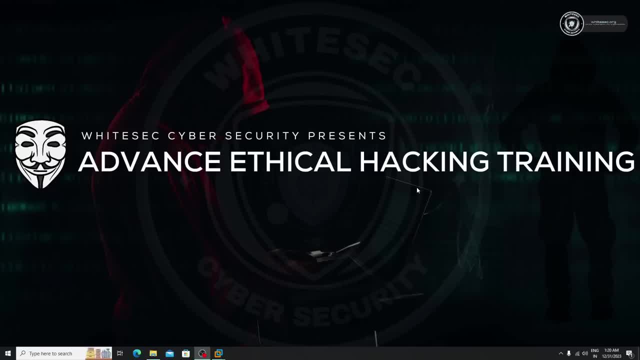 this thing, not this. that okay, this is the thing, okay. and the second thing is: uh, if, if, if you guys want the networking training, okay, for we. we only cover the training for hackers. okay, we, we won't cover each and everything we cover which is necessary for pentesters and ethical hackers. 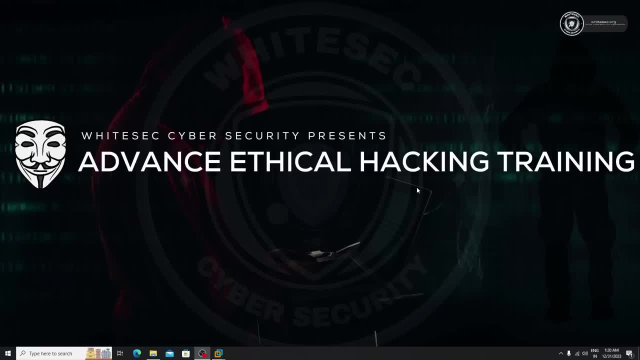 okay, if you want that, then just just comment. okay, we will soon we will launch it, okay, on this youtube channel. you can able to watch it. okay, this is also one thing, just just comment. okay, if you want the training, just comment, we will decide and we will try to create the training. okay, right, hope. 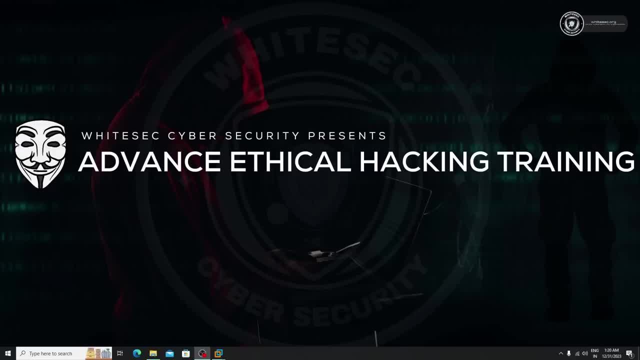 you guys enjoyed this classes. again. i am saying this section is enough for this training. okay, don't be panic here. don't uh do this kind of stuff, right, thank you, have a nice day. in this class we are talking about what is ip? okay, internet protocol. now here, let me tell you, this is just 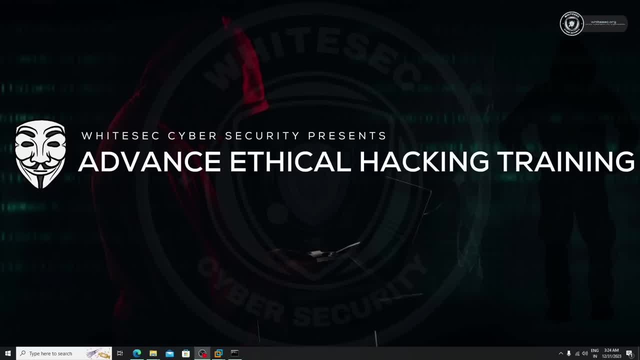 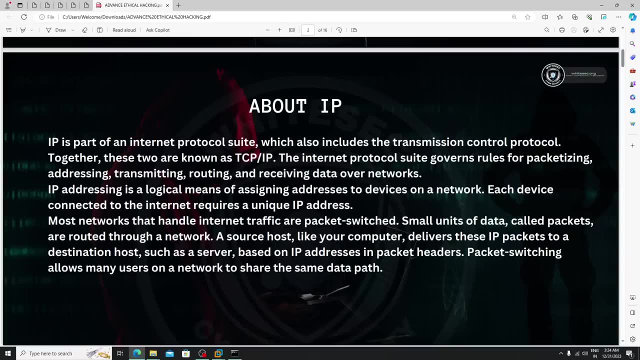 a definitions. once we jump in practical class, you will get each and everything. you don't need to worry here, right, but the definitions is also very important. the points also very important. okay, you need to focus. i'm going to provide this pdf in description. just download it, just read it. 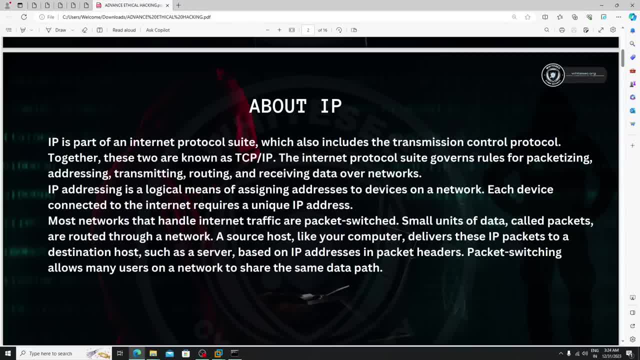 okay, ip. ip stand for is a part of an internet protocol suit which allow you to access the internet, and also includes the transmission client protocol. what is this? this is transmission client protocol is nothing but tcp. okay, just see together. these two are known as tcp, ip. okay, what is this? tcp is nothing but transmission client protocol and ip is nothing. 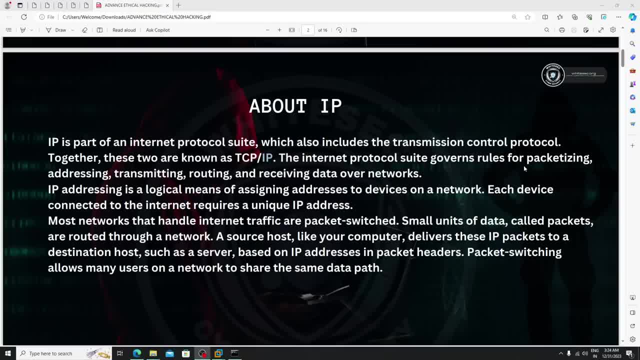 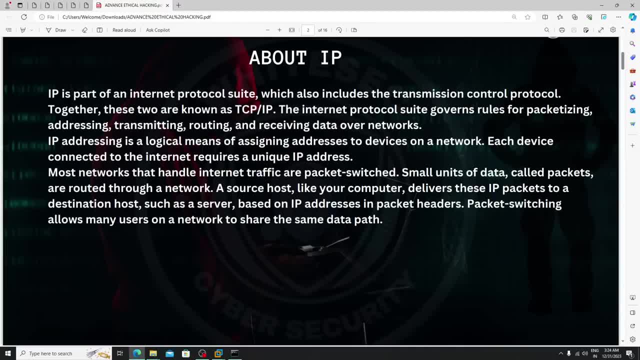 but internet protocol. the internet protocol suit governs rules for packetizing, addressing, transmitting, routing and receiving data over internet. also has the kind of a pdf. you use word Dj innocent prisons. so there you have it. any device, any hardware, any system which is connecting with the internet, connecting with internet, right, the internet will assign the. 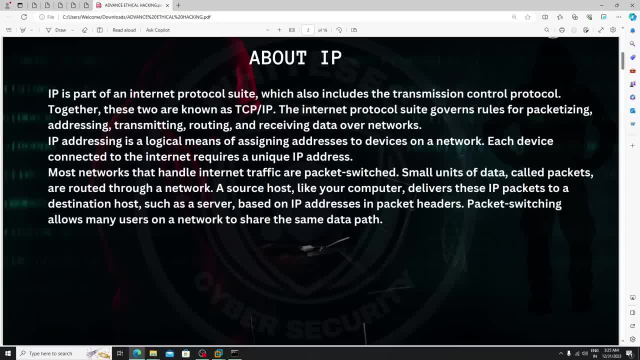 ip address to it. it's a kind of name, okay, but every name is unique. here it's: uh, see, in, uh. let me give you an example of human being. assume that there is a john is there? this is a username. it's a human being name, okay, like human name. now just focus, people will use this name, okay, it's not a unique name. 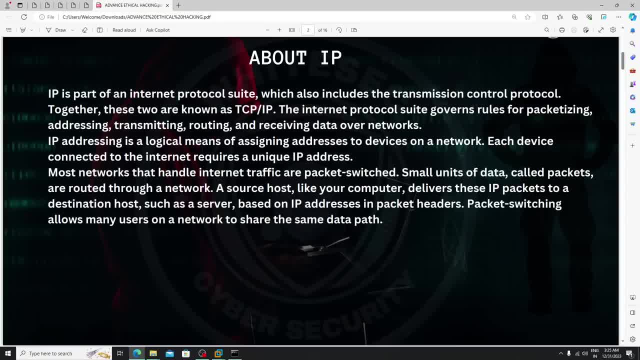 john is not only one guy. there is a lot of users are there. a lot of people are there with the same name like john. okay, like same uh name, like uh john. okay, now here the thing is in system. in computer systems, uh, in the devices which are connected with internet, it doesn't work like. 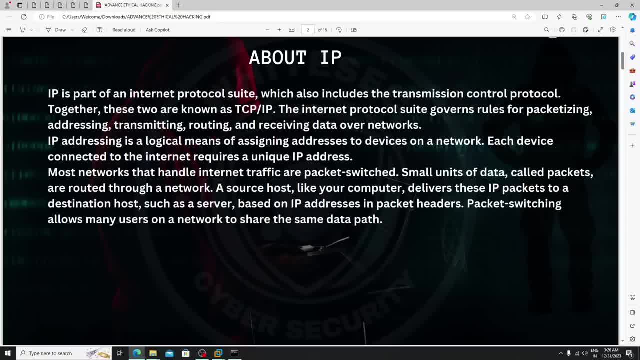 that, okay, every system- again i am saying every system and every hardware which is connected with internet, how their unique name, which is known as ip address. okay, it's not like human being, okay, but you can give an example like that. okay, it's a little bit same, but in, again, i am saying in human. 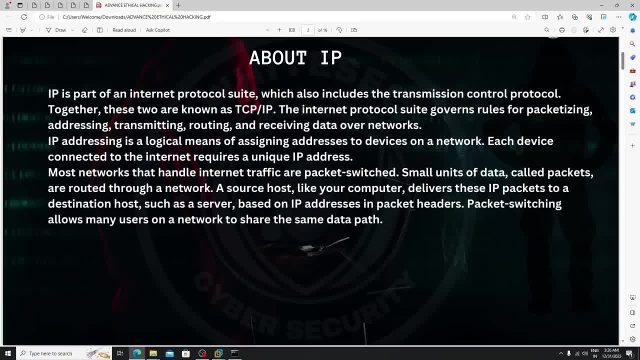 being what we do means in humans: we. we use a name, but the name is: a lot of people use the same name there. okay, but in system in computers, in- uh, this, you can use the same name. okay, but in system in computers in- uh, this. system in computers in. 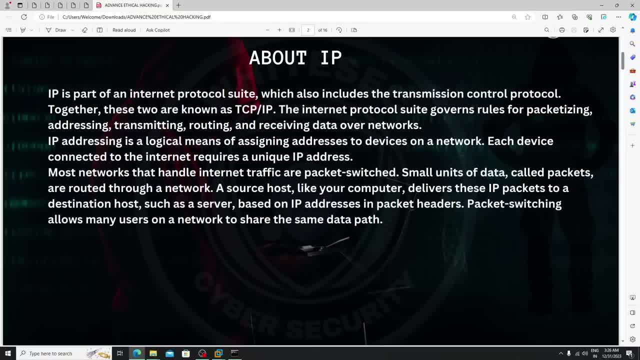 devices. it doesn't work like that. okay, it's have the unique names, okay, which is known as the ip addresses, so we can able to identify the systems here. okay, see here, each device connected to the internet required, say, unique ip address, if you uh, if you uh see connected the devices which are 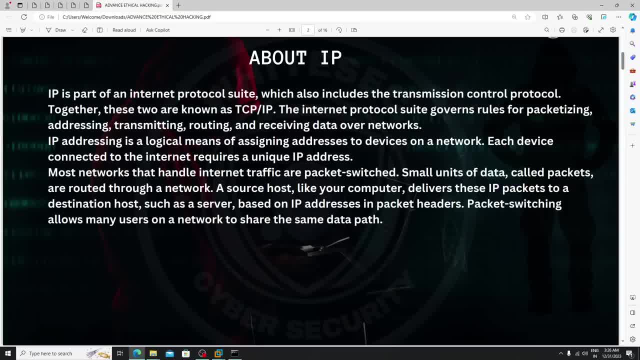 connected with internet, they need the unique ip addresses. okay, most networks that handle internet traffic, or packets, which do small units of data called packets, are routed through a network. a source host, like your computer, delivers this ip packets to a destination host such as a server server. in the trauma of server, you can also say it as a any website. 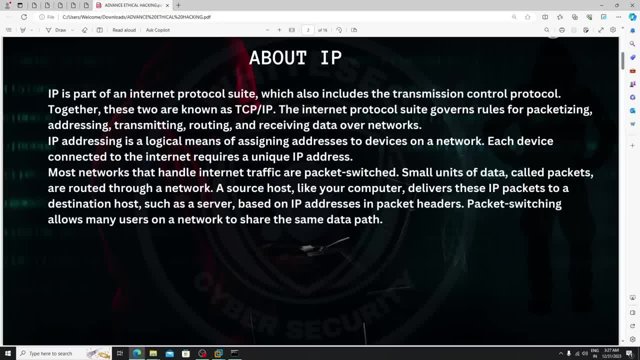 okay, any, uh. in the simple words, you can just take an example of facebook, google or any website, man okay, which is on internet. okay, if you want to serve that website, assume that if i want to open the facebook, at that time what i need first thing, i need ip address. okay, in my system. 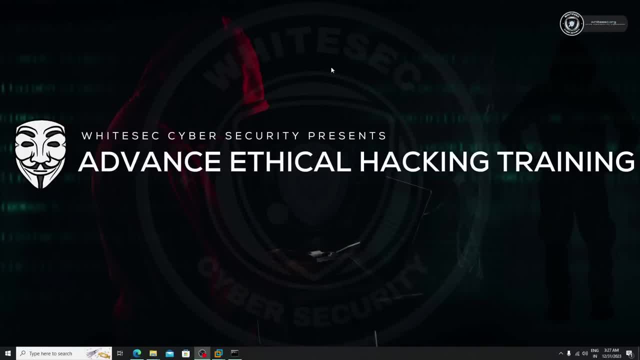 need the ip address. okay, if the ip address is not there in my system, at that time i can't able to access it. okay, now see, simple, if i disconnect the internet, then i can't able to serve the. uh see, there is a wi-fi, right? if i disconnect this wi-fi, then what will happen? you can't able to. 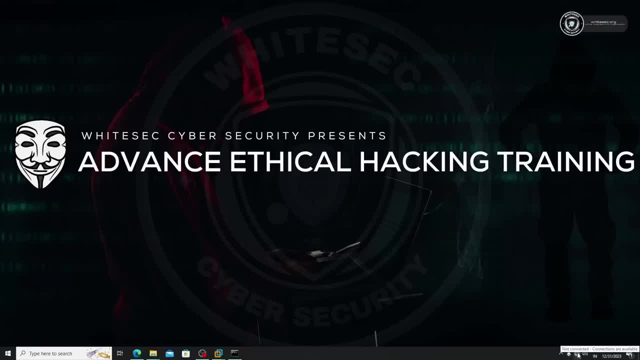 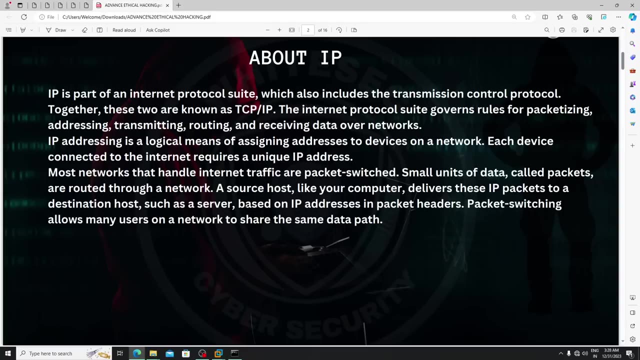 serve. after disconnecting the y uh this wi-fi network, your public ip address will be gone. okay, this is the thing. so that's why you can't able to serve it. okay, hope you guys get it. you get okay. once you jump in practical, you will get it, such as server based an ip address in packet. 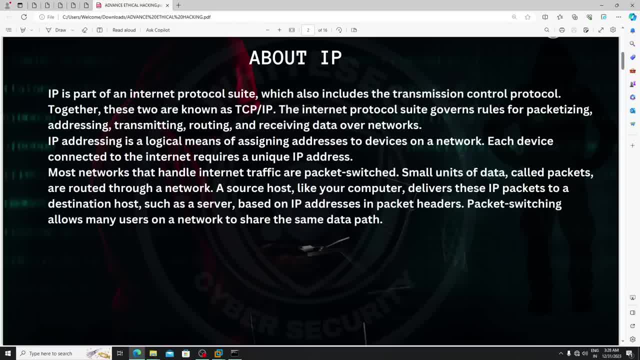 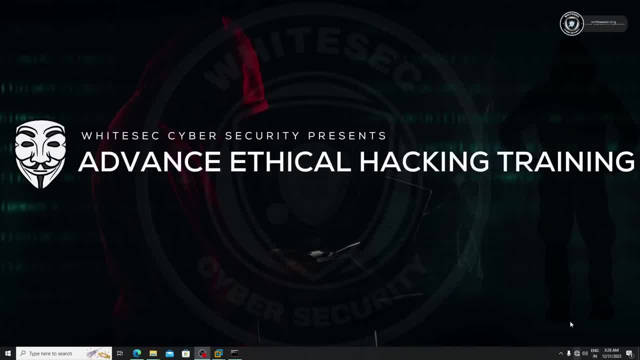 headers. okay, packet switching allows many users on the network to share the same data path. okay, this is a thing. see, let me tell you right now. i just give the example of this internet on the public ip address. okay, don't uh in private ip address without internet. also, you guys can able to. 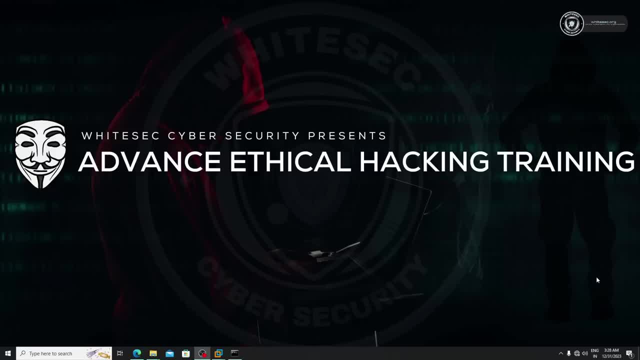 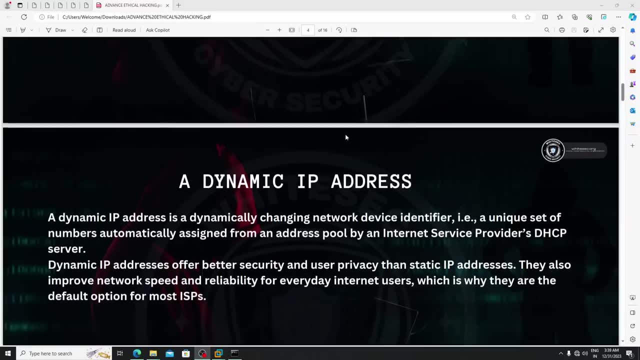 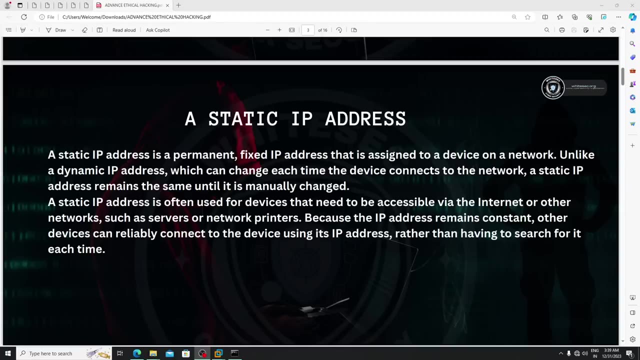 access the server, which are implemented locally. okay, don't worry, just ignore it, you will. in this class, we are learning about a static ip address and a dynamic ip address. see. a static ip address is a permanent, fixed ip address that is assigned to a device on a network. okay, it might be any. 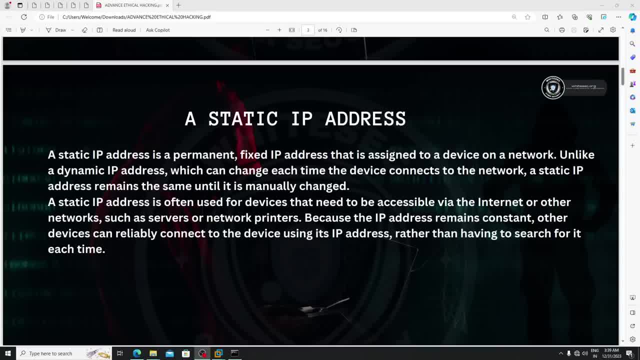 device: okay, any windows device. printer, okay, windows, it doesn't matter. the device which connects with internet: okay, any hardware unlike a dynamic ip address. now, just focus on dynamic ip address. it? uh, a dynamic ip address which can change each time the device connects to the internet. okay, see, there is one machine. i'm gonna explain you one real world. 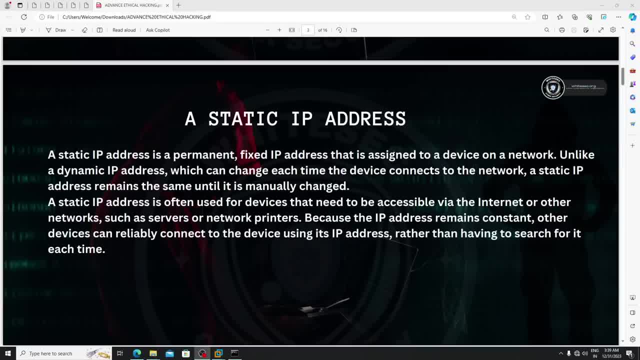 scenario as well, don't worry. see, uh, here a dynamic ip address which can change each time the device connects to the internet. this point you need to be remember. okay, a static ip address remains the same until it's manually changed. see, a static ip address will be same. okay, if i want to. 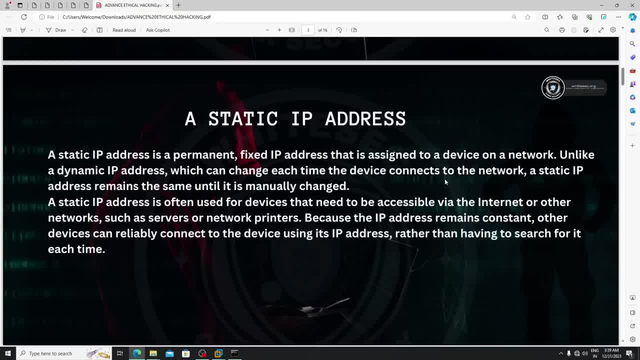 change the ip address, then i need to do it manually. this is a thing, right? the static ip address is often used for devices that use to be accessible via the internet or other networks. uh, the mostly. just take an example of any server. okay, assume that googlecom is here. 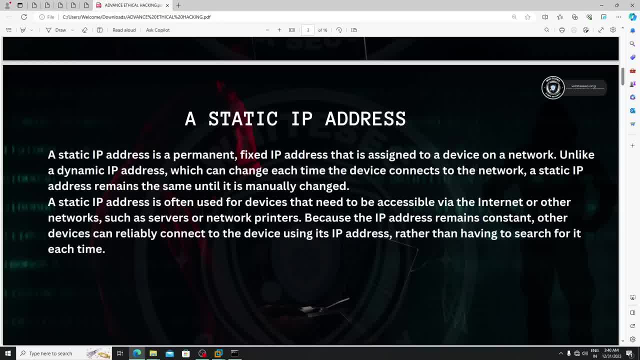 let's use a static ip address. okay, they won't change the ip. this is the thing. uh, mostly the servers use a static ip addresses. okay, such as servers, see, such as servers for network. okay, they won't change the ip. this is the thing. uh, mostly the servers use a static ip addresses- okay. 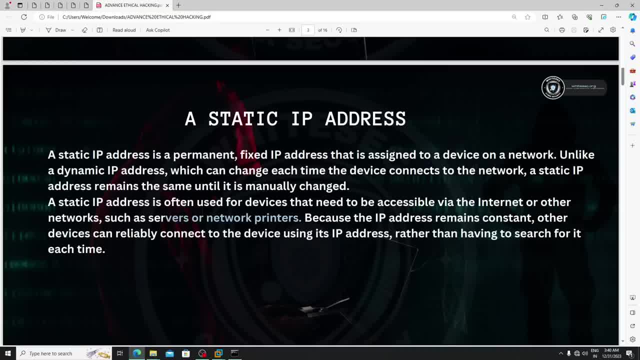 printers because the ip address remains constant. other device can reliably connect to the device using the using its ip addresses. okay, rather than having to search for it each time. the simple thing: if i, if i type the googlecom- that simple i can able to see the website. if i type the facebookcom. 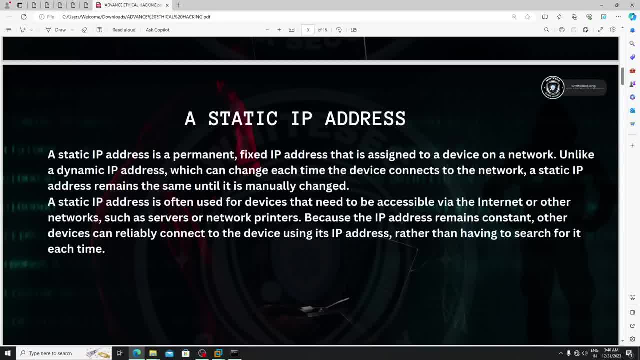 simple. i can able to see the website there. okay, this is also. i know it's a little bit different process, but for explanation purpose i'm i'm telling you these things. okay, there are a lot of students out there who know these things. okay, like this, networking, something like that. so for 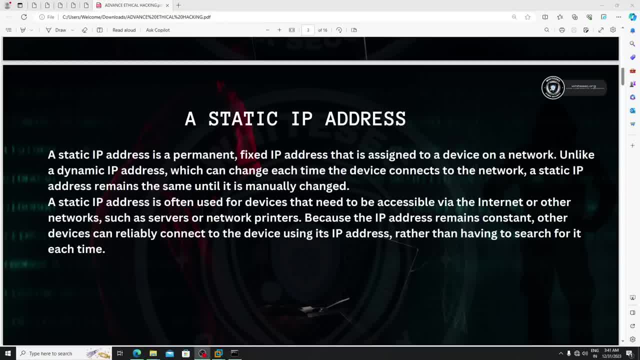 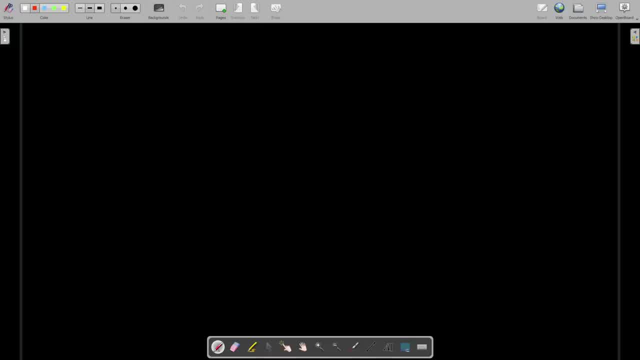 just i'm giving the examples. okay, right now, here, the thing is, uh, just let me explain you here. now, see, let me tell you one real world scenario. assume that there is one organization hired you, okay, to perform pen testing on their internal network. now, you just visited to that. 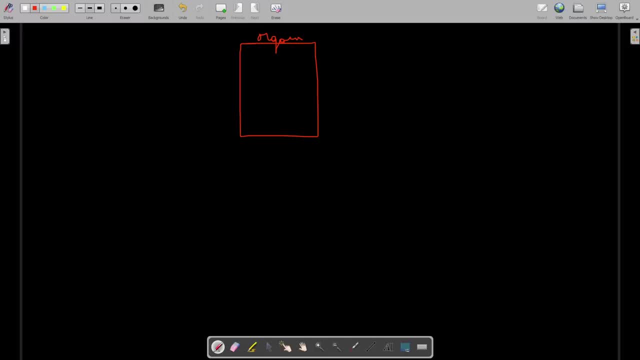 organization and you, you are started the pen testing there. okay, uh, simple, before doing that, they will. they will give some ip addresses where you need to perform the pen testing. okay, assume that that client given you this ip address: 192.168 point okay, 133.137, okay, this is ip address. 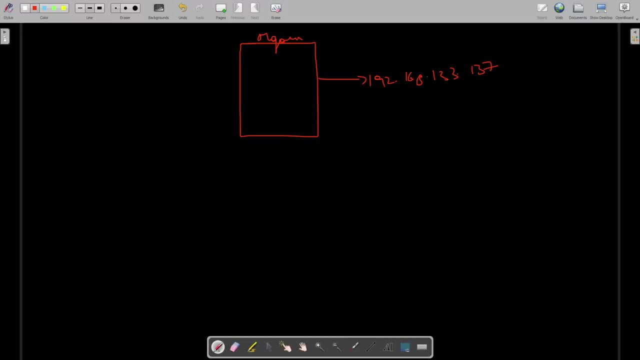 this is your target ip. okay, you need to perform pen testing on this ip address. you need to find the vulnerabilities on this ip address. okay, this is the thing. now you just found the vulnerabilities on this ip, you just would write excellent report right, and submitted it in report. what we can able to see? we see the ip address, we see what kind of 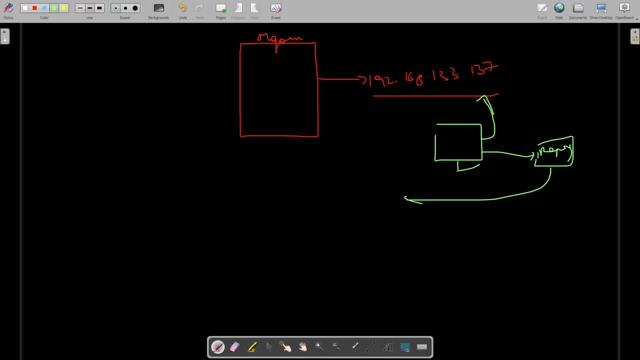 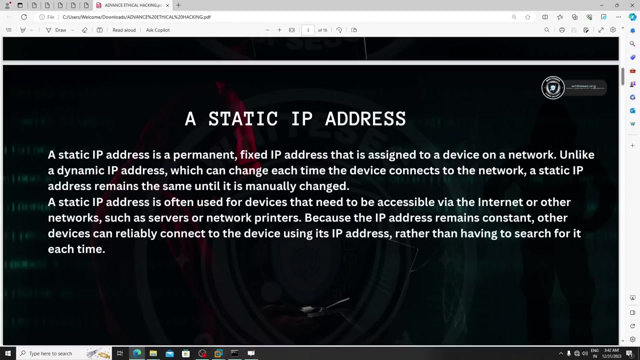 vulnerabilities. we found, okay, which we tools we, which tools we use. we uh the risk. we just write this kind of shops, simple, we just send uh, submitted this uh report. okay, now see, assume that this your target ip is dynamic. what is dynamic here? see that here there is one excellent point: a dynamic ip address which 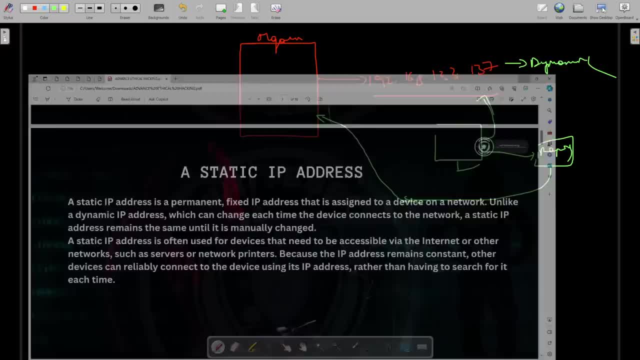 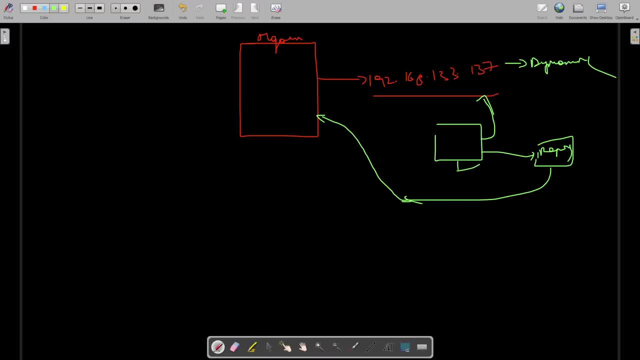 can change each time the device connects to the network. assume that this system, the, the system which having this ip address. assume that it's restarted. okay, due to some reason, the system has been restarted. at that time, what will happen? the ip will get changed. okay, and you just submitted the report. 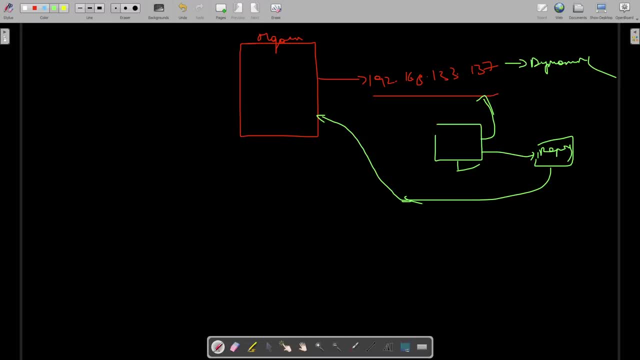 there. assume that there are checking that. okay, is there any kind of vulnerabilities? or something like that. see, after changing that, the uh, after restarting the system, the ip will change to something like this: okay, 192, point 168, point one, three, three point one, two, seven, or something like. 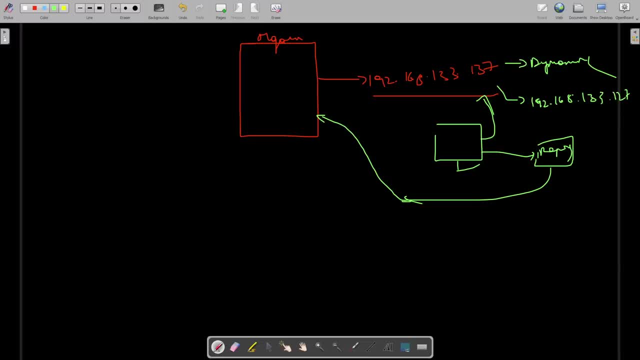 that some different numbers will come here. okay, so the thing is, it might be a huge confusion, right? so what, before performing the pentesting, they need to disable the dhcp protocol on this ip. okay, so it may become the static. okay, so the thing is, i can, i can able to write the report there. they can able. 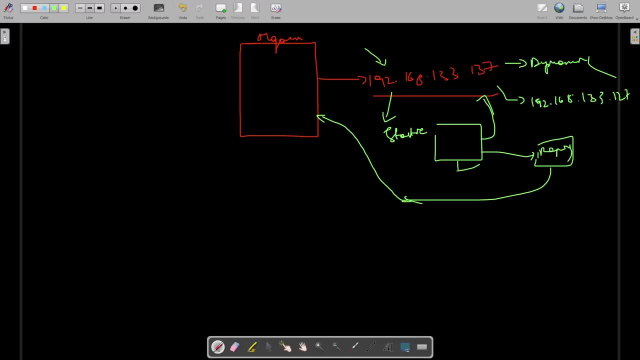 to find it okay, this is the thing. so this, first of all, the thing is: during the pentesting also, you need to take these steps. okay, you need to see this. all kind of steps, right? so this is a kind of d? uh, we will learn about dhcp as well. see the dynamic. 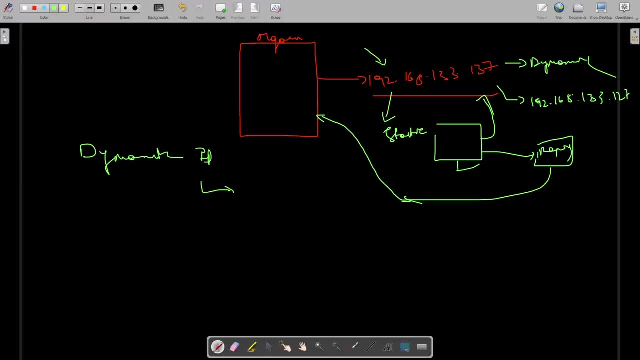 ip depends on dhcp. okay, if dhcp is enabled there on any ip or any system, at that time the ip will get changed. okay, assume that you just disable the dhcp. then there are some manual process or there. by performing that, you can able to set the ip address static. static is nothing but what it is unchangeable like, not unchangeable it. 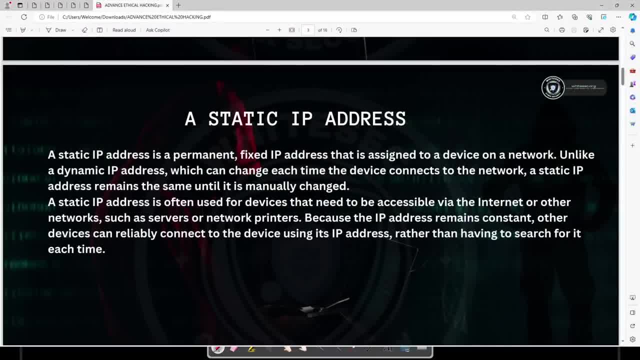 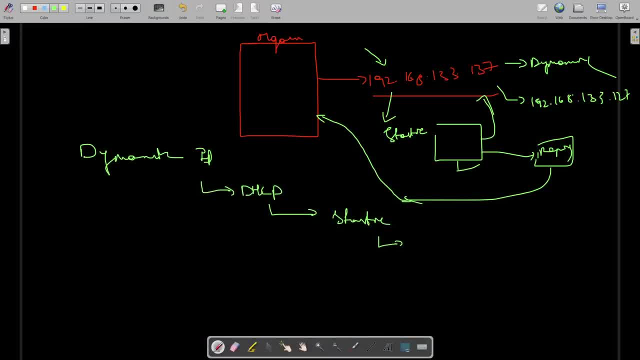 a fixed ip address. i just told you, right? uh, it's a permanent, fixed ip address. i just told you about the servers. if you type simple googlecom, you, you guys, can able to see the page there, okay. if you type facebookcom, you can able to see the page there, okay, this is the thing. assume that there. 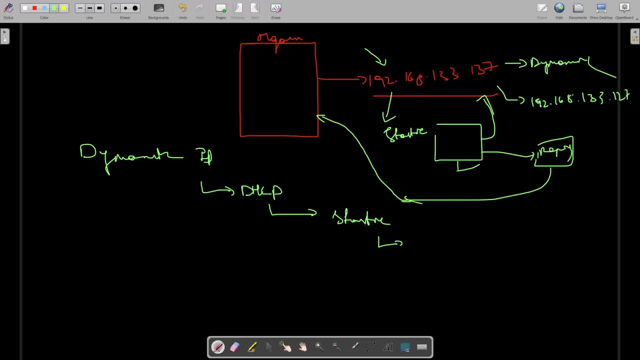 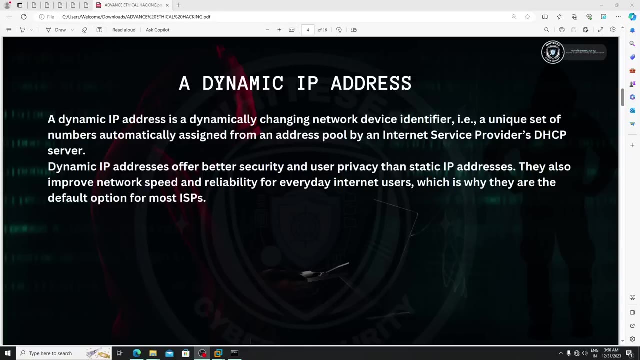 is a one camera ip. assume that you just type the ip address simple. you guys can able to see the portal there. okay, so what is this? this is a nothing but a static ip address. now let's learn about dynamic ip address. a dynamic ip address is a dynamically changing. 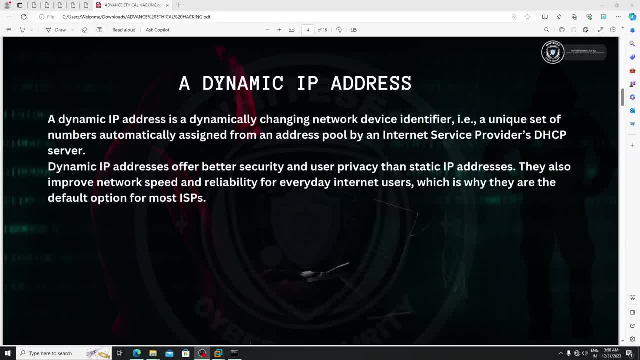 network device identifier, ie a unique set of numbers automatically assigned from an address pool by an internet service provider, dhcp server ds. dynamic ip address offer better security and user privacy than static ip address. okay, they also improve network speed and reliability for everyday internet users, which is why they are the default options for most isps. okay, default. 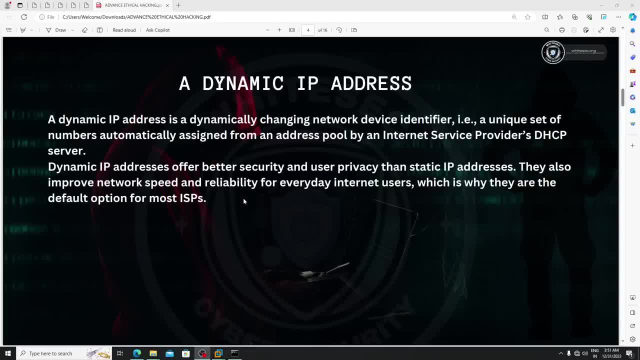 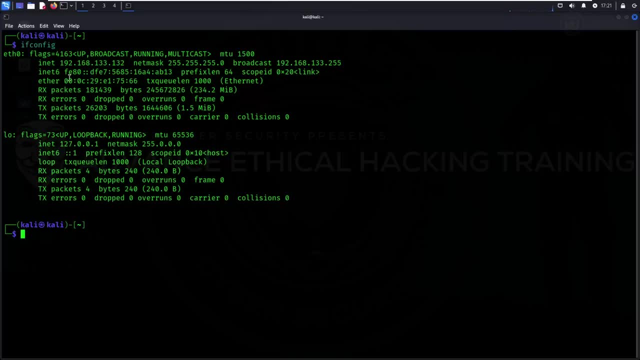 in vmware. once you boot the linux in vmware, okay, at that time also the linux, uh, that ip address have the dhcp there. okay, it's a. it's a dynamic ip. after some days- see, right now you guys seeing, uh, if i type ip config here, you can able to see this is my ip. 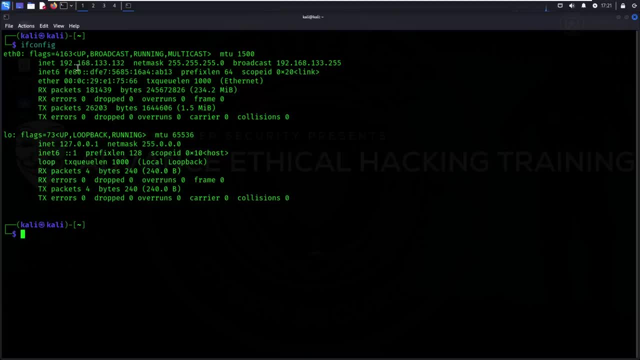 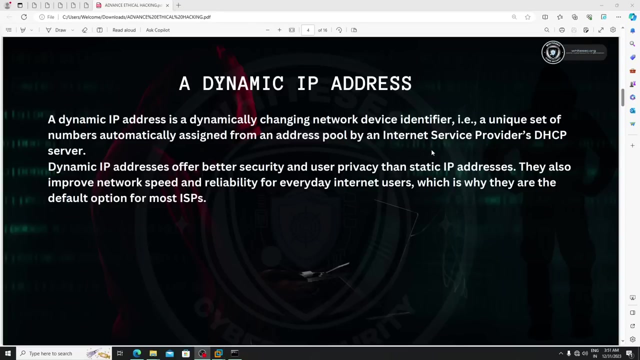 address right now, okay. maybe tomorrow, okay, maybe after some hours, the ip will be changed. okay, this is the thing. by default, it's run on the this thing only. okay, dynamic. basically, if you want to set the static ip address, you need to do the steps manually. okay, this is the thing. 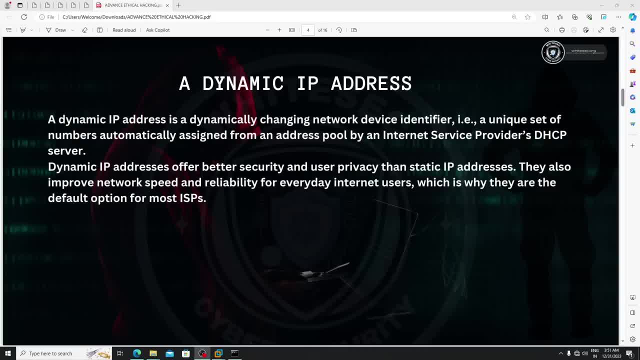 and also it is secured by comparing to static ip address, because the ip will change here. okay, so any attacker can't able to uh focus on it. okay, like, assume that, uh, i am just targeting the any kind of dynamic ip based server. okay, at that time, assume that they they just restarted the. 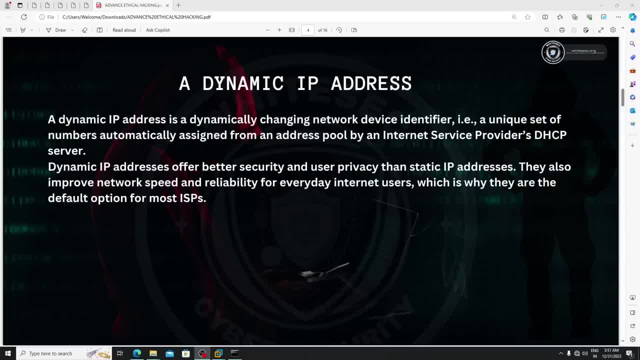 server. at that time the ip will change, okay, so i can't able to target it. i need to find i i can able to find it, but it is a kind of secure okay, like by doing some kind of stuff you can able to do that process. okay, but it is hard, right, okay now. 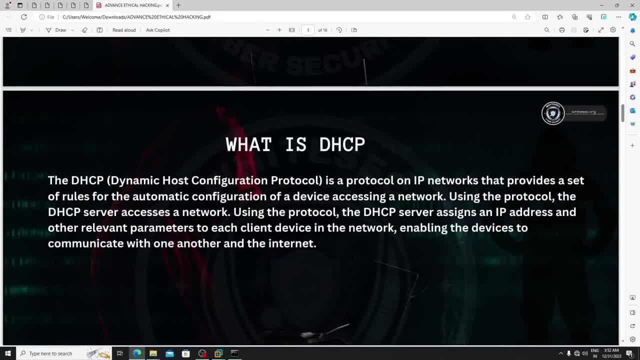 let's learn about dhcp as the dhcp dynamic host configuration protocol. it's a protocol on ip network. i just told you this one as well in static ip address section on ip: ip networks that provide a set of rules for the automatic configuration of a device assessing a network using the protocol. 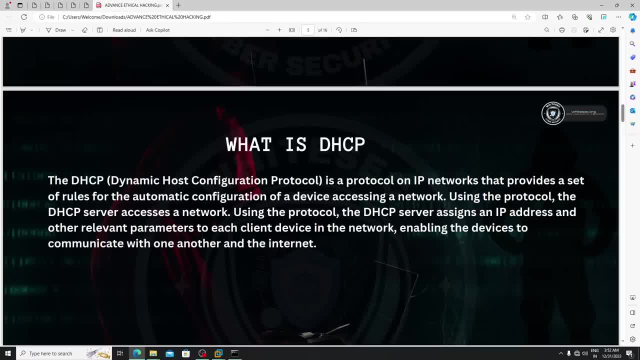 the dhcp server access a network using the protocol. the dhcp server assign an ip address and other relevant parameters to each client device in the network, enabling the device to communicate with one another on uh and the internet. so this is the thing. basically, it assign an uh ip address. 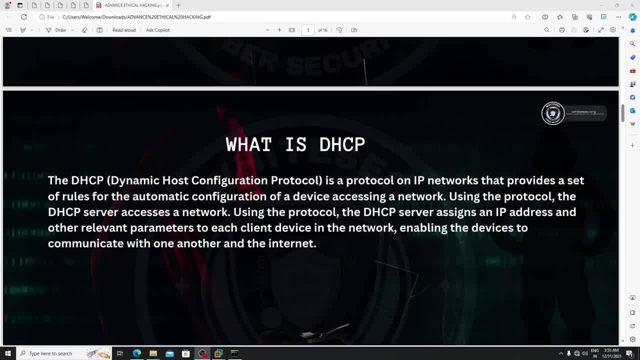 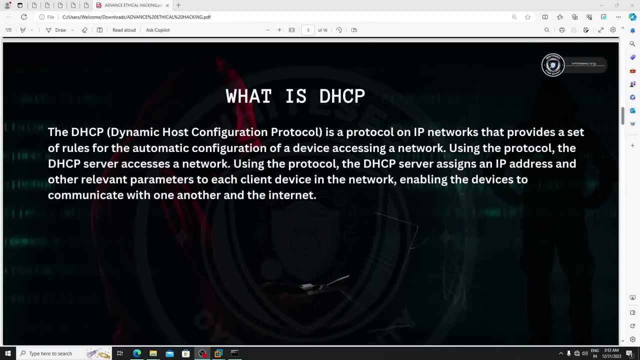 and other real, relevant parameters to each client device in the network. okay, so they can able to ping it. okay, this is the thing. they can share the files. okay, uh, this kind of shops, see, enabling the address to communicate with one another and the internet. so this is a part, it's a, it's a. 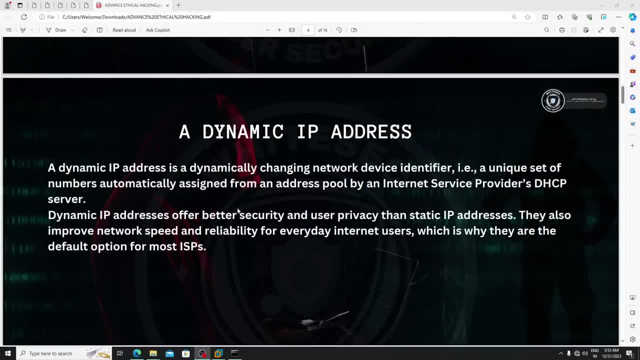 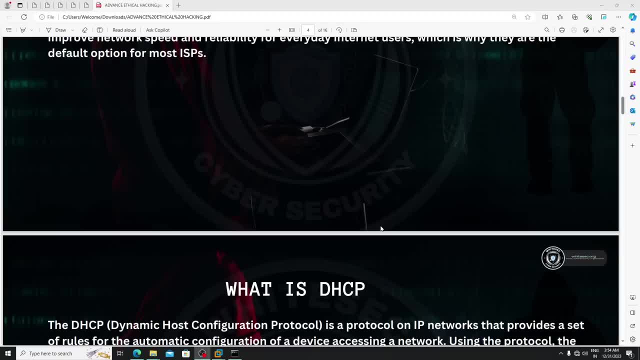 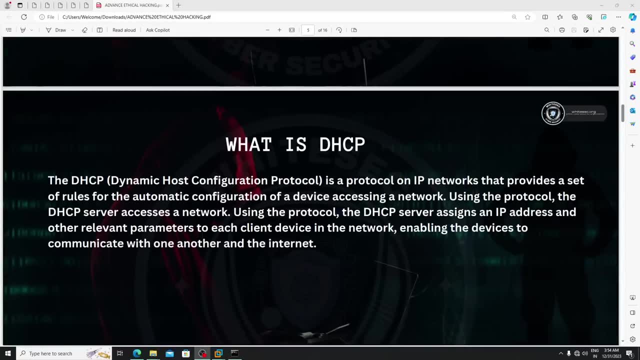 not. uh, this much stops okay. once you jump in practical classes, you will get it okay. just just do the practice, okay, because once you see these things in in your own lab, which we just set up there, you, you will get it. okay. what i am trying to say, each and everything, if you focus on simple, 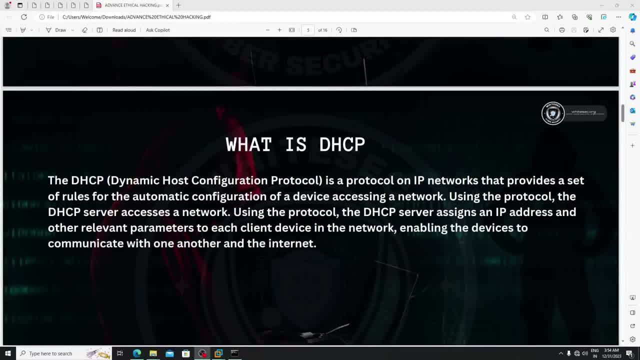 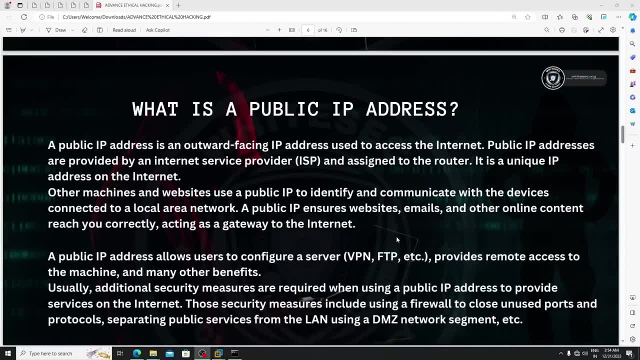 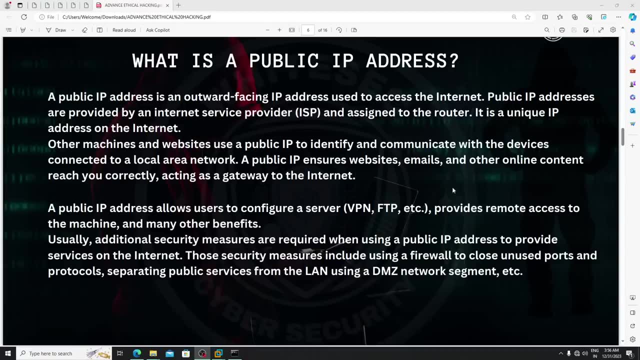 this, this things. then it is hard. you won't get a practical knowledge. okay, just here is some examples. just try to do the practice. okay, you will get it. now we will. in the next classes we are learning about what is public ip address and what is private ip. okay, right now in this class we are 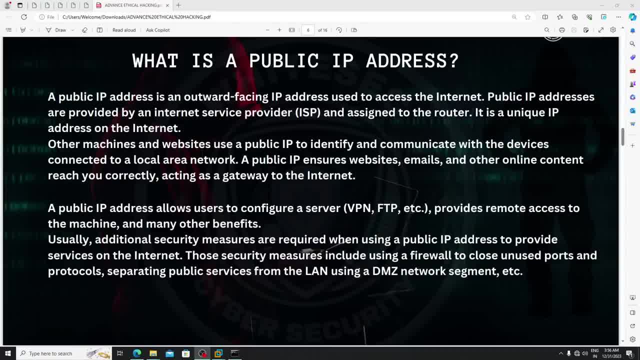 learning about. what is it? uh, what is public ip and what is private ip? okay, private ip address now a public ip address. it is an outward facing ip address used to access the internet. i a public ip addresses are provided by an internet service provider, isp. what is internet? 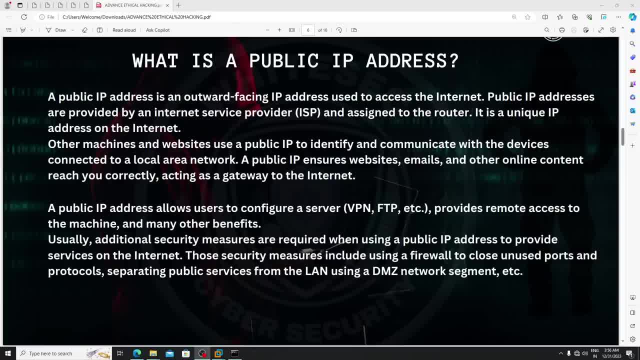 service provider here. assume that you are using the wi-fi router of tp link. at that time, this he is your provider there. okay, now the same thing. assume that you are using atl sim card to get the internet. he is a atl. is your isp there? this is a simple thing which you need to remember, okay. 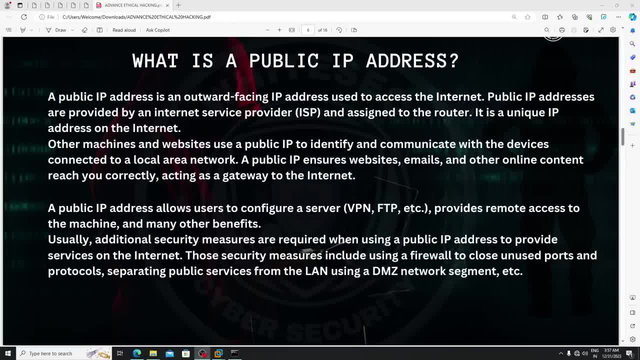 assume that if you are using any kind of vodafone or something like that to access the internet at the time, the vodafone is your isp. okay, don't get kind of confused here. okay, this is a very easy things. okay, right, and assigned to the router, it is a unique ip address on the 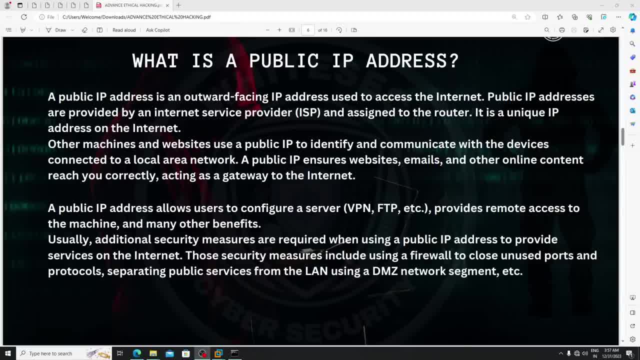 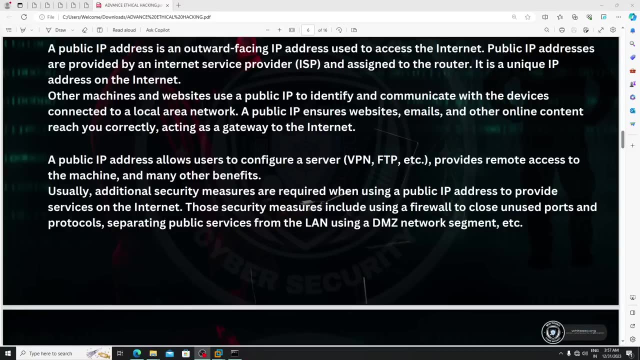 internet. other machines and websites use a public ip to identify and communicate with the devices connected to a local area network. a public ip ensure website emails and other online content reached reach you correctly, acting as a gateway to the internet. okay, a public ip address allows user to configure a server, such as a vpn, ftp, etc. okay, ssh or as well. 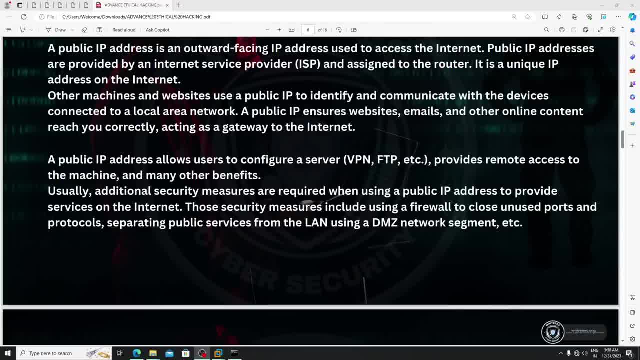 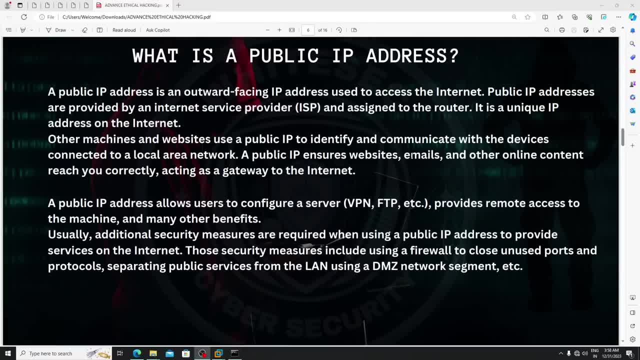 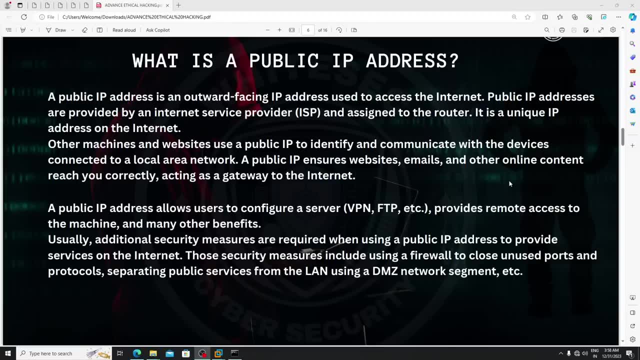 okay, any, any uh thing. okay, like any protocol. assume that if you want to communicate with the machine by using the ip, like we know about ssh, right? if you don't know about the ssh, then watch our uh, open port pens, pen testing training. okay, you will get. it provides remote access to the. 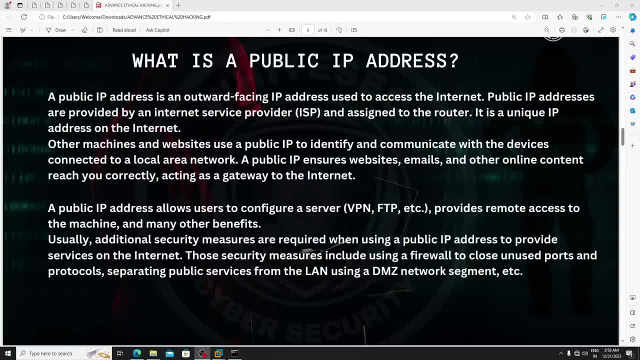 machine and many other benefits. okay, basically, this guy, you can able to use these services on public ip only. okay, assume that if you want to run the vpn at that time the vpn will affect on the public ip. okay, like, uh, well, let me show you what is public ip here. if you, if you type 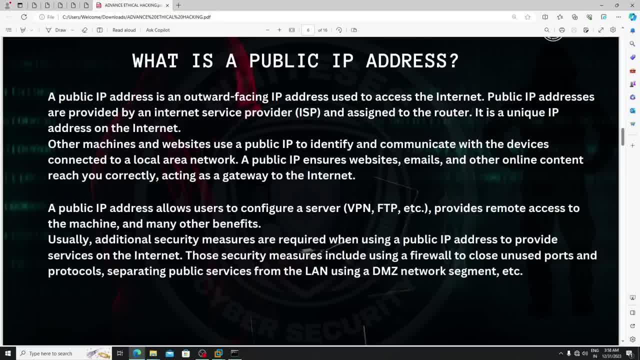 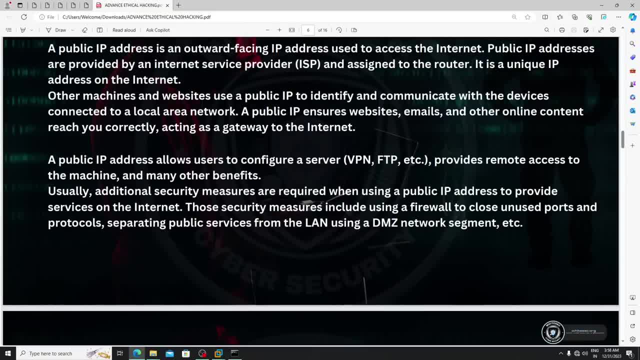 uh, what is my ip on internet? you guys can able to see the public ip. okay, this is the thing. uh, let's cover that in practical class. usually, additionally, security measures are required when using a public ip address to provide service on the internet. those security measures including using a firewall to close unused unused ports and protocols. 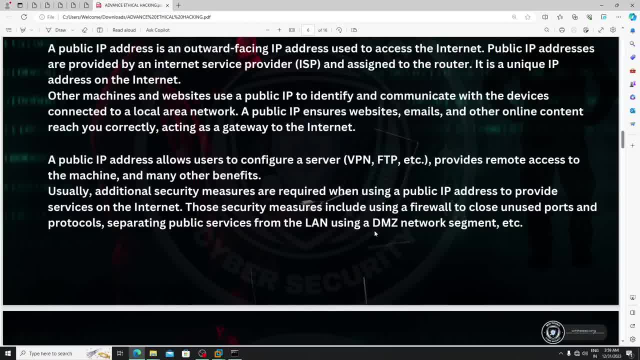 separating public services from the lan using dmz network segments. now, in a simple words, let me tell you this thing. okay, again, i am saying you need a little bit hacking knowledge for it. okay, assume that i am not talking about ethical hacking knowledge. i am talking about the android hacking. 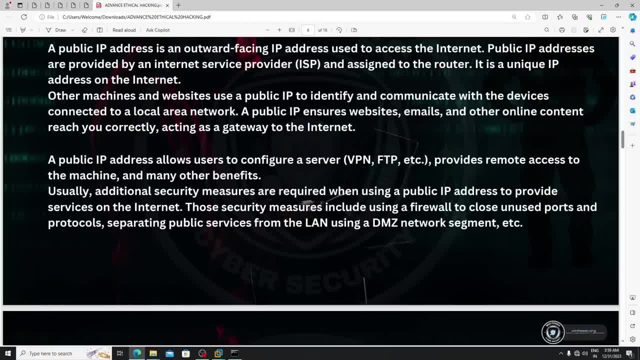 or windows hacking knowledge. okay, assume that, uh, you know about port forwarding, right, mostly the people who are searching about ethical hacking. they know about port forwarding. uh, assume that i want to hack anyone. okay, uh, the guy who is living. assume that i am from uk. okay, my target. 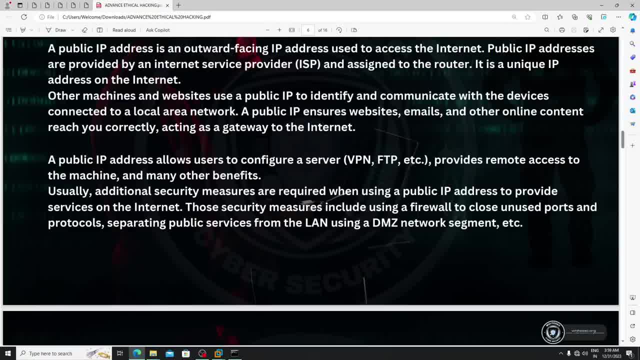 is living in us. i want to hack him. okay, the simple thing is i need to perform the port forwarding here, okay, so this is the thing. so, basically, using the public ip address, the- the security is there. okay, to close the unused firewalls. and also, you guys will see that in some routers you won't have this kind of 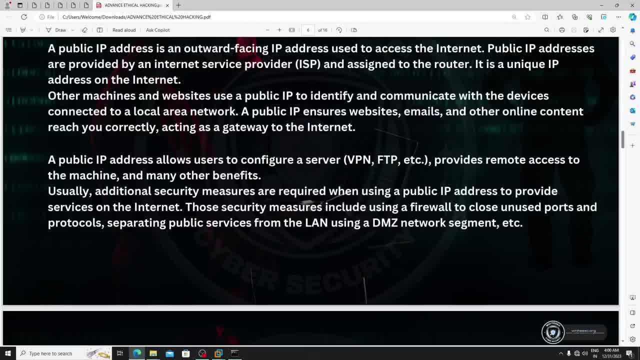 uh, this. this port forwarding features in your router. okay, because your isp is not accepting it. okay in atl. uh, if you are using uh internet, okay in by using the internet, the sim card internet i am talking about. you can't able to perform the port forwarding using that. okay, this is a thing. 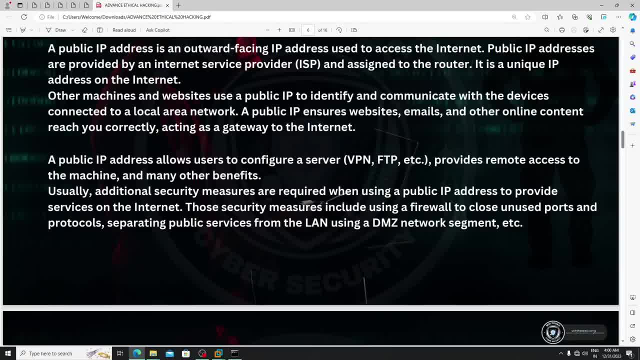 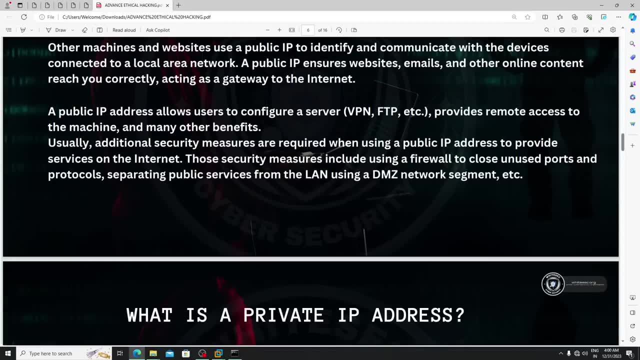 because they won't allowing you to do that process. okay, due to the security reasons. okay, this is, this is a simple thing. okay, separating public survey, public services from the lan, using the dmz network, segments, etc. don't worry, once you jump, uh in hacking you will. 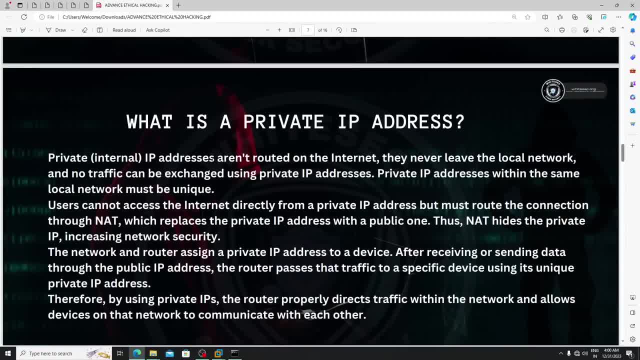 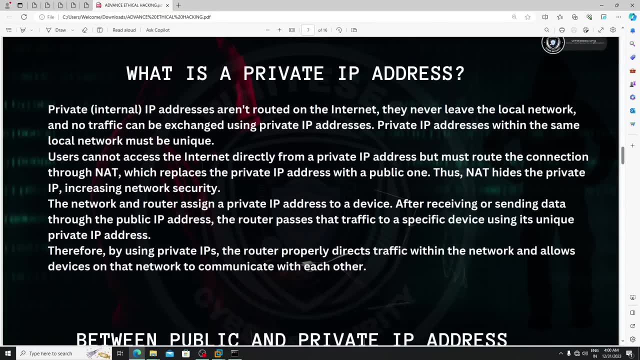 get it, okay, you just. what i am trying to say means: just try to hack your own devices first. okay, then jump for uh, real world pen testing. just set up your own lab and do the practice. this will give you a lot of uh, just like a practice man. it's a very excellent if you practice. 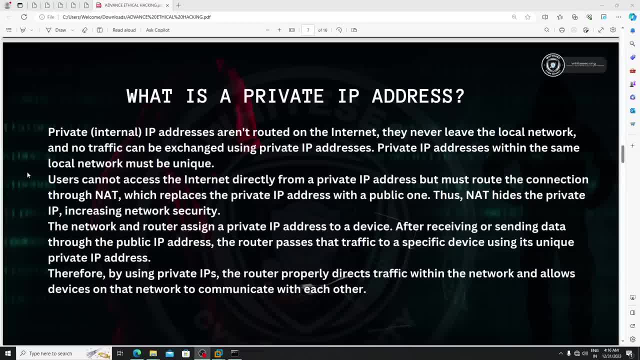 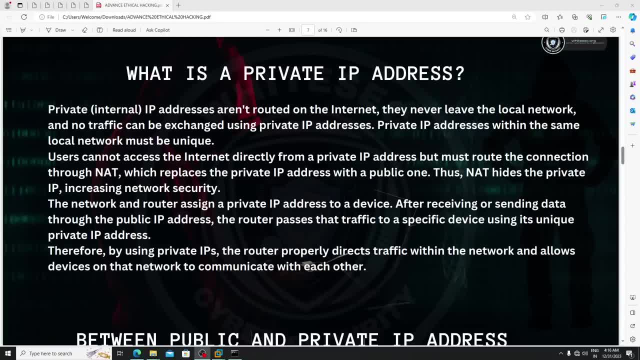 now in this class, we are learning about what is your private ip address. private, internal ip addresses aren't routed on the internet, they never leave the local network and no traffic can be exchanged using private ip address. basically, the thing is, by using private ip, you can't able to. 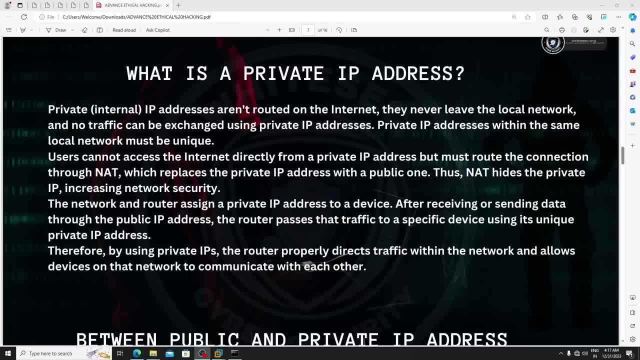 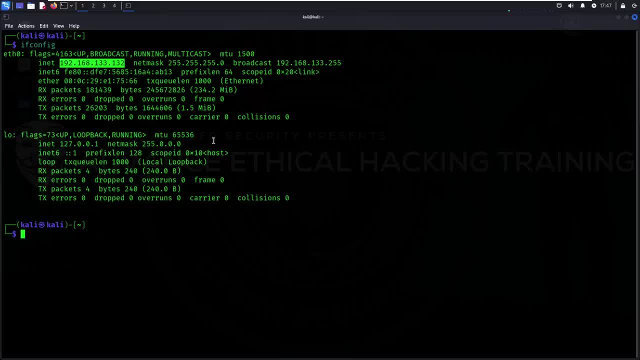 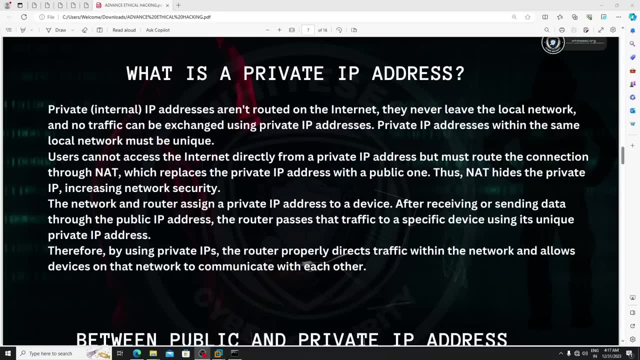 solve the internet? a simple thing, okay, like by using this ipa, you can't able to serve the internet. you can able to communicate locally with the local machines, but you can't able to serve the internet. this is a thing: private ip addresses within the same net, same local network, must be unique. what is this? 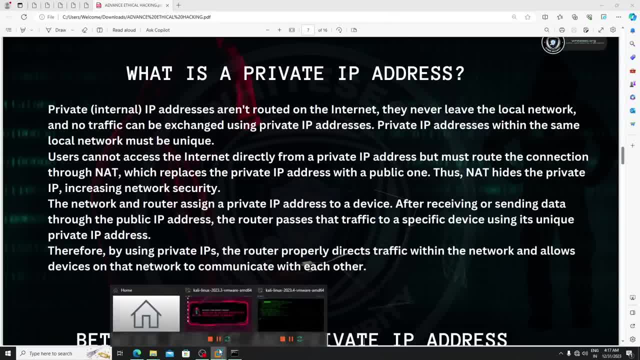 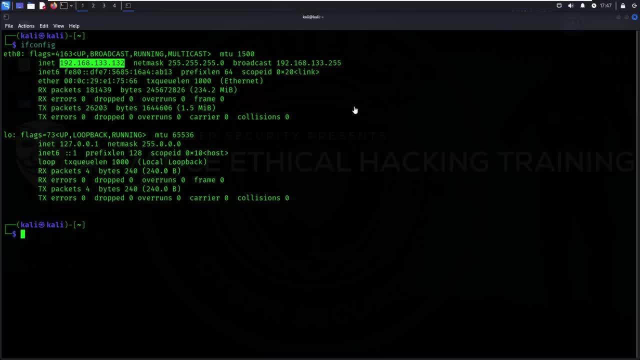 unique. unique is nothing, but see here, after connecting: see, these two machines are connected with the same wi-fi network. okay, now the it will assign the network to the same network. okay, now the uh. it will assign the local, uh, the local ip addresses, which are private ips. if i type, if 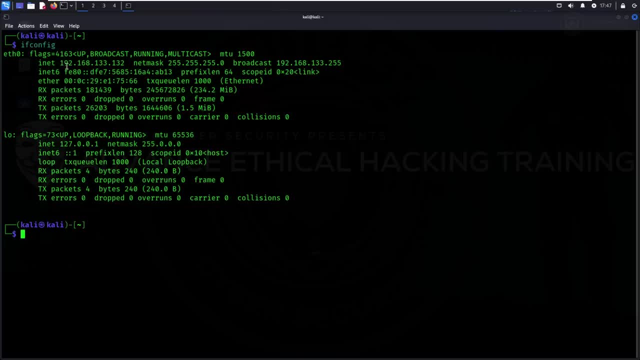 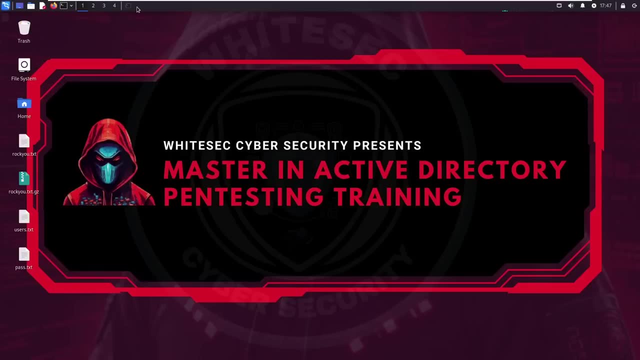 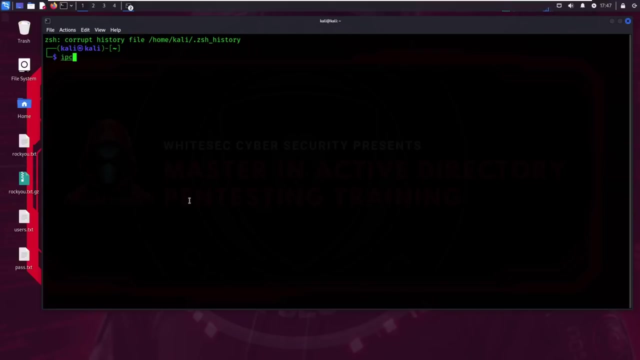 config, i can able to see the private ip right. see: 192.168.133.122 is a ip address of this kali machine. if i go to another kali machine and if i open, okay, if i open the terminal, if i type ip config here- sorry, if config, then you guys can able to see the ip address is different. the. 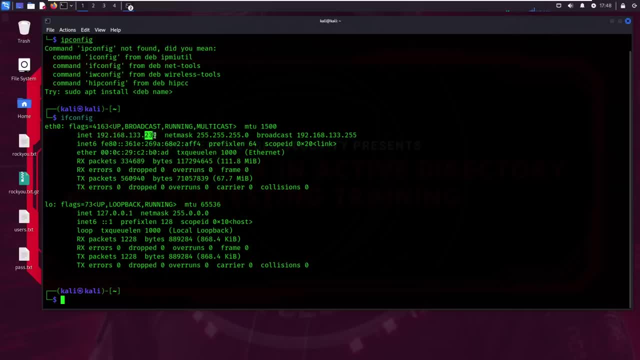 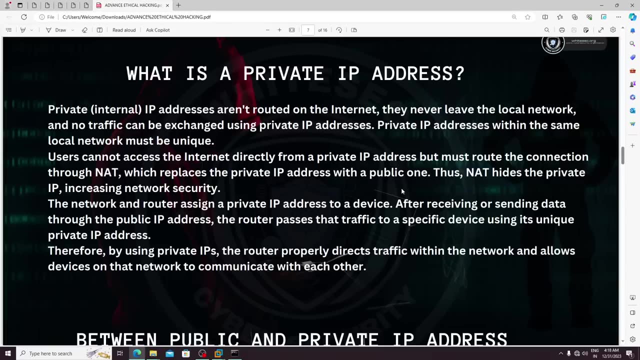 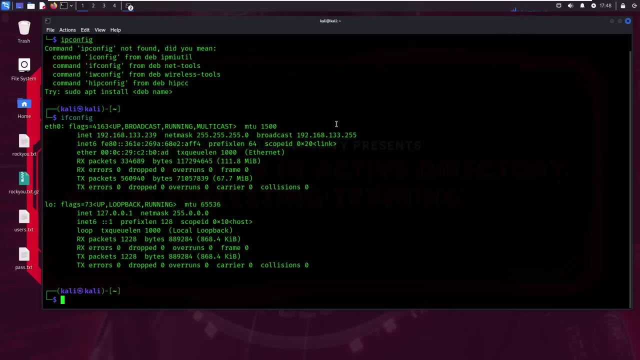 fact that you guys are starting three columns are same, okay, but in last it will be different. okay, this is the thing. it's a unit. just add hundreds of systems. okay, it will give you it will assign that unique ip addresses for the those hundreds of systems. okay, this is the thing. 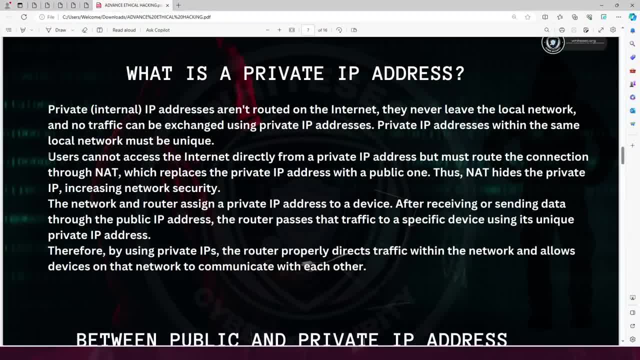 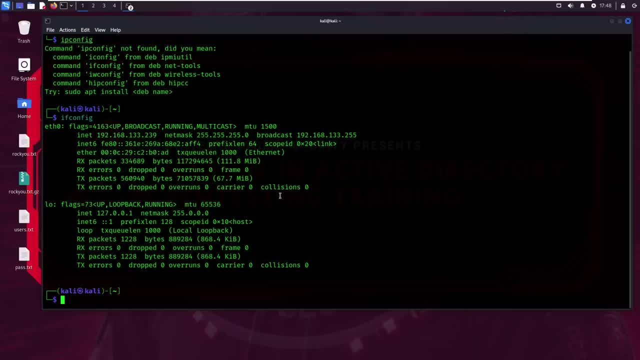 right, okay, user cannot access the internet direct directly from a ip address, i just told you. but most route the must route that connection through, not which we are doing here. only. okay, like we don't need to do that much process. but the thing is here by default. okay, once we boot the vmware. okay, basically, this kali machine is using the local ip addresses. 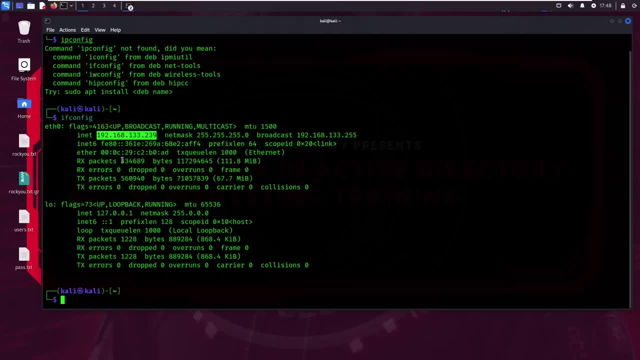 okay, this is the thing because, uh, it doesn't have the public ip. just see here: if i type if config, you can't see the public ip here. right, the simple thing is still, i can able to serve the internet. okay, if i open the chrome or something like that, firefox, i can able to serve the internet because 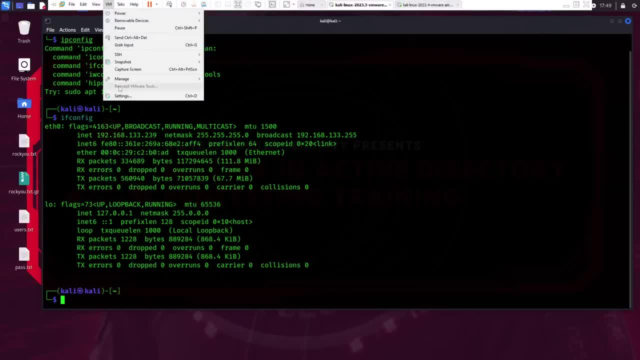 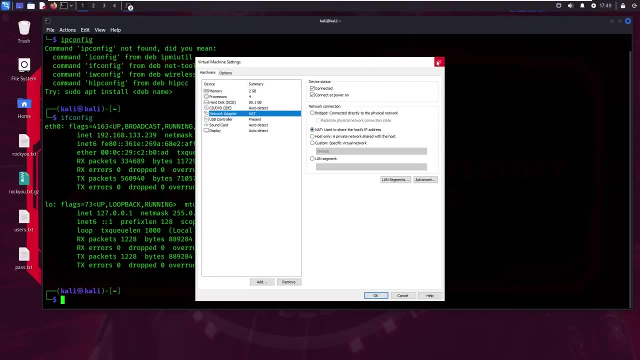 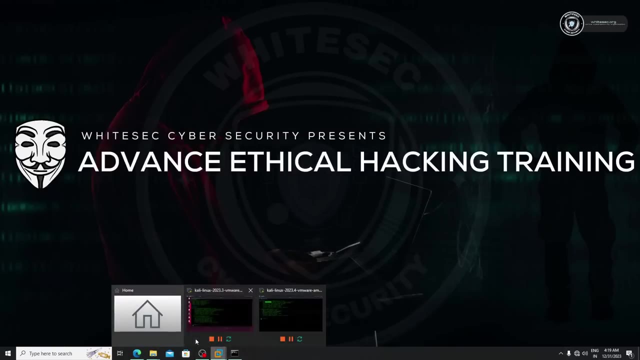 due to the routing. okay, see, simple, if i click on the vm, if i click on the settings and see: here network adapter is not used to share the host ip address. okay, basically it's using the ip address of this machine, the windows machine, this real machine. okay, hope you guys get it. 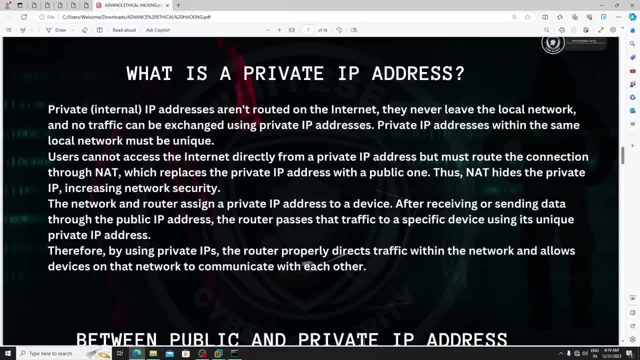 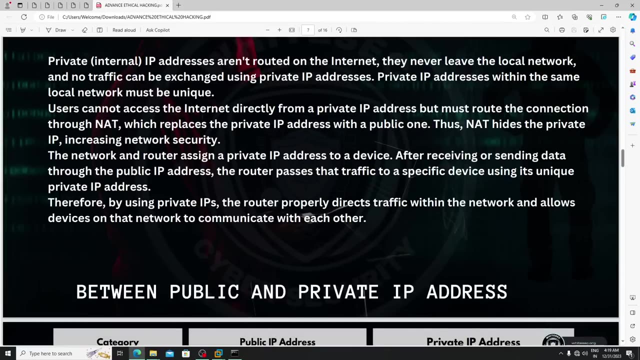 and okay. not hides the private ips- increasing network security, see here- from which replace the private ip address within a public network. does not hide the private ip increasing network security. the network and router assign a private ip addresses to device. after receiving or sending data through the public ip address, the router passes the traffic to a specific device using. 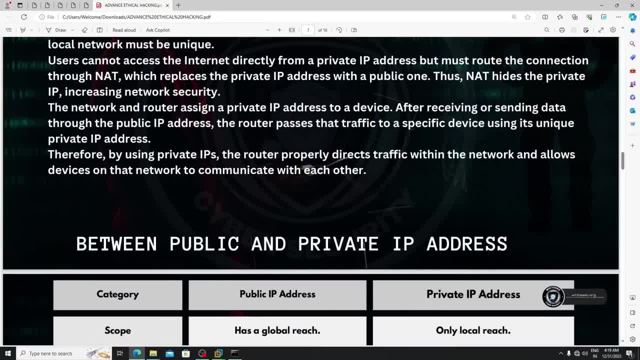 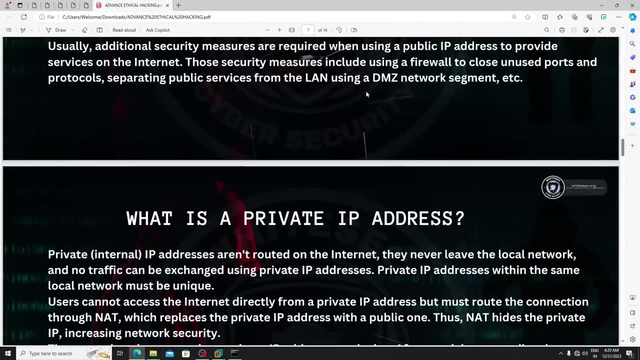 its unique private ip address. thus, for by using private ips, the router properly direct traffic within the network and allow devices on the network to communicate with with each other. okay, so this is how the process will work. it is a opposite by comparing to the public ip, but the 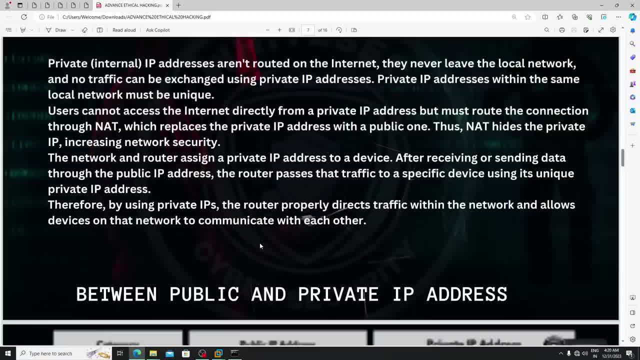 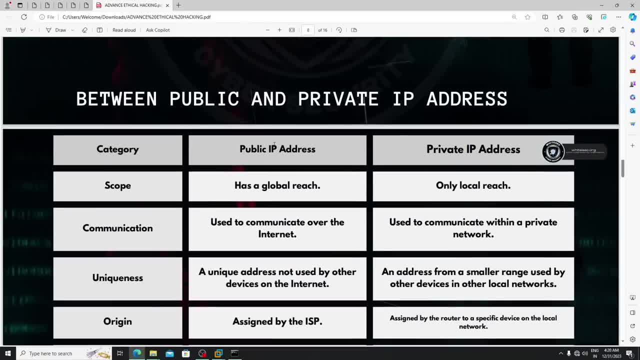 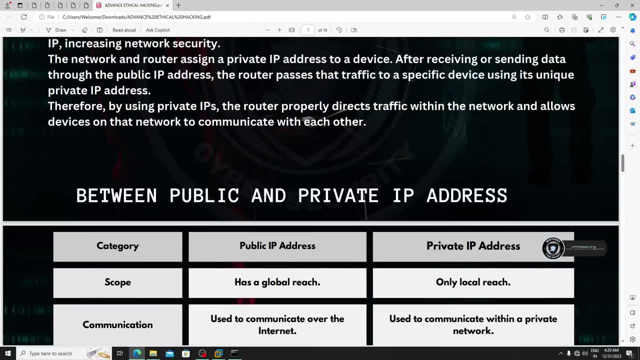 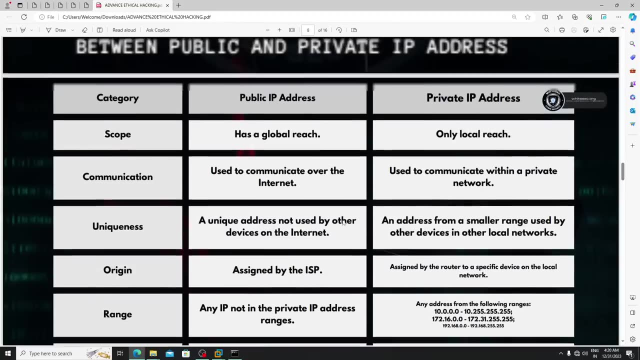 process is little bit big here. okay, this is a thing. mostly in private ip addresses dhcp is enabled. okay, mostly you will see that. okay, between uh in. in this classes we are learning about difference between public and private ip addresses. okay, let's cover this in the next class. it's a huge topic. 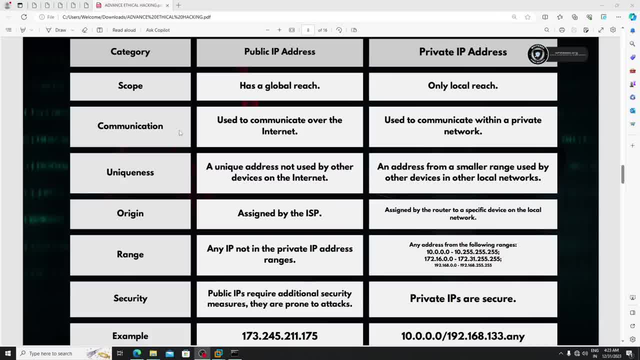 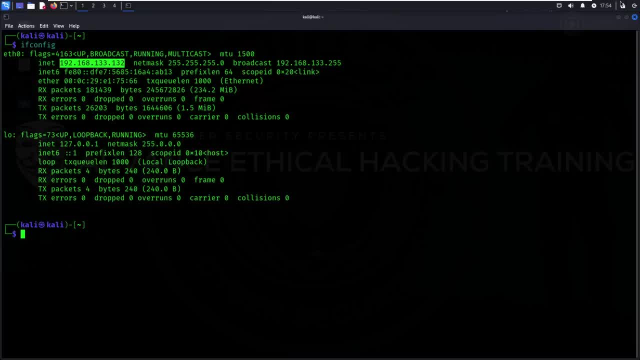 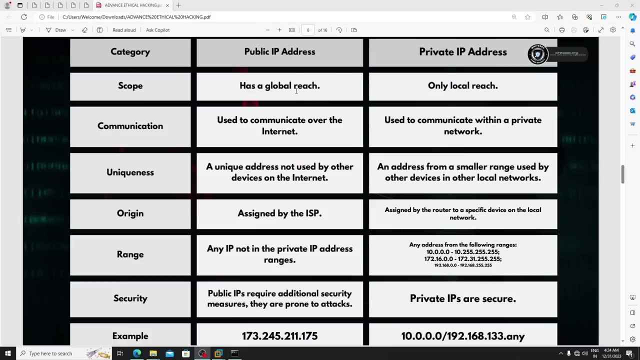 now in this class, we are learning about difference between what local, uh public ip address and private ip address. private is what private is nothing, but it's a local. okay, this is a thing which we, which we are seeing here. okay, this is a what private ip. now, scope has a global reach. anyone can able to reach there. okay, uh, if you copy my public ip, you 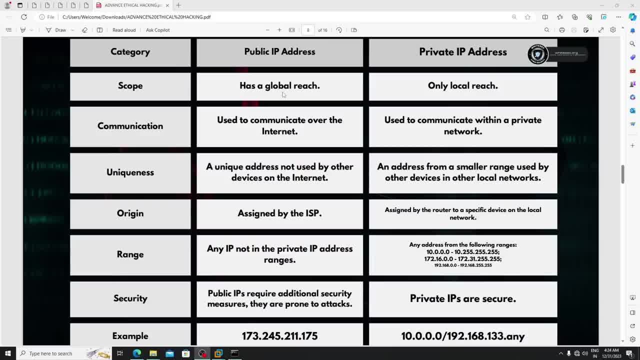 can able to ping it. okay, this is a thing now here, in private, only local reach, only the devices who are in that network can able to ping it. okay, this is the thing now. communication used to communicate over the internet used to communicate within a private network. okay, like only the, the, the users. 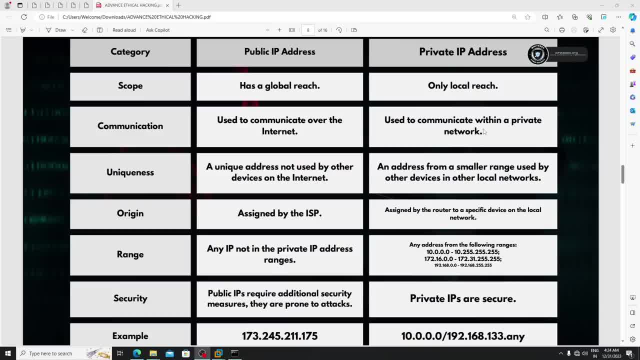 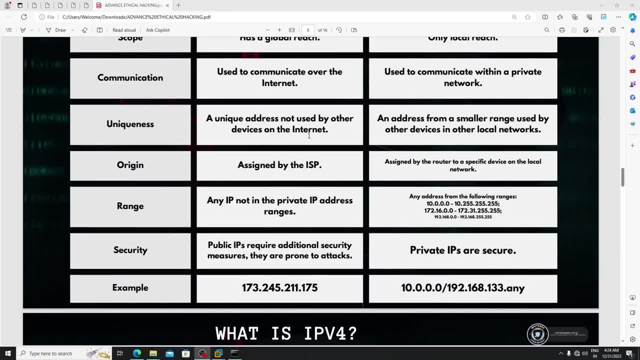 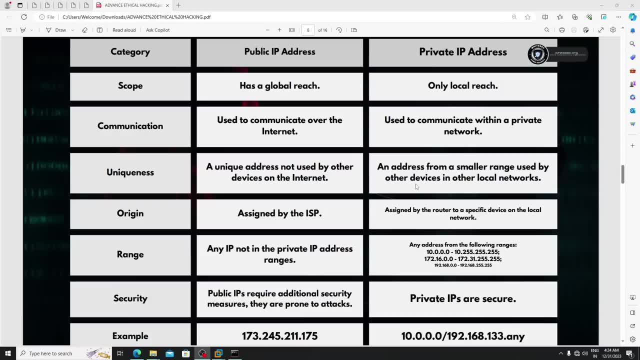 who are in that local network can able to communicate with that machines. okay, now uniqueness: a unique address not used by other devices on the internet and here, in private ip address, an address from a smaller range used by other devices in the in other local networks. the simple thing. what is? 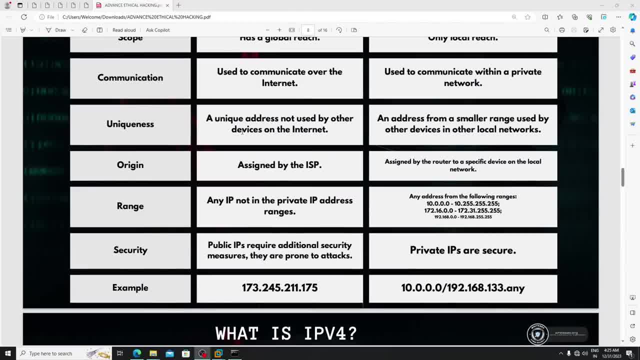 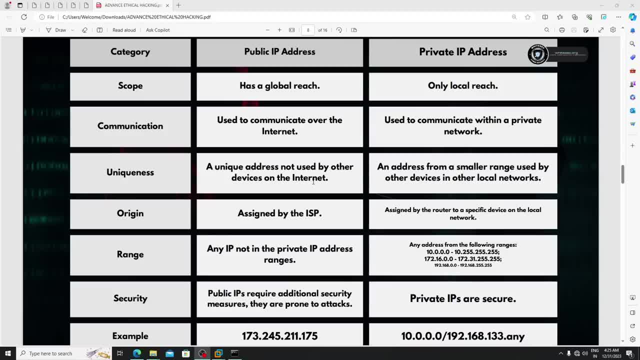 this means let me tell you a unique address not used by other devices on the internet in public, uh public ip address. assume that the isp provided one public ip address to you. okay, no one can able to access that ip address globally. okay, in whole uh world, no one can able to access that. uh, no one can able to. 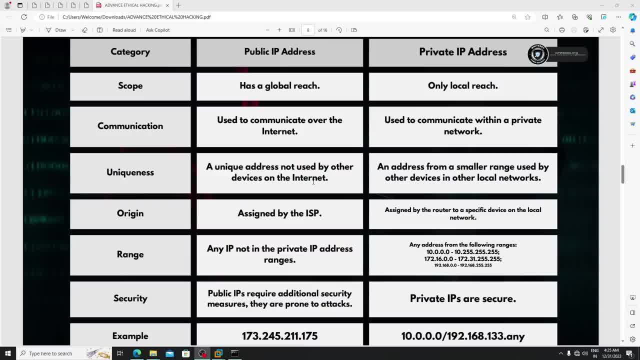 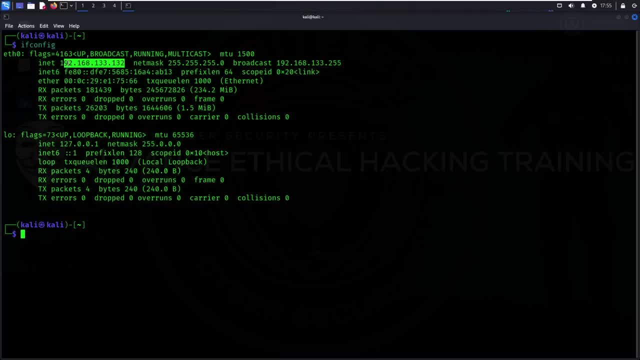 get that ip address which you have. okay, it's a unique, but in low in the private ip address, what will happen means see an address from a smaller range used by other devices in other local networks. see, right now, this is, this is my, this, this is my private ip address. right, assume that there is an. 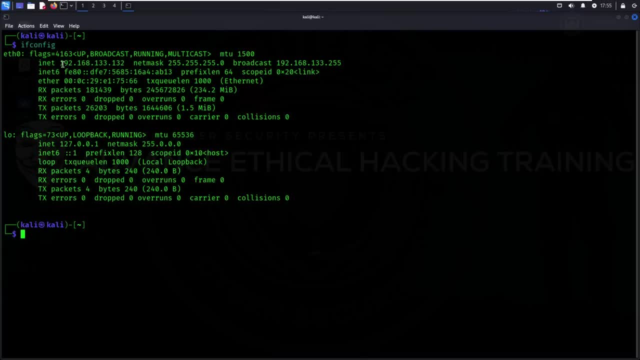 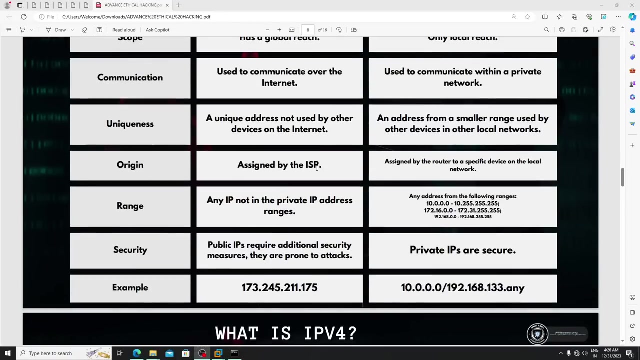 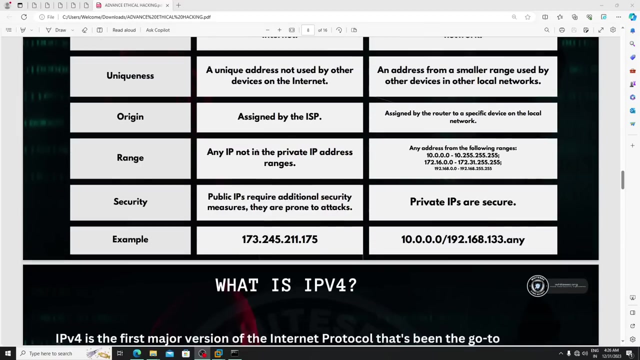 another organization. other organization is there, other network is there? simple, they can able to use the same ip address there, but still i can't able to communicate with that. okay, this is the thing: origin assigned by the isp, assigned by the router to a specific device on the local network range: any ip not in the private. 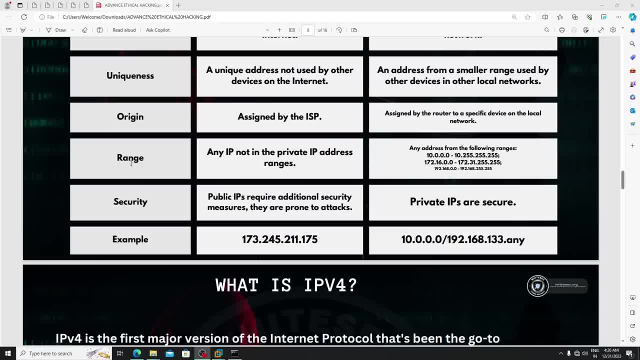 ip addresses range and here range. see in. this is a very important just focus here. private ip: any address from the following ranges: 10.10, 10.0.0.0. and here 10.25, uh, 255.255.255, see if you, if you are. 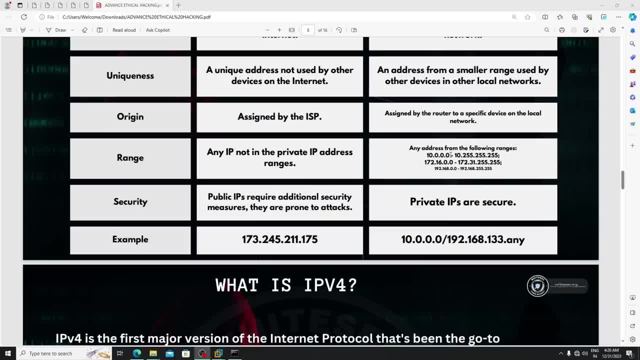 using the virtual machines, then you can able to. not virtual, okay, virtual box. sorry, if you are using the virtual box, you just booted the kali machine in your virtual box. at that time you can able to see your ip addresses. uh, the your local ip will start with 10.. okay, uh, mostly the the smaller. 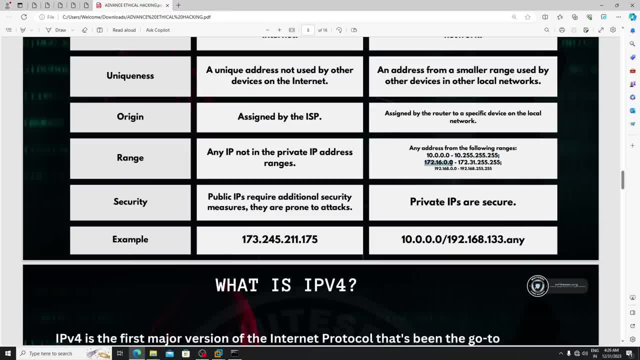 organizations use this thing: 172.1, 16.. okay, assume that if you see any ip is starting with 172, .60, 16.. uh, something like that, from here to here, then it's a. it comes under local ip address. now, right now we are in in our kali machine also. we are using this thing. okay, 192.168. 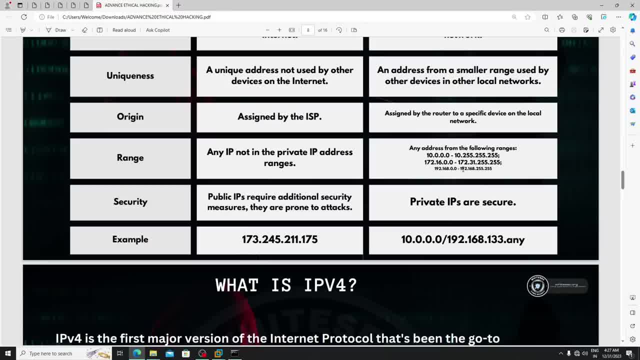 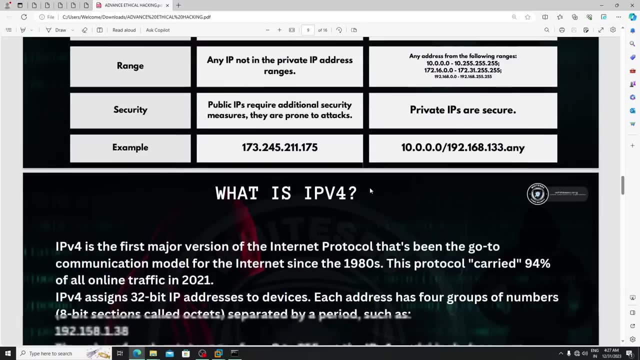 okay, you are, uh, mostly your, your local machines will comes under these ranges. okay, this is the thing now here. see, mostly you guys can able to see this range in banks if, if, uh, in local network, okay, like it, start with 10.. uh, maybe there is a one bank i don't want to tell. okay, just just leave it. 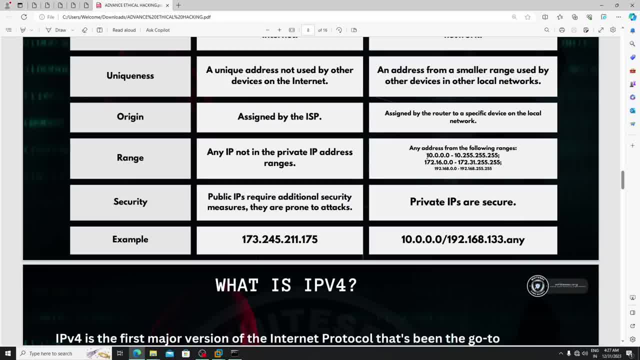 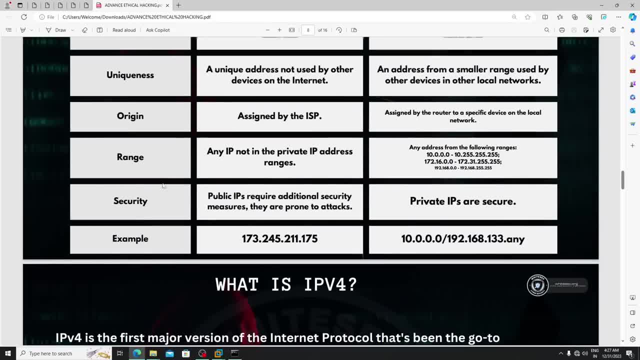 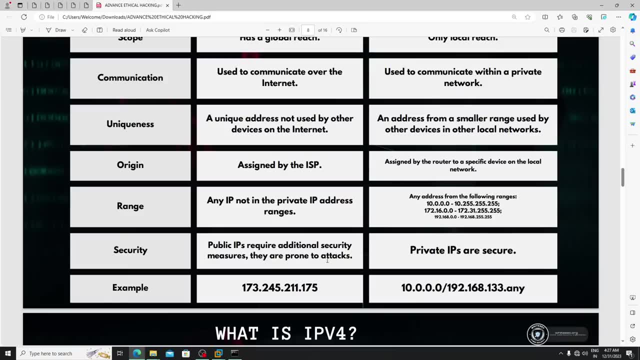 okay, right, and also hospitals as well. they- they use a 10 range. okay, from they start with 10.. and security and in security, public ip: ip requires additional security measures. they are prone to attacks like they need to add a kind of firewalls in their public ip addresses. this is the thing. 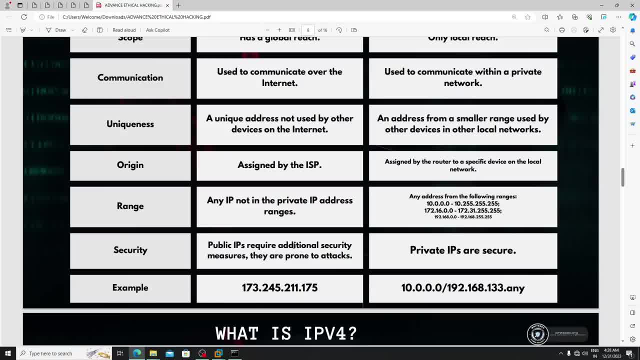 okay, because it's a state-of-the-art system. so it's a state-of-the-art system. it's a state-of-the-art static right. any, if i got that ip address, i can able to perform the attacks on it. i can. mostly the public ip addresses are little bit vulnerable. okay, if they won't implement the. 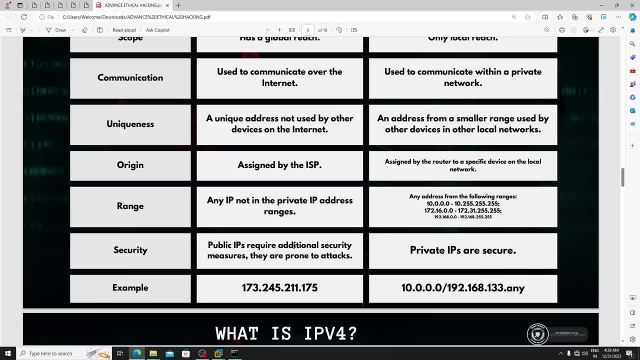 firewall there, then it is, uh, vulnerable. this is a thing, and here, uh, and also the second thing is: if in the server, in the services they are using outdated one, at the time also, the things are there are, chances are there to exploit this public ip address. now the private ips are secure. 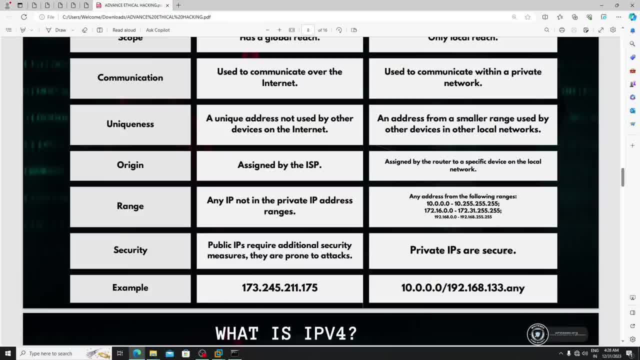 this is the thing, because it will change. this is the thing, and also it is running in local network. assume that if i, if any attacker, want to exploit the public, private ip, then first he need to come to my network and he need to exploit it. okay, this is the thing, first he need to have in a simple 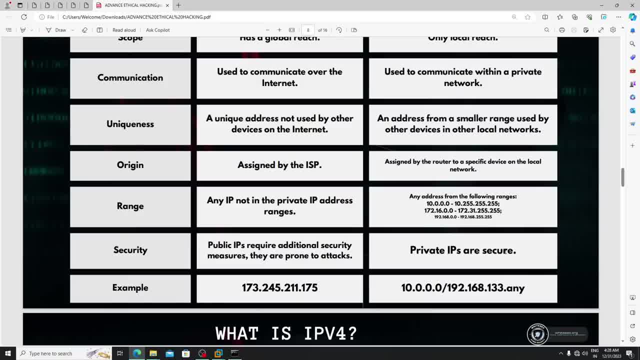 version first. first he need to have the wi-fi network, then he need to uh, come in that network and he just need to exploit it. okay, this is the thing. okay, don't worry, you will get it, just just try to run your windows. but for now it is very simple. you don't need to go through all the same process. 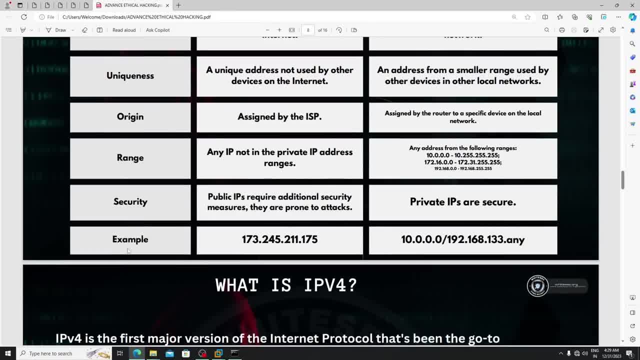 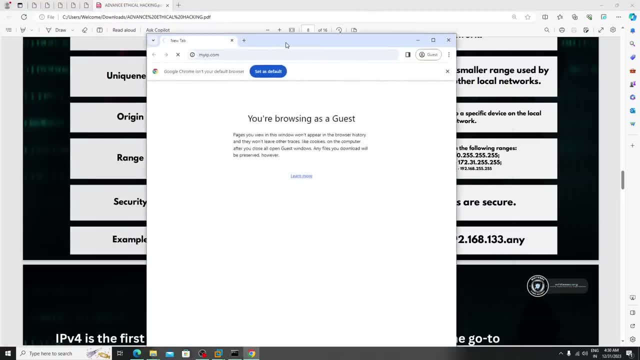 okay, but for now, because of windows, penetration, testing, training. okay, there, i just covered each and everything about this, all things okay. okay, now here is a example. uh, the public ip address look like this: okay, let me show you. just wait the search for myipcom. this is my public ip, okay, 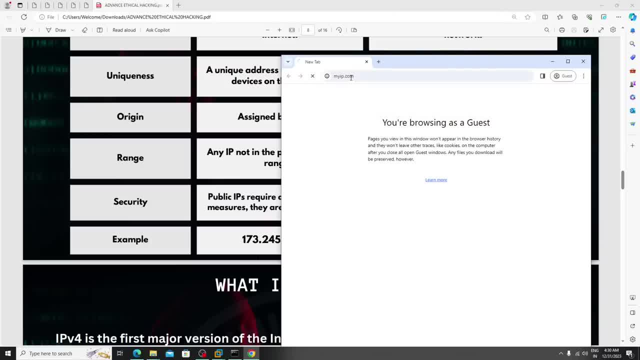 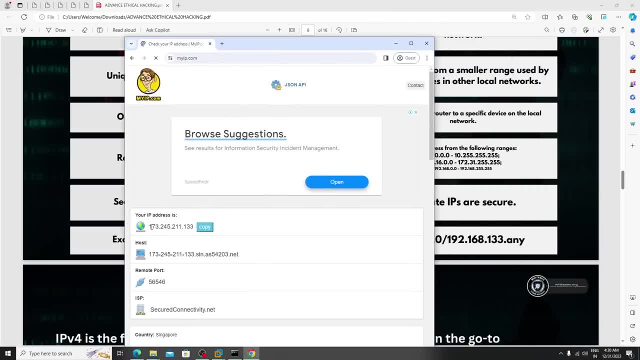 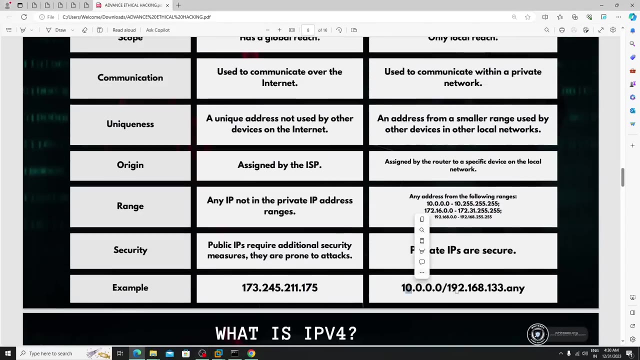 here it is. this is my ip address. right, this is a public ip. anyone can able to ping it. anyone can able to scan this ip. anyone can able to see which port is open, which port is closed by using nmap or something like that. okay, this is a thing now the local ip. you can't able to access it, just. 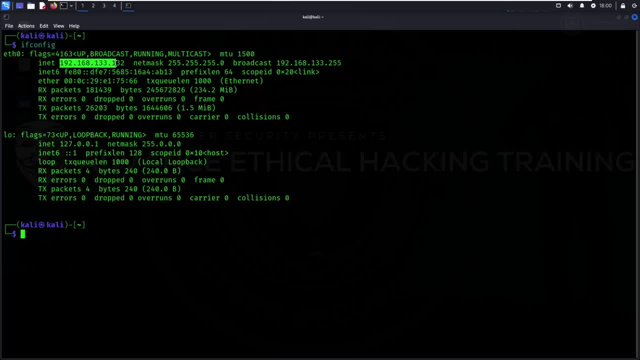 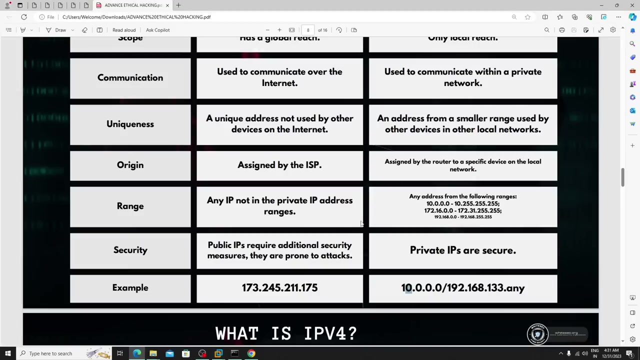 just as is this machine. you can't okay this. just copy, just type this, just perform the nmap scanning on this ip address. you can't do that, okay, because if you want to perform it then you must be in my network. okay, this is the thing, so hope you guys get it. the difference between the public and 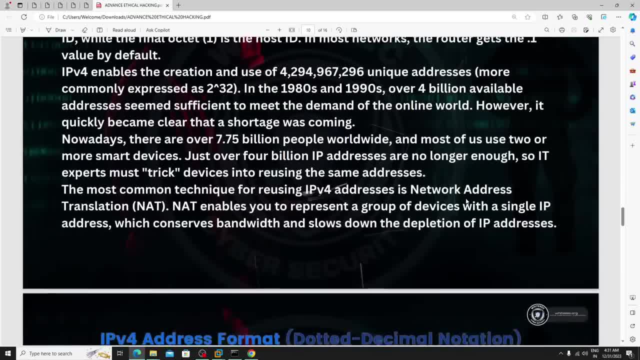 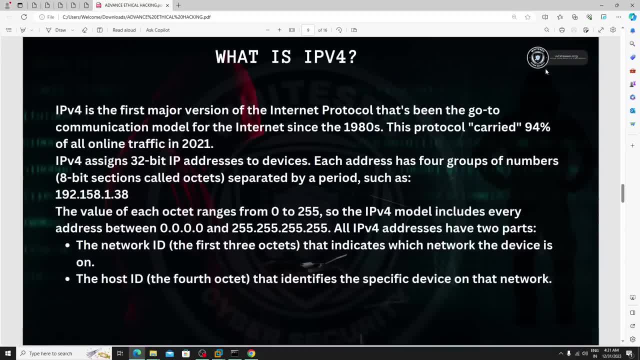 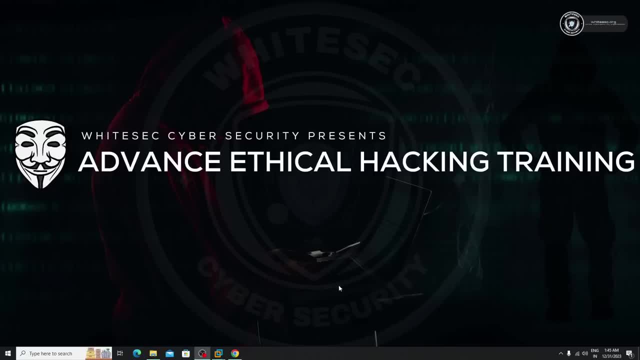 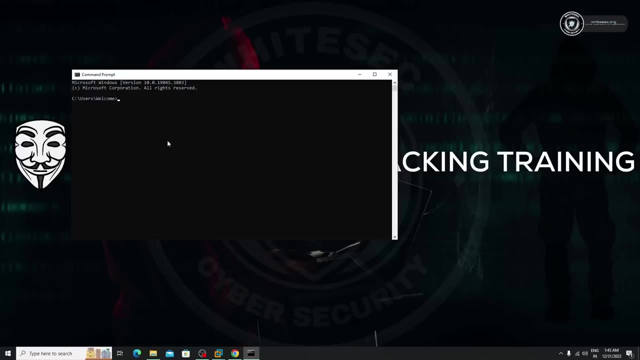 private ip addresses. in the next classes we are learning about ipv4 and ipv6. okay, this is a huge topic, just wait. okay, in the next class we will learn these things. hello guys, hope you are fine. in this class we are learning about ip address. now let me tell you. first of all, let me show you if i open cmd here. let me open cmd and if i type: 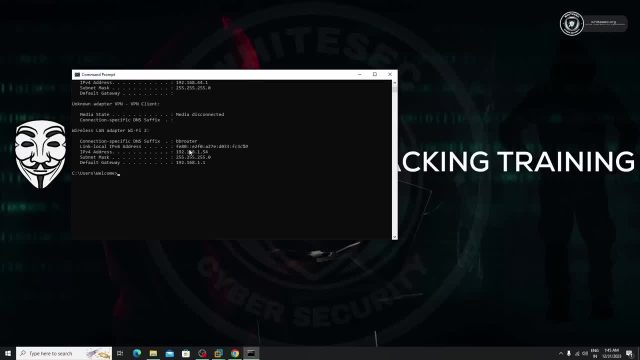 ipconfig. here you guys can able to see there is a ipv4 address. it's look like 192.168.1.54. basically, what is this? it's my local ip, or you can also say it as a private ip. it's my local ip, or you can also say it as a private ip. it's my local ip, or you can also say it as a private ip. 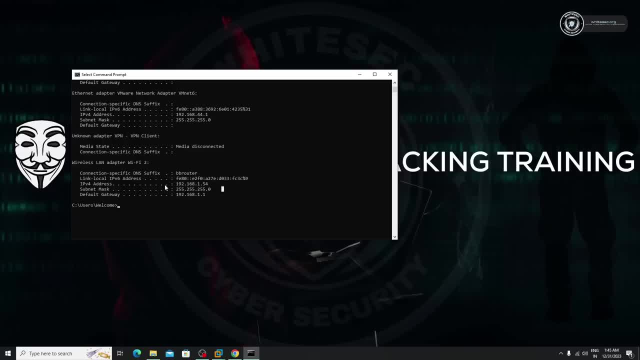 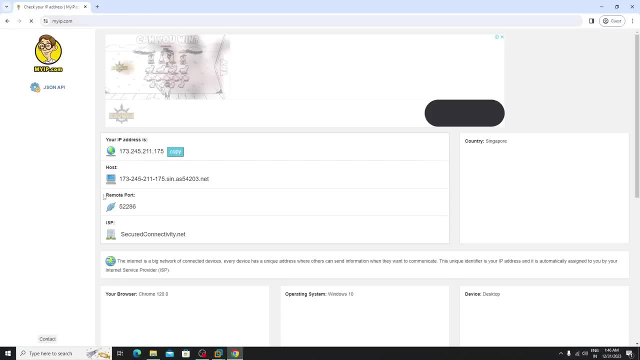 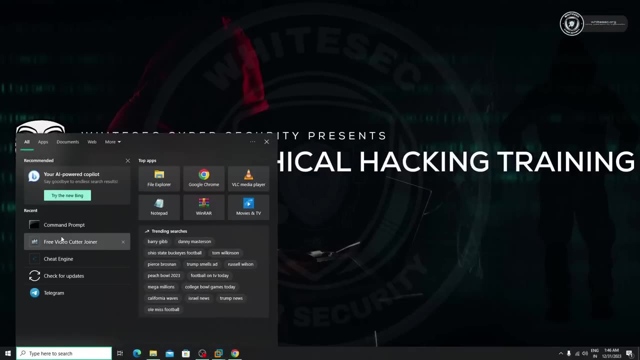 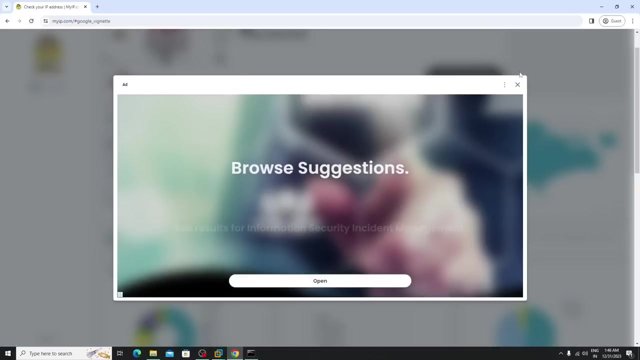 just focus on, just remember this- words: private or local. okay, now, if i open the browser and if i type myipcom, and here you can able to see, this is my system ip. okay, this is my private ip. this is my private ip. okay, this is my public ip. simple, just open the cmd, just type ping and just paste this ip. 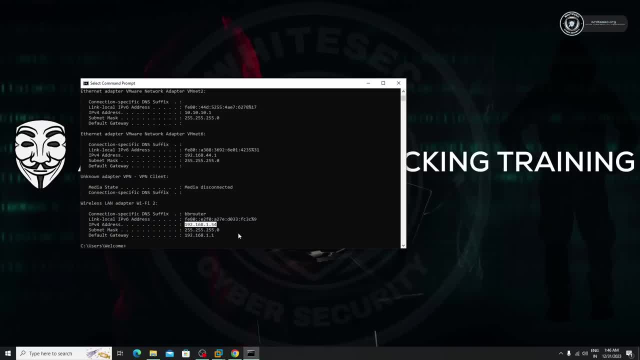 you can't able to ping this. okay, if in your network, in your local network, if you have this ip, then you can able to ping, but you can't ping this system. now, okay, that you can't able to ping this system by using my local ip address or private ip address, because i'm gonna tell you 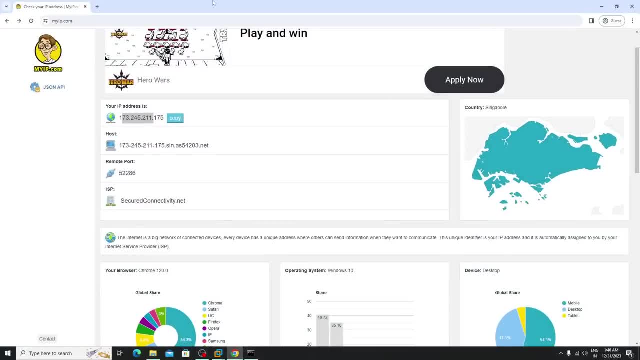 why we can't able to ping it. okay, but you can able to ping it. you can able to check this ip is live or not. okay, just see this ip address. this is my public ip. okay, you can able to ping it. it's not a big deal for you because the 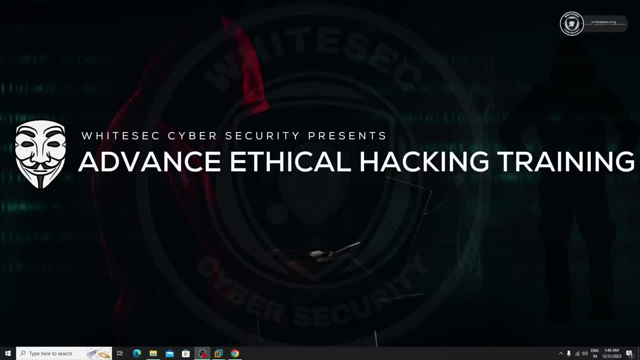 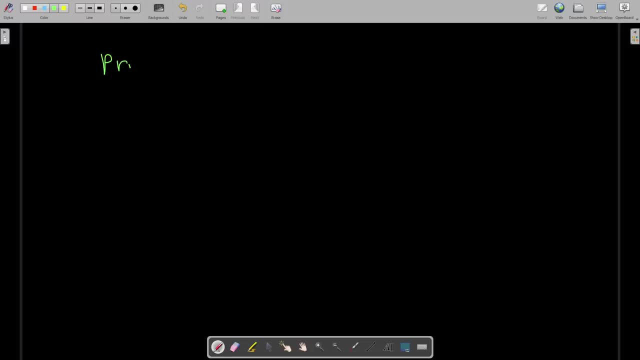 that is a public ip. now just let me explain you here. what is these things you just learn about what here i just showed you about private ip, which is also known as a local ip. okay, and it is another thing which is public ip. now let me tell you about the public ip. 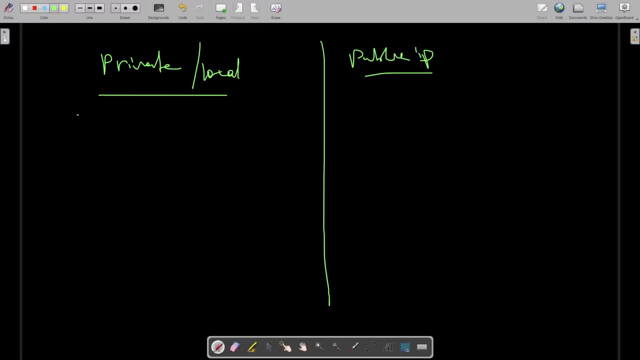 and private ip. see private. the private ip is a, known as a. what? uh, it's the first point. it's a. it's a local ip, local ip, the simple thing is only the systems which are in our network, in our wi-fi network, can able to ping it or can able to access it. see, here, there is a router. okay, the wi-fi router. 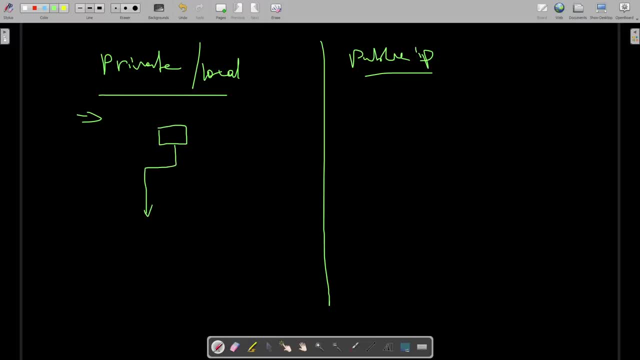 now, with this router, there are different devices are connected, like android or any pc- okay, or any, anything. any device which is, which is used to, which is connect with internet, okay, any iod device, anything. camera, okay, now here, this, this, all devices. okay, just let me take camera like this. 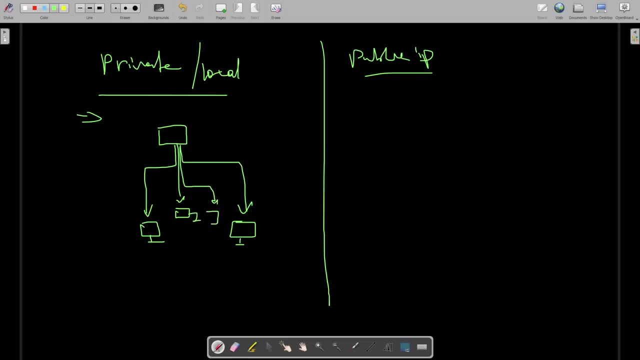 and let me use android and let me use printer as well. okay, every this devices are connected with the same wi-fi network. now, these guys will have the local ip. the router will provide the local ip addresses to these machines. okay, now, now, here the thing is local ip. look like this thing: 192.168.133 point, something like that, okay. 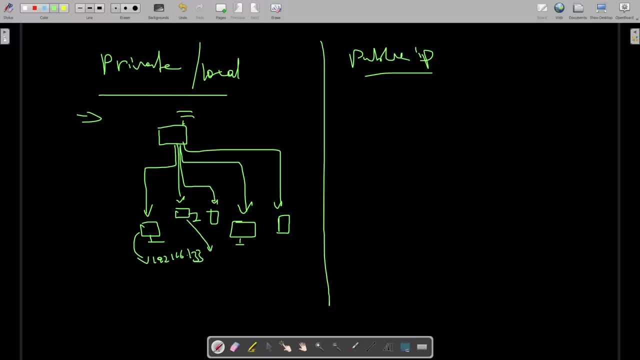 it's how it's. unique ip address: okay, like the, the things will start with 192 only okay, 192 point. it's totally depend upon the organization what they are using. if the organization is big, then they they use 192, okay. if the organization is small, then they they use uh, 172 or something. 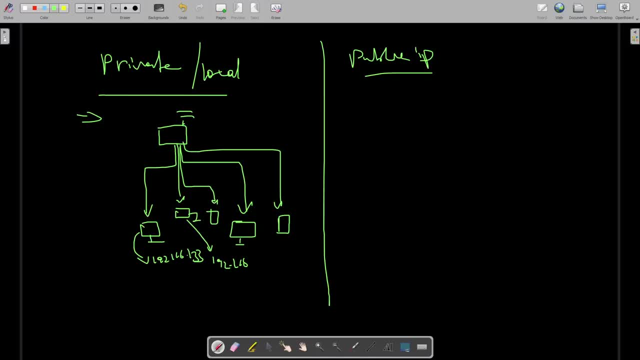 like that. okay, it's not a big deal, you can able to see. okay, once you connect with the, the internet, the, the victim or any wi-fi network, you guys can able to see the ip here. okay, i just showed you right in kali linux also, after typing the if. 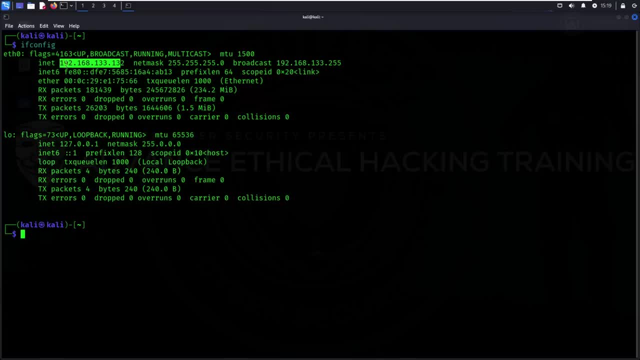 config, i can able to see the same thing. uh, the ip address here, which is local, which is starting with 192.168.133. just focus here. just let me open the cmd. okay, this is my windows machine terminal. okay, cmd, if i type here: ip config. this is my windows machine terminal. okay, uh, cmd, if i type here: ip config. 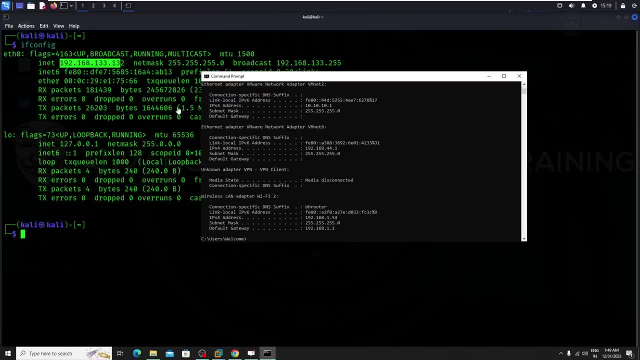 just see the things are very similar here. 192.168- just see it's also starting with 192.168. basically, it's a nothing but. uh, i can able to. this machines can able to ping each other, okay, like they can able to share the file, something like that. basically, these guys are in the same. 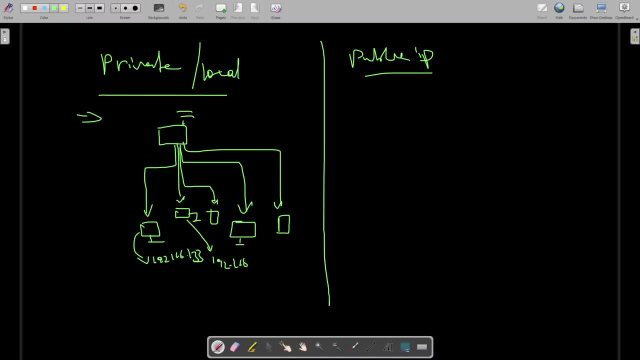 network. okay, they can only access each other. okay, assume that there is one server is running on the local network at that time. they can able to access this server. okay, they assume that the in this server the website is running at a time, they can able to access it only these guys. 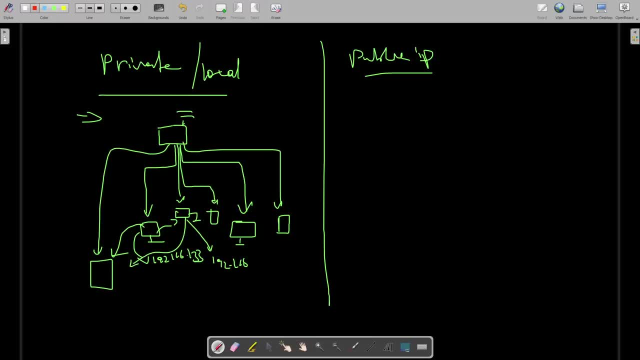 assume that there is a public, okay. uh, there is one guy who is not connected with this machine, this, this wi-fi network at that time. he can't able to ping this ip addresses, he can't able to access the camera, he can't able to access the printer or something like that. the server- okay. 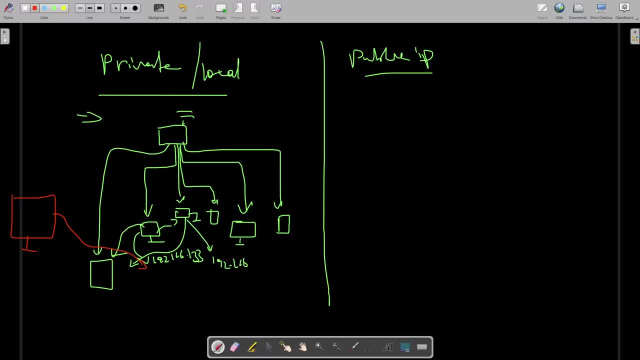 this is a thing. basically, here, the local, uh, or private network will only work with the users who are connected with that network. okay, with that wi-fi network, this is a thing. the same case if you know about android hacking also just focus, uh, if you know about android hacking or any system you know. 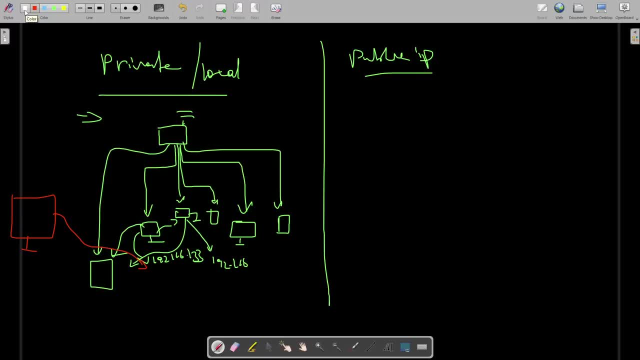 how to hack the system or something like that. then they're all in, i think, in basic ethical hacking training- i just covered these things okay- which is available on youtube channel. see there, what happened means i just told you. assume that just just let me use this one. see, i just told you there what the simple thing is. 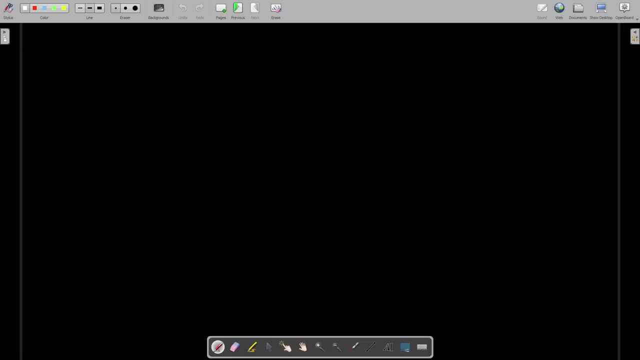 if there is a victim. okay, if i want to hack, first of all let's, let's focus on: uh, let me explain you like this. so let's say: if i want to hack, let me explain you like this. so let's say: if i want to hack, 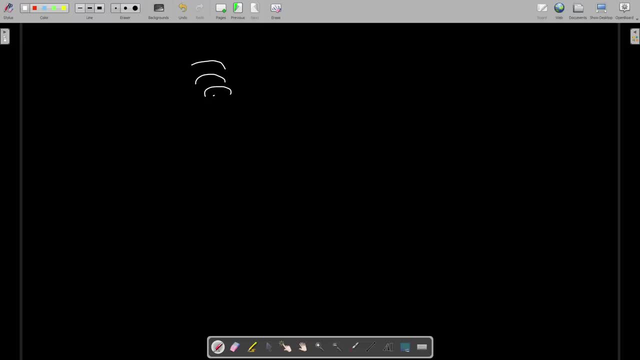 like this: see, there is a wi-fi network, okay, like this: see, there is a wi-fi network, okay, like this: see, there is a wi-fi network, okay, now. now, now, this is my attacker machine, this is my attacker machine. this is my attacker machine. i'm doing this attack locally. what is? 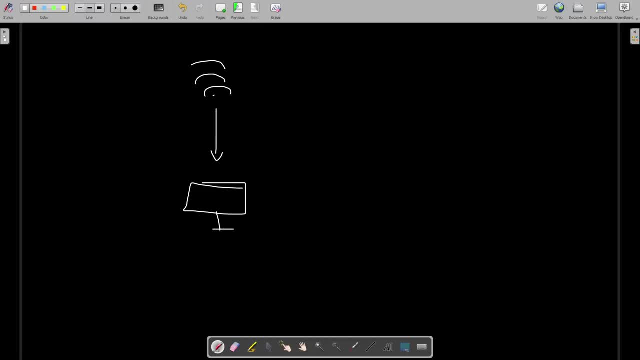 i'm doing this attack locally, what is? i'm doing this attack locally, what is locally now you will get it see locally now. you will get it see locally now. you will get it see. i just generated one payload, okay, which. i just generated one payload okay, which. 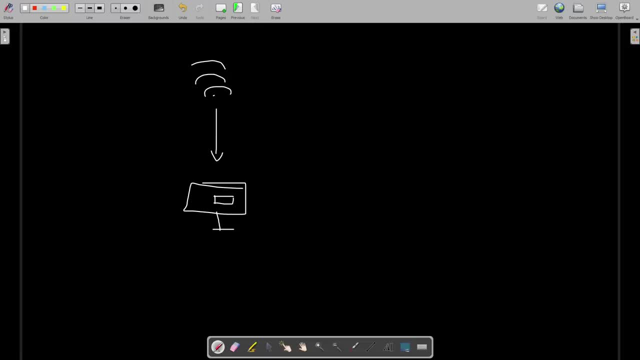 i just generated one payload okay, which is by using this i can able to hack any is by using this i can able to hack any is by using this i can able to hack any android device or any pc: now simple android device or any pc: now simple. 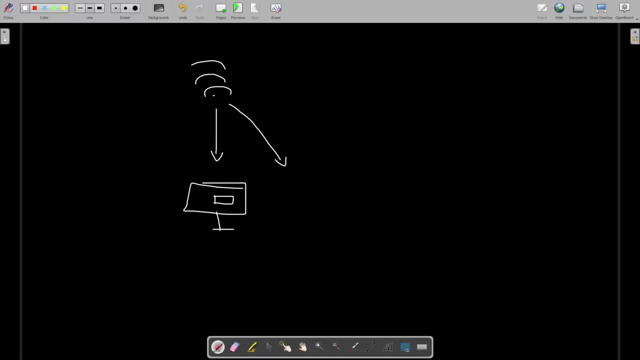 android device or any pc. now, simple: my target, my victim. okay, i want to hack my target, my victim. okay, i want to hack my target, my victim. okay, i want to hack my network with my wi-fi network, at that. my network with my wi-fi network, at that. 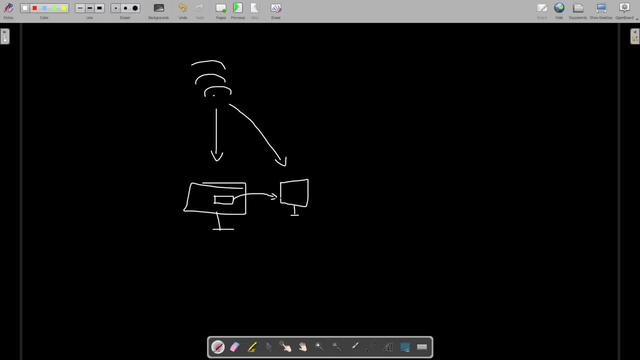 my network with my wi-fi network at that time, if i send the payload to this guy time, if i send the payload to this guy time if i send the payload to this guy, he can able to. i can able to get the. he can able to. i can able to get the. 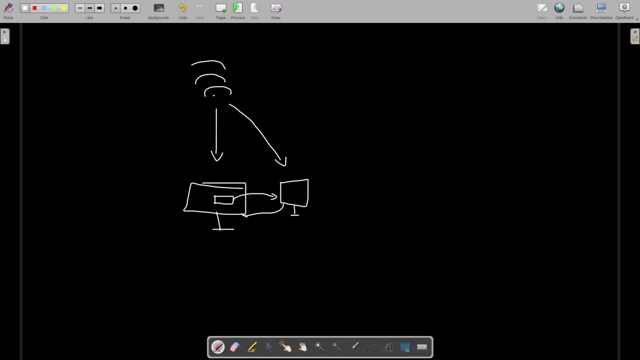 he can able to. i can able to get the connection. i can able to hack him. okay, connection, i can able to hack him. okay, connection, i can able to hack him. okay, assume that. assume that. assume that. okay, he just disconnected with my wi-fi. okay, he just disconnected with my wi-fi. 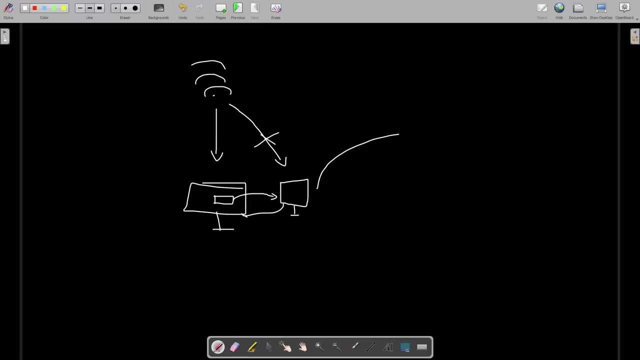 okay, he just disconnected with my wi-fi network network network. okay, and he just moved to different. okay, and he just moved to different. okay, and he just moved to different location. location, location, different location. or he is using his mobile data or he is using his mobile data. 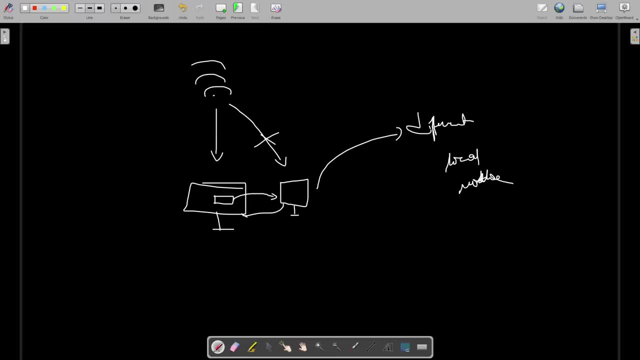 or he is using his mobile data. at that time, i can't able to hack him. at that time, i can't able to hack him at that time. i can't able to hack him because, because, because, the simple thing is: i use the local ip. the simple thing is, i use the local ip. 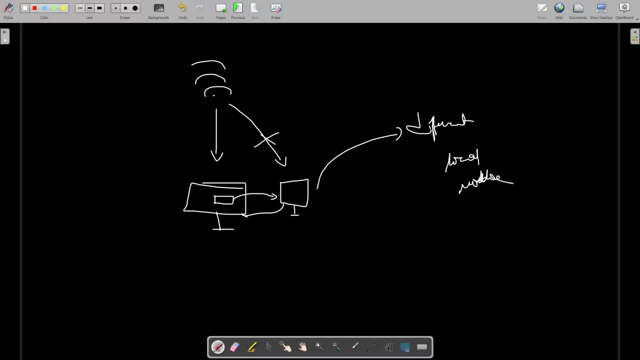 the simple thing is i use the local ip address there. address there. address there: okay, which ip? i just told you about the? okay, which ip? i just told you about the? okay, which ip? i just told you about the local ip. i just use this ip addresses ip. 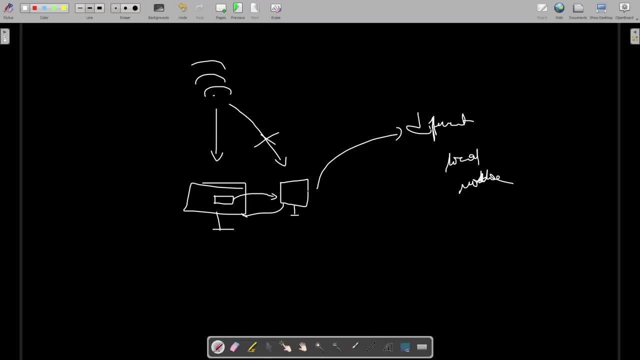 local ip. i just use this ip addresses ip. local ip. i just use this ip addresses ip address to generate the payload and to address to generate the payload and to address to generate the payload and to send it. okay, if we connect with my wi-fi. send it okay if we connect with my wi-fi. 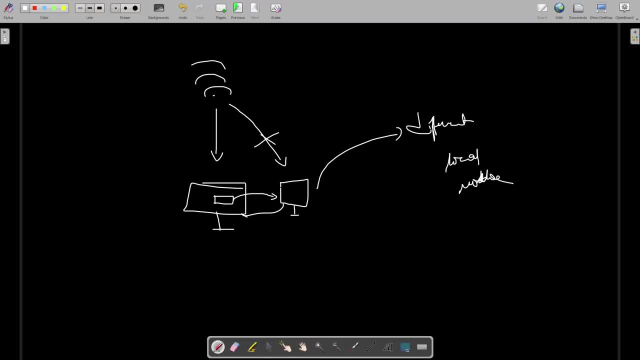 send it. okay, if we connect with my wi-fi network, only i can able to hack him network. only i can able to hack him network. only i can able to hack him. this is a thing. this is a thing. this is a thing. right assumed that. right assumed that. 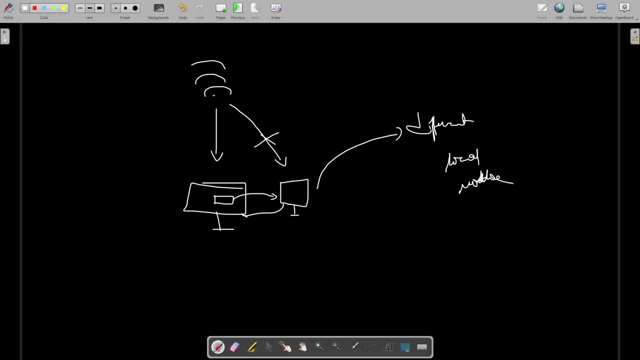 right, assumed that again i am saying he just disconnected. again i am saying he just disconnected. again i am saying he just disconnected from my wi-fi network and you just move from my wi-fi network and you just move from my wi-fi network and you just move to some other place. 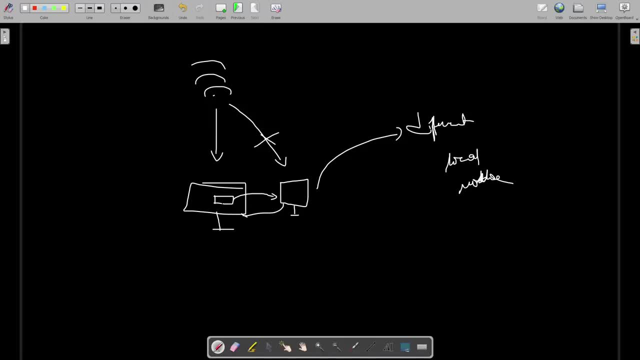 to some other place, to some other place at that time. what i need to use instead at that time? what i need to use instead at that time? what i need to use instead of local ip, i need to use of local ip. i need to use of local ip. i need to use public ip address, which is this one: 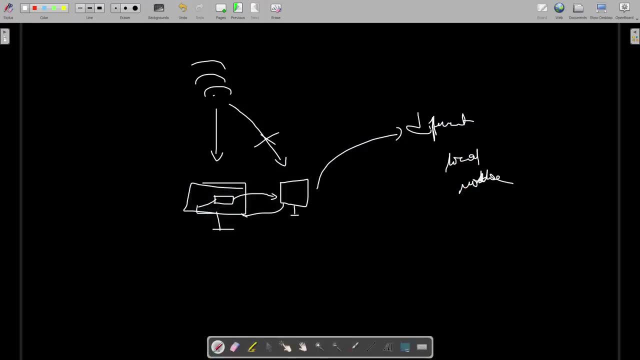 public ip address. which is this one, okay. which is this one, because i just okay. which is this one, because i just okay. which is this one, because i just told you anyone can able to ping, told you anyone can able to ping, told you anyone can able to ping, or anyone can able to access this ip. 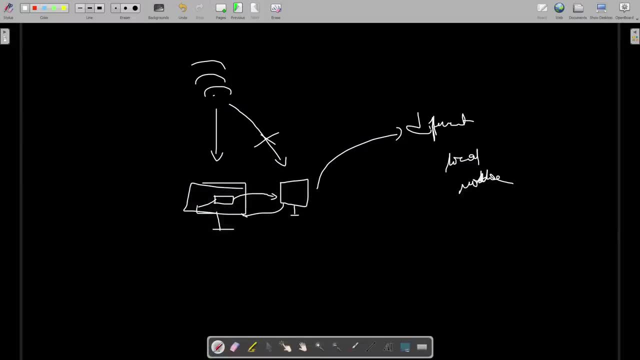 or anyone can able to access this ip, or anyone can able to access this ip. okay, this is the thing. okay, this is the thing. okay, this is the thing. now. uh, if you just disconnected, uh, now, uh, if you just disconnected, uh, now, uh, if you just disconnected, uh, disconnected from network. also, i can. 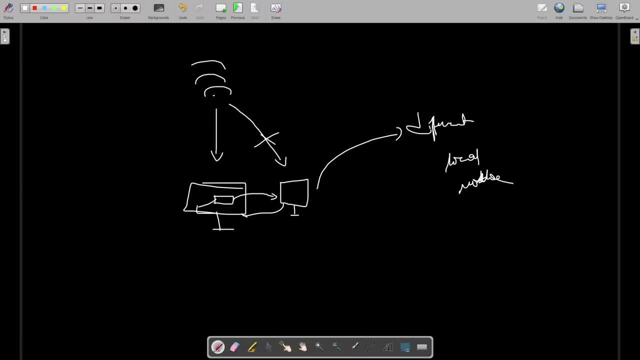 disconnected from network also, i can. disconnected from network also, i can able to able to able to what i can able to control him because i what i can able to control him, because i what i can able to control him because i am using my public ip address there. 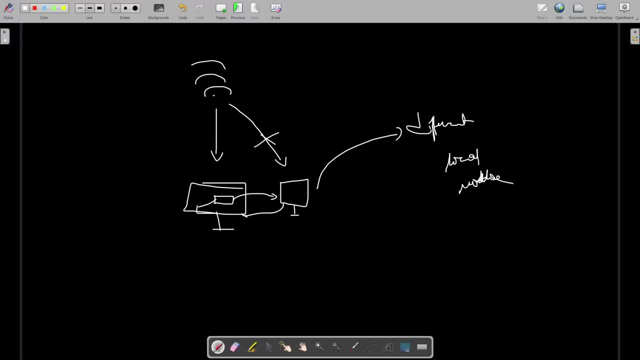 am using my public ip address there am using my public ip address there, which is public, anyone can able to, which is public, anyone can able to which is public. anyone can able to hack your own systems. this, uh, i suggest. hack your own systems. this, uh, i suggest. 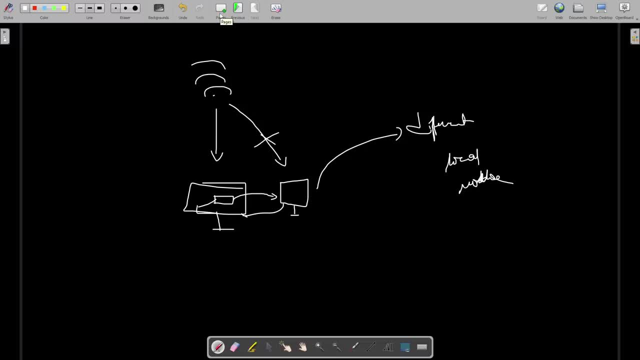 hack your own systems. this, uh, i suggest you these things. okay, just create your you these things. okay, just create your you these things. okay, just create your own lab and hack your own android. hack own lab and hack your own android. hack own lab and hack your own android. hack your own computer machines at that time. 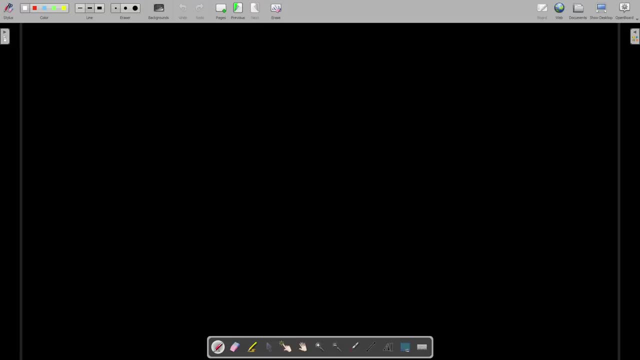 your own computer machines at that time, your own computer machines at that time, you will get it what i am trying to say. you will get it what i am trying to say. you will get it what i am trying to say here. okay, now let's uh again. let's focus on. 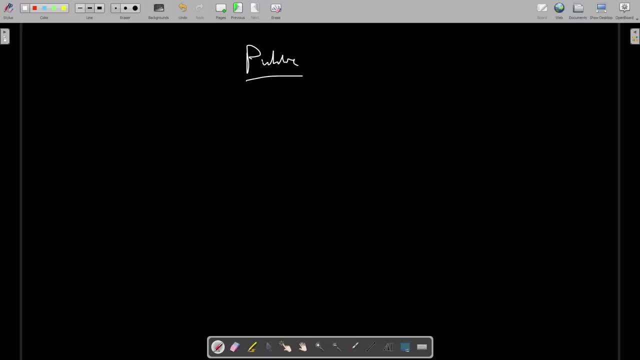 okay, now let's uh again. let's focus on: okay, now let's uh again, let's focus on the public ip here. the public ip here, the public ip here. i just covered about the local ip. okay, i just covered about the local ip. okay, how it's gonna work, the public ip. 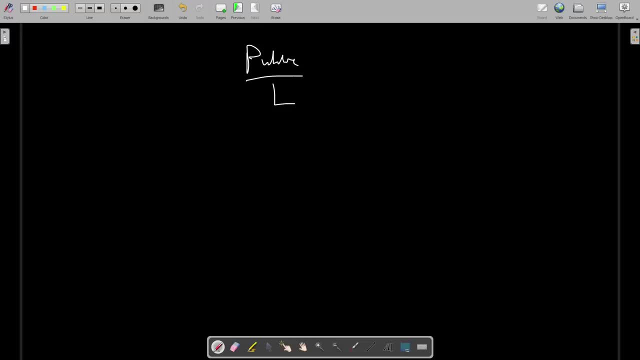 how it's gonna work the public ip, how it's gonna work the public ip. public ip is nothing but public ip is nothing but public ip is nothing. but see, assume that there is uh your office. see, assume that there is uh your office. see, assume that there is uh your office. is there? okay, you just install one. 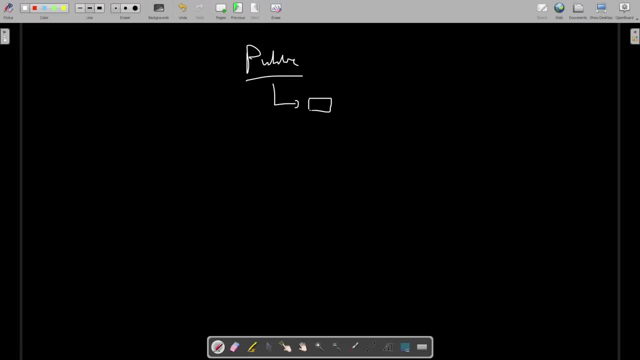 is there? okay, you just install one. is there? okay, you just install one camera there. okay, to spy on your camera there. okay, to spy on your camera there. okay to spy on your employees. or if you want to check employees, or if you want to check employees or if you want to check something, okay, you just install the. 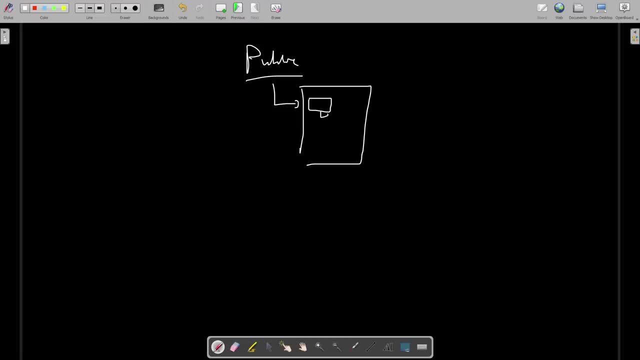 something. okay, you just install the something. okay, you just install the camera there in your office, camera there in your office, camera there in your office. right, right, right, you just install the camera and you just install the camera and you just install the camera and different location. now you want to access this camera. 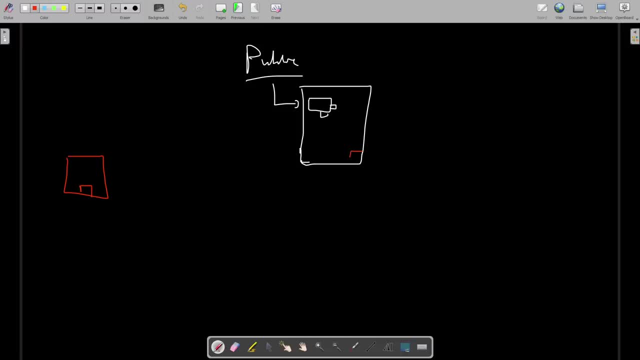 now you want to access this camera. now you want to access this camera. okay, basically, if you, if you are in, okay, basically, if you, if you are in, okay, basically, if you, if you are in office network, you can able to use a office network, you can able to use a. 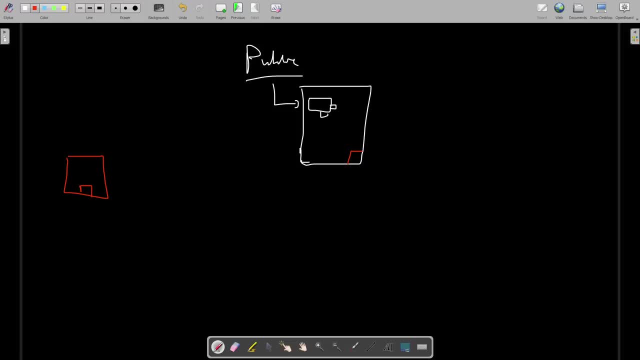 office network. you can able to use a local ip and you can able to local ip and you can able to local ip and you can able to uh see the, uh see the, uh see the. see the things there. okay, but assume that. see the things there. okay, but assume that. 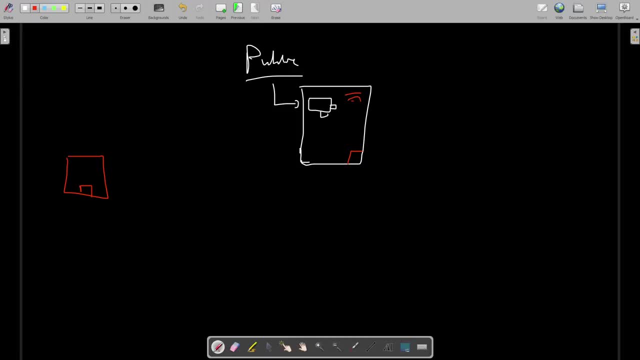 see the things there, okay, but assume that you just disconnected from the office. you just disconnected from the office, you just disconnected from the office network and your, you are in other network and your, you are in other network and your, you are in other location at that time. what you need to 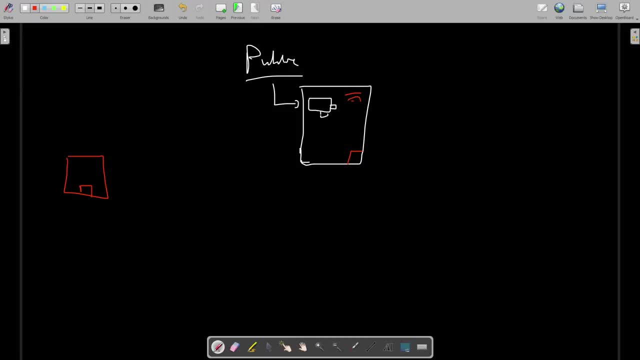 location at that time, what you need to location at that time, what you need to do? simple, the thing is in the camera. do simple, the thing is in the camera. do simple, the thing is in the camera also. you will see the public ip also. you will see the public ip. 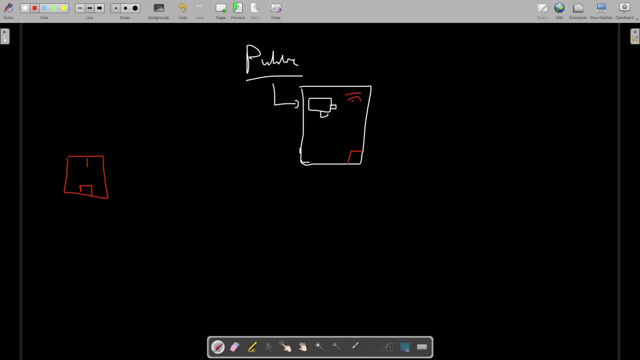 also you will see the public ip. okay, okay, okay, if you uh type the public ip in your, if you uh type the public ip in your, if you uh type the public ip in your search bar, in your search bar, in your search bar, in your- uh the camera application, or something, 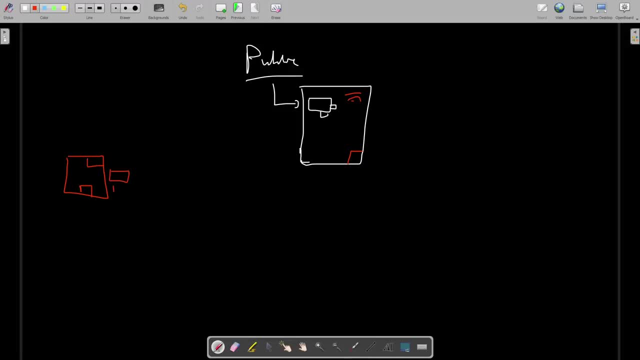 uh, the camera application or something. uh, the camera application or something like that. it will ask for the username. like that. it will ask for the username. like that. it will ask for the username and the password. okay, if you type the and the password. okay, if you type the. 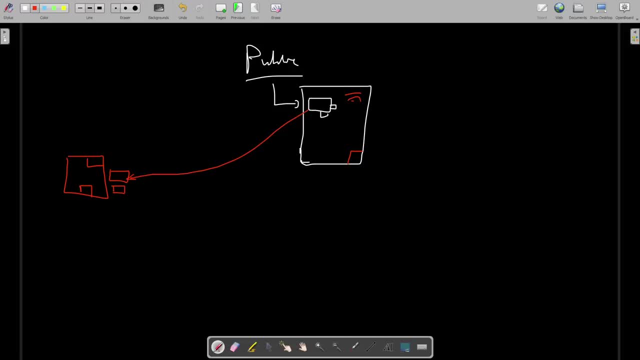 and the password. okay, if you type the username and the password, you can able username and the password. you can able username and the password. you can able to access the. to access the. to access the that that that company camera: okay, this is the thing. this company camera: okay, this is the thing this. 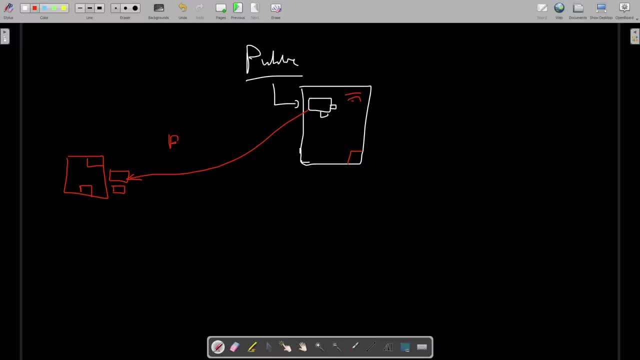 company camera. okay, this is the thing. this is what. this is nothing, but it's a. is what? this is nothing, but it's a. is what? this is nothing, but it's a? public ip. public ip, public ip, okay, okay, okay. public ip. i can able to access this. 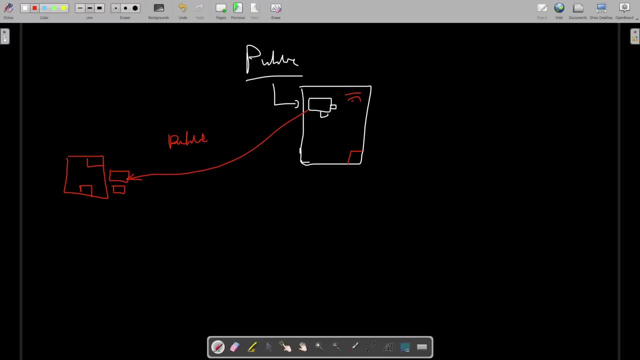 public ip, i can able to access this public ip. i can able to access this camera from any location camera from any location camera from any location, because, because, because this is running on the public ip, mostly this is running on the public ip, mostly this is running on the public ip. mostly the cameras will run on public and 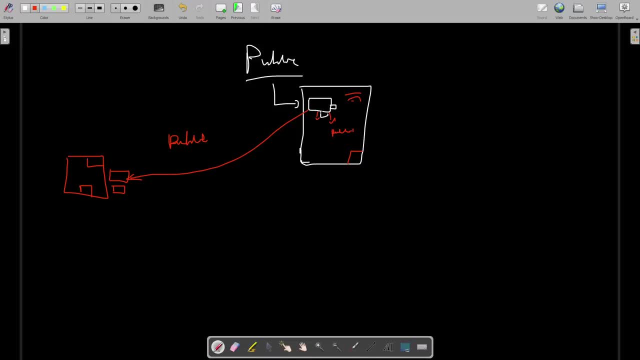 the cameras will run on public and the cameras will run on public and private ips- both okay. it's used both private ips, both okay. it's used both private ips- both okay. it's used both public and private ip addresses. public and private ip addresses. public and private ip addresses- okay. 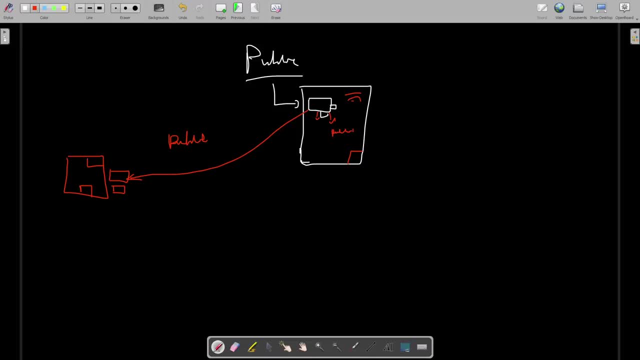 okay, okay, there are some cameras which only use a. there are some cameras which only use a. there are some cameras which only use a private ip address, like they only use a private ip address. like they only use a private ip address, like they only use a local ip. 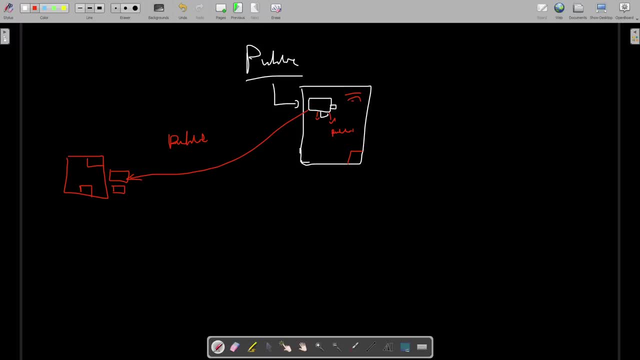 local ip, local ip. if you want to access those cameras, if you want to access those cameras, if you want to access those cameras, then you need to connect with that, then you need to connect with that, then you need to connect with that network and you can able to access it. 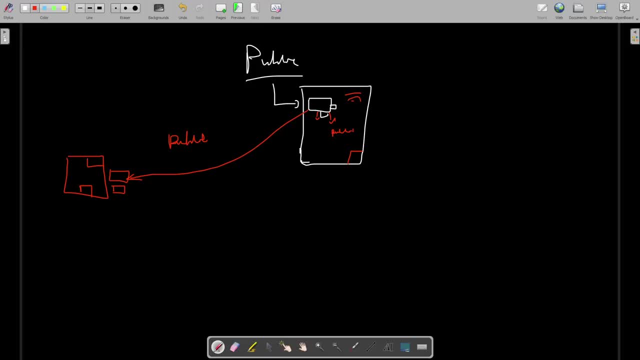 network and you can able to access it. network and you can able to access it. still you need to type the username and still you need to type the username and still you need to type the username and the password there, mostly, the password there, mostly the password there, mostly. let me tell you, this is a half topic. 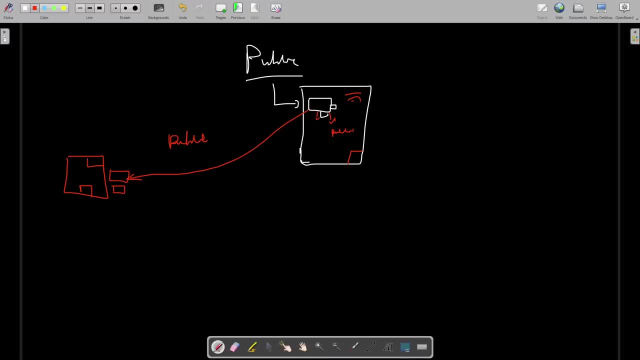 let me tell you this is a half topic. let me tell you this is a half topic, mostly in user. okay, like there is a form, mostly in user. okay, like there is a form, mostly in user. okay, like there is a form is there right once you type the. 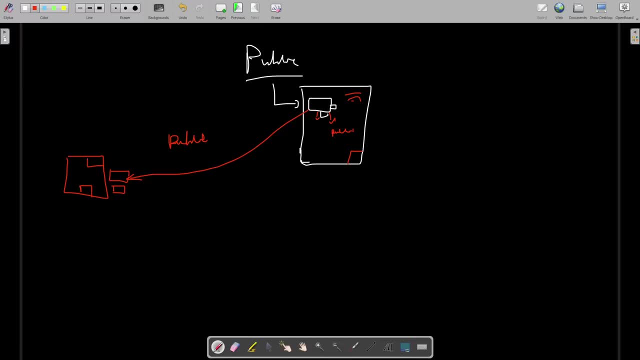 is there right once you type the. is there right once you type the public ip there. public ip there. public ip there. it will ask for the username and the. it will ask for the username and the. it will ask for the username and the password. mostly the vulnerabilities are: 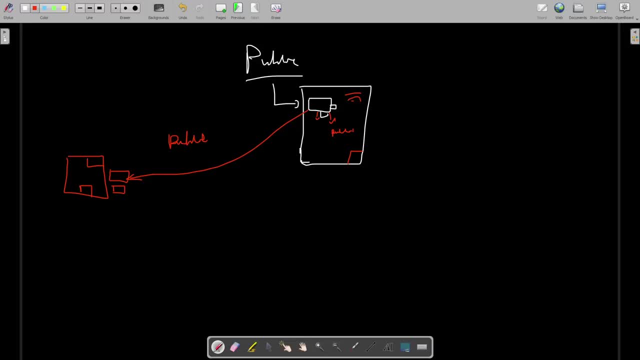 password. mostly the vulnerabilities are password. mostly the vulnerabilities are there there. okay, you can. mostly you can there there. okay, you can, mostly you can there there. okay, you can mostly you can able to bypass the camera. able to bypass the camera, able to bypass the camera, these things if they are using any kind. 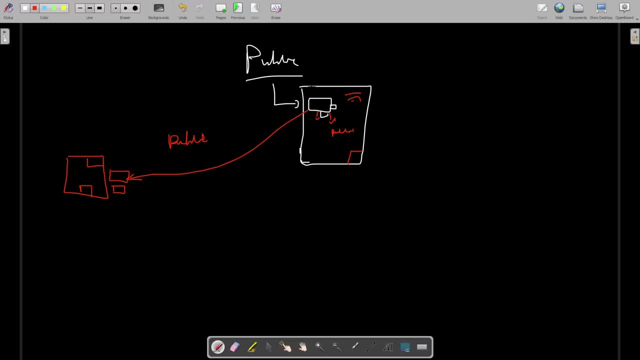 these things. if they are using any kind these things, if they are using any kind of outdated versions of outdated versions of outdated versions for time, you can able to bypass the login for time. you can able to bypass the login for time. you can able to bypass the login as well. but this is a hot topic, okay. 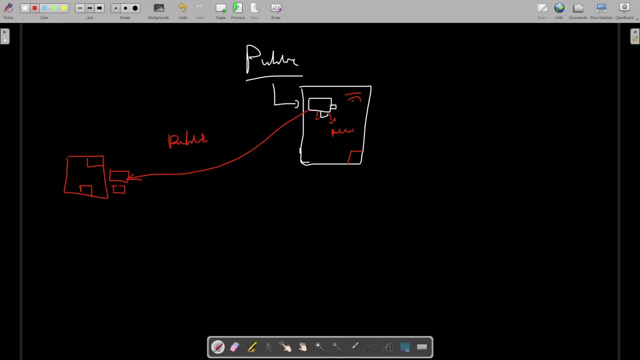 as well, but this is a hot topic. okay as well, but this is a hot topic. okay, now here. hope you guys get it okay, like now here. hope you guys get it okay, like now here. hope you guys get it okay like from any location, from anywhere i can. 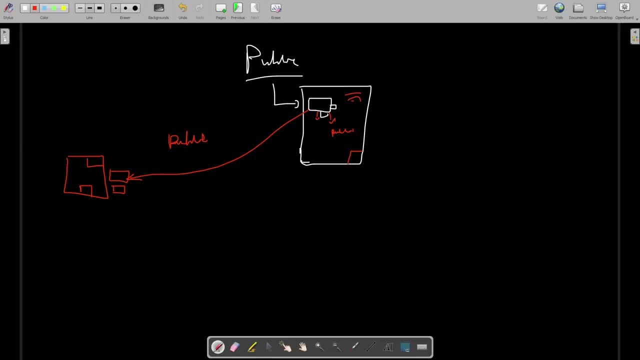 from any location, from anywhere i can, from any location, from anywhere i can able to access the able to access the able to access the camera because i have the public ip camera, because i have the public ip camera, because i have the public ip. okay, okay, okay. this is the thing. 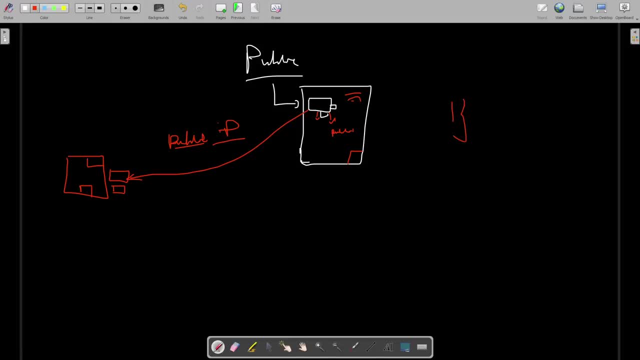 now the thing is again, i am saying ip. now the thing is again, i am saying ip. now the thing is again, i am saying ip address is placed like a name. okay for address is placed like a name. okay for address is placed like a name. okay for uh systems. any, okay, any device which is 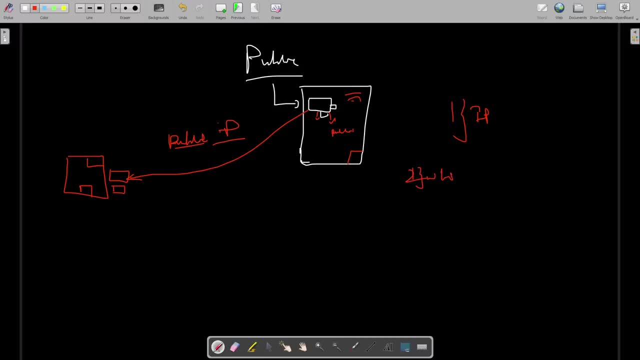 uh systems, any okay, any device which is uh systems, any okay. any device which is connected with sorry, which is connected, connected with sorry, which is connected, connected with sorry, which is connected with internet. how their own unique ip address, how their own unique ip address, how their own unique ip address, unique, i am saying here unique, okay, like 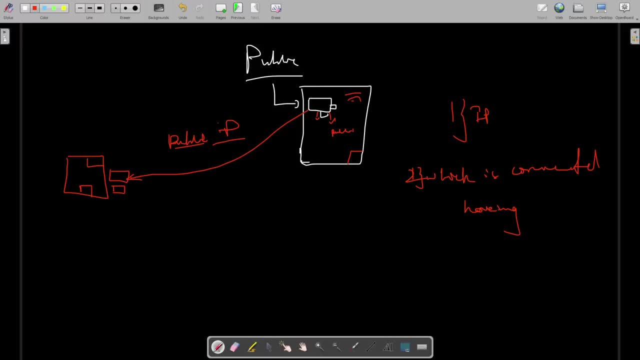 unique. i am saying here: unique, okay, like unique. i am saying here: unique, okay, like, not like a name. human being name. it's a not like a name. human being name. it's a not like a name. human being name. it's a unique. okay, like i just told you one. 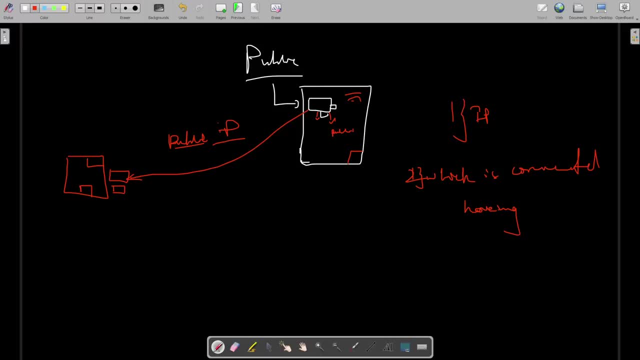 unique, okay, like i just told you one unique, okay, like i just told you one. scenario like right. uh, the example about scenario like right. uh, the example about scenario like right. uh, the example about the john, the john, the john. okay, in any location there are same, uh. 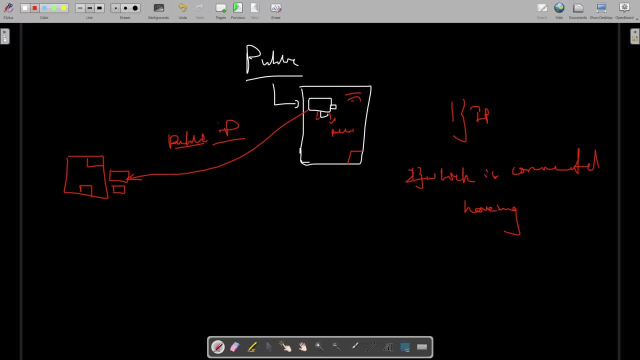 okay, in any location there are same. uh. okay, in any location there are same. uh, there are users with the same names. there are users with the same names. there are users with the same names. right, but in system in this ip address. right, but in system in this ip address. 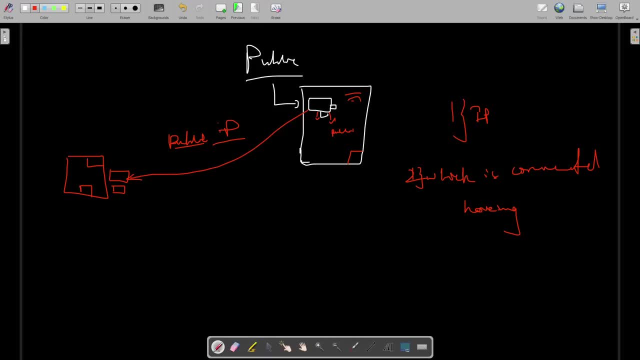 right, but in system, in this ip address, you won't see that. okay, you won't see that. okay, you won't see that. okay, it's how every system, it's how it's you, it's how every system, it's how it's you, it's how every system, it's how it's you know, in this classes we are learning. 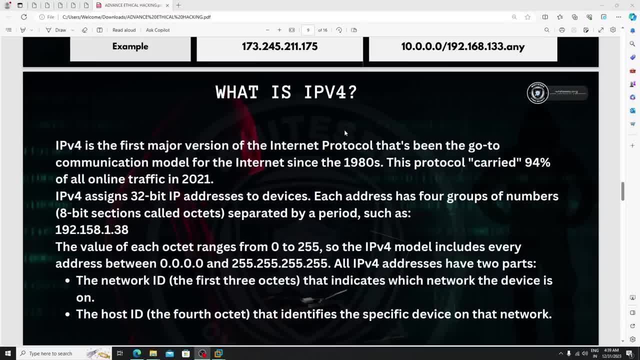 know in this classes we are learning know in this classes we are learning about ipv4, about ipv4, about ipv4- internet protocol version 4. ipv4 is a internet protocol version 4. ipv4 is a internet protocol version 4. ipv4 is a first major version of internet protocol. 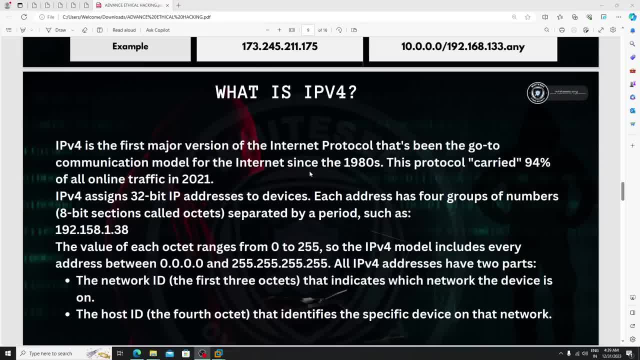 first major version of internet protocol, first major version of internet protocol. that's been the go-to communication. that's been the go-to communication. that's been the go-to communication model for the internet since 1980s. model for the internet since 1980s. 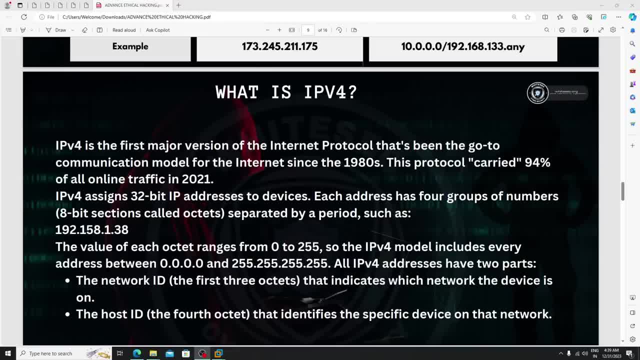 model for the internet since 1980s. the protocol carried 94 percent of all. the protocol carried 94 percent of all. the protocol carried 94 percent of all online traffic in 2021. this is the thing: online traffic in 2021. this is the thing. 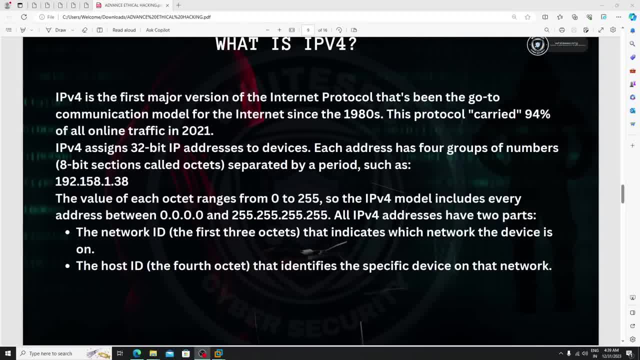 online traffic in 2021. this is the thing. okay, uh, ipv4, assign 32-bit ip address. okay, uh, ipv4 assign 32-bit ip address. okay, uh, ipv4 assign 32-bit ip address. ip addresses to devices. right now, i just. ip addresses to devices. right now, i just. 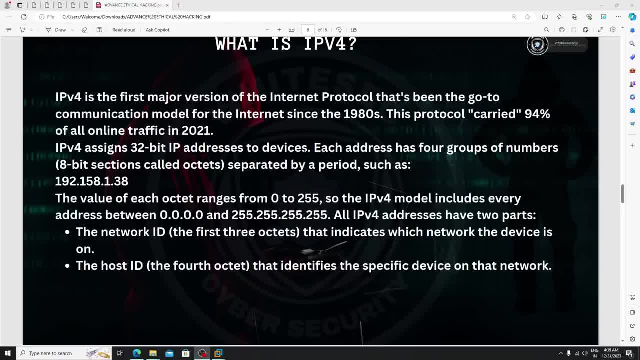 ip addresses to devices right now. i just showed you in the last classes, i just showed you in the last classes. i just showed you in the last classes. i just showed you the. showed you the. showed you the public ip right- public ip, private ip. public ip right, public ip, private ip. 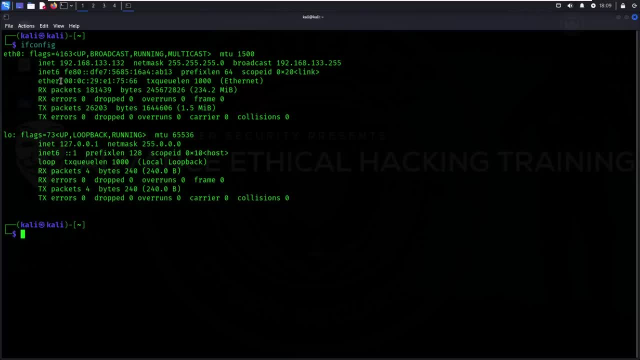 public ip right, public ip, private ip- it's stored it's. it's basically: it's a. it's stored it's. it's basically it's a. it's stored it's. it's basically it's a: ipv4- okay, say ipv4, ipv4- okay, say ipv4. 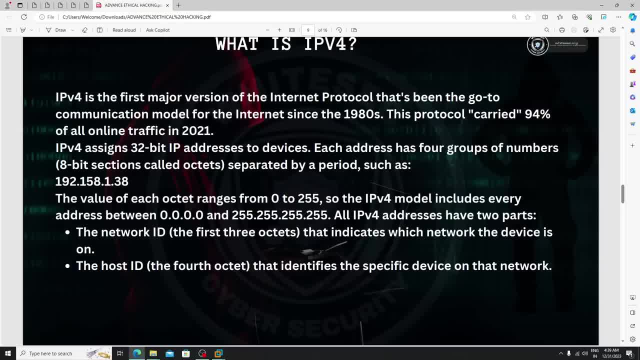 ipv4. okay, say ipv4 right, uh, right, uh, right, uh. where it is ipv4 assigned 32-bit ip. where it is ipv4 assigned 32-bit ip. where it is ipv4 assigned 32-bit ip. addresses to device devices. each address addresses to device devices. each address. 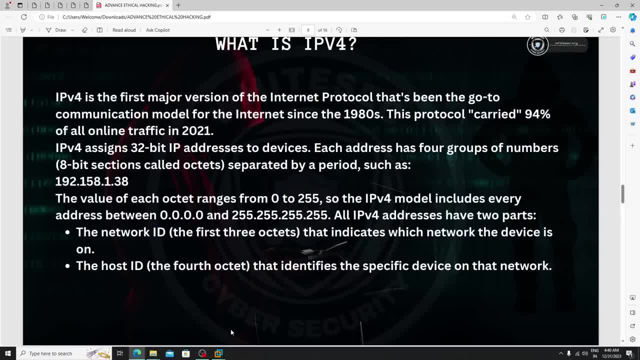 addresses to device devices. each address has four groups of members. okay, what is has four groups of members? okay, what is has four groups of members? okay, what is this? four groups, these things, this four groups, these things, this four groups, these things. one, one, one, two, two, two, three. 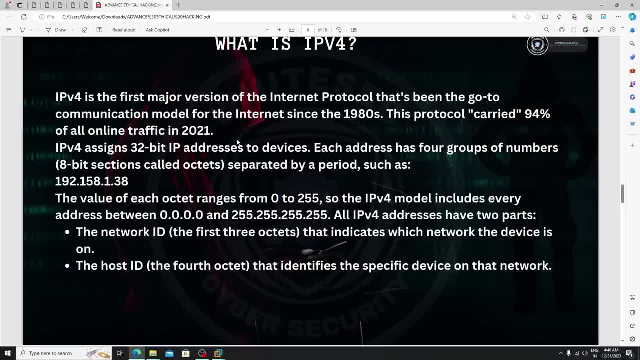 three, three, four, okay, hope you guys get it. four: okay, hope you guys get it. four: okay, hope you guys get it. basically, these are the groups: 8-bit section called octets, separated by. 8-bit section called octets. separated by 8-bit section called octets separated by period, such as like this: 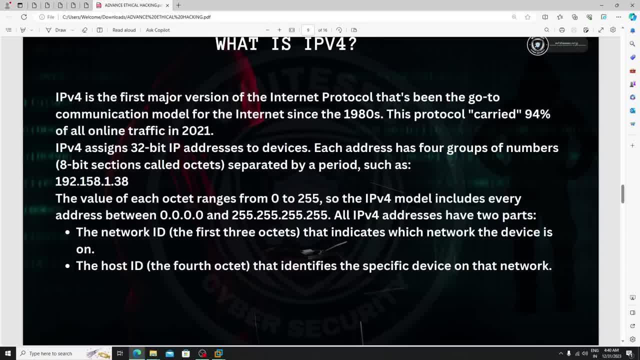 period such as like this period, such as like this: okay dot, okay dot, okay dot. in a simple words: we, we know about dots in a simple words. we, we know about dots in a simple words. we, we know about dots, right, we, we right, we, we right, we, we say as a dot there. 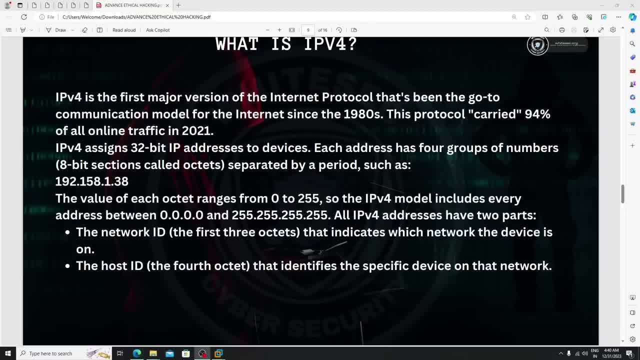 okay, okay. or point, or point, or point: the value of each octet. range from the value of each octet. range from the value of each octet. range from zero to two, five, five. okay, so the ipv4: zero to two, five, five. okay, so the ipv4. 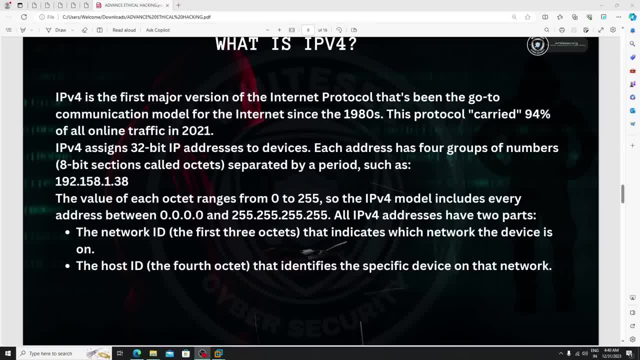 zero to two, five, five. okay, so the ipv4 model includes every address between model. includes every address between model. includes every address between: zero point zero point zero. zero point zero point zero. zero point zero point zero. uh, zero point zero point zero point zero. uh, zero point zero point zero point zero. 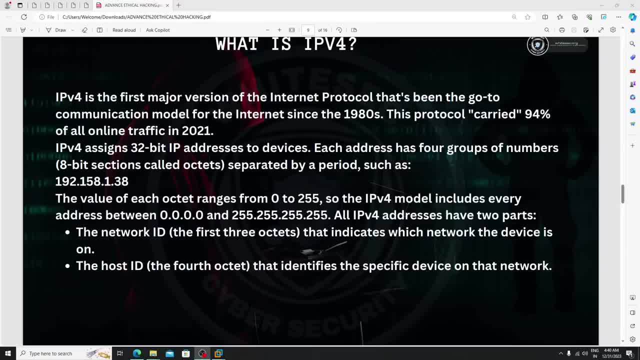 uh, zero point zero, point zero, point zero. and two, five, five, point two, five, five and two, five, five, point two, five, five and two, five, five, point two, five, five, point two, five, five, this is a thing. point two, five, five, point two, five, five. this is a thing. 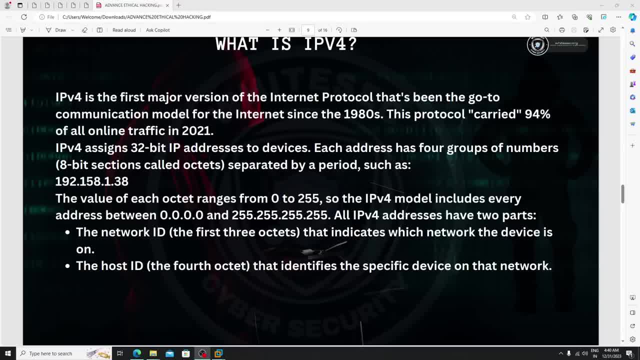 point two, five, five. point two, five, five. this is a thing, see, in a simple words. let me tell you, see, in a simple words. let me tell you see, in a simple words, let me tell you, you, me, everyone who who is using the ipv4. you me, everyone who who is using the ipv4. 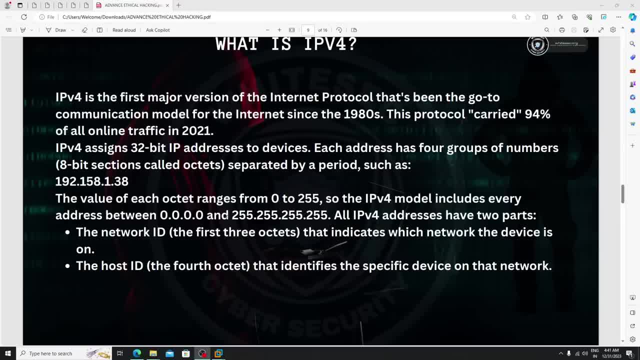 you, me, everyone who who is using the ipv4. okay, comes between this range. okay, this, okay comes between this range. okay. this, okay comes between this range. okay, this is a thing, is a thing, is a thing. your ip address everyone, okay, who are. your ip address everyone, okay, who are. 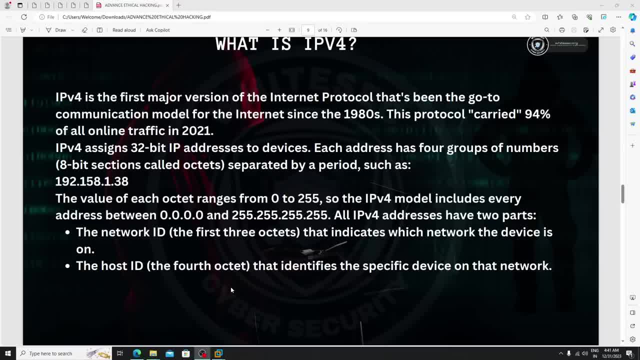 your ip address everyone, okay, who are using the ipv4, using the ipv4, using the ipv4 in a simple words. you can also say it as in a simple words. you can also say it as in a simple words. you can also say it as a: a. 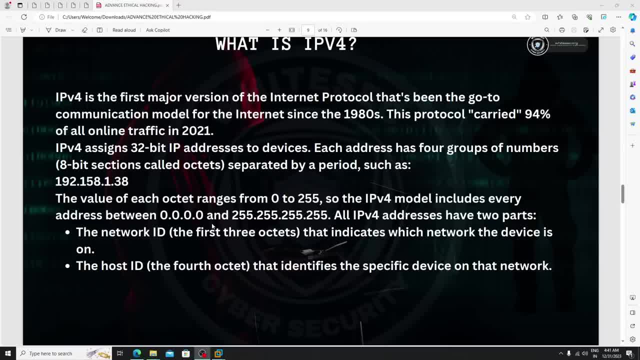 a we are connected. okay, this is the thing we are connected. okay, this is the thing we are connected. okay, this is the thing. uh in a simple words, uh in a simple words. uh in a simple words. this is: it is easy to uh by using this ipv4. 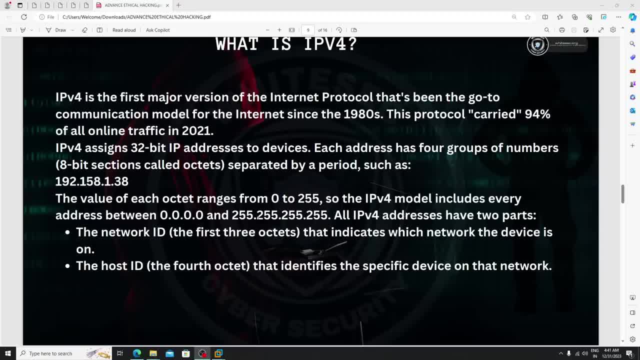 this is: it is easy to uh by using this ipv4. this is: it is easy to uh. by using this ipv4, it is easy to perform the cyber war. it is easy to perform the cyber war. it is easy to perform the cyber war. okay, okay, okay, excellent man, this is this ipv. i, i, i. 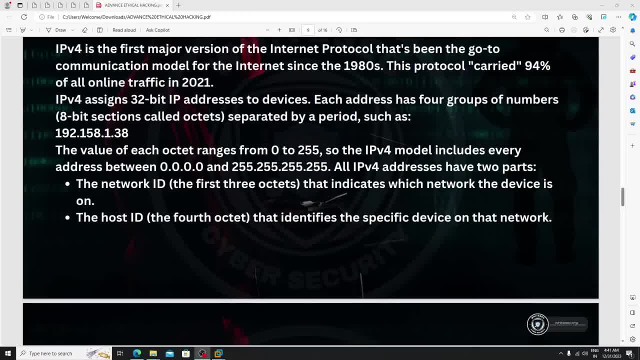 excellent man. this is this ipv i i i. excellent man. this is this ipv i i. i like ipv4. okay, like ipv4. okay, like ipv4. okay, right, all ipv4 addresses have two parts. right, all ipv4 addresses have two parts, right. all ipv4 addresses have two parts: the network id, the first three octets. 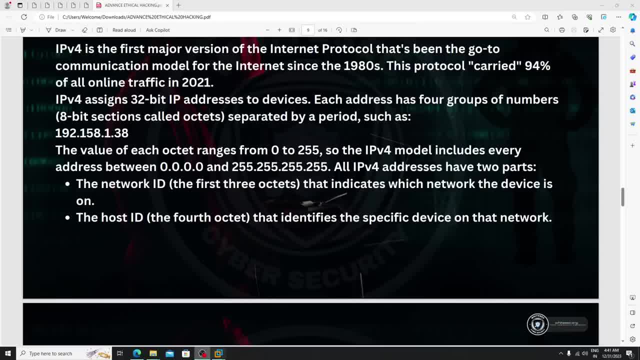 the network id: the first three octets. the network id: the first three octets. what is a network network id here? what is a network network id here? what is a network network id here? network id is nothing but this thing. network id is nothing but this thing. 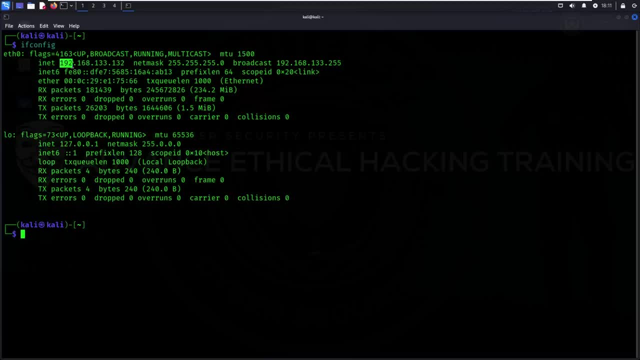 network id is nothing but this thing: first three octets. octets is nothing, but first three octets. octets is nothing, but first three octets. octets is nothing, but this is one octet. this is second octet. this is one octet. this is second octet. 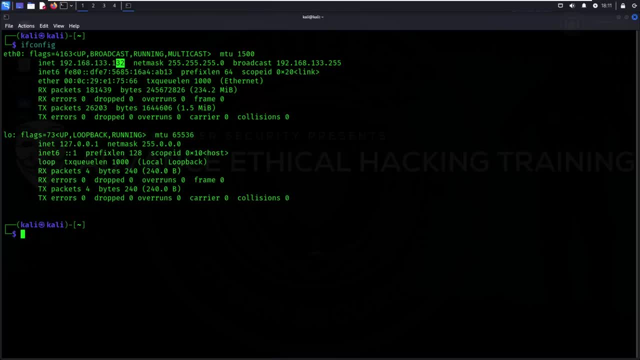 this is one octet, this is second octet, this is third and this is fourth. okay, this is third and this is fourth. okay, this is third and this is fourth. okay, now, now. now, here the net, the first three octets. okay, here the net, the first three octets, okay. 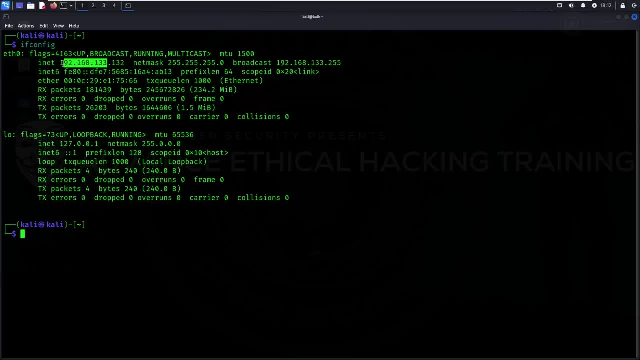 here the net, the first three octets. okay, see the net. this is known as a network id. see the net. this is known as a network id. see the net. this is known as a network id. okay, this three octets is known as a. okay, this three octets is known as a. 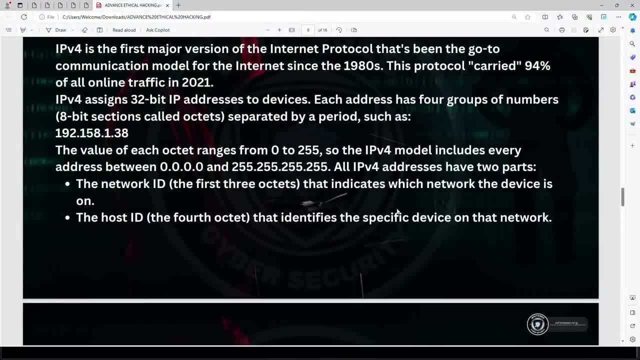 okay, this three octets is known as a network id: the that indicates which network. the. the that indicates which network. the. the that indicates which network the device is on. device is on. device is on the host, the host. you know about the host, the host, the host. you know about the host. 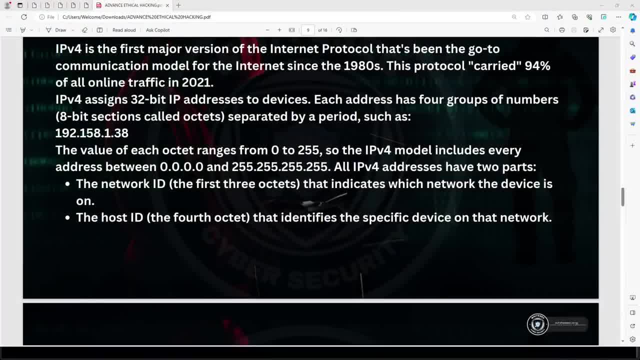 the host, the host. you know about the host. host is this octet okay. host is this octet okay. host is this octet okay. here, it is man here. it is man here, it is man okay. host, is this octet the fourth one? okay, host, is this octet the fourth one. 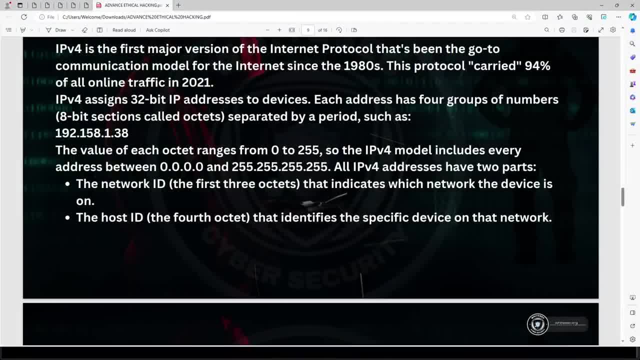 okay, host. is this octet the fourth one? i think i just learned this all stuff. i think i just learned this all stuff. i think i just learned this all stuff, like it's been around three years. i like it's been around three years. i like it's been around three years. i think three to four years, i i don't know. 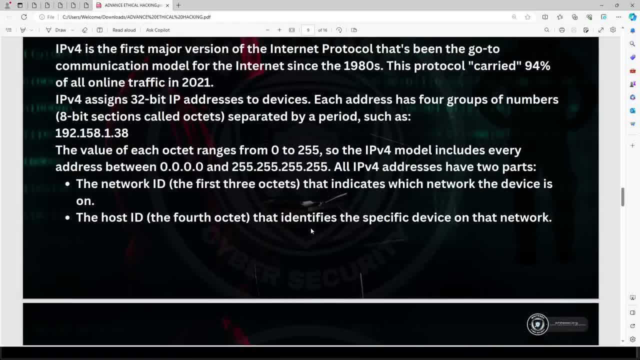 think three to four years, i i don't know. think three to four years, i i don't know. man, man, man, at the time i just learned the networking. at the time i just learned the networking. at the time i just learned the networking like osi model. uh, a lot of shots okay. 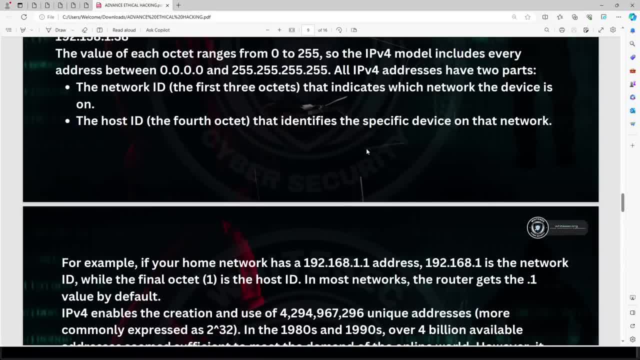 like osi model: uh, a lot of shots, okay. like osi model: uh, a lot of shots, okay, this is the thing. this is the thing. this is the thing. so this is the the host id the fourth. so this is the the host id the fourth. so this is the the host id the fourth octet. 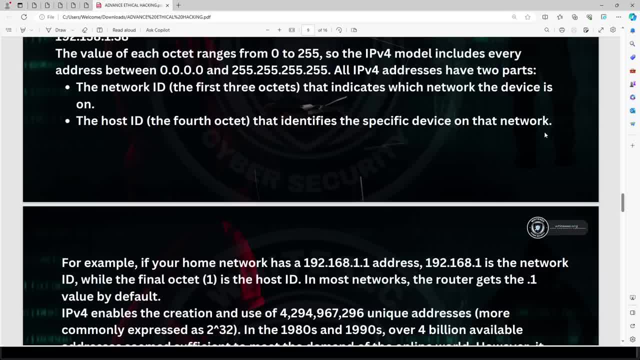 octet. octet that identity identifies the specific. that identity identifies the specific. that identity identifies the specific device on that network: okay. device on that network, okay. device on that network, okay. so that's why the the fourth octet is. so that's why the the fourth octet is. 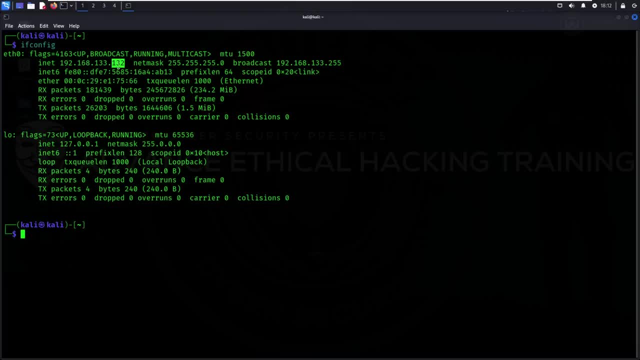 so that's why the the fourth octet is different here. okay see, uh, this is the different here. okay see, uh, this is the different here. okay see, uh, this is the unique, unique, unique. basically, this thing is unique here, see. basically, this thing is unique here, see. 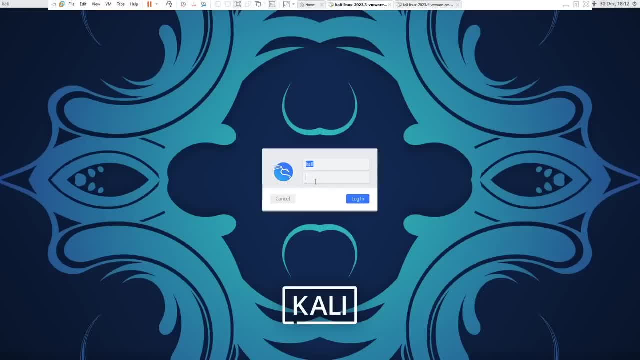 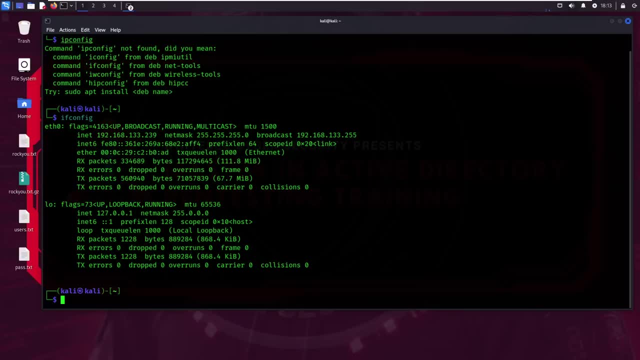 basically, this thing is unique here. see here 132, and here it is uh something here 132, and here it is uh something here 132, and here it is uh something like like, like, what is it? what is it? what is it? 232, 39, okay, yes, 239. 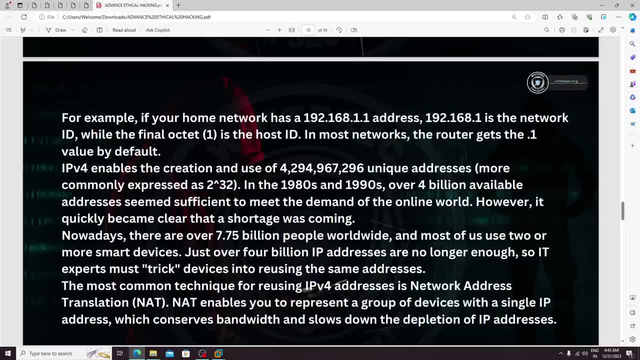 for example, if your home network has a. for example, if your home network has a. for example, if your home network has a 192.16, 192.16, 192.16, 168.1.1. if your home network 168.1.1. if your home network. 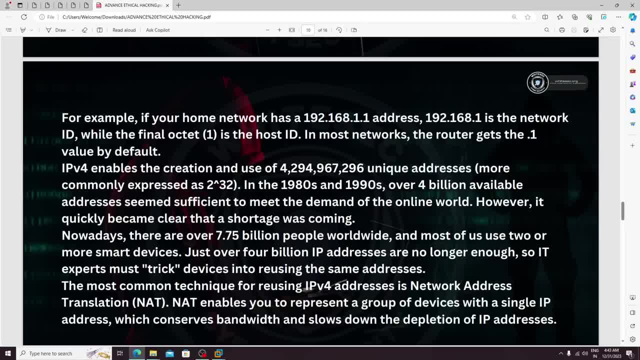 168.1.1 if your home network have. have 168.1.1, if your home network have. has this ip address: okay, has this ip address. okay, has this ip address? okay. one uh one uh 192.168.1 is a. one uh one uh 192.168.1 is a. 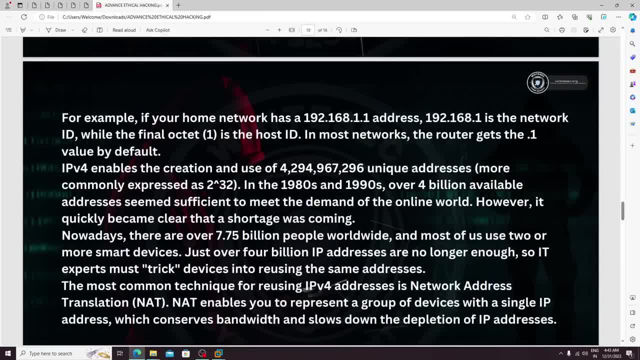 one, uh one, uh. 192.168.1 is a network id. okay, i just told you right, network id. okay, i just told you right, network id. okay, i just told you right, this is the thing here. this is the thing here. this is the thing here. you can also read it. okay, see just. 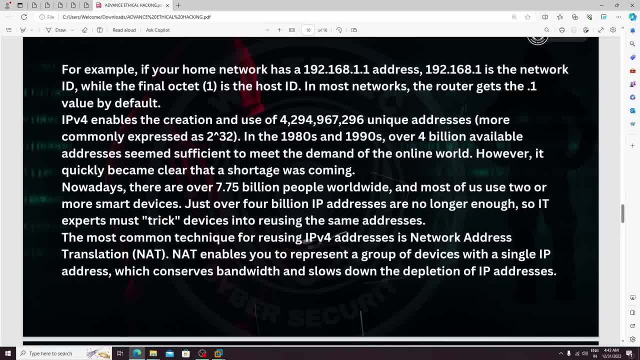 you can also read it. okay, see, just, you can also read it. okay, see, just focus on this point. ipv4 enables the focus on this point. ipv4 enables the focus on this point. ipv4 enables the creation and use, creation and use, creation and use. this much unique addresses more com. 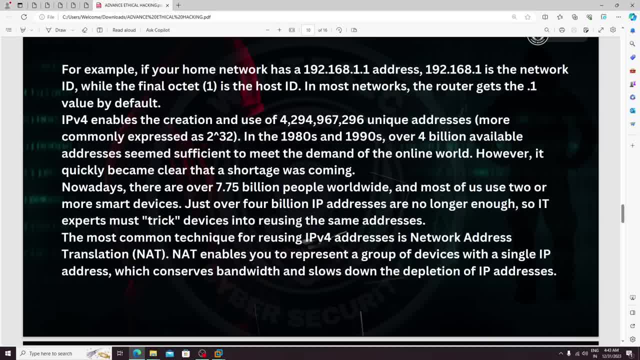 this much unique addresses, more com. this much unique addresses, more com, commonly expressed. commonly expressed, commonly expressed: 80s and 1990s: over 4 billions. 80s and 1990s: over 4 billions. 80s and 1990s: over 4 billions. available addresses seem sufficient to. 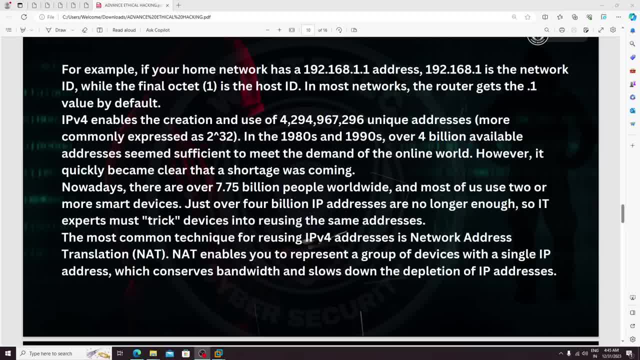 available addresses seem sufficient to available addresses seem sufficient to meet the demanded of the online world. meet the demanded of the online world. meet the demanded of the online world. however it is, it's quickly become clear. however it is, it's quickly become clear. however it is, it's quickly become clear that a shortage was coming. nowadays, i 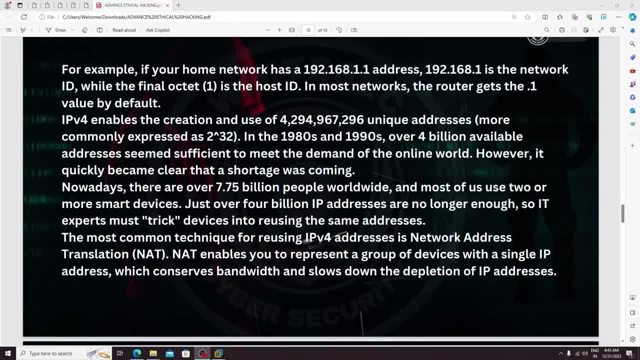 that a shortage was coming nowadays. i that a shortage was coming nowadays. i just told you right, it's become the. just told you right, it's become the. just told you right, it's become the: limited okay. limited, okay, limited, okay. nowadays. nowadays, there are over 7.75. 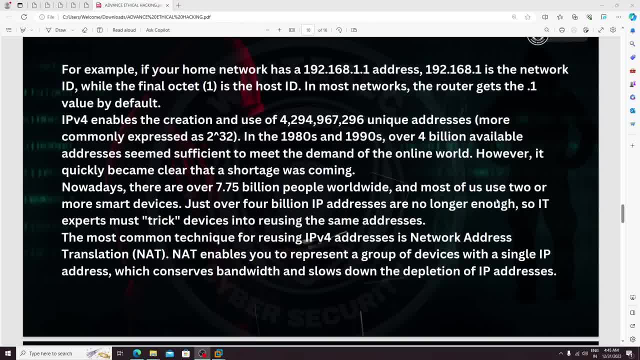 nowadays. nowadays, there are over 7.75. nowadays. nowadays, there are over 7.75 billion people worldwide and most of us billion people worldwide and most of us billion people worldwide, and most of us use two or two or more smart devices. use two or two or more smart devices. 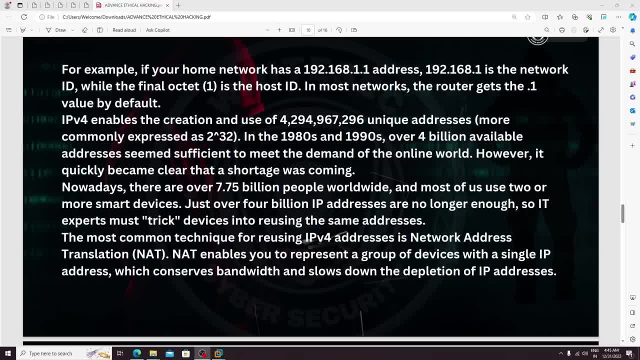 use two or two or more smart devices. okay, just over 4 billion ip addresses are okay. just over 4 billion ip addresses are okay. just over 4 billion ip addresses are no longer enough. so it expert must trick. no longer enough, so it expert must trick. 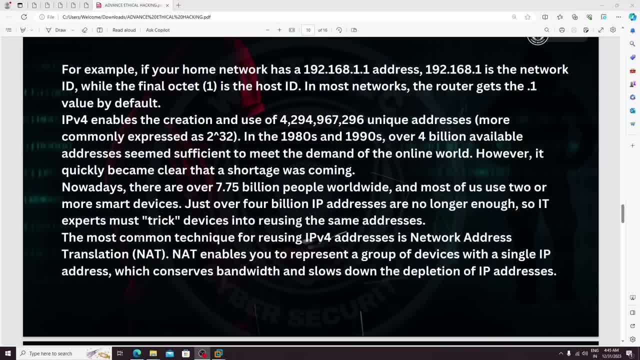 no longer enough, so it expert must trick devices into reusing the same addresses. devices into reusing the same addresses, devices into reusing the same addresses, the most common technique for reusing ipv. the most common technique for reusing ipv. the most common technique for reusing ipv. 4 addresses network addresses translation. 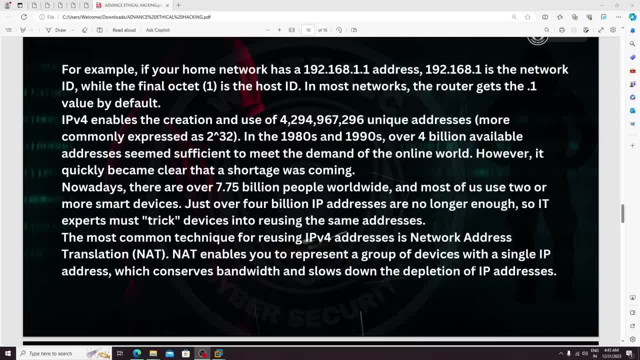 4 addresses network addresses translation. 4 addresses: network addresses translation. not not enable you to represent a group. not not enable you to represent a group, not not enable you to represent a group of devices with a group of devices, of devices with a group of devices, of devices with a group of devices with, a, say, single ip addresses. 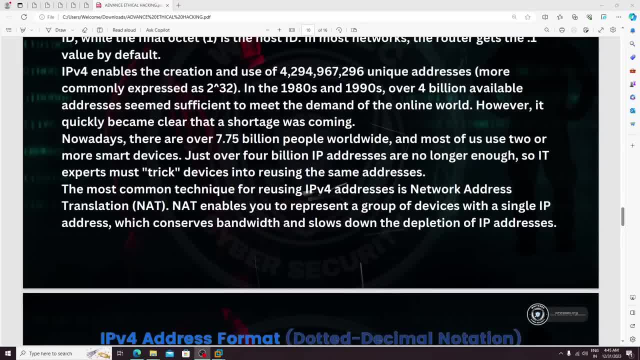 with a say: single ip addresses, with a say: single ip addresses okay, which conserves bandwidth and slow okay which conserves bandwidth and slow okay which conserves bandwidth and slow down, the down, the down. the depletion of ip addresses. now here is a depletion of ip addresses. now here is a. 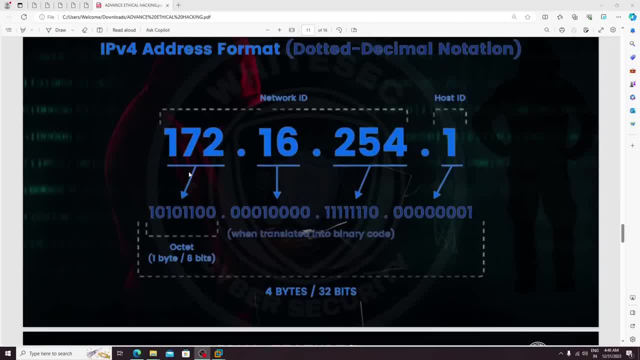 depletion of ip addresses. now here is a format which i just uh format, which i just uh format, which i just uh told you about this: like see ipv4 format. told you about this. like see ipv4 format. told you about this. like see ipv4 format: dotted decimal nation like this one. 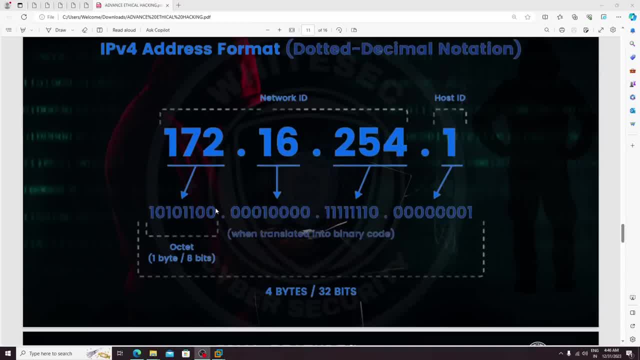 dotted decimal nation like this one dotted decimal nation like this one, now here, basically this. let me explain you now here, basically this. let me explain you now here, basically this. let me explain you this thing, just wait, this thing, just wait, this thing, just wait. there is a one website which is decimal. 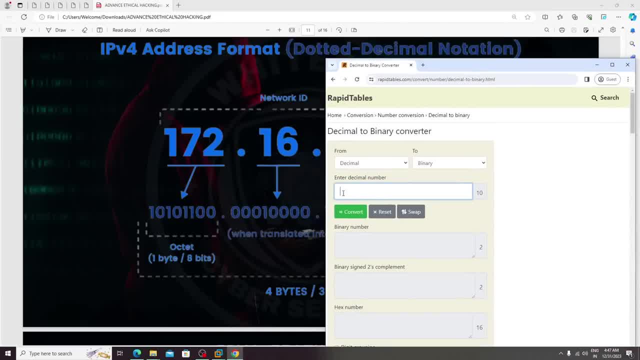 there is a one website which is decimal. there is a one website which is decimal to binary converter, to binary converter, to binary converter. okay, if you type 172 here, okay, if you type 172 here, okay, if you type 172 here in binary, it will be one zero, one zero. 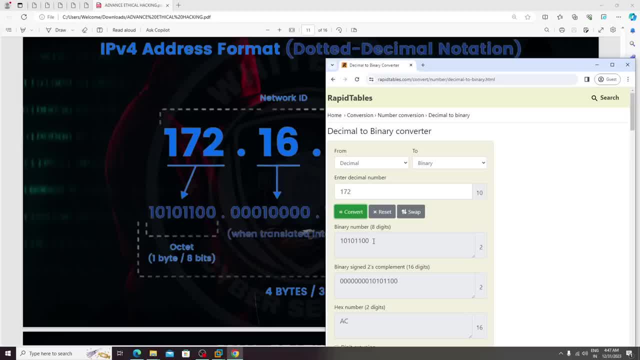 in binary, it will be one zero, one zero. in binary, it will be one zero, one zero. one one zero, zero. okay. one one zero, zero. okay. one one zero, zero. okay. which is understand by the computers: okay. which is understand by the computers: okay. which is understand by the computers: okay. your computer won't understand. 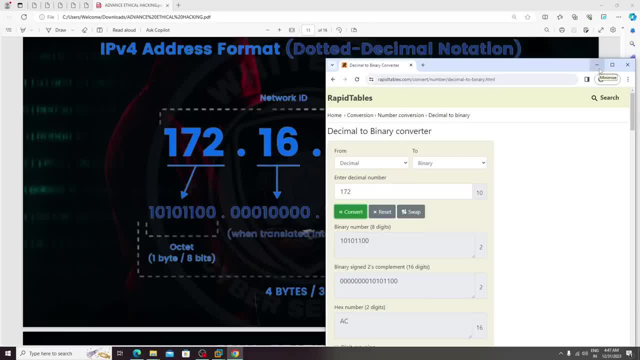 your computer won't understand. your computer won't understand uh the normal language. okay, this is the? uh the normal language. okay, this is the uh the normal language. okay, this is the thing thing thing. now, 16 is if you convert the the 16. now, 16 is if you convert the the 16. 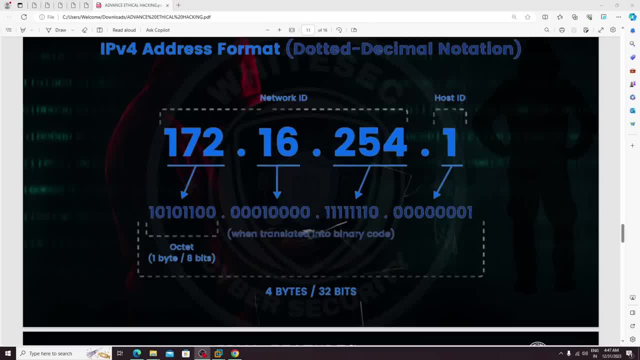 now 16 is. if you convert the, the 16 number to this- uh, this one number to this, uh, this one number to this, uh, this one binary, then it will be this thing, okay binary. then it will be this thing, okay binary. then it will be this thing, okay, this is how it's gonna work. this is how it's gonna work. this is how it's gonna work. this is known. i just told you right this. this is known. i just told you right this. this is known. i just told you right. this is known as one octet is known as one octet. 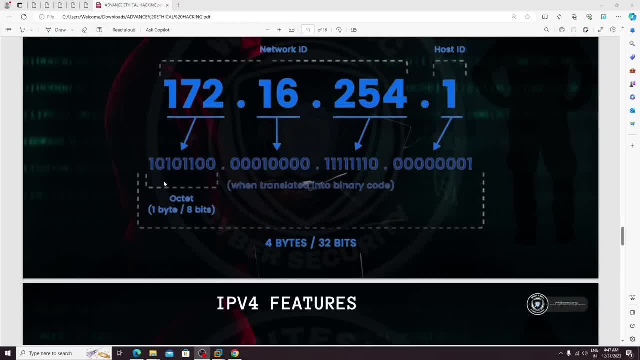 is known as one octet, which is eight bit. okay, why this is eight, which is eight bit. okay, why this is eight, which is eight bit. okay, why this is eight bit. just see one two, three, four bit. just see one two, three, four bit. just see one, two, three, four. one two, three, four. okay, this is the thing. 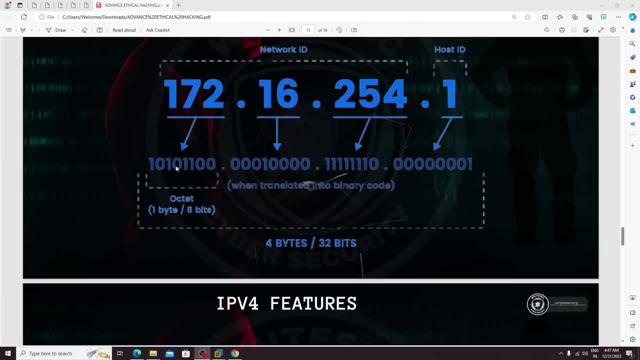 one, two, three, four. okay. this is the thing. one, two, three, four. okay. this is the thing. it's having the eight bit here, okay, it's having the eight bit here. okay, it's having the eight bit here, okay. one value is known as a one. yeah, one. 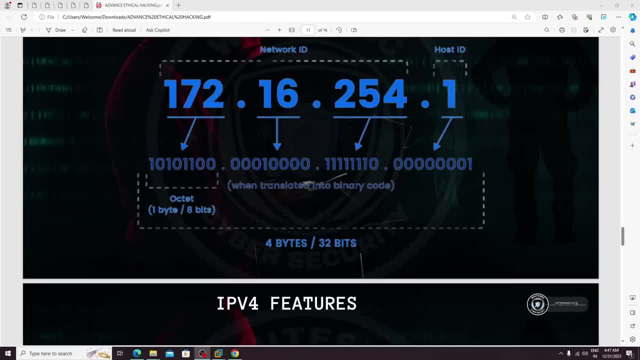 one value is known as a one. yeah, one. one value is known as a one. yeah, one. bit okay, this is the thing. bit okay, this is the thing. bit okay, this is the thing. not bytes. bit okay, bits. this is the. not bytes. bit okay, bits, this is the. 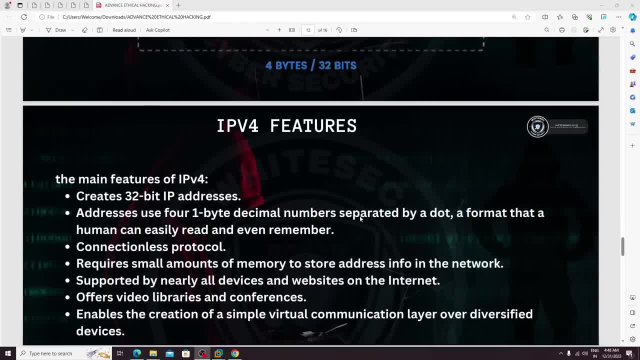 not bytes, bit, okay, bits. this is the thing. okay, hope you guys get it thing. okay, hope you guys get it thing. okay, hope you guys get it now. these are the features of ipv4 now. these are the features of ipv4 now. these are the features of ipv4, the main features of ipv4. create 32-bit. 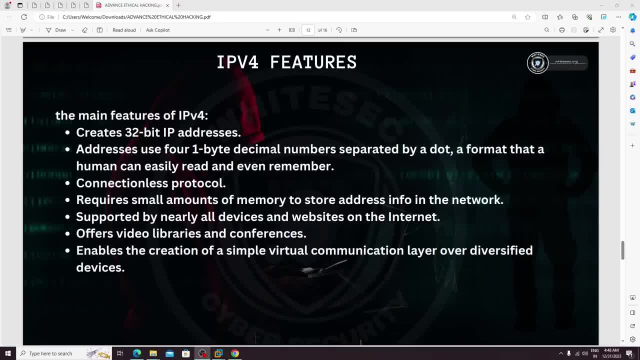 the main features of ipv4: create 32-bit. the main features of ipv4: create 32-bit ip address address: use four: one byte address. use four: one byte address. use four: one byte. decimal number separated by dot: a format. decimal number separated by dot: a format. 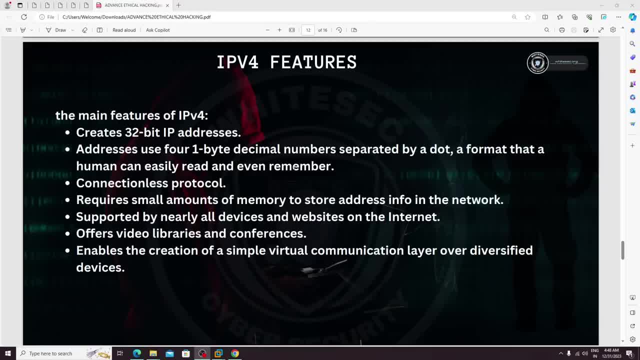 decimal number separated by dot, a format that a human can easily read, and even that a human can easily read, and even that a human can easily read and even remember. this is the thing mostly, uh remember. this is the thing mostly, uh remember. this is the thing mostly, uh. sometimes i can't able to remember it. 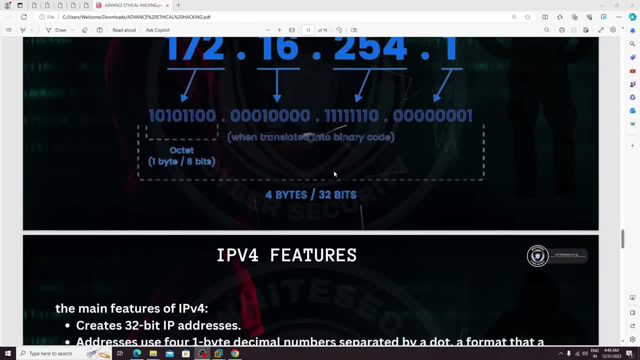 sometimes i can't able to remember it, sometimes i can't able to remember it, but still you can able to remember. okay, but still you can able to remember. okay, but still you can able to remember okay, once you start the pentesting at that, once you start the pentesting at that. 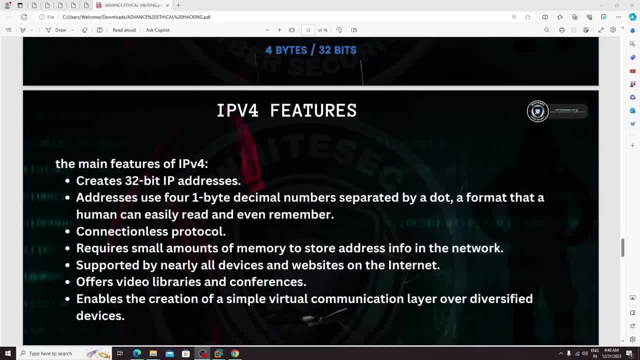 once you start the pentesting, at that time you can able to okay time you can able to okay time you can able to okay now, here, now, here, now here. connectionless protocol required. small connectionless protocol required. small connectionless protocol required. small amount of memory to store address info. 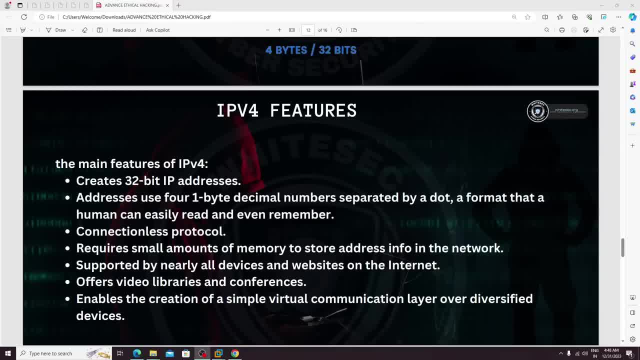 amount of memory to store address info. amount of memory to store address info in the network supported by nearly all in the network. supported by nearly all in the network. supported by nearly all devices and websites on the net to devices and websites on the net. to devices and websites on the net. to internet. okay, mostly, uh, everyone will. 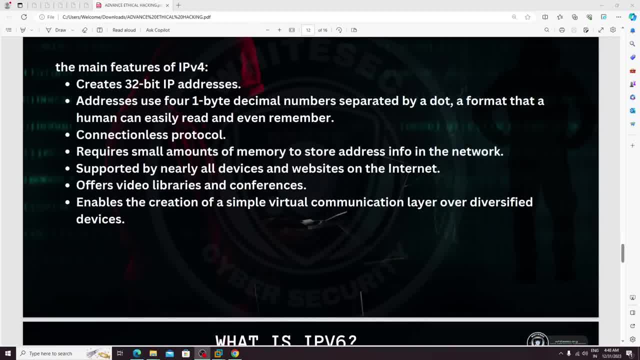 internet. okay, mostly, uh, everyone will internet. okay, mostly, uh, everyone will support it. okay, this is the thing. support it okay. this is the thing. support it okay. this is the thing. offers, offers, offers, videos, libraries and conferences. videos libraries and conferences. videos, libraries and conferences enable the creation of a simple virtual 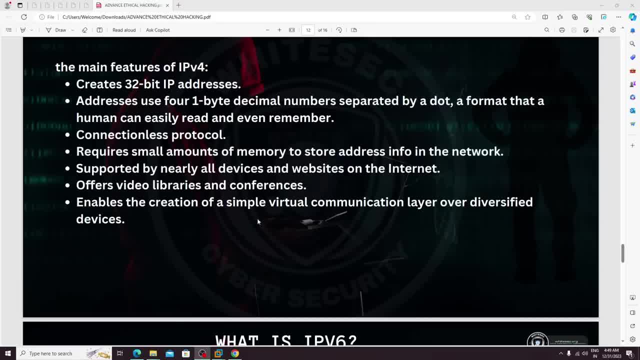 enable the creation of a simple virtual, enable the creation of a simple virtual communication layer over communication, layer over communication, layer over diversified devices. right, hope you guys. diversified devices. right, hope you guys. diversified devices. right, hope you guys get it. this is the ipv4. okay, it's not a 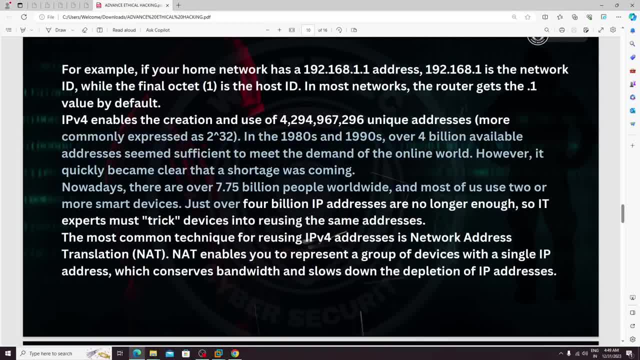 get it. this is the ipv4. okay, it's not a get it. this is the ipv4. okay, it's not a big deal. what i am trying to say is just big deal. what i am trying to say is just big deal. what i am trying to say is just read this one. okay, this is a very 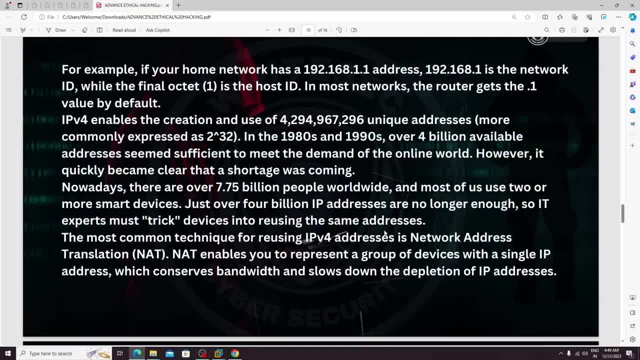 read this one. okay, this is a very read this one. okay, this is a very important thing, important thing. important thing, like why it's become limited, okay, why, like why it's become limited, okay, why, like why it's become limited, okay, why the ip address? uh, this, 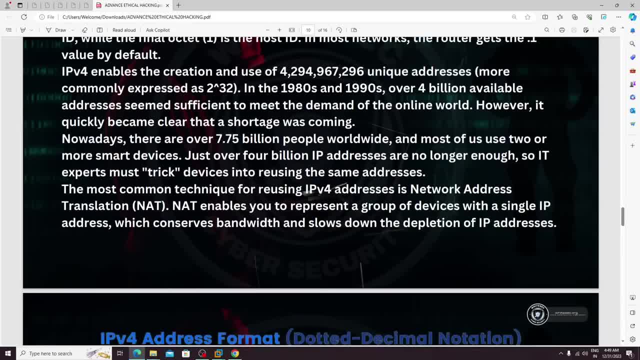 the ip address. uh, this the ip address. uh, this, the simple thing. okay, see here, he's just the simple thing. okay, see here, he's just the simple thing. okay, see here, he's just saying that, saying that, saying that one guy is using where it is, man. 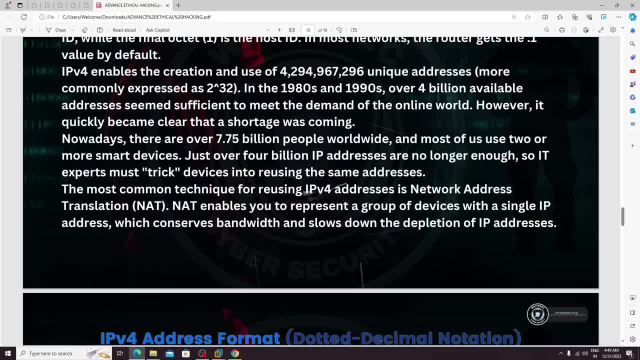 one guy is using where it is man. one guy is using where it is man and most of us used to uh and most of us used to uh and most of us used to uh. use two or more smart devices- okay this. use two or more smart devices, okay this. 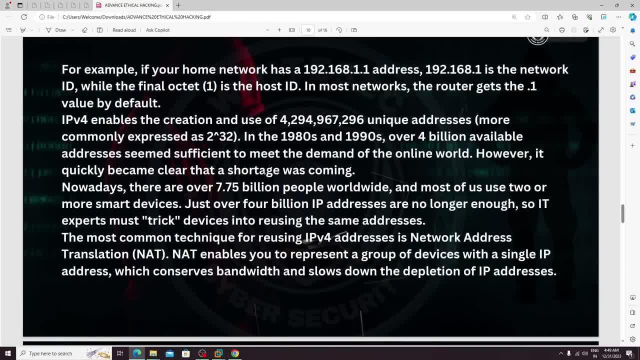 use two or more smart devices. okay, this is the thing. basically is the thing. basically is the thing. basically, assume that, assume that. assume that you, you are working as a cyber, you, you are working as a cyber, you, you are working as a cyber, cyber security engineer, or if you are. 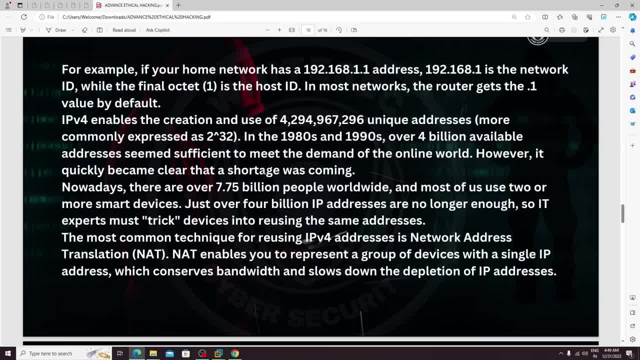 cyber security engineer, or if you are cyber security engineer, or if you are working as a pen tester, just remember working as a pen tester. just remember working as a pen tester. just remember one thing: how many laptops you use okay. one thing: how many laptops you use okay. 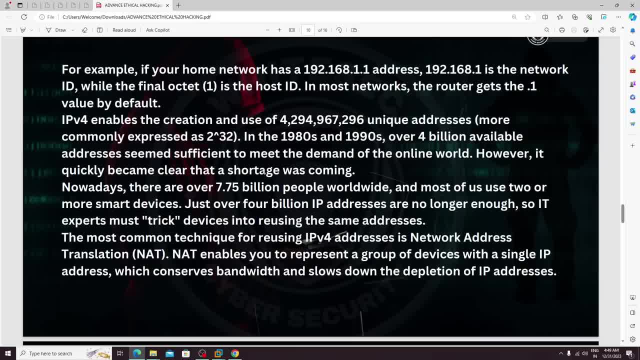 one thing: how many laptops you use, okay, how many devices you use, such as uh. how many devices you use such as uh. how many devices you use such as uh, you use a lot of devices, lot of laptops. you use a lot of devices, lot of laptops. you use a lot of devices, lot of laptops, right? so this is a simple point of view. 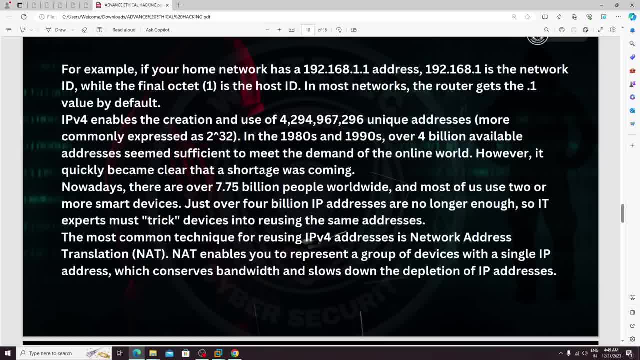 right, so this is a simple point of view, right, so this is a simple point of view. okay, mostly the people are using a lot. okay, mostly the people are using a lot. okay, mostly the people are using a lot of uh devices, uh iod devices, or of uh devices, uh iod devices or. 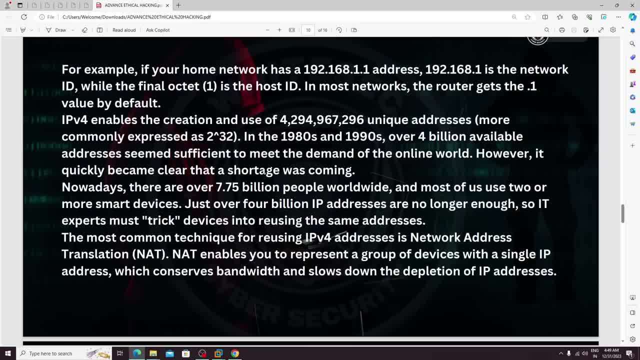 of uh devices, uh iod devices or something like that, okay, something like that, okay. something like that, okay. which are smart like smart tv? is there which are smart like smart tv? is there which are smart like smart tv? is there, okay? smart cars are there simple. okay, smart cars are there, simple. 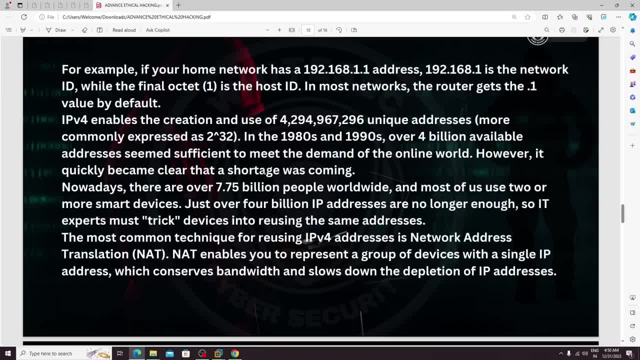 okay, smart cars are there. simple, due to this reason, due to this reason, due to this reason, these things are becoming limited. okay, i hope you guys get it right in the next. i hope you guys get it right in the next. i hope you guys get it right in the next classes we are learning about 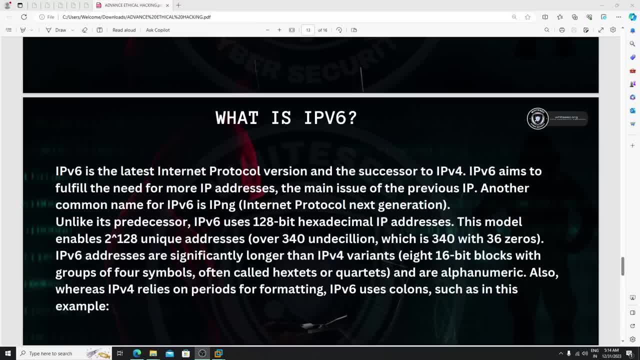 classes. we are learning about classes. we are learning about uh ipv6- right in this class. we are uh ipv6- right in this class. we are uh ipv6- right in this class. we are learning about. what is ipv6 learning about? what is ipv6 learning about? what is ipv6? ipv6 is the latest internet protocol. 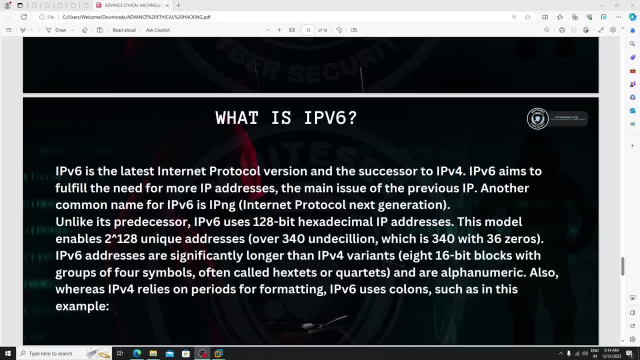 ipv6 is the latest internet protocol. ipv6 is the latest internet protocol version, version version and also successor to ipv4- okay, and also successor to ipv4- okay, and also successor to ipv4- okay. ipv6 aim is to fulfill the need for more. ipv6 aim is to fulfill the need for more. 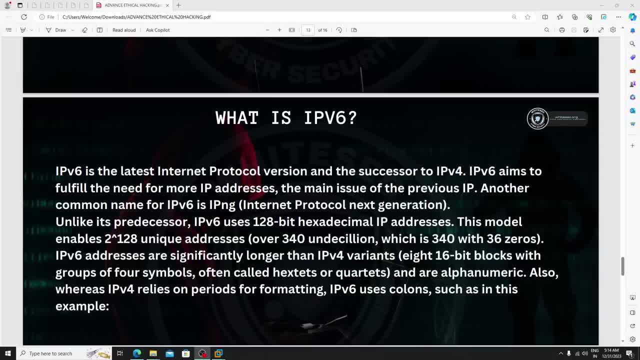 ipv6 aim is to fulfill the need for more ip. addresses ip addresses ipv6 aim is to fulfill the need for more ip addresses the main issue of the previous ip, the main issue of the previous ip, the main issue of the previous ip. see, i just told you right. 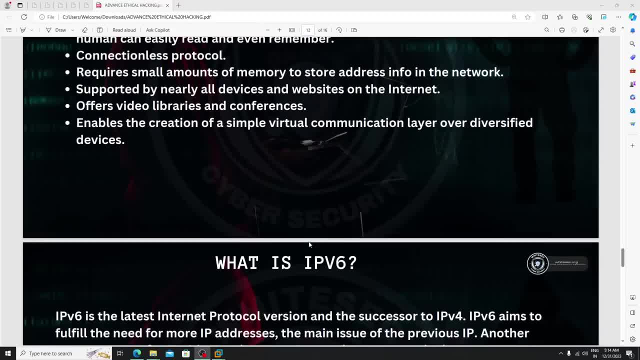 see, i just told you right, see, i just told you right: ipv4 become the limited. okay, because we ipv4 become the limited. okay, because we ipv4 become the limited. okay, because we need more ip addresses now, need more ip addresses now, need more ip addresses now. the simple thing is: so that's why ipv6. 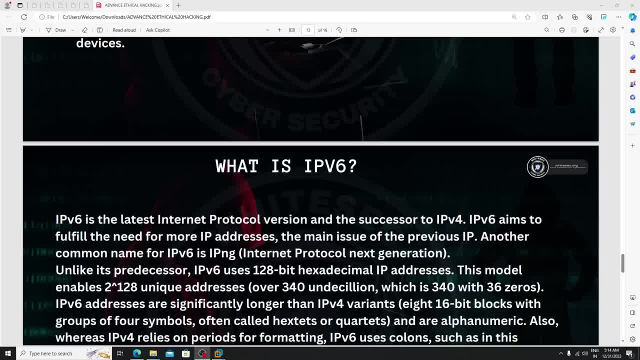 the simple thing is so that's why ipv6. the simple thing is so that's why ipv6 came okay. mostly the ipv6 is used by. came okay, mostly the ipv6 is used by. came okay, mostly the ipv6 is used by iot devices- okay, another. 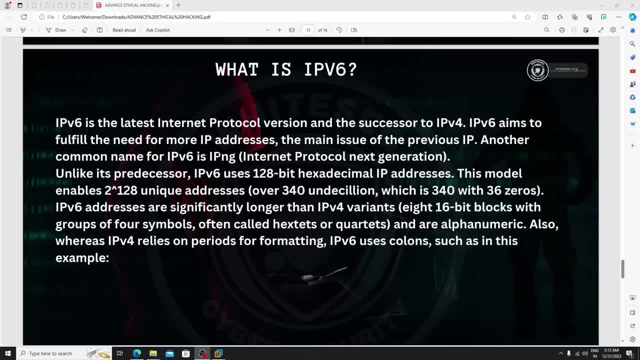 iot devices: okay. another iot devices: okay. another common name for ipv6 is internet. common name for ipv6 is internet. common name for ipv6 is internet protocol. next generation ipng, which is protocol, next generation ipng, which is protocol, next generation ipng, which is known as okay. 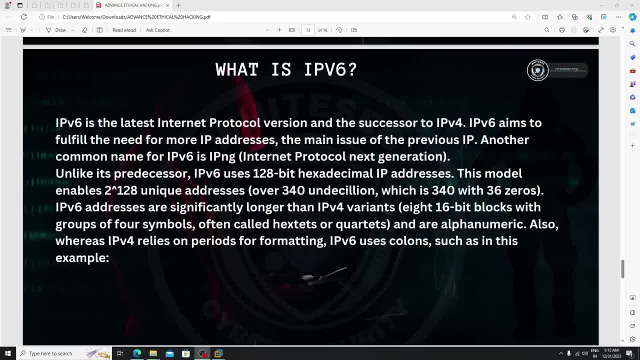 known as okay. known as okay. unlike its predecessor, ipv6 uses 128. unlike its predecessor, ipv6 uses 128. unlike its predecessor, ipv6 uses 128 bit hexadecimal ip addresses bit hexadecimal ip addresses bit hexadecimal ip addresses. this model enabled to carry 128 unique. this model enabled to carry 128 unique. 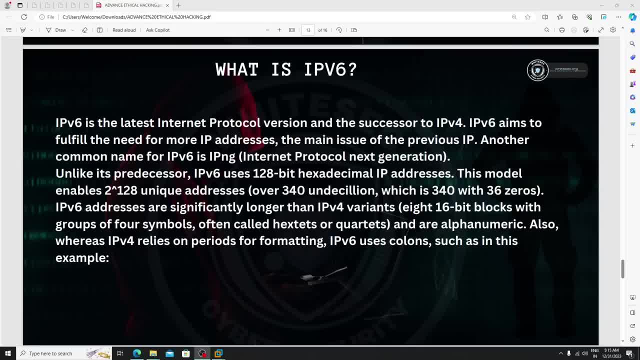 this model enabled to carry 128 unique addresses, addresses, addresses okay over three over three, four uh 340, okay over three over three, four uh 340, okay over three over three, four uh 340, and this is uh decillion which is 340, and this is uh decillion which is 340. 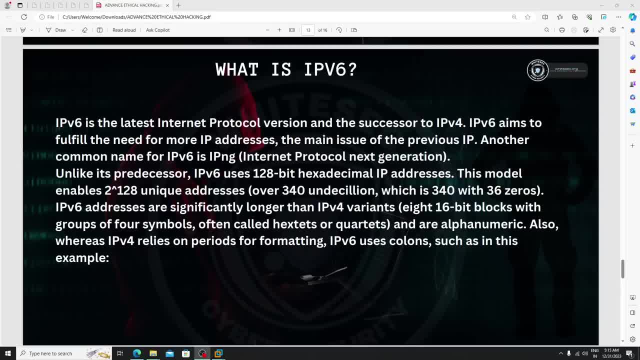 and this is uh decillion, which is 340 with 36 zeros. right ipv6 addresses are with 36 zeros. right ipv6 addresses are with 36 zeros. right ipv6 addresses are significantly longer than ipv4 variants, significantly longer than ipv4 variants, significantly longer than ipv4 variants. uh, here we can able to see that ipv4 is. 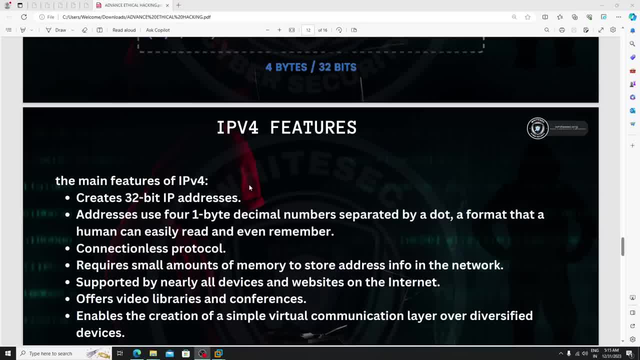 uh, here we can able to see that ipv4 is uh, here we can able to see that ipv4 is easy to remember and it is easy to remember and it is easy to remember and it is uh excellent, right away, it's it comes. uh, excellent, right away, it's it comes. 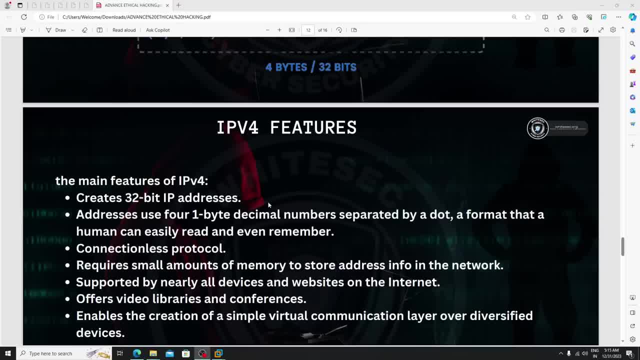 uh excellent, right away, it's. it comes under numeric, under numeric, under numeric. sorry guys, sorry guys, sorry guys. numeric order. like i can able to uh see numeric order, like i can able to uh see numeric order, like i can able to uh see it as a 192.168. 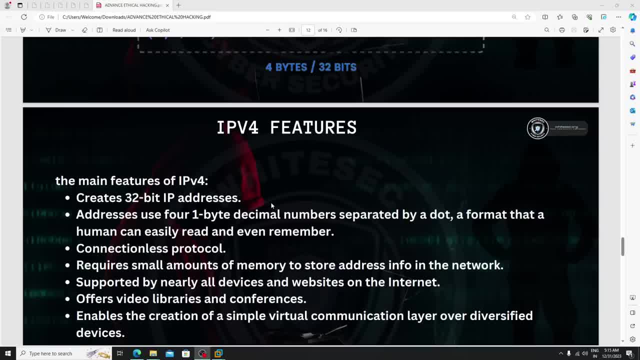 it as a 192.168, it as a 192.168 or 178 or something like that. it comes or something like that. it comes or something like that. it comes under numeric form. but here ipv6 comes under numeric form, but here ipv6 comes. 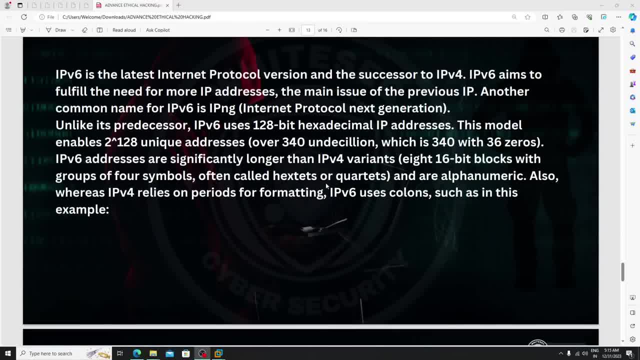 under numeric form. but here ipv6 comes with a lot of alphabetical order, with with a lot of alphabetical order, with with a lot of alphabetical order, with hex states and quarter uh quartets. let hex states and quarter uh quartets. let hex states and quarter uh quartets. let me show you how it look like. okay, if i 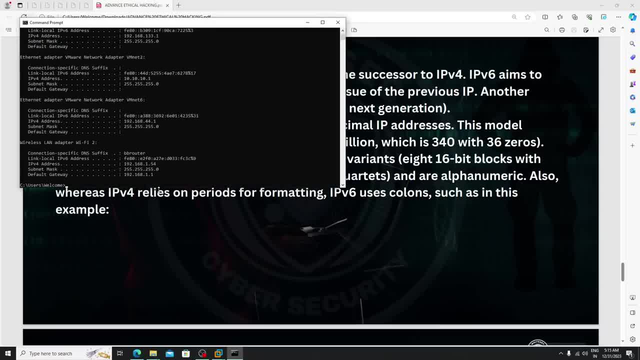 me show you how it look like. okay, if i me show you how it look like. okay, if i type here ip config- here you guys can type here ip config- here you guys can type here ip config- here you guys can able to see, able to see, able to see: see, this is ipv6. okay, see how it's look. 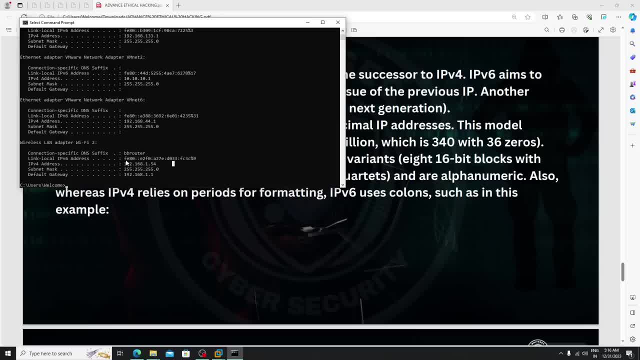 see this is ipv6. okay, see how it's look. see this is ipv6. okay, see how it's look. like: okay, it's contain uh alpha. like: okay, it's contain uh alpha. like: okay, it's contain uh alpha- alphabetical alpha: uh. alphabetical alpha. uh. alphabetical alpha, uh alphabet- sorry, alphabet. numeric numbers. 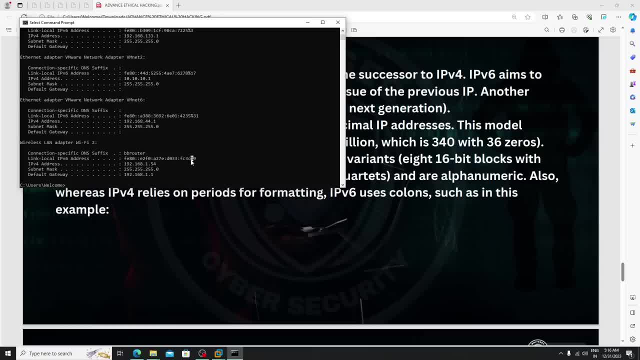 alphabet, sorry, alphabet. numeric numbers: alphabet, sorry, alphabet. numeric numbers: each and everything right. and also we, each and everything right. and also we, each and everything right. and also we can able to see the symbols as well, can able to see the symbols as well, can able to see the symbols as well, okay, and see the ipv4. it is easy, right. 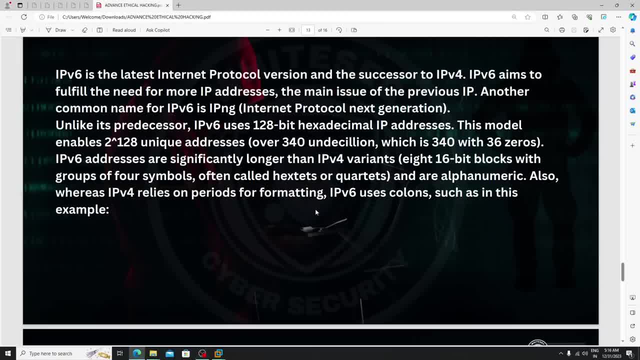 okay, and see the ipv4, it is easy right. okay, and see the ipv4, it is easy right. but comparing to ipv6, this is the thing. but comparing to ipv6, this is the thing. but comparing to ipv6, this is the thing. okay, and also it uses column. 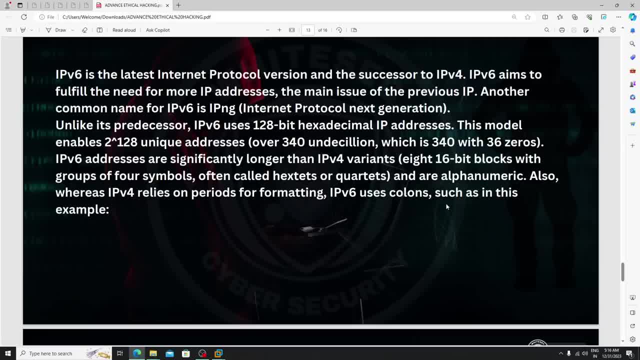 okay, and also it uses column: okay, and also it uses column ipv4. use the dots right here. it's use a ipv4. use the dots right here. it's use a ipv4. use the dots right here. it's use a column such as in this column, such as in this. 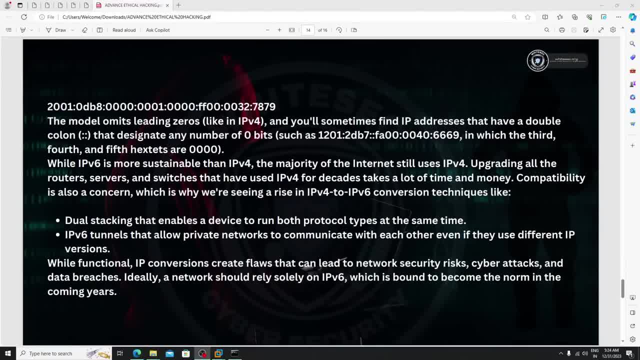 column, such as in this: examples, and here you can able to read examples. and here you can able to read examples. and here you can able to read the examples as well, the examples as well, the examples as well. see the model omits leading zero, like in. see the model omits leading zero, like in. 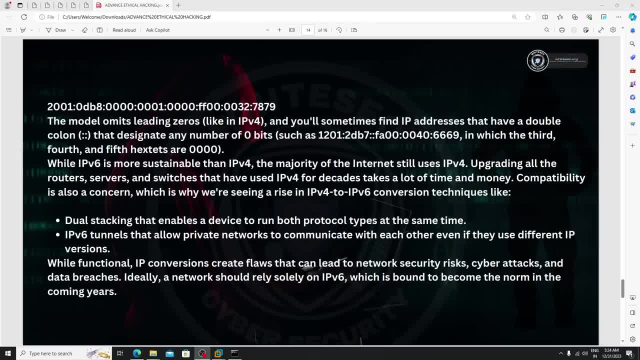 see the model omits, leading zero, like in ipv4, ipv4, ipv4- and you will sometimes find ip addresses and you will sometimes find ip addresses and you will sometimes find ip addresses that have double colon- here you guys can. that have double colon. here you guys can. 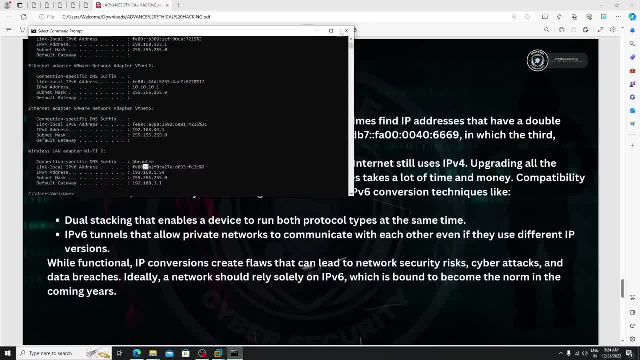 that have double colon here you guys can able to see, able to see able to see. you can also see the double colon here. you can also see the double colon here. you can also see the double colon here. okay, now let's see. first let's focus on. 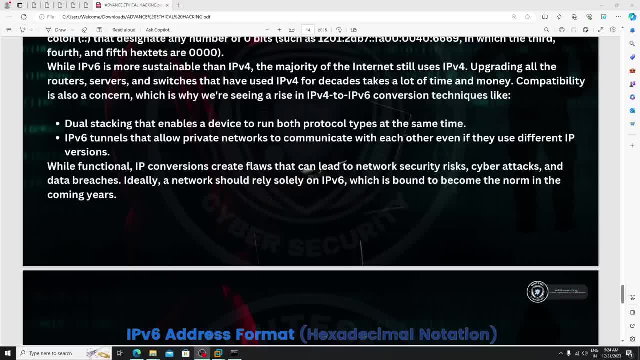 okay, now let's see. first let's focus on: okay, now let's see. first let's focus on these points dual stacking that enable a. these points dual stacking that enable a. these points dual stacking that enable a device to run both protocol types at the device, to run both protocol types at the 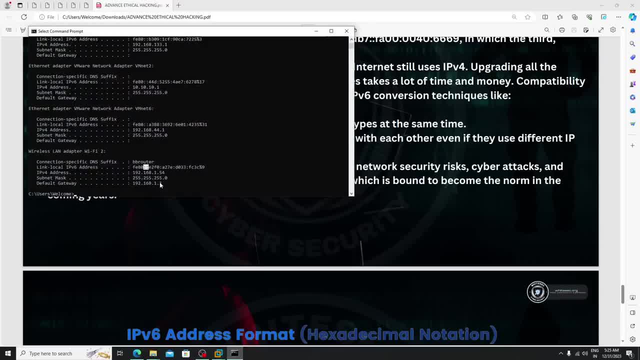 device to run both protocol types at the same time. basically, here you can able to same time. basically, here you can able to same time. basically, here you can able to see the both protocols are running at the see. the both protocols are running at the see. the both protocols are running at the same time sometimes. what will happen? 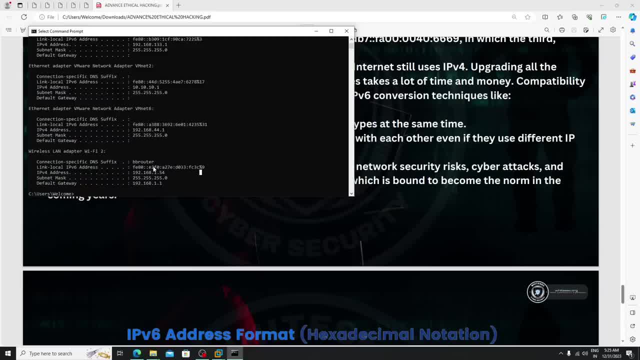 same time. sometimes what will happen same time. sometimes what will happen means mostly in active directory pen means mostly in active directory pen means mostly in active directory pen. testing, testing, testing this kind of stuff. so you guys can this kind of stuff. so you guys can this kind of stuff, so you guys can able to see the ipv4 there. we can also. 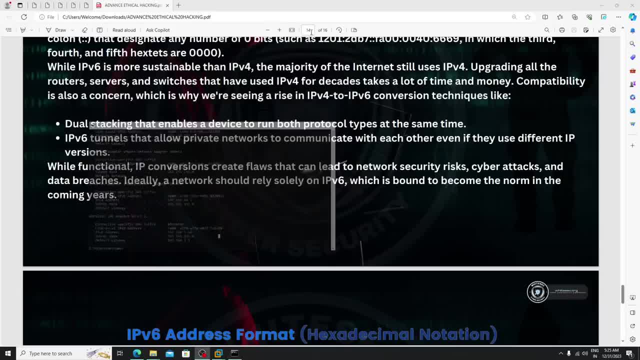 able to see the ipv4 there. we can also able to see the ipv4 there. we can also target the ipv4 as well. okay, target the ipv4 as well. okay, target the ipv4 as well. okay, and here ipv6 tunnels that allow, and here ipv6 tunnels that allow. 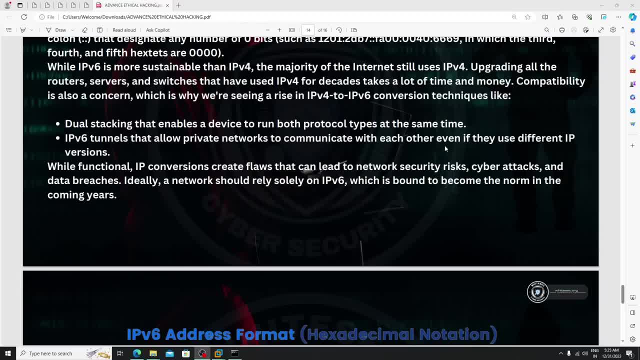 and here ipv6 tunnels that allow private networks to communicate with private networks, to communicate with private networks, to communicate with each other, even if there are, if they each other, even if there are, if they each other, even if there are, if they use different ip versions, use different ip versions. 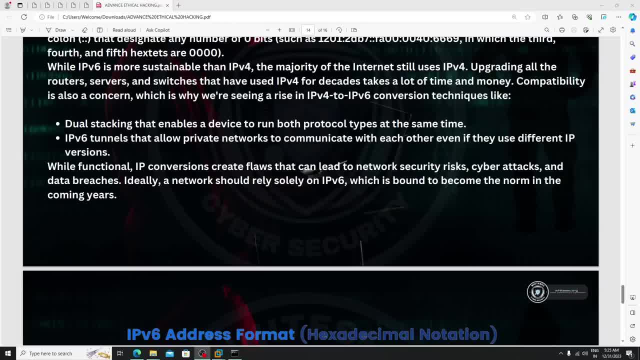 use different ip versions, even if they use ipv4 or ipv6 it, even if they use ipv4 or ipv6 it, even if they use ipv4 or ipv6, it doesn't matter. it can able to, doesn't matter, it can able to, doesn't matter, it can able to communicate. this is the thing. well, 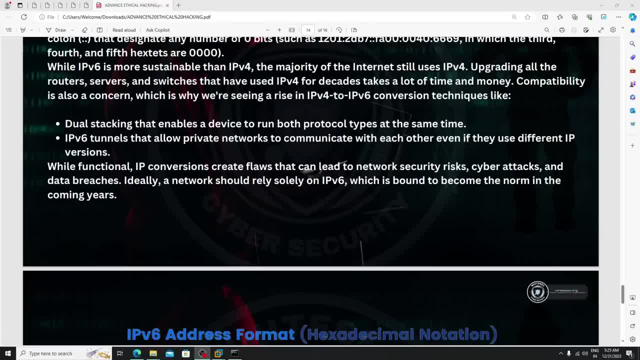 communicate- this is the thing. well communicate- this is the thing. well functional ip. functional ip. functional ip conversions. create flaws that can lead conversions. create flaws that can lead conversions. create flaws that can lead to network security risk, cyber attacks to network security risk, cyber attacks to network security risk, cyber attacks and data breaches. ideally, a network. 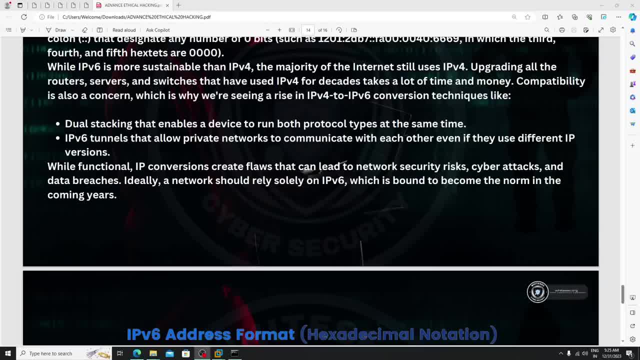 and data breaches. ideally a network and data breaches. ideally a network should relay solely on ipv6. i just told should relay solely on ipv6. i just told should relay solely on ipv6. i just told you: ipv, you, ipv, you, ipv6 is more secure than ipv4. okay, this is. 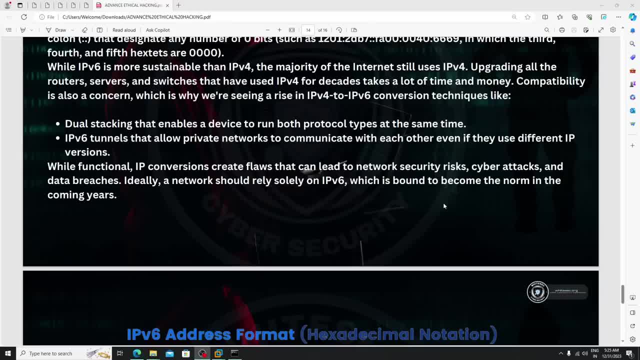 6 is more secure than ipv4. okay, this is. 6 is more secure than ipv4. okay, this is also one thing which is bounded to, also one thing which is bounded to, also one thing which is bounded to become the norm in the coming years. become the norm in the coming years. 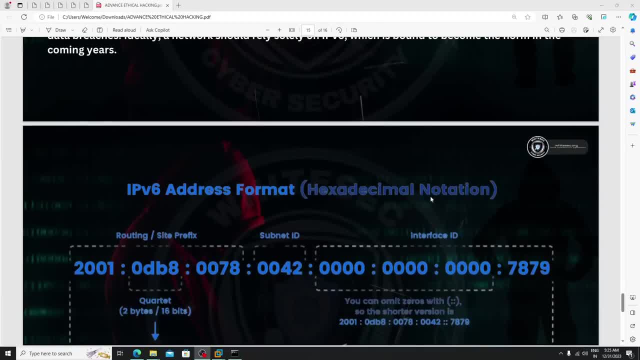 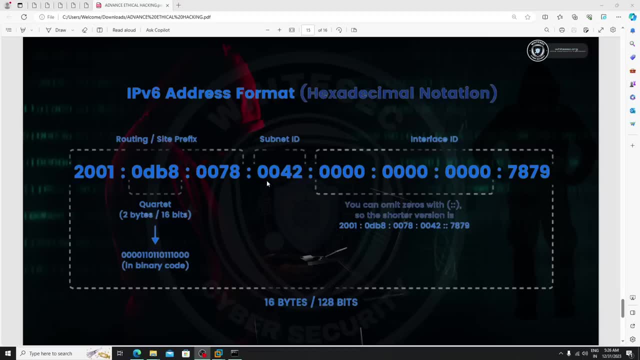 become the norm in the coming years. ipv6 address format- hexadecimal. ipv6 address format- hexadecimal. ipv6 address format, hexadecimal notation. this is a routing site prefix notation. this is a routing site prefix notation. this is a routing site prefix. subnet id. this is a subnet id and this: 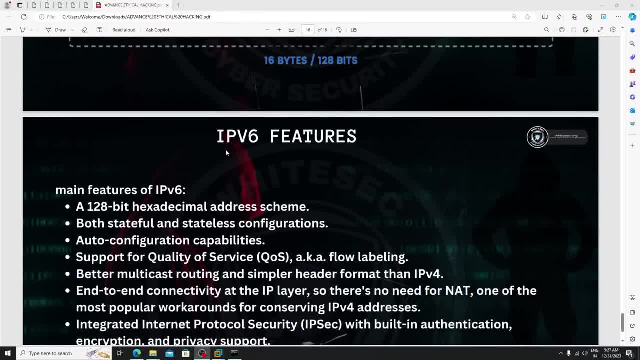 subnet id. this is a subnet id and this subnet id- this is a subnet id and this is a interface- is a interface, is a interface id. now there is a ipv6 features. it's a id. now there is a ipv6 features. it's a id. now there is a ipv6 features. it's a 128-bit hexadecimal address schema. 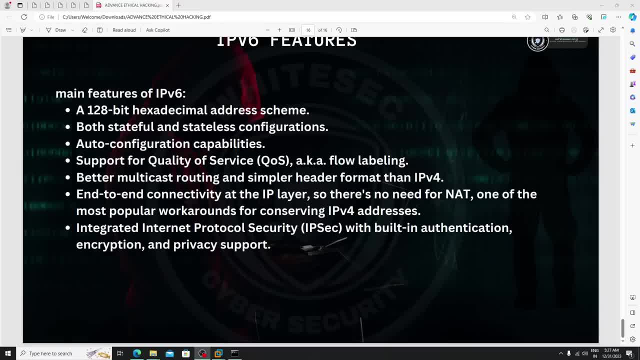 128-bit hexadecimal address schema. 128-bit hexadecimal address schema. and here, both stateful and stateless. and here, both stateful and stateless. and here, both stateful and stateless. configuration: auto configuration, configuration: auto configuration configuration: auto configuration, capabilities, capabilities, capabilities, support for quality of service, which is 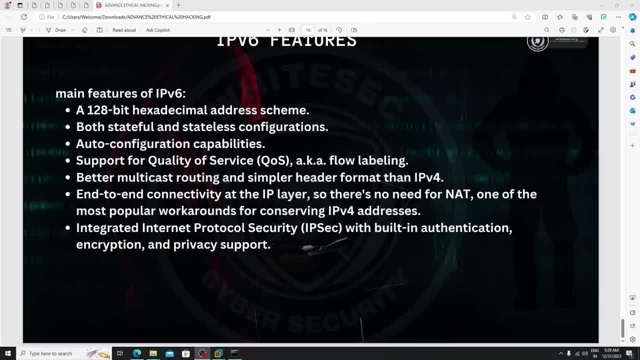 support for quality of service, which is support for quality of service, which is cause, cause, cause aka flow labeling- okay. better multi-cache aka flow labeling- okay. better multi-cache aka flow labeling- okay. better multi-cache routing and simpler handle routing and simpler handle routing and simpler handle header format than ipv4 end-to-end. 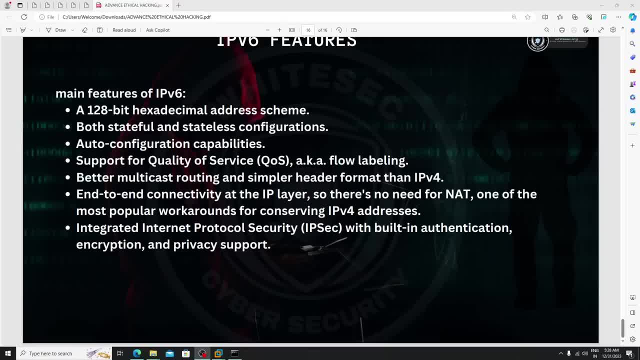 header format than ipv4. end-to-end header format than ipv4 end-to-end connectivity connectivity. connectivity at the ip layer. so there is no need for at the ip layer. so there is no need for at the ip layer. so there is no need for not one of the most popular workarounds. 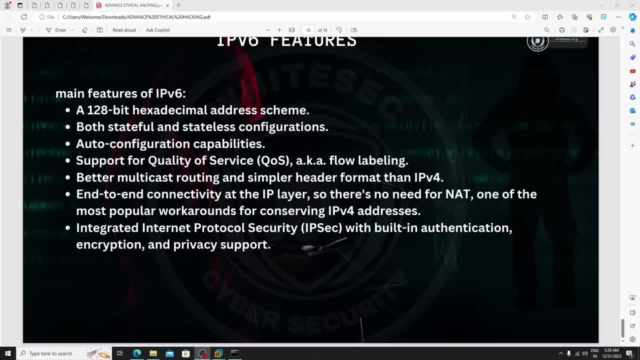 not one of the most popular workarounds, not one of the most popular workarounds for conserving ipv4 addresses for conserving ipv4 addresses for conserving ipv4 addresses. integrated internet protocol security. integrated internet protocol security. integrated internet protocol security. ipset, ipset. 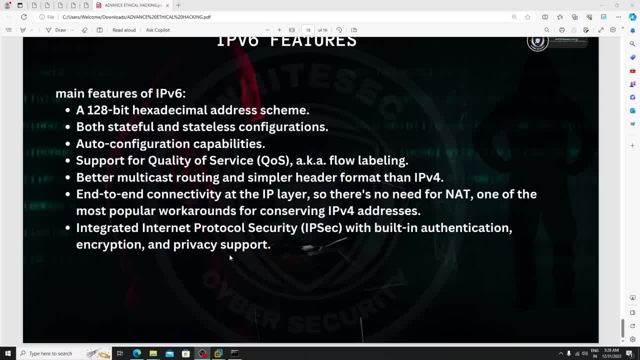 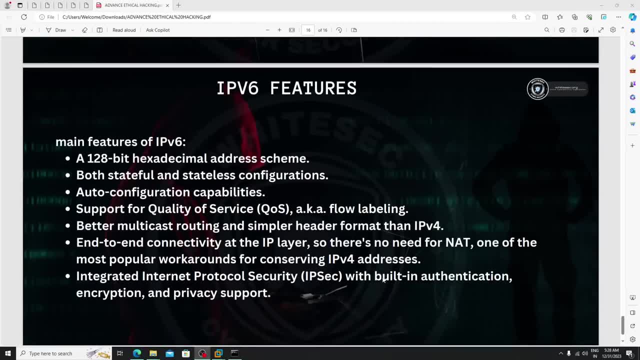 ipset with built-in authentication, encryption, with built-in authentication encryption, with built-in authentication encryption and privacy support and privacy support and privacy support. this is the thing so mostly still. this is the thing so, mostly still. this is the thing so mostly still. you can mostly you see ipv4 only okay. 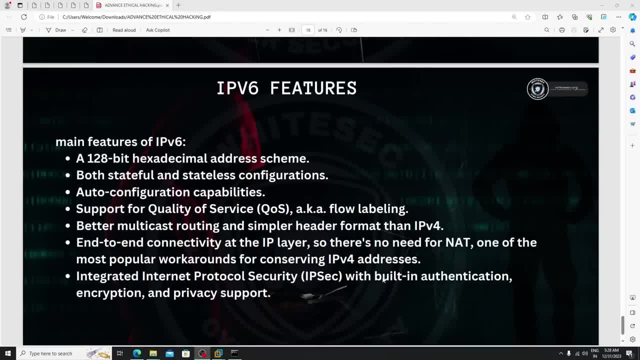 you can mostly you see ipv4 only okay. you can mostly you see ipv4 only okay. this is the thing. this is the thing. this is the thing like, if you see ipv6, there are some like. if you see ipv6, there are some like, if you see ipv6, there are some different attacks on ipv6 as well. 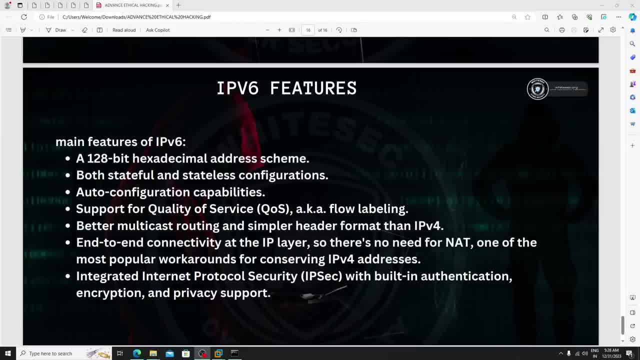 different attacks on ipv6 as well. different attacks on ipv6 as well. hope you guys get it now in the next, hope you guys get it now in the next, hope you guys get it now in the next classes. we will focus on some other classes. we will focus on some other. 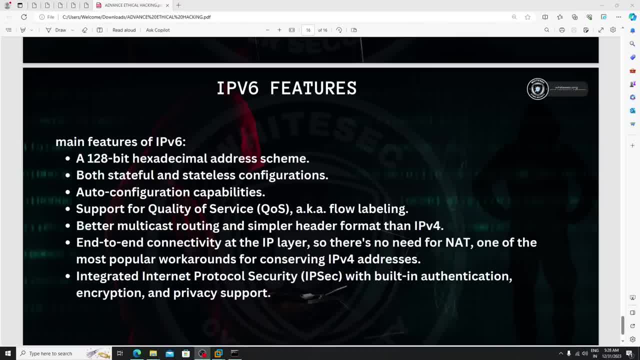 classes. we will focus on some other protocols or ports or something like that. protocols or ports or something like that. protocols or ports or something like that. hope you guys enjoy this classes. thank hope you guys enjoy this classes. thank hope you guys enjoy this classes. thank you, have a nice day in this classes. we 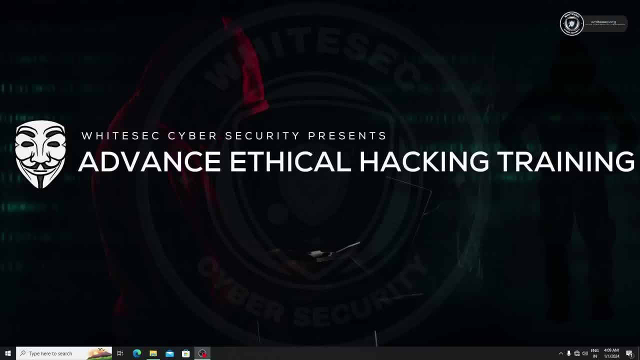 you have a nice day in this classes. we you have a nice day in this classes. we are learning about tcp and udp are learning about tcp and udp are learning about tcp and udp. protocols okay. protocols okay. protocols okay, with examples and i just showed you with examples and i just showed you. 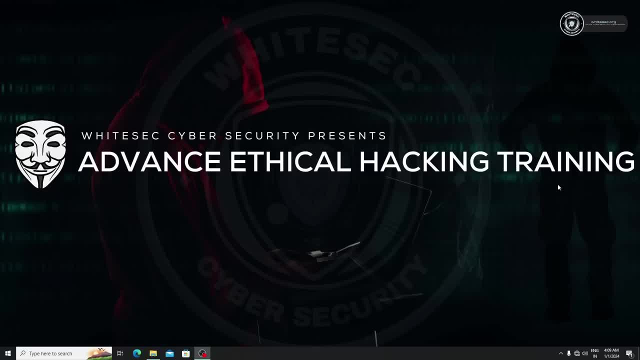 with examples and i just showed you practically, but still i'm gonna cover practically, but still i'm gonna cover practically, but still i'm gonna cover here as well, but the here as well, but the here as well, but the. i'm recommending you to watch that uh. 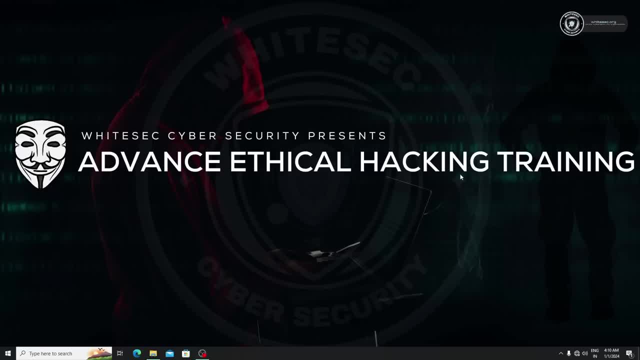 i'm recommending you to watch that. uh, i'm recommending you to watch that. uh, course as well. okay, which is very course as well. okay, which is very course as well. okay, which is very excellent. just watch it in 1.5. excellent, just watch it in 1.5. 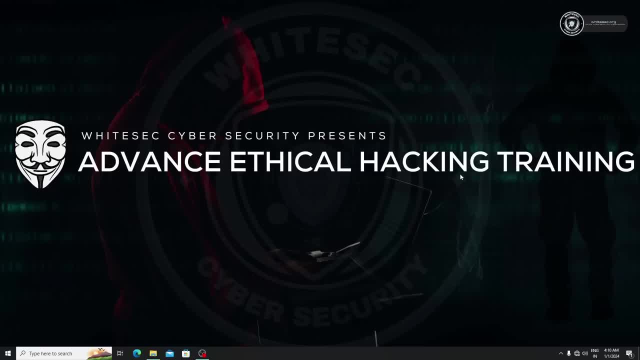 excellent, just watch it in 1.5- 2x. okay, because uh 2x, okay, because uh 2x, okay, because uh, if you watch in this uh speed, then you, if you watch in this uh speed, then you, if you watch in this uh speed, then you will get that properly. now, here the 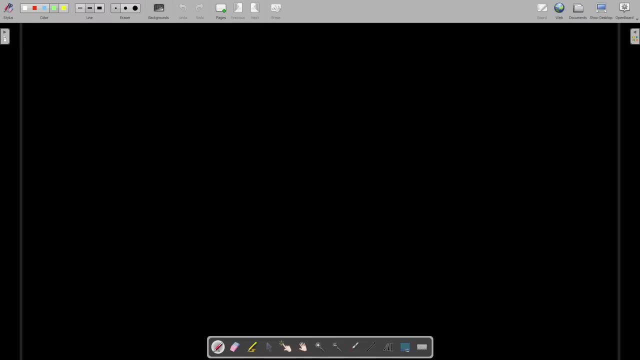 will get that properly now here. the will get that properly now here. the thing is: let's learn about tcp and udp. thing is: let's learn about tcp and udp. thing is: let's learn about tcp and udp. ports, ports, ports. see, tcp is nothing but transmission. see, tcp is nothing but transmission. 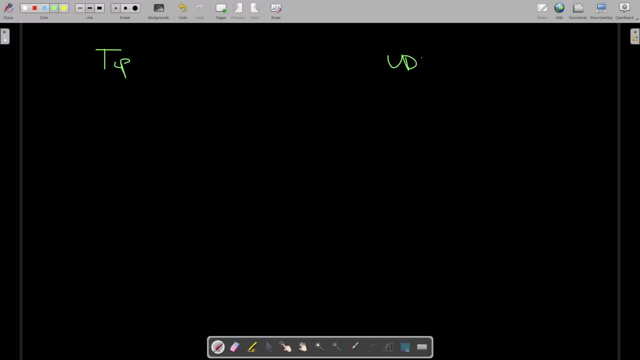 see, tcp is nothing but transmission control protocol and udp is nothing but control protocol and udp is nothing but control protocol and udp is nothing but what user datagram protocol? what user datagram protocol? what user datagram protocol? okay, now let's learn with as a hacker. okay, now let's learn with as a hacker. okay, now let's learn with as a hacker point of view. see if you know how to point of view. see if you know how to point of view. see if you know how to generate a payload for. generate a payload for. 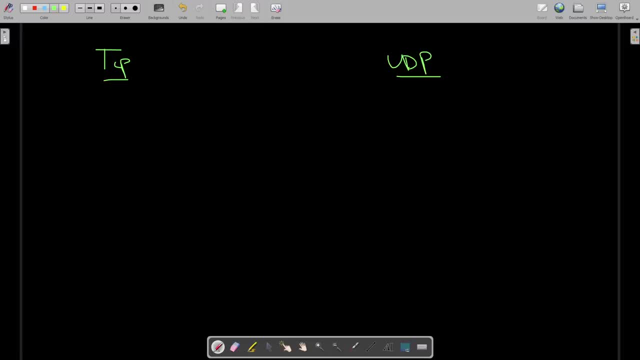 generate a payload for to hack android or to hack windows. you to hack android or to hack windows. you to hack android or to hack windows. you will get it okay. assume that i want to will get it okay. assume that i want to. will get it okay. assume that i want to hack the android by. 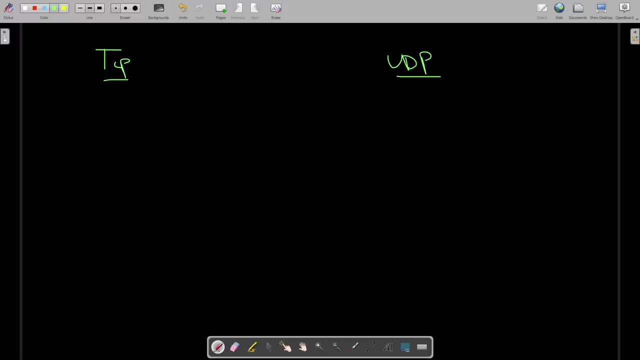 hack the android by hack the android by by using uh msf venom. okay, i want to by using uh msf venom. okay, i want to by using uh msf venom. okay, i want to generate the payload. generate the payload. generate the payload by using msf venom to hack android. 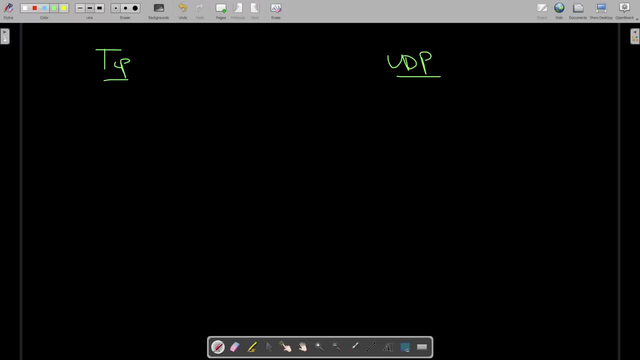 by using msf venom to hack android. by using msf venom to hack android. simple, which command i execute there. simple, which command i execute there. simple, which command i execute there. just focus on this command. i just type msf. just focus on this command. i just type msf. 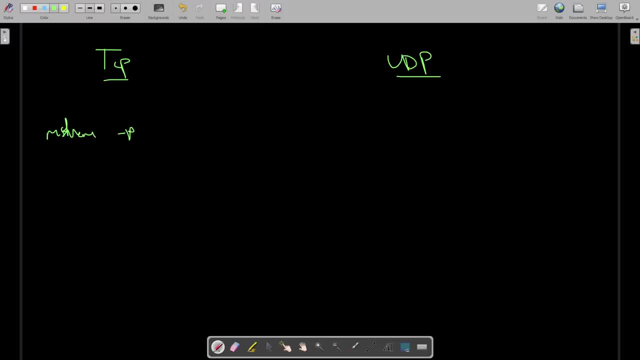 just focus on this command. i just type msf: venom, venom- venom using tcp. why we use this one? because the using tcp. why we use this one? because the using tcp. why we use this one? because the tcp is stable. tcp is stable. tcp is stable, okay, okay. 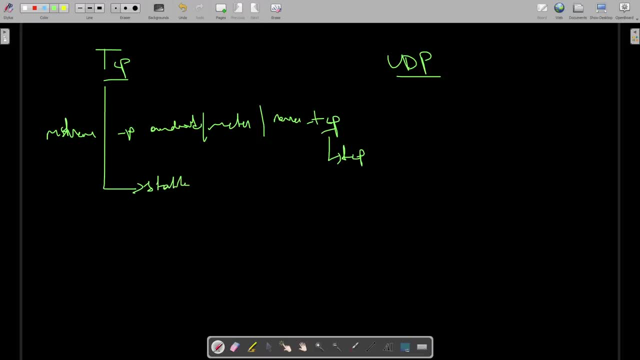 okay, it's stable. assumed that it's stable. assumed that it's stable. assumed that i just created the payload by using the. i just created the payload by using the. i just created the payload by using the tcp protocol here, okay and after. tcp protocol here, okay and after. 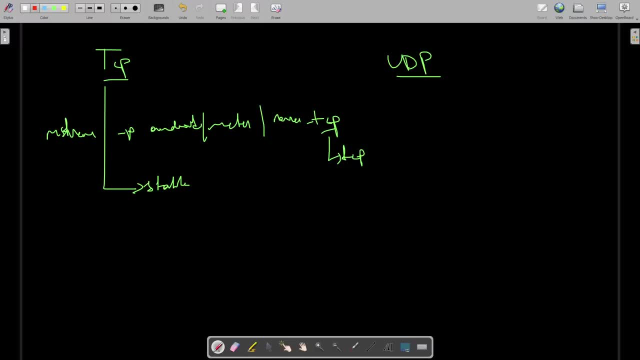 tcp protocol here. okay, and after generating the payload, i just send it to generating the payload. i just send it to generating the payload, i just send it to my target machine. this is my target, my target machine, this is my target, my target machine. this is my target machine or target android. i just send it. 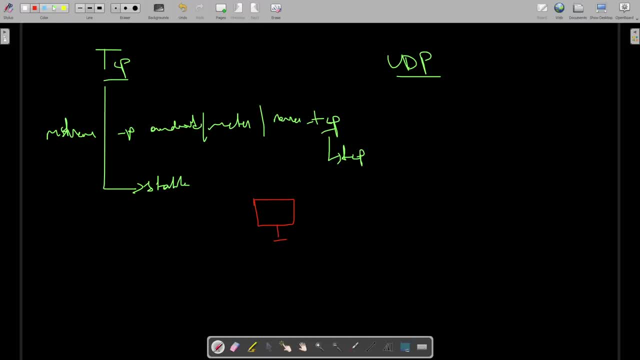 machine or target android. i just send it. machine or target android. i just send it the payload. see, here is the attacker. the payload: see, here is the attacker. the payload. see, here is the attacker. okay, i just send it the payload to this. okay, i just send it the payload to this. 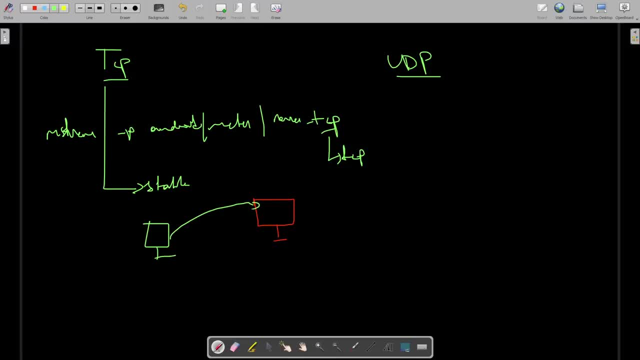 okay, i just send it the payload to this target machine now the main scenario. why target machine now the main scenario? why target machine now the main scenario? why attacker hack any system or any? uh attacker hack any system or any uh attacker hack any system or any uh android simple to spy or to download any 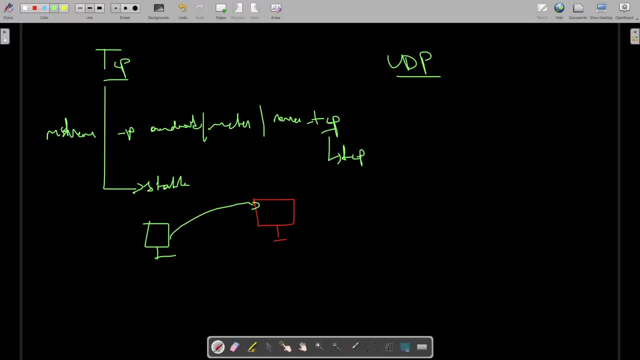 android simple to spy or to download any android simple to spy or to download any files from it. files from it. files from it now. i want to download the file from my now. i want to download the file from my now. i want to download the file from my target machines, the private file like. 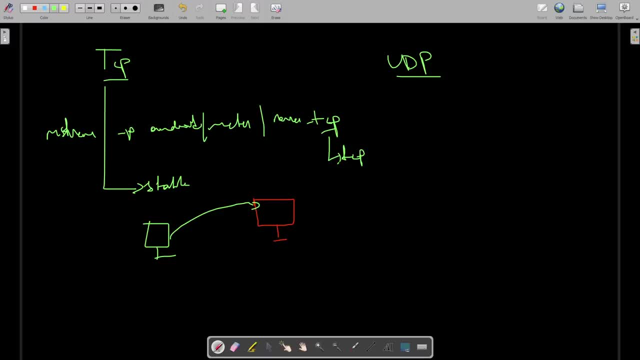 target machines. the private file like target machines. the private file like documents or something like that: simple documents or something like that- simple documents or something like that simple at that time. this play, this tcp play a at that time. this play, this tcp play a at that time. this play, this tcp play a very important role. okay, like i can able. 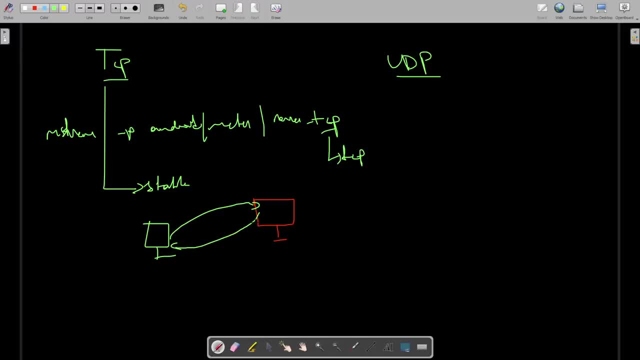 very important role. okay, like i can able. very important role: okay, like i can able to download the files from my victim. to download the files from my victim. to download the files from my victim machine. okay, like without any issue machine. okay, like without any issue machine. okay, like without any issue, without any errors. okay, the connection. 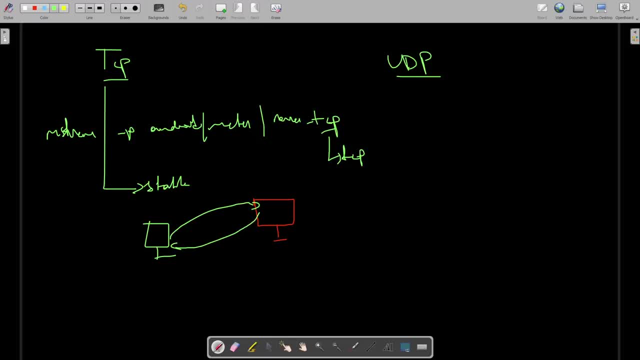 without any errors. okay, the connection without any errors. okay, the connection will be properly set up. okay, it's a will be properly set up. okay, it's a will be properly set up. okay, it's a- persistent- i can able to download it. okay, persistent- i can able to download it okay. 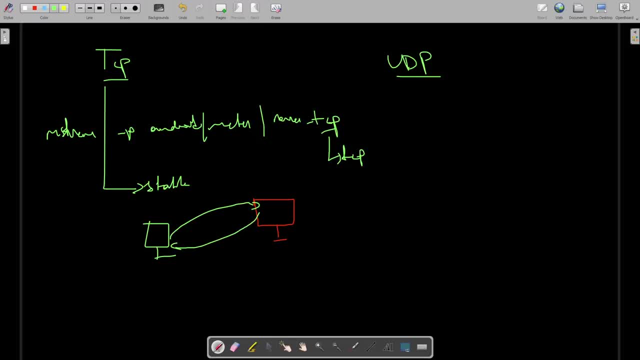 persistent, i can able to download it. okay, this is the thing it doesn't give any. this is the thing it doesn't give any. this is the thing it doesn't give any kind of issues. okay, assume that i want kind of issues. okay, assume that i want. 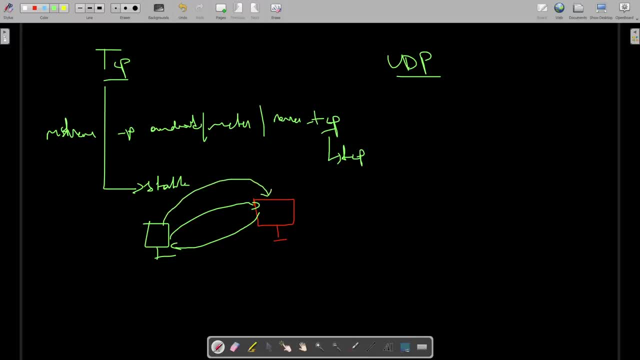 kind of issues. okay, assume that i want to upload some malicious files or any. to upload some malicious files or any. to upload some malicious files or any file to my target machine. at that time i file to my target machine. at that time i file to my target machine. at that time i can also upload the files using this. 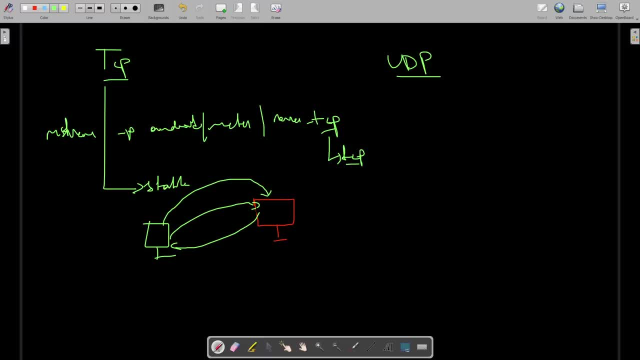 can also upload the files using this, can also upload the files using this protocol, because this one is a stable protocol, because this one is a stable protocol, because this one is a stable. assume that i want to upload my. assume that i want to upload my. assume that i want to upload my malicious file in my target download. 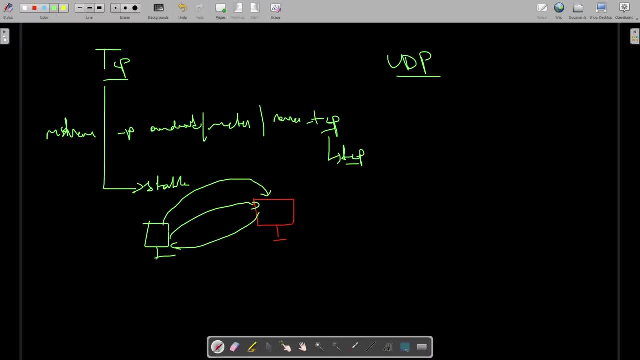 malicious file in my target download. malicious file in my target download directory: okay. download folder at that directory: okay. download folder at that directory: okay. download folder at that time. simple. i can give the command time simple. i can give the command time simple. i can give the command something like upload. and if i give the 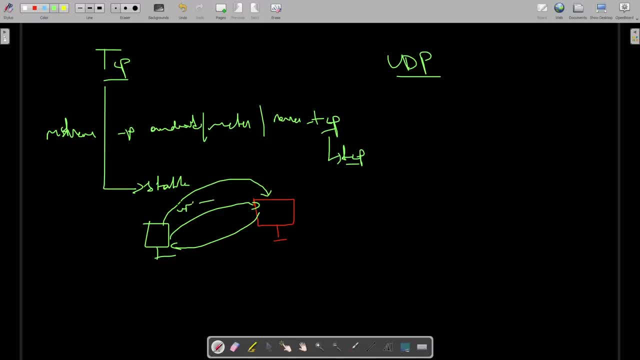 something like upload and if i give the something like upload and if i give the proper location, then it will upload proper location, then it will upload proper location, then it will upload. it will upload the files in attackers. it will upload the files in attackers. it will upload the files in attackers the this specific location which we just 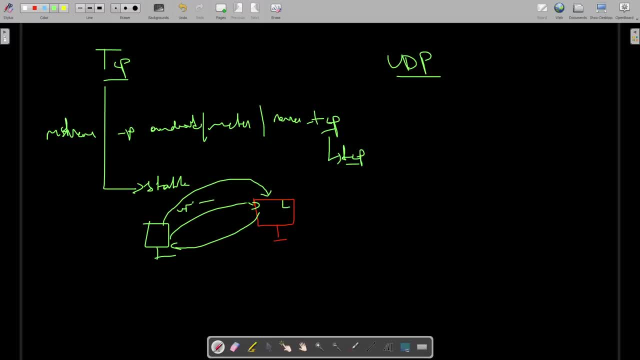 the this specific location which we just the, this specific location which we just given there. okay, given there. okay, given there. okay, so this work properly. if you use udp, so this work properly. if you use udp, so this work properly. if you use udp, then it won't work like that. okay, udp. 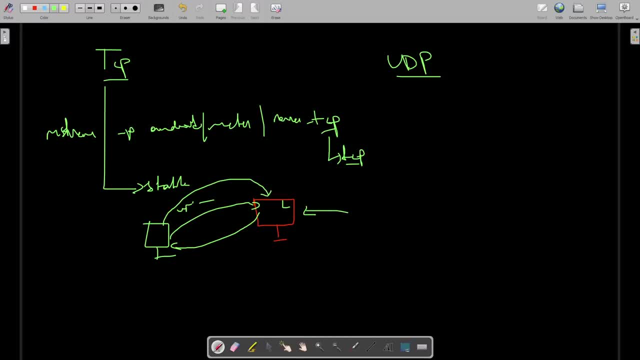 then it won't work like that, okay, udp. then it won't work like that, okay, udp. you won't have any kind of guarantee that you won't have any kind of guarantee that you won't have any kind of guarantee that your file will upload in your target. 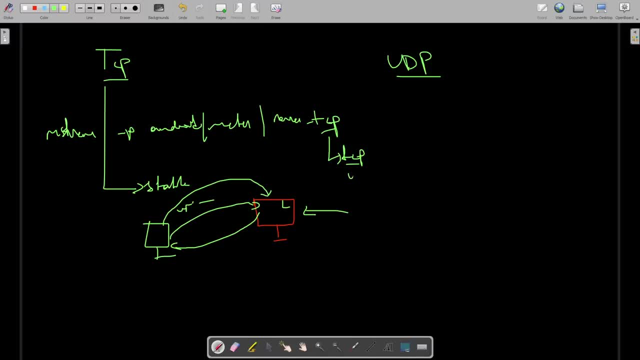 your file will upload in your target. your file will upload in your target machine. assume that, instead of tcp you machine. assume that, instead of tcp, you machine. assume that, instead of tcp you, you are using the udp here. you are using the udp here. you are using the udp here. okay then. 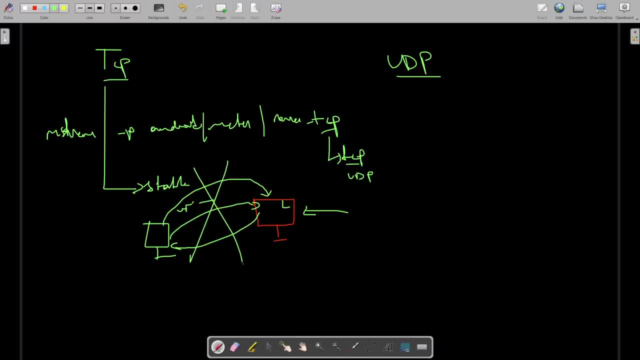 okay, then. okay, then there is, there is, there is no chances okay, no chances okay, no chances okay. maybe sometimes it may upload, maybe, maybe sometimes it may upload, maybe maybe sometimes it may upload, maybe sometimes it won't okay, sometimes it won't okay, sometimes it won't okay. maybe assume that you just given the proper. 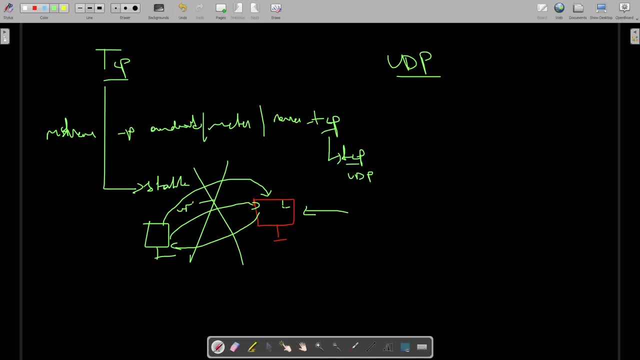 maybe assume that you just given the proper. maybe assume that you just given the proper. location to location to location to upload the file there: okay in that. upload the file there. okay in that. upload the file there. okay in that. udp here: okay. uh, we, we won't generate the. 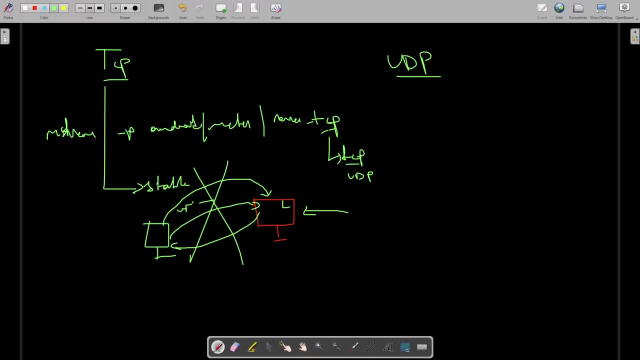 udp here. okay, uh, we, we won't generate the udp here, okay, uh, we, we won't generate the payload using udp or something like that. payload using udp or something like that. payload using udp or something like that. but let me tell you, udp is very fast. but let me tell you, udp is very fast. 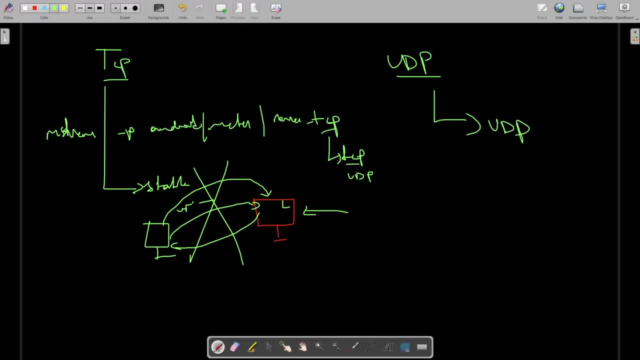 but let me tell you, udp is very fast. okay, udp is very fast. but comparing to okay, udp is very fast. but comparing to okay, udp is very fast. but comparing to tcp: okay, tcp is slow, it's a fast. okay, tcp- okay, tcp is slow, it's a fast okay. 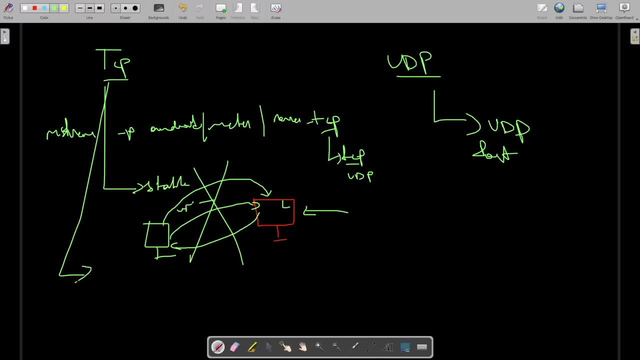 tcp: okay, tcp is slow. it's a fast. okay, udp is fast and tcp is slow. by comparing: udp is fast and tcp is slow. by comparing: udp is fast and tcp is slow by comparing to udp: okay, it's fast to udp. okay, it's fast to udp, okay, it's fast. and the second thing is: let me tell you: 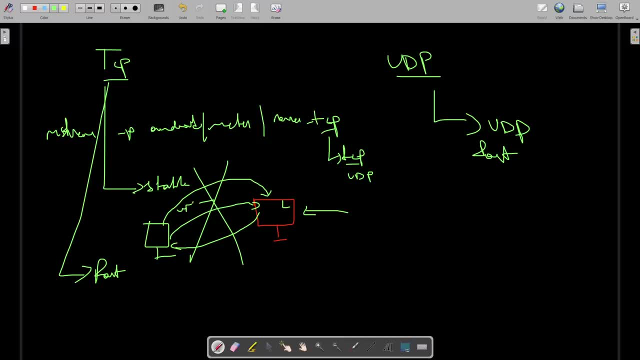 and the second thing is, let me tell you, and the second thing is, let me tell you, uh uh, uh, if you watch the open ports pentesting, if you watch the open ports pentesting, if you watch the open ports pentesting training, which is in this channel, okay, 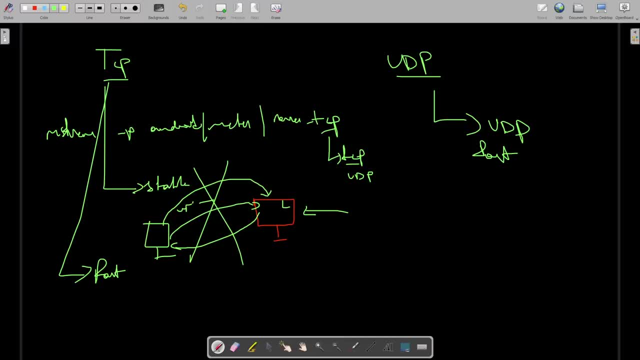 training which is in this channel. okay, training which is in this channel. okay, we just added a lot of trainings here. we just added a lot of trainings here. we just added a lot of trainings here. just try to watch it okay. just try to watch it okay. 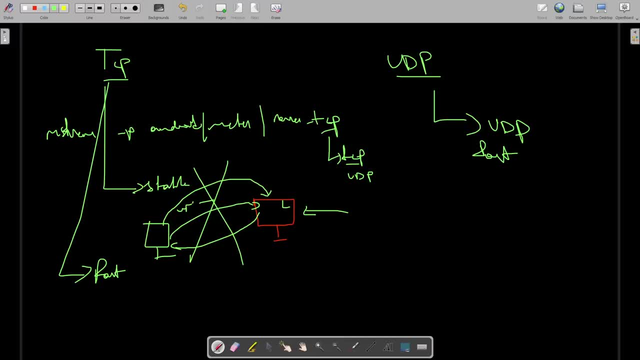 just try to watch it. okay, uh, there, we just perform the pentesting. uh, there, we just perform the pentesting. uh, there, we just perform the pentesting on open ports, on open ports, on open ports like ftp. okay, smtp ssh like ftp. okay, smtp ssh like ftp. okay, smtp ssh, something like that, okay. so basically, 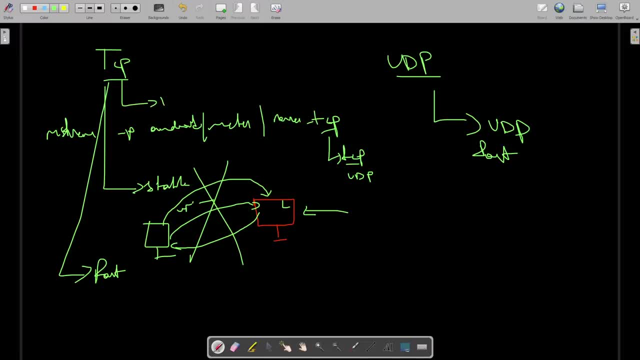 something like that. okay. so, basically, something like that, okay. so basically, this ports okay, which create the. this ports okay, which create the. this ports okay, which create the connections, such as ftp port. can connections such as ftp port, can connections such as ftp port can create the connection right ssh create. 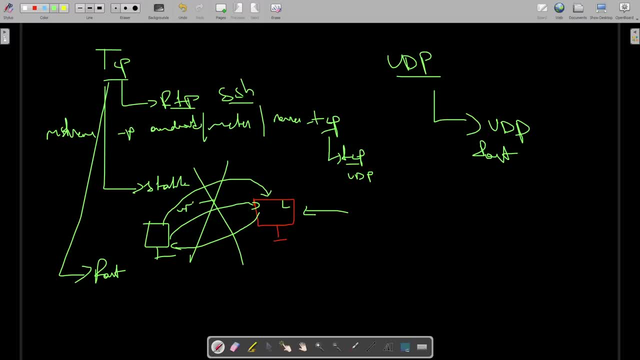 create the connection right: ssh. create. create the connection right: ssh. create the connection. because by using this the connection, because by using this the connection, because by using this ports uh services i can able to connect ports uh services, i can able to connect ports uh services, i can able to connect wirelessly to the. 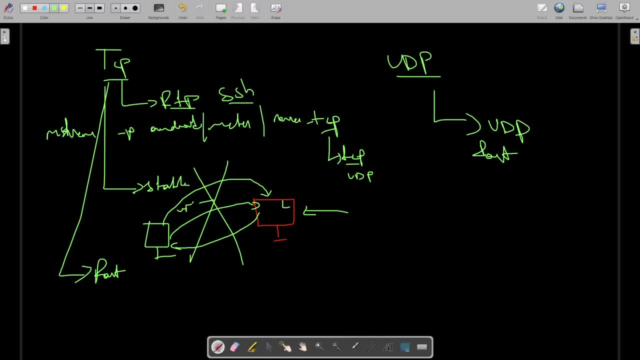 wirelessly to the, wirelessly to the machine- okay, this is a thing more this machine- okay, this is a thing more this machine- okay, this is a thing more. this kind of protocols will work on tcp- okay. kind of protocols will work on tcp- okay. kind of protocols will work on tcp- okay. and in udp we can able to see dns- okay. 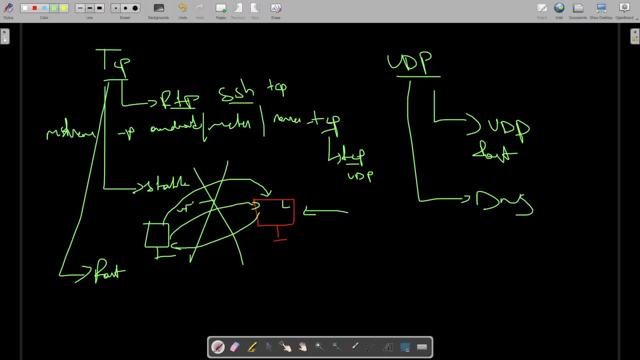 and in udp we can able to see dns okay, and in udp we can able to see dns okay. domain name server. domain name server. domain name server. okay, and you can also see it uh in okay, and you can also see it uh in: okay, and you can also see it uh in zoom application. is there right which? 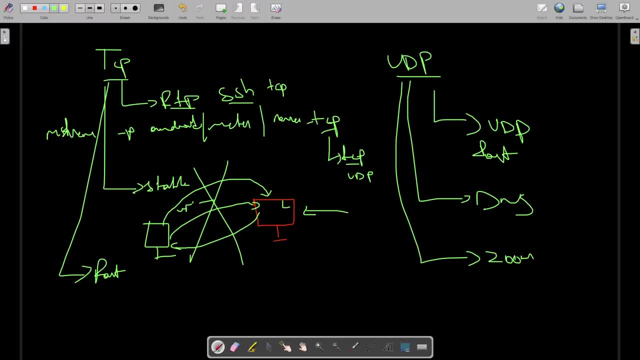 zoom application is there right? which zoom application is there right which uh take live classes or something like uh take live classes or something like uh take live classes or something like that. it's also work with udp, mostly the that. it's also work with udp, mostly the. 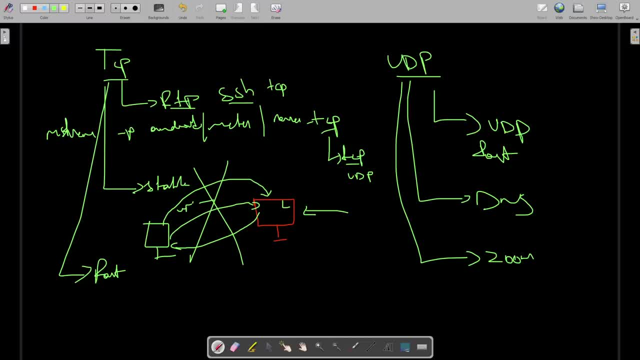 that it's also work with udp. mostly the things which are live okay, like video, things which are live okay, like video, things which are live okay, like video, live streaming. it's totally depend upon live streaming. it's totally depend upon live streaming. it's totally depend upon udp okay. 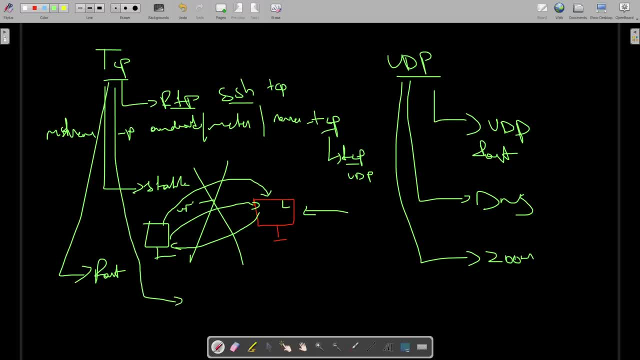 udp, okay, udp, okay. and in tcp you guys can also take an and in tcp you guys can also take an. and in tcp you guys can also take an example. or recorded videos like uh, there example. or recorded videos like uh, there example. or recorded videos like uh, there is a netflix by default in netflix. what? 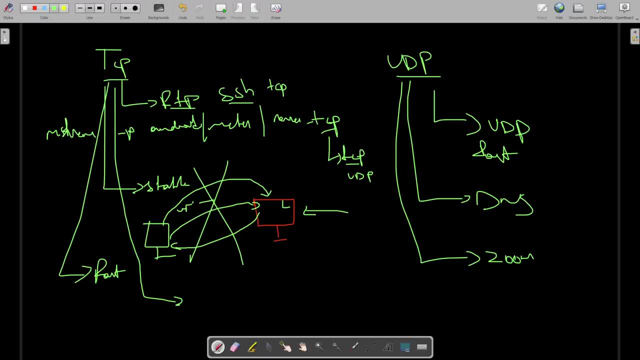 is a netflix by default in netflix. what is a netflix by default in netflix? what will happen? it's not a live right simple will happen. it's not a live right- simple will happen. it's not a live right simple. it's totally depend upon me which it's. 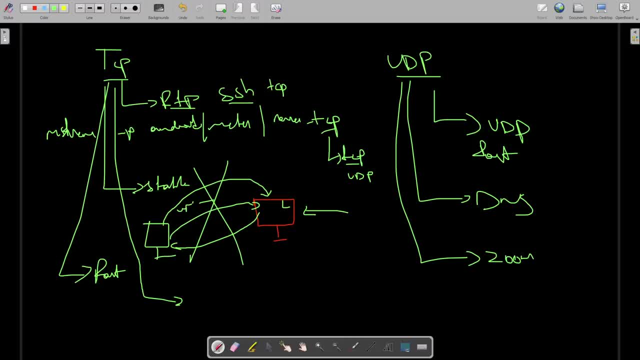 it's totally depend upon me which it's. it's totally depend upon me, which it's already there, right, already there, right, already, there, right, to watch the windows penetration testing, to watch the windows penetration testing, to watch the windows penetration testing training. you will get it okay. 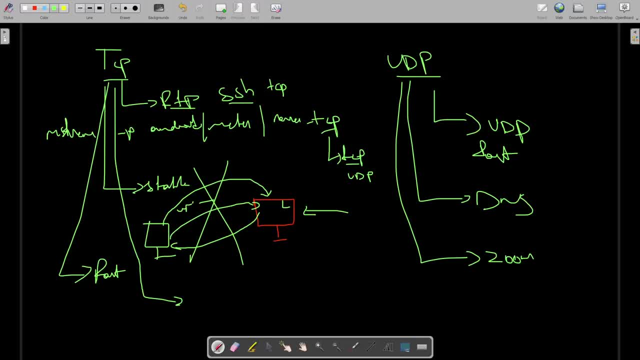 training: you will get it okay. training: you will get it okay. don't watch a complete. uh, do one thing. don't watch a complete. uh, do one thing. don't watch a complete. uh, do one thing. complete this training, then watch that. complete this training, then watch that. 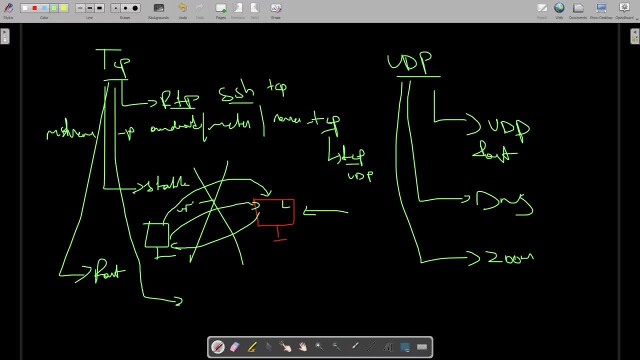 complete this training then watch that one okay. one okay. one okay. hope you guys enjoyed this class. thank hope you guys enjoyed this class. thank hope you guys enjoyed this class. thank you, have a nice day now in this classes. you have a nice day now in this classes. 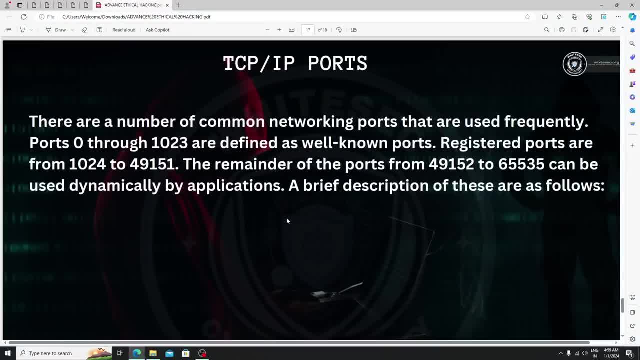 you have a nice day now in this classes, we are learning about, we are learning about, we are learning about ports. right, let me tell you in this ports right, let me tell you in this ports right, let me tell you in this class, in this class, in this. 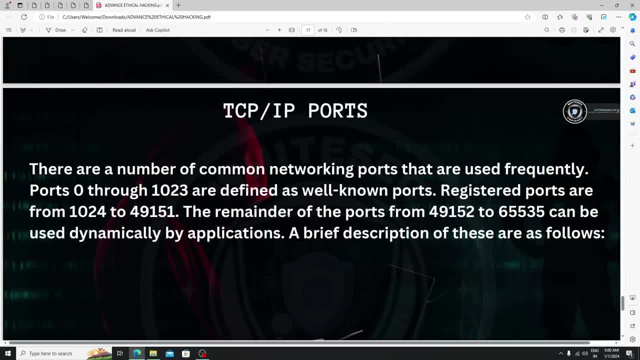 class in this youtube channel. you guys can able to see youtube channel. you guys can able to see youtube channel. you guys can able to see a complete training about a complete training, about a complete training about how you guys can able to exploit open, how you guys can able to exploit open. 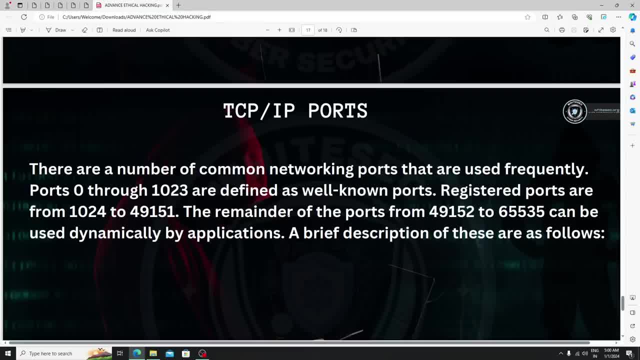 how you guys can able to exploit open ports, right so simple ports, right so simple ports, right so simple. after watching this training, just try to. after watching this training, just try to. after watching this training, just try to watch it, because we just covered a lot of. watch it, because we just covered a lot of. 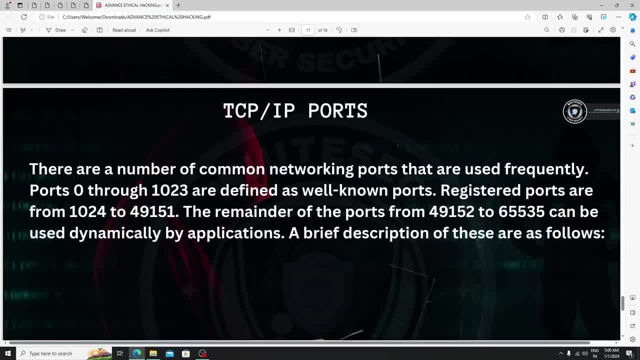 watch it, because we just covered a lot of things there: how to exploit a different things there, how to exploit a different things there, how to exploit a different services- each and everything now here. services. each and everything now here. services. each and everything now here. the thing is: 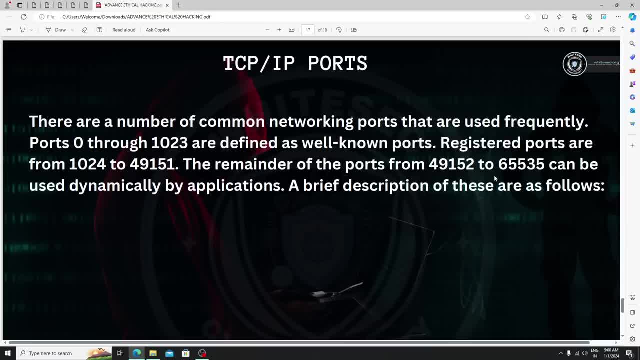 the thing is. the thing is: let's learn first of all, let me tell, let's learn first of all, let me tell, let's learn first of all. let me tell you: in our machine, okay, in our system, you in our machine. okay, in our system, you in our machine, okay, in our system. there are around three, six, five, five. 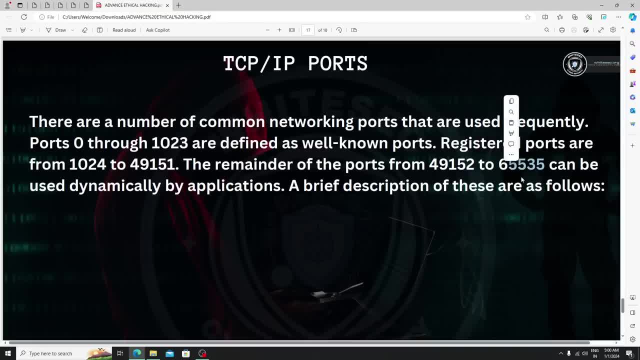 there are around three, six, five, five. there are around three, six, five, five, three, three, five ports are there okay? three, three, five ports are there okay? three, three, five ports are there okay? sixty five thousand five hundred thirty sixty five thousand five hundred thirty sixty five thousand five hundred thirty five ports are there okay, in our machine. 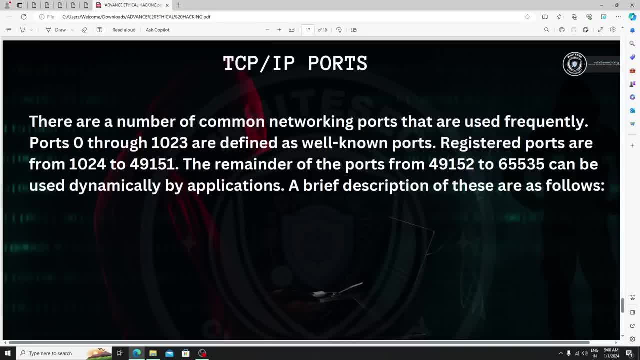 five ports are there, okay, in our machine? five ports are there okay in our machine? basically, uh, there are udp and tcp ports, basically, uh, there are udp and tcp ports. basically, uh, there are udp and tcp ports, both right here, both right here, both right here. this, this ports are divided into three. 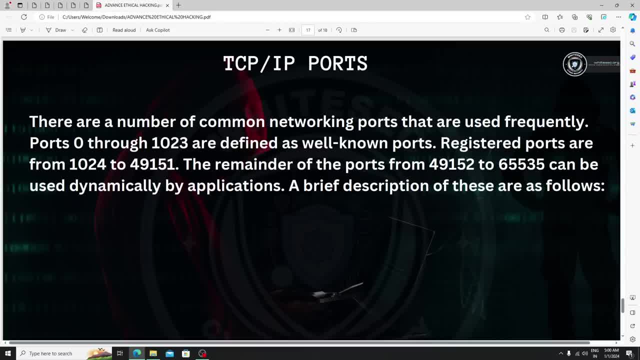 this: this ports are divided into three. this ports are divided into three categories: one is uh, which is known as categories. one is uh, which is known as categories. one is uh, which is known as here. just see here. just see here, just see zero two. one zero two. three are defined. 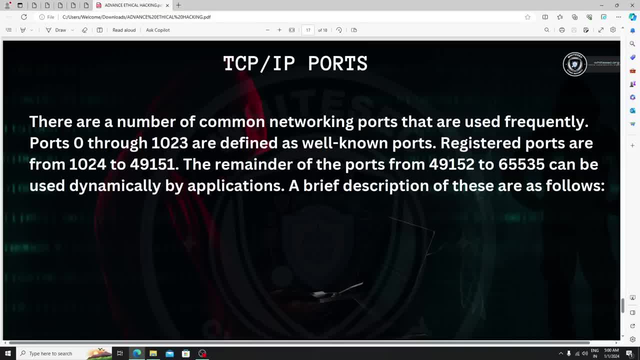 zero two, one, zero two, three are defined zero two, one, zero two, three are defined as well-known ports. okay, as well-known ports. okay, as well-known ports. okay, and uh 1024 to 49151 is known, uh from, and uh 1024 to 49151 is known, uh from. 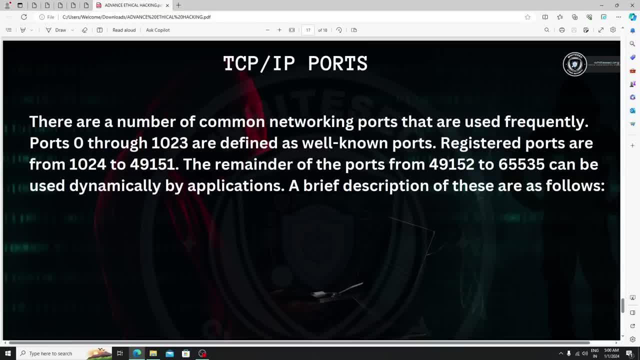 and uh 1024 to 49151 is known uh. from uh 1024 to 49151 is uh. uh. 1024 to 49151 is uh. uh. 1024 to 49151 is uh. is known as a register ports. okay, is known as a register ports, okay. 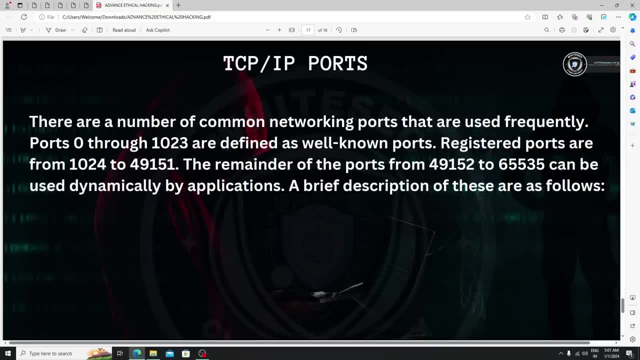 is known as a register ports. okay, and from 49152 to and from 49152 to and from 49152 to 65535 is known as dynamic ports. okay, basically is known as dynamic ports. okay, basically is known as dynamic ports. okay, basically, these ports are. 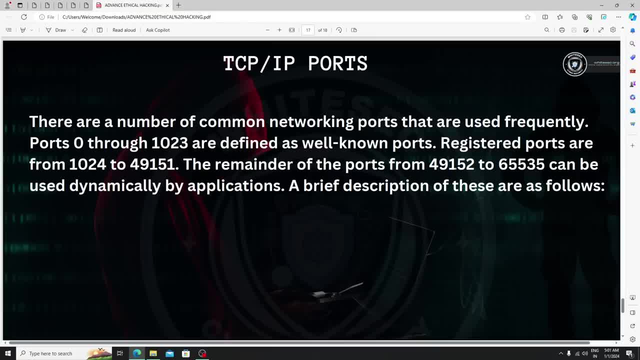 these ports are. these ports are, uh, less usable ports? okay, like no, uh, less usable ports, okay, like no, uh, less usable ports, okay, like no. services, services, services, okay, uh, the applications. okay, won't use, okay, uh, the applications. okay, won't use. okay, uh, the applications. okay, won't use this. ports from here to here, which is. 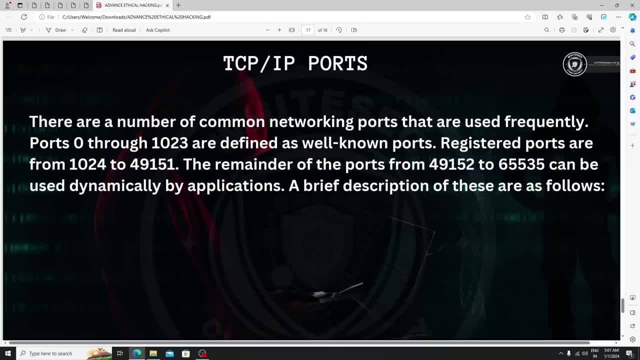 this ports from here to here, which is this ports from here to here, which is known as a dynamic ports? okay, known as a dynamic ports. okay, known as a dynamic ports. okay, these are not assigned with any specific. these are not assigned with any specific. these are not assigned with any specific purpose. this is a thing. 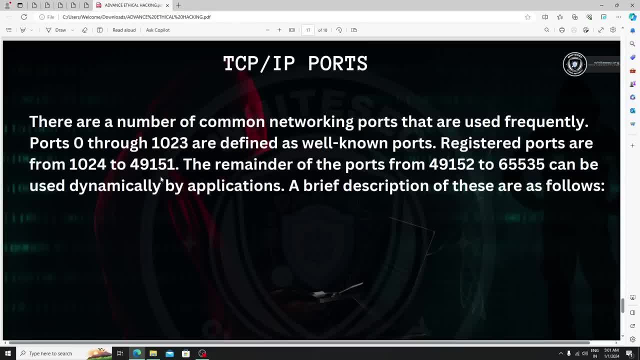 purpose, this is a thing. purpose, this is a thing. and here, basically, uh you can, these are, and here, basically, uh you can, these are, and here, basically, uh you can, these are the main things. uh from uh, the main things. uh from, uh, the main things. uh, from uh zero to uh one zero, two, three is a well. 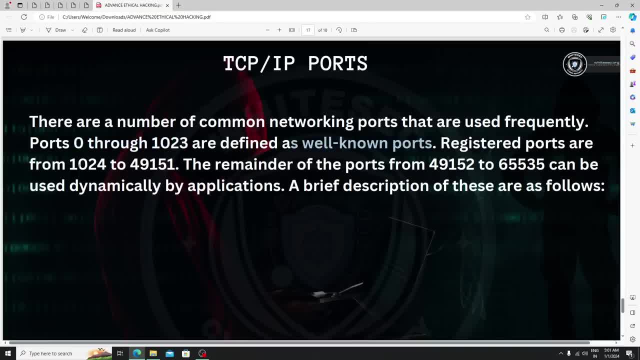 zero to uh. one, zero, two, three is a well zero to uh. one, zero, two, three is a well known- see here it's a well known ports known. see here it's a well known ports known- see here it's a well known ports. and one zero, two, four, two, four, nine, one. 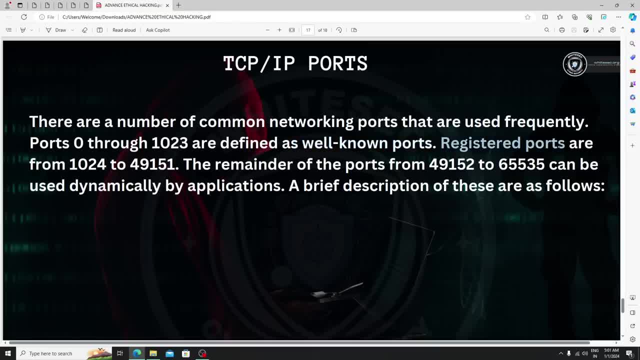 and one zero two, four, two, four, nine. one and one zero two, four, two, four, nine one, five one, five one, five one. is a register force. okay. is a register force. okay. is a register force. okay. assume that if any attacker use any uh. assume that if any attacker use any uh. 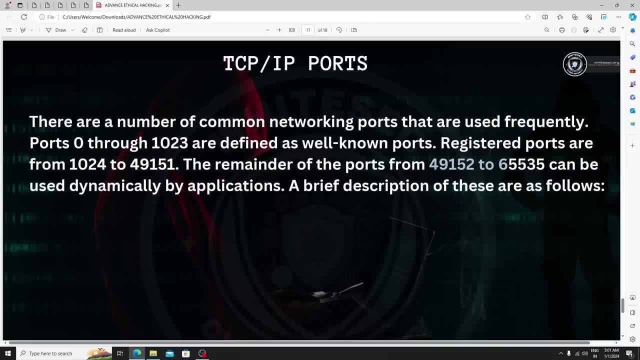 assume that if any attacker use any uh ports in between this thing, ports in between this thing, ports in between this thing, in between this range, then it is easy to to detect. okay, this is also one thing. just try to ignore it. you just need to learn about the ports. 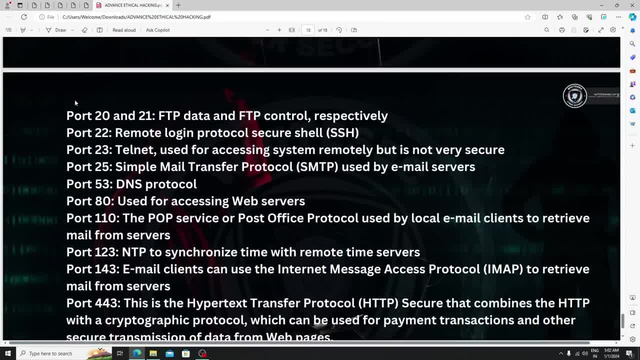 here. see here you can able to see there is a port 20 and port 21 is a ftp data, ftp port okay, which is a file transfer protocol, and 22 port 22 is remote login protocol, secure shell, which is known as a ssh. now ftp is useful for fight file transfer purpose. okay, like assume that i want to upload the. 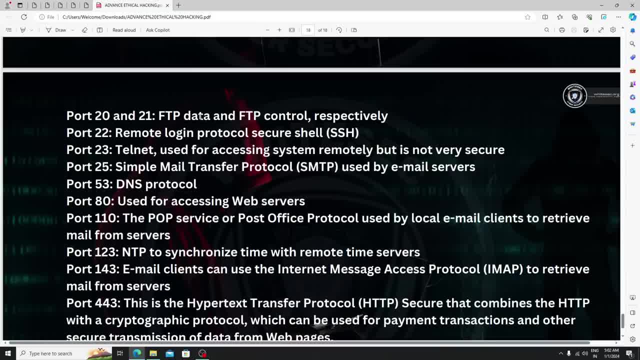 data in server. okay, at that time, by using ftp i can able to do it. okay, and there is a uh ssh. assume that i want to connect this system wirelessly. at that time, i'm gonna use the ssh there. okay, this is a basically services, right, and there is a telnet used for as. sorry guys. 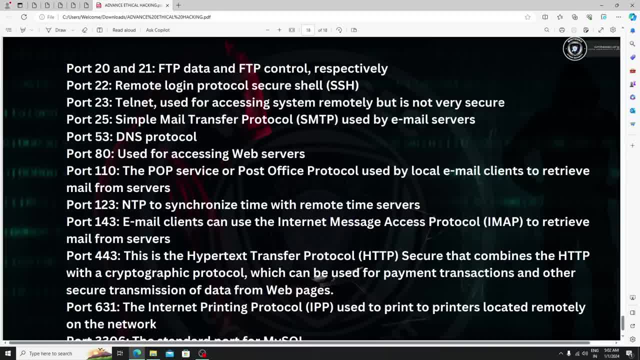 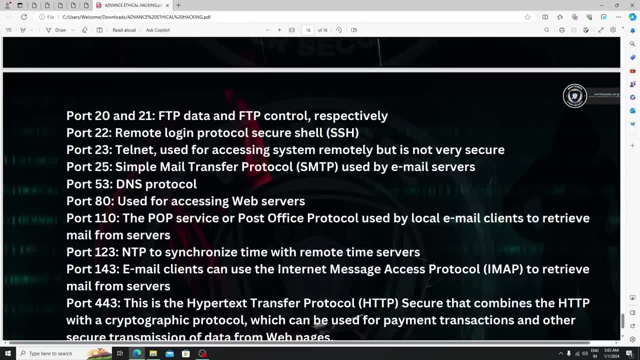 accessing system remotely, but it's not very secure. the thing is, uh, if you know man in the middle, attack at that time, what? uh? if you know that, then you will get it, because here in telnet there is no security. assume that any attacker is uh in our network. he can able to sniff the credentials. 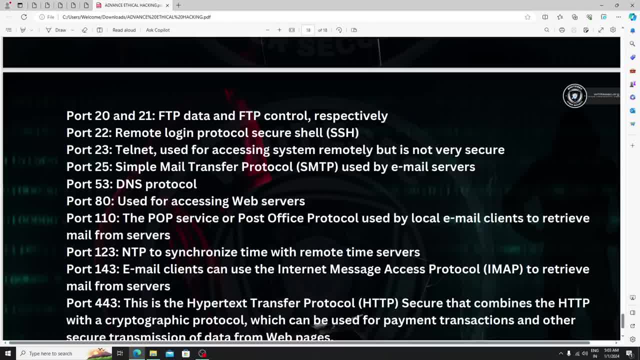 right, see, if you want to access telnet, then you need to type the password there. okay, this is the thing for ssh also, for ftp also. okay, this is the thing. uh, assume that you need to type the password there. okay, this is the thing for ssh, also for ftp also. 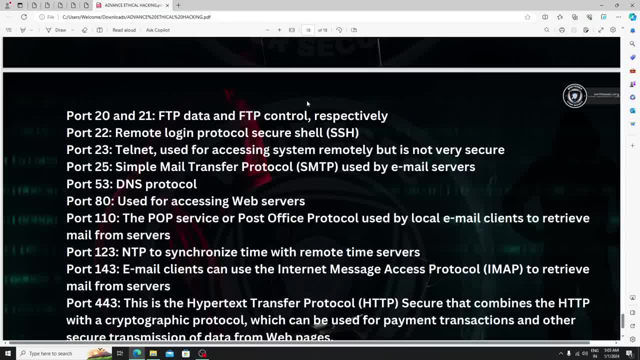 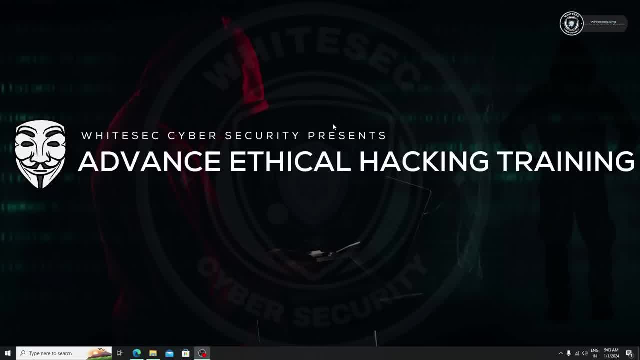 it's the same like the services. okay, uh, now assume that i want to connect with this machine through ssh. what i need to do simple: i need to provide the ip address of this machine. okay, then i need to provide the username. after entering that, it will ask for the password. what is the? 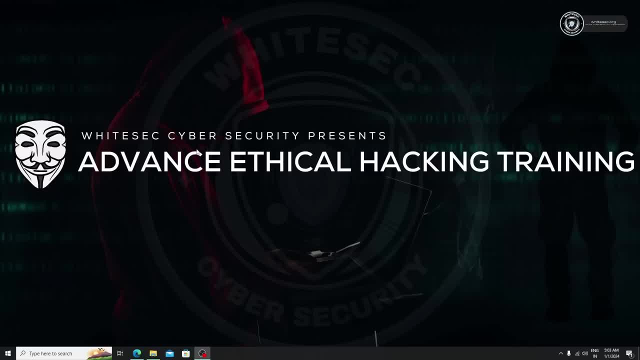 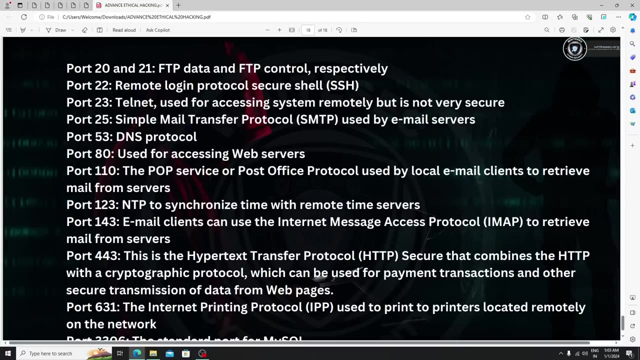 password. it will ask the password of this system, simple. after typing the password, i can able to access this machine wirelessly. this is a thing, right, but it's a secure. even the attacker is in your network, still he can't able to a sniff it because it this is encrypted, right, but telnet, uh, it's not like that the attacker. 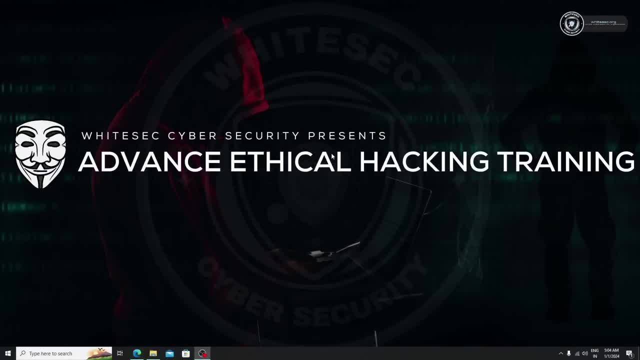 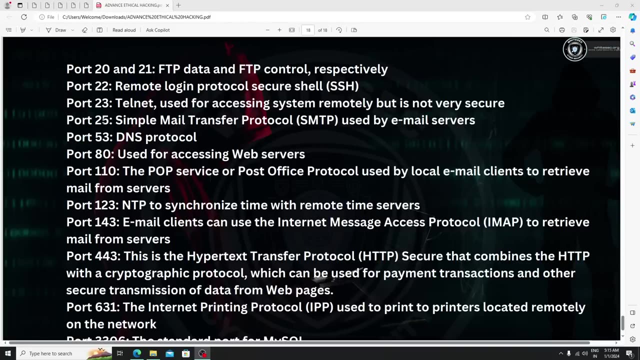 after, assume that there is a legit user- is typing the username and the password there and the hacker is in that network. simple, he can able to sniff that credentials. okay, this is by using tools, or- and here there is a smtp port is here- which use a tcp25 port. okay, 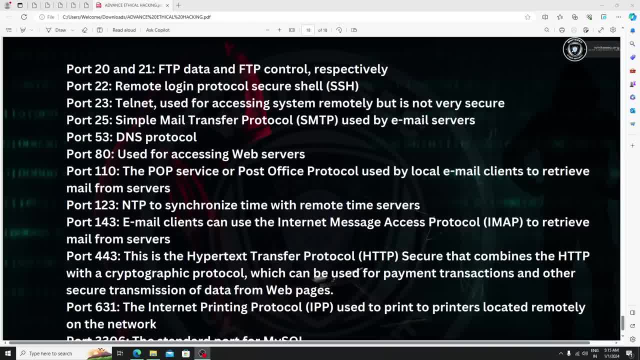 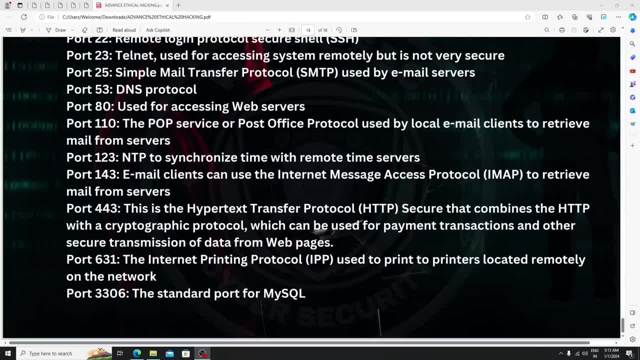 there is a dns protocol which use a 53 see dns pro dns will work on udp and tcp as well. this is the thing. there is a port 80 used for accessing web servers. right, just try to read it. there are. there are huge services, are there? okay, once you perform the nmap scanning, then you will get it. 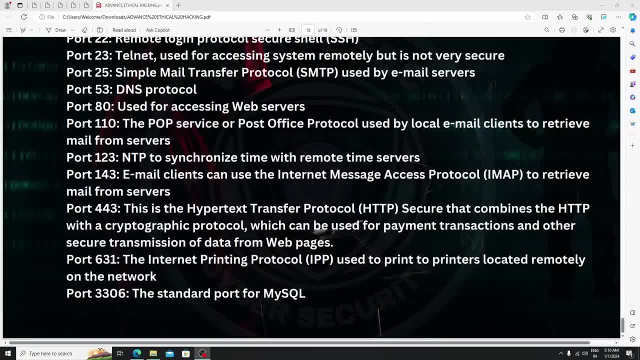 okay, which assume that you got the target you want to. mostly we do the scanning using the ip addresses, right? this is the thing. in rare cases we use the domain names- okay, but mostly we go with ip addresses. the simple thing is the that result will be same. okay, for domain and for ip. the result. 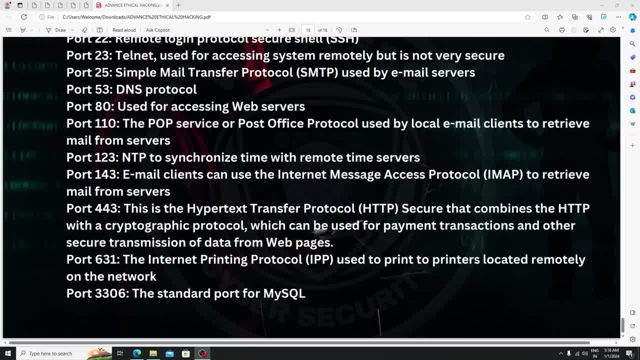 will be same, but sometimes it will be different. okay, sometimes you see some ports, sometimes you won't see it. okay, this is the thing. it's also depend upon your ip address as well. okay, if you are, if you are scanning, assume that there is a kind of firewall there. simple, they will ban. 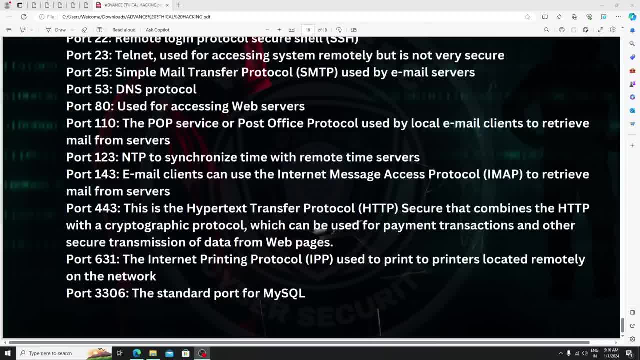 the firewall will ban the ip addresses your ip, okay. so that's why we do some evasion techniques there. if you watch our maybe in windows penetration testing training- we just covered that one. okay. again i am saying: first watch this training, then we jump for windows hacking training. 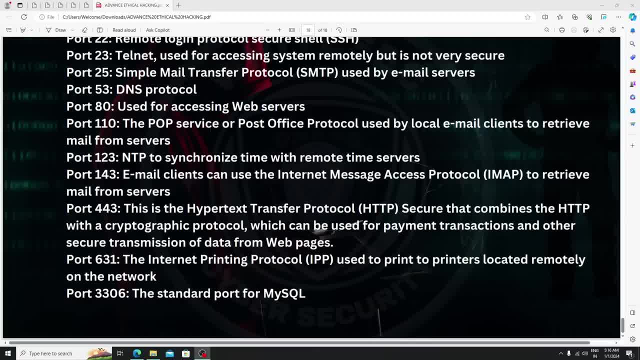 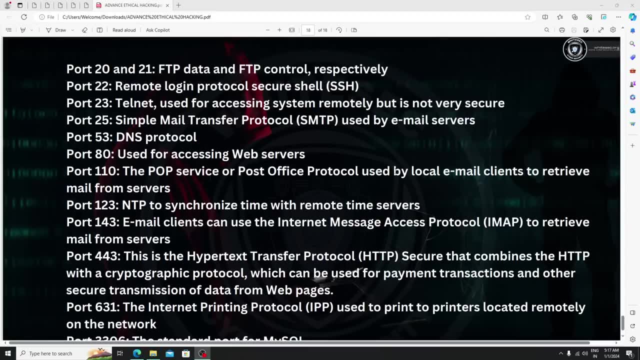 okay, which is very important for you guys, because there we just covered a complete basic pen testing, complete windows basic pen testing there. okay, just try to watch it. it's not a big deal, it is very easy. okay, right, hope you guys enjoy this classes now. maybe in the next classes. 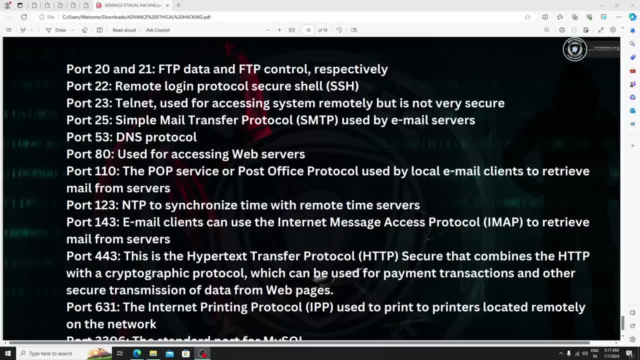 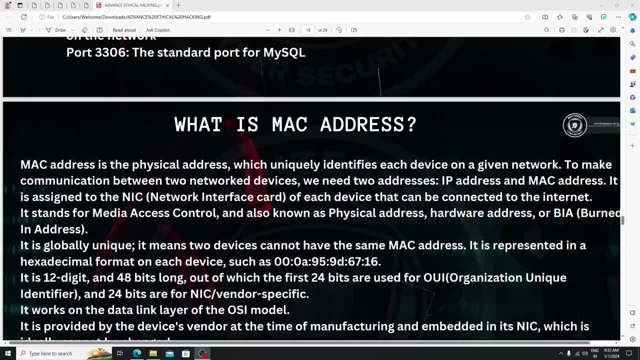 i'm gonna cover about mac addresses. okay, what is mac address? or something like that. hello guys, in this class we are learning about what is mac address. mac address is a physical address which uniquely identify each identifies each device on a given network to make communication between two. 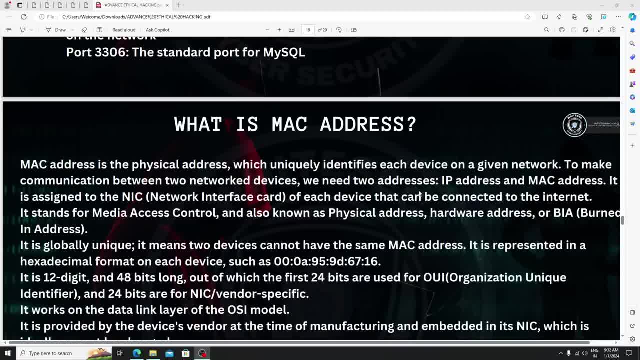 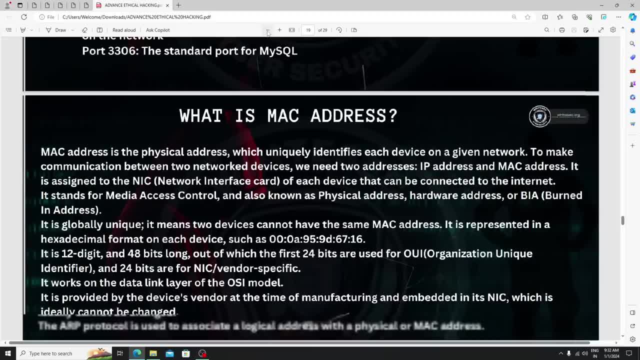 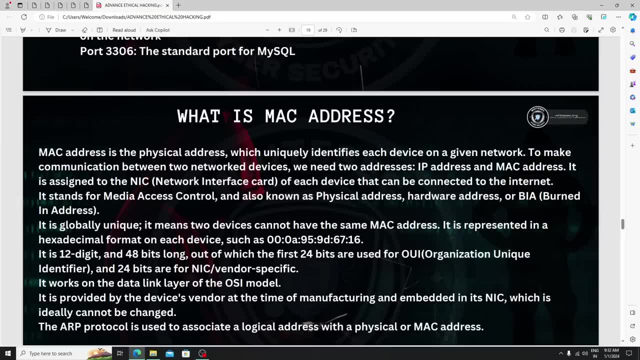 network devices. we need- sorry guys, we need two addresses: ip address and mac address. okay, just wait, let me. okay, now it's good, it is assigned to nic network interface card. what is network inter interface card here? network interface card is a nothing. but your adapter, okay, your wi-fi. 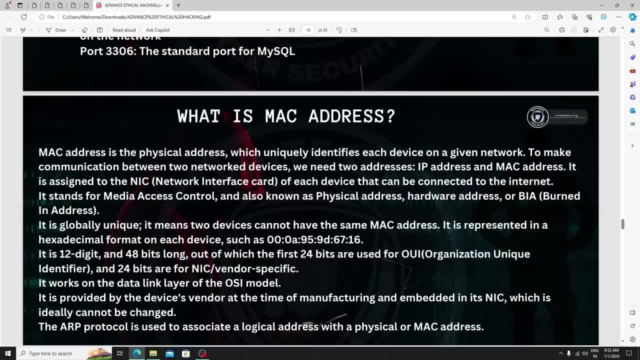 adapter. this is the thing of each device that can be connected to the network internet. it stands for media access control. the full form of mac is media access control and also known as a physical address, hardware address or bia. but in address okay, it is globally unique. it means two devices cannot have. 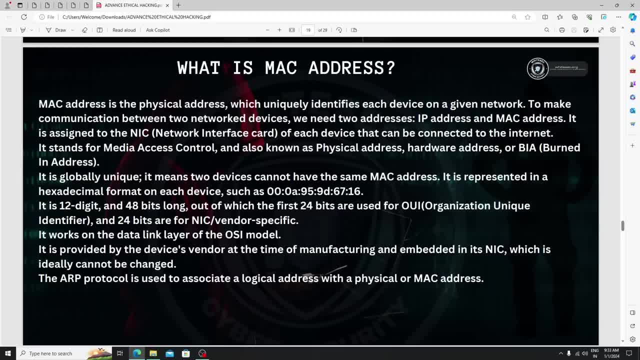 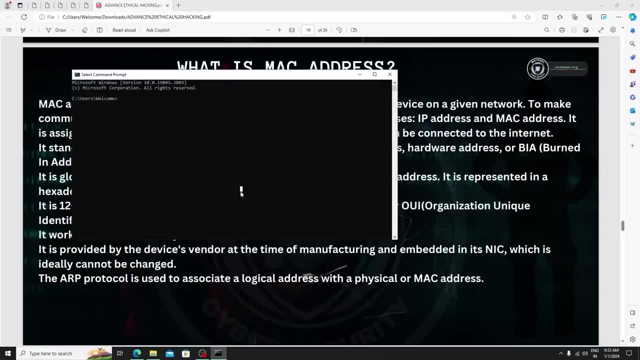 the same mac address. okay it, sorry guys, it is represented in a hexadecimal format on each device, such as like this: okay, let me show you. just wait. in my device, let me open cmd here and if, if i type ipconfig here, okay, i can see the mac address as well. 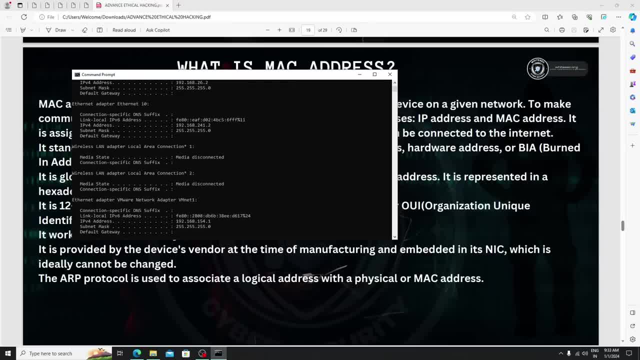 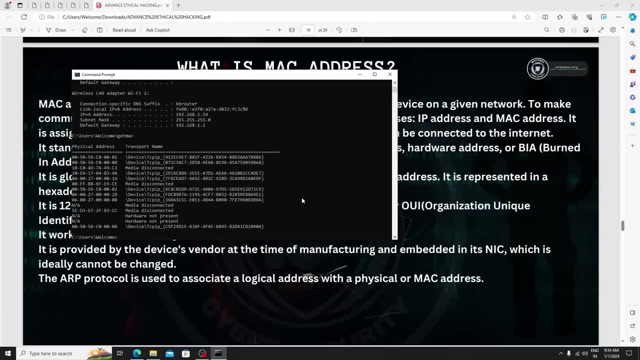 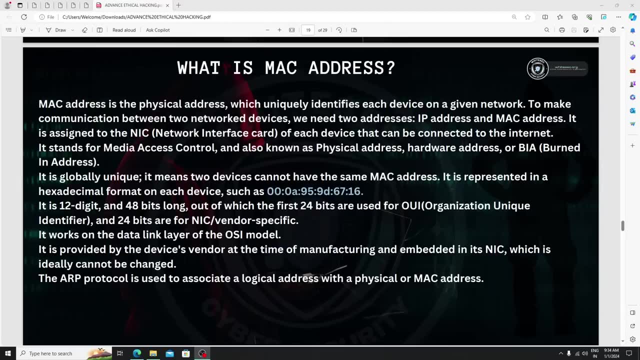 sorry, it's not linux right, so simple, let me type: get mac. okay. hope you guys can able to see. this is how the mac address look like. okay, it is 12 digit and 48 bit long, out of which the first 24 bit are used for. 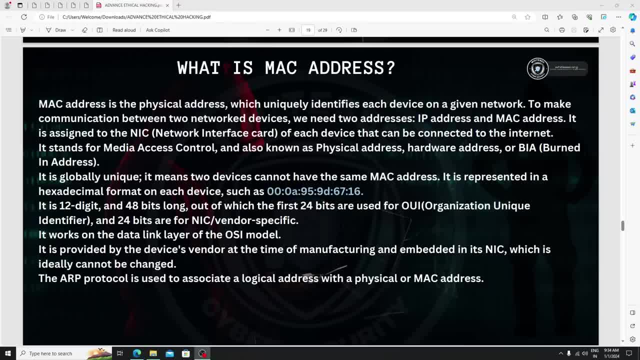 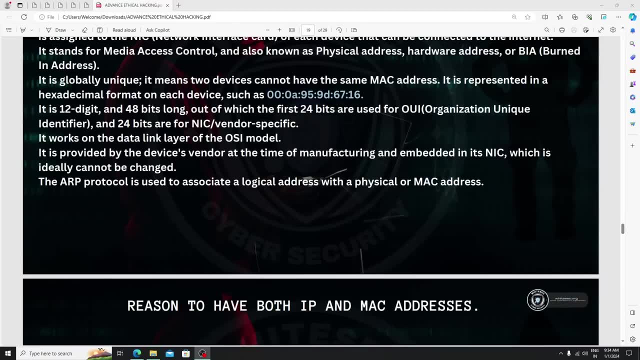 ui organization unique identifier. i'm gonna show you what the mac address looks like. this is this: oui as well, and 24 bit, or for i? uh, nic, network interface protocol. okay, sorry card, sorry man, network interface card. vendor specific it's, it's for a specific vendor. assume that if you. 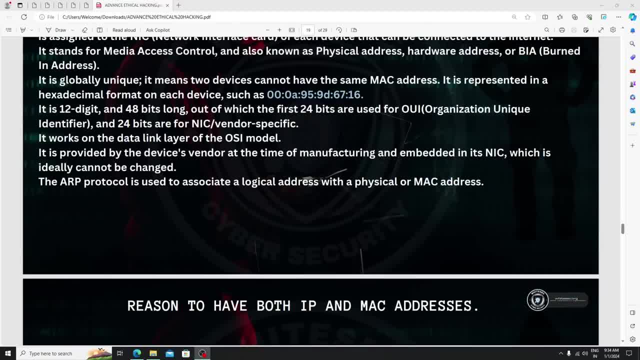 are using atl uh adapter or something like that, for that it will be different. okay, if you are using hui, then it will be different. let me show you. uh, we have the examples. examples as well, you will get it. okay. uh, it work on the data link layer of osi model. it is provided by the device vendor at the time of 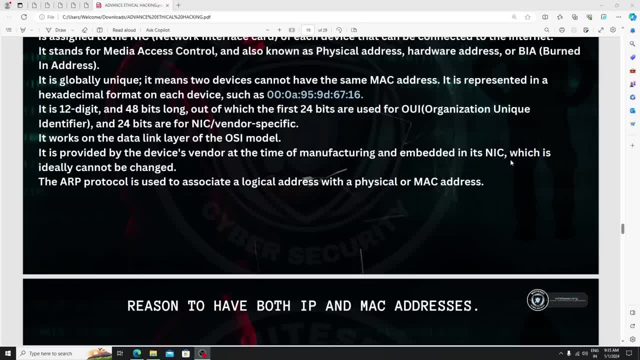 manufacturing and embedded in uh in its nic, which is ideally cannot be changed. the arp protocol is used to associate a logical address with a physical or mac address. basically, the thing is, ma you, you can't able to change some mac address. here you can able to, but still by using some tools. 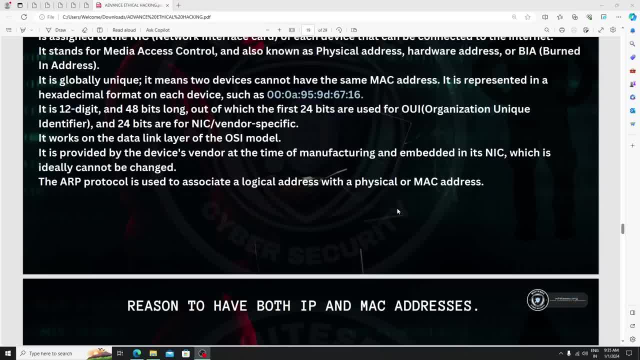 for limited time you guys can able to change it, but uh, it will change to uh by default. okay, once you restart, if you do some kind of activities, then it will be re-change. okay, this is the thing. it's not a big deal, it's a very easy process. i'm gonna. 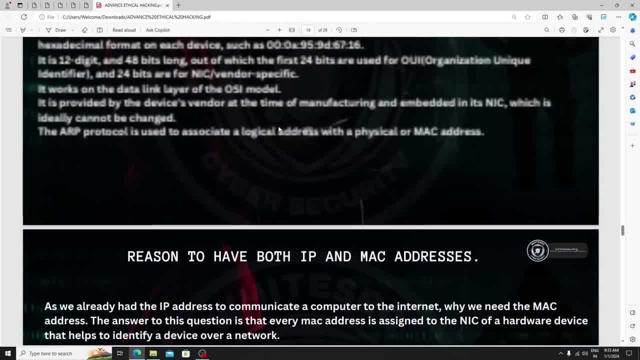 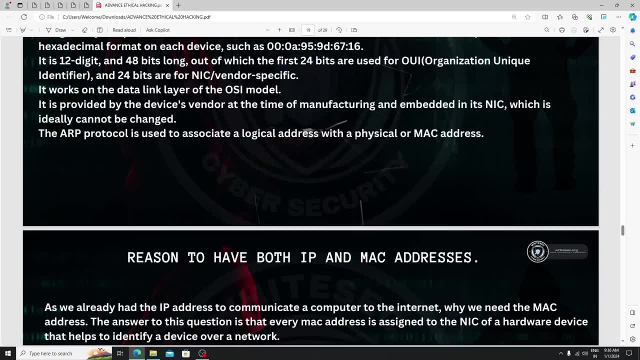 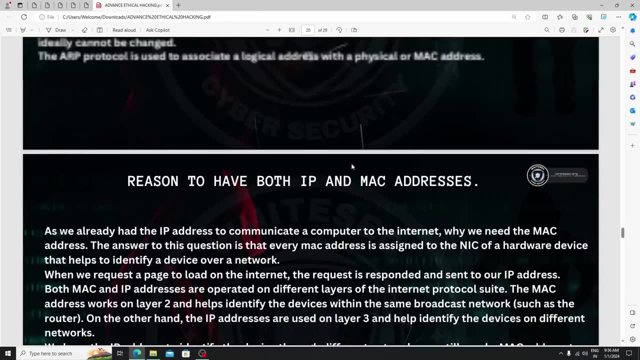 show you: okay, well, you, you can able to perform this mac address spoofing, this kind of attack using automation tools. okay, this is the thing. if you click one, uh, if you type one single command, the attack will work. okay, this is the thing. so that's why, uh, the thing is, you need to focus on 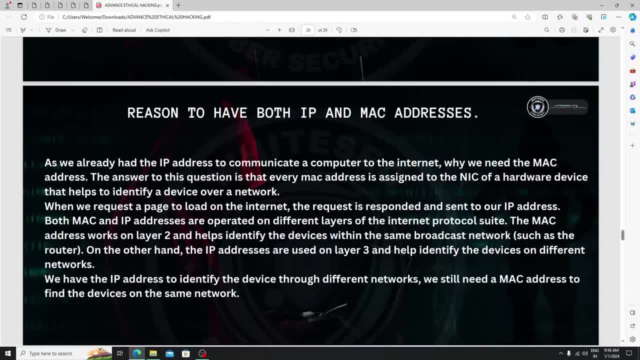 the definitions and you need to focus on the back end as well, how it's working there. now here, there is a reason to have both ip and maxi. we have ip address. why we need the mac address. okay, we learn about ip address right the simple. we have the ip, why we need the mac address. the simple thing is see. 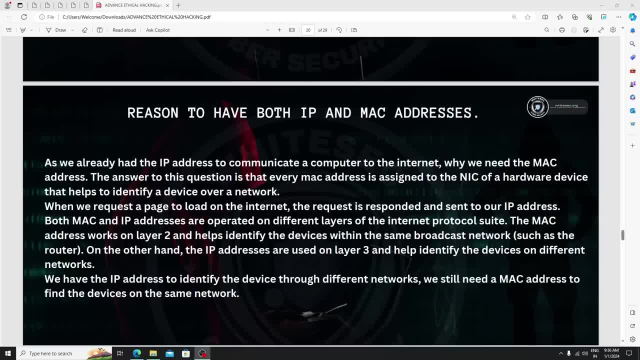 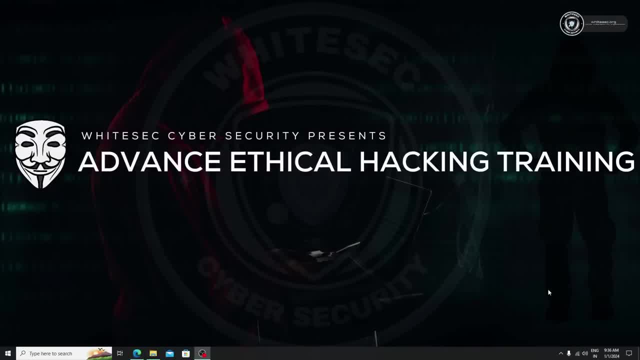 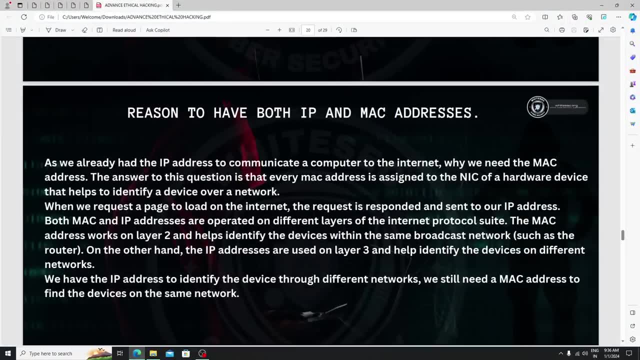 here. let me explain in a very easy way. see, ip is for the network. okay, for this network- assume that i am using the internet for this kind of purpose- i need ip address. but for hard ware, okay, it's need a mac address. okay, this is the thing, as we already had the ip address to. 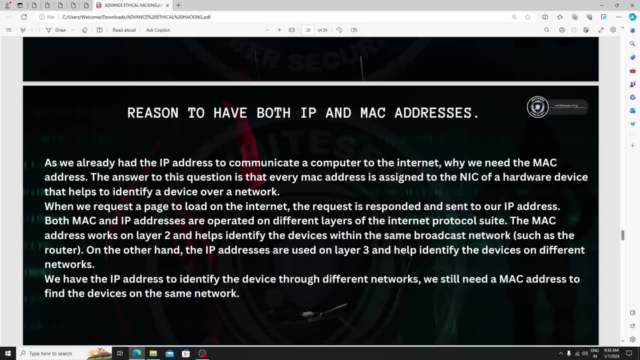 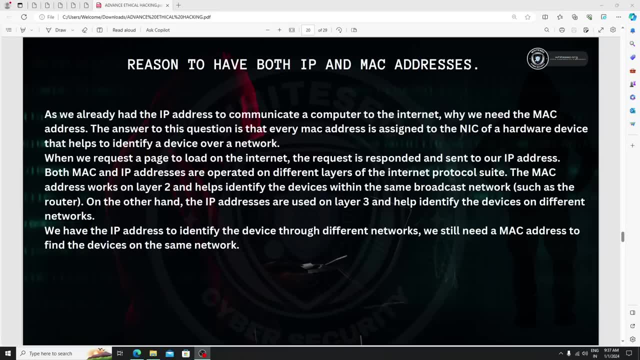 communicate a network to the internet? why we need the mac address? the answer to this question is that every mac address is assigned to the nic of a net. uh, we just learn about this one. what is the nic network interface? what, uh, chip, right, you can say chip card, depend upon you, but the right. 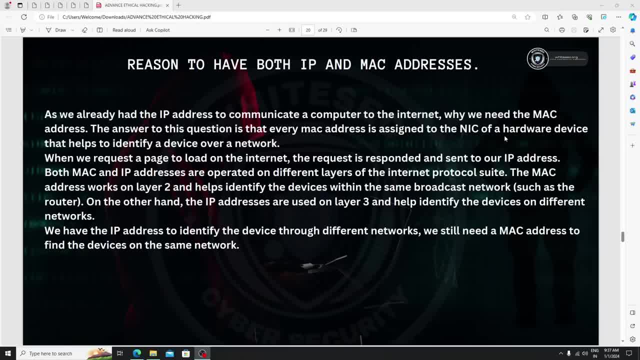 definition is card right of a hardware device. you can say chip card, it's depend upon you. but the right definition is card right of a hardware device- device that helps to identify a device over a network. when we request a page to load on the internet, the request is responded and sent to. 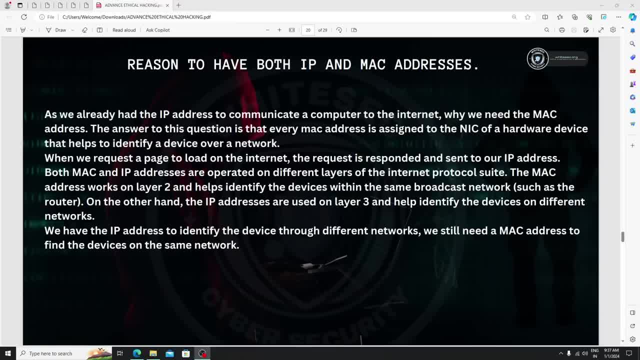 our ip address. both mac and ip addresses are operated on a different layer of internet protocol suite. the mac address works on layer 2 and help helps identify the device within the same broadcast network, such as a router. on the other hand, the ip addresses are used on layer 3. 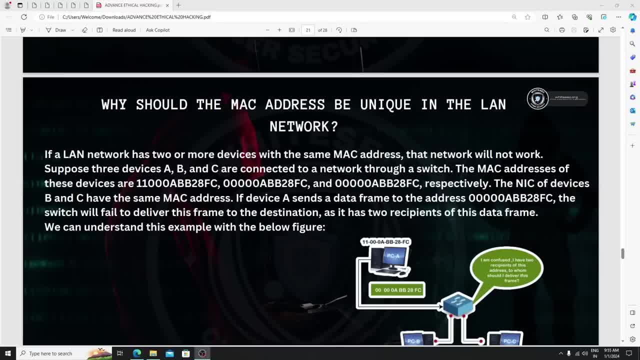 and help identify the device on. why should the mac address be unique in the lan network? what is the lan network here? lan network is nothing but local area network. it's a private network. it's a internal network. this is the thing like. basically it's an internal network. okay, if a lan network has two or more. 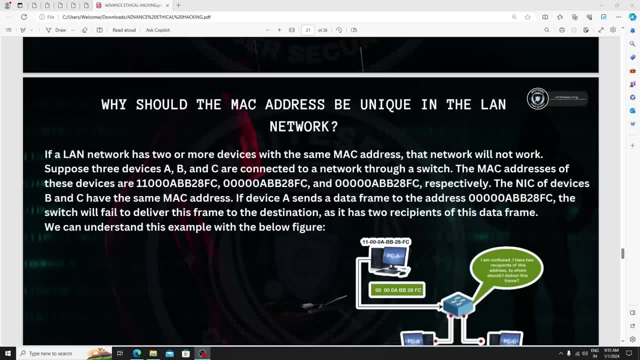 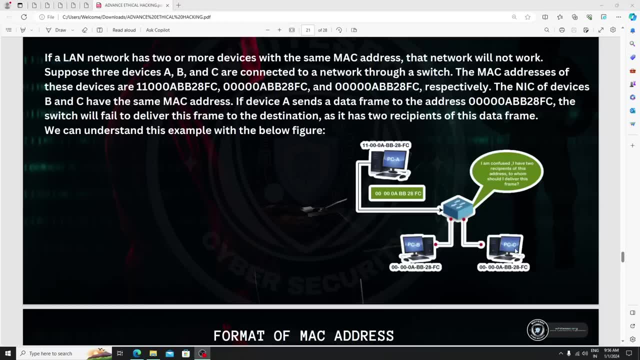 devices with the same mac address, the network will not work. suppose three devices- a, b and c- are connected to the network through switches. here you can able to see the example. there is a devices with the name of pca, pcb, pcc is connected with the same network with. 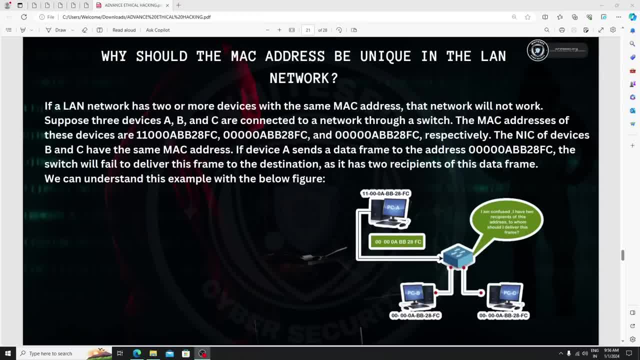 just assume that this is a switch. okay where it is man, okay switch. the mac addresses of these devices are: see this. one is represent to pca, the second one is represent to pcb and third one is represent to pcc. just see the diagram here. see pca having this. 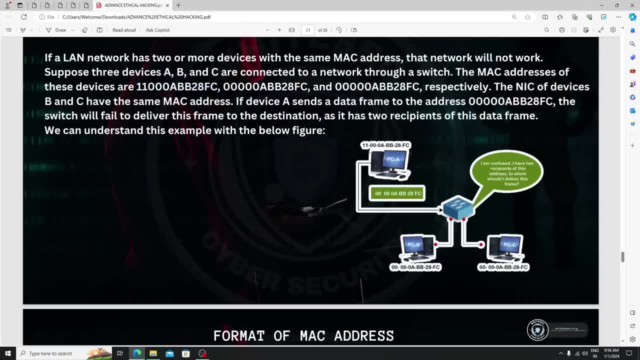 mac address. okay, just focus here. double, double, one, double, uh, double, triple zero, a something like that. okay. and just see the second one: pcb, it's having this mac address. just see the mouse pointer here. okay. and third one having the same mac address as well: pcc. uh, also having the same mac. 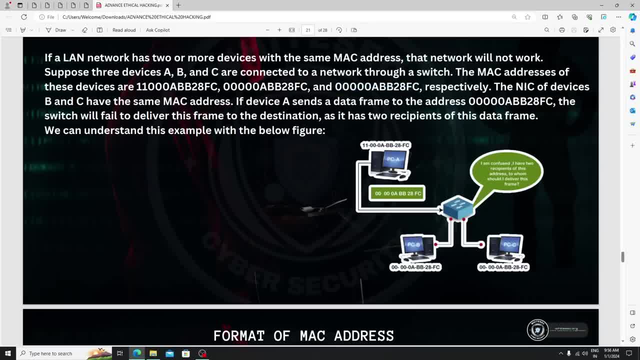 address of pcb, respectively the nic network interface card. i just told you right of devices b and c have the same mac address. again i am telling you this: pcb and pcc having the same mac address. okay, if device a, this one a is nothing, but this device sends a data frame to the address of address this one. assume that this pca want to. 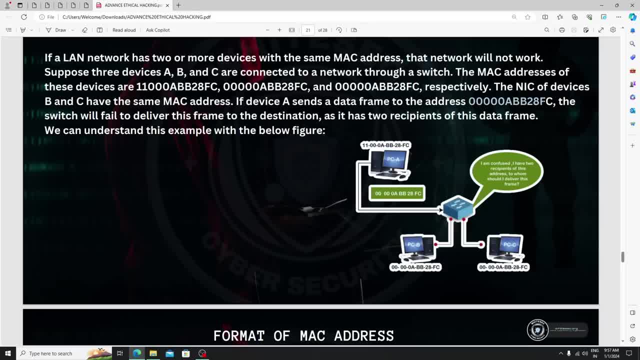 send a data to which address this address? okay, this mac address. at that time, what will happen? the switch will fail to deliver this frame to the destination as it's have. it has a two receptance of this data frame. right, they uses ups forcing the address into acard Soldier. 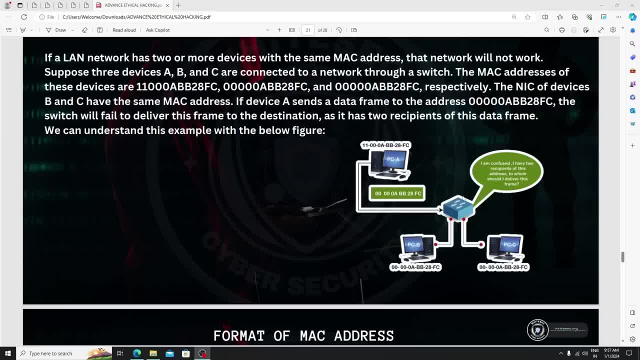 right about II. just three more. it just see the diagram here. pca is sending the data. okay, now this which throw some error here, the this kind of uh error. see, 아주, i am confused. i have two recetant of this address to whom should have delivered this frame in wire shark. 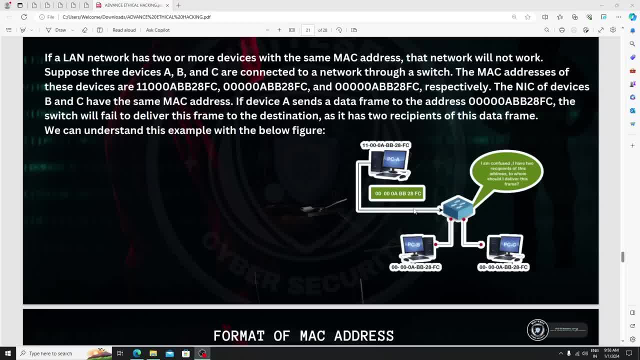 also: uh, once you open the wire shark you will see this thing. okay, clearly it's not kind of uh coding or something like that, in clear what you guys can able to see it. okay now to send the data to this mac address. just see now in the network this: there are two mac addresses. 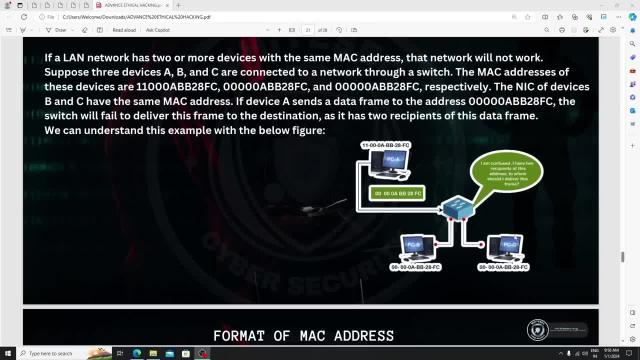 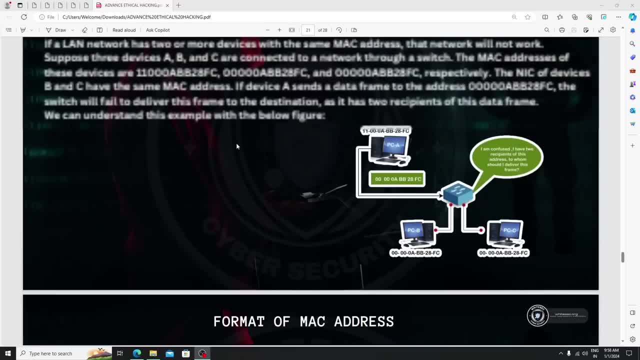 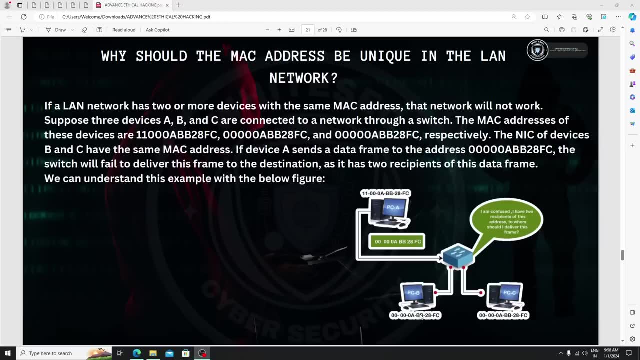 are there with the same address. okay, this is a thing, so that's why it's throw the error there. okay, now there is a for what you learn here. the simple thing is, if there is a two mac addresses, the in the network with with same mac address, then what will happen? the network will won't work here. 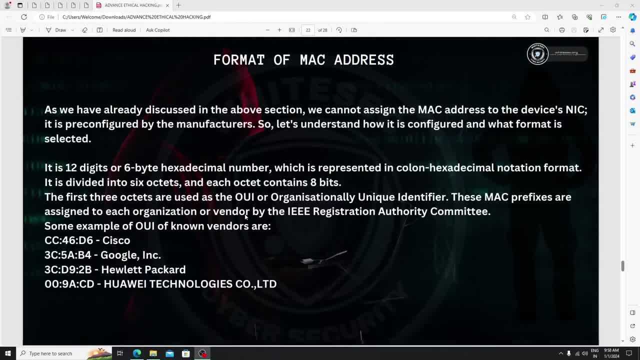 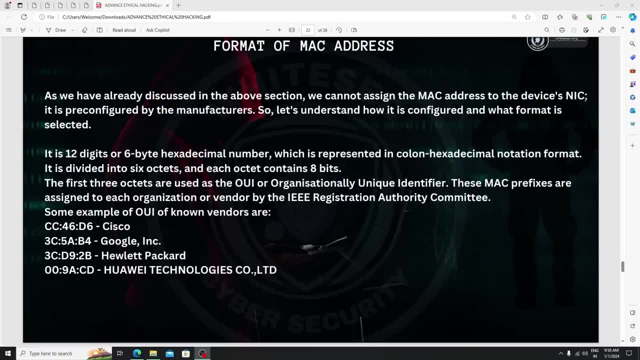 okay, now format of the mac address. as we have already discussed in this above section, we cannot assign the mac address to the devices nic. it is pre-configured by the manufacturer. so let's understand how it's configured and what format is selected. it is 12 digit or 6 byte. 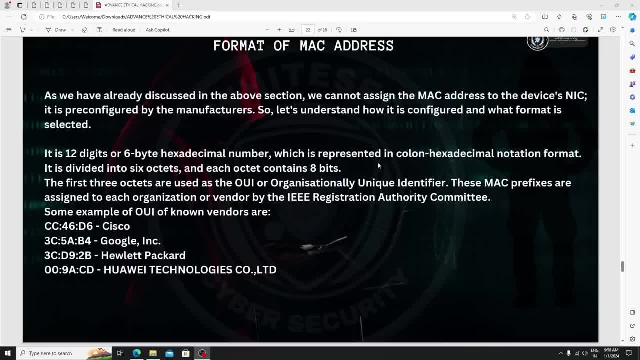 hexadecimal for a number which is represented in colon. okay, where it is? this one? okay, the colon. we just saw this thing in ipv6 as well. okay, which is represented in colon hexadecimal notation format. it is divided into six octet, okay, and each octet contain 8 bit. what is the octet here? this one, this is known as a. 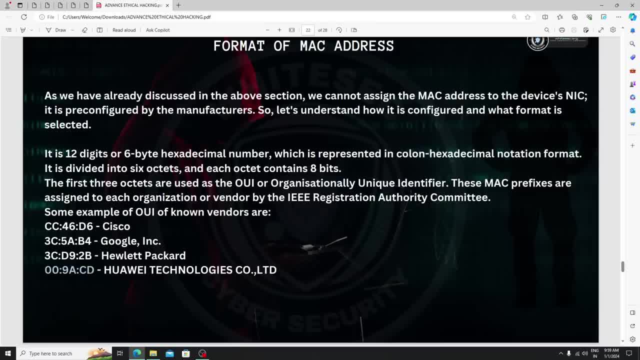 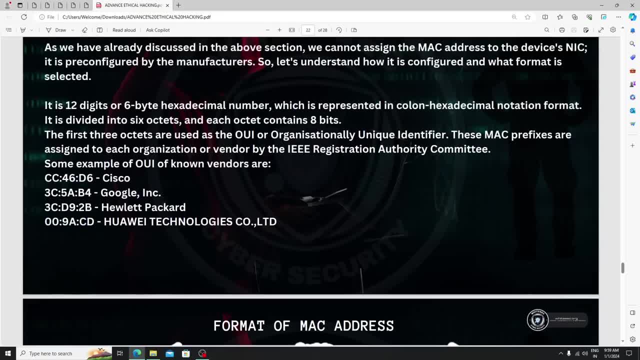 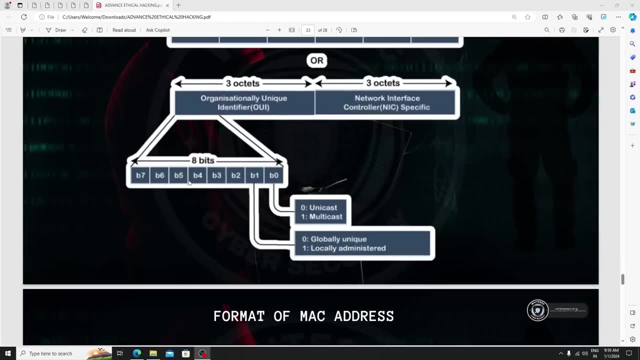 octet. basically, here you can only see the three octet. let me show you. is there any mac address? okay, here you can able to see, not this one, sorry, sorry, here it is okay. one, two, three, four, five, six, seven, eight. okay, this is a thing, and each octet contain eight bits. the 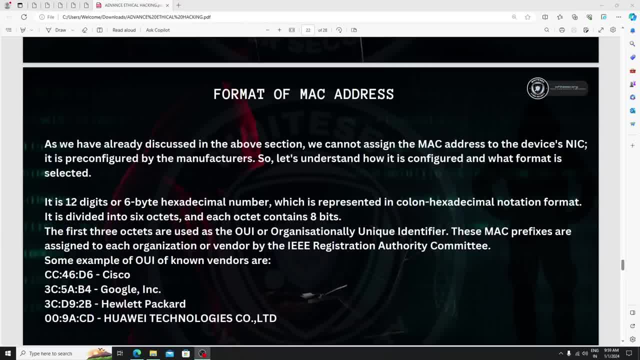 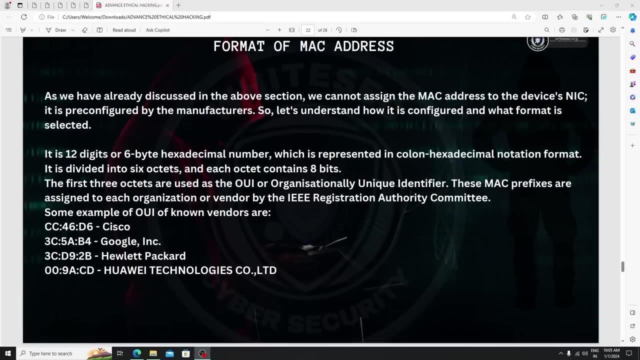 first three octets are used to uh, as used as o, u, i or uh or organized national unique identifier. these map prefix are assigned to each organization or window by high triple e registration authority community uh committee. some example of oui of uh known here you can able to see: if any mac start starting with this values, then what will uh by using this: 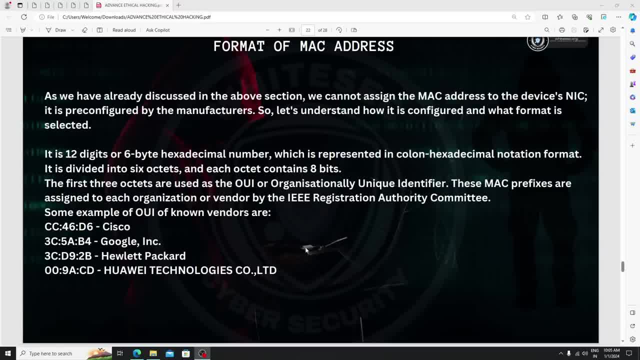 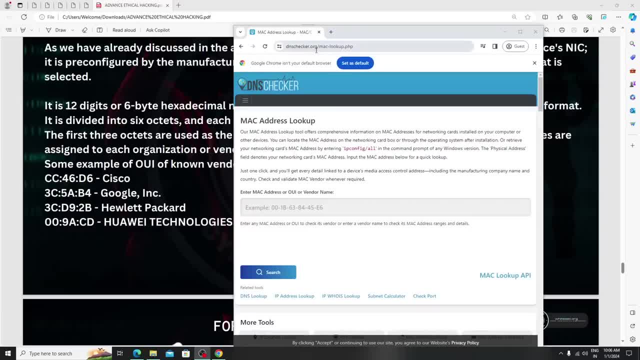 you guys can able to identify the window. okay, this is the thing now: how to identify it. let me show you that one as well. here you guys can able to see, there is one website with the name of dns checker dot org. forward slash mac dash lookup dot php. simple. here you need to paste the target mac. 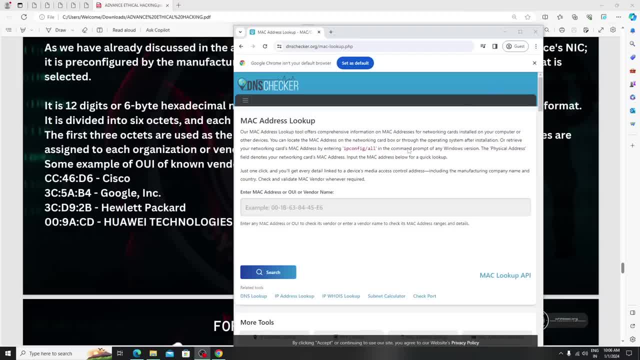 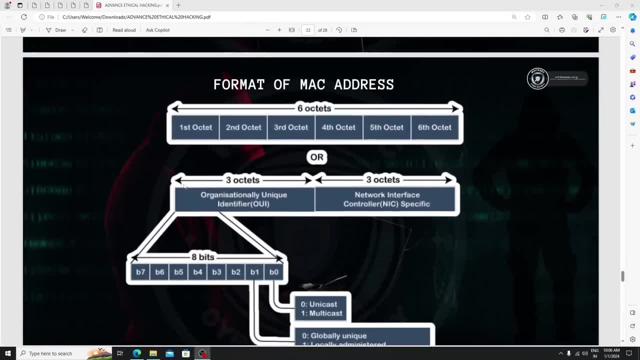 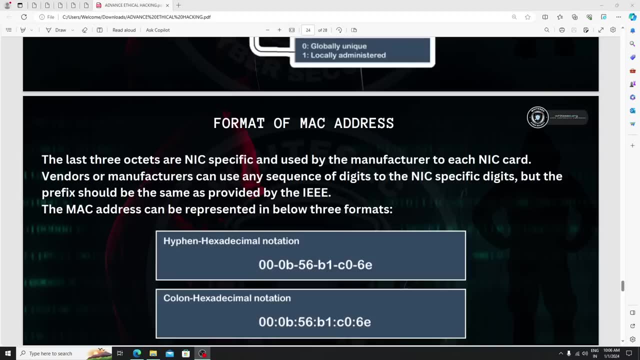 address you guys can able to see the details about that one. okay, like the window this kind of ships. okay, from here you can able to see this one and there is a format of mac address. the last three octets are nic specific and used by the manufacturer. to each nic card vendor or or manufacturer can use. 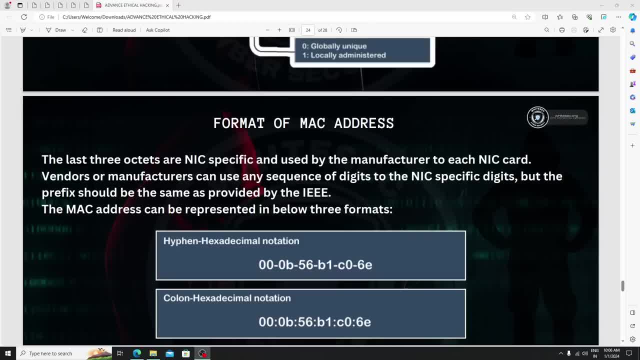 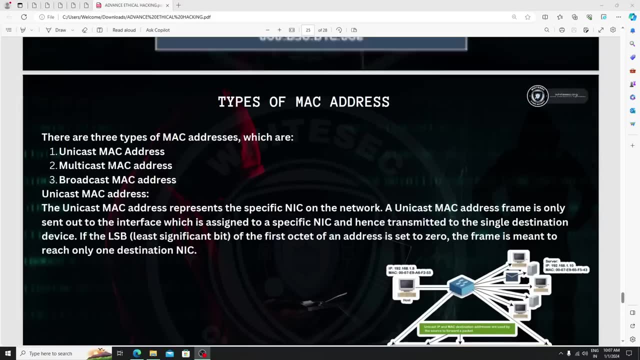 any sequence of digits to the nic specific digits, but the prefix should be the same as provided by i triple e. the mac addresses can be represented in below three formats. here is the three formats. right types of mac addresses. this thing we will learn in next classes, right? thank you, have a nice thing. 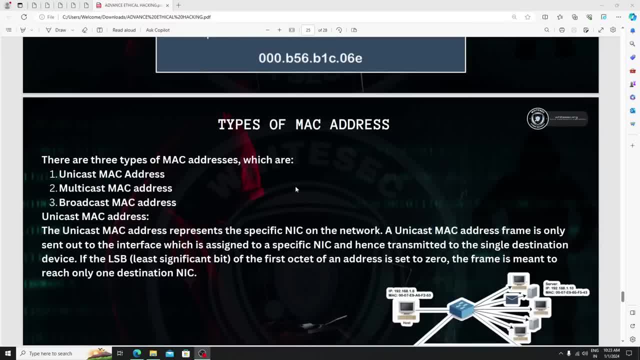 now in this class we are learning about types of mac address. okay, just try to read it to yourself, okay? uh, the thing is, this is not that much necessary for you, okay, but just try to read it. basically, there are three types of mac addresses. one is unicash, multicast, boardcast. okay, uni is. 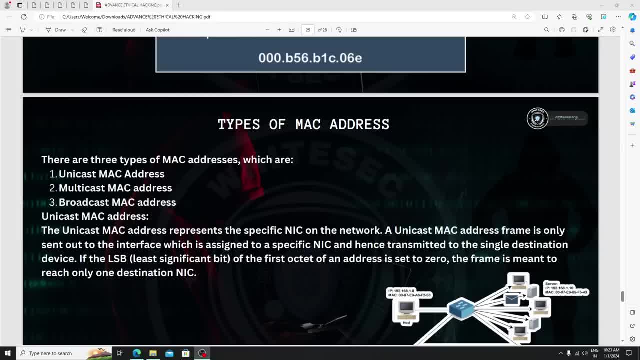 nothing but single. multi is multiple, right, and broadcast is nothing but everything. okay, which is regarding the network. um, i assume there are five types of mac address which is required. okay, you right. and broadcast is nothing but everything okay which is in that network. okay, i am trying to understand. so i am going to estat it and you can. you can see that third one. okay, i guess there are a lot of these things, okay, um, so these two things we can look at, uh, that are actually generated between the mac address of the mac address, right? so then, can what kind of message you say is if an id cardolic marketing account? 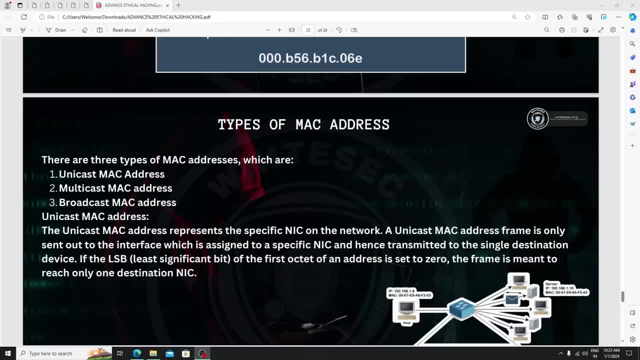 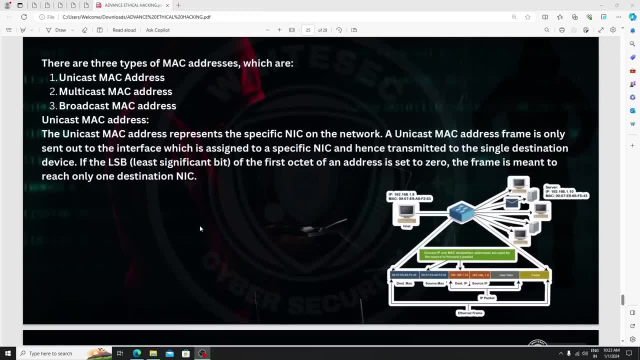 okay, and now just remember this points and read this: uh, definitions. okay, you will get it. if you are not getting it, no need to worry, it's not a big deal for you. okay, once you jump in practical classes, at that time you will get it. okay, yeah, these things are not that much necessary. let me 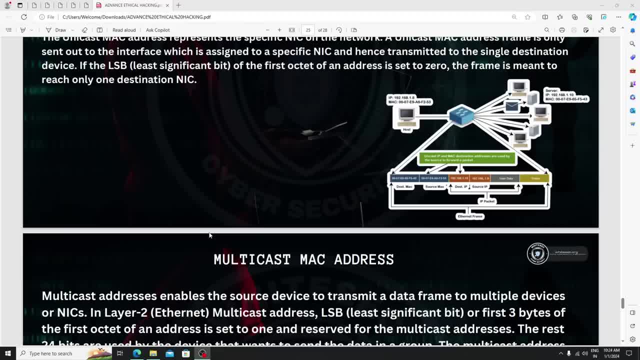 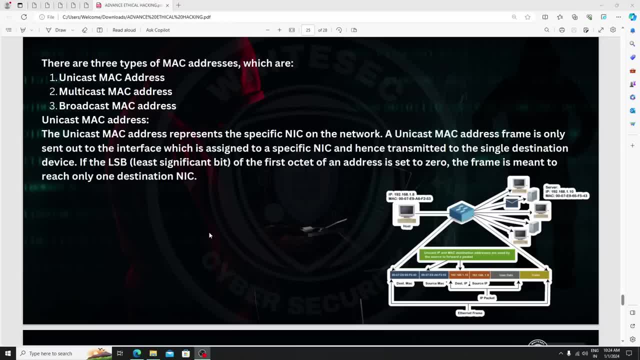 tell you, okay, i don't want to hide, uh, anything, right? the simple thing is this kind of stuffs are not that much necessary. the necessary things are. i will tell you, okay, which, which things you need to focus there. okay, in real world, what kind of challenges you will see. i will tell you this: 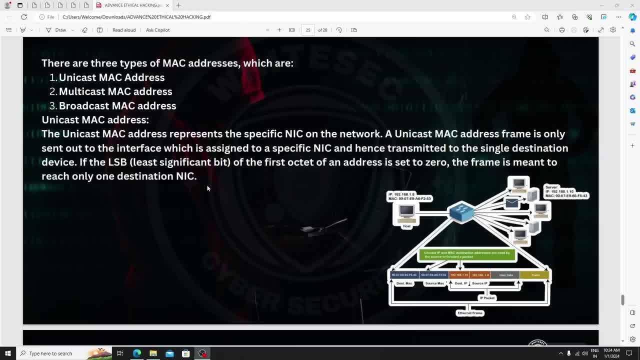 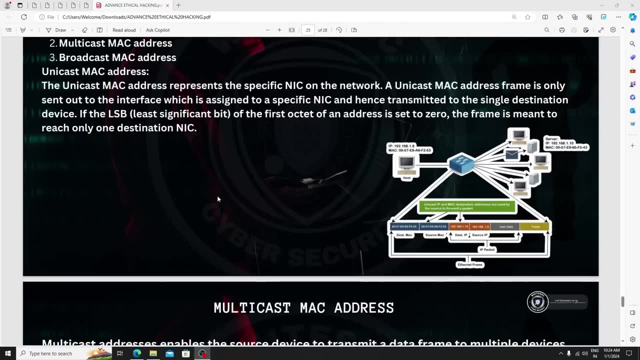 kind of chefs. but let me tell you, this is a kind of thing which you need to learn, okay, like before reading the book. what you learn before reading the book, what you see, simply, you will see the content. right, what is there? something like the same thing. okay, just try to see it. just try to read it, okay. 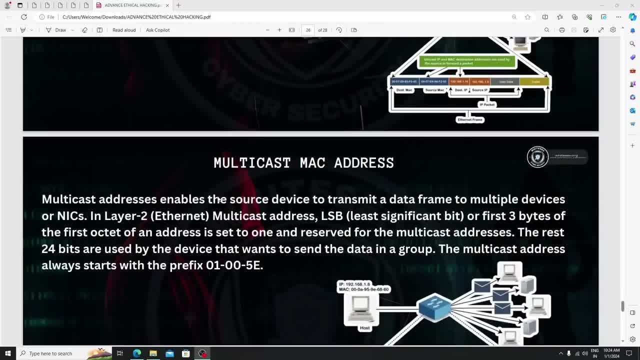 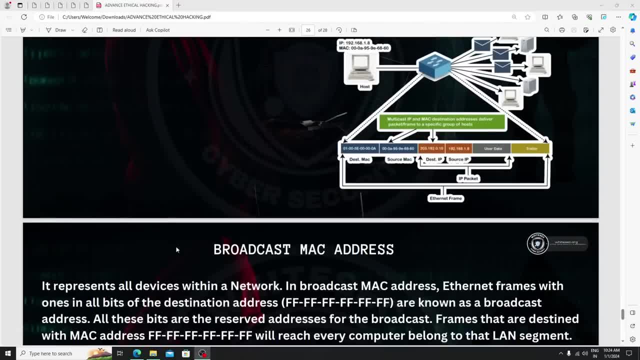 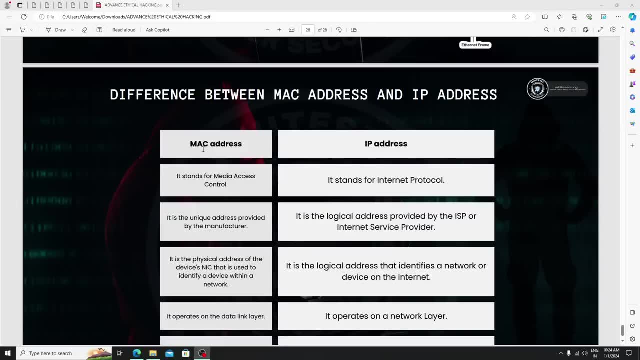 no need to remember. okay, if you jump in again, i am saying if you jump in practical things once you do the attacks, then at the time these things are very easy. okay, now, here is a thing, uh, this, this one is very important for you: the difference between mac and ip address. okay, mac address: it stands for what? 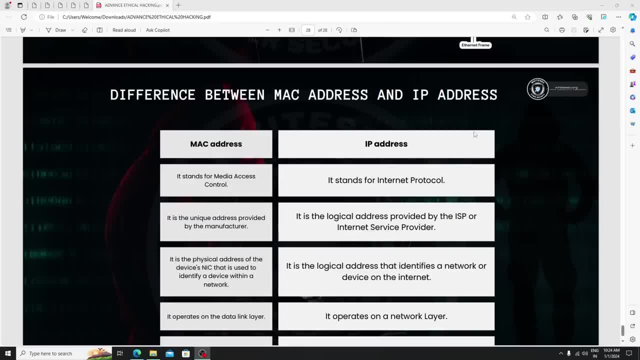 media access control. okay, ip. what is ip? ip stands for internet protocol. we just learn about these things in the in the last classes, right, see, it is a unique address provided by the manufacturer. okay, this, i, uh, this mac address is provided by manufacturer. okay, and the ip address is: 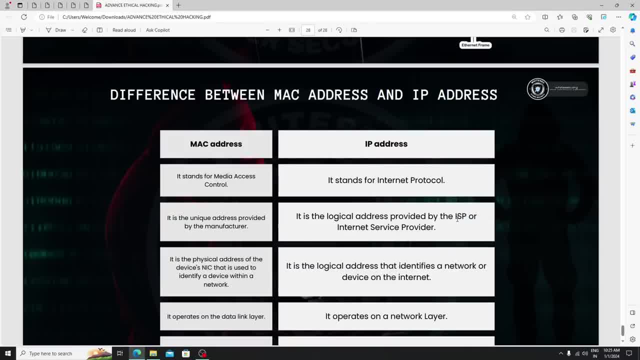 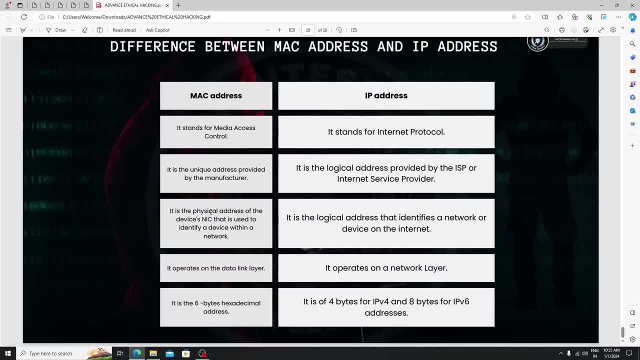 provided by isp internet service provider and the mac address. it is a physical address. physical is a nothing. but once you listen, physical okay. you need to think that. hardware okay. remember one thing here: just remember mac address- hardware okay. this is a thing which you need to remember because 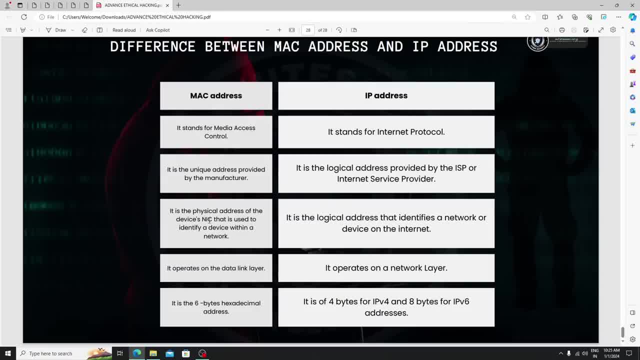 it is a physical address of the device. nic is what here? network interface chip, right? or uh, what is it card? okay, chip card, it depend upon you, but the right definition is card here, that is, that is used to identify a device within a network. now ip address, it is a logical address. 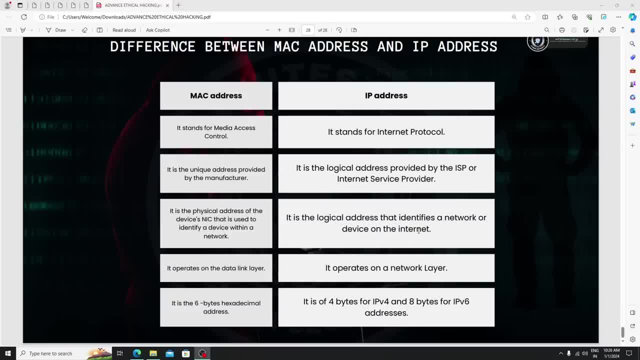 that identifies a network or device on the internet. okay, for internet purpose. okay, it is a logical address. okay, that identifies a network or a device on the internet. this one is important. okay, if you was a last classes, then you will get this, all things. okay. now here MAC address. its operate on the data link layer. basically it comes under osi model ip. 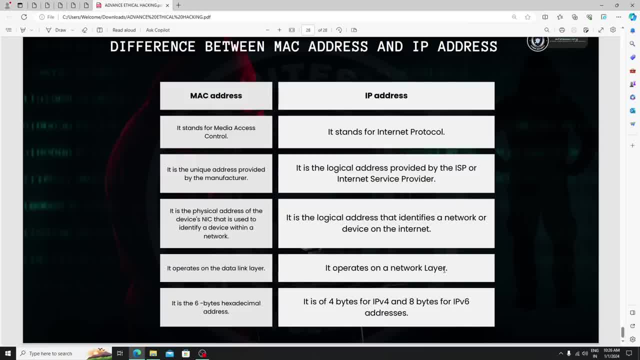 address. its operates on a network layer. now here it is a 6 byte hexadecimal address. ip address is 4 byte for ipv4 and 8 byte for ipv6. hope you guys get it. its not again. I am saying its not a big deal. 3. 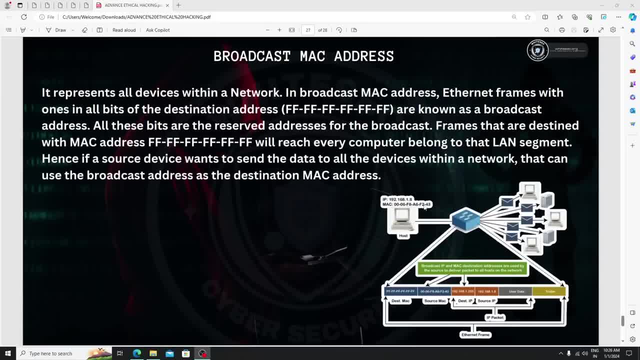 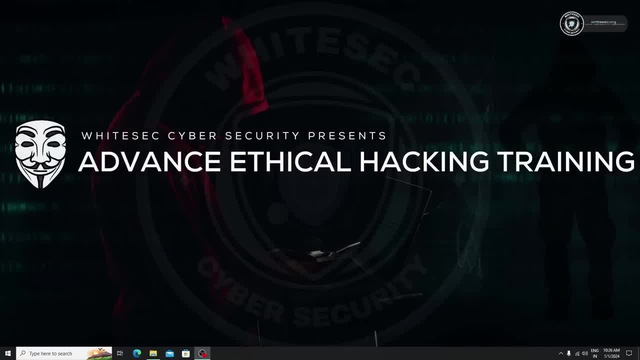 of you guy guys will get some kind of issues with it. just try to ignore it, no need to worry. okay, right in the next classes we will learn about some new things. in this class, i'm gonna tell you which programming language you need to learn. okay, the first thing is you need to learn c. second, 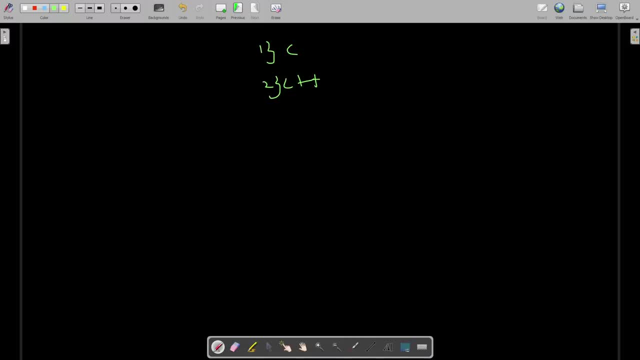 is c plus plus. third is python. okay, see, after learning c and c plus plus, you will get that why python is a easy language here. okay, and the third thing is: just learn basics. majority of people what they do means they learn, uh, from they. they join this kind of boot camps or they they 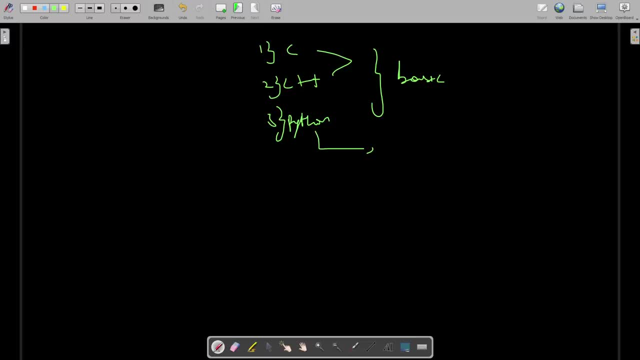 just watch this kind of trainings, which is like basic to advance. don't do that, because the thing is, you are not a coder, you are a pentester. your work is to exploit the things. okay, before exploiting the things, you need to learn about the technology, about that technology. okay, assume that you are. 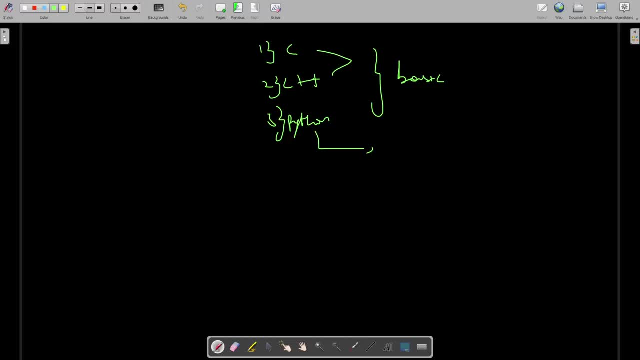 performing cloud pentesting at that time, you need to learn about cloud. okay, this is the thing. assume that if you are a performing scada pentesting there at the time, you need to learn about scada. okay, you no need to go deeper like a engineer. okay, like uh uh, you no need to develop the things. 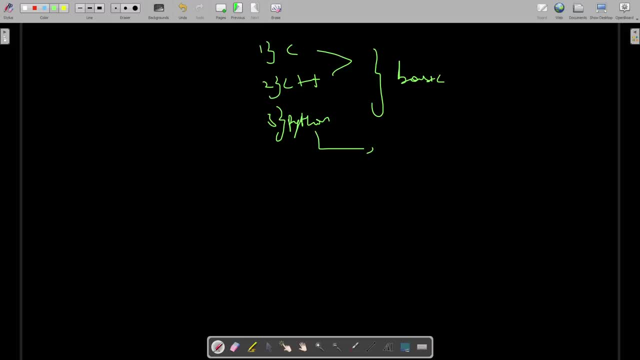 here. you just need to learn the basics- okay, how the technology is working there, okay, how the things are going there, something like that. then you need to go for the exploitation phase. this is your work. you, you are not a coder. remember this thing. see here, this is. a lot of beginners do this mistakes. okay, like they learn coding and they won't get anything. 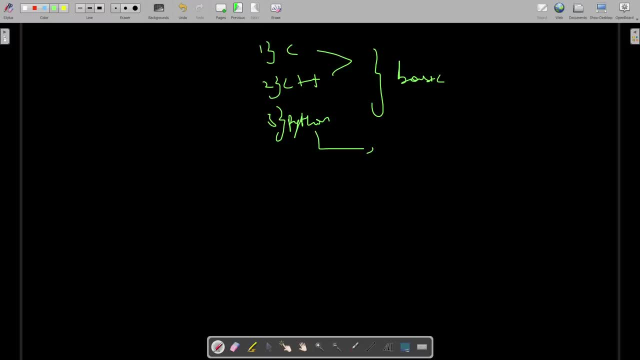 like, uh, after learning some coding, they they become bored, okay, and also they lose the interest in hacking as well. so the thing is: just learn, sorry guys, just learn the basics first. okay, and this languages is necessary for you, okay, just learn c, c plus, plus, python- basic, uh, in youtube. you. 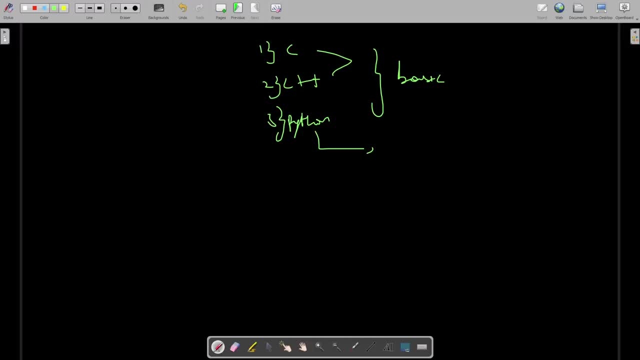 will see a lot of videos. okay, just try to watch it. just try, uh, do practice here. okay, that's it. this is how you need to manage. assume that you are working with a source code review at a time. you need to become expert there, but uh, mostly, uh, my work is as a pen tester. okay, i, i don't do these stuffs. okay, in source code review. 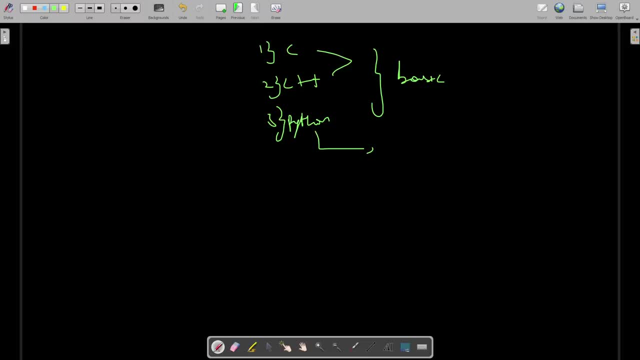 what will happen means you need to analyze the code. okay, by using automation tools. assume that the the client, okay, the client is asking you to do the manual. at that time you need to know the coding there, okay. but if you uh, by using the automation tools as well, you you can able to do that. but still, if any student is, 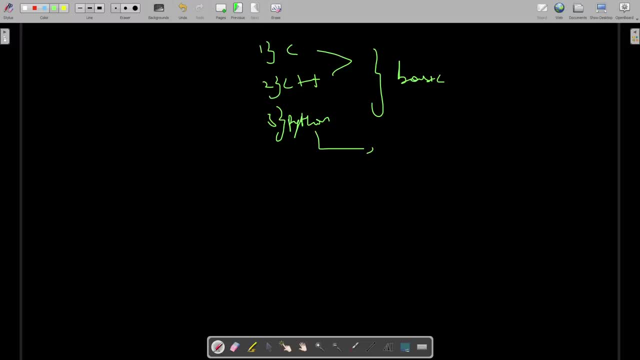 interested, uh, in the source code review or this kind of shops, at that time they need to become expert, okay. but as i told you previously, our work is, uh, we are pentesters. right, we need to work with different technologies. okay, assume that if somebody uh hired you for drone pen testing, at that time you need to do the other process there. you need. 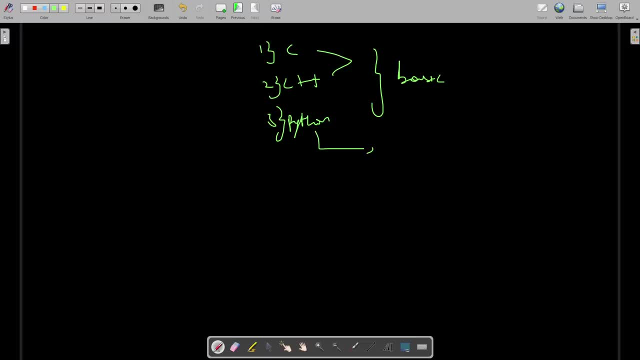 to learn about the drone technology, how it's working, okay, uh, which technology they are using? like, like, wireless bluetooth, this kind of shops. you need to focus, okay, this is the thing, but the the the necessary thing is you need to learn these languages, okay. what i am trying to say is: 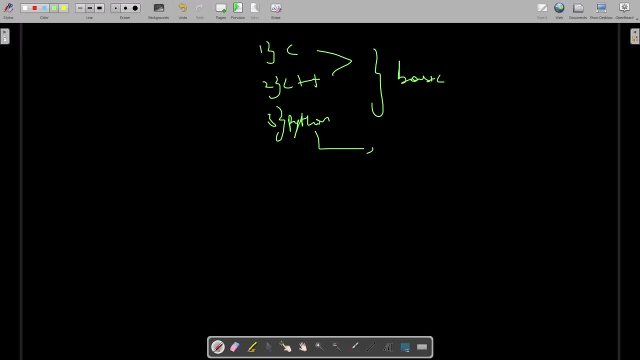 if you, if you want to become a pen tester or ethical hacker, then this language is necessary, but not uh. sorry, but not that much. okay, like uh, you no need to become expert here, you no need to uh develop the softwares or something like that. learn that much, which is uh necessary. 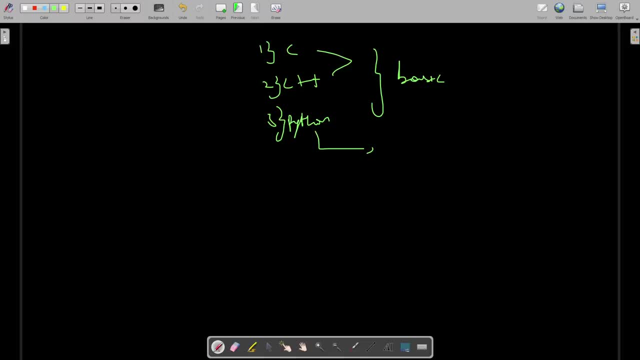 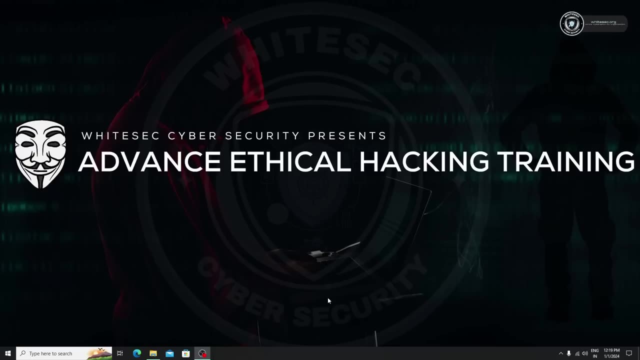 okay, like as i told you, hope you guys get a complete idea right what i am trying to say here. see, the thing is, once you jump in real world projects, at that time you will get it. okay, if you are a beginner, then just try to ignore this words. 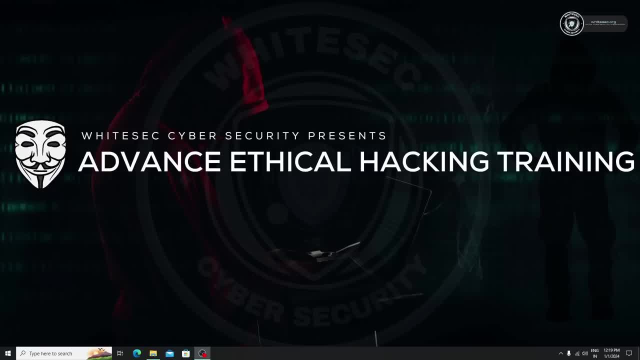 right, we will. in the next classes we will learn about wireshark. hello guys, hope you are fine. in this class we are learning about wireshark. let me tell you wireshark is a network analyzing tool. you can also say it as it's a sniffer. okay, by using wireshark, you guys can able to sniff the. 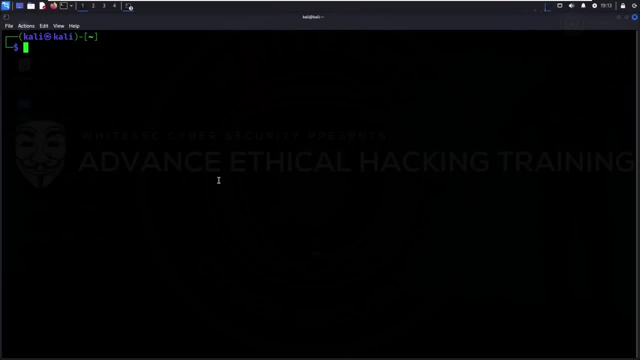 network there. okay, let me show you practically. you will get it, just type if you want to open wireshark, just uh, type sudo wireshark. always remember you need to open wireshark as a sudo user. okay, so let me show you how to open wireshark. 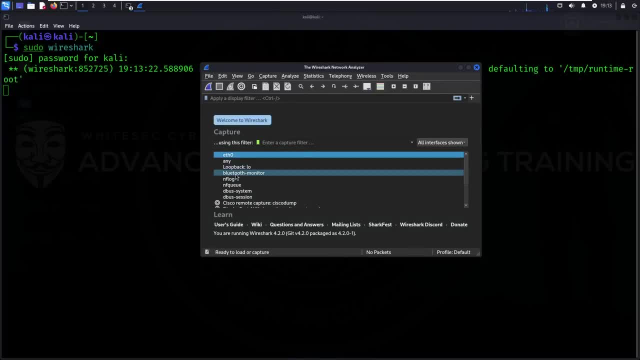 now there is ets0, any loopback? okay, loopback is nothing. but here, 127.0.0.1, is there? right, it's a loopback address. uh, here there is a bluetooth. if you are perform, uh, if you are, if you have the bluetooth adapter, by, by clicking on this interface, you guys can able to analyze the 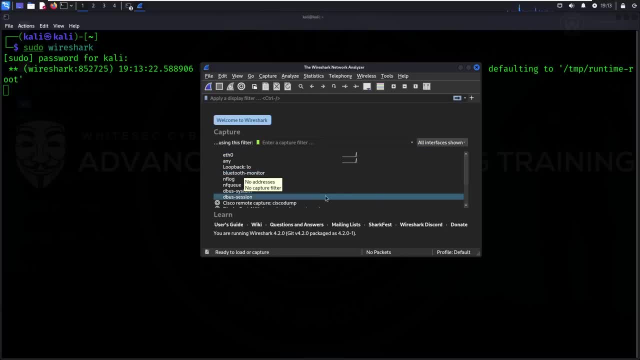 bluetooth traffic as well. okay, this is the thing. there is a cisco remote capture. there is uh ssh remote capture. is there udp listener? is there wi-fi remote capture? right, there is a lot of things, but we are focusing right now. just see the graph here right now, in uh, here ets0 having uh, the huge traffic. okay, if, let's see, assume that. 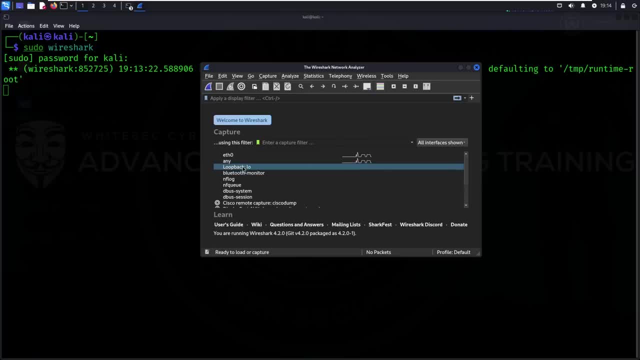 you just connected the bluetooth adapter with this kali machine. at that time, what will happen means: uh, it will analyze the bluetooth results. here, in a simple words, assume that you are sharing some data through bluetooth. at the time, you can able to see the graph here. okay, so this is how you can able to identify, but right now we can able to see the graph on ets0. that, uh. 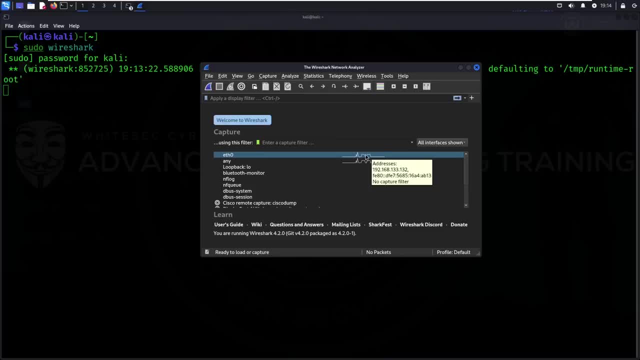 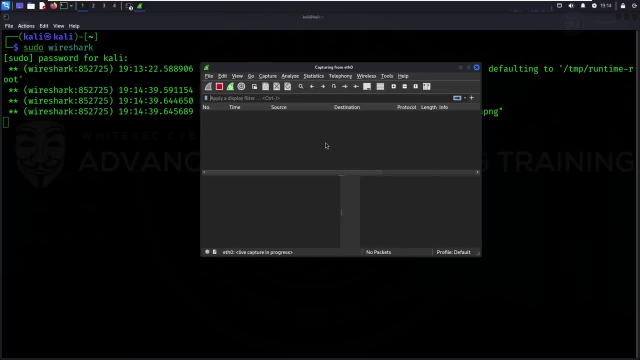 that means in this interface: uh, there are packets, are there, or uh, the connection is going on, something like that. okay, just open it. here you guys can able to see. just uh, just click on. after opening, after selecting ets0, the simple. this is for what? this is to stop capturing packets. okay, this is for what? restart. 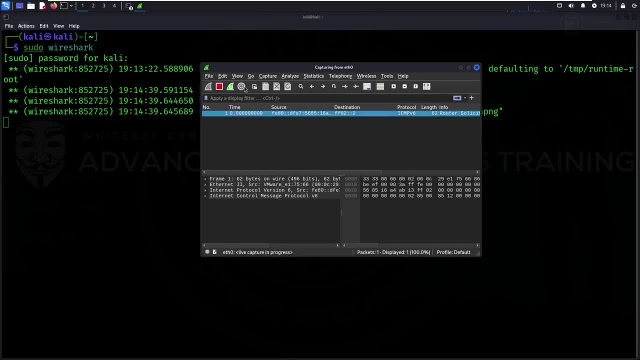 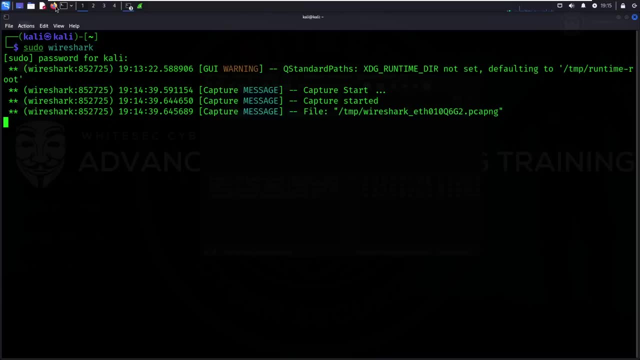 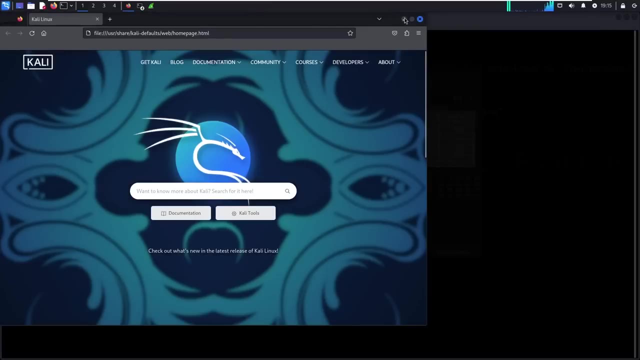 if you want to restart this process, then here, from here, you guys can able to see it. okay, now let me tell you, let me open any browser. uh, let me open browser here. see, after opening the browser, you guys can able to see there is a huge traffic, right? so basically, 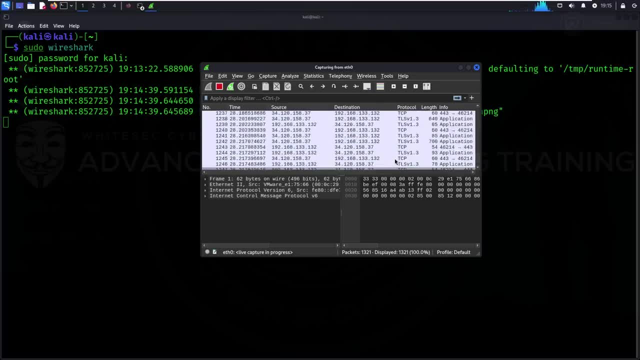 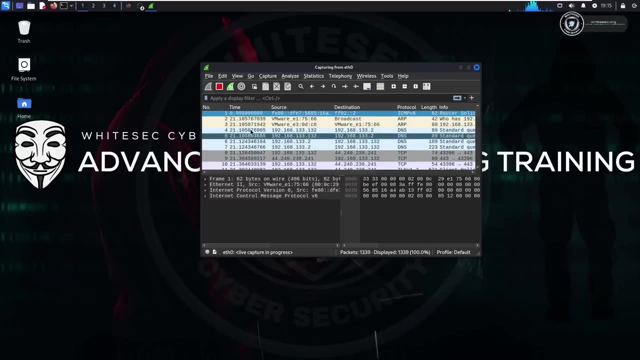 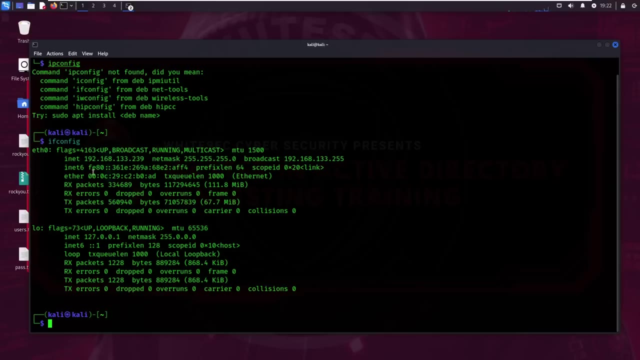 what is this? uh, that's why we say it- as a network analyzing tool. let me tell you one thing, guys. here we, uh, we are not only capturing the traffic of this machine. assume that there is another machine, okay, in that same network. okay, just see the machine ip address, which is 192.169.133.239. okay, now, if i open the, 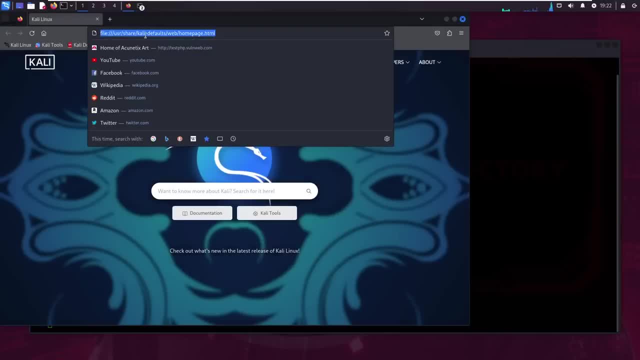 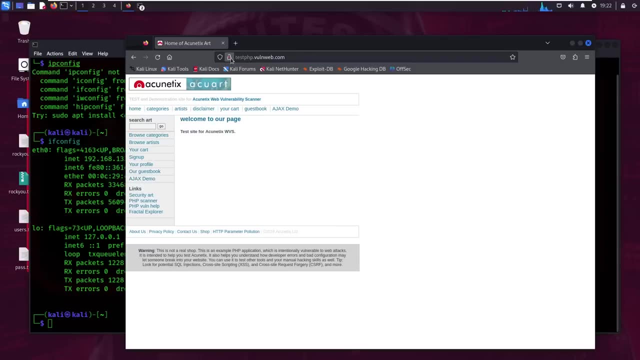 browser here, and if i visit to this website, let me visit to this website, which is test php.1 web. okay, basically, this website is not using https. okay, so it is easy for, uh, it is easy- to access the data there. okay, assume that here in http websites, what will happen means. 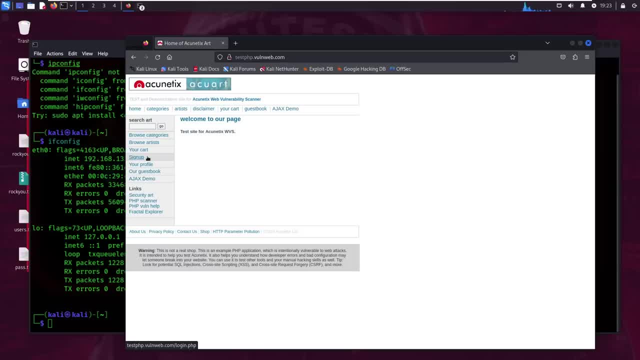 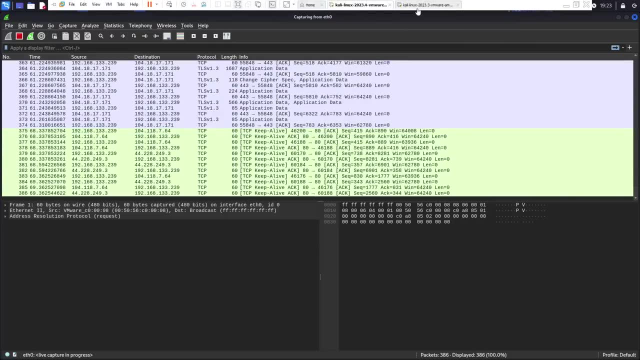 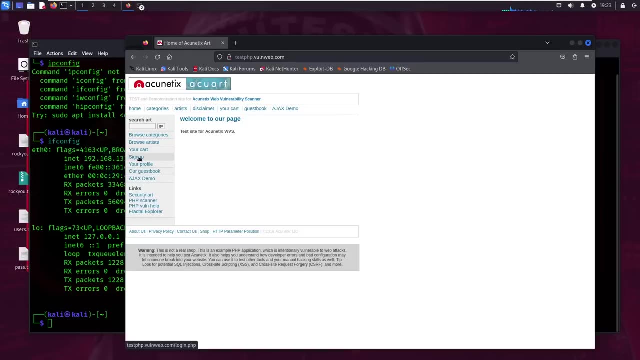 assume that if the victim or any user just type the credentials here, we can able to capture it, okay, in a clear text. so this is the thing. so let me show you. see, let me restart it again. okay, see, there is a sign up button. let me type: uh, anything such as the username is test and password. 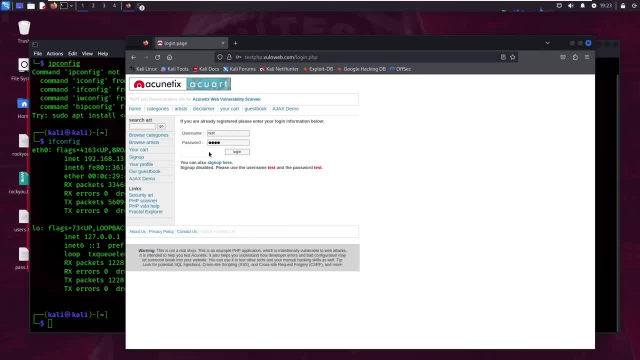 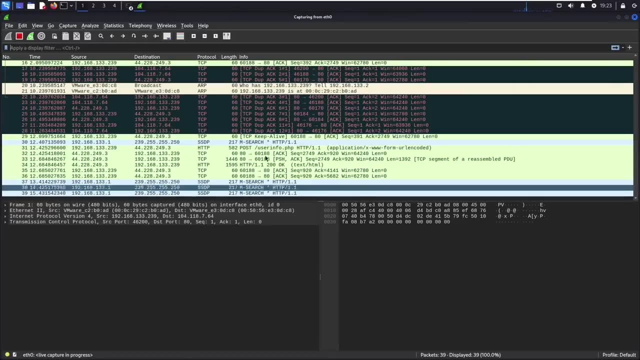 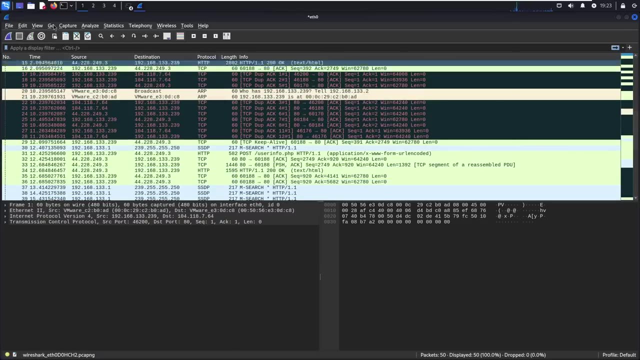 is test here. just type: let me click on login button. okay, here, if i go back to my target machine, you guys can able to see some data. okay, just just wait. just let me stop the traffic here. see, if you want to stop the traffic traffic then simple, just click on this button, the red button. 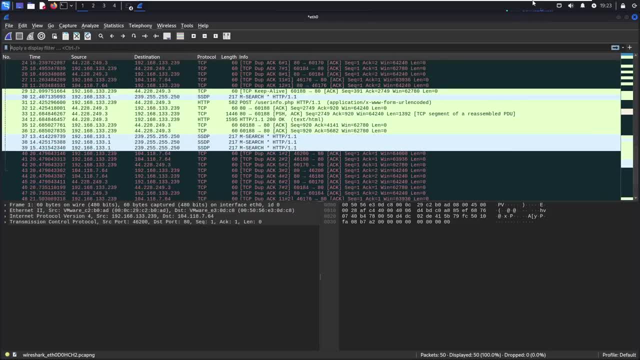 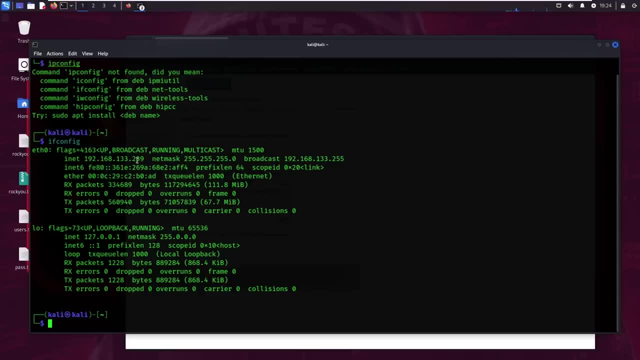 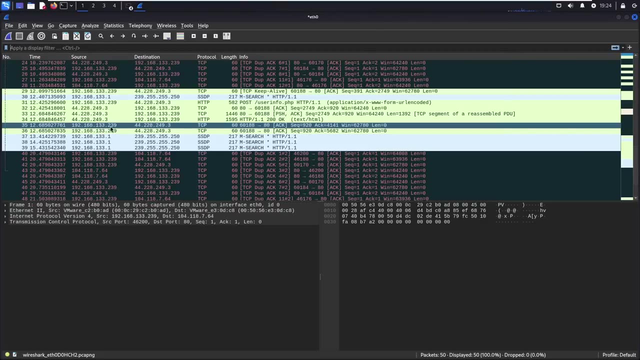 now here you can able to see that. just see the source interest. what is my? what is a machine ip address? it's a one, nine, two point one, six, eight point 133.239. just see for this ip. see here it is 192.168.133.239. okay, thus the thing is here. 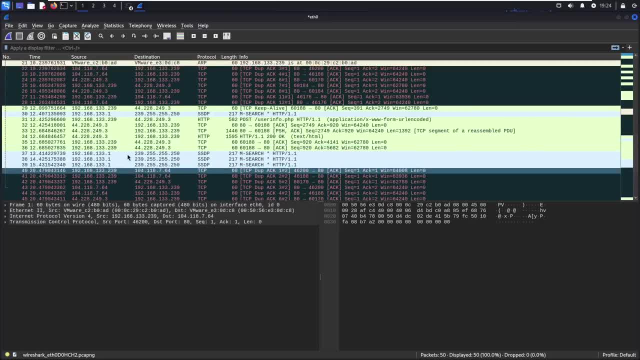 it's a huge right how you can able to analyze, uh, how you can able to see for the specific ip. the simple thing is just use this filters. okay, apply a data display filter here. assume that i want to see uh about the specific ip. now, simple, just type here: ip. okay, here it is ipaddr that. 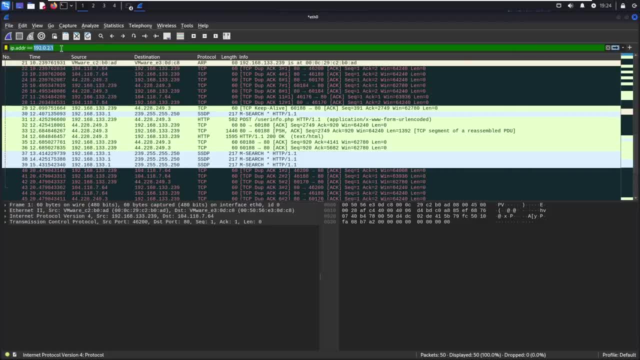 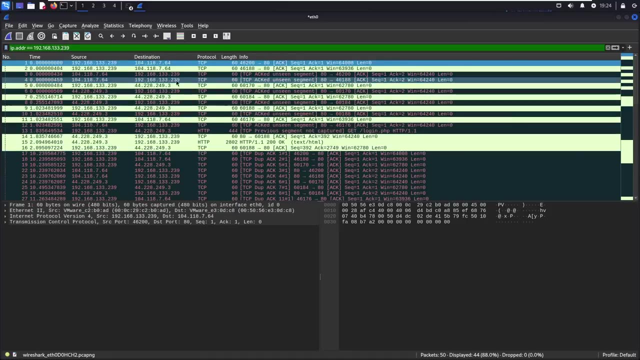 means ip address, and just type your target ip. in my case the ip is 192.168.133, point. okay, what is that? 239, right? 239? just type, enter here you can able to see a about that specific ip. okay, just see. now let's see the data. okay, which we just type there. 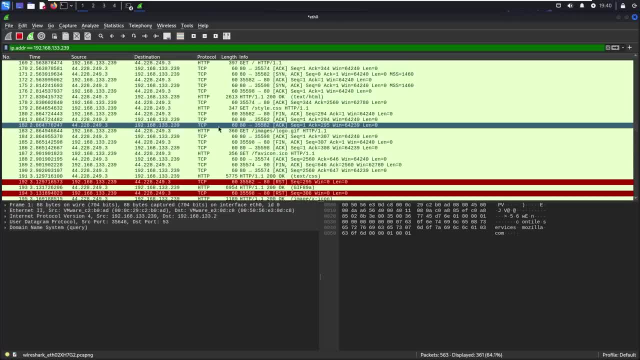 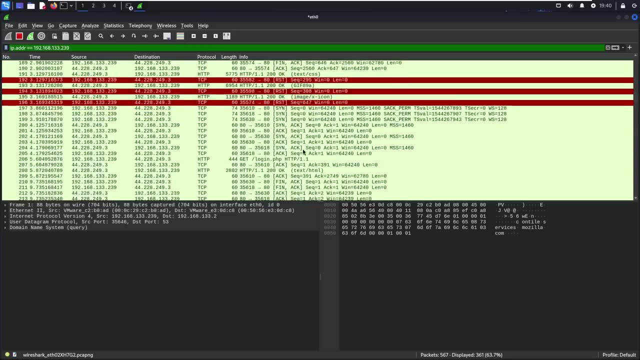 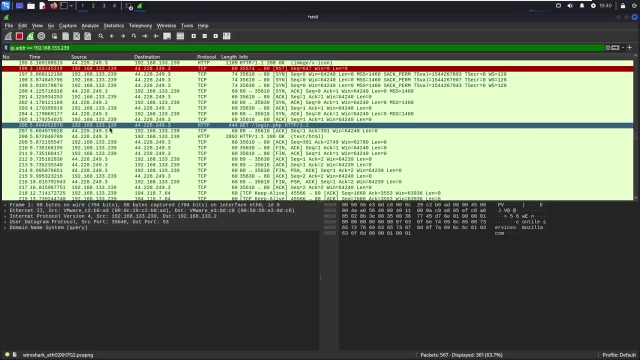 which comes under http protocol. so here it is okay. you need to see for form. let me okay, here there is a loginphp, if i just see the source ip. source ip is 239, which is our target ip. okay, and this is a destination ip. destination ip is a nothing but the website ip address. you can also say it as a: 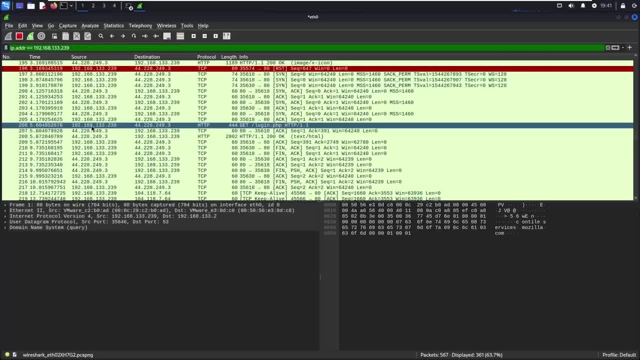 website ip. source is what? okay, source is what here? source is a nothing but your, your target machine or your machine. okay, the machines which are in your network. this comes under source machine. okay, destination machine is nothing, but assume that in your network one, uh one of the 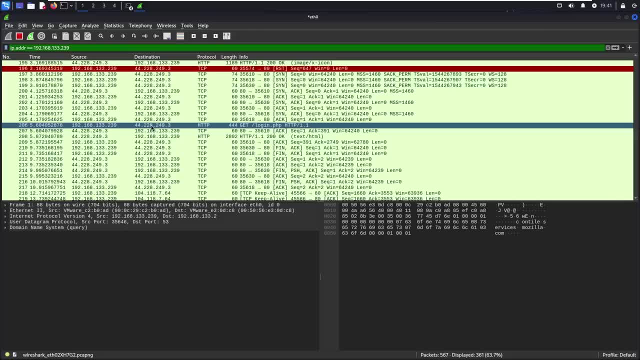 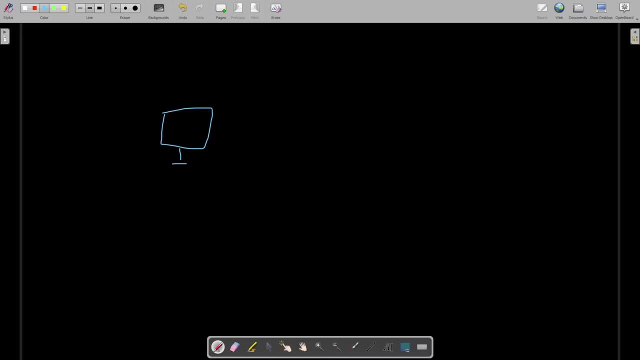 user is uh visiting one website. okay, that is okay. the the website, uh your target website, uh ip address us. okay, this is a thing. let me explain you here, man, just wait. the source: okay, let's take this machine as a source. source is what? here it might be your machine, any user who are in your network. 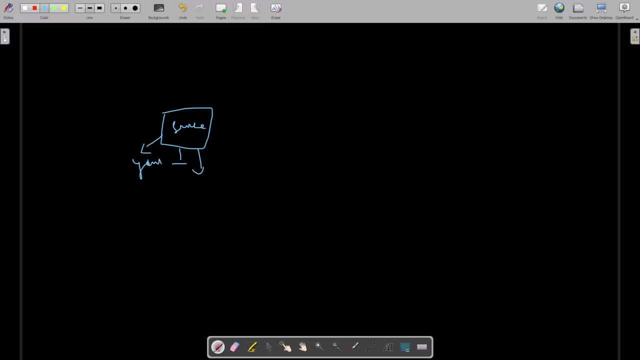 okay in that wi-fi network. now assume that the user want to serve googlecom. simply you open the browser and there you just type googlecom, right, simple. googlecom is a destination here. okay, google. sorry man, googlecom is a destination, right, so it doesn't show the url. it will show the. 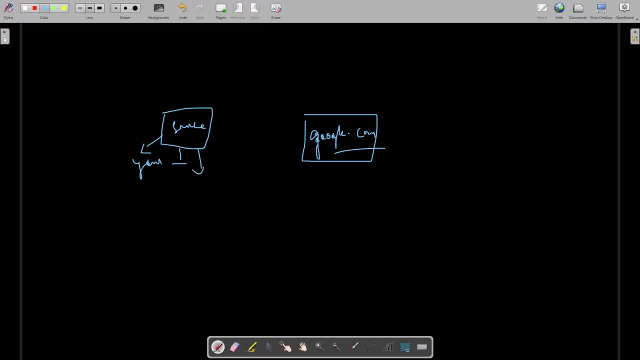 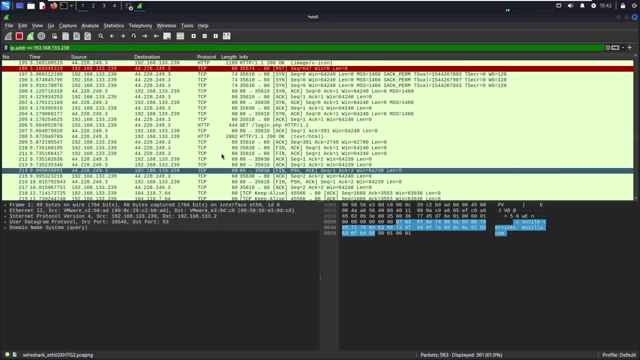 url in destination bar, it will show the ip address. okay, this is the thing. okay, let me show you how to see the url as well. it's not a big deal here right now. first of all, let me here: there is a http. you need to see the http request because the website is. 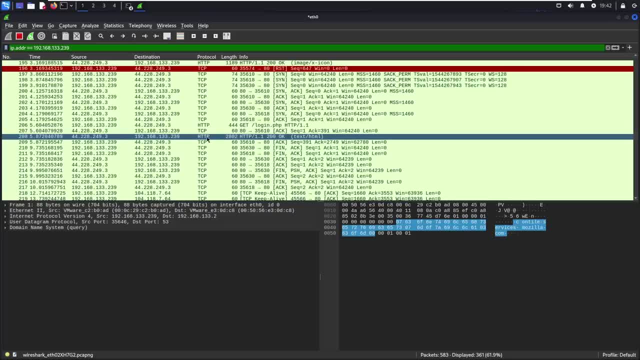 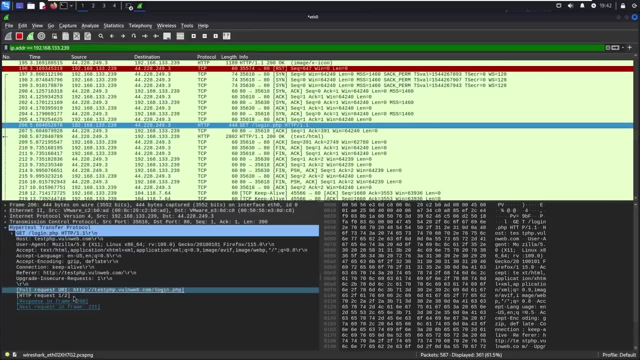 running on googlecom and googlecom is a destination, right. so googlecom is a destination running on http, so that's why you need to focus on http here. there is a loginphp and if you see the hypertext transfer protocol, then here you can able to see the website. 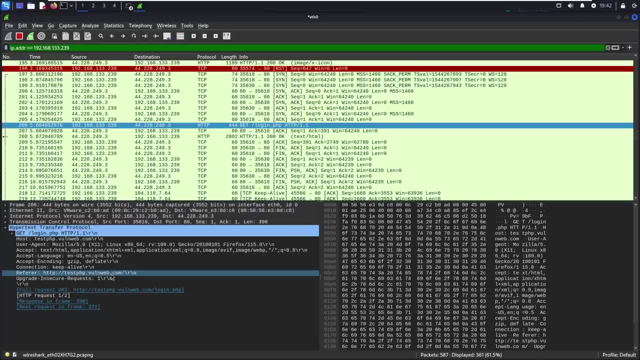 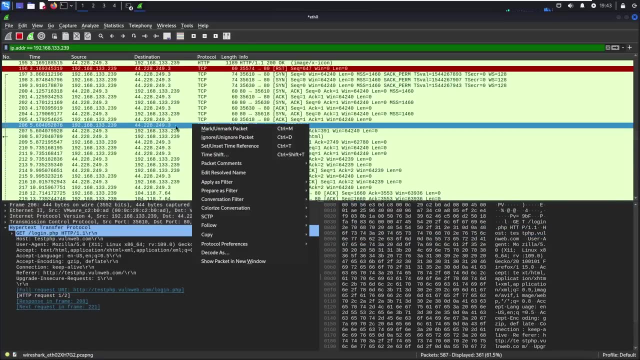 as well. referrertestphponewebcom- okay, and in the host also, you can able to see the website url. okay, and here also right. let me just see the username and the password. okay, now, if you click on the follow, if you click, just select the packet. okay, just select it. and 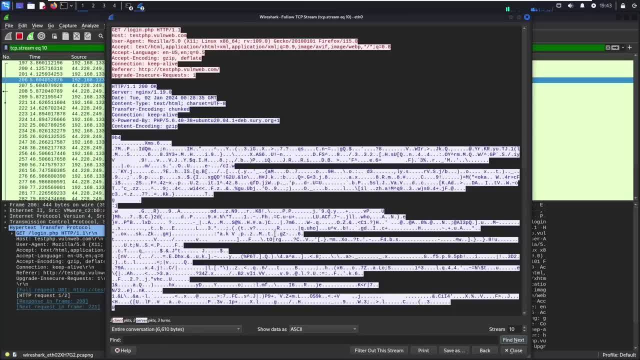 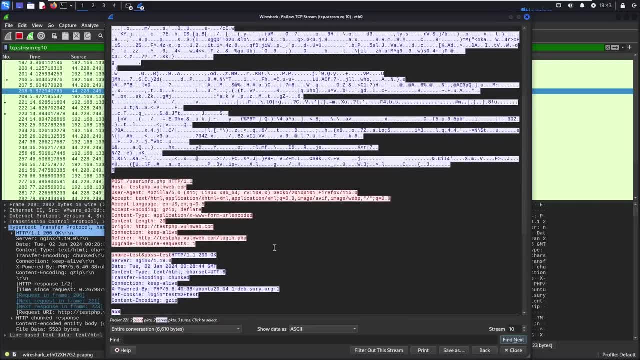 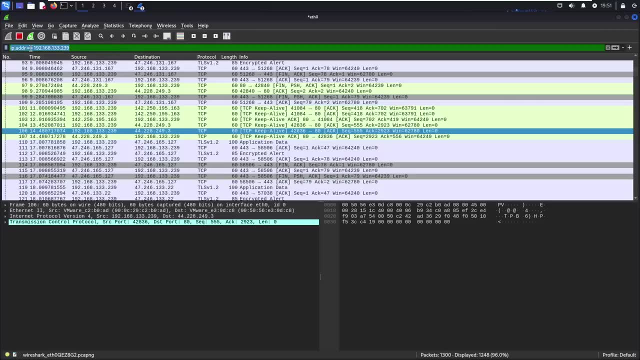 click on follow and click on tcp stream and here you will see some data which is encrypted. okay, but the username- here you can able to see the username- is test and password. you can also filter destination ip as well. So filter destination ip. what you need to do just type ipdht. dht is nothing, but it stands. 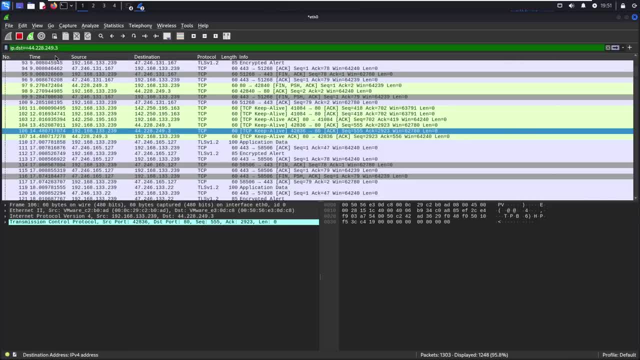 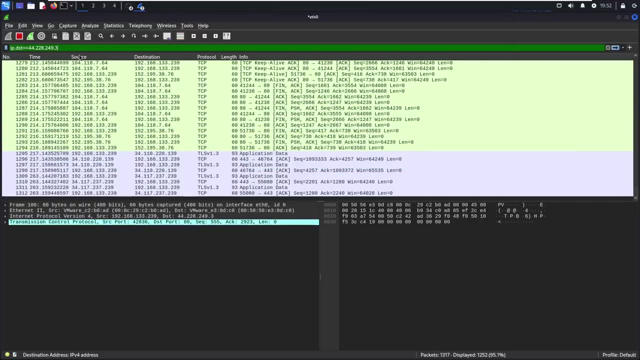 for destination and just type any ip address. assume that your victim is in. your victim or any user in your network is visiting continuously to one website. okay, at that time. simple, you can also select that website ip and you can also monitor it. okay, it's not a big deal, right. 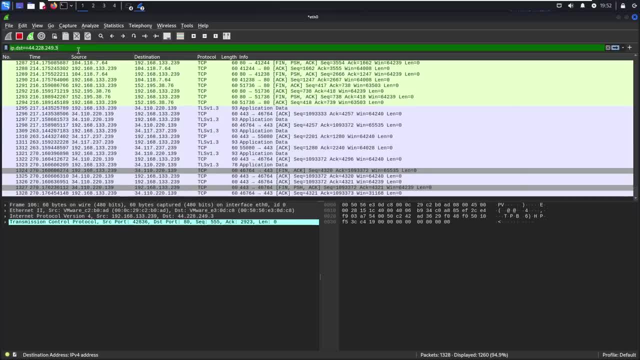 assume that he is using the website. the target website is using https protocol there. at that time, what will happen is right now we just see the test test there, the username and the password there. simple, the things will be encrypted there. you can't able to see the text in clear. 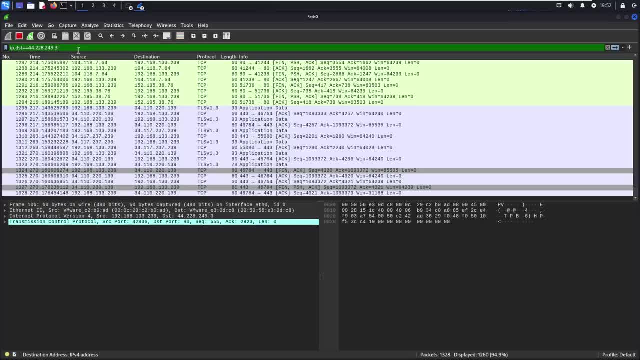 in a plain text. right, so it will be encrypted. you can't able to do anything there. simple, you can able to identify that. okay, your victim is visit visiting a lot to one specific website. okay, assume that in your network they are using the telnet protocol at that time also. 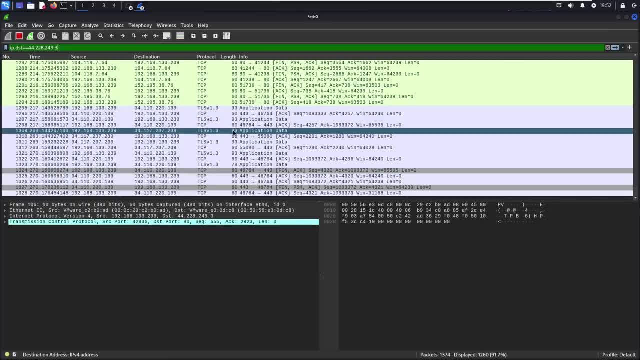 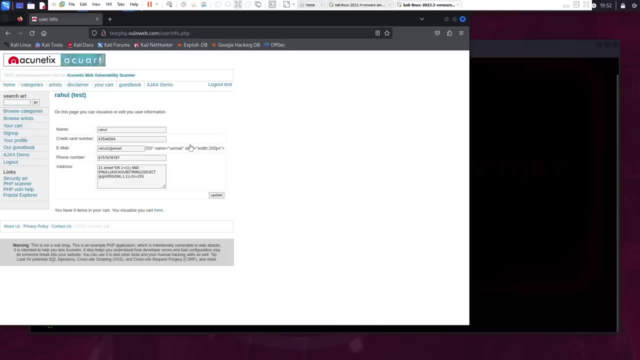 you can able to see the telnet username and the password in clear text. okay, this is the thing like we just saw: test test, right? so this is the thing like here in this website we just type test test. the simple thing is here. we just saw the username and the password. 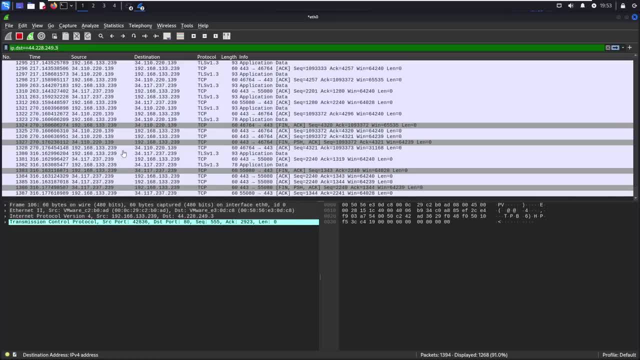 in a clear text, right? so because it's due to http, okay, http is not secured, so that's why we can able to see it, but mostly see in internal network in servers they host some websites. okay, they mostly it's used http protocol at that time. it is easy for us to: uh, you know. 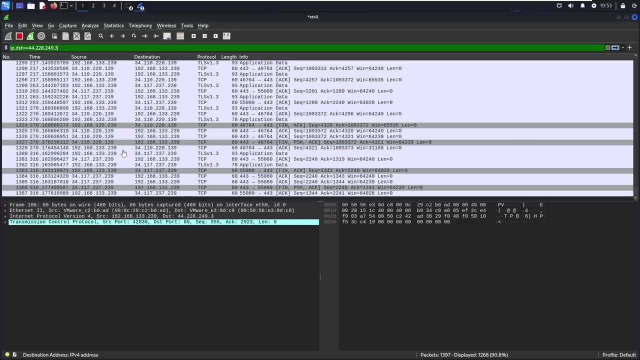 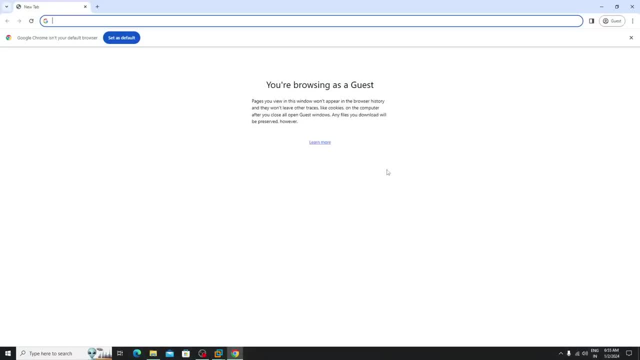 send an email to him. see the username and the password. okay, so you need a hacker. mind here this thing. okay, that's it now. in this section we are learning the backing right. so to perform the backing you need to set up a lap. was so, to set up a lap, what you need. 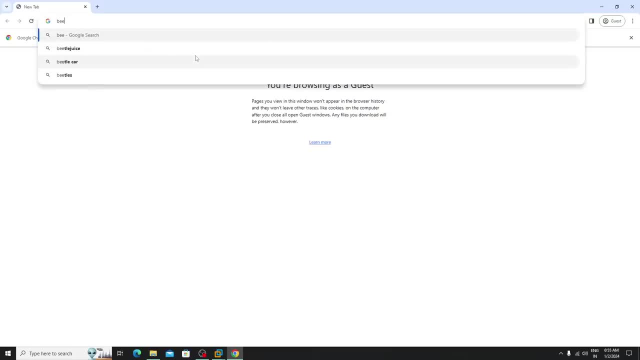 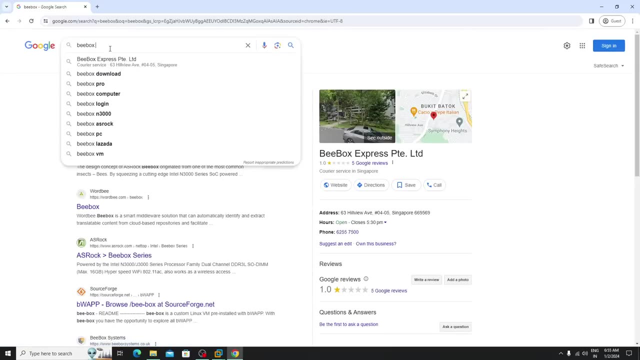 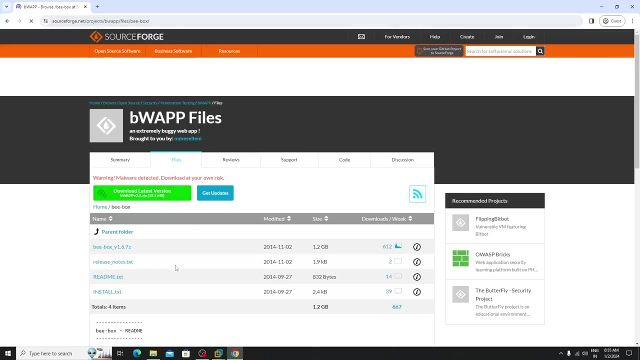 to do with just open Google and search for the box. okay, so here is a big box. on this one, let me talk it. here is a source: work: 0.. 0.. this url: just visit this url and from here, just download it. it's around 1.2 gb. 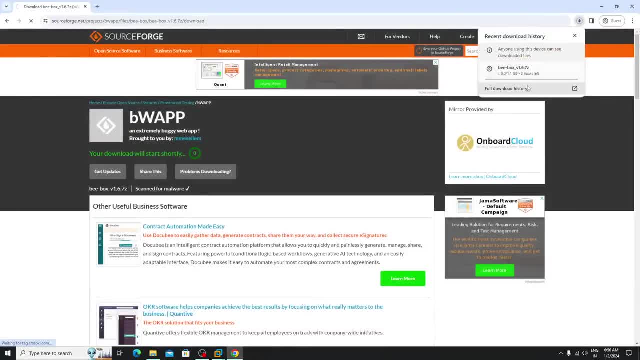 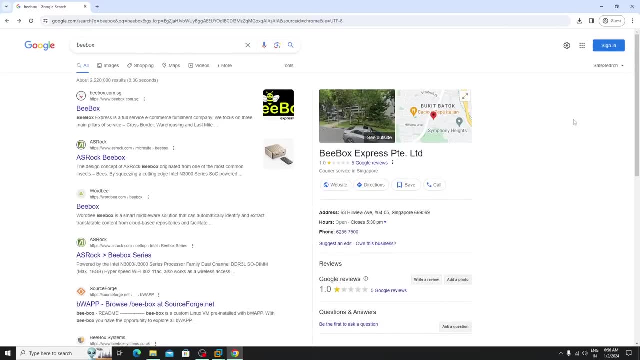 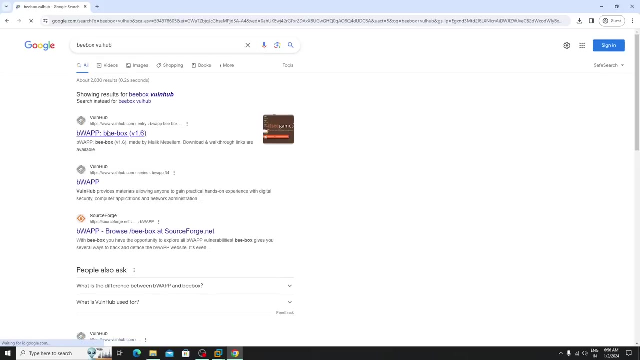 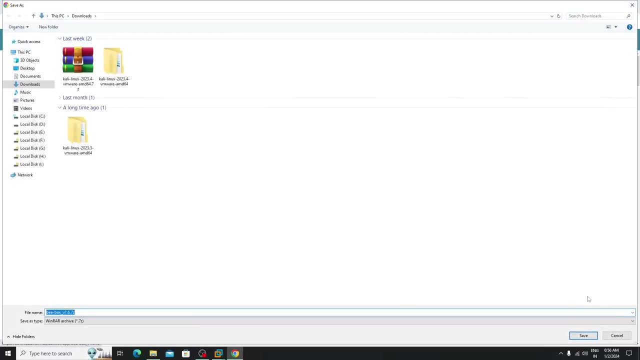 let me save it. it will take one to two hours, or let me go with. just wait, i think it's very slow, right, let me cancel it and let me go with fun hub. okay, here it is vbox version 1.6. let me download from here mirror link. okay, now it it, now it will. 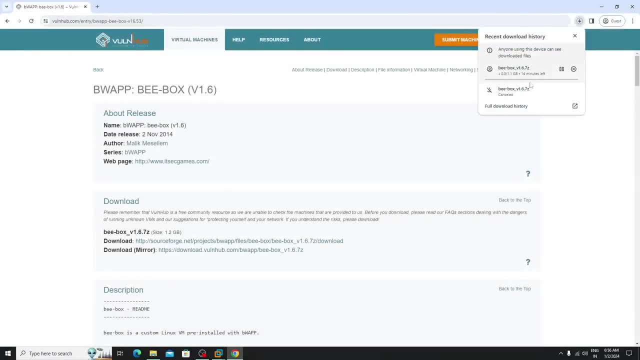 be fast. okay, just wait. okay, it's around 14 minutes now. so this is how you need. uh, let me show you how to set up a lap. it's a very easy. the same thing how you set up the kali linux right, simple. uh, unzip it so simple, double click it, it will. 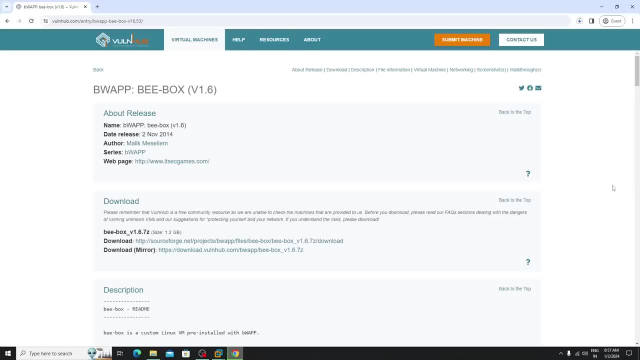 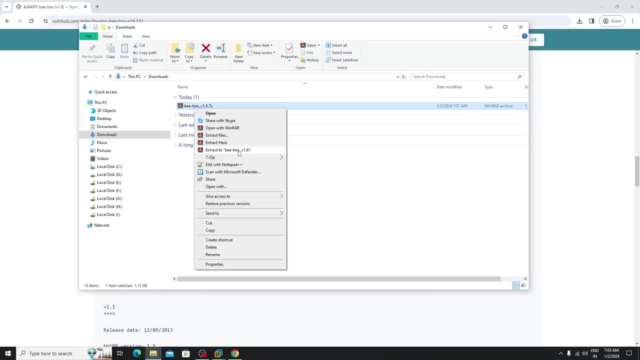 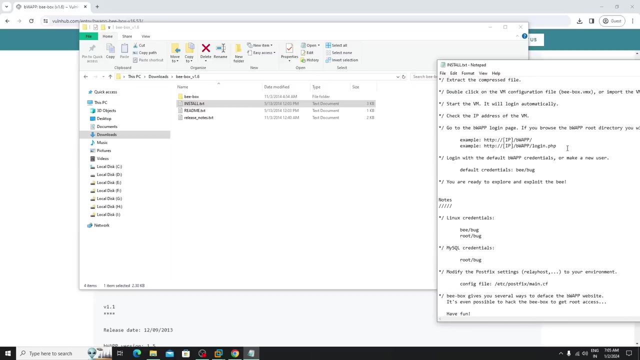 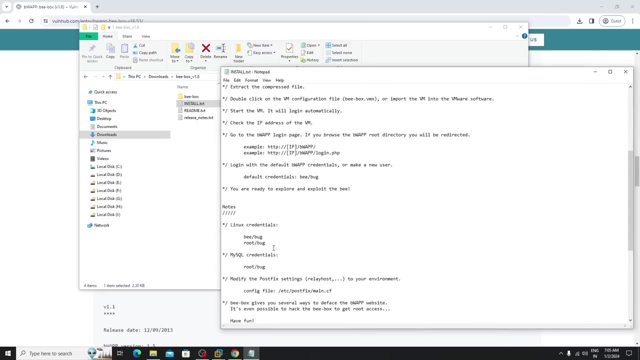 automatically open in vmware. this is the thing. okay, let me show you practical. okay, don't worry. so here it is. let me click on extract. so here it is simple. double click it here. there is a installation process like how you can able to install it. linux credential: uh, is here b bug, something like that. let me uh click on here you need to. 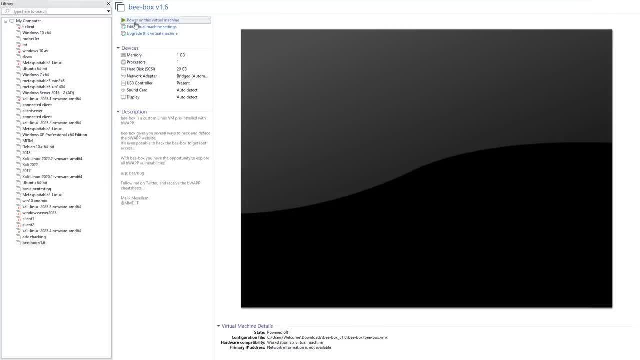 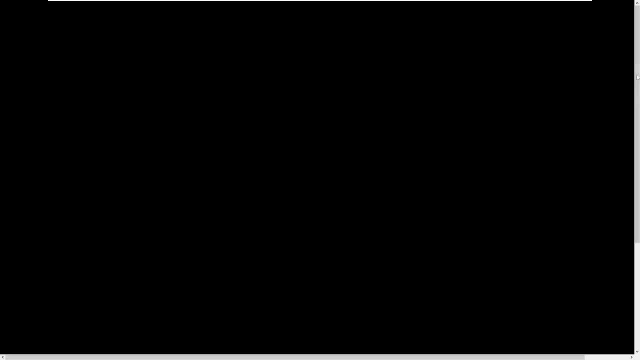 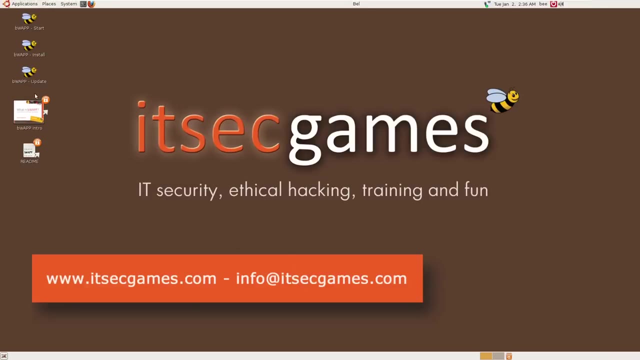 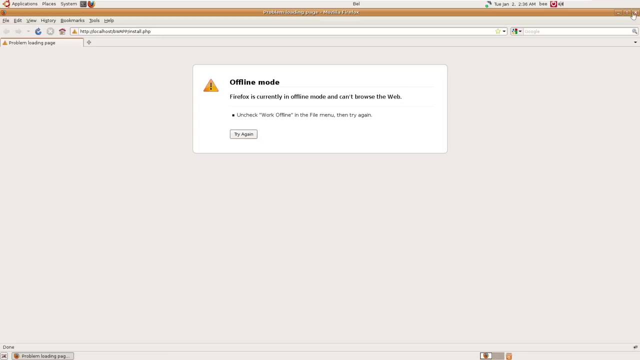 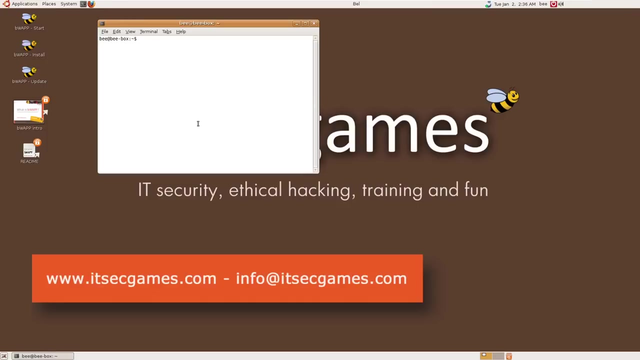 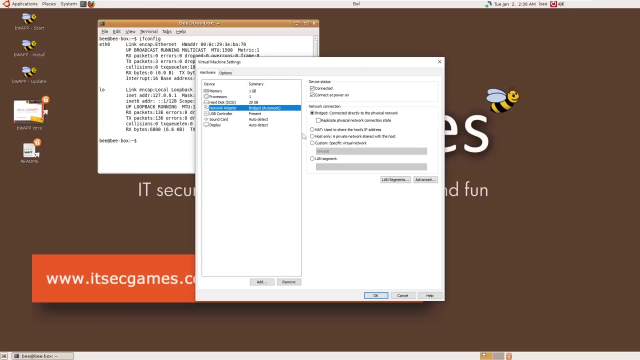 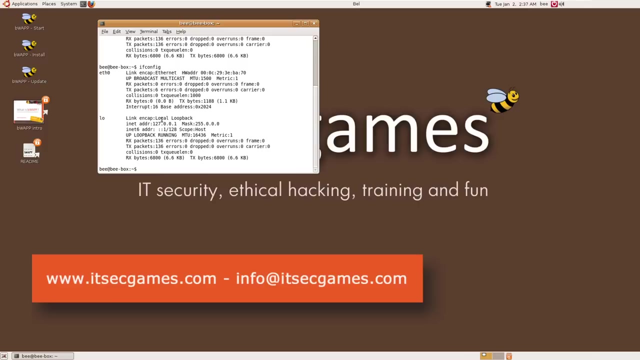 open vmx file and just power on. so here it is, just wait. see you have beenpe₊ install here. bbapp install is here. file again. let's type here ifconfig network adapter. just change it to not. ok, just type ifconfig again. let me restart it. 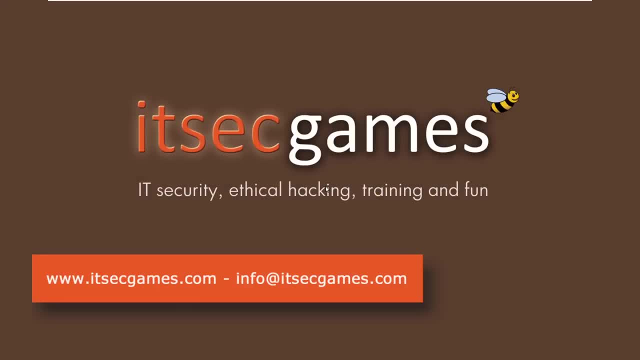 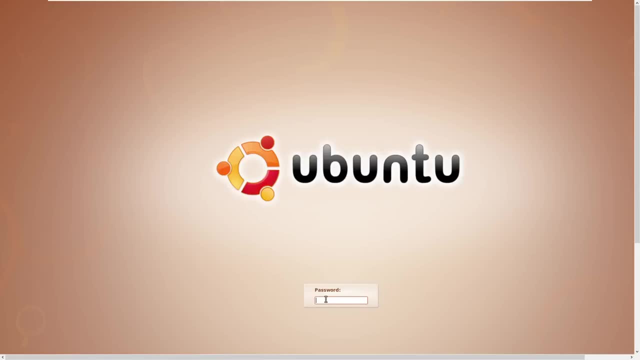 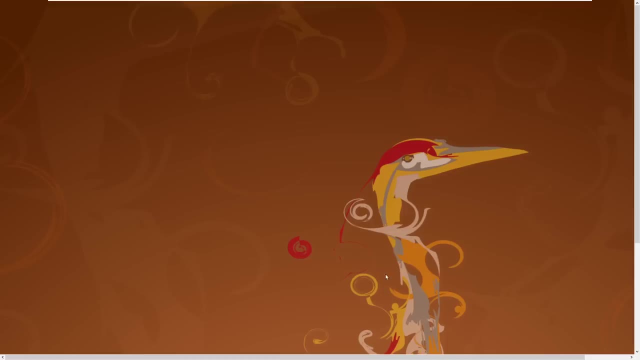 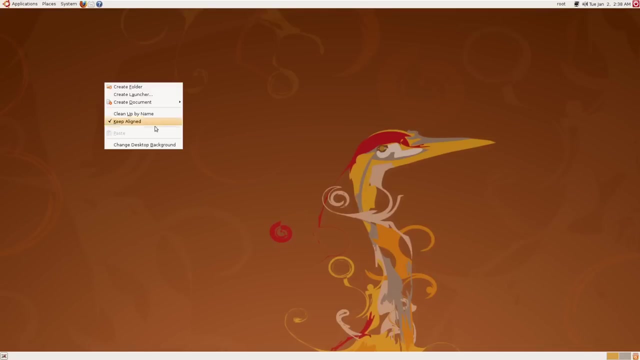 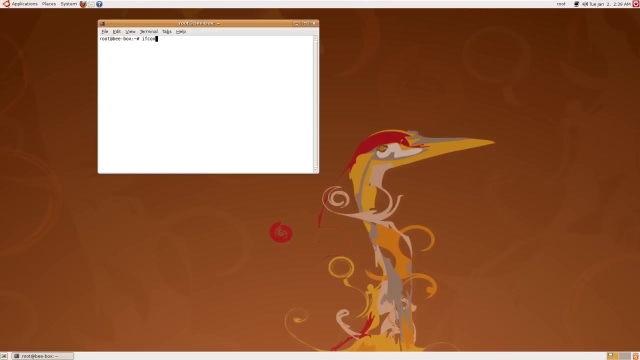 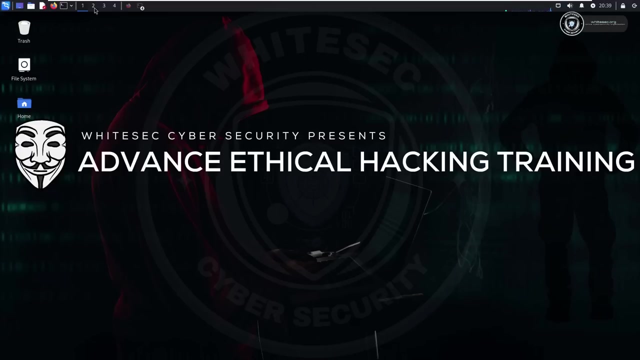 now, here it is. the username is root here. password is bug. click on continue. its a old version of, so here is the terminal. if i type ifconfig, this is ip address. right, simple, just copy the ip. let me use a linux machine here, so there is a. 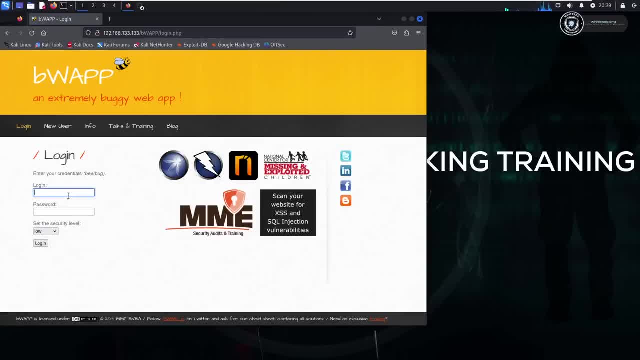 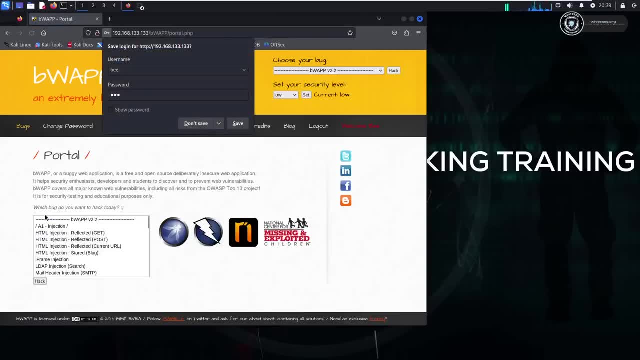 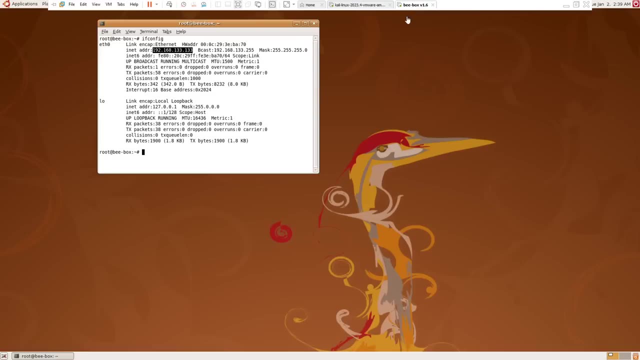 bbapp, simple click here. what is the username? username is b, sorry, login is b and the password is bug. ok, so here we successfully setup the lab. from here we need to perform the testing. don't have this machine, ok, because this is necessary if you turn off this. 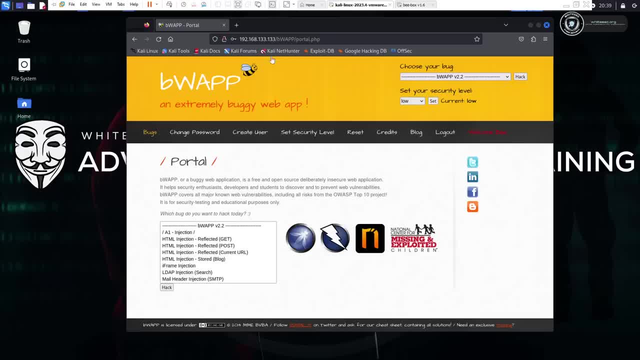 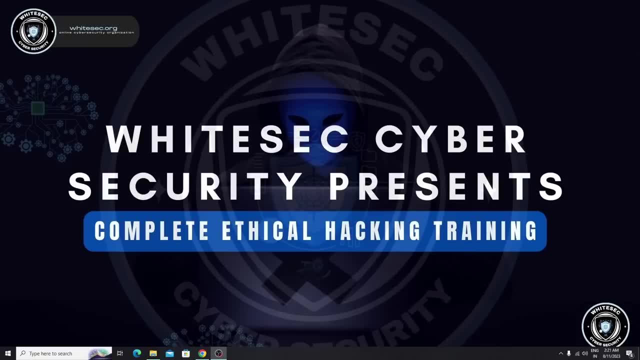 virtual machine, then what will happen? you can't able to access this page, this, this lab. ok right, hello guys, hope you are fine in this classes i am gonna teach you about google hacking. see what is this google hacking and how you can able to use it. its a very easy process. 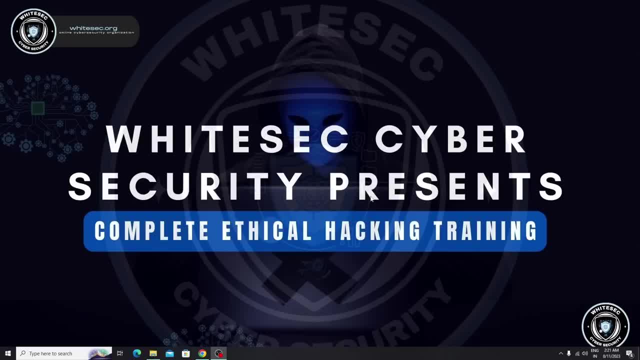 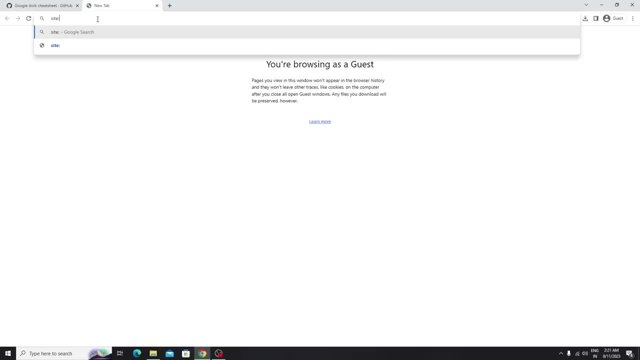 ok, first of all let me show you the practical thing, then we will. i am gonna try to explain about some theory there. ok, first of all the thing is: let me type one google dot here. ok, such as: just type here site semicolon, sorry, colon- just type here: 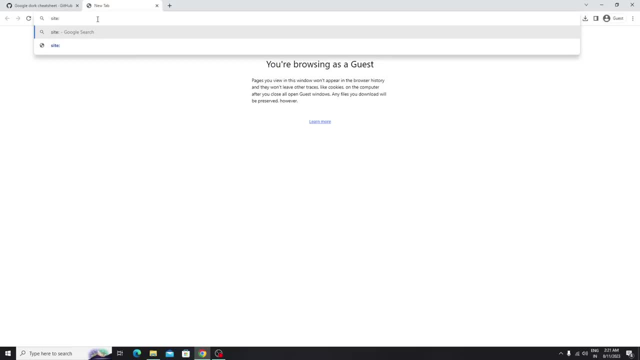 just select any site here, ok, such as uk, us, com, in pk, any site fr. ok, its totally depend upon you. like you can also target the country wise as well. ok, this is the thing. and in in title is there. ok, i am gonna tell you what is in. 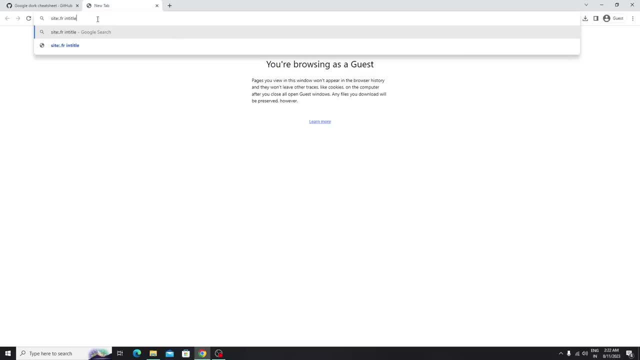 title each and everything. but for this no need any kind of explanation. ok, after since the results, you will automatically get what we are typing here. ok, this is the thing now, simple. in title, let me add colon again and just type the user name. ok, and again, let me. 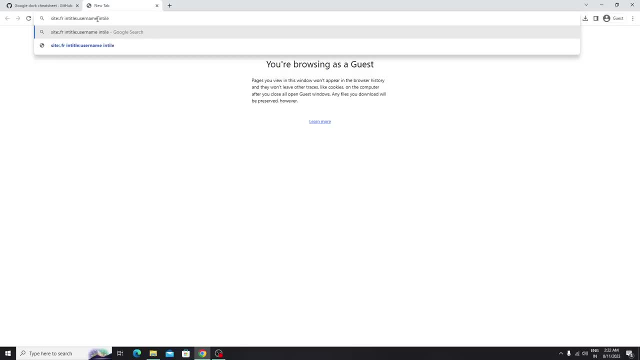 type in title and let me type here password. ok, now, if you type here file type, then here you guys can able to mention the file type. the file must be in pdf or xls or any document format. if i type here pdf, ok, just see what will happen. 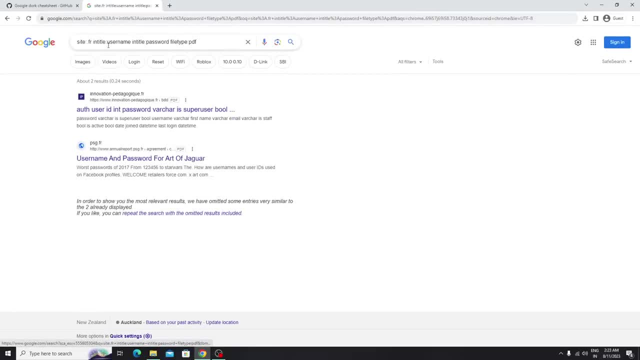 i can able to see the see there is a sites. ok, i got the two sites here. ah, here you guys can able to see at last there is a fr domain extension. ok, fr and fr. again, just see here: fr now in title. what is in title, in title is a nothing. 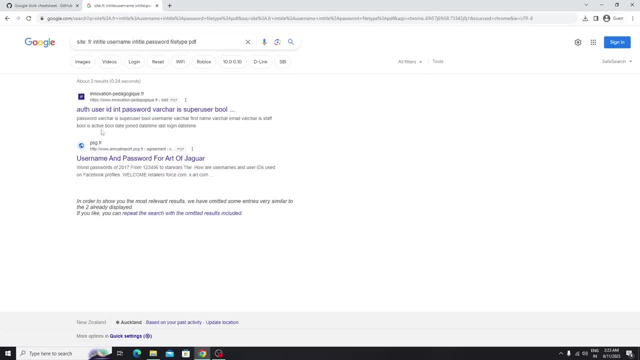 but this one, ok, here you guys can able to see password. here you guys can able to see user name and the password for art of jaguar. ok, if i open this one, then what will happen? let me see. see, here i got some stuffs, ok. ah, some kind of things. 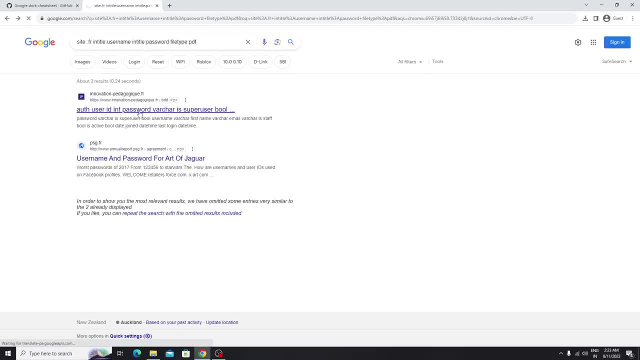 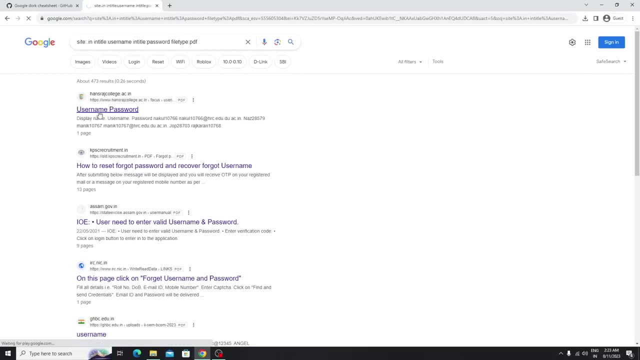 if i type this one here, i can able to see some ah pdf. now see if i type here ah, some kind of ah, let me type here dot in. see here i can able to see user name and the password. if i open this one, then what will happen? i can able to see the. 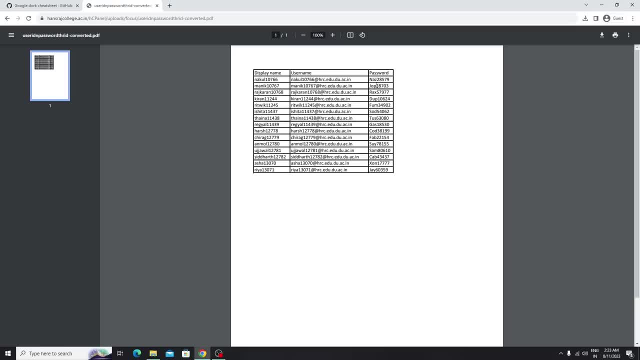 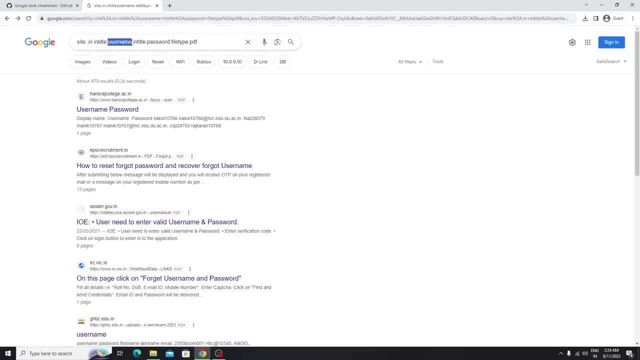 user name and the password here. ok, sorry, the user name and the password. basically, we can able to: ah, see the stuffs. ok, the files related to the keywords: ok, like i, i want to search for. ah, just assume that. just type any document name here, such as: let me. 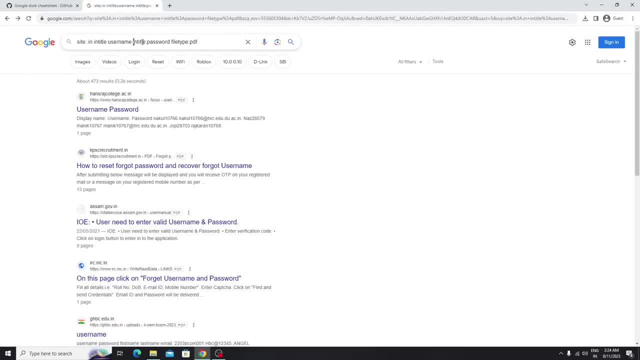 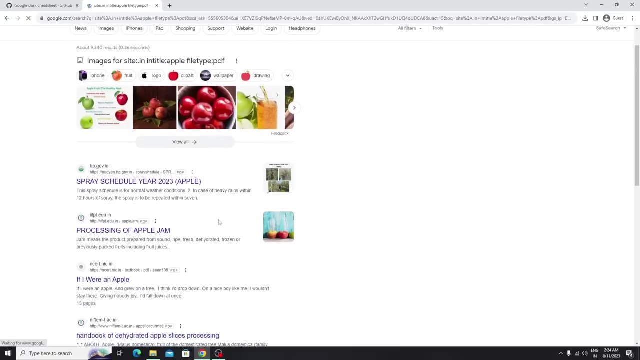 ah, type apple, something like that. ok, apple. and if i type enter here, i can able to see the apple. see in apple. i can able to see the apple in in: ah, in title. this is a in title. ok, i can able to see the apple and in which site? in. 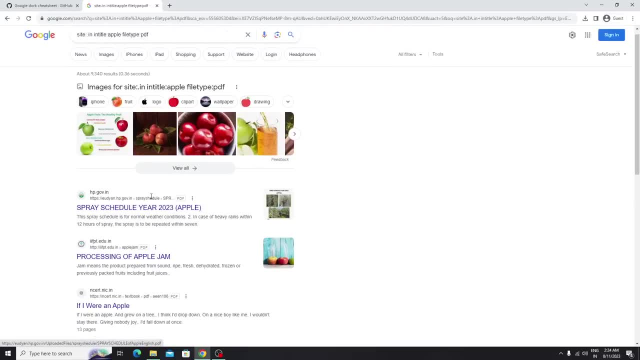 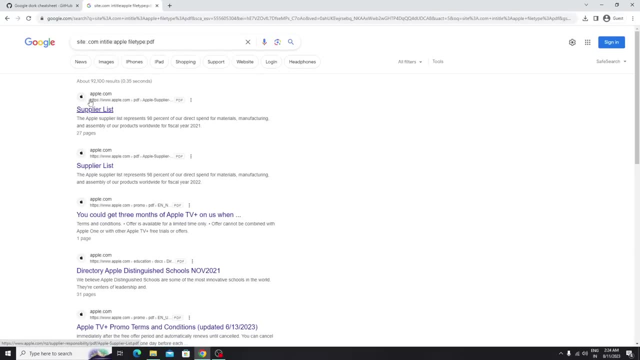 that extension of dot inside. ok, assume that if i change here dot com, ok, just add com there instead of in here. you guys can able to see the all the apple stuffs. ok, basically i can able to see the apple dot com here. ok, this is the thing, basically you are. 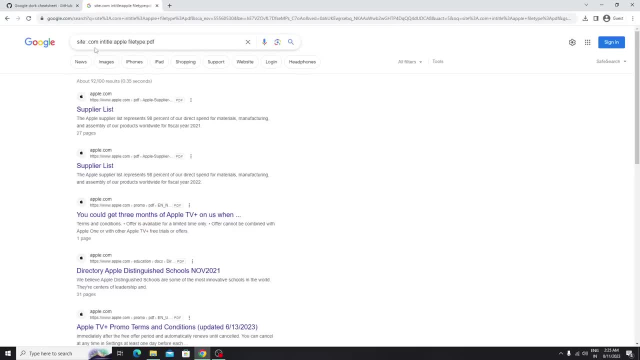 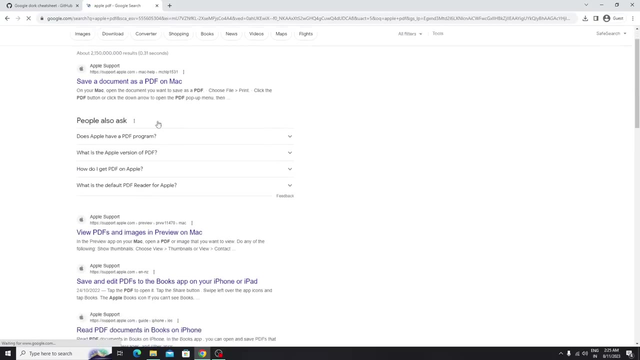 gathering the information which is necessary for you. ok, assume that i, if i type something like apple and just type here pdf or something like that, then what will happen? its ah, its ah. show me some kind of stuffs. ok, which i dont want to see. this all stuffs right. 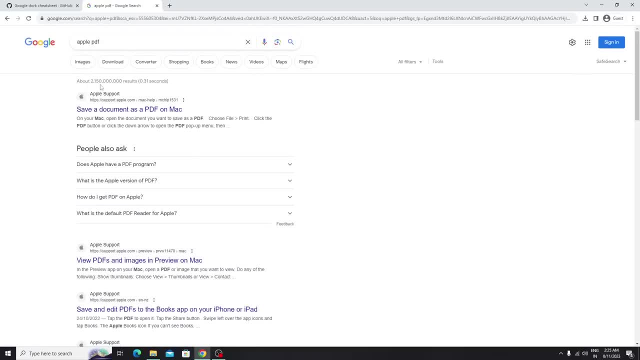 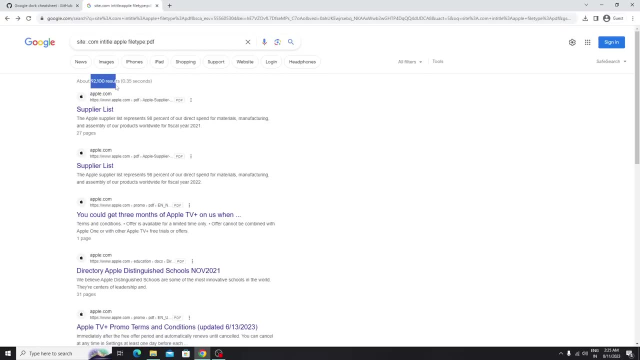 because its a very huge information. just see how many results are there. ok, what if i type something like this: ok, now see the results. its around ninety two thousand or something like that. ok, this is the thing. see each and every document here you guys can able to. 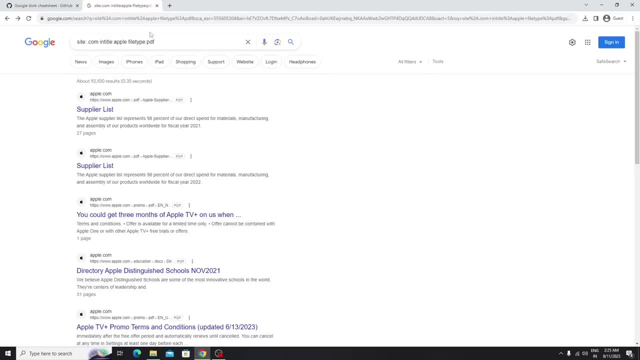 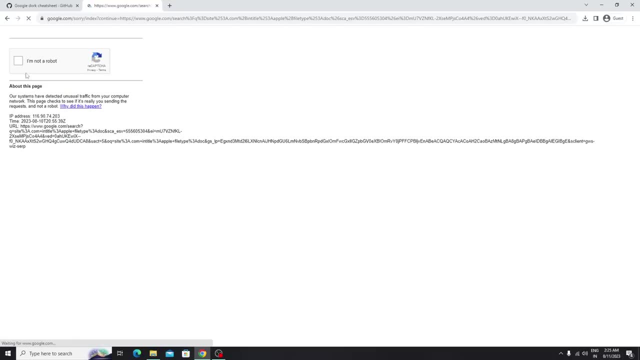 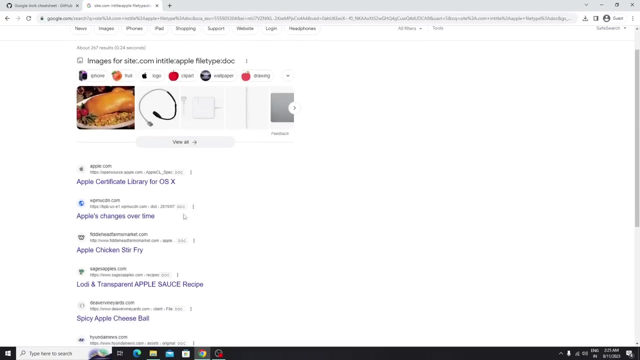 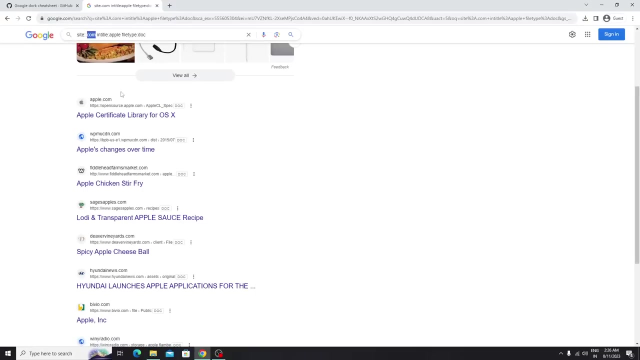 see the logo of pdf, pdf, pdf. if i type here dot doc, here you guys can able to see the doc extension. just wait, doc extension, just see doc doc. and in the website of what dot com? ok, just see, because i just mentioned the dot com, here you guys can able. 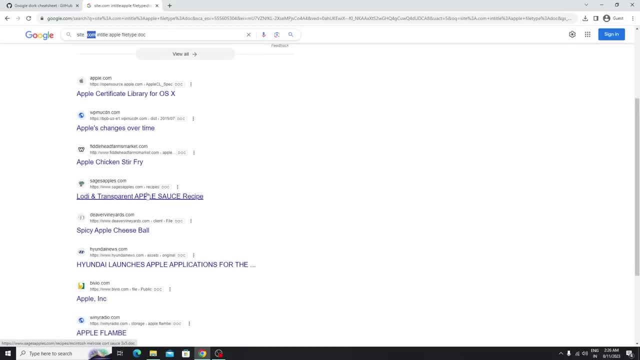 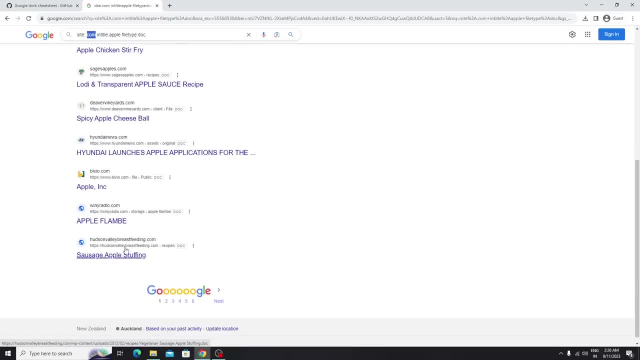 to see only dot com domains. ok, this is the thing. and also you can able to see in title. you can able to see apple, apple, apple, just see each and everything is apple here. right, this is the thing, guys. hope you guys get it, ok, what i am. 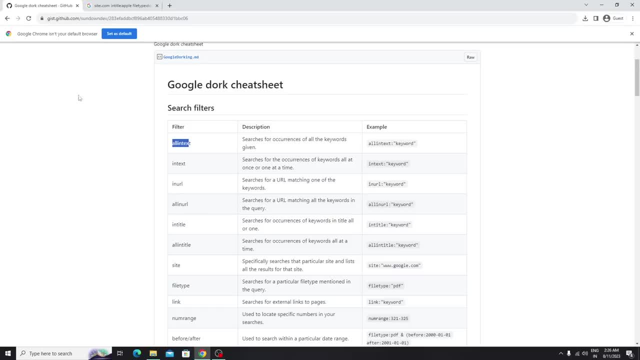 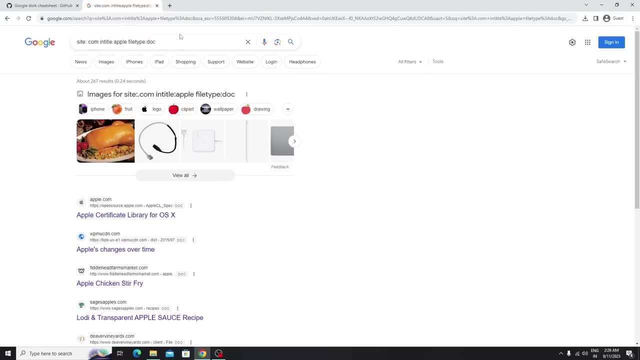 trying to say: now lets go to the google doc cheat sheet. here you guys can able to see each and everything. its known as a filters. ok, what are the filters here? see in: title is a filter, ok, and file type is a filter with colon- ok, remember one thing: with colon, 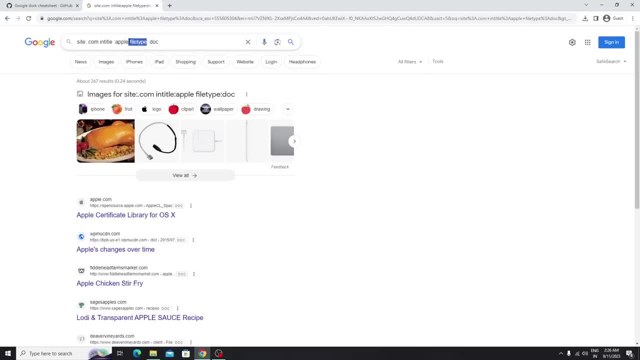 without colon, it doesn't work sometime. this is the thing with colon. ok, basically, what is this? this is a filter, filter. this things are filter. ok, this is the thing. just remove this dot from here. see, whenever you for search for the website. just see, let me show you another thing. 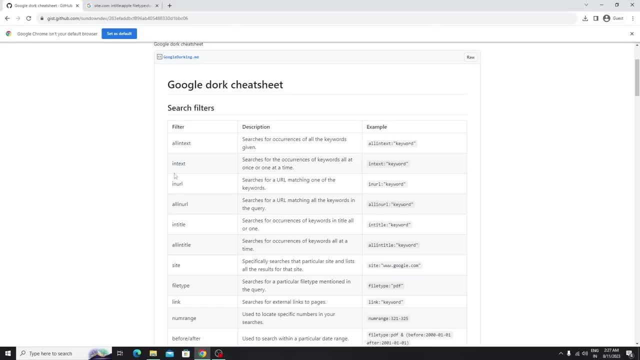 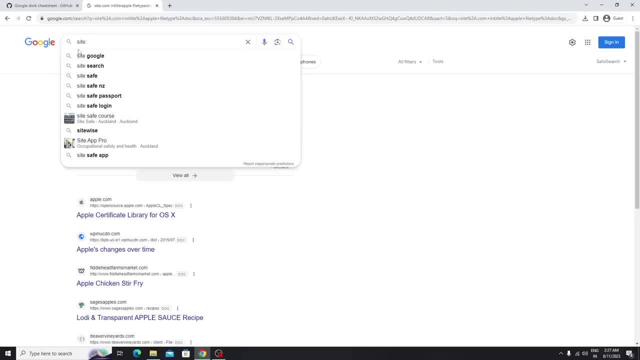 if i type here, just leave it. i am gonna show you later. ok, just first of all lets go with the filter. ok, now here what i used. i use the in title in the previous classes. ok, in title. where is the in title in title? here it is search for occurrence of. 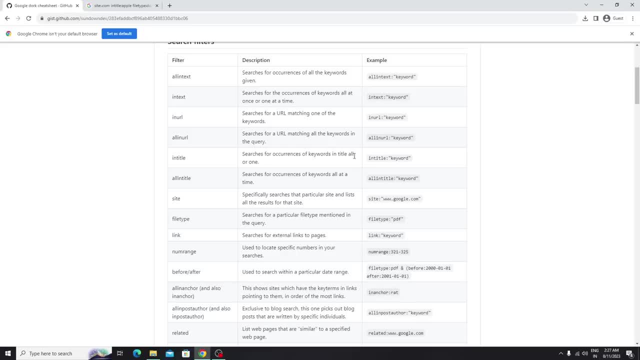 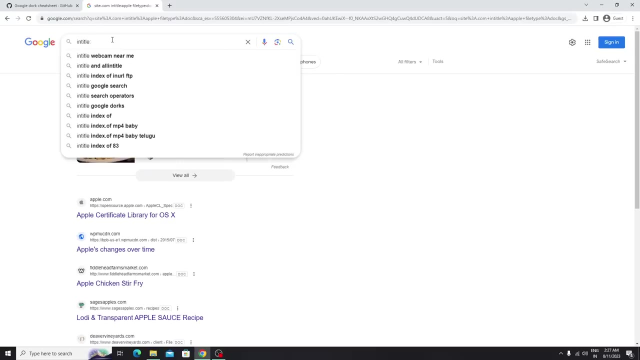 the keyword in title, all or one. basically here, if you type the in title and if you type any keyword, ok, just assume that. if simple, let me type here in title: ok, say colon, just simple, just type any name. ok, any name. let me type here something like nokia. 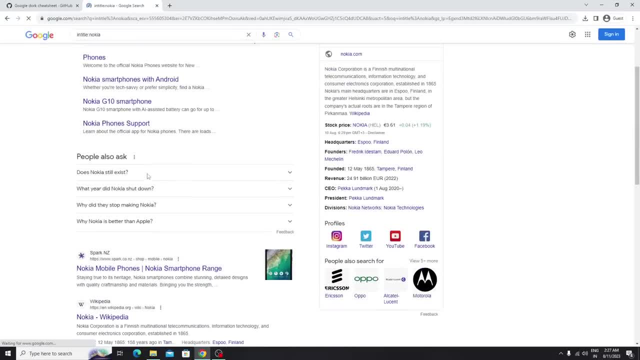 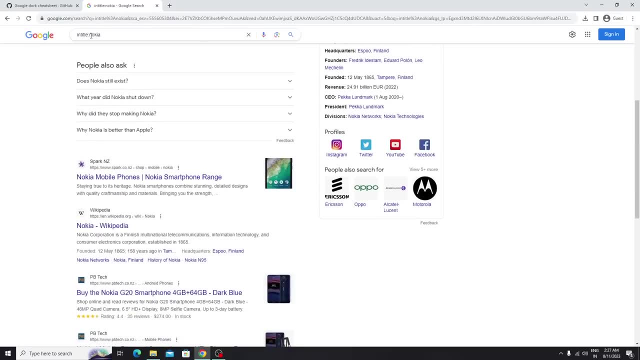 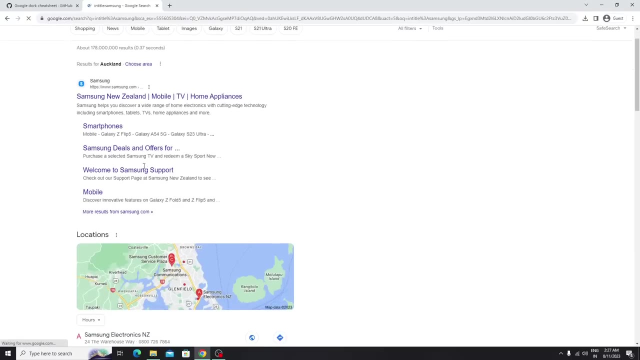 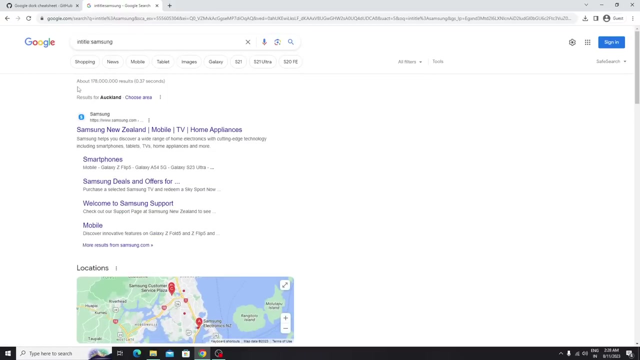 ok, here you guys can able to see all the information related to nokia. ok, this is the thing. if i type here samsung, you guys can able to see only the results about samsung. ok, see what is results. now the search results: it is around 178, blah, blah. ok, a lot of. 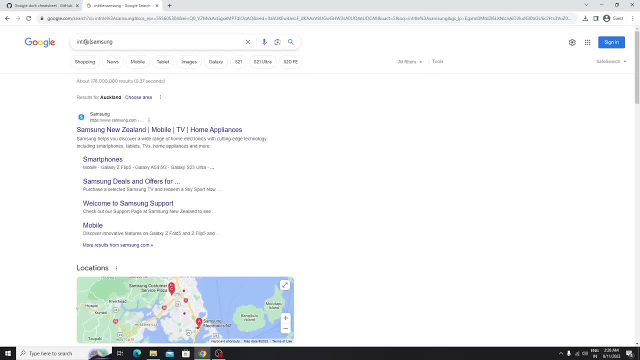 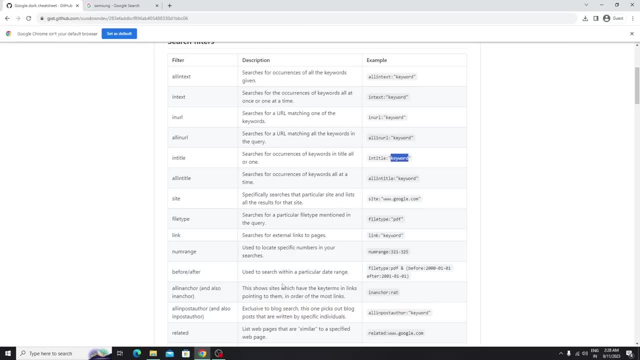 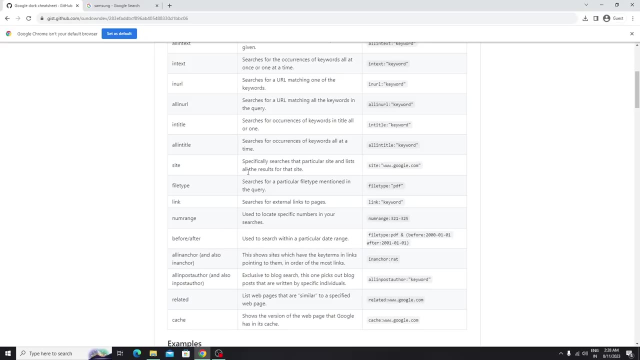 results are there if i remove this in title from here this filter, and let me search now see the results. ok, this is the thing. basically, we are filtering it. ok, now here is a site which we used specifically: search that particular site and list of sorry list. all the results for the. 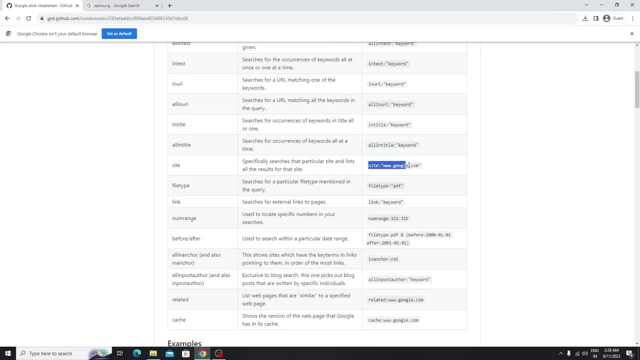 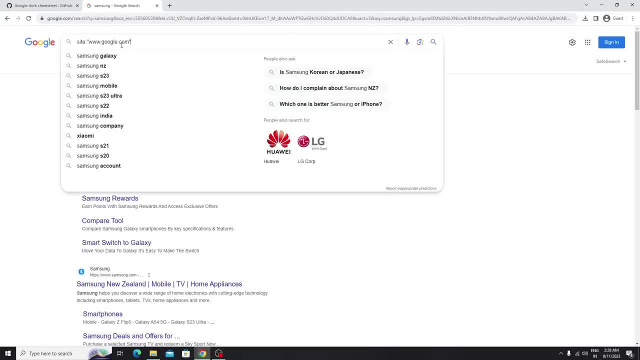 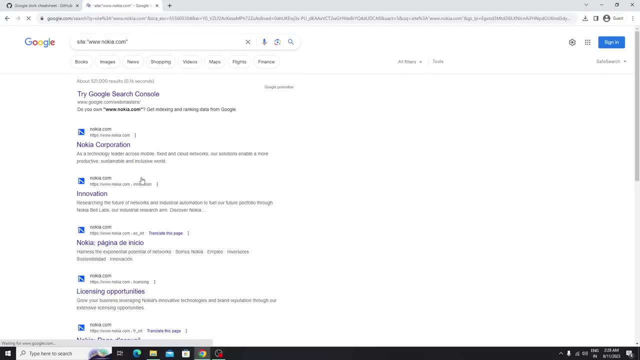 site. ok. if i type here: google dot com: see, this is a thing. ok, this is a example here. if i paste this one instead of google dot com, let me type here: www dot nokia dot com. simple, i can able to see the results about nokia dot com. ok. 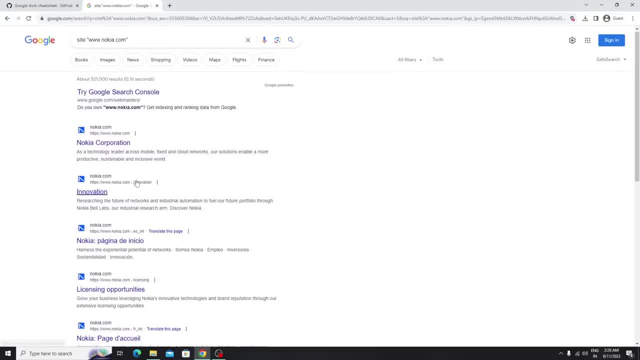 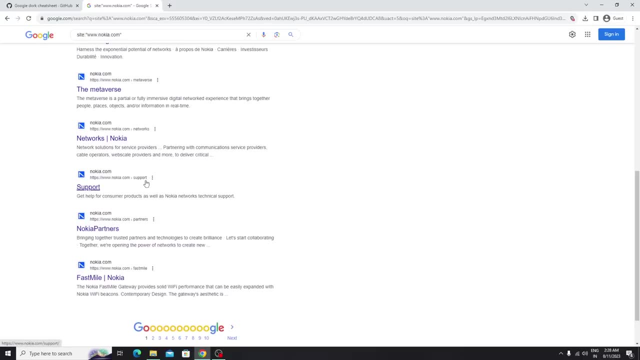 like see you guys can able to see the pages here. ok, how many pages are there? see, there is a metaverse is a one page here and network is a one page here. support is a one page, see here i am talking about here. ok, partner is a one page. 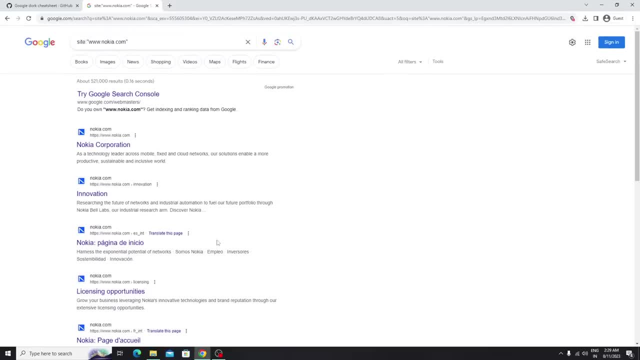 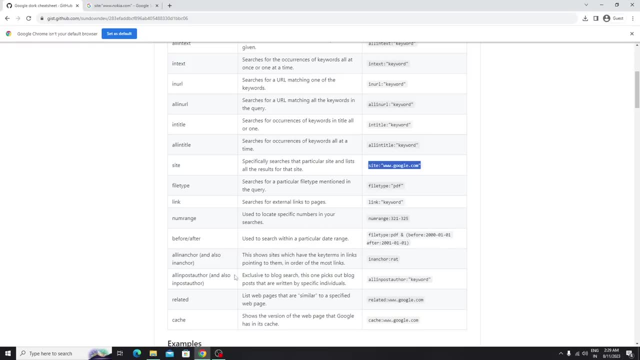 ok, this is a. this is a thing. ok, you guys can able to filter the pages, you guys can able to see the subs here. ok, this is a very excellent thing. and here there is a file type. i just use a file type search for the particular file type. mention it in the. 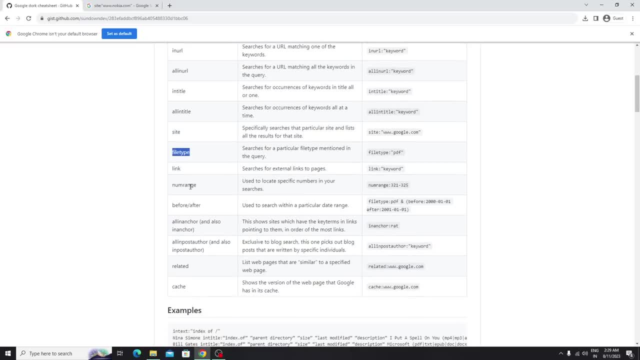 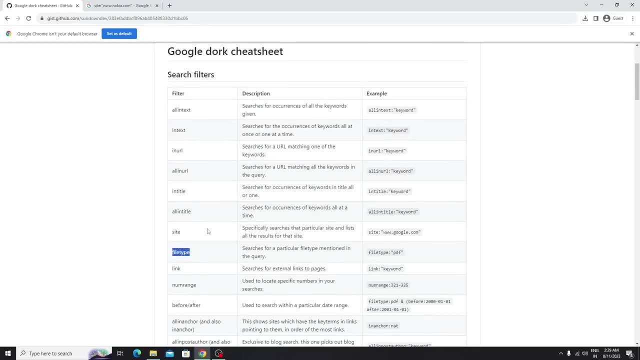 query. this is a thing and here is a number range. is there before, after all, in anchor? is there? ok, mostly we will use this. things only ok in title, in text, in url site. ok, file type, this kind of subs. now, here you guys can able to see some. 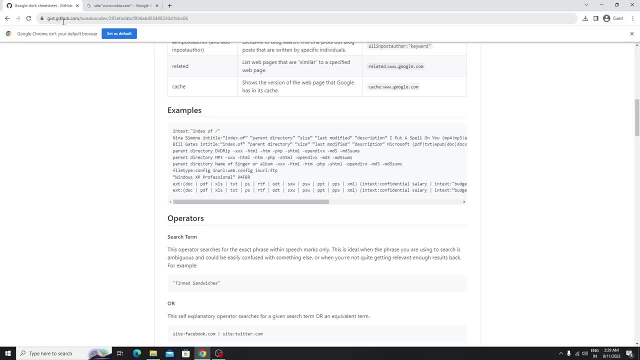 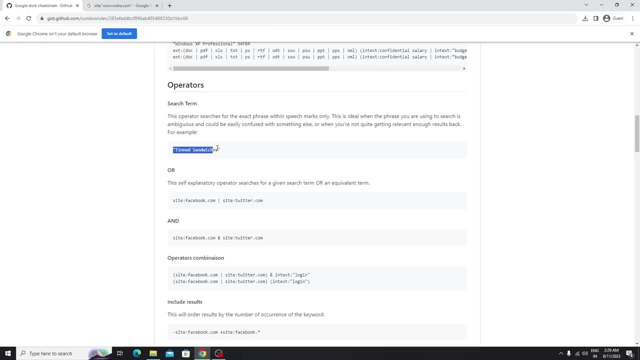 examples. just read this one: this is a github url, ok, and here you guys can able to see. some examples are there such as see: basically, if you search like this, then what will happen? it will show you some results. ok, see, basically, this is a keyword. ok, this is a keyword. 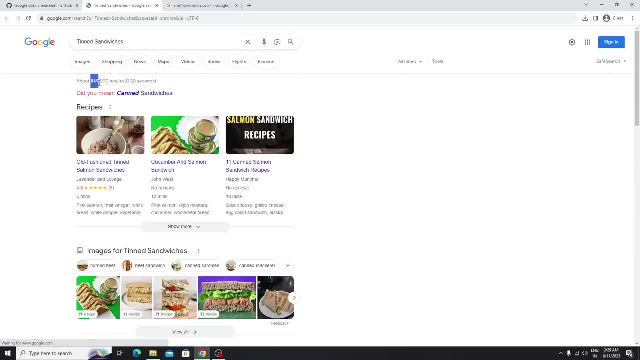 if i search like this, then i can able to see 849- some results there. if i add double quote here at the starting and the beginning, then what will happen? the results will be changed. see right now it's a 849. if i search for like this, then it's. 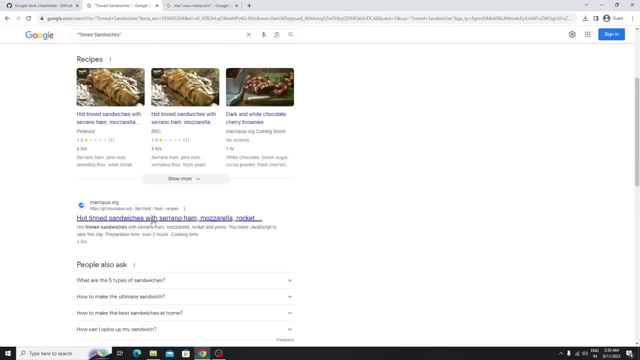 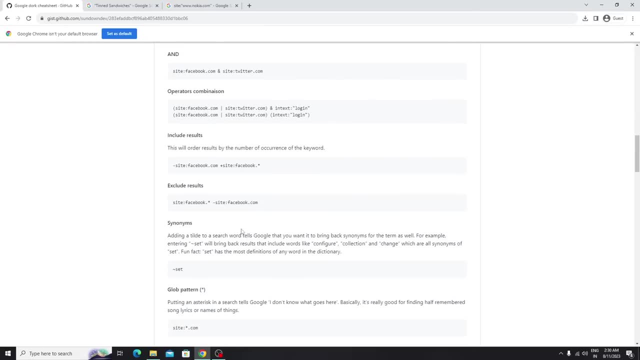 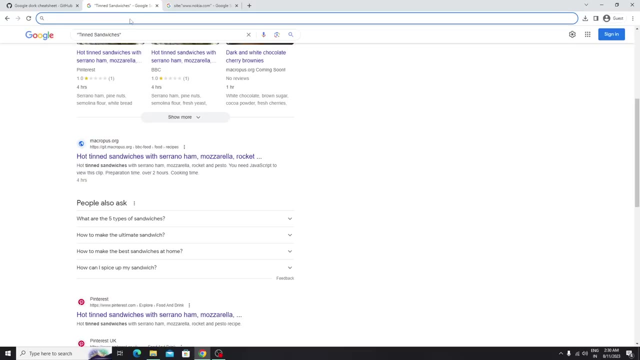 around 5180. so this is how you guys can able to filter it. ok, and you can able to do a lot of search. ok, it's not a big deal. just let me show you. if i type here, what is it- sorry, i just forget it- the google. 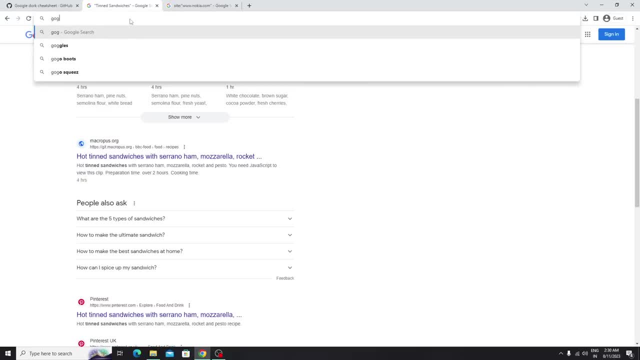 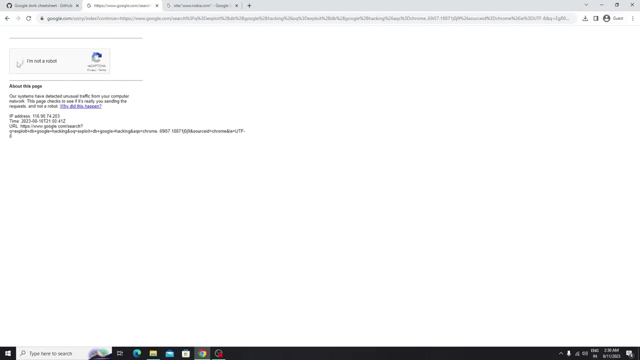 google, google. just let me show you this one. here you guys can able to see all the docs, ok, which are useful in real world scenarios. ok, what will happen means, time to time they will update the docs. ok, this are the limited docs. they are all unlimited of shops are. 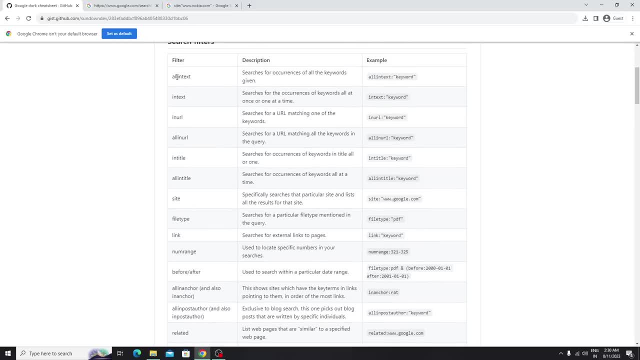 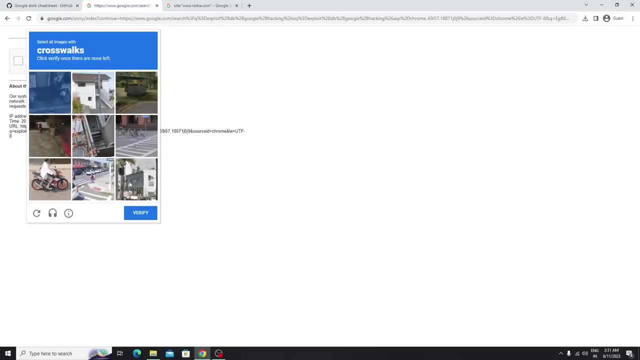 there. assume that sometimes it won't help you. ok, you can't able to figure out which i need to use. ok the simple. so that's why we are using this site. hell man, it's showing me a captcha, just wait. ok, now here you guys can able to see exploit db. 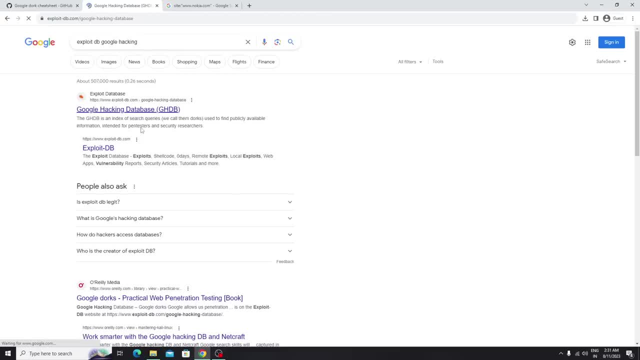 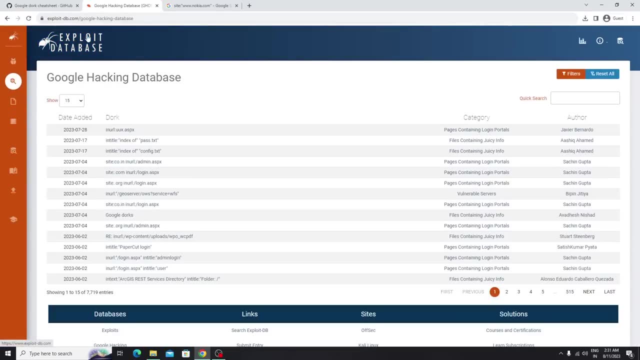 google hacking database. this is a best friend for you. ok, in the ethical hacking or pen testing, this site is a friend for you. ok, like a best friend. ok, this is a thing: here you guys can able to see the all the google docs here. ok, like, assume that in text is here we. 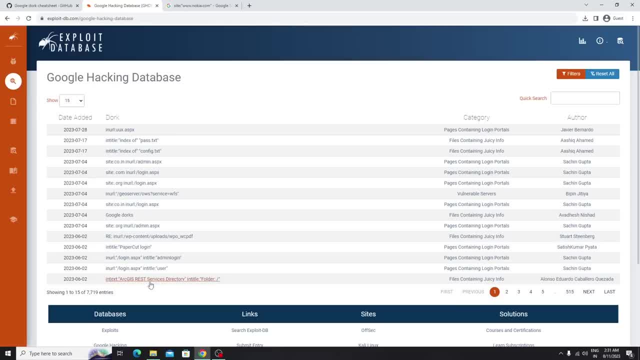 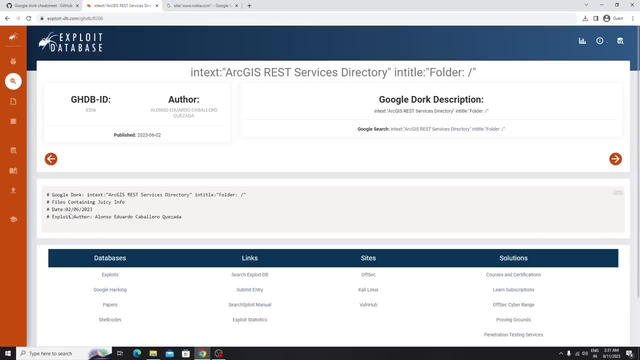 just learn about in text. and here, if i click this one, then you guys can also see the description file containing juicy info. date is 2013- 2023. here you guys can able to see the description as well. just wait, let me just assume that i want to search for the camera. 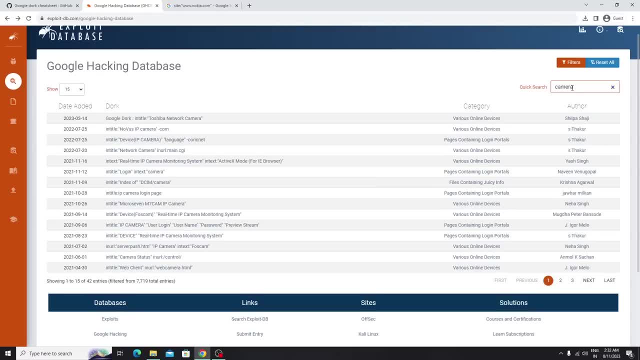 just type here: camera. ok, simple, just type, enter there and here you guys can able to see the. if you want to search for the camera, then this or the doc you need to use, ok, basically this is known as a docs. ok, now let me use this one. ok, i want. 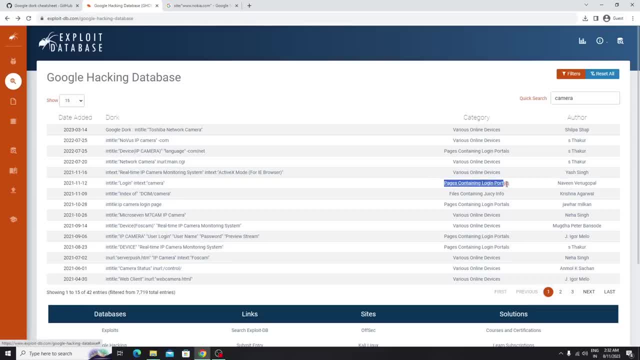 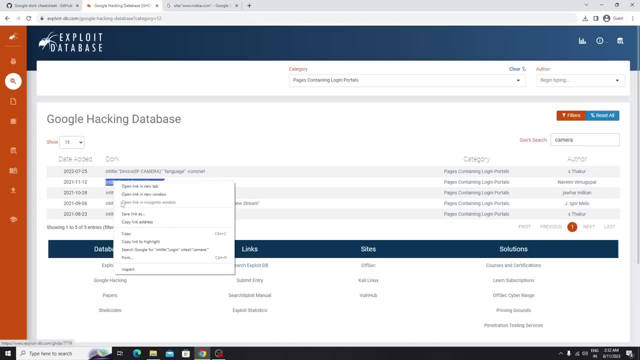 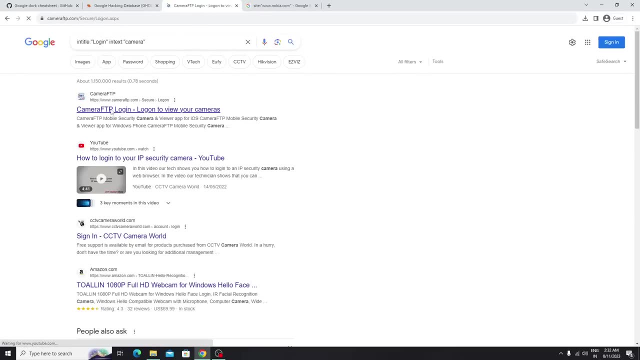 to identify the see pages contain login portal. see the category here. if you use this one, then what will happen? you guys can able to see the login portal there. ok, if i search here, see, i can able to see the login portal. if i open this one, then what will happen? it will ask for the 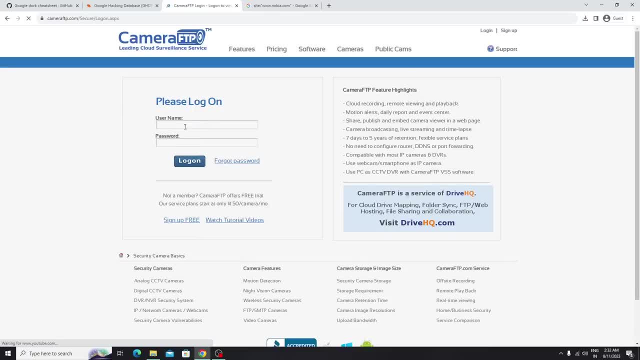 username and the password simple. in hacking, we we will perform the brute force attack, we will perform some kind of vulnerability assessment here or some kind of web pd. ok, this is the thing and i can't able to see. ok, now, here i can able to see the login. 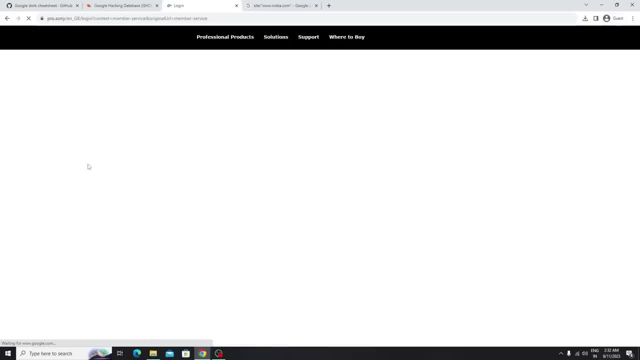 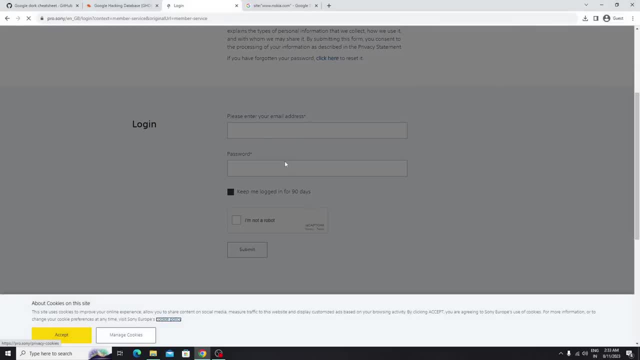 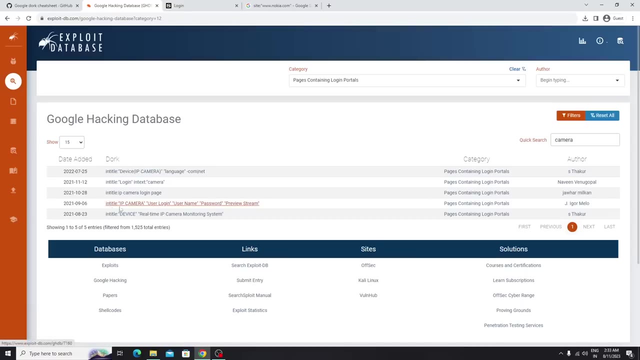 pages here. if i open this one here, you guys can able to see some login forms. ok, basically, you guys can able to perform the account takeover vulnerability here, such kind of stuff, ok. and there is a intitle- ip camera, see intitle. its also using the intitle ip camera keyword. 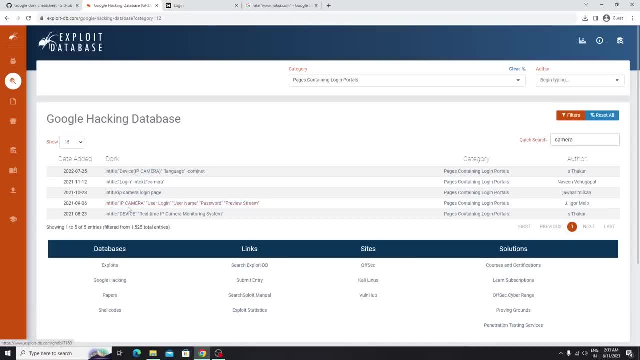 ip camera is what here? its a keyword, ok, and its specifically its looking for the user login, username instead of intitle. he can also add intitle, user login or username or something like that. ok, if i copy this one. ok, see, here you guys can able to see some. 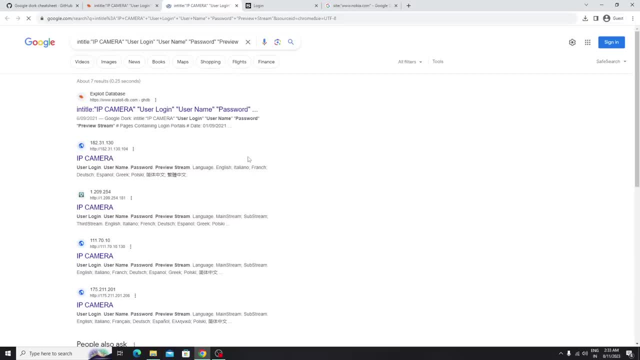 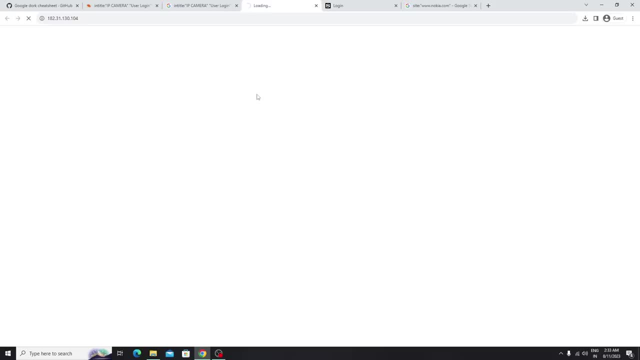 results. ok, i got one ip address. if i open this one, then i can able to see some username and the password. basically this is a exposed ip, so you can also say it as a exposed ip. if you exploit this ip, assume that this ip, this network, is running in. 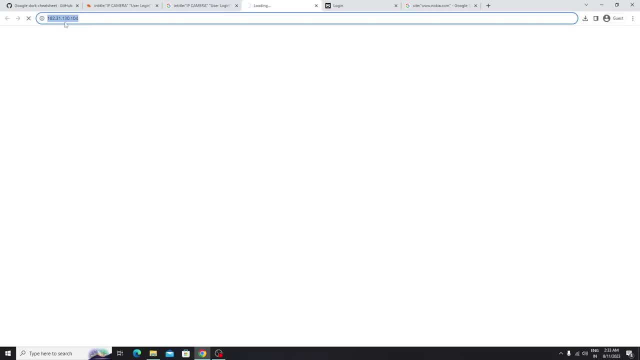 one real, from the real world organization. ok, ok, assume that this is a vulnerable. if you exploit this one, then what will happen? you know, you can able to take the control of that stuff. ok, you can able to enter in that organization. from there you can able to perform the. 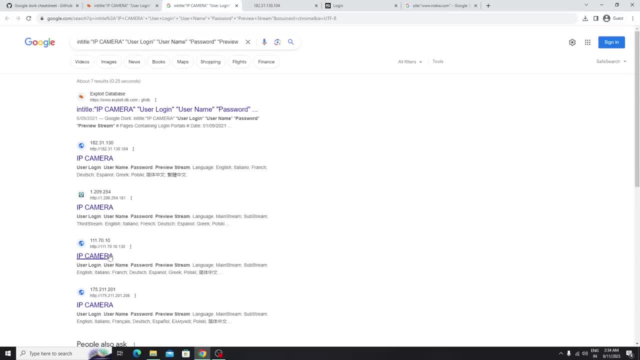 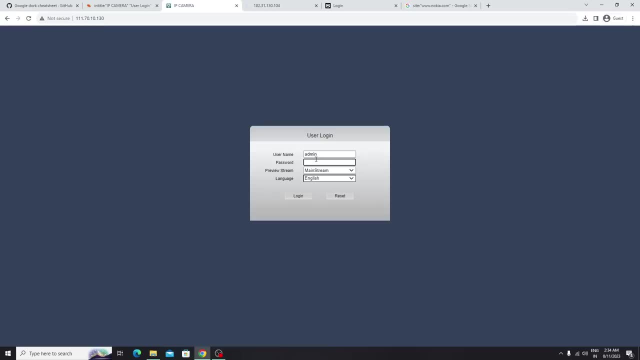 some other attacks. ok, this is a thing. see, you guys can able to see a lot of ip addresses, ok, and here its asking for the username and the password. now let me tell you one. real scenarios, ok, like in the, maybe in yesterday or something. what happen means i just 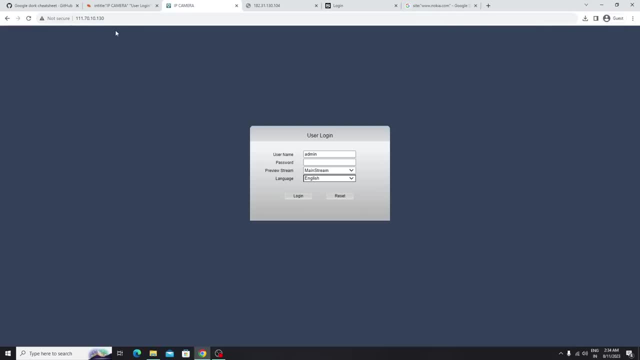 scan one network. ok, like its a. basically its a government ip address. ok, like i just scan its a public, its a- basically that is a public domain. ok, like gov or something like that. i just scan that domain and i can able to see huge ip addresses there. i can able to see one. 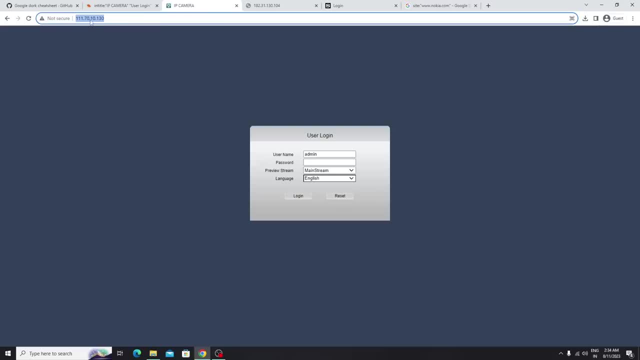 camera. ip address: same like this one, only ok from there. what happened means the portal is vulnerable. ok, simple, i got the reversal. i just dumped some credentials there, i just entered in that organization. ok, simple things. ok, its a very simple thing, its not a big deal, ok, basically. 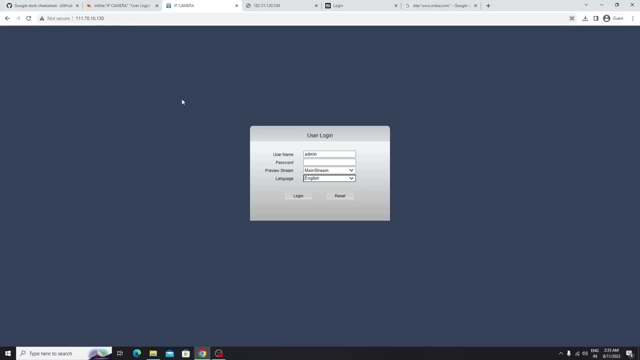 its. i just told you one example. right, its not that much easy. i just find some admin panel. its a process, but here from here what will happen means you guys can assume that if any user using the same username and the password for the admin login, you can able. 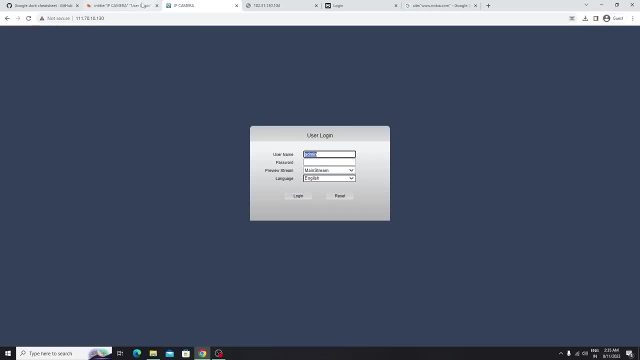 to dump it. ok, like its a very easy process. its not that much hard. but let me tell you, by hacking this one, you guys can able to do a lot of shoves. ok, by hacking this ip address, you will learn each and everything how to scan this ip. 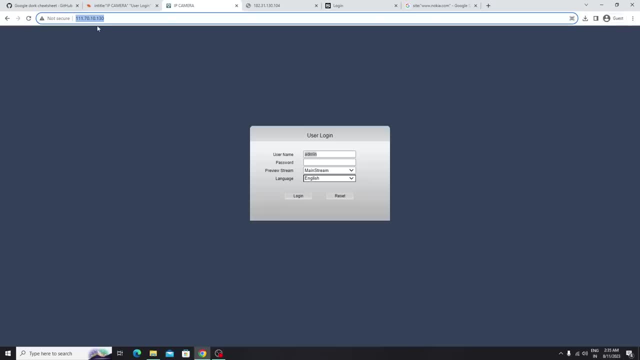 address how to find the vulnerabilities. each and everything. you no need to worry here. assume that you are not getting my words. ok, right now you cant able to understand the things. still, you no need to worry. ok, you will see each and everything in the real world scenarios. 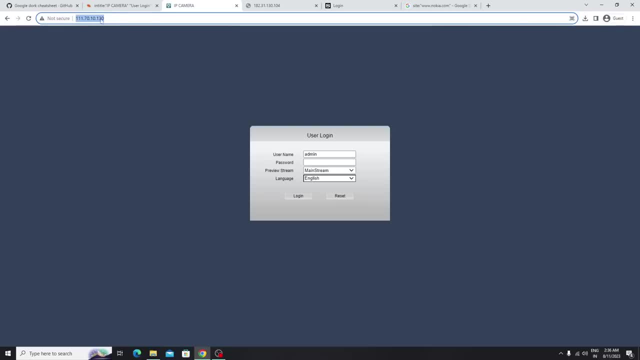 as well. ok, see, i got the ip address. simple, i can able to copy this ip and i can able to start the scanning on it. ok, assume that i found some vulnerable servers there. simple, i can able to exploit it and i can able to enter in that network. ok, from there i 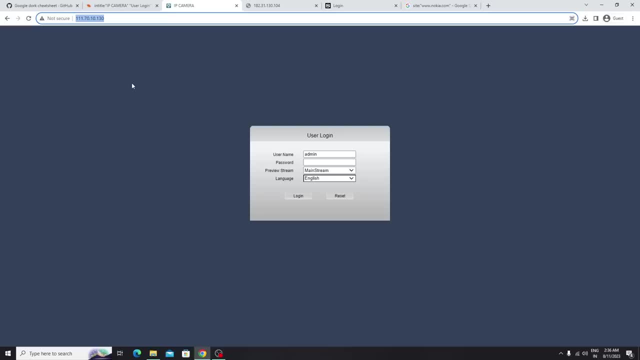 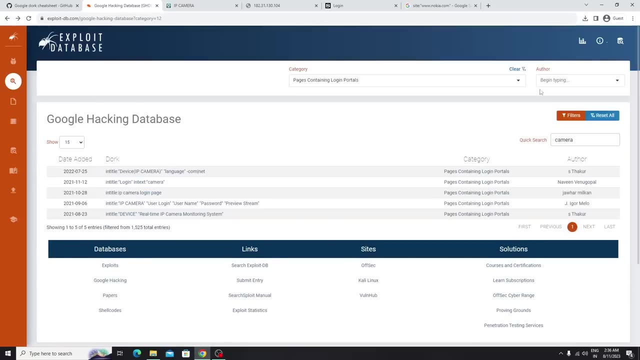 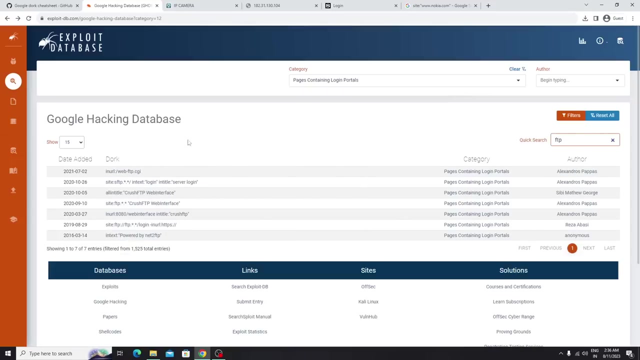 can able to perform the credential dumping. ok, its some kind of shoves. you will see that in windows pen testing. ok, this is the thing. now lets go back and let me search for some other shoves. ok, now i want to search for the ftp. now, here i got some cool things. 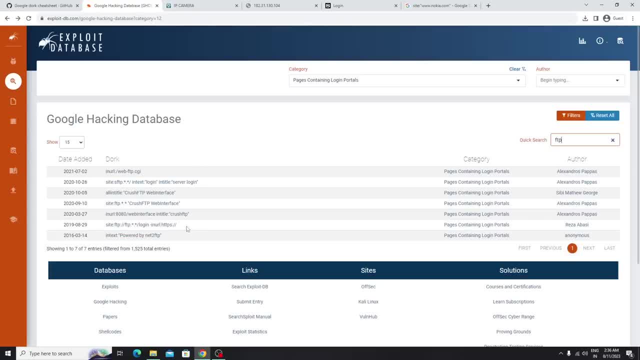 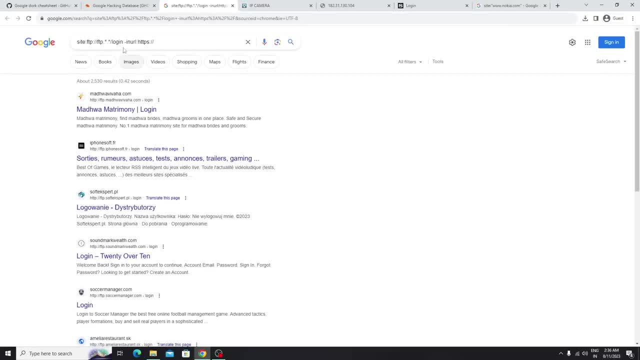 about the related to ftp. ok, and if i copy, let me copy this thing and let me search here. ok, and here this is a protocol. instead of this protocol, you can also add the http as well. just remove it. you can also modify it. its not a big deal, ok. 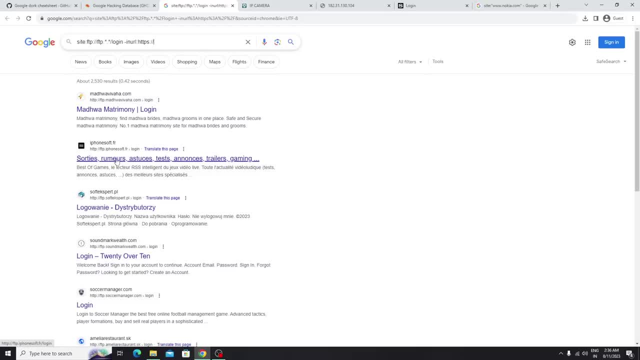 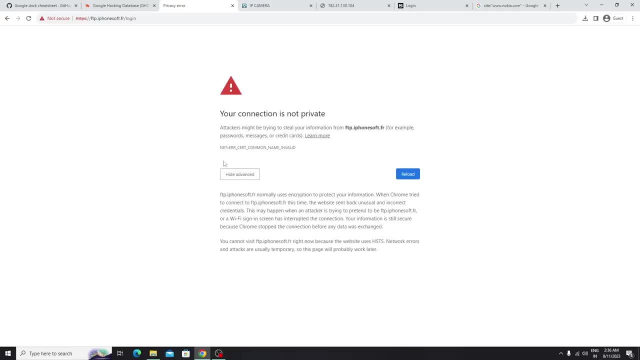 and here i got some related to fr. if i open this then you will see some login. ok, see, your connection is not private. if i click on the advance, if i here you guys can able to see there is a. the hell man i cant able to see. 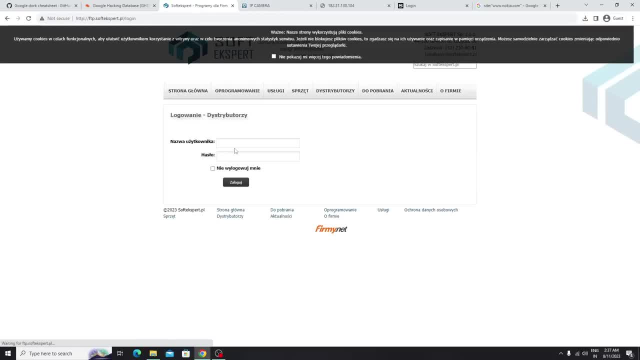 i can able to see the username and the password here. simple. see, you can also perform the brute force attack. ok, its not a big deal simple. what is the default username and the password? its always admin and admin. ok, if i type admin and admin, if i type enter, then 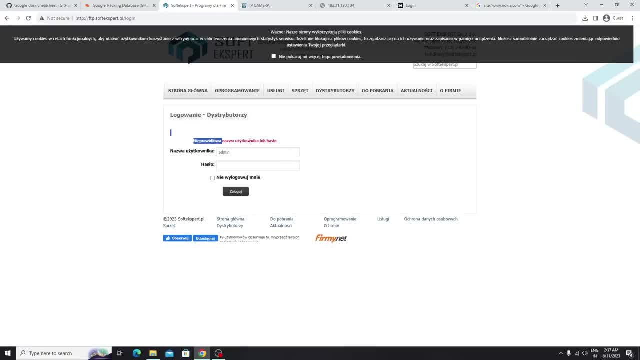 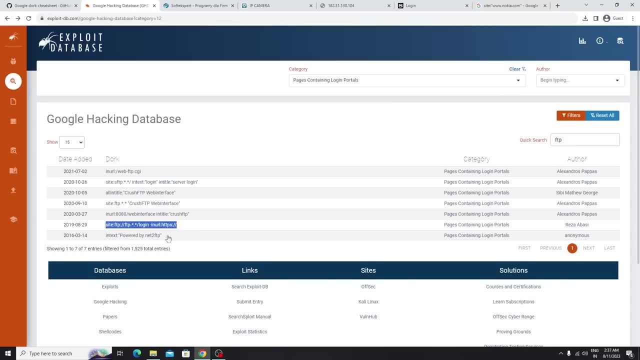 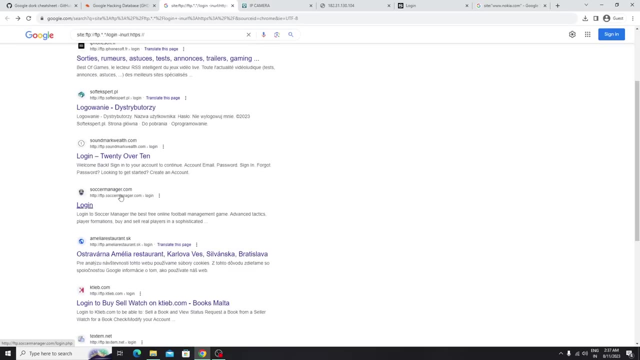 now its a username and the password is wrong. there are two chances: just find the vulnerabilities in one- this page- or simple, just perform the brute force attack. ok, what i am showing. i just ok. here there is a soccer manager, is there? ok, this is ftp server. if i login here now its ask for the. 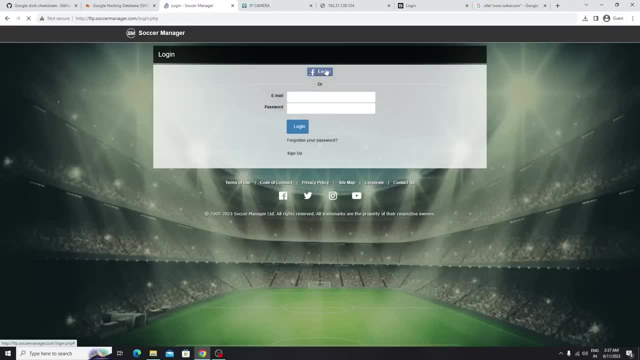 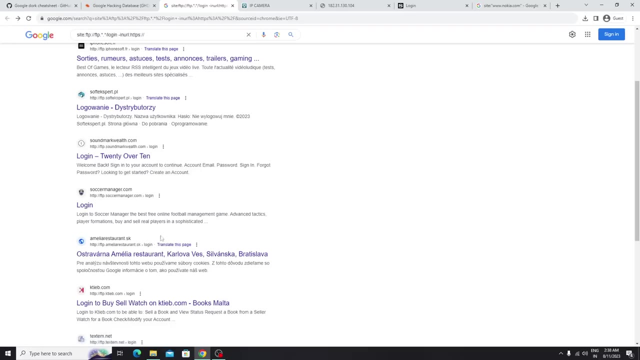 username and the password. ok, you can also login using the facebook, ok, and here you just need to enter the username and the password. ok, this is a thing. ok, you guys can able to find this portal. see, mostly this portals are vulnerable. let me tell you in real world, whenever i perform the 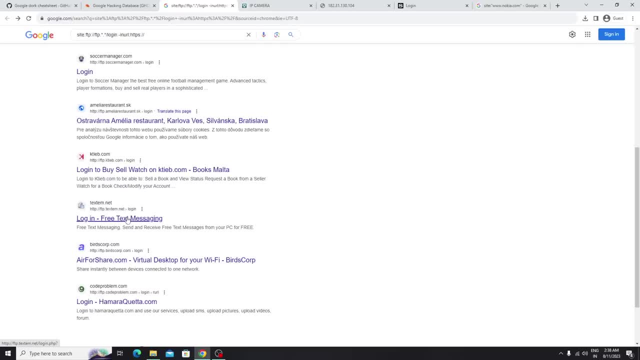 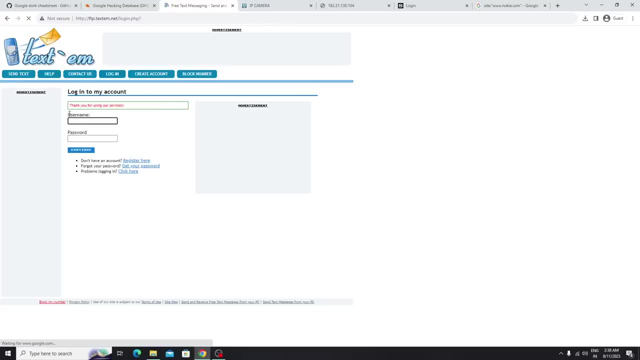 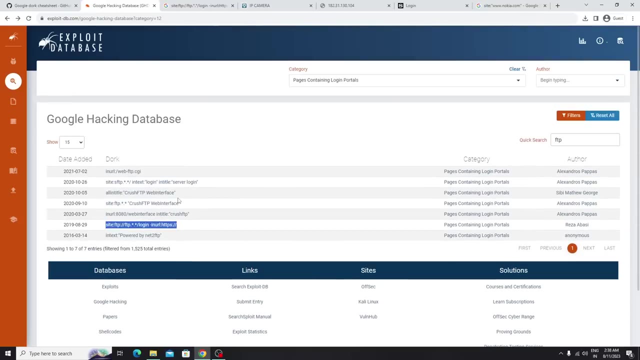 pentesting on this kind of ports. mostly there are vulnerable. ok, this is a thing. now, here i got another one. ok, let me go back and let me search for see. assume that you want to search on the particular site. ok, this is very important. assume that, if you want. 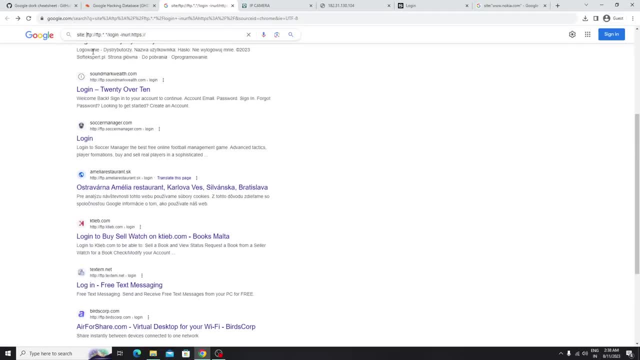 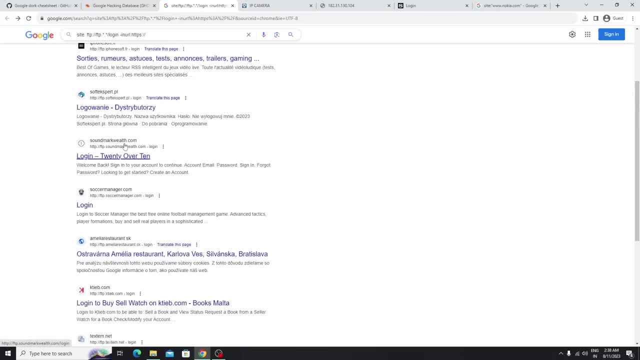 to search on the particular site. simple, just add the site name there, complete site url. ok, this is a thing. see, this is a sound make mark: health wealth dot com. is there? simple copy that complete domain with the http. ok, just paste there. ok, you guys can able to find the results about the particular. 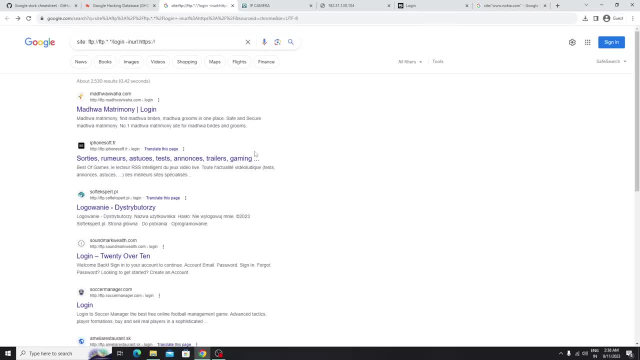 website. ok, mostly whenever you perform the pentesting on particular domain or or on website on ip. at that time you just need to mention the particular stuff there. at that time we will use the site- ok, this, this filter site- and just add the domain there. simple, it's not a big deal. ok here also. 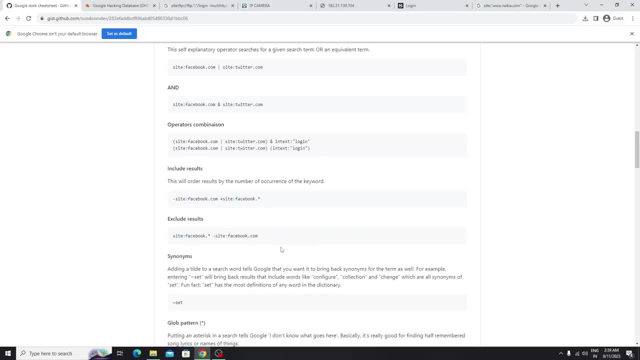 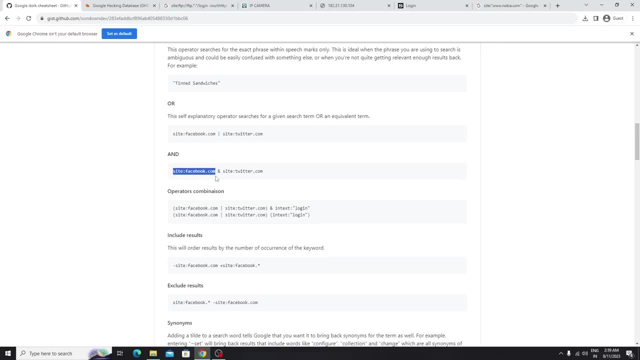 you guys can able to see the, this one, what the example. ok, just see site and just type the complete domain. or just type the with the, with http or something like that. ok, this is a thing and let see another stuffs. ok, if i type here, smtp. 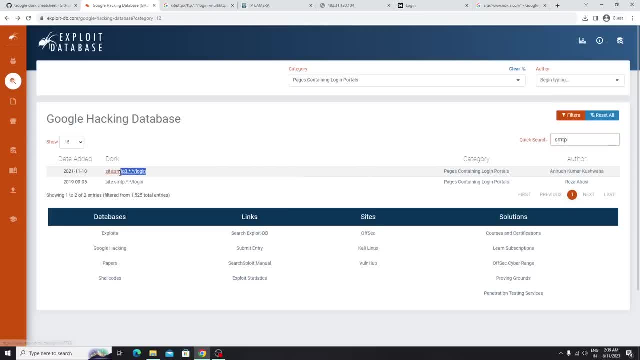 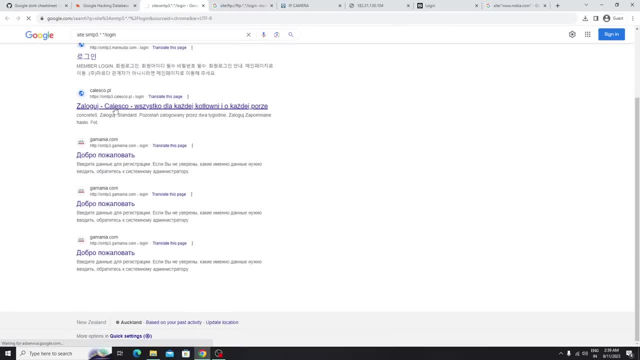 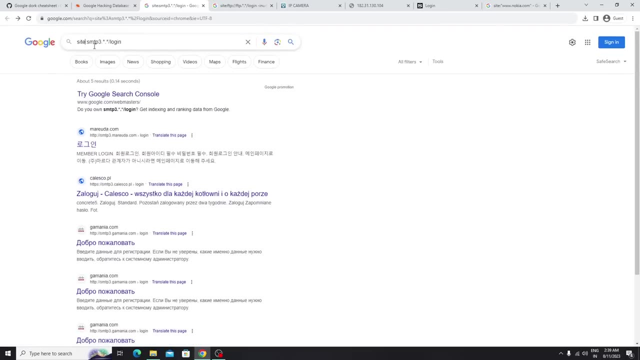 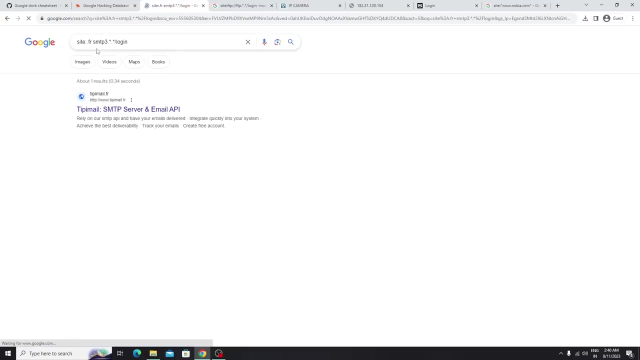 here i can able to see the related to smtp. see, i got something. now see how to use the particular. now i want to search only for france. ok, fr, just type here, dot fr and just type enter there. here you guys can able to see the only about the fr. 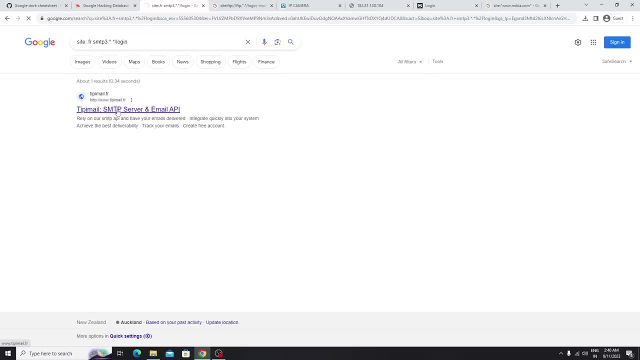 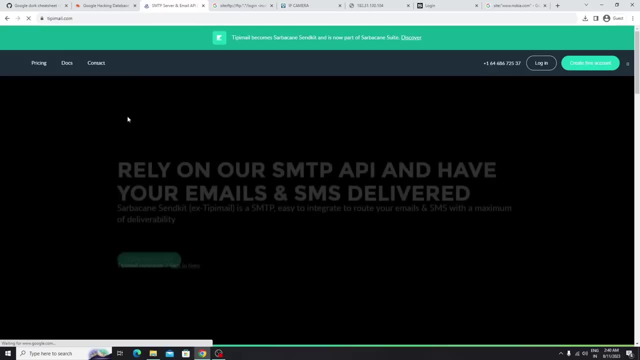 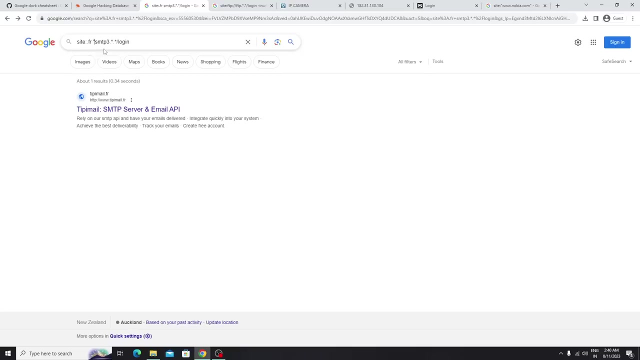 ok, just see the domain in last. it's a fr. if i open this one, you guys can able to see some smtp server there. i think no, no, no, no, it's not a, but it's related to kind of smtp. but if i add here, double quote and let 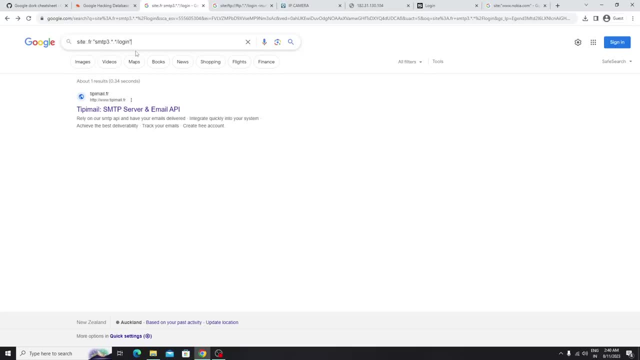 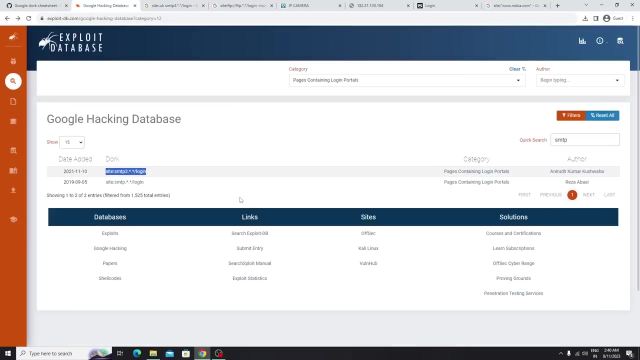 me close it with this double quote as well. last search: ok, i am seeing the same thing. right, if i type here something like uk, then i can able to see some kind of php mailer there. ok, if i open this one, i can able to see. ok, now let. 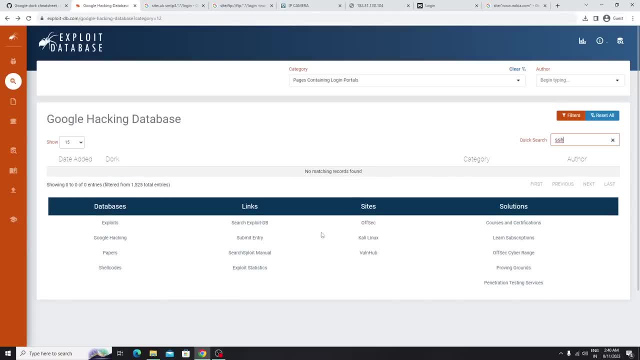 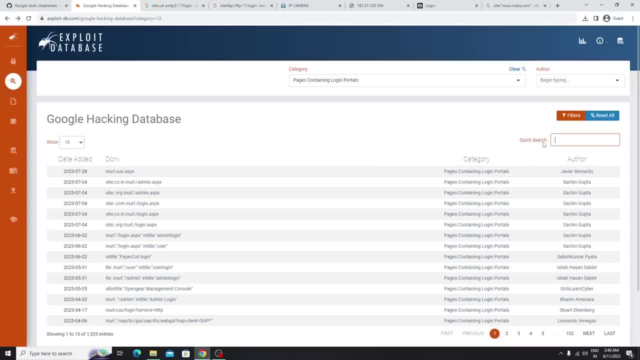 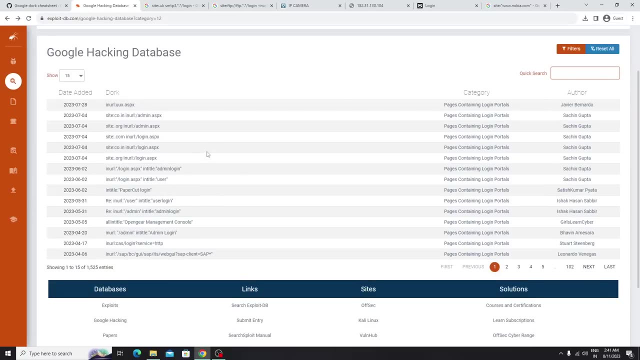 me search for the ssh. see, if you are not getting this one, what i am typing here, don't worry. ok, you will learn a lot time to time. ok, in the windows hacking series. ok, there you will learn about this all: ssh, smtp, each and everything. and here there is a. 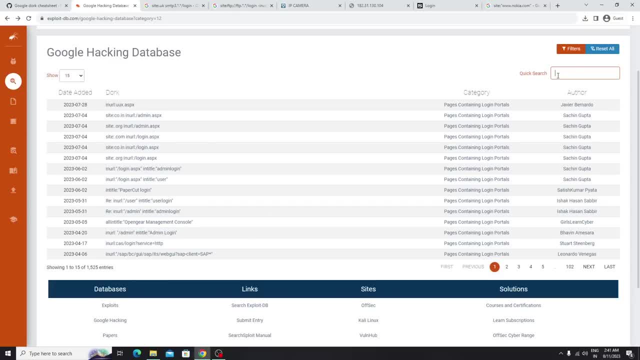 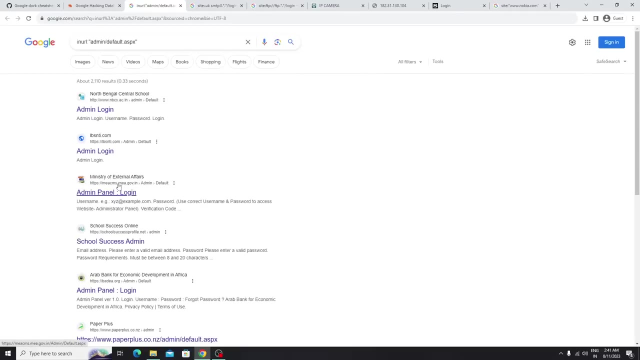 url entitled. let me search for the admin pages. ok, if i type here admin. ok, here you guys can able to see about the admin pages in url: admin, default aspx, something as well. let me copy this one and search it. here you guys can able to see each and everything. 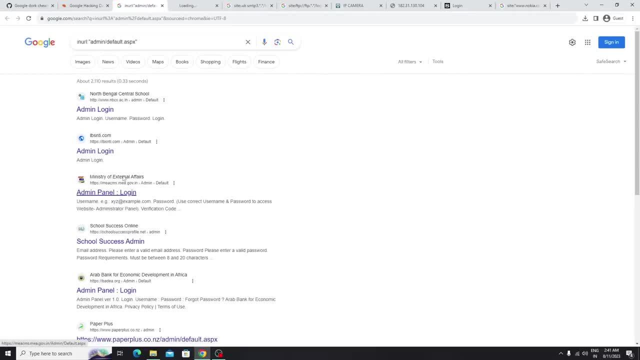 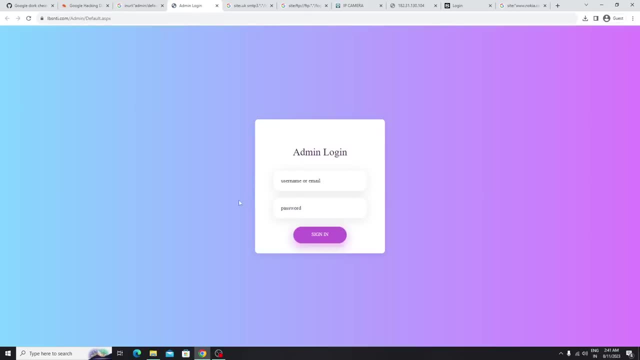 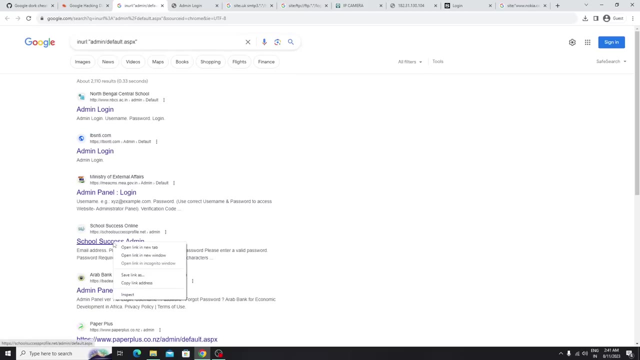 about the admin panels. if you open this one, see, it will ask for the username and the password. ok, see, we can able to bypass this one. ok, we will learn in sql injection section how we can able to bypass this things. ok, see, if i open this one, then what will? 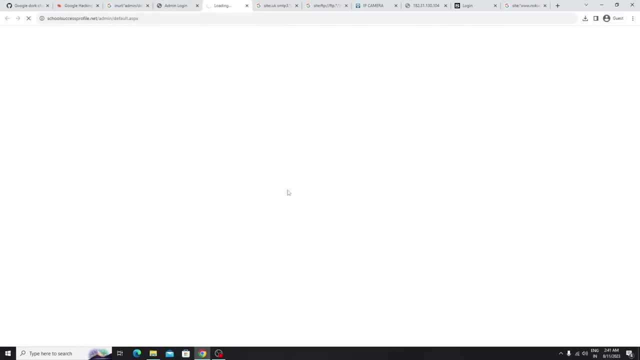 happen. it is also a one portal. ok, sso, simple at that time. here you guys can able to use some by default credentials as well. ok, here there is a lot of stuff: paper plus dot com. ok, there is a admin dot. login is here which is related to washington university. 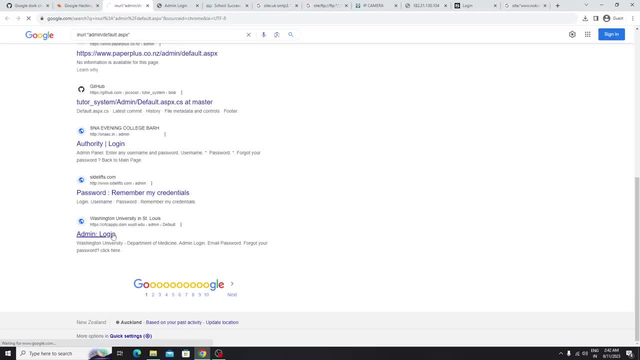 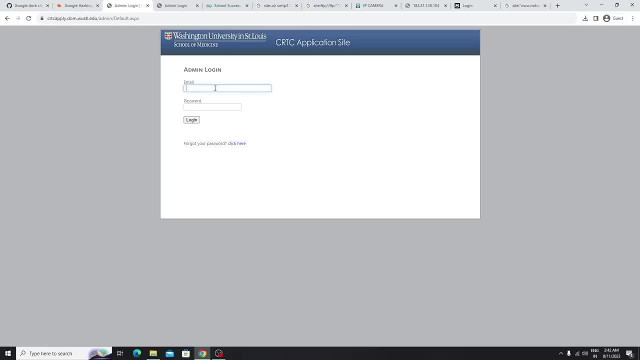 if i open this one, then what will happen here? you guys can able to see the username and the password. if you bypass this one, then you guys can able to get the admin access. ok, from there. you can able to change the results. ok, or you can able to. 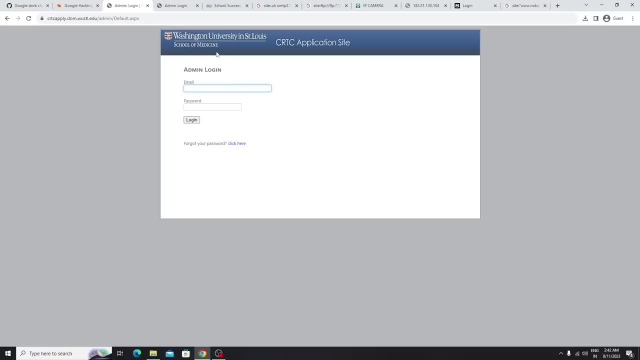 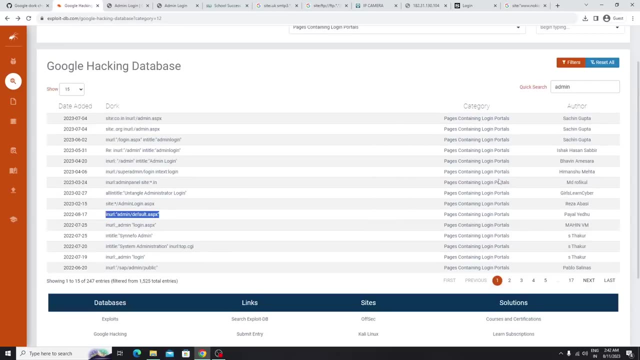 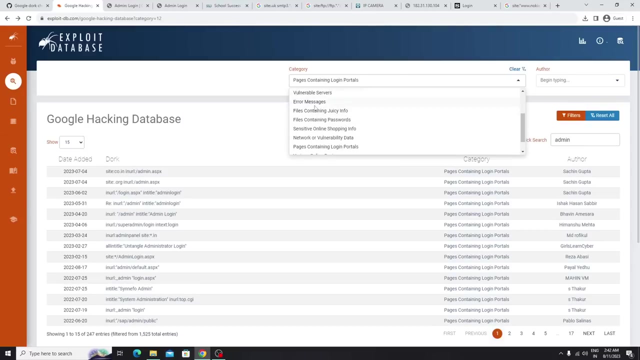 change the attendance or such kind of stuffs. ok, this is the thing. and there is a sap. its related to sap pages container login portal. ok, if i click on here, you can also check through the categories as well. its a vulnerable server. ok, let me check through the. 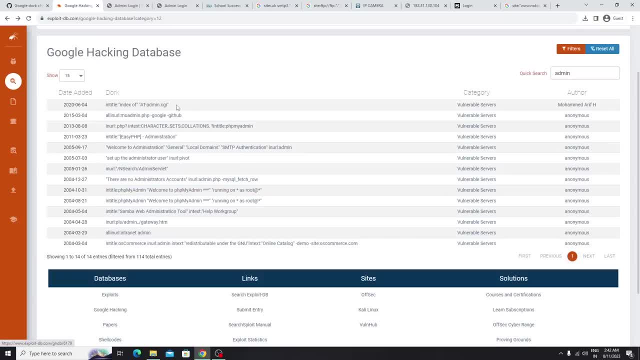 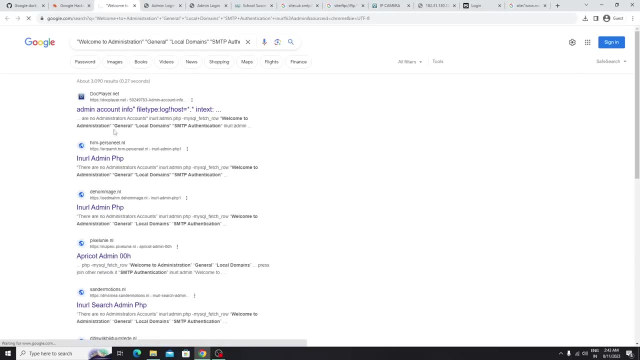 vulnerable server as well. now here there is a cga. you can able to bypass this, all stuffs. ok, its not a big deal. this cga? ok, and welcome to administrator. ok, let me search this. here i got something. here i got something, not this one man. 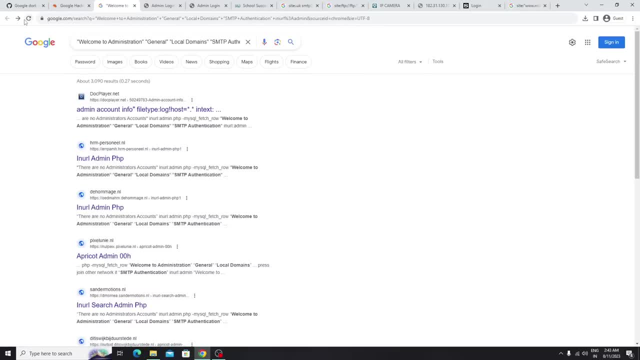 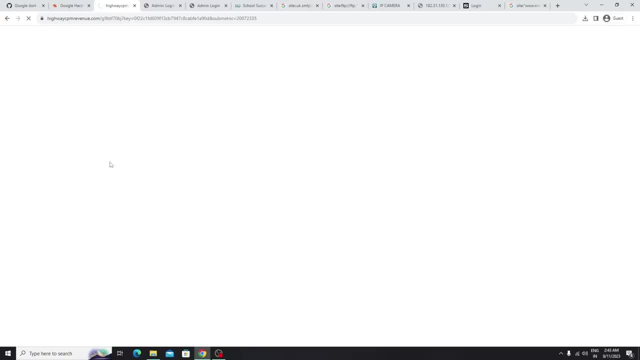 let me, let me open this one in url: admin. see what will happen now. maybe it will try to buy. ok, its redirecting to google dot com. basically, it will show you the admin page. ok, this is the thing. ok, its redirecting it. we can also stop this redirection. 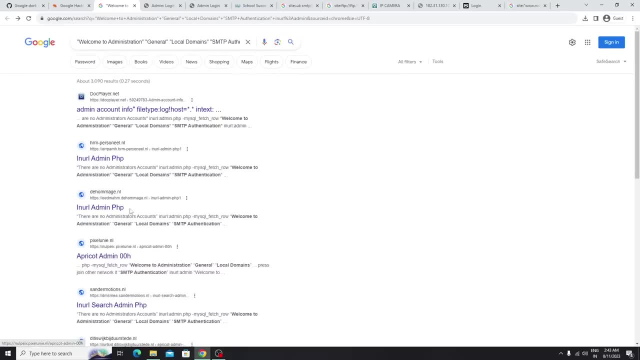 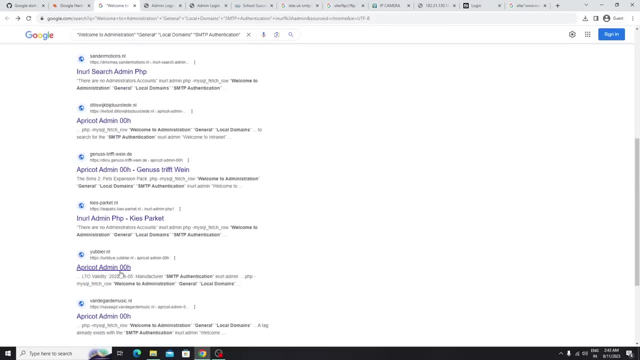 process as well. its not a big deal. basically, what its doing its a kind of security. ok. what its gonna do means it will redirect to google dot com. ok, we can able to access that admin portal. but there is some kind of function, is there? ok, if we can able to bypass it, its 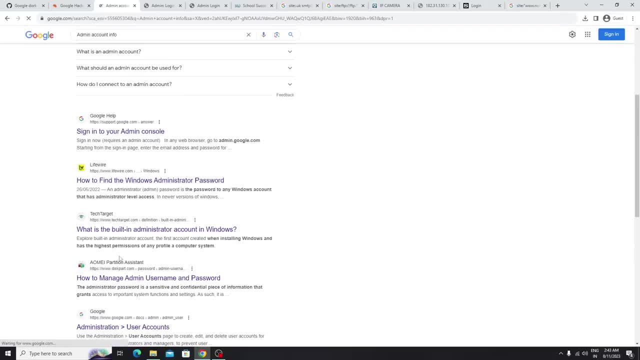 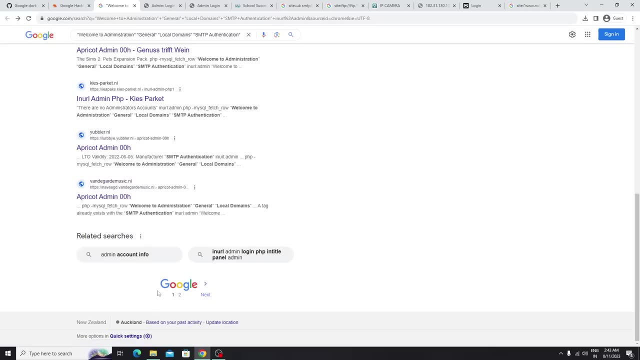 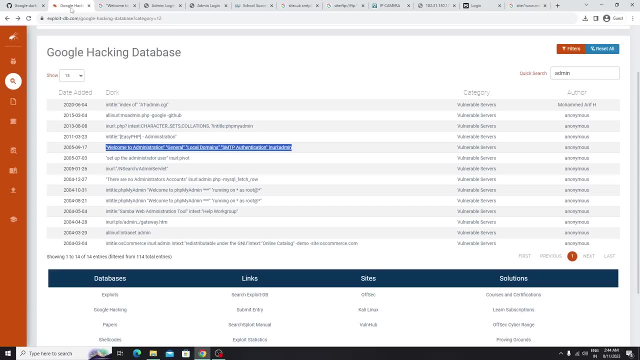 not a big deal. i can. now i can able to see some other legit websites, which is not necessary for us. ok, i just clicked here. ok, so this is the reason if i click on the second page. i didnt see any results. now let me search for any. 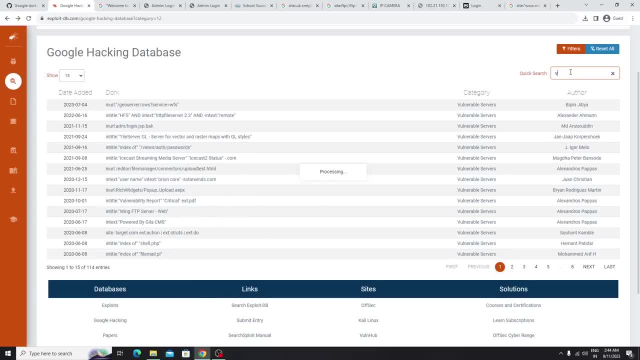 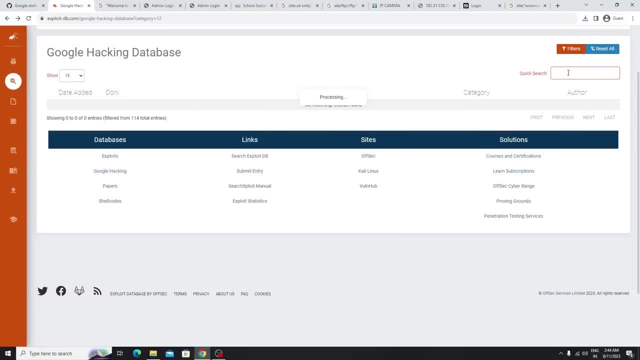 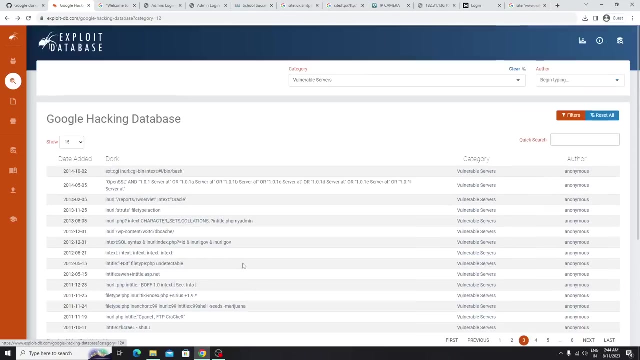 other servers ok, such as vncz- if any vncz, sorry- rdp, microsoft, microsoft- if there is any kind of microsoft stuff- are running. sorry, i think it will show some results. ok, ok, sorry, sorry, sorry, i need to do the stuff manually, ok, so this is the thing guys just try to. 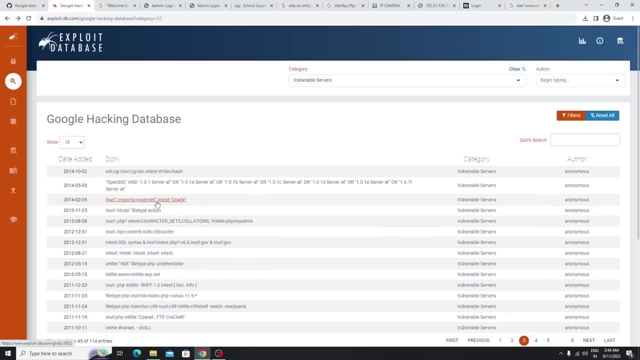 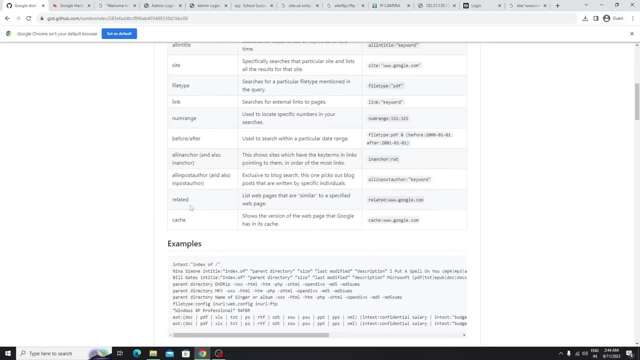 do one by one. ok, you will get it. ok, its not a big deal now here, lets go back and let me see this. all stuff. ok, again now see what its using: file type. if i go back here, its using any kind of file type. ok, here there is a file type. 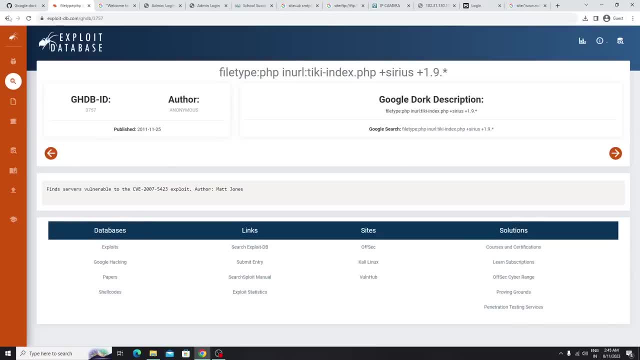 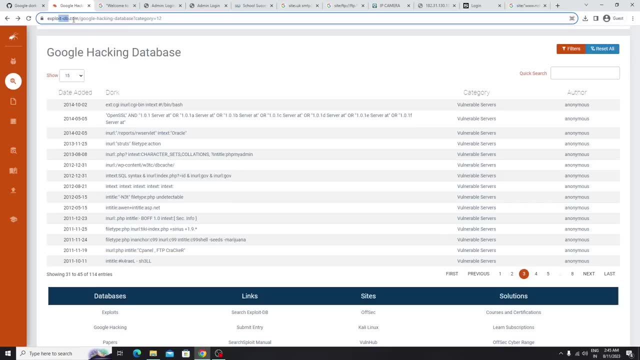 php in url is there? ok, just see there is a in url. its nothing but in url. in a simple words, its saying that in url, in this url, just find this kind of information which is related to boff 1.0. until that, this is one filter and from here, 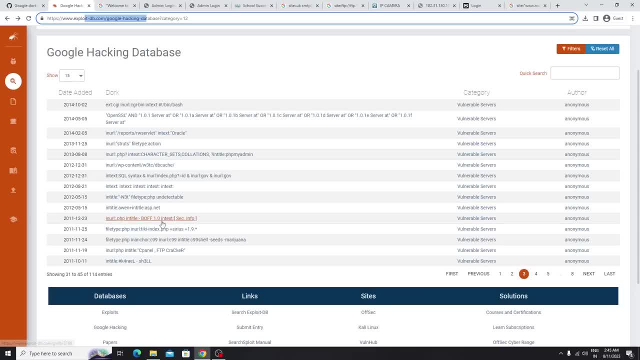 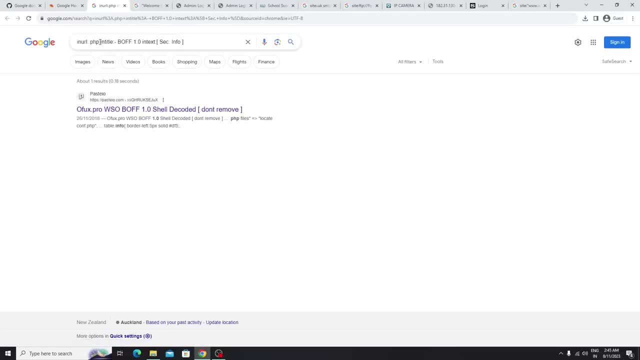 there is another filter. is starting from where in text? just let me copy it and let me explain you. ok, see, basically this is there are three filters. right now its using three filters. one is this one: ok, in url is one filter. and also its using in title: this is one filter from. 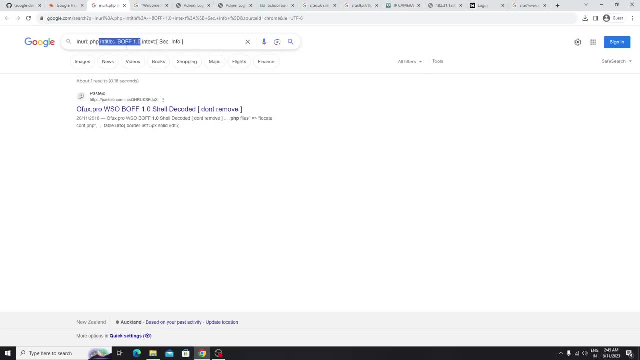 here to here. this is a one filter. ok, basically, its a keyword. ok, its a keywords. its searching for the three results. ok, basically, its searching for one and this, this is a second one and this is a third one. ok, this is a thing, basically, here you guys can able to add anything. 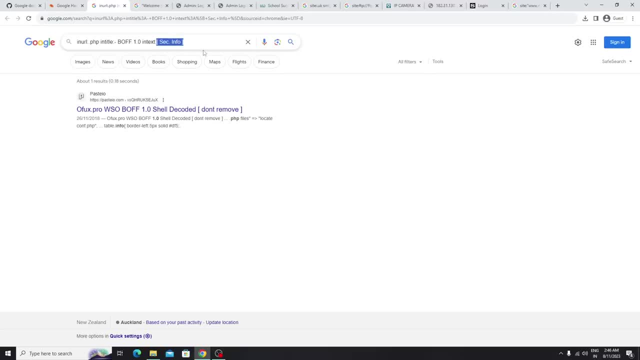 ok, any keyword, its totally depend upon. you most probably assume that there is a boff. ok, let me type here something like microsoft or something like that. maybe i wont get the results, but still let me type it. i can able to see some results here related to microsoft. 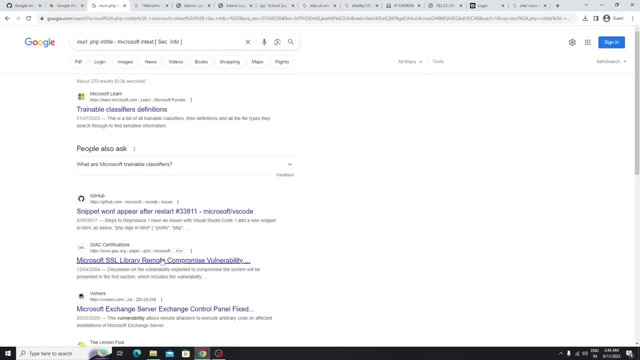 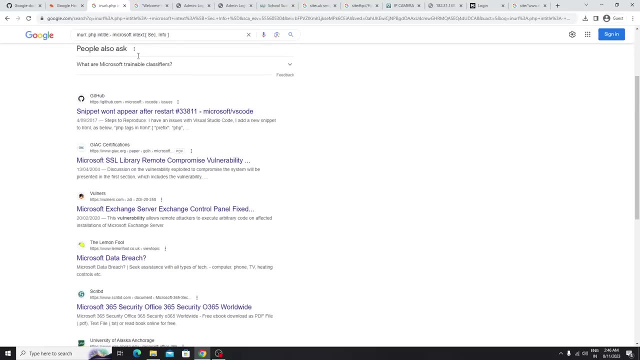 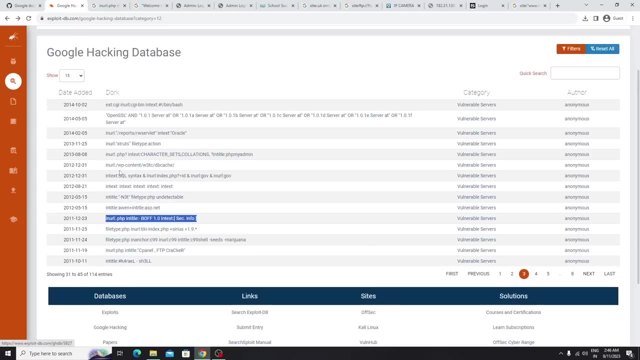 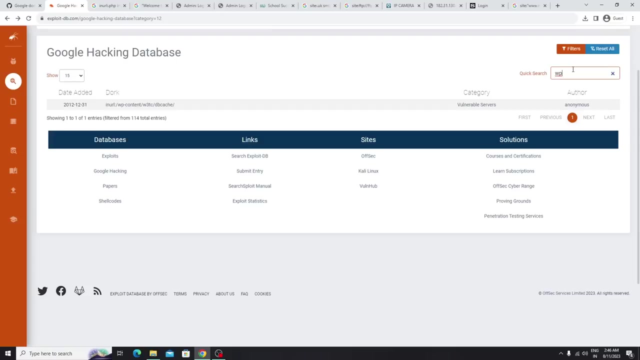 and i want to see the. its showing me the pdf. ok, its not a good results. ok, basically, you can search for anything. ok, this is a thing and see, here is a. you can also see for the wp wordpress as well. ok, maybe there is a for wordpress. 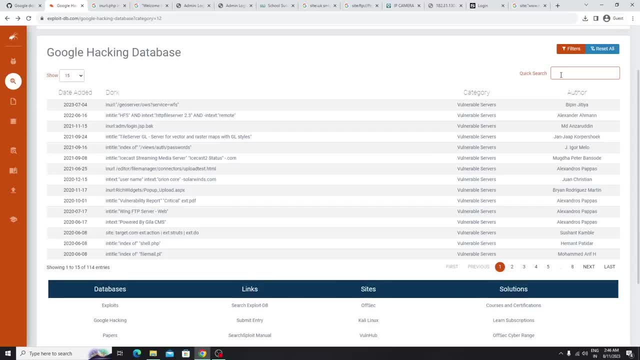 i think there is a docs for wordpress as well. i think they did. ok, ok, ok, i know you just need to search through the themes. ok, this is the thing. like in wordpress: there are themes, are there? right simple? you guys can able to search the docs by. 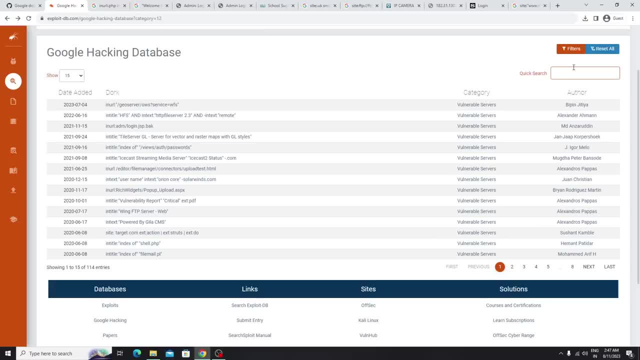 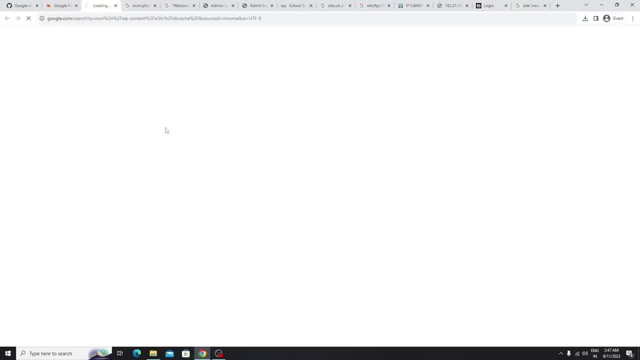 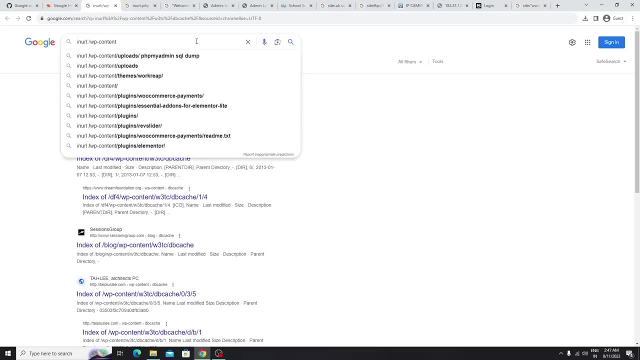 pasting the theme name as well. ok, now, here you guys can able to see wp. if i search for this one now, its only find the subs. ok, now assume that let me remove this one. ok, simple, let me add wp content. see each and every website which i am. 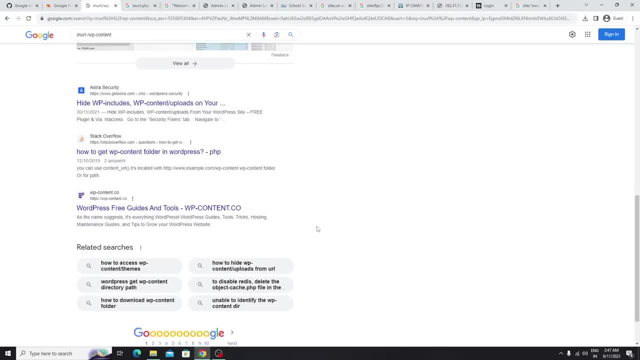 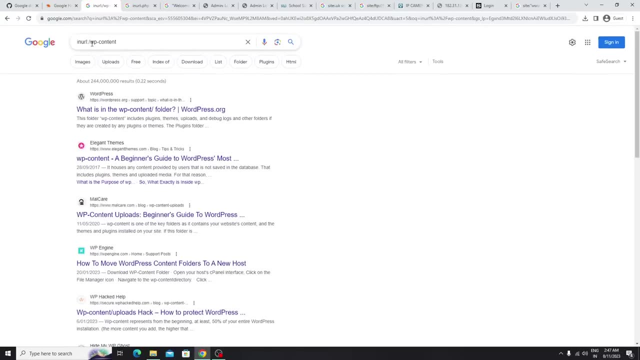 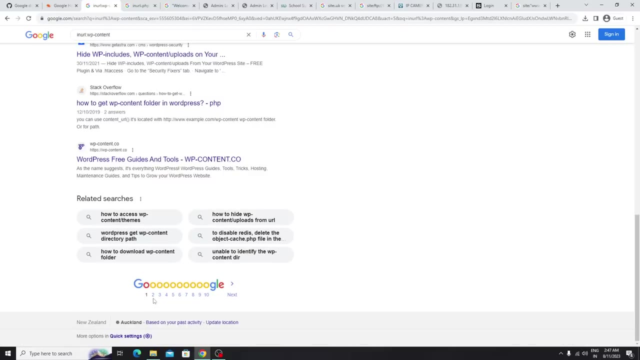 seeing right now, its a wordpress website. ok, this is the thing, i think. ok, no, no, no, no. just let me remove this one which are related to wordpress: see wp, where you guys can able to see the wp content. wp content is a folder in wordpress. ok, this is the thing. 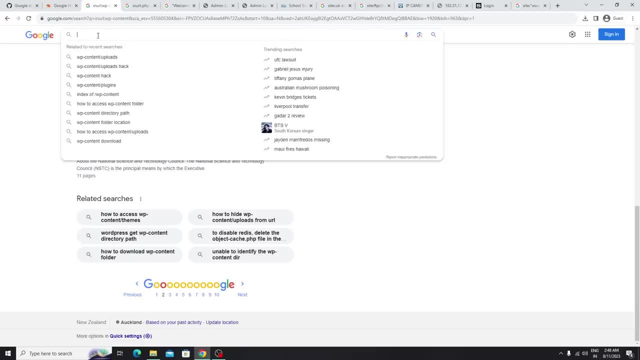 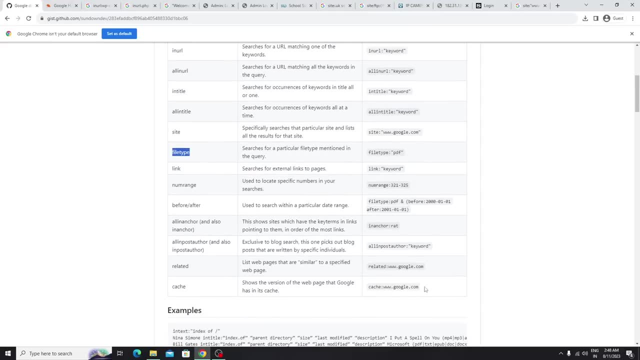 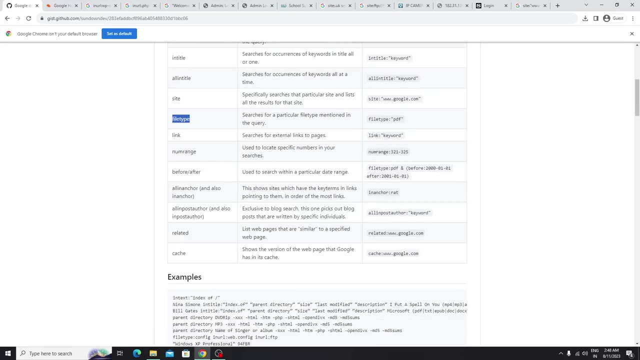 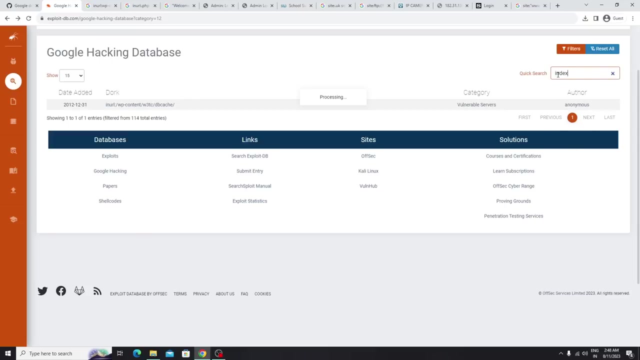 now there is a another thing, ok, which is very excellent. hope i can able to see here there is a file, the name of file. ah, yes, they didn't mention here. just wait, ok, let me type here: index ok. index of ok. here i got the index of. 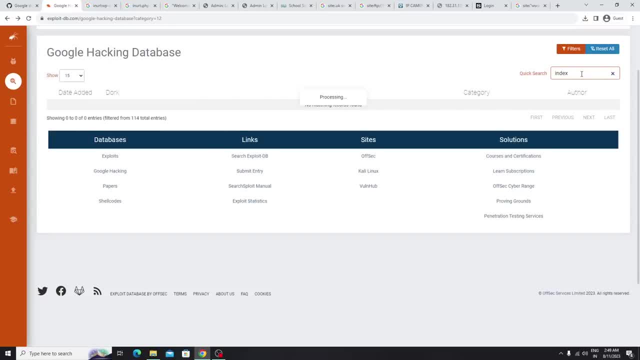 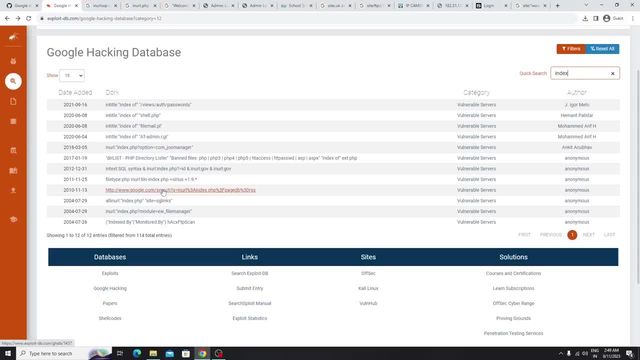 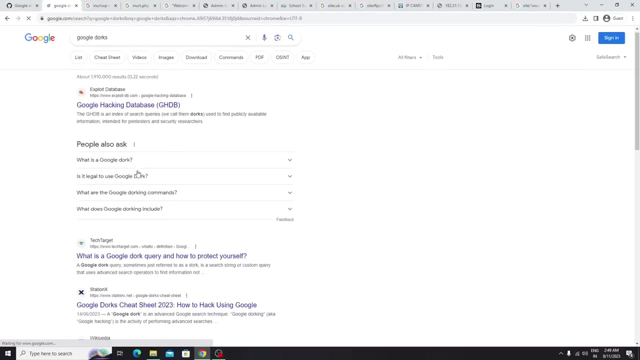 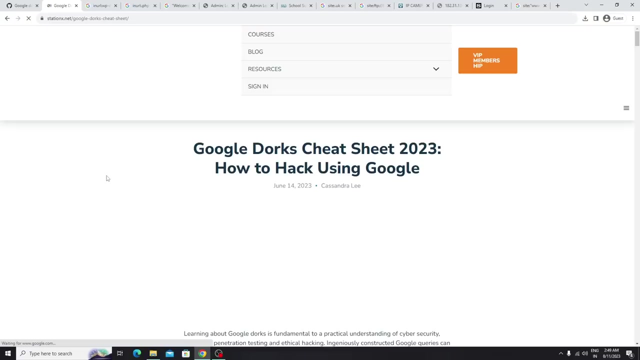 simple. let me remove it. here i can able to see the index. ok, what is this index? let me tell you. instead of this one, let me there are some docs, are there? let me search manually here. here you guys can able to see there are, you can see the. 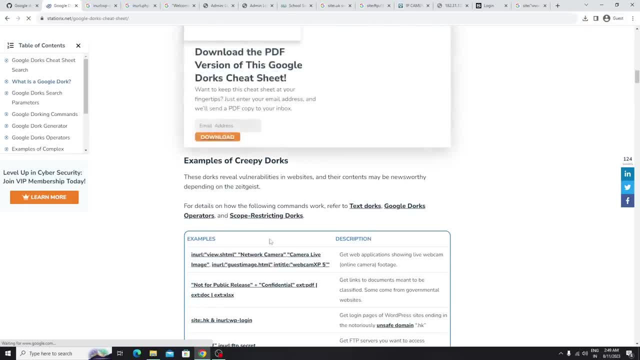 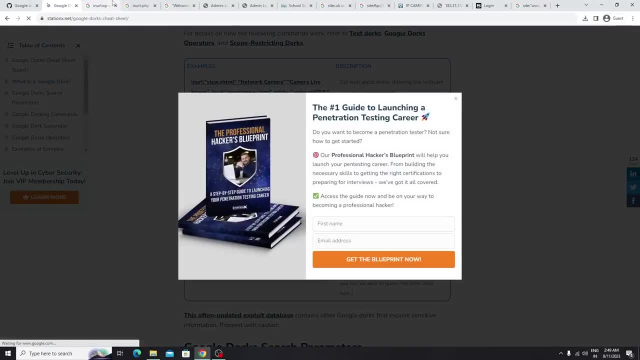 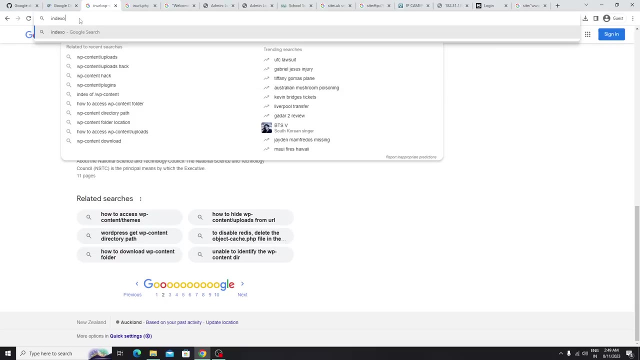 docs of this one, 2013: see here i can able to see index of: is there ok? basically, from here, let me show you practically: ok, i don't want to go with theory, just type here: index of. ok, just add the colon here. and simple, just type. 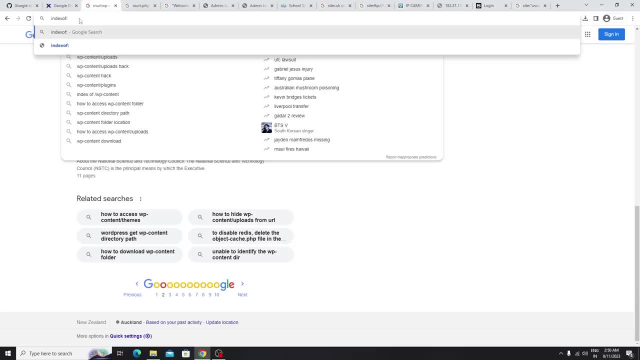 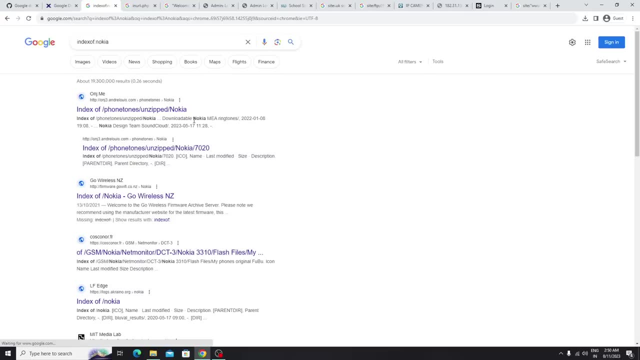 any website. ok, just type any website or any domain. ok, simple, let me type here: nokia. just type: enter here. i can able to see the folders. ok, which are in that nokia. ok, simple. assume that if somebody is selling the courses or if somebody is trying to selling the software, 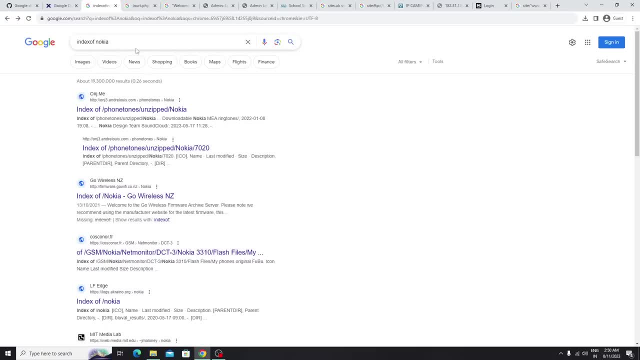 ok, there are in website you guys can able to see. they sell the software, the courses or something like that. at that time, what will happen means, due to this doc, we can able to see the content in that website. ok, we can able to download it as well. ok, this is the thing. 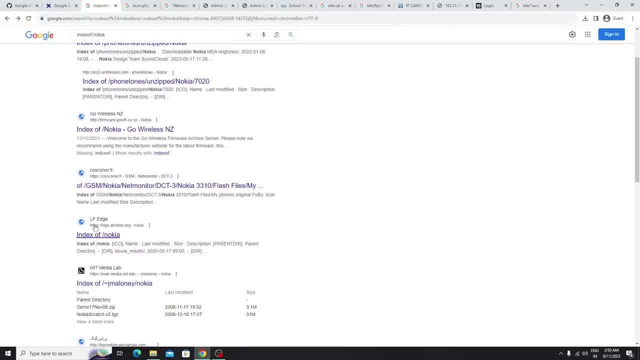 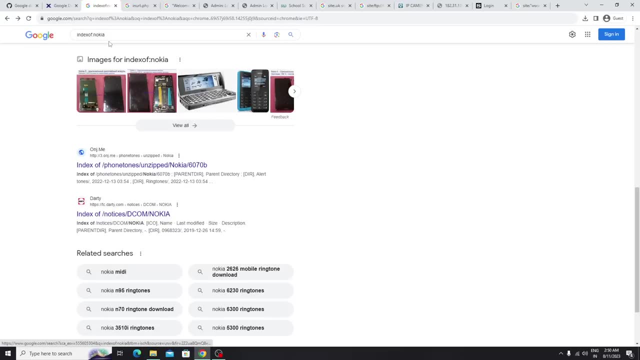 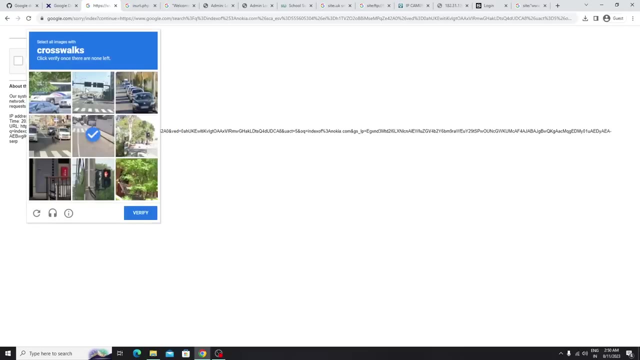 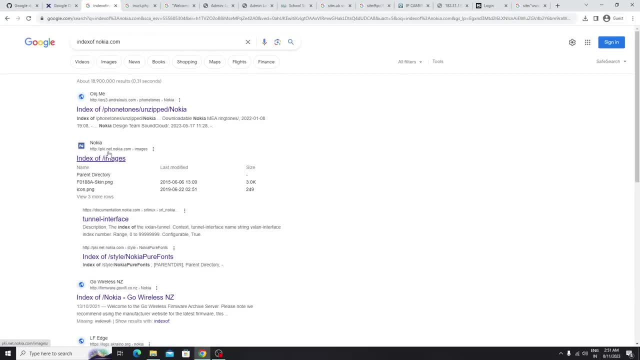 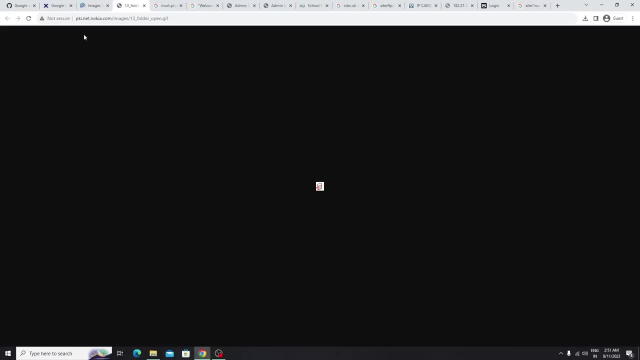 ok, now see it. say nokia- pkinetnokiacom. pkinetnokiacom is there. if i open this one here, you guys can able to see the images. ok, you can also open this one as well. its not a huge data and here there is a. 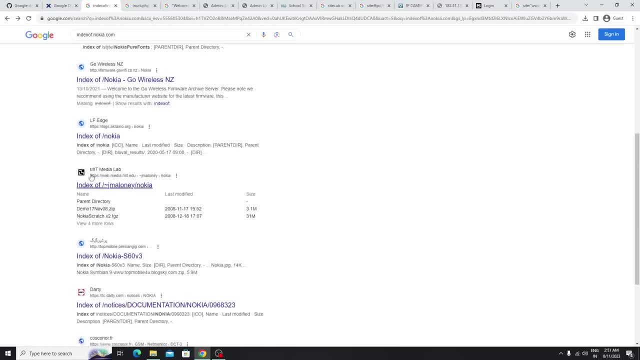 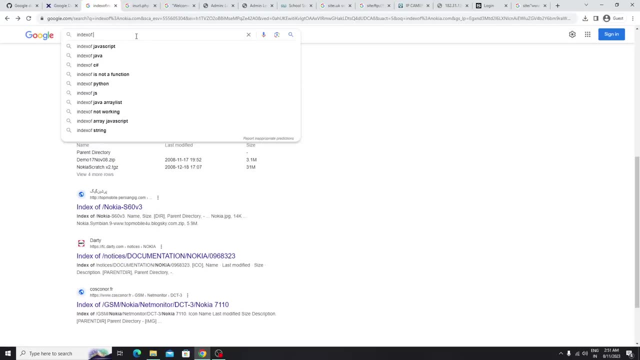 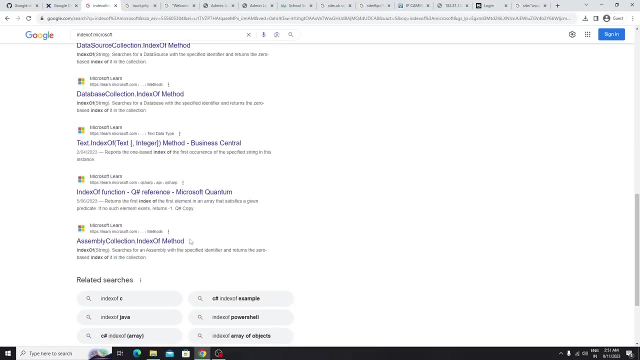 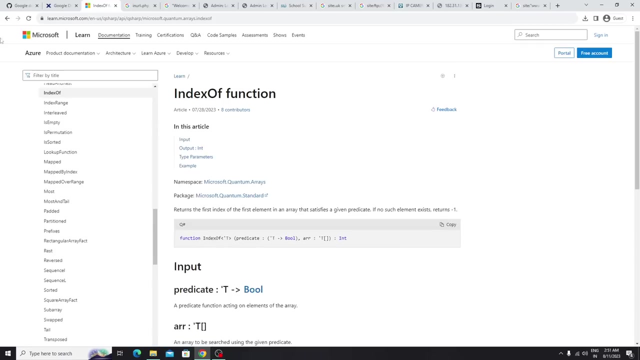 nokiacom. no, its so odd if i type here something like any other, any other website, such as um, um, um, um, so, and here you guys, you wont see that much results on this kind of sites. ok, ok, but whenever you perform the bug bounty or any kind of 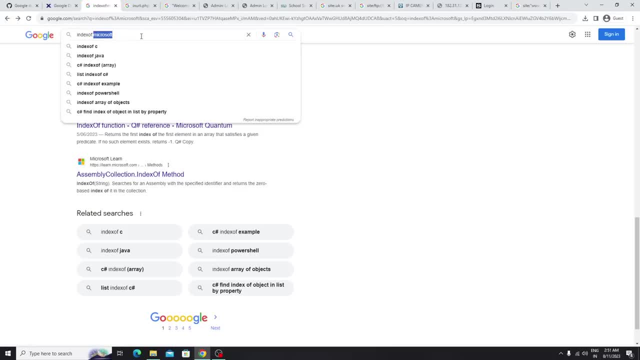 shoves. you need to check this, all things. ok, this is a thing. now, if i type here some kind of ethical hacking or index of, i dont want to type this type of command shoves. ok, let me type some kind of images. or let me type here images. 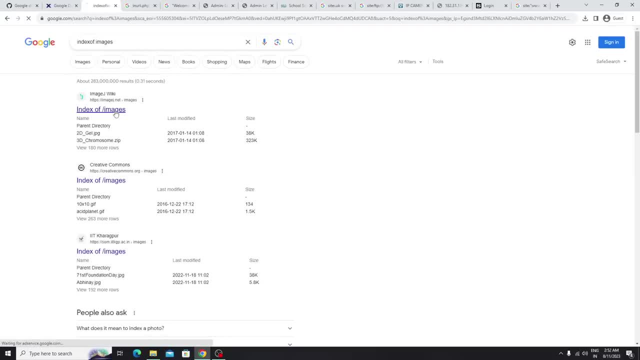 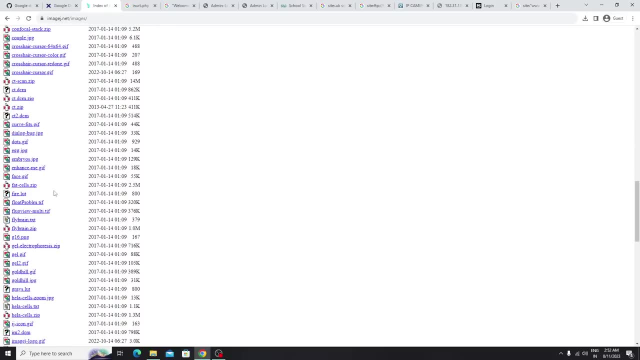 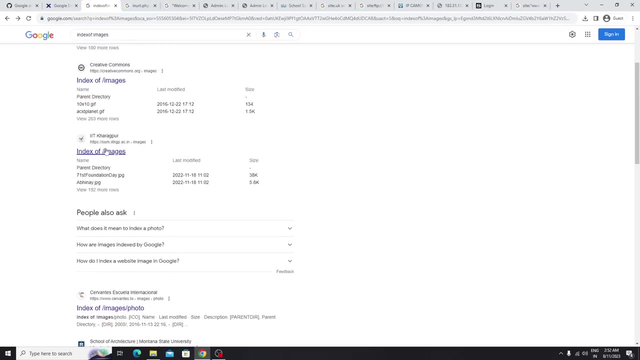 now, here you guys can able to see the images. ok, zip files, right gif, each and everything. you guys can able to target a specific website as well. again, i am saying its not a big deal, but i dont want to show you that one. now, here i can able to see. 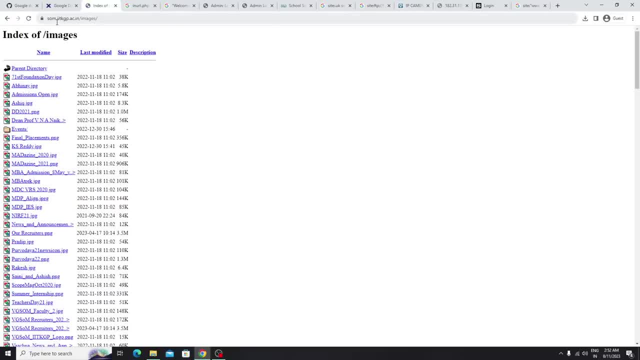 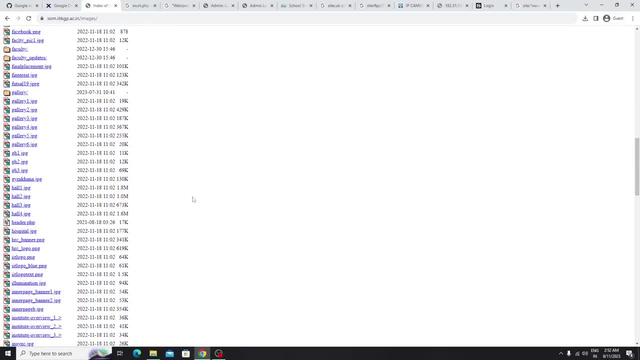 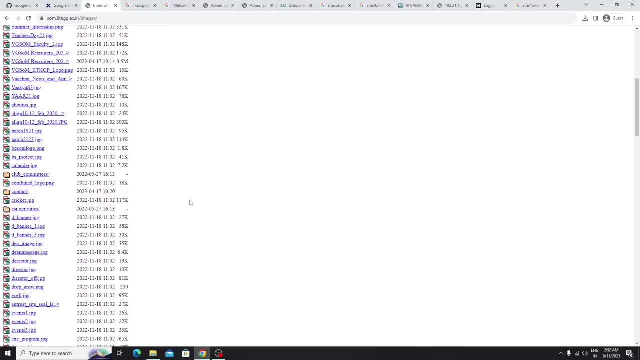 iit some kind of uh kgpacin- ok, its not a vulnerability. basically they add this one for seo purpose- ok, some such kind of shoves. but sometimes what will happen is, uh, mostly they add the courses here- ok, courses or any kind of private document. 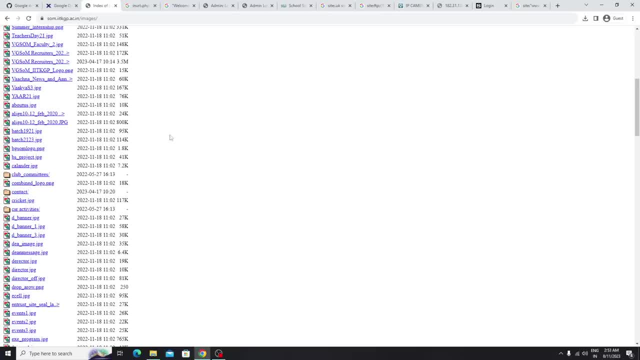 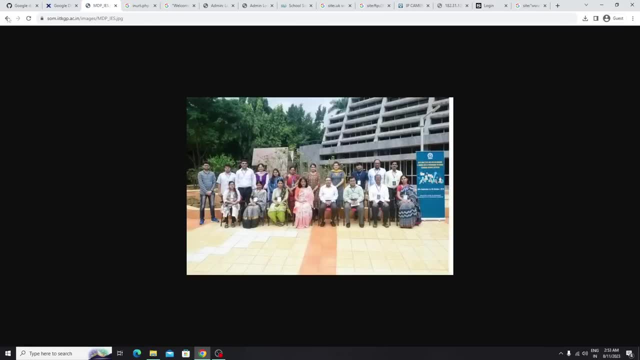 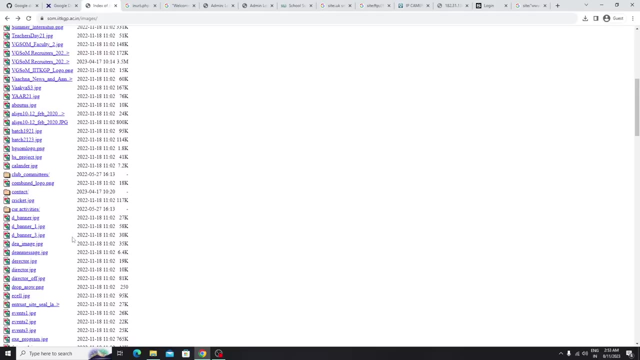 which they store in that website. ok, it can also reveal that one as well. ok, anyone can able to download it. ok, this is a thing. assume that there is a zip file. ok, zip file. maybe i can able to see the zip file. you can, if there is any kind of 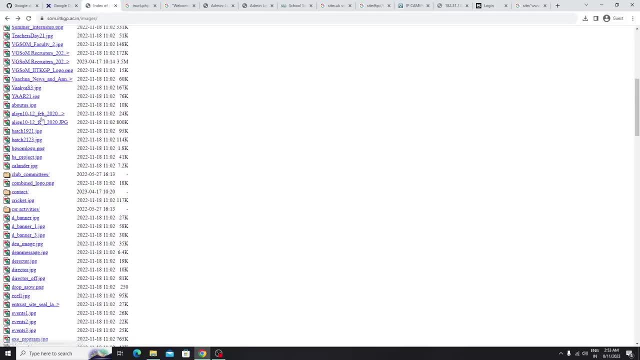 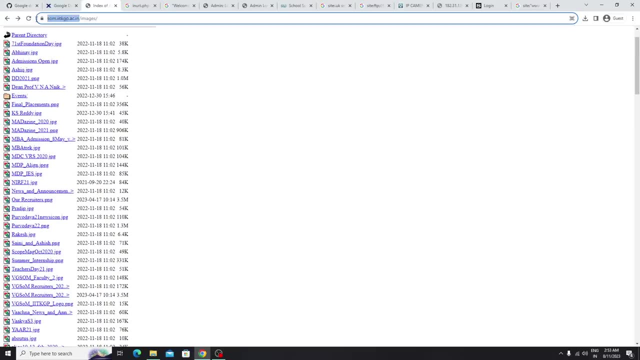 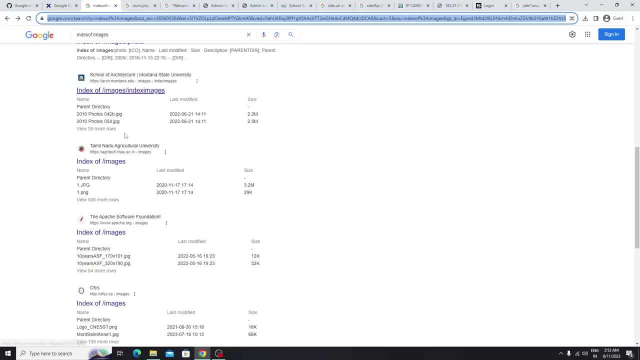 zip file, you can also download it. if is there any kind of mp4, then you can also download it. basically, these are the content which is in this website. ok, i can able to see each and every content here, so this is a thing, ok, uh, here is a. 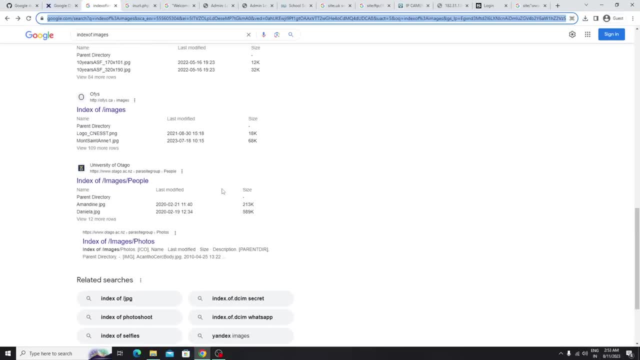 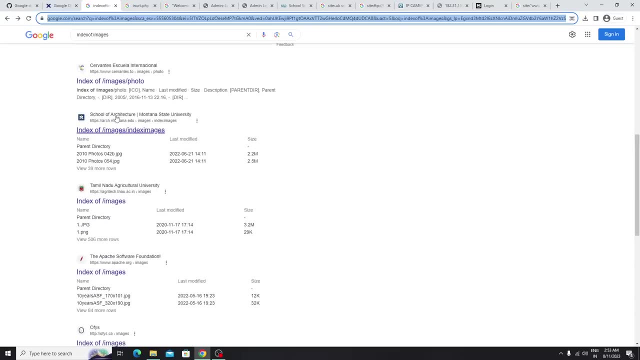 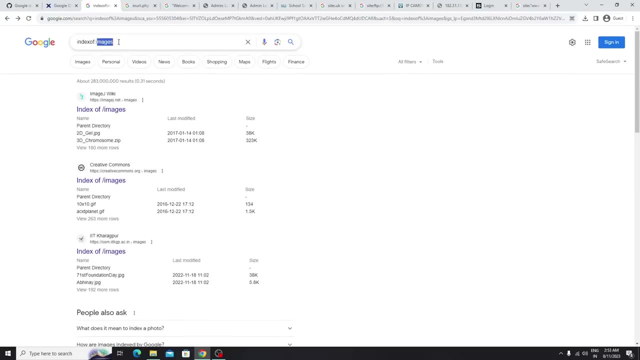 thing: mostly this kind of sites are vulnerable. ok, but with different vulnerability. but i just saw in real world this kind of sites which reveals uh, this, uh, this kind of shoves, uh directories. this kind of websites are vulnerable. ok, mostly this kind of sites are vulnerable. ok, this is a thing. 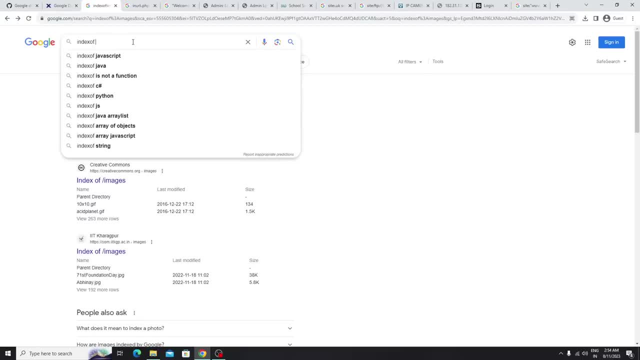 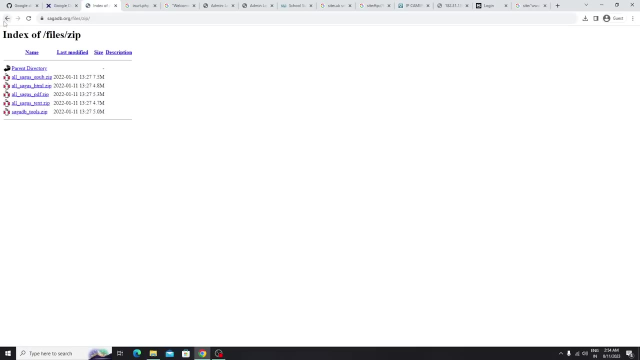 and let me type here index of any other stuffs. ok, if i type here index of zip or here i can able to see the zip files. ok, this is a thing IIT college of agriculture- here i can able to see. see in file there is a zip folder if you open in that. 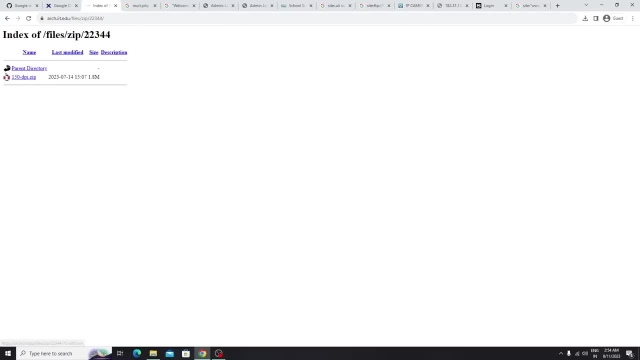 zip folder. there is a one file with the name: uh, what is it sorry? in zip folder there is a another folder with the name of 2234. in the 2234 i can able to see 150 dpi, dot, zip, some kind of stuff, if you click on the parent. 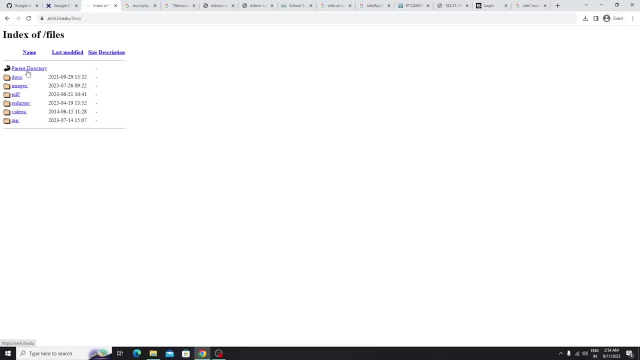 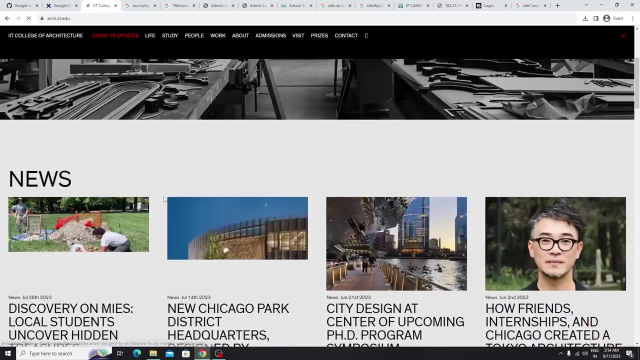 directory again. let me go, and here you guys can able to see the videos as well. we can able to see the videos if i click on the parent directory again. still, i am in. ok, here i am in the main website. ok, this is a thing. this is that website. 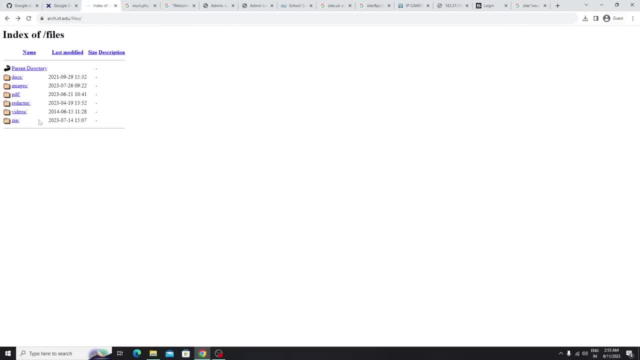 which is having, uh, having the vulnerability of directly listing. ok, this is a uh, basically it's a not vulnerability, but mostly, see, assume that you are uh using the blocks. ok, at that time you can able to add this kind of stuffs. ok, it's not a big deal, but assume that you are. 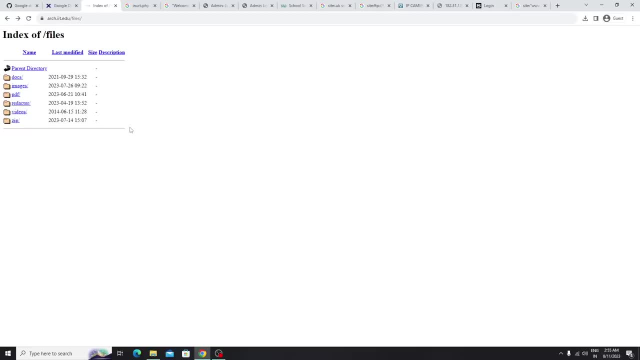 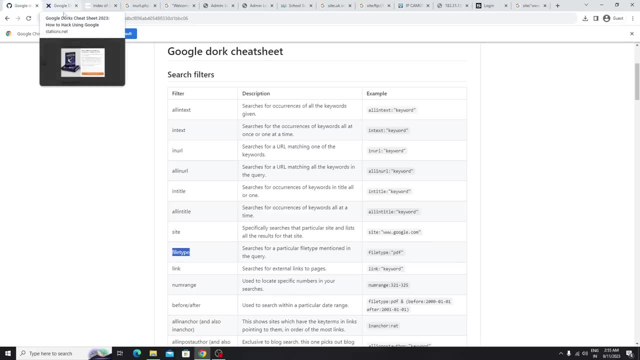 selling some kind of software or products or some kind of stuff at that time. this is very dangerous for you. ok, this is a thing- hope you guys get it- about the google docs: see it's, i can able to cover a lot about this one, but i just cover the things which are necessary. 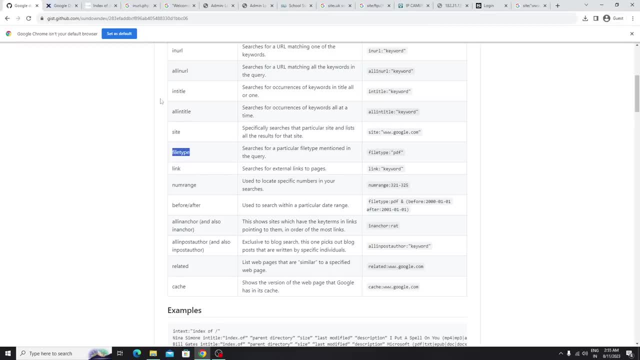 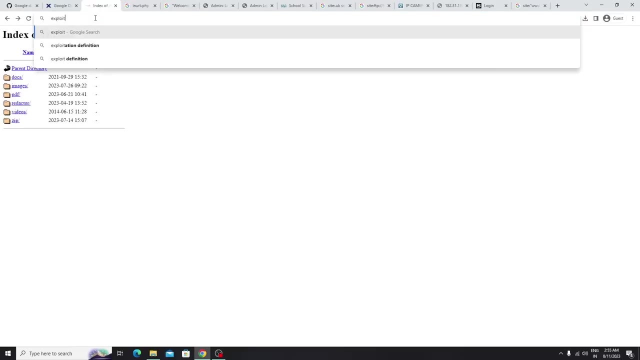 for you. ok, it's, it's not a complicated thing. ok, it's a very easy. assume that you are not getting this one. ok, assume that you are not getting it. ok, simple. what you need to do? simple: just open the exploit db. just type google hacking here. 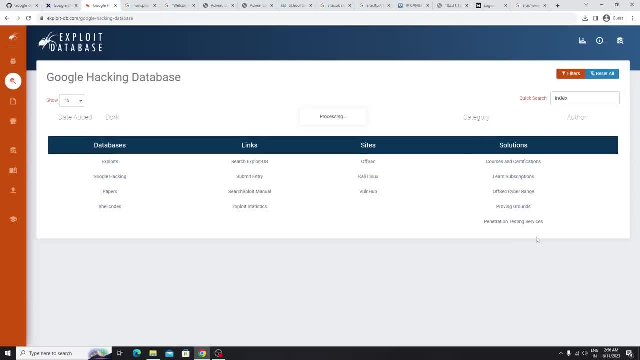 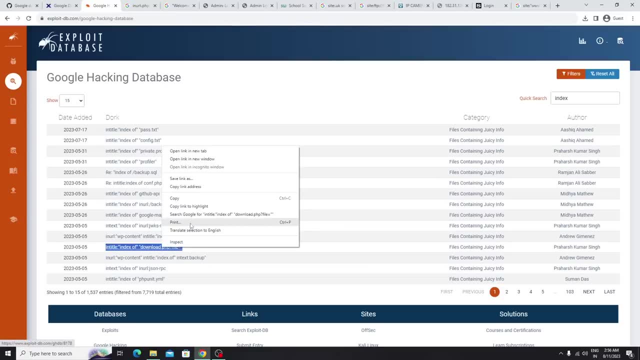 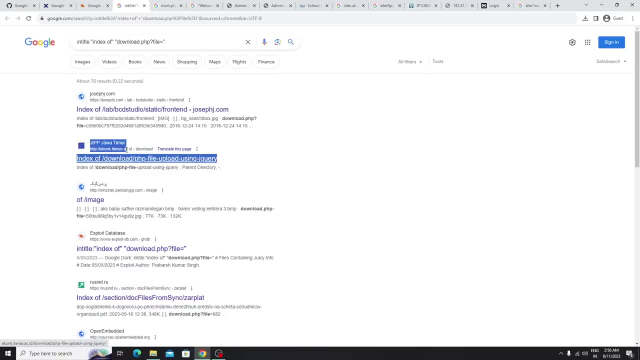 you can able to search here. ok, it's not a big deal, again i am saying alright. and here you guys can able to see index of download dot php. here i can able to see see, basically it's running in the local host. just see the xampp logo. 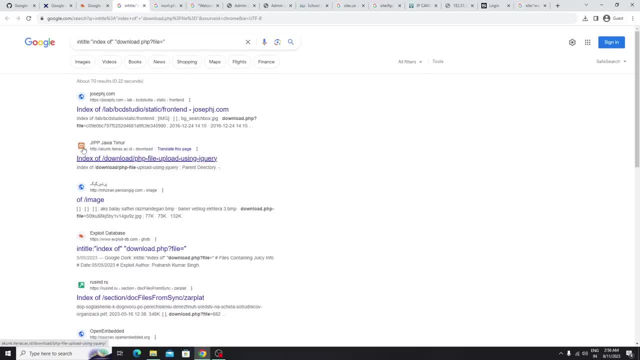 here. it's running on the local host. maybe it's vulnerable. ok. i can able to say that if you perform the website pen testing on this domain, there are maybe 70% chances are there it might be vulnerable. ok, because first thing is it's running on the local. 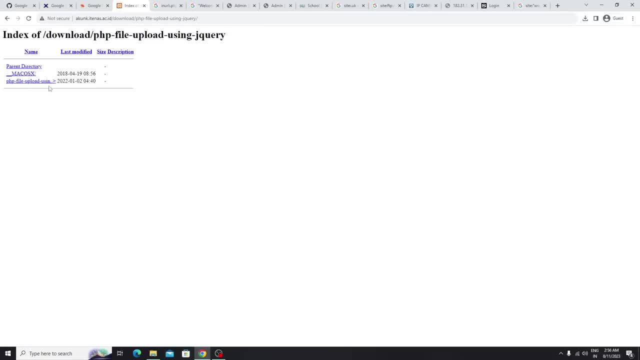 server ok and also it's having this kind of vulnerability. if i click on the parent directory here you guys can able to see the downloads ok, and if you see the upload folder is here in upload folder, you guys can able to upload the files. here you can also upload the shell. 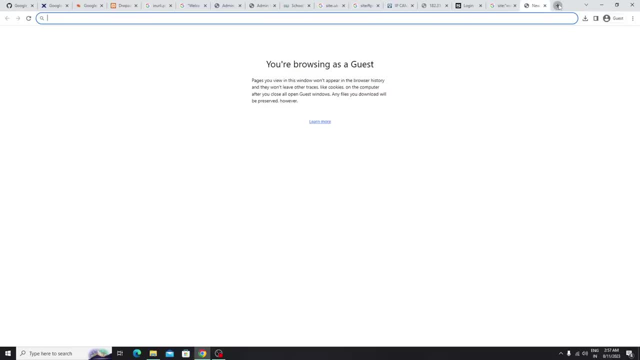 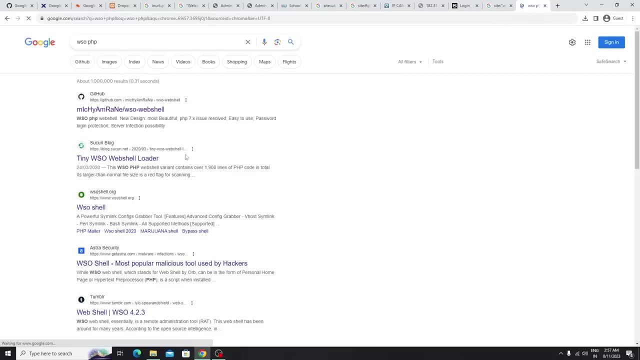 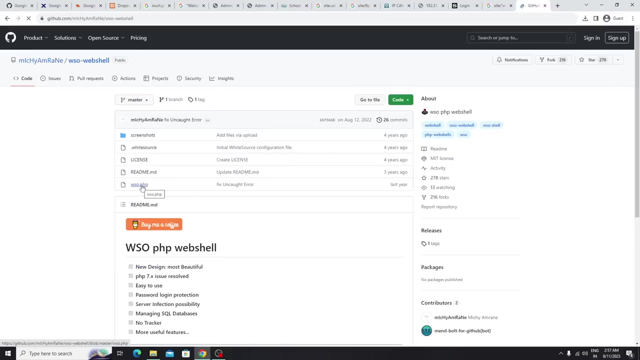 you know that. let me show you how to upload the shell as well. if you type here wsophp, mostly it's comes under webpd. but let me cover here as well. mostly people know ethical hacking, ok, so that's why i am covering this thing as well. assume that. 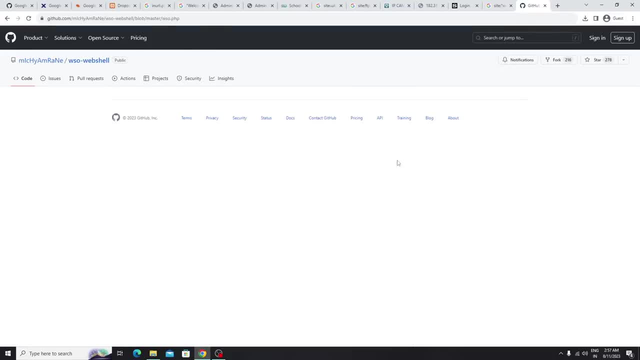 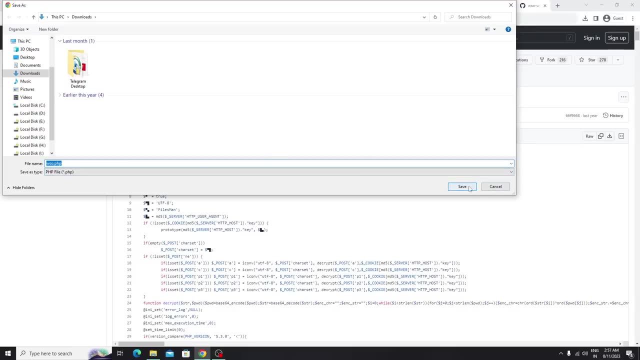 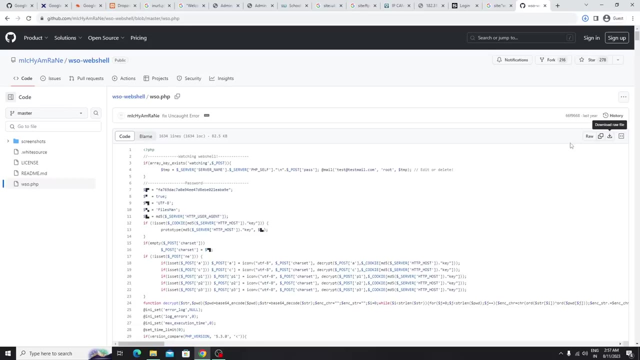 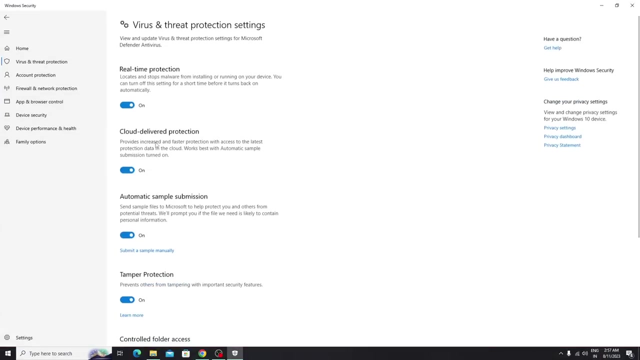 you are not getting it, just leave this video. ok, you no need to worry. simple, if i download this one, ok, it detect this one as well as a virus. i know, just wait, it will detect as a virus. just let me disable this windows defender here. right, hope you guys can able to. 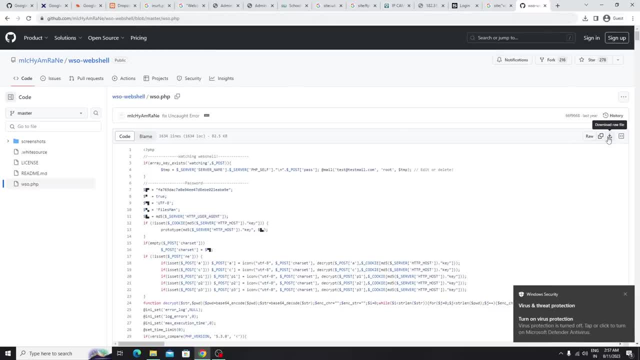 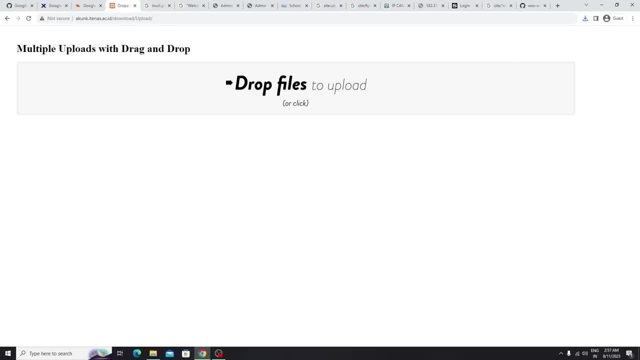 see the screen. now let me download again, save, and here let me drag and drop this one. ok, successfully uploaded. we can, if there is any kind of filter we can able to bypass, it's not a big deal. ok, we can able to bypass this one. basically it's a. 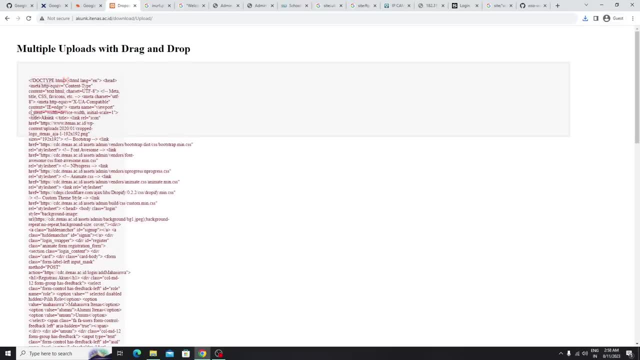 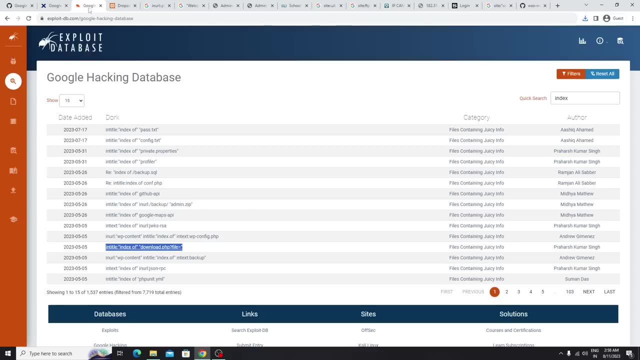 kind of vulnerable. ok, by using some methods, we can able to bypass this one. basically, it's a kind of filter or security. you can also say it as a security as well. ok, this is a thing, guys, let me see more about. let me see we will find this kind of websites. 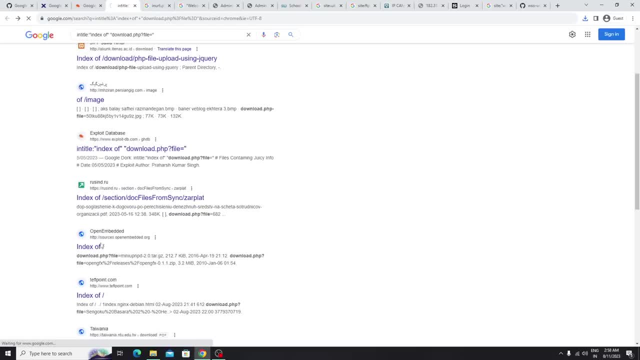 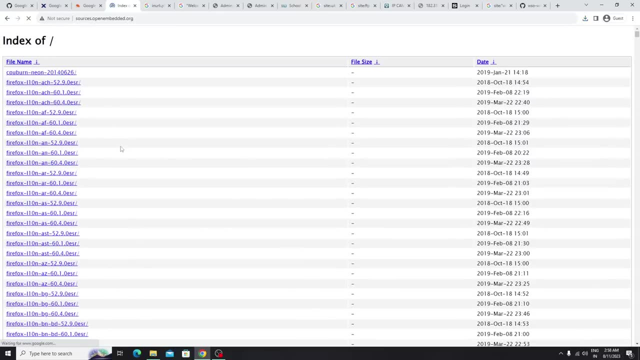 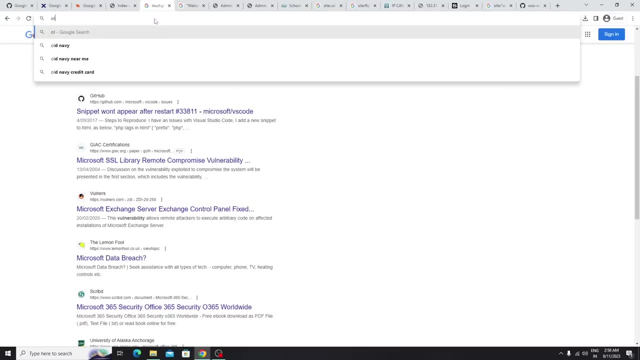 ok, now here i can able to see a lot of shows. ok, now see why i am saying this is not a kind of vulnerability, because if i type here kali kaliorg, ok, just type here old kali, see, you can also see the same thing on the on this website as well. 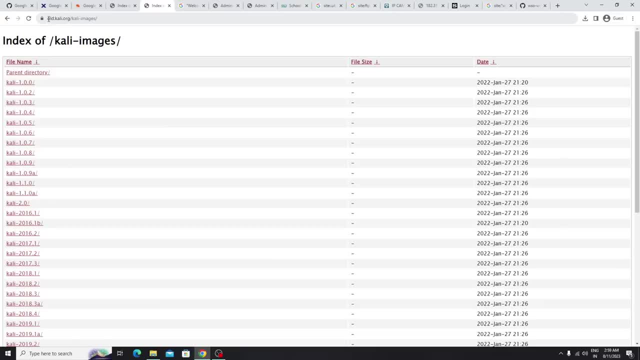 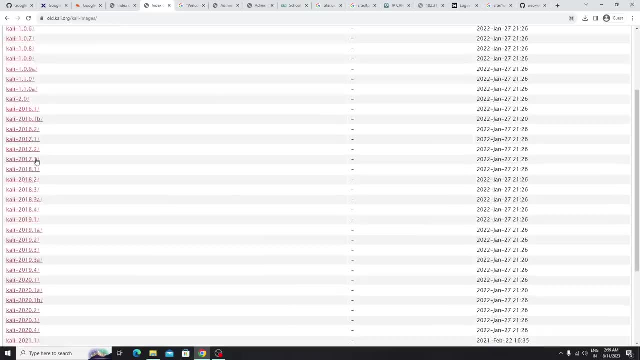 kaliorg old is a. it's a nothing, but it's a subdomain. ok, this is a thing, but you can also see the same thing here as well. the same directly listing, ok, but the thing is, it's not a vulnerability. ok for this website, because it's saying: because 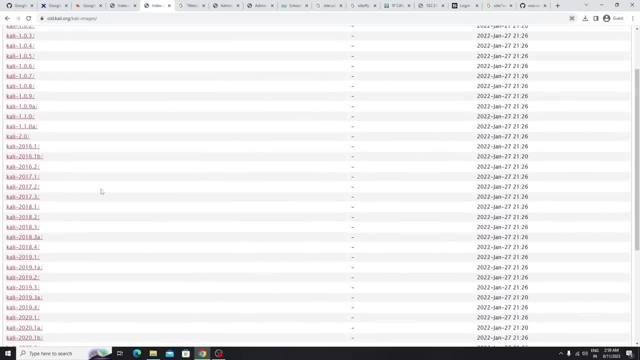 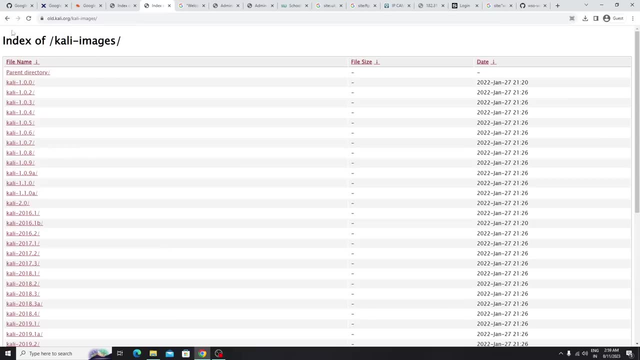 it's providing the images for free right. assume that you are providing some kind of videos or courses for paid at the time. this kind of things are very dangerous for you. ok, you can able to avoid it within few clicks. you guys can able to avoid this vulnerability on your website. 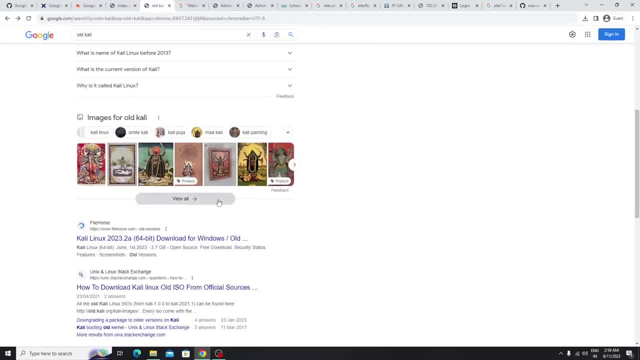 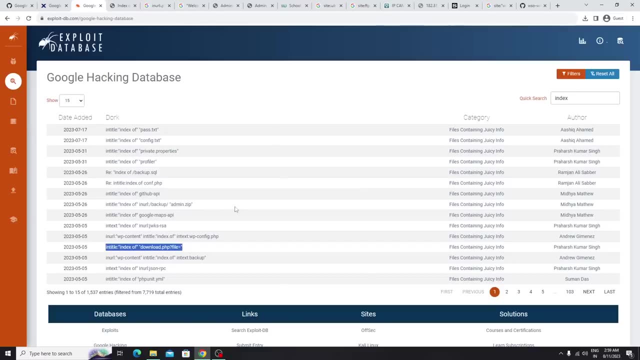 ok, this is a thing. right, hope you guys enjoy this classes again. i am saying maybe i didn't cover a lot about this thing, but let me tell you, just try to use this one. ok, just try. if you are not getting this one as well, just try to copy. 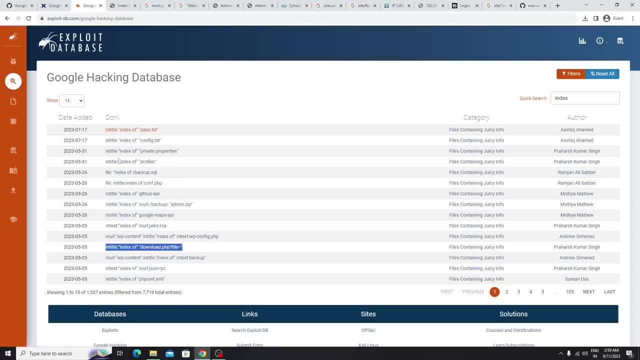 the things this docs or some kind of stuff. just paste it on google, you will see the results. just try to perform the. don't perform the attack. just try to see the results there. ok, that's it. don't perform. don't harm anyone. ok, don't perform the pen testing on this kind. 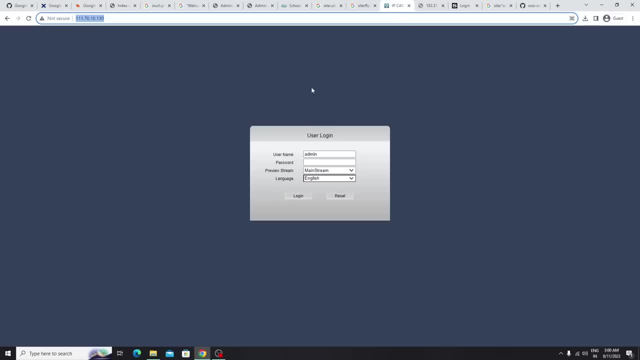 of ip addresses. ok, don't perform. ok, basically, we don't have the permission. i just told you we need a permission. first thing is we need a permission. i am not doing any kind of malaysia stuffs here. simple, i am doing the research. ok, that's it. it comes under what? 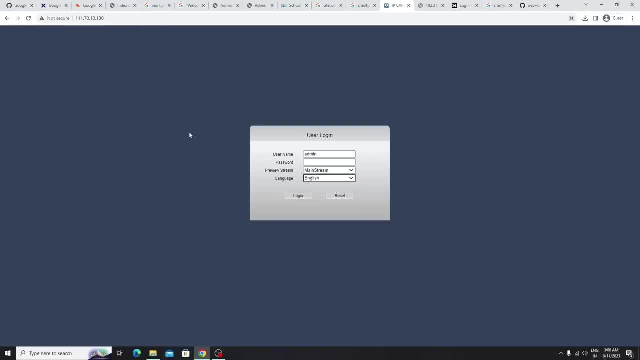 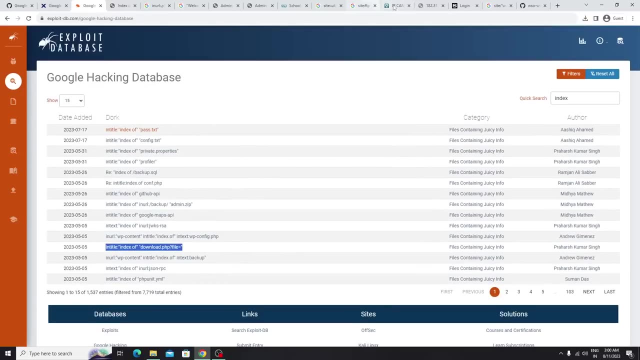 it comes under passive information gathering. i am gathering the information from where? from the internet. ok, this is the thing. ok, i am not scanning the ip address. i am not doing anything, i am just trying to look the stuffs here. ok, this is the thing. hope you guys get it. 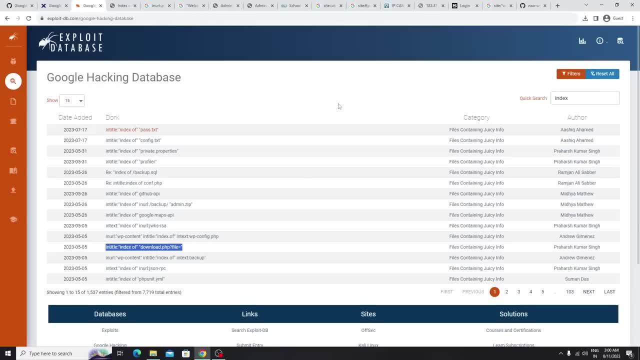 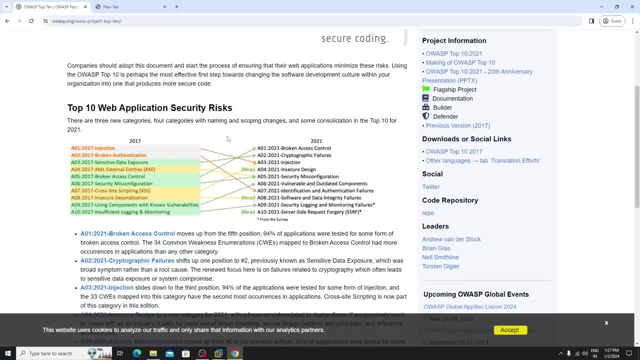 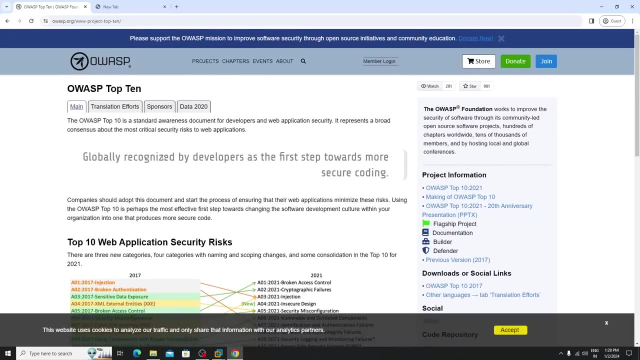 ok, maybe we will learn some new things here. alright, thank you. have a nice day. hello guys, hope you are fine. in this classes we are learning about OWASP. top 10 see the full form of OWASP is open web application security project. here you will see top 10. 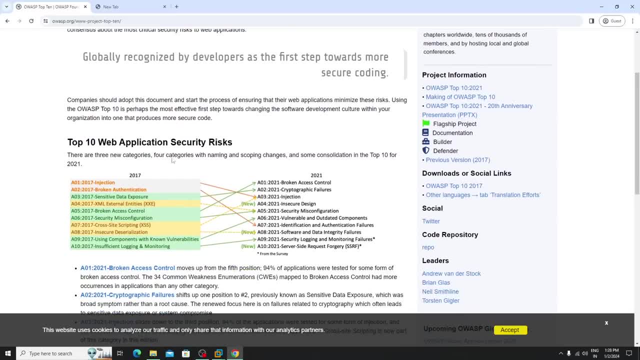 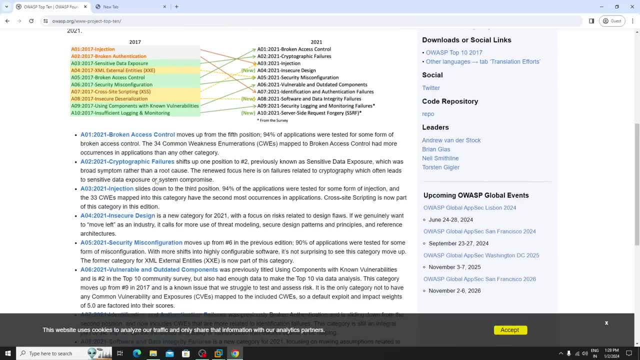 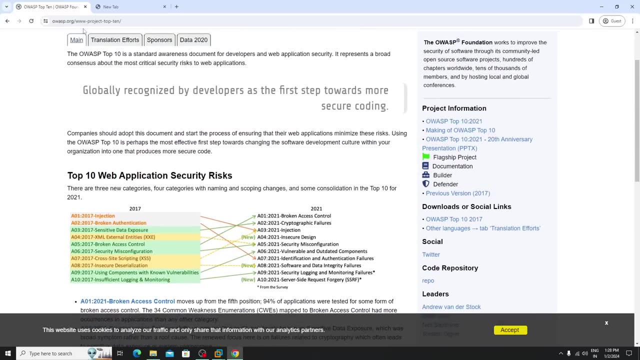 vulnerabilities. ok, like first, let's focus on 2017. in this classes, we are learning about the well known vulnerabilities. ok, we will learn practically how we can able to exploit it right. so the thing is here: you just need to visit this website and you need to learn. 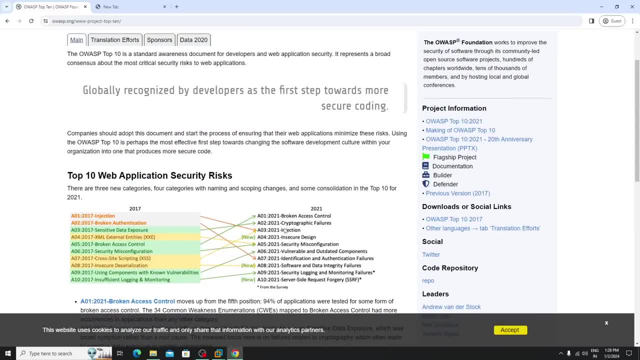 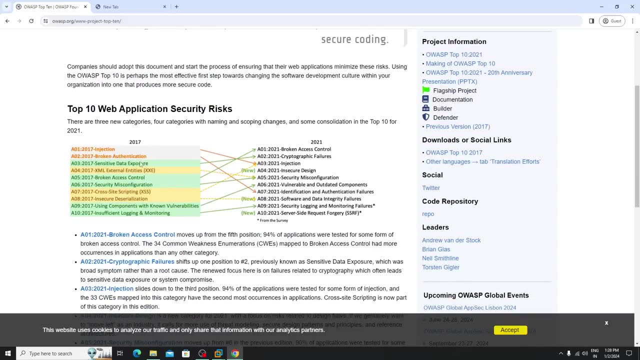 yourself here, because they will update it and they will add huge details here. ok, this is official website, right? so first of all, the thing is you need to learn we will cover injection, then broken authentication, then sensitive data exposure, then external entities, which is xxe and broken. 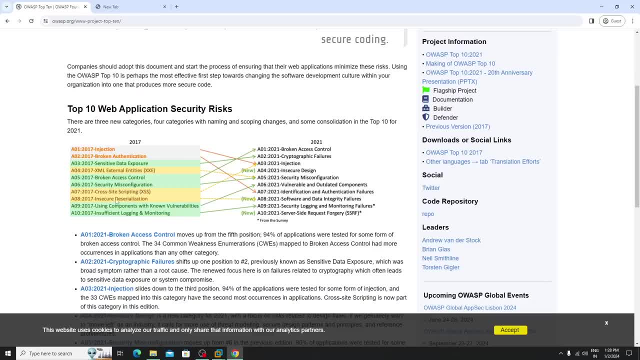 access control, security, misconfiguration, cross site scripting, insecure decentralization and then using components with unknown vulnerabilities like here. assume that there is a wordpress website. is there? assume that the wordpress- that website- is using outdated version of wordpress. ok, basically, in outdated versions. what will happen is there are. 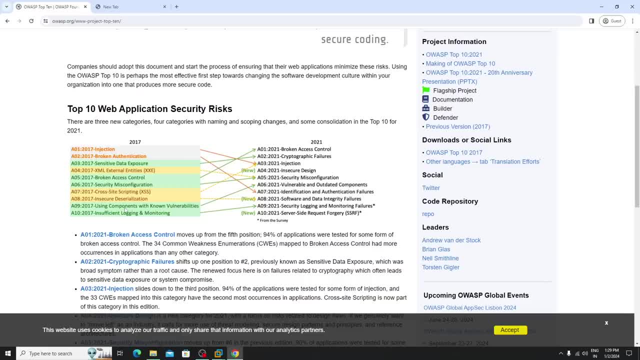 huge vulnerabilities are there like. assume that in elementor 3.7 there is a one vulnerability by like a rc remote code execution vulnerability is here simple. we can able to take control on that website. ok, this is the thing. we will get a like shell there. ok, 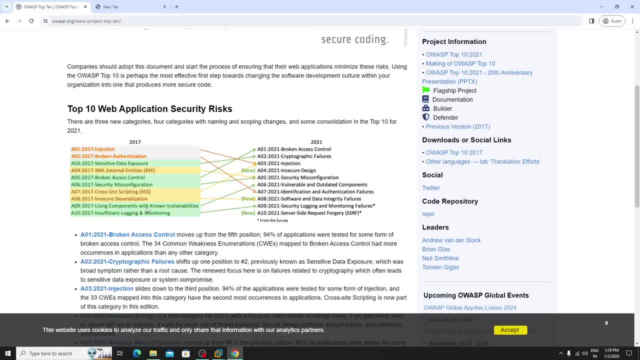 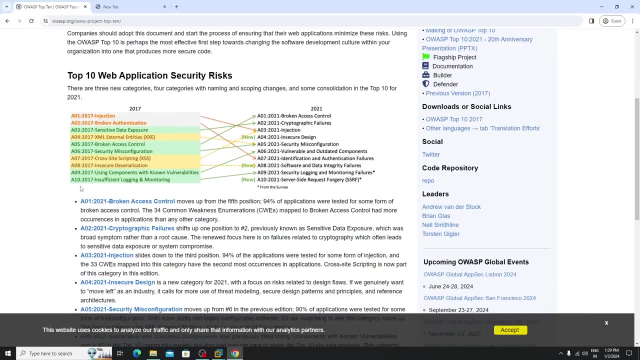 so this is the thing. basically, if your client is using outdated software, is there? those softwares are vulnerable? simple, it comes under this: ok, using components which known vulnerabilities, insufficient logging and monitoring. ok, this is a10 2017. now here, they just added some more, such as ssrf. 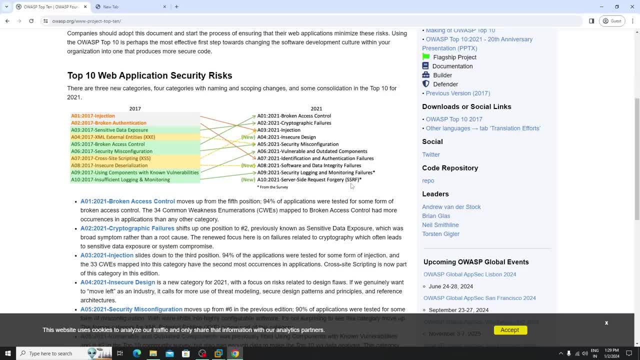 in 2021. ssrf has been added. first of all, again, i am saying don't, sorry guys, don't jump in it. ok, like, first learn 2017, just focus on 2017, then go for one one updates. ok, because these are the basic ok which you need. 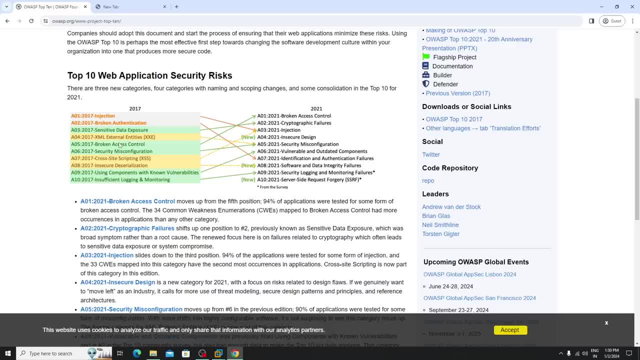 to cover. it's a- like a basic thing. first, you need to cover this, then you will get idea what are these things, or something like that. ok, the updated one: see here in 2021. they just added insecure design, but let me tell you here: insecure design is a, not that. 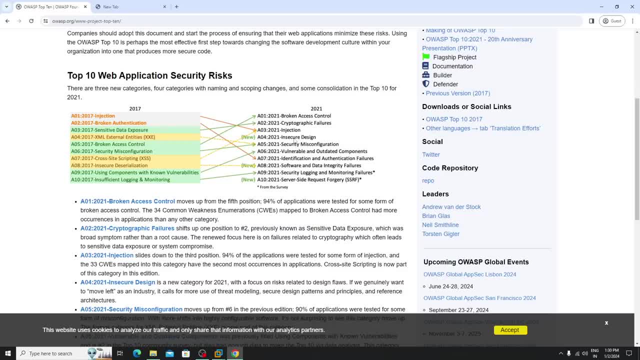 much different. ok, once you learn, you will get a idea about what is insecure design there. ok, what is software and data integrity failure, server side request forgery like ssrf? it's not a big deal. first you need to learn this. ok, we will cover this one. 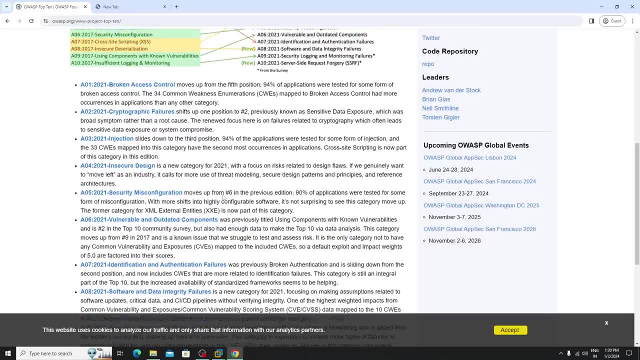 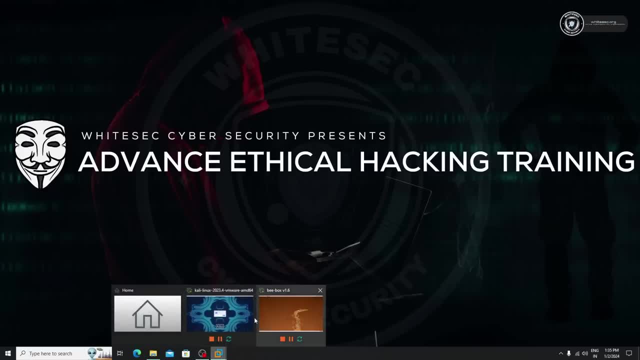 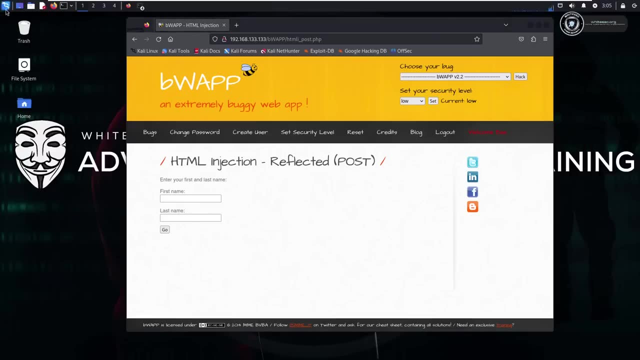 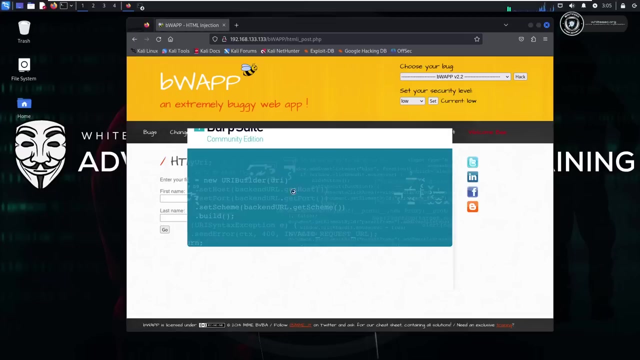 because this is very important right now: here there is a broken, as is control. see, i am not covering now. in this classes we are learning how we can able to setup bup suit. simple search for bup suit: see, here you can able to see the community. 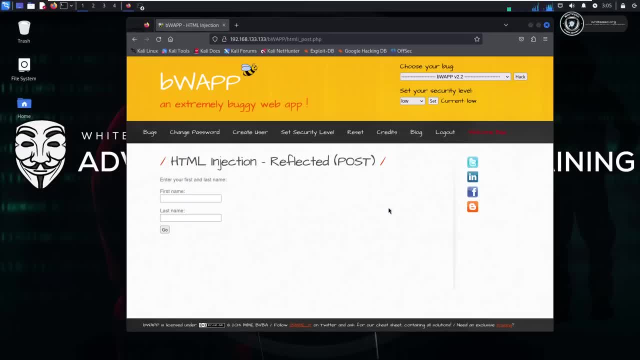 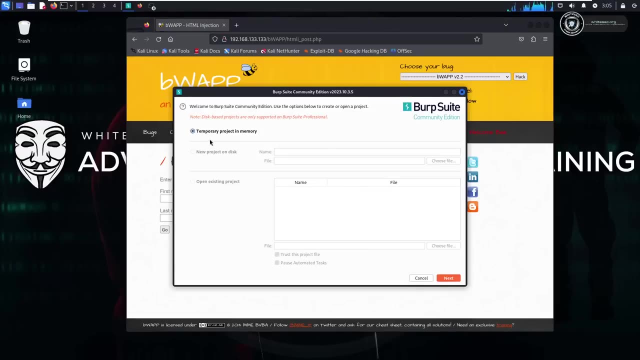 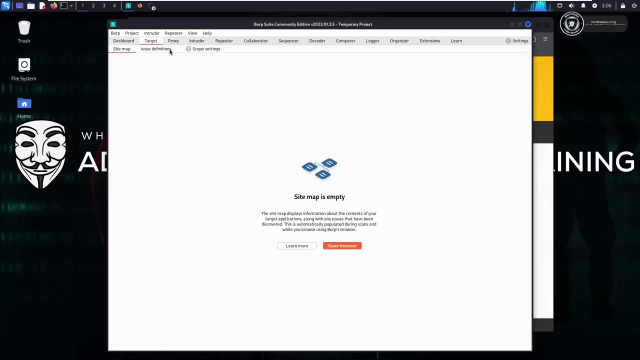 edition: simple, use it, ok. ah, in pro version, you guys can able to use this features. let me select the temporary project here. use bup suit above default. ok, here, it is right, this is a dashboard. this is a target. ok, this is a proxy from where you can. 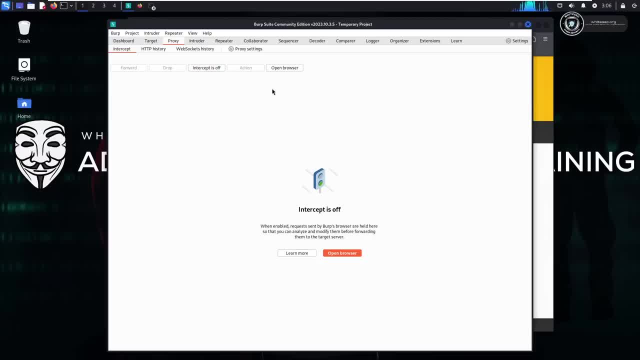 able to intercept the request. ok, you will see here that this is a proxy. ok, once we jump in practical class, you will see what is this decoder. assume that we got any kind of hashes, the encrypted value- at that time, from here we gonna paste it and we. 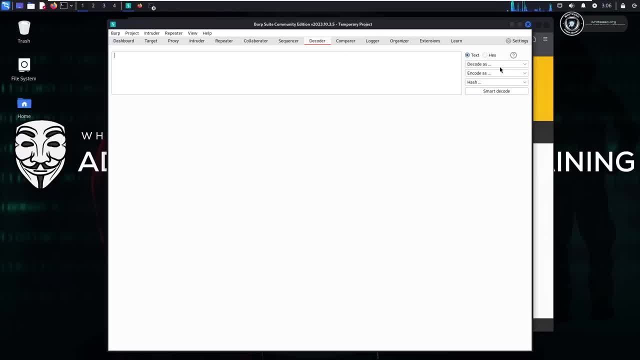 gonna decrypt it. ok, like from here you can able to see, you can able to decode as url: html, base64, ascii, hex, octet. ok, binary gzip. then there is a comparer to compare the results. ok, there is a logger, there is a organizer- ah, organizer, and there is a extension. 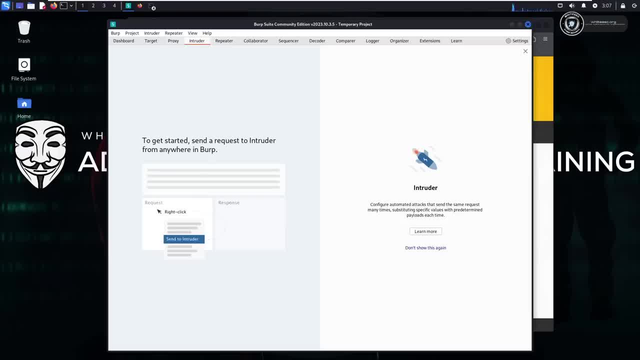 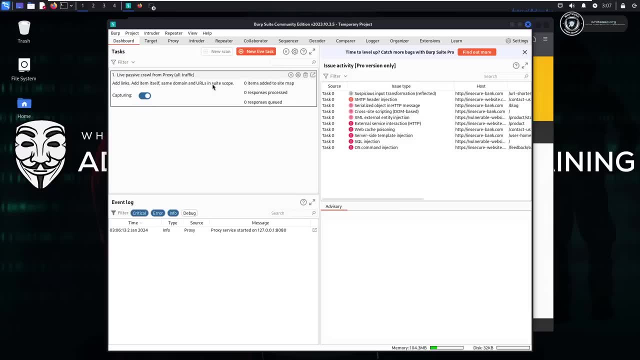 there is a intruder is here. ok, there is a see. basically, this dashboard is nothing but. ah, here you can see the results. ok, it's a automation scan or something like that. it's only work with pro version. ok, right here you can able to see issue definition. 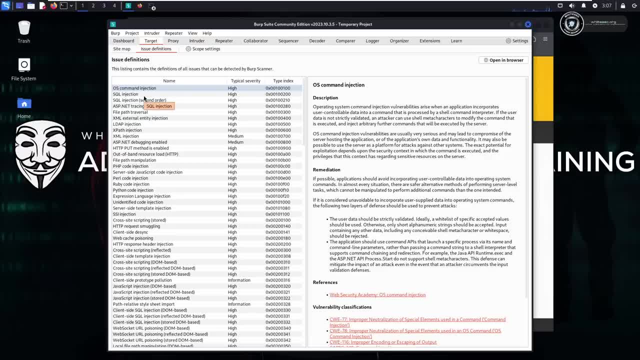 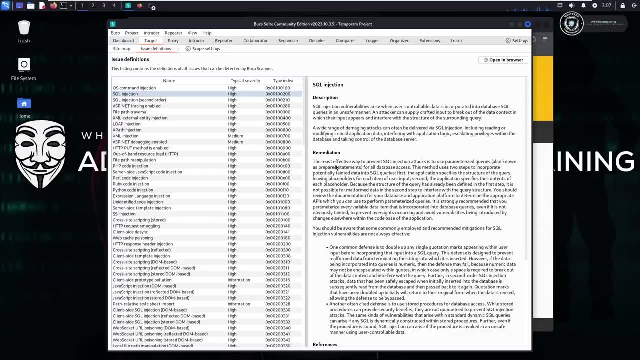 assume that if you want to learn about, if you don't know, what is sql injection? simple, from here you can able to learn it. ok, there is a remediation, how to avoid it? ok, something like that. so here is a list, from here you can able to read it. 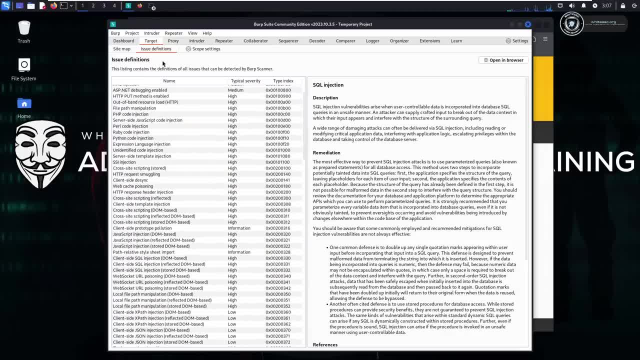 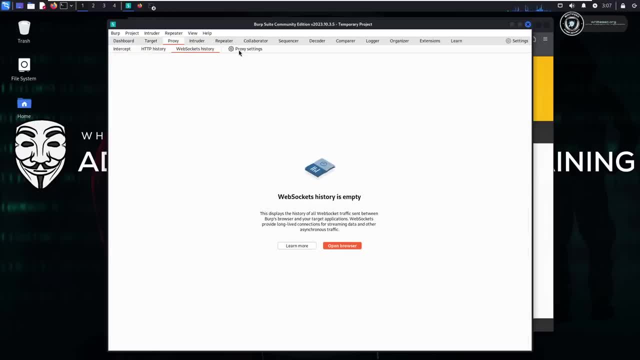 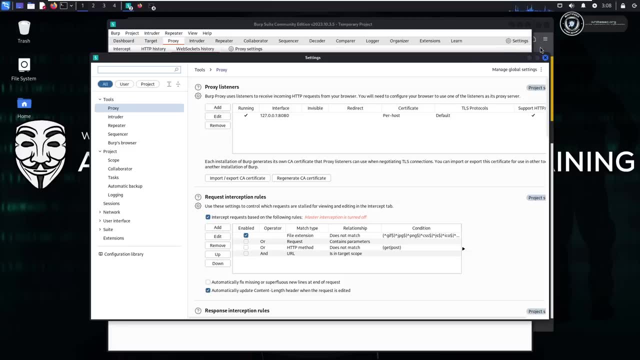 but still, i will try to explain you in the classes as well. right now there is a http history, is here websocket history, proxy settings. now proxy settings: how? first of all, you need to setup this thing. how to setup it. this is very easy process. ok, just open your wireshark. 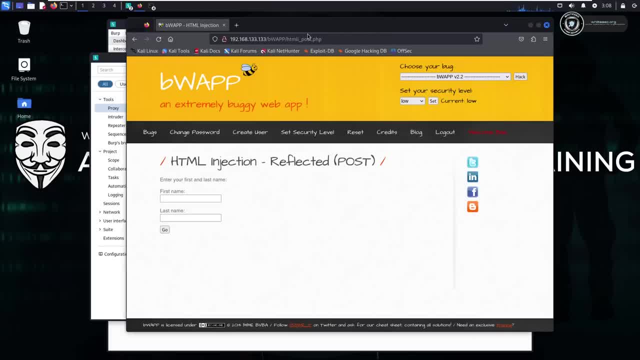 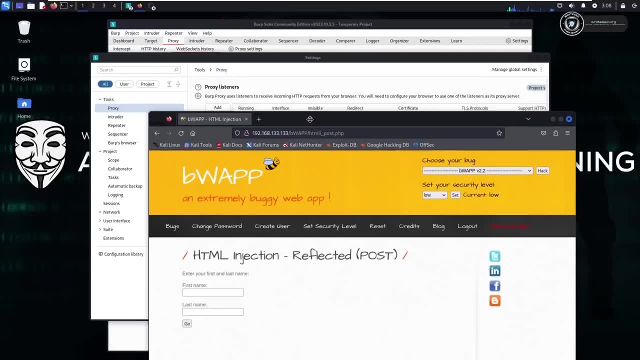 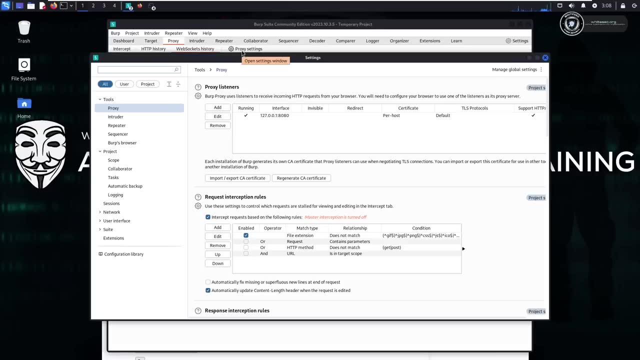 if you are using- ah sorry, not wireshark man- firefox. mostly we use firefox here right now. simple how to setup it. see here. let me show you again. click on proxy settings. in proxy settings you guys can able to see there is a proxy. you can also edit it. 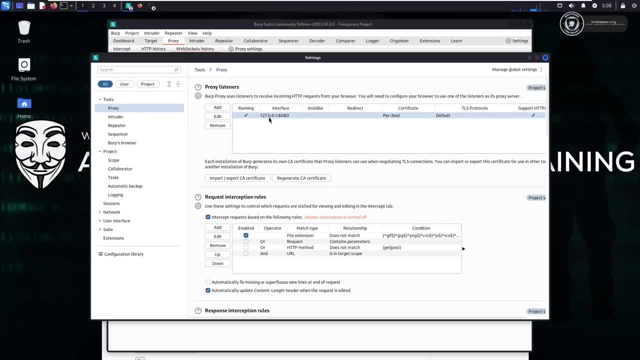 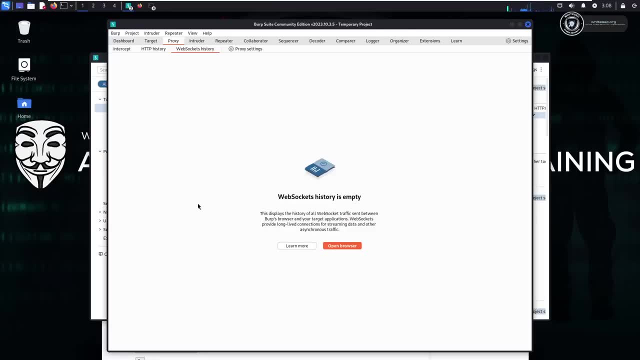 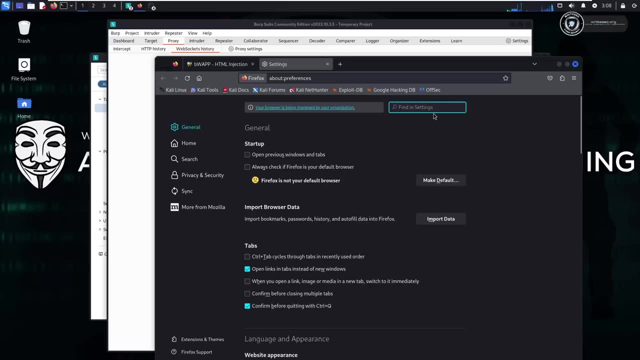 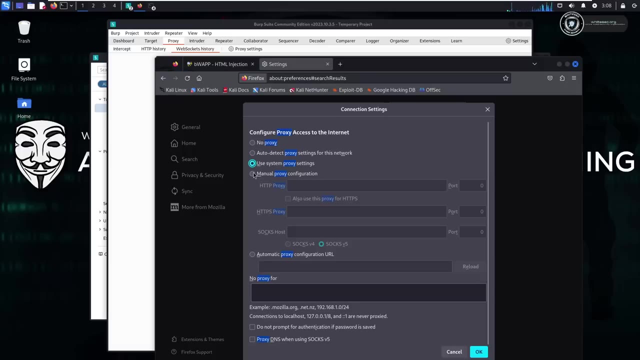 it's a loopback ip address, basically 127.0.0.1, and the port is 8080. ok, now, simple. it is a firefox. click on settings, just search for proxy here, just settings. click on settings and simple. change to manual and add the. 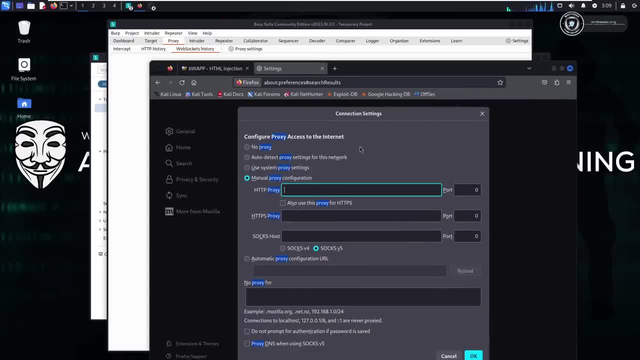 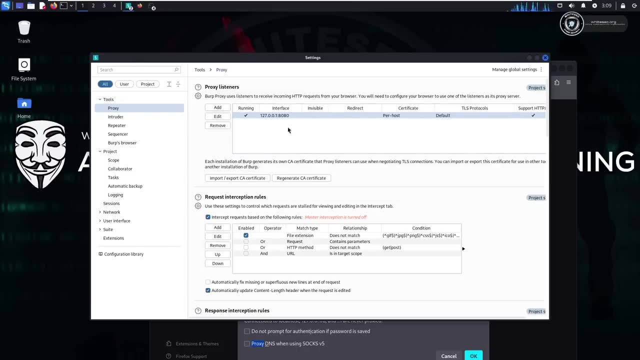 ip address here, which is loopback ip, which is 127.0.0.1. ok, here you can able to see that this ip address. ok, you can also- sorry guys- change it. go for by default. ok, and change the port to 8080 because it's using 8080. 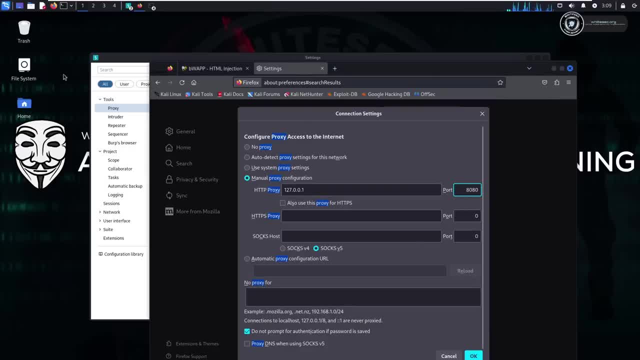 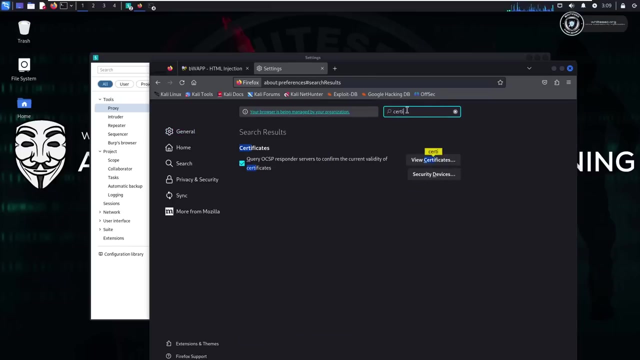 right, ok, and here just check this one and also check this soc5. also use this one, ok here. copy and paste it here. change the port to 8080. right after doing that simple, click ok. and then search for certificate. ok, here there is a click on view certificate. 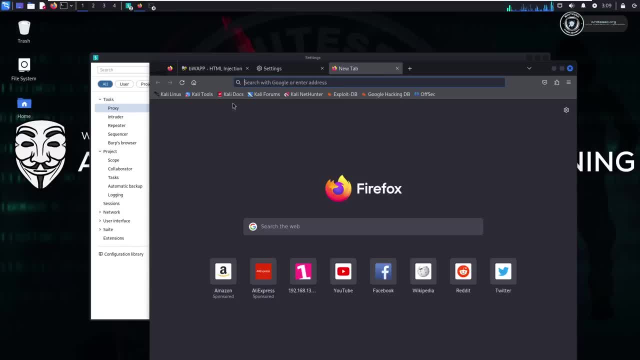 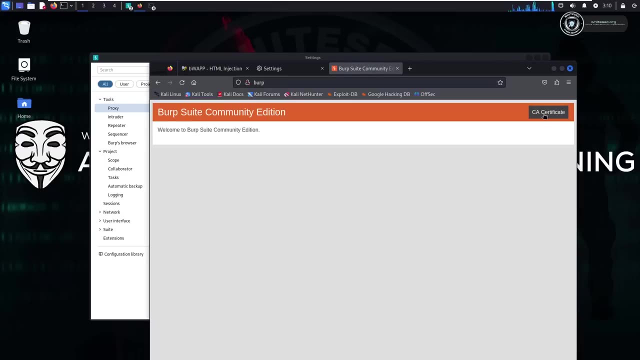 now you need to download the certificate simple. just search here: http forward slashes, view rp. ok, here you can able to see the simple click on this icon, see a certificate and download the certificate here, because if you don't, if you didn't setup this certificate, then you can't able to. 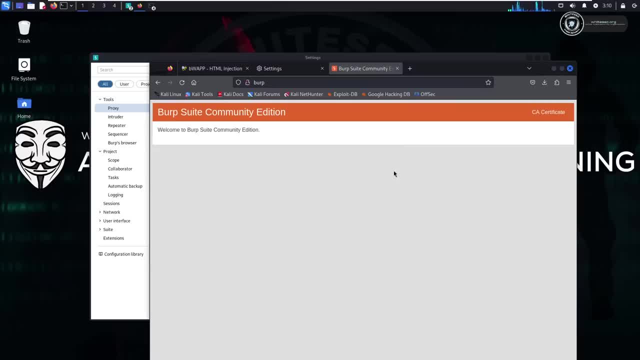 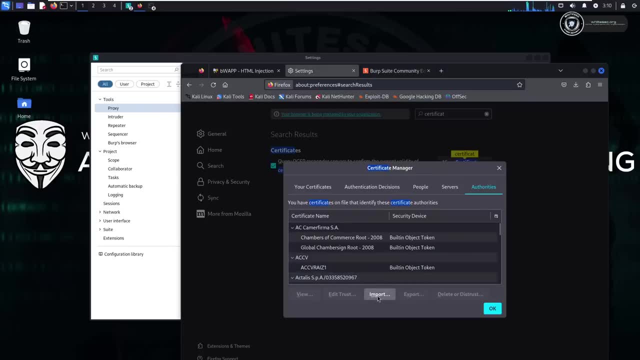 perform pentesting on https websites. ok, it can't able to. basically, it's a kind of man in the middle. ok here, simple click on import and select that certificate which you downloaded. just select it, ok, and click on trust the check this icons. ok, checks, sorry, man checks ok. 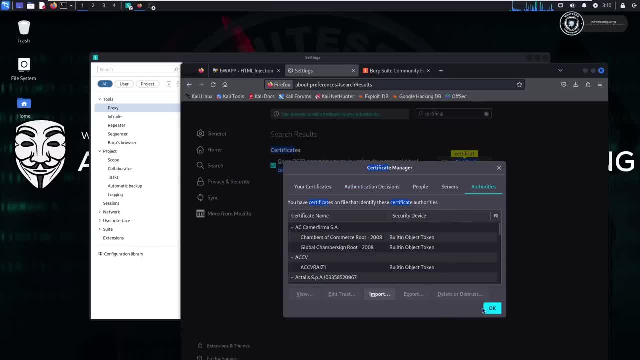 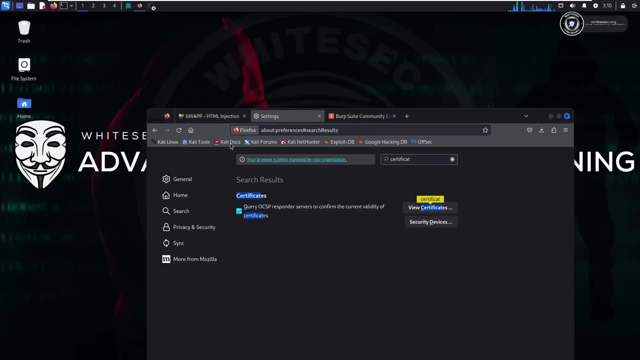 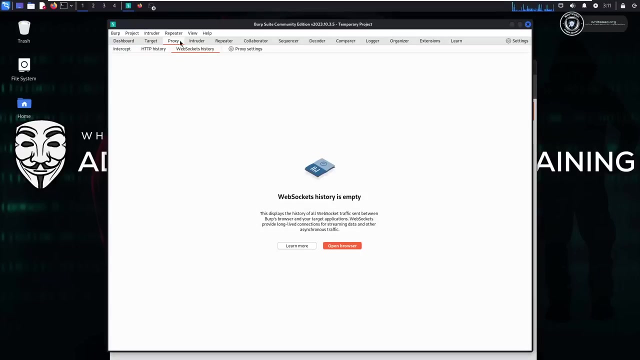 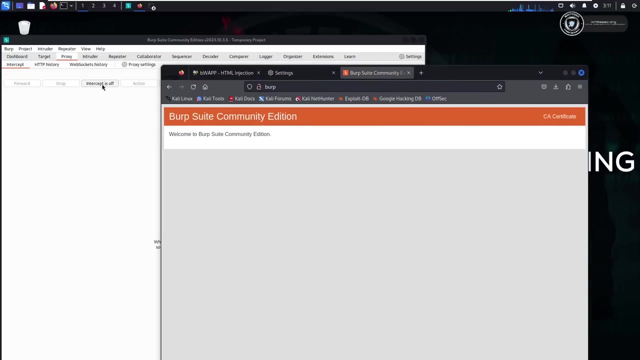 simple click on ok, successfully uploaded right. just click ok there. ok, ok, ok, ok, ok, let me see if I can able to intercept that data or not. ok, ok, click on that data again. this click on intercept. ok, click on this right now. its half. let me search for google. 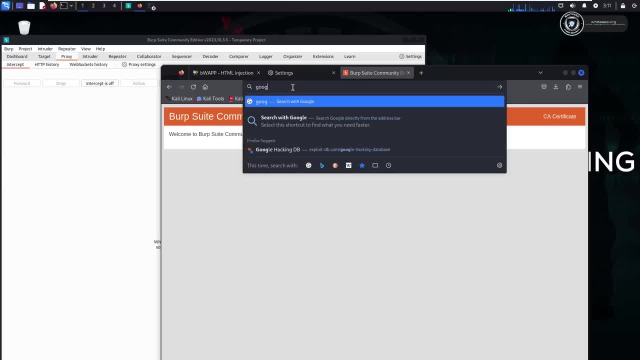 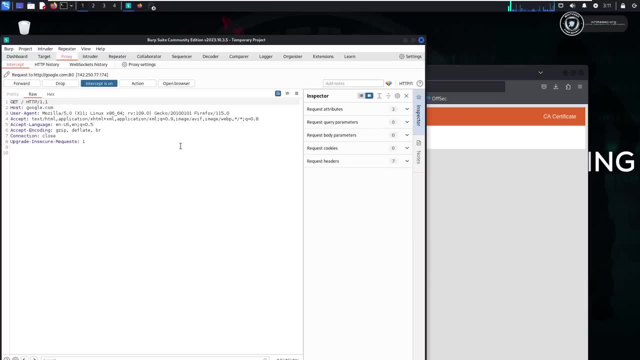 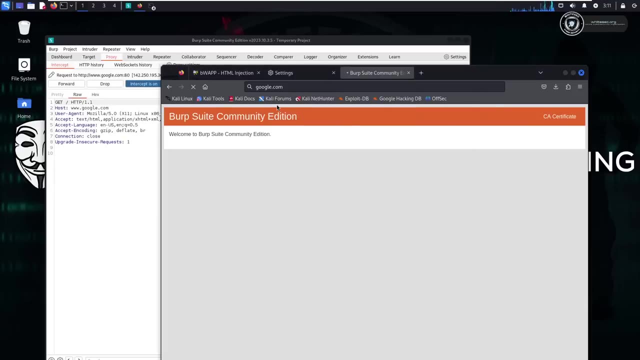 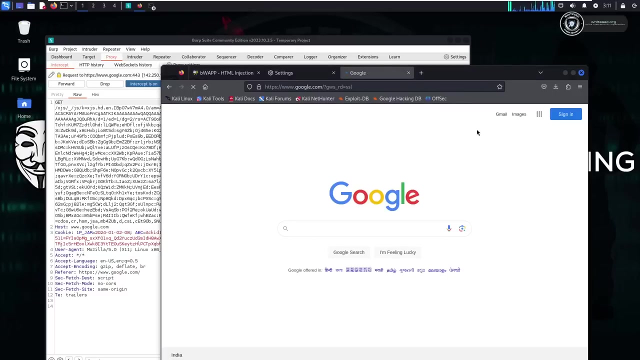 com here, simple, let me intercept on. let me search for googlecom. see, here i can able to intercept the request. if i click on forward, then only it will uh show us, okay, the googlecom results. hope you guys can able to see the the basic thing: what i'm, what. 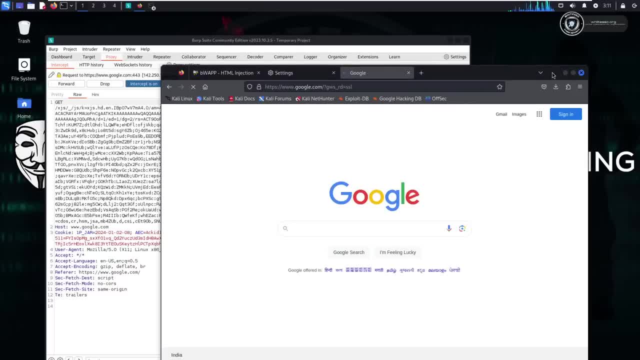 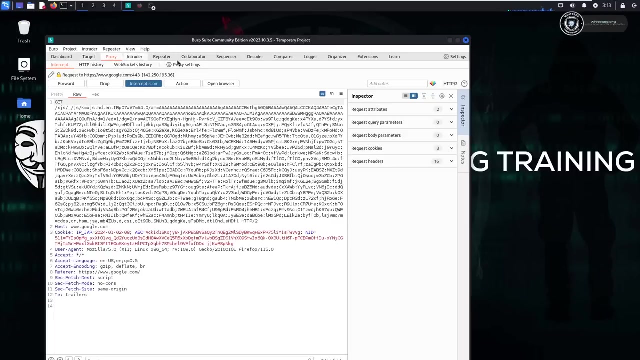 i'm trying to say means here. the thing is, basically we are intercepting the request. here you can also intercept the response as well. basically you are intercepting the request and response. okay, this is the thing right. once we jump in practical, in practical classes, you will get it. okay, you no need to worry about this bup suit, it's not that much difficult. 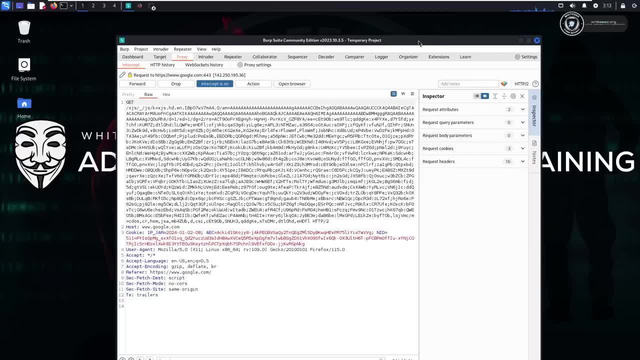 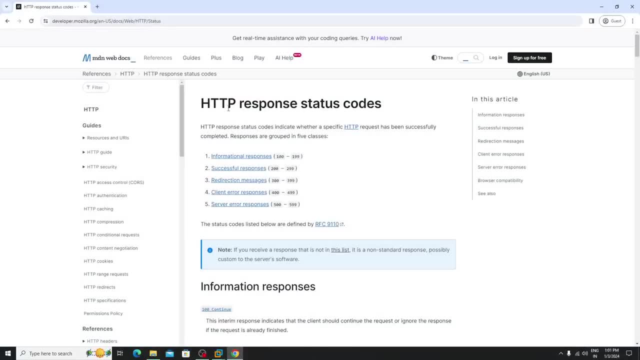 if you learn how to use bup suit, then it is excellent, man, okay, right. so guys hope you are fine. in this classes we are learning about http response status code. this is a website which you need to visit and just learn about status code. let me tell you this. 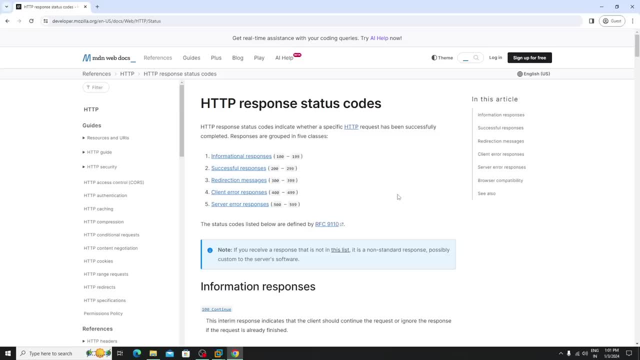 status code is a website which you need to visit and just learn about status code. let me tell you this status code is a website which you need to visit and just learn about status code. let me tell you status codes plays a very important role in web hacking. okay, let me tell you right now: you won't. 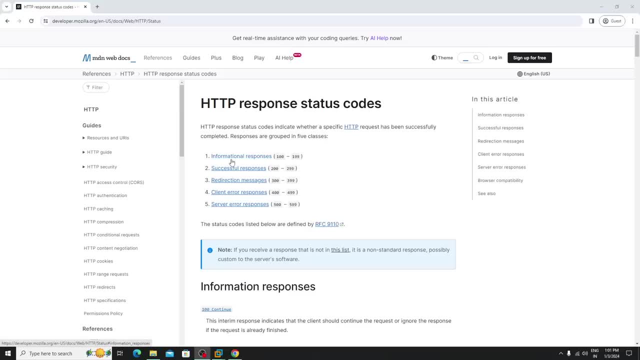 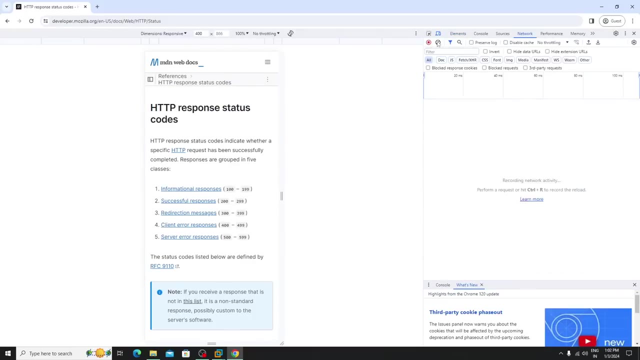 get it. if you don't know about status code, then no need to worry, just remember this website. okay, now see, assume that let me click on inspect, right click and inspect and click on network here. just let me clear this, okay, and let me load this website. let me take any request from here. okay, see. 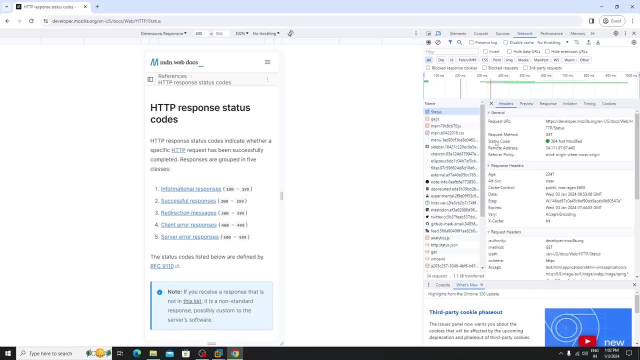 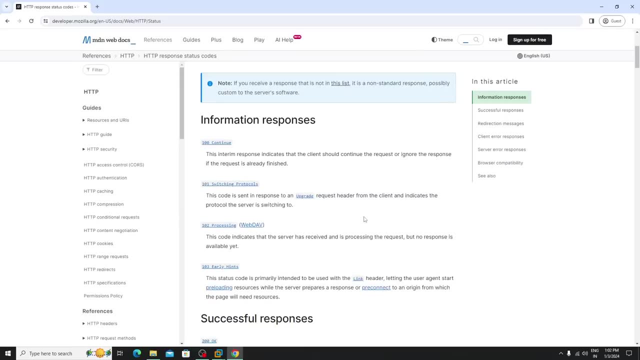 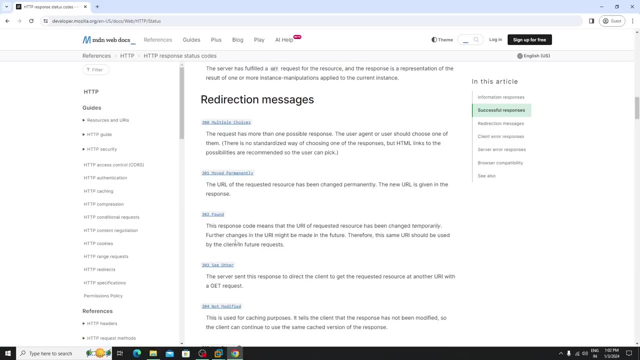 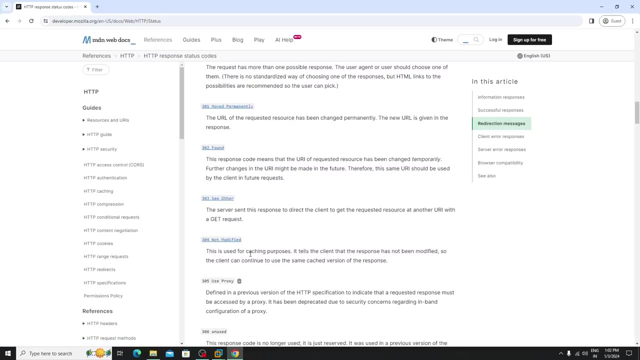 here there is a status you can able to see. there is a status code which is 304, not modified. okay, what is this? let's learn about this thing. what is it? 302, right, sorry, 304. so here it is 304, not modified. what is this? this is used for the caching purpose. 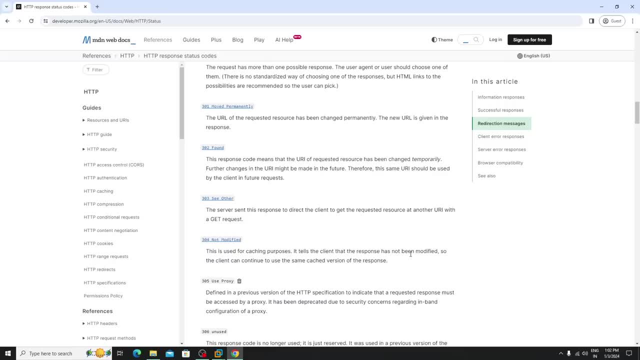 it's still the client. that response has been modified, so the client can continue to use the same cached version of the response. if you want to learn about this status code, then simple, just type here. uh, just click on 304, and from here you can able to learn. 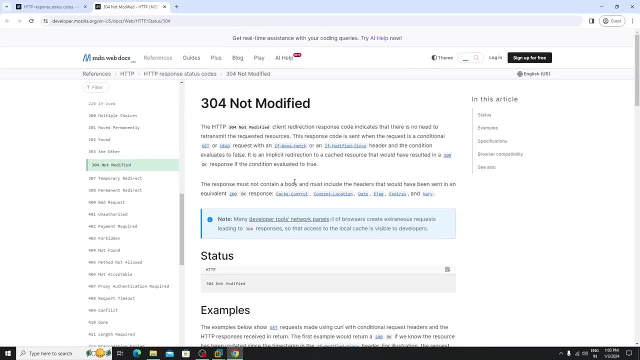 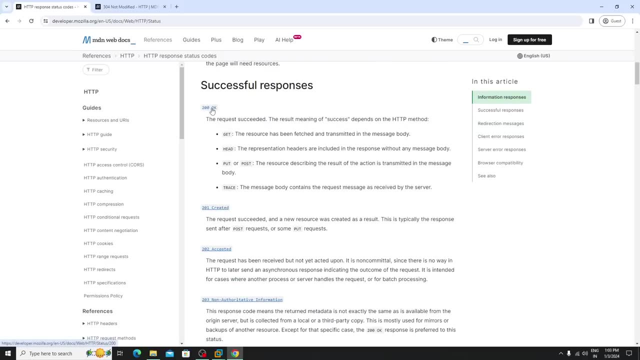 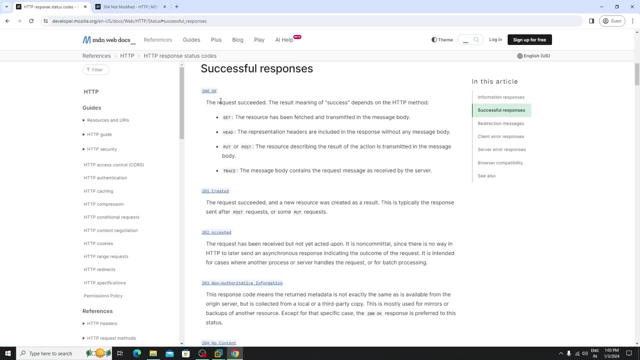 it okay, but the thing is here, you no need to go that much deep here, but the uh, the thing is, you need to focus on this status code: okay, which is 200. okay, just see, there is a uh successful response. just focus on this thing. see, successful responses are 200. 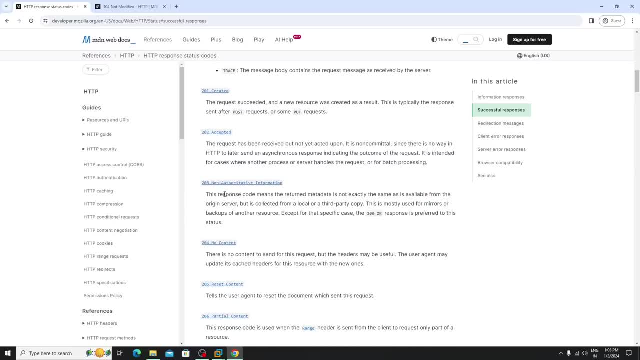 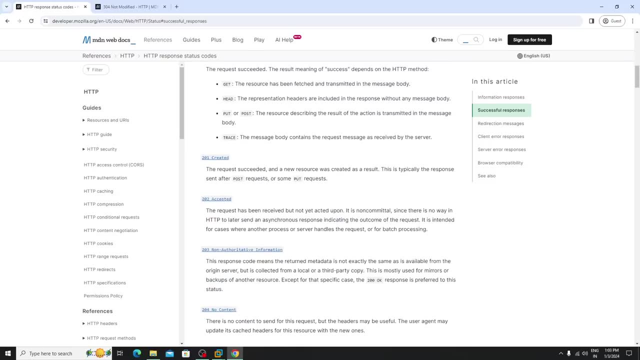 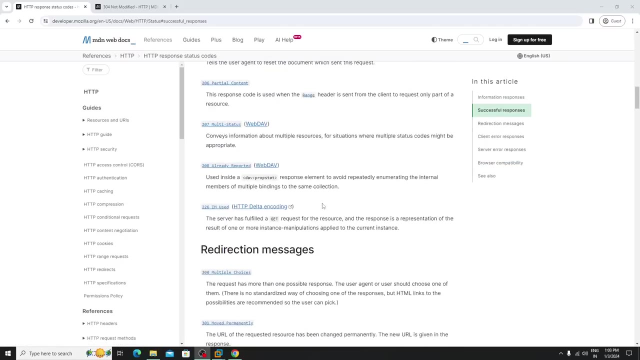 201, 202, 203, 204, okay, 205. this comes under successful response. okay, basically, we perform some kind of fuzzing kind of stuffs at the time. these things are very useful for us, okay, basically, sometimes, uh, what you need to focus means here, just see. 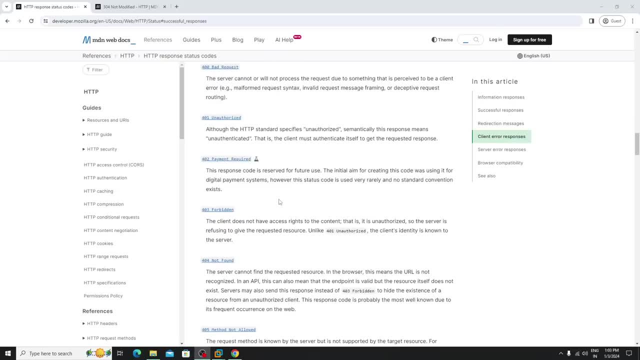 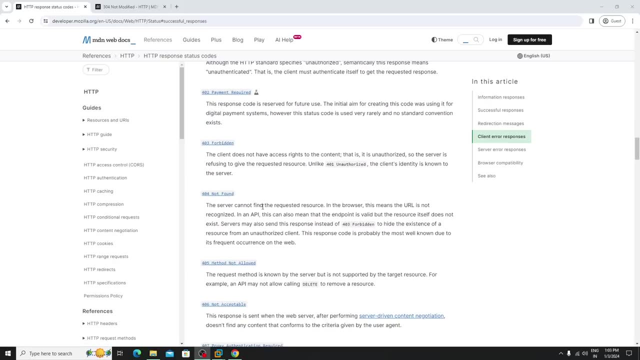 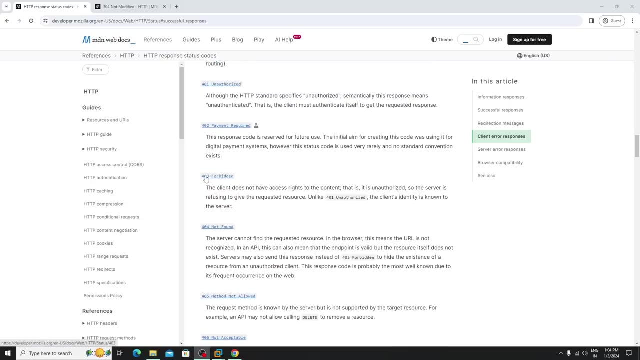 mostly when we perform the fuzzing. okay, at the time we see this thing: 404- not found. okay, what is this? server cannot find the request resource in the browser. this means the url is not recognized. okay, there is a 403- forbidden. sorry, forbidden. this thing also play a very important role assume. 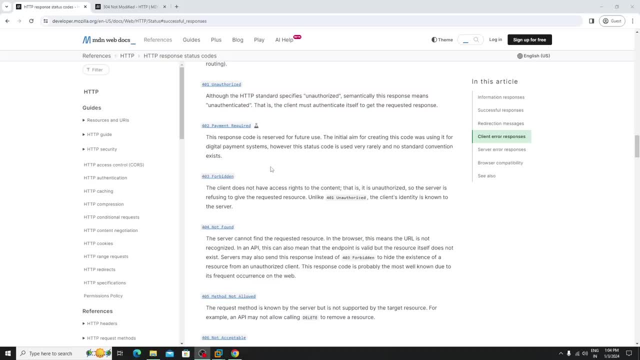 that you just found some subdomains or some private ip addresses. you found the private ip address as well. you can't able to access it to page that uh ip address in your in your search bar. at that time, what will happen means it will show the error, okay. 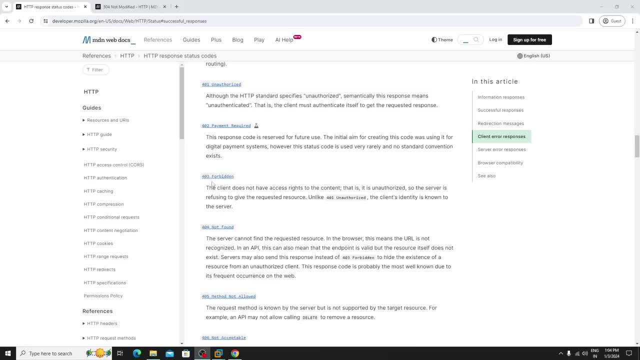 this kind of error, such as 403 forbidden. that means the client does not have the access right to the content. that means, uh, you can't able to access the content is there, okay, but you can't able to access access that content, like you can't able to see that panel. you can't able to see. 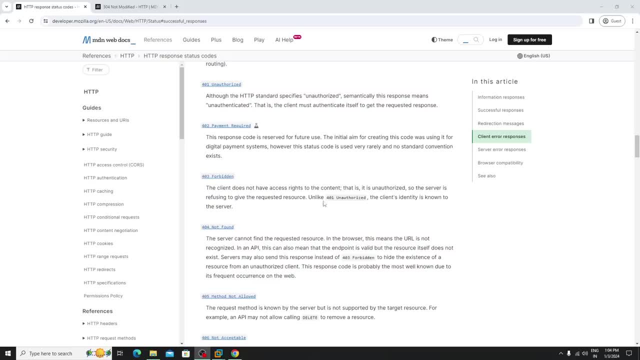 what is there. this is the thing you can also bypass this one. it's not a uh mustang, but mostly there are some kind of subs. uh, by following that we can able to bypass it. okay, let me tell you right now, if you don't know about web hacking, then you won't get it, okay. 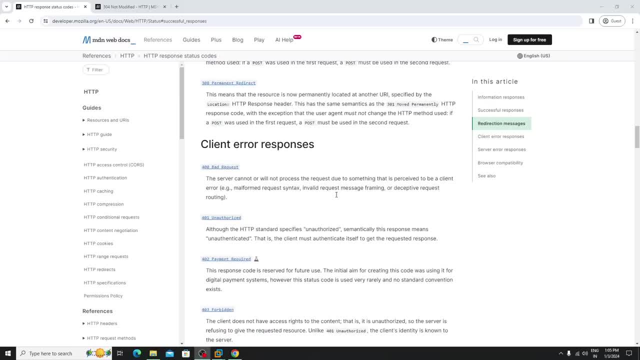 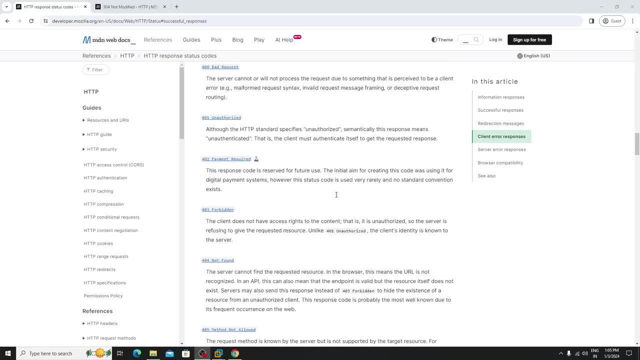 you won't get that much about the status code, but once you jump practical, once you start the practice, uh, on web hacking, at that time this play a very important role. okay, here this is again. i am saying this is a very excellent website from where you guys can able to read about the 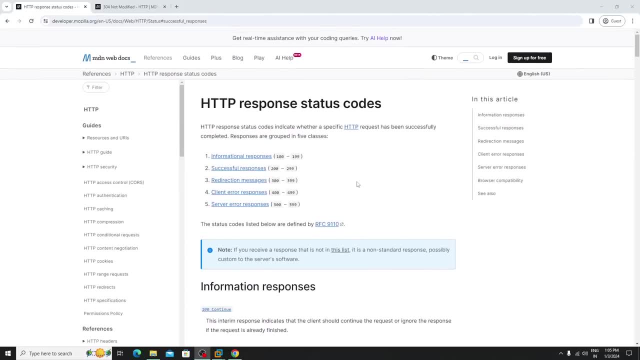 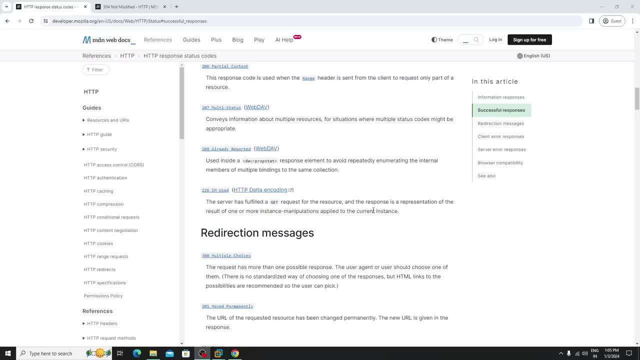 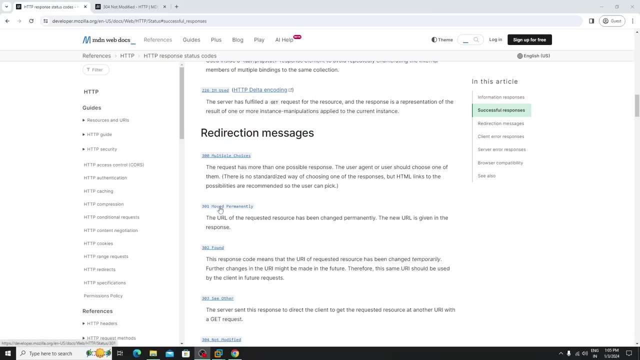 status codes as well. you can go deep drive there, but let me tell you, uh, assume that what i do mostly uh during beginning, okay, when i am beginner, at that time, what i do means, when i found this kind of status code, i come to this website and simple search for it. okay, i just 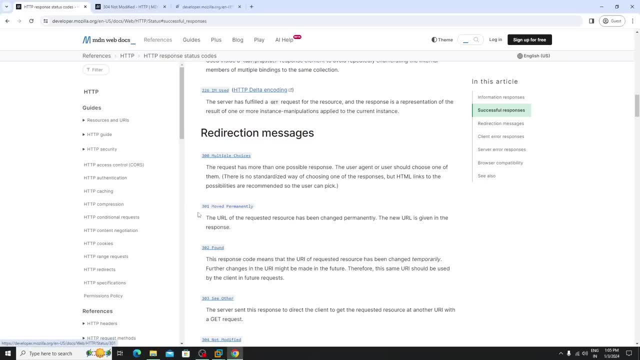 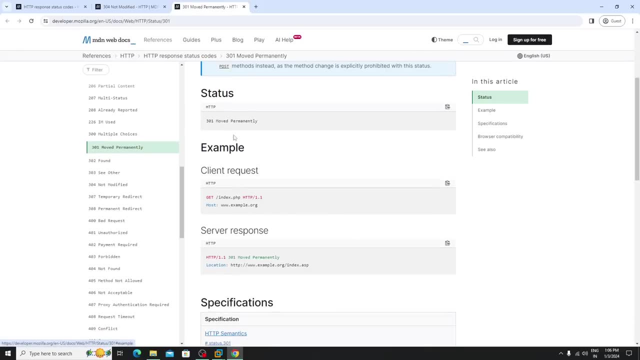 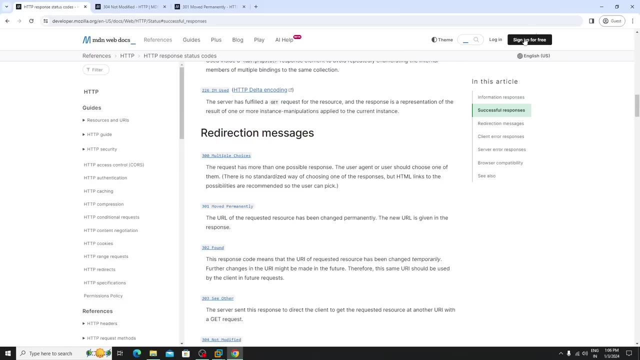 uh, i'm gonna simple read about that status code. okay, this is the thing. so here is the thing. client request is that you can also see the examples here. okay, so display a very important role here. you just need to mark this page, just bookmark in your chrome or something like that. it. 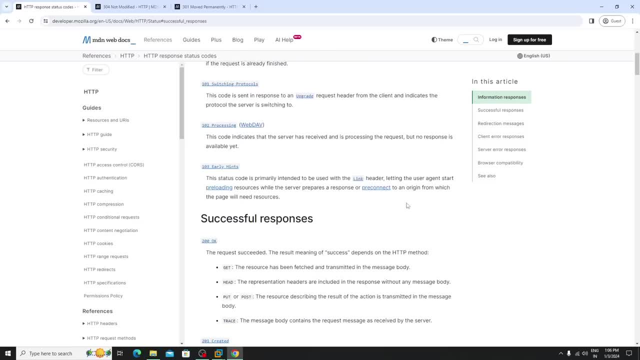 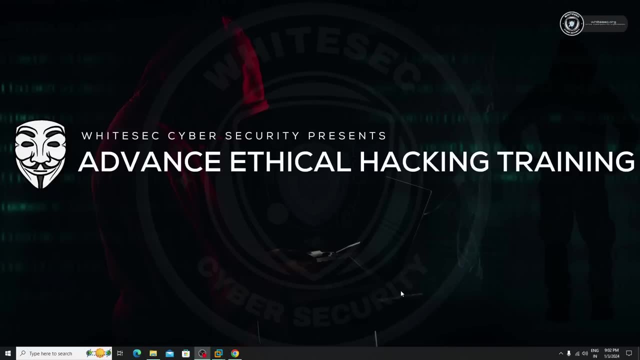 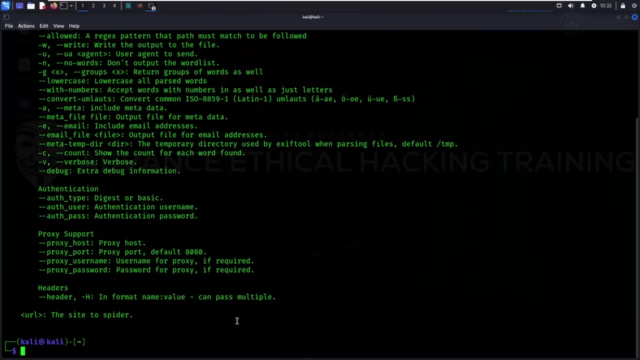 will very useful for you. i hope you guys enjoy this class. once we start practical at the time, you will get it. thank you, have a nice time now. in this class we will learn how we can able to generate good list. okay, according to your target website. now see: just select any target website. assume that here we have one website which is: 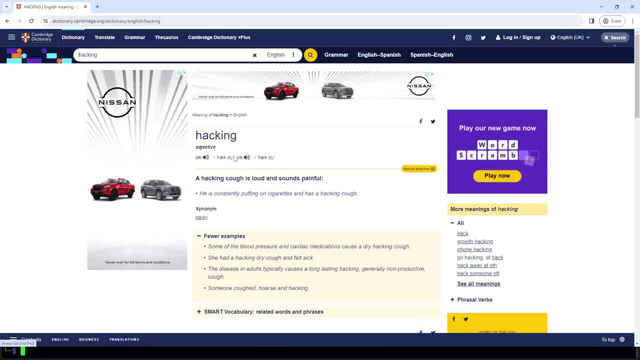 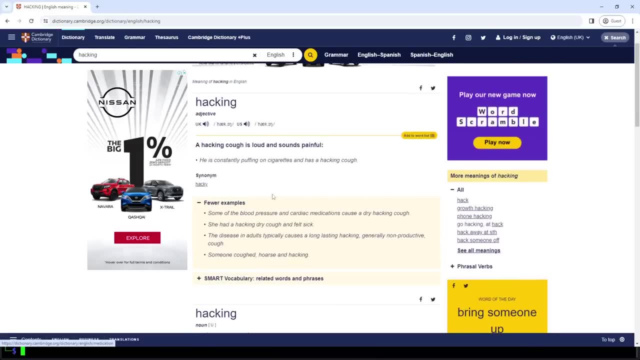 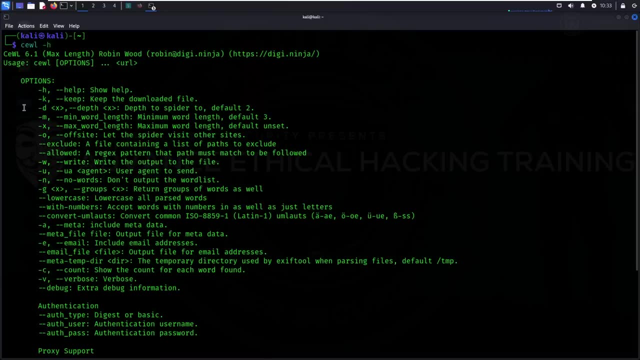 eriecambridgeorg. here i just search for one keyword, which is hacking. okay, you can select any website here, simple. what it will do is by using it is a tool. type here space. dash h, you can able to see there is a. the main commands are here. dash d, which is depth. okay, i'm gonna. 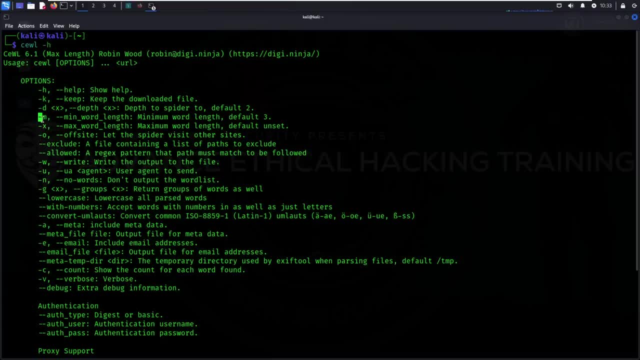 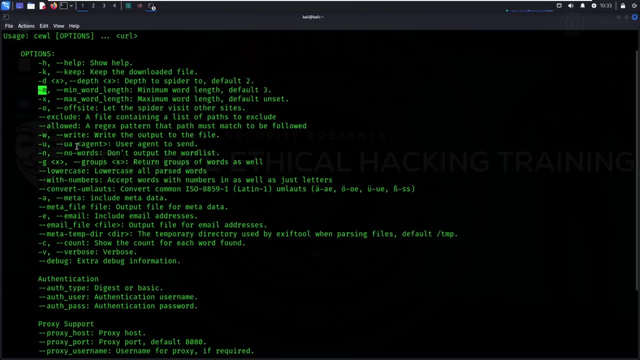 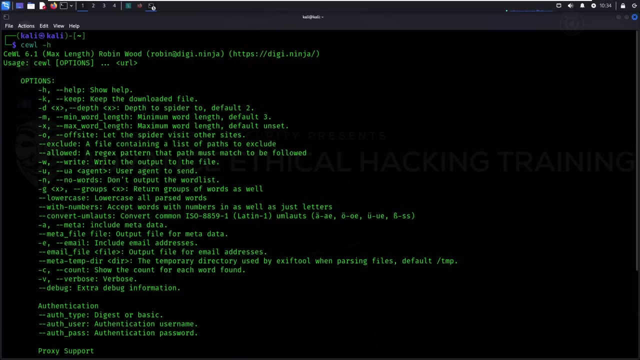 explain you what is this depth? and dash m is for a minimum word word length. right, and here you can able to see. you can also save the word list here by just typing dash w, write the output, the file. okay, no problem, let me. let me. first of all, let me show you how we 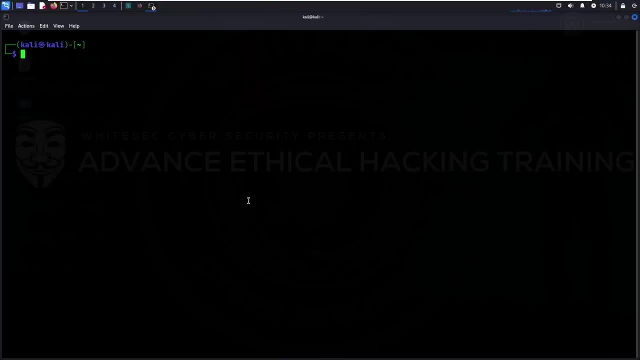 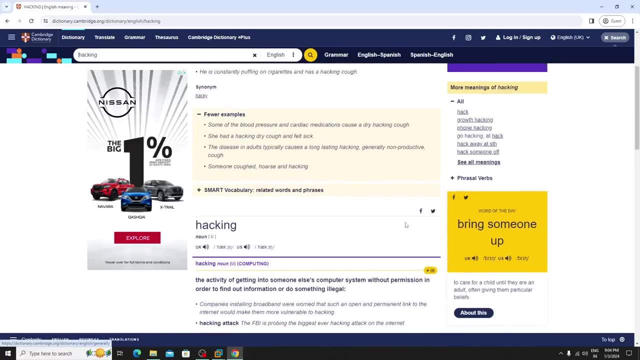 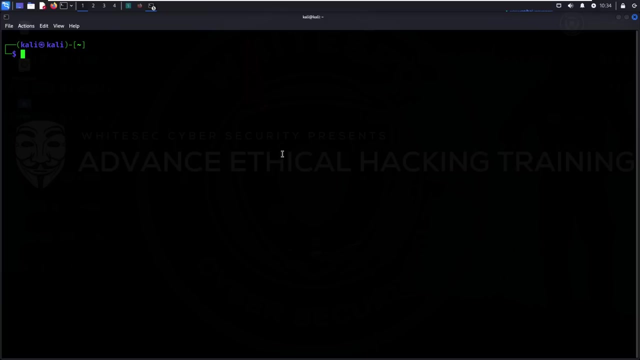 can able to do it. okay, not a big deal, to generate a word list according to the site. now, bottle of this website. let me type here quill. okay, let me type here dash d depth. okay, here, depth. what is definitely here? there is a website, right, website- in this. 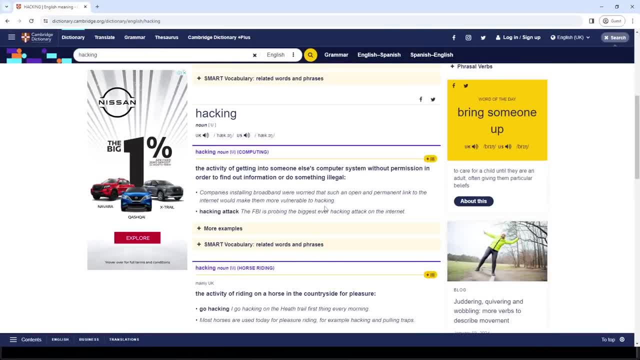 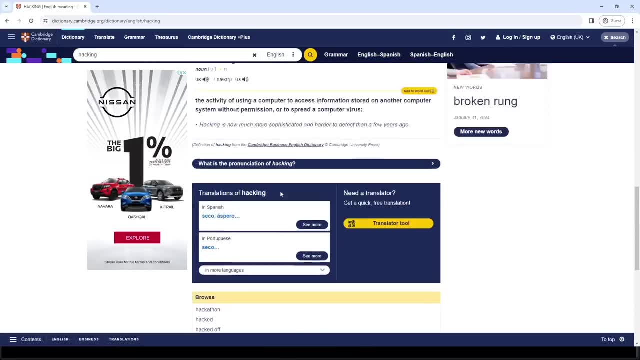 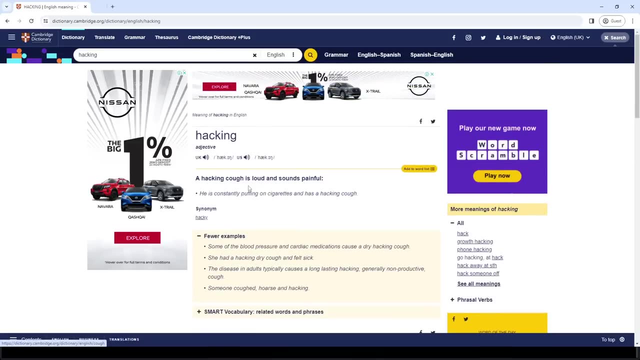 page you can able to see some keywords. have the links as well by there are some keywords here you can able to click and redirect to another page. see, there is a cough. is there a click here? then redirecting me to another website. see, assume that the depth is nothing but. 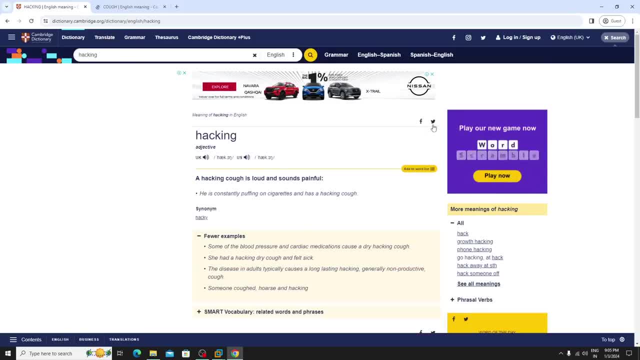 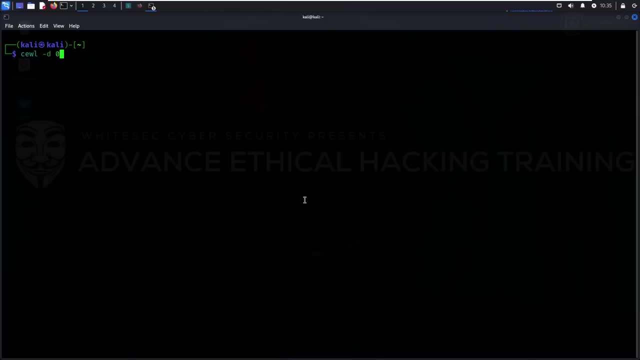 here. it will gather the keywords from here as well, from this website and also from those website which having sub links in it. okay, this is the thing assumed, let me show you. assume that if i type here, zero depth is equals uh, dash d depth. uh means zero. that means what i am. 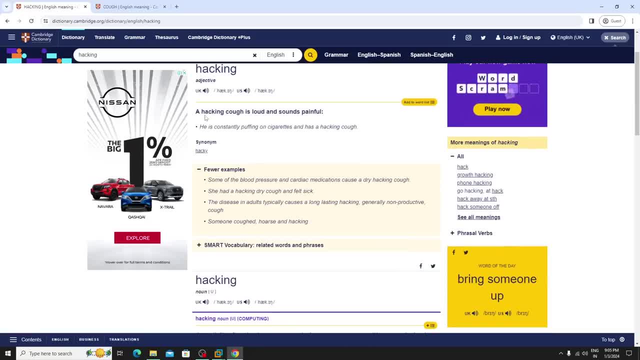 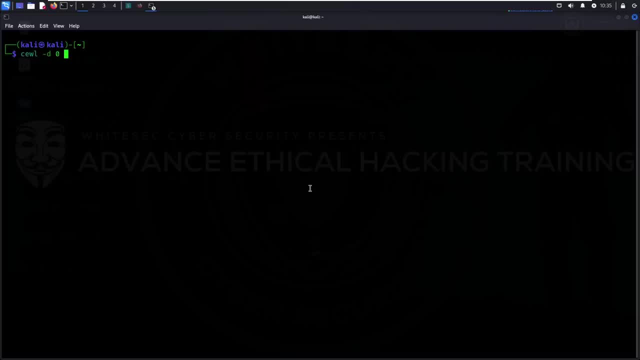 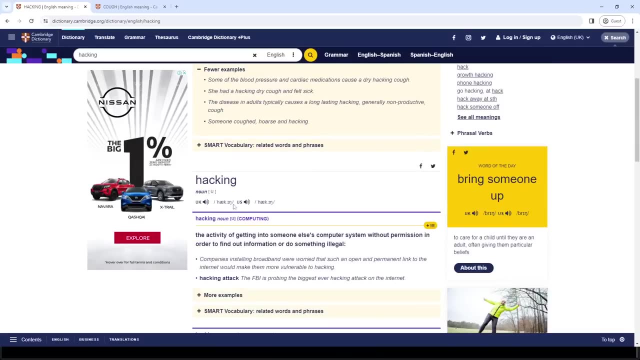 doing here. i'm just gathering the keywords from this page. okay, i'm not digging in this links or something like that. assume that if you type here dash instead of zero, if you type one, then what will happen means it will start digging from this. uh, urls as well. it will open this urls, okay, like. 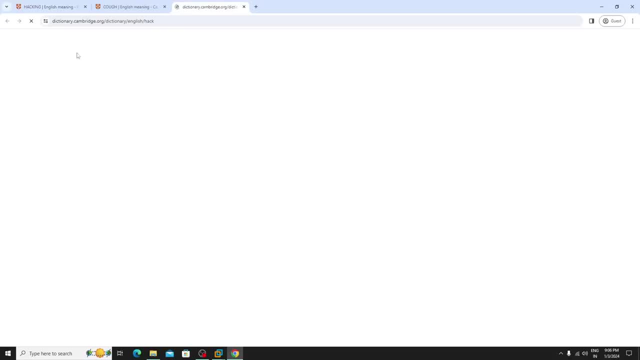 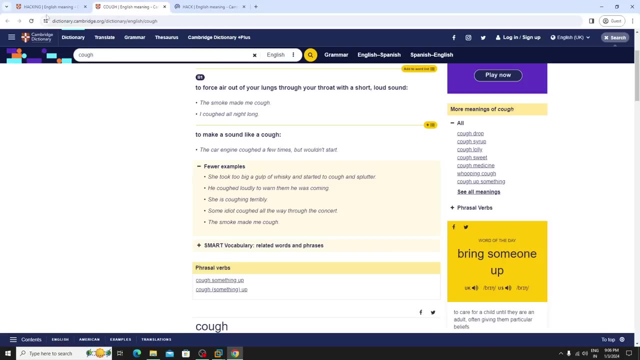 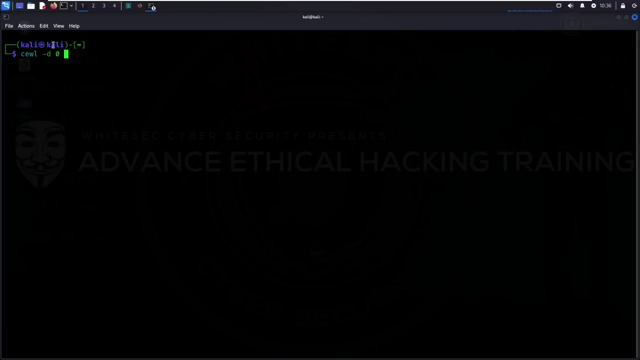 this, then it will gather the keywords from this page. okay, this is how it's gonna work, right? so that's why let's go with dash d hero, then dash m for minimum length. uh, here, what is the minimum length of the word? we assume that here you are just. 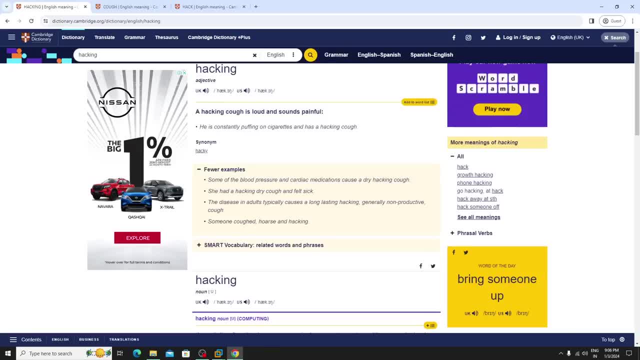 targeting six characters, right. assume that here there is a constantly. is there in constantly? how many characters are there? oh sorry, how many alphabets are there? simple, there is a, c, o, n, d, uh. six, seven, eight, nine, right, there are ten characters here. assume that, if i type, 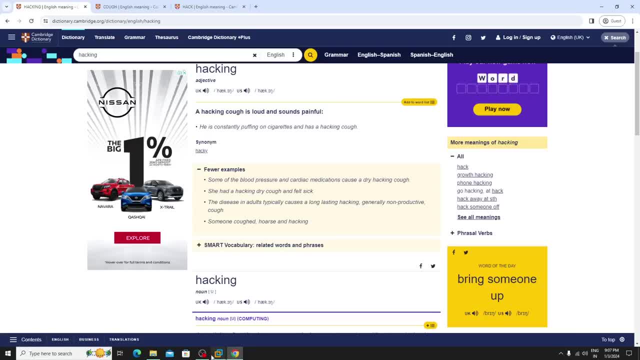 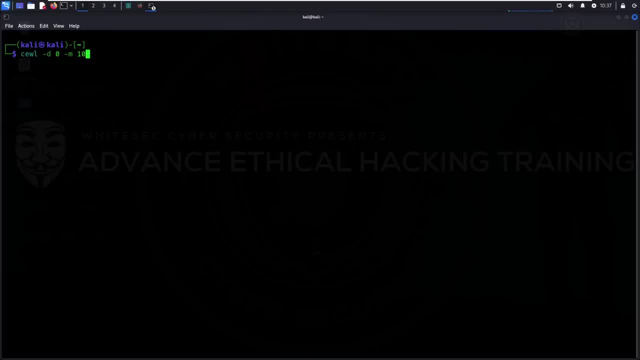 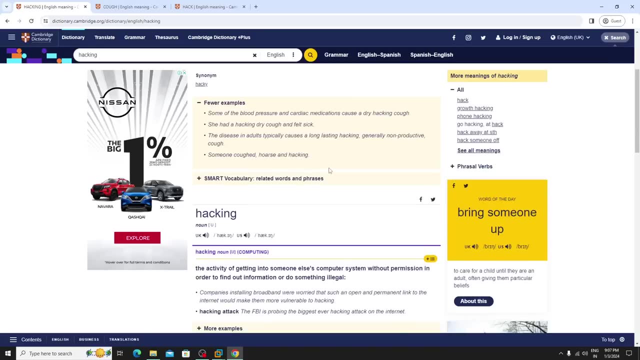 ten here, then it will only gather those keywords which, uh, which? having ten characters? okay, this is a thing. assume that there is a eight. mostly the password will be around eight characters, something like that. at that time we need to choose like that, okay, like we will select eight there, okay. 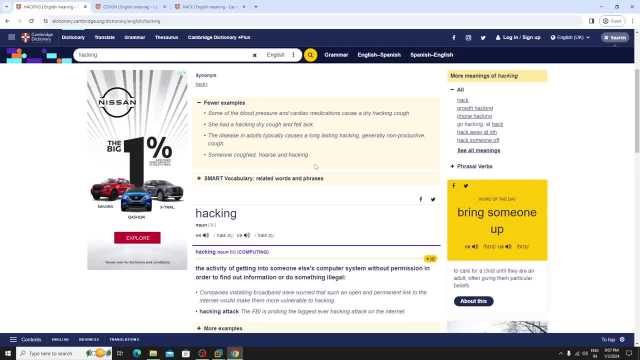 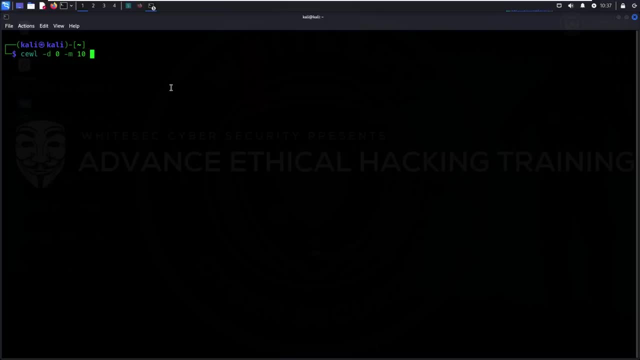 mostly you will target according to username. the thing. okay. this things plays a very important role during fuzzing. okay, now, here let me use 10 characters and then you need to type url. just you paste url and paste it url there. so here i just generated, you no need to add dash here. type like this instead of adding url: okay. 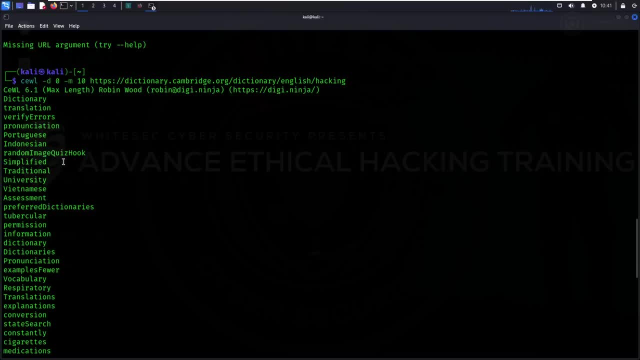 now it generated the this, the keywords: okay, which, having 10 characters, sometimes you will see more than 10 characters here, one, nine, ten, okay, so mostly you guys will see the 10 characters here. assume that mostly there are duplicates here. okay, uh, you see, the thing is it doesn't uh, doesn't say okay. 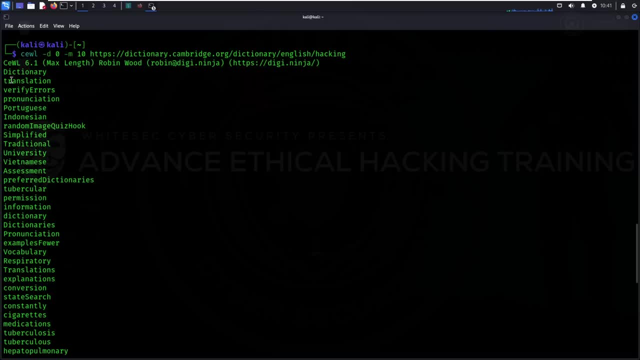 like we can only uh, we just need to copy this like this, and we need to get one text file and we need. but in quill there is also one option. if you type uh, fill here, so let's say you type, you can copy this one. it is a right option, is. 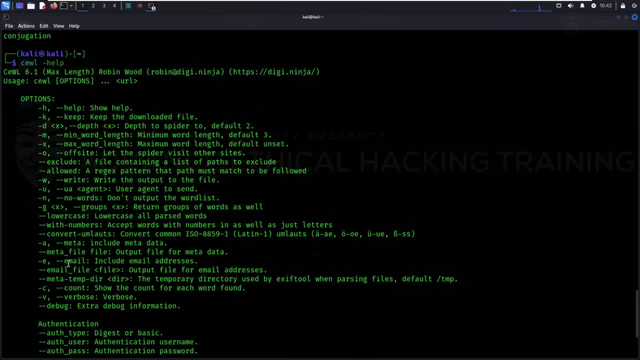 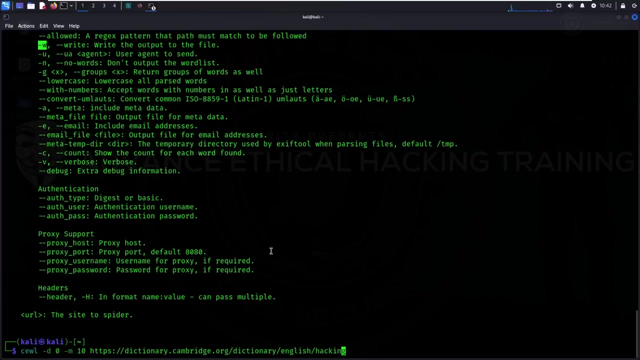 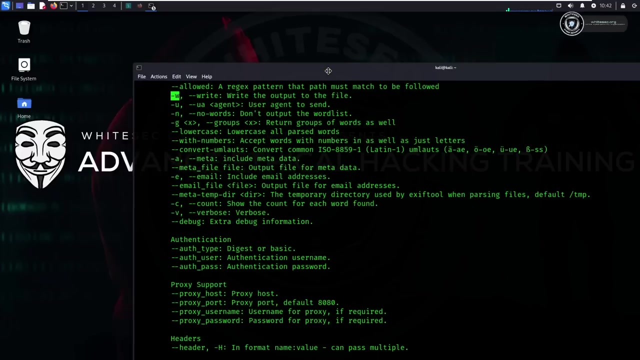 you can also gather email addresses from urls as well. uh, i'm gonna cover that right here. it is dash w- write the output to the file. okay, let me how to do that. just give space and just type here: dash w and give any file name. okay, let me do one thing. let me save this file on my desktop. 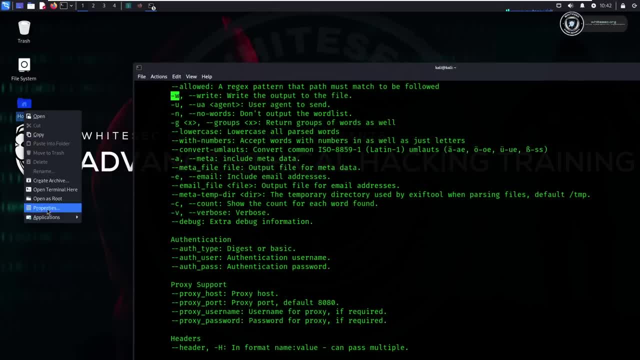 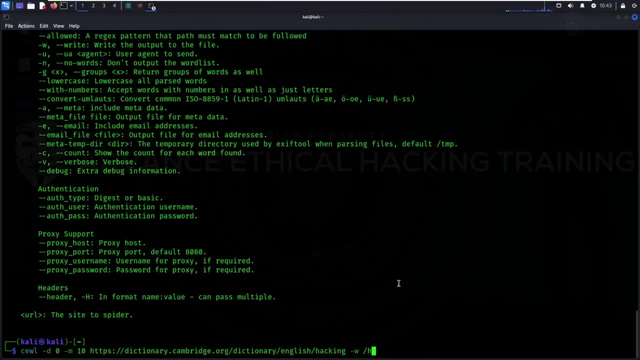 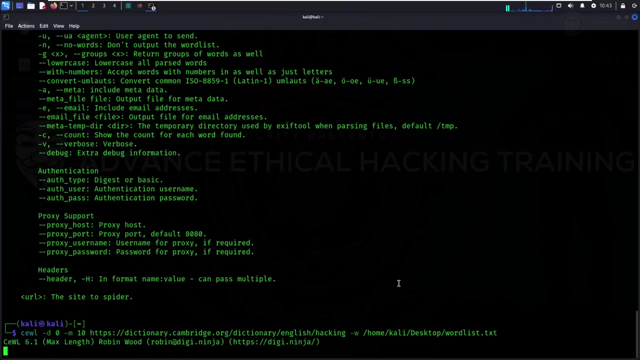 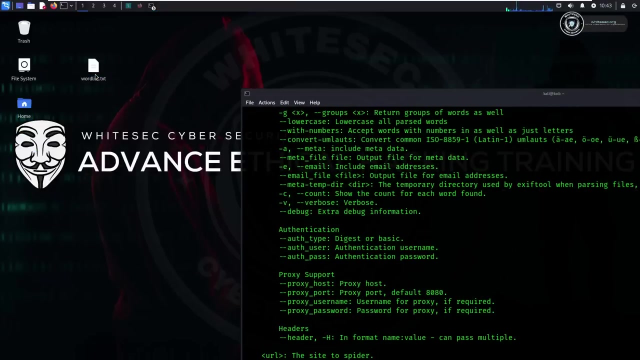 the location is home forward slash. like this: okay, home forward slash, kali forward slash desktop. okay, in desktop, let me create one file with the name of word list, not txt. okay, like this: now it will create one word list on my desktop here. it is right, open this. here you can able to see the word list. okay, now. 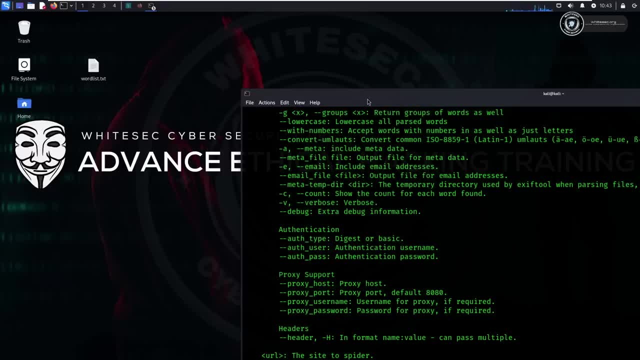 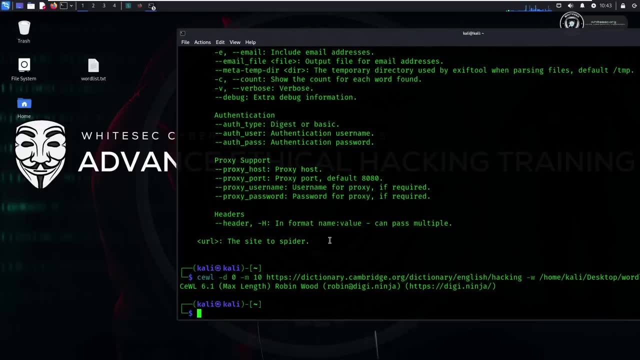 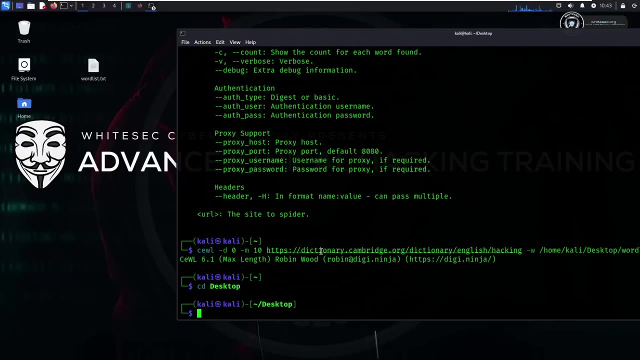 you want to see how many characters in this word list simple. you can also do like this. let me navigate to desktop, cd desktop, and first of all let me show you how to duplicate it. it is a one tool with the name of sort. by using sort, you can able to do remove the duplicates from this. 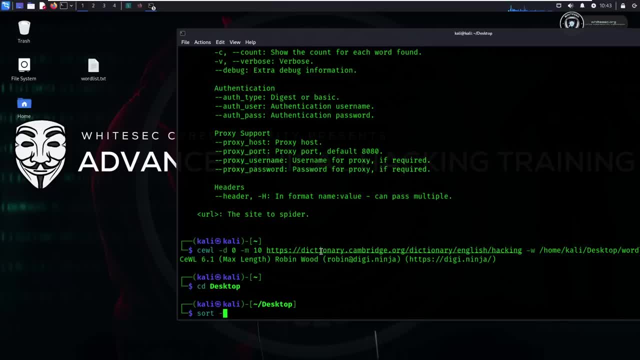 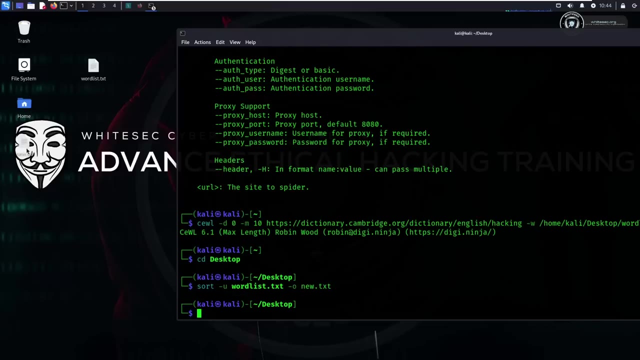 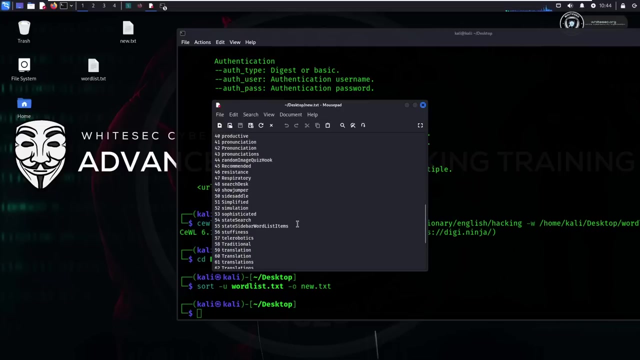 file. okay, just type here: dash u and just uh, type the file name. okay, now let me show the new output here with the name of new dot txt. okay, this is how you can able to remove duplicates from the word list. okay, let's hope you guys get it. now how to uh. 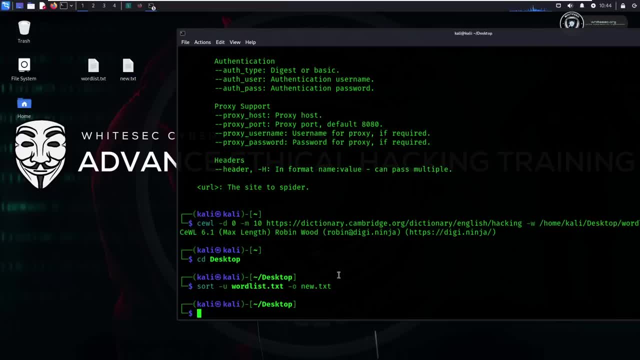 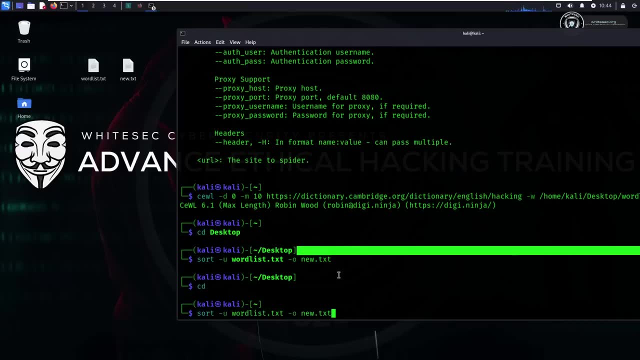 how to extract the email address. how to extract the email address: any page, okay. there is also one excellent feature in it: simple. what you need to do means just type will. okay, just type dash, dash email, right. then provide any website, your address here, right, url website. let me just show you how to to do this. all right here. just drag this one from here. 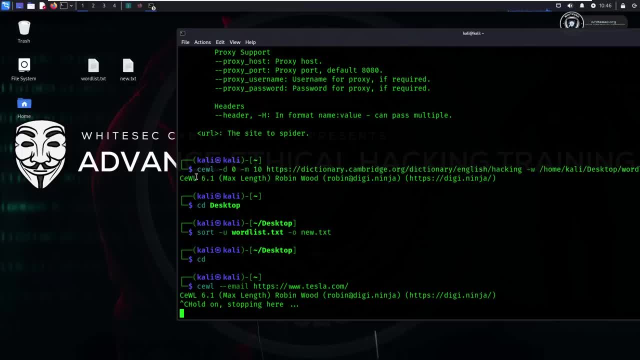 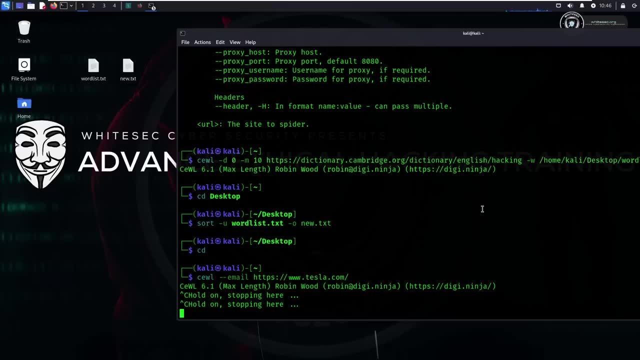 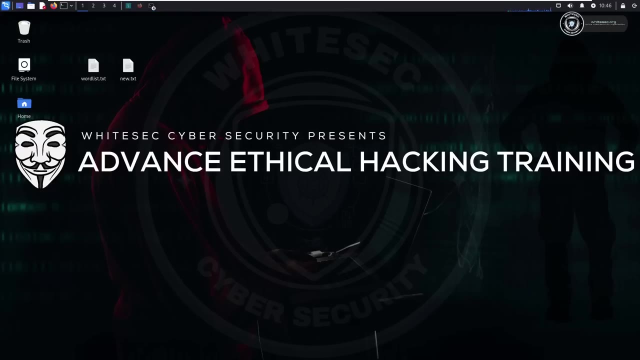 drive it during time, when it's take some time, and just type quill, dash d, zero and specify the page url and able to dump. don't want to dump it? this is how you can also dump the email address. now in this class, we are learning how we can able to generate. 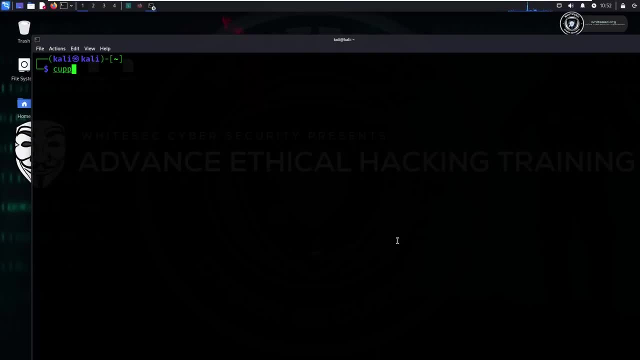 the word list according to your target right. assume that you got the username okay, or you got any kind of wi-fi network. you just hacked one wi-fi network. how you can able to generate the word list to crack that kind of hashes. this is the thing. now, here, the cup is also. 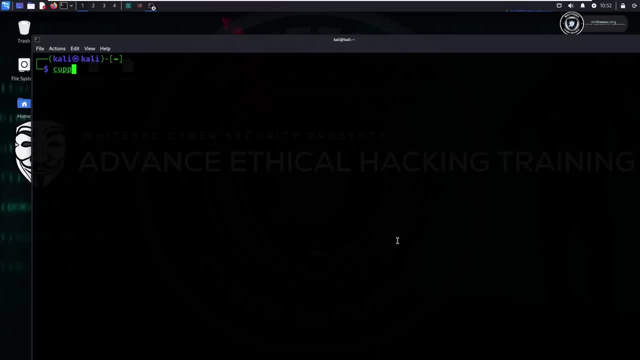 an excellent tool. by using this, you can able to generate the word list according to your target. okay, by providing his phone number, by providing his data, but by providing his kind of names, okay. this is a thing like if you watch mr robot series, you will get it okay. 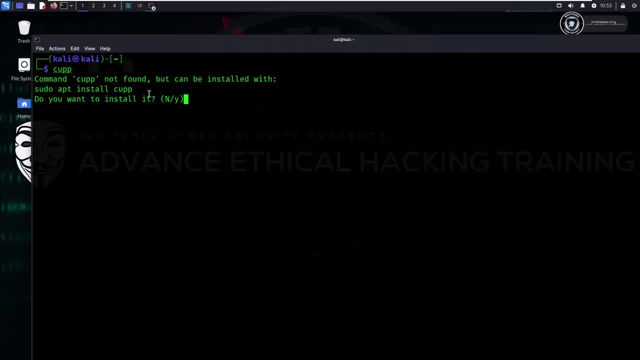 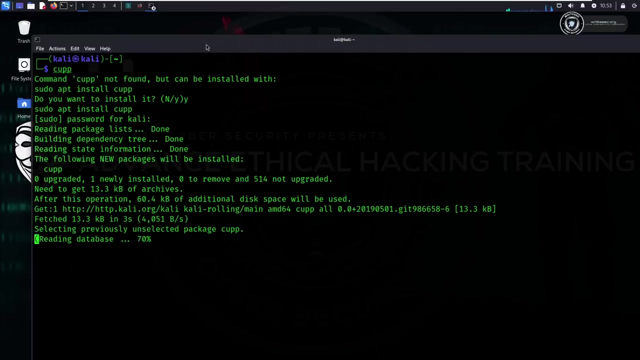 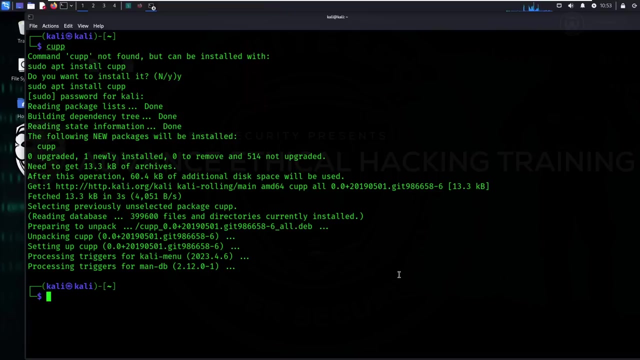 okay, now just type here cup. in my case the cup is not installed in macaulay linux, so the simple thing is let me install it. just type y there. so here it is now simple. just type here cup. here you can able to generate the word list. 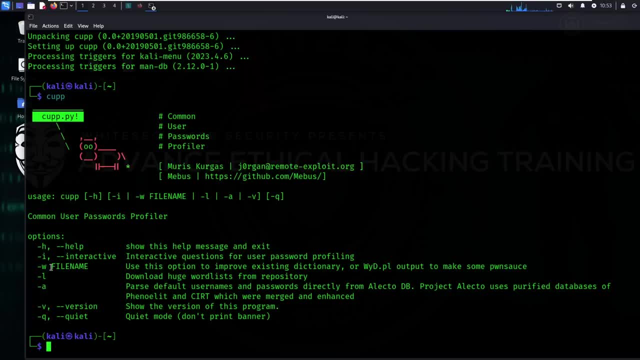 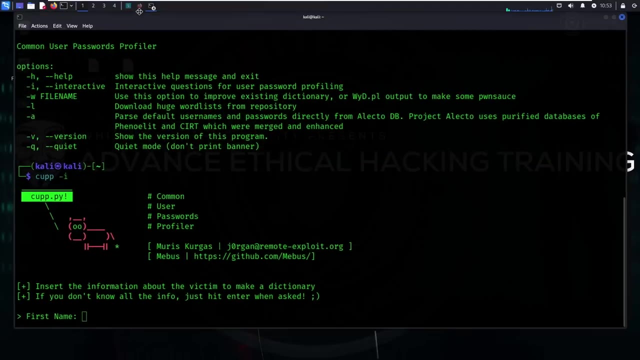 okay, so you can able to see. dash h is here now simple. you no need to go with a dash h or something like that. just type here: cup dash i to interact. you okay now here. from here, the game will start here. you need assume that if you are generating the word list according to your 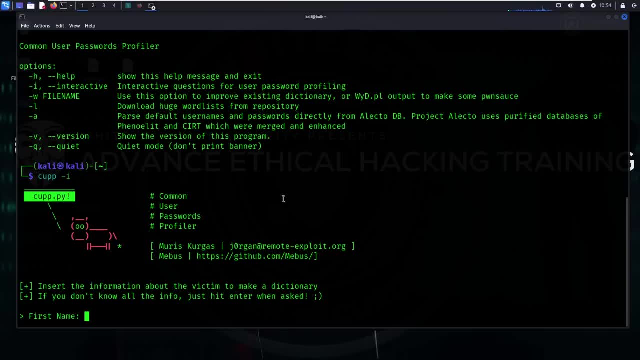 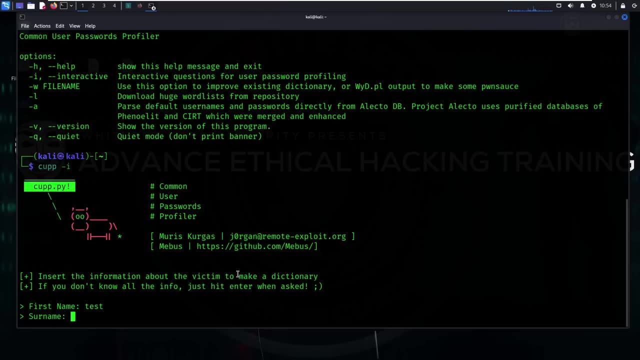 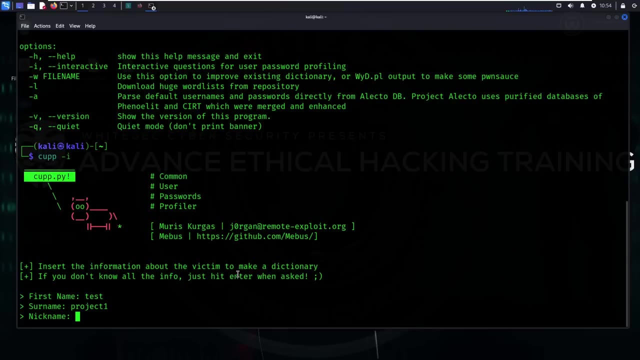 target. you have his username, at that time you can type his username here. okay, something. let me type here test as a username. and there is also a surname. let me type here project one and nickname, if you have, if you know his, your target nickname, then just add. 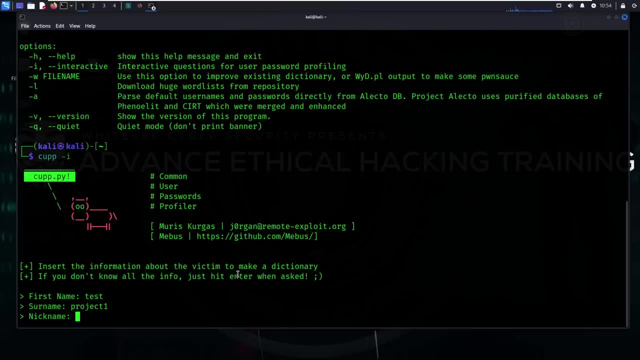 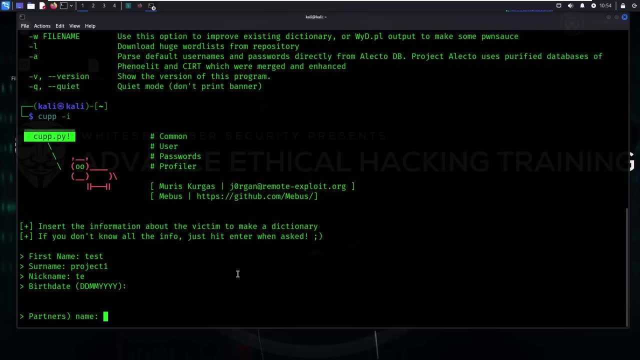 his nickname as well, like a t. now, if you have that date of birth, then add it. if you don't have, just type enter. that's it. it will ignore it. if you have his partner name at that time, you can also add his partner name as well, mostly in this cases in partner's name. what will happen is: 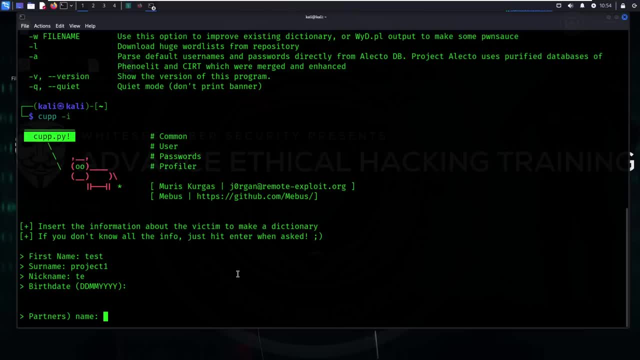 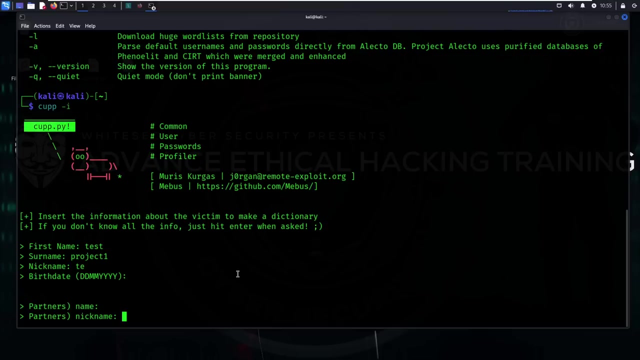 they use starting letters of their partner names. okay, like starting letters means assume that like starting word. assume that john is here. here mostly they use j or something kind of letters. okay, starting letters. it's totally depend upon you how you think right now. just it will ask for. 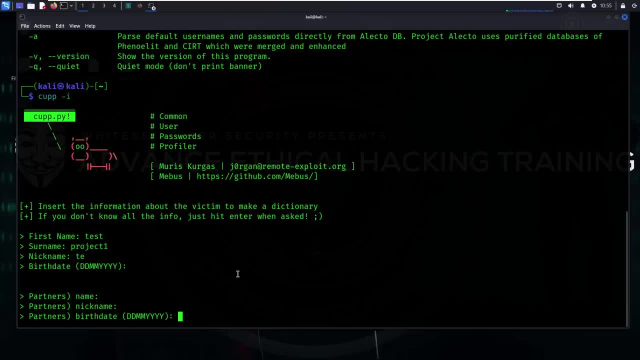 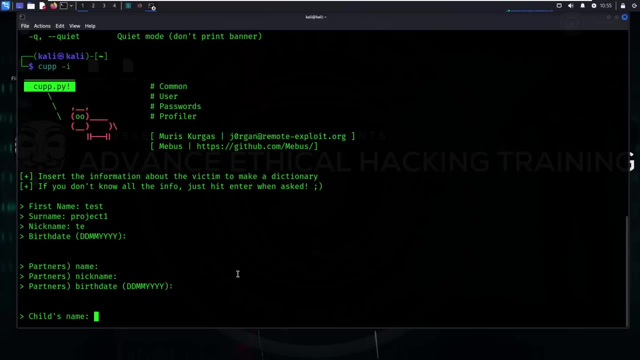 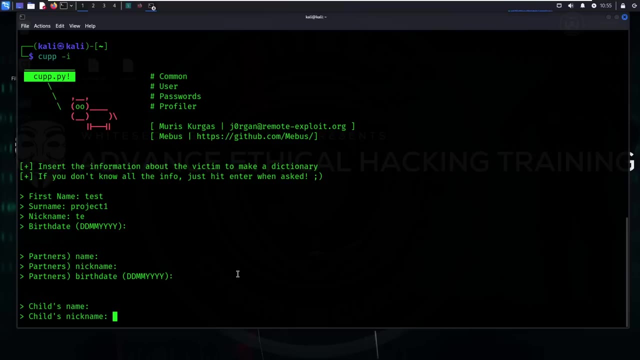 the partner nickname as well. there is a partner date of birth. what is this heard? are the name, number of the child names okay? so this is important. ode the child names is ok. this is also play one important role: child link, a nickname. if you add this following things here, then it will generate excellent word list for you. okay, mostly it will. 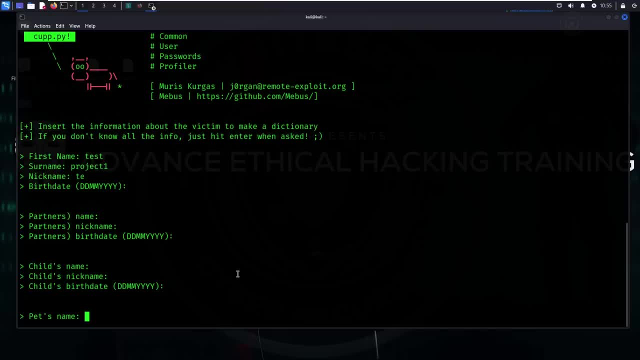 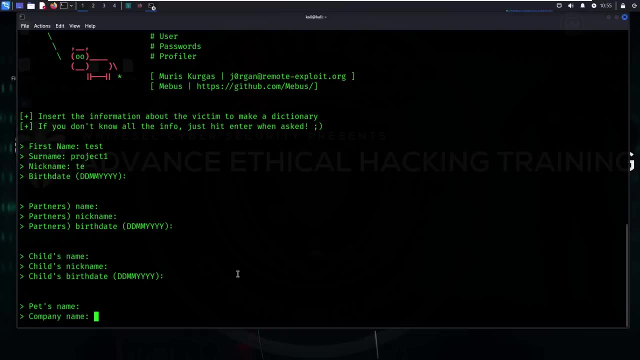 work. okay, this is the thing people in real world pen testing rock you dot p? x? u. is there right? sometimes it won't work. this is also one important thing. there is a default word: most of the time you you know will not be, won't be made. this is the kind of change people will get- what we got, for an example. 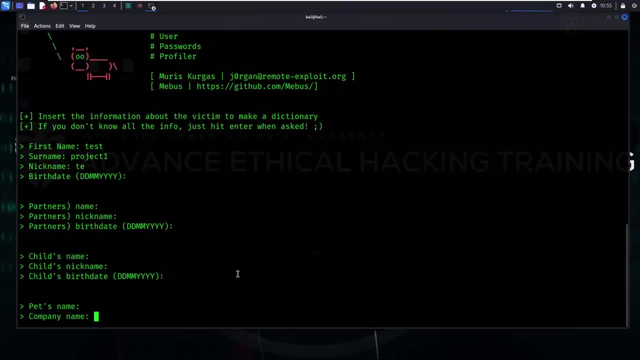 there is a default word list user, which is rockutxt. if you watch our ethical hacking training there- we just covered about that word list. okay, in wi-fi hacking training also, you will see that thing, but sometimes it won't work. this is also one important thing at that time. 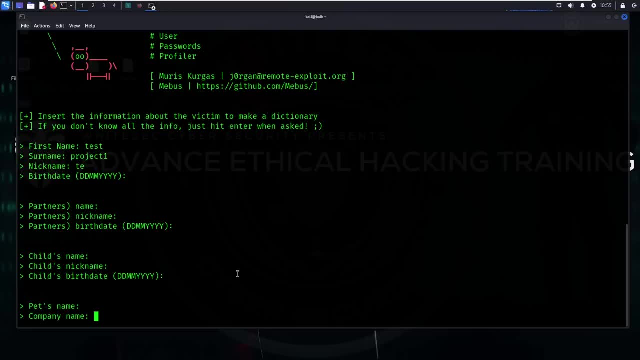 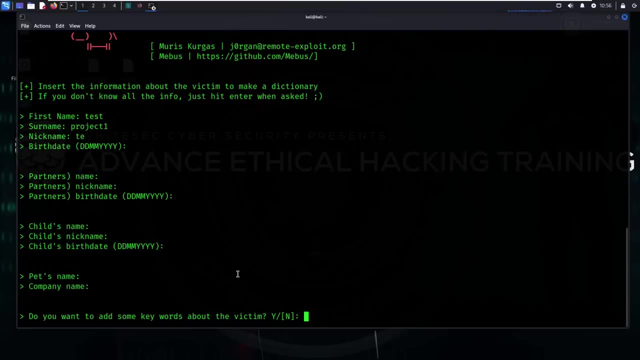 we will generate our own word list by using these techniques. now, do you want to add some keywords? assume that. if you want to add some keywords about your victim, okay, assume that here it doesn't ask for those keywords. if you want to add more than from here, you can able to add it right, simple. 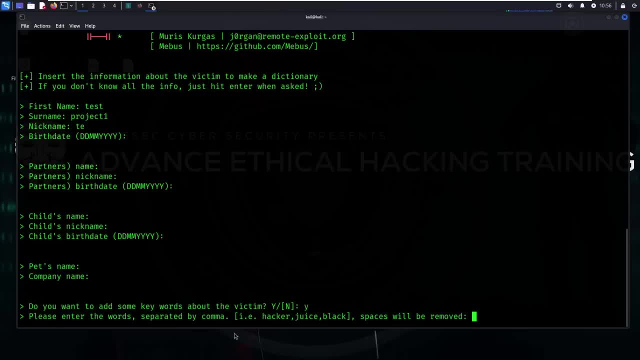 just type here a why there and just add it now. please enter the word separated by comma. so a simple like this: okay, test forward slash, okay, and there is a offa like like this one: okay, if you want to add, then you can add it now. do you want to add special characters of words as? 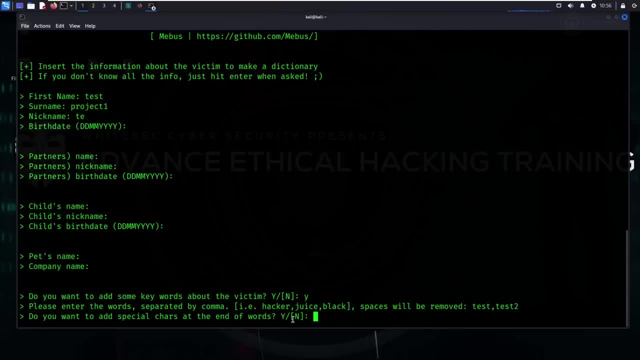 you want to add special characters of words, as you that mostly see websites require. assume that if you are creating a user account in one website- mostly the websites- what they do- they ask for the special characters in the password. okay, simple, you can also add the special characters here. you want to add some random numbers at the end of the word? 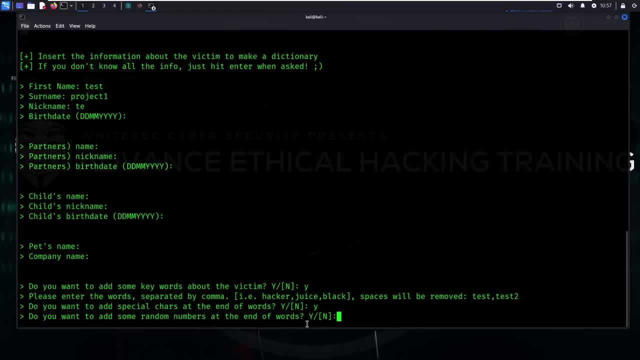 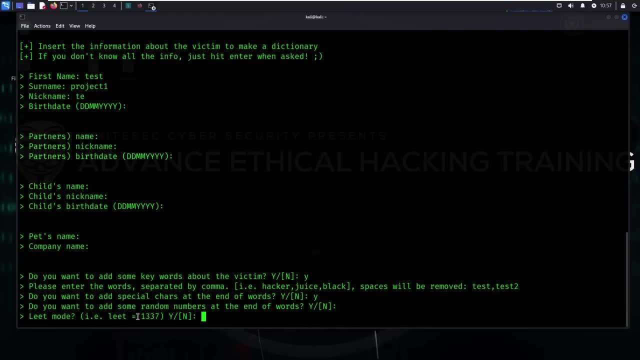 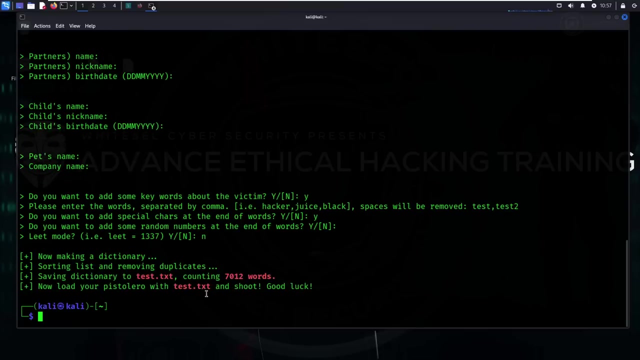 if you want to add a random characters, then you can also add it. okay, i don't want to add lead mode, like it doesn't require lead mode here. so here the the word list has been created, see. please enter the word list separated by comma. here you can also use the phone numbers as well. okay, mostly. 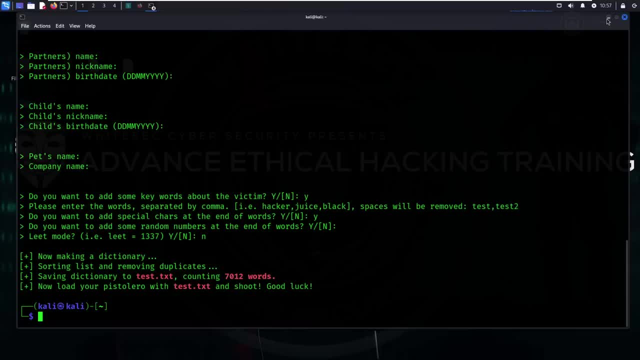 there is one scenario, uh like say years back: okay, mostly people are using their phone numbers in instagram password. okay, like a assume that if you want to log in someone instagram, mostly at that time people use their phone numbers here. simply here, you can also add the numbers as well. okay, the phone number of your. 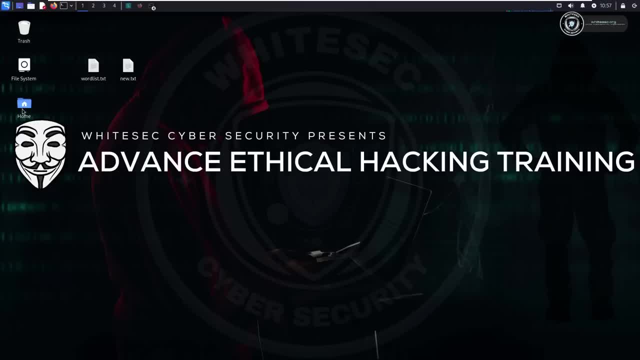 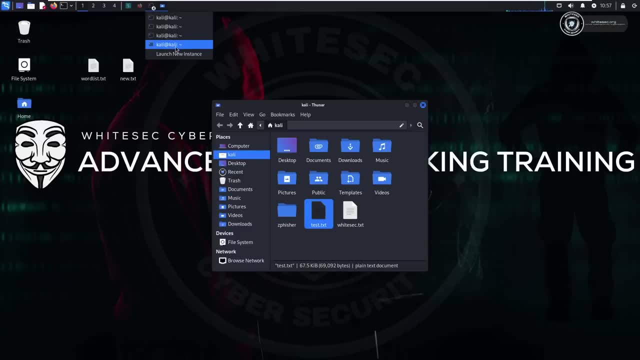 target, it will work, but you need a kind of thinking there. okay, here you can able to see that is a word list which is created with the name of testtxt. here it is. if i open this one, this is the stitches wordlist through text panel. if i take one word下, Paste it to Everyי Wordlist, Then hit Enter, then click the headerさー. 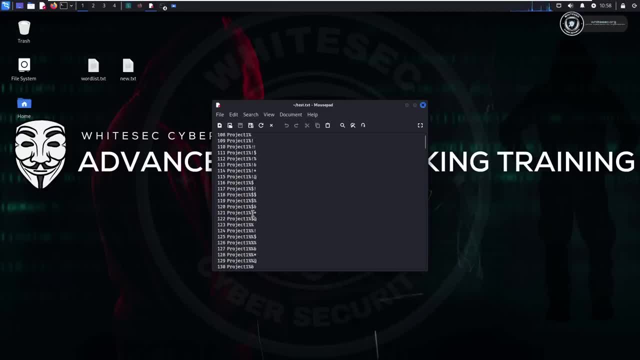 if i open this one, here it is. if i open this one, this is a Wordlist- then i take one word of the name of a specific place in this page. This is how the file look like. okay, so excellent. just think and create your own word list, okay. 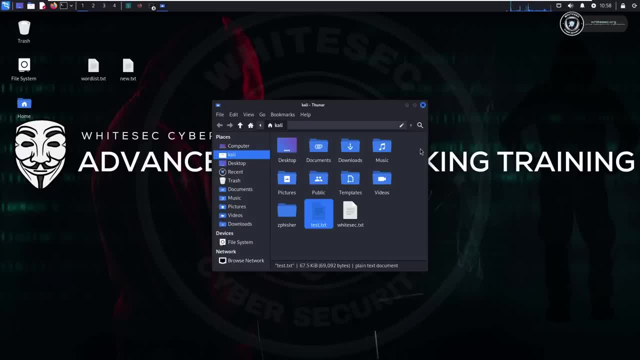 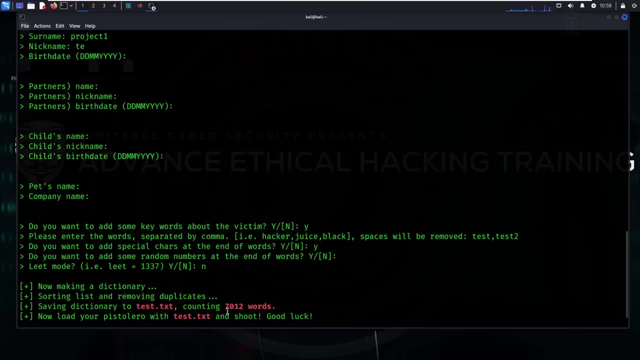 If you add date of birth also, it will play a very important role. if you add the university name from where they just qualify, it will work. okay, this is a thing In real world, what we do. basically, we won't generate 7200 words here or something like. 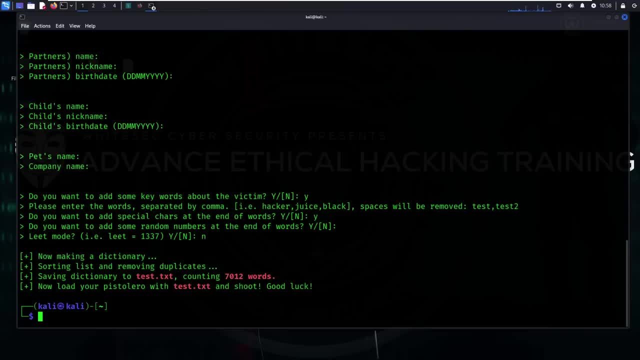 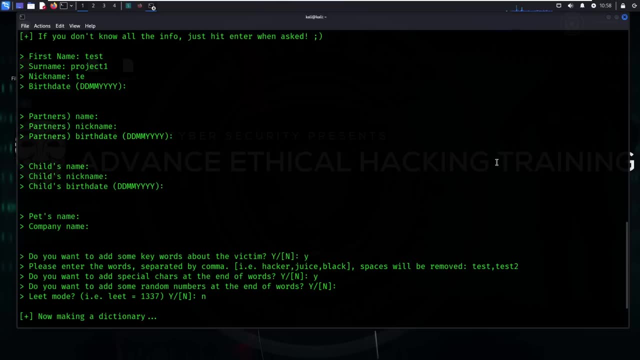 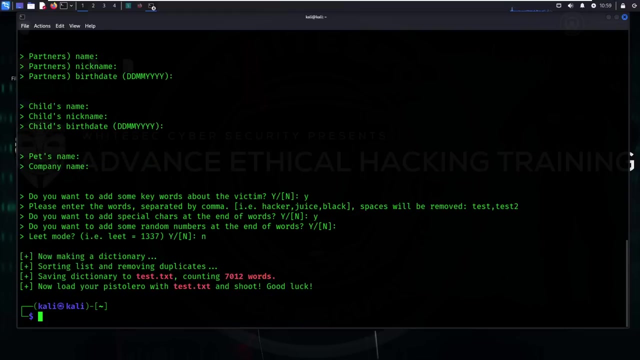 that we will generate in a huge. okay, the file size will around might be. in last case, I just generated, not by using some different tools. okay, I just generate almost like 2 GB of word list. okay, this is a thing. the size of the file will be 2 GB. yes, it will. 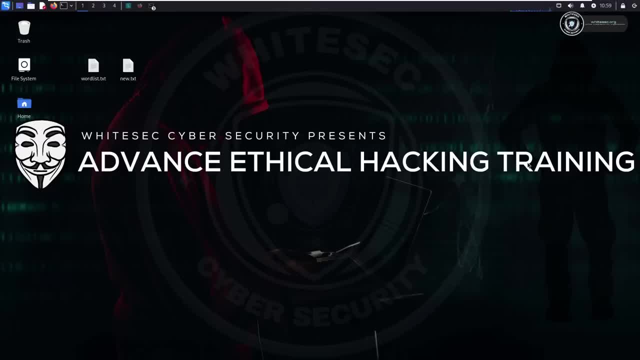 work. okay. If it doesn't work, then I am gonna generate a lot of words, So this is how it works, So I am gonna create a new one. I am gonna search for in data bleachers. there are some private things which we subscribe. 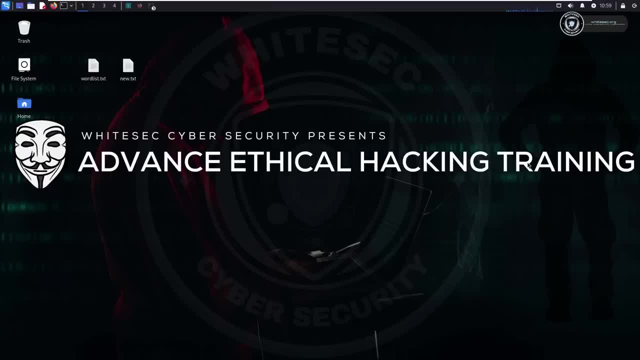 for it. there we will get those things. okay, this is also one way. see, once you jump in pentest string, once you jump in redcaping, what will happen means you need to go for some premium things as well. okay, like you need to go for some kind of subscriptions. 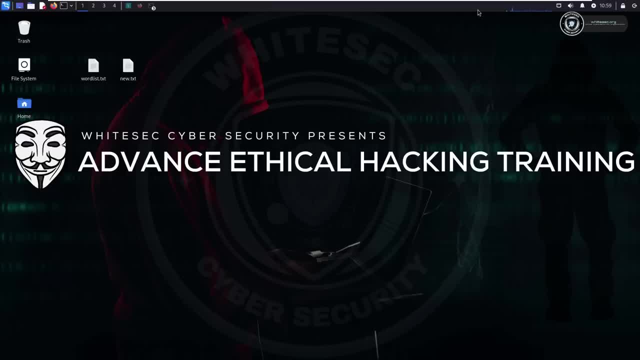 this kind of things, because always these things will take a time. okay, your client, in your, in your case, assume that you got a project at that time. the timeline is three months. okay, it won't work like that. okay, like, assume that, assume that you won't get any kind. 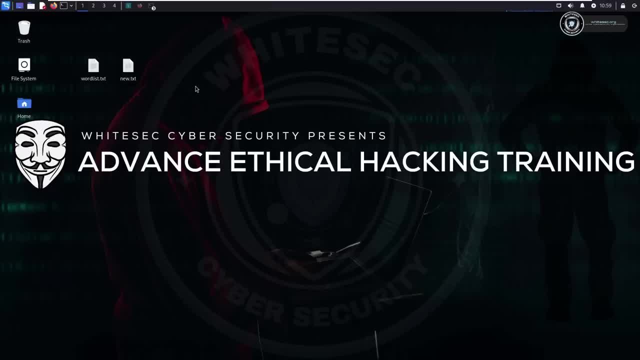 of password. assume that you can't able to gather kind of much information about your target. it will a time consuming process. okay, this is the thing at the time. if you, if you are getting a good budget, just just try to go with a premium things there. okay, i hope you guys get it. thank you, have a nice. 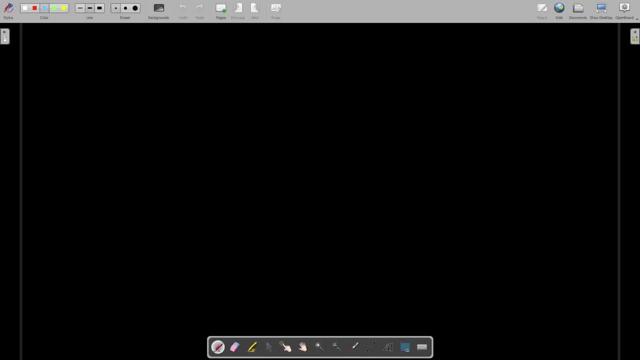 now, in this classes, we are learning about faces of hacking, which is very important. without learning faces of hacking, you can't perform a successful attack. okay, like you can't able to figure out, like, from where you need to start. okay, once you got the ip, once you got the domain, what? 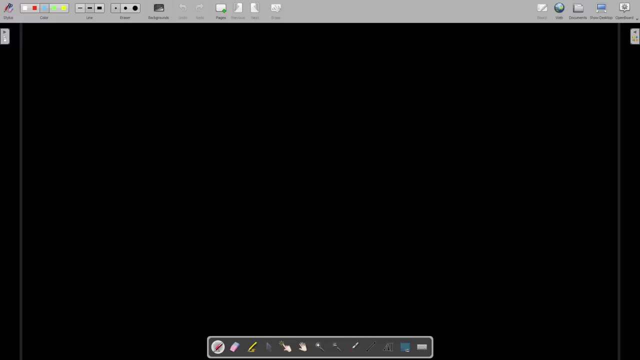 you need to do. okay, this is the thing here. okay, so, first of all, we will start with reconnaissance. this is the rule. basically, i didn't created it. okay, this is. this is a thing which you need to remember. it's a kind of keywords in python. okay, if you? 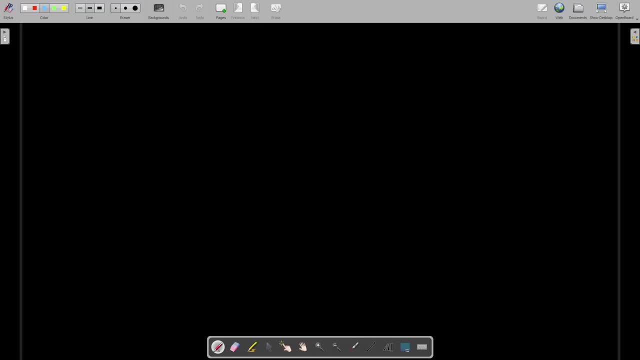 know python, then keywords play a very important role there. okay, this is kind of keyword here in python also, the keyword will update. okay, they, they add a keyword z time to time. okay, if, if python will get updated, the keywords will added there. okay, the same thing here. 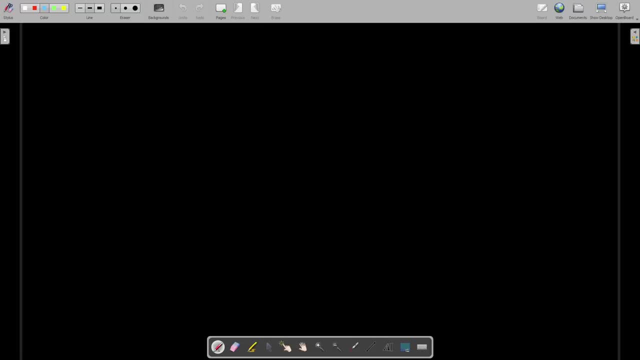 okay. but let me tell you, in pen testing, in red teaming, okay, the faces will be different, okay, we will in here in pen testing what we say faces in red teaming. we will say as a tactics, okay, this is a thing which you need to remember. see, pen testing is a beginner thing. let me tell you beginner thing. 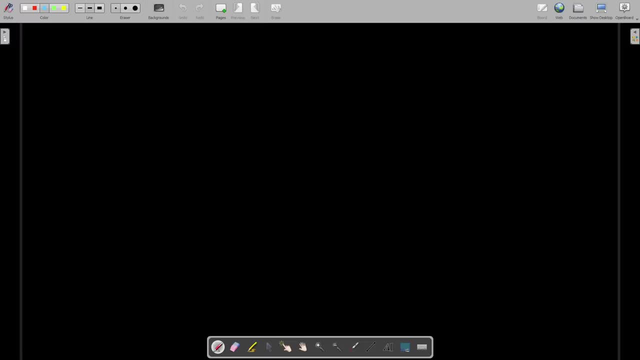 means what? uh, just assume that if you, if you want to learn how the tools will work, if you want to learn, then pen testing is there. but if you want to learn a complete attacker point of view, then red teaming is there. this is the thing which you need to remember. see here, red teamer is a nothing but. 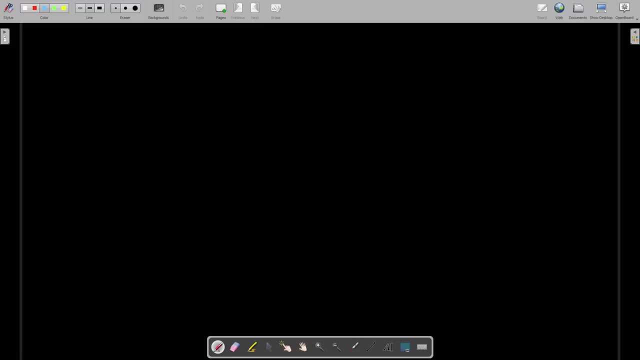 uh, you can also say it as a red teamer- is a guy who is a black hat hacker in his own company. just assume this is a simple scenario, but he, even he performed the black hat hacking there. uh, he, uh. he will give a proper report there. okay, but uh, why i am saying black hat hacker here in? 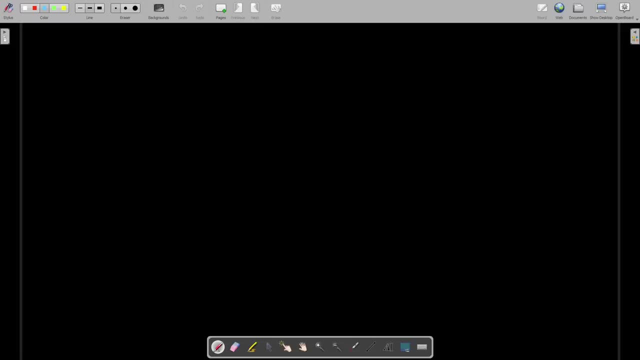 uh as a red teamer, because mostly the employees won't know that there is a red teaming, is going there. okay, like uh, somebody is trying to hack them, he, they won't get it. okay, because mostly red-teaming, uh, we conduct rectifying. because because to uh to check the technology, uh, to check the vulnerabilities here, to check the. 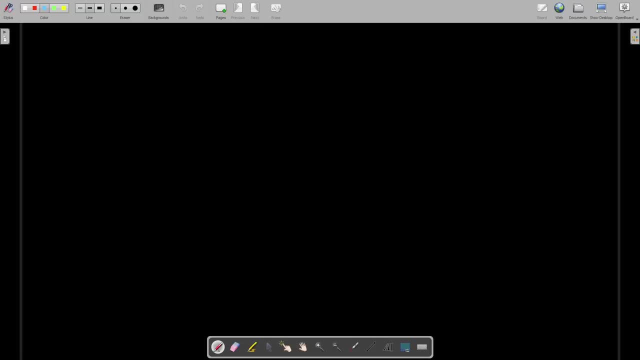 employees having the proper cyber security knowledge or not? okay, this is why we we perform the red teaming. the simple thing is: it will make your company more secure. red-teaming- okay. i am talking about red-teaming because the thing is, even if you not play with red teaming, teaming okay. can't do that. you can calculate the same for veg suuggle at least 20 times to see what you are dealing with. every two team. because the thing is you drums and red teaming and baby softening rs too and makes the red teaming smarter. the sub γ 170 teamung- um, they are the psychic better teamer teaming. okay, uh, the. 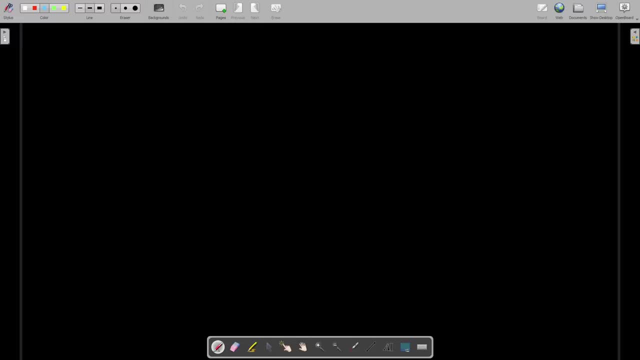 a complete phases, okay, uh, which black hat hacker perform? okay, we, we conduct a complete uh things there. okay, which black hat hacker do? right, this is a thing now. just just forget this. also just focus on the faces, because we are learning here, pen testing, right. so in pen testing or in hacking, 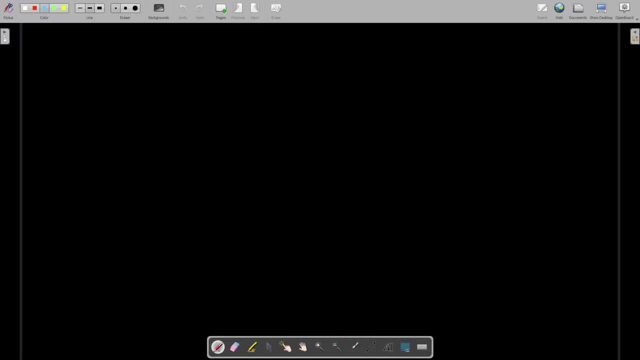 there are faces which you need to focus. without without learning this, without knowing about these faces, you can't even focus on red teaming as well. this is a thing. see faces, the faces of hacking or faces of prime testing. first phase is reconnaissance. okay, you can also say it as a recon, or you can. 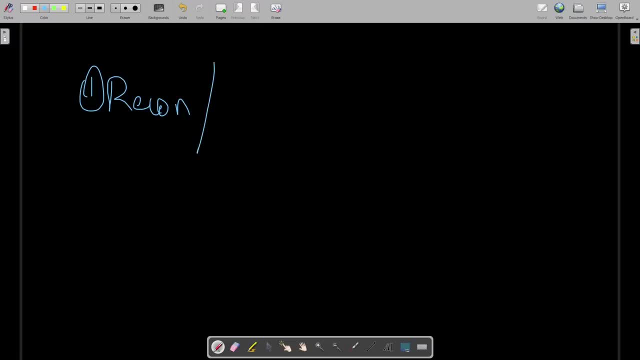 also say it as a footprinting: if you watch our ethical hacking training, then there, i just told you about these things. okay, reconnaissance is a first step. okay, you are gathering information about your target here. okay, if you don't gather information about your, your data, you don't gather. 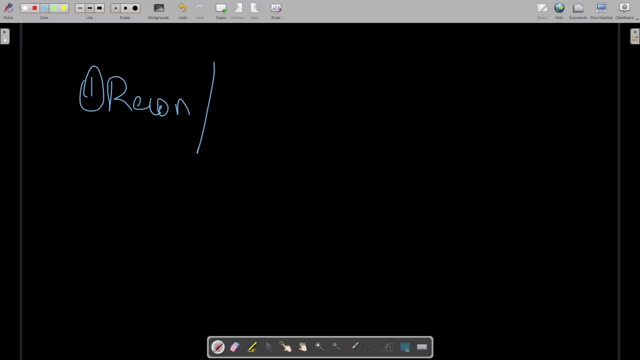 information about and, in circumstances, after a time extra, more resources shining, hence the Henna target. then you can't able to attack him. okay, this is the thing. basically, before targeting any company, we will study about that company, okay, like how many employees are there, who is the head of? 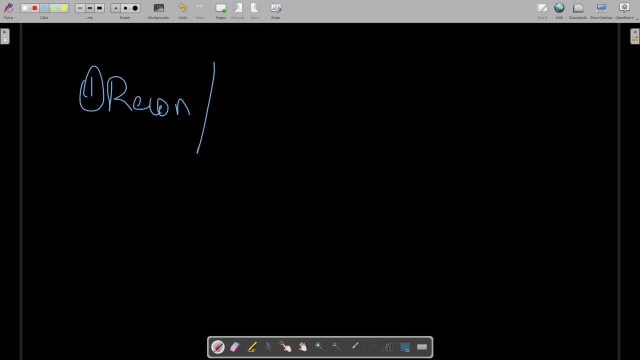 that marketing team? okay, who, uh, who is, uh, hr there? these things we will now. the second thing is what scanning see? scanning also very important. without, without following this phases, you can't able to achieve your goal. okay, this is the thing. scanning see. assume that during reconnaissance process, 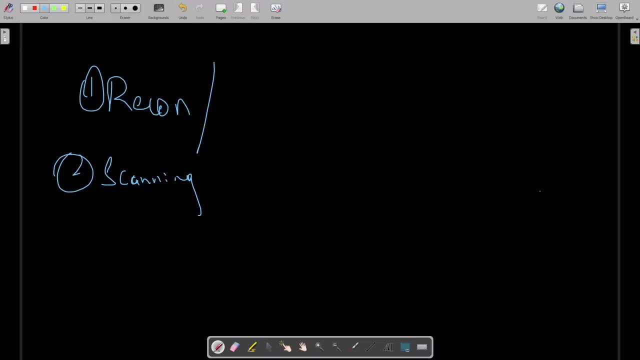 you got some subdomains, some ip addresses there. simply you perform a scanning on it, such as vulnerability scanning. okay, just take this one as example: verna, uh, verna, uh. sorry man, let me vulnerability scanning. like, by using some tools, you will perform vulnerability scanning on it, such as: uh, there is a nmap, is there? okay, there is an ss is. 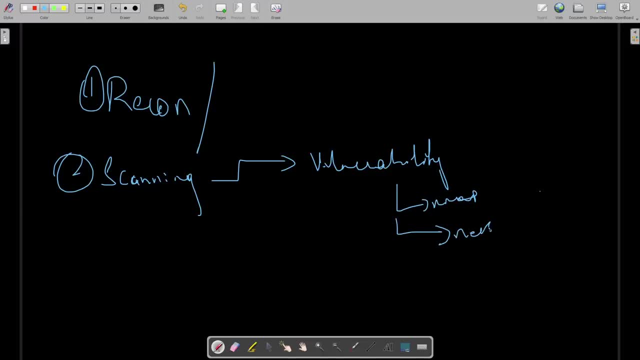 there. mostly i use nss. okay, there is an expose. is there? okay, there is a open was. is there? okay? these are the tools. by using this, you can able to perform scanning, which we uh did by using these tools are very advanced. okay, like uh, it will do a huge work for you. 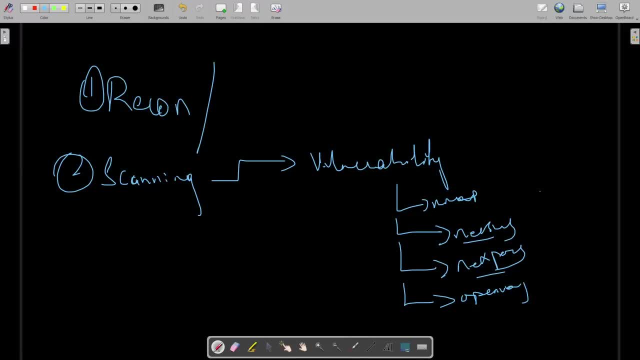 but still, if the client approach you to do manual pentesting, at that time you need to go with manual. this is the thing which you need to remember. sometimes, these tools will give you a false, positive, positives right. so this is the thing. so that's why what you need to do, uh, if, if it's 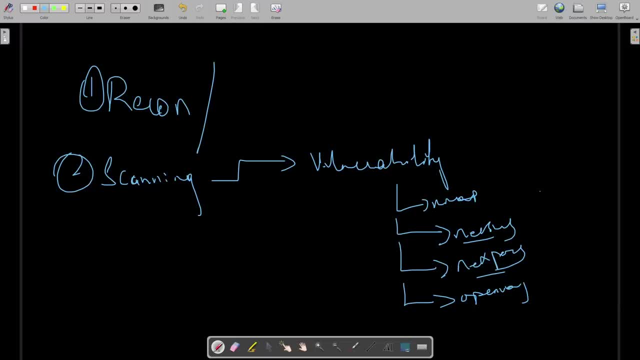 totally depend upon the client. okay, this is the thing. now, this is the thing: scanning, like, uh, knowing their uh port, uh, which ports are there? okay, which we just learned, this is the thing, right. so the third thing is, after scanning, like gaining access. assume that you got some kind of 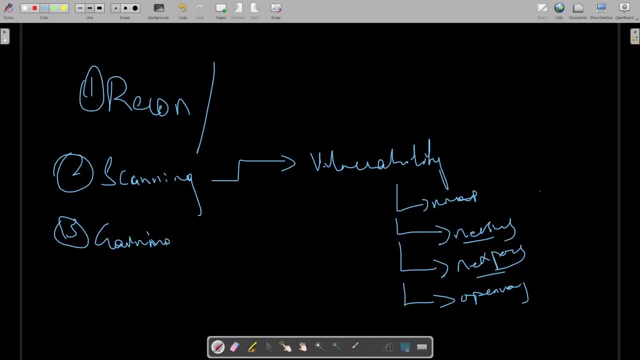 vulnerabilities in it. okay, we just found that some devices are vulnerable. gaining access to that vulnerabilities: this is the thing simple. let's take an example of eternal blue vulnerability. you just scan the ip, you go. you just got that. okay, this system is vulnerable. by using this vulnerability, we can able to control on that system. simple, gaining access to that uh system. 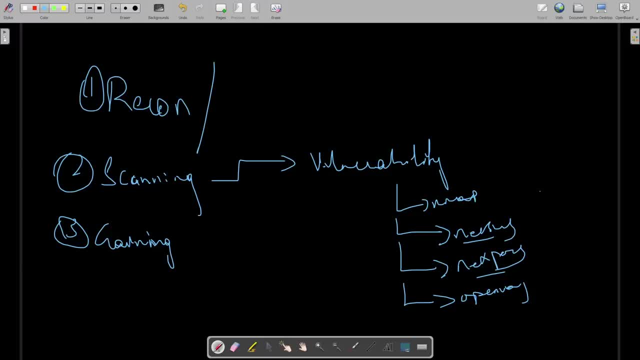 by using this vulnerable this. see, let me tell you, in pentesting or in hacking, the faces are very small, but if you jump in red teaming, then it's a huge man. okay, you need to remember this. like there is a uh, we say as a tactics: i just told you right, okay, so these are the kind of beginning, uh. 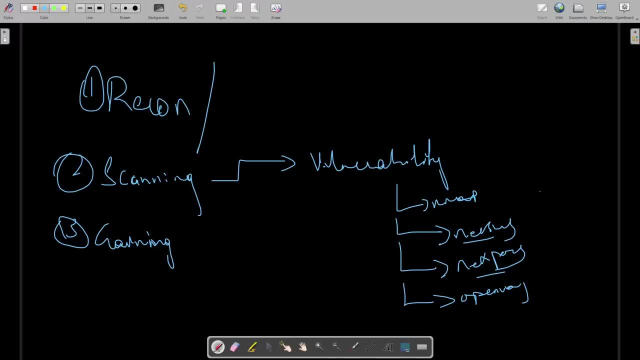 beginner things okay, which you need to remember. now there is a gaining access, then there is a maintaining access. you can also say it as a persistence, like see maintaining- i hope the spelling is right. okay, right, maintain em. okay, just let me write here: maintaining asses, okay, like after hacking the system. assume that you just hacked the system. 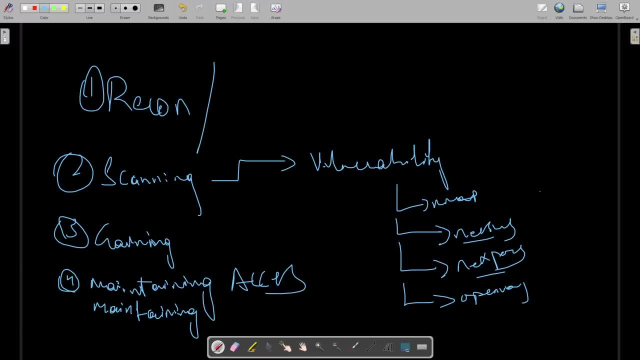 by using some vulnerabilities, sorry, by exploiting some vulnerabilities right now. assume that after some days, the- uh, the clients know that, okay, this system is vulnerable with this vulnerability, okay, let's patch it. after patching it, you, you lost the connection there. okay, you can't able to exploit it again. the simple thing is: 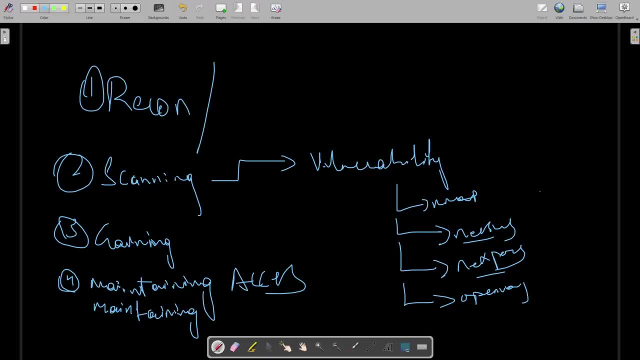 attacker. what you do is, after exploiting the system, he adds some kind of uh prescissions there. okay, so he, after patching the vulnerabilities, solves a vulnerability. also, he can able to connect with the system. okay, he can able to maintain the access in it. this is a thing. 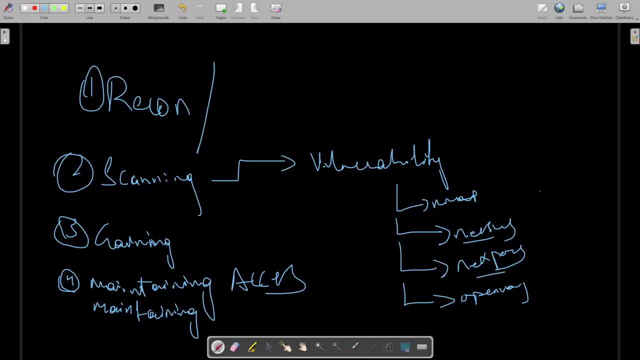 it's also known as a maintaining assets, or you can also say it as a persistence. okay, this is a thing. and the fifth one is clearing tracks. okay, clearing tracks now in windows penetration testing. we just learn about this thing about clearing tracks after hacking the system, after doing this all. 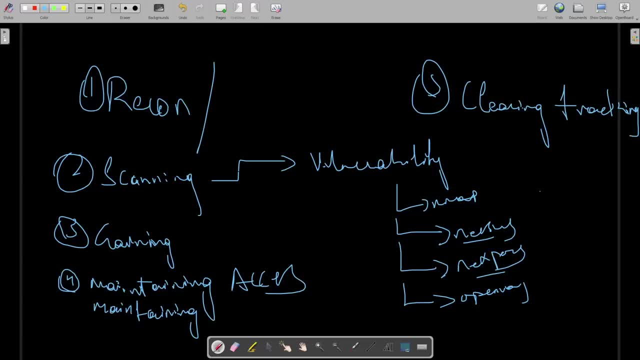 stuffs. see, you just perform hacking. right, you just exploited one vulnerability and there he they there. you just did a lot of stuffs. you just downloaded some kind of files. you just uploaded some kind of files in windows. okay, in that machine either. it's a windows on anything. okay, any machine. 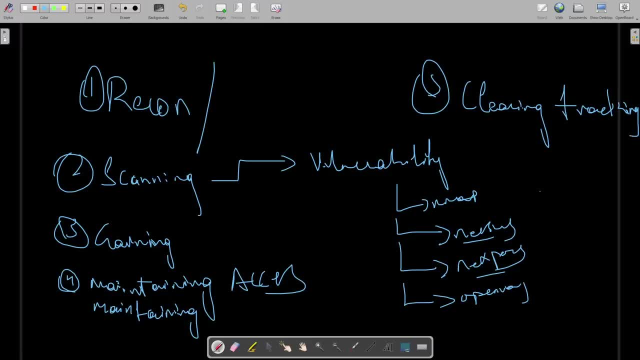 it doesn't matter like it's supply on every device. this is the thing. now. you just did a lot of stuff there. okay, let's take an example of windows machine. only because. why i'm taking the example of windows machine? because in this youtube channel, i just added a lot of tutorials related to 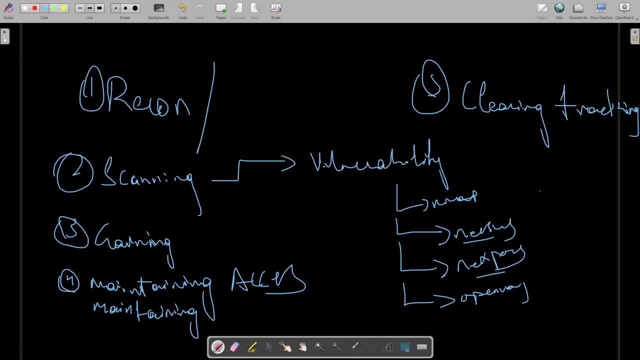 uh, windows, right, okay, just just take an example of windows, because there it is easy to understand the things. okay, assume that in that i exploited the windows machine there, i just uploaded some malicious stuffs- okay, malicious file- there. and also i just downloaded some victim data- my, my target data. 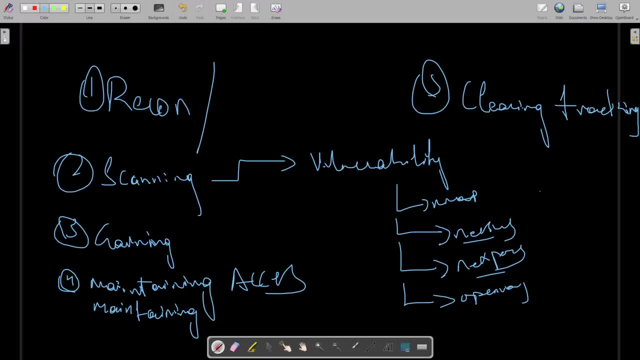 from his machine to my machine. okay, so this process, what i did there, like copying, okay, the things from my downloading, the things from my victim machine will be stored in the windows machine. okay, and then i just took the data and i just uploaded it to the windows machine. 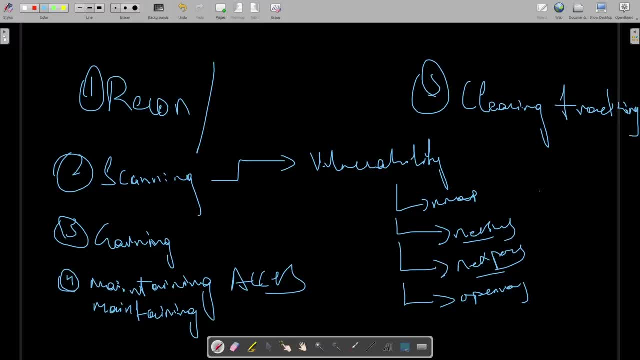 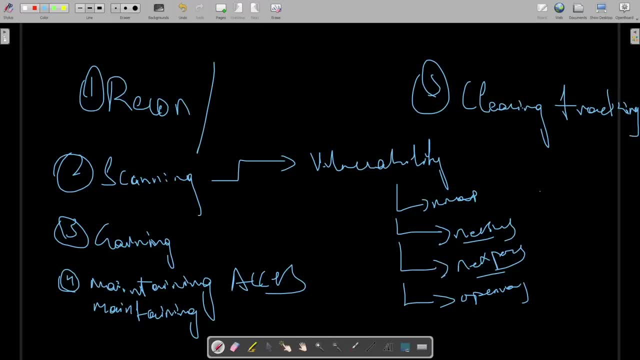 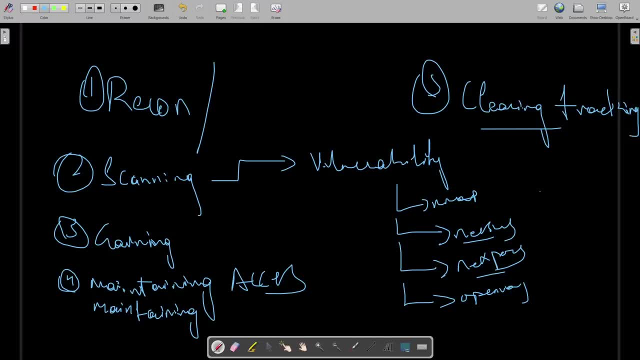 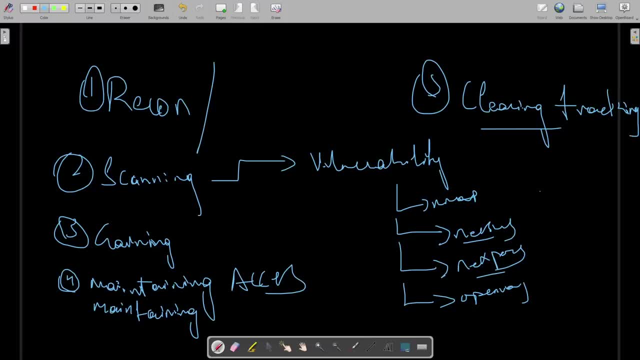 to implement these things. okay, physique, what is a physical pentesting here? let me explain you in a very easy way. seen, physical pentesting, what we'll do means we, we just check the physical things, such as locker: is there, okay? such as doors, such as cameras: are there? we check this security there. 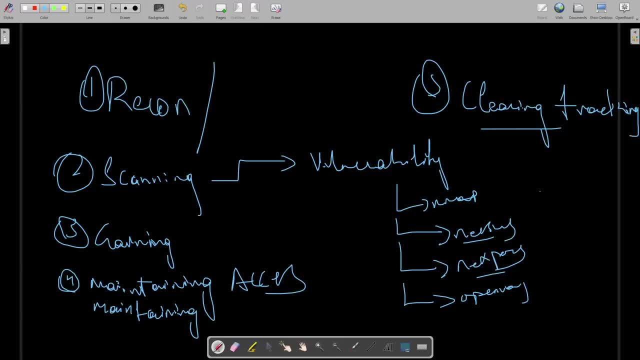 okay, like we will test those securities like fingerprint, this kind of biometric, okay. so here there also we, we, we follow this thing. okay, like clearing tracks. okay, everywhere you need, you will focus these things. okay, you will see these things in hacking, in pentesting field or in hacking field. 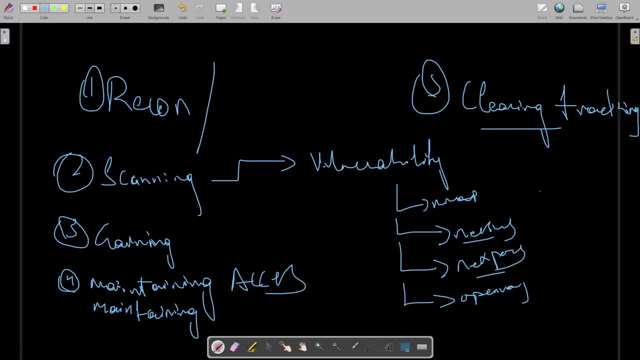 okay, these are the phases, which is very important, which you need to remember. just remember this thing: first one is what reconnaissance? second one is what scanning. third one is gaining assets- okay, gaining- sorry, let me write here, gaining assets. and fourth one is maintaining assets- okay. and fifth one is what clearing tracks? this is the thing which you need to remember. 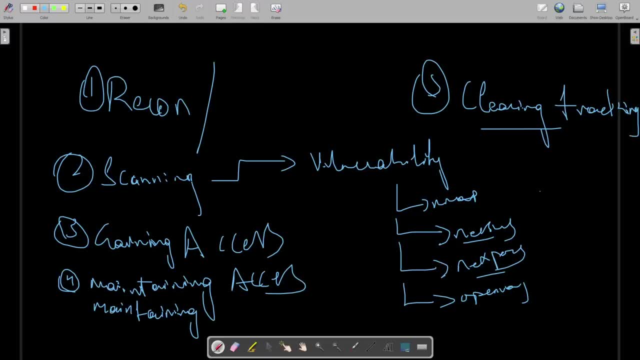 see the what's. the keywords are very easy. if you, if you know basic hacking, if you watch our ethical hacking training, then you no need any kind of definition for it. if you see the keyword, then you will get it what it is right. so hope you guys get it right. in the next classes we will start our 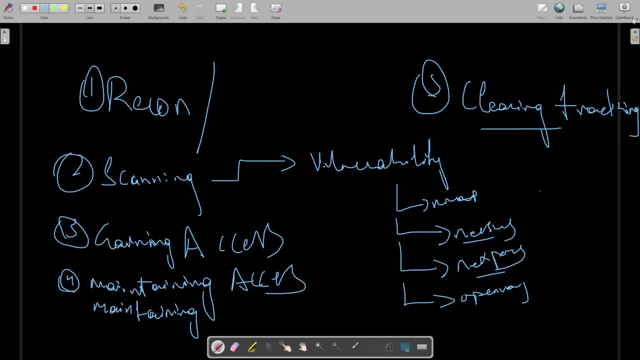 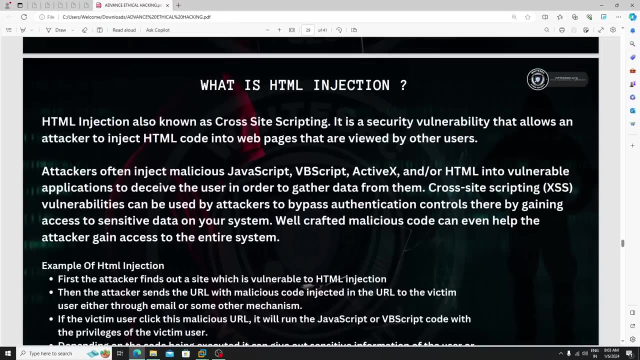 website hacking right. hope you guys enjoy this class. hello guys. hope you are fine in this classes. we are learning about you. what is html injection? see html injection, also known as cross-site scripting. it is a security vulnerability that allows an attacker to inject html code into the web pages that are viewed by. 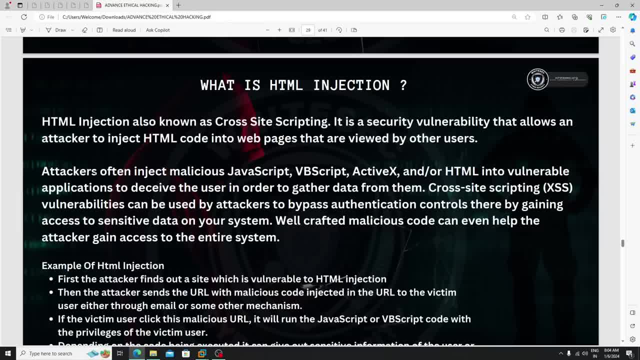 other users. okay. attackers often inject malicious javascript, pb script, activex and or html into vulnerable application to deceive the user in order to gather data data from them. okay. cross-site scripting- sss, xss vulnerability can be used by attacker to bypass authentication controls, thereby gaining access to sensitive data on your system. well-crafted malicious code can even be. it can. 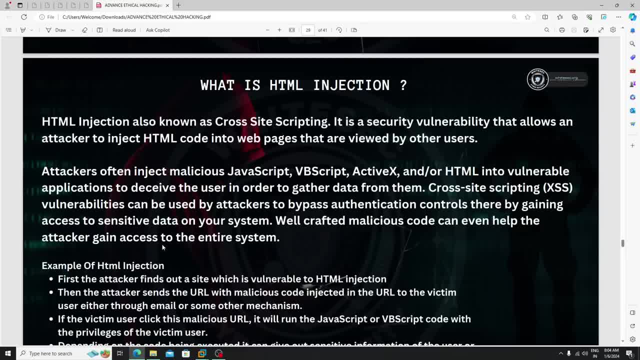 even help the attacker to gain access to the entire system right here. the thing is basically this: html injection is performed by attackers right to gain access to that system, or you know, to see here html into the vulnerable application to deceive the user in order to gather data from. 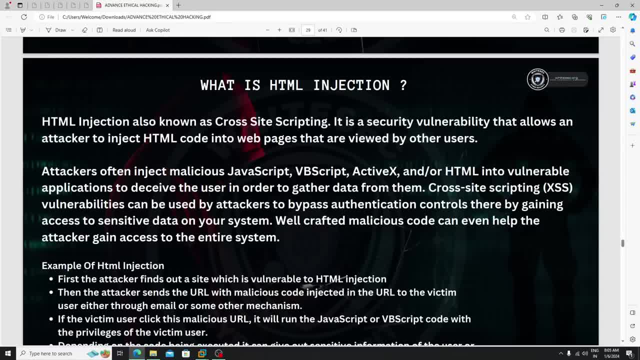 them. okay. the simple thing is here they can also add this kind of uh, mostly in html injection. what we see means. let me tell you the real world scenarios. see, sometimes when you visit the size site, you guys can able to see, uh, the deface page there. okay, like something, like. okay, this site is. 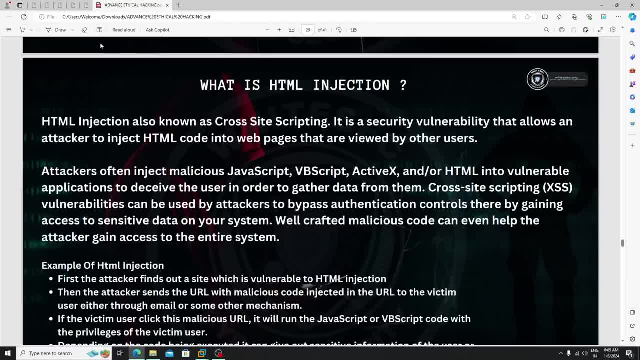 hacked by attackers mostly. you can also visit and see how the defense page is setting stuff like: oh see in that page title as well: hacked by the group name, the hackers group name. okay, the things you will see there. okay, so maybe some in some cases what will happen means uh, not maybe it will happen. 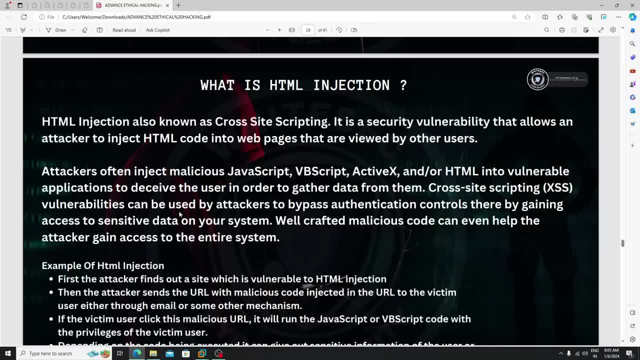 uh, this, uh, they create some kind of button there. if they click on the button then it will redirect to phishing page or this kind of chefs. okay, mostly they add the messages. okay, such kind of messages. okay, uh, like, uh, the based on the politics message or any kind of message. okay, they add there. okay. 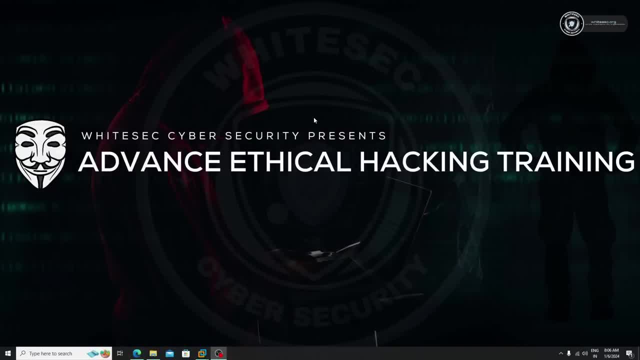 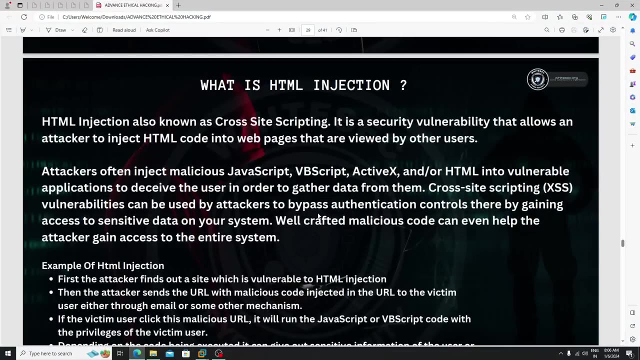 once you visit any hacker website, what will happen means mostly you will see hacked by the group, the hacker group. you guys can able to see there. okay, so this is the thing. mostly. it is used to, uh, gather information about the victim. okay, it will use to redirect the victim to malicious page as well. okay, 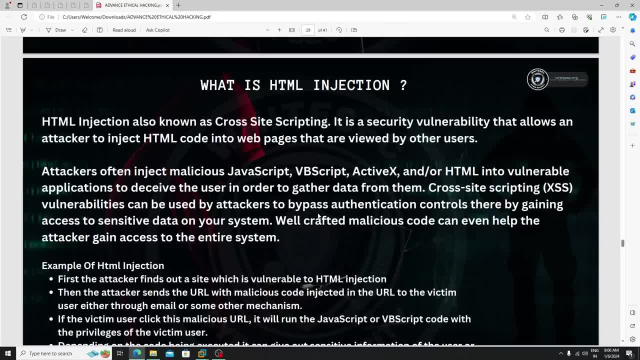 to uh, it will useful to uh like. mostly, uh, this html injection is used to spread the malicious viruses as well. okay, like, i just uh saw this scenarios as well. the assume that there is a one website which is very popular. uh, traffic is used there. okay, people are reading articles from that website. 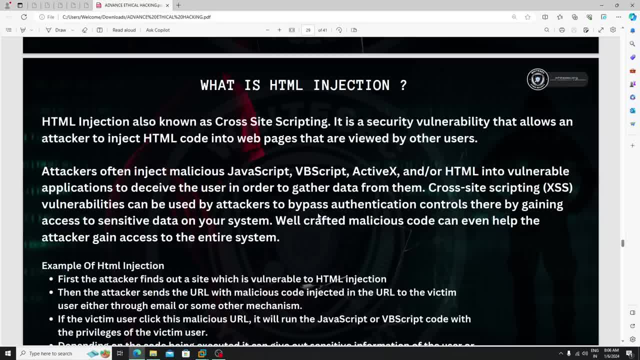 simple. assume that in that website there is a html vulnerability. is there the attacker? what he can able to do means he can able to add kind of button there. okay, he can able to add this kind of buttons like: click here to, uh, join course or click here to get some kind of rewards. 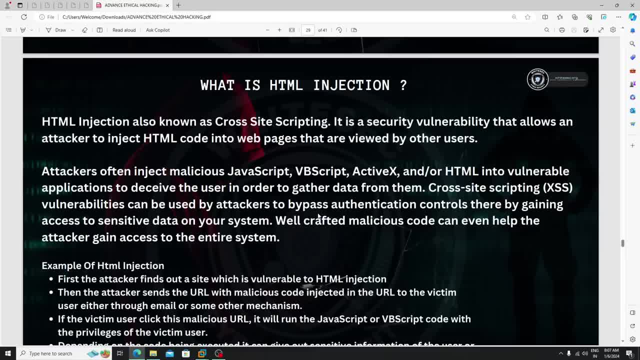 click here to learn more this kind of buttons. okay, he add there: if you click on that button, then the malicious file will be downloaded. okay, then you, uh, if you execute that malicious file, boom you, your system will be hacked, okay. and the second scenario is: uh, there is a links, okay, the. 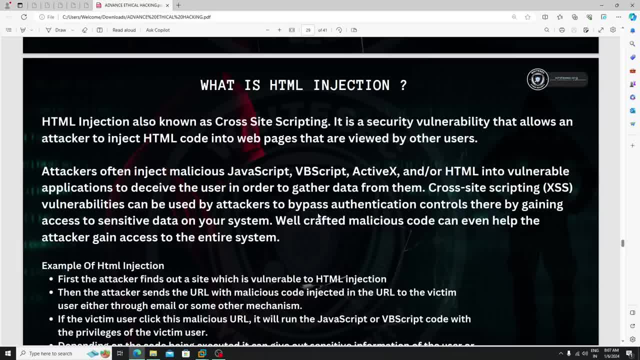 same button is there. if you click on that button then it will redirect to you to phishing page. okay, if you click on the, if you type, assume that you don't have the knowledge about cyber security or this kind of hacking steps at the time you guys will enter the pages. uh, the, the credentials are: 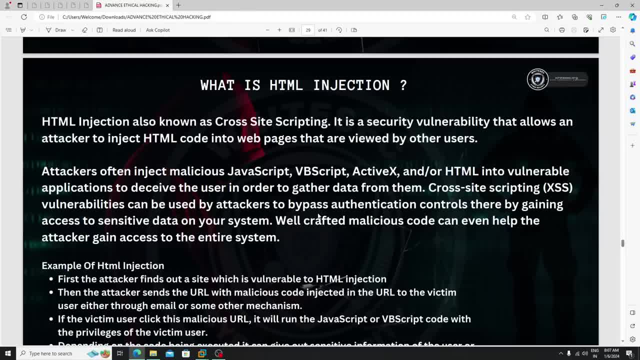 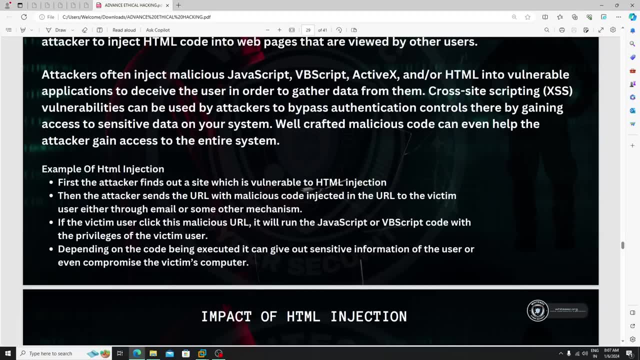 simple: he, he will get that. okay, this is the thing. mostly. i just saw this scenario since spreading botnets and viruses. okay, this is the thing. okay, and here example of, uh, html injection. first, the attacker finds out a site which is vulnerable to html injection. this is the first. 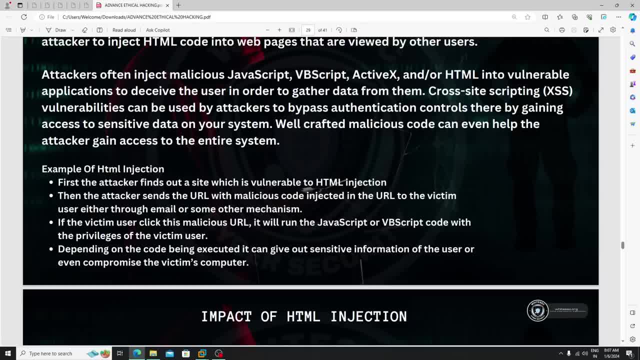 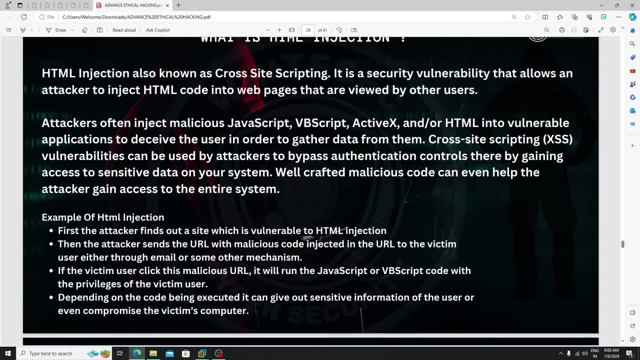 you need to hunt the injection here. okay, the html injection on your target website. then the attacker send the url with the malicious code injected in the url to the victim user, either through email or some other mechanism. okay, like we will see this thing as well. if the victim user basically what will happen means the attacker will send the url there, okay, 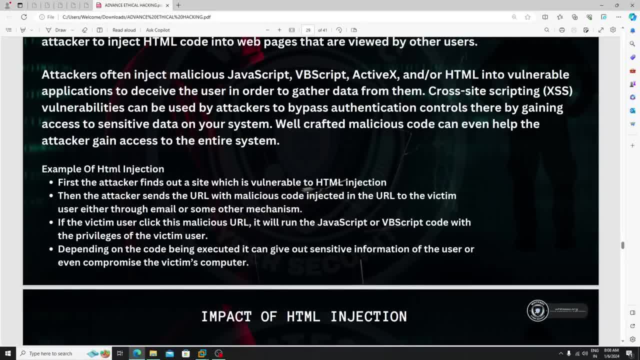 we will see it practically okay once we jump in practical class. it will easy for you. if the victim user click this malicious url, it will run the javascript or vbscript code with the privileges of the victim user. depending on the on the code being executed, it can give out a sensitive 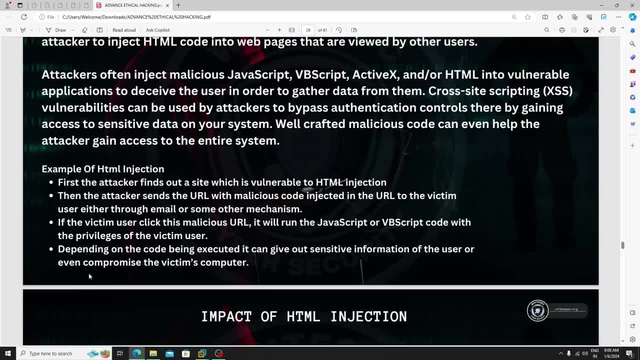 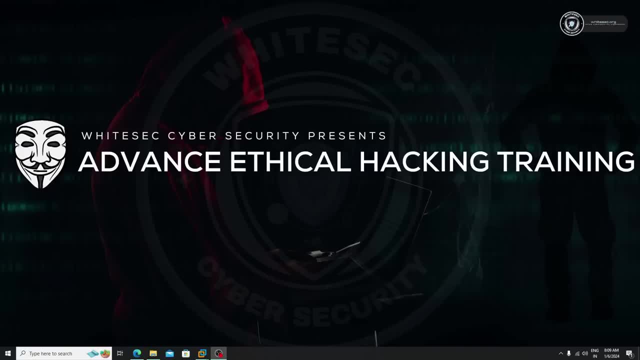 information of the of the user or even compromise the victim computer. we just learn, uh, in red teaming i think we just created the html payload there simple. if we execute it, then we will get the reversal okay. so this is the thing. now in this classes we are learning about impact. impact is very important. 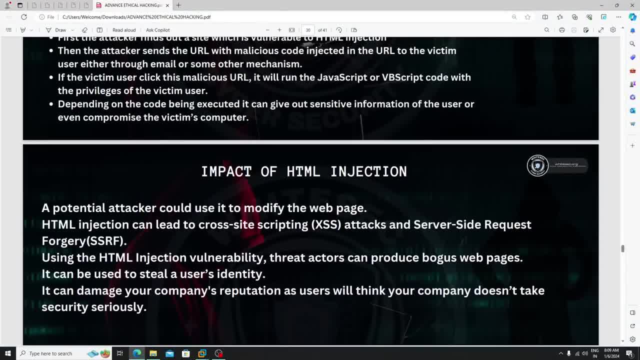 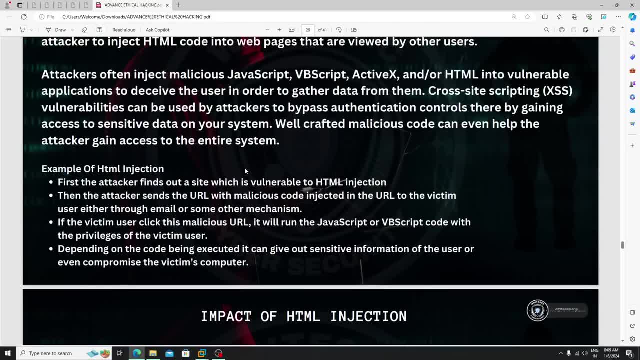 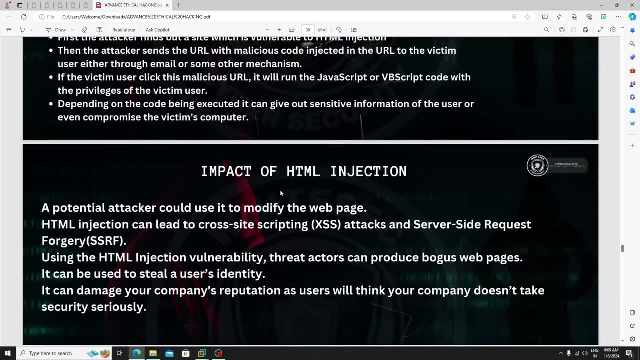 guys, see you, a potential attacker could use to modify the web page. what is the impact of this? uh html injection like what it can able to do, what type of damages it can able to do. okay, this is the thing. now. html injection can lead to cross site scripting as access vulnerability attacks. 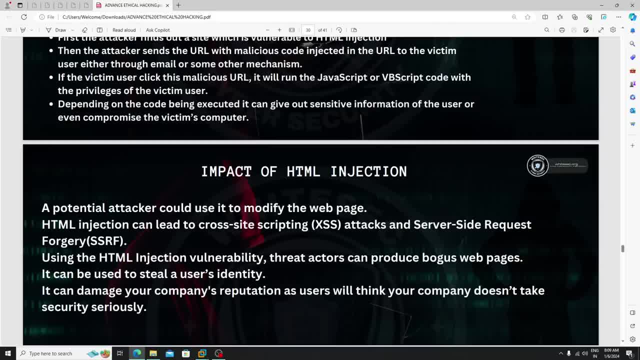 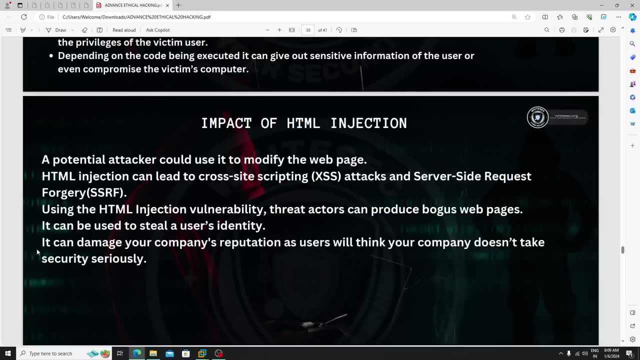 and server side request froggery ssrf using the html injection uh injection vulnerability threat actor. that means the attacker can produce bogus web pages. it can be used to steal a user identity. this is the thing. okay it? it can damage your company reputation as user will think your company doesn't take a secure securities uh. 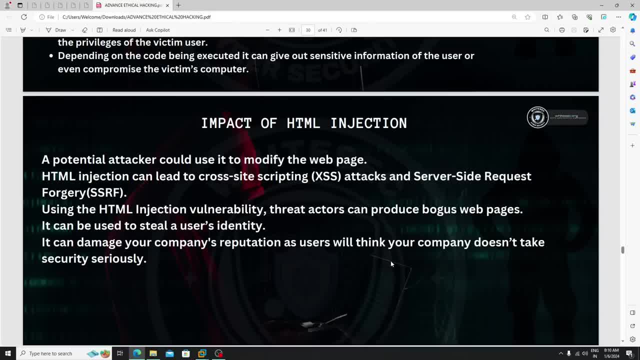 seriously, okay, like it will damage the reputation as well. okay, assume that you are providing the service, you have a company. okay, you are providing the services here. simple, somebody hack would have hacked your website. then what will happen? the people will think that your, your clients, will think that, okay, this, uh, the company doesn't have the security. okay, there, if the simple thing is. 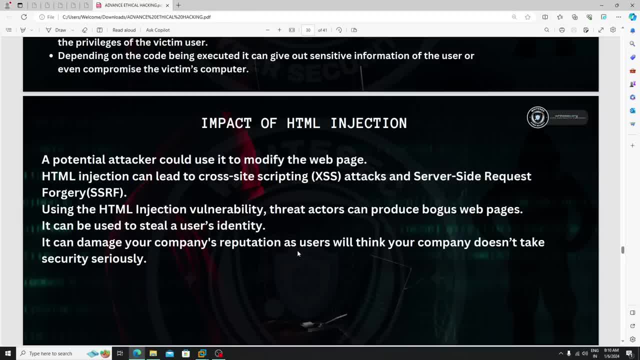 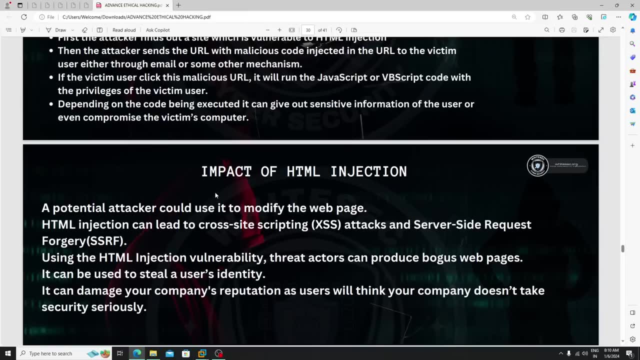 they think that, okay, our data is also not secure. simple, they they avoid the services from you. this is the thing. mostly this will happen in in companies, okay, so this is a very important thing, guys. in the next classes, we will learn about how we can able to find this html injection- uh, html injection vulnerability and 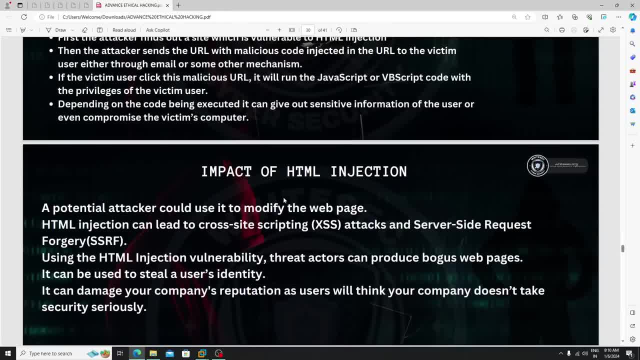 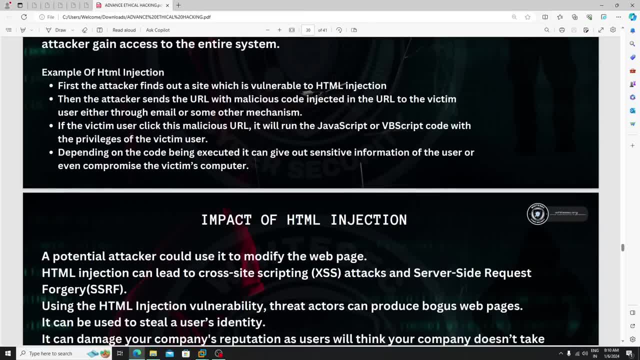 how we can able to exploit it now, and also it is totally depend upon you. here we are covering the main things. uh, main things. okay, which which is need for beginners? okay, like, uh, there are a lot of things are there which you need to learn yourself. okay, all right, hope you guys get it. 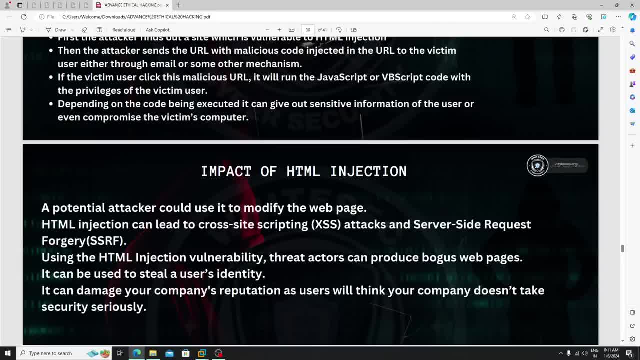 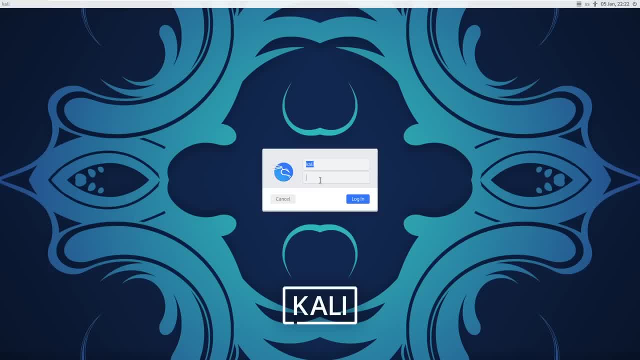 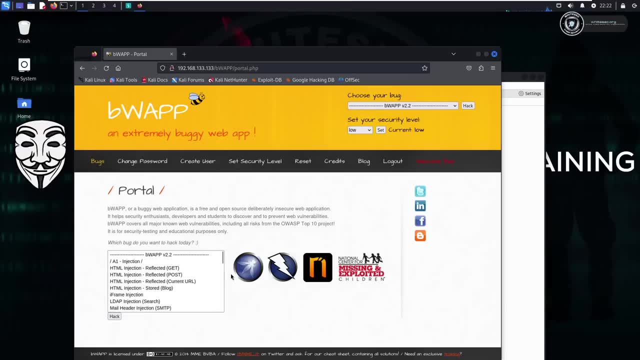 right in the next classes we will see practically how we can able to exploit the html injection right now. let's perform the html injection here now. first of all let's go with reflected get and first let's go with the reflected get. what is a reflected here? see? 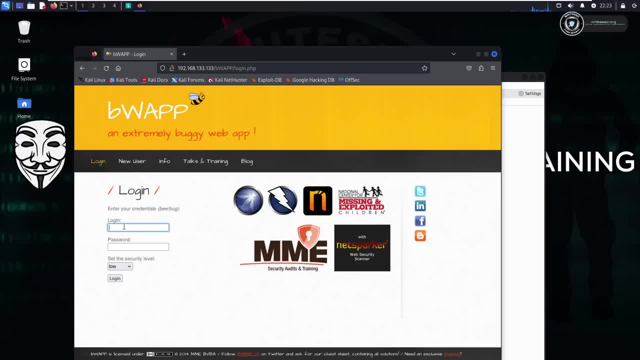 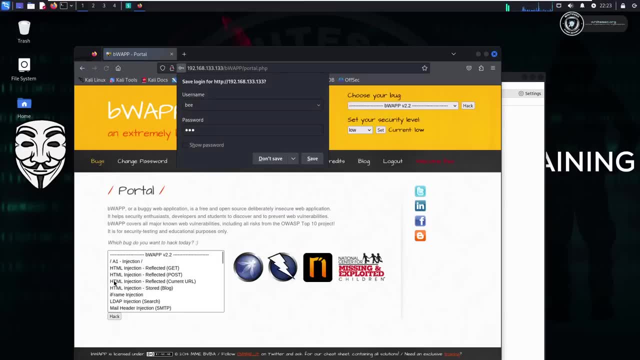 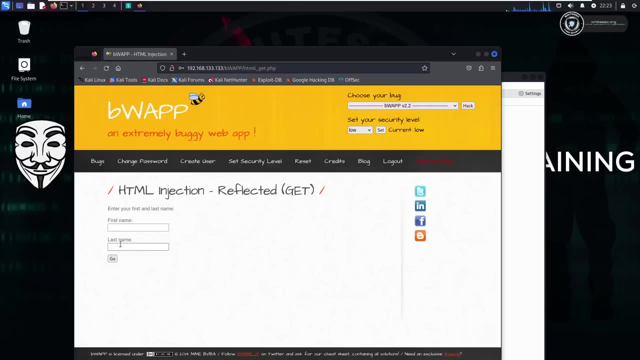 let me tell you here: uh, let me add the username and the password. okay, let me go again. reflected now. here there is a first name and password. okay, sorry, the last name. now, if i type anything here, so such as hi as a first name and hello as a last name, then here you can able to see. 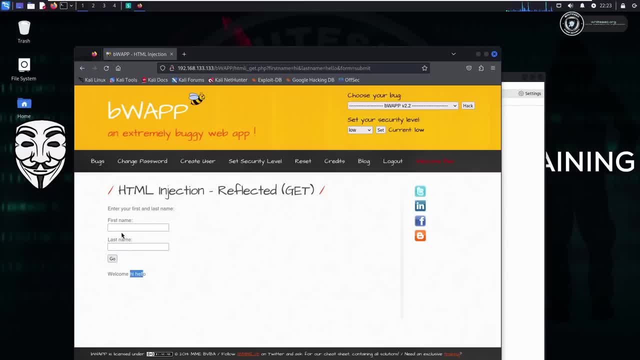 welcome, hi, hello. basically, the values we just entered there, the, the name or something- it's reflecting in web page. okay, this is the thing it's known as reflected right, and also what is a get here? get is a nothing, but see here the request, okay, the data which we just type here. 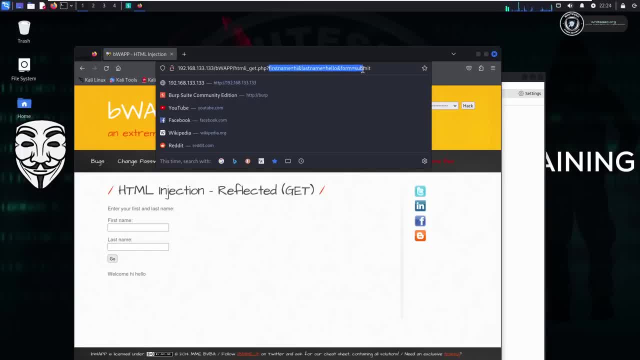 or send it through url. see, here in url you guys can able to see first name as a hi and last hi and last name as hello, right? so basically, it's known as what. when you see the data which you type there, it's going through the url. then that means it's a get. okay, this is the thing you no. 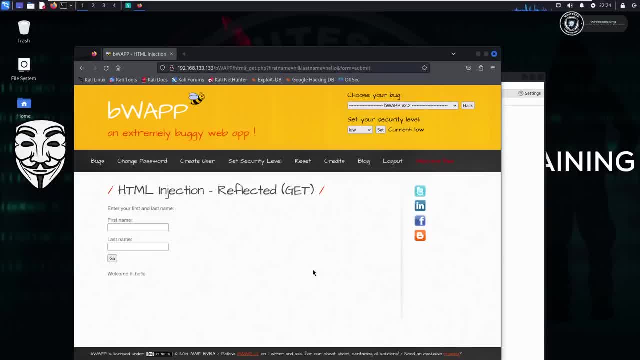 need to worry here. okay, now the simple thing is: let me capture the data which we just typed here. let me capture this request in bup suit. now, simple, let me run on this interceptor and let me- sorry guys, let me type here: hi, hello, as a last name. if i click on go, then what will happen? the request. 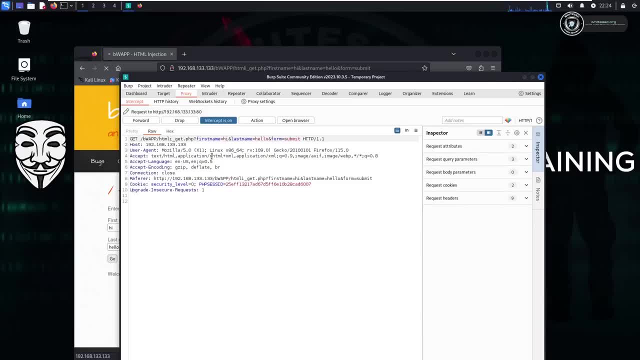 will comes in bup suit. okay. again i am saying: get request is nothing but the data which you just type there is going in url through. url is known as what get request. okay, now here we need to change this into put request. okay, so we want to say that, uh, the view we are just going to keep minimum. 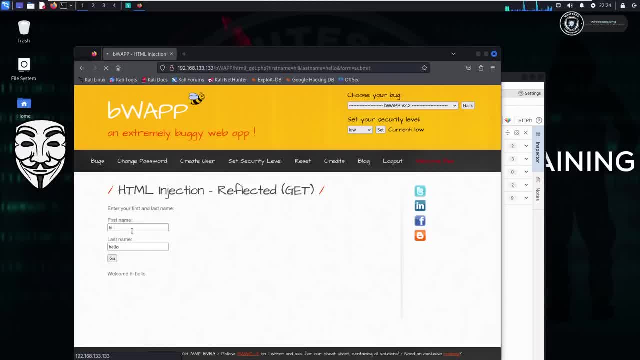 of the piece. so, as usual, we need to make a new header just so that a new link can be made. so click enter a new event code, paste the host name back to Appian tag, ok, and then type in the 365 series, and then you will get the option that we wanted to choose for our client, whether or 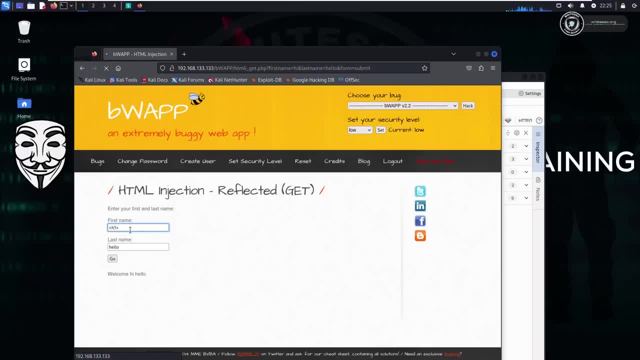 not. we wanted to use this feature for음. let me bounce it- sensitivity. okay, sorry, i need to write some more, like one at a time, in order. Let me type the username in as a high, or let me type here: I could out something. If it's executed, then that means the vulnerability is there. 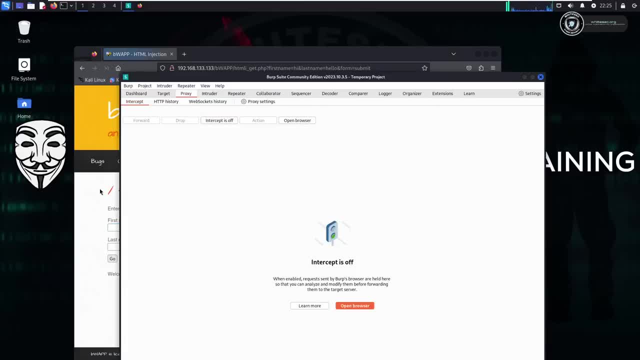 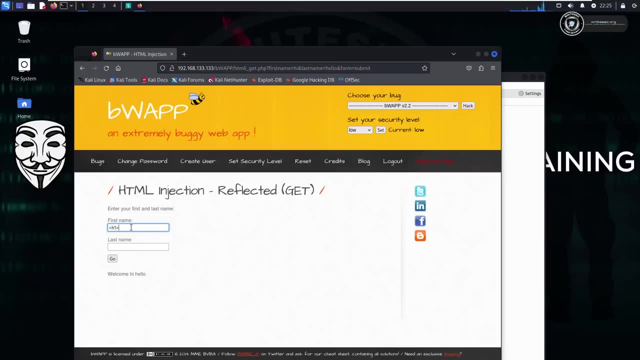 But type here, let me have this one, just let me do it again. If I click on go, let me type the last name as hello. If I click on go here, see it's executed. Okay, The attacker can also execute the anything here. okay, which is reflected in a page. 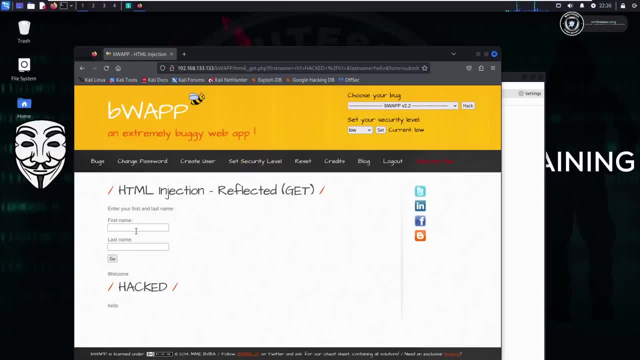 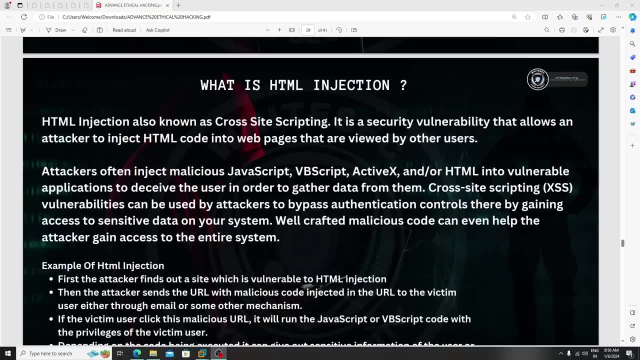 This is how it's gonna work. Okay, Like you are in your basically here attacker, okay, can able to inject the HTML code into web page. okay, we can, let me. let me show you first of all the example here. let me. 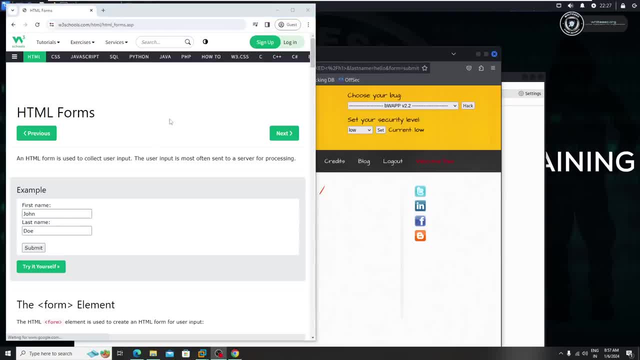 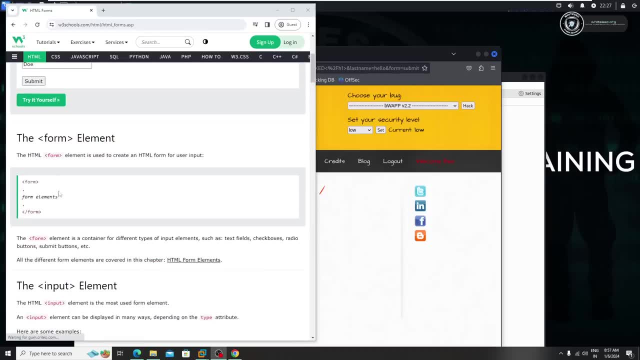 use a form. Okay, There is a one website which is w three school school. From here, you can able to get the forms, each and everything. Right, Let me take this as this form. Okay, let me copy this code. 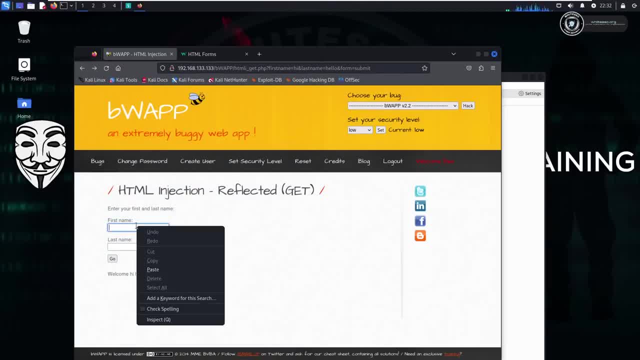 The field of first name. let me paste the code there. Okay, And in the last name also. no need to paste the code. Let me check for first field. Let me type your last name as hello. Right, If I let me use another form here. 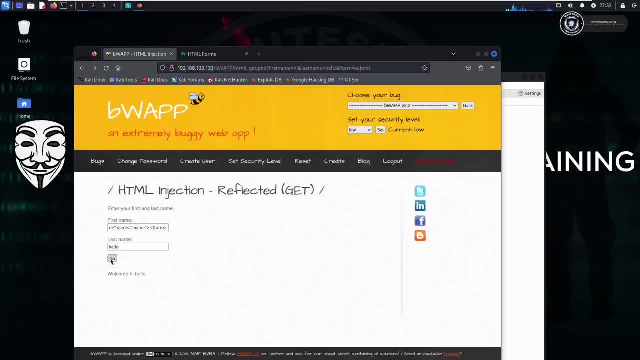 No need, Okay, just simple click on. go there. Now what happened? The form has been created, a new form, right? So see here? That means it is vulnerable to HTML injection. You, the attacker, can do that. Okay, You can able to add any HTML code there. 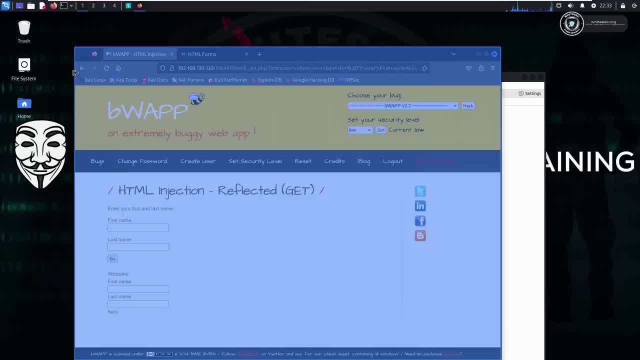 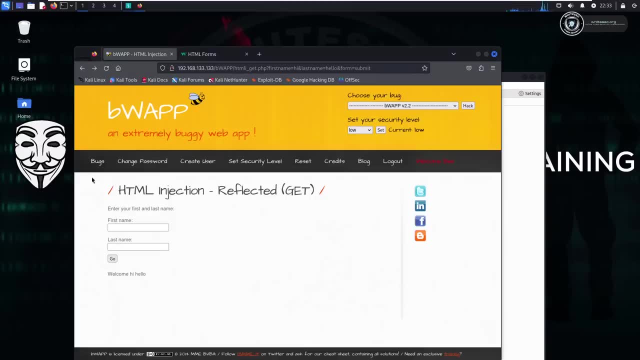 Okay Now how to do this process using bup suit. The simple thing is first of all just click on intercept on okay. Now here just add any name, the normal values first. okay, such as hi, hello, if I click. 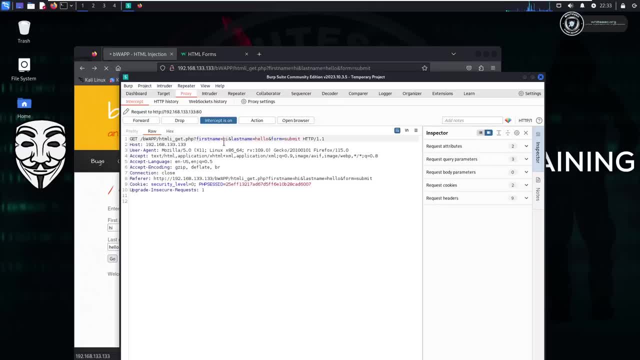 on, go Now. here you guys can able to see there is a request now instead of hi, what I, what I need to do, See always remember where you need to insert the payload here. Mostly the beginners will get kind of confusion here. 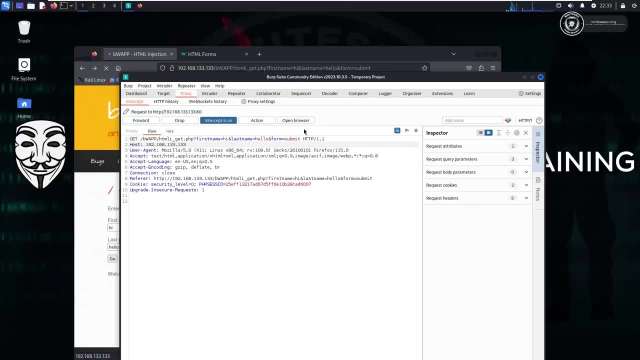 Let me zoom it. Okay, I can't able to zoom it. Just see here There is a first name. right After first name there is a is equal sign. Okay, After is equal, There is a high is a right. simple, instead of high. just remove that high and insert your. 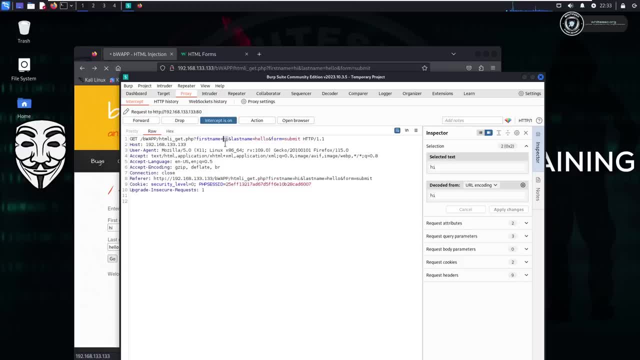 payload there. Okay, Which is our form code. And see after he. after that value, there is a and sign is there. Okay, Don't play with the science and don't remove it. Basically It is differentiating Kind of first name and last name. 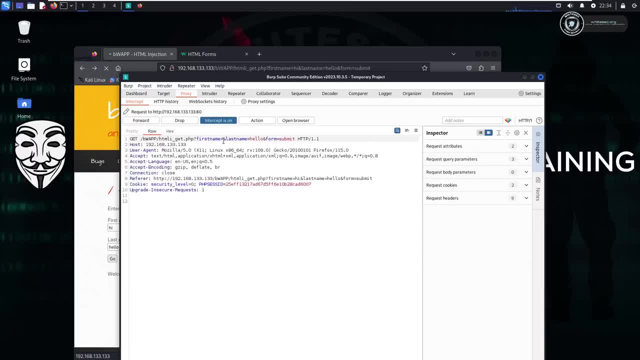 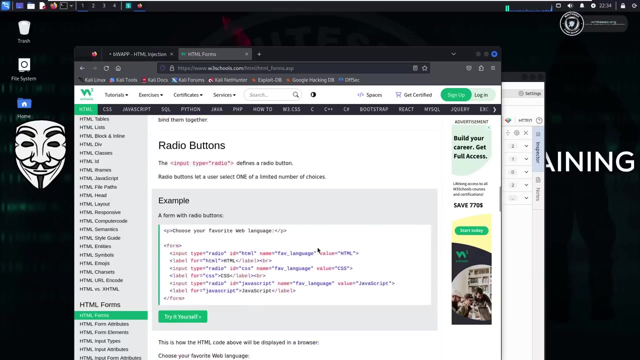 Okay, This is the thing, So simple. just paste the form there. just told you, just paste in for until and? okay, Now there is a last name, is a last name also. see here, last name is equal to there is a hello instead of Hello. let me add another form. 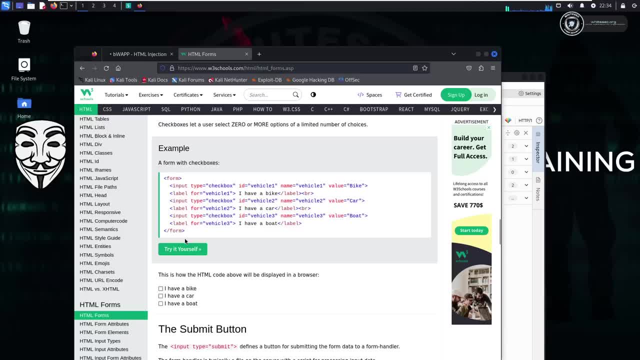 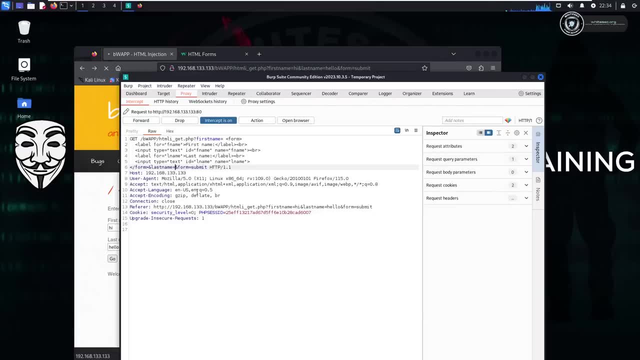 Let me add checkbox. Okay, So checkbox. Let me copy this And let me paste it here. Okay, It's not a big deal. Again, I'm saying, instead of doing it for you guys in bup suit, you can also execute. 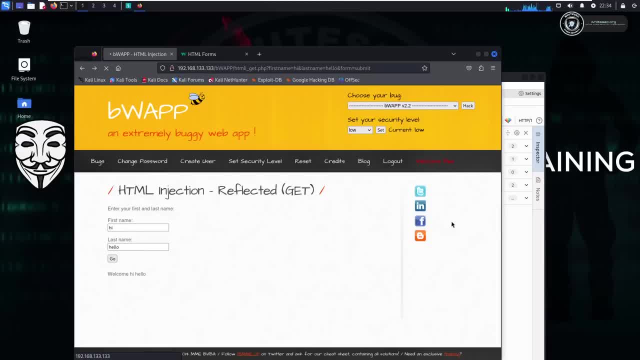 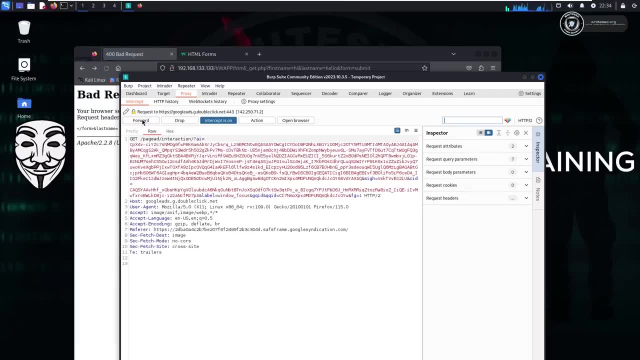 these things here as well. Okay, it's not a big deal because why we are using this web suit? because things are very easy here to get it. okay, Now, if I click on the forward, then what will happen? It is a bad request. 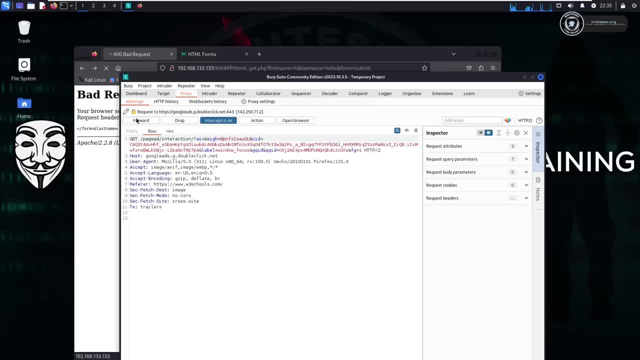 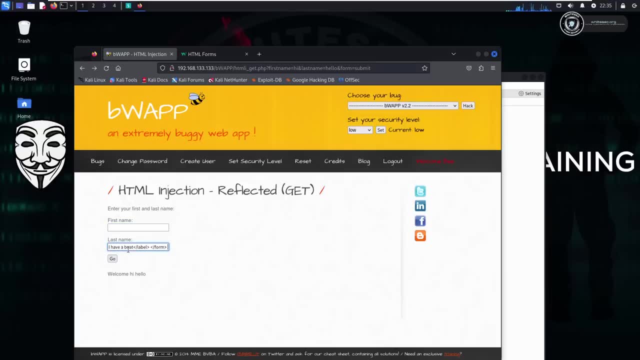 Okay, let me execute here only So see, here the form has been created and the checkbox is also easier, right? So this is how it is going to work. Hope you guys can able to see. this is this is known as what HTML injection reflected? 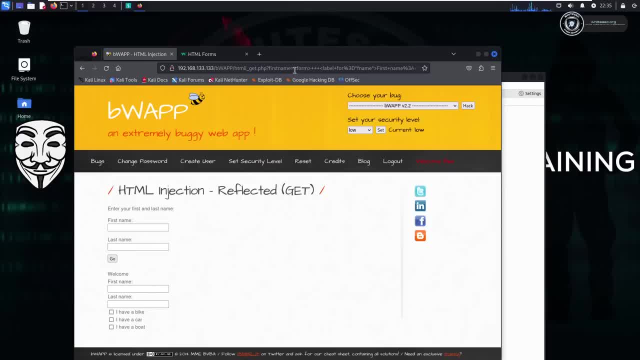 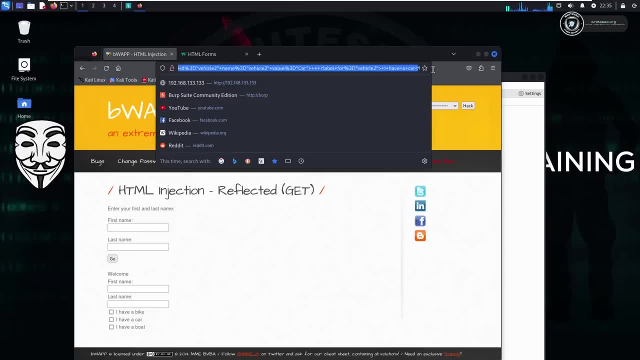 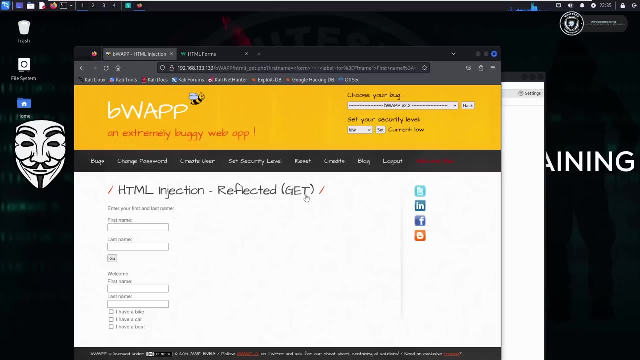 See. So basically, the data which you just added here, typed here, is in URL. See, this is in URL, right? So this is known as reflected HTML. sorry, HTML injection- reflected, get. okay, I just told you what is good here, right. 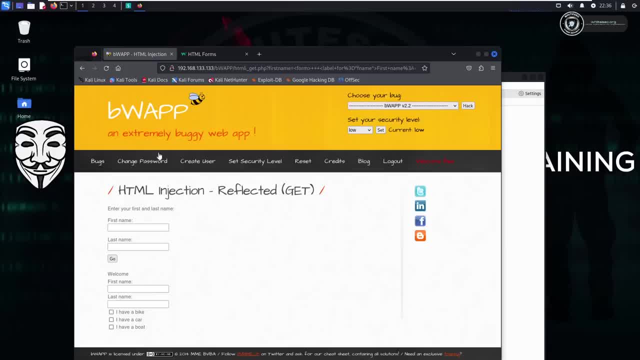 Let me tell you this will affect on every user who is using visiting this site. okay, he will see this kind of forms or something like that, if I how he can able to see simple. what you need To do means simply, you need to send this URL to your victim, okay. 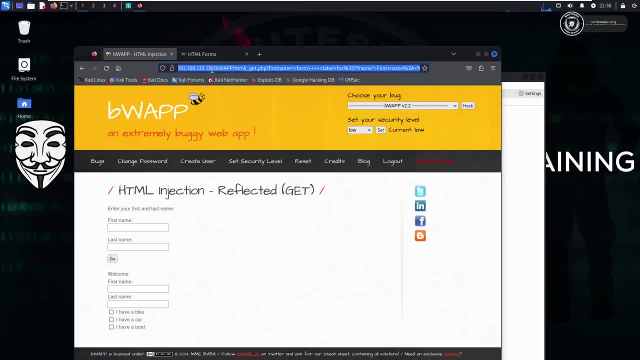 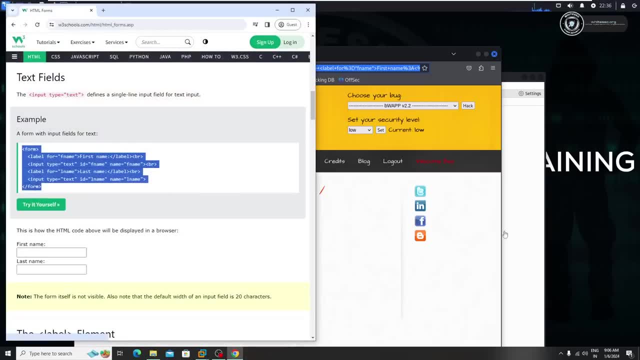 It's not like he also need to visit the domain or something like that. you need to send this URL like this: okay, just copy the URL and let me open this URL in Chrome browser. okay, See here also. it's not a VM machine. 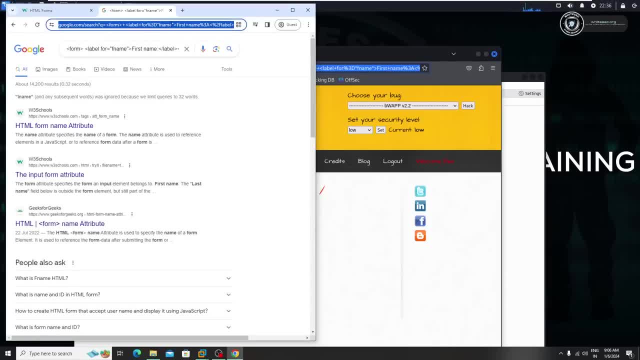 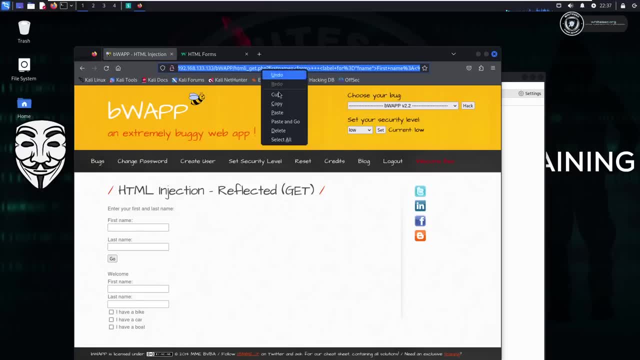 It's a Chrome. Okay, Hell man, why I can't able to copy here? just simple. let me copy it simple. just assumed that this is a URL. Okay, let me turn off the this interceptor as well. assume that you, if you send it this. 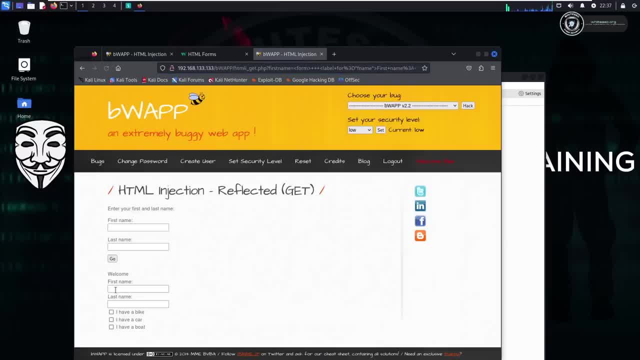 URL to victim. then it will look like this: okay, So this is a thing. assumed that you your victim just going manually there without didn't send the URL, and he just visiting this page normally as a normal user, then what will happen? 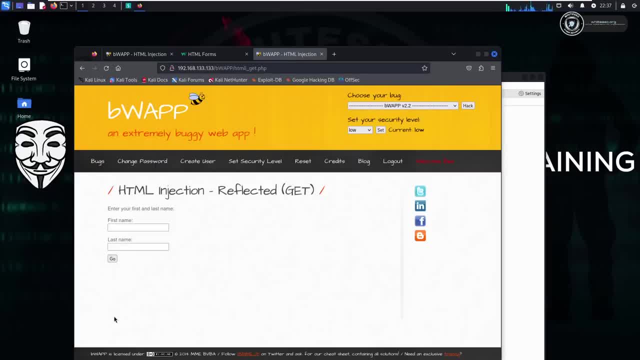 It won't affect that. okay, Because it's a good. it's a reflected, okay. This is a difference between Reflected and stored. stored, what will happen means you no need to send URL there. Okay, simple. Anyone who is using this website can able to see the result in store. okay, let me show. 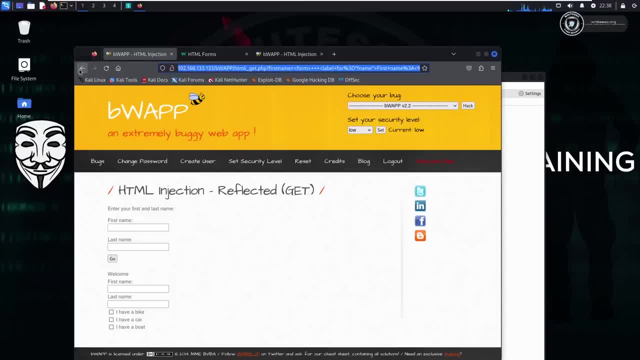 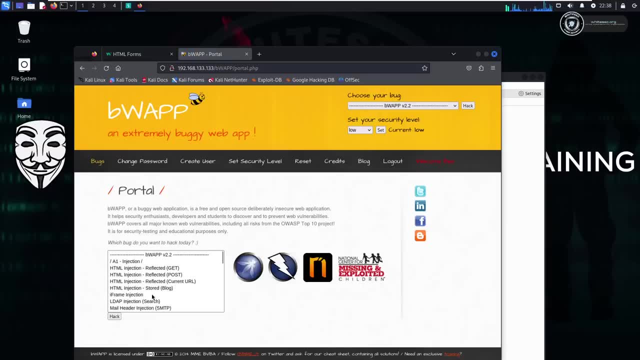 you that one. practically you will get it. okay, it's a very excellent thing right here. Let me use a stored blog here. This is excellent Thing. Okay, now assume that there is a comment section or any kind of messaging section in that website. 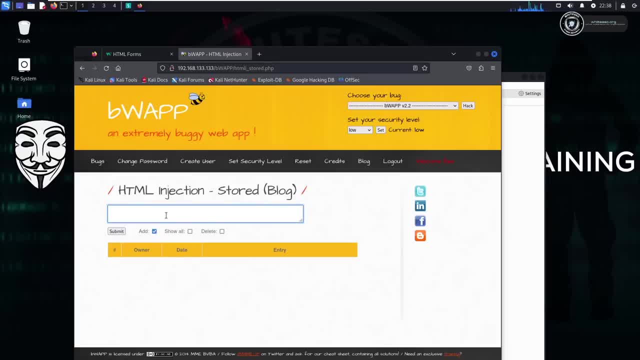 or anywhere. Then assume that you just type here: hi, just assume that I just typed the high. Now it's stored here. okay, assume that if anyone visit this page, then what? what will happen? he can able to see. see this, no need to send the URL, nothing. 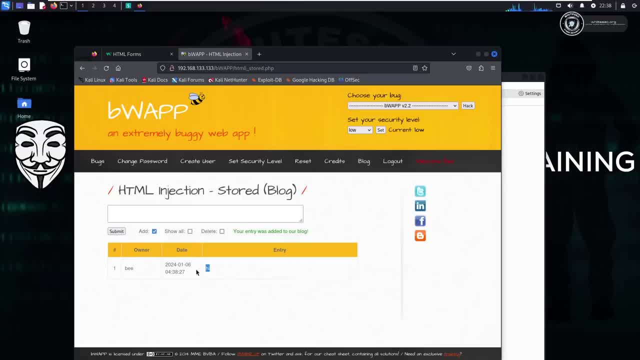 If you visit manually in that page, and what will happen? you can able to see the comments of other users. right, the simple thing. okay, Now assume that instead of hi, what I, what I'm gonna do, miss, let me inject the form. 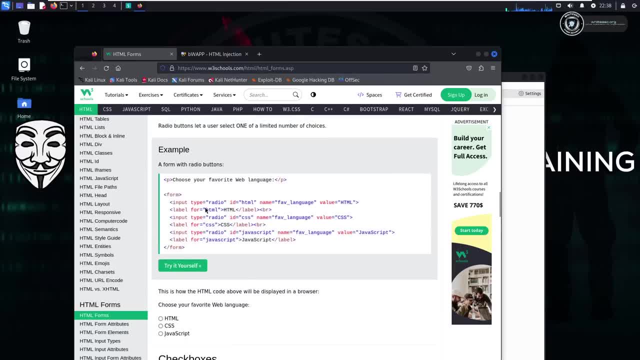 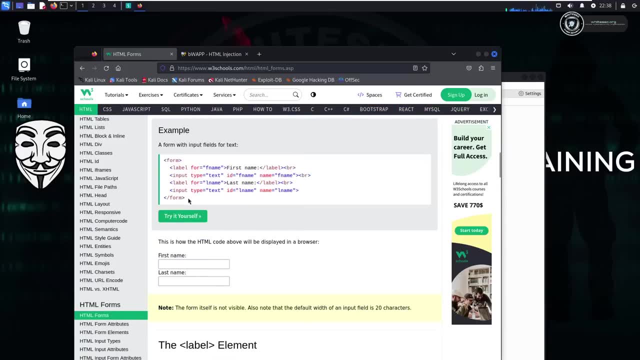 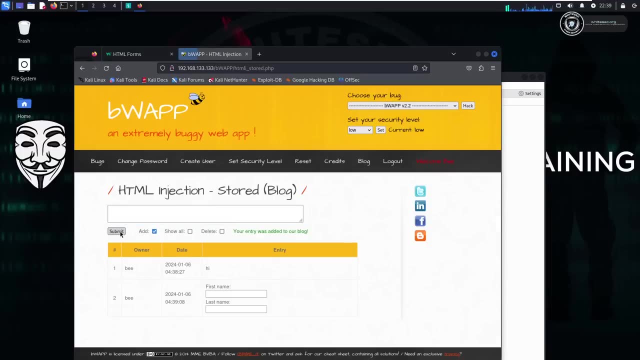 here The normal form, which is this one. Let me paste it here. And if I click on submit, then what will happen? the form has been created. any user who is using this website can able to see it. okay, if you type the username and the password. 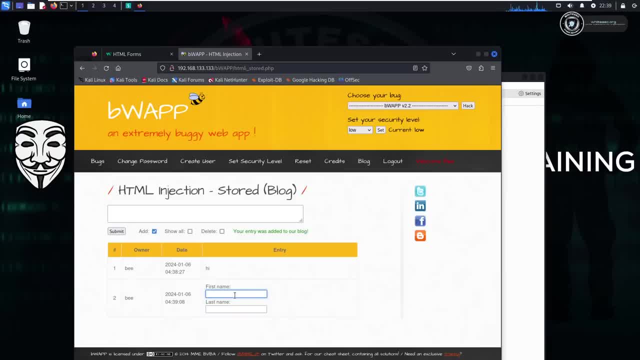 then what will happen? the attacker can able to steal it. Okay, So this is the simple thing which I'm explaining you. it's not a big deal. This is the difference between stored and reflected right. What is a reflected? see the keywords there. what is a reflected? simple seeing right. 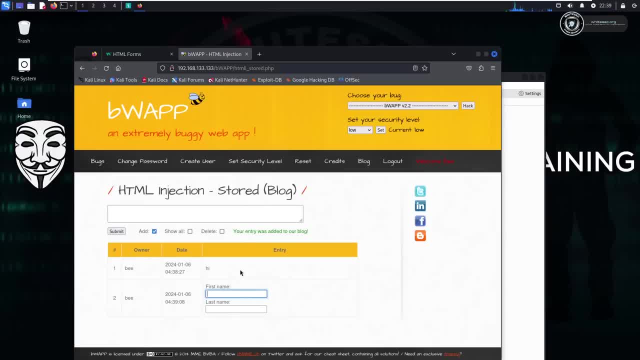 What is stored there. store is nothing but storing something in that database or website or something like that. Just remember this thing stored and reflected. it's not a big keywords, Everyone knows this. okay, like storing something, right, And let me, let me tell you here. 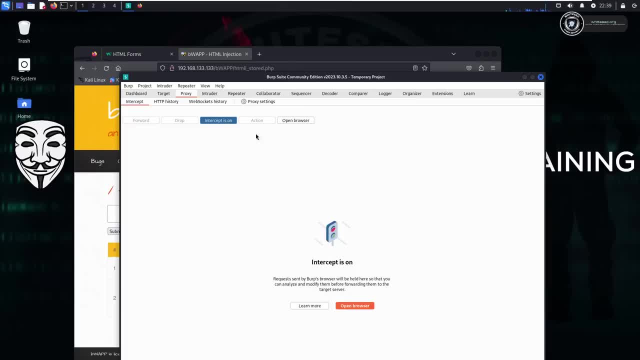 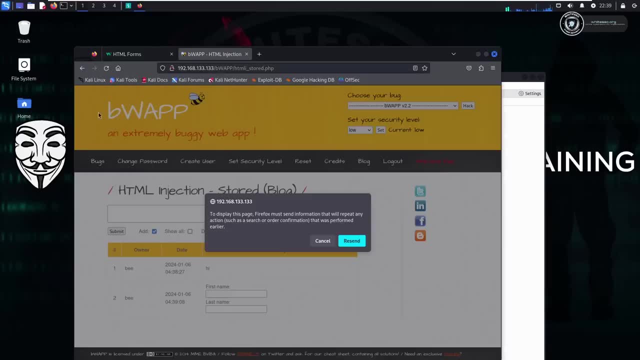 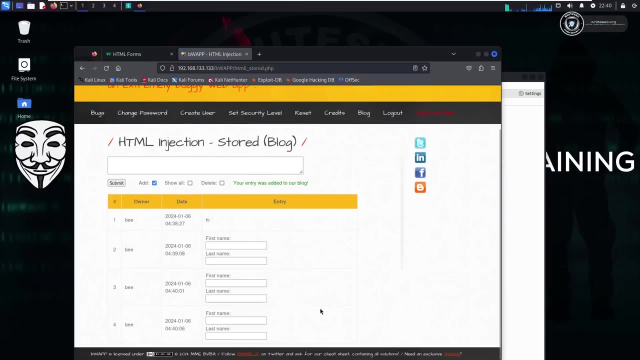 Let me Let me on this interceptor intercept And let me refresh this page. let me turn off this one. Let me refresh this. see, here again it's executed right. So here, basically, by comparing to last class in last class, what will happen in reflected? 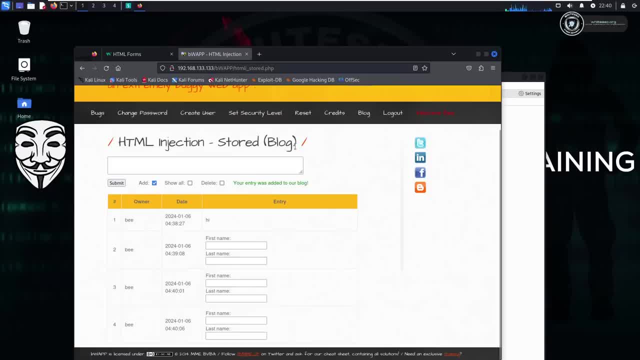 one in: get in, get request. what? what happened means the data is sent. Send it through URL. Okay, here it doesn't work like that. it will send it to to post request. okay, what is this? Let me show you. 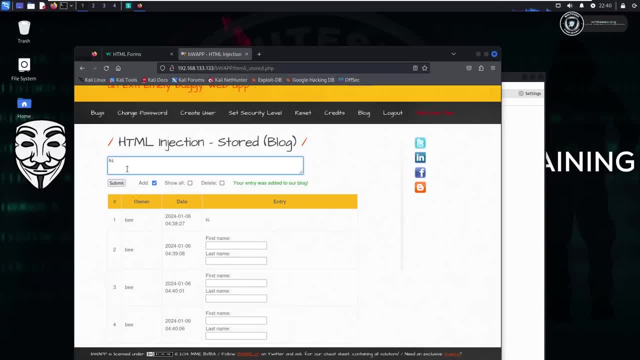 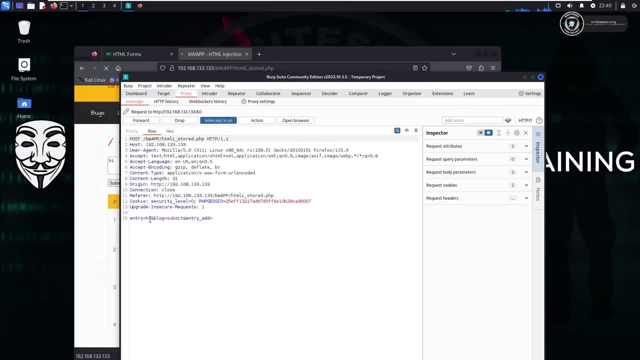 See, let me page any, any keyword here, such as hi, and let me intercept it: Submit. See, there is a entry highs here. okay, and there is a submit button. the request is post right Here. The data is sending separately here to see. 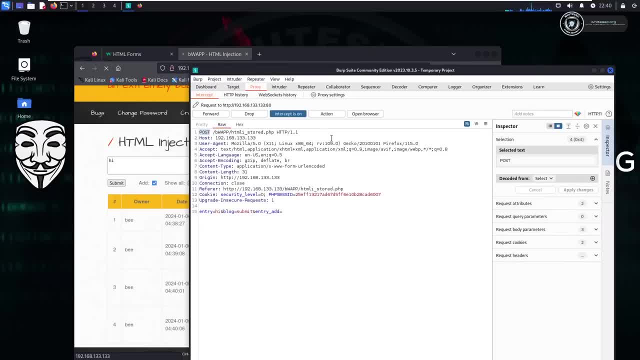 It's not sending. It's not sending through what? through URL. This is a thing. assume that if I want to perform this one to one to test this, then what I need to do, simple, I'm going to use a repeater here. let me show you about repeater. 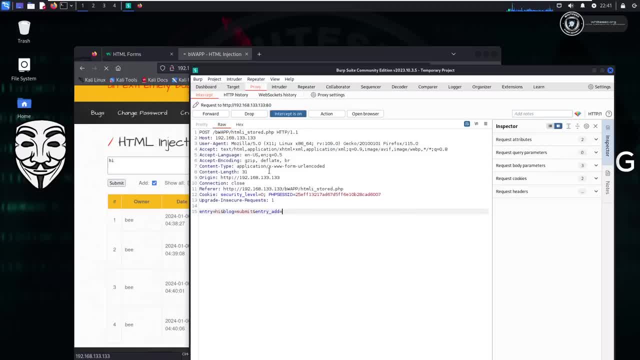 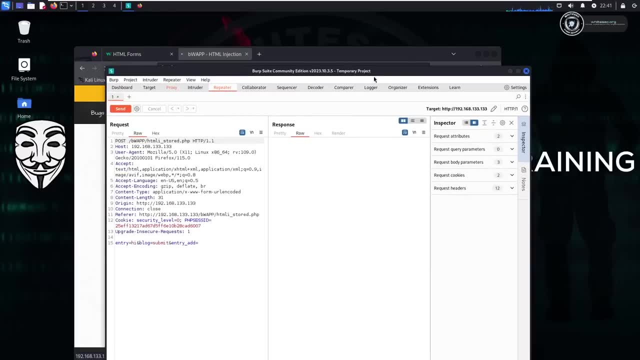 as well. If I click on, just just click anywhere, right click here and send it to repeater. Now here you can able to see. this is a repeater, basically without going to this website. okay, this normal browser or something. 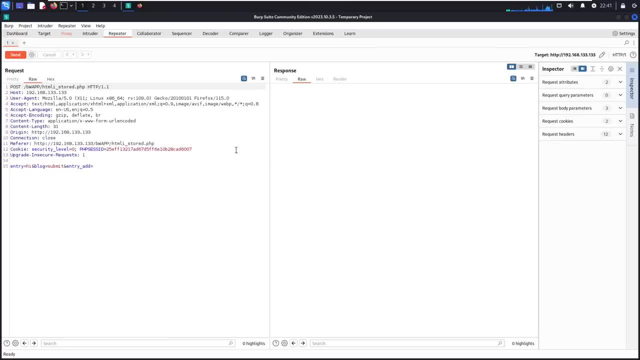 Like that you can able to see each and everything here. only, okay, this is a thing like you can continuously try to test it. okay, now, simple, assume that in entry here let me use a form. okay, paste it here, the form. then if I click on send here you can able. 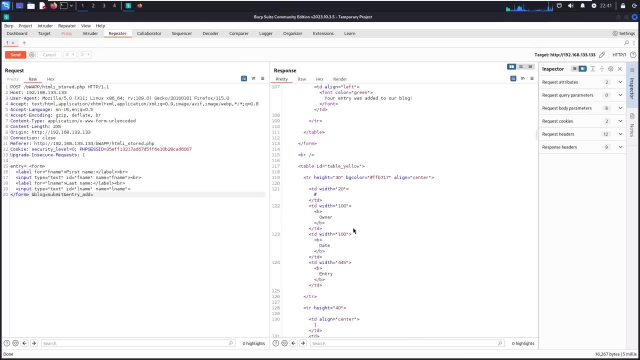 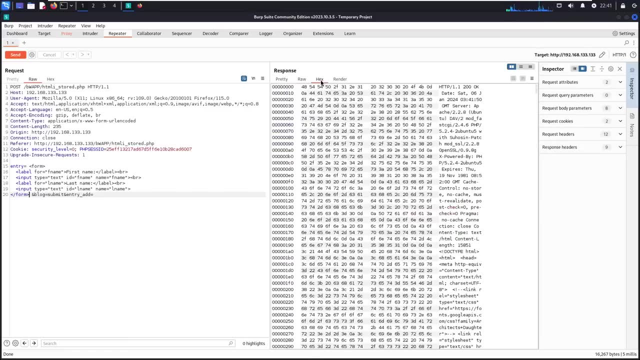 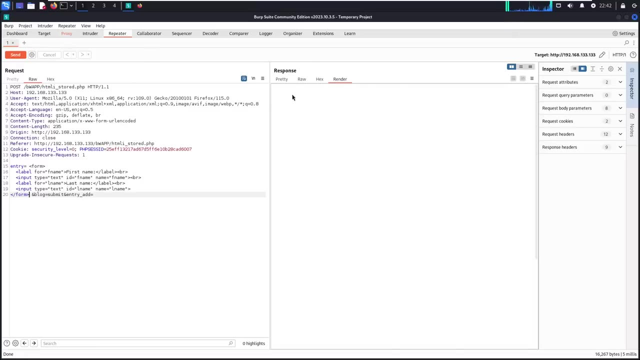 to see it successfully executed. So that's why the code is this much: If I click on raw, see 200.. Okay, That means success. If I click on render, then here you can able to see the web page See before doing this. okay, here you can able to see the web page right now, before. 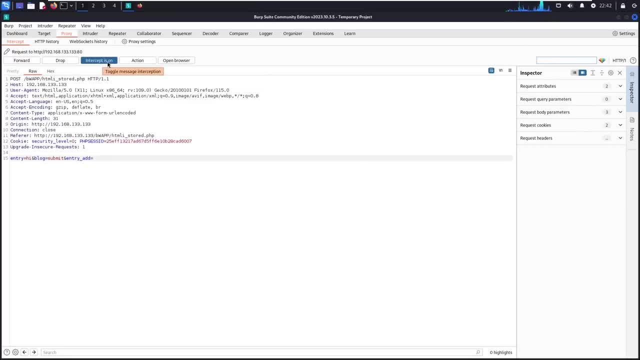 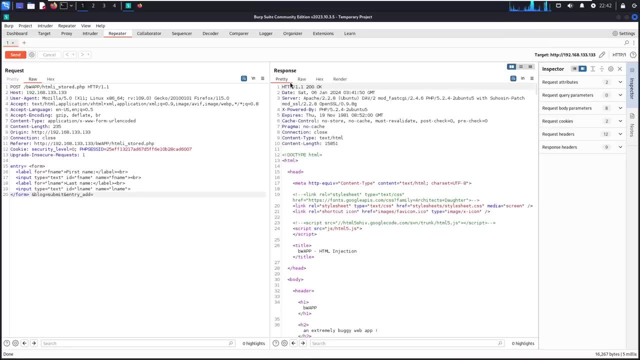 doing this. just run off your interceptor here. okay, go to repeater And from here you need to play. okay, See, I'm in this course. I'm just covering the beginner things. there is a lot you need to learn in web, pretty okay. 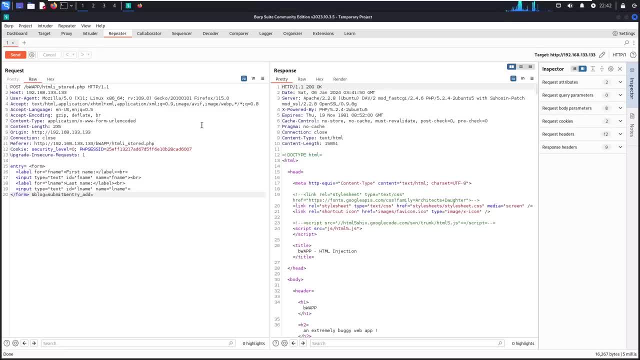 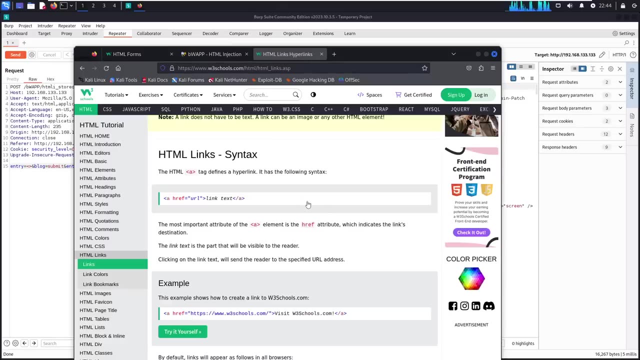 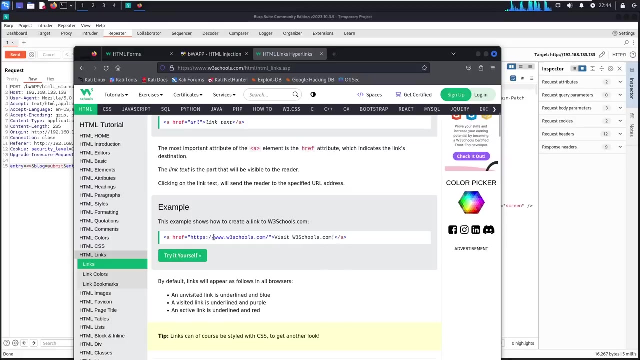 So here, Instead of form, let me add something like this: Let me add the button there. So let's go with button. So here is a code for a button: simple, you can also use it. I need button man this way. 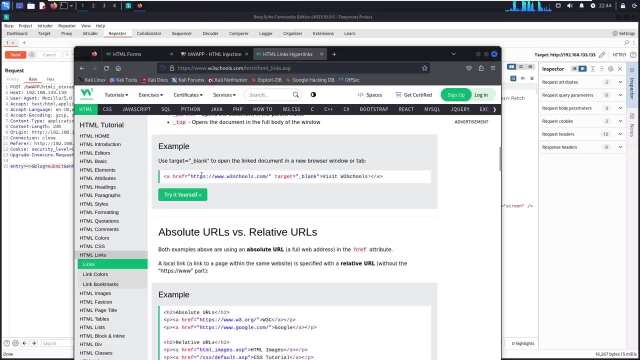 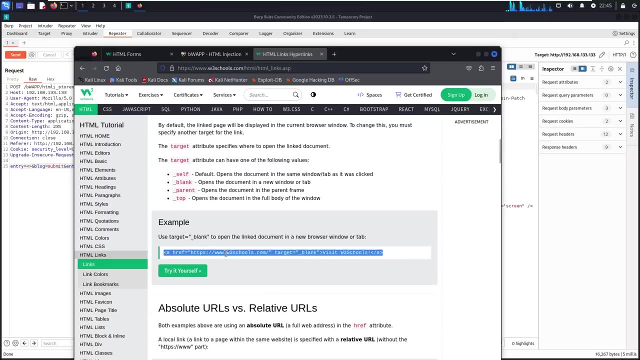 Start a button. It's a redirecting link, So basically how it's worked. let me show you this thing as well. See, let me copy this code. See, instead of here, attacker will add his payload URL. okay, direct URL if you click. 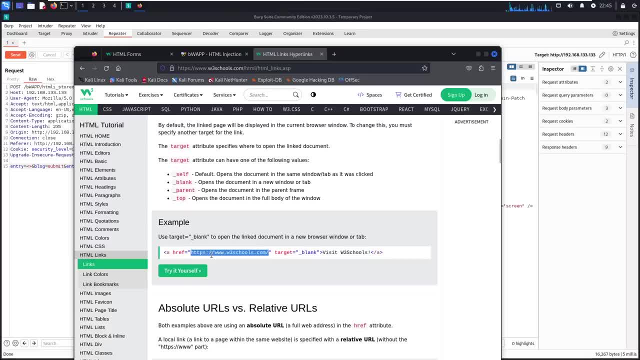 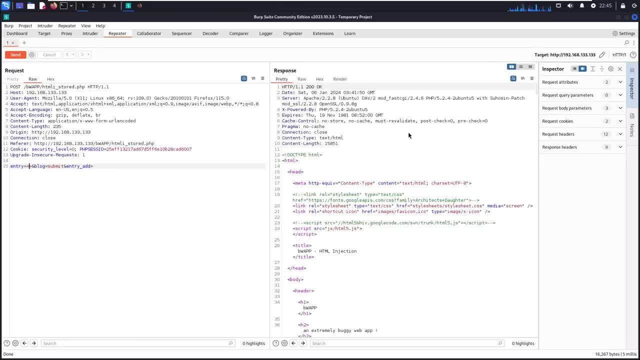 there. then what will happen? The payload will be downloaded in his machine. okay, in victim machine, not victim: anyone who is visiting this website. Okay, Now, simple. Instead of entry the here, let me add that URL. okay, like this: this: remove the spaces. 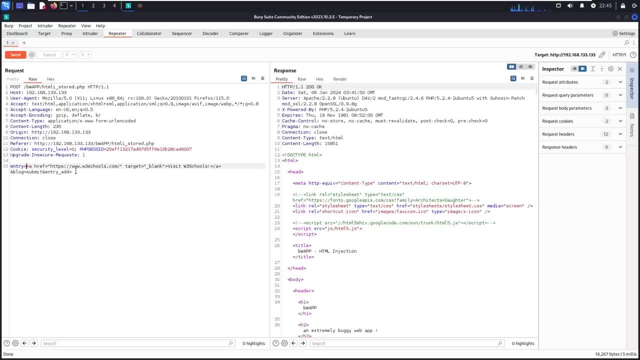 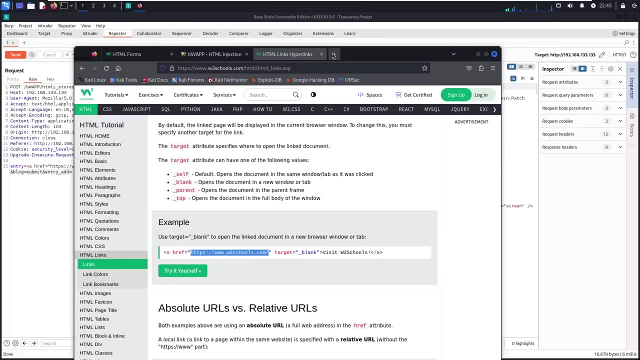 from there. Okay, now let me click on the submit. It successfully executed say 200. Okay, if I copy URL, see here there is a one, one option, which is copy URL. just copy the URL, And if you visit this URL, then what will happen? 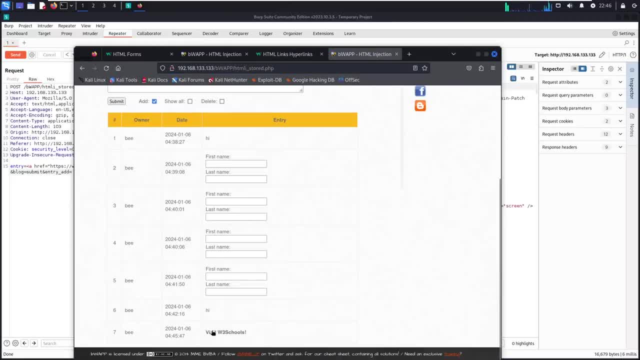 You can able to see The the this one here, right, It's successfully executed and there is a visit w three school. is that instead of w three school, the attacker will add some legit names here. okay, so just click here, or something. 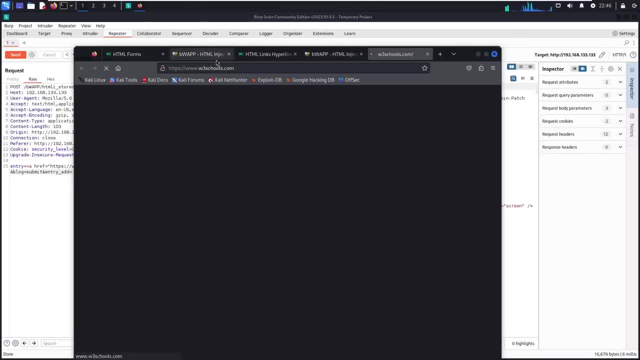 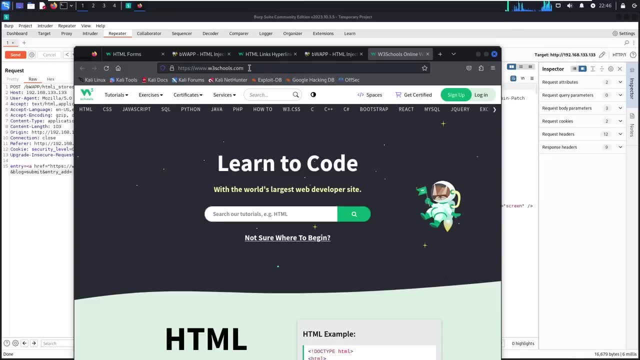 like that: If we click there, then what will happen? it will redirect to that page. Okay, this is a thing again I'm saying in real world. the attacker will add kind of phishing pages, scam pages, this kind of stuff here. 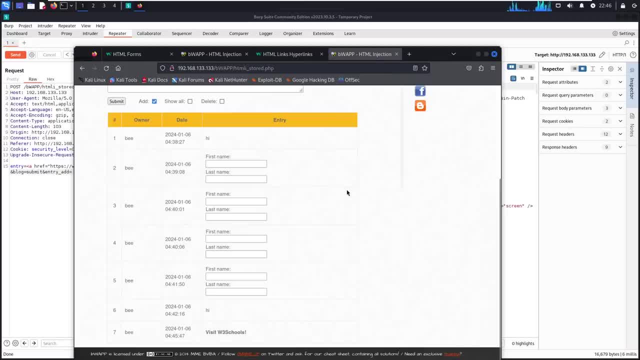 Okay, this HTML injection plays a very important role in spamming, Okay. So let's see, Let's see. So basically this is spamming, okay, like stealing the credit card information, this kind of stuff. It basically they target the attackers will target those website where the traffic is. 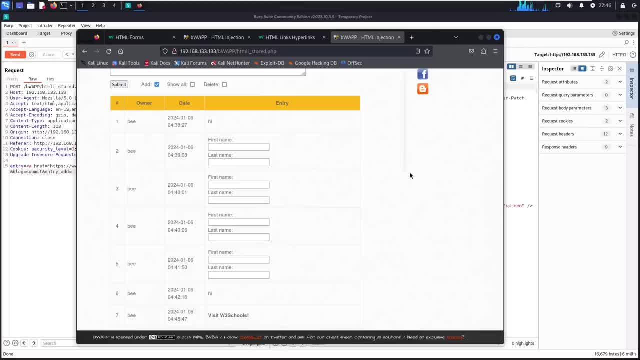 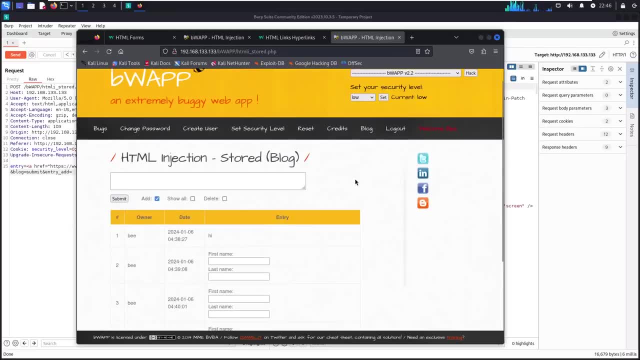 huge. Okay, like day by day, people are using that website, right? So this is the thing. So let me show you the button as well. button also play a very important role here. See again, I'm saying it's stored. 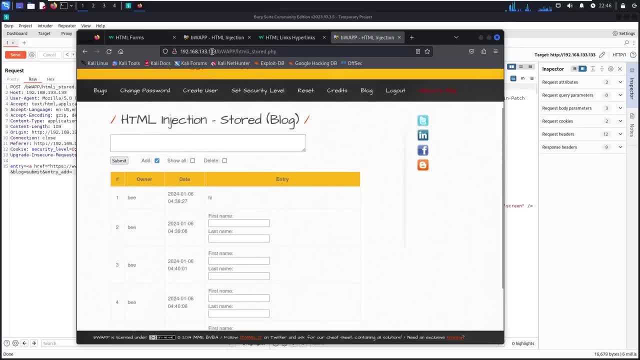 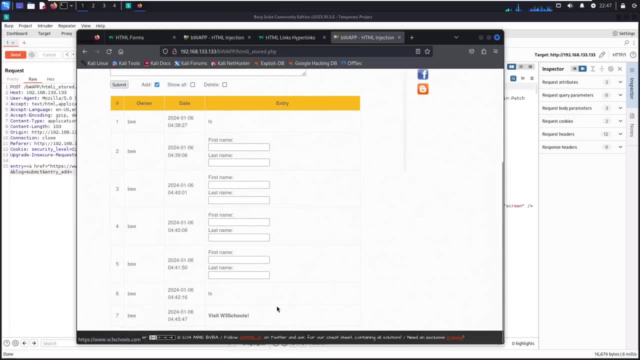 Okay, anyone who just accessing this page assumed that any user just visited this website and visited to this page At the time, he can able to see it. it's not like reflected- Again, I'm saying in reflected- what will happen. you need to send the URL to your victim. then. 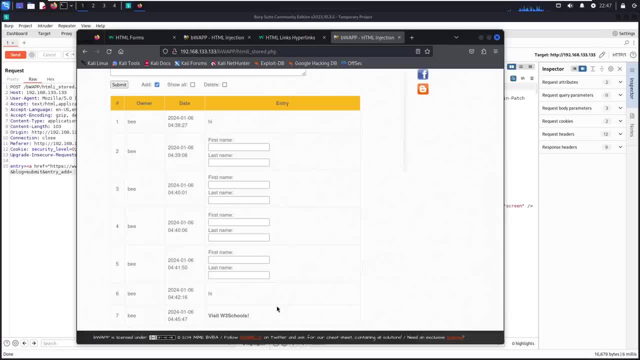 only he can able to see that form or something like that. You can also say it as a reflected URL. will work in phishing- Okay, mostly in phishing. steps are: if you want to steal username and the password of your victim, at the time it will work. 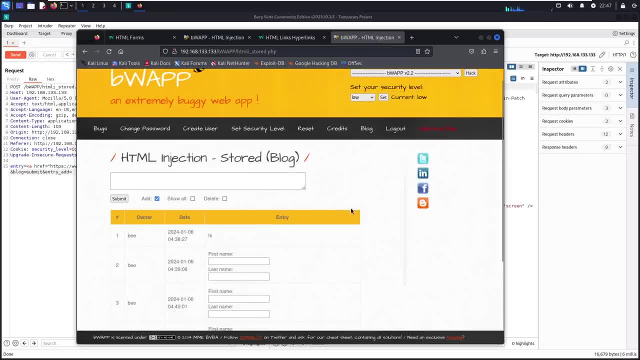 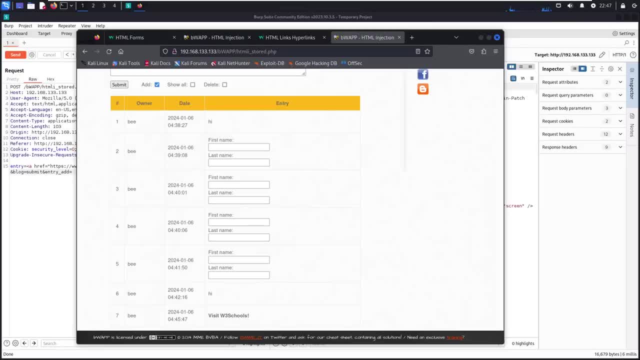 Okay, but mostly the websites are secure. Okay, but you, if you want, this is for beginners. okay, this is a thing You don't know about web hacking, then this is for you. right, It is a lot. again, I'm saying there is a lot. this is just a drop, okay, not drop less than. 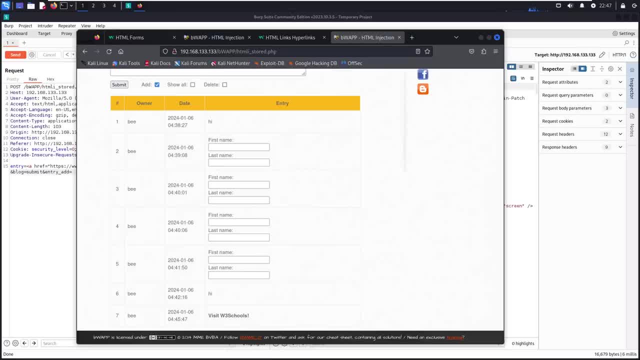 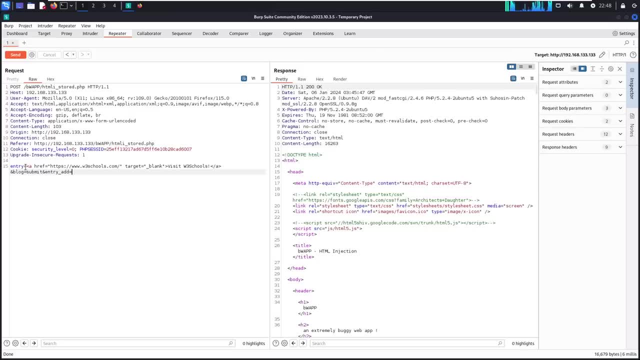 drop. Okay, Right, See, it is a button tag. Okay, Simple, Let me copy this button tag And instead of this one, let me add the button. paste the button tag here, Right, Let me send. submit. See the status code. is what here? 200.. 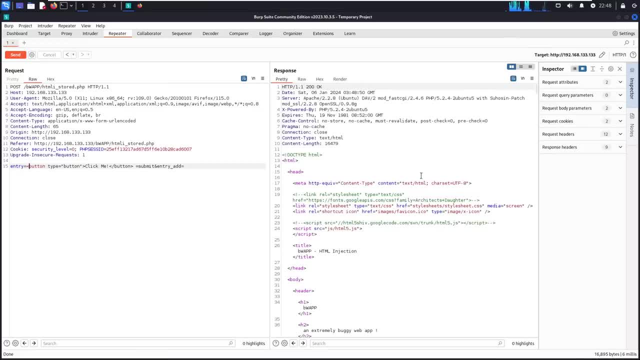 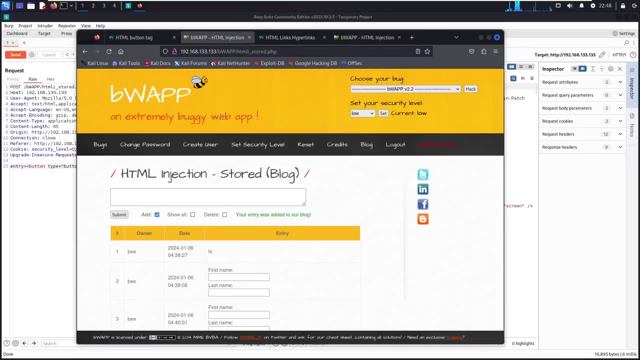 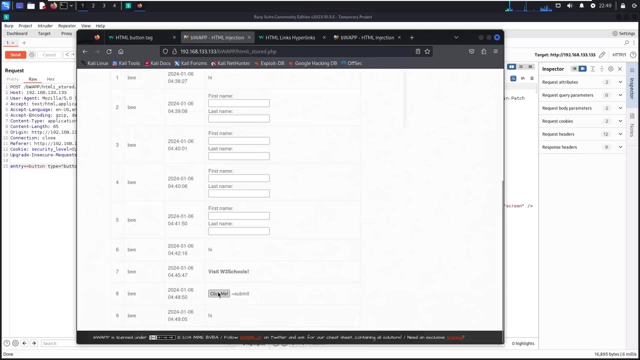 So that's why I just told you about the status codes. Just let me copy it, Copy URL or simple without copying the URL. Let me visit this site. Okay, let me refresh it. Here you can able to see: click here. button has been created. if I click on the button. 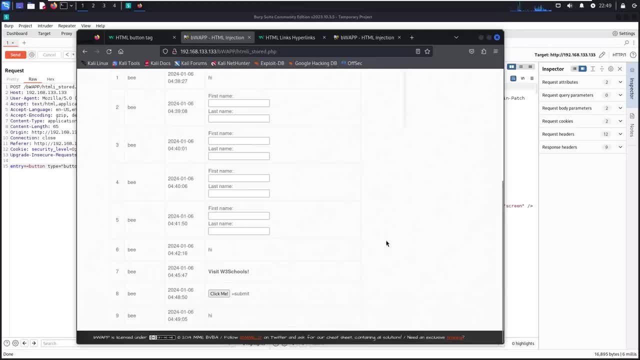 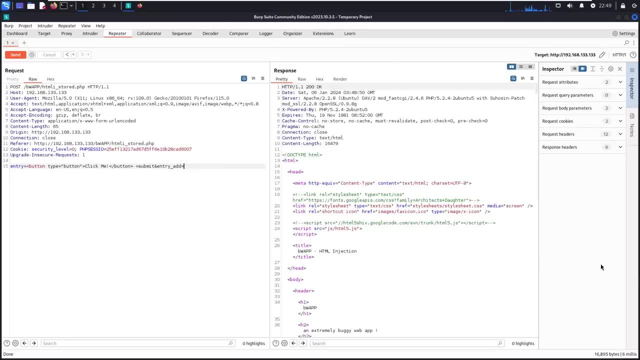 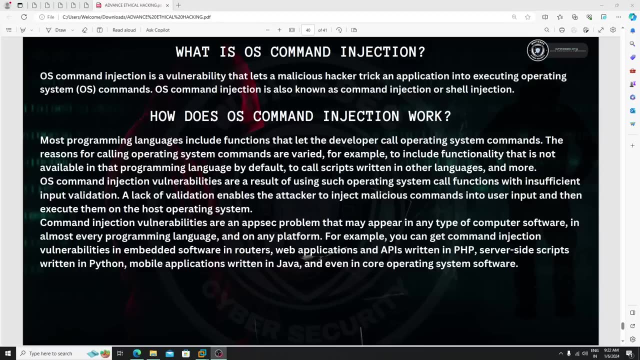 then what will happen if we redirect to another phishing site or something like that? Here you need to add the URL. So this is how it's going to work. Hope you guys get it. What is HTML injection? Hello guys, hope you're fine. in this classes we are learning about what is OS command injection? 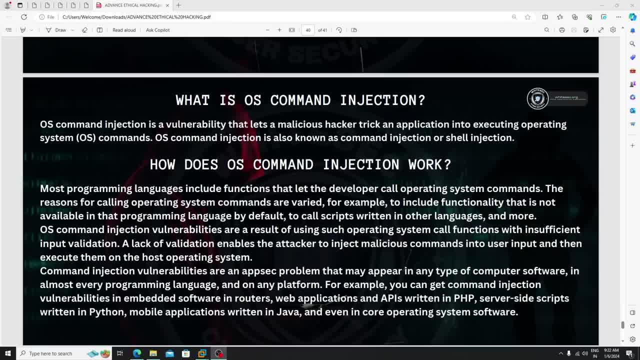 OS command injection is a vulnerability that, let's say malicious hacker it can application into executing operating system OS commands. OS commands, command injection is also known as command injection or cell injection. right Now, how does a command injection work? What is the OS? 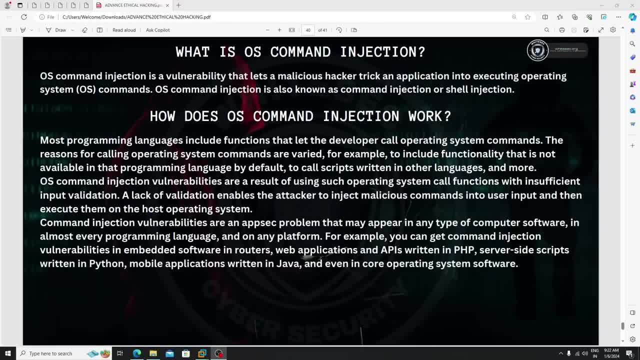 OS is a nothing but operating operating system. right, This is the thing. How does OS command injection work? Most programming languages includes functions that let the developer call operating system commands. The reason for calling operating system commands are varied, For example, to include functions: 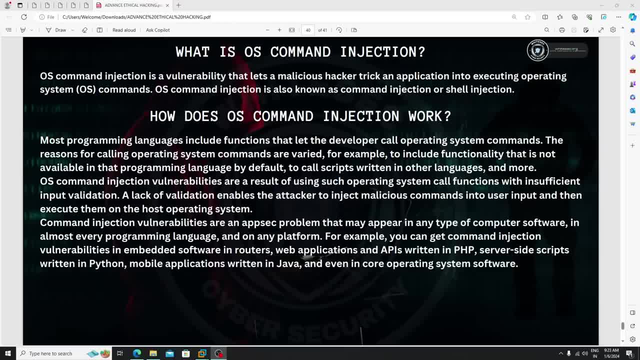 Include functionality that is not available in the programming language by default to call script written in other language and more. OS command injection vulnerabilities are a result of using such operating system call functions with insufficient input validation. A lack of validation enables the attacker to inject malicious commands into user input. 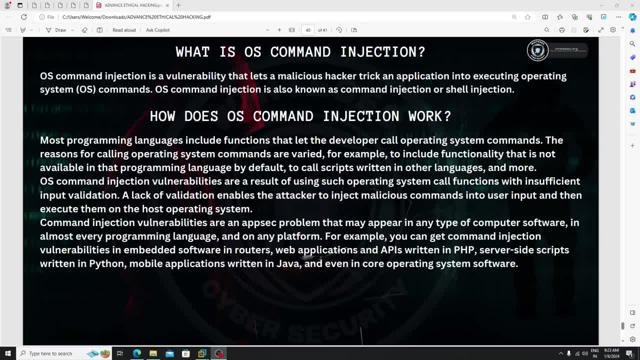 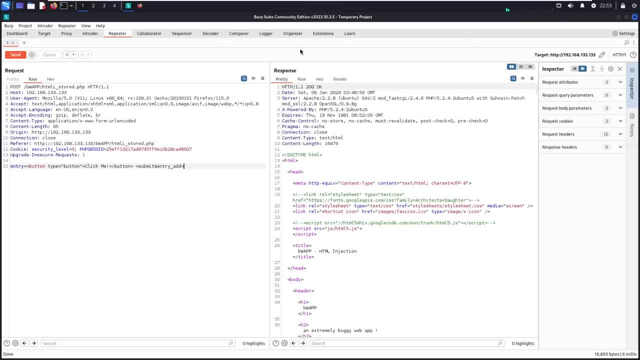 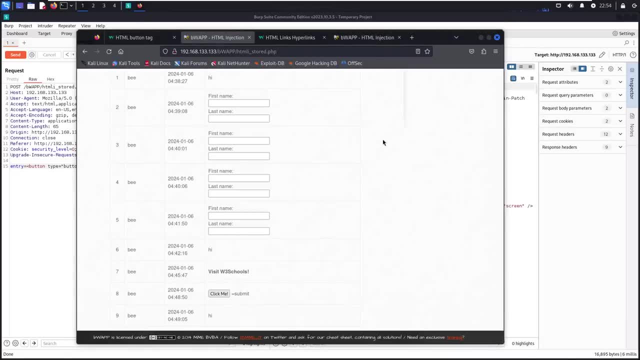 and then execute them on the host operating system. Now assume that you just found in any website you just found OS command injection. At that time, what will happen? You can able to take control on that website. Assume that that website is running in one server. 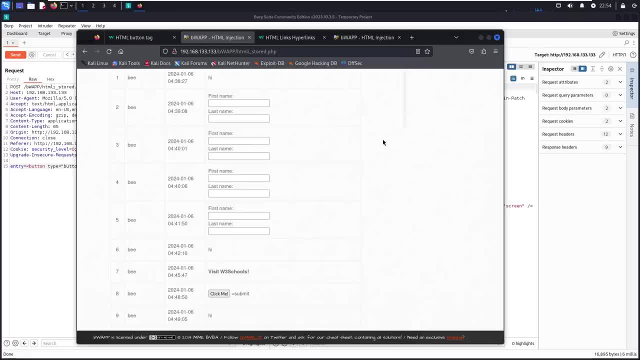 And you just found the vulnerability- OS command injection vulnerability on that website Simple. what will happen by? due to that vulnerability, you can able to control whole server there. So this is the thing. If you watch our penetration testing training, Okay, Hacking using Android class. 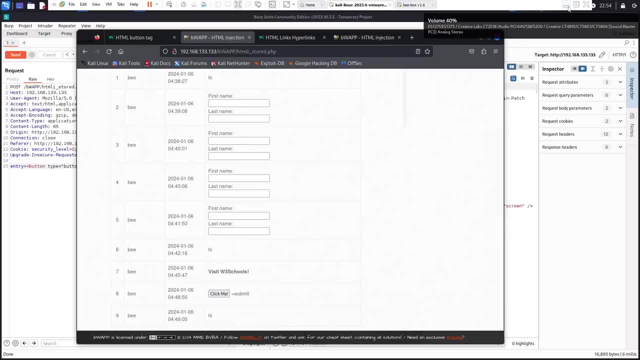 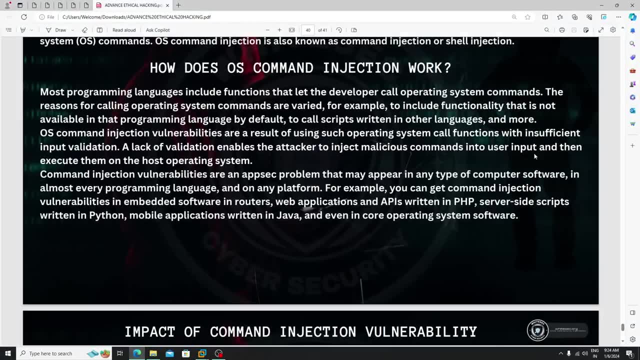 We just covered there, Okay, Like by using WordPress website, we just compromise the server there, Okay. So this is the thing: A lack of validation enables the attacker to inject malicious commands into user input and then execute them on the host operating system, which we just learned. command injection. 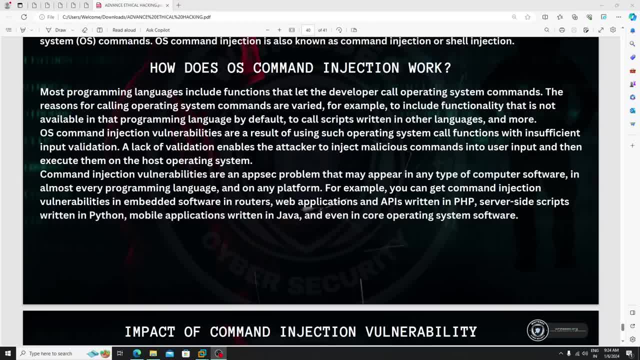 vulnerabilities or appsec platform. Let's see what it looks like. So, for example, in every server you can get a computer software in any of the language and on any platform. For example, you can get- you can get command injection vulnerability in embedded softwares. 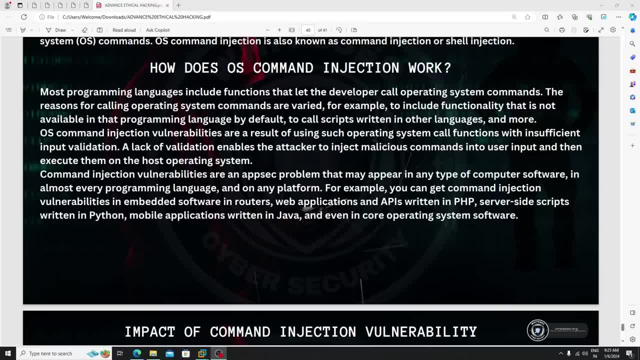 in router web application and APS written in PHP, server side scripts written in Python, mobile application written in Java And even in core operating system softwares. Basically, softwares are useful in. you can also say, say it as a framework. okay, now see here appsec is. 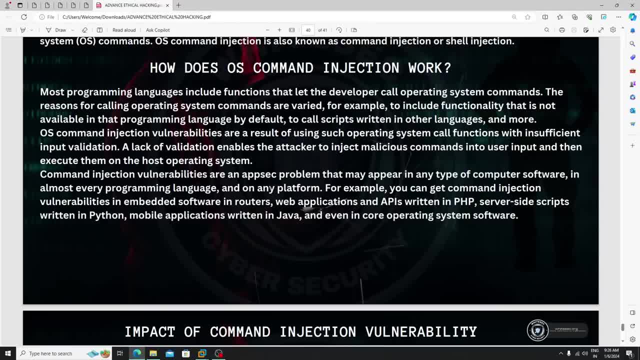 nothing but application security. it's not a big deal, okay. always remember: sec is nothing but security there. okay, the full form of sec is security, right? so this is a thing. now. in the next classes we will learn about the impacts of this command injection. let me tell you again. 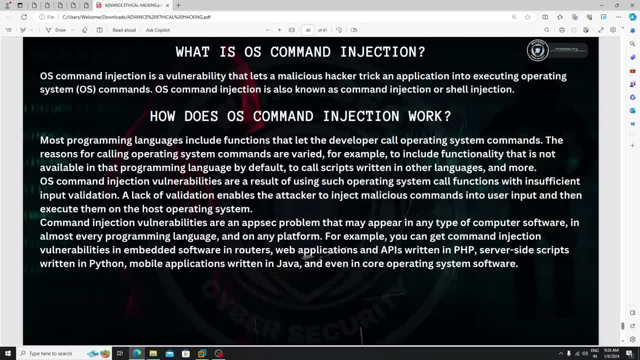 what is a command injection? in a very easy way. see, you just take any script, okay, which is written in python. okay, there they use some modules. okay, import os or something like that. there is a one, this is a module name os. okay, if you use that module in that script, then what will happen? 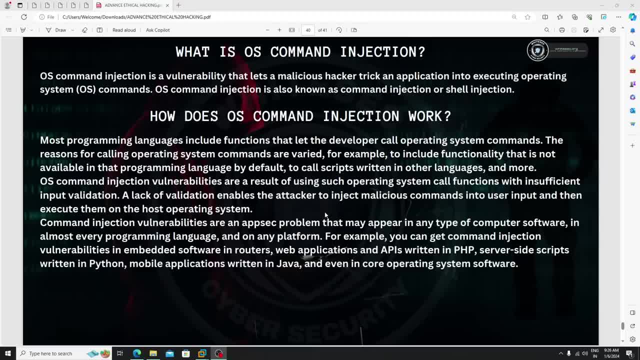 assume that there is a vulnerability in that script. assume that the code is not secured there. at that time, what will happen? by using the script, the attacker can able to hack the those systems. okay, like, assume that in my system that the the script is running, the service is running. let's. 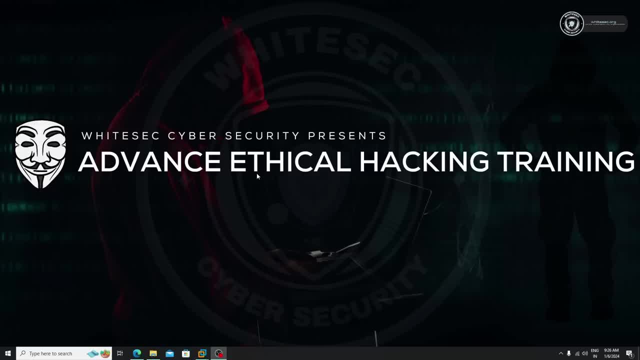 take an apache service. okay, in apache service, assume that it's vulnerable. okay, you can also take. take it as a. take an example of eternal blue as well. okay, if you. what happened there in eternal blue vulnerability? simple, after exploiting that system, we got the complete as is there. okay, like it's not a good. 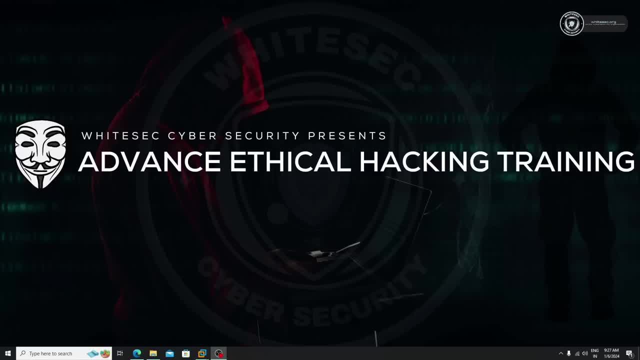 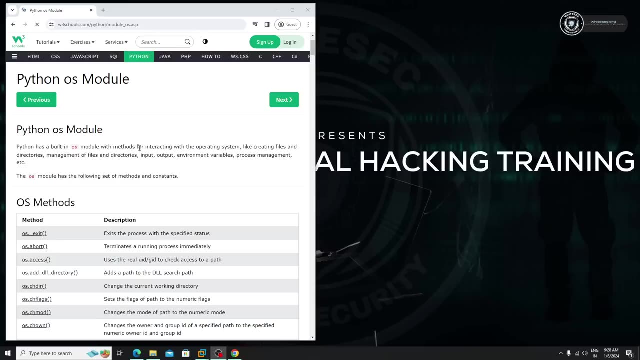 this one the example. let's take a python one only. okay, see in python what will happen. i just told you we use some modules okay, such as os module is here. okay, here it is os module. see, python has a built-in os module with with method for interacting with. 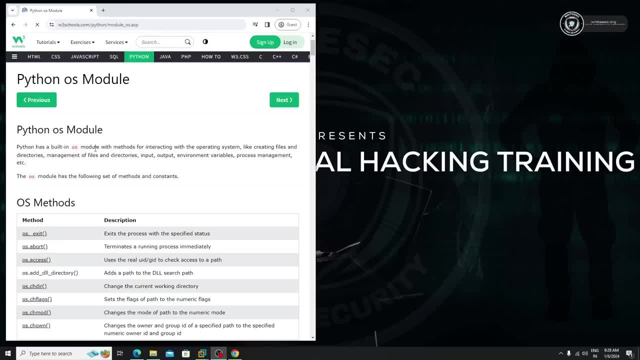 operating system. this module is useful to interacting with the operating system, like creating files and directories, management of files and uh directories. okay, input, output, environment, variable process management, etc. simple: if you got assumed that the- the service is vulnerable, okay, at that time, what will happen? assume that the service is using the os module. 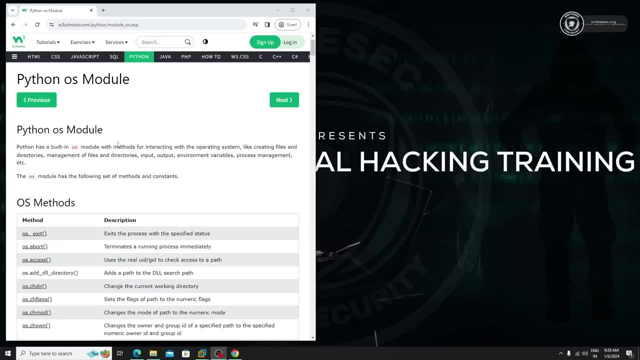 there, that time i can able to interact with the switch, with the, the, and i can able to do the same stuff which i do in command line interface. okay, this is the thing like: uh, in cmd, what i do basically in kali linux. uh, there is a terminal, is there there? what i execute there? simply if i type: 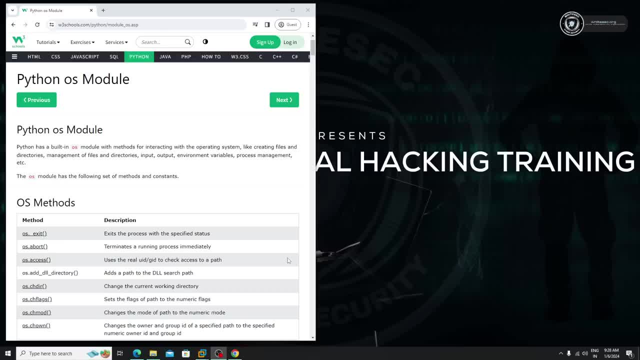 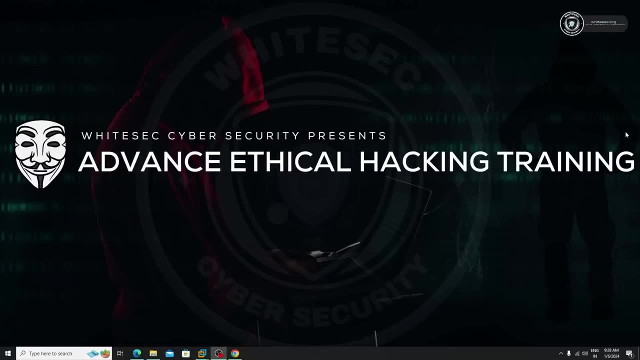 ls, then i can able to list out all the the files there. okay, simple, this will happens due to this module. okay, this is the thing. okay, if you are not getting it, it's not a big deal. okay, once you learn it, then you will get it. okay, just try to learn and do, do practice. okay, now in this classes. 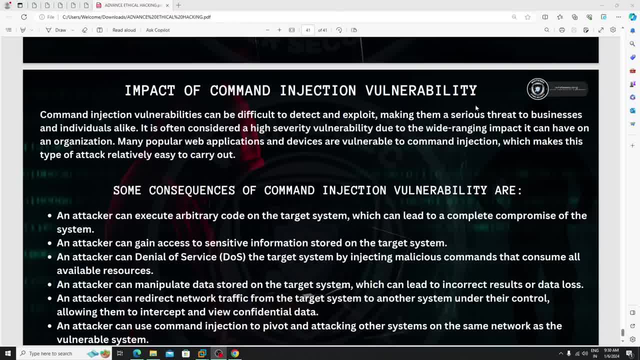 we are learning about impact of command injection vulnerability: see command injection vulnerability can be difficult to detect and exploit. this is the first thing. it is difficult to detect and to exploit it okay, making them a serious threat to business and individual alike. it is often considered as a threat to business and individual alike. it is often considered as a threat to business. 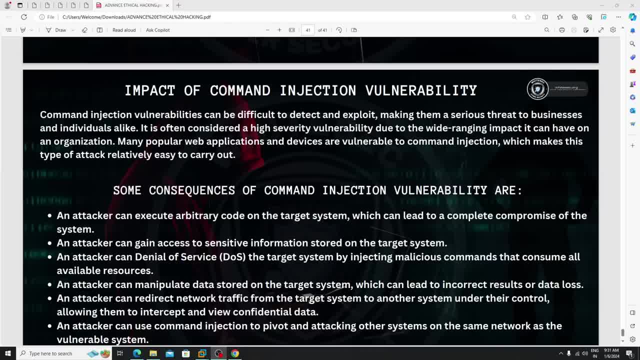 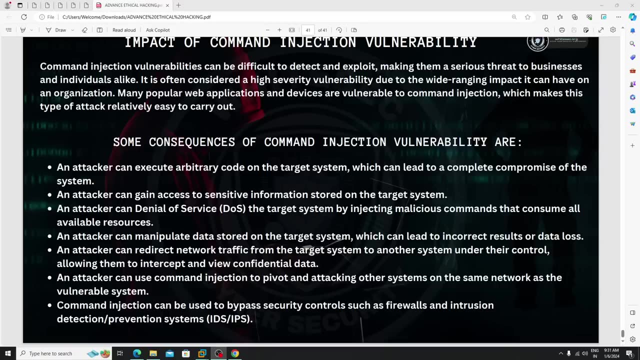 a high severity vulnerability due to the wide ranging impact it can have on any uh an organization. many popular web application and devices are vulnerable to command injection, which makes these types of attack relatively easy to carry out. see, there is a some consequences of command injection vulnerability. or an attacker can execute arbitrary code on the target system. now just take 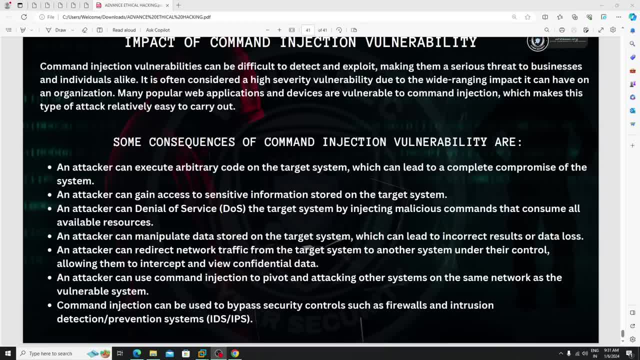 example of what this eternal blue vulnerability- okay, which can lead to complete compromise of the system. okay, if you watch our windows plantation training there, i just covered these things. an attacker can gain access to sensitive, sensitive information stored on the target system- okay, an attacker can denial of service the dos system by injecting malicious command that consume. 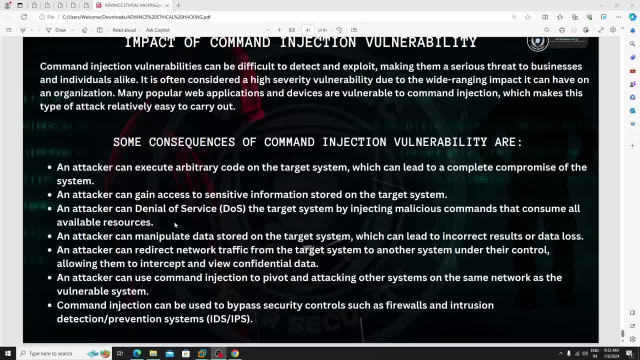 all available resources. he can able to shut down the server as well. okay, the system okay. or make make that system slow. an attacker can manipulate data stored on the target system, which can lead to incorrect results or data loss. an attacker can redirect network traffic from the target system to another system and under their control, allowing them to intercept and view confidential data. this is also very- this thing okay, very dangerous things. an attacker can use command injection to control a target system by injecting malicious data, and that system is a very dangerous thing. it is also very useful inRIP. 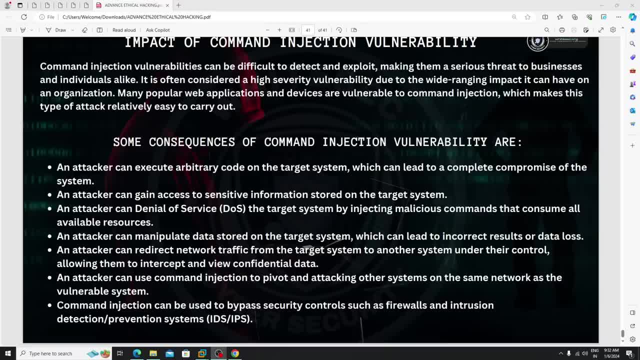 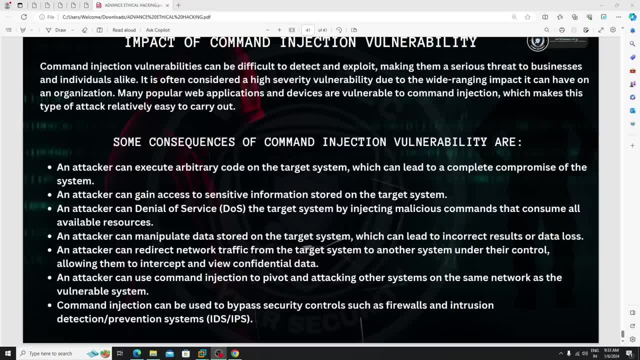 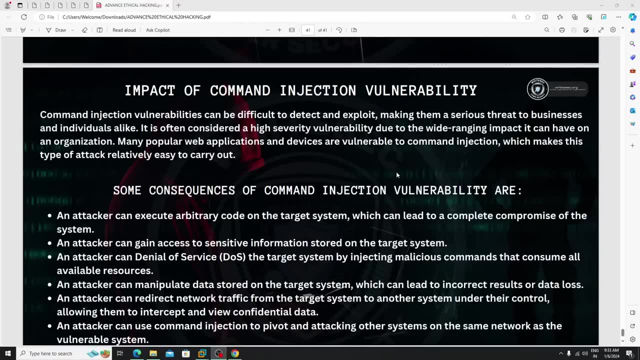 command injection can be used to bypass security controls such as firewall and intrusion detection. uh, intrusion detection and prevention system, which is known as ids and ips. right, so this is the command injection. assume that you, if you found the command injection vulnerability in any website- uh, you are hunting some bucks, okay, in buck road or something like that. if you found the 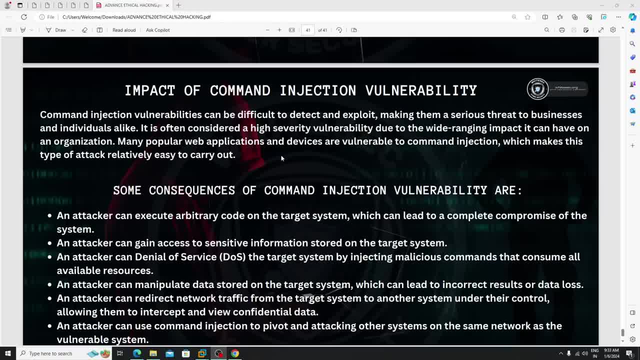 command injection vulnerability there, then they pay you a lot. okay, this is the thing. this is a very severe vulnerability. it is like here it is. it is difficult to detect, okay, but you can able to detect it once you do a see, if you perform lot of reconnaissance on any site at the time. 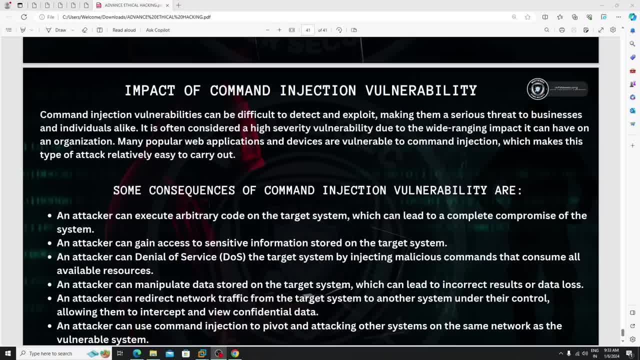 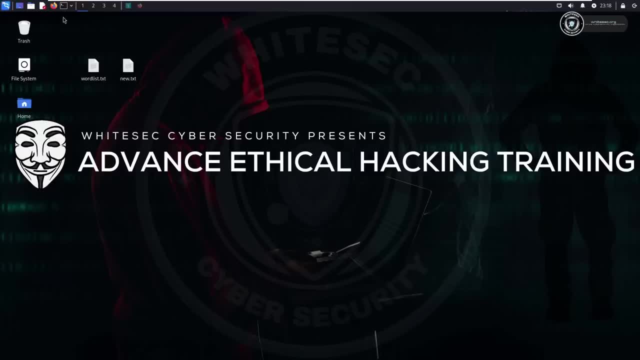 there are chances, are there that you can able to find vulnerable days? okay, this is the thing, right, hope you guys get it. in the next classes we are learning about how we can able to find it now here. before performing the command injection, you need to know some basic linux commands here. okay, see, assume that if i type here. 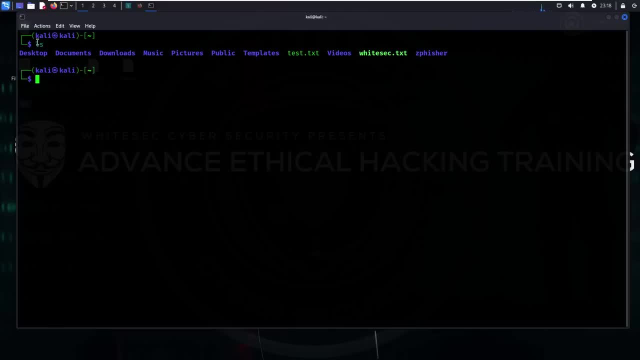 ls, then what will happen? i can able to list the commands here. right, sorry, i can able to list what? okay, what folder is there? okay, something like that. now here: if i type pwd, then what will happen? i can able to see present working directory there. okay, now assume that i want to execute this two commands at the same time. at that time, what i? 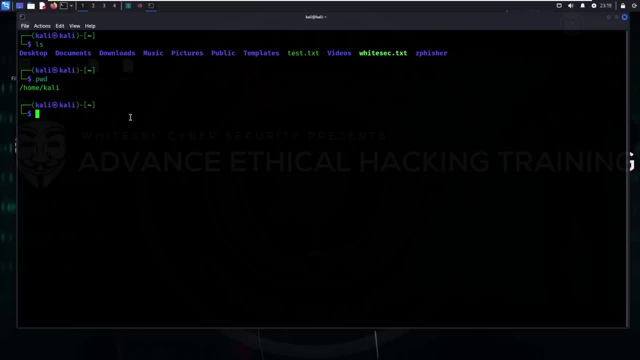 need to do simple. i can use semicolon here, ls, then semicolon, then let me type here pwd. then what will happen? the two commands has been successfully executed and i can able to see here the same things. right, i can able to see the files and folders and also i can able to see the pwd results. 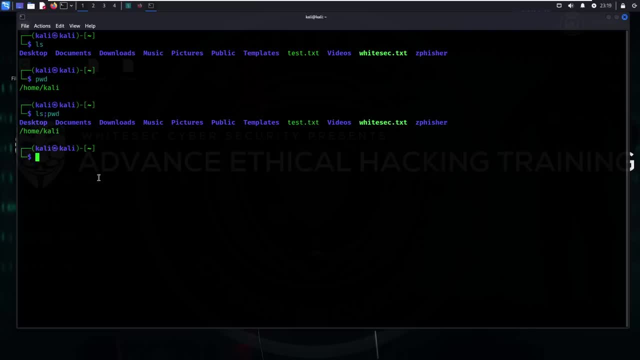 as well. okay, so this is the thing now, if i use- uh, sorry guys, if i use and and, okay, and it is, and here it is- if i use, and then also it will work like that. only okay, see here successfully executed the first in, and what will happen means it will execute pwd. then this one, right, okay, if i use pipe. 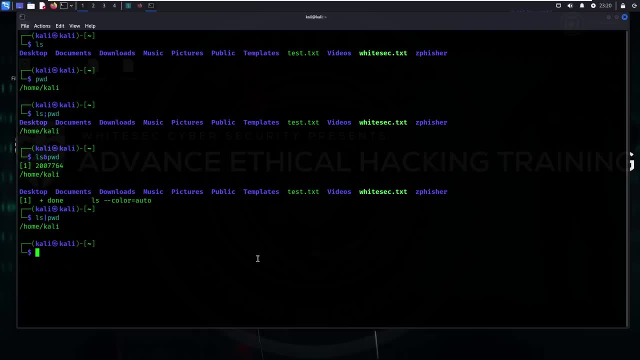 if i use pipe, then what will happen here? let me use now. see pipe in pipe. what will happen means the first command which you just type there will get ignored and the second command will be executed. this is the thing. see here what happened. ls has been executed. 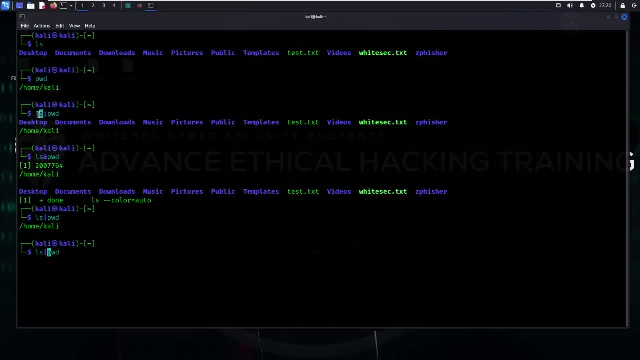 executed in semicolon. ls has been executed and pw also has been executed and i can able to see the results. but in pipe, just see what is uh, what are the results here. if i execute it, then ls, i can't able to see that. okay, the results of ls. but i can able to see pwd commands there. 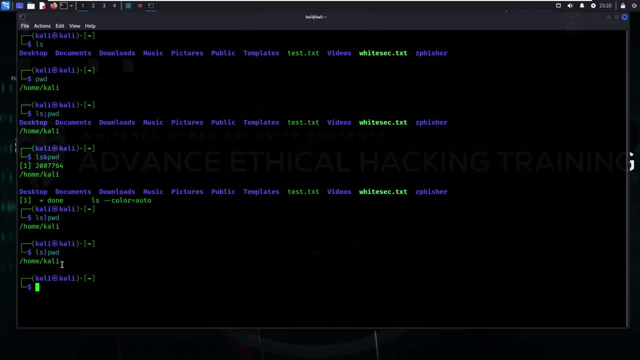 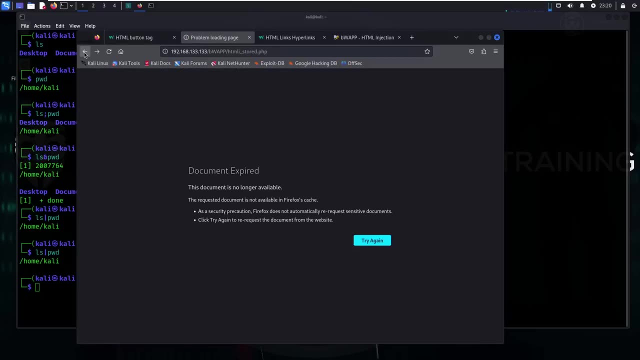 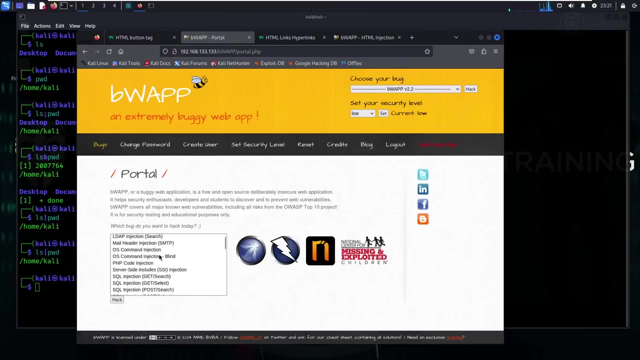 okay, sorry, pwd results. this is the thing. okay now here. let me type here: hack now let's go with command os command injection. let me type here: hack now. here there is dns lookup. here you can add any uh site or something like that if you type look up there. 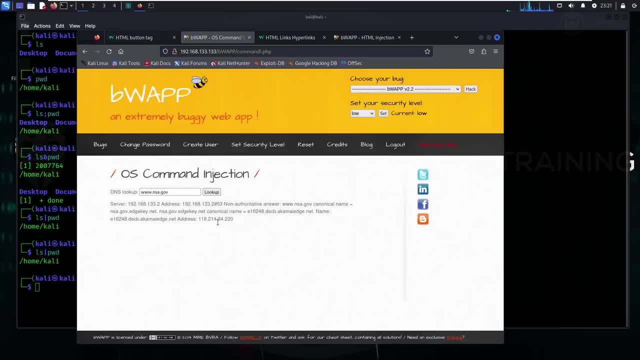 you can able to see the site details, right, ip address and these things now assume that let me use semicolon here. okay, let me use semicolon, let me type ls, then what will happen? i can able to list out all the files. hope you guys can able to see it. it's a critical, vulnerable day. 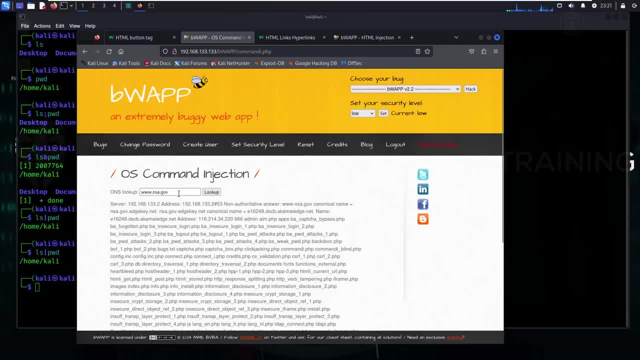 okay, this is the thing. if i use uh this thing and and if i type ls or any, any command, linux based command, why i am typing linux space command here? because the server is running on linux base. okay, see, it's using the ubuntu. ubuntu, right, this is the thing. assume that if you are uh target server in running in windows. 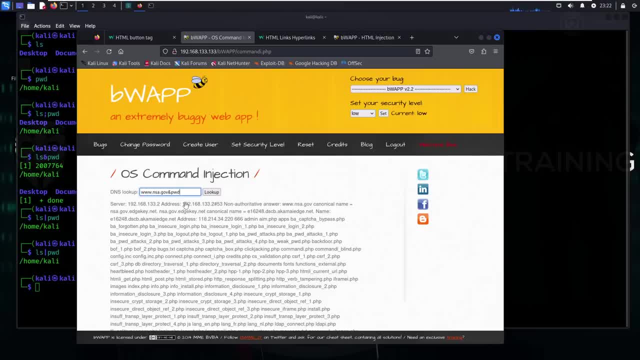 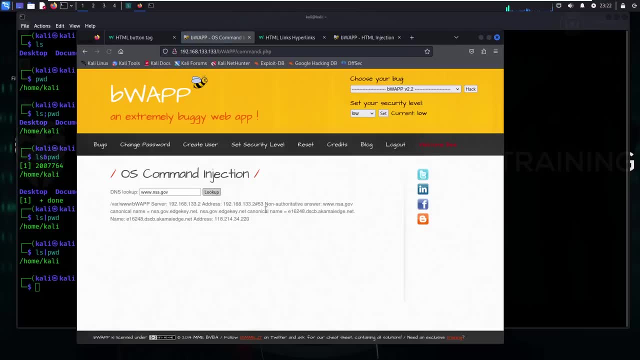 at that time you need to execute the windows commands here. this is a simple things which you no need to worry. okay, now here, sorry guys, if i click on pwd, then here i can able to see what www b wrap. okay, this is the thing. now, if i see the, if i click on me. 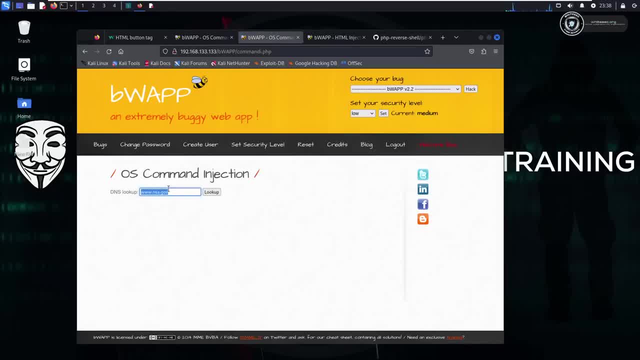 now, if i type uh, this semicolon and if i type ls here now, it's not executing the ls right because the semicolon has been filtered there. right now, instead of adding the semicolon, let me add and sign there. okay, and let me add ls now it's also filter and sign. also filter. if i use pipe, pipe is here and let me type. 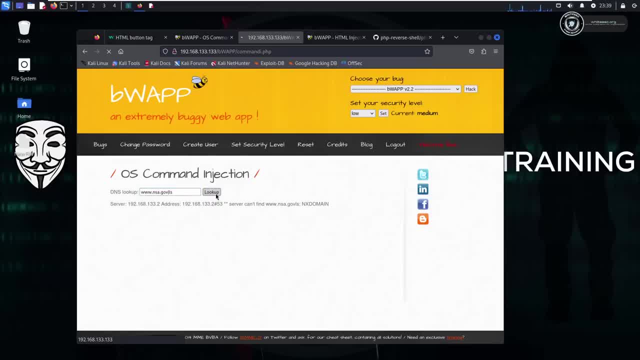 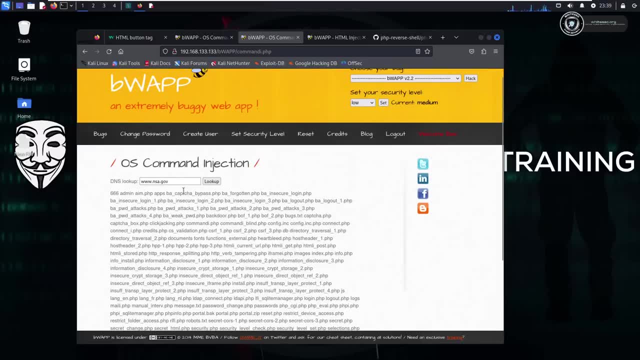 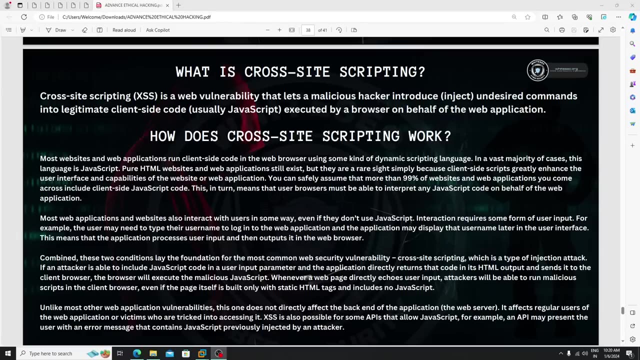 ls. now pipe is working there. okay, this guy didn't filter uh pipe there. okay, this is the now. in this classes we are learning about what is cross-site scripting. cross-site scripting xss is a web vulnerability that lets a malicious hacker introduce, inject undesired command. 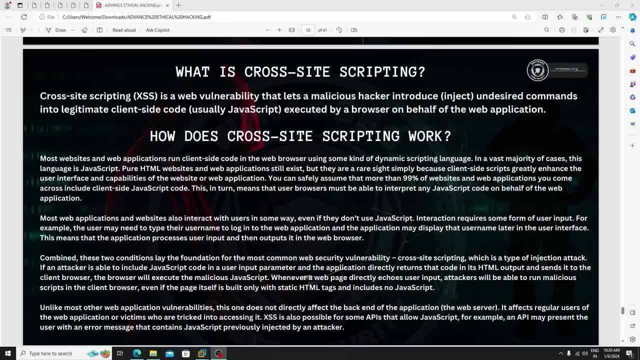 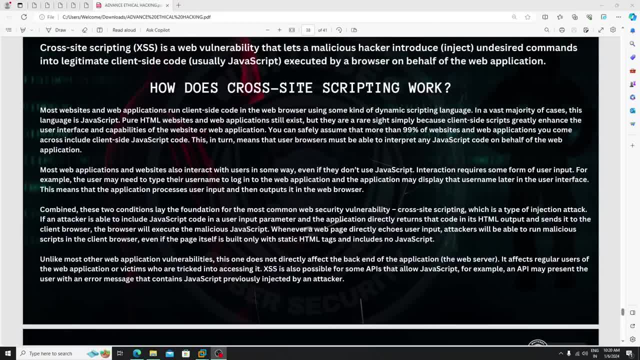 into legitimate client-side code, usually javascript, executed by a browser on behalf of the web application. how does cross-site scripts work? most websites and web applications run client-side code in the web browser using some kind of dynamic scripting language. in a vast majority or majority of cases, this language is javascript, pure html. website and. 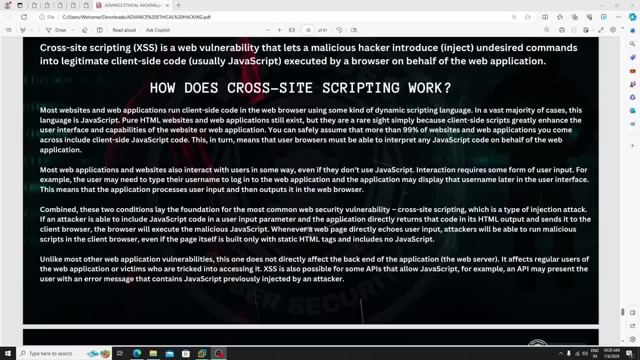 web applications still exist, but there are a rare site simply because client-side script greatly enhance the interface and capabilities of the website or web application. you can safely assume that more than 99% of websites and web applications you come across across includes hindsight JavaScript code. this is this in turn. 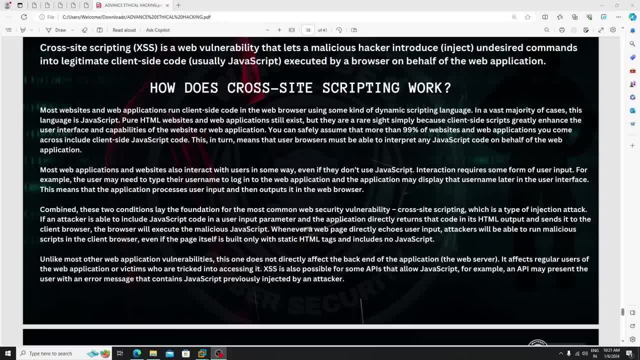 means that user browsers must be able to interpret any JavaScript code on behalf of the web application. most web application and websites also interact with user in some way, even if they don't use JavaScript. interaction requires some from of user input. for example, the user may need to type their 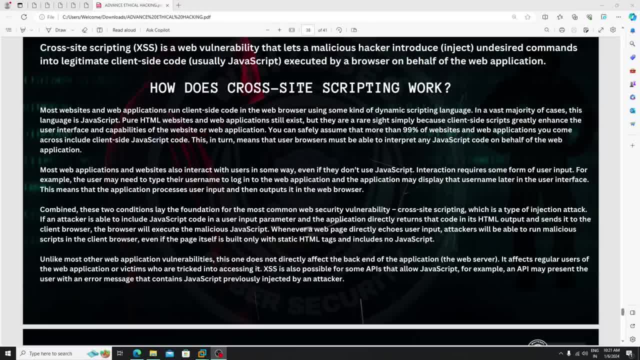 username to login to the web application and the application may display the username later in the user interface. okay, now assume that you just there is a one website there. you just type the username there, simple, you can see your username there. okay, like assume that I just search something. like assume that. 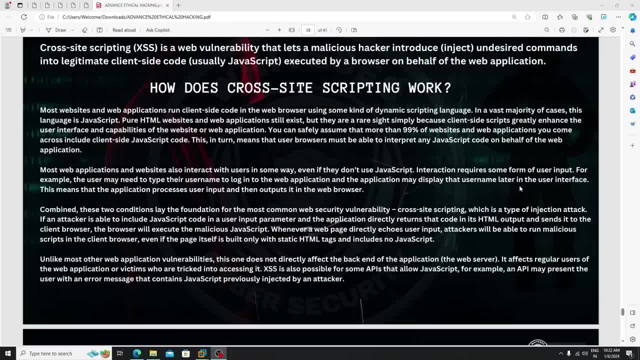 there is a Amazon. I just search for hack RF or any application or any product. simple it will show the product name there. or just take an another example: you just type your username and password there. then you will see the one page welcome and welcome your name. okay, assume that your name is John at the time. what will happen? welcome John. 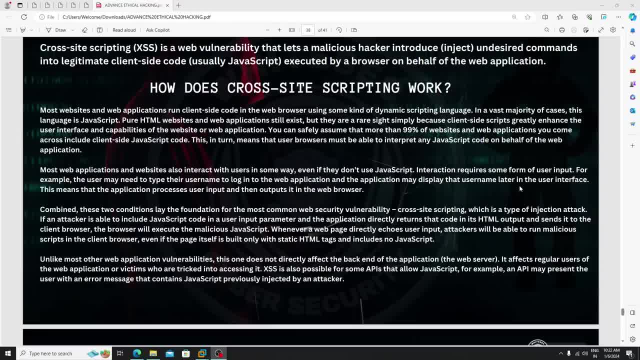 it will display like that: okay interface. this means that application process, user input and their output it in the web browser combined- sorry, browser combined. these two conditions lay the foundation for the most in common web security vulnerability, which is cross-site scripting, which is a type of injection attack if an attacker is in 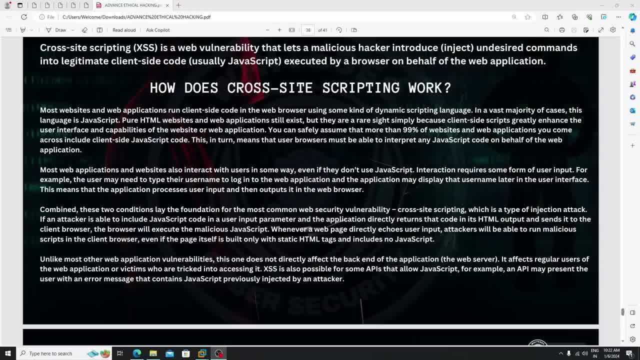 able to include javascript code in a user input parameter. what is a user input parameter here? it might be any form or anything where the user type something okay, or any comment section which you just saw in html injection. like we, there is a forms. are there okay? where we just added our. 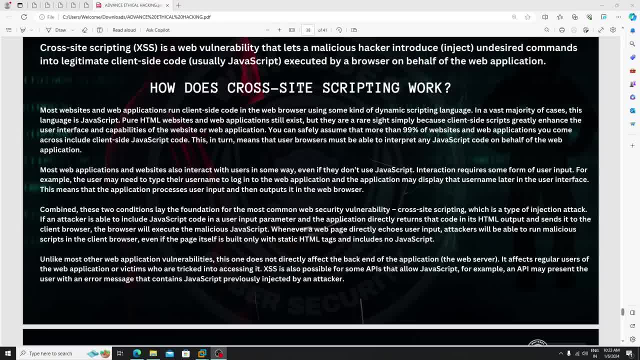 payload the same thing and the application directly return the code into in its html output and sends it to the client browser. the browser will execute the malicious javascript whenever a web application direct echoes user input, attacker will be able to run malicious scripts in the client browser even if the page itself is built only with a static html tags and includes 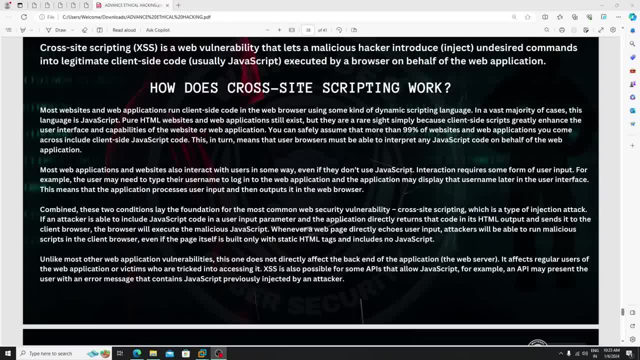 no javascript. even there is a no javascript, still he can able to run the malicious scripts in client browser. unlike most applications- other application vulnerability- this one does not directly affect the back end of the application. see, this is the thing. this does not. this one does not directly. okay, if it will affect, but not. 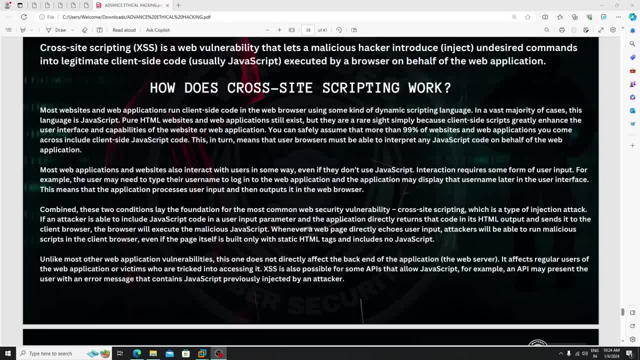 directly affect the back end of the application, the web server. it affects regular user who use that application. this is the thing you see. it's affect regular user of the web application or victims who are tricked into accessing it. xss is also possible for some apis. 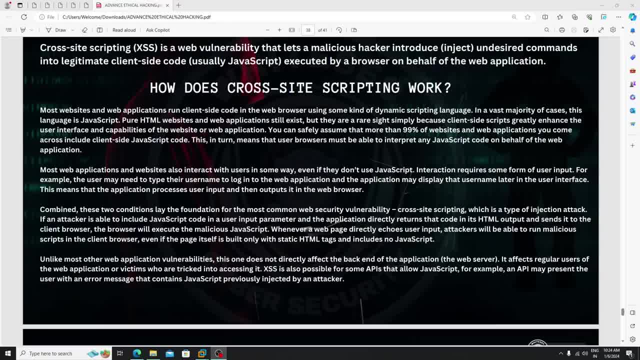 xss is also possible for some apis that allows allow javascript. for example, an api may present the user with an error message that contains javascript previously affected by an attacker. so this is the thing. now. in the next class, we will learn about impact as well. in this class, we are learning about what is the impact of. 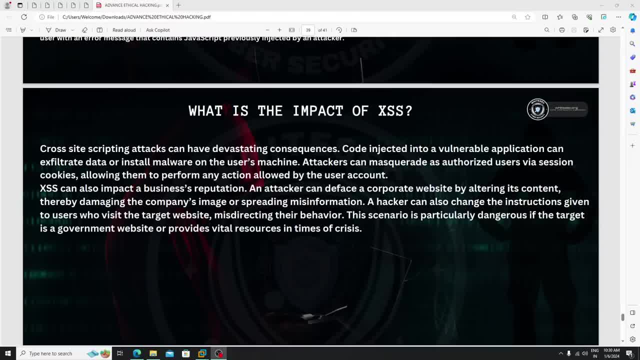 xss broadside scripting attack can have a devastating consequences. code injected into a vulnerable application can exfiltrate data or install marvel on the web server. so this is the thing that ties down the user machine. attacker can masquerade as authorized users via session cookies. 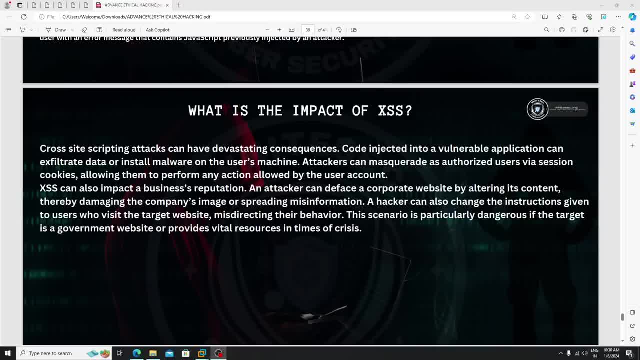 allowing them to perform any action allowed by the user account. xss can also impact a business reputation. an attacker can deface a corporate website by altering its content, thereby damaging the company image image or spreading misinformation. a hacker can also change the instructions given to user who visit the target website, misdirecting- sorry, misdirecting- their behavior. this scenario. 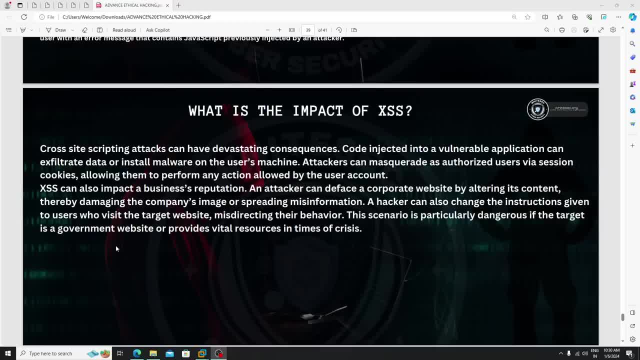 is particularly dangerous if the target is a government website or provide virtual resources in time of crisis. basically, here attacker can able to the main aim of attacker here: damaging company reputation. okay, like he can add any message there, he can add any image kind of serves. okay, this is a thing right. so this is also basically by using this attacker. 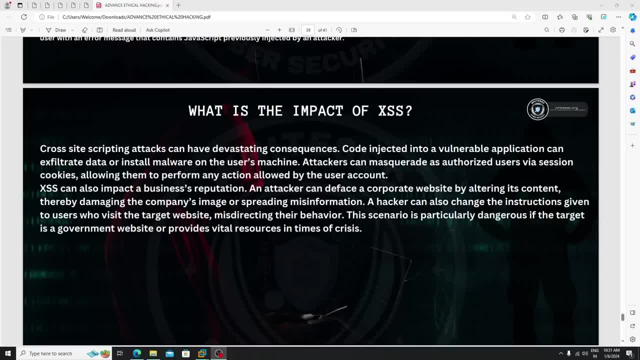 can able to steal user cookies as well. okay, you can also do XSS to RCE as well. it is a little bit kind of intermediate topic, okay. so this: there is a lot of things by XSS you can attacker can able to achieve. okay, this are the main reasons which we just added here. 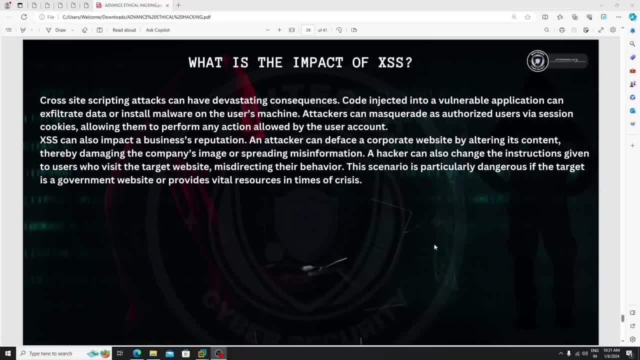 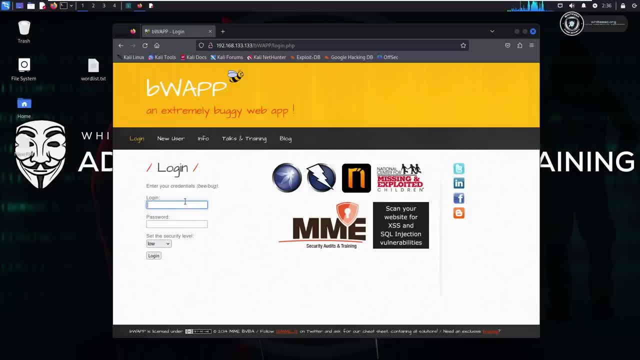 right, So if you want to know more about the XSS and how to use it. So in the next classes we are learning practically how we can able to do this XSS. now in this class, we are learning about how we can able to find XSS vulnerability. okay, now let us. 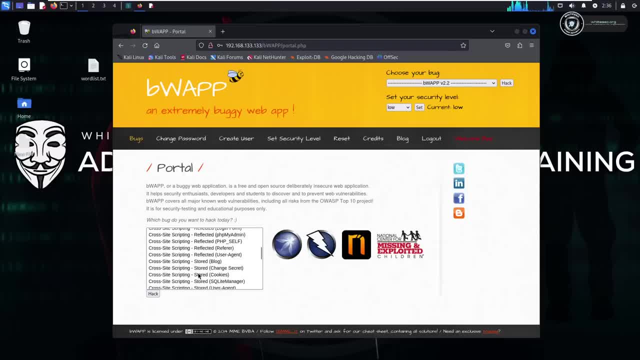 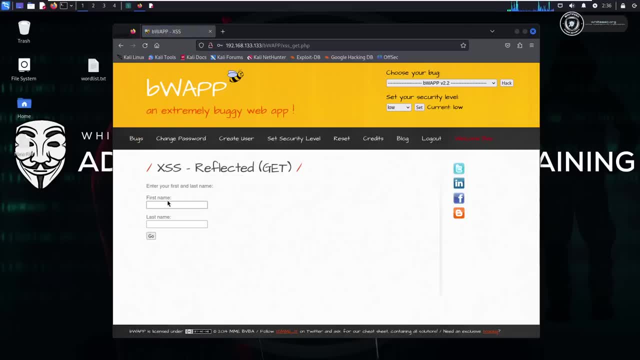 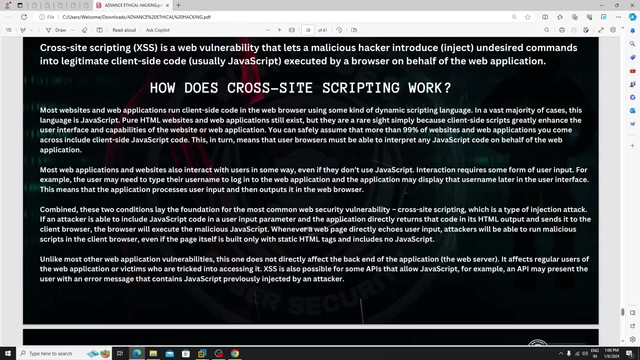 select cross site scripting reflected. I just showed you about what is reflected, right? okay, so we are going to see, for example, the user. this point, okay. the user may need to type their user name to login to the web application and the application may display that user name later in the user interface. this means that the application process user input and 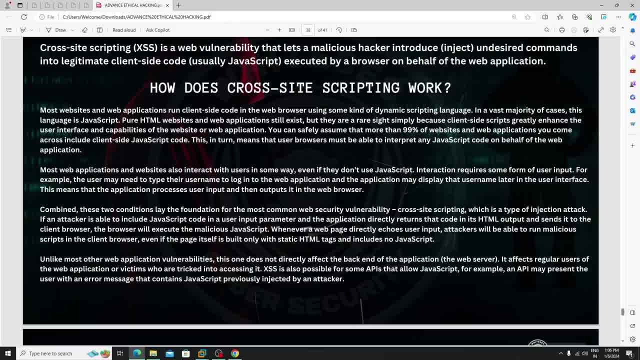 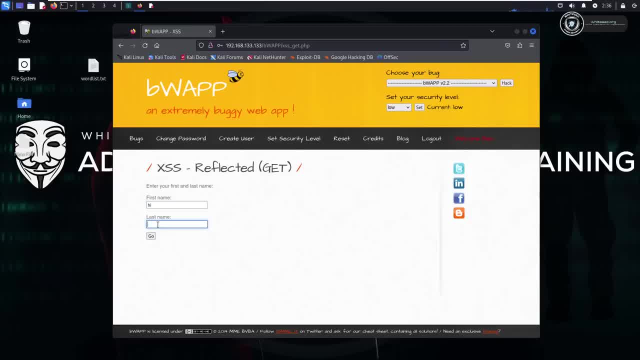 then output it in the web browser. the simple thing is assumed that if I type here something like hi, and let me type here, hello Now. see if I type here, hello Now. see if I type here, hello Now. see if I click on go here, you guys can able to see the the things which you just 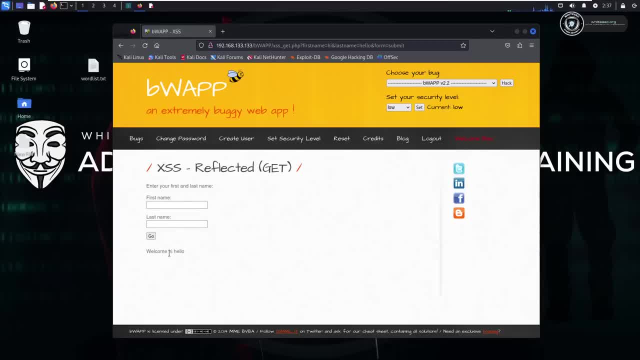 type there. okay, now, the same thing which you, which we just in the HTML injection class, just inject the payload here. okay, in this kind of user input fields, okay, and also I just told you about this, things right about reflected how the in get request. what will happen? the data which you just type there will be going URL. 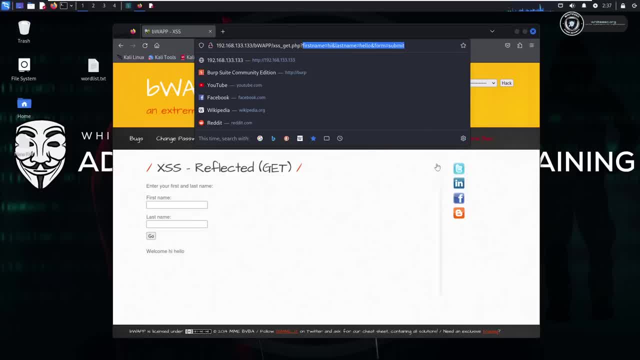 In the in URL, sorry, through URL, right now. this things is known as parameters- which is in front of equal. okay, this is known as what. this is known as parameters, not the value which you just typed here. this is not a parameter. okay, this which which end with equal right. 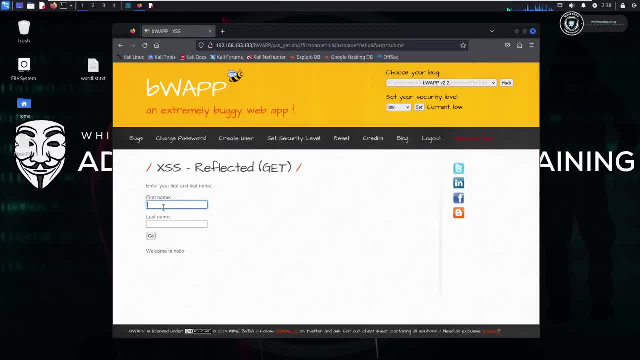 okay, now here, Just let me type in normal javascript payload here. Okay, Okay, Let me start with the script. Let me close this and let me type here alert 1 and let me close that script here. right again, I am saying the first thing is you need to check that it's reflecting or not. then 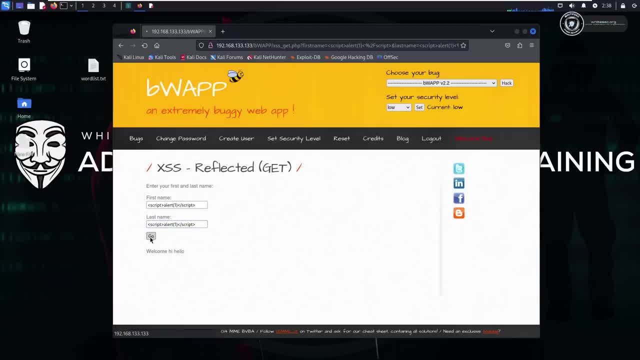 just execute it. if I click on go in here, you guys can able to see the pop-up right. so that means it is vulnerable. okay, this is the thing. now, here the attacker. what he do means he inject the malicious payloads here to steal cookies, this kind of stuffs. simple, how, how? 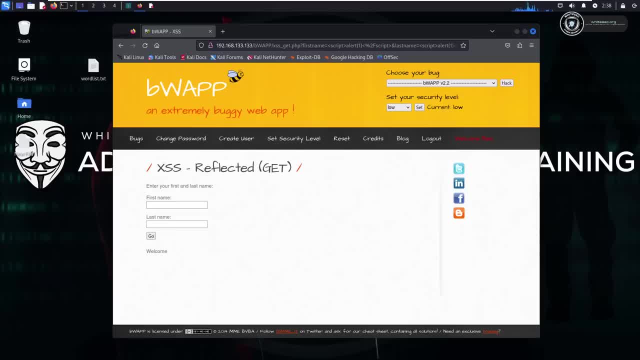 the attacker can able to steal it the simple, by using payloads. okay, first of all, he need to find the vulnerability in it. right now, this is a reflected. I just told you, for reflected, what we need to do. we need to send the URL there, we need to send the link. but in the 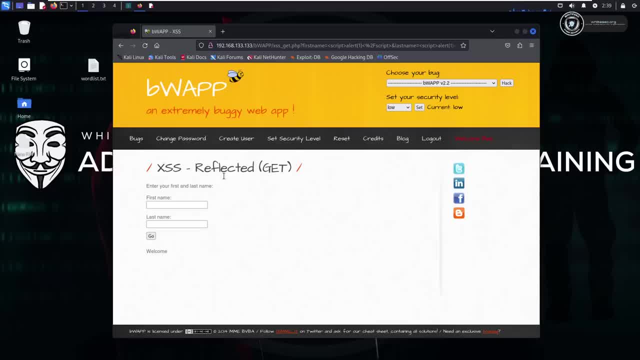 stored. what will happen? it will be stored in that website. anyone who is accessing that website can able to see it. okay, this is the thing now here. let me do one thing. just let me use the same script here instead of let me type here: documentcookie. just see what. 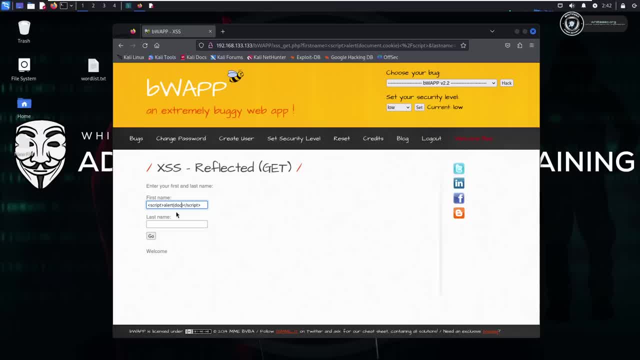 will happen. now you know about cookies, then it is excellent. if you don't know, then try to watch our ethical hacking training. just let me type here cookie right now, see what will happen. but click on, go here you guys can able to see the user cookies. simple the attacker can able to steal. 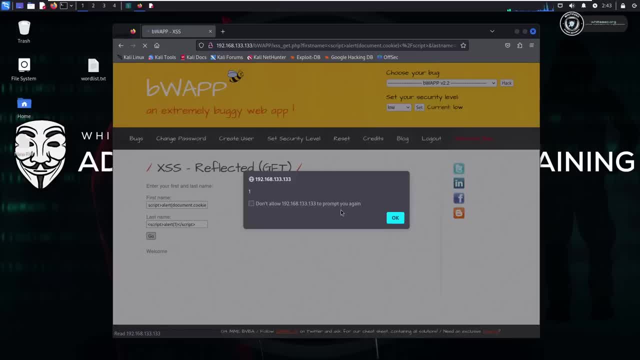 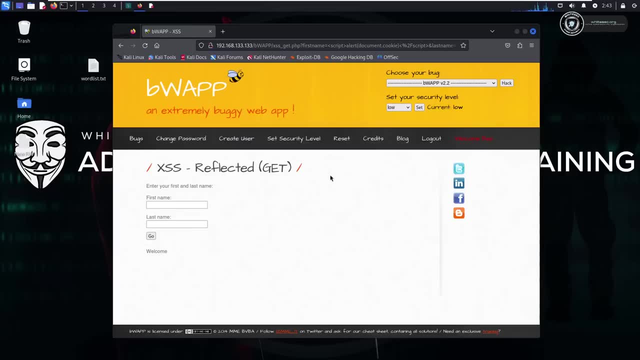 it. okay. what he need to do? simple: he need to send the URL to his target, then he can able to do it. okay, this is the thing now. the this is. this is a reflected one. now, let us see stored as well. okay, let us go with stored. okay, the same thing which we, just, in the, did in the last classes. 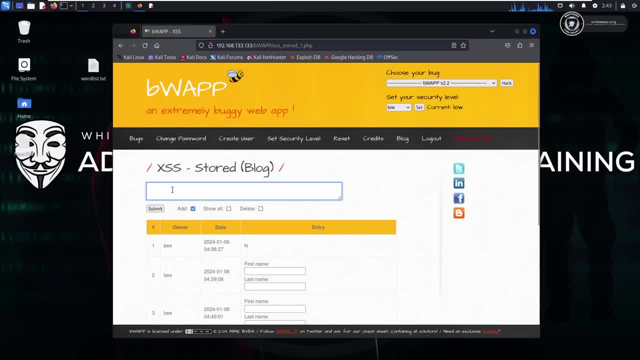 now here also. let me do one thing: see in stored what will happen. you no need to send any kind of URL or something. assume that if your target using this website and he just visited to this page at the time, he can able to see it and also the attacker can able to steal those cookies. okay, how he can able to steal it. basically. 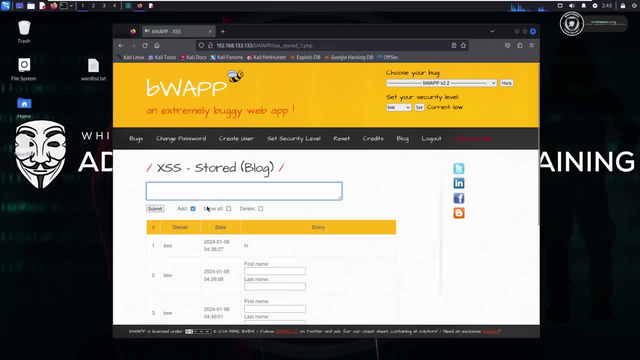 the process go remotely. okay here. instead of adding documentcookie here, the attacker will add the URL of his website. okay, first of all, the attacker will host one website there. then let me show you practically now. first of all, let me see for the stored as well. same thing. 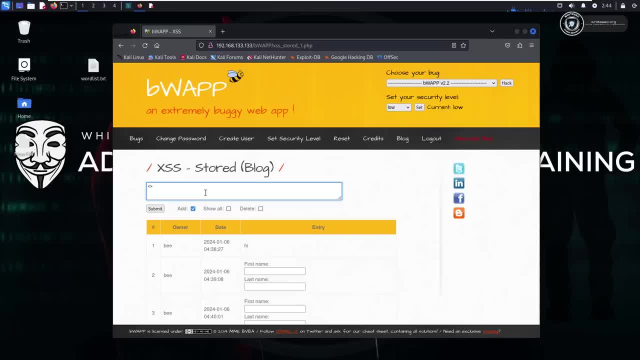 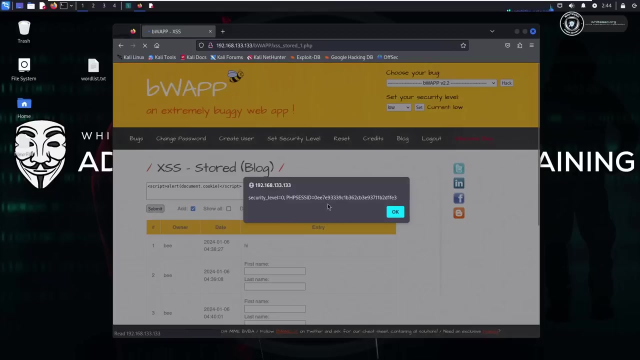 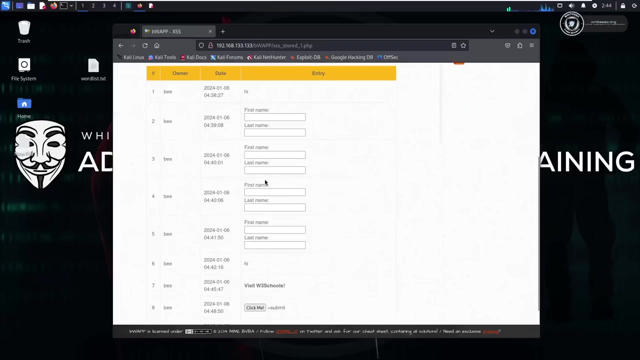 use this script now. let me see for the stored as well. same thing. let me use this script alert here. let me use document: documentcookie. let me close this script now. if I click on submit, then what will happen? it is work, okay, now here. anyone- okay, anyone- who access this web page will see that pop up. this is the 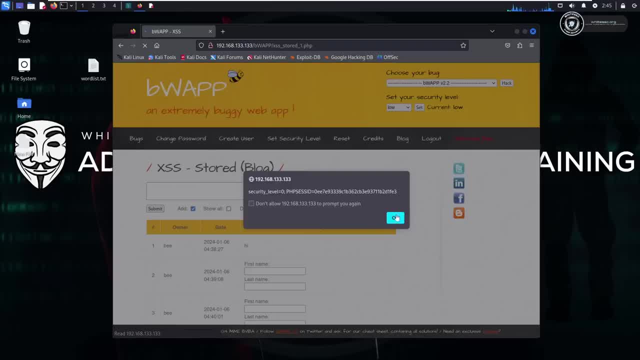 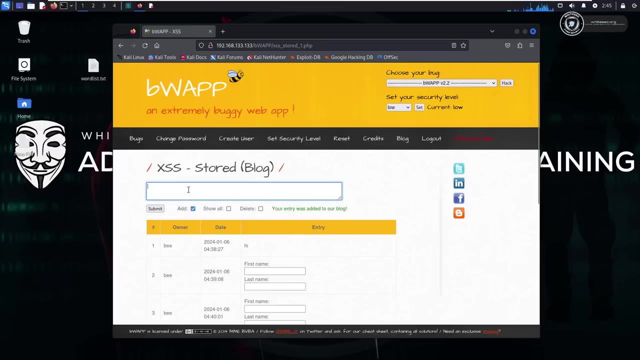 thing, right, simple. see, let me refresh the page. I can able to see it. okay, see, I can able to see it. this is the thing, see, it is created. now the attacker, what he, what he will do, he will- I just told you right- will host kind of website there. 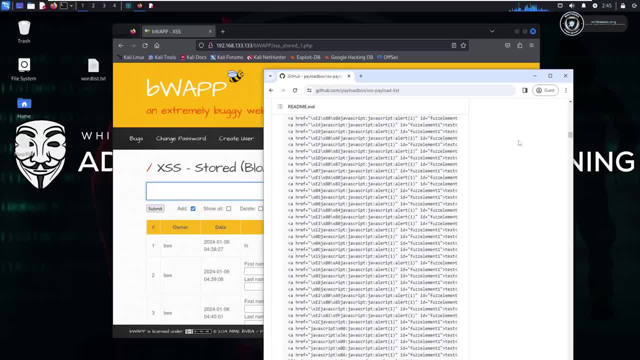 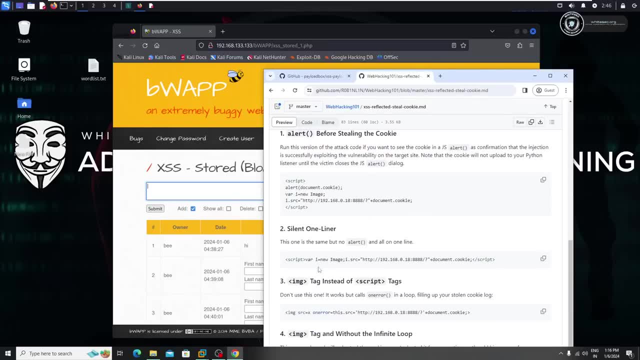 from there he can able to steal it. let me show you the payload as well, how it is look like. okay, here is a payload. this is a one liner one. here, instead of IP address, you can also add the domain name. okay, simple, no need to add anything simple there, you just need. 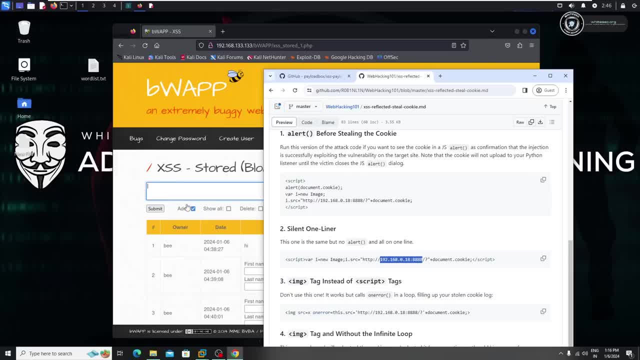 to execute where the vulnerability is here at the time. what will happen if any user visit that, your website, that page? what will happen means in your site you can add the domain name. what will happen means in your server it will generate some logs. in that logs you guys can. 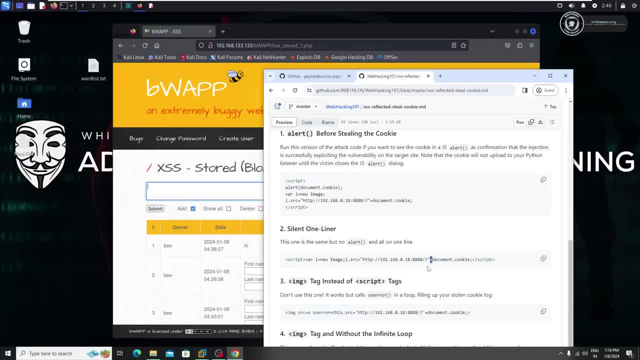 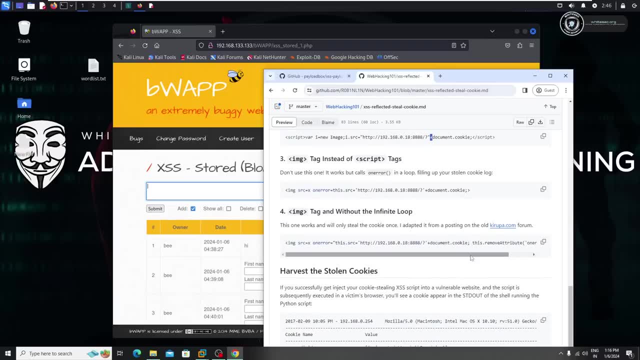 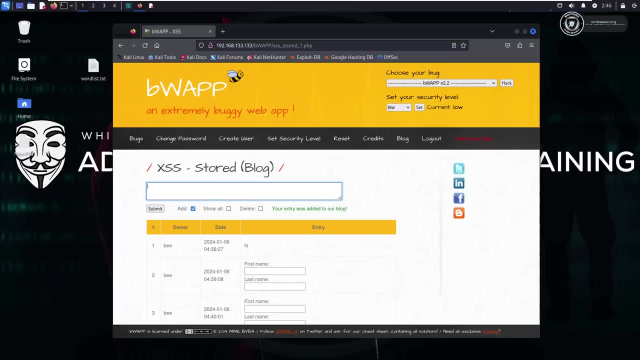 able to see the cookies there. okay, this is how it is gonna work. so simple, just read it. this is a url. this is excellent attack man, right? so this is the thing. in the next classes we are learning about CSRF. right now, in this class, we are learning what is cross site request. 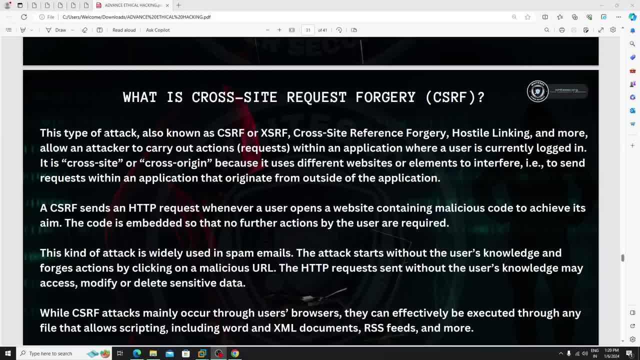 for jerry- CSRF. this type of attack, also known as cross site request for jerry. it is also known as CSRF, XSRF- cross site request for jerry. reference for jerry. okay or shell linking and more. allowing. allow an attacker to carry out actions, request actions. 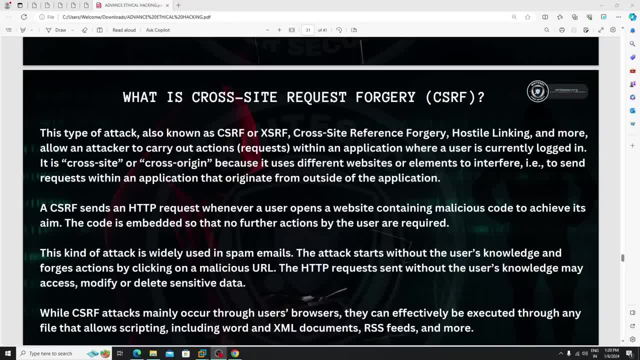 means it's a request within an application where a user is currently logged in. it is cross site or cross origin because it use uses different websites or elements to interfere, ie to All what it is actually. it is a or not a and it is also a user only did not have a operator. 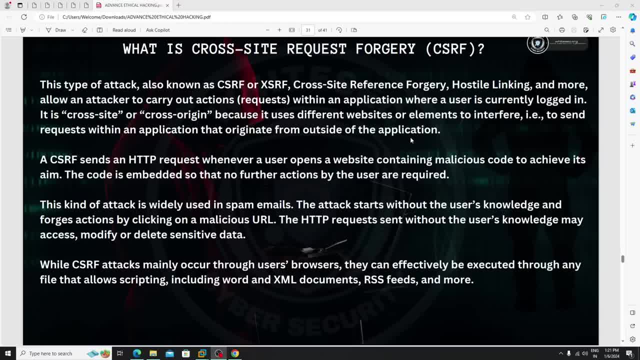 request within a applicationorg. From outside of the application, A CSRF sends an http request. whenever a user opens a website containing malicious code to achieve Its aim, the code is embedded to that. no further actions by the user or required this. You will see it what. what is the CSRF? as well, it is also one excellent vulnerability. 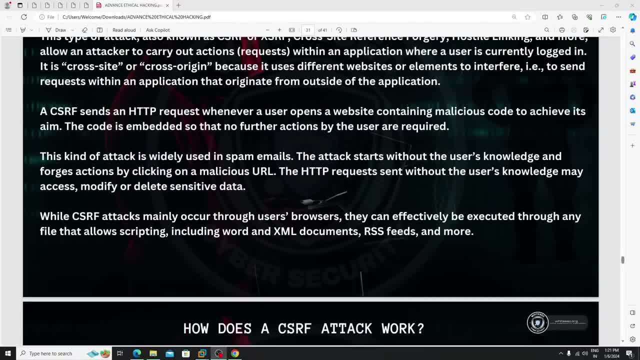 okay, Like. this Kind of attack is widely used in spam emails. the attack starts without the user knowledge and forges action by clicking on a malicious url. the simple thing. you no need to do anything. assume that the attacker okay, the attacker just sended the url. if you click on the url, then everything will be the 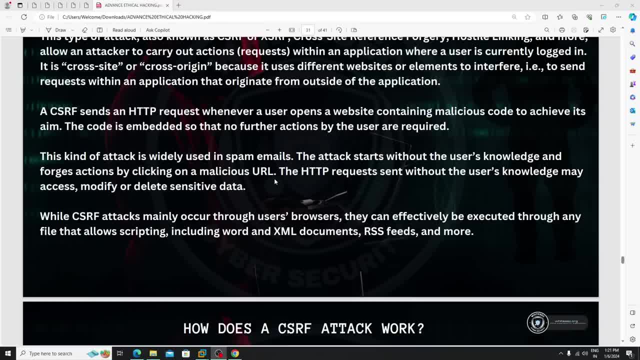 things will be hacked. okay, this is the thing. you no need to do anything simple. the the victim need to click that url. that's it, the http request send without the user knowledge. users knowledge may, as is, modify or delete sensitive data by using that link. the user 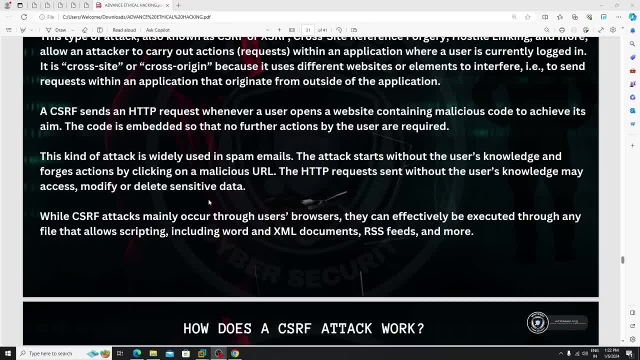 can able to- okay, the attacker can able to delete victim data in that website, which is vulnerable, okay. or he can able to do a lot of stuffs there, okay. like there is examples as well. you will see that modify for or delete. delete sensitive data, well, as is a. csrf attacks mainly occurs through users, browsers. they 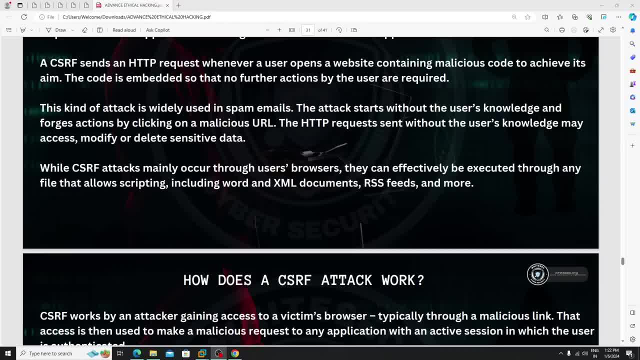 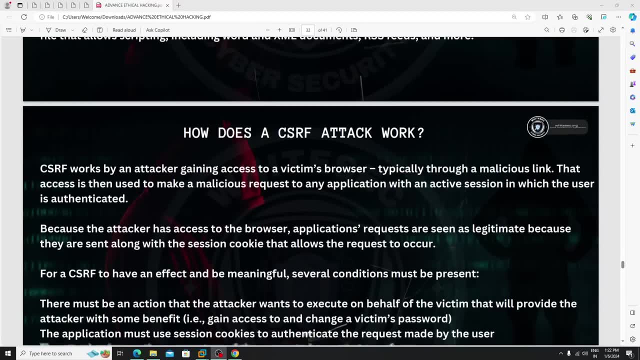 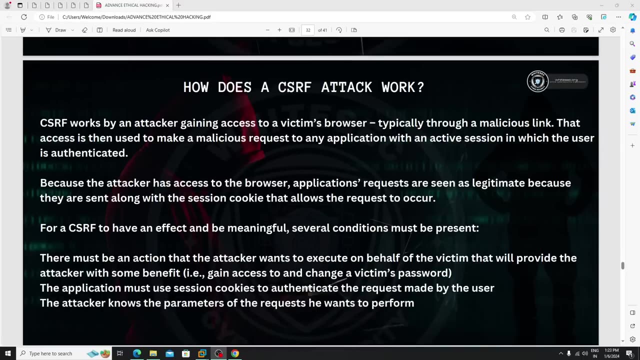 can effectively be executed through any file that allows scripting, including word and xml document, rss field feeds and more. how does a csrf attacks work? see csrf work by an attacker gaining access to a victim browser, typically through a malaysian server. okay, so this is the issue here. you can see that really the attacker has access to the malicious link. 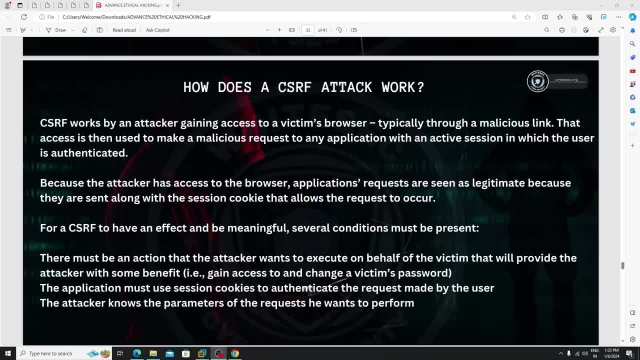 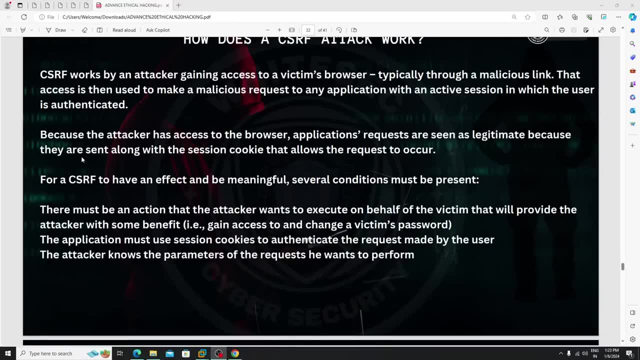 that as is, is then used to make a malicious request to any application with an active session in which the user is authenticated, because the attacker has access to the browser applications requests are seen as a legitimate because they are sent along with the session cookie that allows the request to occur. for a csrf to have an effect and meaningful several. 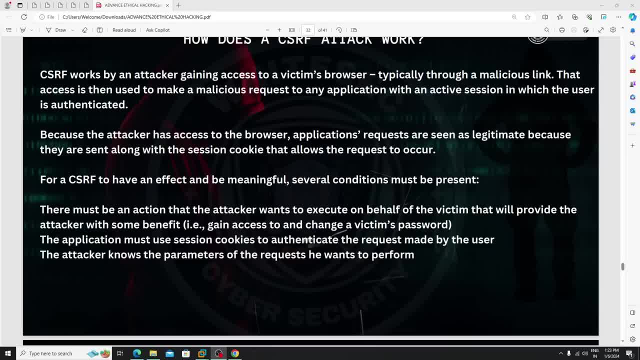 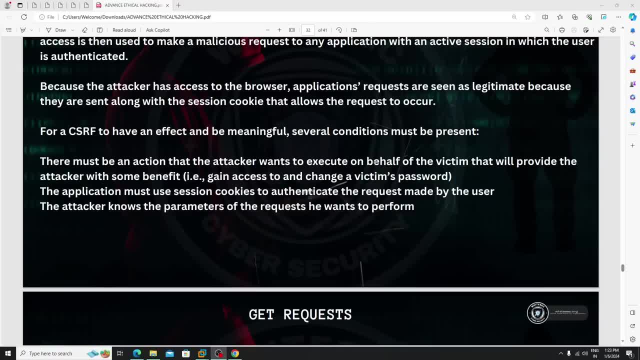 conditions must be predicted. okay, I have not yet completed all the exercises in this series agent. what are those conditions there are must be a, an action data that the attacker want to execute on behalf of the victim. that will provide the attacker with some benefit, ie gain access. 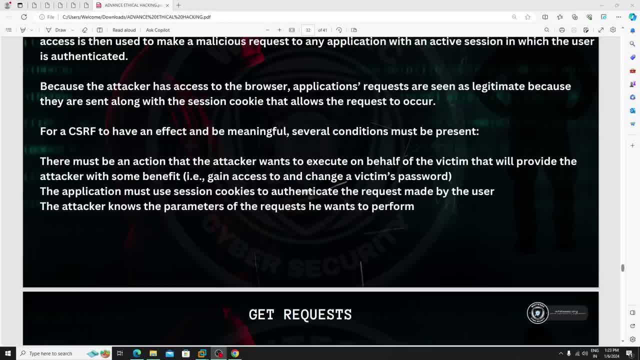 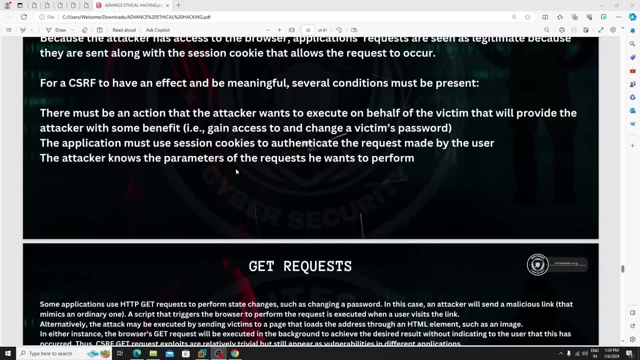 and change a victim password, the. the application must use session cookie to authenticate the request made by the user. the attacker knows the parameter of the request he want to perform here. this is depends upon the parameters. okay, you will see it, don't worry. now, here in this class. 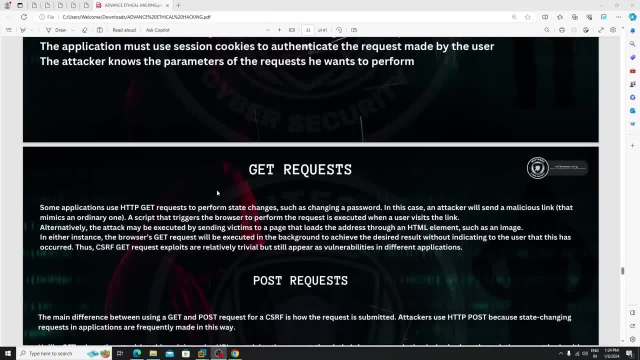 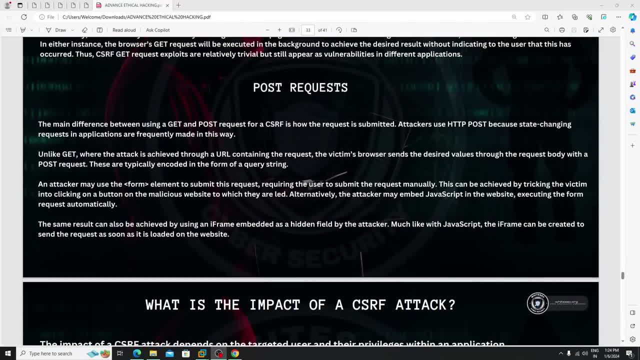 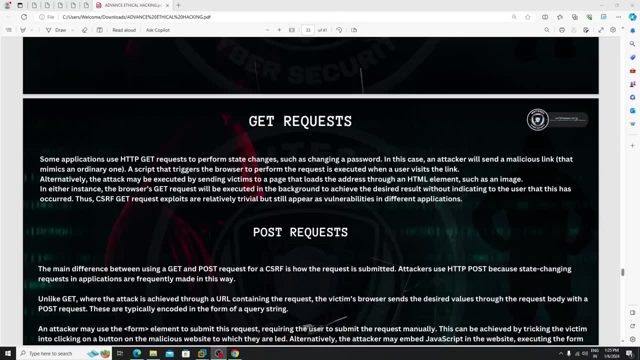 let's let's cover in the next slides. let's cover about get and post request as well. now there is also impact. now let's learn about get and post request. see some application. use http get request to perform state changes, such as changing a password in this case. 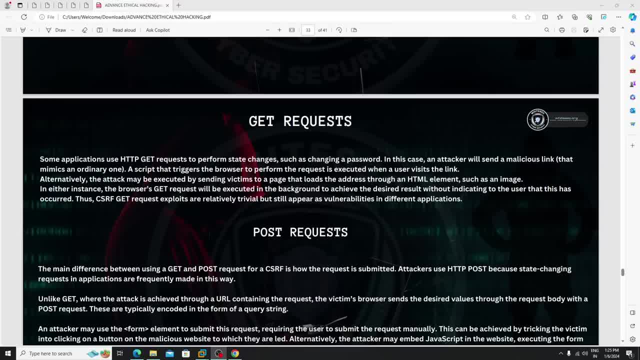 and an attacker will send malicious link that mimics- okay, just see the bracket here. that mimics an ordinary one is a script that triggers a browser to perform. the request is executed when a user visit that link. this is the thing. you just need to visit it at the time after clicking on that link. 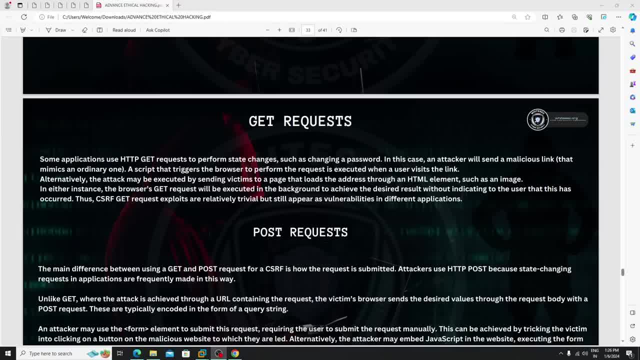 the, the, it will trigger. okay, thus the script will trigger. alternative. the attacker may be executed by sending victim to a page that loads the address, and then it can by�g цем julian. another thing you can do is just through an html element such as an: 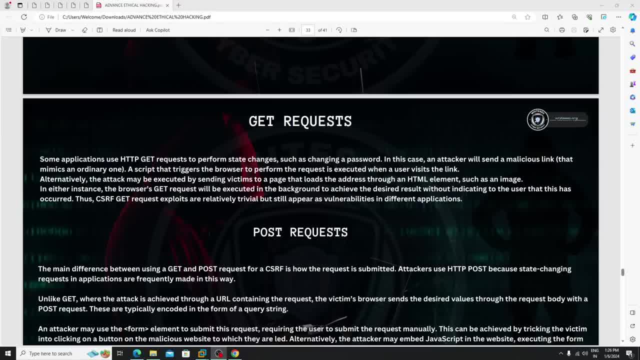 image. in either instance, the browser get request will be executed in the background to achieve the desired result without indic indicator to the user that this has occurred. the csrf get request exploit or relatively trivial, but still appear as vulnerable in different application. now let's learn about the content. that wasoshd entrepreneurship via html. he made just a simple application request and that was one a request. two was showed up in the next twolet. our guide of this workshop. also our guide of this workshop channel. attachedйuar sc. annoying scheduling text intake site, but remaining 16 seconds can be fueled by the Reading is hard and every image or extension test, unfortunately, must carry it in our core to make the scenes text size, specificacaedNG and and future sets. 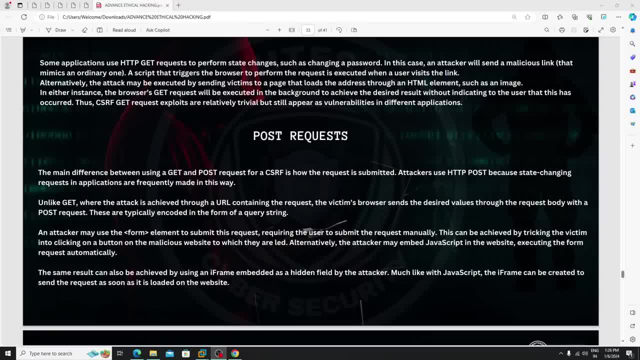 the main difference between using a get and post request for a csrf is how the request is submitted. attackers use http post because state changing request in application or frequently made in this phase. unlike get, where the attacker is achieved through a url- we just learned in the last classes as well- it's achieved through the url containing the request the victim browser sends. 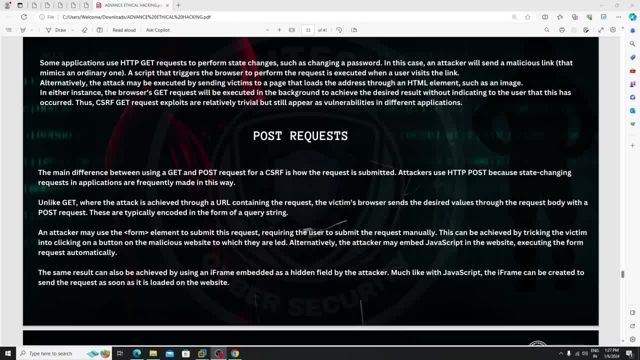 the desired value through the request body with a post request. these are typically encoded in the form of query string. an attacker may use form form tag element to submit this request, requiring the user to submit the request manually. this can be achieved by tricking the victim into clicking. 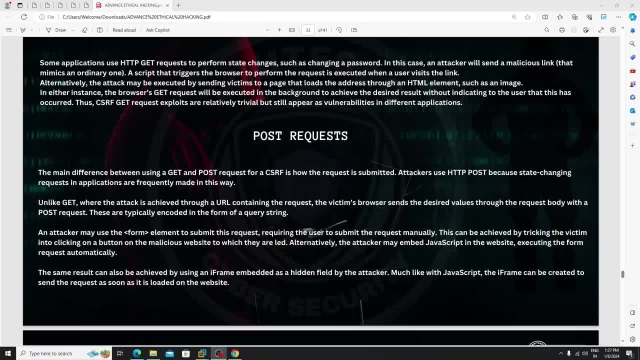 on a button on the malaysia's website to which they are lead. we just- and also we just covered this in html injection as well. alternative, alternative, alternative: the attacker may embed javascript in the website, executing the form request automatically. this is the thing here. now, here the attacker, the victim. no need to do that process, okay, simple by using this. 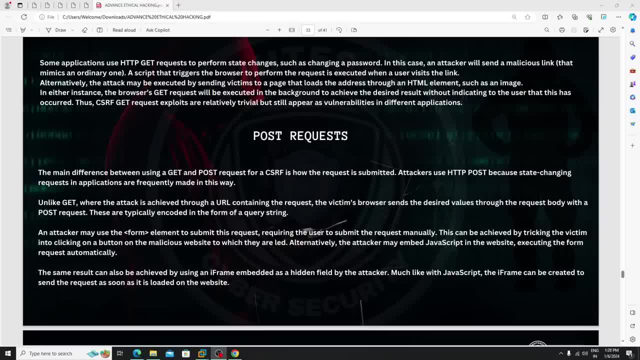 uh, csrf, attack the victim. no, see the victim. no need to type anything there. simply he just need to visit and open that url, that's it, okay. the same result can also be achieved by using a iframe embedded as a hidden filled by by the attacker. much like java, much like with javascript, iframe can be created to send the. 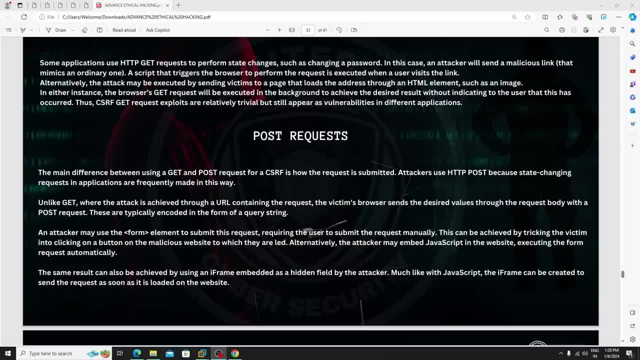 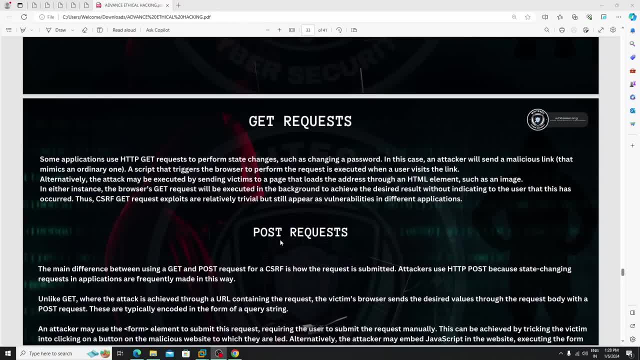 request as soon as it is loaded on the website. okay, you will see. but let me tell you one thing, guys, here it's not a big deal. the definitions are sometimes. sometimes you won't get it. okay, just try to do the practice and read it again. okay, this definition. at that time you will get it, just. 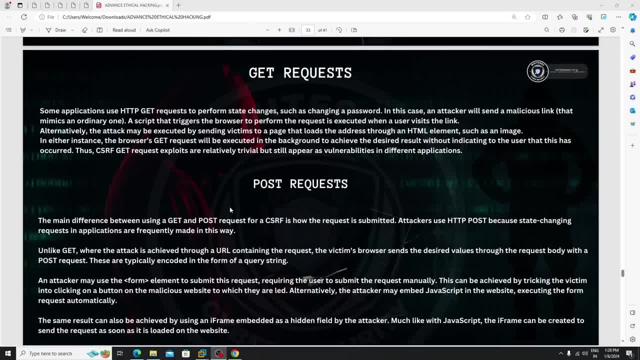 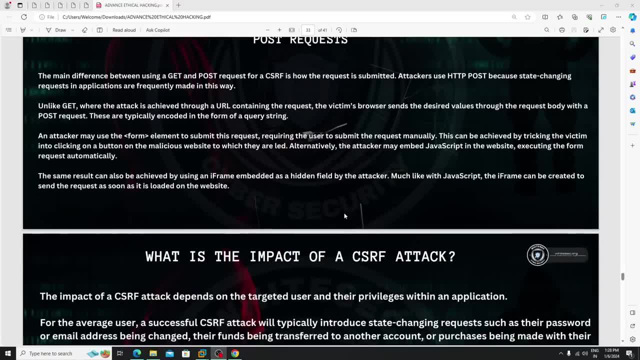 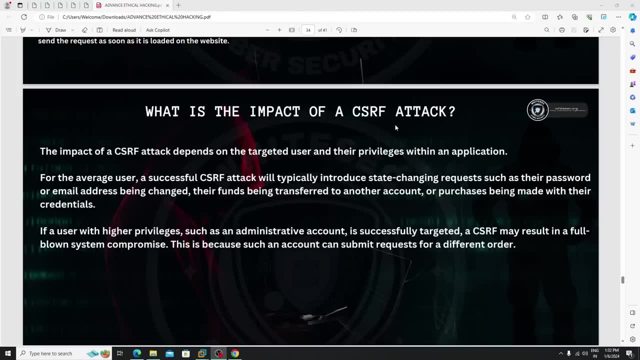 uh, stop the video, take screenshot, something like that, and try to read it again after executing the attack. okay, this is the thing. in the next class we will learn about what is the impact of, and of, a csrf attack. now, in this class, we are learning what is the impact of a csrf attack. 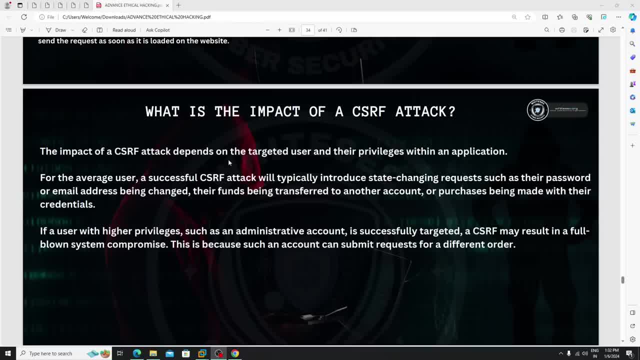 the impact of a csrf attacks depends on the targeted user and their privileges within application. for the average user, a successful csrf attack will will typically introduce state changing requests, such as their password or email addresses being changed, their funds being transferred to another account or purchases being made with their credentials. 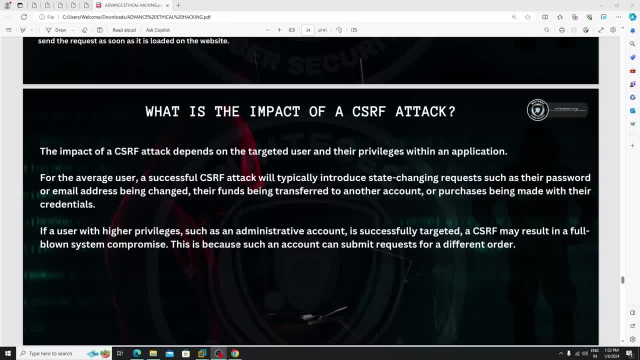 if a user with high privileges, such as an administrative account, is successfully targeted, a csrf may result in a full blown system compromise. this is because such an account can submit requests for a different order. this is the thing. this is a kind of dangerous vulnerability, right, but the thing is here. the user need to click on the link, that's it. 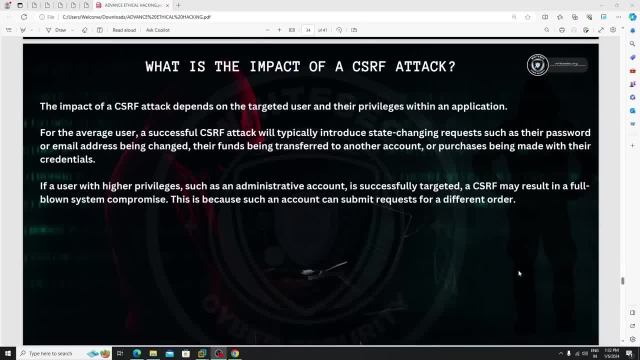 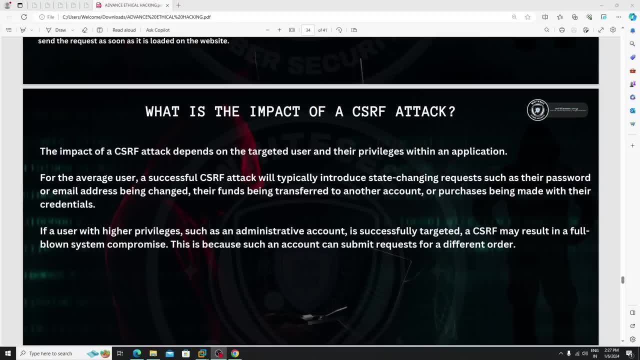 right now. in the next classes, we are learning how we can able to exploit it. now, in this class, we will learn how we can able to perform csrf attack right now. the thing is here. you can take any example. let me take this one: their funds being transferred to another account. you can also change the password as well. 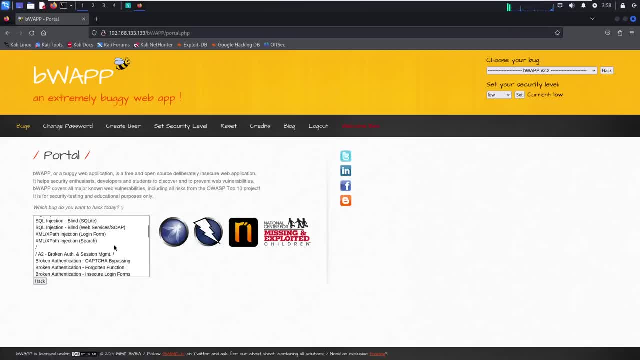 first of all, the thing is, let me select the csrf from here which comes under age eight. okay, here it is a8. let me use this one transfer amount which is easy. okay, you guys can able to uh get this thing in a very easy way. see, here it's a kind of bank account in my account. 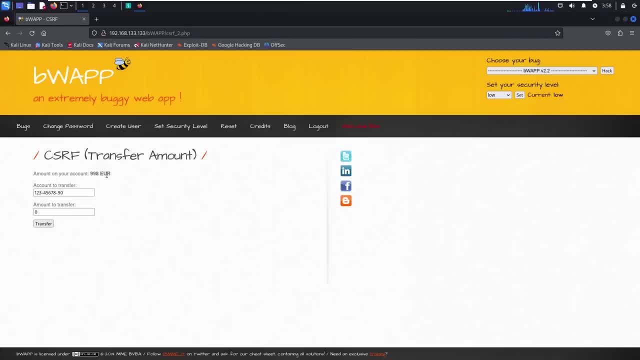 there is 998 euros out there, right? this is the account to transfer money. see, here you can add any number. it's totally like in real world. what will happen? assume that if you want to send any amount to your uh uh anyone at that time, what will happen? we, we type the account number there, right? the simple thing. 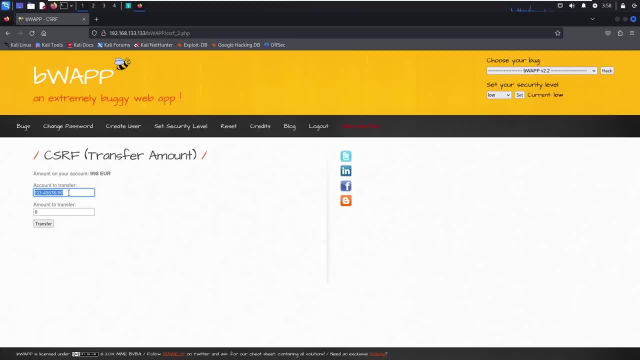 here. assume that you just type the account number and the value- how much money you want to send. assume that i want to send one euro. after sending it, now the value has been changed to 997 euro. okay, so this is the thing. now let's see how the csrf attack will affect this one. 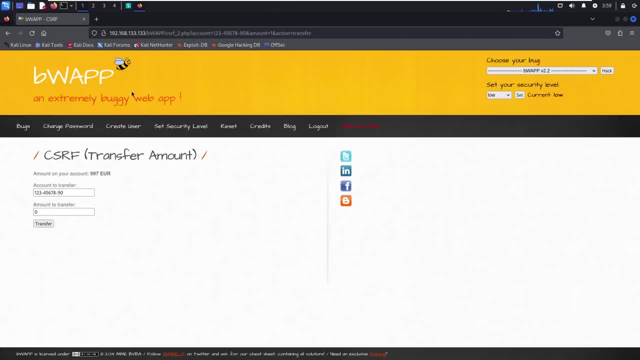 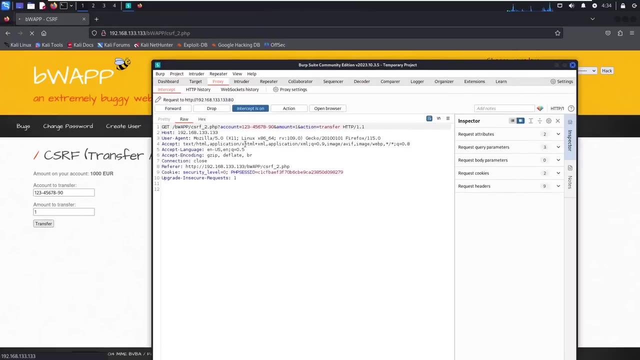 right, right. first of all, the thing is: let me use a, let me click on and intercept, and let me transfer one, one euro. and here you, you can able to see the request has been captured. now, simple, do one thing, just uh, here, engagement tools are there if you click on. 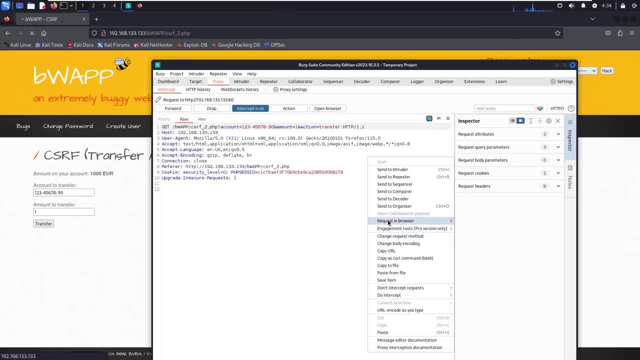 generate csrf poc, then it will automatically generate the csrf poc for you. you need to upload it on the web server. this is the thing now here. it will only work with pro version. if you don't have the pro version, what you need to do? simple just, you need to do manually. okay, now, how to do manually? this is also one thing. 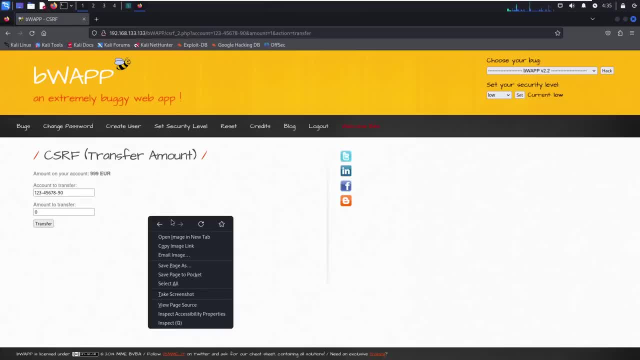 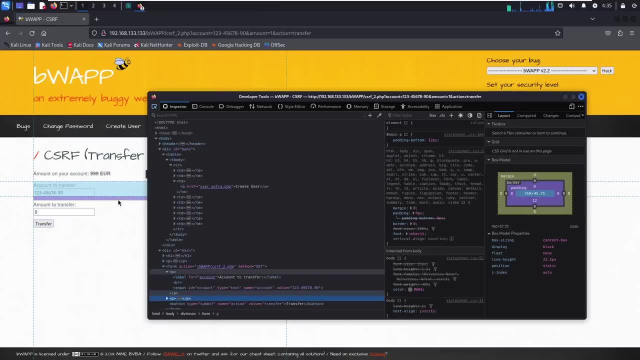 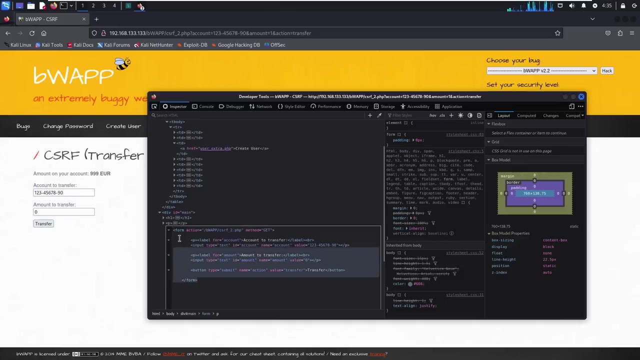 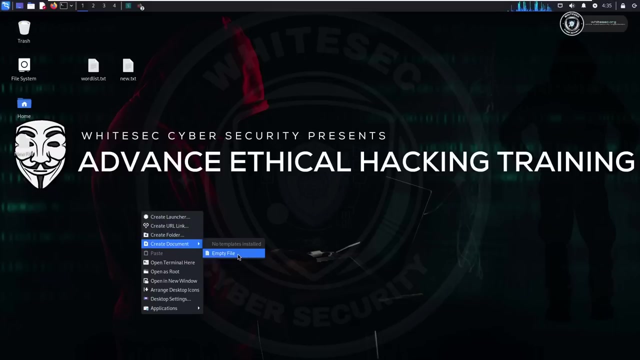 see here. click on inspect, select this icon and just select the form here. this is a form, simple, selected, all right, after selecting it. here you can able to see the form. okay, now, simple right click and edit as html. just copy this form. okay, after copying it, create document here. empty file. user: the attacker. what he will do means he will create one html file. 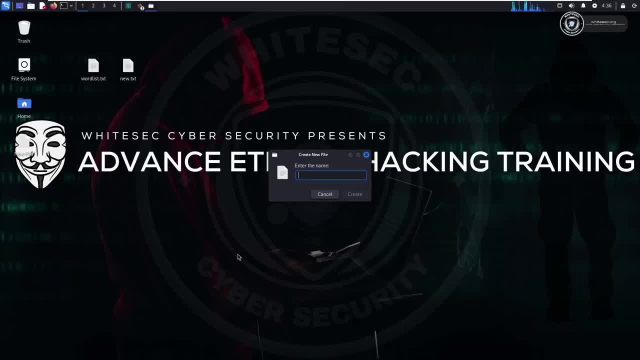 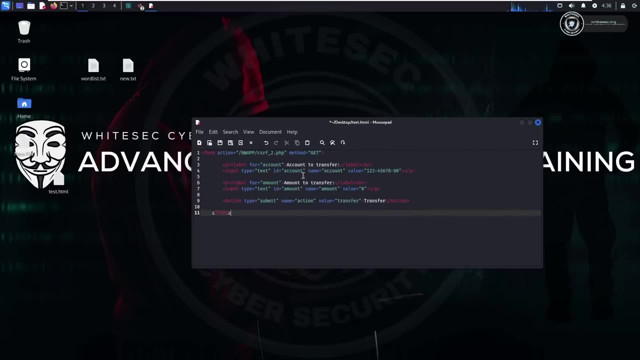 is some with legit name, some such kind of name. okay, like, let me use testhtml here, let me create, let me open this one, and here the attacker, what he'll he will do means he will try to modify this one. okay, like, if you have a html knowledge, you guys can able to modify it. okay, you just change. 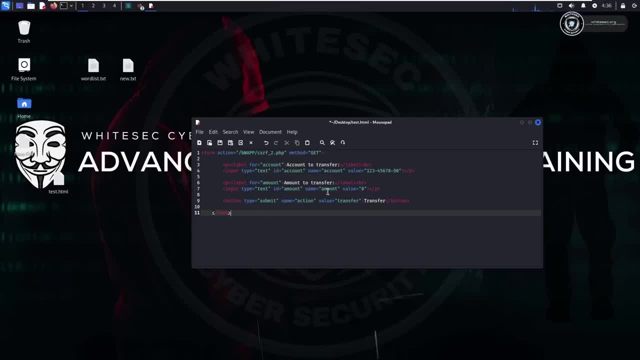 the names, this kind of stuff. and here the main things are value, okay, just see, here value is the account number. here attacker will change the account number okay to his account number. this is the thing, and here the amount value will be the account number and here the amount value will be. 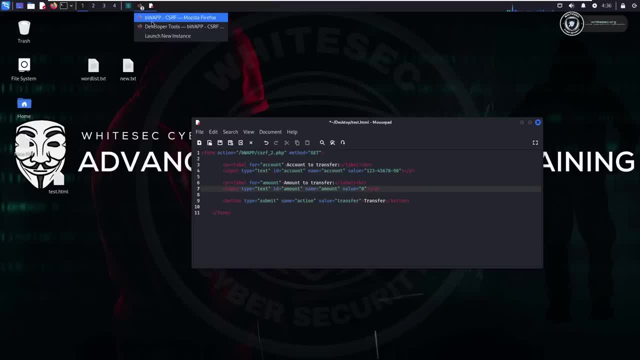 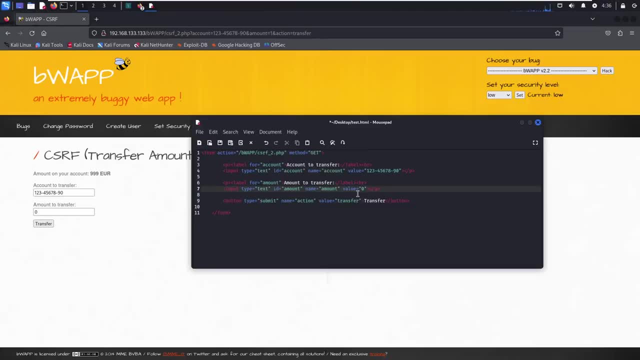 the money value. okay, so you can change here the amount value and here this way. um right, my just assume that right now in this account there is around 999 euros or there. simple, let me assume that the attacker want to steal around 500 euros. other time he will change it to 500. then he will change the. 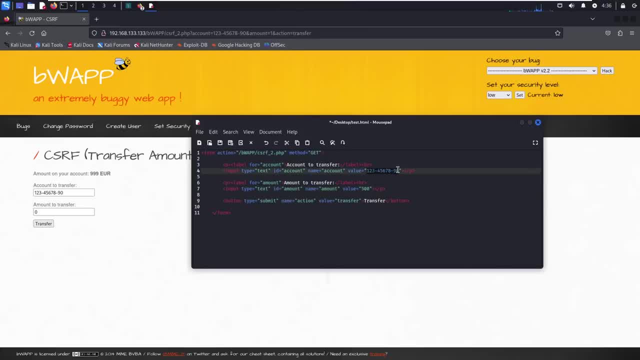 account number there. okay, just assume that here. let me use the same account number right now. simple, uh, there is a text type, type is there? or new image? has fucker transfer option? repeat: explain it. you know you can also also goш floor For money. my screen proof. these are easy, so just try to search any of this form. 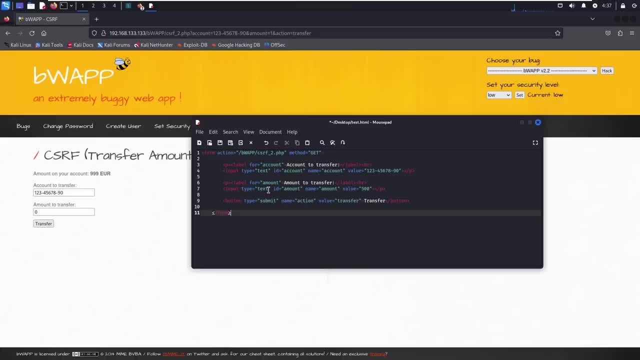 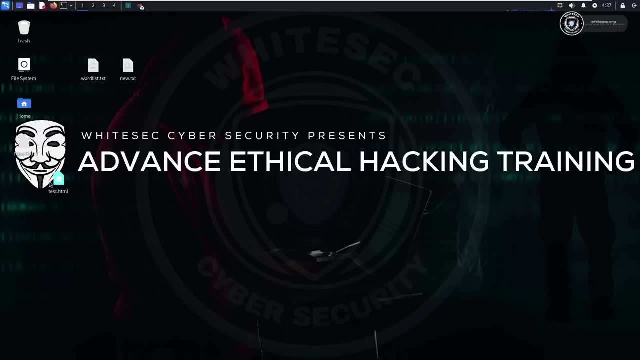 You can also hide this type. if you type here hidden, then just let me show you. let me show it. let me copy this html file: see, in real world scenarios, the attacker will host this in cpanel, right, so we, right now, let let us take this one var html. ok, just just click. 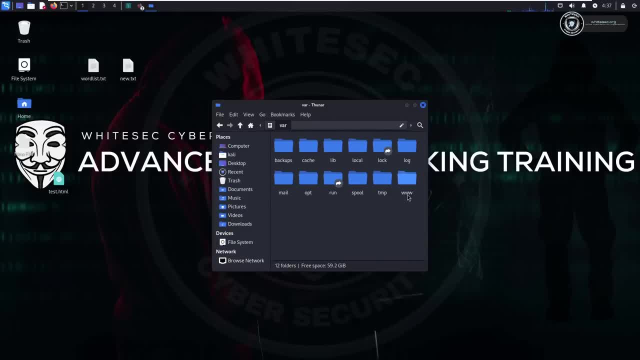 on file system. go to var. ht- ww- there is a html- and paste this here. you can't able to paste it because you need to open this as a root. just paste that html file and from here just add the apache server. open terminal here and just type here: sudo service- apache. 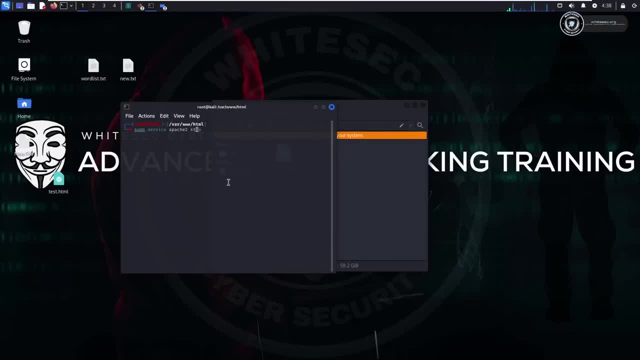 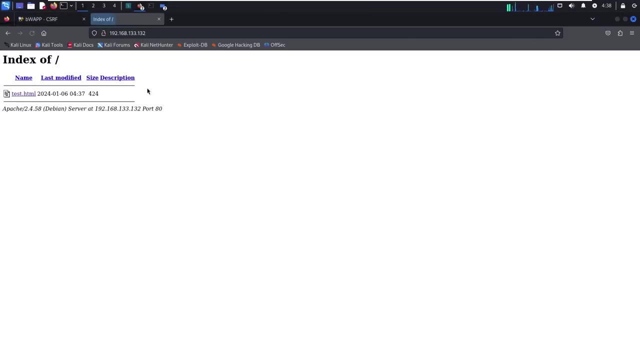 to start. ok, the apache server will be started Now, if you want to open the apache server, you can open the apache server by clicking here. if you type ifconfig, this is your ip, right, let me open the browser here. open this, then here you can able to see the html. now the attacker will send this kind of link to: 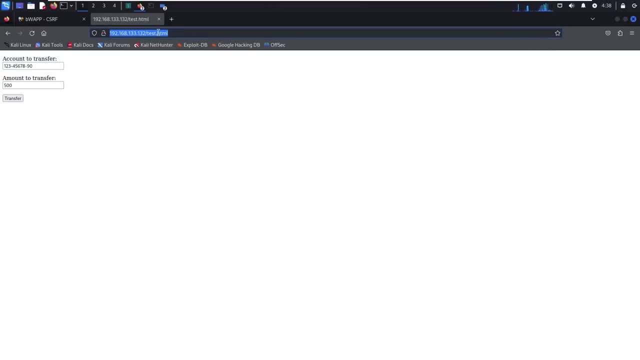 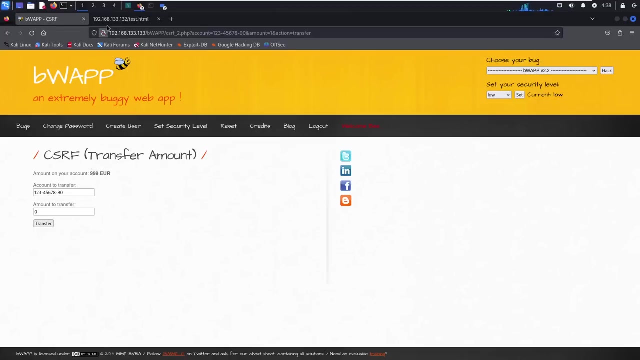 the victim through email or something like that. if you click on that, then what will happen? you will see this kind of page. if you click on the transfer, then the amount has been detected from here in his, from his, bank account. this is the thing. ok, So this is a kind of dangerous vulnerability. you need to edit this. ok, you need to kind. 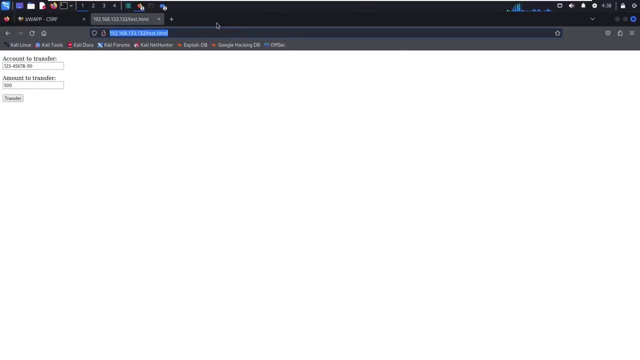 of social engineering there and you can able to edit it. see, in csrf there is a lot of advanced techniques as well. ok, right now we are only covering the basic things, right? so if I click on the transfer, then what will happen? the amount will be detected from here, right, right? 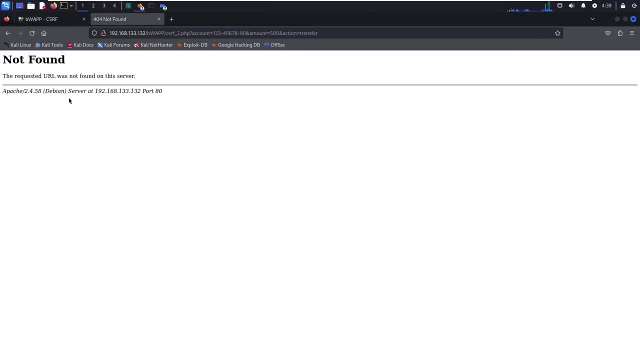 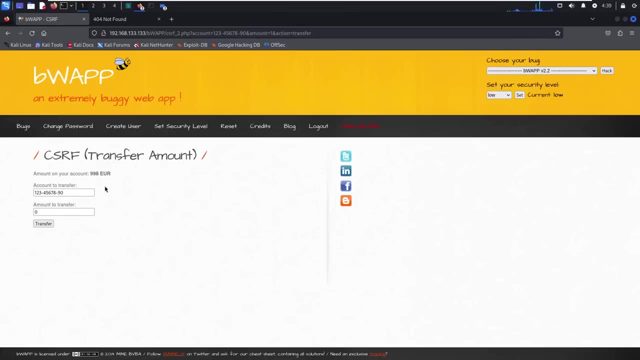 now it's not detected because there is a kind of issue here with this port 80 right in realworld scenario. What will happen? the amount will be detected. this is the thing, right? hope you guys get it. it's not a big deal, it is very easy process if you open the bup suit from here also you 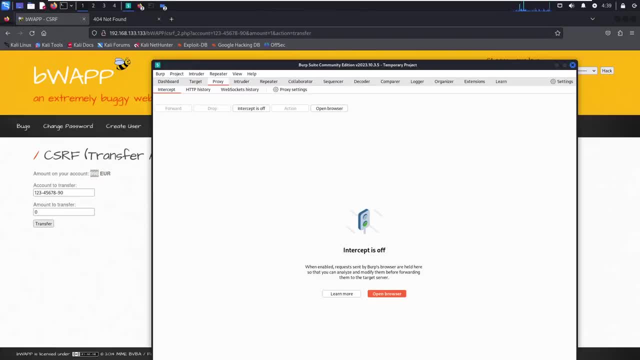 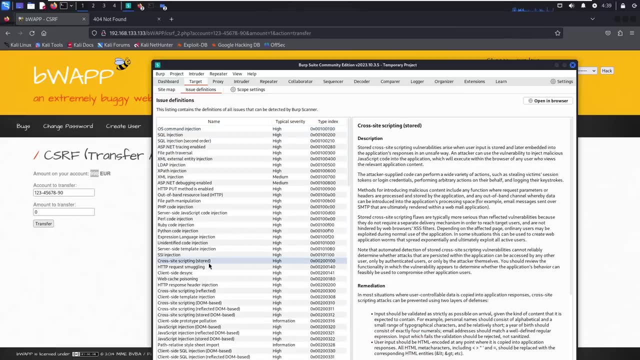 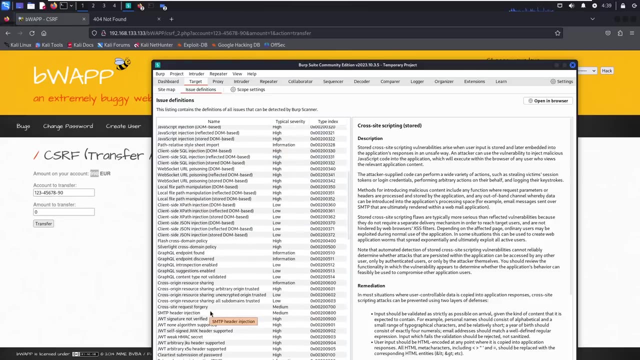 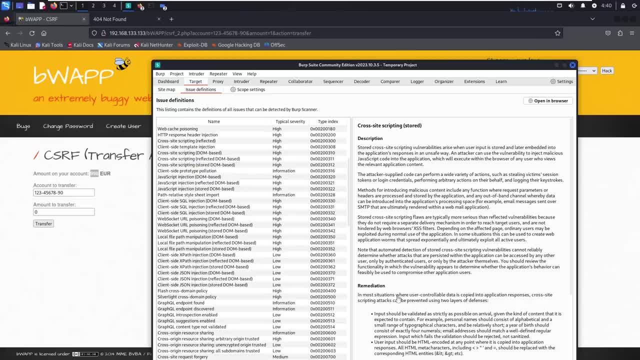 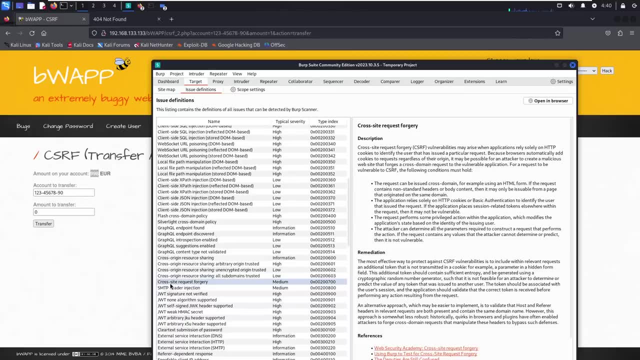 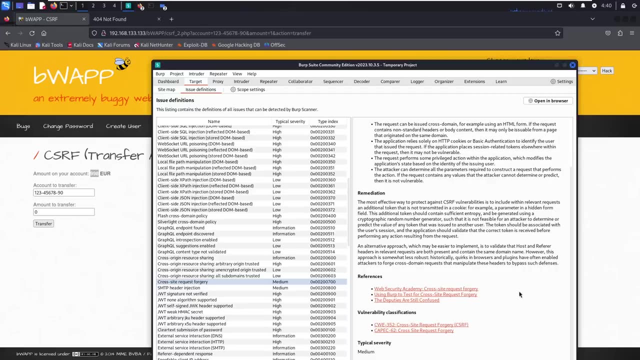 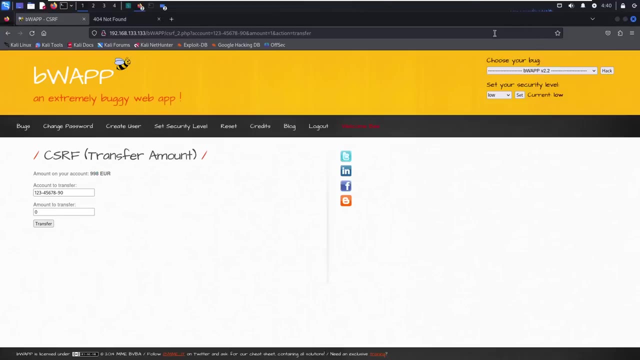 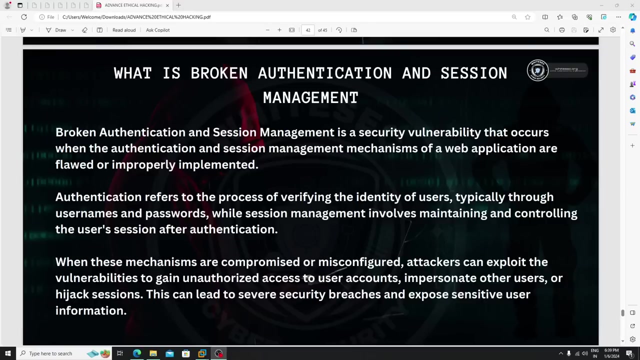 Let's see for the csrf. It is for crowd site requires for January. It is for crowd site requires for January. It is a- it is okay- crowdsite request from here. authentication and session management: broken authentication and session management is a security vulnerability that occurs when the authentication and session management mechanism. 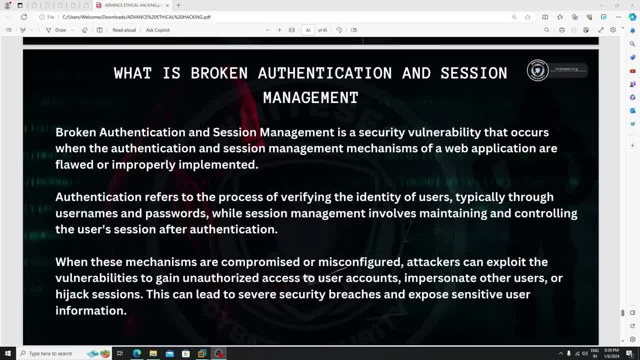 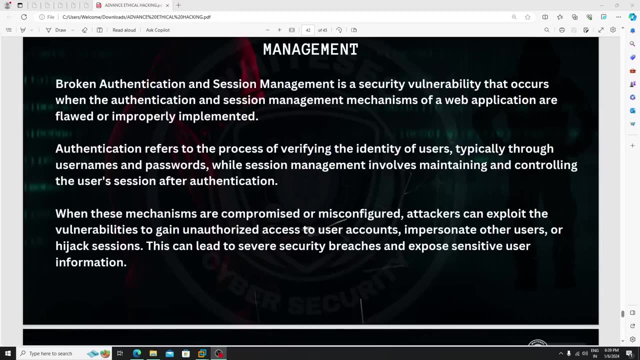 of a web application or flood are improperly implemented. authentication refers to the process of verifying the data of users, typically through usernames and passwords, while session management involves maintaining and controlling the user session after authentication. when these mechanisms are compromised or misconfigured, attacker can exploit the vulnerabilities to gain unauthorized access to user accounts, impersonate other users or hijack. 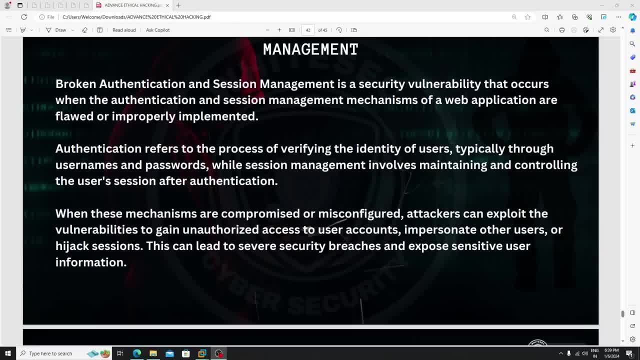 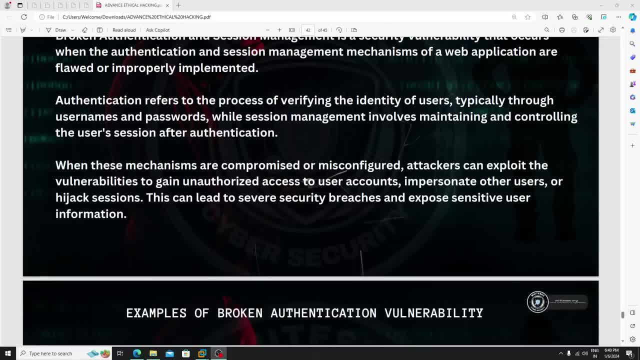 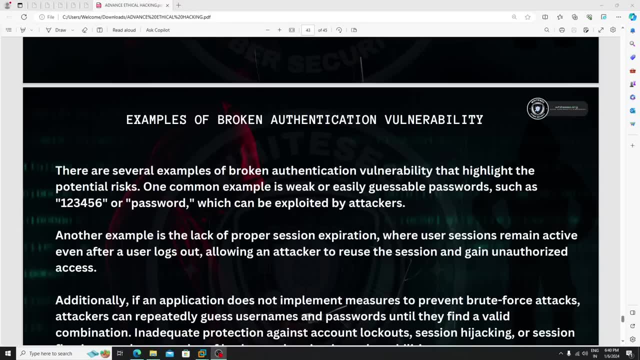 session. this can lead to severed security breaches and expose sensitive user information. now let's learn about examples of broken authentication vulnerability. there are several examples of broken authentication vulnerability. that highlights the potential risk. one common example is weak or easy guessable passwords, such as one, two, three, four, five, six, or password which can be exploited by attackers. 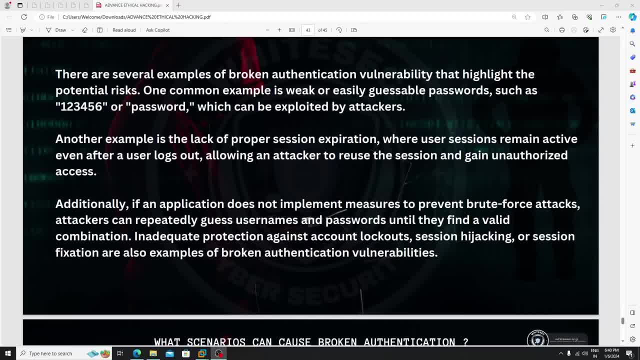 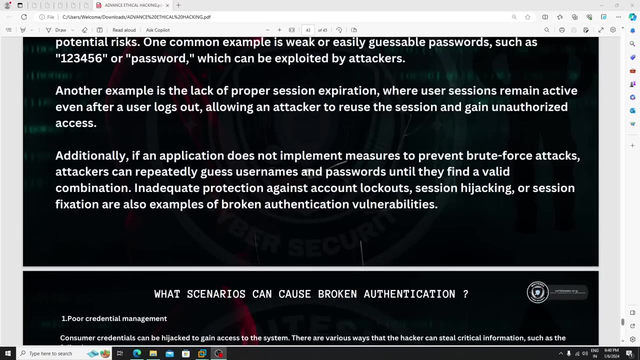 another example is the lack of proper session expiration. expiration like expiring okay way. user session remains active even after a user logout, allowing an attacker to reuse the session and gain unauthorized access. additionally, if an application does not implement measure measures to prevent brute force attacks, attacker can repeat. 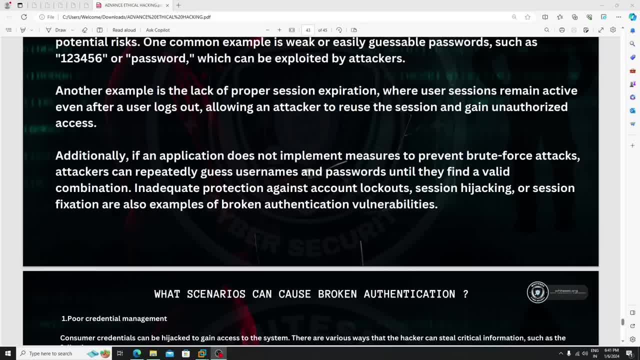 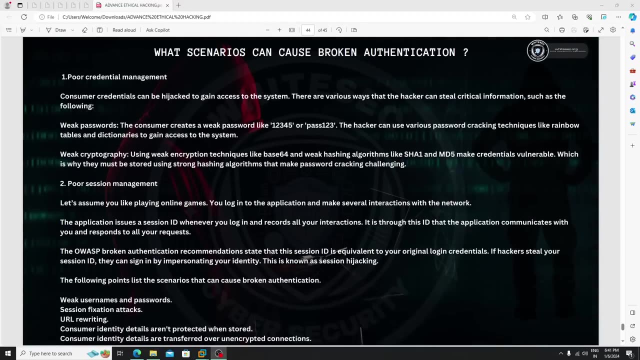 repeatedly guess usernames and password until they find a valid valid combination in a inadequate for protection against account lockout. session hijacking or session fixation are also example of broken authentication vulnerability. now here let's learn about scenario as well. what scenarios, what scenarios can cause broken authentication? first scenario is poor credential management. 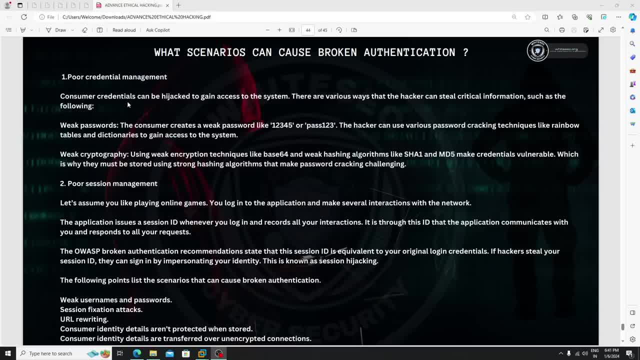 consumer credential credentials can be hijacked to gain access to the system. there are various way ways that the hacker can steal critical information, such as the following: weak passwords and weak cryptography. in weak password, the consumers create a weak password like one, two, three, four, five, or pass one, two, three. consumer is nothing but the user. 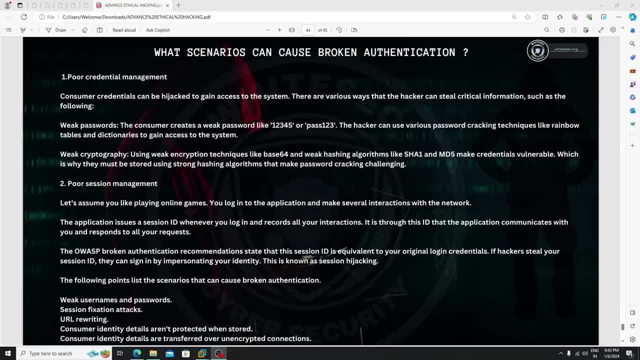 okay. the hacker can use various password cracking techniques, like rainbow table and dictionary dictionaries, to gain access to the system. weak cryptography using weak encryption techniques such a like base 64, and weak hashing algorithm like sha1 and md5. make- make make credentials formable, which is 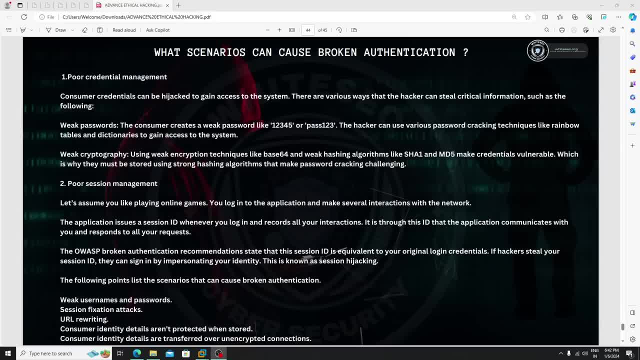 why? why they must be stored using strong hashing algorithm that make password cracking challenging. if they use a strong encryption there, then what will happen? it will take a huge time to crack that password. you can able to crack, but it will take a huge time there. this is a thing right. 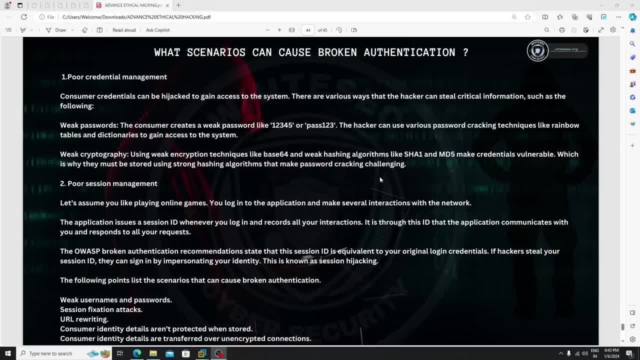 and there is also salt, uh salting, as there is a one uh way to make your password more secure: by adding something to your password. so this is a way to make your password more secure: by adding something to your password. so this is a way to make your password more secure by adding. 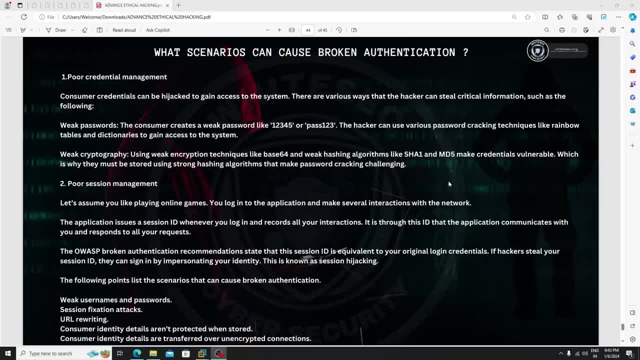 something to your password. so this is a way to make your password more secure by adding salt there. okay, there is also one uh thing right, which is make your password complex like uh. if you add that algorithm, then what will happen means it is hard to crack. now, poor session management. let's assume you like playing. 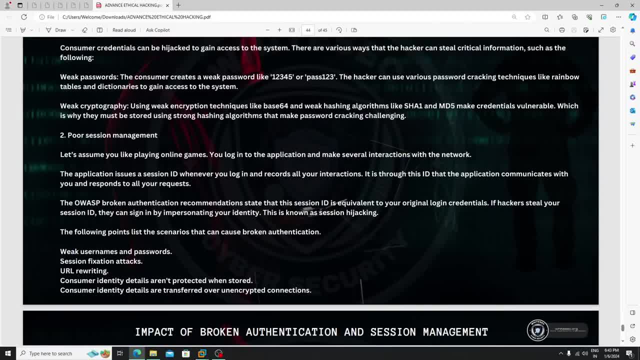 online games. you login into the application and make several interactions with the network. the application issue a session id whenever you log in and records all your interactions. it is through the id that the application communicates with you and responds to all your requests. okay, the ovas broken authentication recommendations. 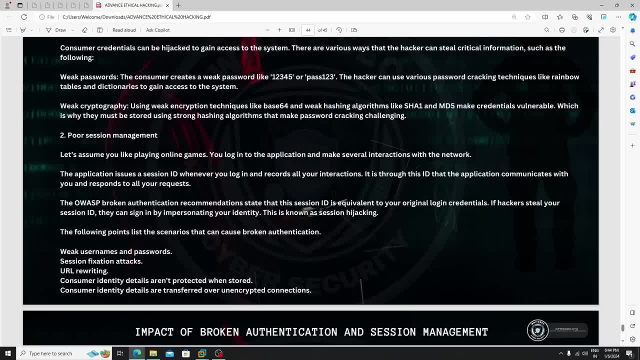 state that this session id is equivalent to your original login credentials. if hackers steal your session id, they can sign in by impersonating your identity. this is known as a session hijacking right. so, basically, if the attacker steal that id, then what will happen? he can able to log in. 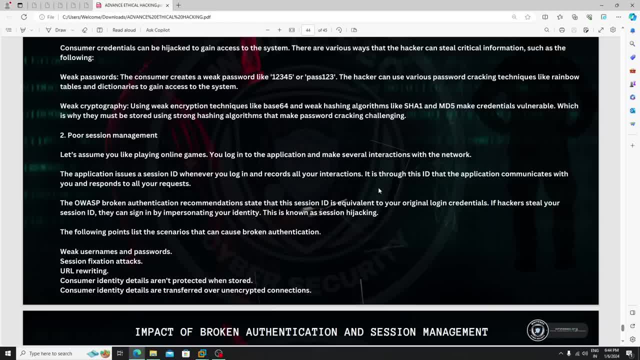 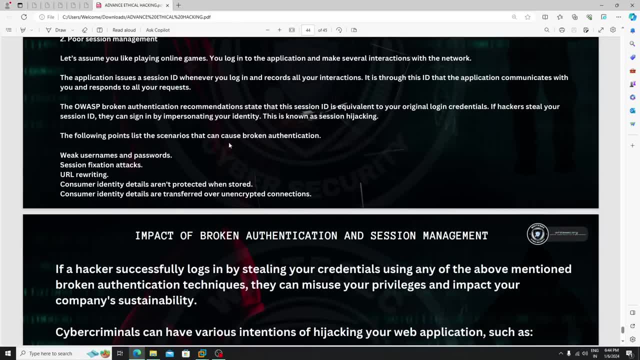 in your account without using the username and the password right. the following points list the scenarios that can be caused: broken authentication: there is a weak username and the password. username and password session fixation attacks. url rewriting. consumer identity details are not product protected when stored or not protected like if see. basically, there are two ways. 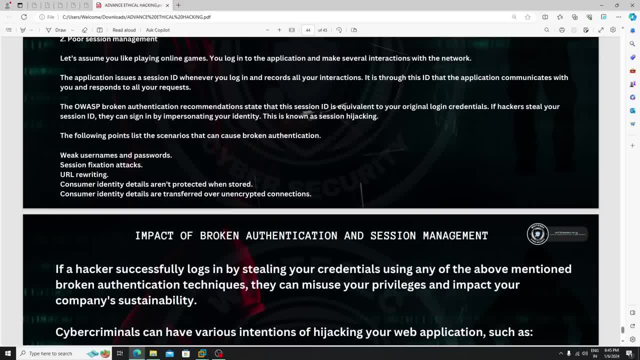 okay, first is they? uh, by default they use md5, right or base64. now, see what will happen means assume that there is a one website. i just created the account in that website. okay, by default, the data will be stored in encrypted format there. my username and the password. okay, my username will be: 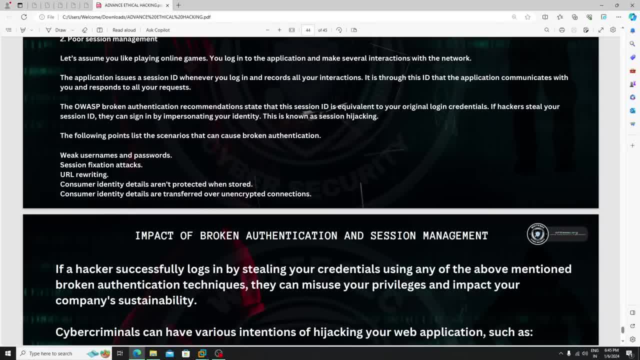 uh, plain text, i think. okay, it's mostly i just saw in plain text. the password will be encrypted there. okay, assume that if they are not using the this kind of algorithms which are hard to crack, assume that they are using, such as base64, this kind of algorithms. at the time, it will make a high chances. 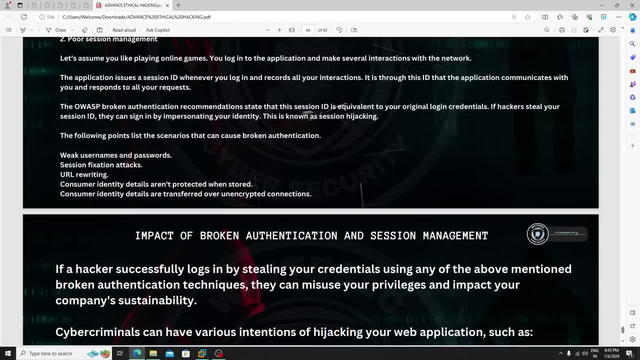 okay, like it is easy to crack consumer identity details are transferred over unencrypted connection http. uh, we just learn about http. right, why http is dangerous. like there is also ftp. is there telnet? is there? okay, now in the next classes we are learning about impact of broken authentication. 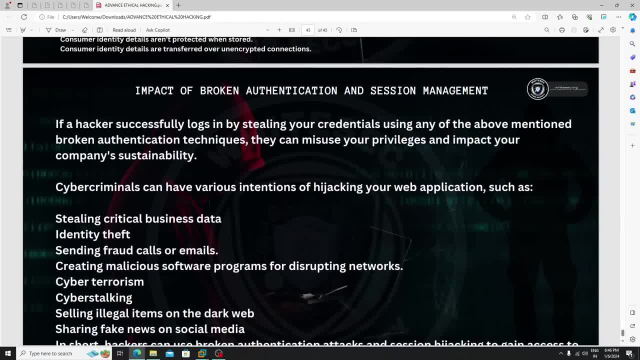 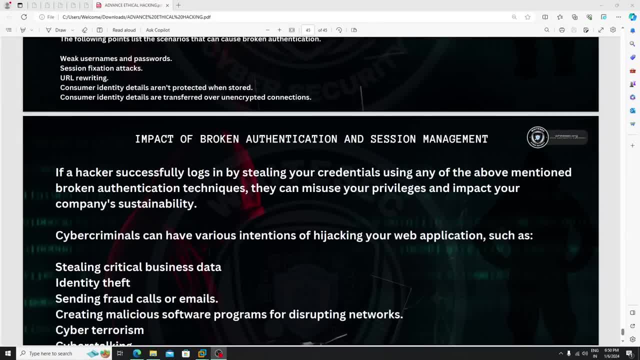 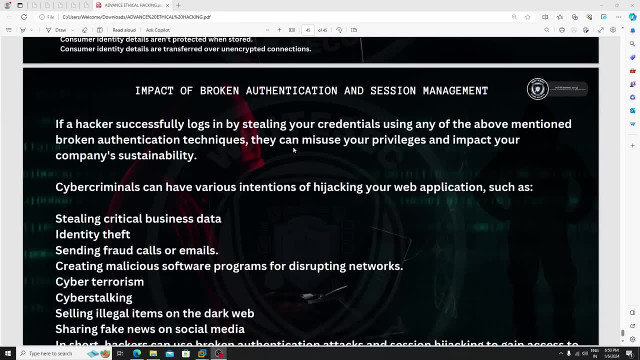 and session management. now in this class, we are learning impact of broken authentication and session management. if a hacker successfully logs in by stealing your credentials using any of the above mention mentioned broken authentication techniques, they can misuse your privileges and impact your company's sustainability. cyber criminals can have various intentions of hijacking. 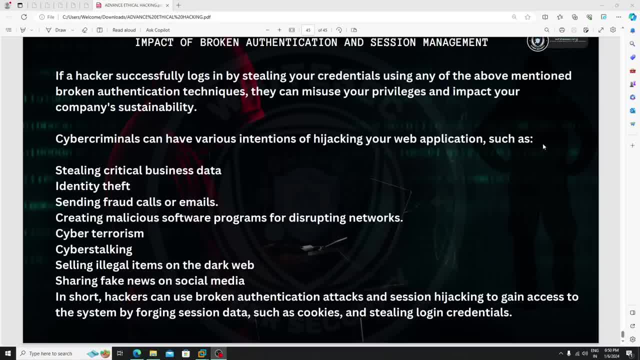 your web application, such as stealing critical business data, identity theft, sending fraud calls or emails, creating malicious software programs for disrupting network, cyber terrorism, cyber stalking, selling illegal items on the dark web, sharing fake news on social media. in short, hacker can use broken authentication attacks and session hijacking to gain access to the system for 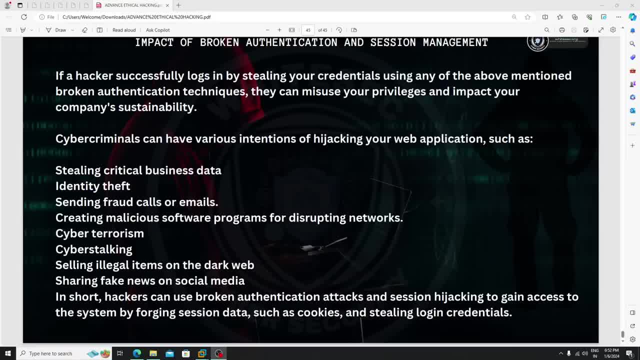 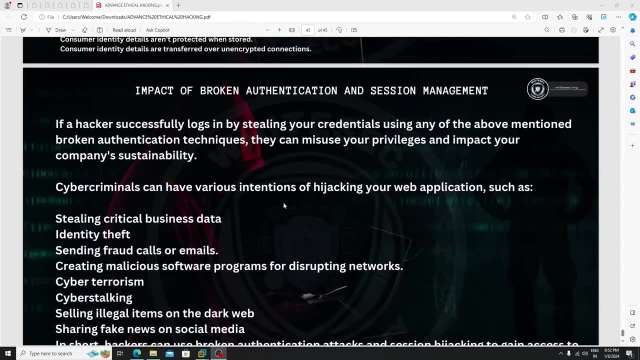 forging uh session data, such as cookies and stealing login credentials. the main aim is stealing the cookies and stealing login credentials here. okay, so uh, in the next classes. in the next class we will learn practically how the attacker can able to do it. now in this class we are learning how we can able to perform session management. 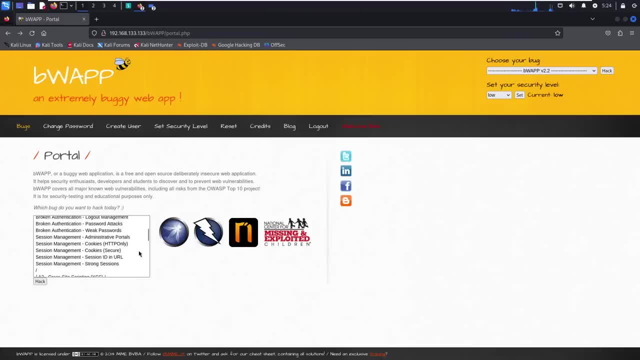 how we can able to exploit this session management and broken authentication in session management. just select any. let me select this administrative portal here. simple hack it, okay. simple click on hack here. the thing is you can't able to see the this one. okay, session management administrator portal. this page is locked. if i want to see this space, then i i must be admin here. this is the thing. 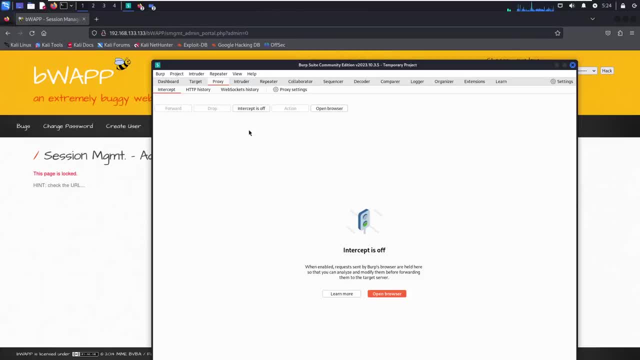 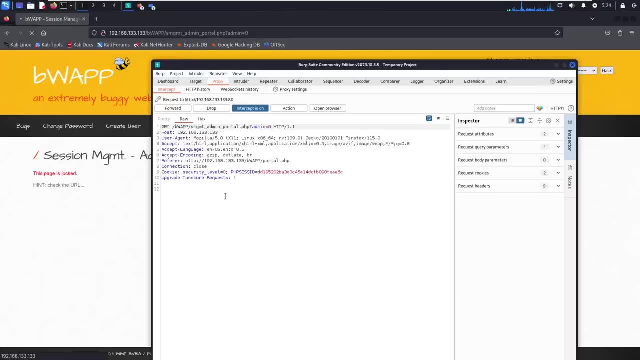 so assume that let me do one thing, let me click on intercept on here and let me refresh it. this page- here you can able to see there is a request. right here you can able to see the admin is equal to zero. see, zero is nothing, but it's false. okay, if i change this zero to one, then what will happen? 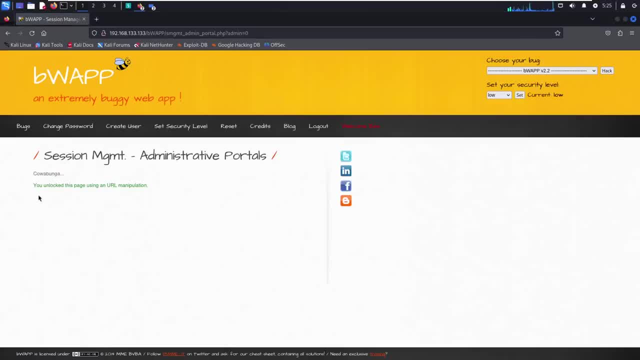 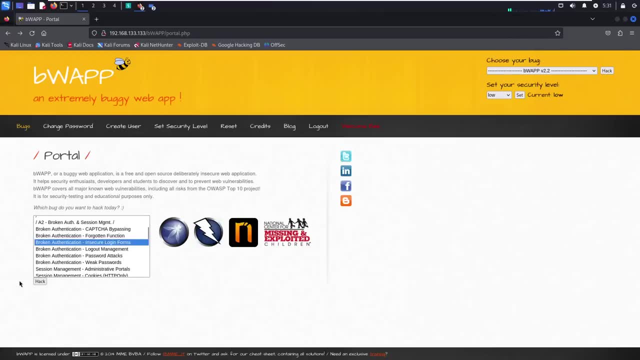 just let me forward it. now you are, you unlock this page using a url manipulation. now let's go for in secure login forms. now, see, here there is a credentials. you just need to type login and the password here, since in insecure login forms, what will happen means: let me show you, let me. 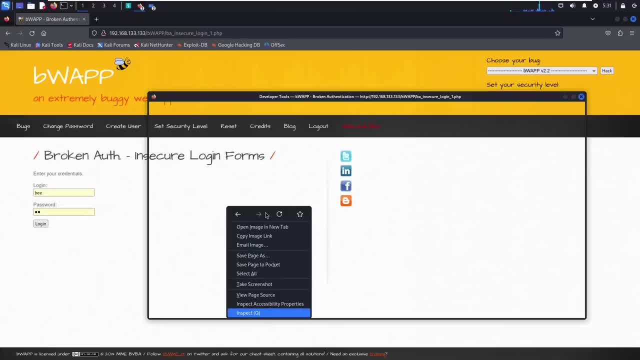 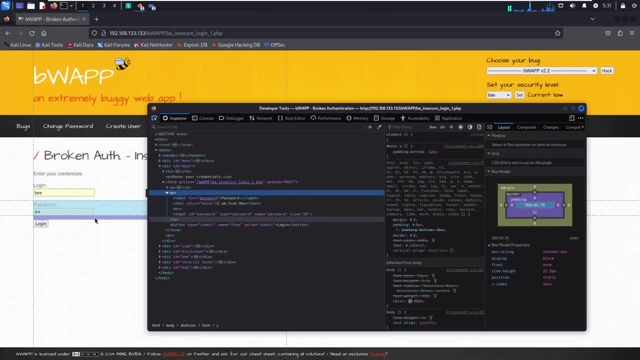 click on inspect elements here. okay, now let me select this form. okay, this is the form. see, simple, it's not a big deal simple. you need to select this icon here, right, select it and just over there, when it's covered, the complete form here, at that time you need to select there. 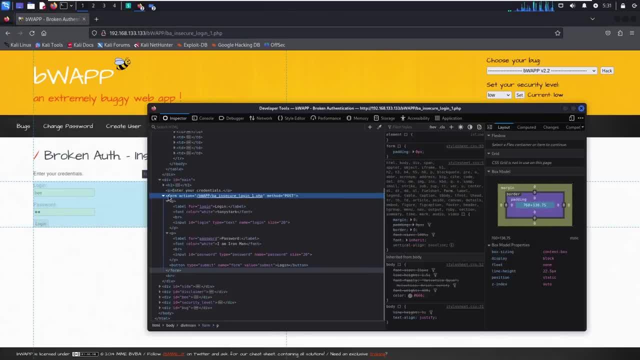 and simple. here is a form. okay, now let me edit as html. here you can able to see the login, which is tony stark, right, and the password is i am iron man, right. so this is a username and the password. right now let me use it: tony stark. 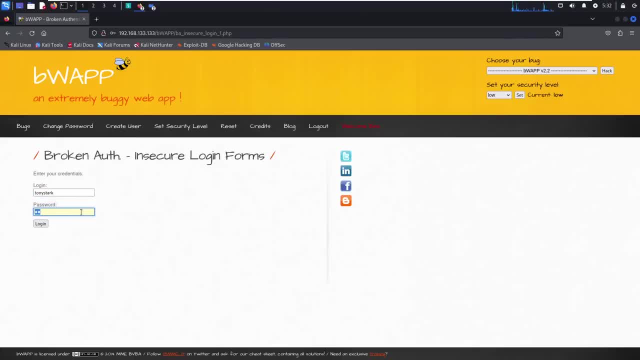 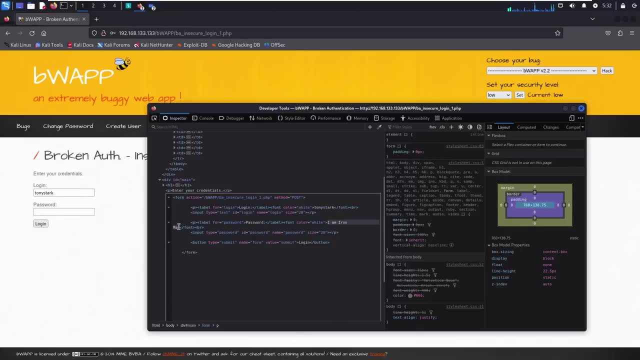 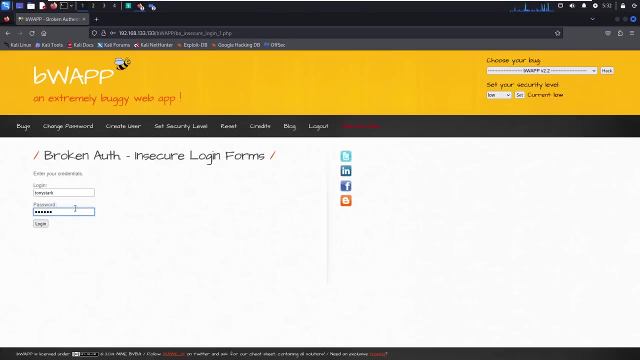 what is this? this is a nothing but insecure login forms. okay, so let's go here and look at what i am doing here. you see, successfully login you. you're really are iron man. this is the thing. basically, this is nothing but insecure login forms. right, just try to practice it. practice it. let me see some other. 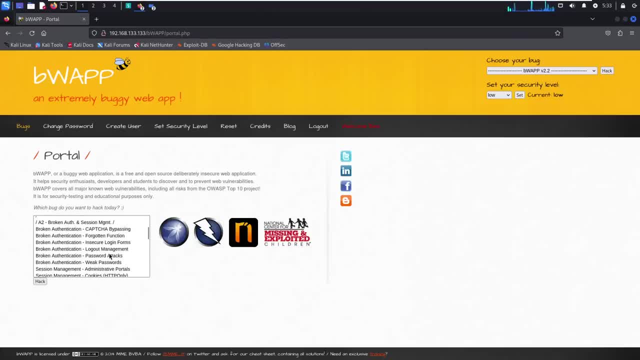 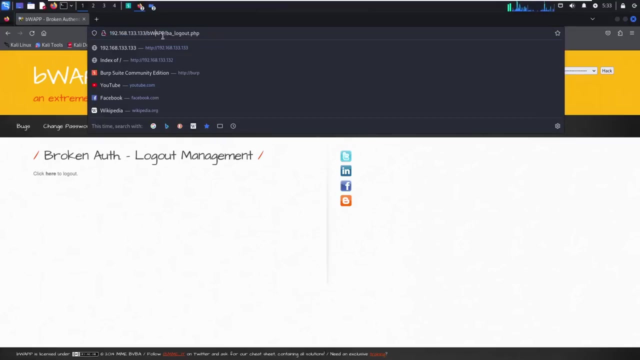 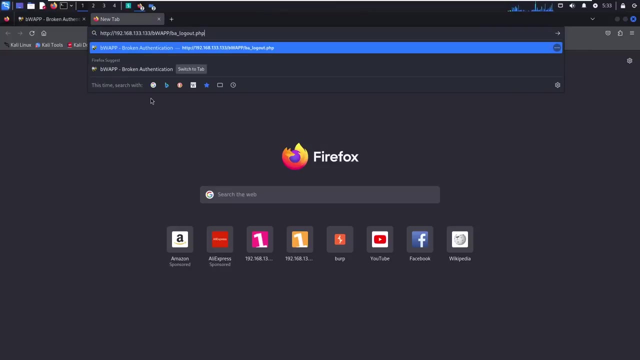 things here. there is a which we just weak password. is there, right, like testing? a which we just learn in the last classes. see, there is a logout management. is there. what is this? let me tell you. see there is a. let me open the same URL in another tab. okay. 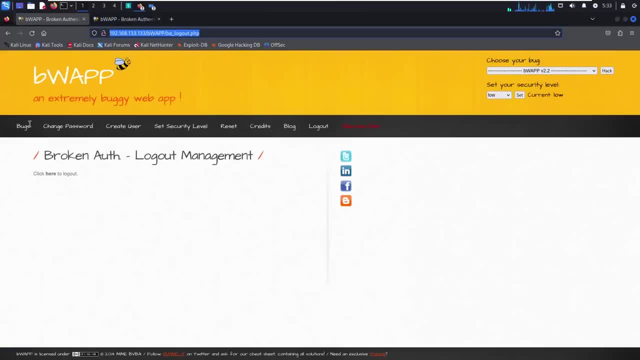 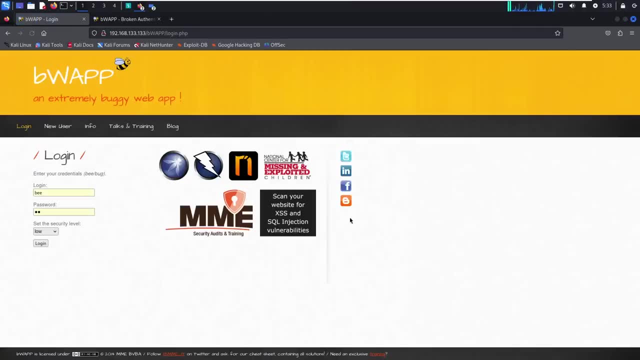 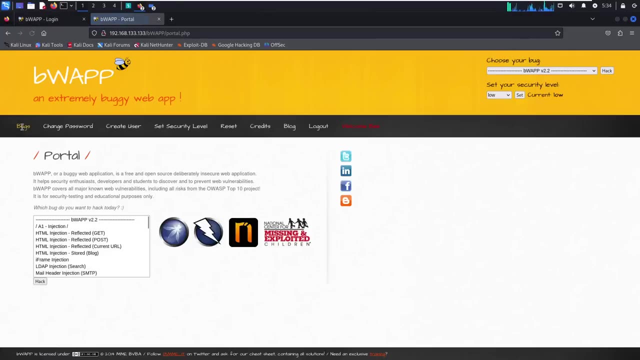 This is the same URL. see, if I type click here to logout, let me click here to logout from here. okay, simple, click. okay there, right, I successfully logout from here and let me go back to this page. is simple here, still, I can able to access this page, right? this is the. 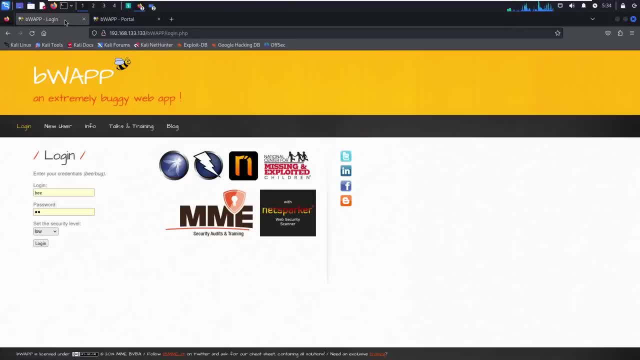 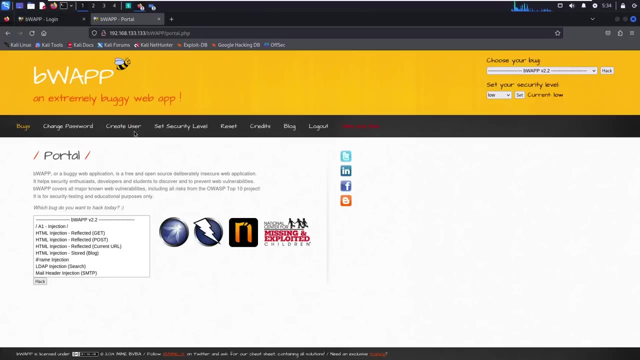 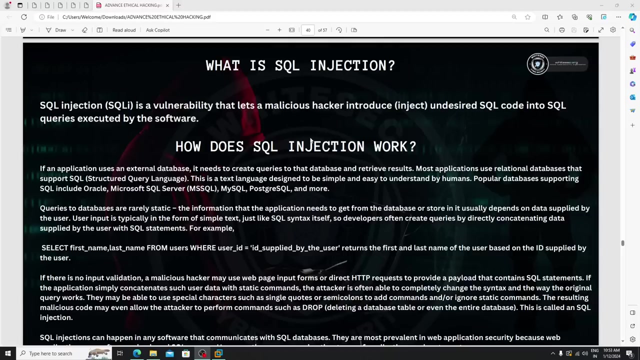 thing. basically it comes under what? insecure login, sorry, logout management, right? So this is the thing, basically: the once we logout, So logout from any page, then it will automatically it's a logout from other pages as well. okay, this is the thing. now in this class we are learning what is SQL injection. SQL injection: 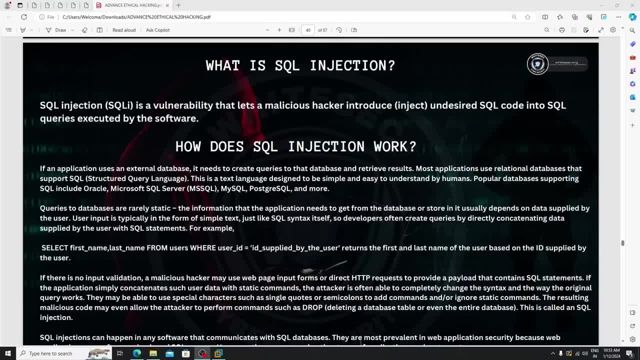 SQL is a vulnerability that, let's say, malicious hacker introduce, inject undesired SQL code into SQL queries executed by the software. this is the thing Now. the thing is, you just need to learn a basic of SQL. what is a basic of SQL here, like how it's working? 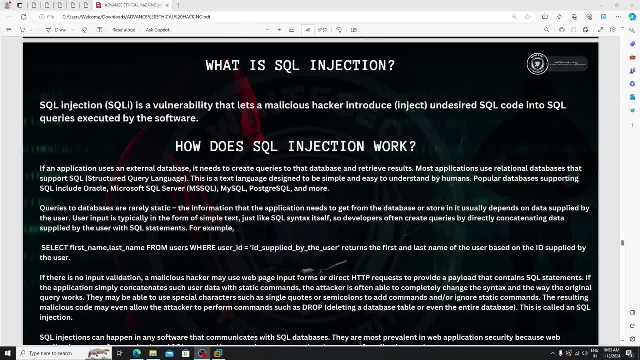 That's it. no need to go deep in it, simple, just try to. there are a lot of half an hour videos as well, one hour videos as well on YouTube channels. just try to watch it. you no need to practice it, no do nothing there, just try to watch it. okay, and just try to. 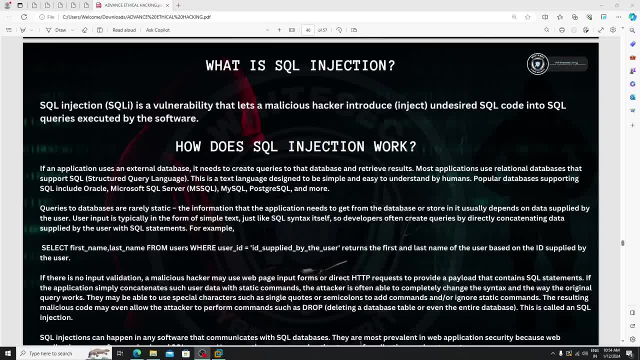 understand how it's working. okay, it's a very easy way to understand. it's not a kind of coding or something. it's a clearly in plain text like you guys can able to understand it in a like in 10 minutes It's you guys can able to understand the concept that this is the thing. so here there are some. 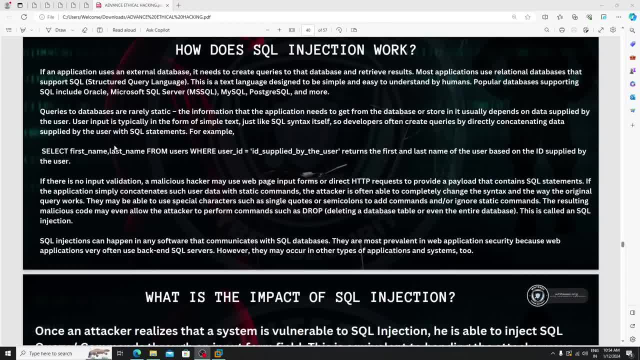 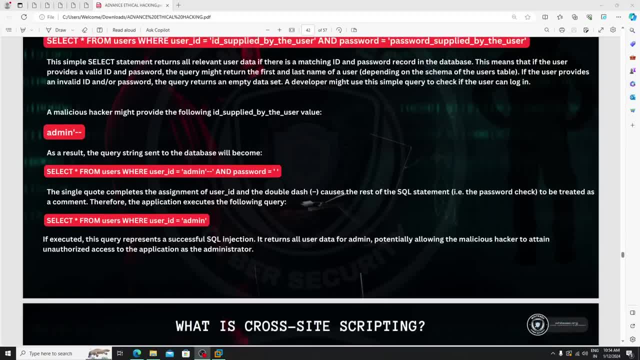 examples. just try to read it. it's not a big deal for you, just try to read it. and also there are examples of SQL injection. this is how it will work. okay, so read it, it's not a big deal. again, I am saying majority of people will think that, okay, SQL injection is also. 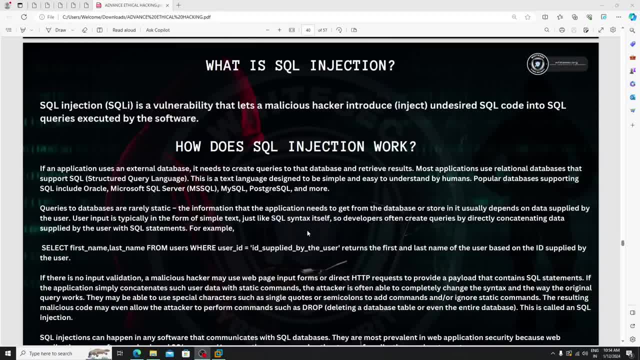 a kind of Python or something like that. No, it's not like that. it's a very easy language. like I don't do the projects on developing simple You get see. our work is what our work is: to test the software right, so simple we need. 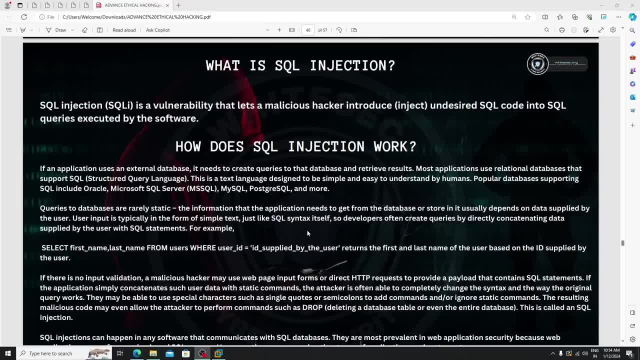 the basic things, that's it. okay. then we will use some tools, some automation tools, to perform this attack. this is a thing. just keep this in your mind. you are not a developer here. you just need to learn the basic thing, that's it. after, just assume that you are doing a. 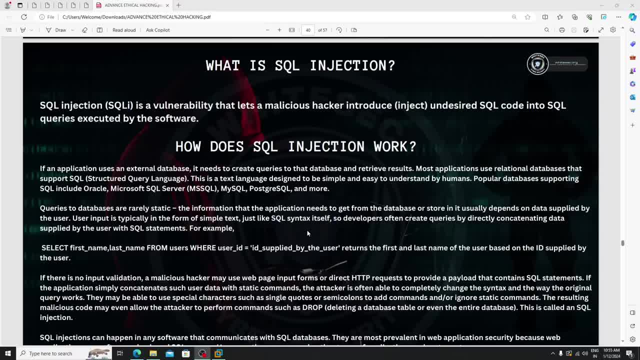 lot of pen testing projects there. automatically you will get that experience and you will learn a lot there. this is a thing. But As for a beginner, what you need to do just learn the basic things about the programming language, about this SQL. again, I am saying no need to go deeper in it, just learn how. 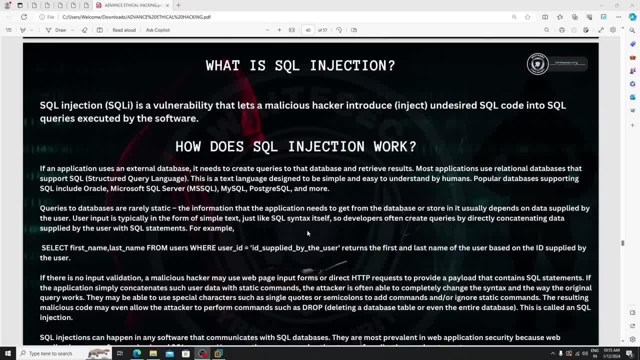 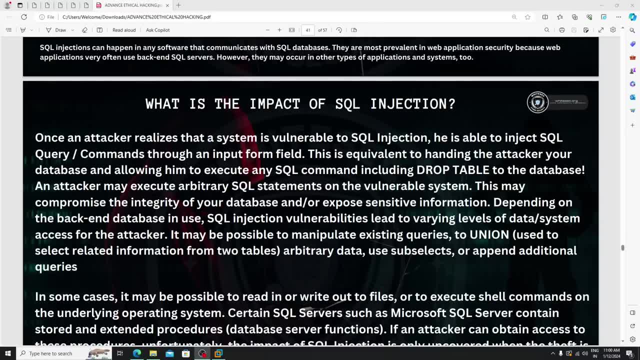 the things are working. that's it okay, right? So in this class we are learning what is the impact of SQL injection. once an attacker realizes that a system is vulnerable to SQL injection, he is able to inject SQL query commands through an input form field. This is equivalent to handling the attacker to a database and allowing him to execute. 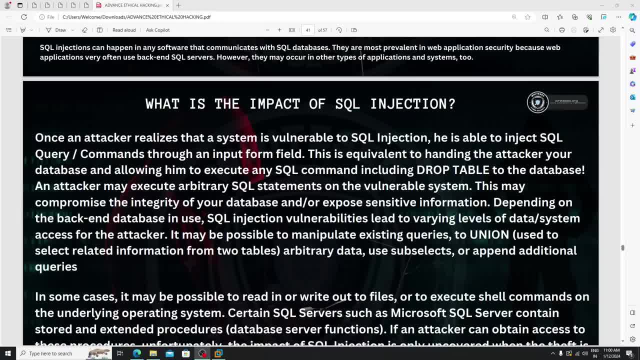 any SQL commands, including drop table, to the database. an attacker may execute arbitrary SQL statements on the vulnerable system. this may compromise the integrity of your database or expose sensitive information, which we see in this classes. you will get it okay once you jump in practical class. you will get it okay. 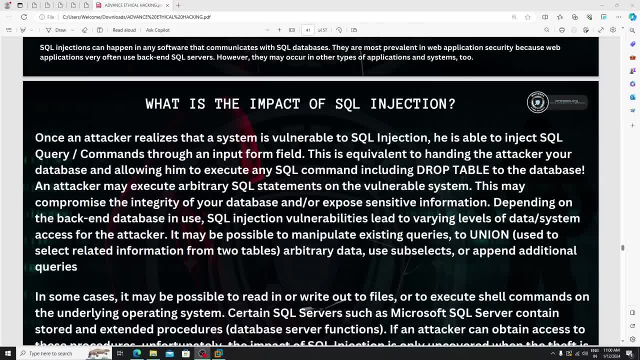 Depending On The Data base in use. SQL injection vulnerabilities leads to varying level of data system assessing for access for the attacker. It may be possible to manipulate existing queries to union used to selected, select related information from two tables, arbitrary data use sub selects or append additional queries. 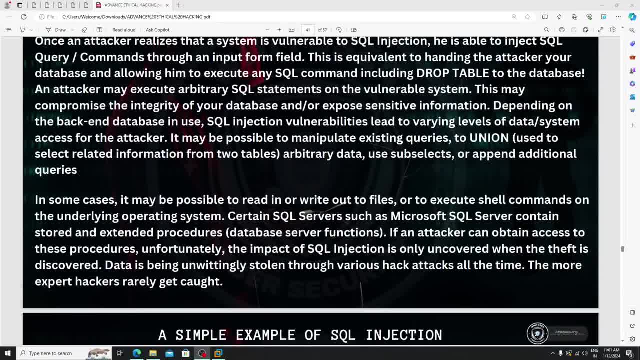 In some cases, it may be possible to read in or write out to files or to execute shell commands On The Underlaying operating system. Certain SQL servers, such as Microsoft SQL server, contains stored and extended procedures- database server function If an attacker can obtain access to this procedure. unfortunately, the impact of SQL injection. 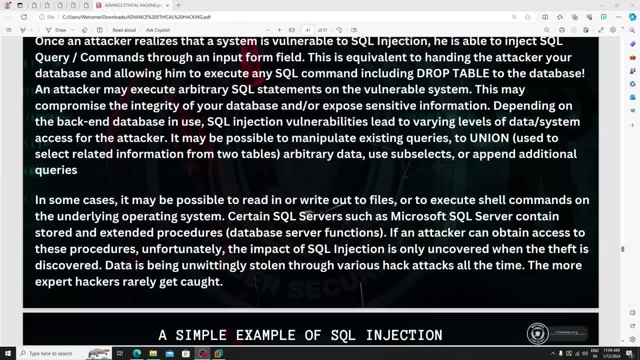 is only uncovered when the theft is discovered. Data is unwittingly stolen through various hack attacks all the time. the more expert hacker rarely get catch. So basically, the main of main aim of this SQL injection is to get the shell on the server. yes, by using SQL, you can able to get the shell there. okay, like you will get the access same. 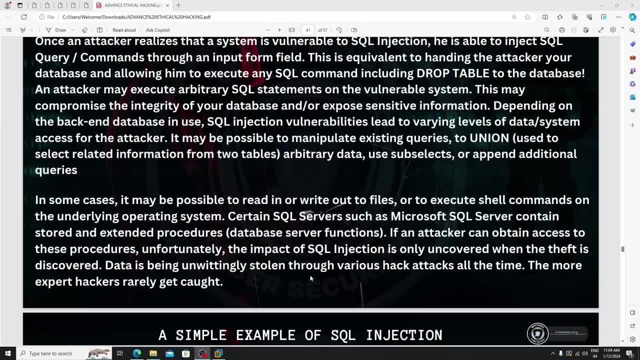 like command injection. and the second thing is we can able to the attacker can able to do what he can able to show, steal the data from it. like assume that in the SQL server, in that SQL database, there is a credit cards are there. simply he can able to steal it okay. 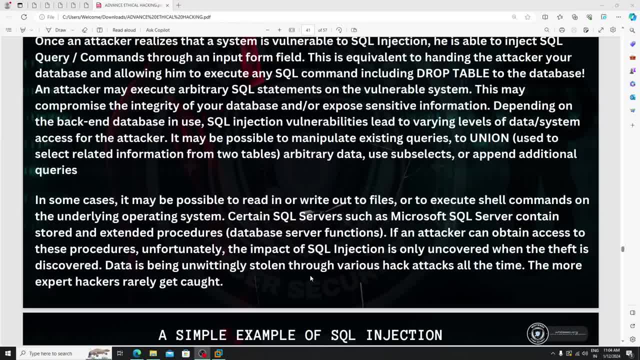 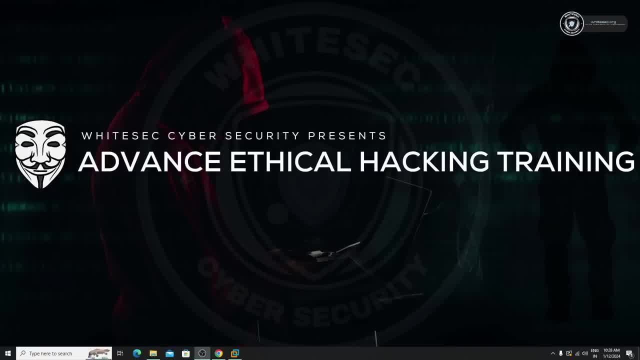 if there is a user e-mail address is there. simply he can able to steal it. this is a thing will happen. you will see in the practical class. hello guys, hope you are fine in this class we are learning how we can able to perform it. simple thing is: first of all, you need to. 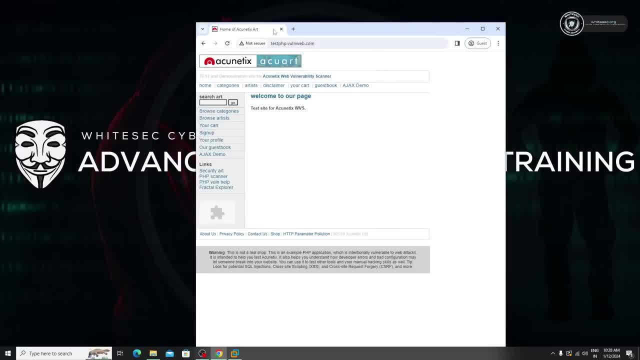 find parameters. assume that this is your target domain. here you need to find the parameters. how to find the parameters? in ethical hacking training, we just covered a very easy way to find the parameters. Let me show you manual as well. Let me show you how to find the parameters. 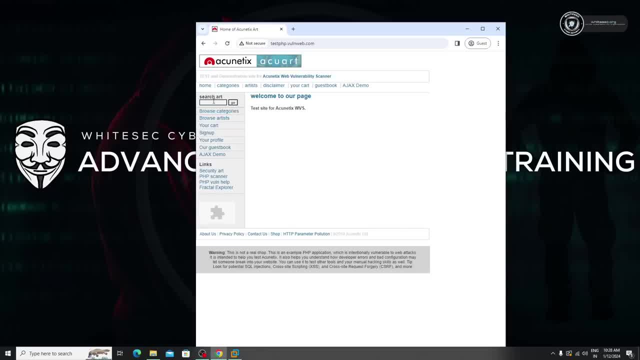 First of all, see the input field. if there is any kind of input, such as search or enter your name, this kind of field, then simple, just type your name just here. just type something, right? if I click on go here you can able to see the parameter. okay, what is a parameter? 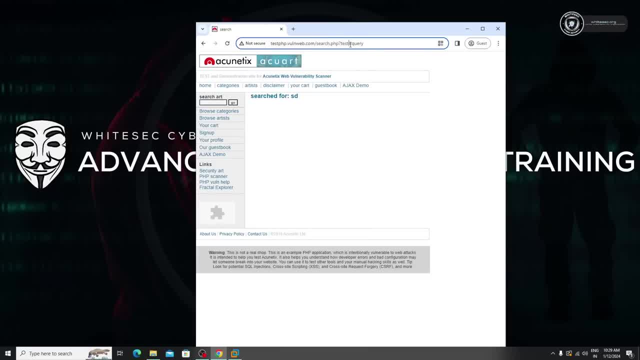 parameter is nothing, but just think this like this: okay, which is shows is equal. okay, right, and here there is a lot. now let's explore it. there is a browser artist is there? there are three artists. basically, if I click on any from here, anyone from here here, I got. 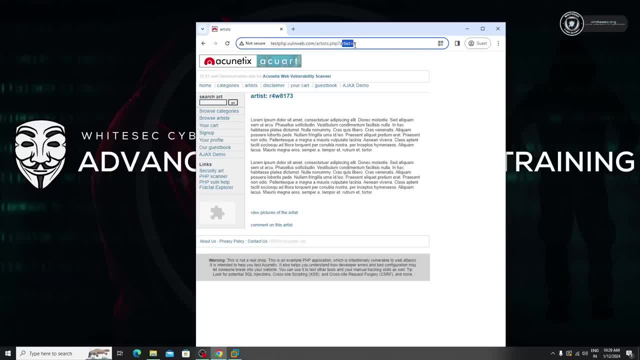 one parameter again. artist is equal one. okay, now how to check: is there any kind of vulnerability in that parameter or not? simple see at ending. okay, at ending after one. just type single code, just type enter. if you see any kind of error here, that means the site is vulnerable. 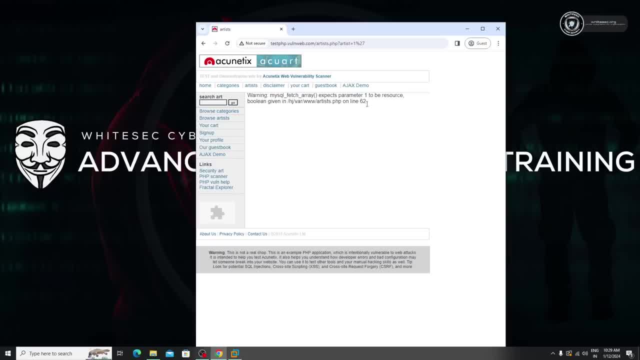 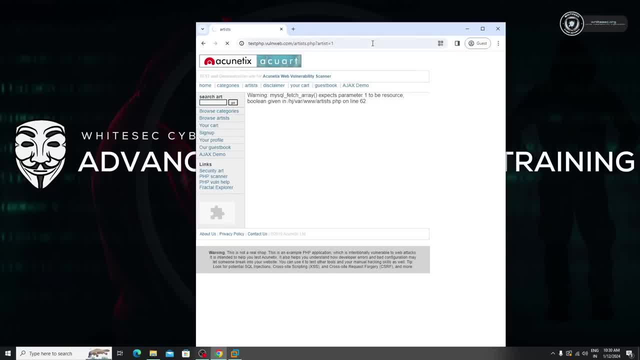 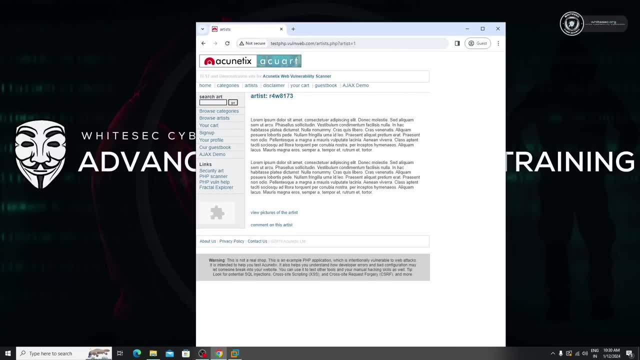 I got the error: ury expect parameter 1 to be resource. now I got that this. this one is a vulnerable. simple what I need to do, simple from here, also from URL. you guys can able to hack it. okay, by just typing the query. you can able to do it. okay, but let's do it by using a SQL map, because 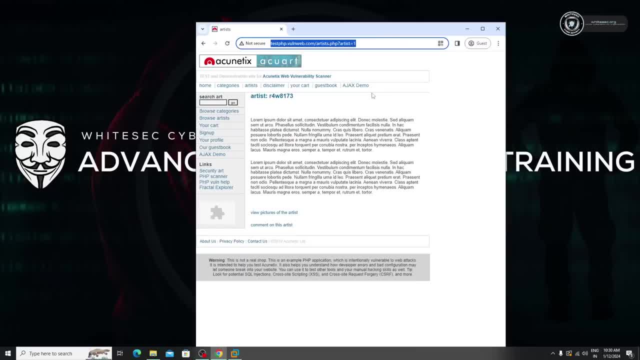 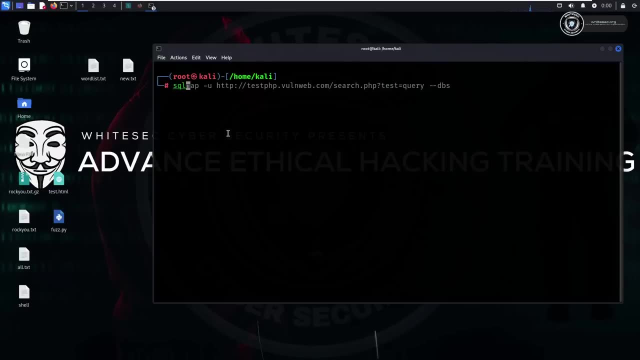 SQL map is a one of the excellent tool. by using it, we can able to perform full in a automation way. Okay, let me copy the URL here. Let's go back and see here: just type sql map, dash u for url and paste the url again. i am saying with parameter. okay, you need to paste with. 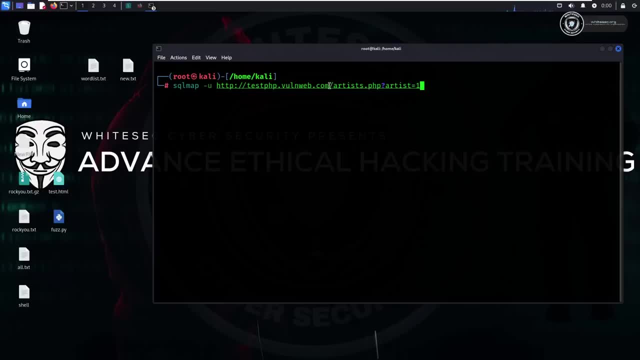 parameter. mostly people will think that okay, let's also paste with domain. don't paste with only domain there, you just need to paste with the parameter here. now then just type here: dash dbs, because we are getting the database here. okay, simple. by executing this command, what will happen? 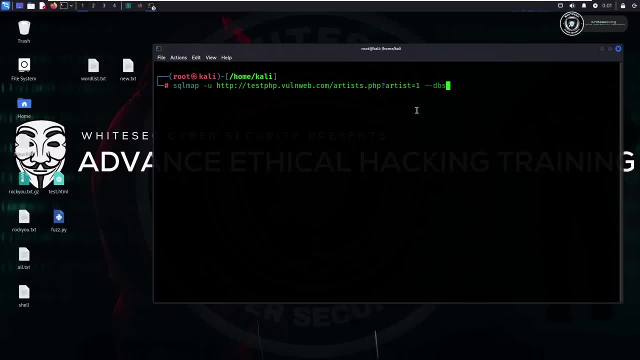 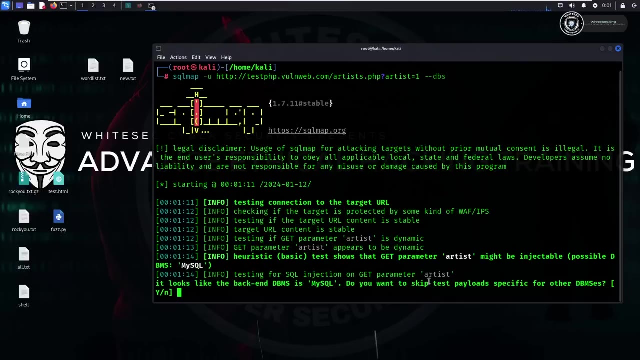 means we'll share the database names for us. okay, by executing this command, what we can able to see? we can able to see the database names here now. simple, just type enter. now it started. see here. uh, skip the test, uh, payload, sorry. okay, let me select y here. 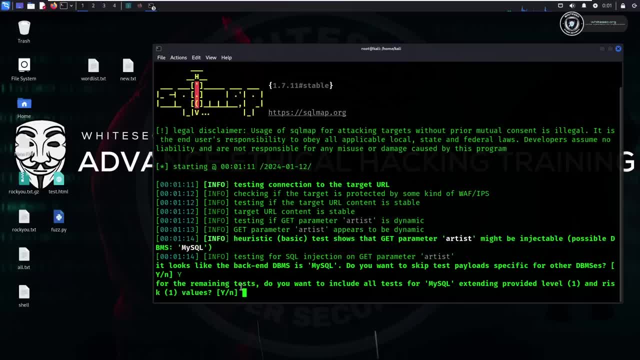 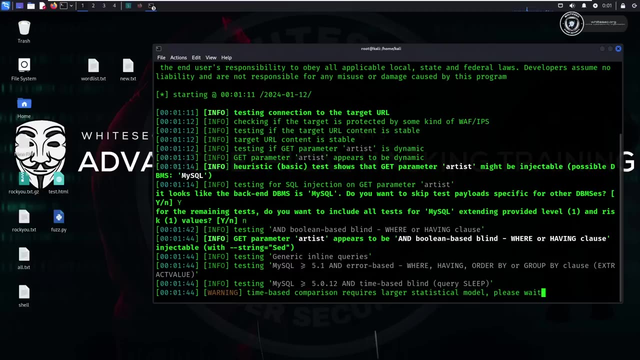 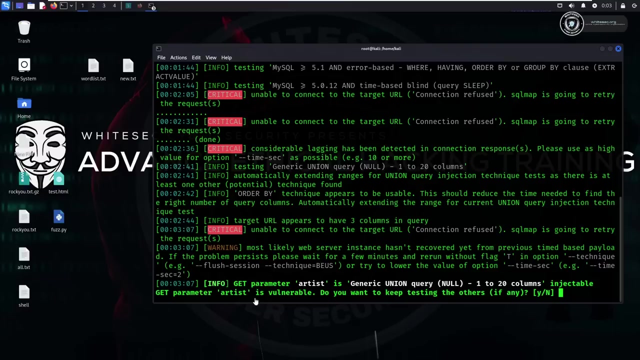 okay, now for the remaining test. do you want to include all test for mysql? just type here: n now it started. now here i can able to see: get parameter: artist is vulnerable. the parameter of artist. this is vulnerable. okay, now here, just type. i don't want to do it, just type. 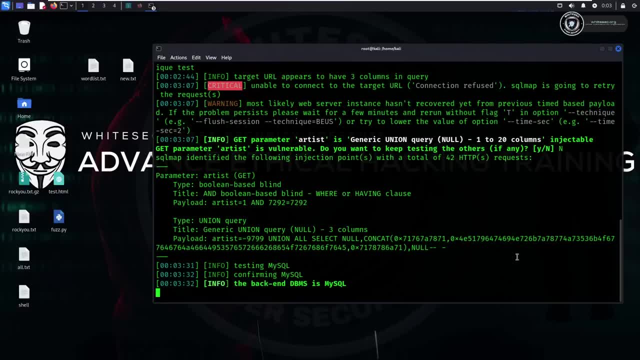 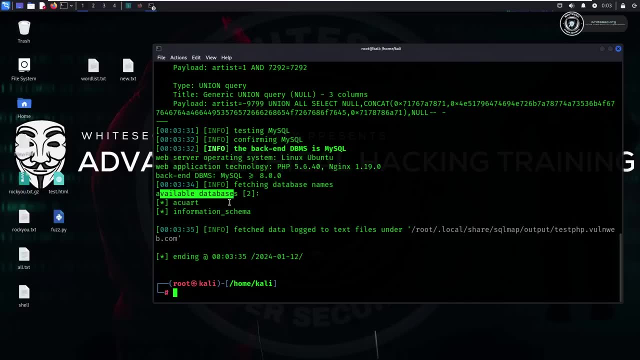 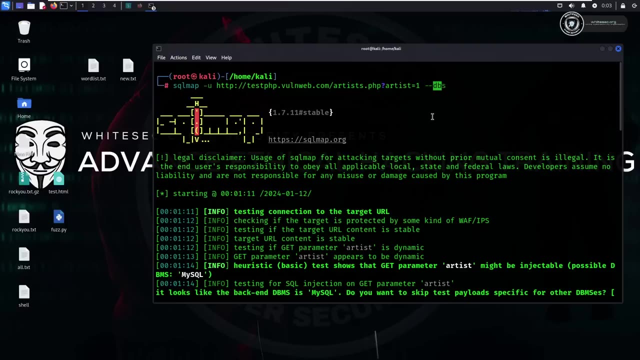 n there, just wait. so here you guys can able to see available databases. what is the aim of this attack? basically, first of all, i need to know the database names here. okay, because, uh, this database names are very important, right, uh, why it is important? you will get it without the database. 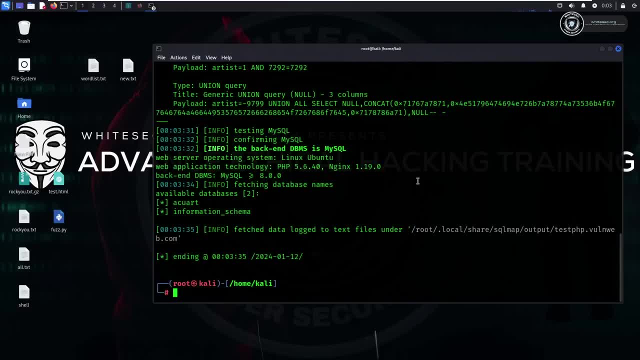 name, you can't able to extract the data from it. okay, this is the thing. now, here i got two database. one is uh, accurate and one second one is information schema. see information schema is a by default one, mostly insights. you guys can able to see it, just try to see. there is a data with the username of the site. 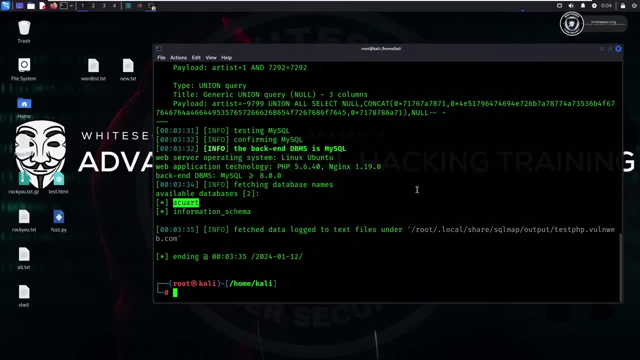 okay. so this is a kind of juicy thing. let me select this one. i need the database name here. now let's run the command again. just type here sql map- the same command, and remove the database from here. okay, just you can also add uh dash d and paste the database name now accurate, okay, is the 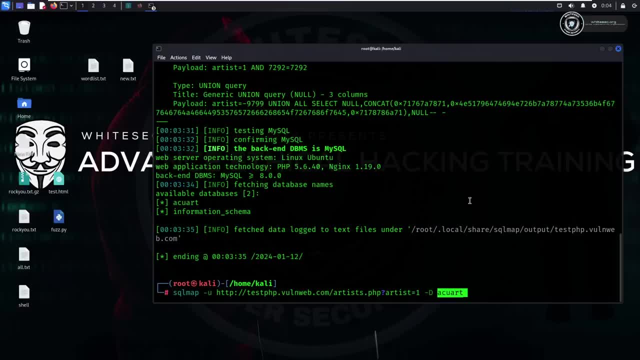 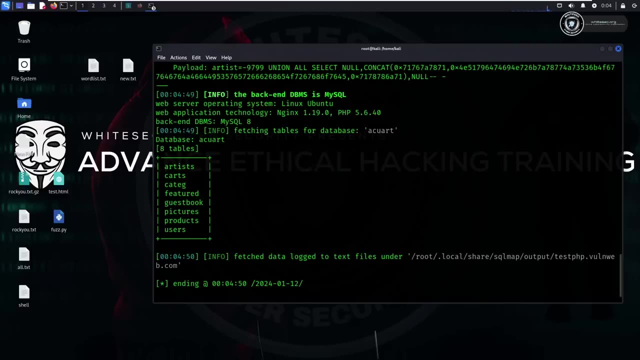 name. then now let's see the tables here. just type here, dash, dash, tables. just type enter. now see what. uh, you will get it. what are tables? see in tables what you guys can able to see in database name, in this database. there are tables out there such as username. 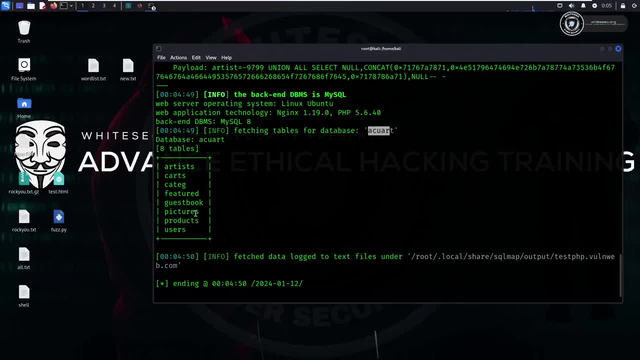 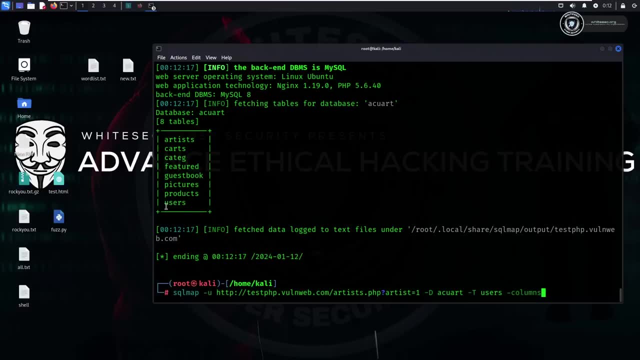 okay, users: products pictures. guest book. last table users. now let's see the columns here. it's a kind of: this is a folder. just take an example of this is a folder. in this folder there are some files with the name of email or something like that. let me show you. just type: enter here now. here you can able to see the real database. 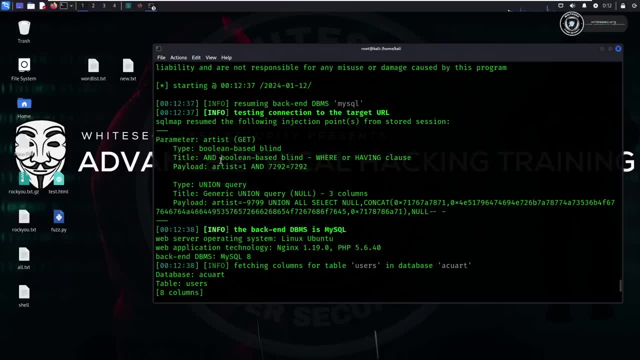 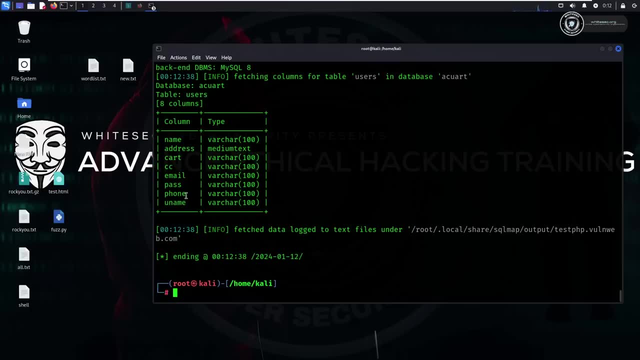 this is just a table, it's a kind of folder for you. okay, now these are the main files which you, which you need, which attackers need you attackers target? what here? the user information? right, so simple the thing is. here. we got the huge amount of juicy information, such as: uh, cc is there, which is credit card email. 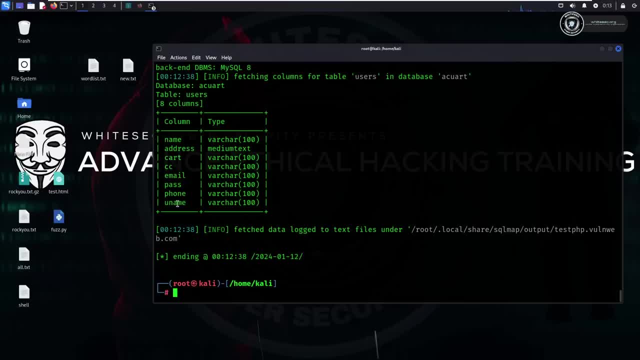 okay, pass phone you name. now i want to download this one. how to do it? simple thing is like just type here. i want to see the data here. simple, just execute the same command and just type here: instead of uh column, just type c, capital c there. okay, it's also a column, let me. 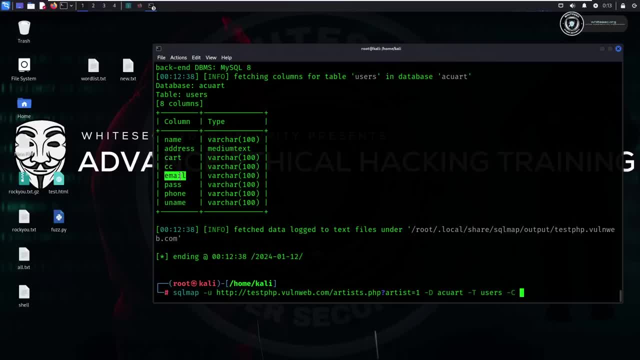 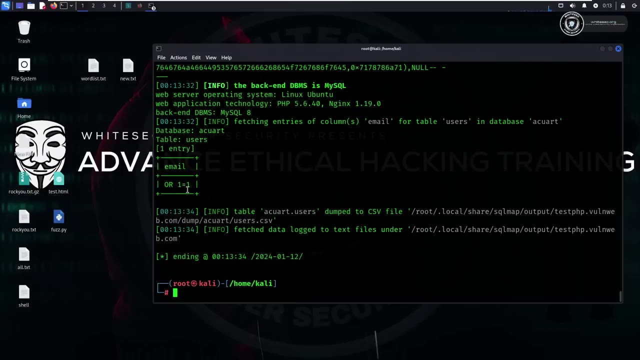 uh, dump this one which is email. just let me copy the name here and just simple paste it. just type here: dash, dash, dump. just type enter. now i can able to see the emails. see, there is a email which is one is equal to one. now, if i see the cc, uh, there is no data there, so that's why i can't able to see the email. 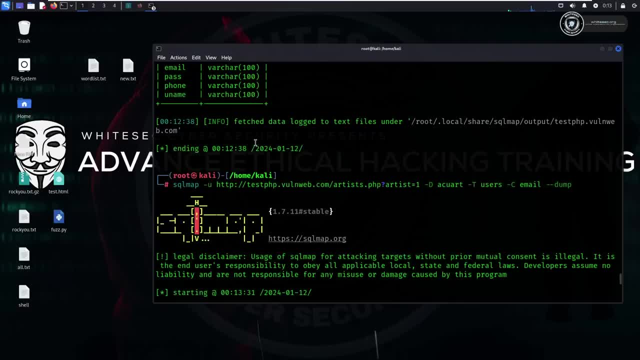 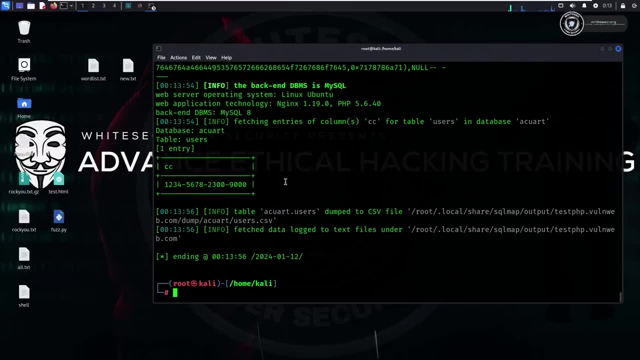 instead of email. let me see cc there, okay, so here i can able to see the credit card information. this is a test site, so that's why we can't able to see that much, but in real side can able to see a lot there. a huge websites are vulnerable with sql section. need to get it okay. 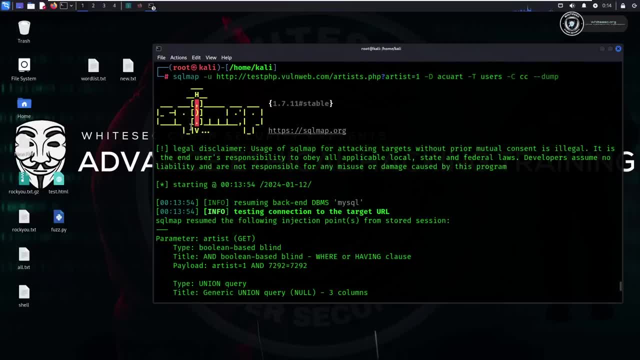 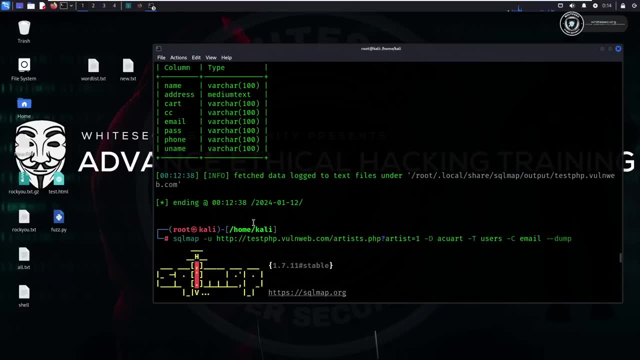 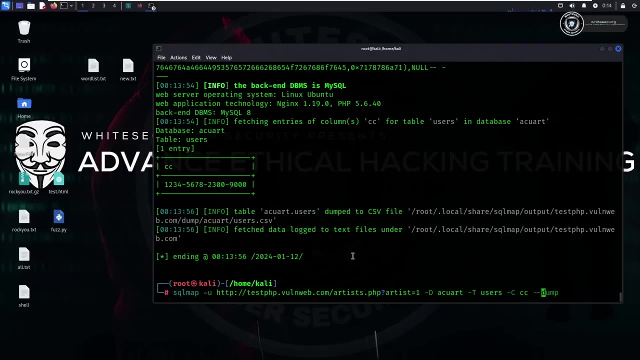 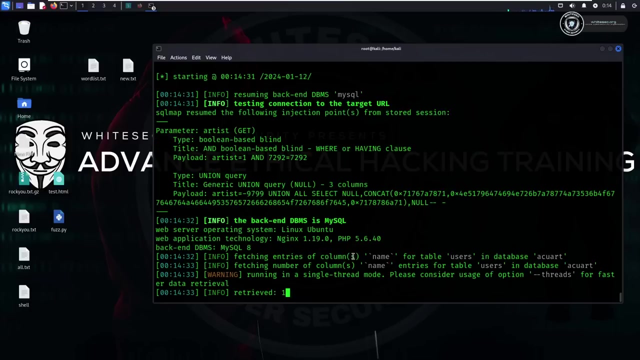 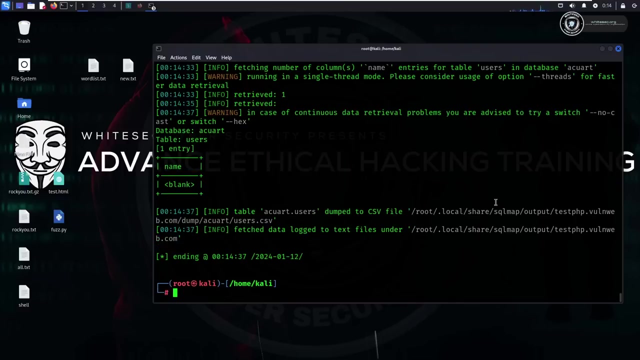 this sql map make our work very easier. okay, now let me dump other one. another one is: uh, there is a name is here i can able to see there is a blank, very blank. so this is how you guys can able to use a sql map. you guys send your classes. thank you, have a nice day now in this class we are learning about: 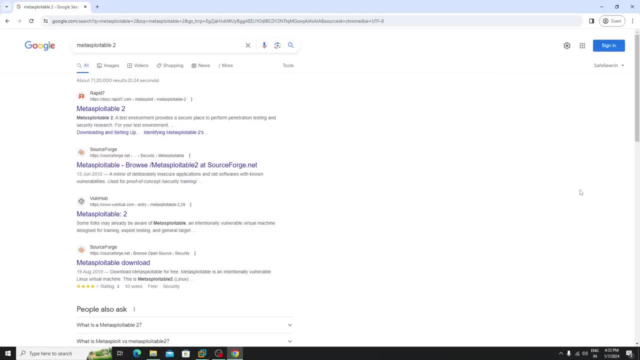 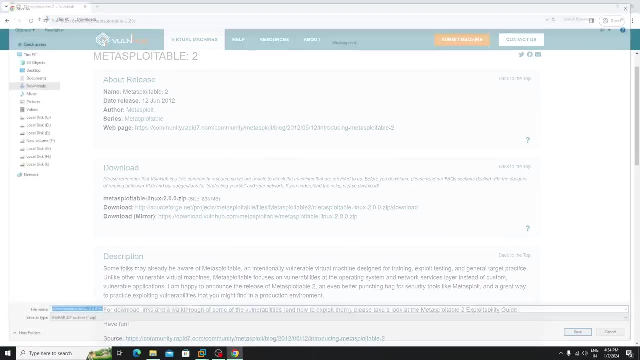 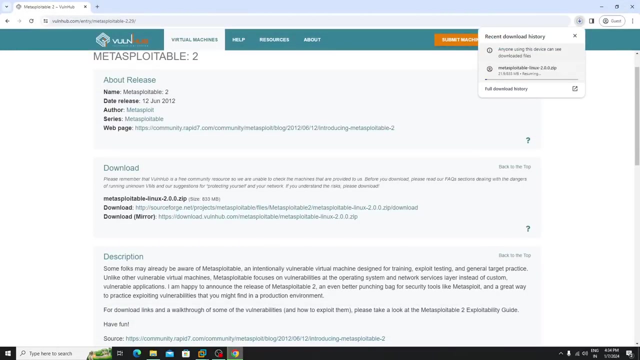 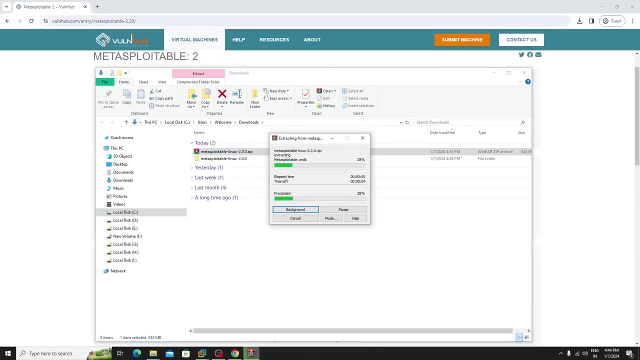 vulnerability scanning. let's go with metasploitable 2 here. simple, just search for metasploitable 2 and let me download it from one hub. it will take around 4 minutes. so here it is. let me extract it now. here you can able to see the vmx file: simple double click it. 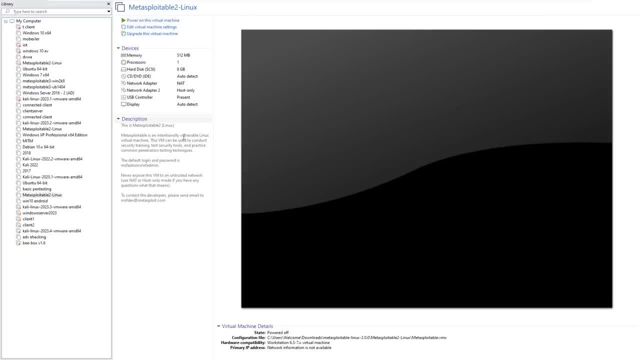 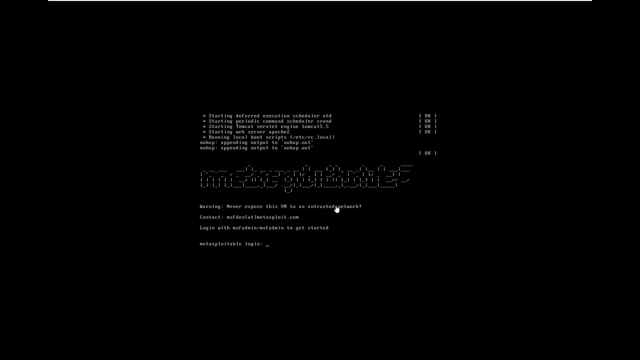 and here is a metasploitable 2 right. simple power on this virtual machine. see, the password is msf admin and, sorry, user is an msf msf admin here and the password is msf admin right, so simple you can't able to see mouse there. simple, you just need to type manually. uh, you. just need to type. that's it. just type your msf admin as a username and the password is msf admin. let me tell you you can't see password there while you are typing. simple, just type it msf admin and just type enter there. now i successfully log. 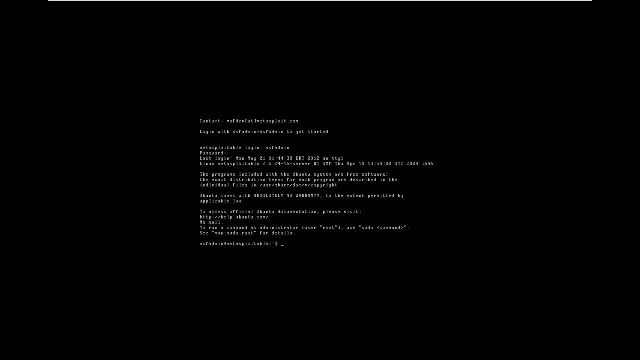 uh, log in here. now i successfully log. log in here. simple, just type here ifconfig. here you can able to see the ip address: 192.168.133.178. so in the next classes we are learning how we can able to exploit it. now in this class we are learning how we can able to perform nmap scanning right. so the thing is: 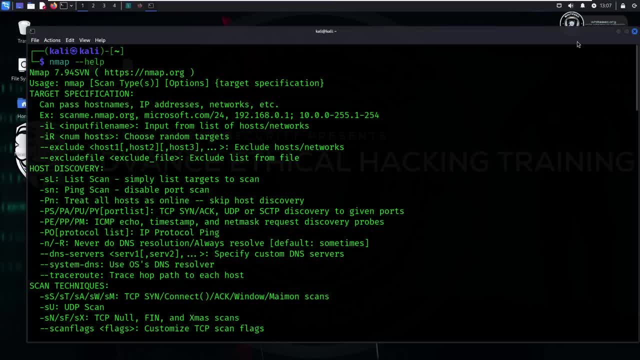 here. very simple. we just added a lot of classes as well about nmap in windows penetration testing, training in ethical hacking, training in kali nethunder training. also, we just use nmap a lot there. after watching this class, just try to watch those findings after completing this training. just 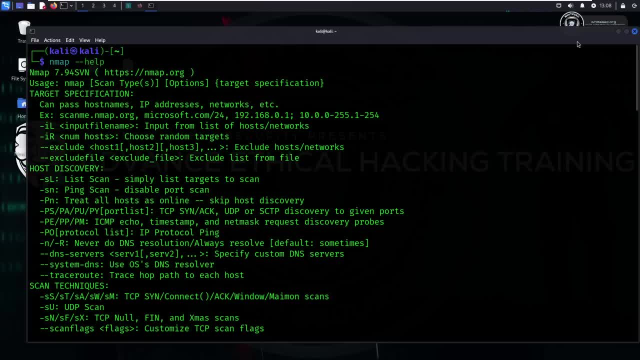 try to watch those trainings as well, because those things will help you a lot. okay, because here we just covered a lot of things, right? so this is the thing, right? uh, here the thing is just type in map space dash help. here you can able to see. 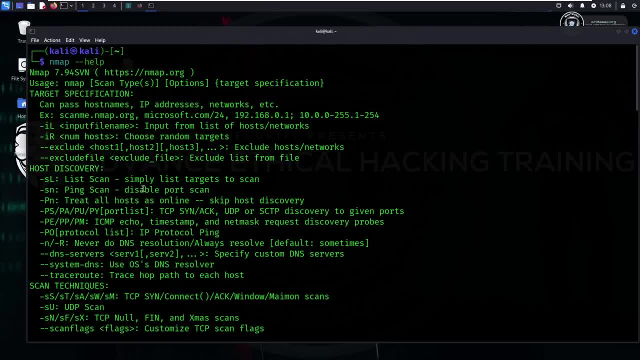 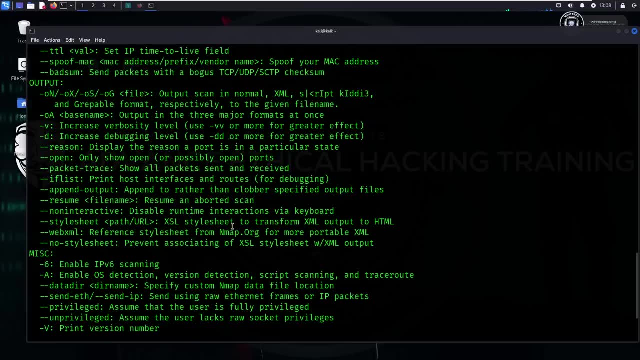 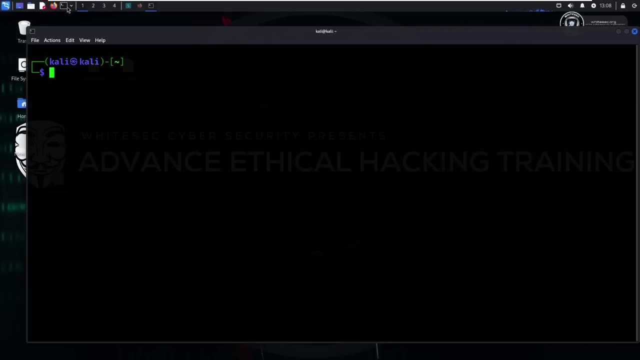 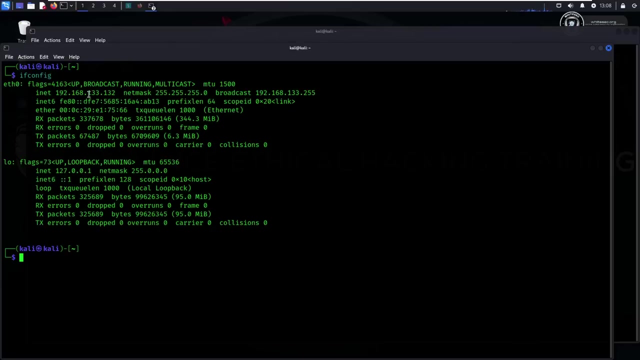 the help, right, so let's come now. the thing is, i want to scan, i want to see how many devices are connected in my machine, in my, in my network. okay, simple, what you need to do, just open another terminal here and just type ifconfig. this is your ip, right? just copy your ip address and just type here in map dash. 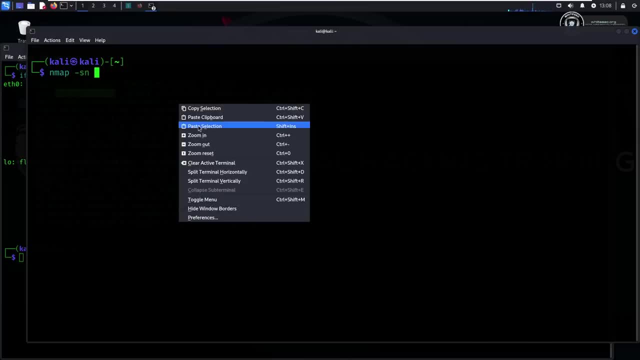 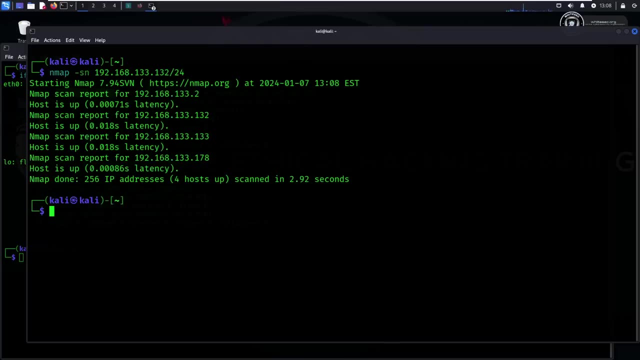 and paste your ip address and just type here forward: slash 24.. now it will scan for the devices which are in your network, right? so here the thing is, you can able to see this or that devices, right? uh, which is in my network. let me see my metasploitable ip address. 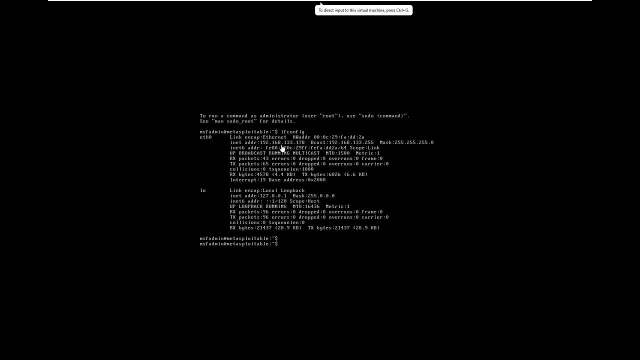 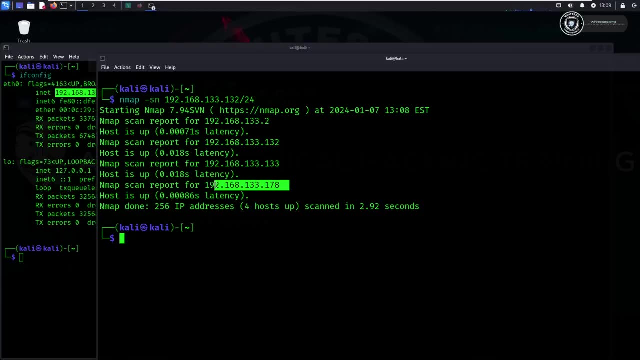 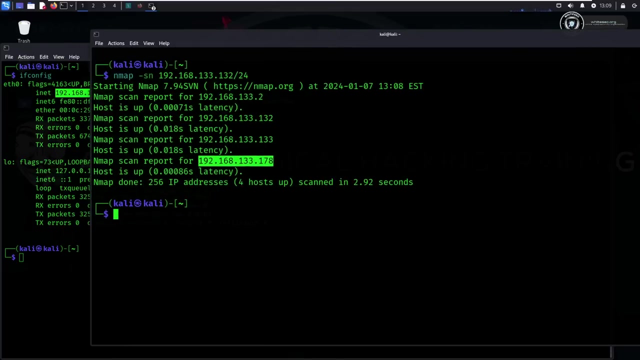 what is ip here? 192.168.133.178- the offices in my network. now a job. so for moment i will think crippleAND stuff with Numbers and documents. let me ask the same thing to acceptaza. all right, so now it thinks can theございます hair is basically 100. 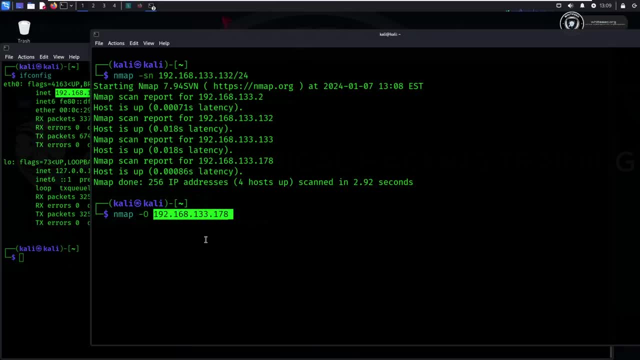 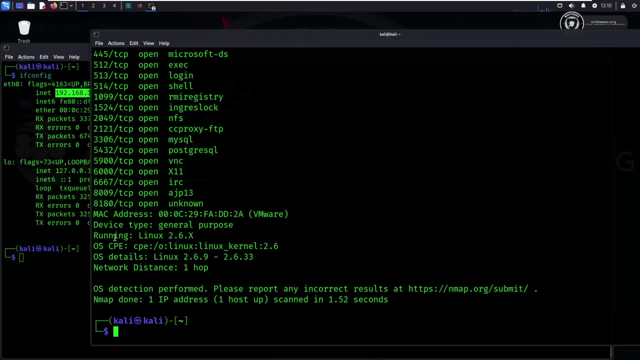 sorry, ah address and just type enter there. now you need to run this as a pseudo. if you run it as a normal user, then what will happen? it won't work so simple. you just need to type pseudo and you can able to scan it. now, here you can able to see: sorry guys, mac address and running is linux 2.6.x and here. 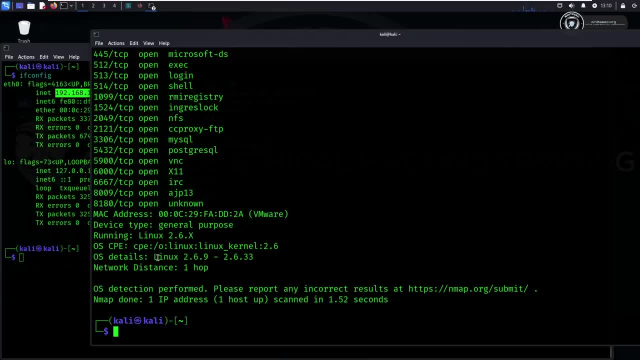 you can able to see the os details. here is the main thing, which is linux 2.6.92 or 2.6.33, right, okay, now here, these are the most common ports, right? if you want to scan, come, uh, all open tcp ports, then what you need to do 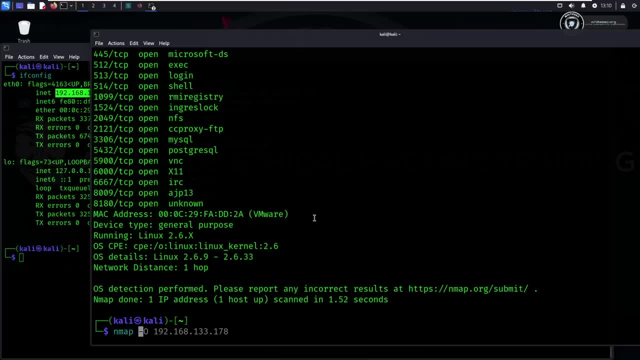 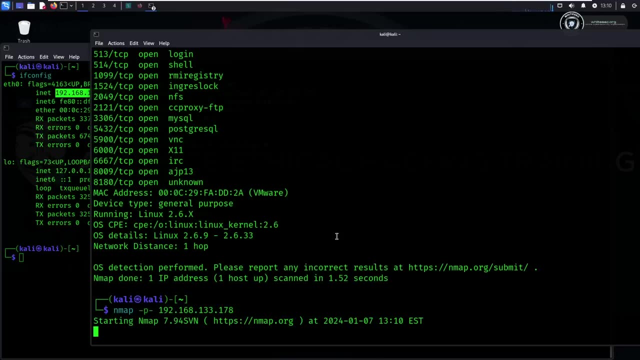 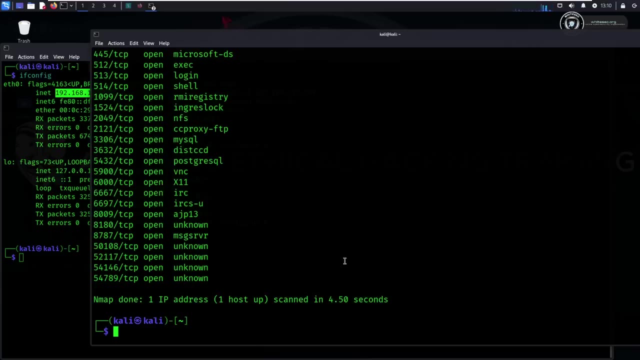 simple: just type here: nmap, dash, p, dash and paste your target ip. now it will scan for all open tcp ports here right now, let me tell you, a lot of students just ask that, uh, we are scanning nmap in real world, okay, and we are getting a lot of uh. 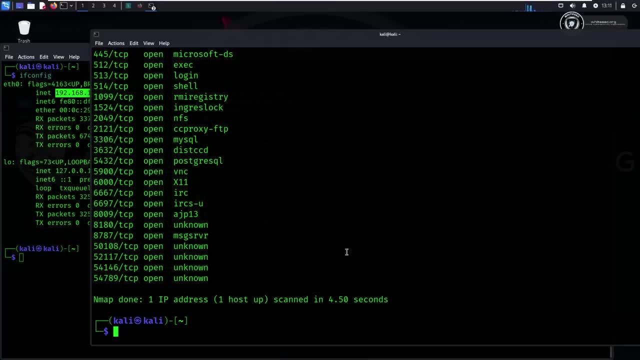 like the port is open there, but still we can't able to uh seen through nmap. okay, this is a thing. now, the simple thing is it might be due to firewall, or the port is open there, but still we can't able to uh see through nmap. okay, this is a thing. 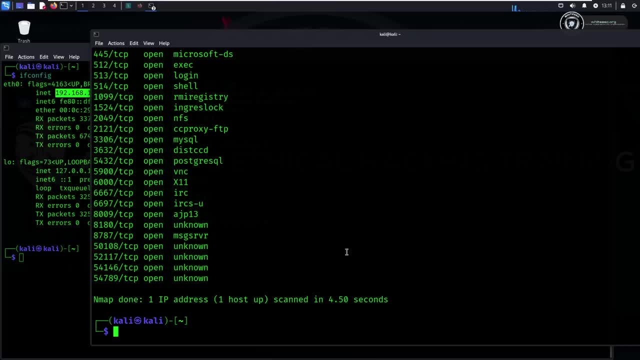 you are. you are generating a uh, huge noise there, such as you are executing a heavy command, such as, agree you are. if you perform the aggressive scan there, then what will happen means the firewall will detect it and they block it. okay, this is a thing. now here, what you need to. 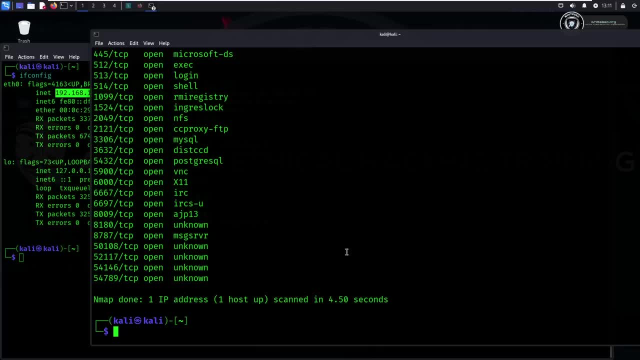 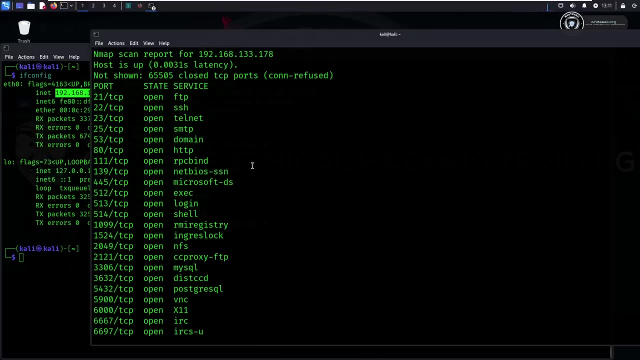 do means you need to perform a slow scanning here. okay, you need to do uh to scan the uh, the port which you want to target. now assume that i want to target uh telnet port. at the time we should check for a slot, okay, so first look, what should i do now? i need to do for dat Program. 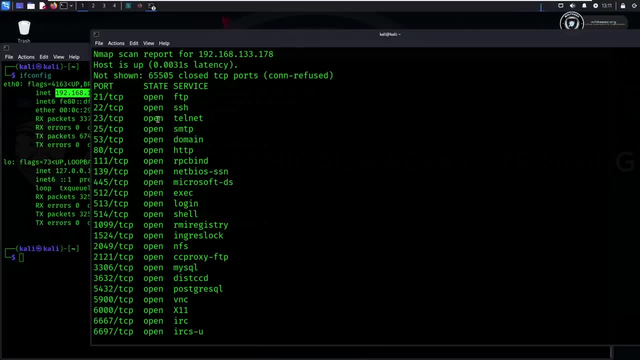 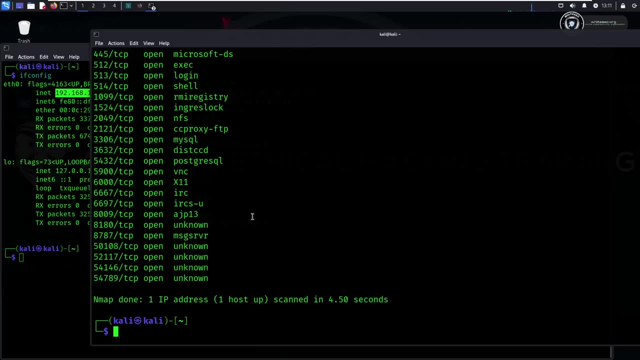 first. i am going to show you guys how i can uh test obtain if the systems telnet port is open in my target system at the time. what i need to do first: i need to check that in my target system telnet port is open or not at the time. what i need to do first: i need to identify telnet will. 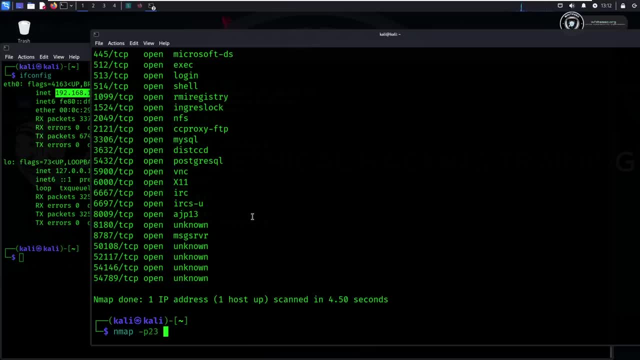 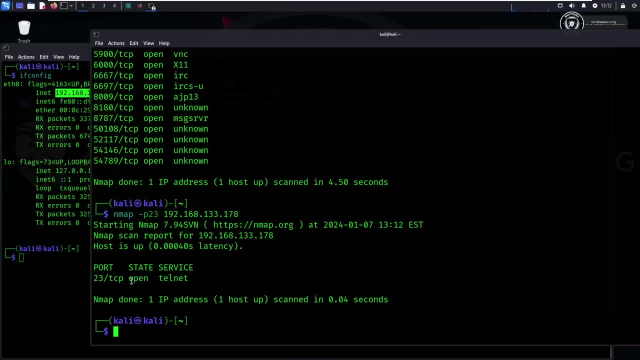 run on which port? simple telnet will run on port number 23. first i need to identify simple like this: nmap, dash, pe, simple. let me specify only one port here and then let me paste my target ip address. the state port is open. okay, the service is telnet here. this is the thing. it doesn't generate a huge. 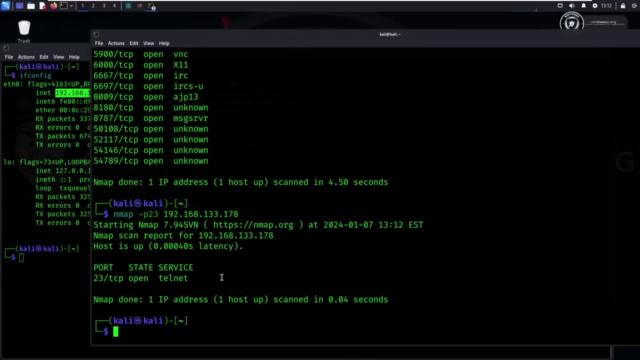 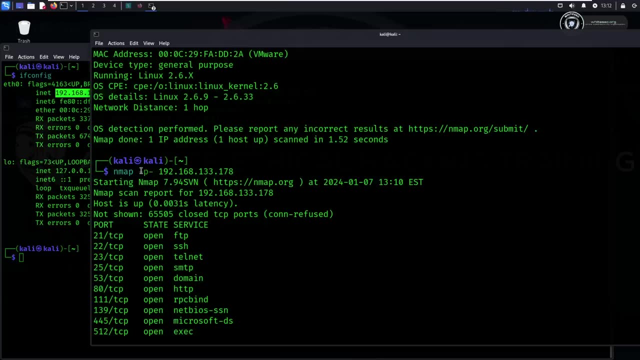 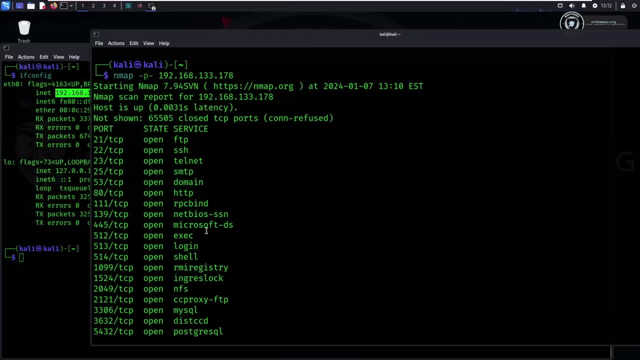 noise, right, so it is easy to. uh, we can able to see it. okay, assume that in real ip addresses, if you, if you type, such as nmap, dash, p, dash, then what will happen? it will generate a huge noise and firewall will detect it and it gonna block it. okay, this is the thing. you can't able to see. the 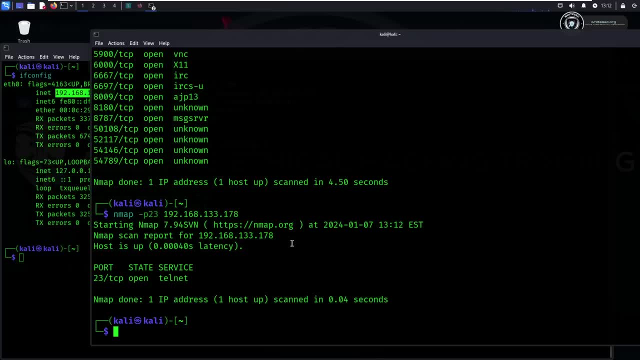 results here now. and the second thing is, a lot of students also see that there is here. they will see tcp map. let me tell you it's also due to firewall right? so at that time what you need to do means just perform this scan, such as nmap. just use dash p1, capital t, and just type dash p. 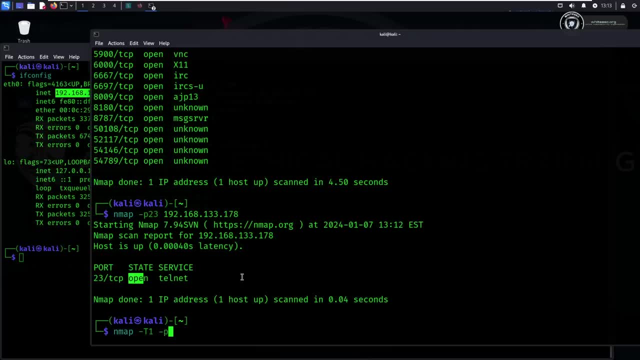 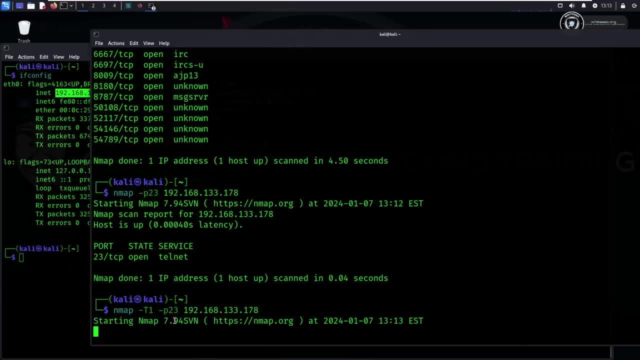 and specify that port, your target port, and execute that command there. if you want to add a service version, detected detection, you can also add it, but you don't run it uh in in all ports. okay, this is the thing. you need to target specific ports there which you want to attack. but in uh labs or in ctfs you can able to do it, mostly you. 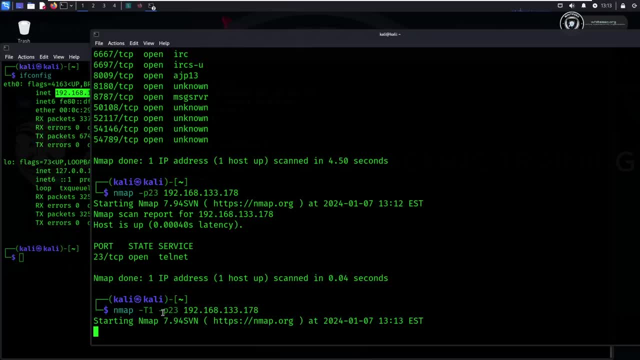 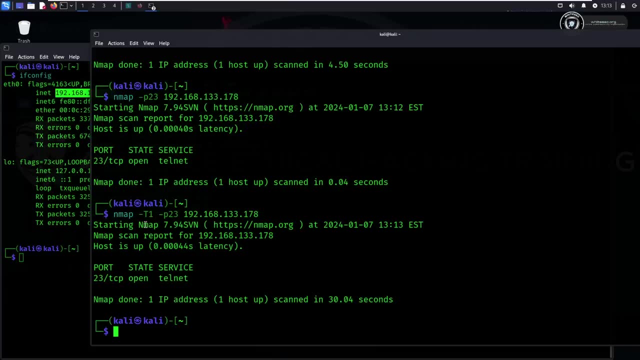 can't see the firewalls here. okay, this is the thing. now see how slow it is. even scan will very slow, man. okay, like it doesn't. uh, it give you a very excellent results, but it will take a huge time. now here i can able to see uh state is open, uh, and also remember if you see tcp. 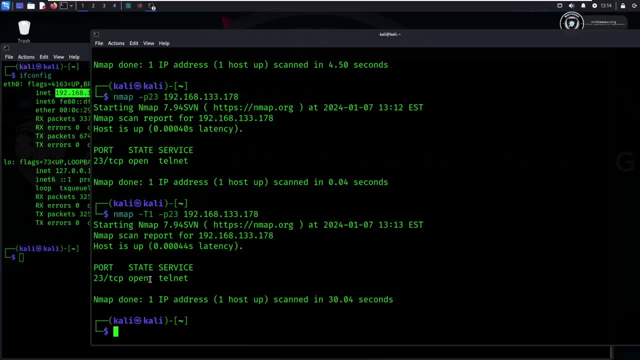 wrap the uh, then what you need to remember means: sorry, tcp wrap. if you see this kind of uh state here at the time, just assume that you know the firewall is in a state like this. you can see that it's enabled there, or uh, the port is closed. this is also one thing. so the thing is, if you just try to 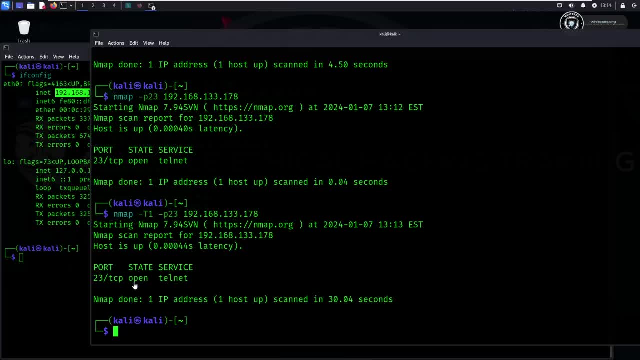 watch our windows penetration testing training. i just covered there how you guys can able to identify- because by checking uh in wireshark you can able to get it. okay, like assume that here, due to some firewalls issue, you can't able to see it, but in wireshark what? what will happen means you. 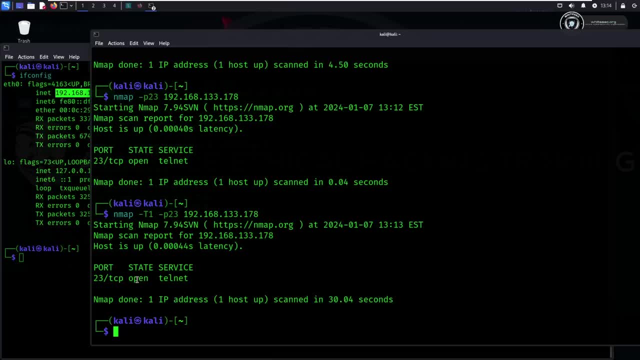 will get a synapt packet from there, from your target. okay, then, if you get the synapt pack, then a packet, then what will happen means: uh, that means the port is open there. okay, this is the thing. you won't get, this words. i know that. uh, i just told. 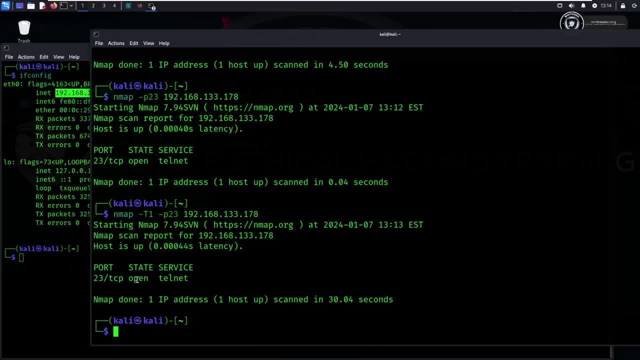 you synapt right. mostly you guys are beginners. you won't get it, so the thing is just ignore it. after completing this training, just watch the windows penetration testing training. there. you will get it okay, because you need to watch that complete training. don't practice simple. first watch the training, then 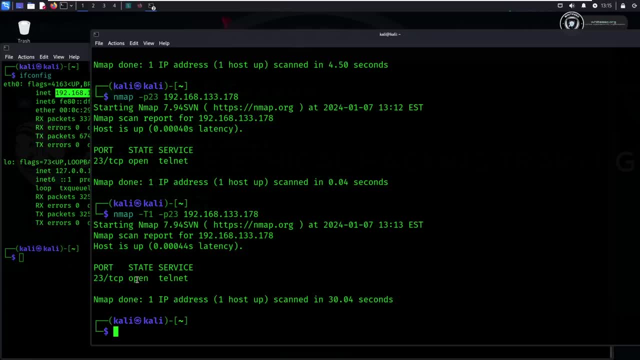 start the practice. okay, this is the thing. just try to watch it in 1.x, 2x, something like that. just complete it, because that training is very important if you want to learn more about nmap. okay. so this is the thing, guys. it's not a big deal. okay, it's not that much difficult. it is very easy things. 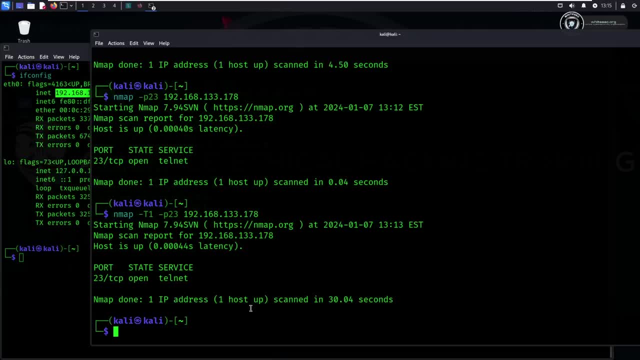 right, but you need to know what is going on back end okay, like how the things are working. if you learn these things, then the things are very easy for you. now here. the second thing is there is also a script scan. okay, so if you execute this uh script scan, what will happen means it will give you a. 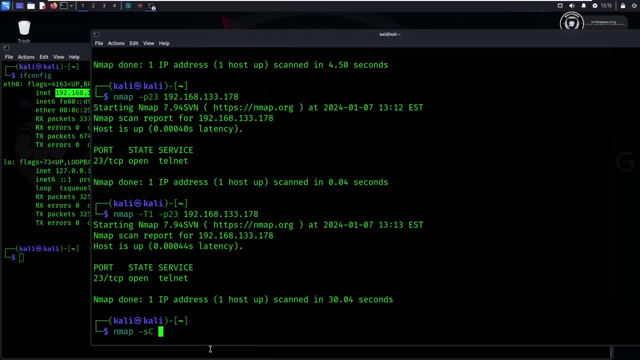 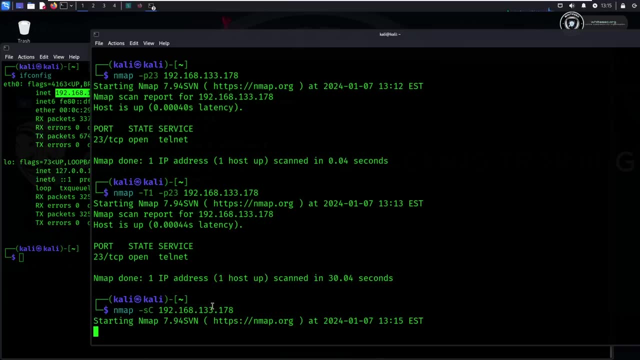 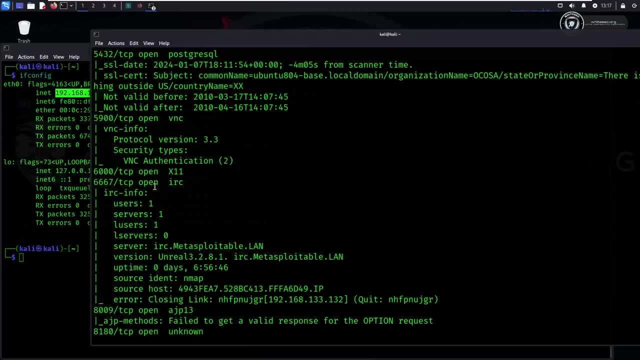 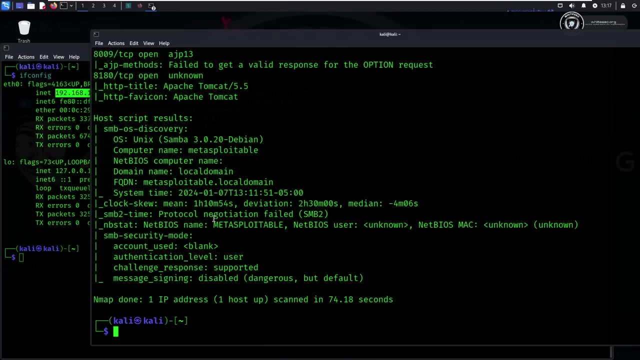 more details about your target ports. okay, like, let me show you. so here is a results. okay, here you can able to see the details, a huge details about your- uh that ports which are open. right, so this is the thing. and also there is also a vulnerability scan. by using this, you can able to perform. 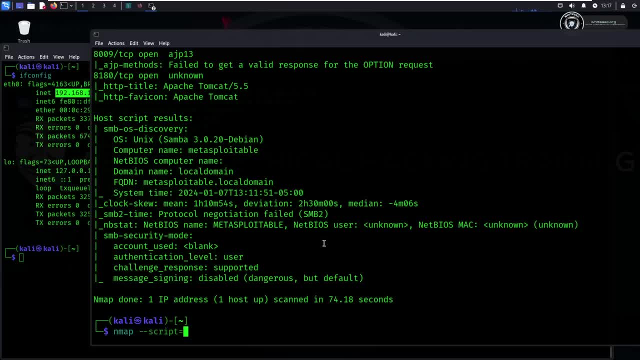 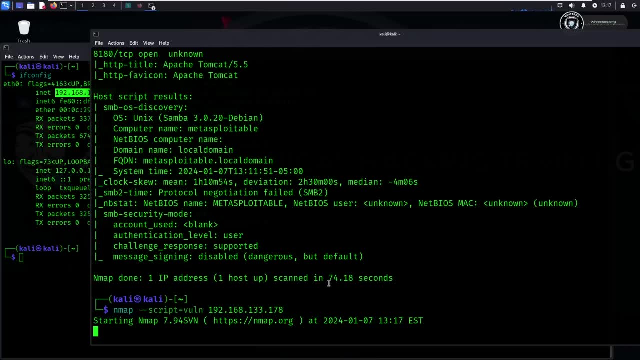 this service is vulnerable and how you can able to exploit it will give you a complete idea. if you want to perform the script scan, you also need to add aggressive. I think, just wait. I think, uh, service version detection. you need to add there, just wait. if it doesn't work, then 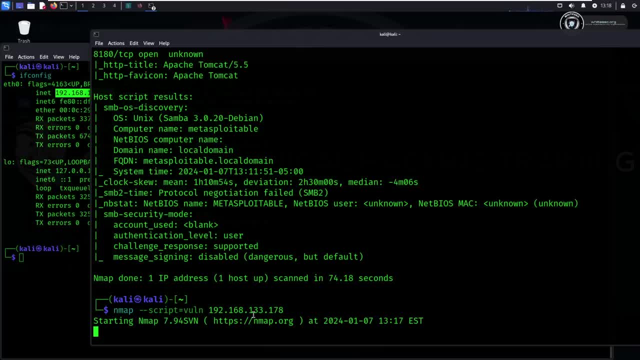 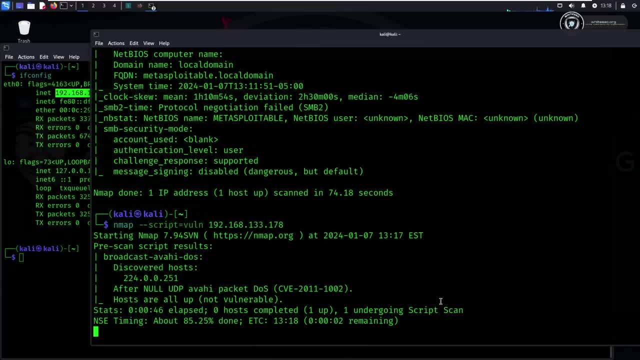 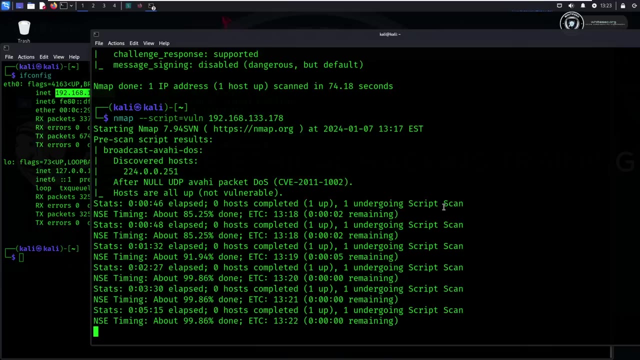 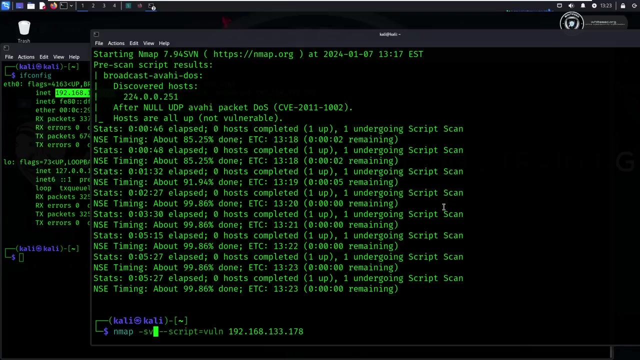 we need to add service version detections uh flag there. just wait, okay, so it's taking a huge time here. let me do one thing simple: if you want to execute this script, then just add service version detection here. basically it will. by adding this flag, what will happen means it can able to detect the services. 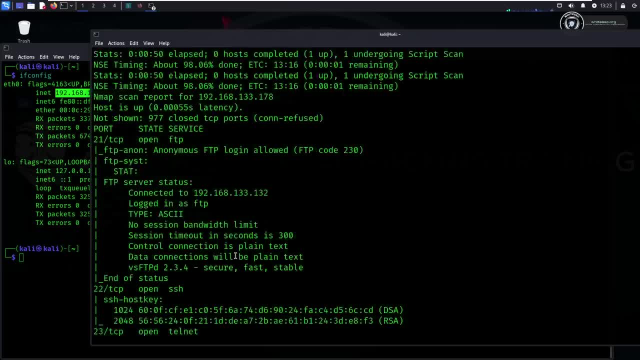 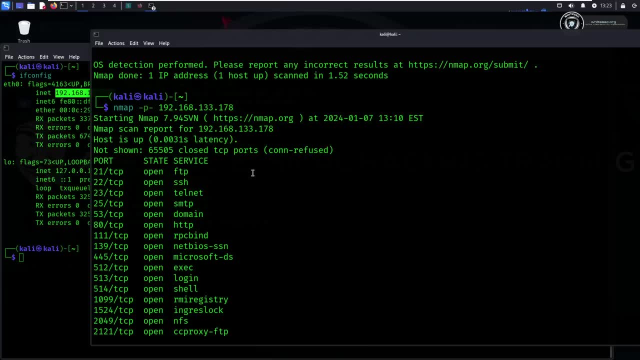 which running here. see these are the services: raise right. by using dash capital b flag, it can also tell the versions of these services. okay, it's which is known as banner grabbing. okay, so by using these versions we can able to fix these features which are available for this platform. you can also do that. you can mandatorylly see that if you need any support, then the service denotations feature will help. 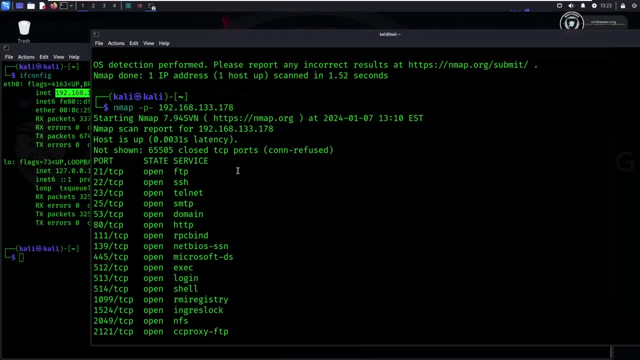 to figure out that which exploit we need to use. assume that some services are outdated. okay, assume that this service is using a out, uh, outdated, uh, sorry, outdated- version. at that time, simple, i can able to search that version. i can able to find exploits for the for that. 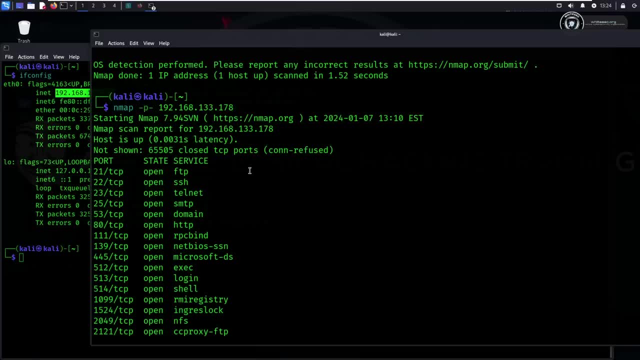 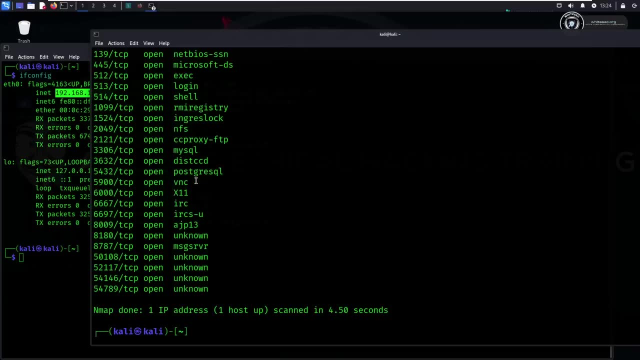 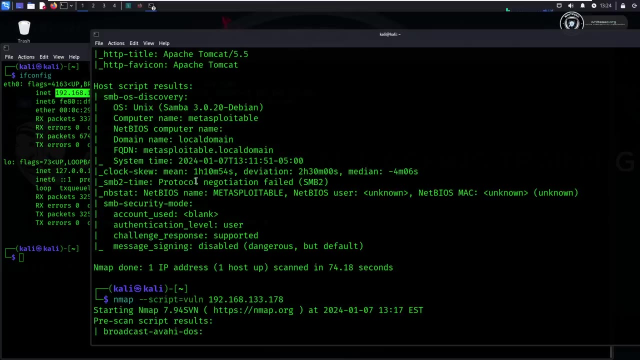 version. okay, by using that exploit, i can able to hack it. okay, this is the thing, simple things. you no need to worry about this force because, uh, we, we created a complete running on it, okay, which is on this channel. just try to watch it. so this is the thing. now, if i execute this command, then 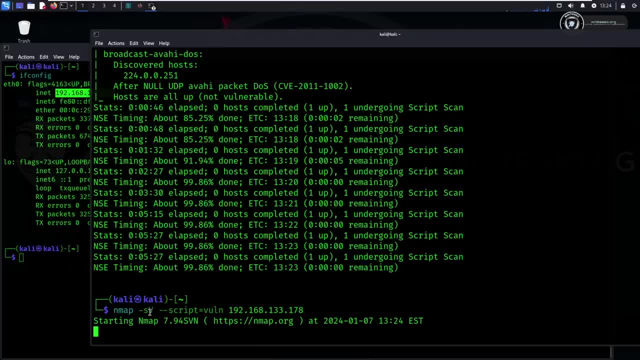 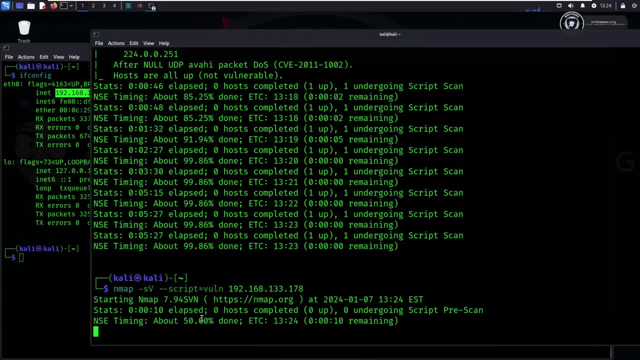 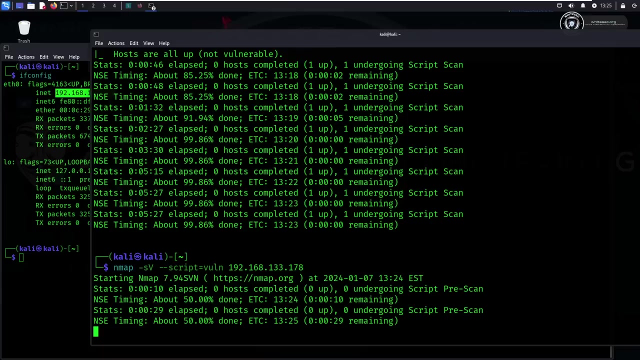 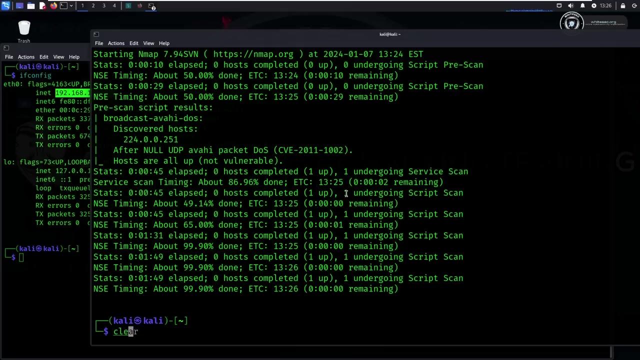 what will happen. let me tell you, you can also add a verbose mode there by just adding dash v, but i didn't added that. one don't worry, in the next classes we will cover about this thing. it will take a huge time, right? so this is the thing, guys. in the next class you will learn. 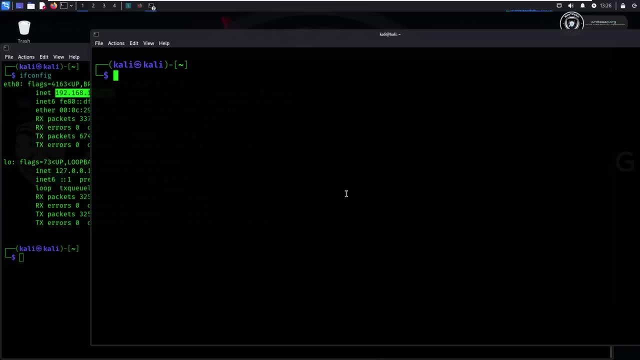 about zenmap as well. see, zenmap is also same same, it's a nmap, but in graphical user interface. all right, so let me cover that one as well. hello guys, hope you are fine in this class we are learning about this thing. okay, so let me cover that one as well. hello guys, hope you are fine in this class we are learning about. 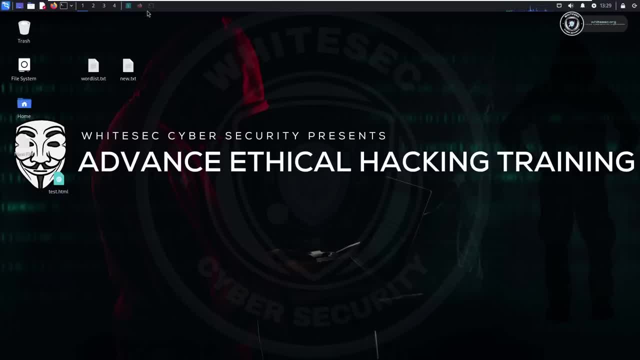 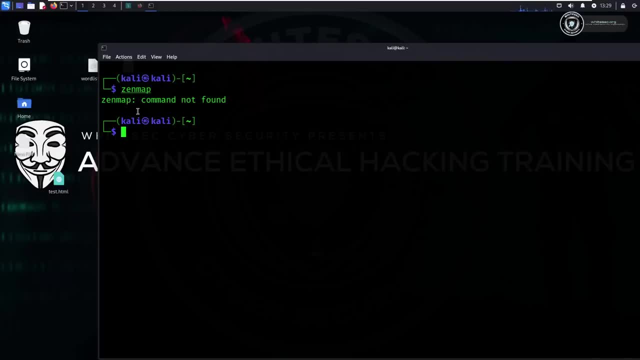 zenmap. first of all, you need to download the zenmap. if you open the terminal and if you search type here: zenmap, then you can't able to see it here. okay, because you need to download it. to download it first of all. the thing is, what you need to do is you just need to install. 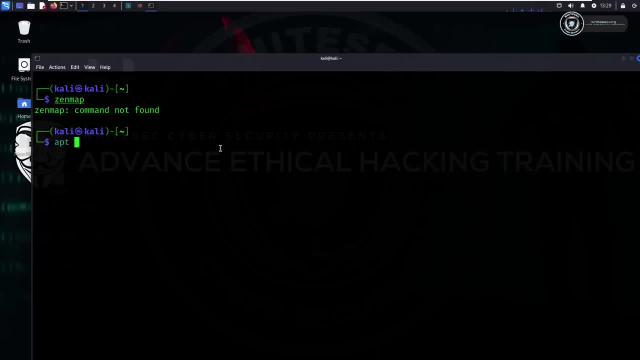 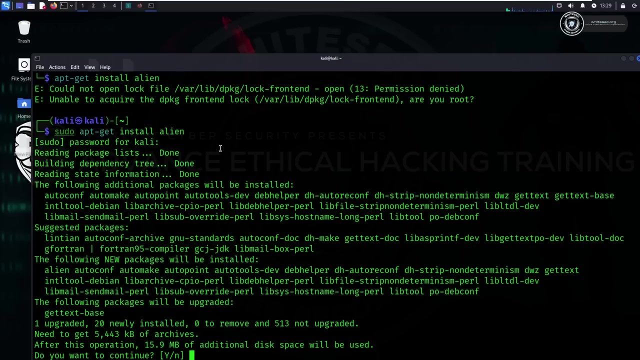 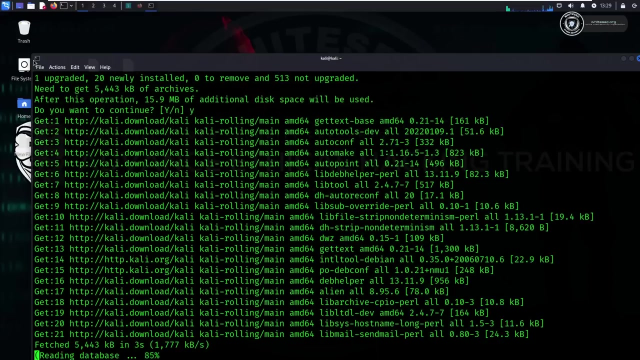 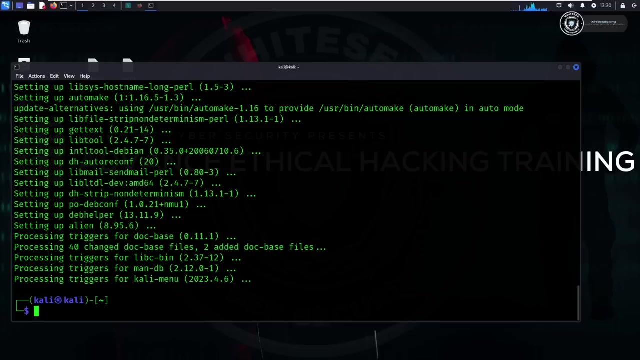 this package: apt: get install. just type this one. just use alien. just type enter. simple, just type sudo and execute it. okay, just type y there. now it successfully installed. right, just wait now. simple the thing is just visit this url. nmaporg forward slash zenmap from. 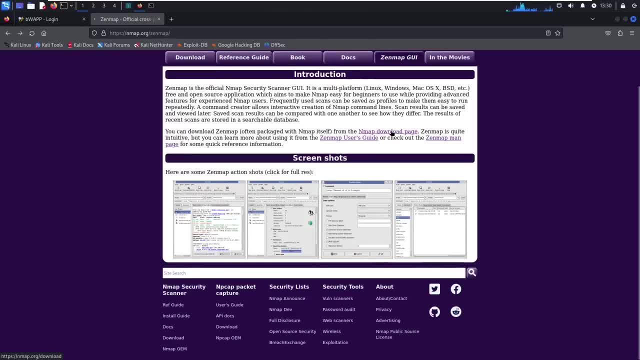 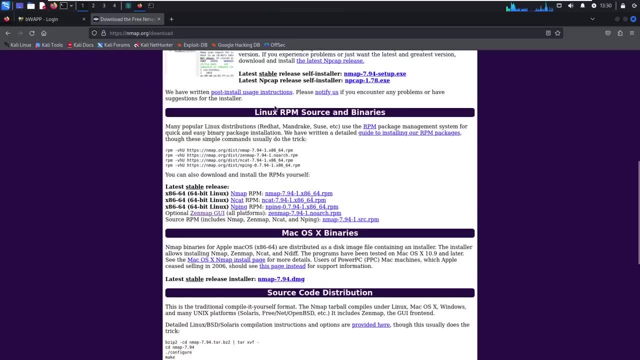 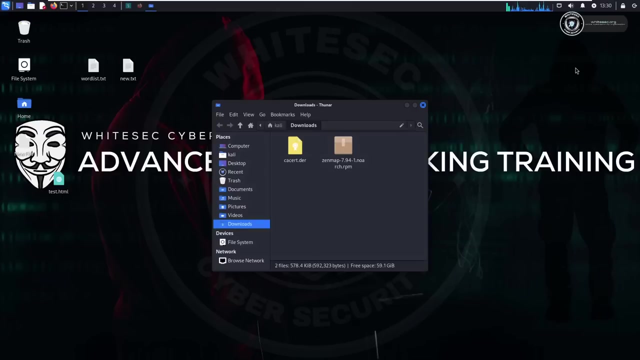 here. just click on nmap download page, just go down. there is a linux rpm source and binaries- this one- and here you can able to see zenmap. okay, the extension is what rpm? simple download it. okay, it successfully downloaded it. here it is right now. simple thing is: just let me open terminal from: 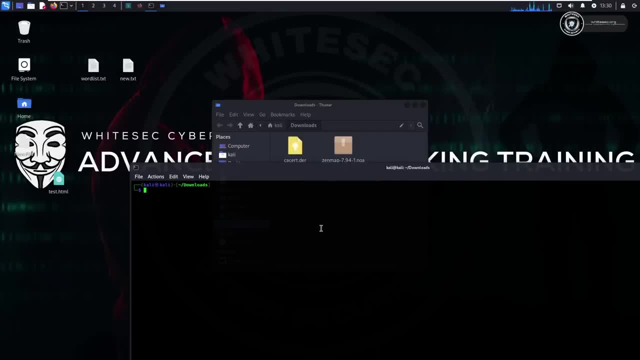 this folder. let me zoom it. just type here alien right and just type zenmap. just type enter here you must need to run as a root. just type here, because we need to convert it to deb. this is a thing. just type enter and it's successfully converted this way. okay, here it is okay, it's. 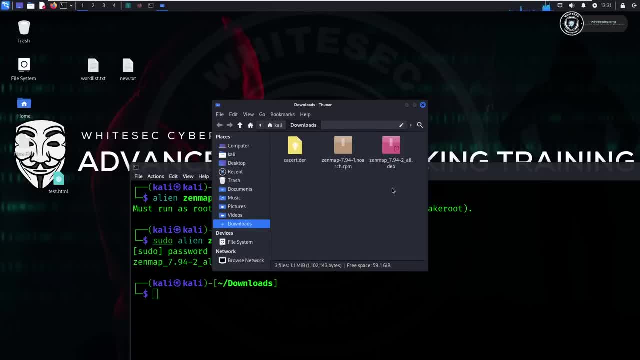 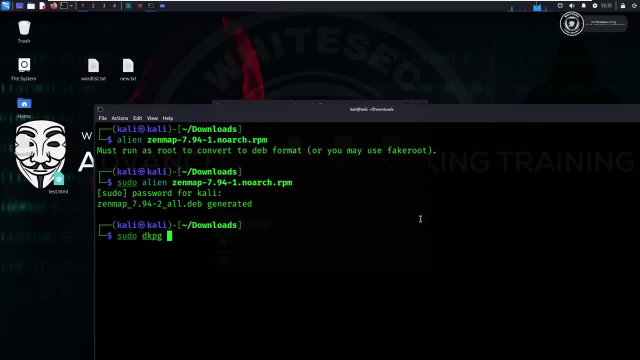 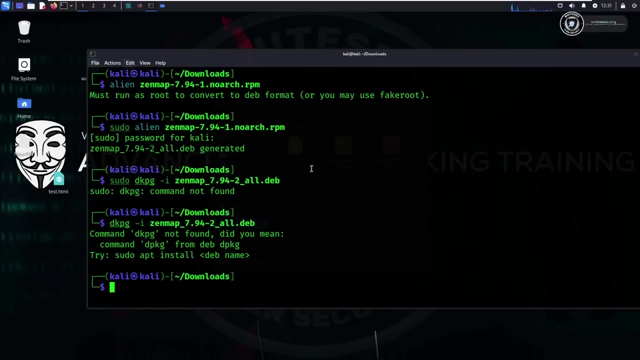 successfully converted. right now, what you need to do just type here: sudo, dkpg, dash i. what is the name there? zenmap. okay, deb, just select this one. just type enter there: sorry. okay, i need to install the sorry man, spelling is wrong there: dpkg. this is a thing with linux, it's a case sensitive. right here it is. 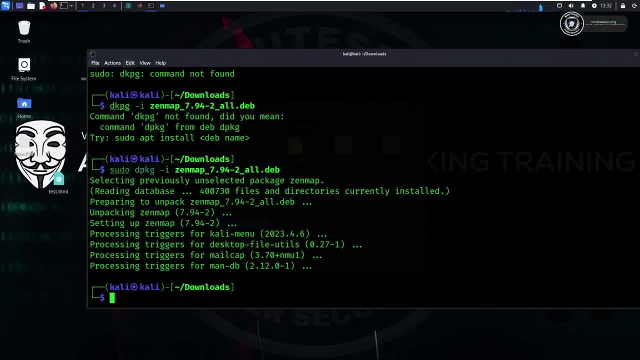 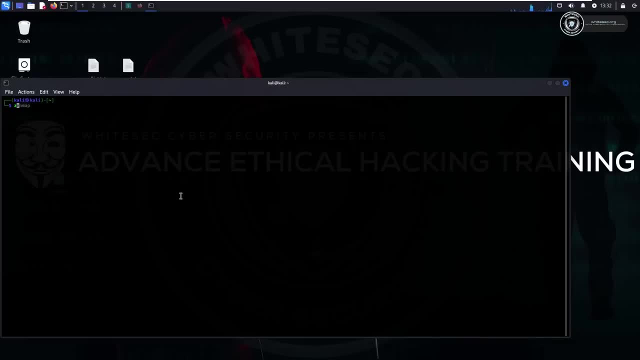 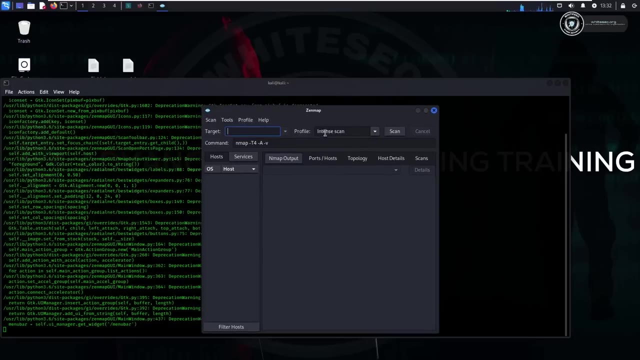 now simple, let me close it. it will be successfully. install the genmap here. simple: open terminal and just type here genmap. here you can able to see the genmap. i need to open it as a sudo user. if you are not opening as a sudo user, also it will. 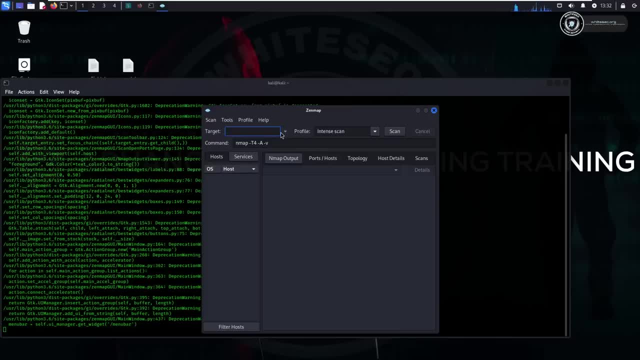 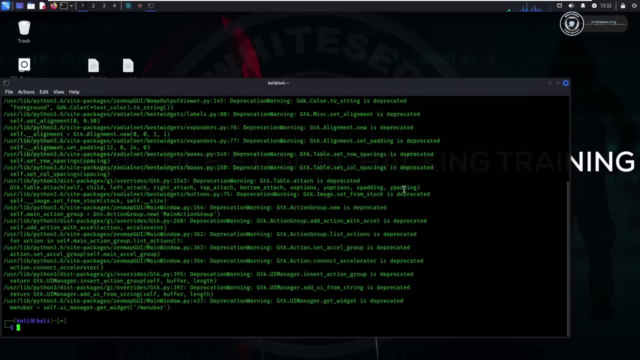 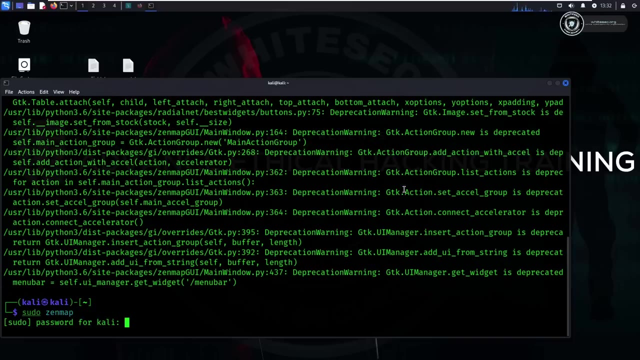 you can able to see it, but you can't able to perform os detection here. so the simple thing is just run it as a sudo. just let me zoom it and let me type here: sudo genmap, right, and just type kali there and here. it is so simple. here you need to paste your target ip and there is a profile. 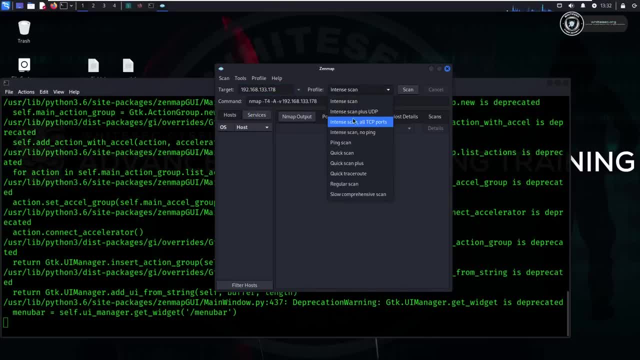 there is a intense scan plus: udp quick scan is here, ping scan is scan scan. scan scan is here like regular scan is here, right, and there is a services here. you need to type the commands which we just type there, such as nmap, dash s, capital V, something like that. 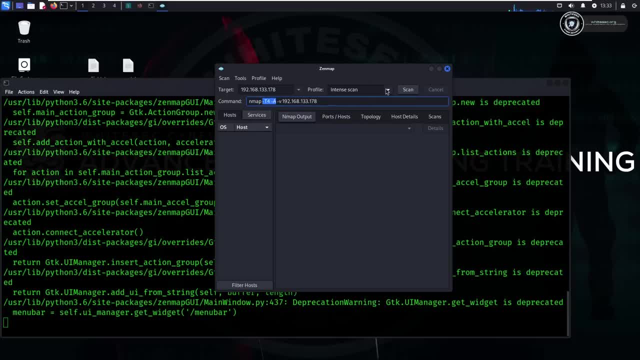 right. So let me perform the quick scan, right. this is the quick scan, ok, which is t4, t4 is nothing, but if you are using t4 or t5, then the scan will be very fast. so don't do this, don't use. 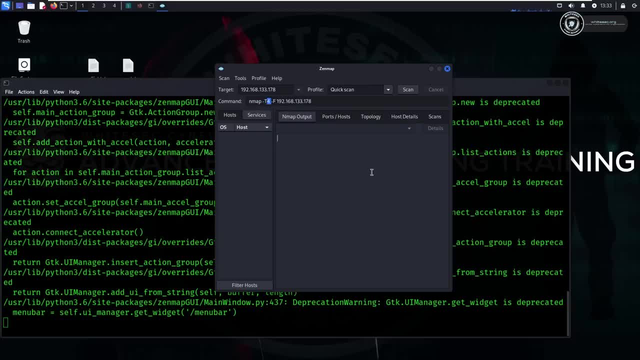 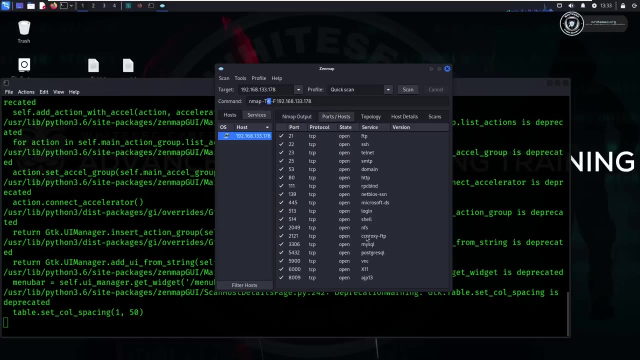 this t4 or t5 in real world scenarios? ok, because it will generate a huge noise there. so simple, just scan it. see. here is a details. if you go to the ports here, you can able to see in a very clear: topology is here and there is a host details. 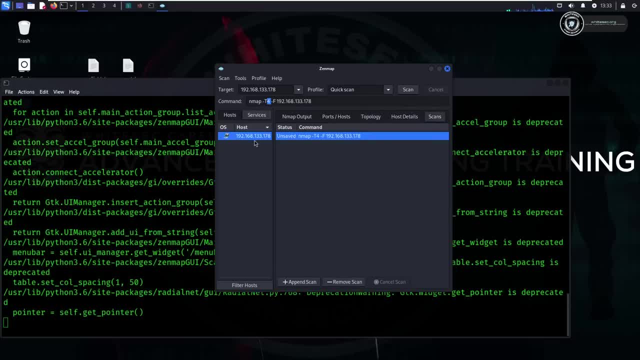 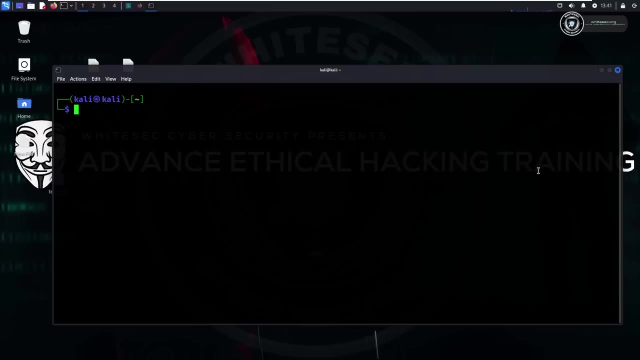 And there is a scan right. this is how you can able to use zenmap in graphical user interface. hope you guys get it right. thank you, have a nice day. hello guys, hope you are fine. in this class we are learning about necto. see, by using necto, what will happen means you. 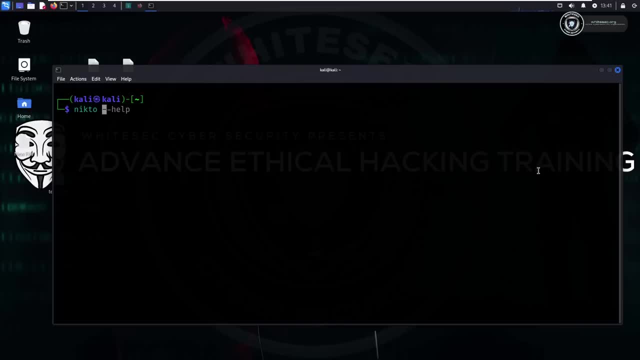 guys can able to find a lot of juicy information about your target, assume that it is vulnerable, within any vulnerability or by any means. So let me show you how to use necto. Using necto, mostly, you guys can able to see directory listing or assume that if your target 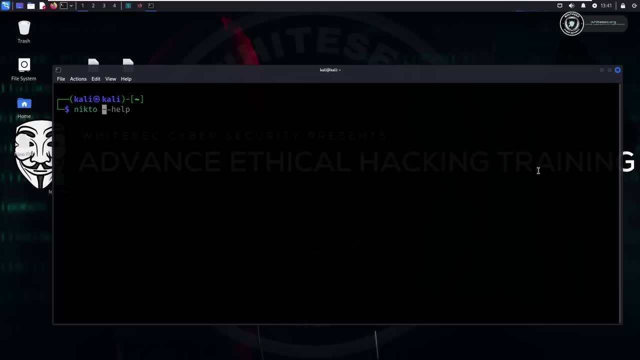 is using get or delete put request, then you can able to see it here. ok, this is the thing. assume that your target is accepting put request there. simply, you can able to upload shell there. this is the thing. ok, so let me show you simple. just type here: necto space dash. 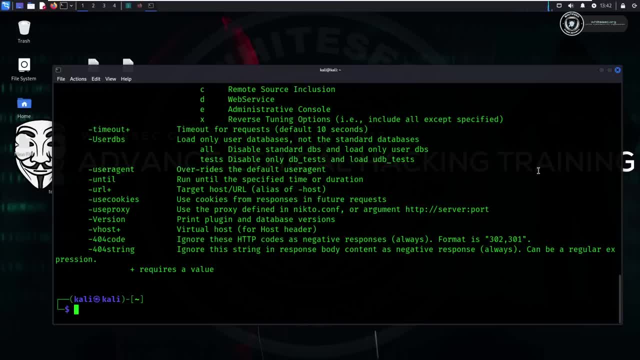 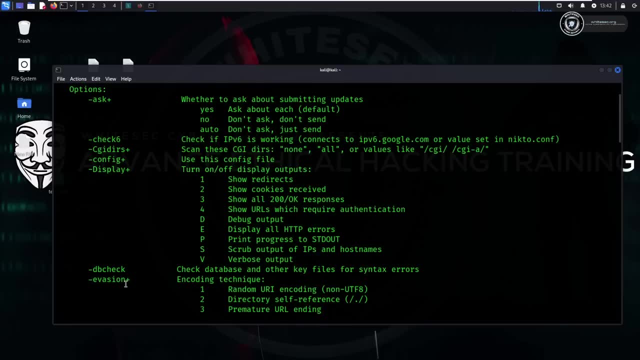 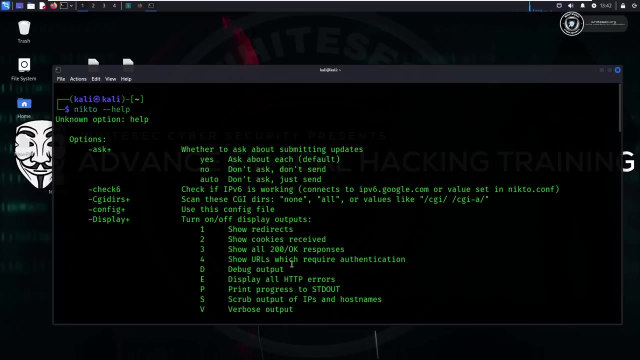 dash help. here you can able to see a lot of options as well. The cool thing about necto is there is a evasion techniques as well. right, you can able to use a fake parameter, change the case of the urls, such kind of stuffs, but the thing is, let's. 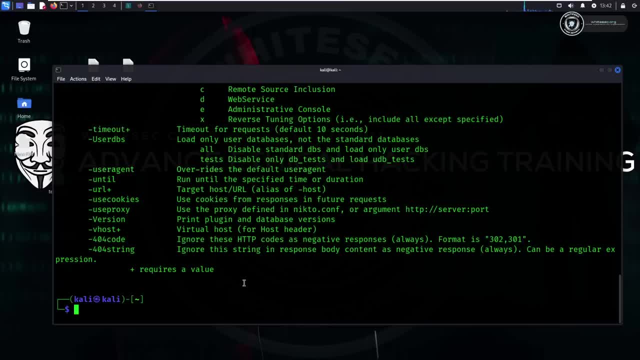 learn. run this necto. ok, simple how to run it. simple: just type here: necto, dash h. this is for host. here you can also type the url. you can also paste the url or just paste the ip address as well. ok, url means not complete url. you need to paste the domain there. ok, this is the thing. ok, let 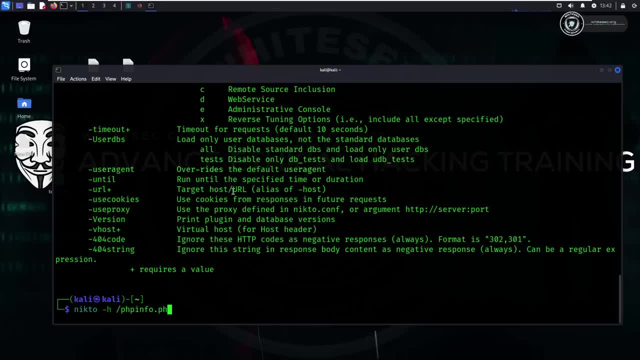 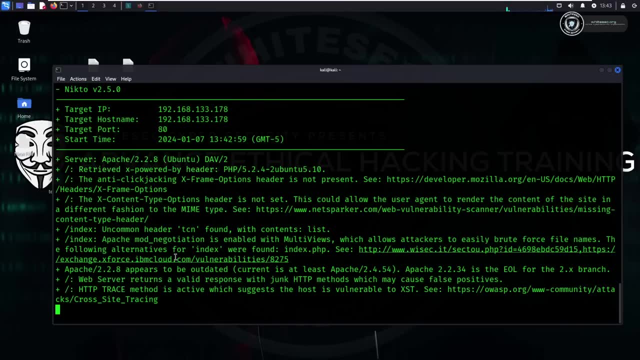 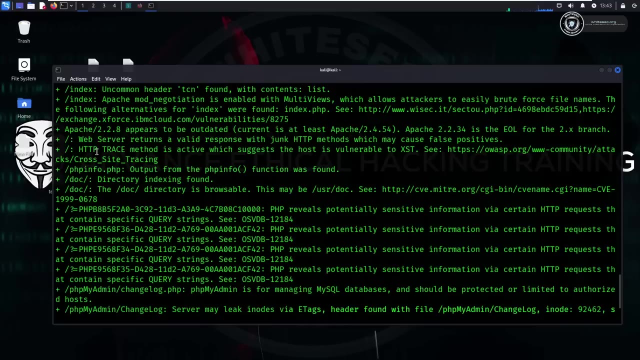 me paste the ip address here So it will show you a lot of juicy informations. see, here I can able to see directory some directories here, such as phpinfocom, php doc and there is a php rebuild potential sensitive information via certain http request. now here there is also a the links by. by using this, you guys can able to read about that. 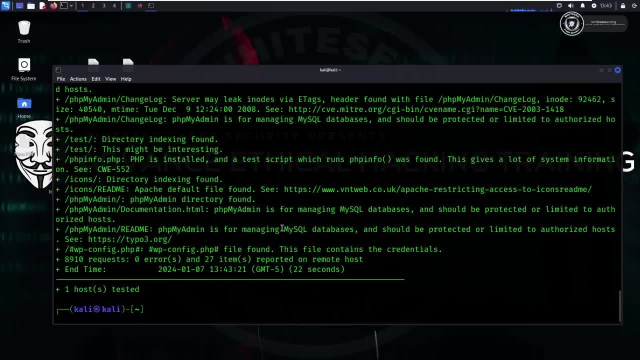 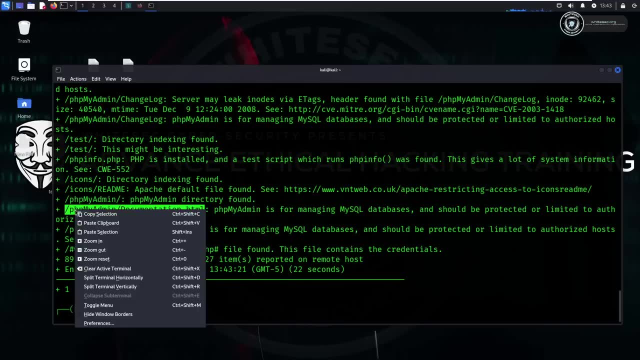 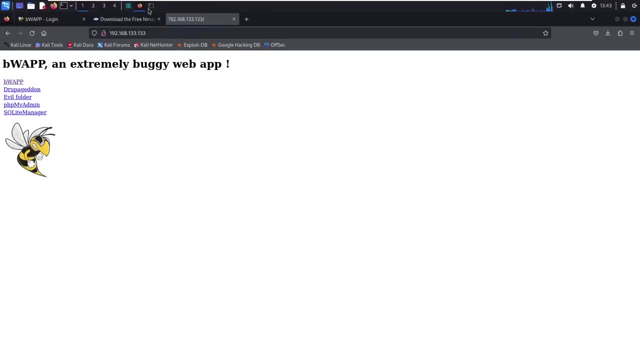 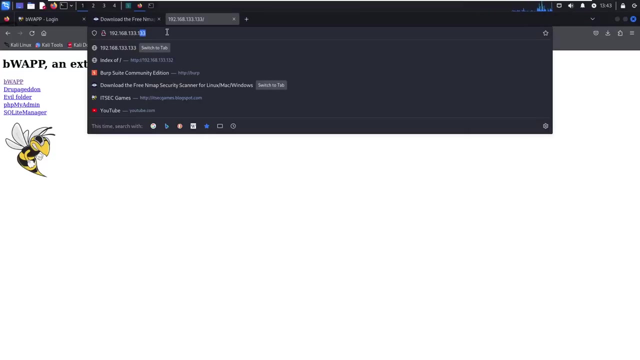 vulnerability. ok, So you can able to see a lot of things here. see, let me copy this path and let me open the browser. So what is the ip address of my target? it's 133, 178, right forward slash, and let me paste. 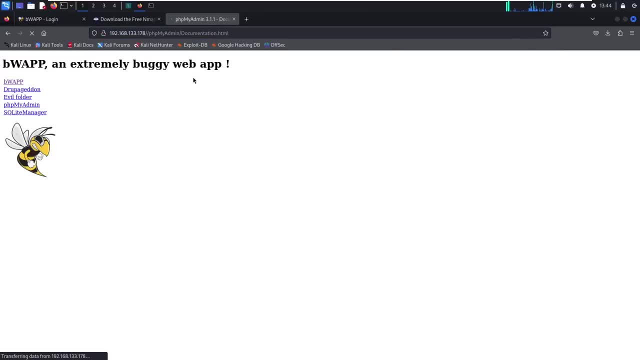 that path here, but type enter: here you guys can able to see the, the documentation of phpmyadmin and here, phpmyadmin page. there is a lot you need to analyze here. So let's see here. So let's see here. So let's see here. 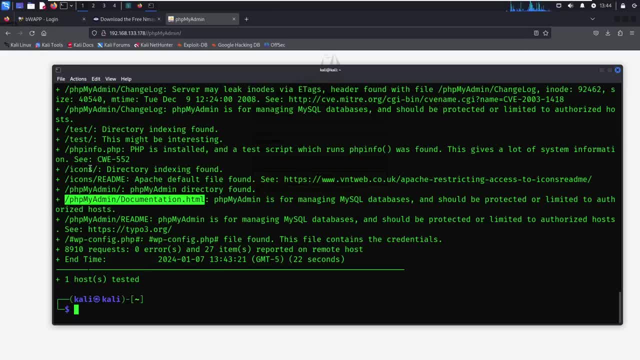 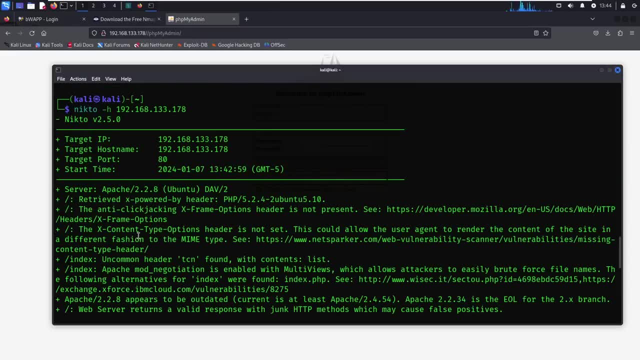 Let's see here. So let's see here. here is the interface, then. let me do this just a bit to analyze it. It will come. mostly It is useful to see the directory listing. ok, If I like. basically it is useful to find the juicy information about your target. sometimes 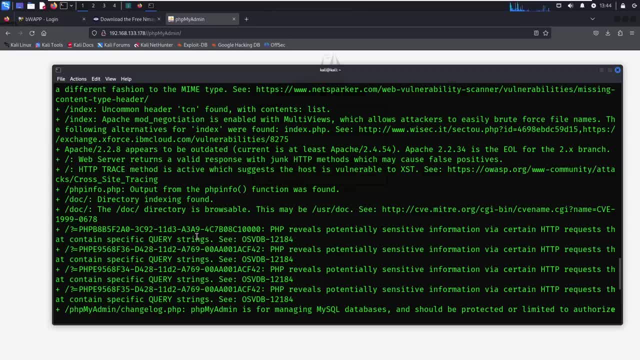 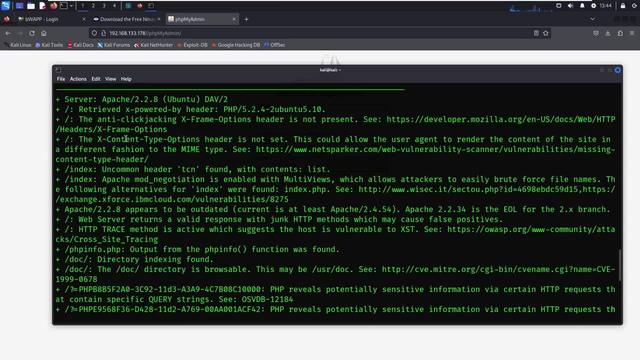 it will give you a lot of things. are results, are results. ok, such has just told you, right, such has you. by using by, after by scanning, using this nicko, you guys can able to see the request as well. like run. So let's see here. 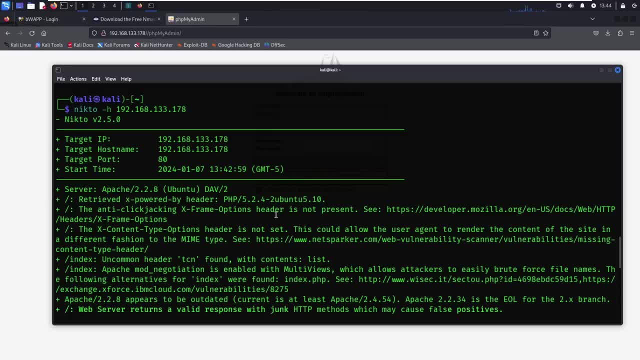 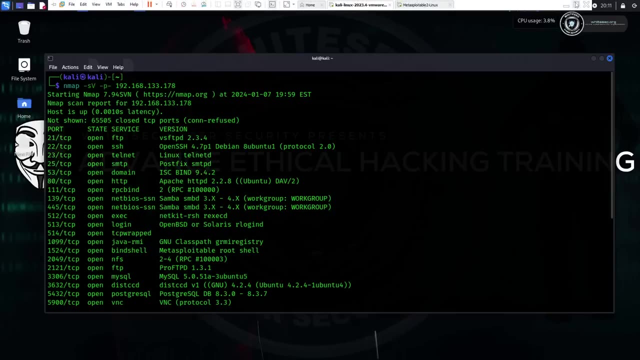 as well, like the. if it's using uh put request, then what will happen? we can able to uh upload the shell there. okay, in the server. this is the thing. hello guys, hope you are fine. in this class, we are learning how we can able to exploit this- open ports. right now. the thing is, we in in this. 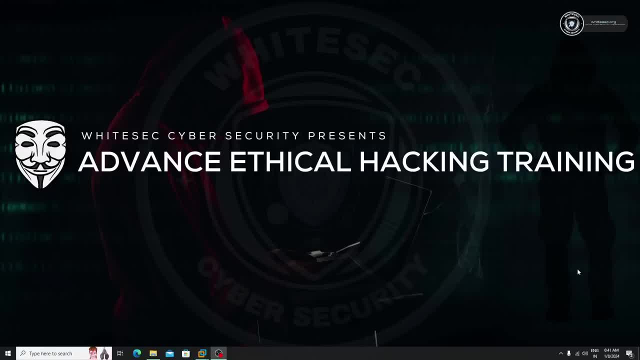 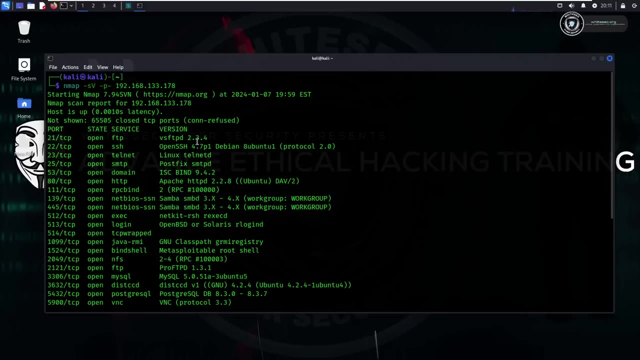 youtube channel you can also see a complete course on how we can uh open ports. hacking, right simple. just try to watch it, because there we just covered a complete uh topics okay, like how we can able to exploit ftp, de open, ssh, linux, telnet. okay, post fix smtb. 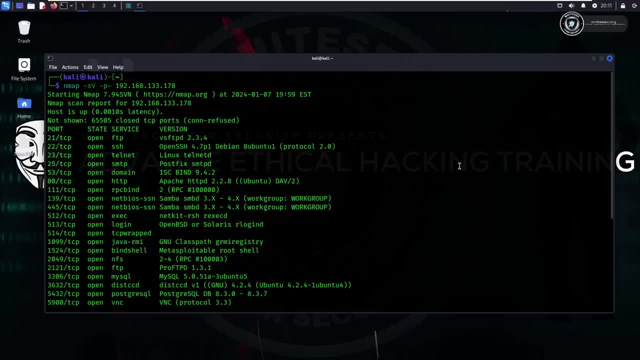 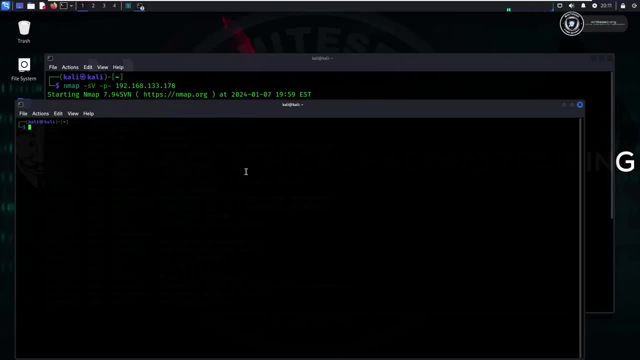 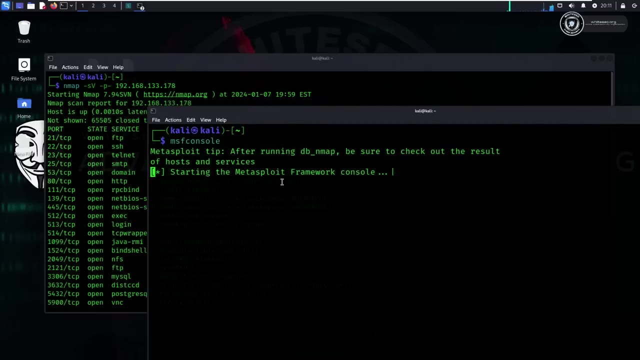 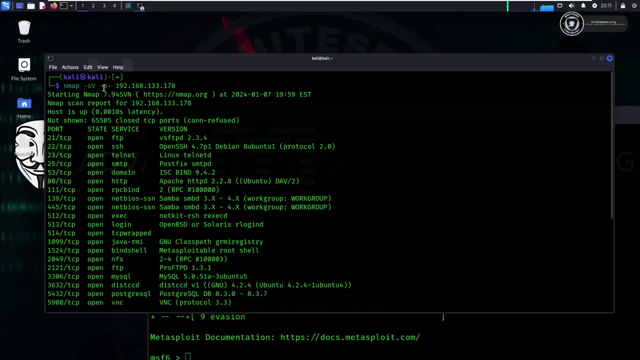 smtpd. so we just covered each and everything. just try to watch it after completing this course. now, here the thing is. let me exploit it. now, here we are using msf console. see simple. uh, we just executed this command, which is nmap, dash s capital v, dash p dash and the ip address. what is this dash s capital v? it's a service version. 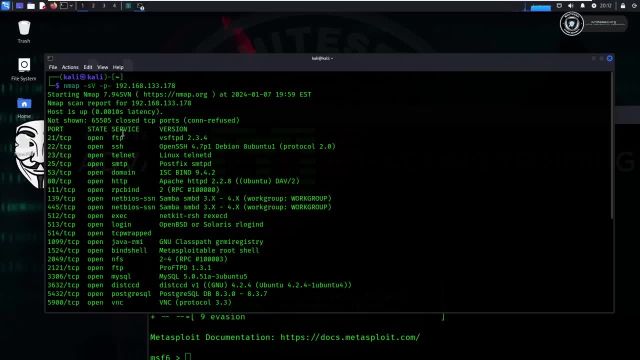 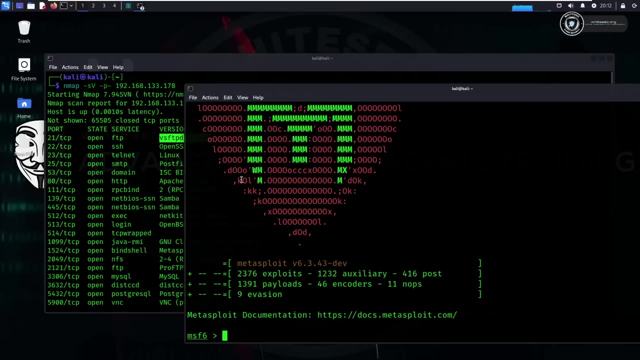 detection here. the thing is, service is ftp and the version is what? here v s f tbd 2.3.4. basically, i need to search this version in metasploit, okay. so, uh, if i see any kind of exploit, then i can able to use it and i can able to hack this system, this one, metasploitable. 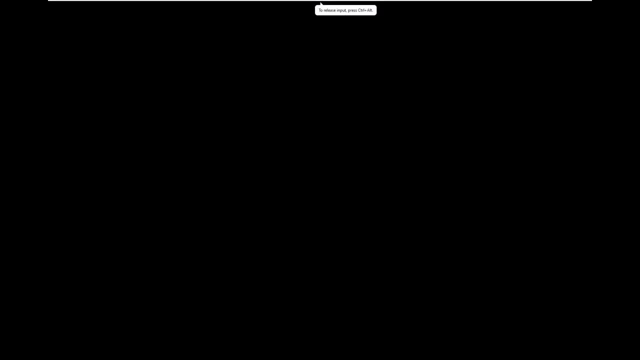 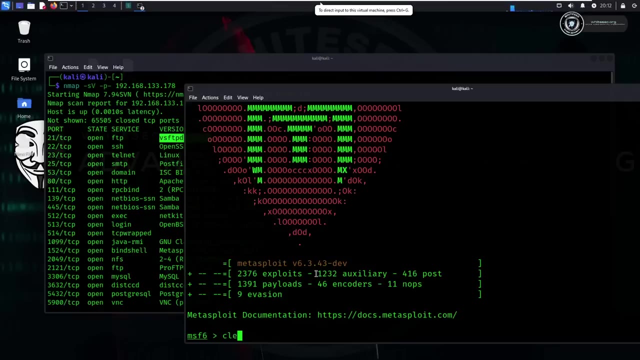 to machine, right? see, let me tell you, metasploitable is different, metasploit is just different. okay, metasploit is nothing, but this is a tool. by using this, we can able to generate the payload, we can able to listen for the connection, we can, uh, exploit the vulnerabilities. 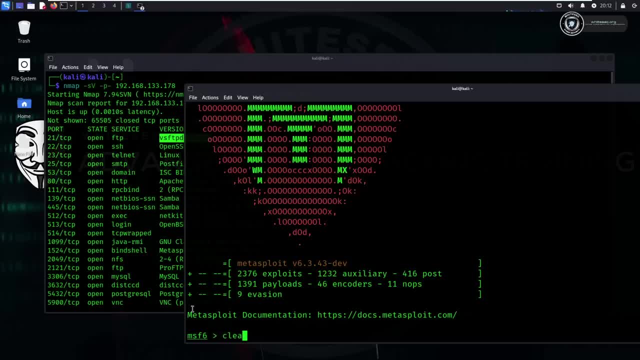 right, so it is a metasploit. now, this is what this is: a metasploitable machine, right? which is use, uh, like, if you want to hack any like, metasploitable is what here? it's a vulnerable machine, right? let me clear it. now, let me search. there is a, there is a feature. by using search, you can able to. 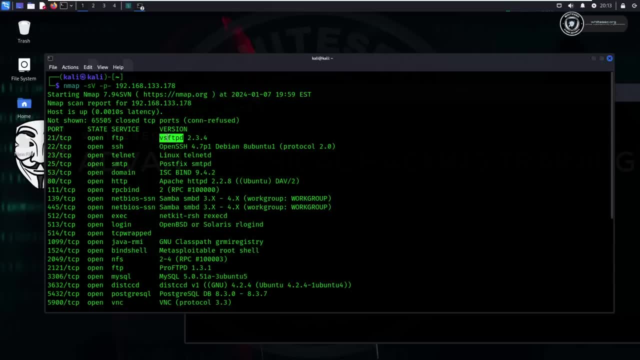 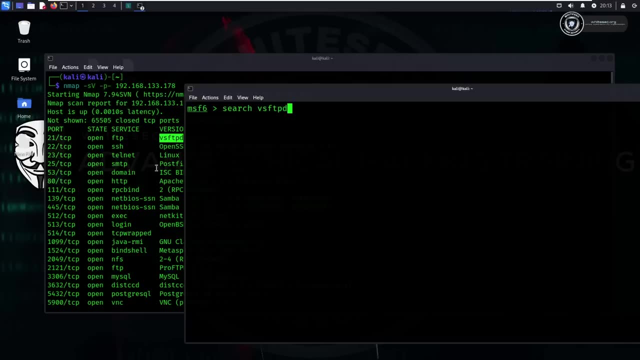 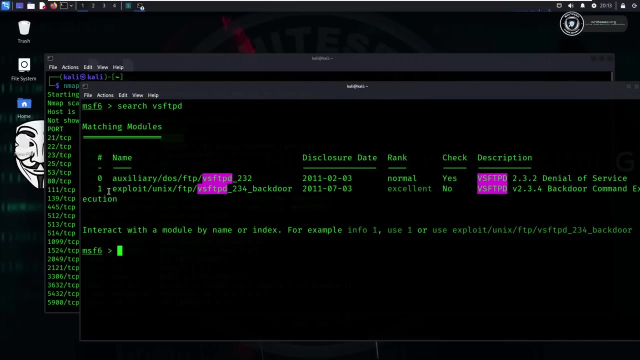 uh, sorry guys, let me search exploit for this version. you can also type the service name as well. now, here there is a exploit. auxiliary is nothing, but it's kind of scanning. it will scan for the vulnerability. right now, here there is a uh exploit is there? let me use this one. simple, just type here, use now. there you can also choose. 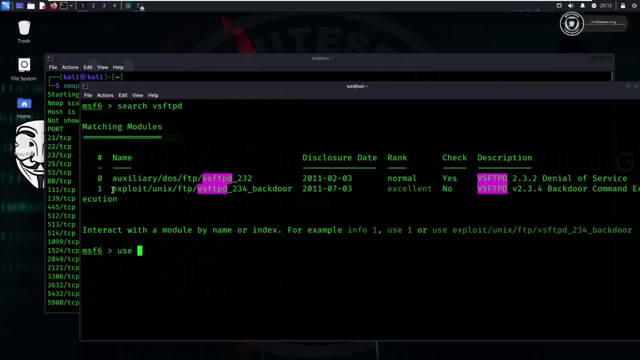 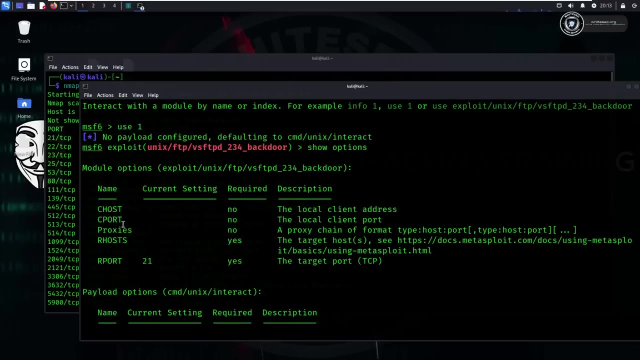 a number there, or you can simple copy the complete name and you can paste it. okay, let me choose a number here, use one now. simple, just type here: show options. now you no need to set the c host, c port, some thing like that. now the thing is here. let me, uh, choose our host. our host is nothing, but what here? 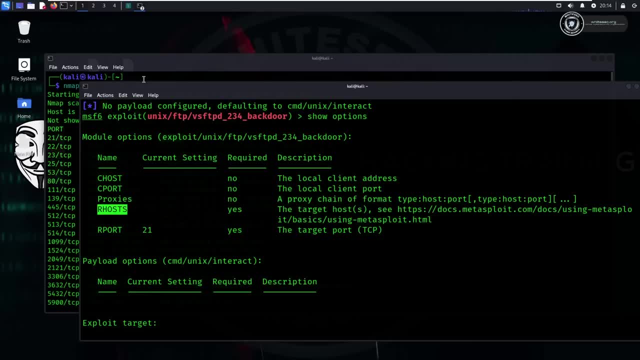 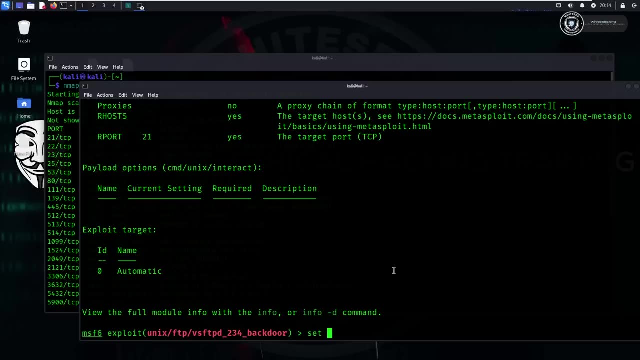 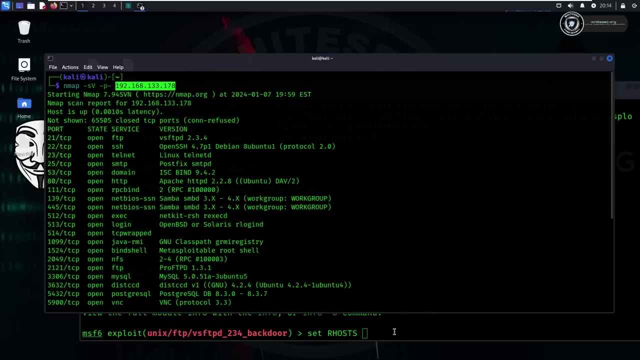 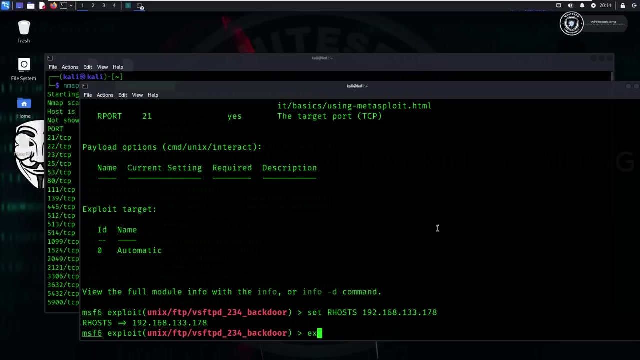 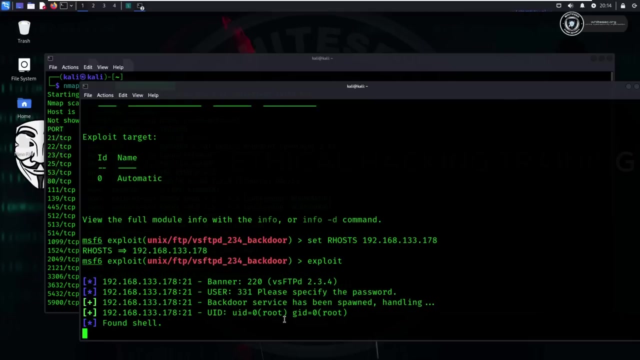 the target host. target host means your uh target ip address. this is the thing now simple. let me set it. just type here: set our host and your target ip. which is this now simple. let me exploit it. thank you, now here i got session found shell, right. if i type ls now i can able to list the 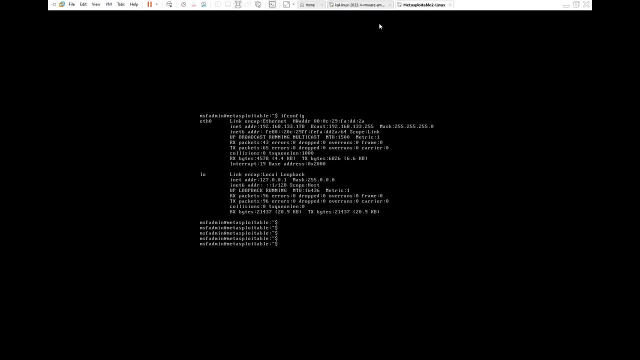 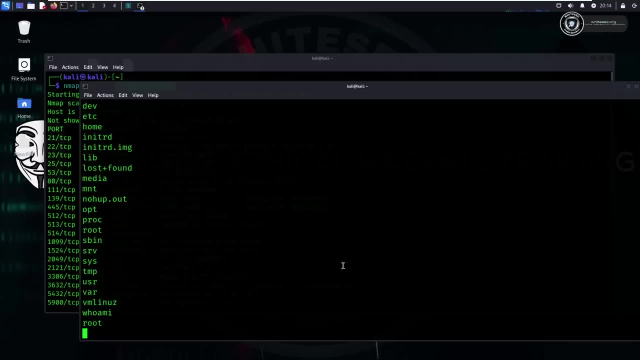 things here. okay, i successfully hacked this machine. this is a thing, right. and also just see, if i type who am i? i'm a root here. i can do anything. i can dump the password, i can see the shadow file. i can do a lot of things. that arenelle css. all right. the venrod ball is a. 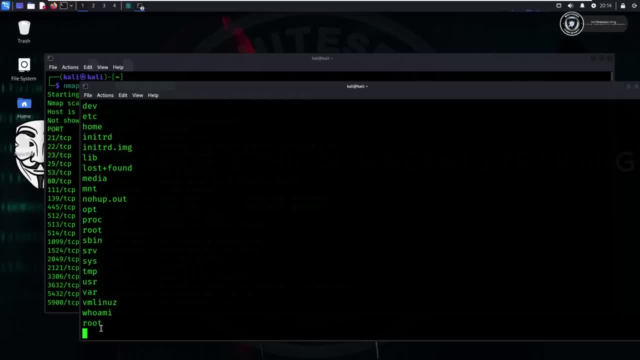 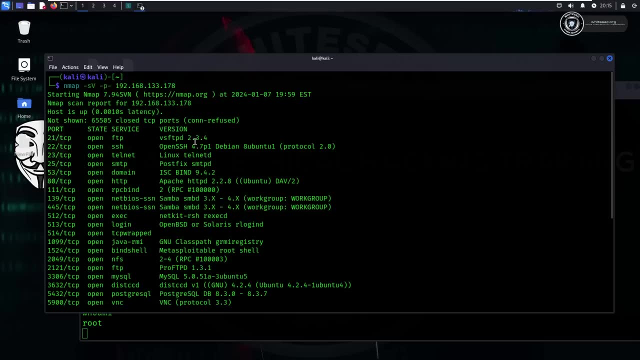 of stuffs. here I no need to perform privilege escalation as well. this is the thing, guys. basically this kind of vulnerabilities will find in internal network. ok, like mostly in internal network. so in the next class we will learn how we can able to exploit ssh. it is. 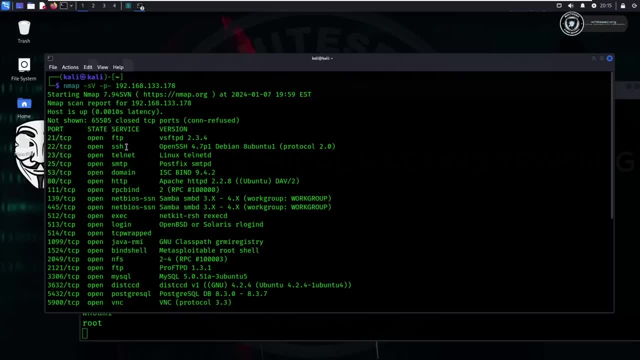 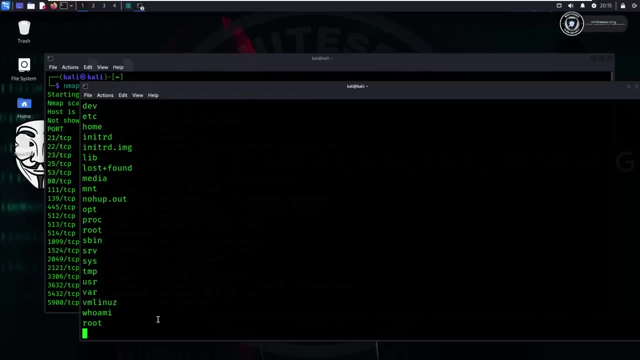 not a exploitation, it is a kind of brute force attack. ok, how to perform it, let me see in the let me cover in next class. ok, type here back and let me clear it now. in this class we are learning about, we can able to exploit ssh simple, the. 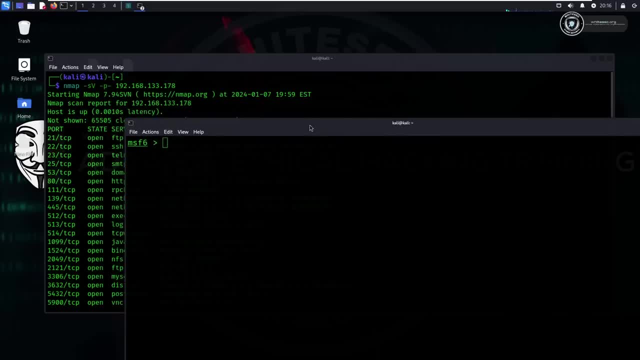 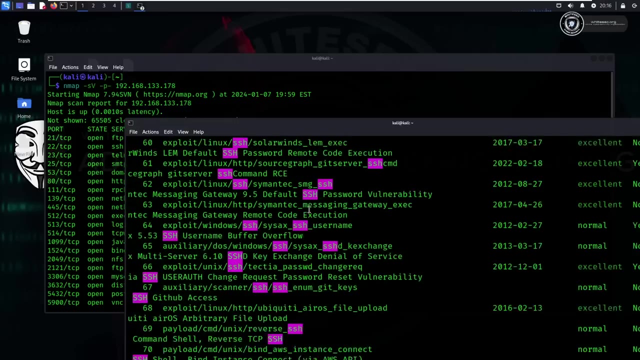 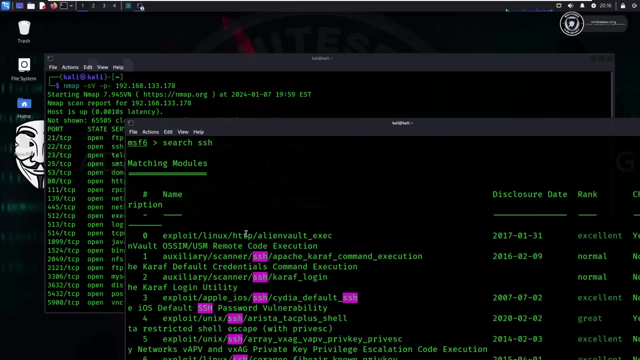 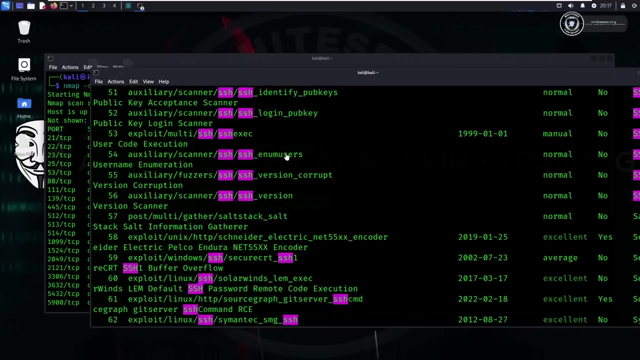 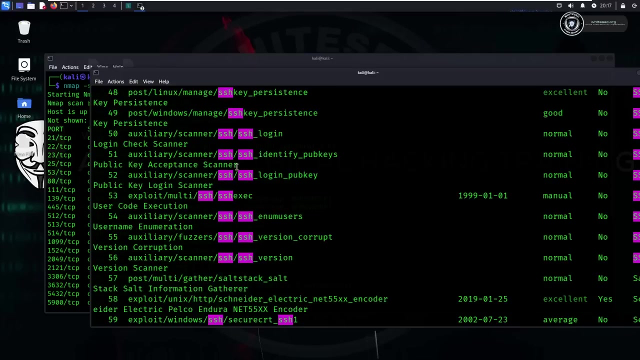 thing is the same thing. just a serves for this type search, simple search for the Ssh. here we can to see a lot of things. it is a fuzzer, just use. assume that if you want to perform username enumeration, you can also use this one. perform username enumeration. that is a ssh. login is here. 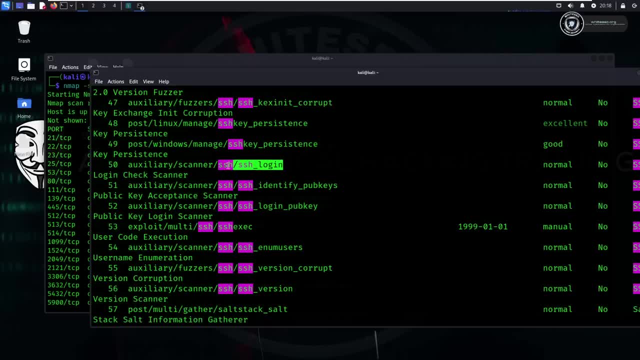 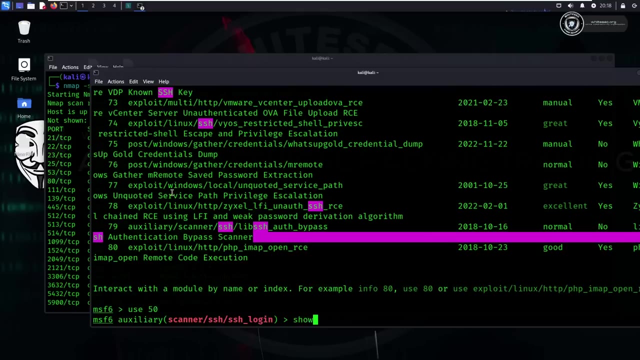 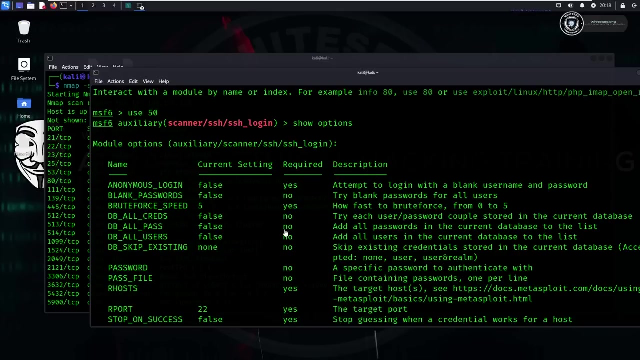 basically, by using this, you can able to perform brute force attack. now let me use it. number is what here? 50. let's type here: use 50. now just type show options. now here you need to set the rhost right. just try to watch that. open ports- open port hacking class. 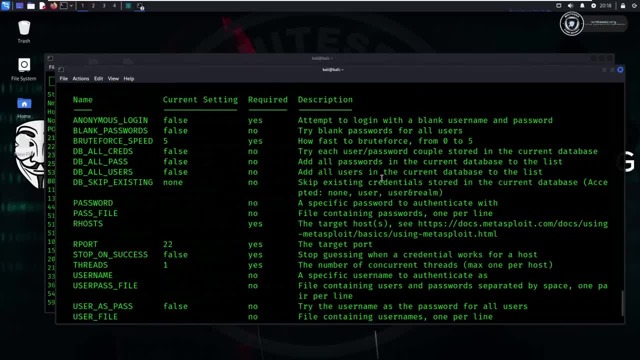 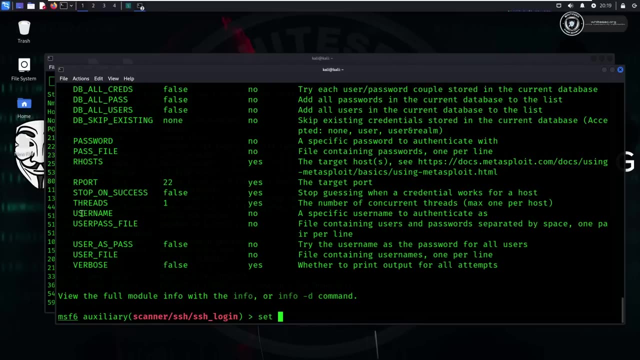 there, we just added a lot of things. okay, basically, i just covered each and everything about the modules: how we can able to use it, how we can able to exploit it right. the simple thing is: here, let's, let's go for basic things right now. here there is a rhost. rhost is what here? 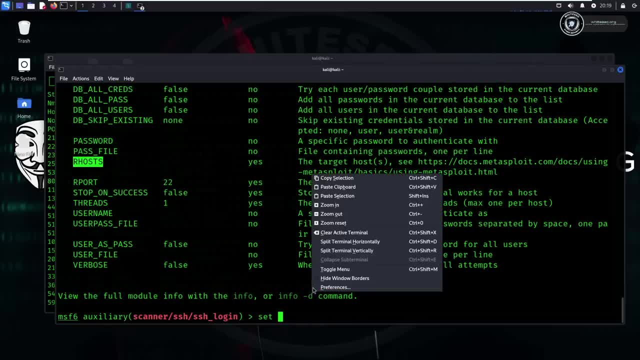 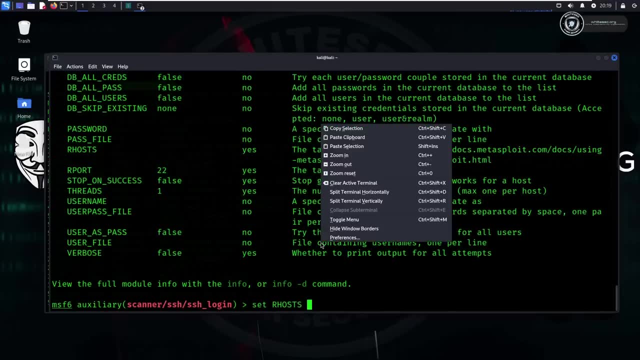 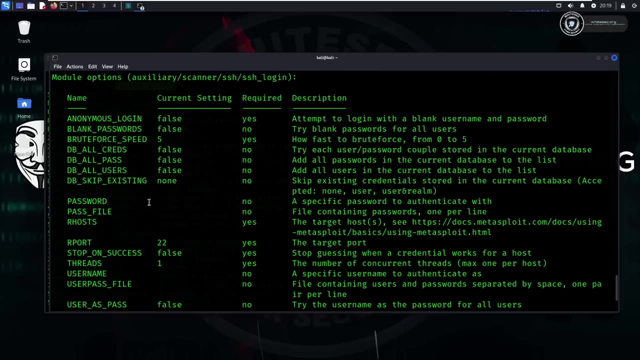 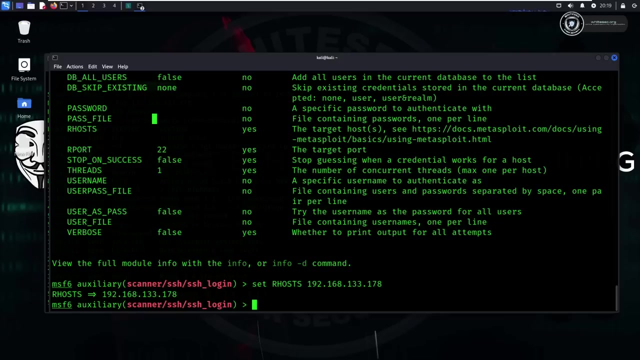 is nothing, but here we need to add our target ip. now you need to select the pass file and there is a. what is this pass file is here and there is a username file. if you want, if you have the username file, then you can add it here. let me see, is there? 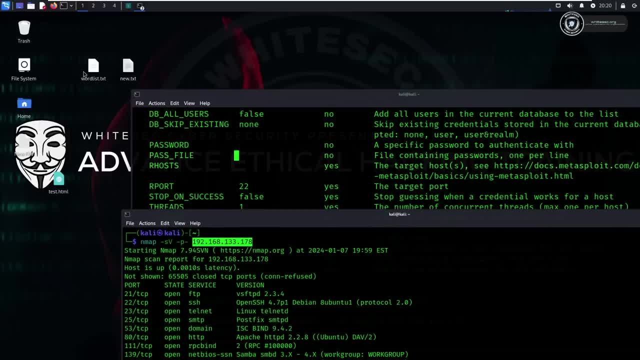 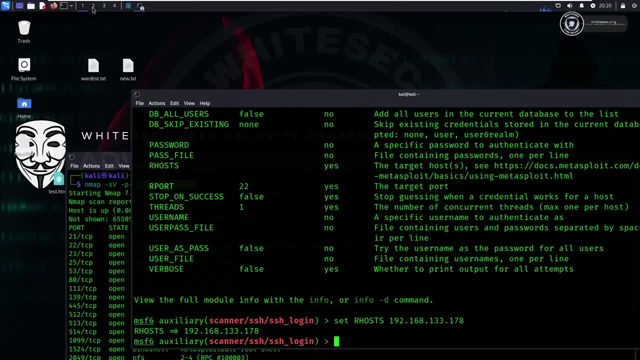 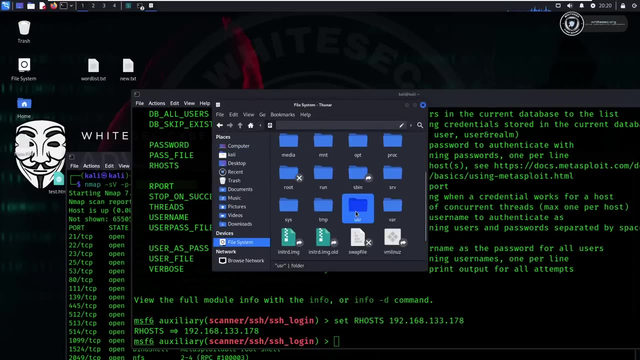 rock you dot pxc. there is a word list or pxc is here. let me use the rock you dot txt. simple, open folder and click on file system. there is a user, there is a share. here you can able to see the folder with the name of word list. 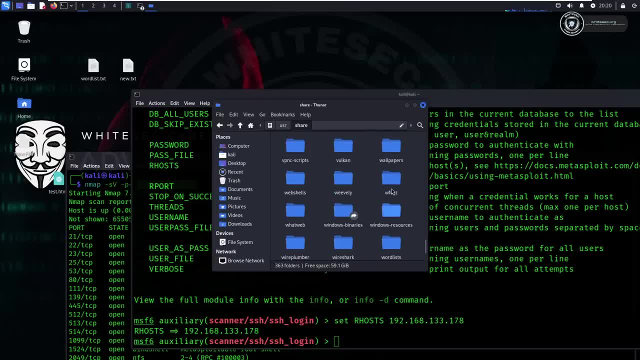 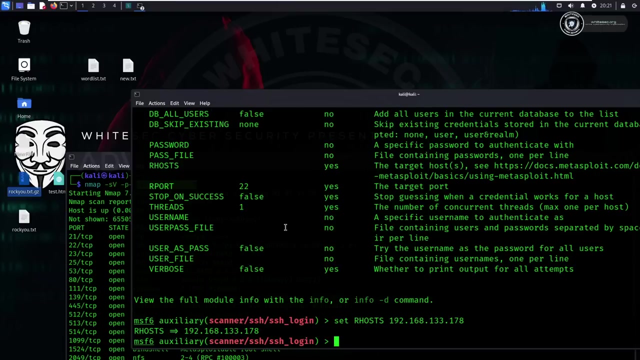 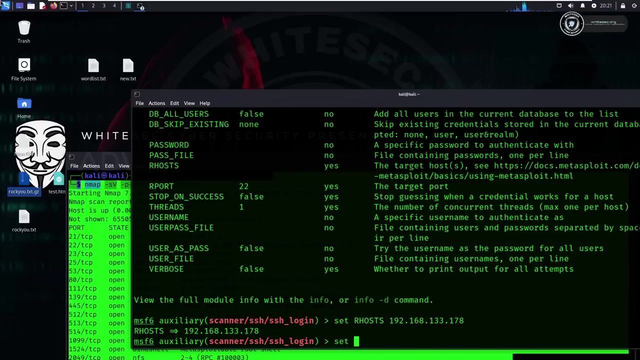 okay, here it is. now let me use this rock. you paste it here and let me extract it here. so here is rock you dot txt. now, simple. let me set the pass file here. file containing password, one per line, just type here: set pass underscore file, simply just paste it there. 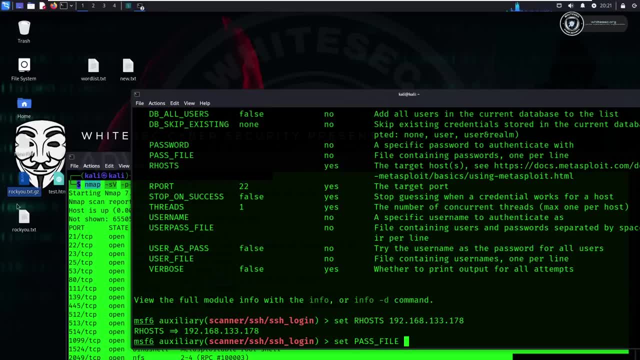 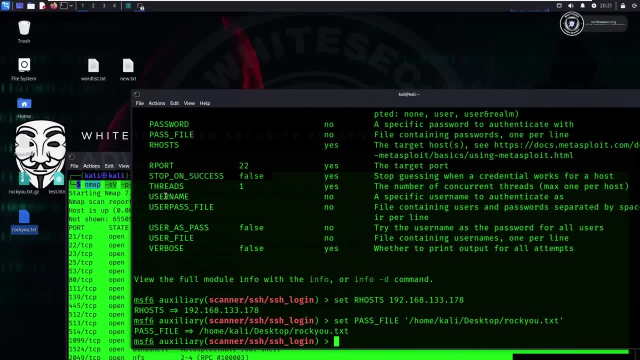 now, then what you need to do? simple: just drag and drop the file. okay, just type: enter. now the same thing: username also. let me do like that, like set user. there is a user pass and then you need to do the same thing here. let me do like that, like set user. 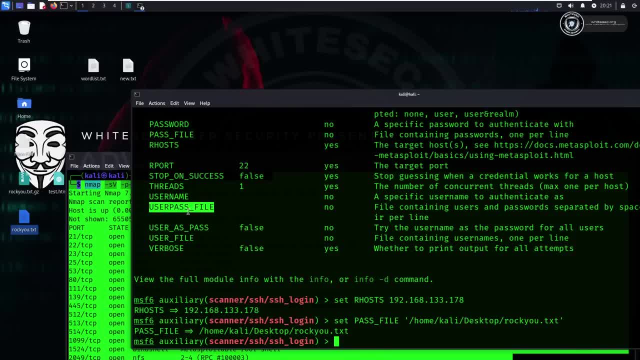 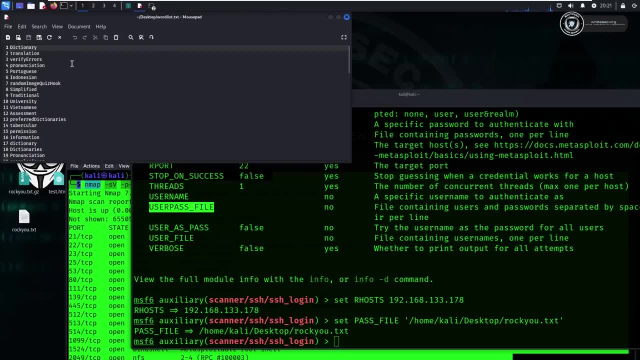 user pass is nothing but in one file it will contain the username and the password, like this. if i open, let me open the word list here like this: okay, like it will add the semicolon. then there is another keyword like this: so this is a kind of file which comes under use user pass file. 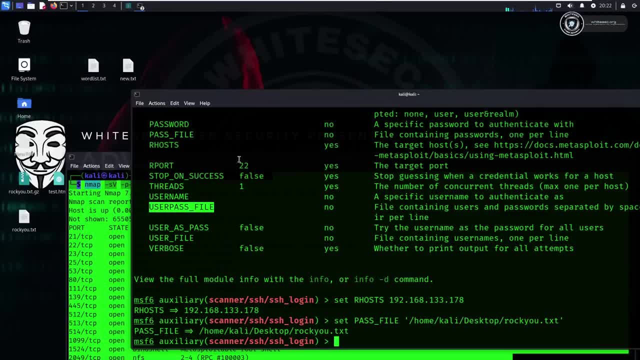 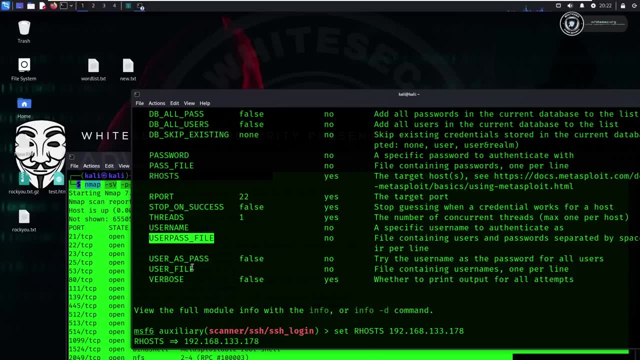 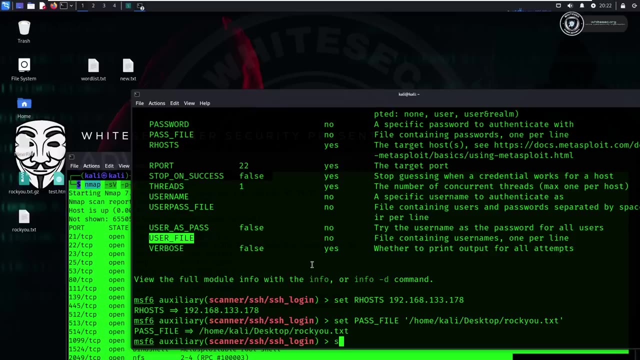 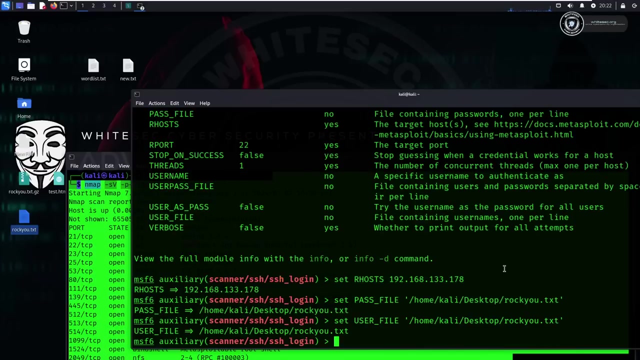 okay, so right now we don't have that. so simple the thing is, we will use user as pass. where it is sorry, user file. let me use this one set user file. let me use the same file here. just type enter and let me set the verbose to true. 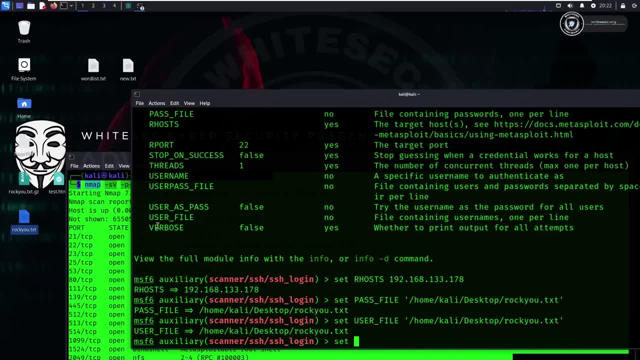 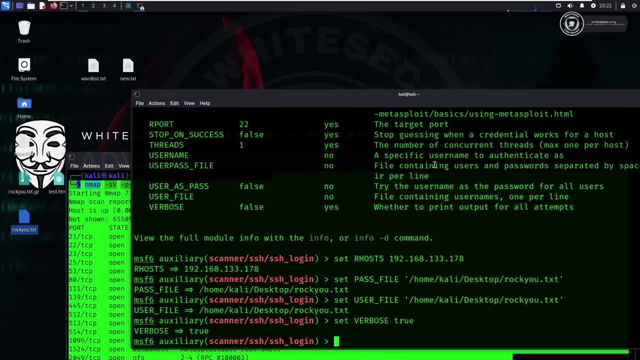 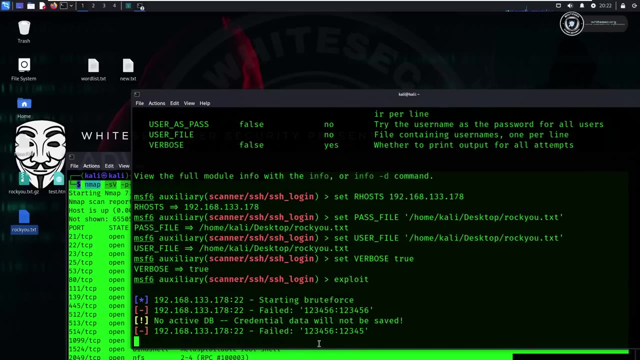 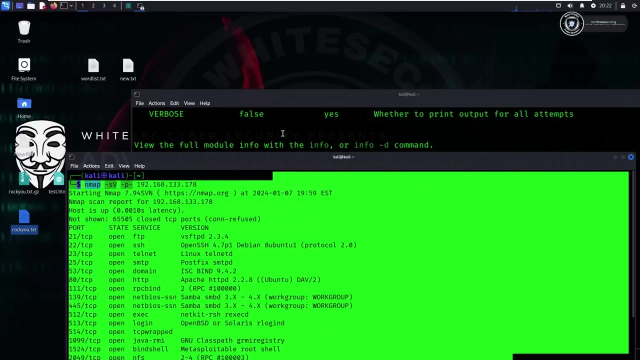 set so i can able to see the output there. paste it here and let me set it to true and let me exploit it. now see what will happen. it will start the brute force attack. so this is how you can able to perform brute force attack on ssh. 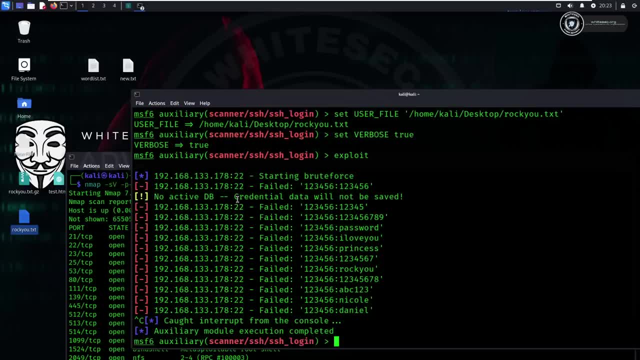 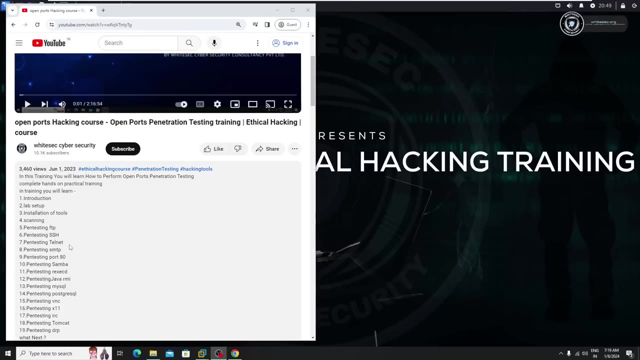 so let me stop it. hope you guys get it right. so, uh, to perform the brute force attack, you can use ssh underscore login. just try to watch this course. okay, here you will learn how to perform uh, pentesting on ftp, ssh, telnet, smtp ports. there is a lot. okay, you will learn a lot here, just try. 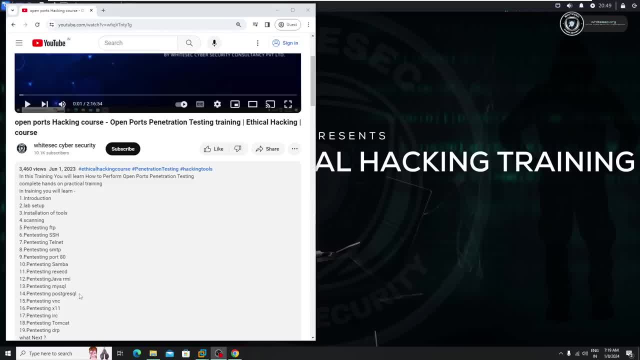 to watch it right, so it's not a big deal. it is a easy process. once you learn some techniques, you can able to implement those techniques in other services as well. it's not a big deal, okay, so just try to watch it. just try to watch our ethical hacking training as well, because there we still. 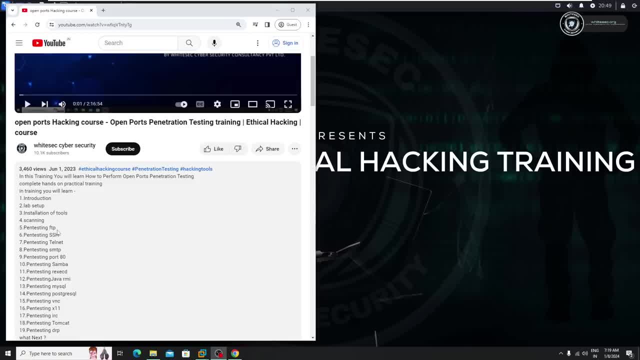 just covered a lot of things, okay, which is necessary for beginners. so let me tell you again, in this whole uh, in this channel, okay, in this white cyber security channel- we will add courses, not videos, right? so, which is necessary for beginners, we will add a lot there in future. 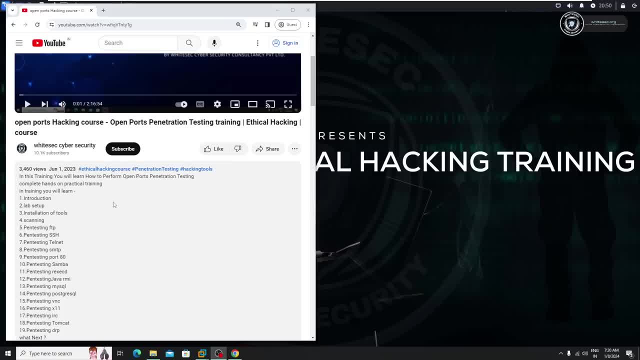 you will see a lot of things here, such as: uh, i just told you right, uh, networking course. we, we want to add here and there is a- uh, we just decided to add one other one course as well, which is: i think, uh, it's a reverse engineering something. okay, we just uh, we decided. 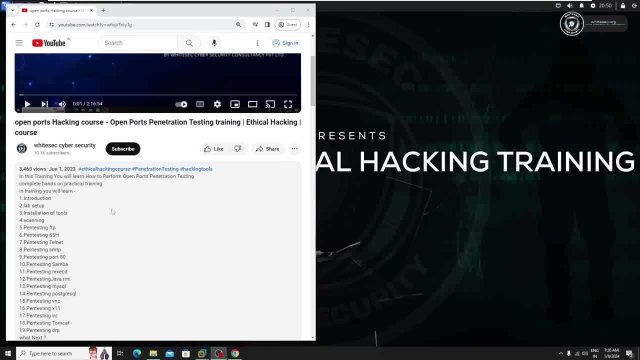 to add a lot of things here, right, like a sql injection. see, sql injection is a very uh huge topic. okay, so we are, we are deciding to add, uh create a complete course on it. let me, let's uh add in this youtube channel, so just just watch it. okay, it's not a big deal, just try to watch it in. 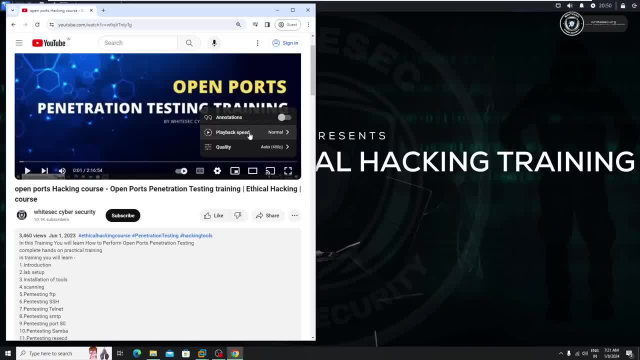 one point. okay, it is good for you, or you can also watch it in 1.75. so it's totally depend upon you. just try to watch it and complete the course, because you will learn a lot here. it's uh, don't think that these are the free tutorials. it's not, uh, that much important or something like that. see, if you didn't. 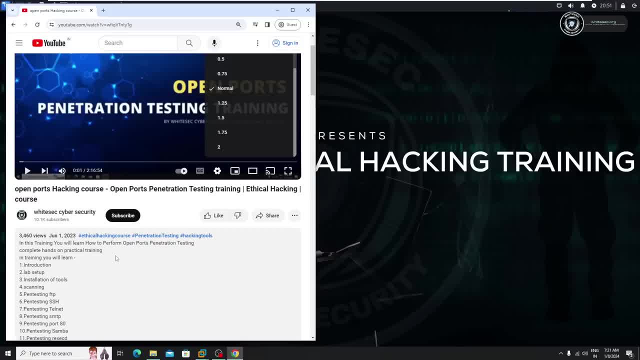 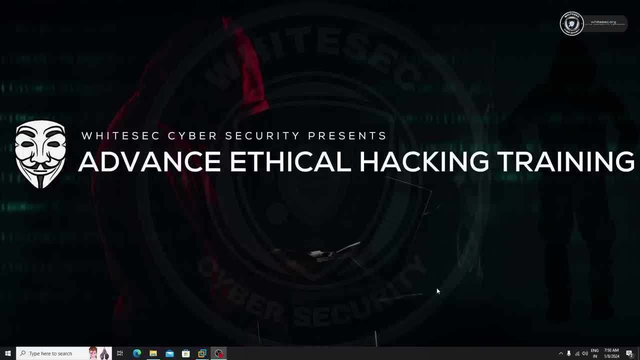 learn these things, then you can't go for advanced steps. this is the thing. so here we are learning penetration testing. see, i am adding some videos here, which is from our udemy course, right, so just watch it and see if you can do it. it's a cdf challenges, right? so, uh, first of all, you need to 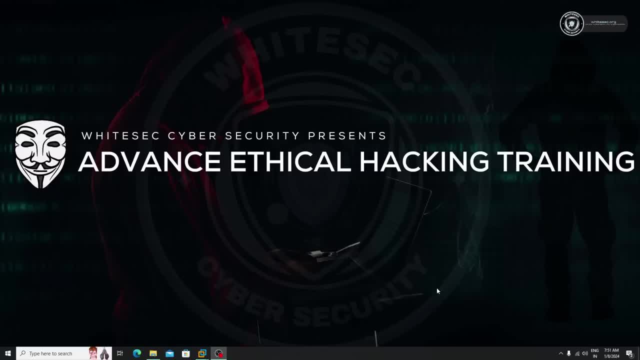 download the lab, then you need to set up it. it's a kind of uh, easy process. you no need to worry here, but the thing is you need to practice. that's it. uh, it's a very popular labs, right? so just try to watch it and practice it. hope you guys enjoy this training. thank you, have a nice day, hello everyone. 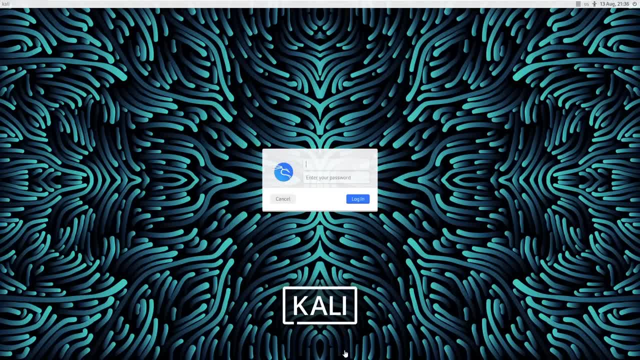 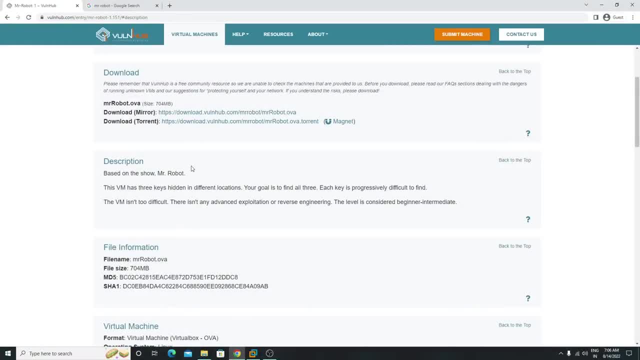 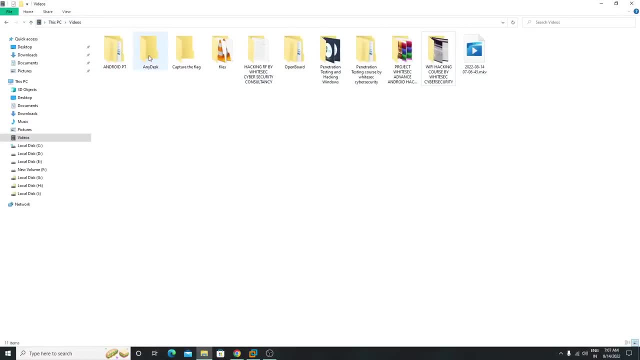 how are you all in this class? we're gonna use this virtual machine, which is known as uh, mr robot. okay, it's based on the tv show mr robot. to download this, here is a link: simple click here and download it now. i just already downloaded this one, right, so here it is. double click it now. uh, just type here. 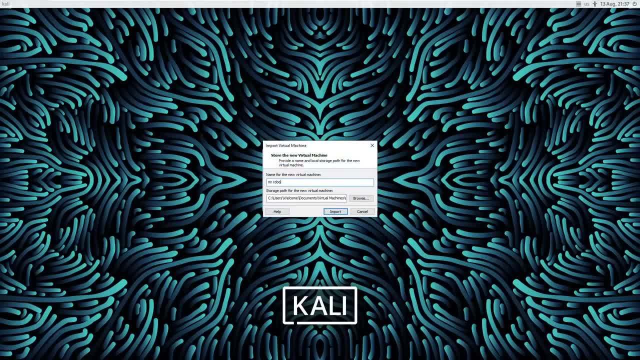 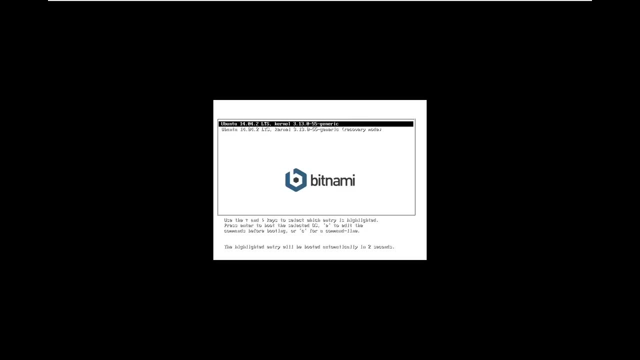 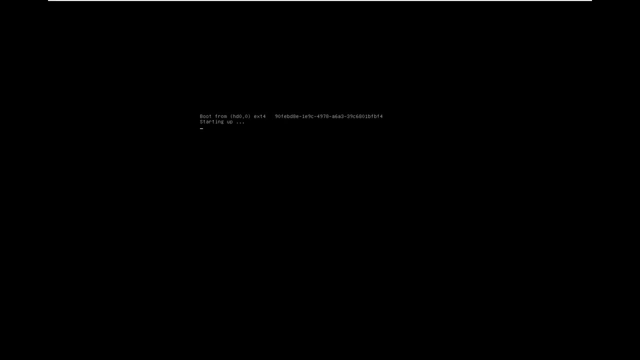 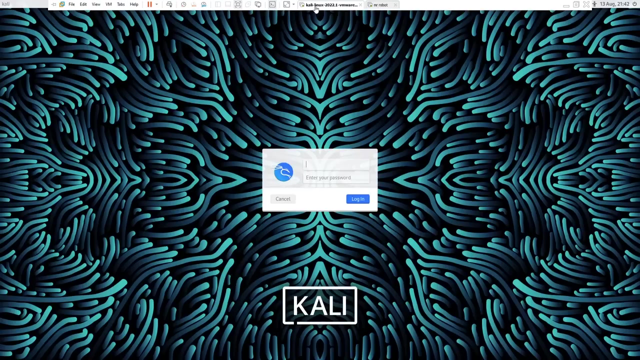 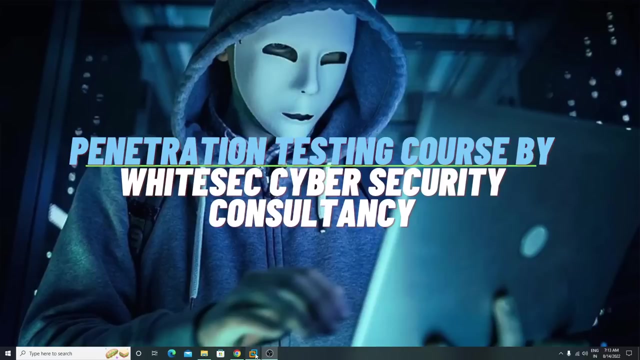 mr robot. simple click import, just wait. simple click on power on this virtual machine. just type enter so it's successfully booted now, uh, let's hack this one. okay, in the next class. thank you have a nice check. hello everyone, how are you all? the first thing is you just need to find the ip address of this machine, okay. 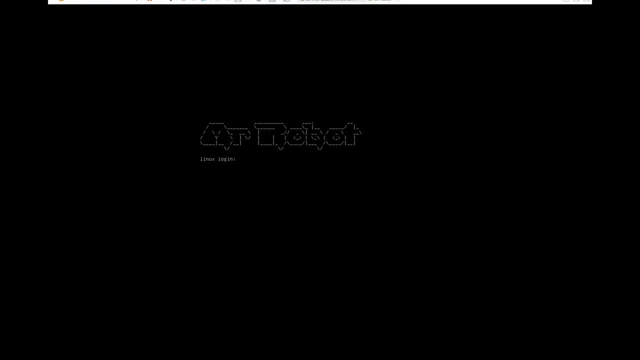 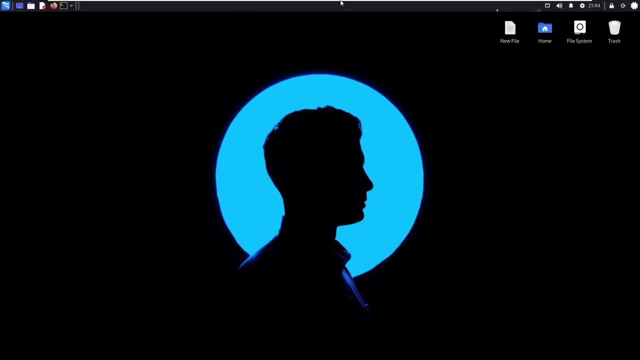 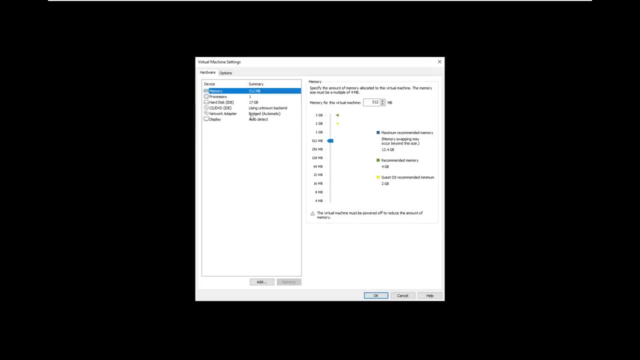 you need to find the ip address of this vulnerable machine. to find the ip address of this vulnerable machine, just go back the same. uh, you just need to use the first of all, just check. click on the vm, click on the settings using bridge network. just change the bridge network to not network. okay. 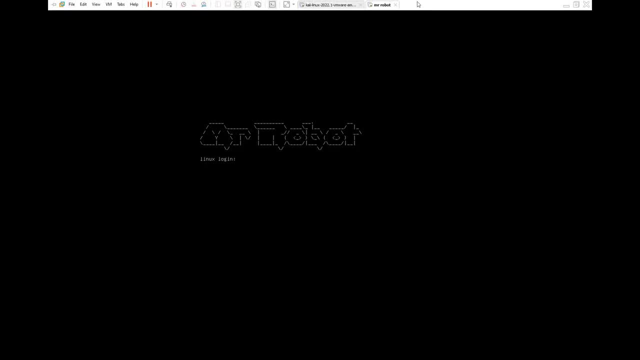 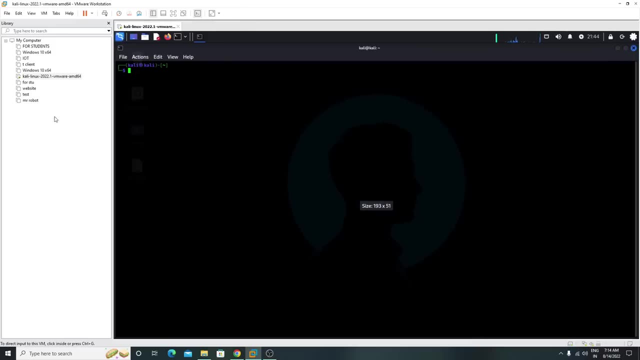 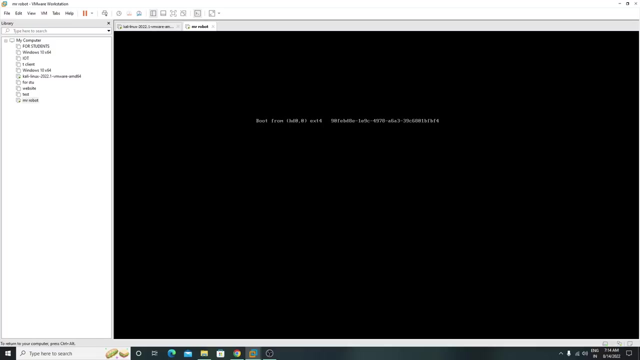 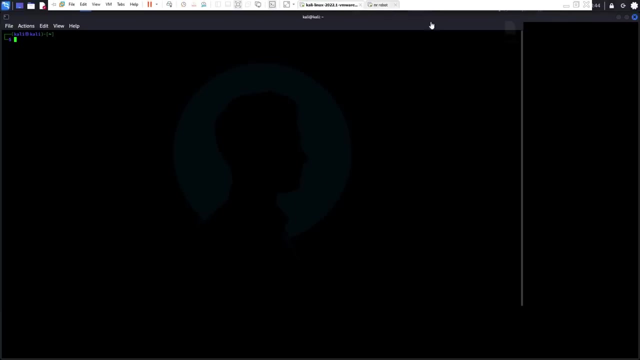 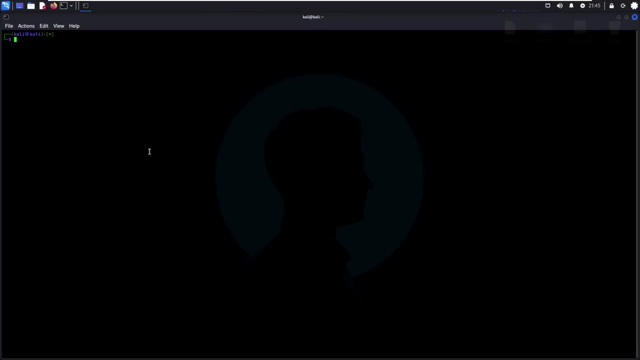 just click. ok, now, simple, close this one, just power hop this one. then again just uh, click here again. just start it, just type enter. it will take some time to reboot, just wait. so to identify the ip address of this virtual machine, just type here: sudo net discover. 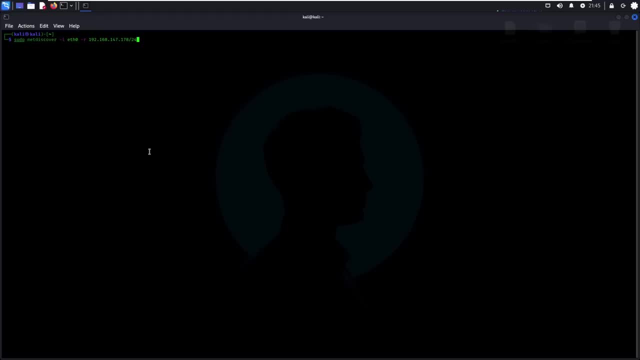 sorry guys, pts0 dash range. just let me now here. there is a range, right, just copy this one and from here remove the 24. let me type here: 0.0 forward slash 16. right, just type enter. it will take some time. so here i got some ips right, so simple. let me scan. it is a 130, is it right? let me scan this one. 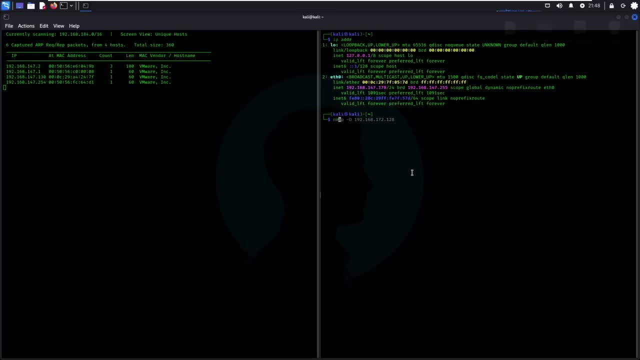 just type here: nmap sudo. first of all, just type sudo: nmap dash, capital o and copy this ip address and simple paste it here. just type enter now. here i got the results. right now it's saying: uh, this is a linux virtual, uh, linux machine. okay, the same. uh, see, this is also a linux machine. 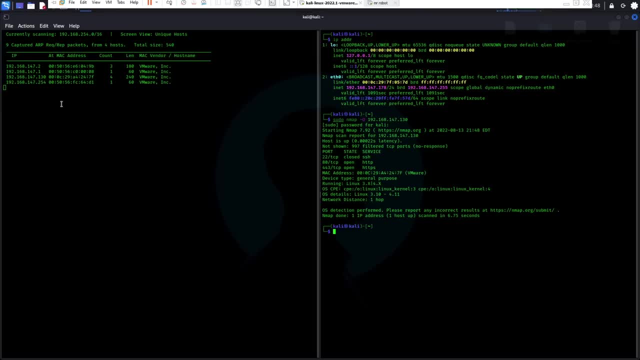 so this is our target. let me stop uh. stop this one right now. you just need to perform some scanning here, identify the ports. let me scan for all open tcp ports: okay, nmap, dash, p dash. and then let me scan for uh. scan its script, scan as well. 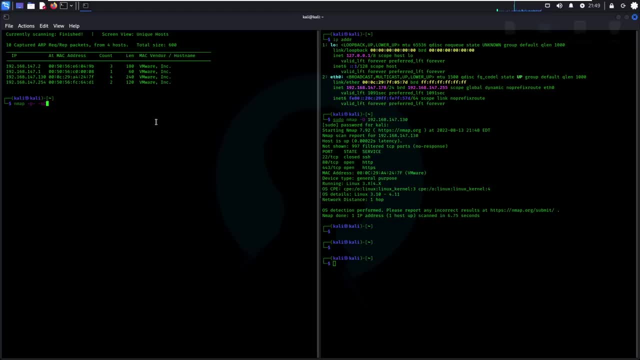 sc. right, then let me identify the service versions- sv. then let me find the identify the vulnerabilities. okay, don't, no need. in the next plan i'm gonna scan for the vulnerabilities, right, simple, copy this target ip. let me paste it here now. here you guys can able to see. just see it's open only, uh, three ports, okay. 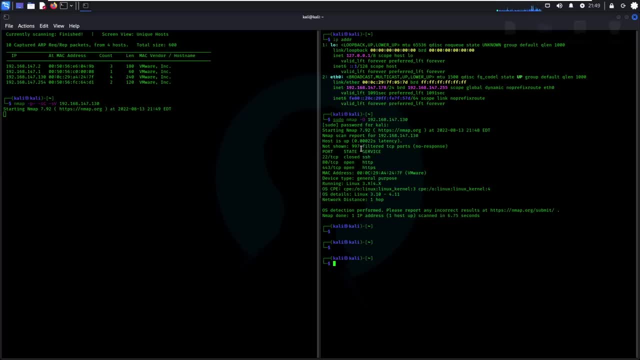 so and uh, 997 ports are filter. no response from that ports. just wait now here. uh, here is the results. right, simple. i can't able to find the version of ssh because the port is closed. now just see, there is a 443 is there and there is a 80 is here in 80, as we know. 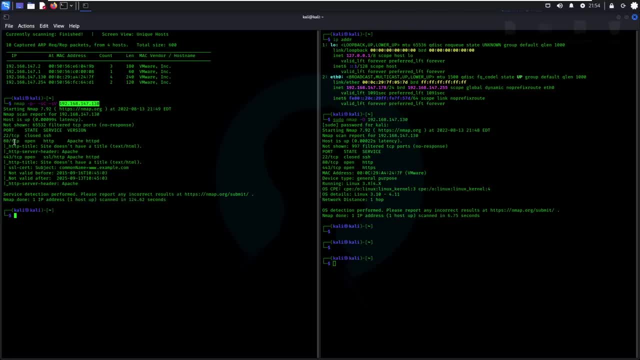 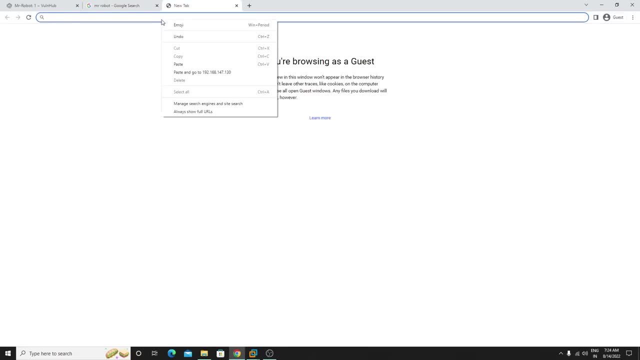 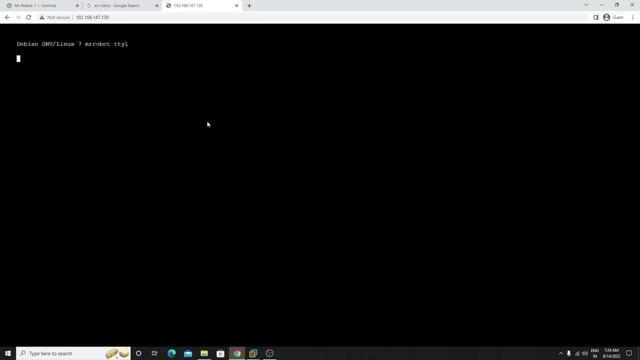 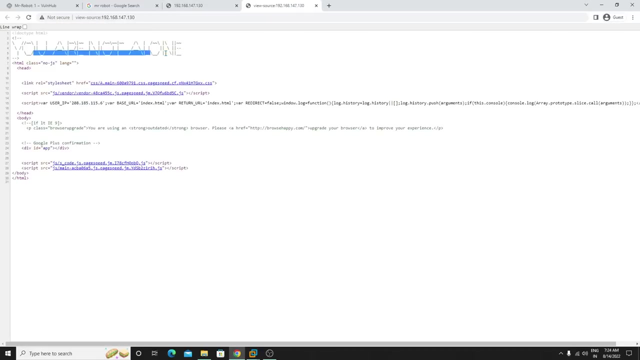 uh, it's for the web server. okay, like, uh, to host a websites or something like that. now, simple, let me paste that ip address here and here you guys can able to see there is some terminal. okay, um, you have for a reason. okay, just click on the view page source. uh, you are not alone, okay, alone. 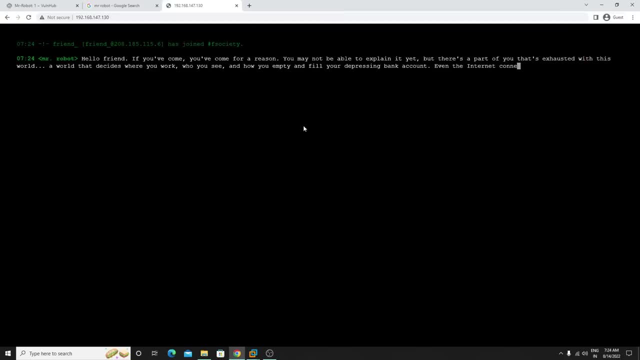 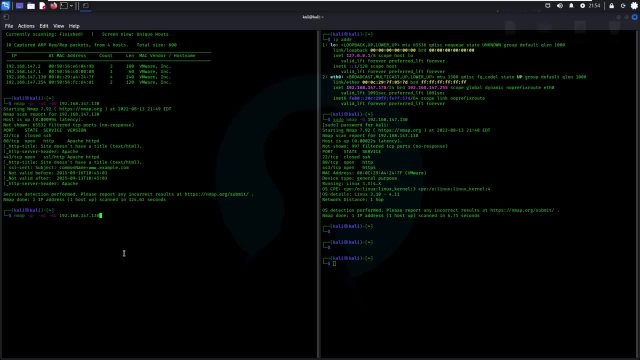 sorry, just see. let me go back and simple. let me type for uh, search for the vulnerable days. okay, just type here: dash, just script is equal one, right, just type it. and map, just type i, uh t there. so here you guys can able to see the map, here you guys can able to see the map. here you guys can able to. 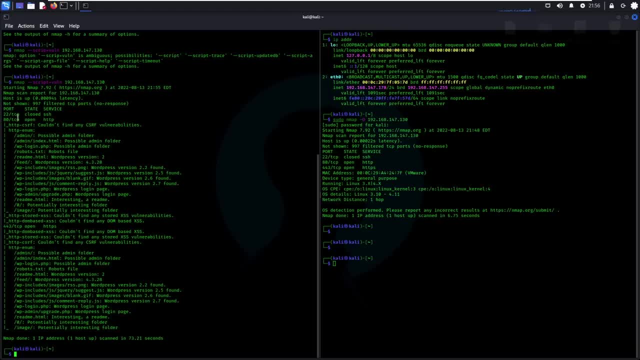 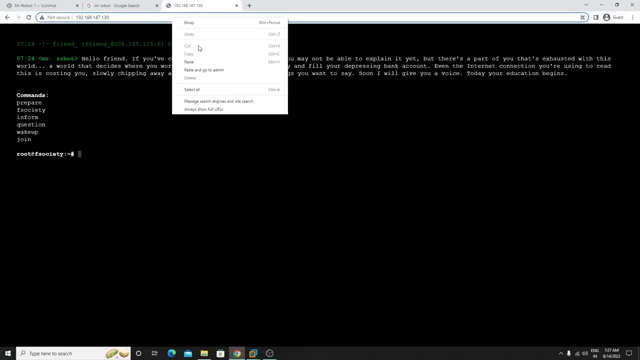 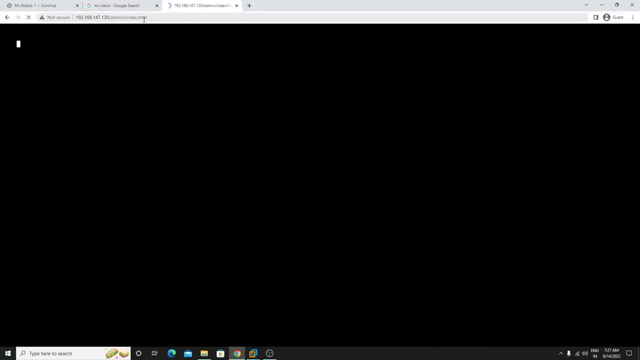 see uh it scan for the port 80. in port 80 we can able to see: uh, the folders are open like admin is here. let me copy this admin and simple, let me paste it here and just type enter. so it's redirecting to admin index dot html. okay, it's not loading anything, just wait. so it's not loading anything. 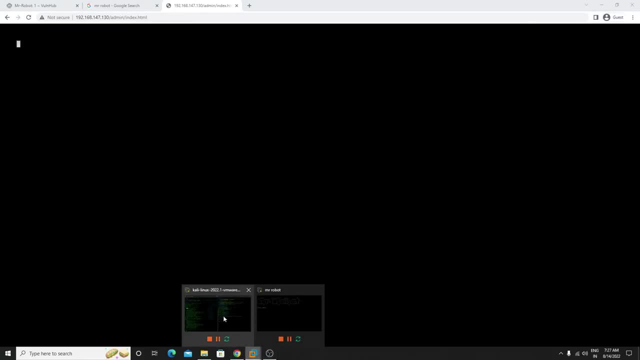 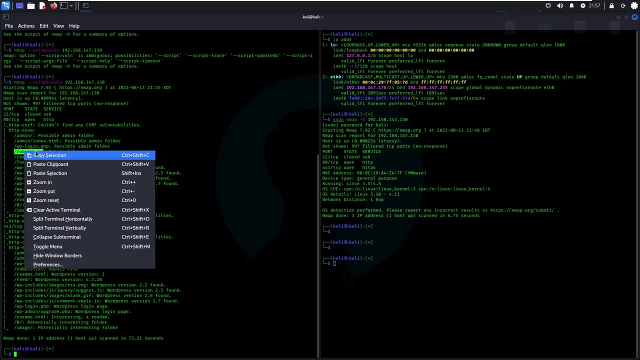 let me go back. so it's not loading anything, just wait. so it's not loading anything. let me go back now. there is a wp login is here. see, there is a robottxt is here. what is this robotph txt? let me tell you. just first of all, let me see for this robottxt. 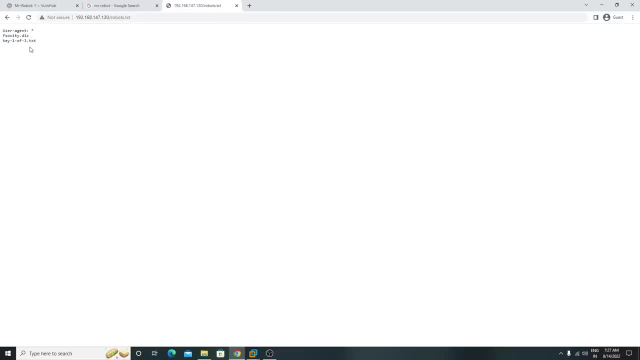 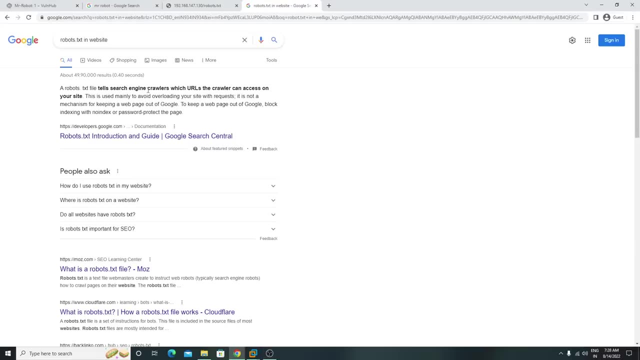 just type enter. so here is the results. now, what is this robottxt? robottxt tells search engine, uh like, see. let me tell you in the frank way. it will tell, uh, just see. it will tell the search engine, uh like, which folders we can able to access, like which. 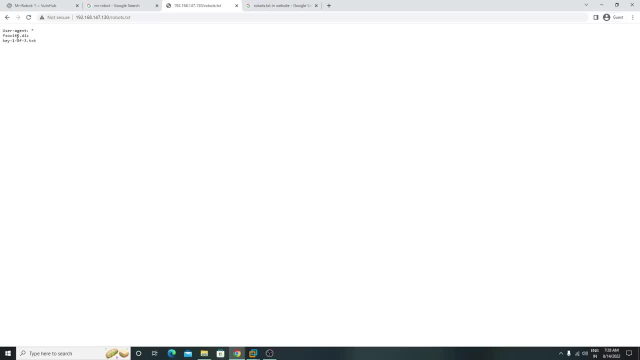 directories we can able to access, right like. assume that here you guys can able to find like, uh, like this, uh file: simple, just copy this one like this names: just simple, copy this one and simple, just paste it here. right, just paste it now. let me type here forwards: 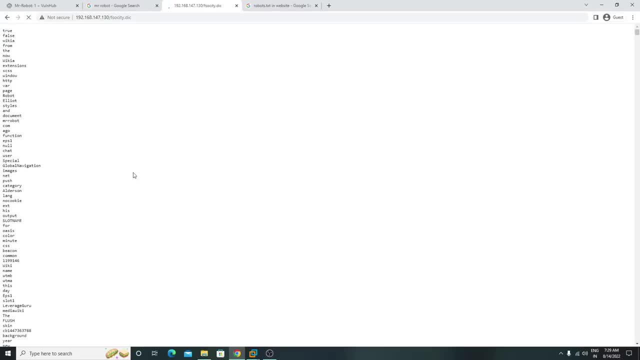 slash and just type enter. now here you guys can able to see a huge amount of word list, right? so let me go back now. here is a key. one of three dot txt is here. just remove this and just paste it here. so so, so, so, all right, just type enter now. here is our first key. we just completed our 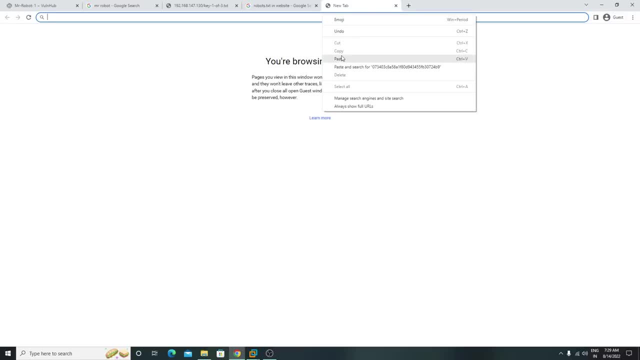 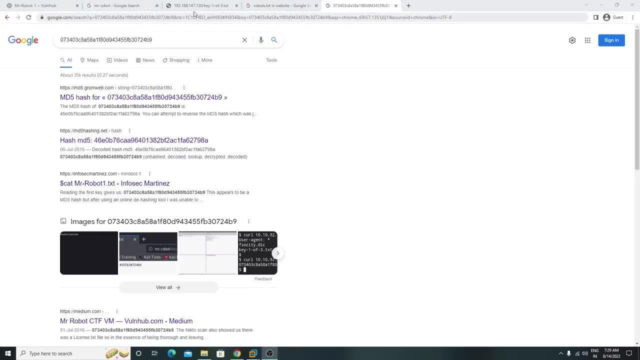 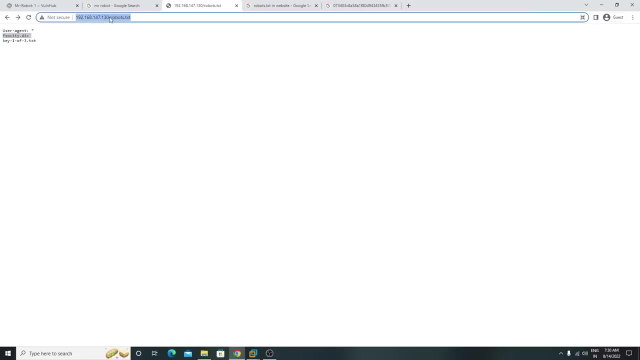 first challenge: right, just let me paste it here. so let me go back. and this is a file: okay, let me copy this. just let me paste it here. just type enter: let me download this one. okay, and this is a one, just let me copy this whole. uh. 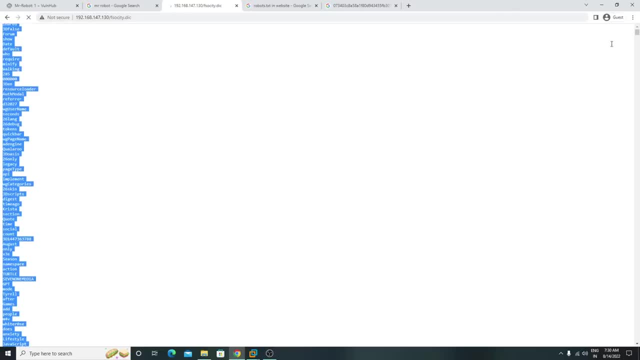 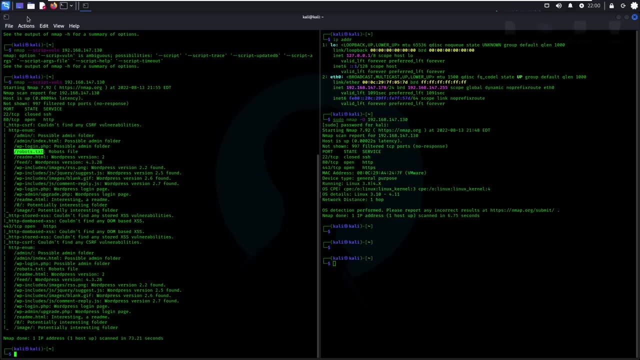 but see it's a such a long file, let me open this in my linux machine, but let me go back open the browser. let me go back open the browser. so so let me download this one, just so. let me download this one. just click on the save and click okay. 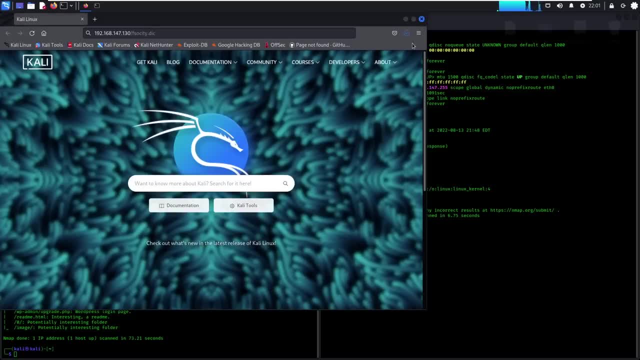 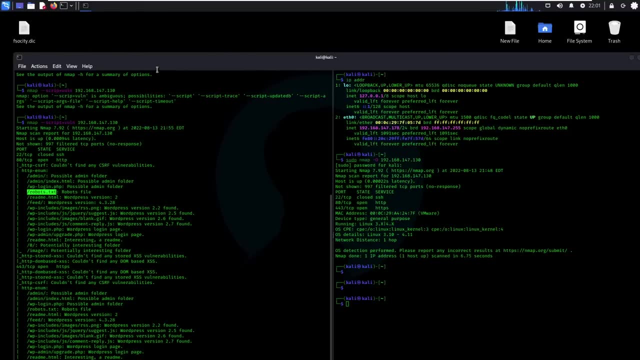 successfully downloaded. now simply i just paste it on the and click ok. now this is a nothing course. have just done. i'm happening. now. this is a nothing courseings, and still i'm Korean. not a part of it right now. go back. check is a nothing, but this is a word list, so this is how you guys can able to scan for the hidden. 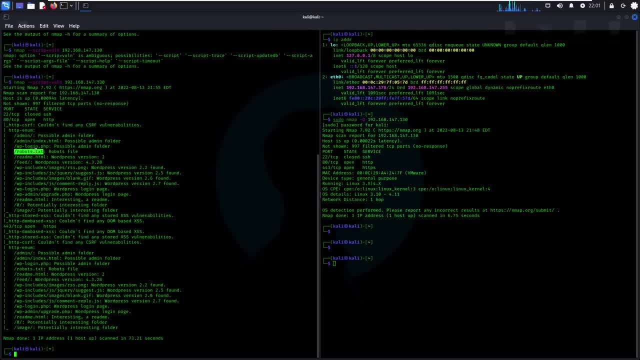 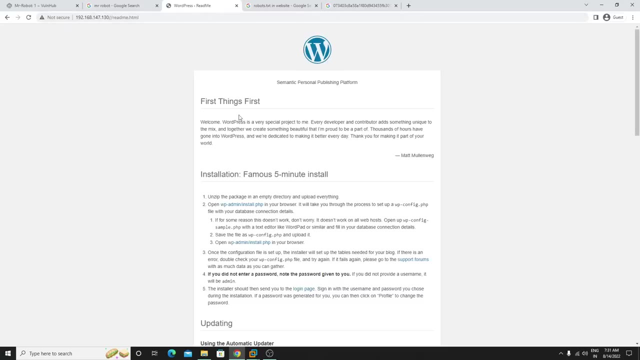 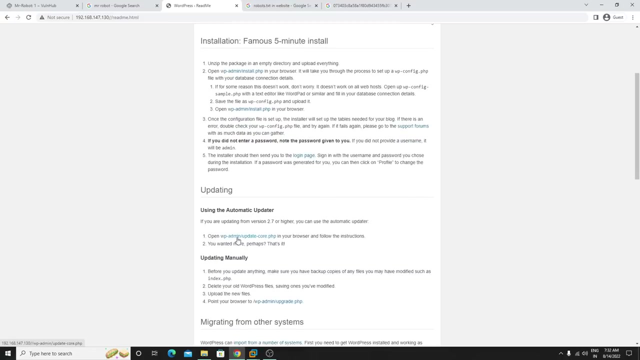 folders by using robottxt. right now there is a readmehtml, is there? let me copy this and let me paste it here. so first thing is first: uh, it's having the wordpress website, so let me tell you: uh, just see here, open. let me open this: see, i got the login page. okay, so we can brute force this one. 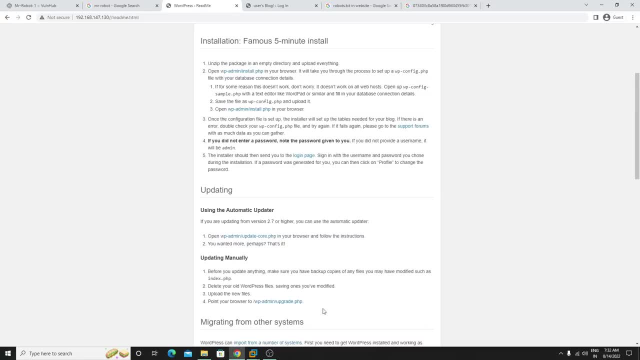 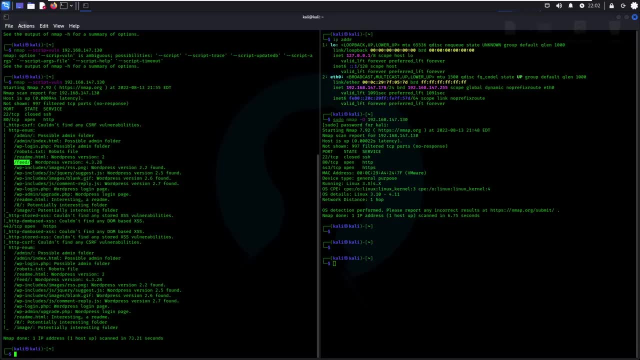 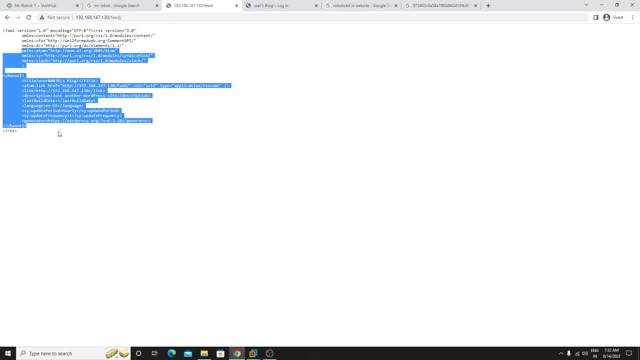 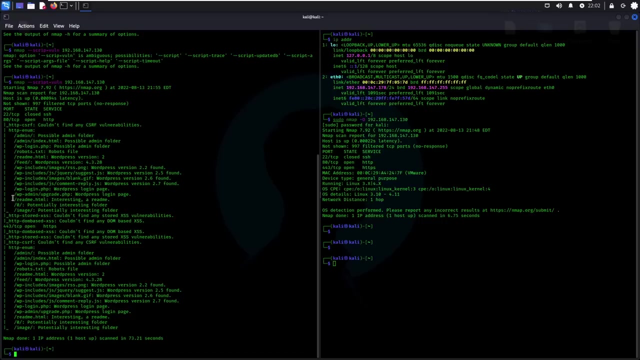 or see there is a another. let me scan for the other stuff. there is a. feeds is here. let me copy this and let me paste it here now. here is a something, uh, which is xml version. is there? okay, now let me go back. wp in: uh includes images or the login php, upgrade php. let me copy this. upgradephp is there. 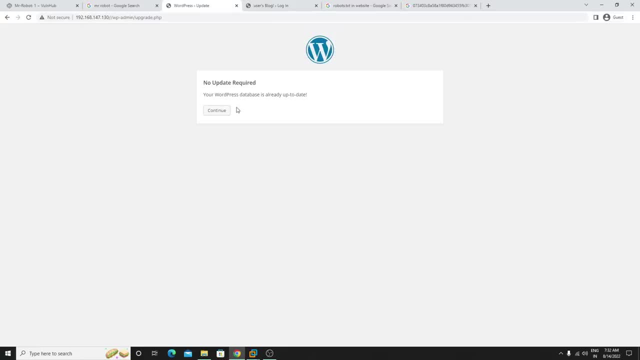 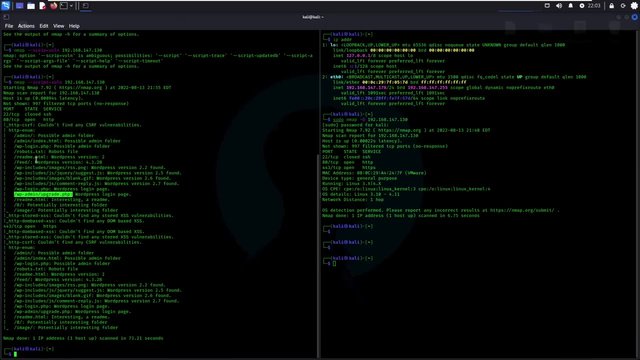 now here is a. no update required. okay, let me go back and see. here is a readmehtml. the same file is here now. here you guys can able to see, there is a zero is a. let me copy this and let me paste it here. we need to identify the web server first, okay, 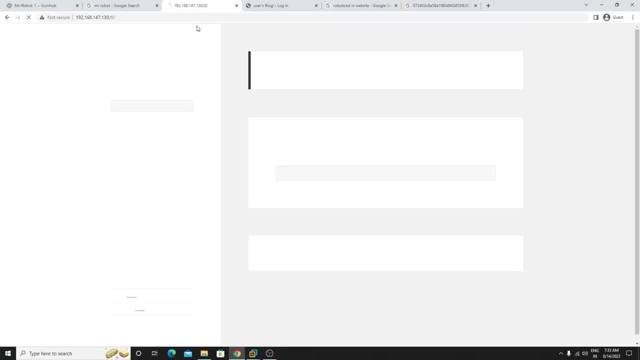 now let me paste it here. now, here is our uh website. okay, sorry, website. now, if i click on this commentsrss, oh, here is the feeds. okay, if i click on the login, here is a wp loginphp. simple, we guys can able to brute force this one by using wp scan. okay, 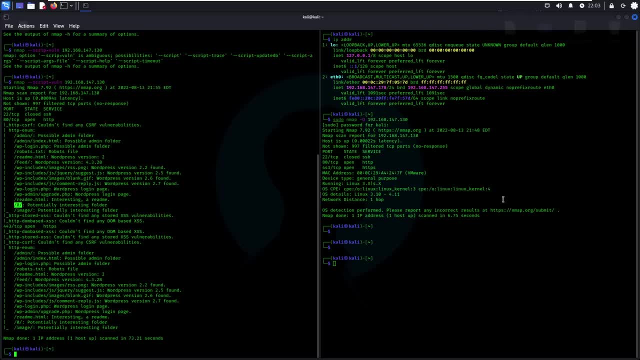 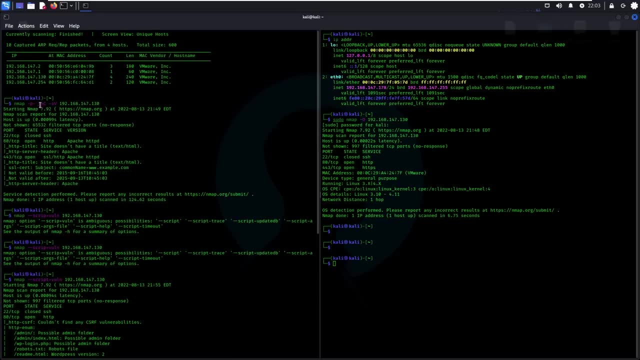 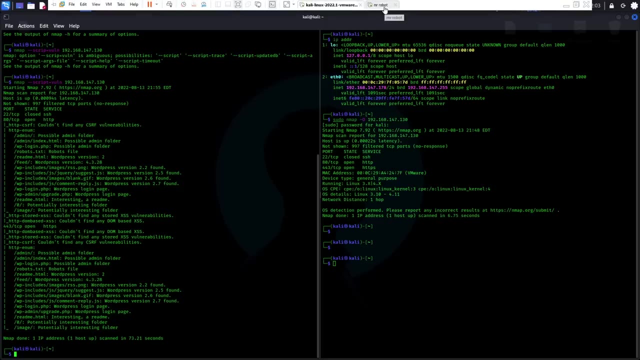 first of all, what we did means we just uh, scan for the vulnerabilities. let me tell you one thing, guys: if you are scanning the internal networks, just follow these steps. okay, if you are a beginner, then go for this one, just scan. i just download this kind of vulnerable virtual machine and practice. 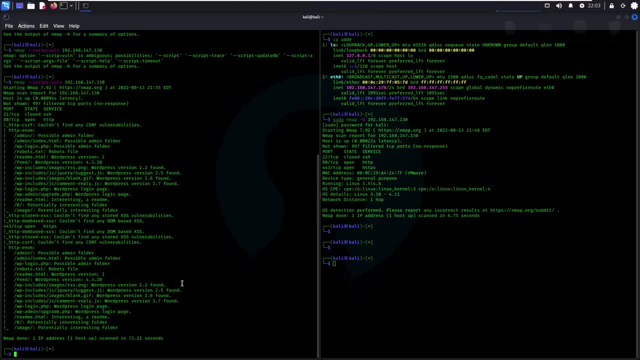 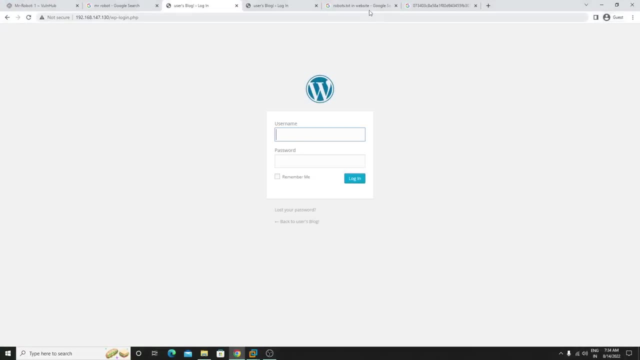 this one. okay. now, the main reason is: see, assume that there is a robotexe. uh, i just forget it about this robotexe, right? so what is this basically? just assumed, uh, see, you just need to read the google results because, uh, i can't explain you this one, okay, uh, due to my slang. 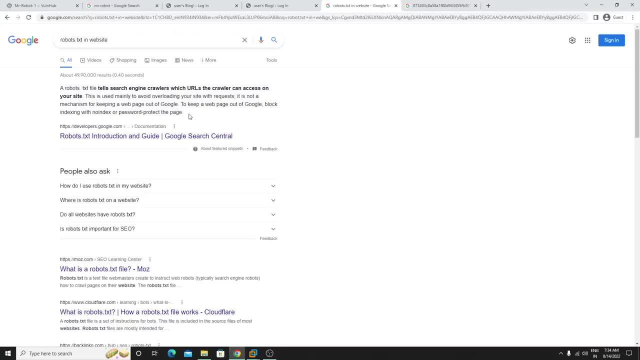 you guys may won't understand that, okay, so that's why just uh read this. uh results okay. uh, this stuff's from the google. you see, this is used mainly to avoid overloading your site with requests. okay, request. it is not a mechanism for keeping a web page out of google. to keep a web page out of google. 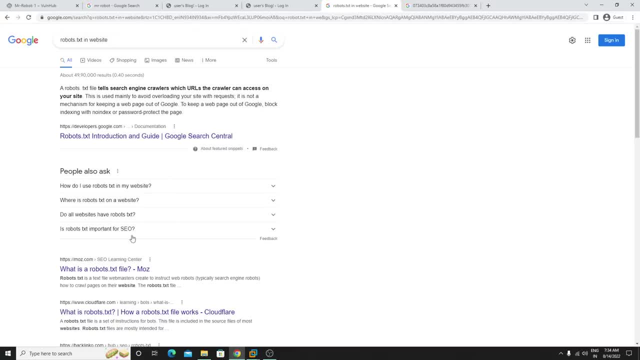 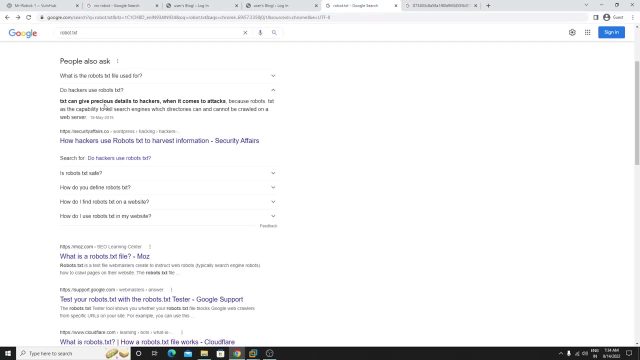 block indexing. uh, just see, here there is a. just let me go back now here. do hacker use robottxt? txt can give pre uh, pre uh vicious details to hacker when it's come to attack. because robottxt has a capability to tell search engine with directory can and can't able to. uh, cannot able to on a web server. okay. 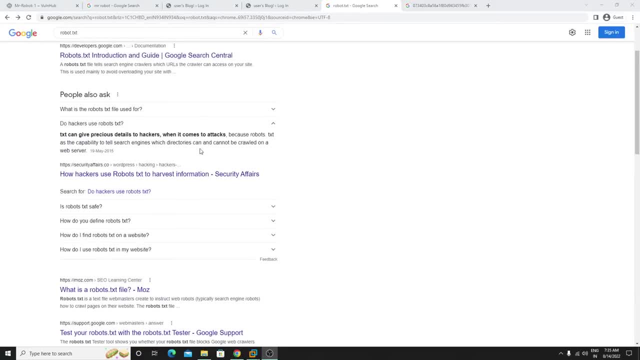 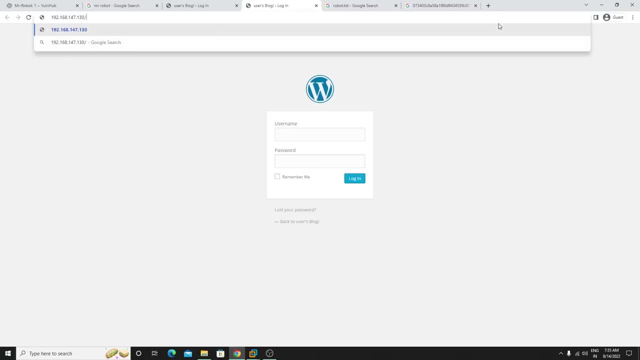 so the main reason is: uh, it will tell the web server which directories and which folders can are accessible by the users. okay, simple, i just type here, uh, robottxt, where it is so simple, let me type here. robottxt here. uh, where is a robo. okay, man people, let me. 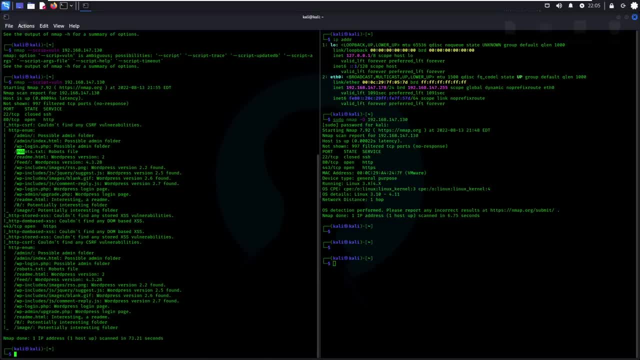 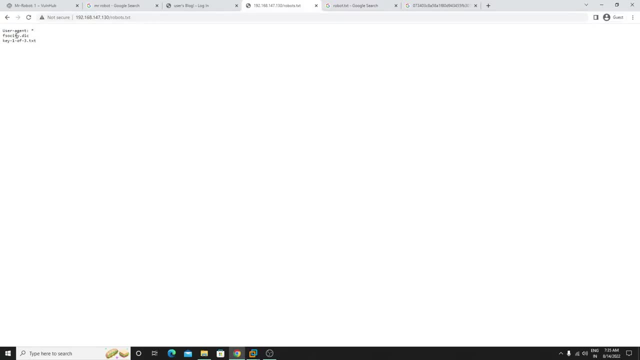 sorry, robots dot txt right. so it said: uh, it's telling us we can able to access this stuff. okay, like we can download this one. uh, this is a key or something like that. let's see this. uh, same site on our real websites. okay, see, here is. 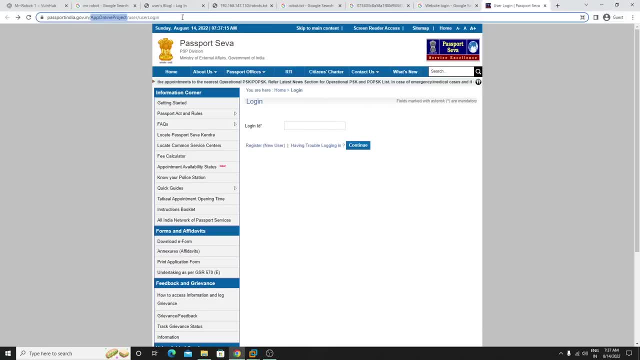 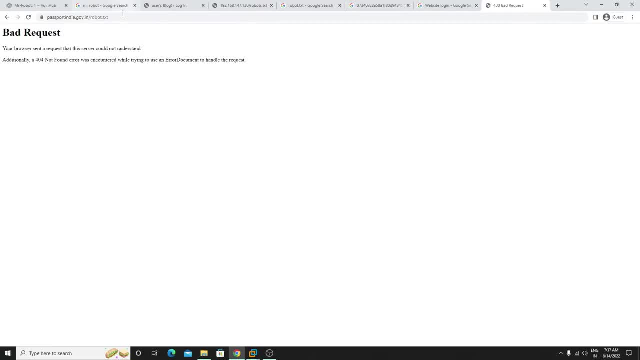 a one website. simple, i just type here robot dot txt. see, i am getting the bad request request here. right, so just type robotstxt. same thing, okay, because, um, we can't able to access this because this website is secure. uh, from this robottxt, right, we can't able to see the more. 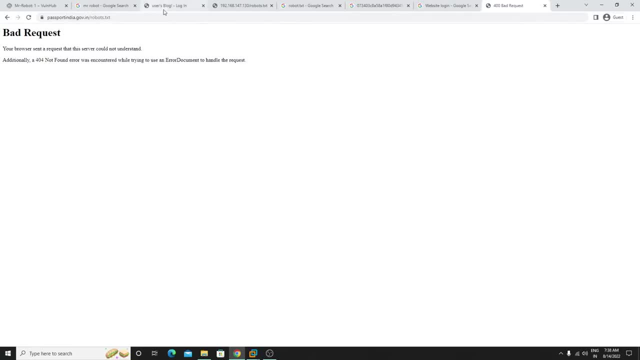 informations like: uh this server right. uh, here we guys can able to see. uh we can access this website, uh this files. okay, but here, whenever we just type the robotstxt here, we can't able to uh perform this request. okay, that means it's secure. so this is the main reason. try to uh read this. 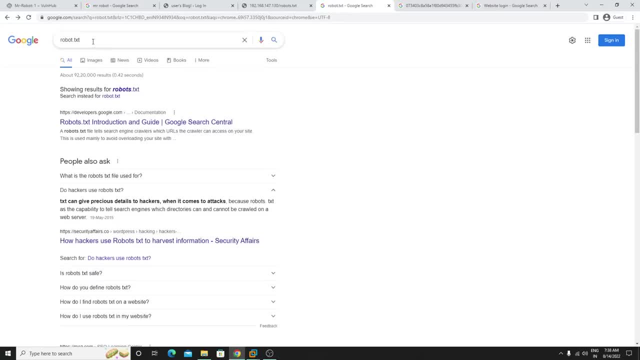 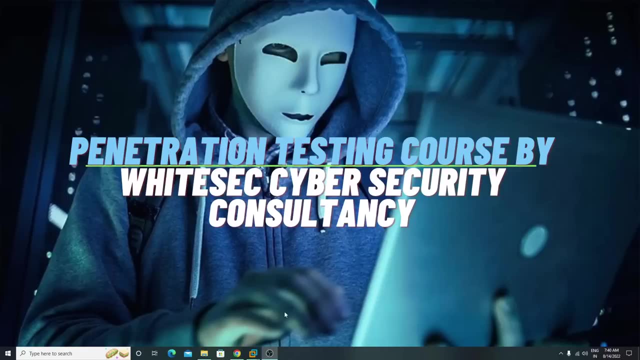 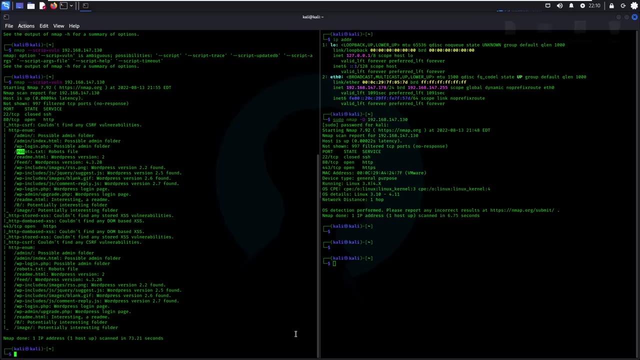 robottxt: right right right, right right right from google. thank you, have a nice day. so in this class i'm gonna show you how to perform user enumeration in this web server. right, so simple. in the last classes we learned about how to perform the user enumeration by using wp scan. right uh, to perform uh user enumeration. 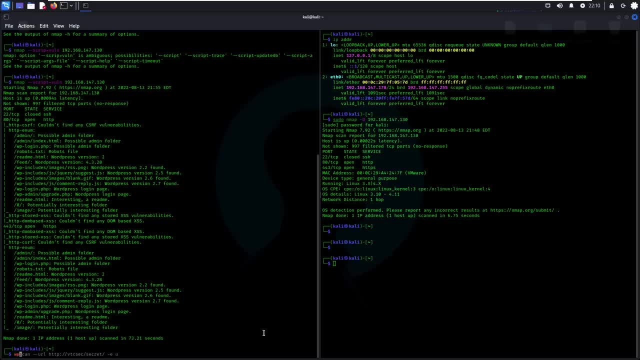 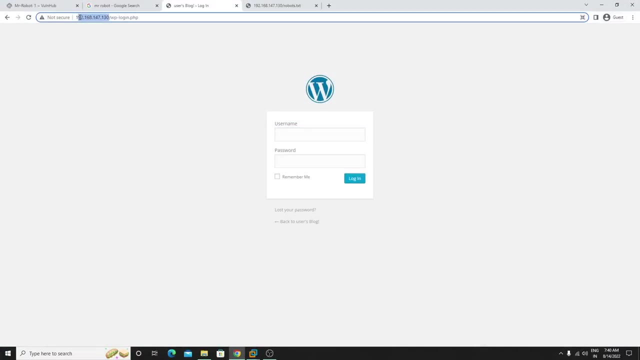 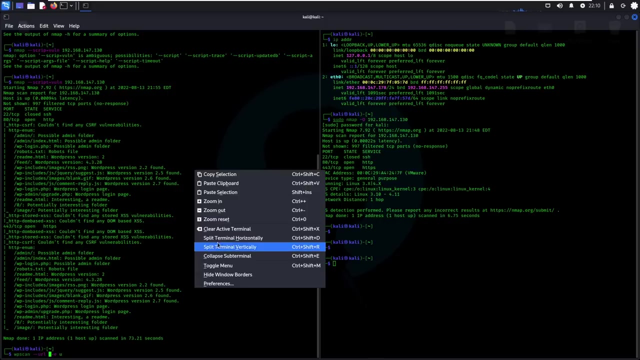 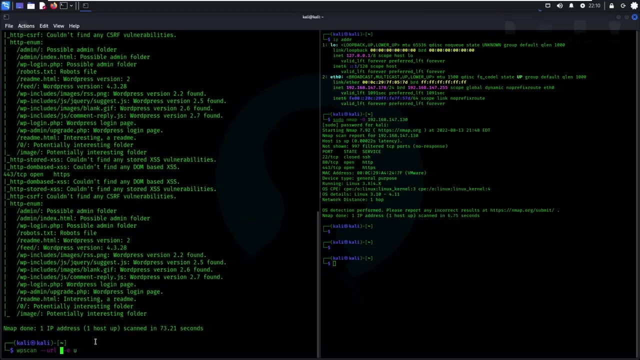 just type wp scan there, just change the website, uh name, just copy. just go here and copy this one, just copy this one, just copy this one like this ip address, like this ip address, like this ip address, and simple and simple and simple. it's simple. let me paste it here. 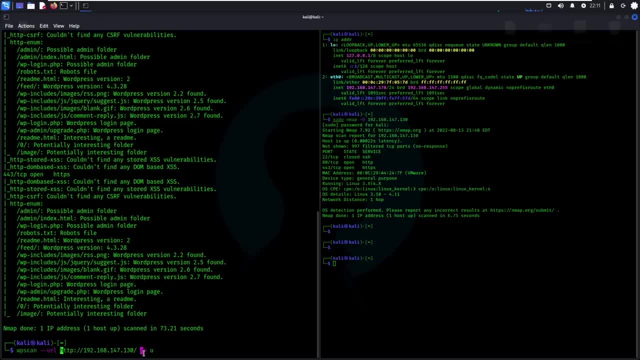 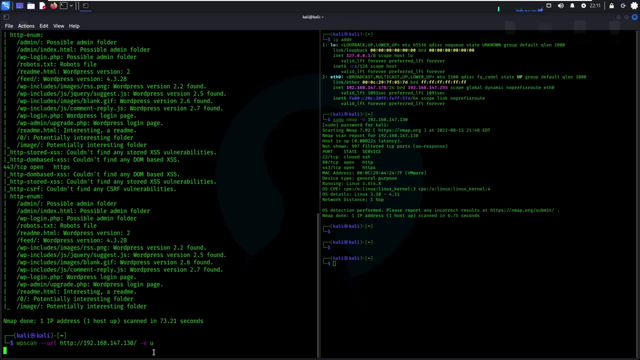 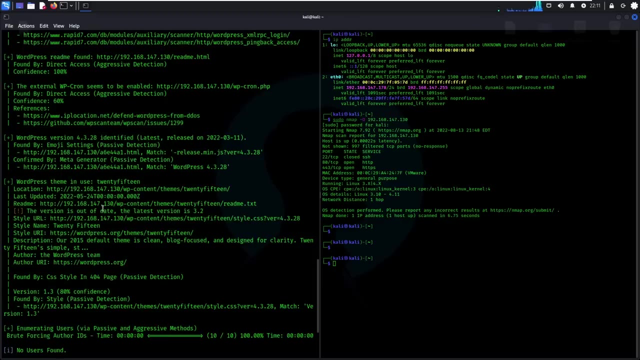 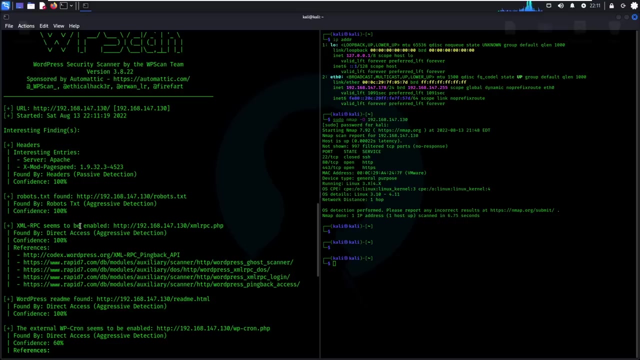 and just type here: dash e u. okay. enumerate user. just type: enter the last classes. we see this right. so from here you guys can also find. just see here there is a robottxt. found is here xml rpc to be enabled so we guys can able to perform the penetrate, uh brute force attack here. okay. 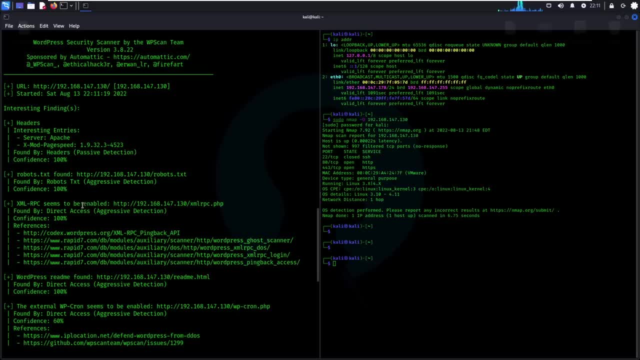 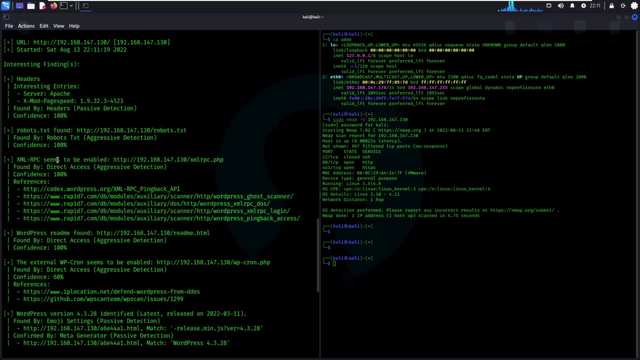 see, let me tell you, if, if there is xml, rpc is disabled, then you guys can't able to perform the brute force attack. because if you can't perform the brute force attack, then you guys- because, just let me tell you- it will block your request. okay, if it disable, then it will. 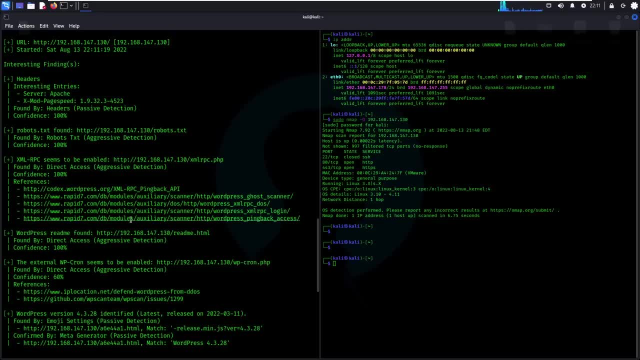 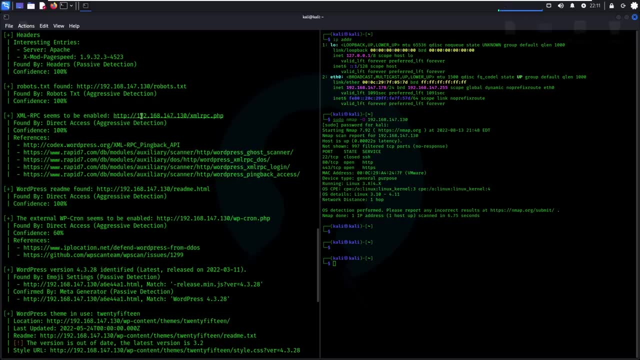 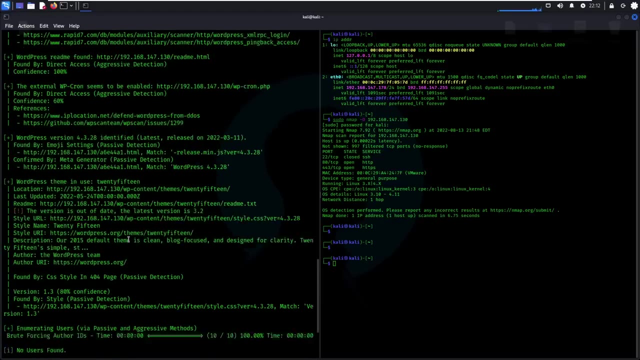 block your request like you can. you guys can't able to uh send the multiple uh request request to this web server. okay, so that's why xml rpc is very important in the brute force attacks, right? so let me see for the wp wordpress readme from uh is found here now, just the theme is. 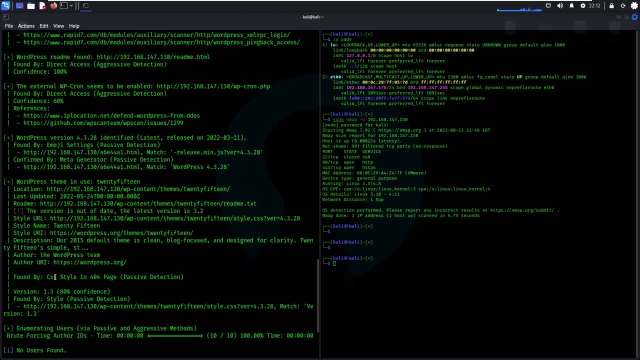 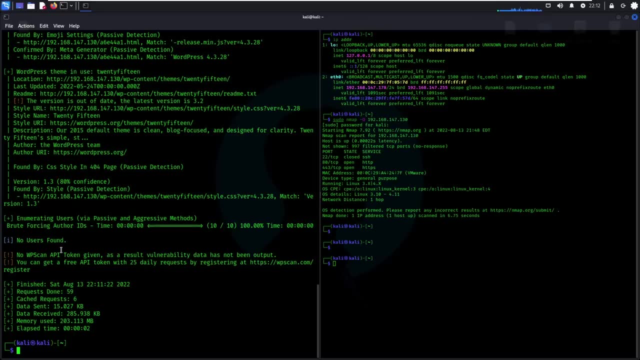 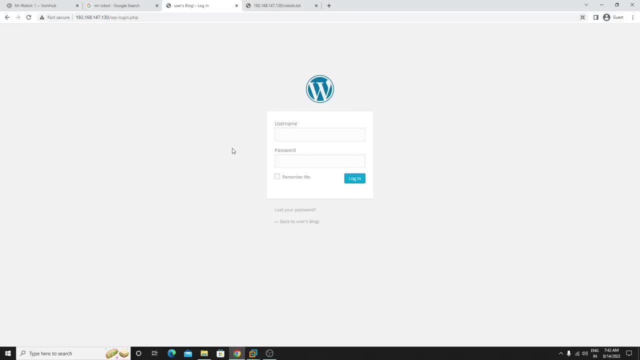 outdated. okay, now, no users found. just see, here we won't find any kind of user in the last classes. uh, we found a user with the name of admin, right, but here in this case is we can't able to find any user. okay, now, simple, assume that this is a kind of organization. then what you? 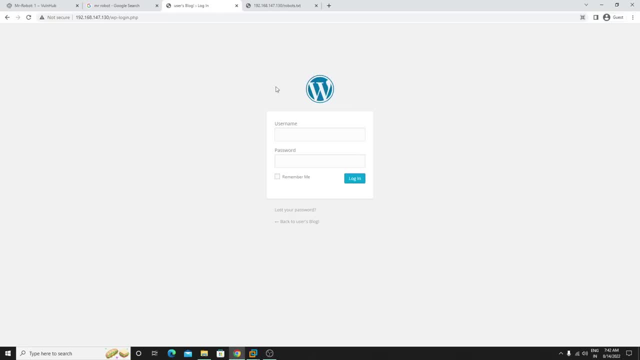 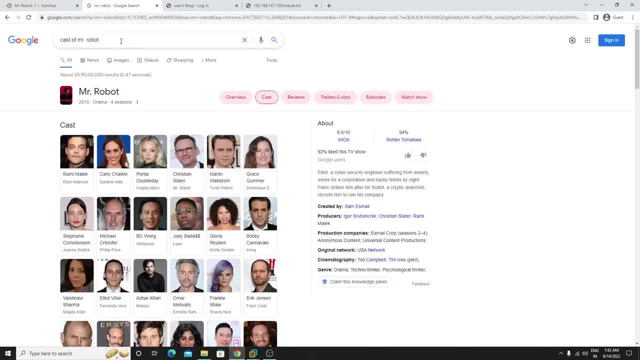 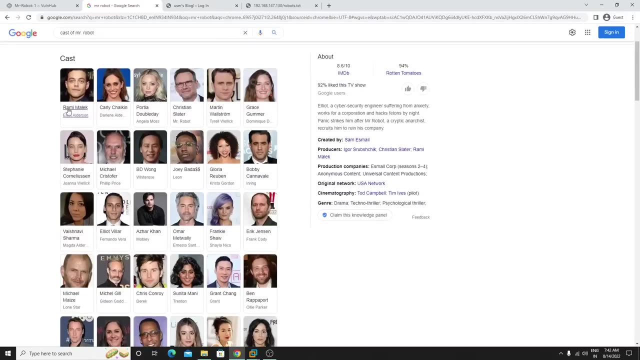 white sake or something like that. you will do a recon or something like that. okay, then you will find a results like: uh, the about the employees, about the ceo cto, or something like that. you just find the information about them and simple. uh, you guys just assumed it. 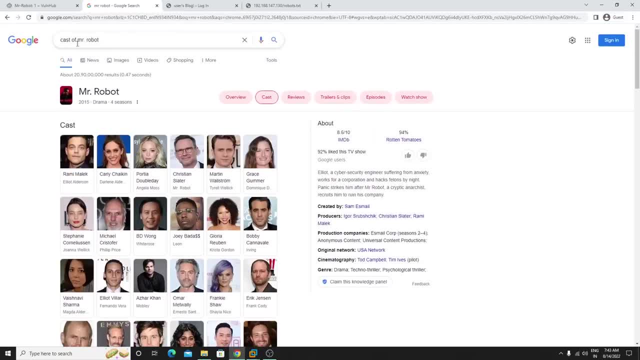 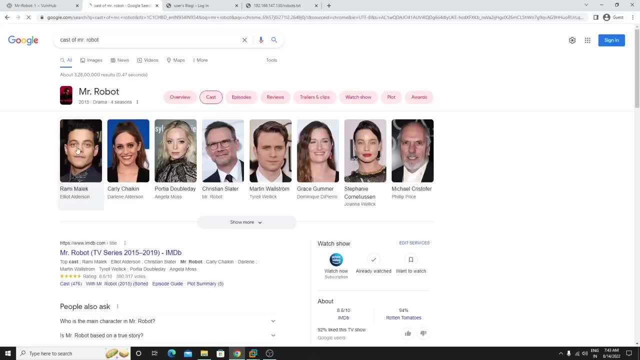 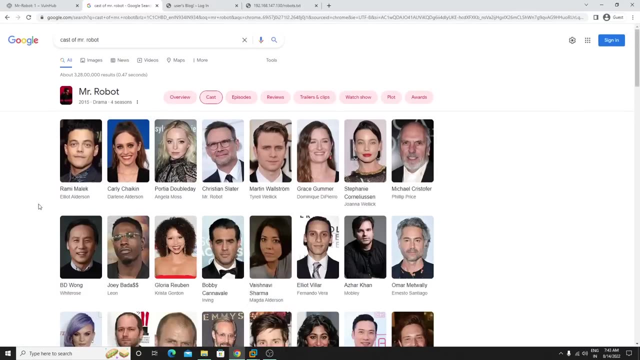 uh, i just searched about mr robot. okay, first i searched about, uh, mr robot. then here i i can able to see the cache of mr robot. simple, let me click on the show more see the main character of this. mr robot is elliot right now. simple, just copy his name. this is a kind of thinking. 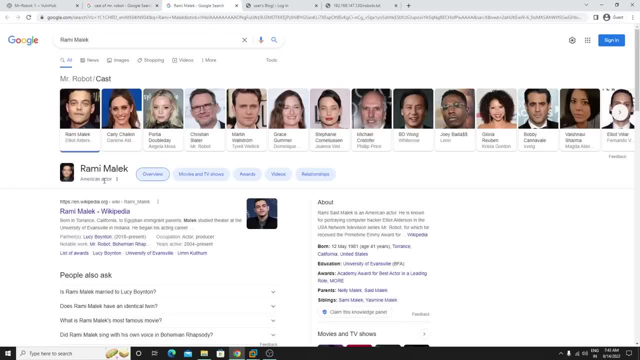 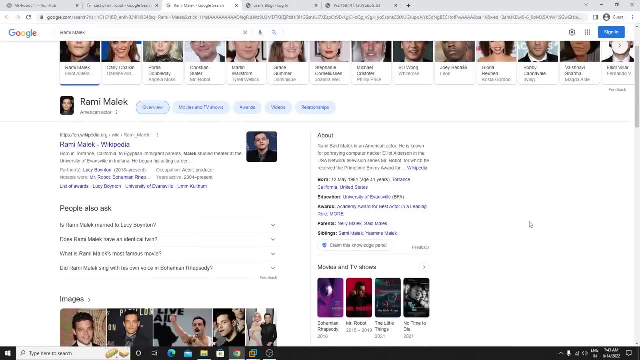 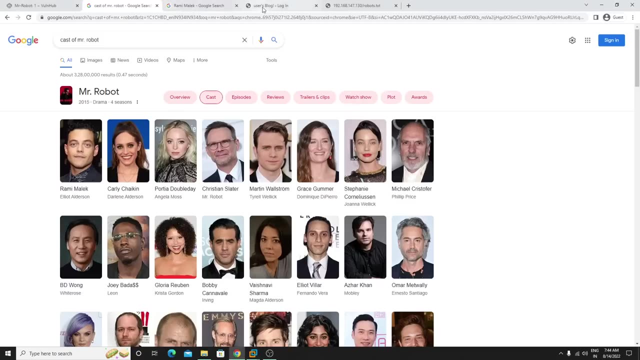 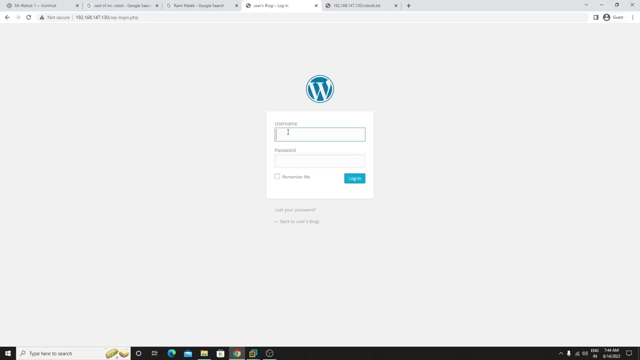 okay, the hell man- uh, let me copy the name of this mr robot- is elliot right now. so simple. in the last classes we use the admin and for something like that, but i don't want to waste your time here, okay, by typing that. uh see, the main reason is you just need to in the real world, you just need to perform recon. 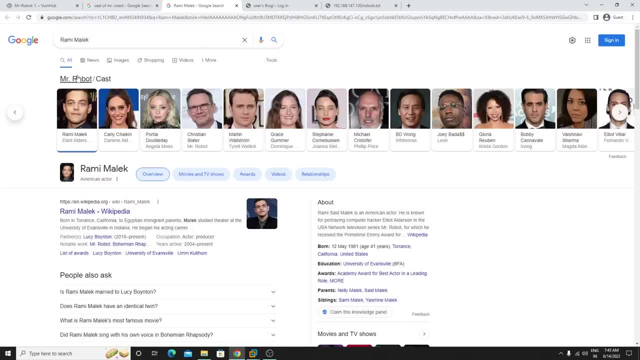 okay, like you just need to gather the information about that uh specific surfer, uh, about that organization, then you guys need to perform the brute force attack by using the username and the. don't worry, i'm gonna show you right. so how to perform the brute force attack, or? 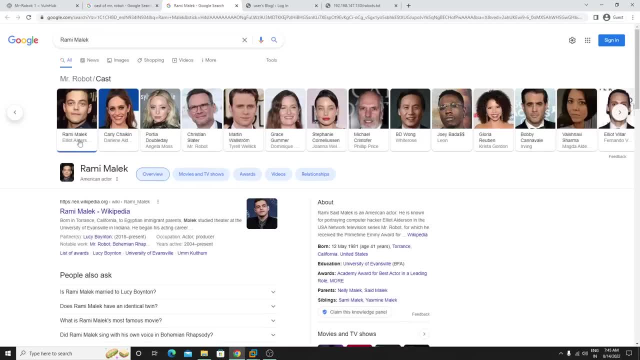 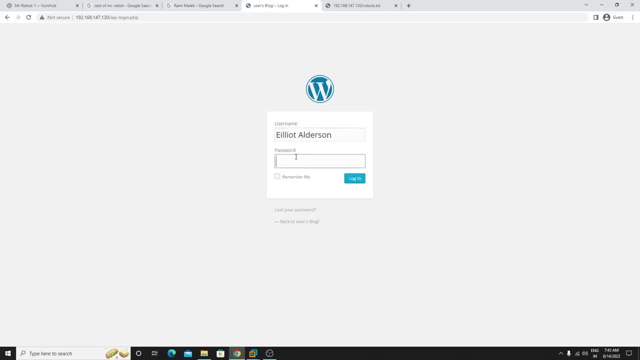 something like that. first of all, uh, i'm gonna target this main character. let me paste. paste his username here, elliot, and just type the password as a password. all right, error. now let me change this to elliot. okay, just type the password to password. simple, here is a. elliot is here. now let me change this capital to small and let me. 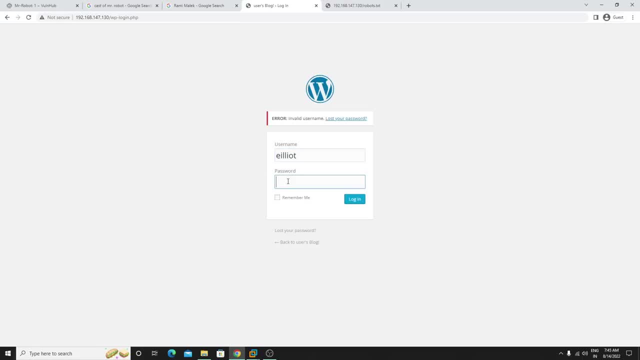 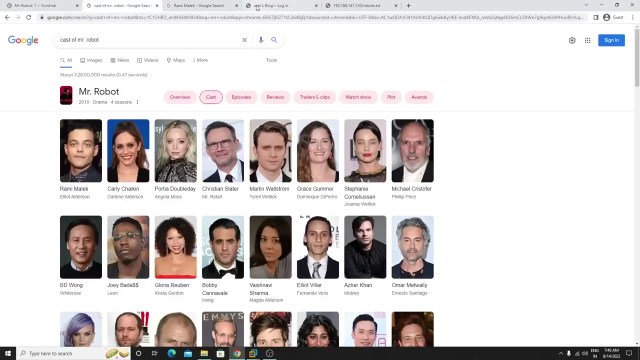 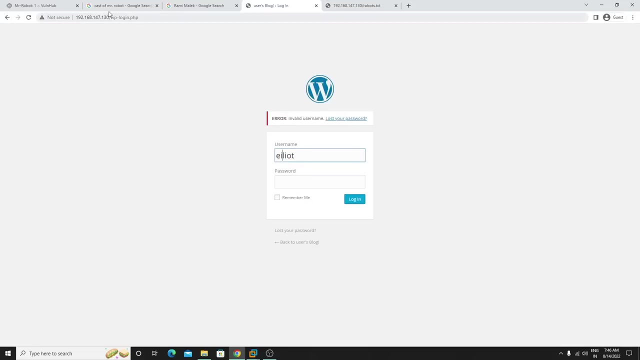 see, it will give you some idea. okay, so that's why i'm doing this. just type here password now same. sorry, i just typed there, right right, simple. let me type here password. just click login now. here you guys can able to see that for the email that youbly check um. here you can see, uh, just uh, the password you entered. 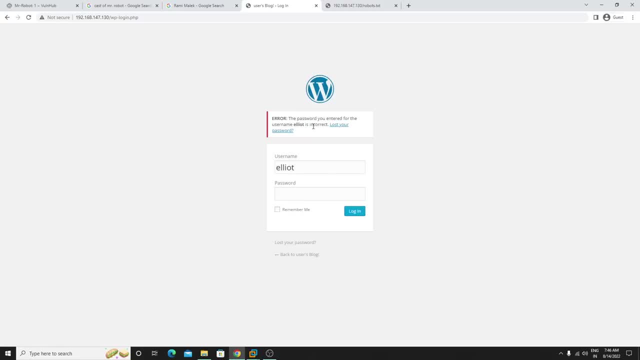 for the username elliot is incorrect. now we understand. the elliot is a user of this uh server. okay, we have the user with the name of elliot, because just see the same steps here. just whenever i just type the correct name there, it's showing the password you are entered. 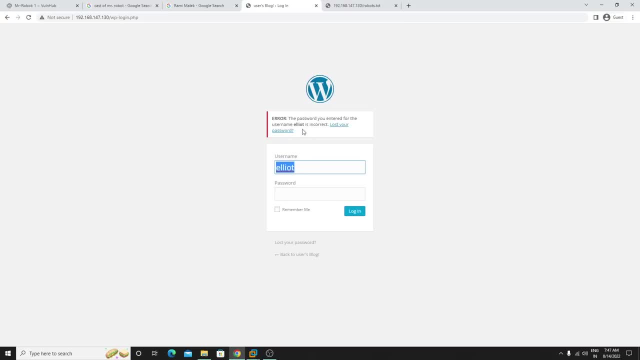 for the elliot, for the username elliot is incorrect. if i type elliot's here and just see, let me type the password. just click, then you get the again. the password is provided and then also there is the name and um, see, right here we can enter the username and there. is the password there, right here. so that is how you know that i'm going to title this object, we're going to call that right there, we're going to display that and then just type this and just like that. you just need to open our application here and 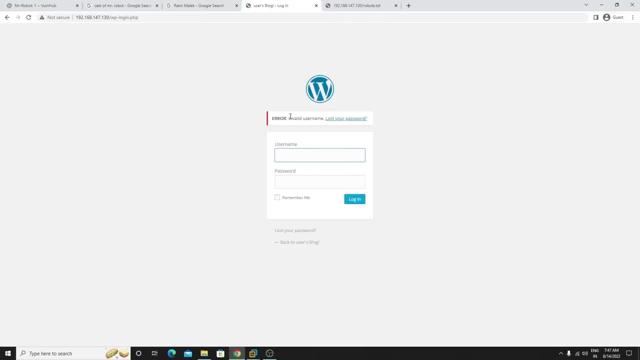 click on the login, just see the different. the error is different here: invalid username. so this is a reason. okay, if I type Elliot here, maybe the spelling is right. right, Elliot, you see we got the username. okay, now we just need to crack the password. if you remember, in the last classes you just downloaded one file from here. okay, a key. 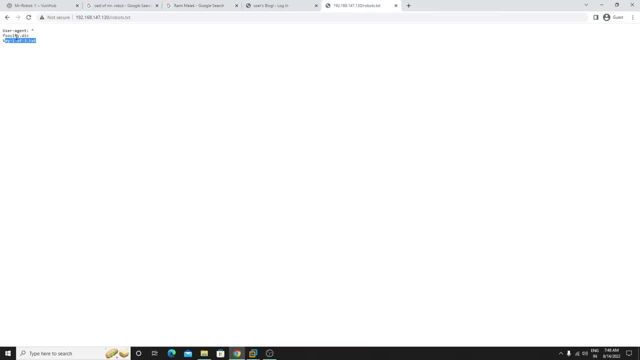 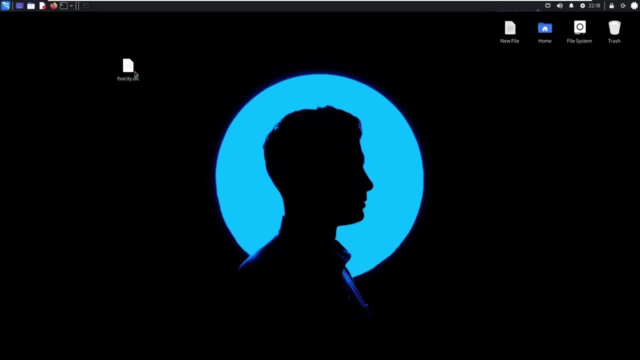 file, the sorry F Society dot big. just let me show you this one we just downloaded in the last class. if I open this- this is a kind of word list- okay, see in the real scenarios what will happen- means: make sure that you have the password in the last class. if I open this- this is a kind of word list- okay, see in the real scenarios what will happen. means: make. 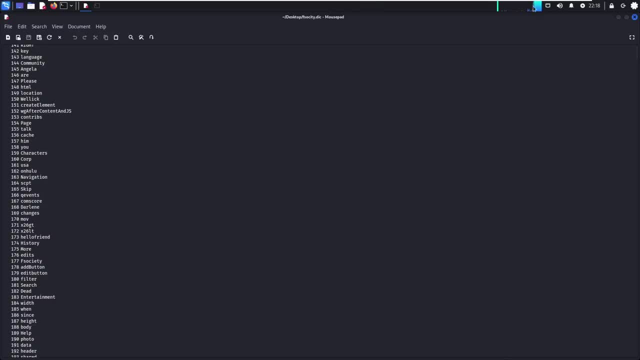 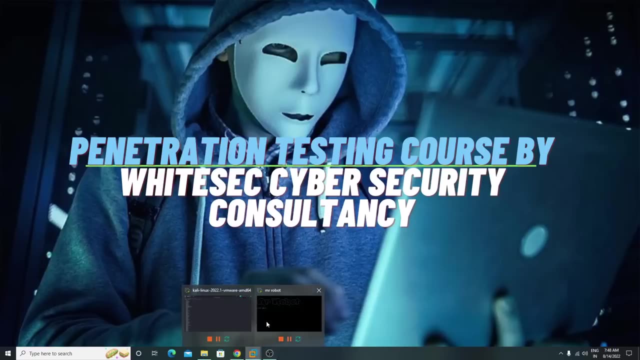 sure that you have the password in the last class. if I open this, this is a kind of word list. okay, see in the real scenarios what will happen means majority. okay, like, if you are scanning for real world server or something like that, then you guys can able to see the database files there. okay, like in the 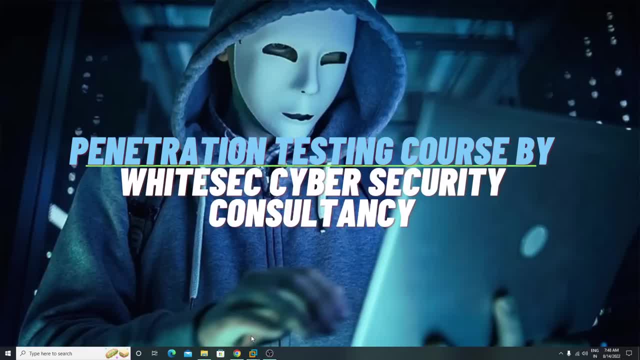 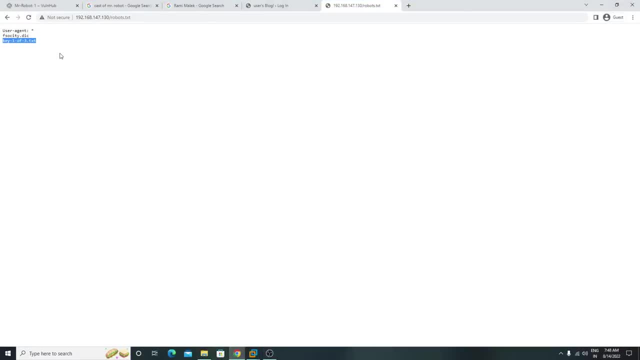 robottxt or, in majority, you guys can able to find a database password here. okay, yes, according to me, I just find a huge the database, but not in robottxt. but whenever you just do a fuzzing on the website, on the server, you guys can able to see the database passwords and a user names, etc. 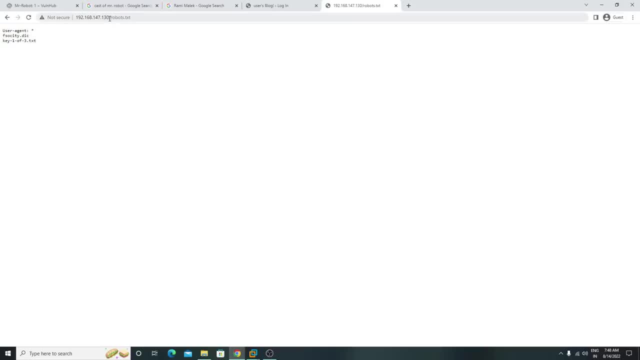 in the just let me dot ENV or something, or type ENV there in the real world website. this is the extension. okay, dot ENV. here you guys can able to find the. don't worry, in the next classes I'm going to show you this- all the shops, okay. 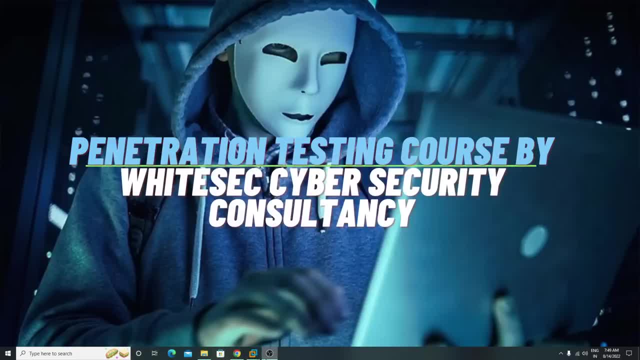 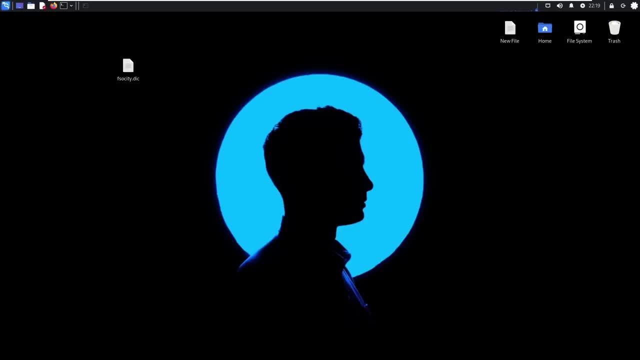 now let me go here. let me start the brute-force attack. right, the next classes. I'm going to show you how to perform the brute force attack. thank you, have a nice day. hello everyone. how are you all in this class? I'm going to show you how to perform the brute force attack, right, so in the last classes, we. 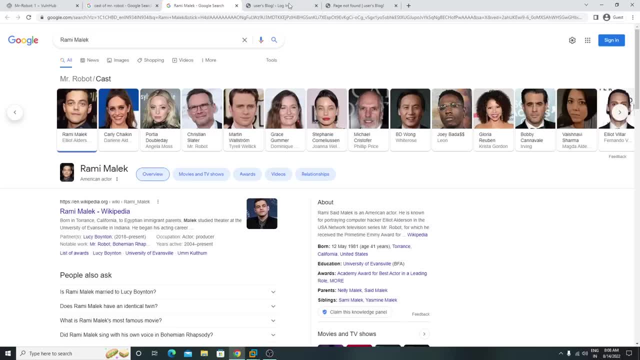 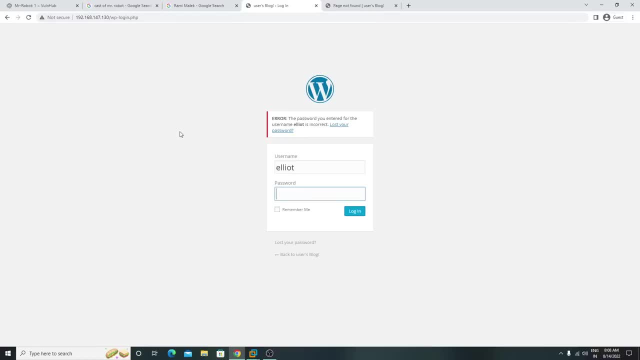 grab the username. we just grab the username with the name of Elliot. now, just see, you just need to. if you are a ethical hacker, you just you know about ethical hacking, then it is easy for you. okay, like how to create the list, or something like that, or simple. the thing is. 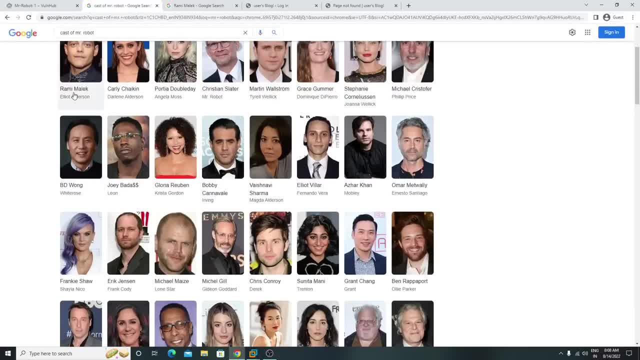 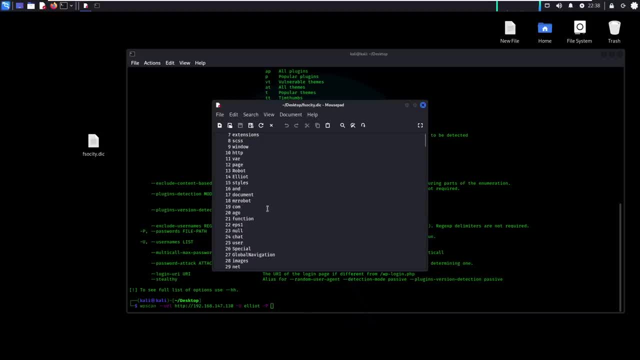 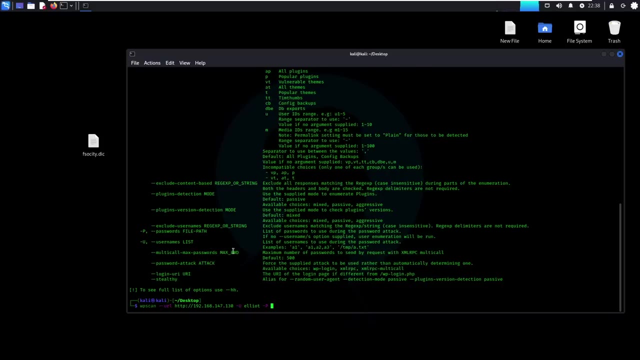 just see here is a. in the last classes we got one file right. if I open this file, just see there is a, some kind of list like x says here like false Wiki from the now Wikia or something like that. okay, so simple. I'm gonna use this as a password check. so just see, just type here: WP scan, WP scan. 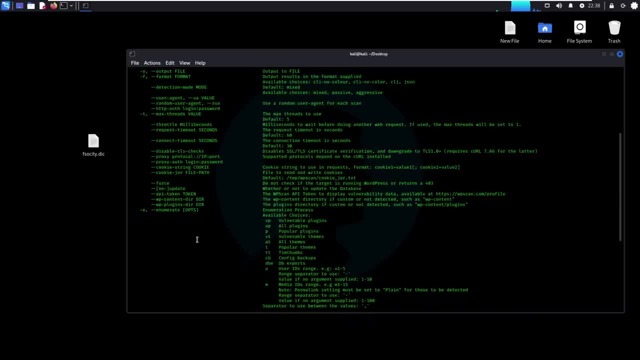 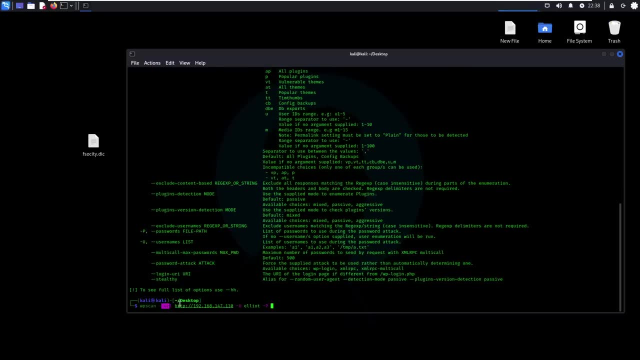 dash, dash, help, then you guys able to see this. helplines right now. wp scan dash, just url and specify the ip address of your uh web server. okay then, dash u, dash. u is nothing but username. to specify the username, right, but in my case i i know the username, okay, the username is elliot, okay, and the password i don't. 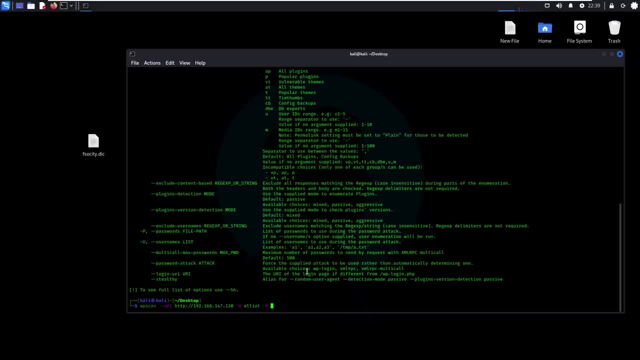 know the password, then, uh, if i don't know the password, i'm gonna use this list, okay, see, this is a ctf challenge, so that's why it's easy. but in the real world- penetration testing- you just need to use uh something. you just need to create your own list, okay. 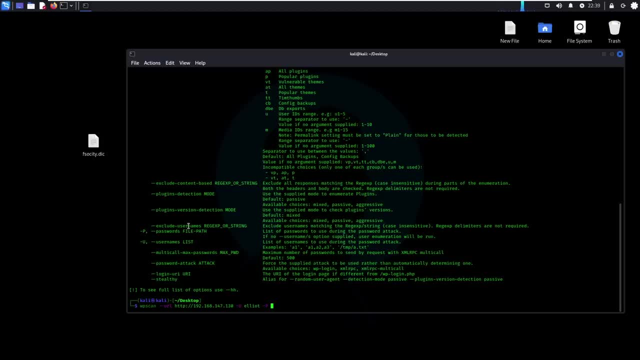 then you guys can able to perform, uh like, assume that after scanning this, after using this word list, you won't find the password, then what you, what you will do, okay, then you just need to create a manual list, okay, such as: see: there is a elliot right for elliot. 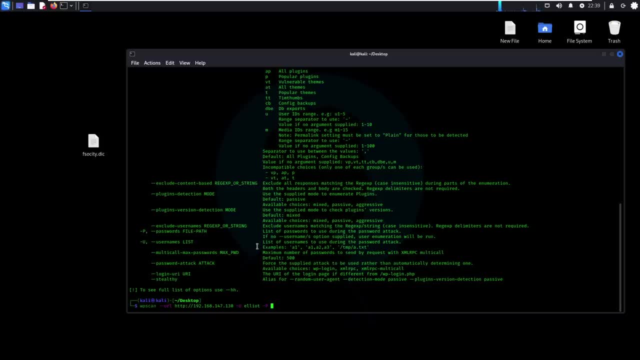 just think how the elliot password look like. okay, it's low f. first thing is the basic thinking: is Elliot password? is also Elliot? okay, like people think like this. okay, assume that if he is, if you know about technology or cyber security or something like that, then he use capital letter. assume that there is Elliot. he use L as a. 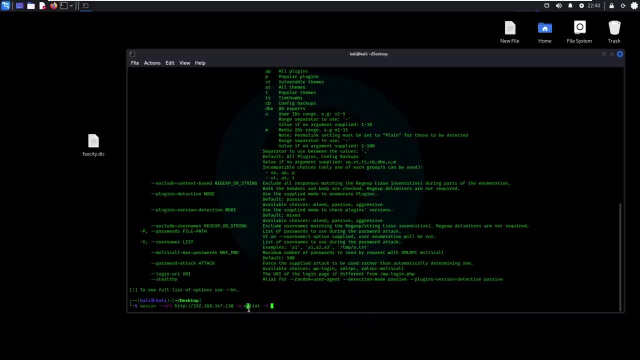 capital, I as a capital, E as a capital or something like that. then he just use the numbers as well. okay, like 6677 or something, or majority of people use the numbers as his database. assume that Elliot born in 1999. okay, he use Elliot 1999 and also he use a special characters. 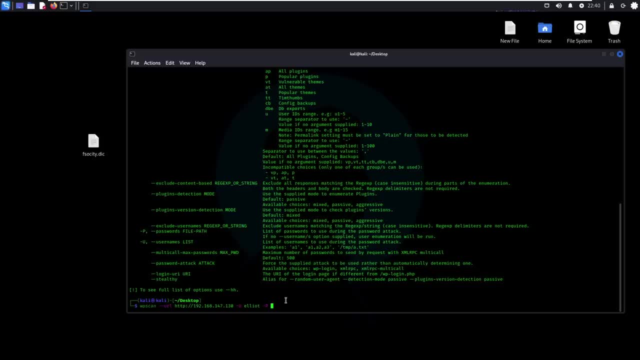 as well. okay, like something like dot. majority of people use the hash. okay, like this, this hash. they use this kind of hash star or something like that. then you just need to create a complete word list. okay, Just need to think a lot, man. you just need to think a lot, then you will create one list. 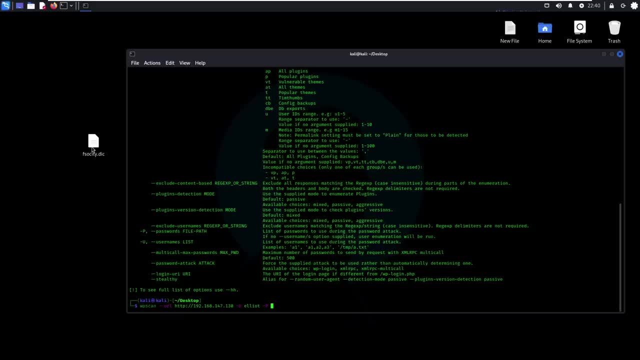 and write for brute force. okay, in my case, I got the the list from the website, like from the robottxt. I just founded this one. okay, so sometimes I told you in the last class in. sometimes what will happen means if you are scanning for if you are performing fuzzing. 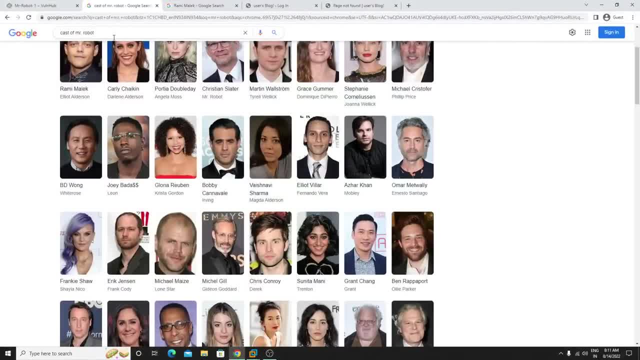 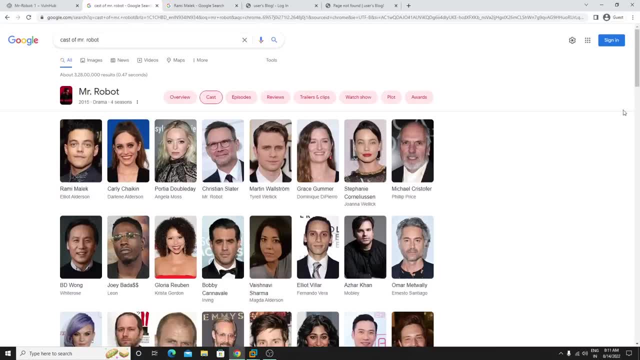 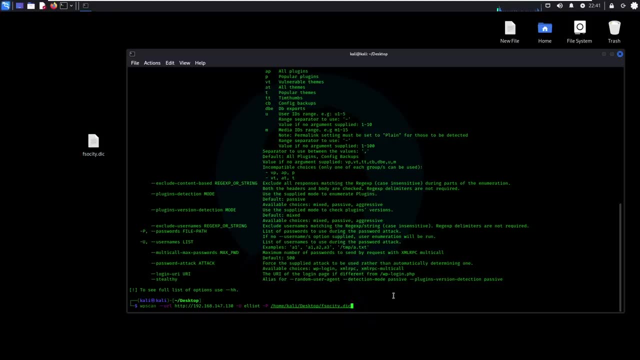 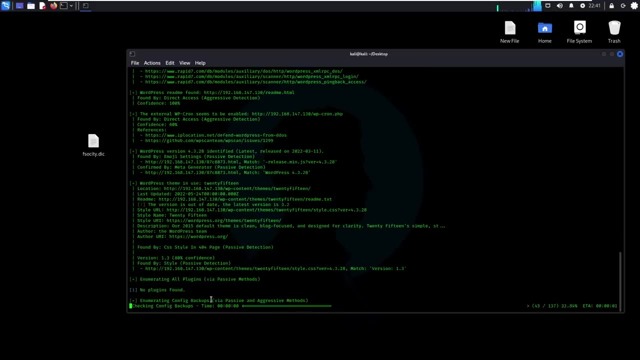 on the website. then you guys can able to see the Some file, some txt is there. okay, don't worry, I'm gonna show you practical. okay, just let me drag and drop here this file. okay, just type: enter: it will start the brute force attack. first of all, it will scan, then it will start the brute force attack. see, I told you xml rpc. 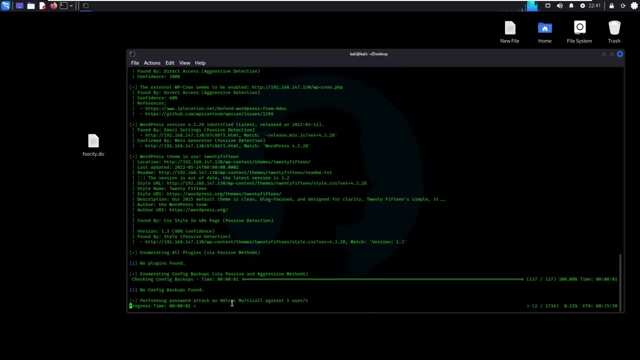 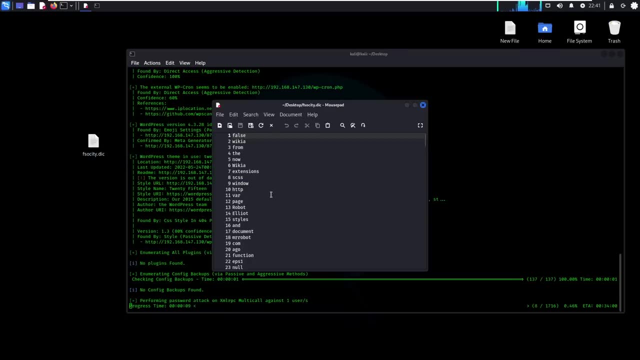 is very important in the brute force attack. just see it will taking 34 minutes right now, maybe in this website in text file. I got the xml file. I got the xml file. I got the huge amount of duplicates right like duplicate username or something like. 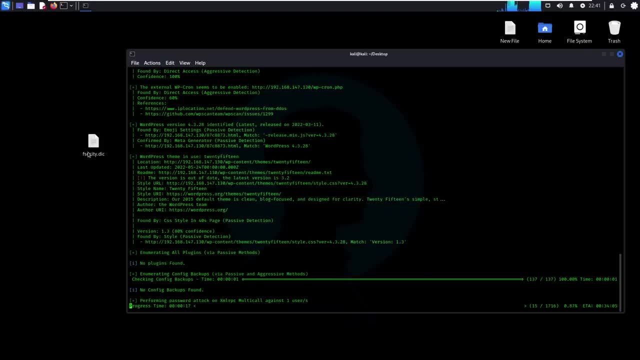 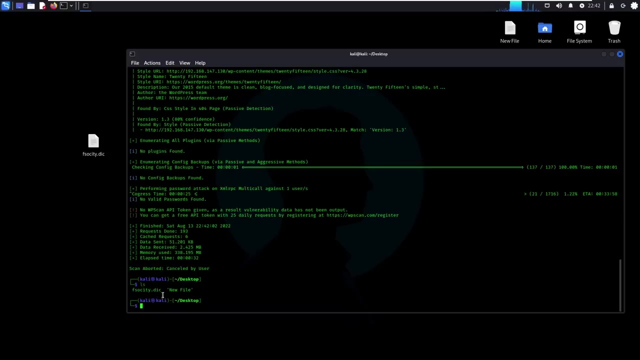 that. so first of all, let me remove the duplicate lines from this stuff like this, this file. so let me stop this attack now. simple, just type here. ls. now here you guys can able to see fsocietydirectory. right, simple, just type here in the last classes. I just told you first. 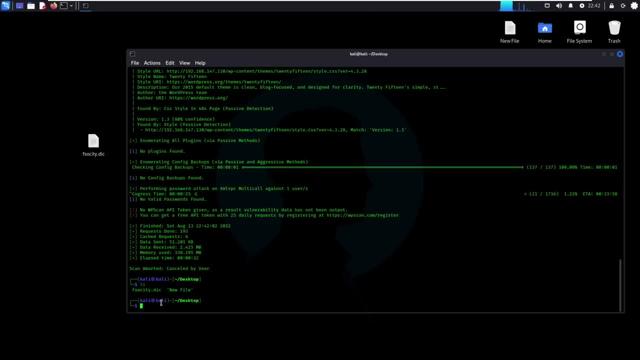 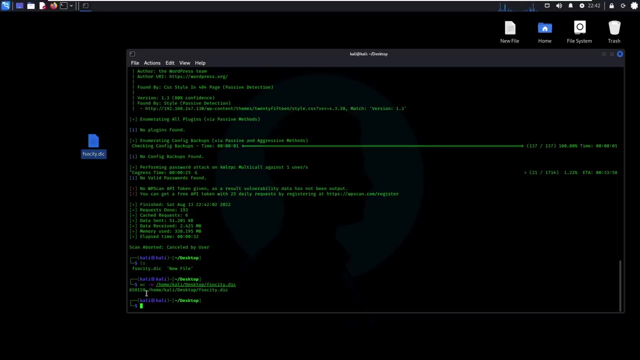 of all, let me check how many lines I have. okay, Just type wc-w. just drag and drop this one sorry words. okay, now I got see how many are there. okay, like 858159. simple, I'm gonna remove the duplicate lines from here. so to remove. 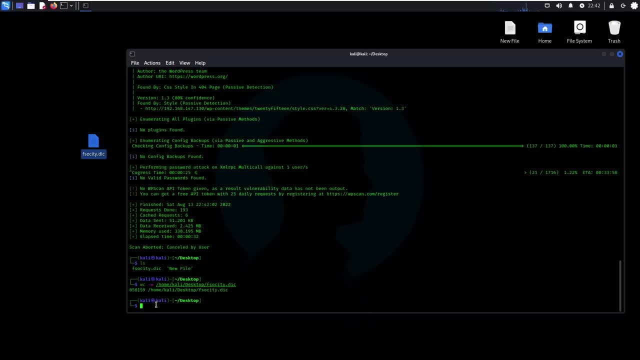 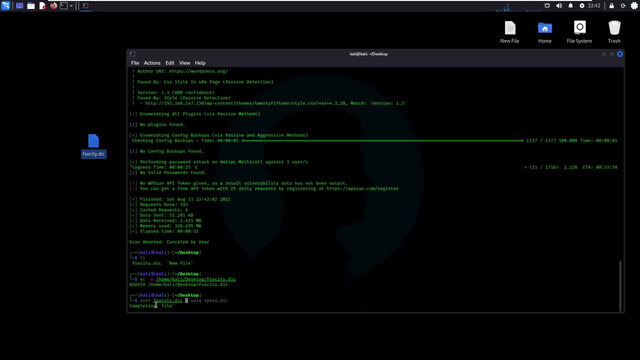 the duplicate lines I just told you in the last classes. you just need to use a future sort- fsocietydirectorydirectory- fsocietydirectory the dick. then just use a pipe, use space and use type pipe here. then there is a unit. let me give the output as a password. now I am telling: just remove the. 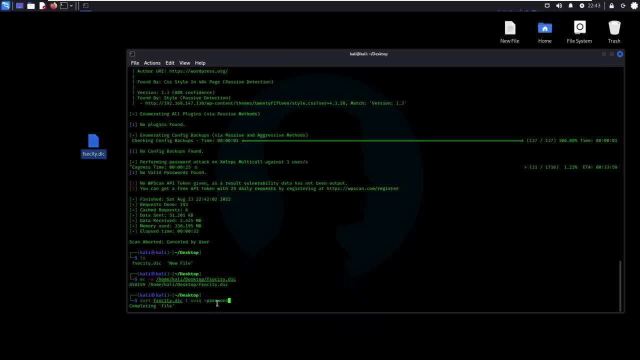 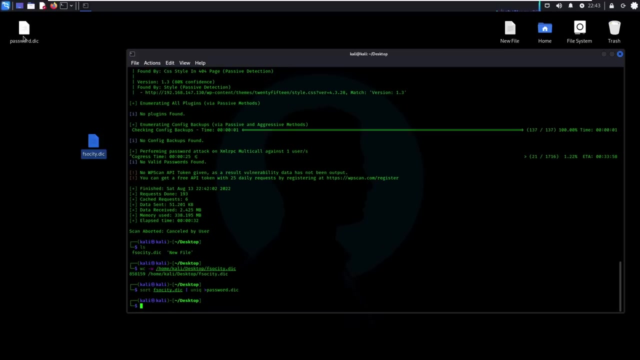 duplicate lines and give the password. you the just create a one new file with the name of password, password, password, password. I just type enter it. it's just created one on a new file. right see, here is a new file. now, simple, if I type here wc-w, if I drag and drop this one, just type enter. now, just see. 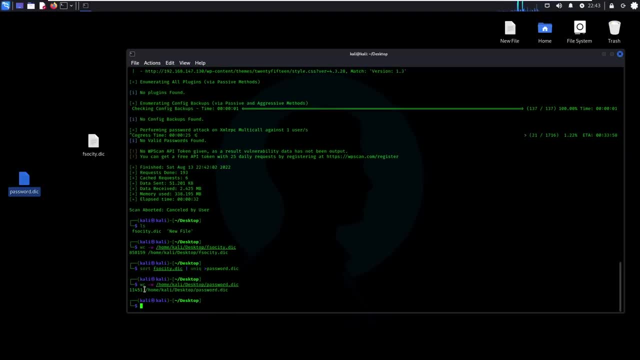 it's removed, removed, removed the all duplicate lines. okay, just see, just compare this: previous shops and the right now. okay, see, we just remove the duplicates line, duplicate lines, just perform the attack again. okay, just remove this fsociety and let me drag and drop this password. 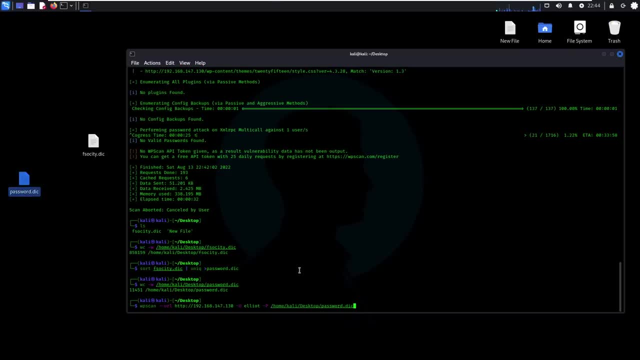 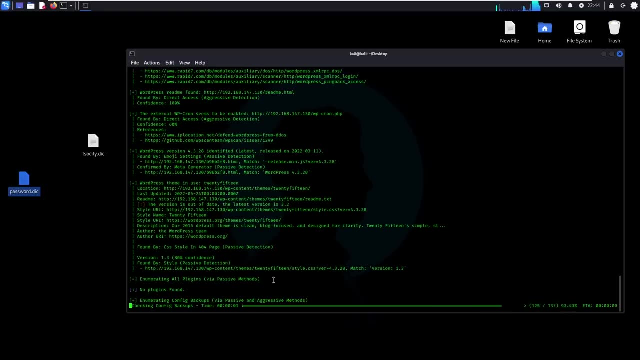 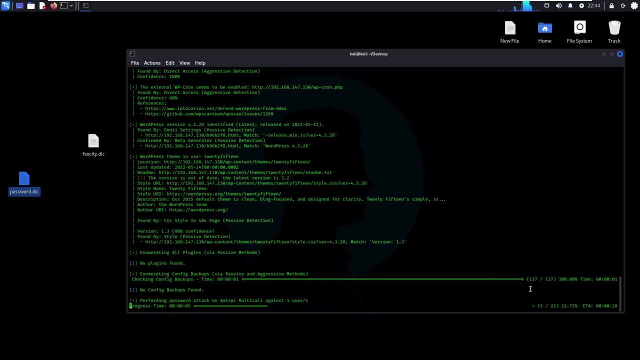 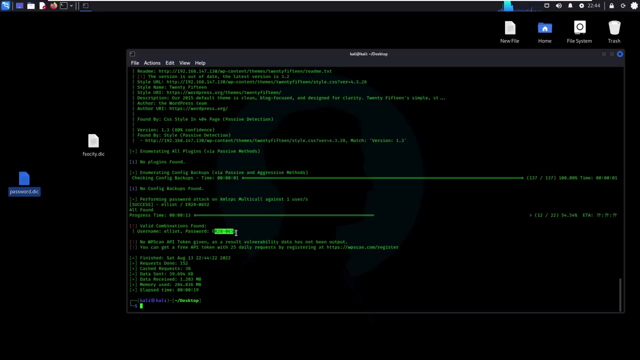 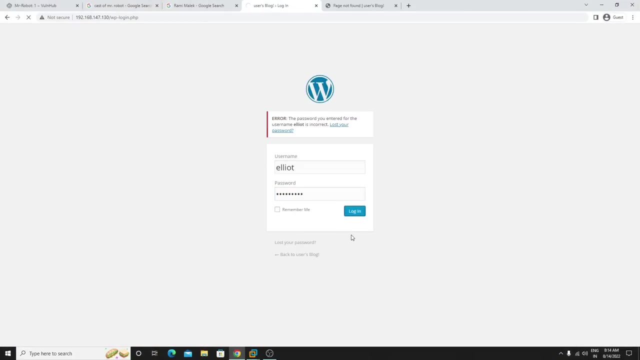 ok, just type enter here now. just see the time here: 13 seconds, or something like that. now here I got. username is Elliot and the password is this one. ok, this is the password. let me copy this and let me paste it here. right, just login now here. 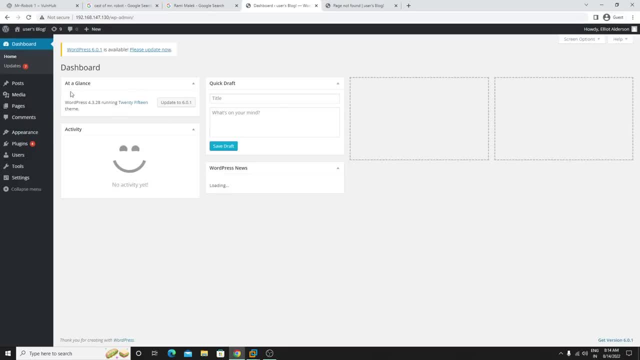 I successfully hacked this one. ok, hello everyone. how are you all in this class? I am gonna show you how to gain the shell access right. the last classes. we just hacked this wordpress website right. so simple. you just need to check, first of all, user role. ok. 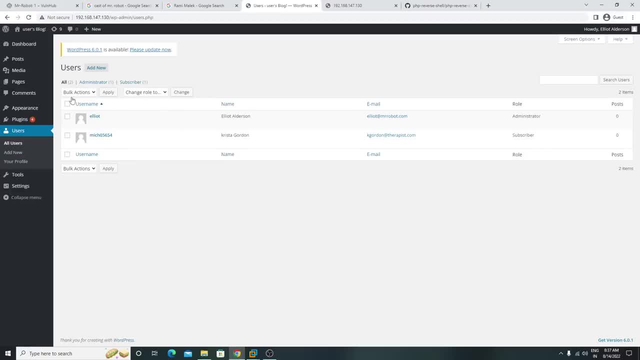 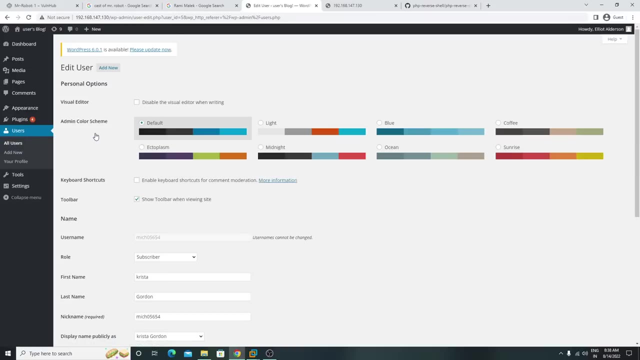 the role is administrator here. now click on the appearance editor. now assume that if there is a subscriber, then you. you can't able to see the editor option here. ok, let me open this guy. sorry I can't able to go. just click on the appearance. click on the. 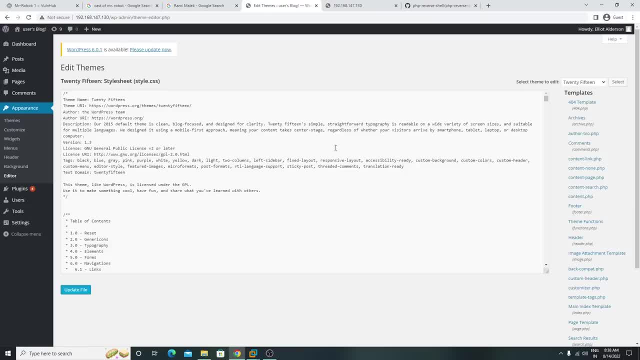 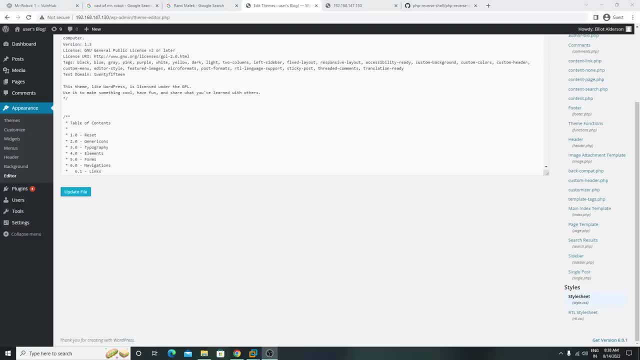 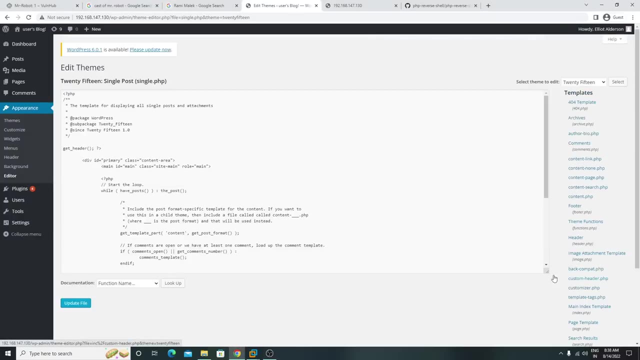 editor. right now, simple, the last classes. so you guys can able to see this one sliderphp, right sliderphp, ok. ok, we just added our dot php. sorry, single postphp, instead of here, we just added our reversible here. now in this class, let me target the 404 php. ok, this template now simple. go back. copy. 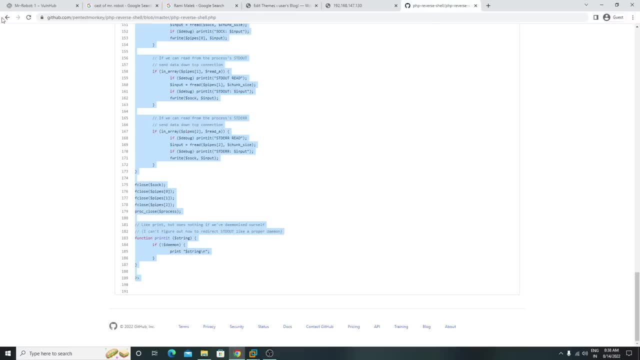 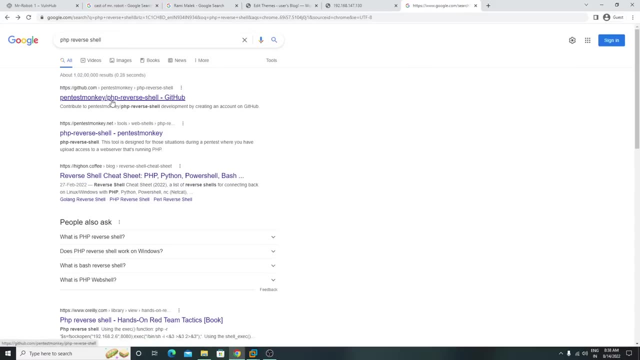 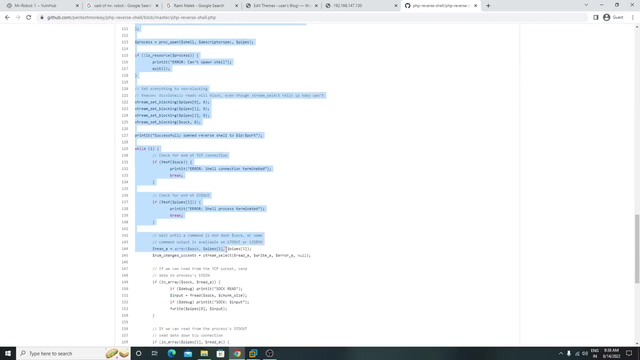 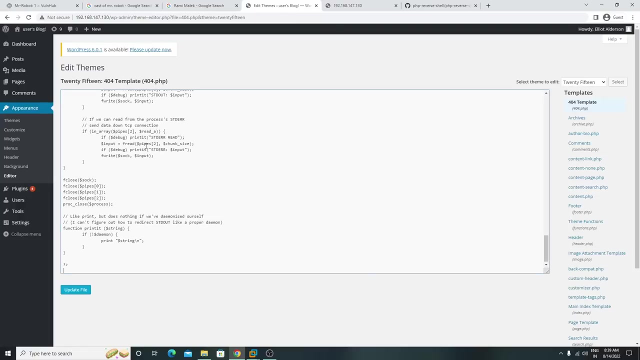 this reversal, the simple search here, php reversal, then you will get see the first link: pen test monkey. right now, simple click on the php reversal. just copy this until here. just copy it and simple paste it here right now. change the ip address of this one. okay, this one. add here your system ip address. 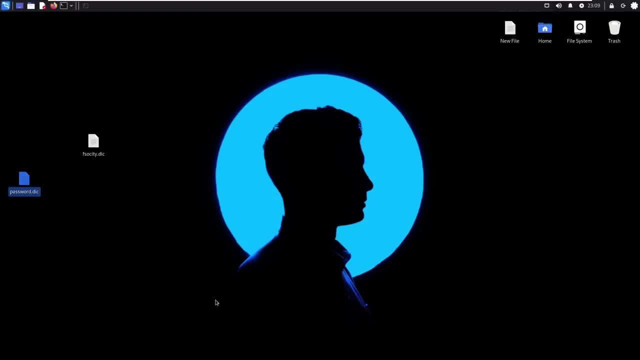 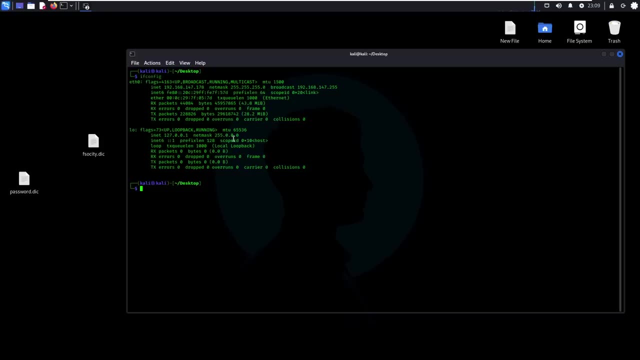 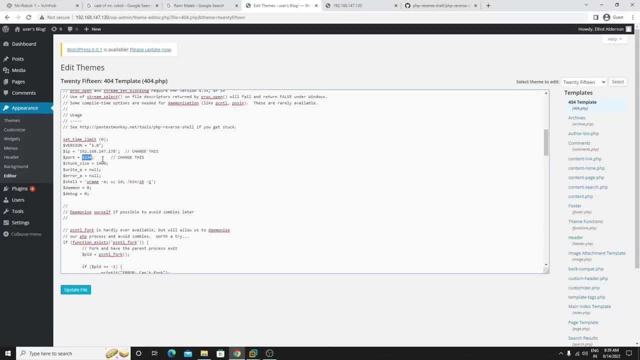 so simple. go back to your linux machine, open terminal, just type here ifconfig, and there is a ip address just copied and simple paste the ip address here. and let me listen. the port, uh symbol, just by default. one, two, three, four, just click update here. then go back on your linux machine, just type netcat. 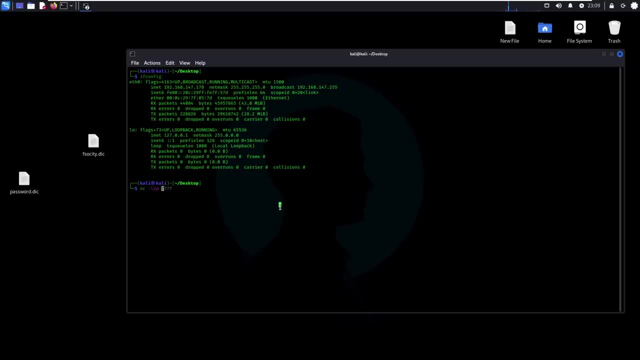 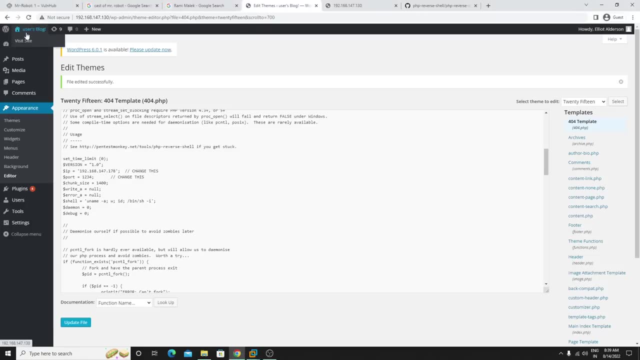 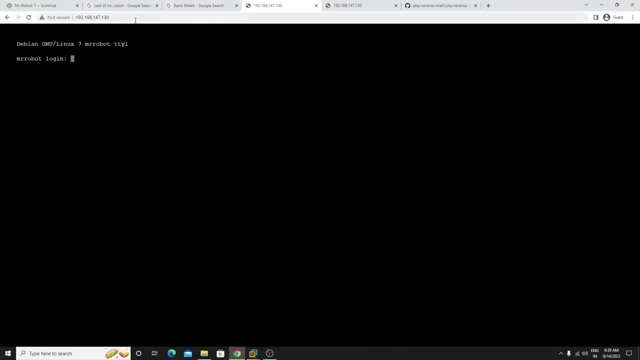 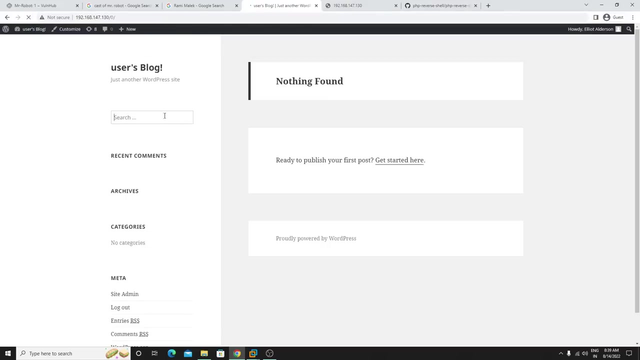 lvp. uh, just type here: one, two, three, four, just type enter to go back here. click on visit site. right, i see, here now i just need to visit this site. just type zero, forward slash zero. just type anything here. okay, see, you just need to do uh, such a search, something which doesn't have in this website, okay. 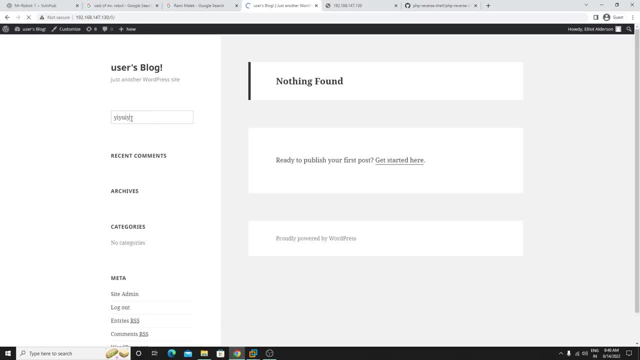 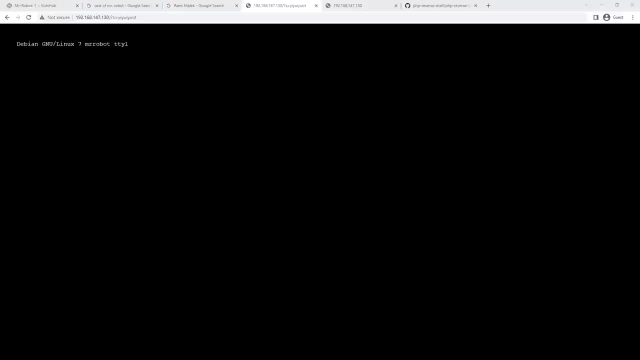 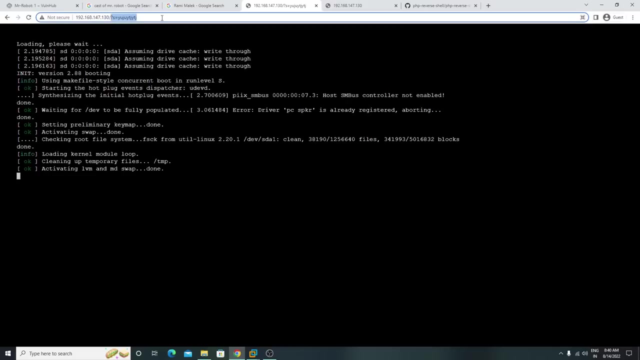 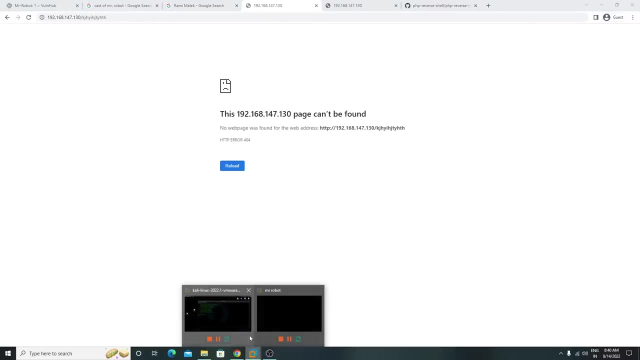 uh, let me search about something like this. just type enter here. go back now. just wait, you actually can. i don't need uh to browse myself, so i need a stalker here. let me just type fork in here. let me go back here. just type something. uh, let me do one thing here. just type anything here. okay, now, this is a can't found. okay now, let me go back here and see i got the pivot shell. simple, this is simple. let me just type it here: the들이 million plus a point number. but it will not substitute anything just because the products are not available in the right class picture. 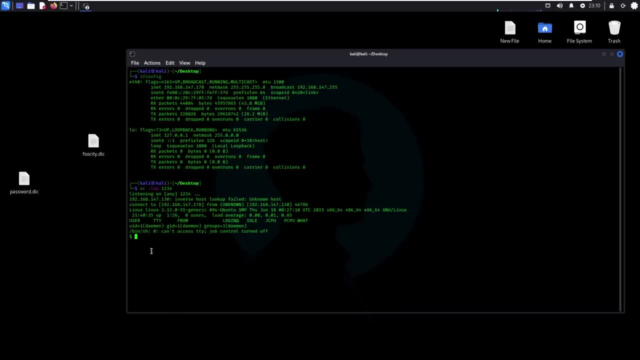 is how you guys can able to do this. okay, now you just need to stabilize this one. okay, bin forward slash bash is not a stable one. okay, you need to stabilize by using this command, Python that see: import the mod modules, such as import a module PD. why AP y dots span? okay, I'll just type: 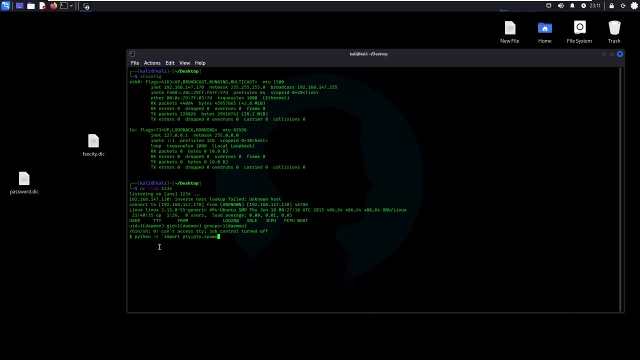 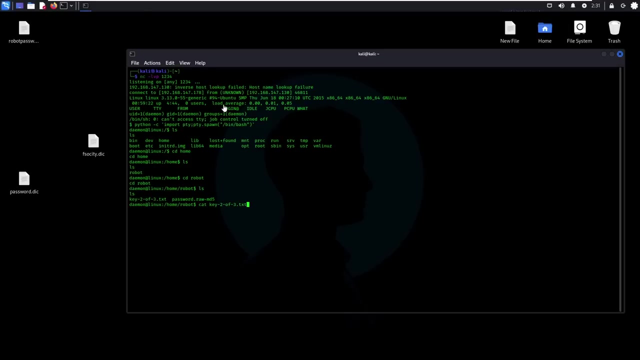 this same command there. okay, now opened. I open the bracket and just type: double code forward, slash, bin bash. sorry for good, slash and double good, close this and single. hello everyone. how are you? hope you are fine. in the last class classes we got the shell right. after getting the shell to stabilize it, you just need to type: 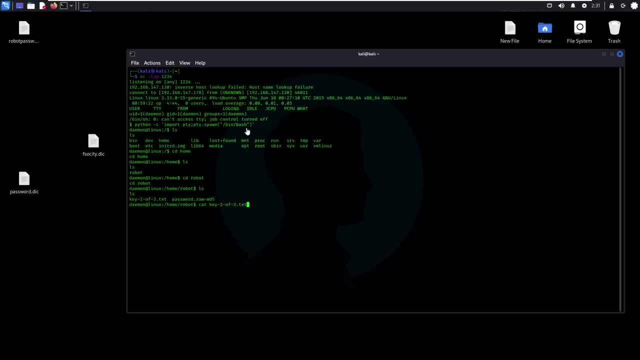 this command right after typing it. just type ls and ls. just type cd- ls again and you guys can able to see the robot folder there. okay, just move to that folder. just type cd robot and type ls. here you guys can in the robot folder. you guys can able to see key and the password right now. simple. 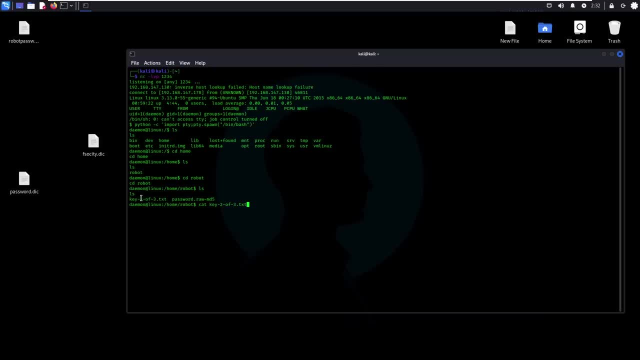 click on cat. this is a nothing, but this is our second flag, okay, uh, just type here cat key to uh this one and just type enter here. now you guys can able to see sorry guys, you guys can able to see permission denied. so to access this file, we need a pseudo permission right in this class. i'm 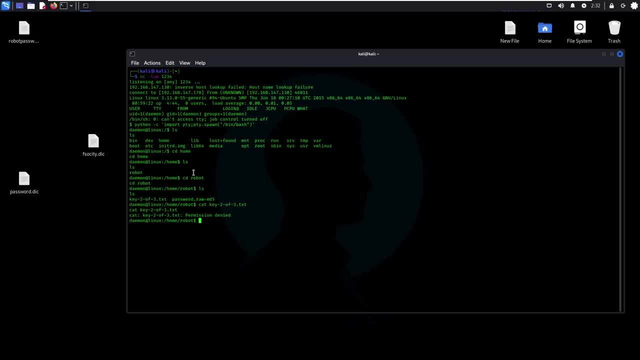 gonna show you how to privilege escalation uh to user right now. simple, uh, we can't able to see. to access this. to access this, we need a pseudo permission. right, for pseudo permission, we need a password. so simple, sorry guys. simple, uh, there is another password. is there right now? sorry, another. 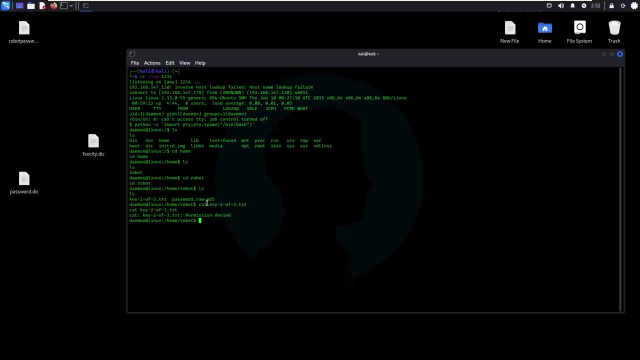 file is there. the extension is raw dash, md5. right now, simple, just type here, cat, and copy this file name and let me paste it here. now you guys can able to see the username is robot and the password is encrypted here. right now, simple, let me split the terminal. uh, create one new term. let me open one new terminal and just type here, let me. 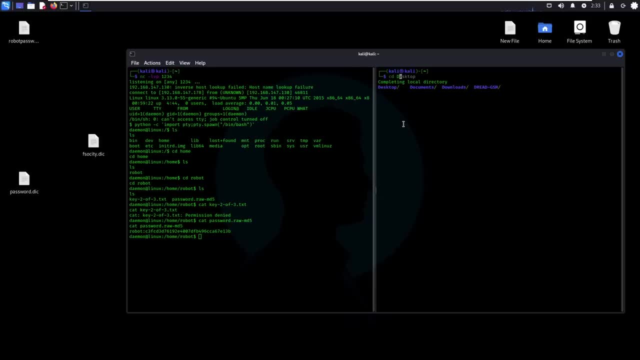 cd desktop. right now, let me do one thing: just copy this hash right and just type here nano, and let me create a file with ha, with the name of hash. okay, let me paste this string here, then just type ctrl x, y, enter. now it successfully created one hash file. this is a nothing but uh, this is our encrypted 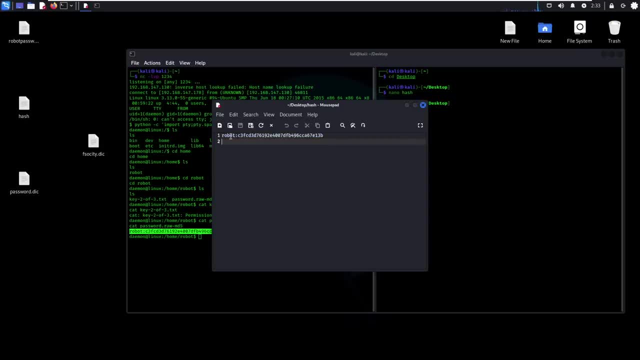 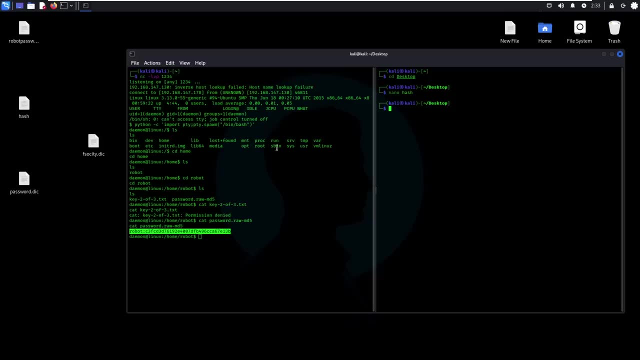 password and the username right. so simple, by using john the ripper, i'm gonna crack this one, okay, uh, i'm uh, i'm gonna crack this cat, uh, hash, okay, so just type here john and simple, just uh, just type hash here, just type enter now here. see, in john the ripper there is a one excellent future. 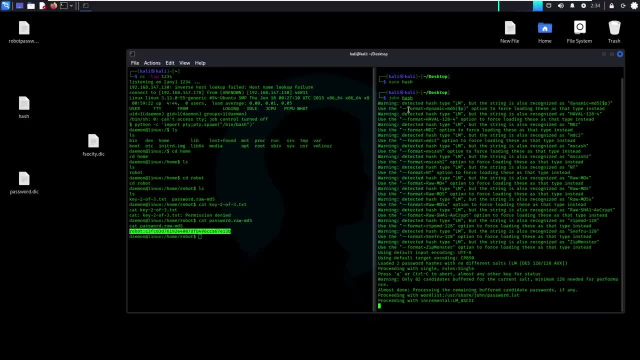 it can identify the hash, right so, but in our case we can't able to uh here. it can't able to detect the hash type. okay, let's see detected hash type lm. but the string is also recognized as dynamic md5. and here also just see the another error. how well, uh, haval and md. 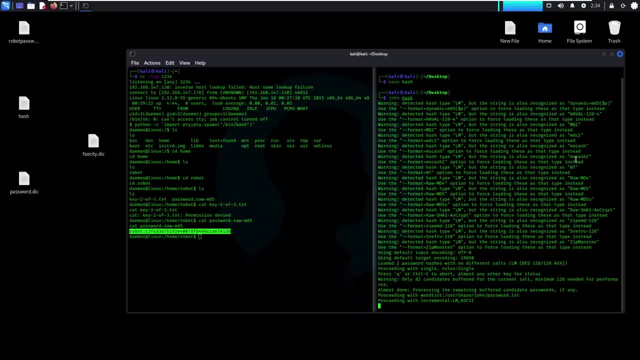 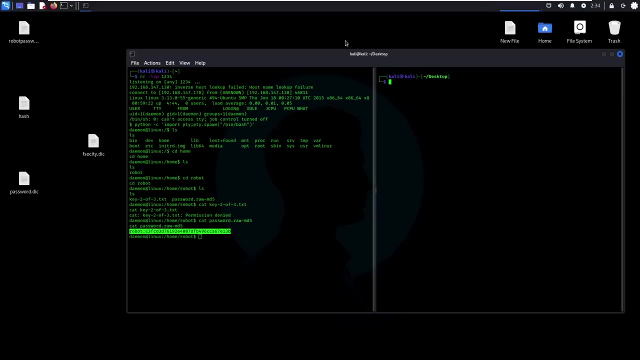 to MDC to insert. he's just recognizing each and everything, like it has little bit confusion to John the Ripper to identify this hash, okay, so that's why what we do means we gonna specify it manually, right, so simple. ctrl C to stop, just type here clear. so to clear this now, do one thing. first of all, we need to 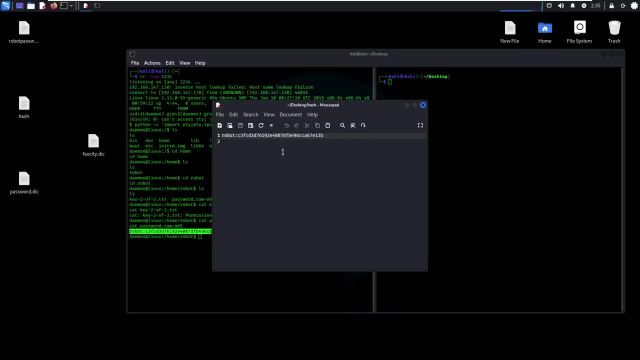 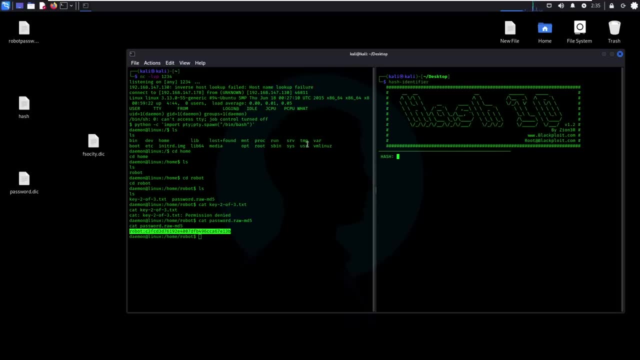 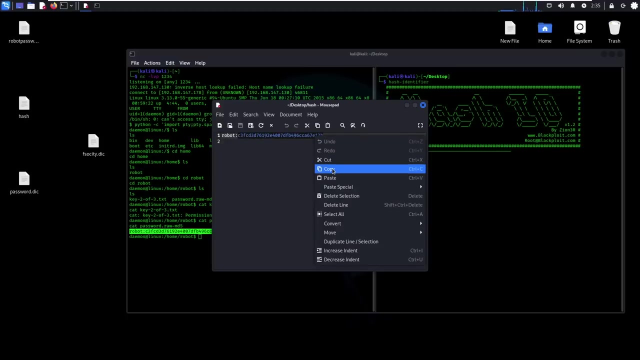 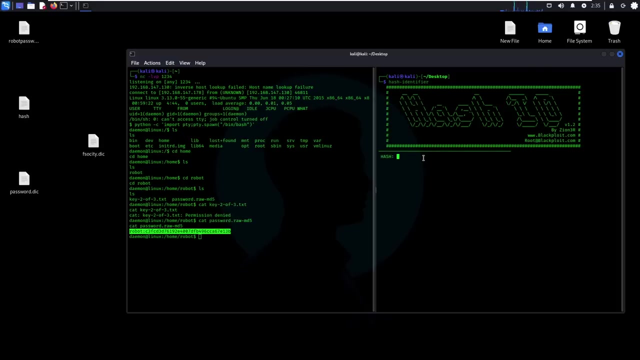 identify this hash type. okay, so identify this. you just need to type here hash identifier. right, so simple. just open this and copy this hash file. only password. okay, this one. see, this is a nothing, but this is a encrypted form. okay, so simple. what I'm gonna do? just copy it and paste it all here right after the. 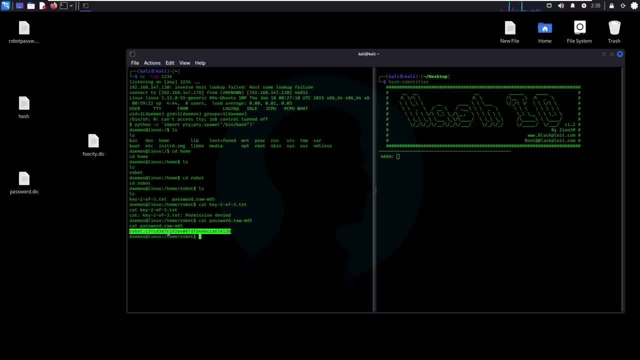 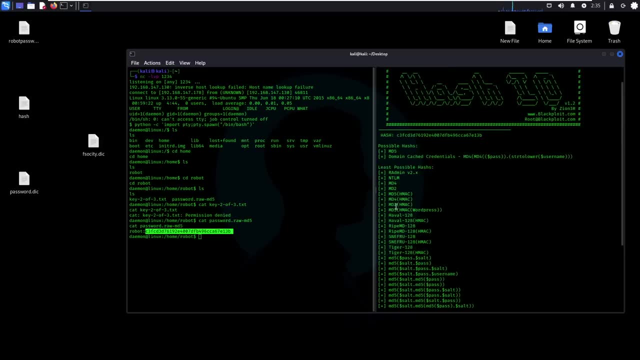 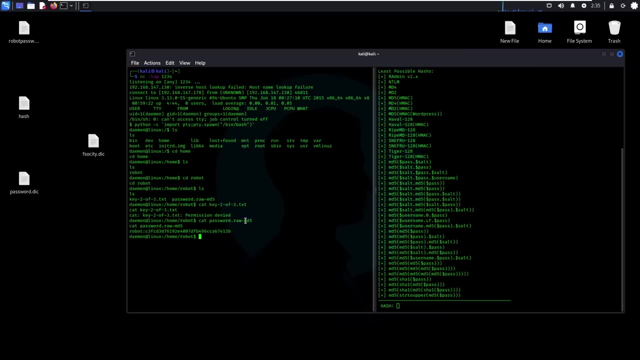 hell, man, let me copy from here, let me paste it here now. here is showing possible hashes. is MD file right? yes, there is a MD file, because here is the extension. is also a MD file right? so let me close this one, just have clear again. and then to specify the format, and John just type here: John. 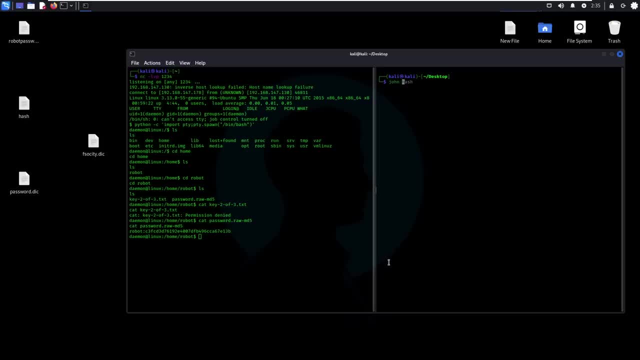 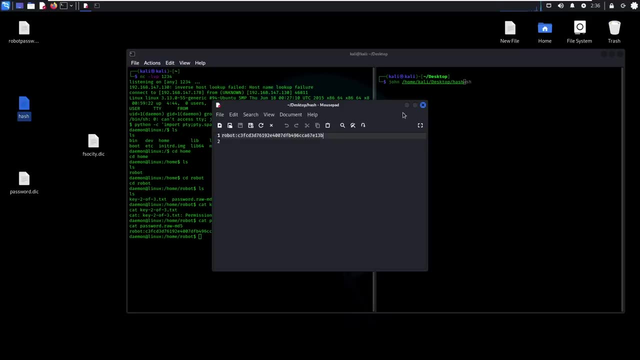 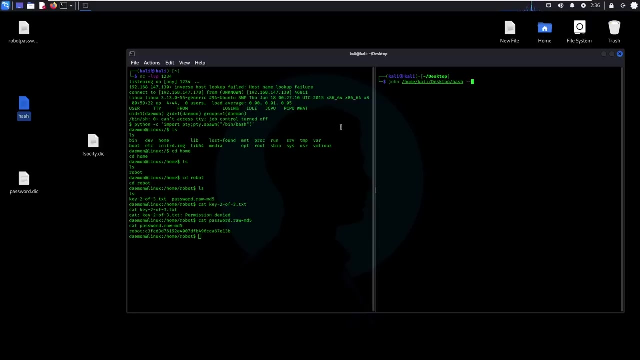 then just type here, then drag and drop your file. sorry guys, file, the hell man. okay, now simple. just type here: dash dash. format is equal raw right, dot or sorry, dash md5, Agnes, right then, dash dash. now specify the word list as well, because in the last 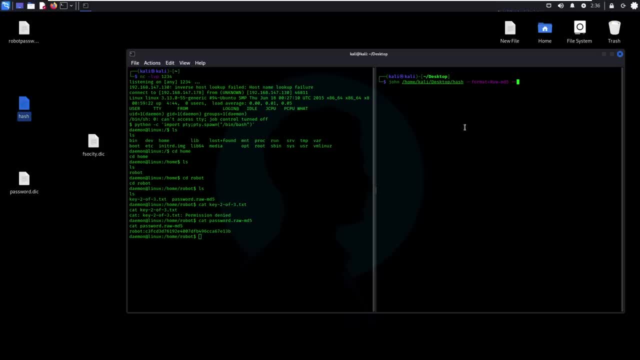 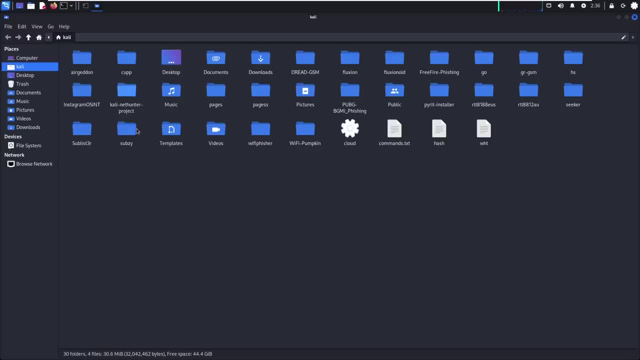 classes. we use a by default a word list of this, John, but here in this case we are using the RawQ word list. just open the folder. so here you guys can able to see. see here there is a file system, right in file system there is a user. in user there is a. 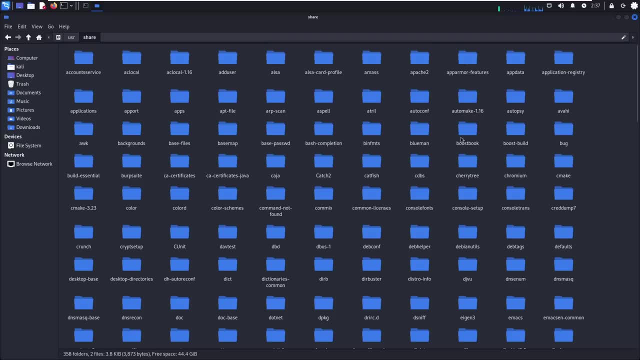 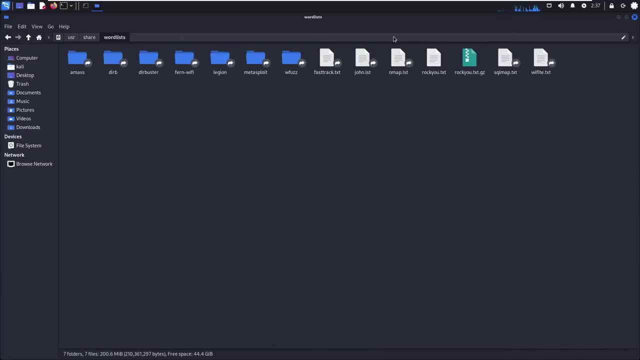 share in file system. there is a file system menu, user and share in share. just go down here you guys can able to see the folder name world list. okay, now here there is a rock you dot, txt or simple. let me do one thing, let me drag and drop this here like this: 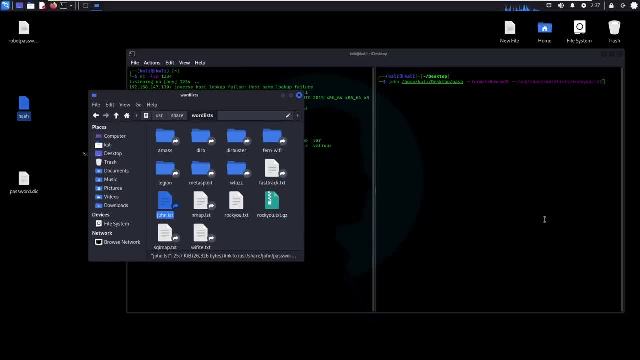 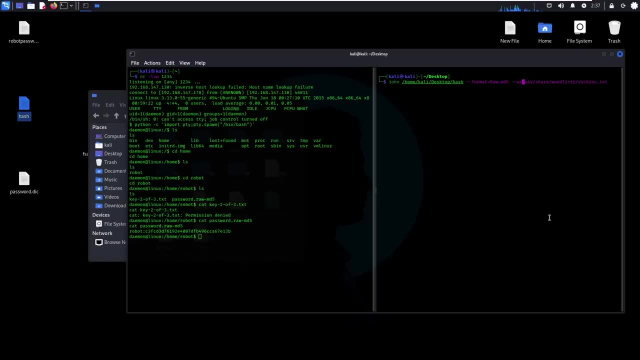 now, first of all, let me specify this world word list. okay, dash, dash, you is equal right now. simple, enter. now it's saying the no password hashes left to crack. okay, now, simple, just give the sudo permission to it. now, here you guys can able to see it successfully. 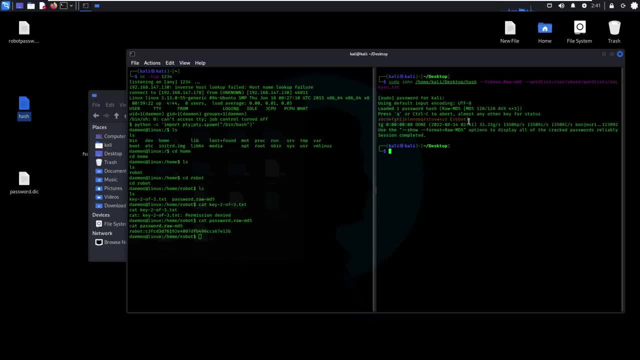 cracked our password. right now, the password is abcdefgh until a to z, right now, simple. let me copy this right now. simple. after copying this, you just need to switch the user to robot. okay, how to switch. just let me show you. just type cd now. just type here su robot. right, the password is this one. 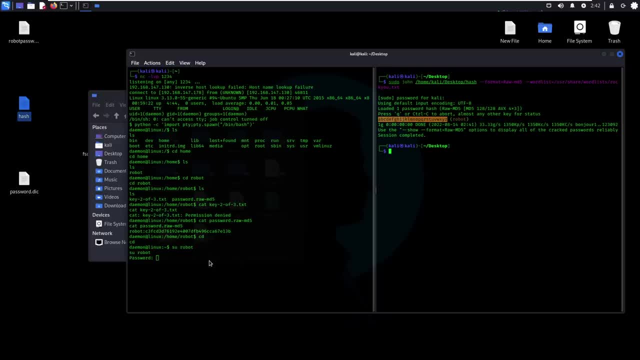 and simple. paste it here and just type enter. now i am, i am a right. now i am a robot. okay, now, simple. you just need to type here: id. now, uh, you guys can able to see. uid has a robot. okay, gid group. okay, each and everything is fine. now just type here: ls right. 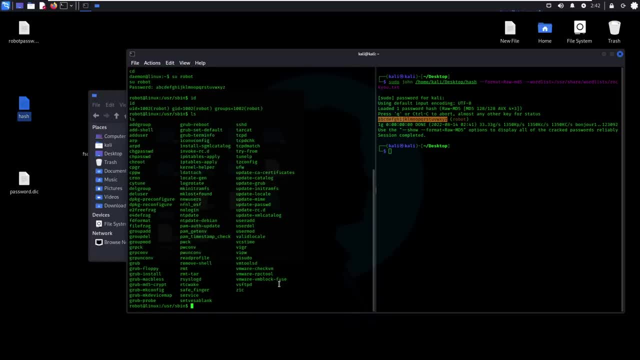 okay, now just type here cd home. no, no, no, just type cd again and just type ls. here you guys can able to see the key. okay, now just copy this and just type cat and simple paste it here. just type enter now. here you guys can able to see we successfully. 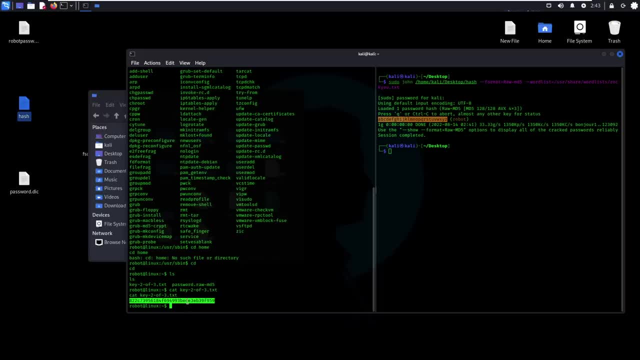 uh, completed our challenge too, okay, so in the next classes i'm gonna show you how to hack the third key as well. right now, the. the main thing, uh, we learned in the in this class is: we just cracked the password by using john the reaper and. 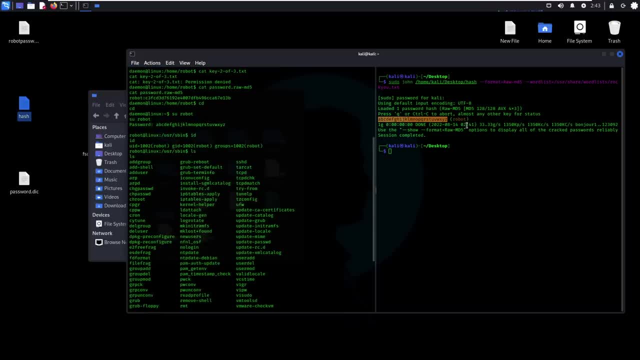 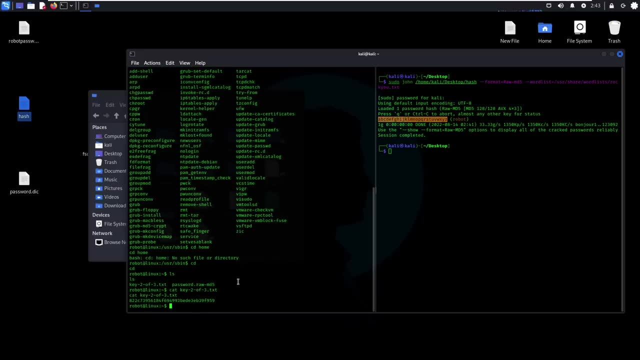 that's it right. after cracking it, we're gonna switch. we learn about how to switch the user as well. like it is a basic things, right, so just practice it. okay. if you're not getting this one, then practice it. you'll get it, okay. uh, like you will learn a lot if you practice this all. 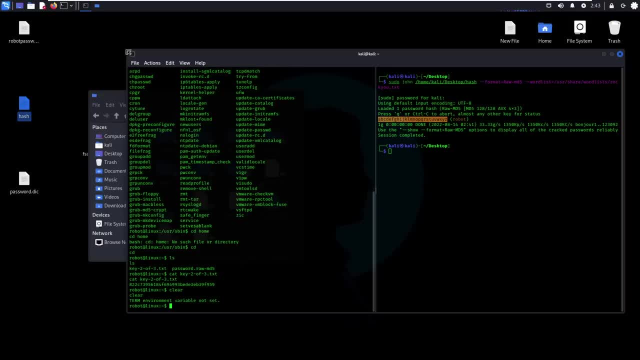 stuff right, thank you, having nice day. in the next classes i'm going to show you, uh, how to change this robot to root user. okay, like a privilege escalation topic, okay, uh, hoping this can help you guys enjoy this classes. thank you, have a nice day. hello everyone. how are you all in the last? 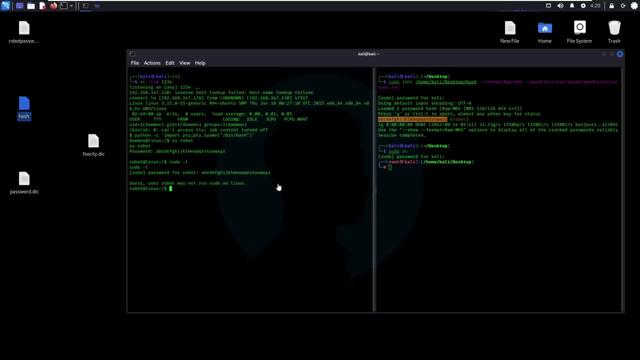 classes. we captured the flag right, the second flag. just see, in this class i'm gonna show you how to perform privilege escalations to grab the that flag right. so just type sudo l. you guys can able to see. sorry, user robot may not run sudo on linux, so here i can't able to run as a sudo, right. 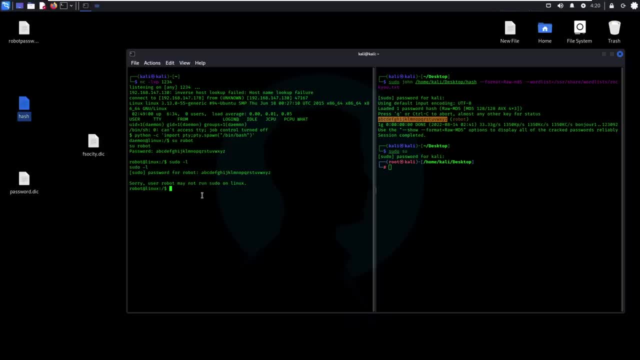 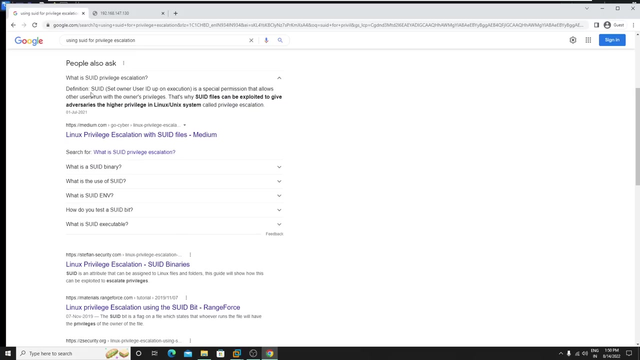 so simple thing is i just need to search for- sorry guys, i need to search for uid permissions, right? what is uid? let me tell you uid definition: su. uh. suid set owner user id upon execution. it's a special permissions permission that allows other user run with the owner privileges that. 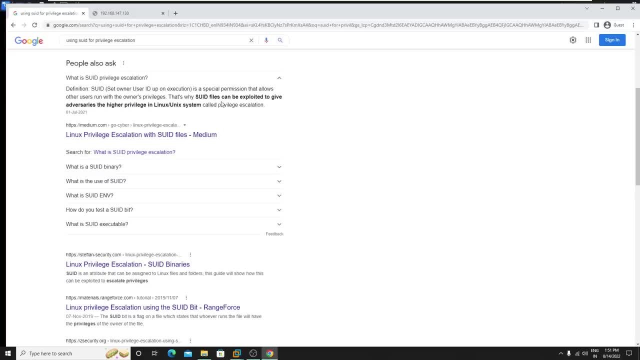 that's why suid file can be exploited to give adversaries the higher privi, uh privileges in linux, unix systems called privilege escalation. just let me tell you see, special permission that allows other user run with the owner privileges. right, so in our case we are a normal user. okay, we don't have any super. 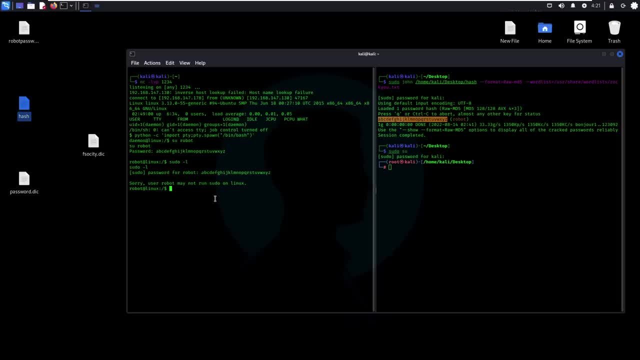 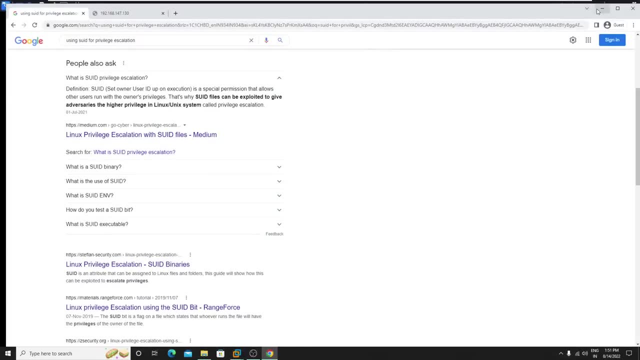 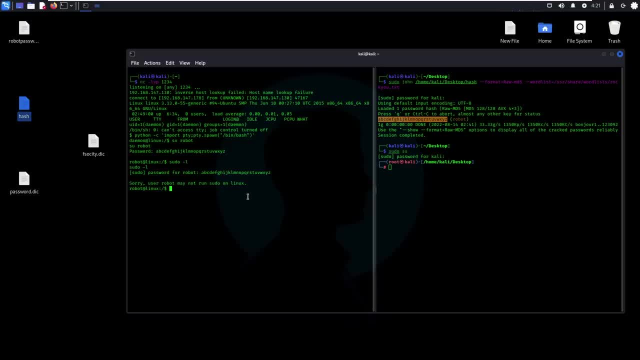 practically right. let's see, the thing is we just need to find a suid files. okay, to find it, just type here: find, uh, in entire linux. uh, like entire linux directory. uh, we just need to find it. okay, just type: find and forward: slash in entire linux. okay, i just need to find each and. 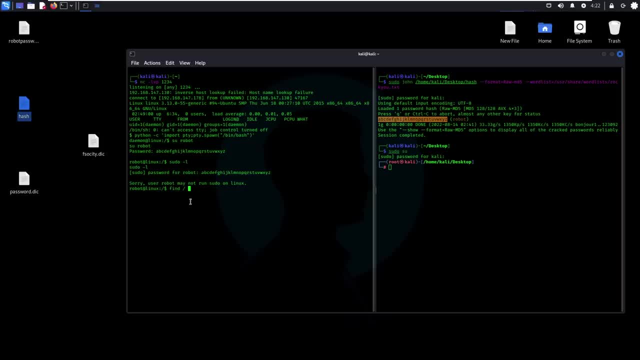 every uh folder. right, just type forward slash and then just type here: dash p permissions. uh, dash p is a nothing. uh, dash p? e? r m is a nothing, but it's a short form of a permission, right? so simple. just type here: dash u is equal. yes, right, so it's a nothing but set uid files. 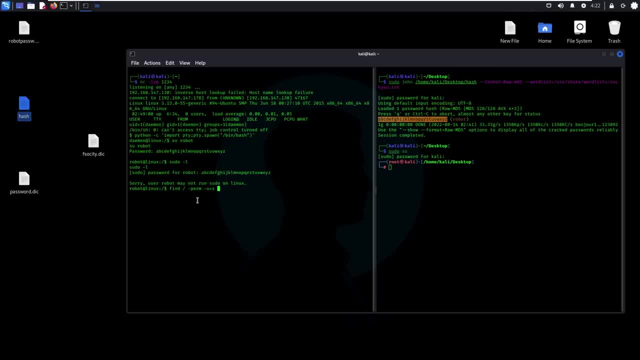 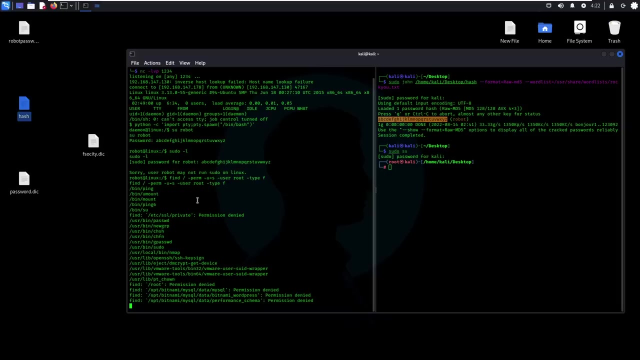 okay, dash user. user must be root. okay, now just type: must be file. now search it. so here you guys can able to find the applications, uh, the files which have uid permission, right, so it will take a while to find it. so it will take a while to find it. 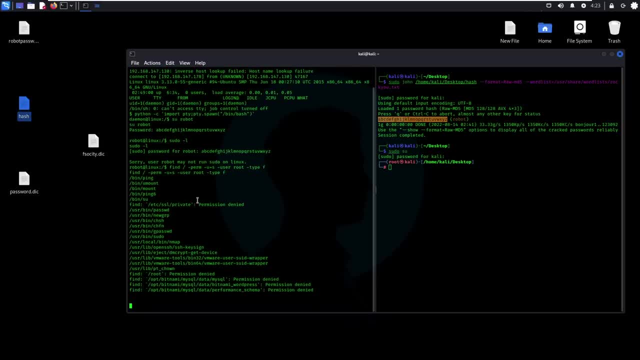 some time to get this one. just wait. see, i just told you how to uh remove this kind of errors, uh, this lines, okay, like this errors. just let me just read. i'm gonna show you practically now. just see, i got a huge files with the errors, just. 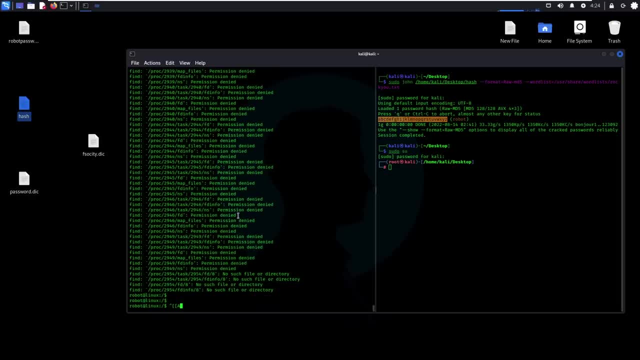 just simple type the same command again. okay, the same command. find the files in entire linux file. dash permission must be set. user: uh, set uid. uid is nothing but u. okay, this is a short form of uid is equal to set. this is uh like this. okay, set uid. 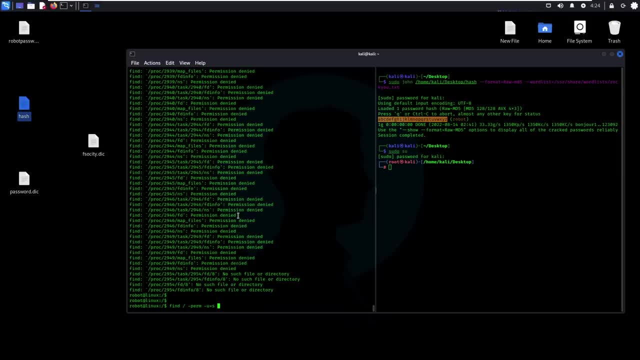 now just type dash user root. root. user must be root and the type must be file. then just type here: the errors will be denoted by two, right, so just type: uh two forward slash, dev, forward slash, null. just move this to null. uh see, i just explained you in the last classes, right, okay, just type: enter here now. here you guys can. 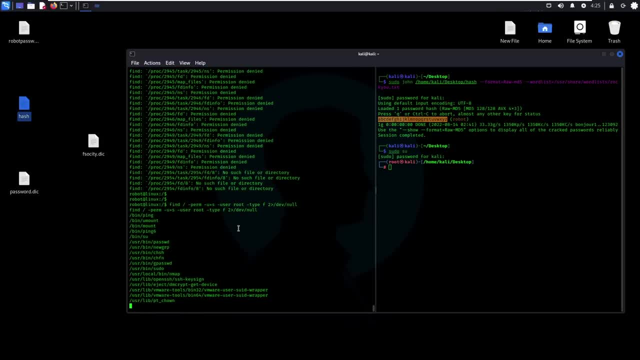 able to see the files without errors right now. just see here. see, you just need to interact with any application. okay, there is a nmap. nmap is a uh, just see, by using nmap, you guys can able to interact with. uh, just let me show you practically right now. just see here. 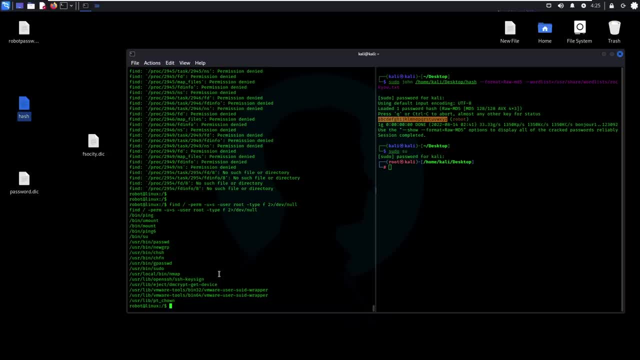 to interact with the files. you guys can able to see the files without errors right now. just interact with nmap. just type nmap, dash, dash, interact, interact you and just type enter. now here you guys can able to see: i just interacted, uh, interactive with the, interacted with pipeline map. okay, now just type here: 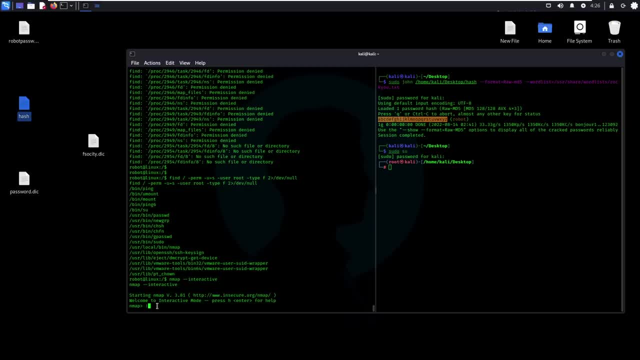 shibang dot sh. okay, i'll just. uh, see, i got the shell. it's like a shell, right, it's a shell. okay now. just type id. here you guys can able to see: the id is root. right, uid is root. so simple. just do one thing: just type ls here now. here you guys. 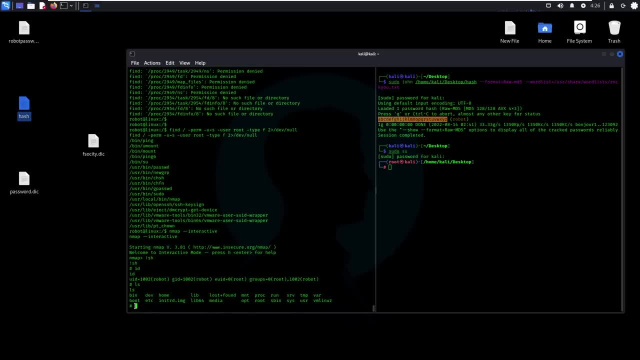 can able to see. uh, this, uh, the things are there right. uh, just type here, let me access this folder. just type root. just type cd, forward slash, root, forward slash. just type enter. just type ls here. see here, sorry guys, here you guys can able to see the key 3. just type here: cat. 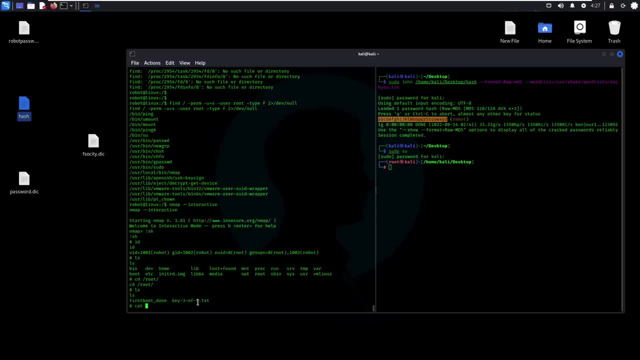 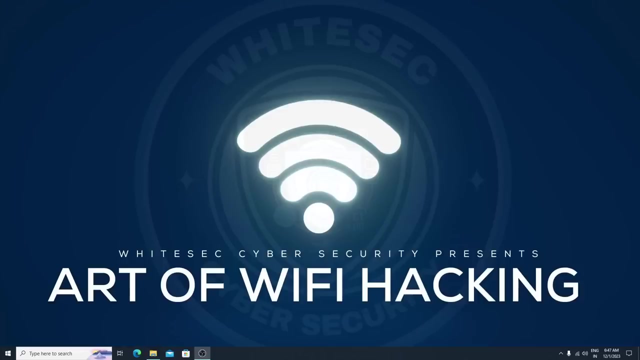 key. dash 3, dash off. dash 3 again. dash 3 again, dot txt. just type enter. now here you. hello everyone, hope you are fine. in this training you will learn how you can able to perform wi-fi penetration testing or wi-fi hacking. see, this training is completely for beginners if you don't have knowledge about wi-fi hacking. 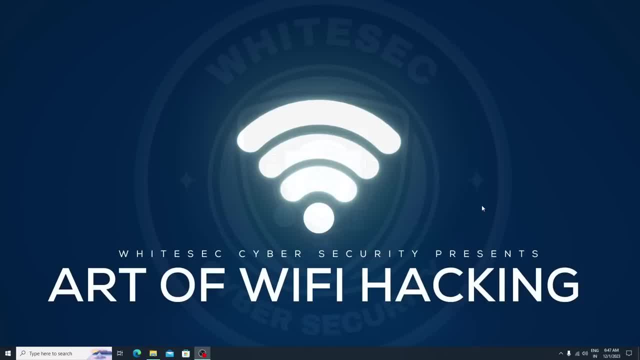 then this training is for you. now let me tell you: you just need to follow me. okay, assume that. if you are not getting any theory, uh, if you are getting any kind of confusion, then what you need to do? simple: just do the follow the same process which i am doing here. 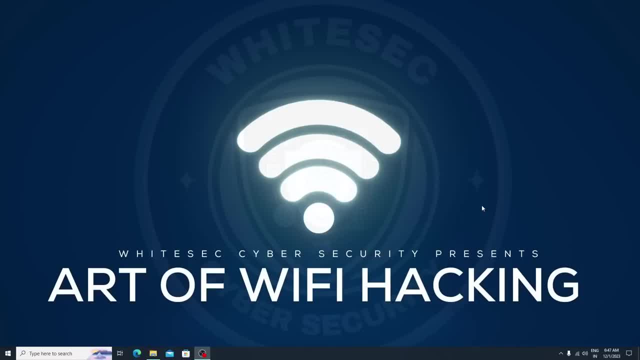 okay, like assume that if i am executing any command, then execute the same command in your linux machine. see, i just covered how you guys can able to install the linux each and everything. again i am saying uh, in previous trainings also i just told you that. just try to watch. 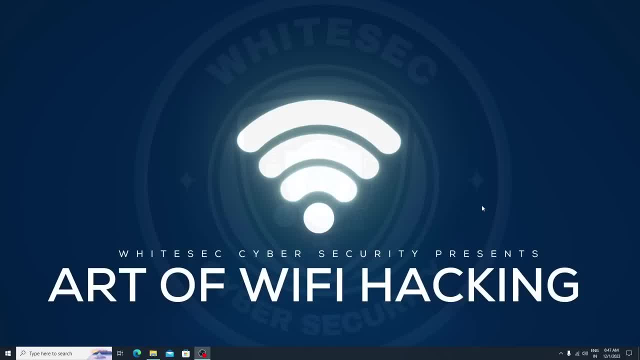 the trainings in 1.3 or 1.5 x because, due to my slang, maybe sometimes i am slow, maybe sometimes i am okay at a time. the thing is the the good way to complete this training is: just try to watch it in 1.3 or 1.5 x. now let's см mouve her for let's just write it in the first training again. let's do that right now. this is an amazing training- 1.3 or 1.5 x- because, due to my sl53, maybe sometimes i'm slow, maybe sometimes i'm fast, okay other times. the thing is, uh, the good way to complete this training is first try to watch it in 1.3 or 1.5 and see how it goes. 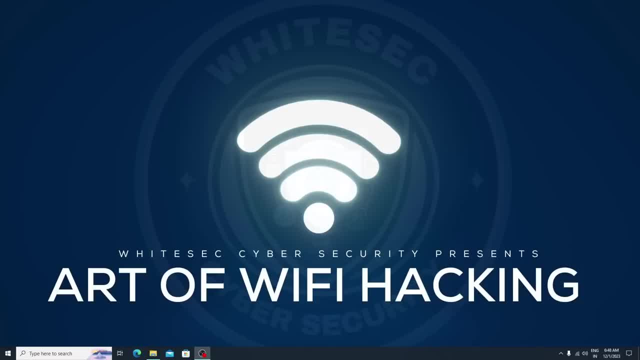 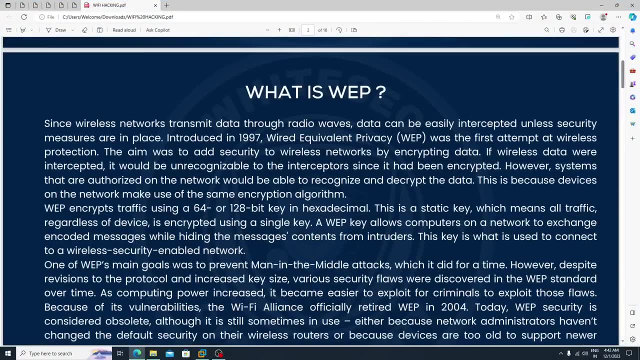 hope you guys enjoy this training. thank you, have a nice day. in this class we are learning about what is WEP, since wireless network transmit data through radio waves. data can be easily intercepted, like anyone can able to see it unless security measure are in place. introduced in 1997, wide equivalent privacy, which is known as a WEP. WEP full form is what here? wide equivalent, 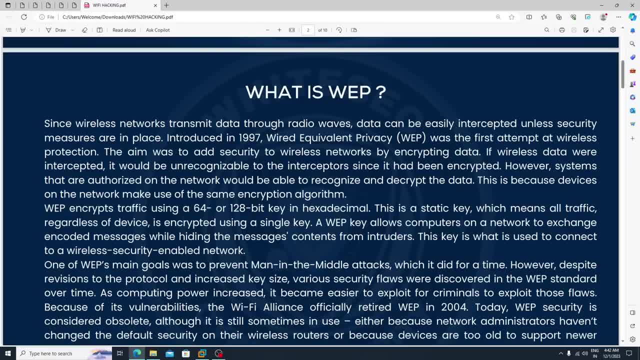 privacy was a first attempt at wireless protection. this see before this one. there is a no security in the wireless network. ok, this the thing which you need to remember. the aim was to add security to wireless network by encrypting a data. this is the thing if wireless data 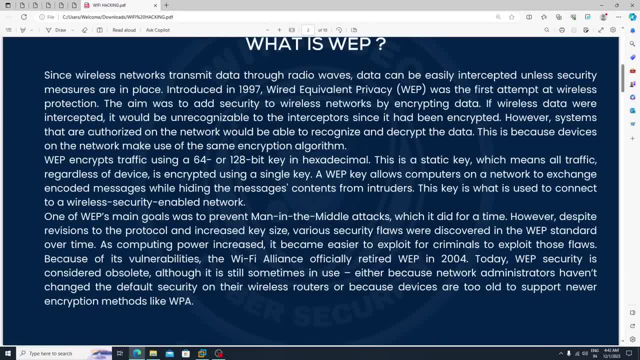 were intercepted like a. if anyone try to read it, it would be unrecognizable to the interceptors, since it has been encrypted. now the thing is anyone can able to see the data anyway, can able to capture the data, but the thing is they can't able to read it. this is the thing. 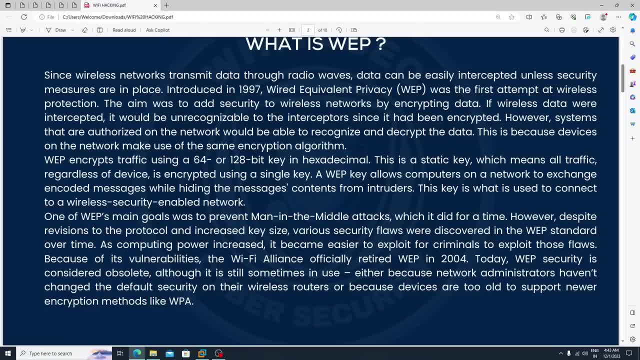 they can able to capture it, but they can't able to see the data. what is there? okay, or something like that. the data is completely encrypted. if the wireless data were intercepted, see, it would be unrecognized to interceptor. since it it has been encrypted. however, system data are authorized on. 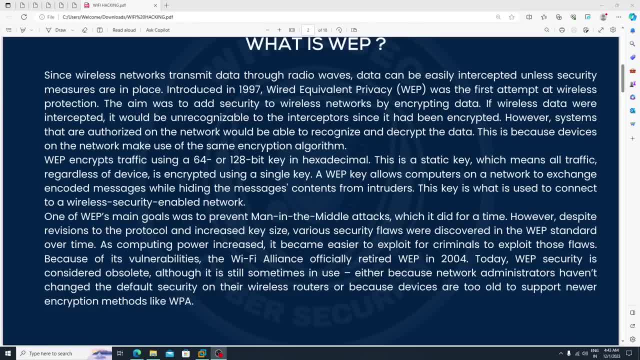 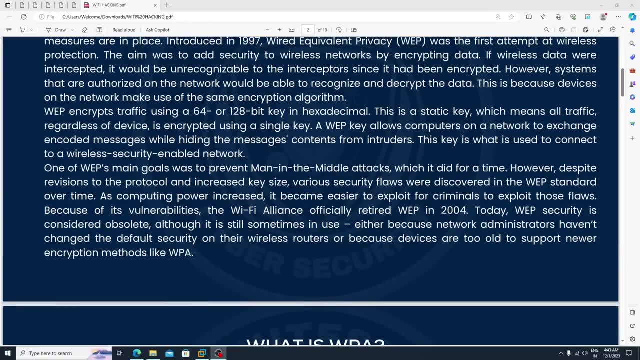 the network would be able to recognize and decrypt the data. this this is because device on the network make use of same encryption algorithm. see here: WEP encrypts traffic using a 64 or 128 bit key in hexadecimal. this is a static key, which means all traffic, regardless of device, is encrypted. 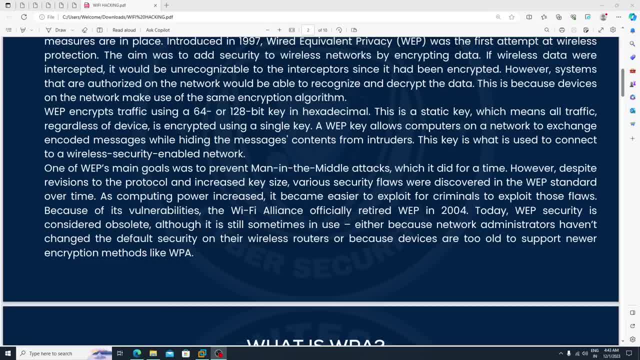 using a single key. this is a thing. a WEP key allows computer on a network to exchange a encoded message, while hiding the messages contains front-end and back-end information on the network, which means all traffic is encrypted from intruder. this key is what is the intruders here? intruders is nothing but hackers- a black hat. 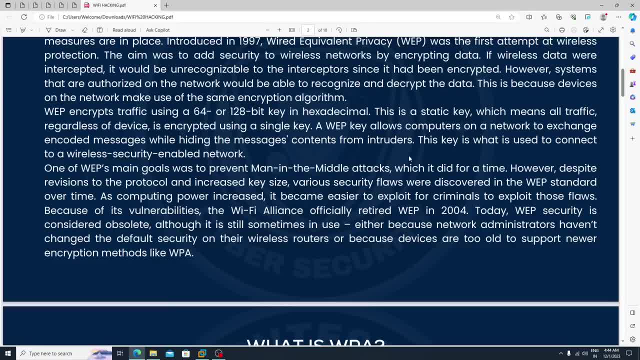 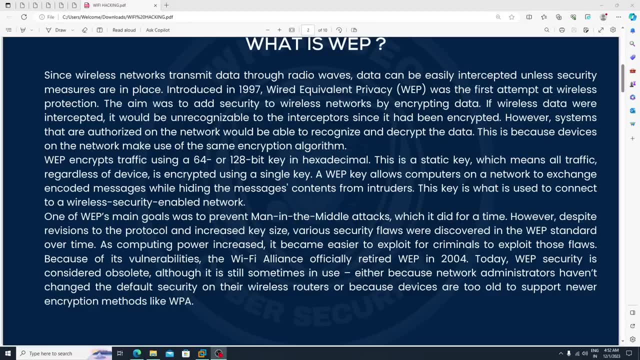 hackers- you can also say it as a black hat hackers. this key is what is used to connect to a wireless security enabled network. one of WPS main goal was to prevent man-in-the-middle attacks, which it did for a time, however, despite. over time, as computing power increased, it become easier to 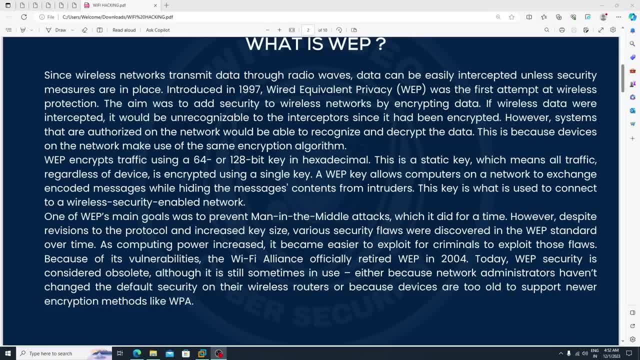 exploit, for criminals to exploit those flaws. in a simple words, WEP become a vulnerable. it is very easy to hack WEP network. mostly people won't use it. assume that if the router is old, okay, here you guys can able to see the point: the default security. just just read it. okay, the Wi-Fi. Ali aliens officially retired WEP in 2004. 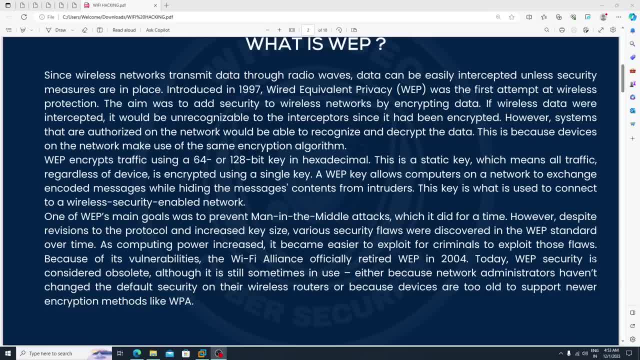 today WEP security is considered absolute all through. it is still sometimes in use okay, either because network administrator haven't changed the default security on their wireless router or because device are too old to support newer encryption method like WPA. see, sometimes what will happen means the router won't support the new encryption there by default. the 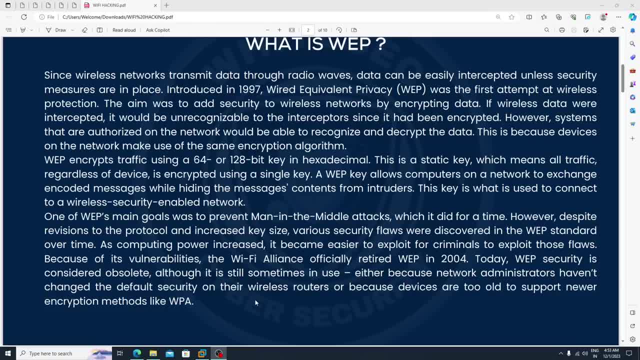 the router will run on WEP network only okay, like mostly you guys can able to see this thing. this thing's in old WEP network- only like mostly you guys can able to see this thing. this thing's in old WEP network only okay, like mostly you guys can able to see this thing. this thing's in old 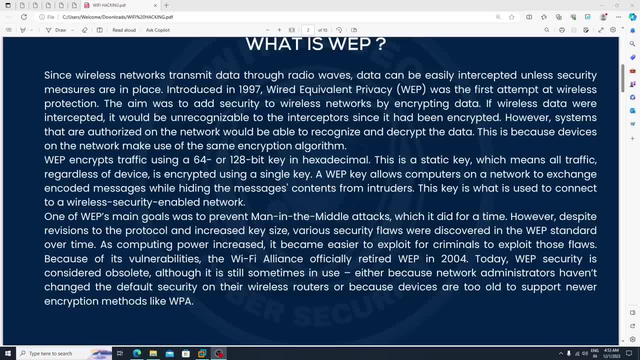 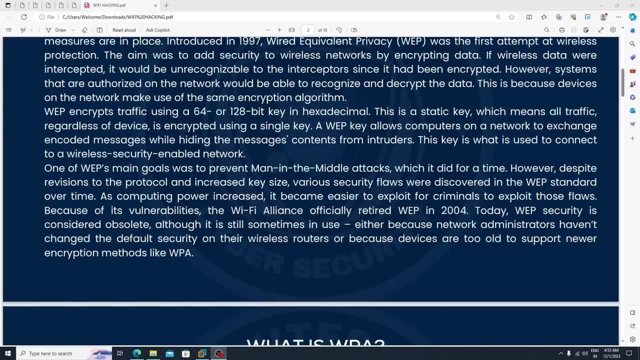 routers. okay, here, they just added the point as well. see, old, the devices are too old to support newer encryption method like WPA. the simple thing. again I am saying sorry guys, okay. again I am saying the thing is hacking or cracking this WEP network is very easy by following the, the techniques. 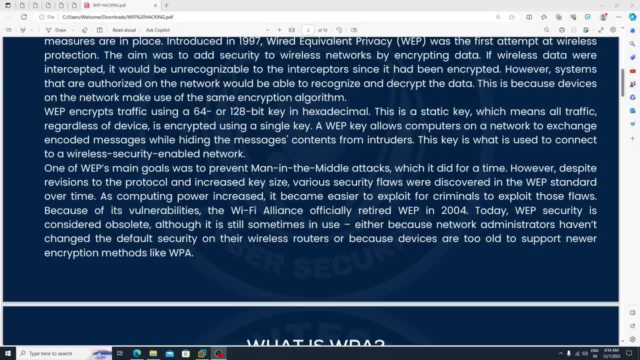 which we are covering in this course, you can able to easily hack the WEP network. if you found that, like, don't hack anyone, just assume that if you just visit it for assessment or for pentesting purpose, at that time just try to exploit it. if it's using WEP network, it is very easy. again I am saying 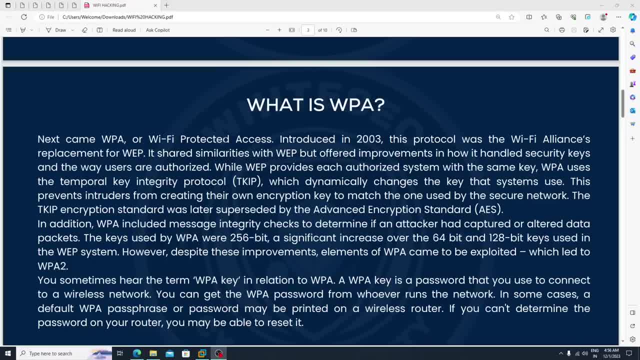 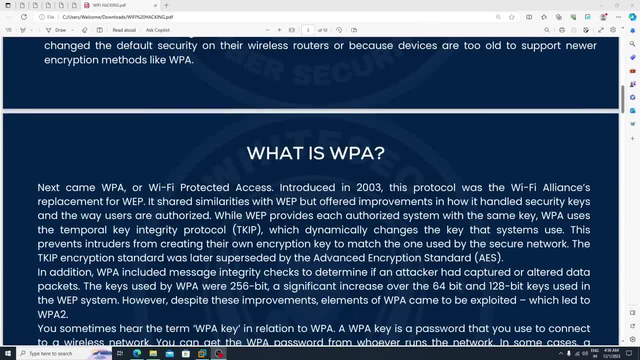 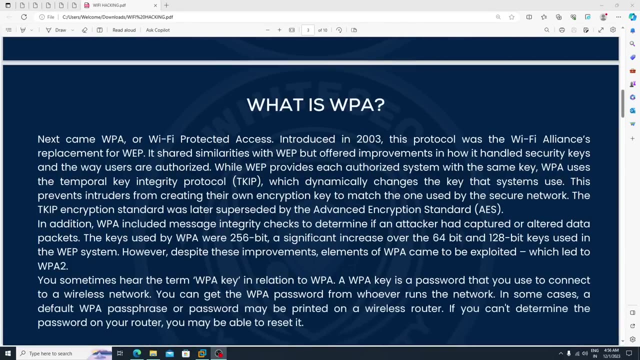 now, what is WPA? next came WPA after WEP. next came WPA or Wi-Fi protected access. the full form of WPA is what? Wi-Fi protected access? not a significant cabeça. introduced in 2003, this protocol was a Wi-Fi alliance replacement for WEP. it 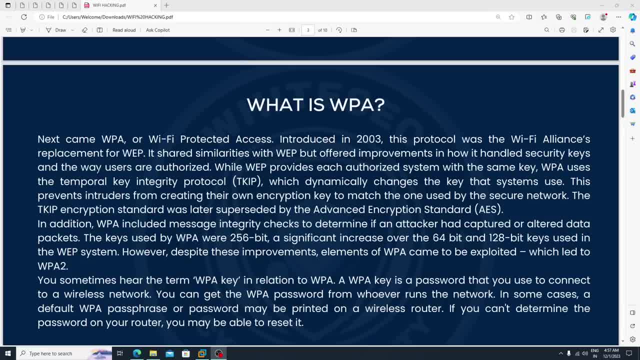 said: basically WPI 0's replacement of WEP. okay, it shared similar similarities with WEP, but offered improvement in how its handle security keys and the way user RF lowerço temporary key integrative protocol, which dynamically changes the key that system uses. This prevents intruders from creating their own encryption key to match the one used by. 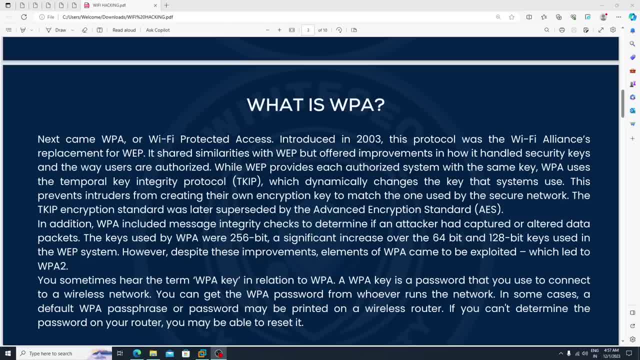 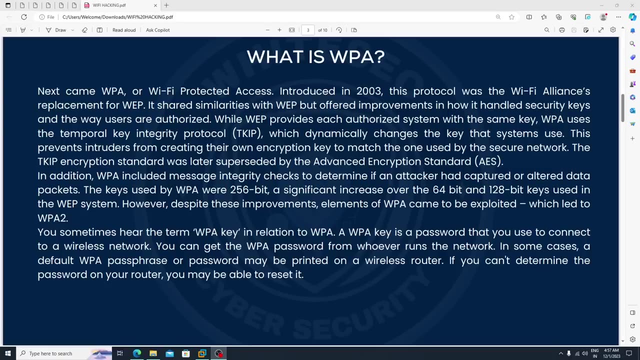 the secure network. The TKIP encryption standard was later superseded by the Advanced Encryption Standard protection. In addition, WPA includes message integrity checks to determine if an attacker had captured or altered data. The key used by WPA were 256-bit, a significant increase over the 64-bit and 128-bit keys. 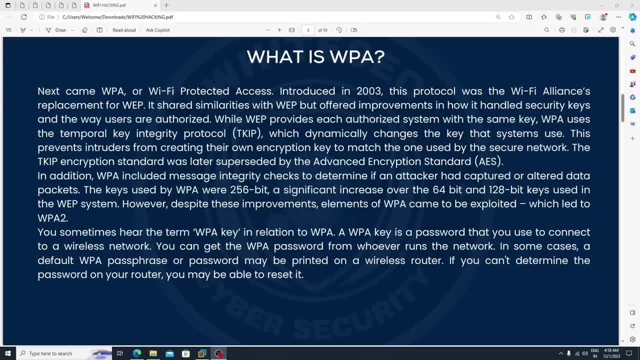 used in the WEP system. However, despite this improvement, elements of WPA came to be exploited. Just focus: Elements of WPA come to be exploited, Which leads to WPA2.. See, here it's become exploited. okay, like it's become vulnerable. 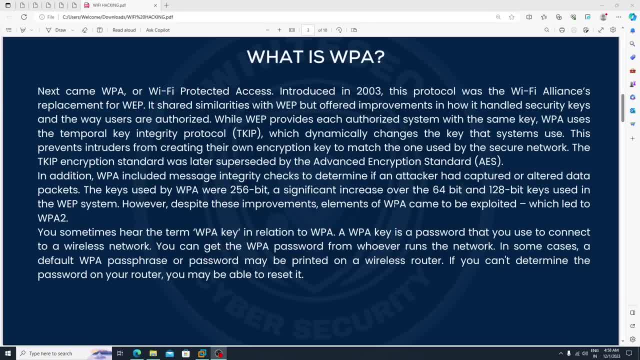 Then, after this WPA, they just launched the WPA2.. You sometimes hear the term WPA key. It's related to WPA. sorry, man, WPA key in relation to WPA. A WPA key is a password But you use to connect to a wireless network. 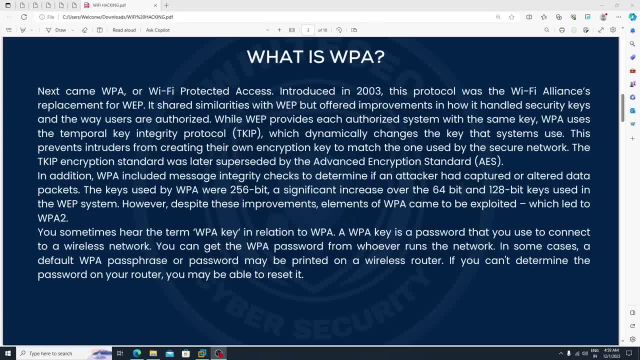 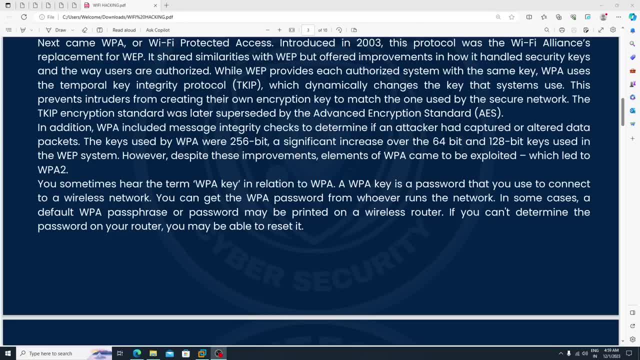 You can get the WPA password from whoever runs the network. In some areas, a default WPA password may be printed on a wireless router. Yes, this is a thing You can. if you see your router in backside, you guys can able to see the WPA password. 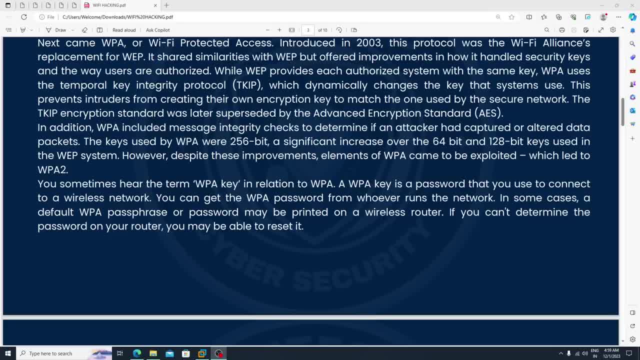 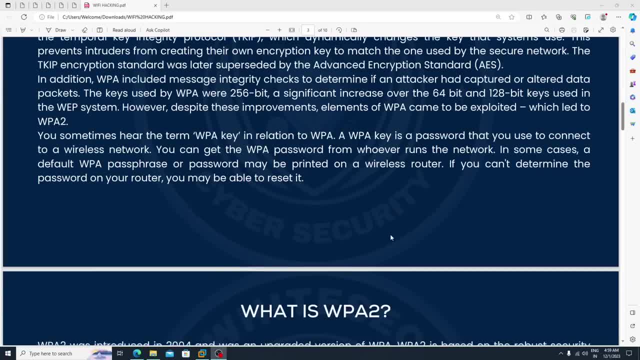 there. Okay, If you can't determine the password on your router, you may be able to reset it. This is a thing. If you are using the Wi-Fi network, then you guys can able to know this, all stuffs. But don't worry if you are not getting this. 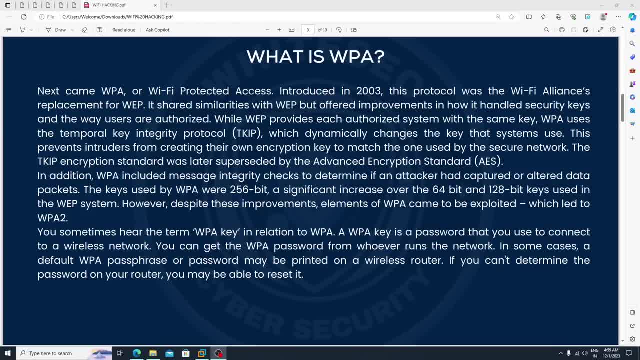 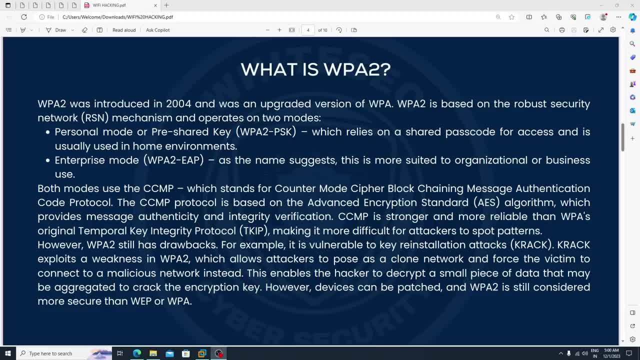 Once we jump in the practical sections, you will know this. all stuffs okay. What is WPA2?? See, WPA2 was introduced in 2004 and was an upgraded version of WPA. WPA2 is based on the robust security network RSN. 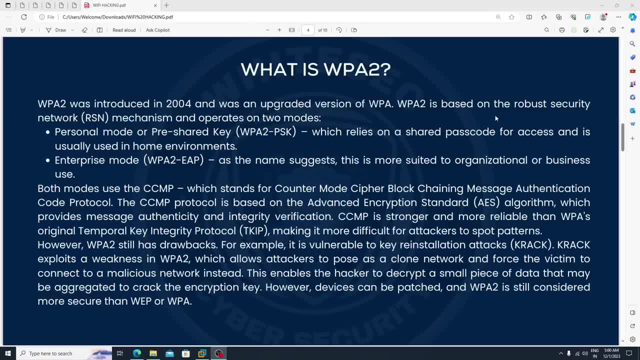 The full form- sorry, the short form- of this robust security network, which is known as what RSN? RSN. basically, it's a mechanism- Okay, See mechanism- and operates on two modules: personal mode or pre-shared key, which is 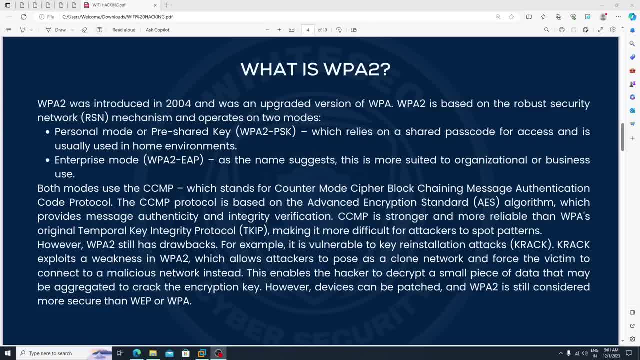 known as a WPA2 PSK, which relays on a shared passcode for access and is usually used in home environment- Okay, In mostly in home routers. you guys can able to see this one Enterprise mode: WPA2 EAP. 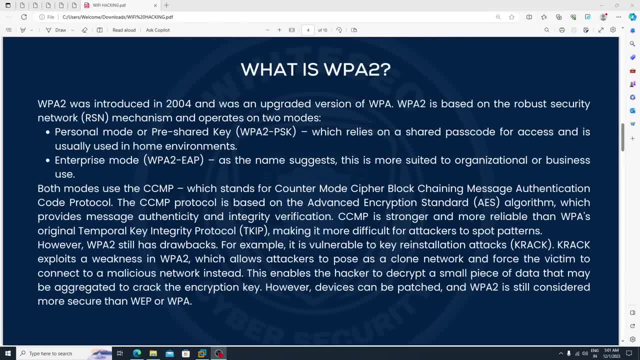 As the name suggests, this is the WPA2 EAP. Okay, As the name suggests, this is more suited to organizational or business uses, Mostly in companies, you guys can able to see enterprise mode. It is also very easy to have. 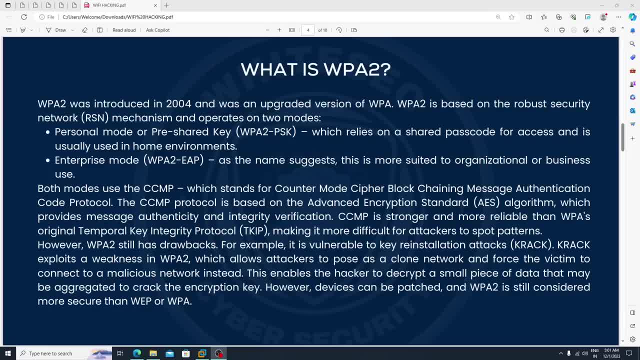 Okay, You no need to worry Now. both modes use the CCMP, which stands for the counter mode, cipher block chaining, message authentication code protocol. It's a very huge but simple. You can say it as a CCMP. You will see what is the CCMP once we scan for the WPS enabled network. 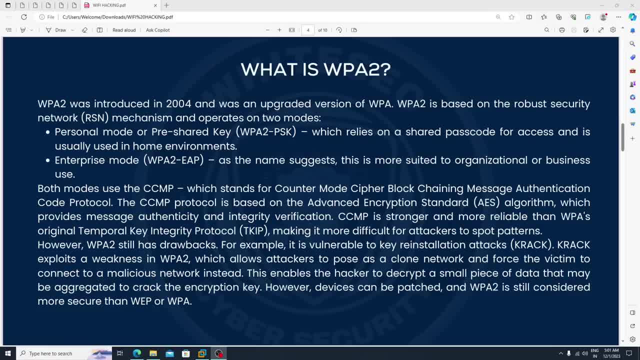 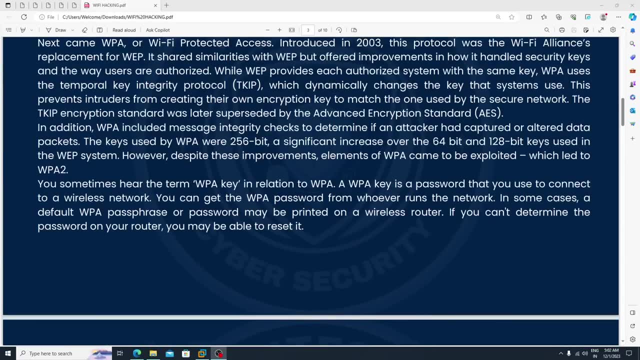 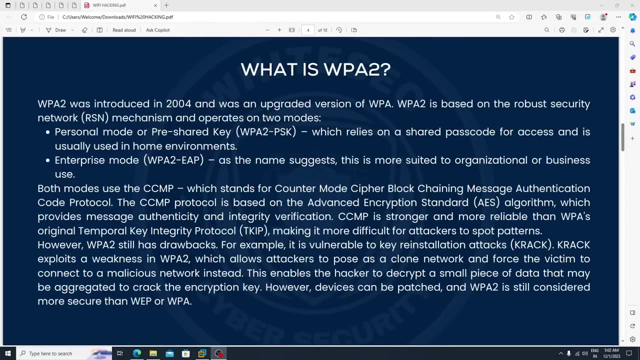 Now the CCMP protocol is used on the advanced encryption standard AES algorithm- See, we just covered this AES in the in this one as well. Right See advanced encryption standard which provides message authenticity and integrity verification. CCMP is stronger and more reliable than WPS original temporary key integrity protocol. 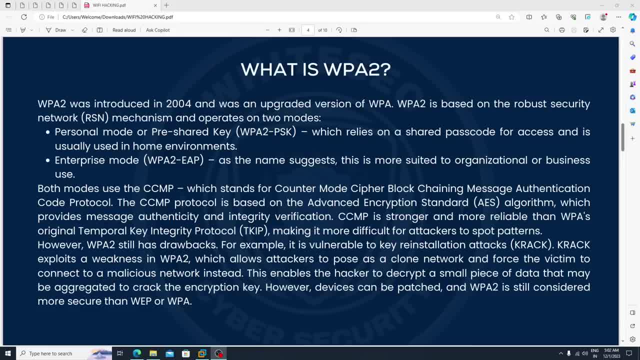 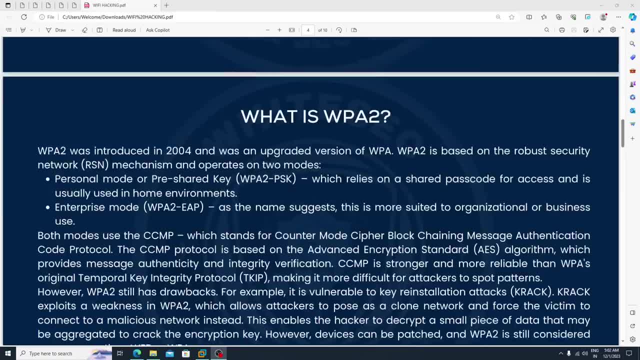 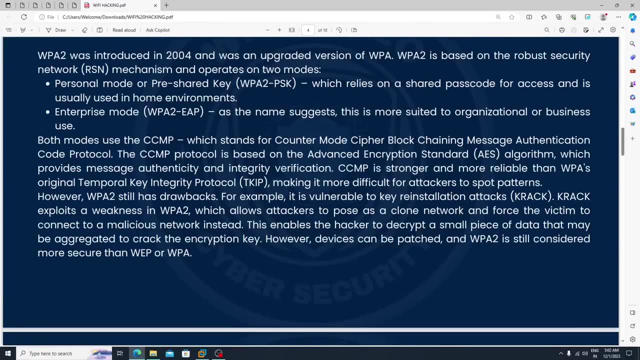 Okay, Now let's talk about the key integrity protocol which we this TK- I am sorry TK IP is- is present in WPA Right. So here you guys can able to see making it more difficult for attacker to spot patterns. However, WPA2 still has drawbacks. 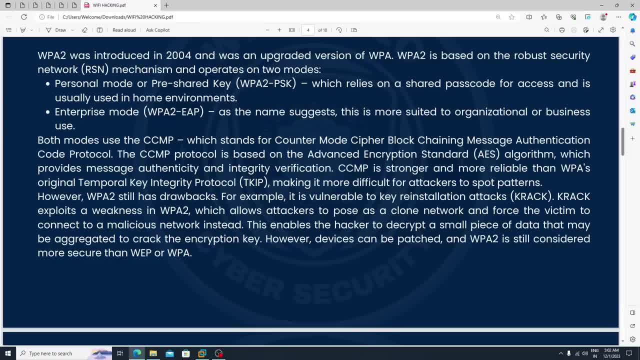 For example, it is vulnerable to key reinstallation attack, which is known as a crack crack exploit, a weakness in WPA2.. Okay, Which allows attacker to pose as a clone network and force victim to connect to the malicious network instead. Basically, it's a evil twin attack. 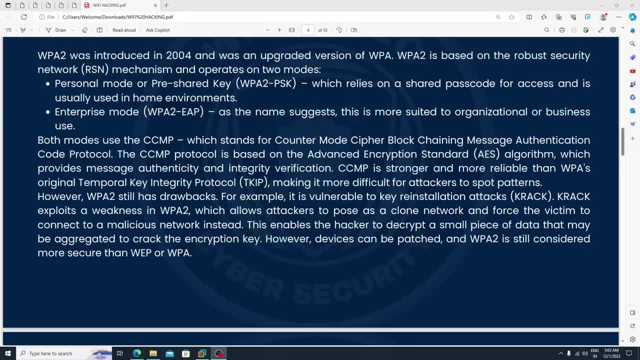 Okay, Like any evil twin attack, what will happen means attacker perform the deauthentication attack on the real network, So the victim, the clients who are connected with the real network, will get disconnected. Then what attacker gonna do means he will create the same network, the network with 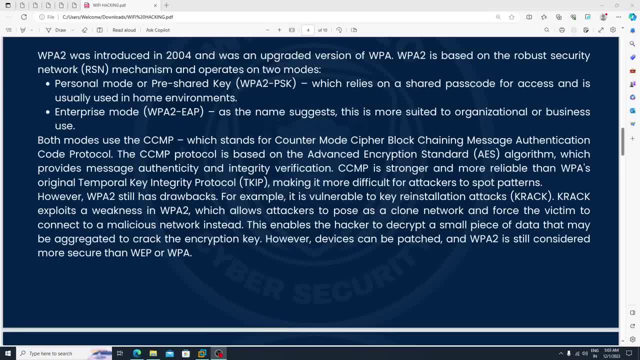 the same legit username. Okay, Then he will force to connect the victims to the clients, okay, to that network. So if they type the password there, he can able to steal it. So this is a thing, It's a kind of phishing. 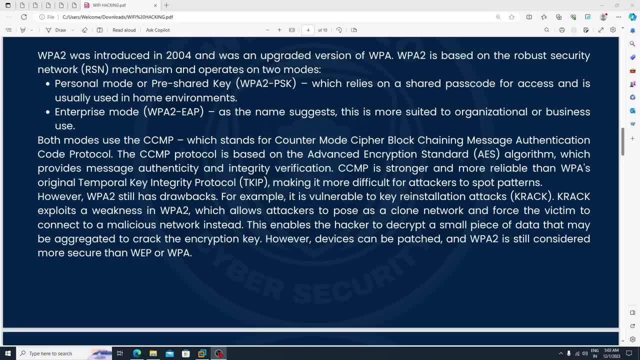 Okay, This enable the hacker to decrypt a small piece of data that may be aggregated to crack the encryption key. Basically, you can also capture the handshake here. Okay, We will learn this also Practically, you know, need to worry again. 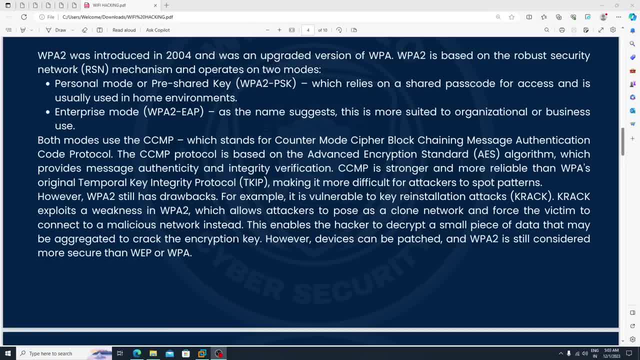 I'm saying The definition is a little bit some kind of hard for you. Okay, Like there is also a four-way handshake in it? Okay, I didn't add it that one because it is very confusing for beginners. Okay, However, device can be patched and WPA2 is still considered more secure than WEP or WPA2.. 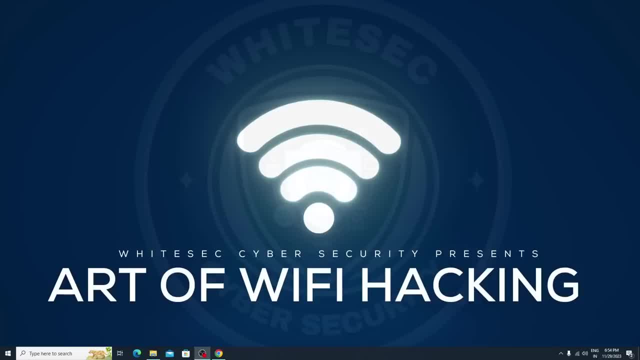 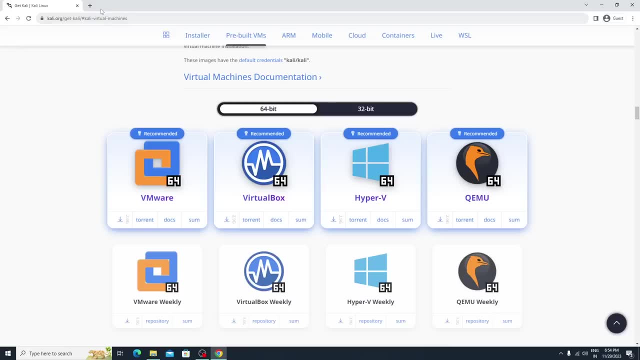 Now in this classes, we are learning how we can able to set up a lab. Now, first of all, the thing is, you just need a virtual machine. first of all, download the VMware workstation from here. Okay, Just type here: VMware workstation. 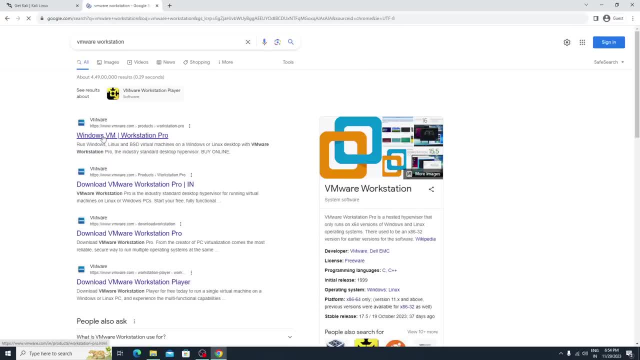 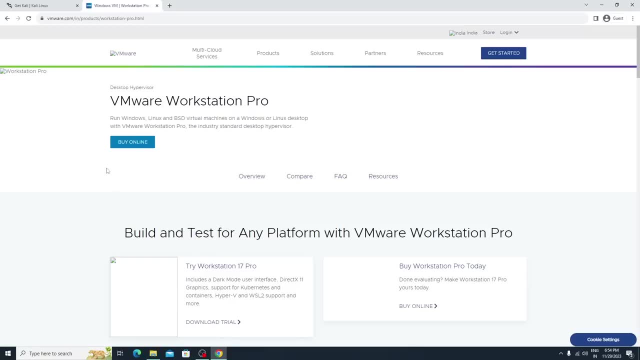 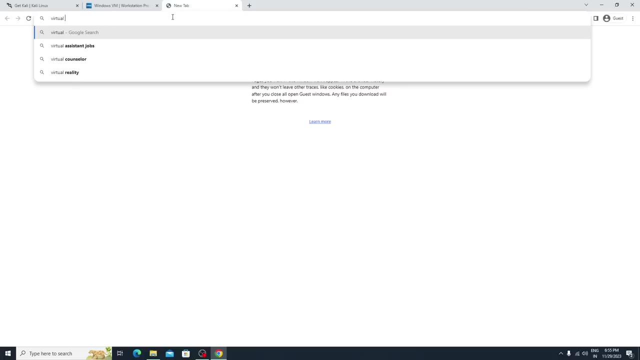 See, you can also use a free version. pro version is totally depend upon you. Okay, If you are using the free version as well, it will work, Okay. Now, here the thing is, you can also use a virtual box. If you watch our Android hacking- ethical hacking using Android training- there we just cover. 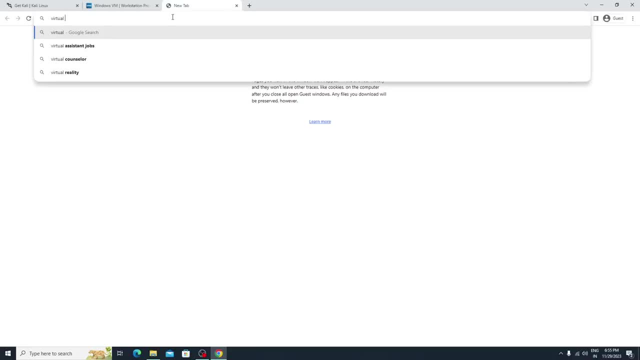 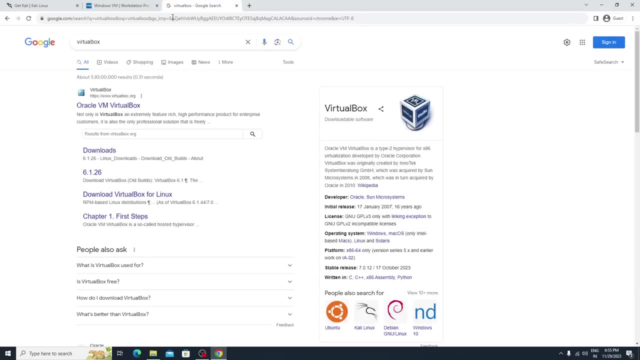 this one, Okay. About this virtual box: how to install it: Okay, If you want to learn about VMware, if you are a completely beginner, you don't know what the VMware, then watch our previous trainings, Okay, Which is available on in this YouTube channel. 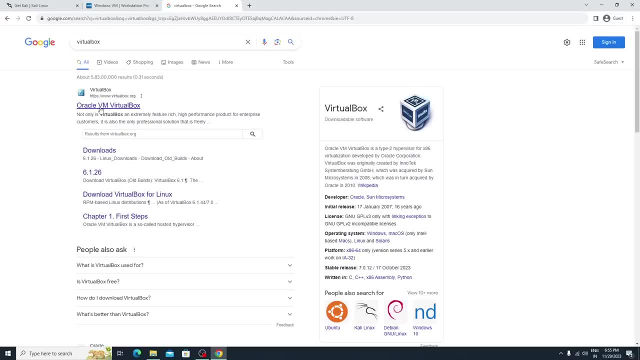 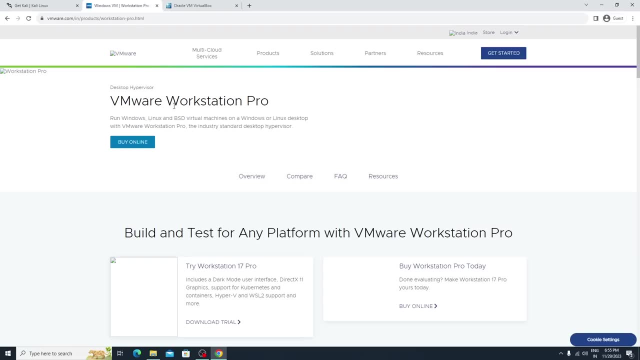 Okay, Simple, Click on Oracle VMware, Just download it. It's a completely free. Okay Now, if you want a VMware workstation keys, simple, just try to search VMware workstation key GitHub- you can able to find it. Okay Now, simple, you just need to download it. 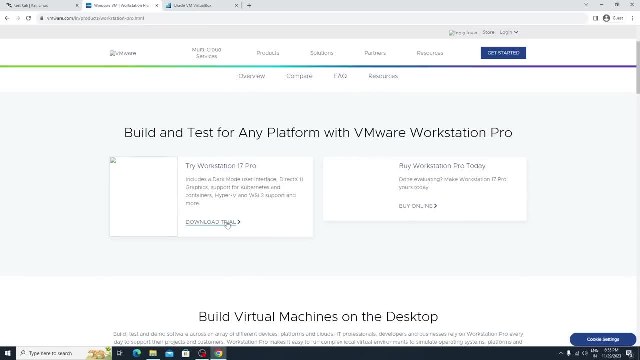 Okay, Simple, Just download the trial. It will work. Okay, You don't need any kind of key For a key here. Okay, Now, here, just use any of this. virtual box or VMware is totally depend upon you know. just focus here. 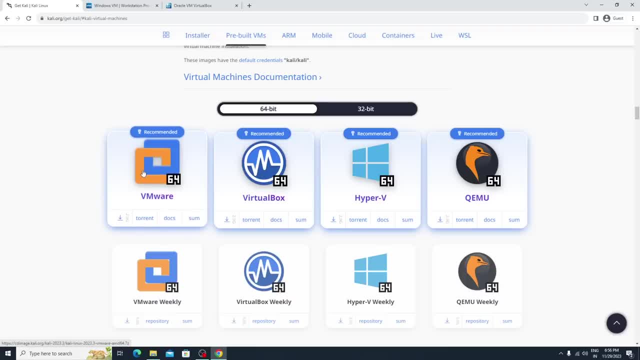 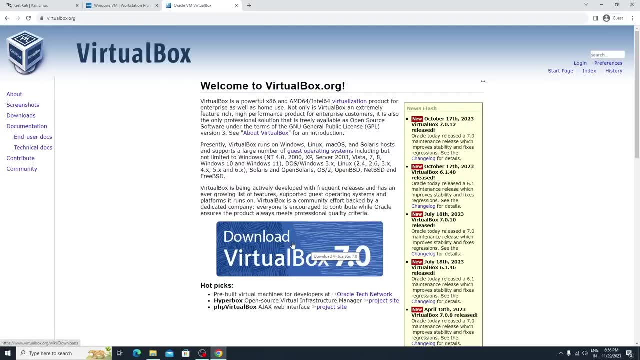 Assume that if you are using the virtual box, Okay, If you are using this one, this virtual box, you just download. download this one, simple click on next, next, next, install it. Okay, After installing that, Now again let me say this thing: 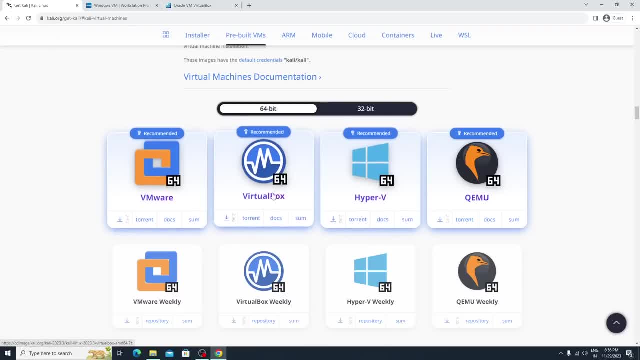 Okay, If you are using the virtual box, then download this one. If you are using the VMware workstation, then download this one. Okay, Now, in this classes, I am using the VMware. So simple, click on the download and let me show this one. 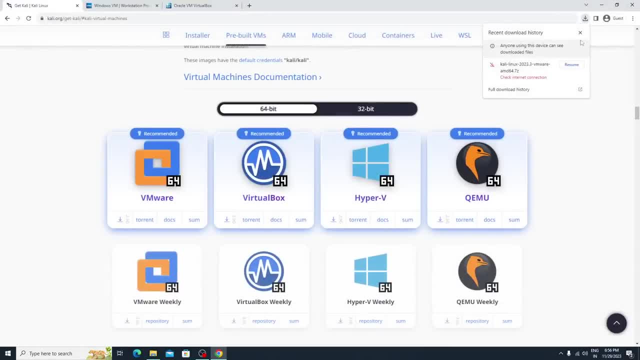 So it will take around 1610 minutes, almost. Let me tell you, after downloading this one, you don't need to set up anything simple: extracted, double click it. It will directly open. It will let me show you. practically. okay, just wait. 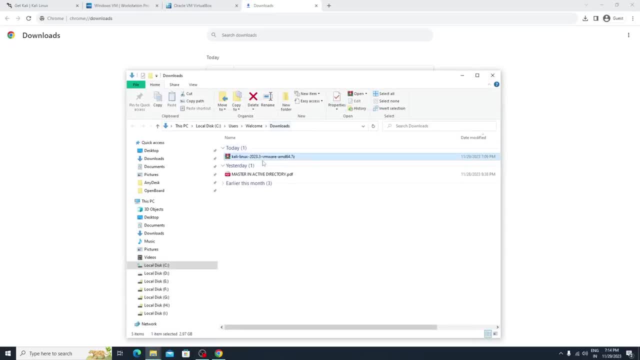 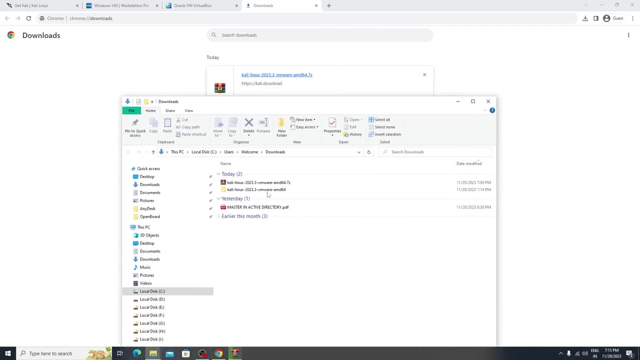 So we successfully downloaded it. So we will try to provide the PDF as well. Related to this course, I think Mostly for ethical hacking. mostly the students ask us to provide the PDF, but I don't know that. Wait, they just keep that, this PDF. just if you want this PDF, just try to message our 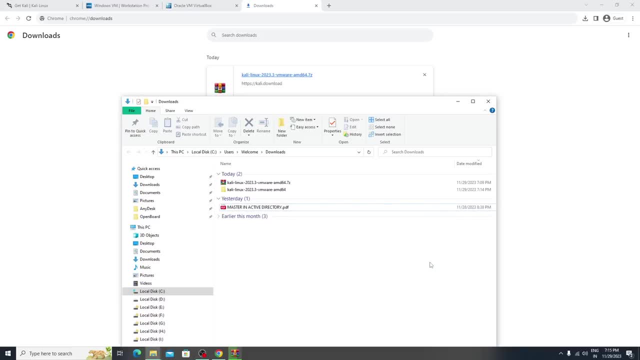 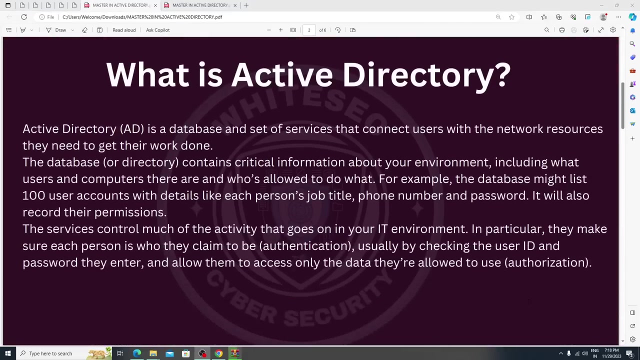 support team. They will provide it. Okay, I don't have right now. I'm just working with Active Directory, So that's why I got this one, Okay. So this is how the PDF look like. So we're going to provide the PDFs related to the topics as well. 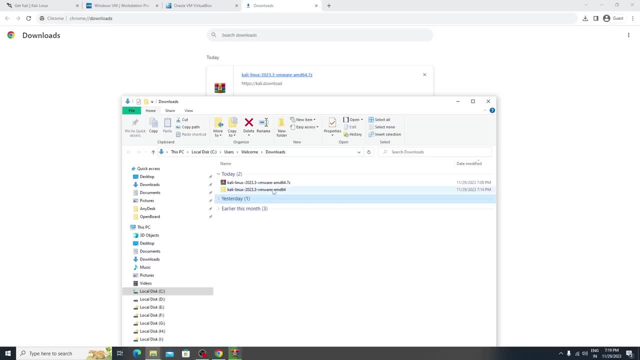 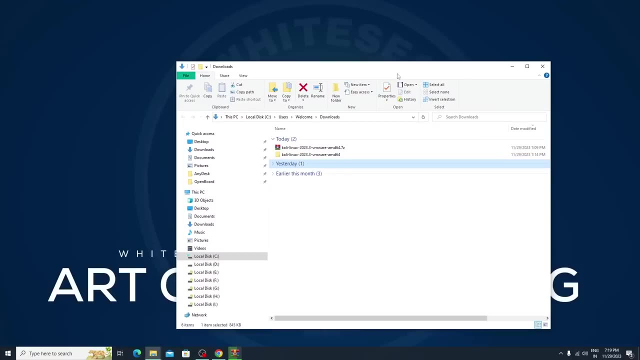 Okay, right now we are working with what Wi-Fi hacking. right out of Wi-Fi hacking, You will get the PDF as well. Okay, Just check the description. There you guys can able to see the link. If the link is not there, then contact our support them. 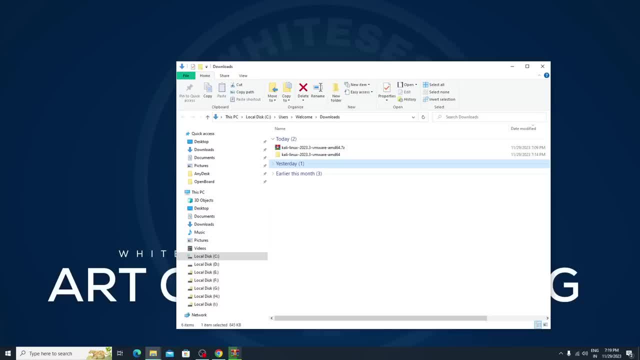 They're going to provide you. Okay, You no need to worry, You just message them. So here it is, Double click it. So let me tell you no need to set up anything, Just simple click on view and click on file name extension. 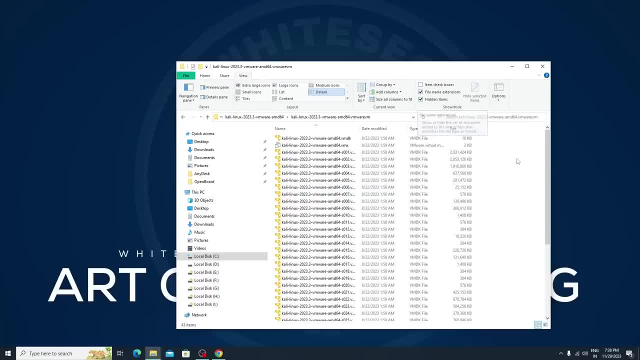 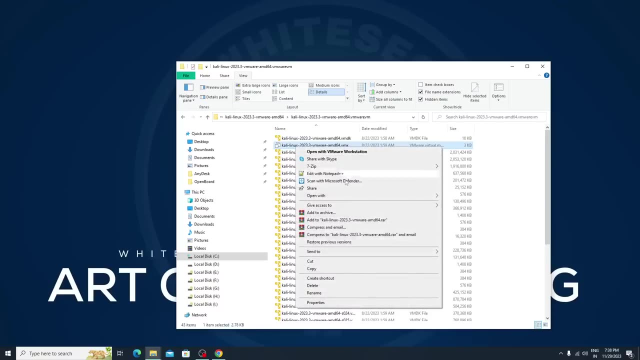 Check this one. After checking it, Just focus here. There is a dot VMX extension is there? First of all, you need to install the VMware workstation. Then see here, Right click, Open with and simple select VMware workstation from here. 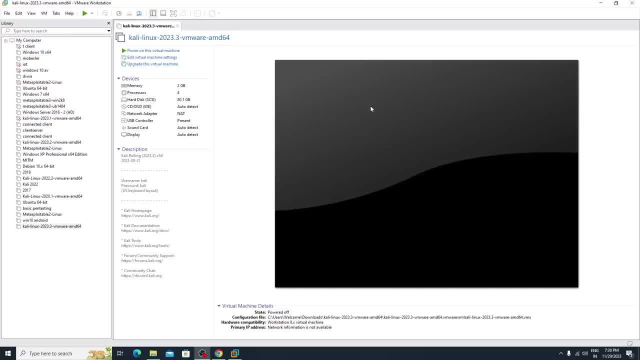 Here, it is Okay, You no need to do anything. Simple click on. if you want to change any RAM processor, Okay, Memories are nothing, but it's a RAM and the username and the password is kali kali. You can also change it. 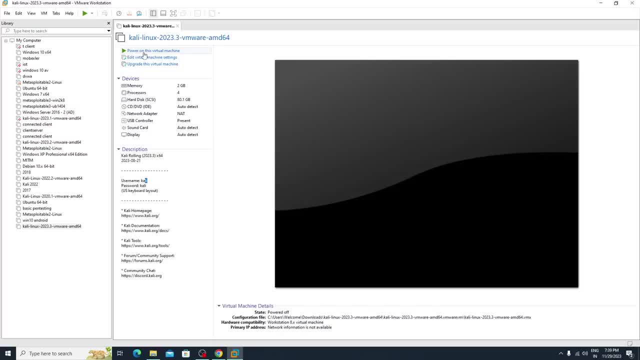 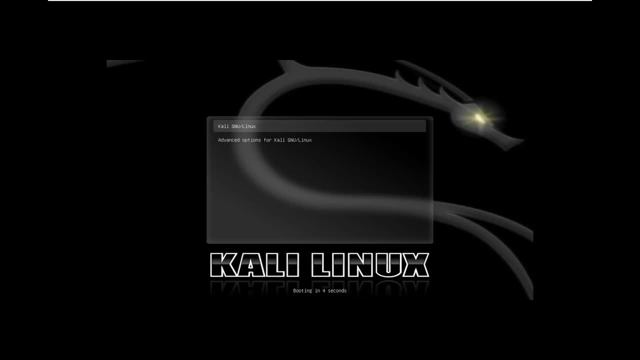 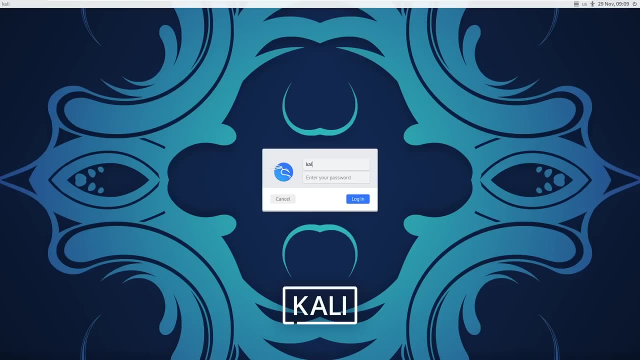 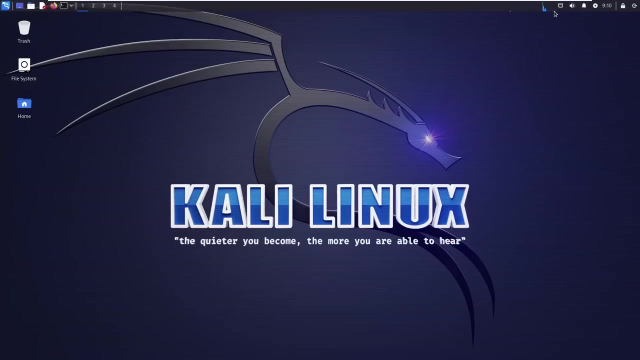 No simple click on power on this virtual machine Enter. So here it is Okay. The username is what here? Kali, and the password is kali. So in the next classes we will learn which adapter we need to select. Okay, 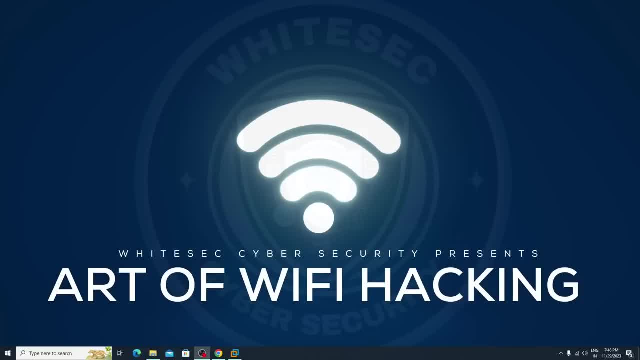 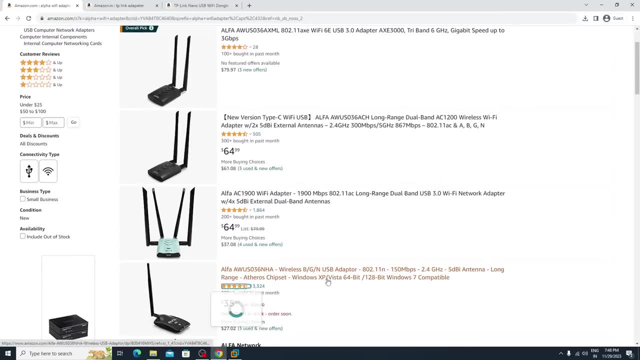 Now in this class, I'm going to teach you which adapter you need to select for Wi-Fi hacking. See, the best adapter for Wi-Fi hacking is alpha adapter. If you have any other adapter is support monitor mode. packet injection: Okay, Evil twin attack. 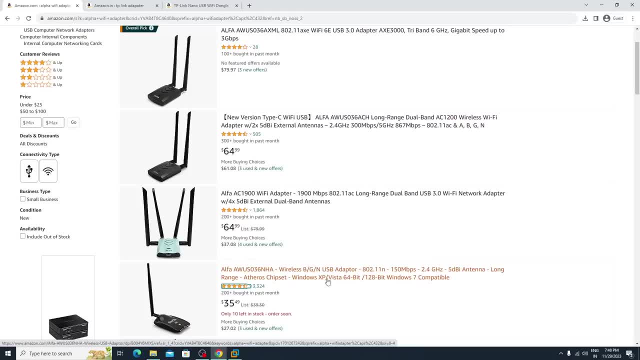 Then go with it. Okay, It's not a big deal, But the thing is, mostly the attackers use this one, Okay. The pentesters, attackers, Okay, Even me- use this Wi-Fi adapter which is alpha, Okay, Which is stable one. 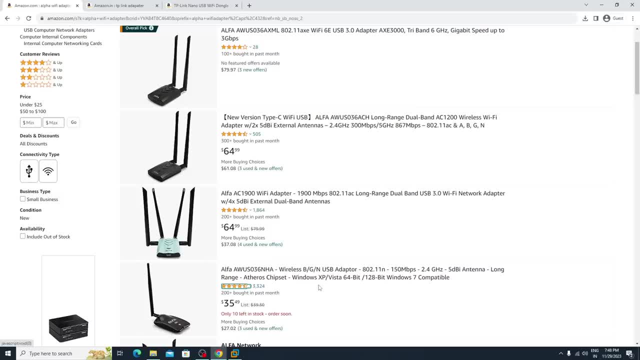 Okay, Assume that if I choose alpha adapter, That means I can able to use it. That means I can able to perform each and every Wi-Fi attack by using it. Okay, It's a simple thing. Now the thing is: if you want to learn Wi-Fi hacking or Wi-Fi pentesting, if you want to, 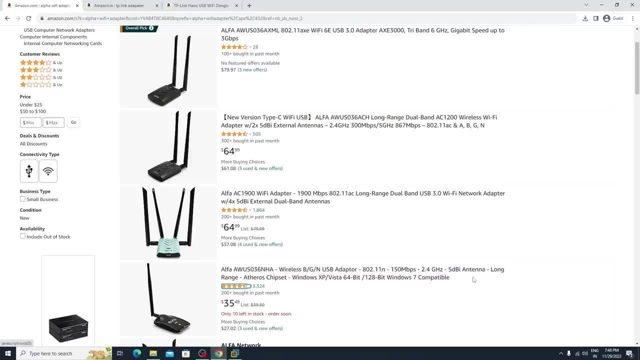 perform a successful attack. at that time I'm going to suggest you to go with the adapter, This alpha adapter. Now there are a lot of beginners are there who just want to test a network, like for fun purpose. They want to hack the Wi-Fi network by watching movies, by watching some movies. 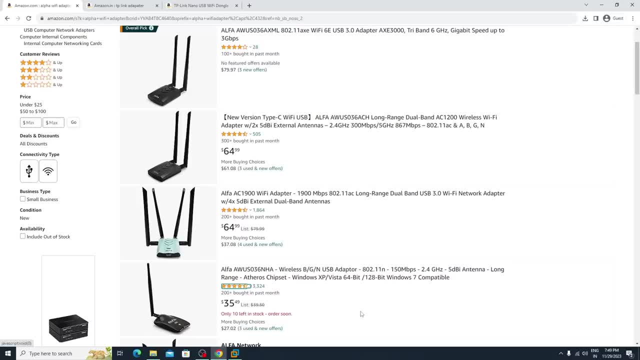 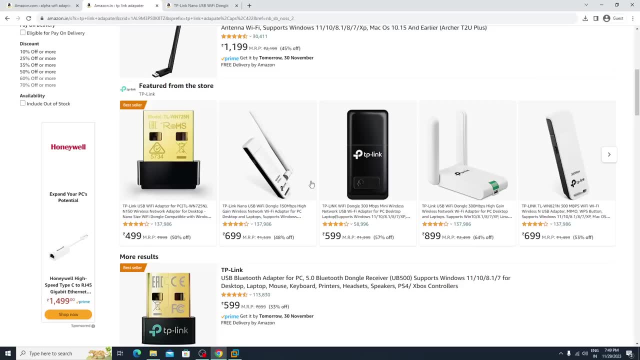 Majority of people will get the interest. Okay, So let's hack something or some kind of shops at the time. Just go with TP link Wi-Fi adapter. Okay, If you want to test your own network, See, let me tell you, the whole attack which I'm doing here is doing on my own network. 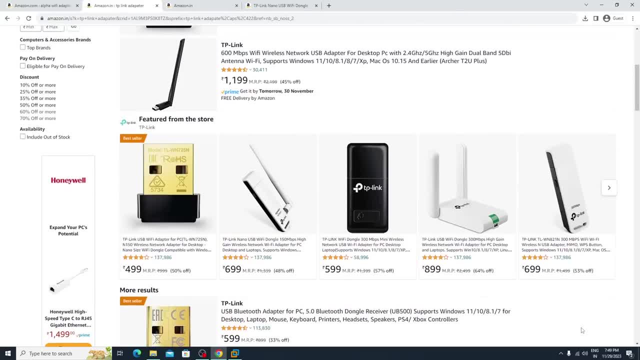 Okay, This is the thing Now here. there is a TP link Wi-Fi adapter is here. by using this TP link Wi-Fi adapter, You can able to perform 70% of Wi-Fi hacking. Let me tell you this thing: There are a lot of attacks, are there? 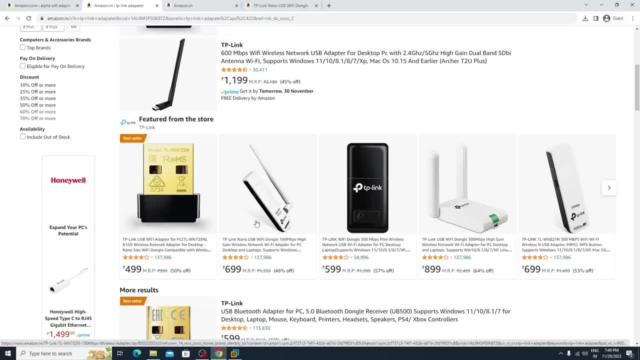 Which you can't able to perform using this TP link, such as evil twin attack, is there? Okay, You can't able to perform on the attack by 5 gigahertz base networks- Okay, This is a thing. There are some limitations when you use this TP link adapter. but let me tell you again. 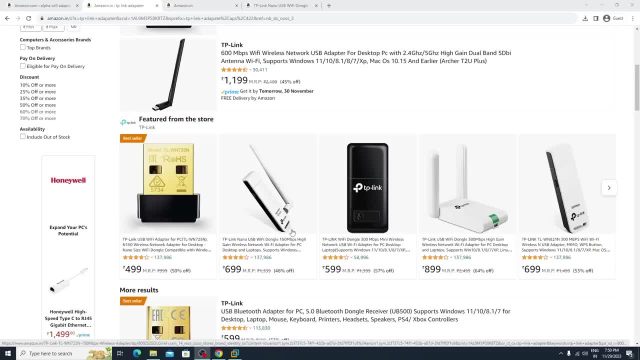 if you are targeting the home networks or a companies which doesn't use a expensive stuff, Okay, At that time you guys can go with this one. Okay, This is the TP link Wi-Fi adapter. Now the thing is here if you want to target a, like if you just visited to one organization. 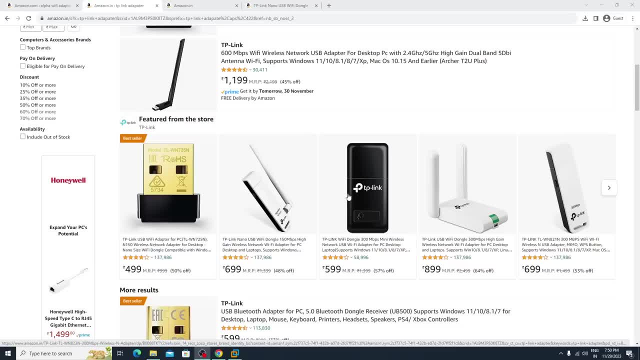 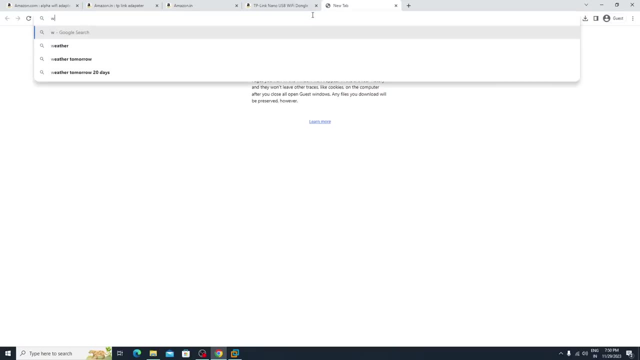 and you want to perform a pen testing there? Okay, On wireless networks. at that time, what you need to do? simple. I'm going to suggest you to go with. what are you guys? Wi-Fi pineapple? Okay, Wi-Fi pineapple is a one of. just let me show you. 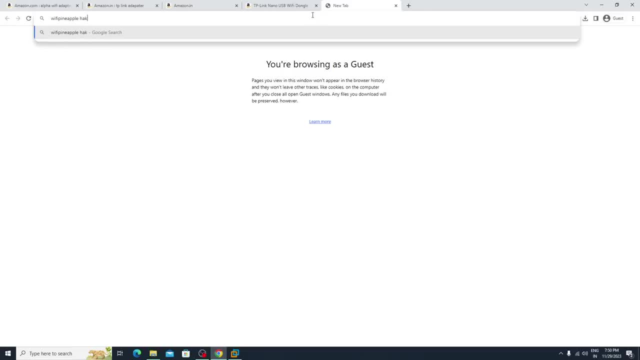 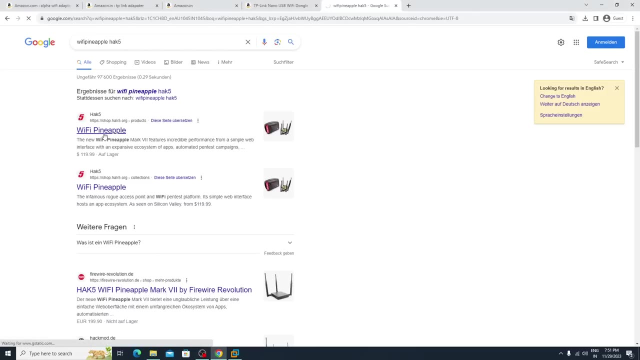 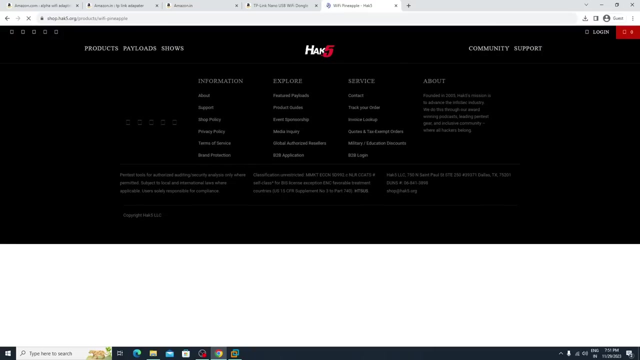 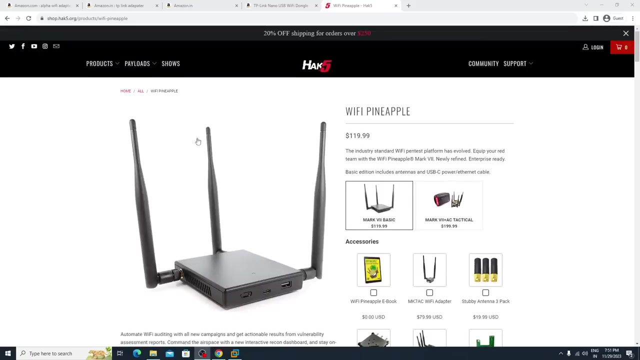 There is a hack for a Wi-Fi pineapple is there you can. you can go with this one if you are performing pen testing. So this is a one of the excellent hardware. by using this, assume that you are using this one. Okay, you no need any kind of Kali Linux. 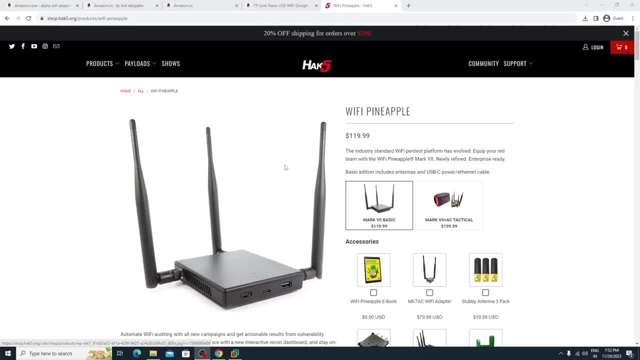 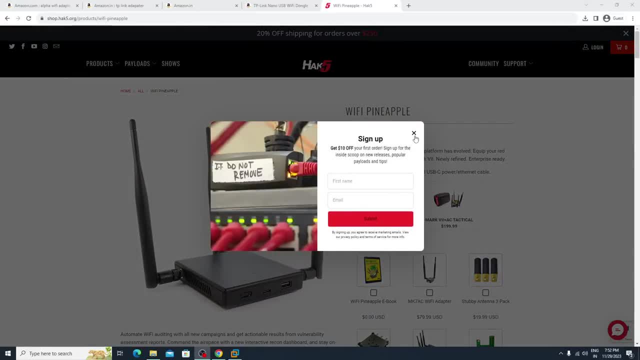 Let me tell you, For example, you can able to connect this Wi-Fi pineapple with your Android device wirelessly and from there you can able to conduct the attacks. Okay, This is the thing. you no need any kind of Linux knowledge for this, like every pen test. 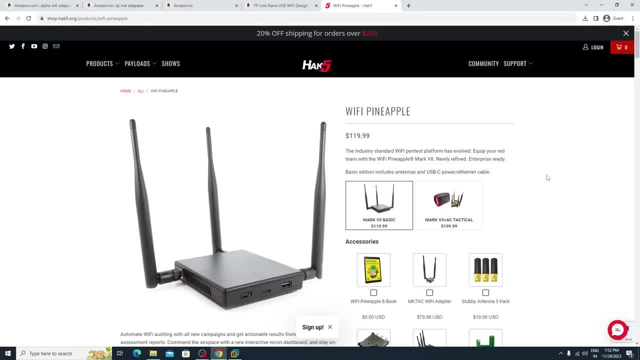 pen test and need a Linux knowledge, But here, when you use this Wi-Fi pineapple, at that time you no need to type any kind of commands. Okay, Simple, within few clicks, You guys can able to execute the attacks. This is a thing which is very easy to use. 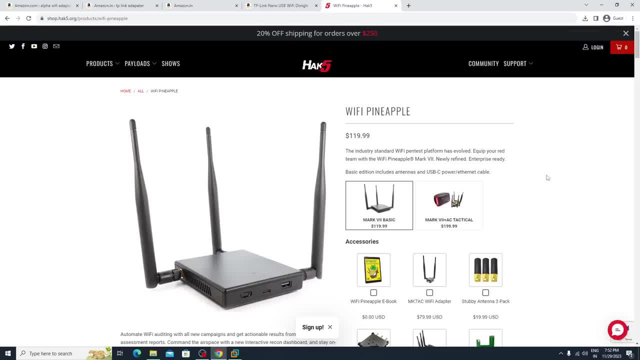 Okay, This is a important thing. If you are. If you want to become a real pen tester, at that time go with Wi-Fi pineapple. Okay, in this section, in this class, we are not covering about Wi-Fi pineapple, but still, I am just showing you that. okay, if you want to become a successful pen tester, if you want. 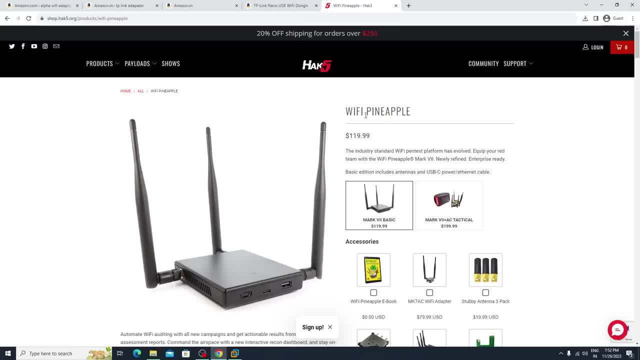 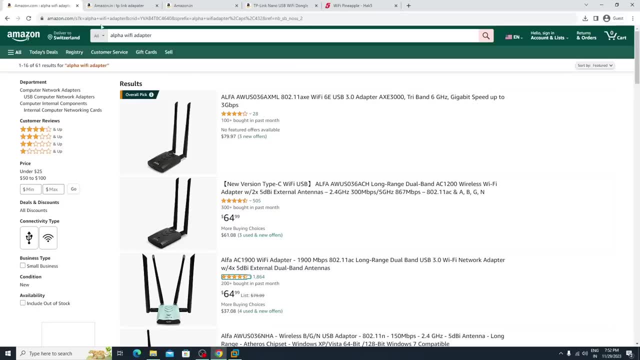 to perform a wireless pen testing in one company at that time, just go with Wi-Fi pineapple, Okay. Now, here what I said. let's recap this one: If you want to learn, okay, the Wi-Fi pen testing. or if you want to perform a hundred percent. 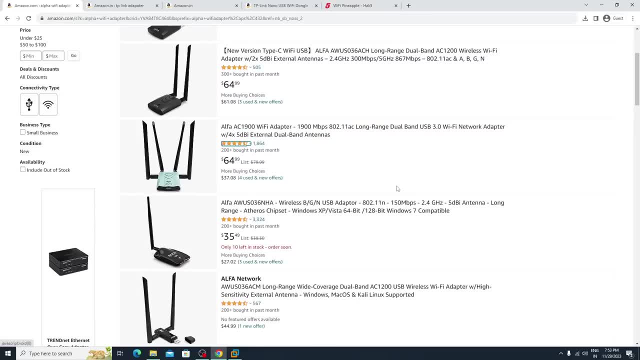 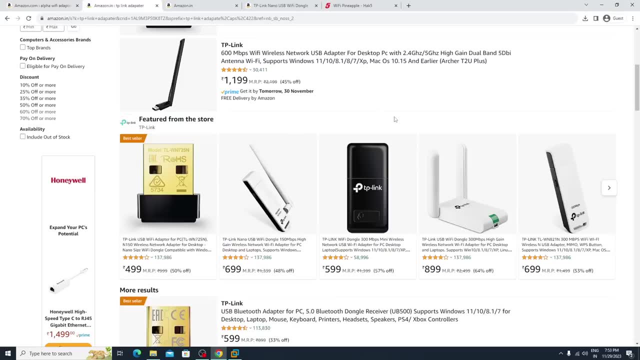 attack At that time. go with alpha Right Now. if you just want to learn- Okay, You just want to test the other time- go with TP-Link Wi-Fi adapter. That's it. It's not a big deal, Okay. 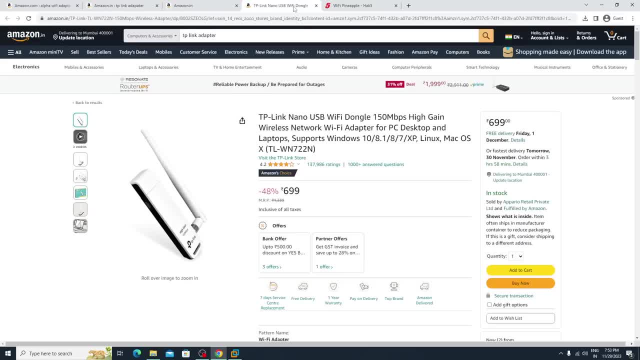 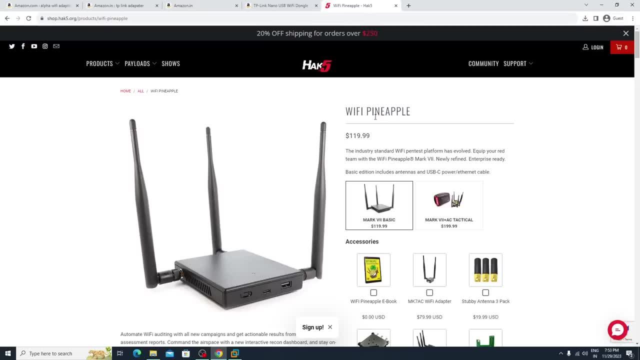 If you are performing, if you want to learn a Wi-Fi this one, want to become a successful pen tester, or if you want to learn a real thing like how to perform the pen testing in real world organizations, or at that time, simple, you guy, at that time you guys can able. 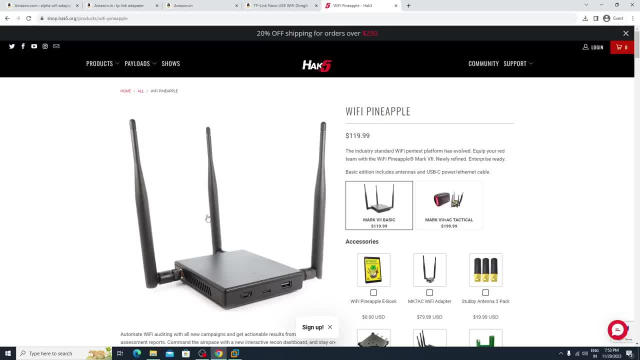 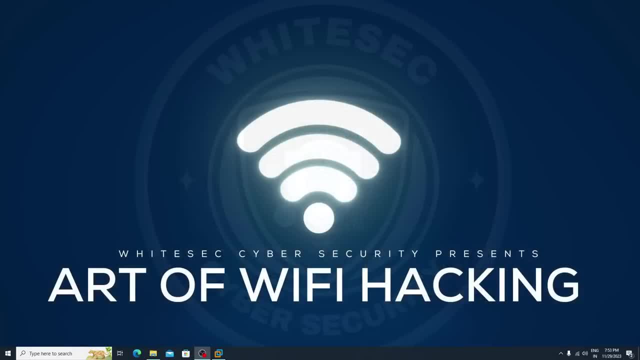 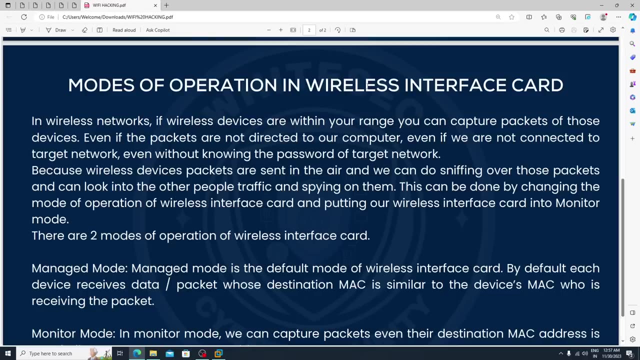 to use this one. Okay, This is a very handyman which I use. Okay, Right, Hope you guys get it Now. in this class, we are learning about modes of operation in wireless interface card. wireless interface card is a nothing but Wi-Fi adapter. 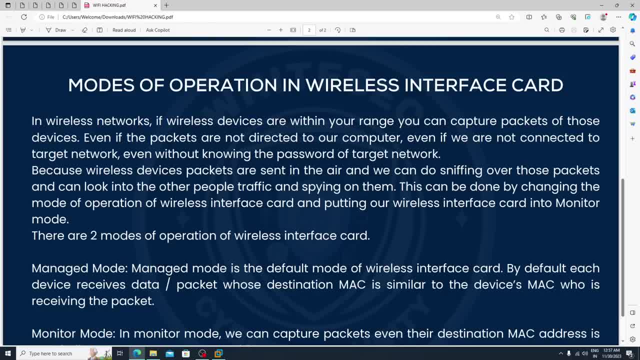 Okay, Just remember this point: in wireless networks, if wireless device or within your range, you can capture packets of those devices. Okay, Now just focus here. if wireless devices or within your range, wireless devices or what here? in our case, wireless devices are nothing but APs. 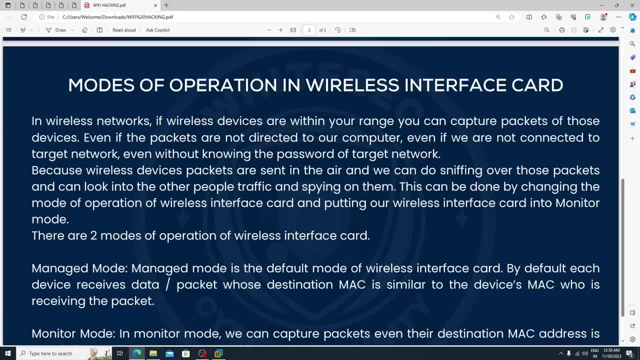 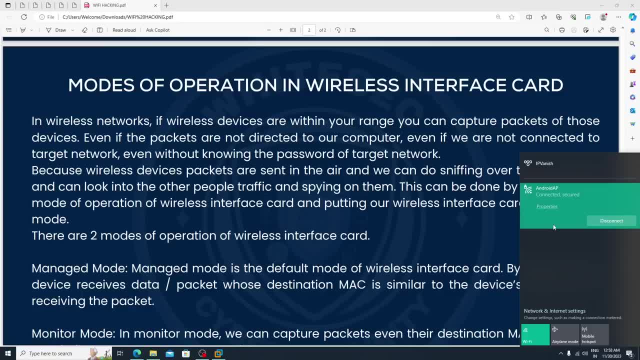 Okay, Like once. just see here, there is a Android APs here. Let's say, in our case, wireless devices are APs. Okay, As is points Okay, Or within your range you can. you can capture packets of those devices, Okay. 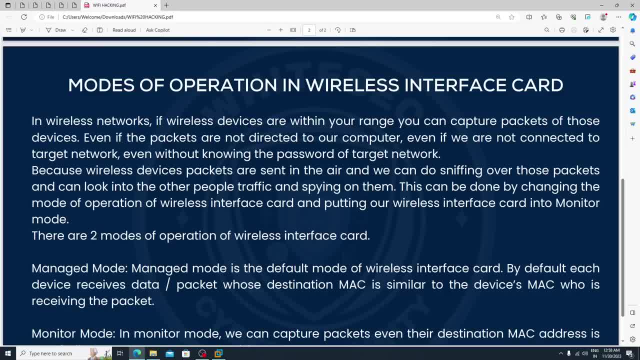 In a simple words, You guys can able to capture the data of those devices. Okay, This is the thing I'm going to explain. it, Don't worry. Even if the packets are not directed to your computer, Okay, Even if we are not connected to the target network, even without knowing the password, 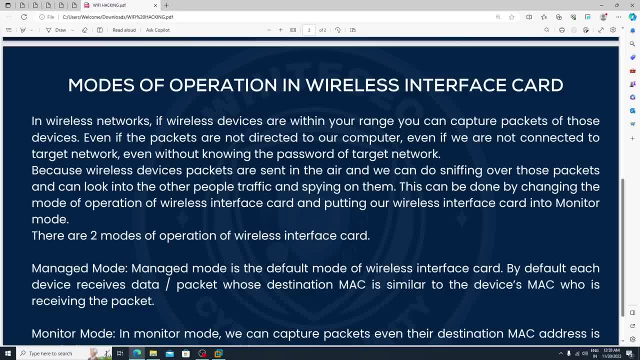 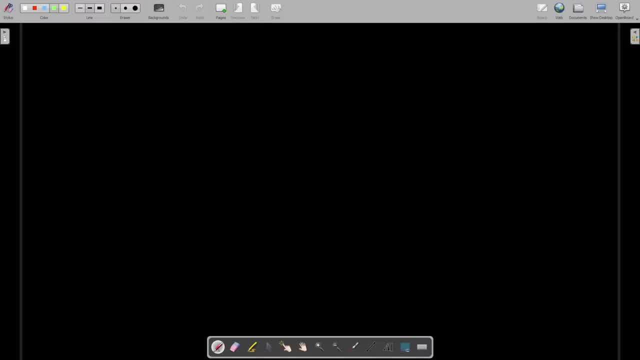 of the target network. now here once you just just wait. now you just scan the Wi-Fi network here. Okay, After scanning the Wi-Fi network, You guys can able to see a lot of Wi-Fi networks here. Okay, Like there is a enterprise, one is there. 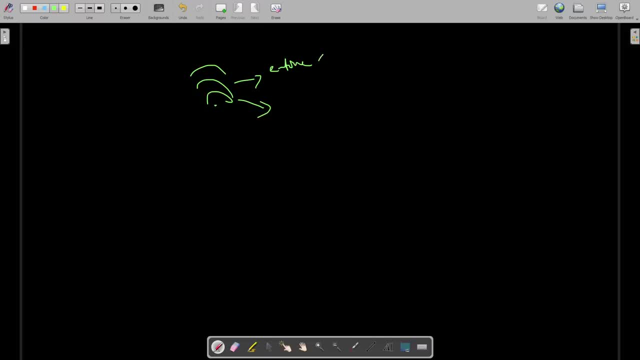 This is also a Wi-Fi network. Okay, Enterprise two is there. Okay, This is also a Wi-Fi network. These Wi-Fi networks are not owned by me. Okay, Simple, I don't even know the password of this networks. Then also, I can able to capture the data of this networks. 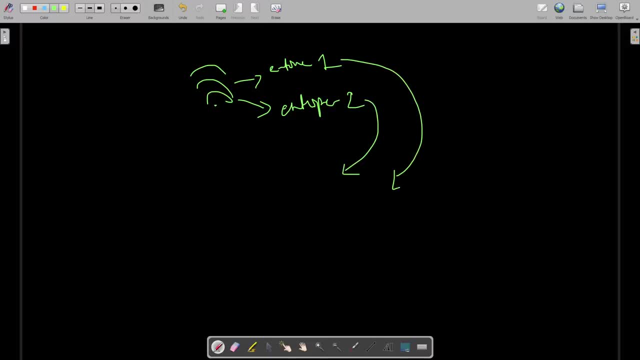 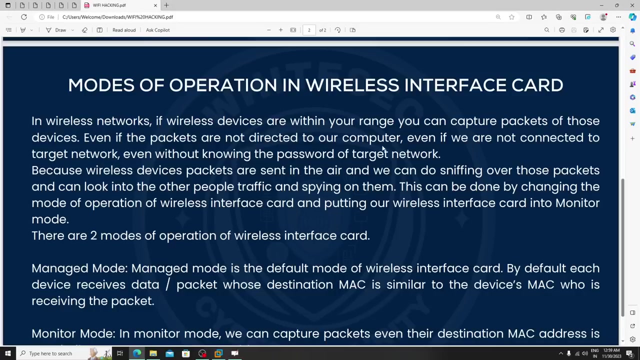 Okay, Without typing the password, Without knowing the Knowing the password of this network, Okay, Even, see here the point. Even the packets are not directed to our computer, Still, we can able to capture the data there. Okay, This is the thing. 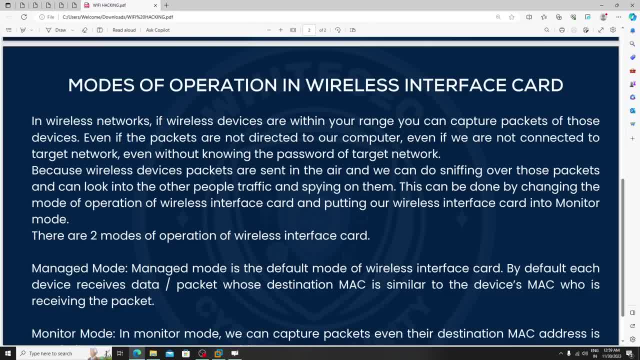 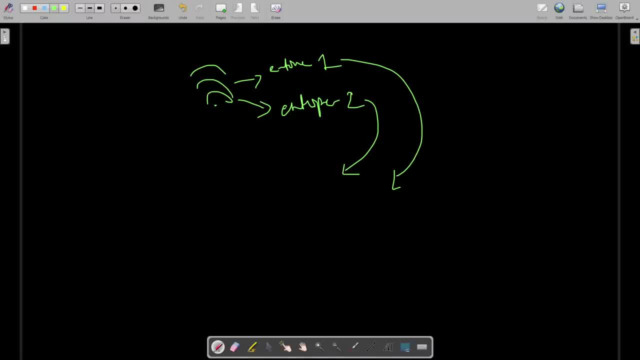 Whenever you see the packets, just assumed it It's a data. Okay, Simple. This is the thing. Why? Why it's happening here? Just see here. Because wireless devices- packets- are sent in the air And we can do sniffing over those packets. 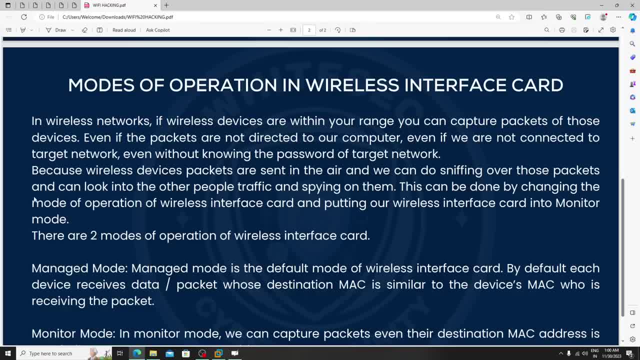 And can look into the other people traffic and spying on them. This can be done by the changing the mode of operation of wireless interface card. Again, I am saying wireless interface card is a nothing but your Wi-Fi adapter. By changing the mode of operation of your wireless card. 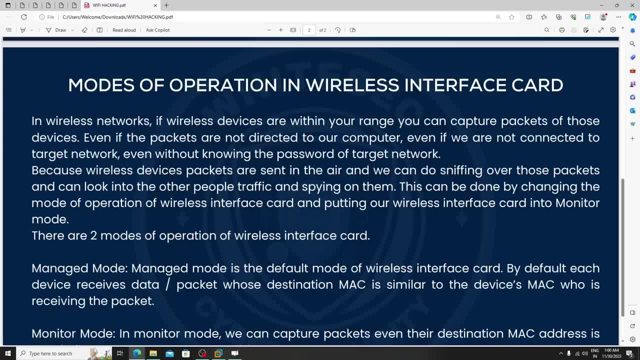 And putting our wireless interface card into monitor mode. This is the thing. See Here, monitor mode plays a very important role in Wi-Fi hacking. If your adapter doesn't support monitor mode, Just forget about Wi-Fi hacking. Okay, Every adapter doesn't support monitor mode. 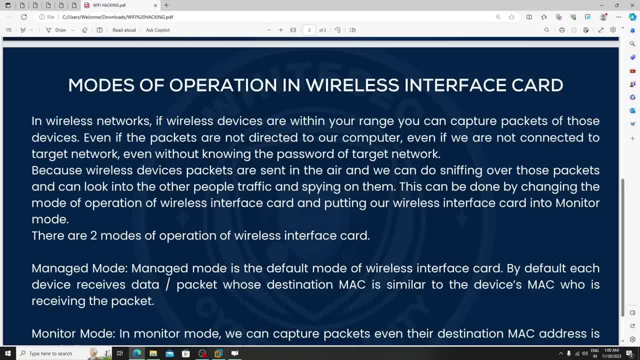 You need to remember this point. Okay, There are some adapters are there Which supports the monitor mode, Such as this. I just told you in the last classes Which adapters you need to use for Wi-Fi hacking, Like TP-Link is there. 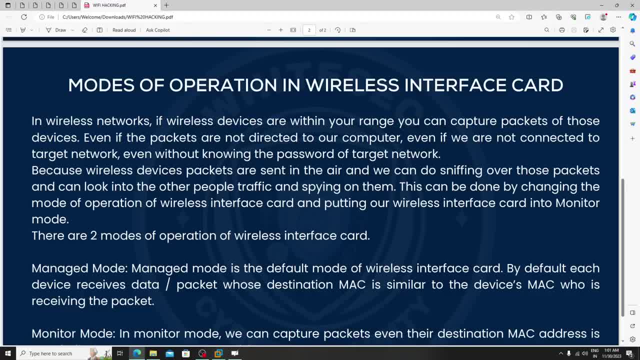 Okay, Mostly adapters support monitor modes, Like right now it's a 2000.. From 2021, every adapter, Almost every adapter, it's supporting the monitor mode, But the problem is it doesn't support this one Evil twin attacks, This kind of attacks. 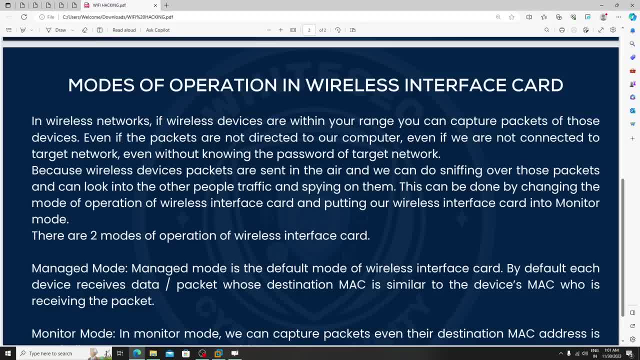 But still, you can able to perform Wi-Fi hacking If your adapter supports the monitor mode. Okay, Just focus on this point. Monitor mode is a very important. Okay, How to change your adapter in the monitor mode. We will learn each and everything in the next class. 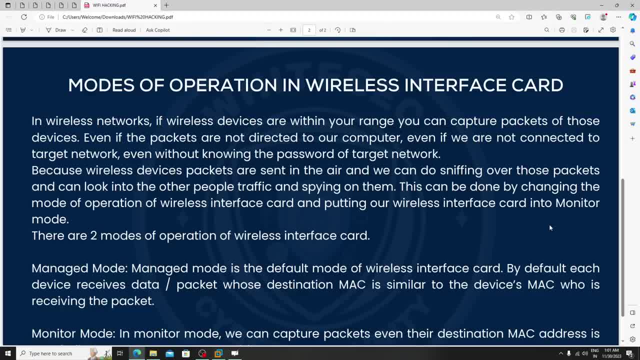 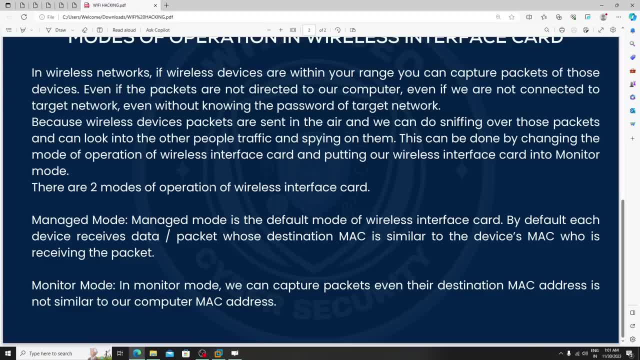 Okay, You no need to worry about this all stuff. See, Here there are two modes of operation of wireless interface card. Mostly there are. There are lot of modes, are there Okay? Not only two modes, There are huge Okay. 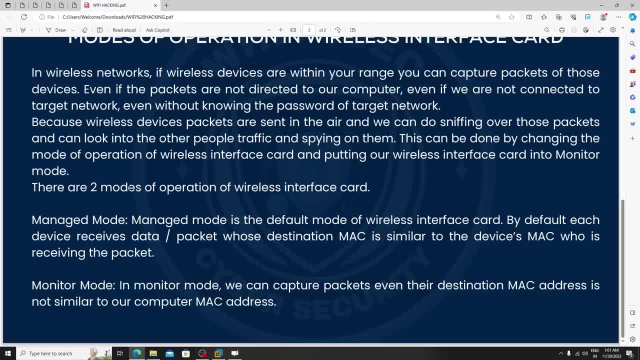 But the main things. we need to focus on Manage mode and monitor mode. What is a manage mode here? Manage mode is a default mode of wireless interface card, By default. By default, each device receive data packets whose destination MAC is similar to the device. 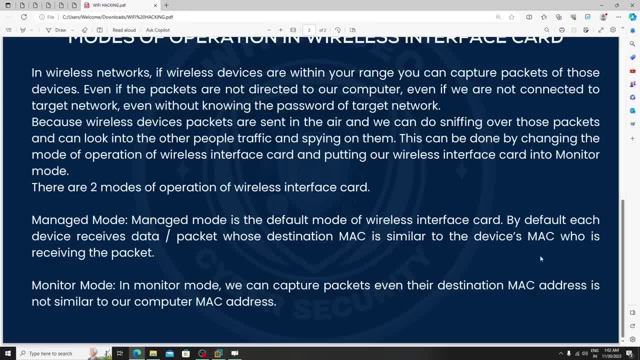 MAC? who is receiving the packets? Just, if you are not getting this point, Just ignore it. Just focus on this point only. Manage mode is a default mode of wireless adapter card, Wireless interface card. What is a default? Let me tell you. 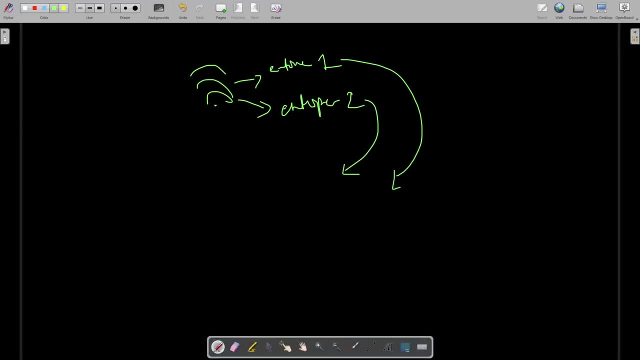 See, you just purchase one Wi-Fi adapter, Just assumed it. You just purchase a TP-Link Wi-Fi adapter here Once you connect your TP-Link Wi-Fi adapter with your computer, Or assume that you just connected with your Kali Linux. 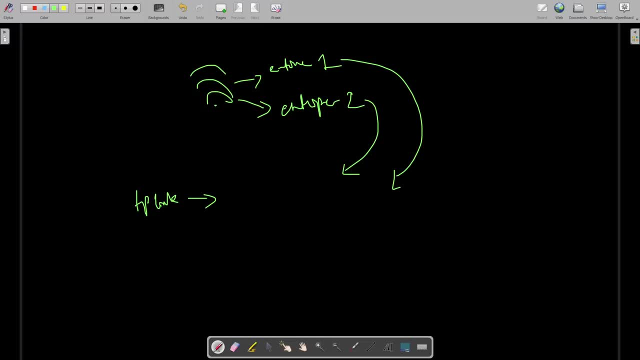 At that time, What will happen? You guys can able to see the Wi-Fi networks, Okay, Which are surrounding. Okay, Like your home network, Okay, Your office network, Something like that. You guys can able to see those networks. 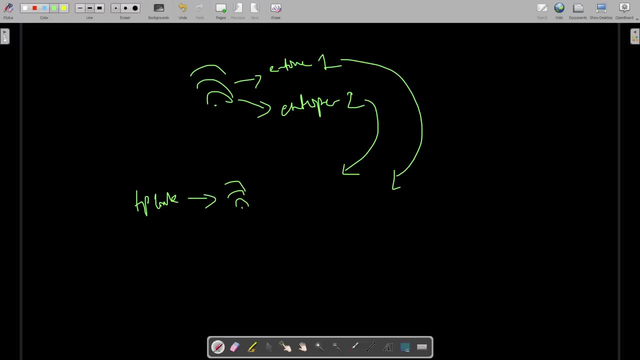 Now the thing is here: By using the manage mode- Okay, What is a manage mode? Manage mode is a by default mode. Okay, This is a thing which you need to remember. By using manage mode, You guys are, You guys can able to surf the internet. 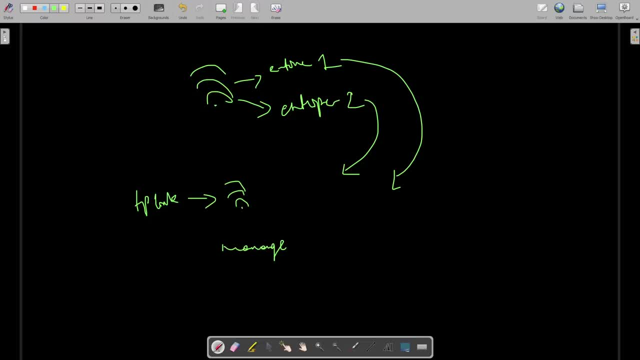 Okay Now, manage mode Is responsible To connect with the Wi-Fi networks, So you guys can able to use the internet. This is a default mode. Okay, Now there is another mode, Which is what It's? a monitor mode. 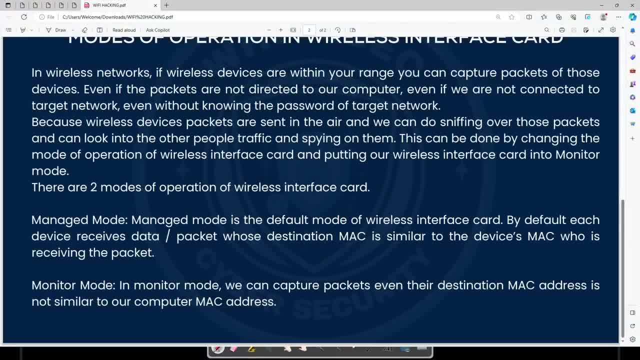 In monitor mode We can capture packets. Even the destination MAC address is Not similar to our computer MAC address. In a simple words, You guys can able to capture The packets of other. This device, This Wireless networks, Okay. 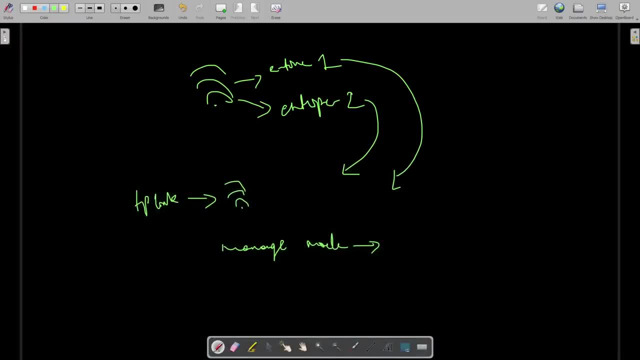 Like a wireless access points. Just see Monitor mode Is a nothing but To capture the In a simple words Here What we are, What we just learn here. See Where it is Okay If wireless device Are not within your range. 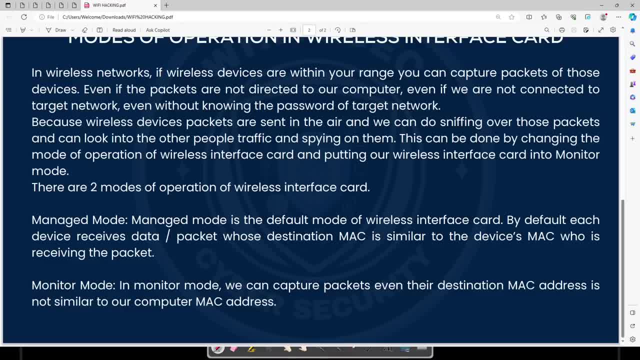 You can capture the packets. In a simple words Here, What we are, What we just learn here, See, You can capture the packets, See, If your wireless device Just focus on this point. So that's why I just told you. 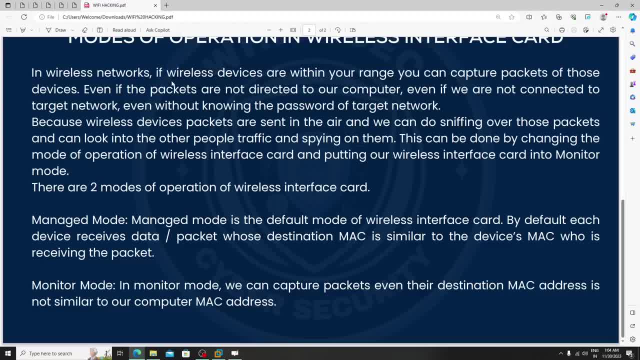 I am gonna explain this again. Okay, If wireless device Devices are Within your range, You can capture packets Of those devices. Even the packets Are not Directed To our computer. Okay, Even If you are not. 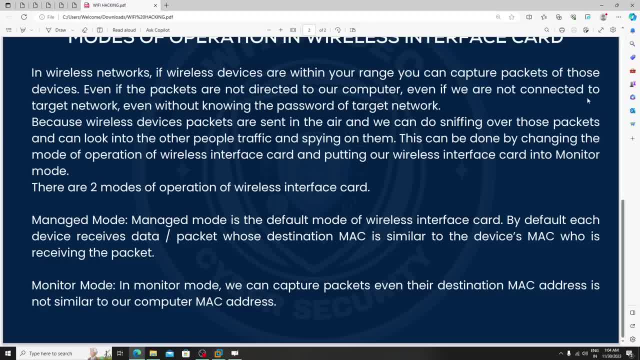 Connected To the Target network Even Without knowing the password Of the target network, Because Wireless device packets Are sent in the air And we can Do sniffing, Like We can able to see that What is a sniff? 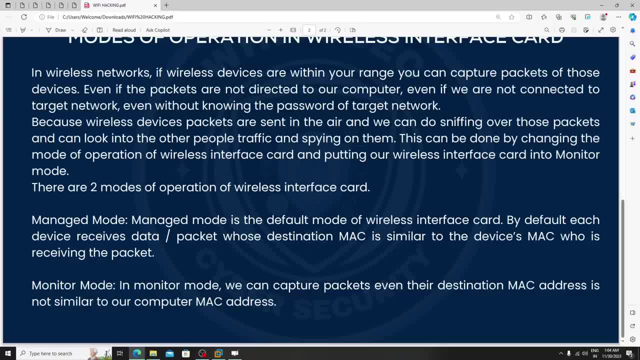 Okay, You know about sniffing Right Okay, Over those packets And can look into the Other people Traffic. Okay, And spying on them Simple, Without connecting with, Without having the Your target password, Assume that. 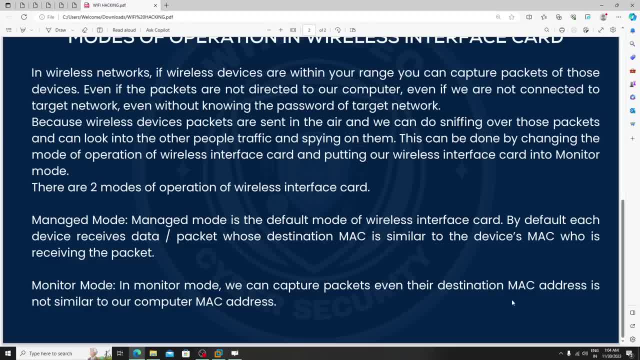 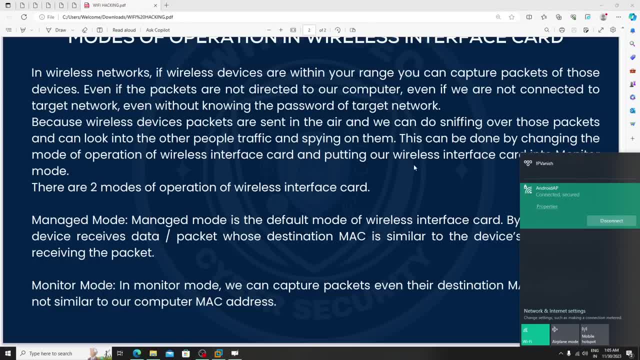 If you want to. In a simple words, I am saying: Assume that If I I want to hack this Android AP network Simple, I no need to connect with this network. Okay, I can able to perform The attacks on it. 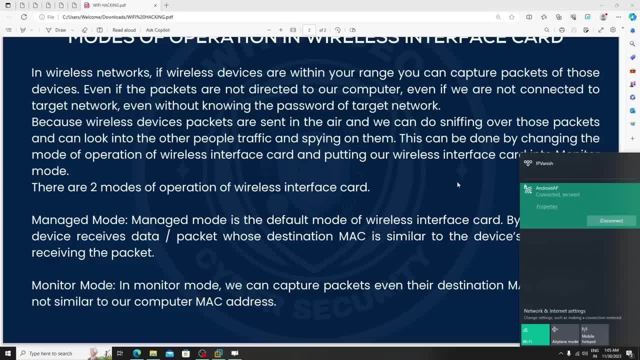 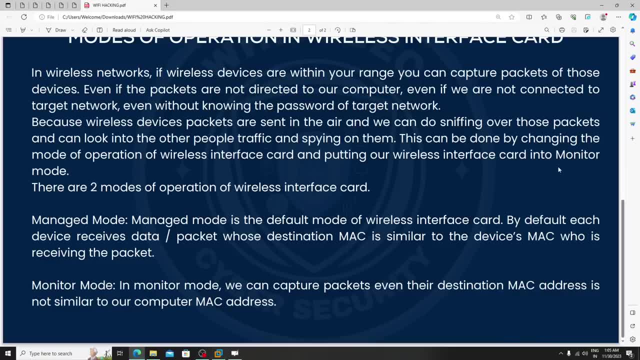 Okay, We will see How we can able to perform This, all stuffs. But the thing is Here, Monitor mode Is Very important for you. Without monitor mode You can't able to do the Hacking here. 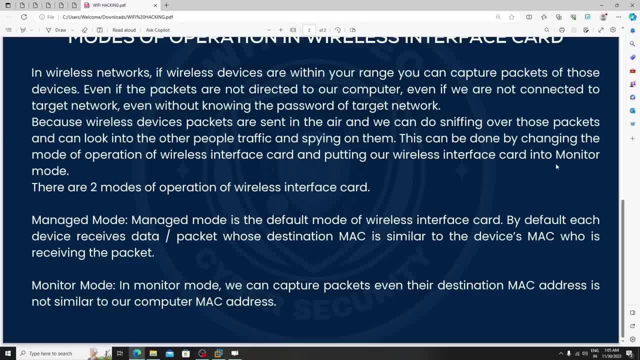 Okay, Simple words. Monitor mode is Responsible to Perform this Whole attacks. Okay, Like you can Able to capture The packets, Something like that. You can able to capture The handshake. You can able to perform The deauthentication. 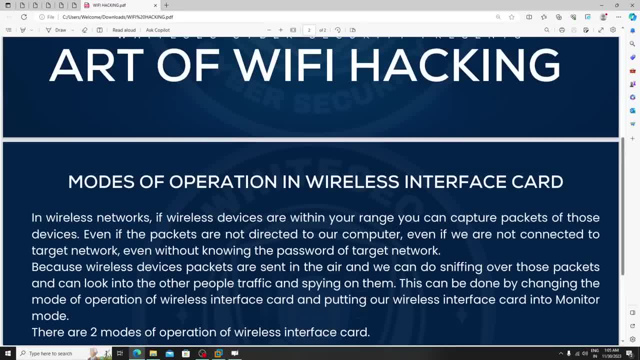 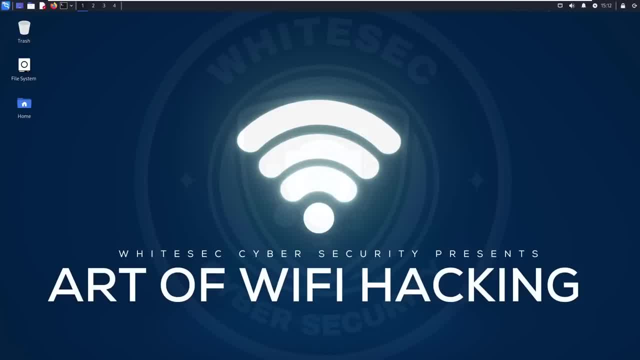 Attack Practically In the next class, Right. Hope you guys get it. You will get the PDF, Don't worry. Thank you, Have a nice day. So in this class We are learning How we can able to. 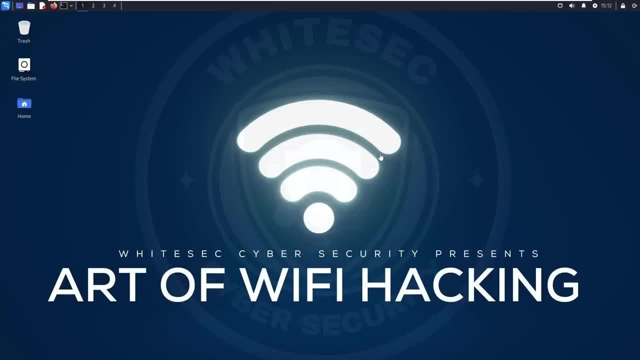 Set our Adapter- Wi-Fi adapter- in Monitor mode. I just told you. Normally, By default, The Adapter is in Manage mode. Okay, So let me show you That one as well. See, The thing is. 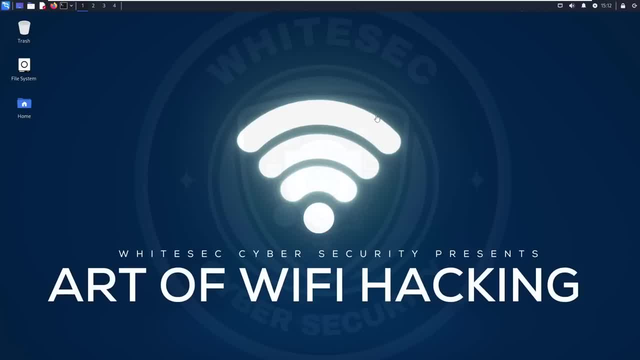 You need to connect Your Wi-Fi adapter With your computer Or laptop Or Vm. See Why we are doing This whole process Simple. We are running The Kali Linux In The VMware Workstation. 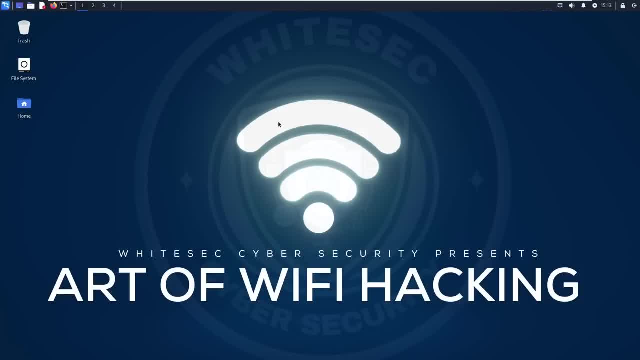 Right. So that's why. That's why We need to do this process. Okay, Assume that If you just connected Any hack, Hack, RF Or some other Hardware, Same process You need to do. Okay, You need to connect. 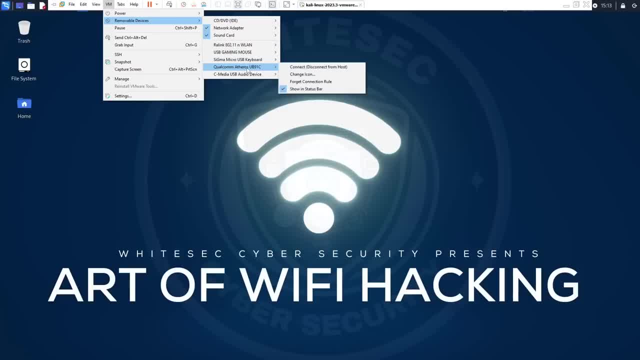 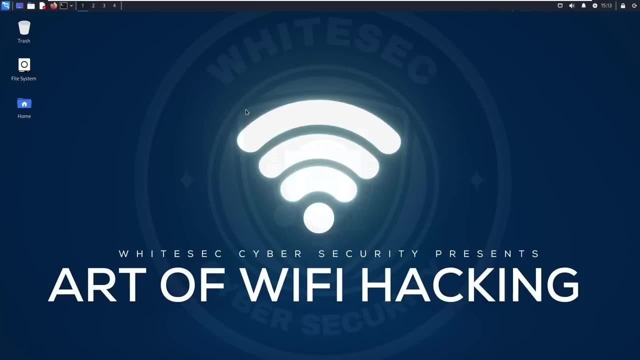 Here. Okay, Simple. Now Let me Disconnect My Wi-Fi Adapter From here. Okay, After Disconnecting The Wi-Fi Adapter, See If I Click On The Vm You. 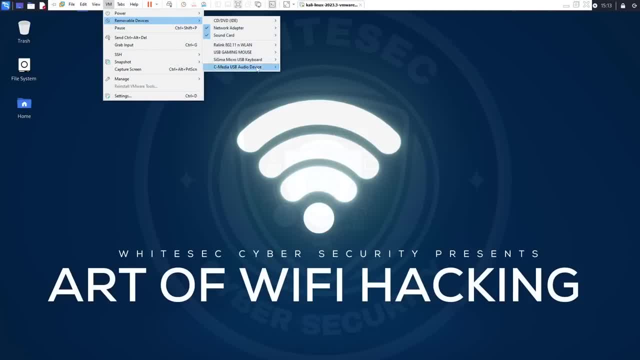 Can't Able To See The Arteros. Okay, So This Is. So Let Me Connect Back Here, Okay, Before Doing That Process Simple, Just Let's. 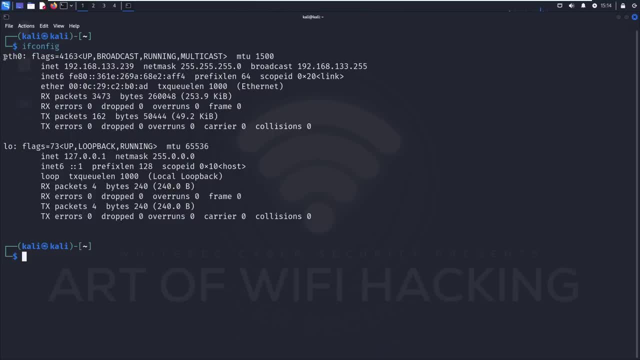 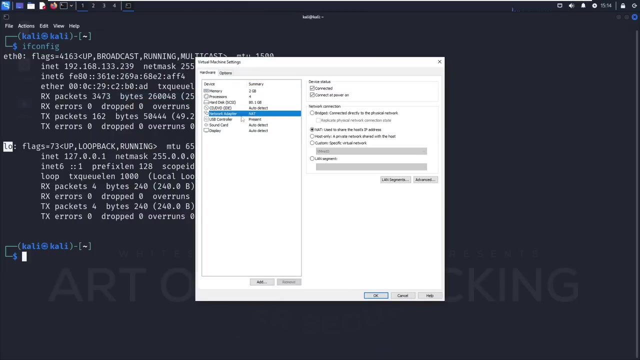 Open The Terminal. Okay, Let Me Zoom This One. If I Type, If Config Here System, Okay, This Is A Thing, Because Right Now We Are 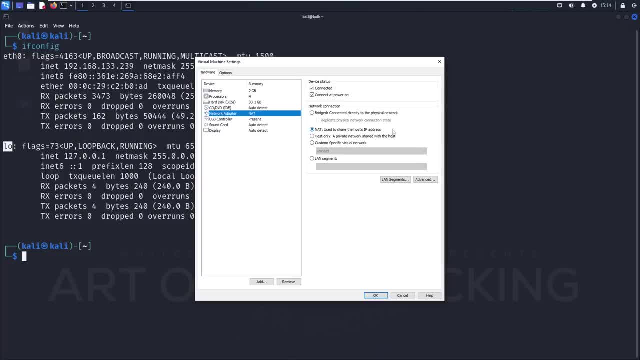 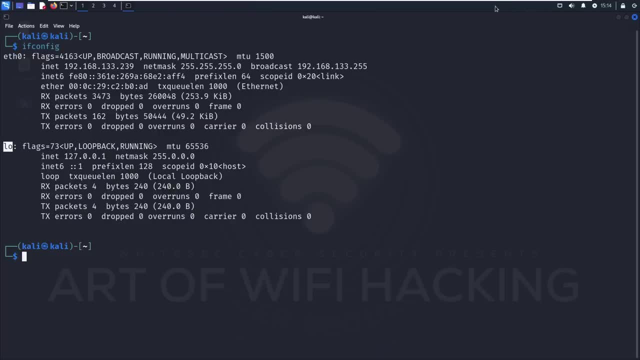 In Not Network. Let Me See. Click On The Settings. Okay, Right Now I'm Using The Not Network Just. I'm Not Saying You About Just. 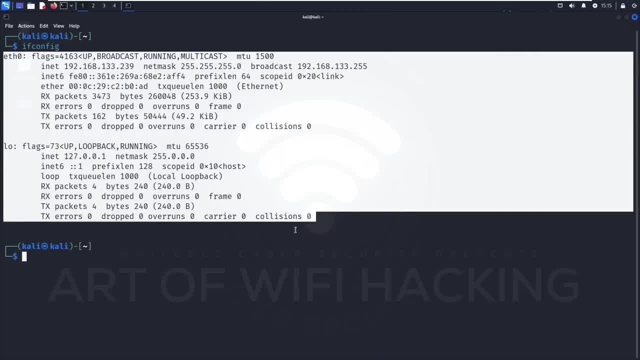 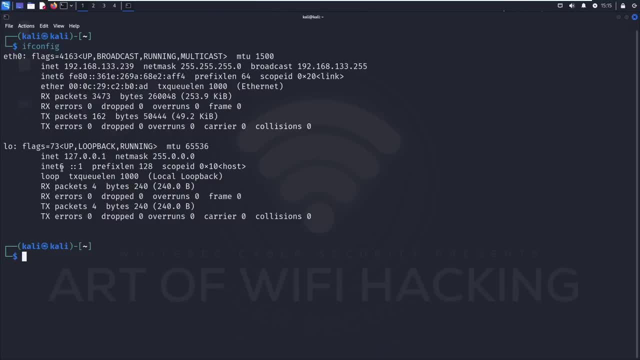 Learn About This. Also Simple. Just See Right Now, There Are Two Networks. Are There- Okay, Sorry, Two Interfaces Are There? One Connect. So You Guys, 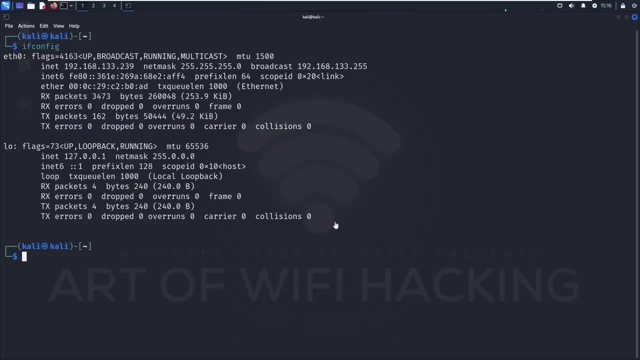 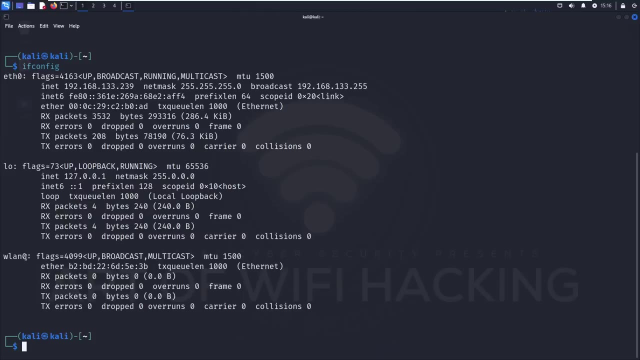 Can Able To See This Kind Of Popup. Simple Click On Okay There, Then See Previously, I Just Execute The Same Command. If Config, If Let's. 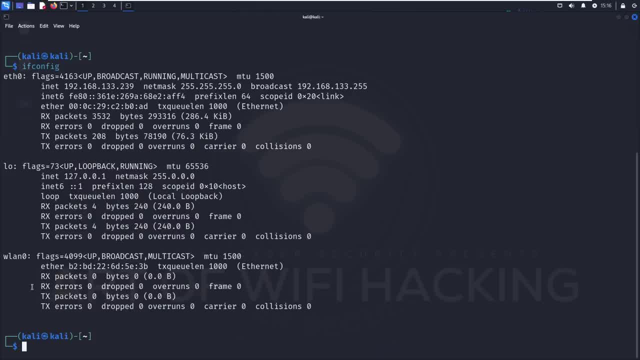 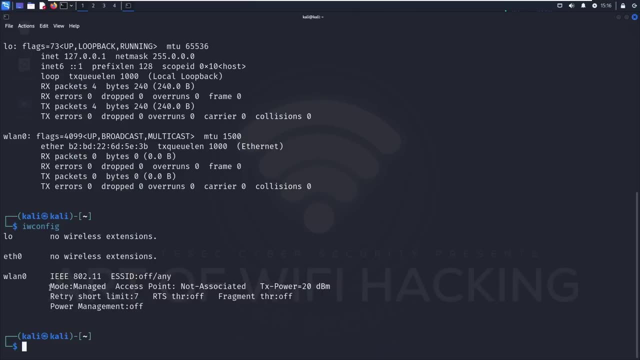 Learn. First Let's Learn About The Manager And Monitor Mode. See If I Type I W Config Previously, I Just Type What If Config Now. 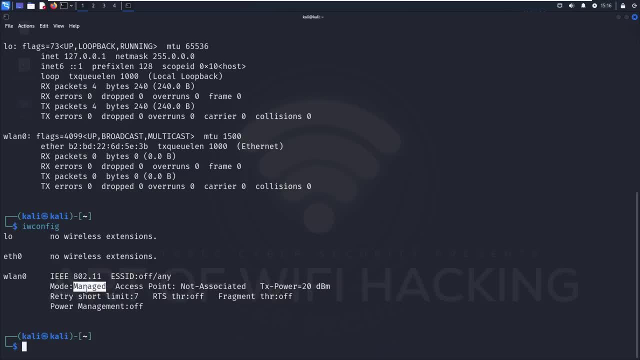 I Am Typing: Change This Manage Mode To Monitor So We Can Able To Use Our Wifi Adapter For Hacking Purpose. Okay, How To Do. 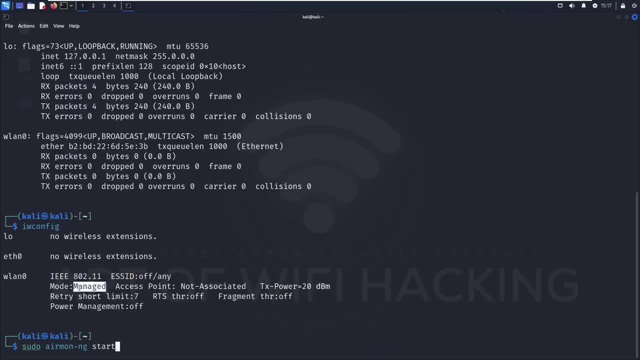 That The Simple Thing Is, You Just Get, If You Get W1. There, Okay, At That Time Uses The Name There, Okay, This Is A. 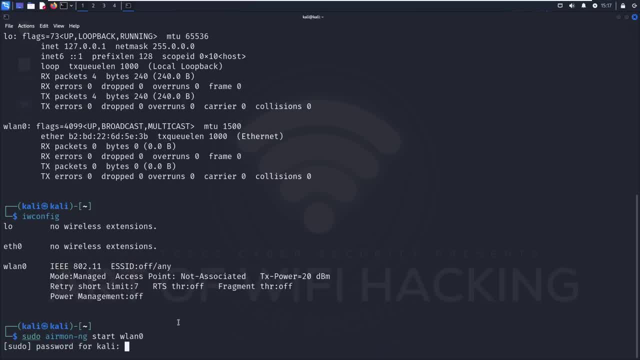 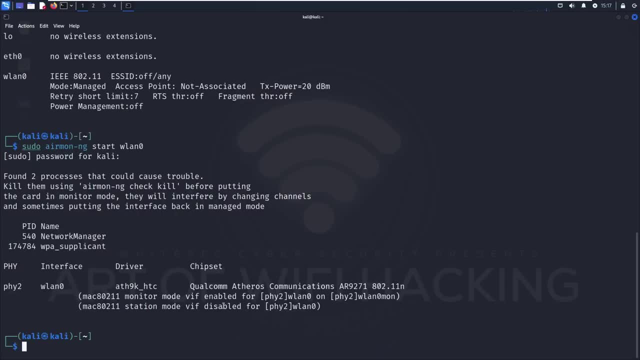 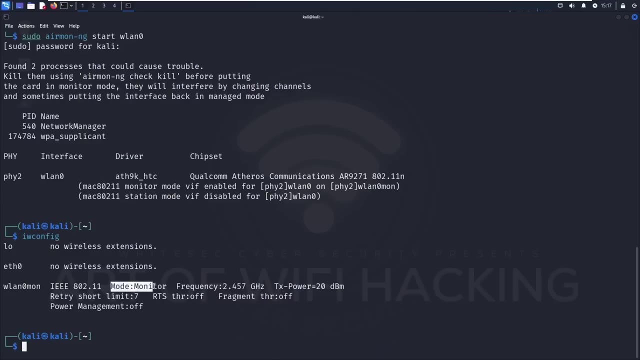 Thing Now Here, Just Just Type It: Copies Totally Depend Upon Using Again. Here You Guys Can Able To See The Mode. Is What? Here Some 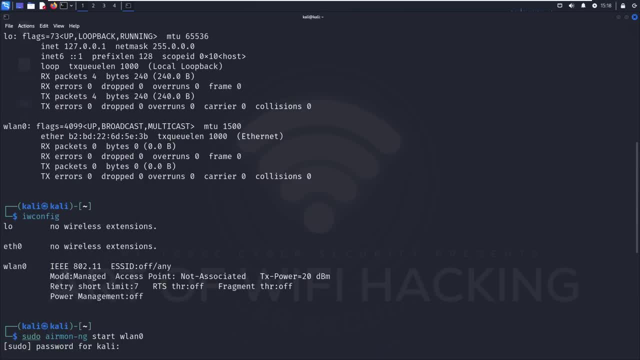 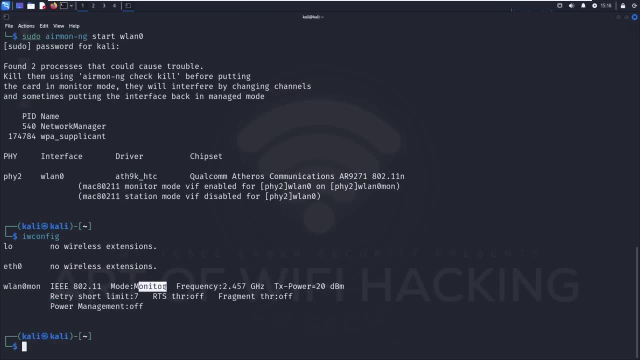 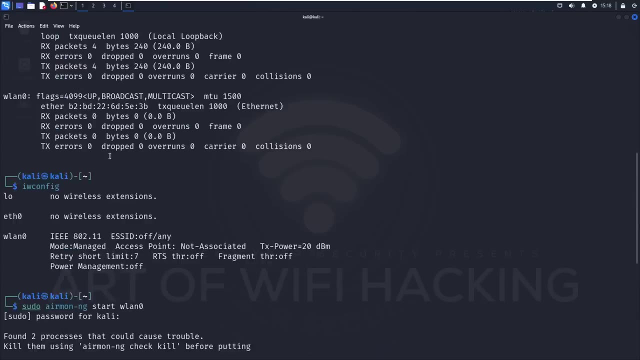 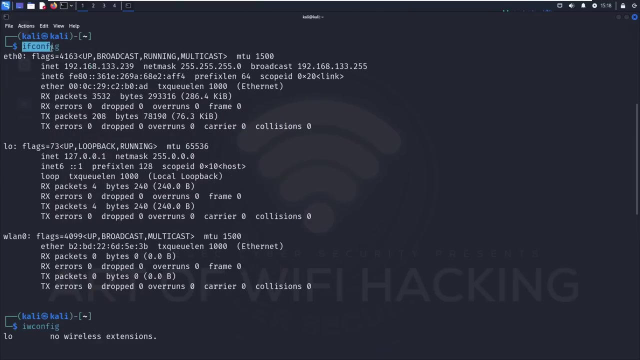 Monitor. Now I Can Able To Use This Wifi Adapter For Hacking. Purpose. Simple Now See Here Previously After See. After Connecting The Wifi Adapter. 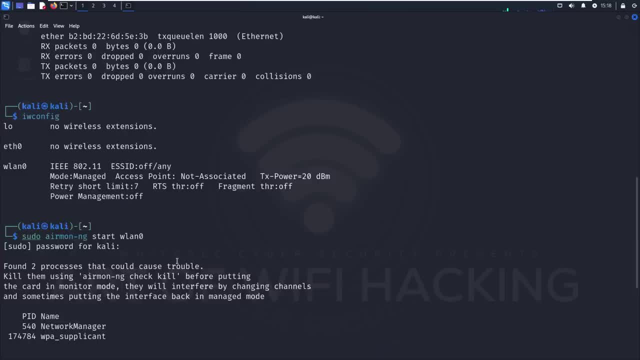 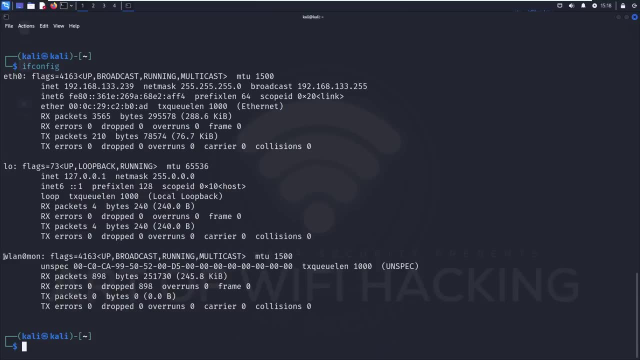 I Just Type The If Config Right Here. I Can Able To See. The Interface Name Is WLAN 0. Mode. If You Are Using TP. 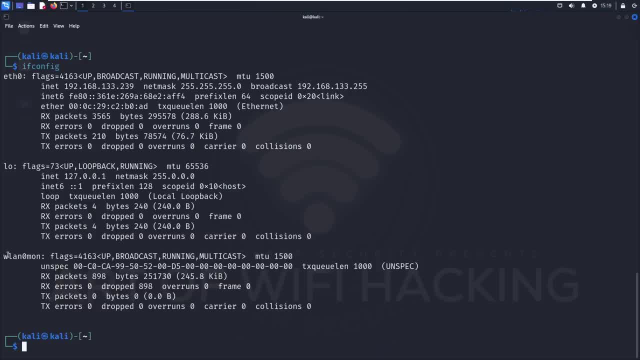 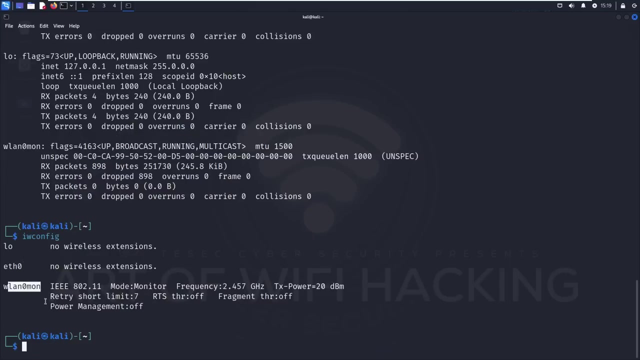 Link, Then The Adapter Name Will Won't Change. Like If You Are, You Just Change Your Adapter To Monitor Mode. Still, The One Is Monitor. 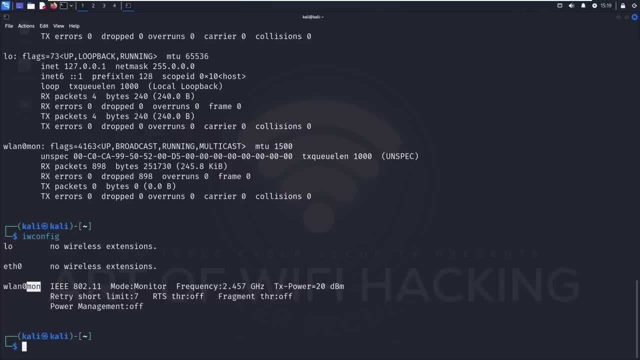 Okay, In Your Case It Might Be WLAN 0. If You Are Using The TP Link, You Won't See This Extension. If You Are Using. 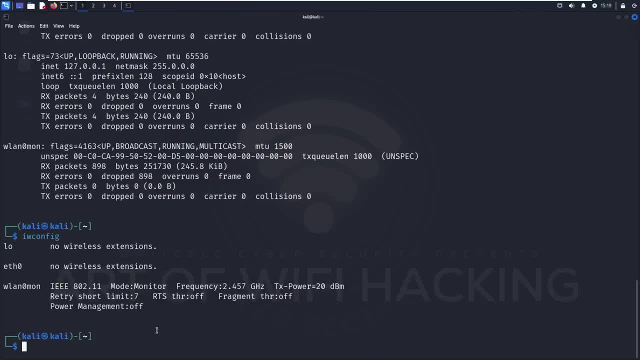 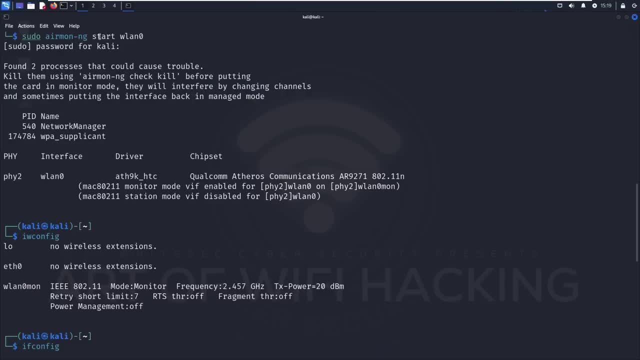 TP Link. Now I Will Start WLAN 0.. Okay, Simple, This Is A Simple Command. Okay, If I Want To Stop? Okay, Then I Need. 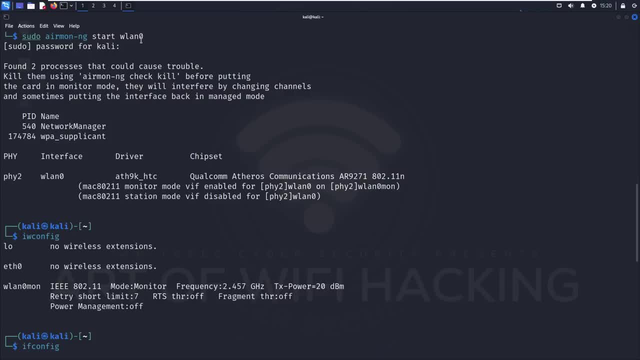 To Add The Interface Name. If You Are Doing The Monitor Mode, The Interface Will Get Changed Right. Mostly It Won't Okay If You Are. 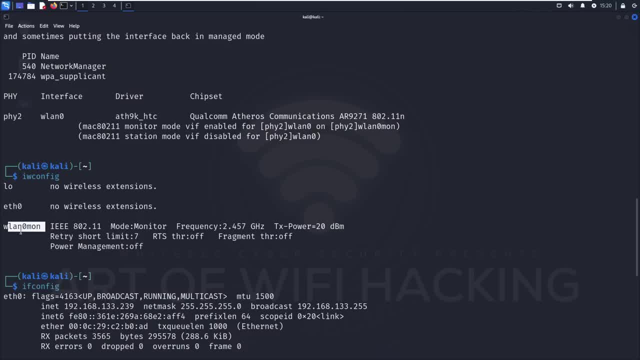 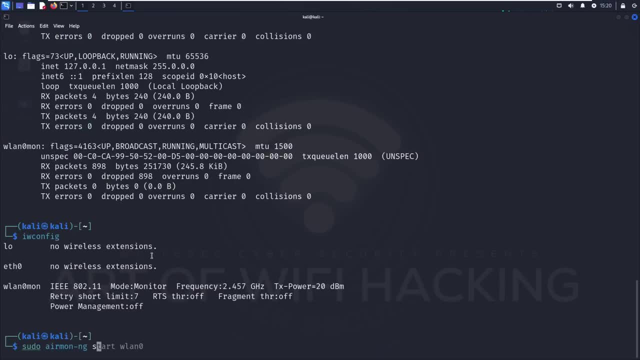 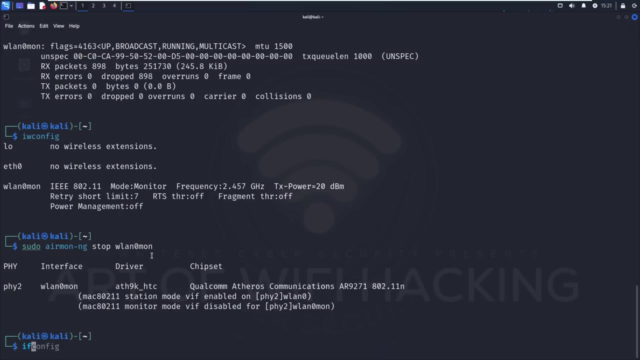 Using The Alpha Adapter Or Some Other Stuff, Then Set Off, Start. I'm Gonna Type Stop. Then What Is A Interface Here? Interface Is WLAN. 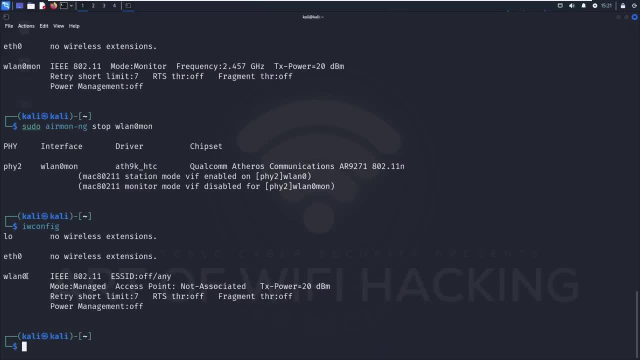 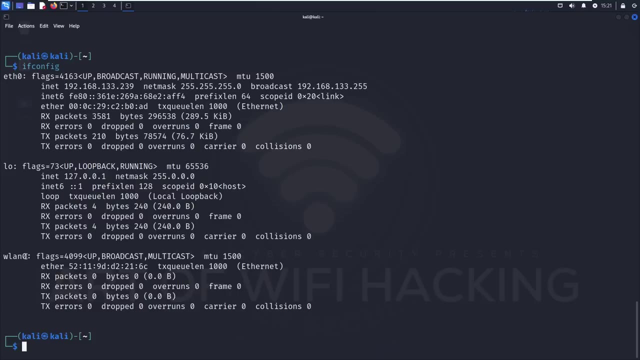 0.. Then I Need To Add The Moon As Well. Okay, This Is How You Guys Can Able To Change Your This Adapter To Manage. 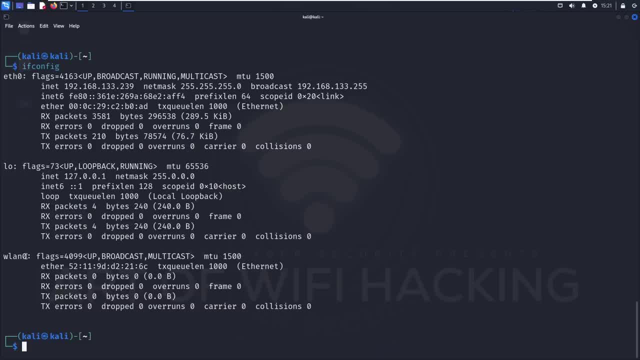 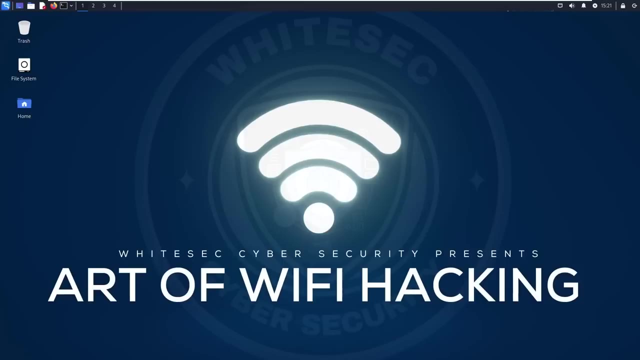 Our Monitor Mode. Okay, This Is A Very Easy Things. You No Need To Worry. Assume That WPS Attacks. WPS Attacks Includes Any Attack. 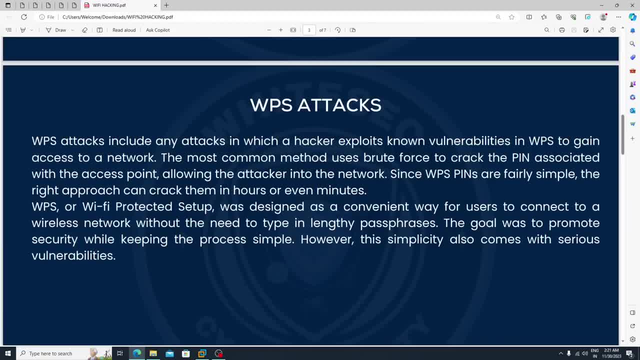 In Which A Hacker Exploits No Vulnerabilities In WPS To Gain Assist To A Network. The Most Common Method Uses Brute Force. The 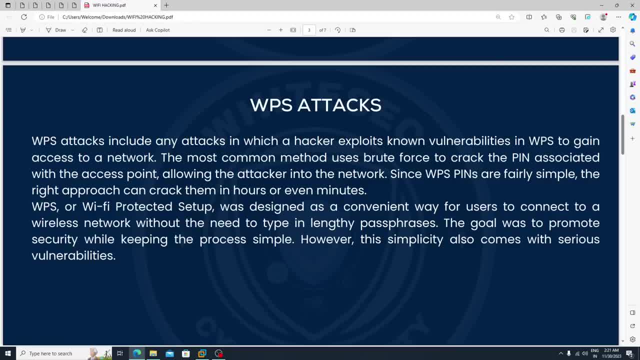 Right Approach Can Can Crack Them In Hours Or Even Minutes. Let Me Tell You, Even In Seconds, You Guys Can Able To Crack The WPS. 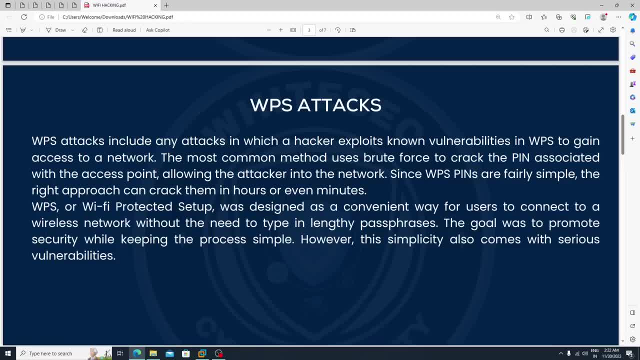 Pins. Okay, Six, Seven, Eight. Mostly The People Who Don't Know About This, Things Like Hacking, Or They Don't Know This Kind Of Service. 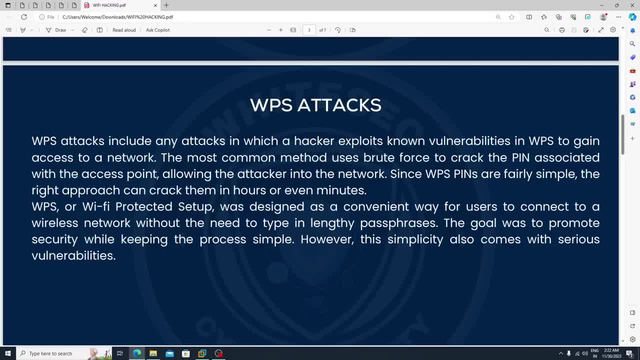 What They Do Means They Won't Change. Okay, The Goal Was To Promote Security, Well, Keeping The Process Simple. However, This Simplicity Also Come. 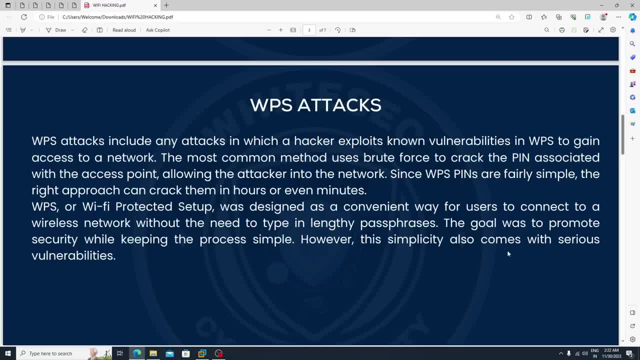 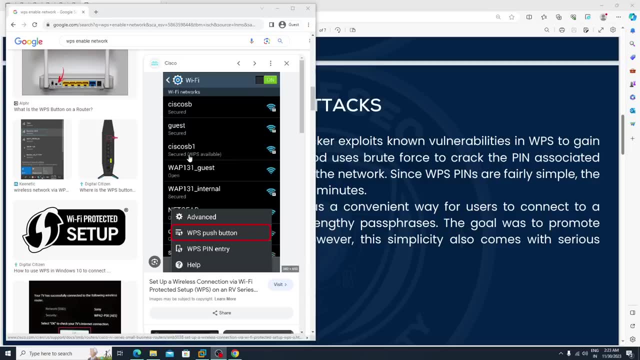 With The Serious Vulnerabilities. Okay, This Is A Thing, It's A Very Clear One. WPS Available Is A Right. If You See This Thing. 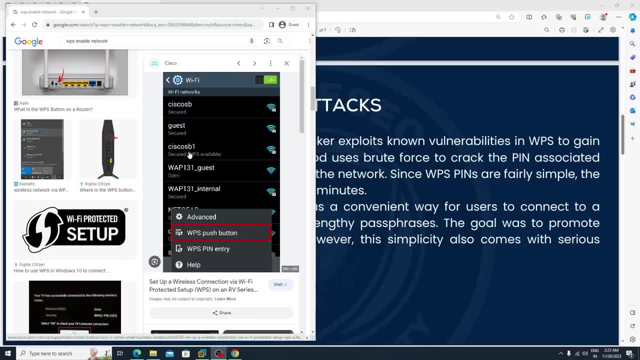 Then The Network Is Very Easy To Have. This Is A Thing Okay, Mostly You Will See This Kind Of Things That You Need To Use. 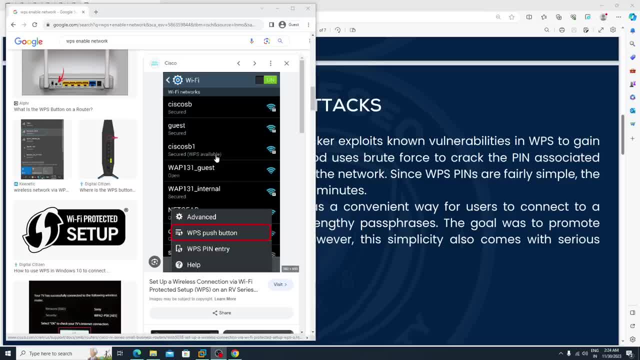 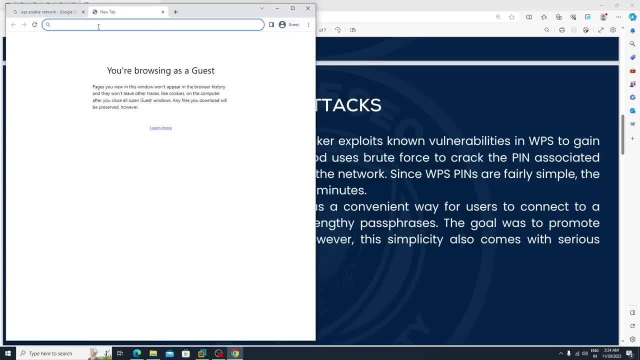 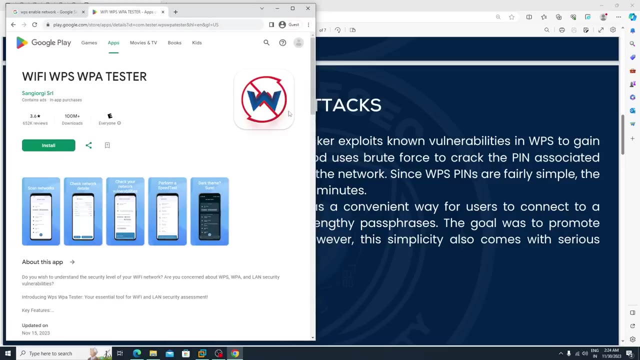 The Kali Linux For That Simple. You Can Be Able To Hack Those Networks By Using Your Mobile Phone. Which Application Mostly We Use This? 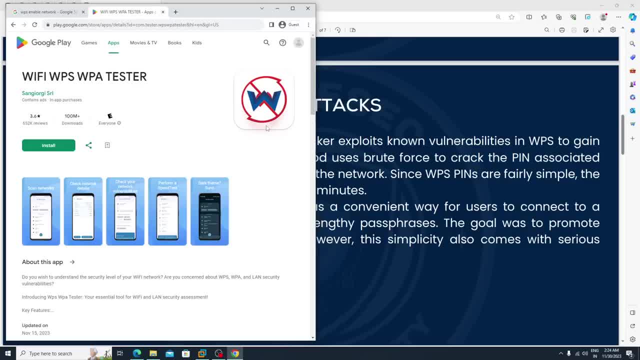 Application. Okay, Simple, By Using This Application, You Can Able To Hack It. Okay, This WPS Network. But Let Me Tell You, Sometimes You Can't. 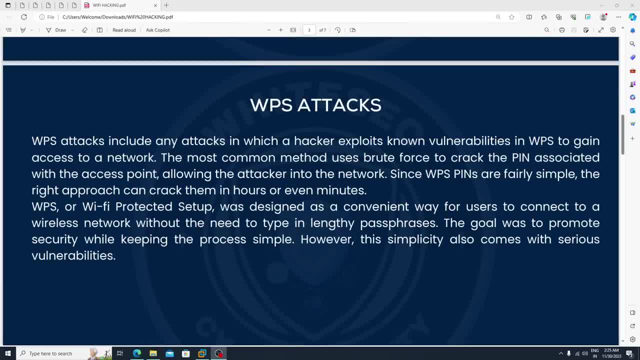 Able To Crack Other Process Or There, By Following Those, You Guys Can, Able To Do The Attack. Okay, Now, Here The Thing Is See Basically: 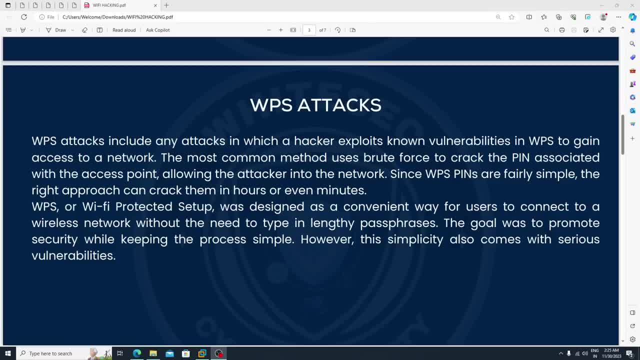 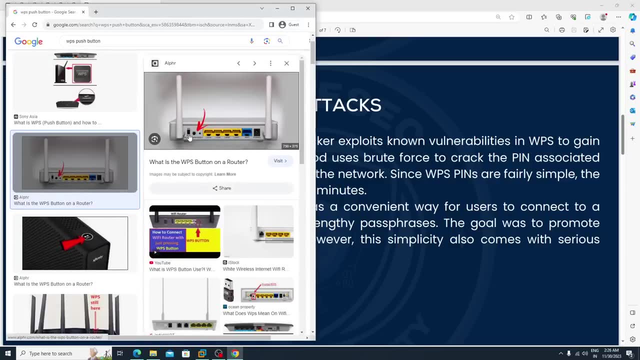 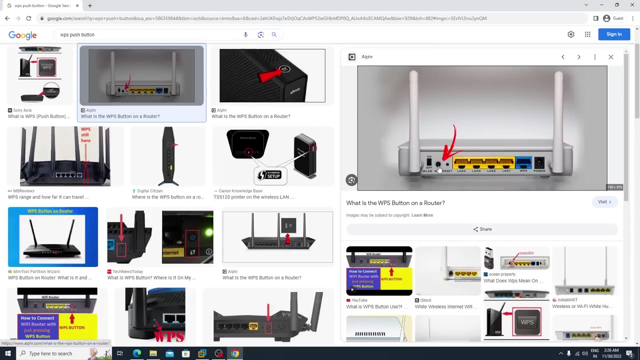 This WPS Thing Is For You Can Able To See The WPS Push Button There. Simple If You. Let Me Show You That One As 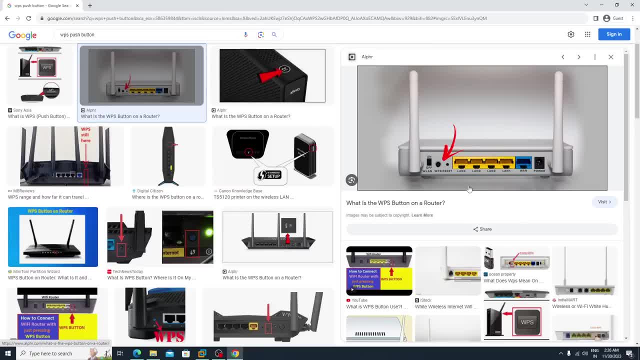 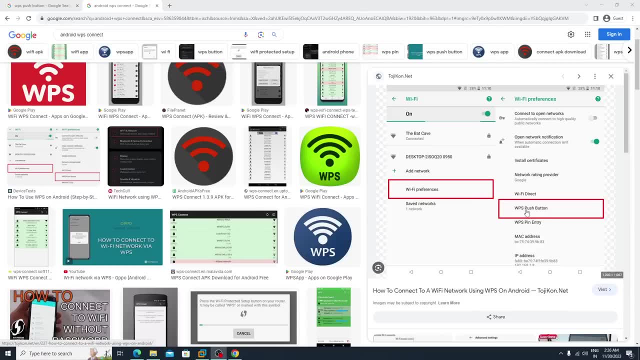 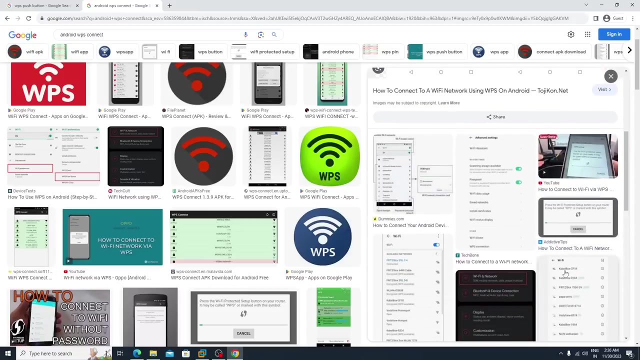 Just See Here, In Every Router. Okay, You Guys Can Able To Connect With This Router. Okay, Now Let Me Show You How To Connect With. 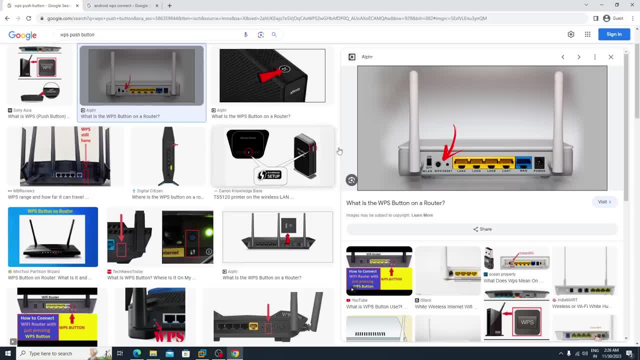 This Router, Okay For Three Seconds To Mostly It's For It's Take Three Seconds To Connect With Your That Router. Okay, Without Typing Any. 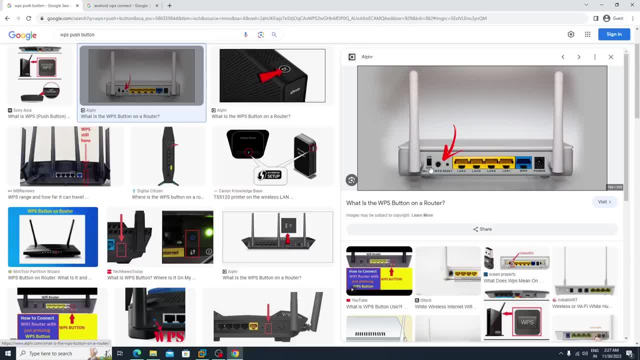 Kind Of Password. So This Is How This Is Going To Work. Okay, Once You See The WPS Or Office, And We Can't Able To. 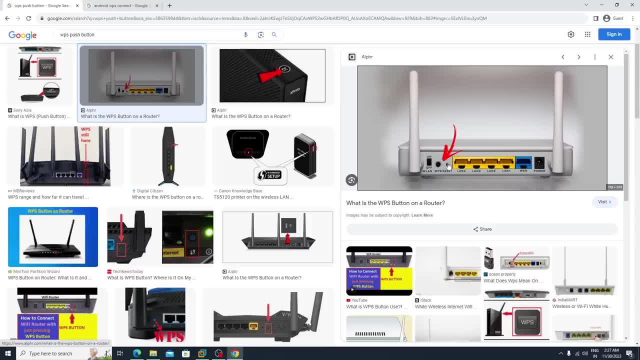 Click There. Okay, It's A We Can't Able To Do This Process. Okay, So That's Why There Are Some Scripts. Are There Simple Within? 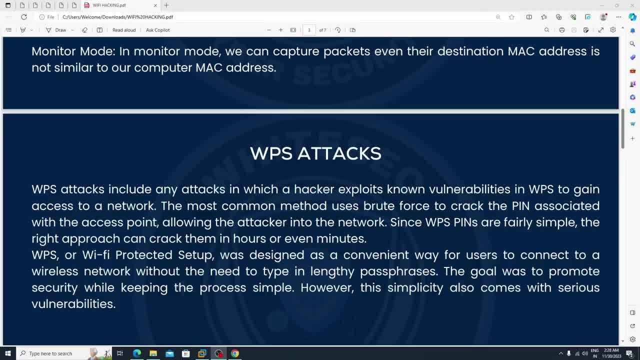 Few Clicks You Guys Can Able To Hack This WPS Attacks Mostly. You Will See, Just Just Visit. I'm Gonna Show You How You. 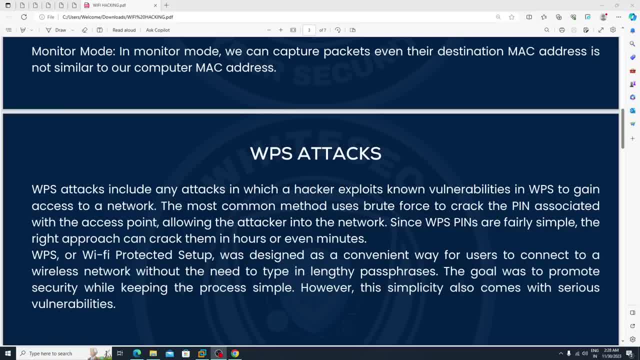 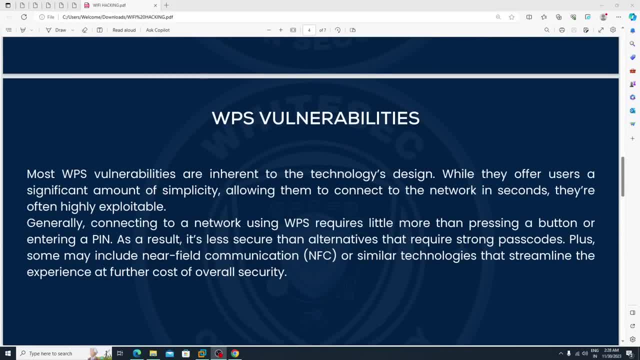 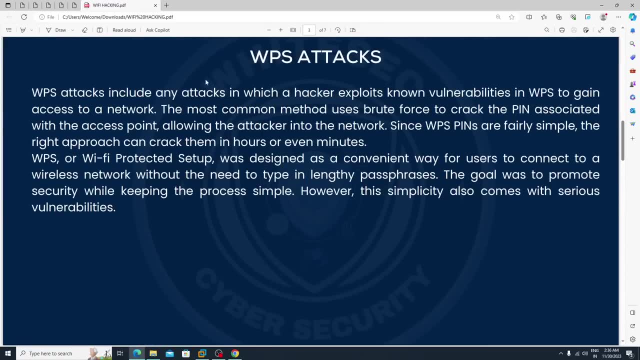 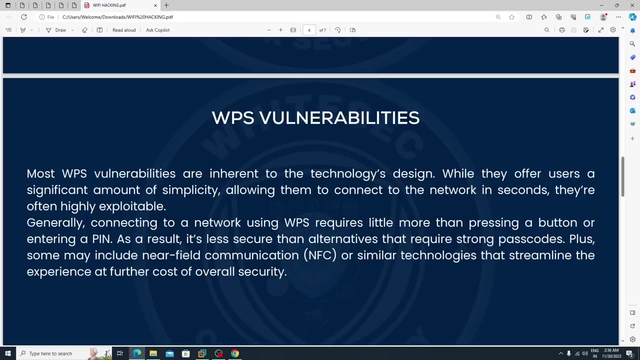 Guys Can Able Now. In The Next Classes We Are, We Will Learn About WPS, Vulnerable Days. So In This Class We Are Learning About. 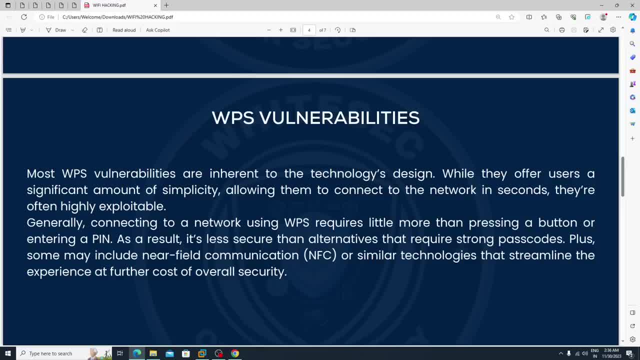 WPS Vulnerable Days, Which It's A Same Little More Than Pressing A Button Or Entering A Pin. As A Result, It's Less Secured. 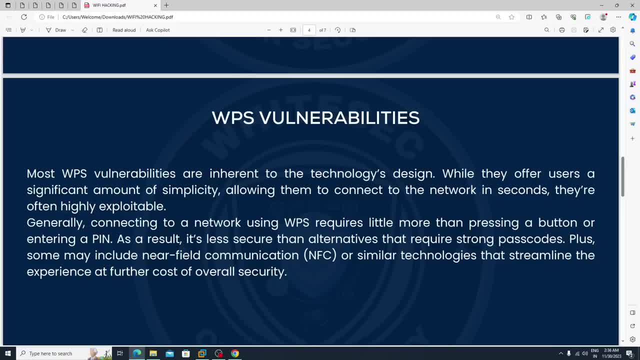 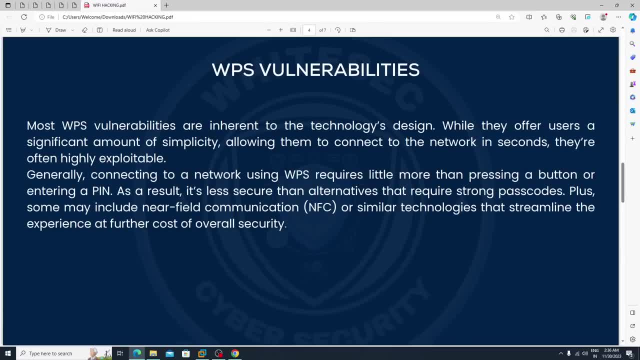 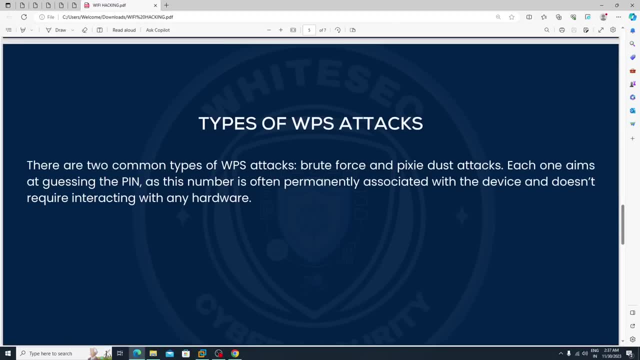 Than Alternates. Alternatives That Requires Strong Pass Codes. Pass Codes Okay, Plus Some Different. See, There Are Two Common Types Of WPS Attacks: Brute. 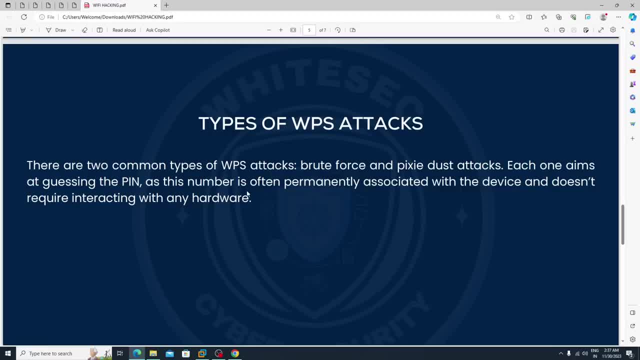 Force Attack, Fix, Industrial Attack. Okay, Each One Aim At Guessing The Pin, As This Number Is Often Mostly The People. What They Do Means. 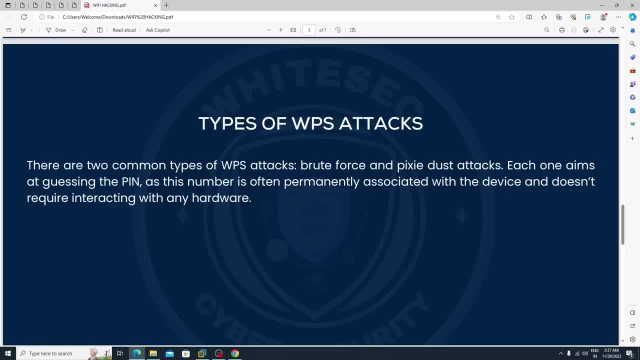 They Won't Change A WPS Pin There. Mostly The W By Default WPS Pin Is One, Two, Three, Four, Five, Six, Seven, Ten Eleven. 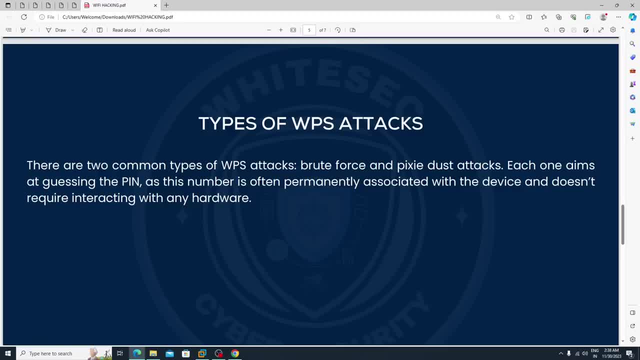 Ten, Ten. So What You Are Using Of These Pins To Crap. Now Just Assume Your Victim Is Using A Different Pin. Okay, In Every. 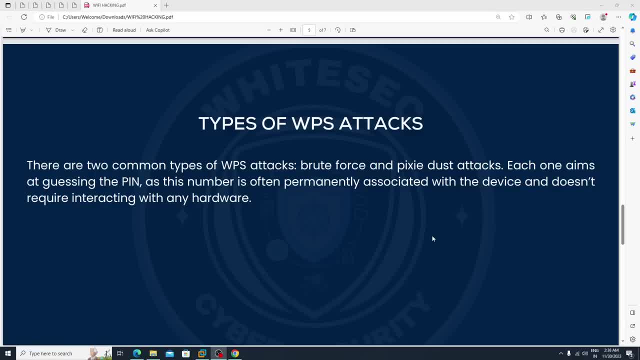 Router, There number or something like that. we don't know that. okay, the simple things at the time. what we do means we perform the brute force attack. mostly, the brute force attack will work. okay, once you are targeting the wps network, brute force attack will work. and let me tell you again: don't uh panic. 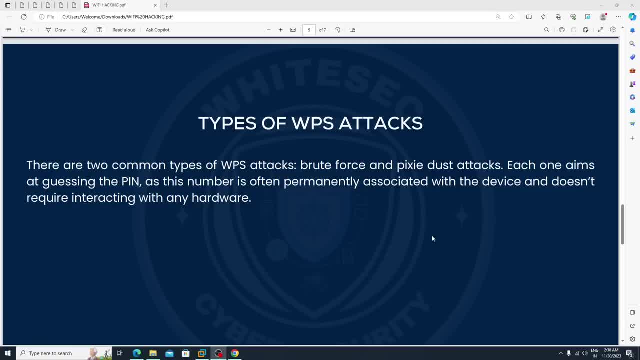 okay, once you see the wps network, it is very easy. okay, people will think that, okay, maybe in training you are cracking it because you know the password or something like that. no, in real world also. okay, once see. uh. in pentesting and redeeming what i do means once i grab the, this hashes. okay, this uh. 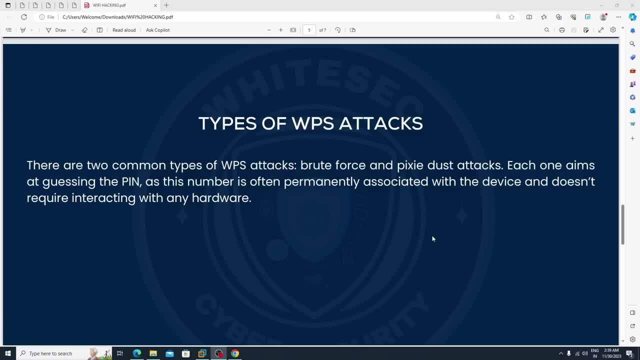 how i, if you, if you watch this ethical hacking or windows pentesting training what did? what we did there means we just capture the hashes. okay, to crack those hashes, it sometimes it will take around 15 days. okay, this is the thing. this is my work. okay, as a red teamer, this is my work. i. 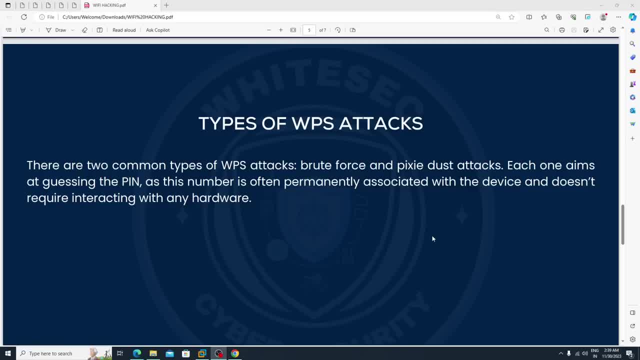 i continuously need to do the process like i don't do that simple. i uh, there are graphic cards, are there? okay, simple, i just use a hashcat to crack it. thus the thing is, i can able to crack it, but it will take a time. this is the thing which i want to tell you. 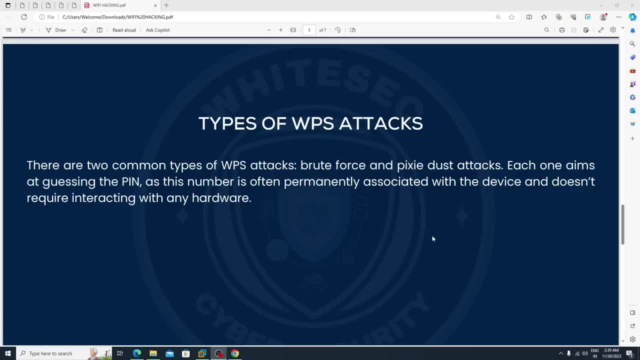 okay, it will take a time. don't think that brute force attack never uh will not work. okay, it will, because i am a pentester man. okay, like uh sometimes, yeah, uh, it will take a huge time. okay, this is the thing. sometimes three days, okay, sometimes it will take uh, uh, yesterday only okay. 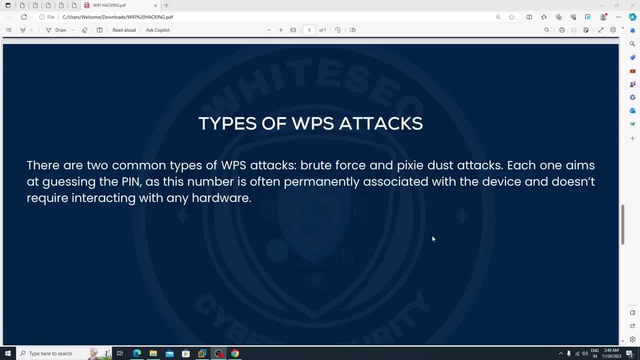 it's to- uh, it's take around seven, seven hours. okay, this is the thing, so the thing or this will work, but you need to implement these things. okay, don't learn this and live it. okay, just implement these things in your own network and just try to do it. okay, if you have a good amount of graphic card. 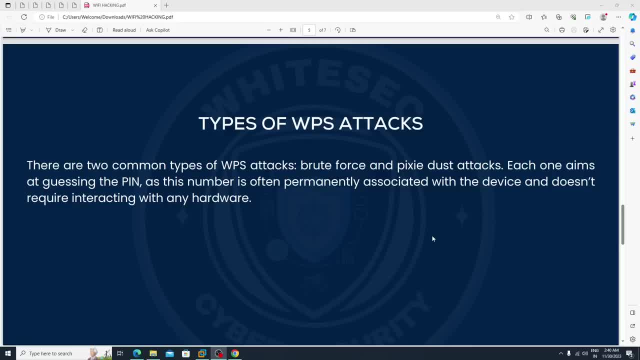 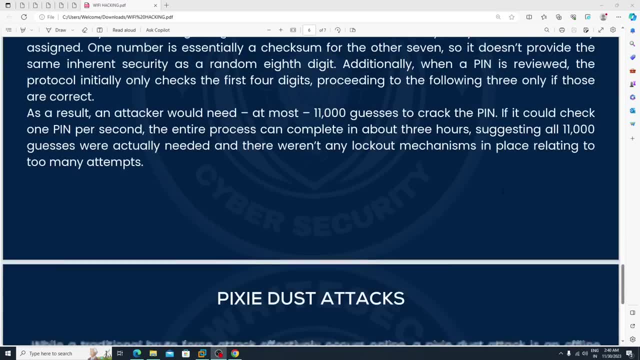 good, okay, like you can able to crack it any any hash. okay, right now let's learn about brute brute force attacks. okay, uh, maybe in the next class we will see this one. the definition: right now it's four minutes. okay, just just, let's see in the next class. 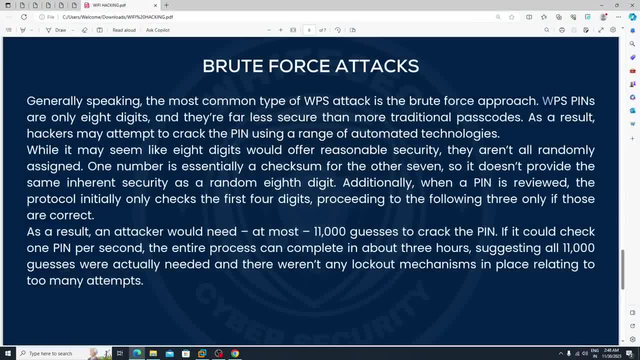 now in this class we are learning about brute force attack. generally speaking, the most common type of wps attack is a brute force approach. wps spins are only eight digits. just focus this point in your drive over. here we can use the wps pin for wps or only eight digit, and there are far less. 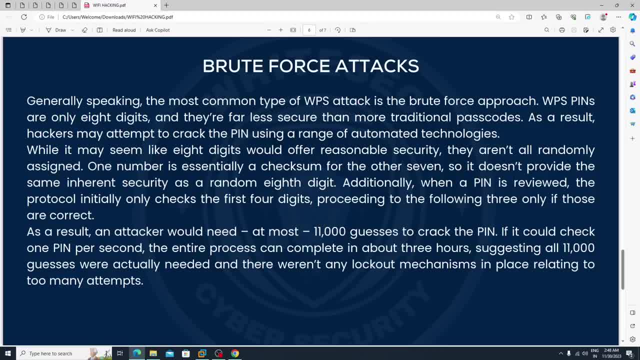 secure than more traditionally? uh, traditional approach, sorry passcodes. as a result, hacker may attempt to crack the pin using a range of automated technologies. fail, it may seem like eight digit would uh offer reasonable security. yeah, okay, or randomly assigned. one number is essentially a checksum for other seven. this is a thing. 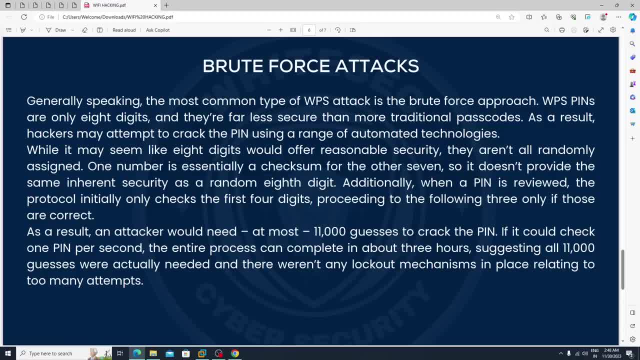 it doesn't. it does not provide. it doesn't provide the same inherent security as a random eight digits. additionally, when a pin is revived, the protocol initially a only checks the first four digits. this is the thing here. process proceeding the to the following three only if there are correct. if you 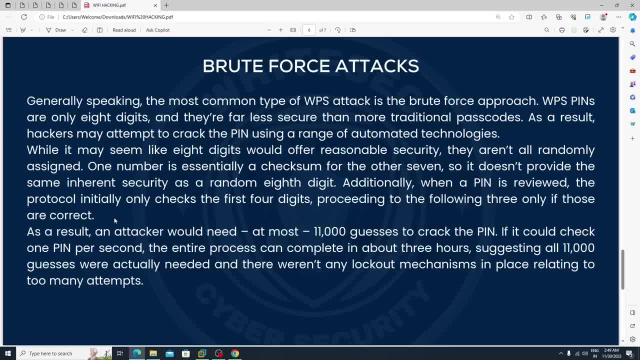 are not getting this, then what you need to do? simple, you no need to worry. okay, the process is completely done by the scripts. okay, just try to read the definition, because it's a little bit confusing, but it's not a hard. okay, it's, it's not a big deal. now see, this point is very easy for you. as a result. an. 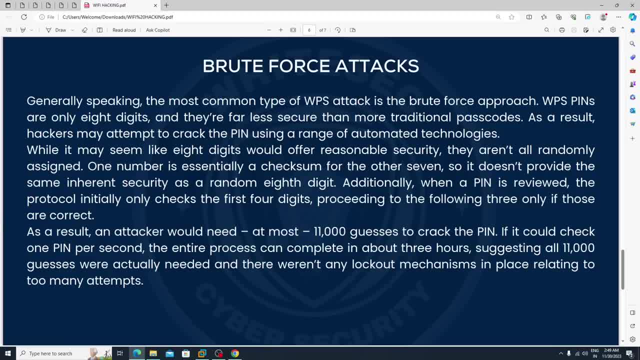 attacker would need at most 11,000 guesses. if you want to crack anything- this thing- then you need 11,000 guesses to crack the pin. if it could check one pin per second, the entire process can complete in about three hours. okay, it will take a horse. I just told you. 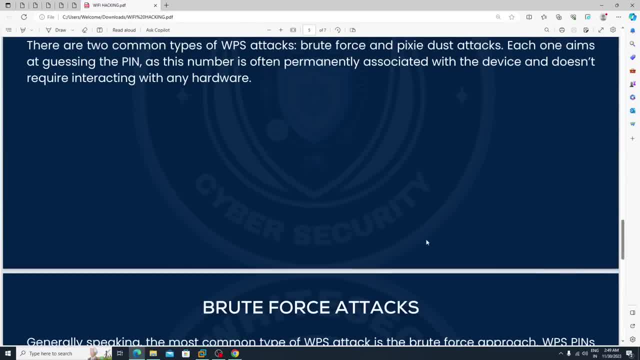 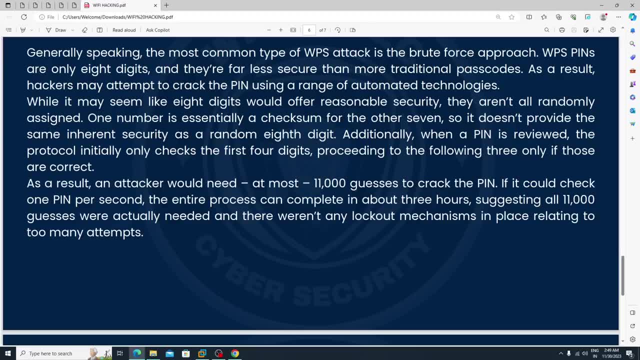 right here, also suggesting all 11,000 guesses were actually needed and they weren't. any lockout mechanism. there is no, any kind of lockout mechanism in place relating to many attempts. see, sometimes what will happen means it might be a lockout. sometimes there is a lockout mechanism. is there okay, once you? 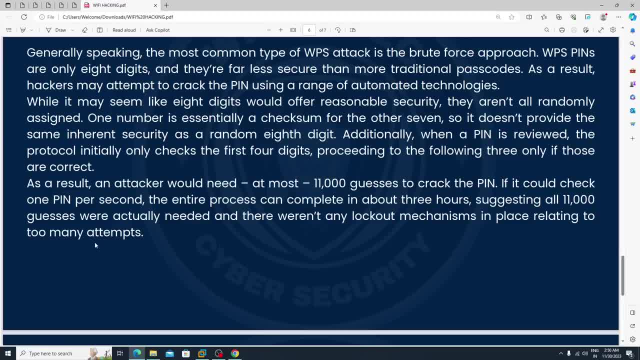 just attempt the brute force continuously. you just send it the perform brute force attack on the router, then what will happen means the router will get lockout. okay, they, they just stop your request there, okay, in a simple words, what you need to do simple: you need to send the d authentication package to the. 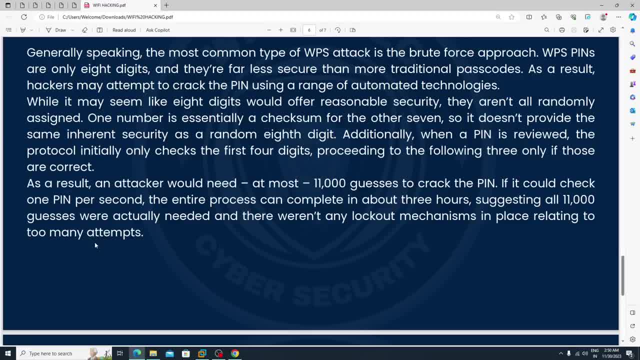 network that router. so what will happen? is it? the clients who are connected with that network will get disconnected, but with that network, so they will restart the router again. okay, this is the thing. it's not a big deal. okay, you will learn deauthentication- how to perform it. it's not a big deal. the simple thing is, if the lockout mechanism 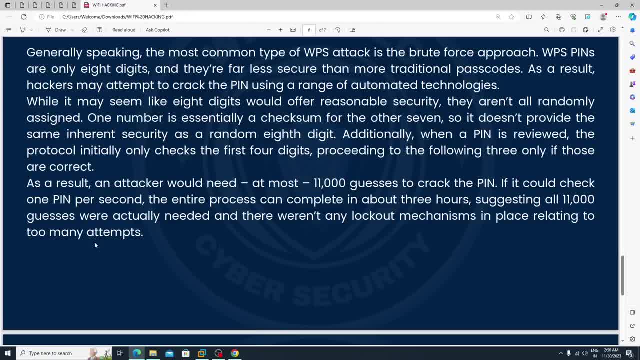 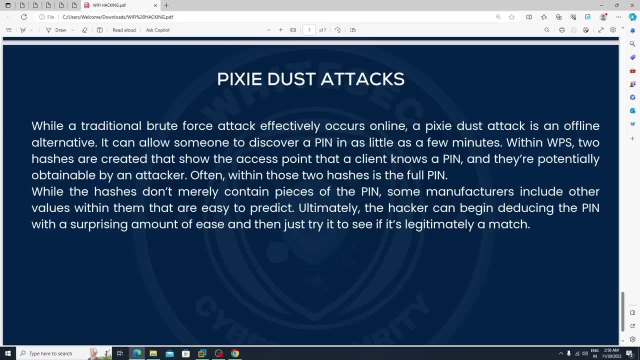 is there in that router, then you need to send the deauthentication packets to that router so they can restart it. okay, this is the thing, pixie dash attack. well, a traditional brute force attack effectively occurs online. a pixie dash attack is an offline alternative. it can allow someone to discover a pin in as little as few. 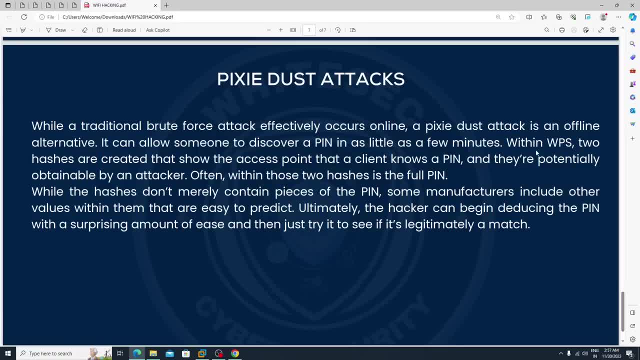 minutes. within wps two hashes are created. that shows the assist point that a client knows a pin and there are potentially obtainable by an attacker. often within those two hashes is a full pin here, okay, while the hashes don't merely contain pieces of the pin? some manufacturer. 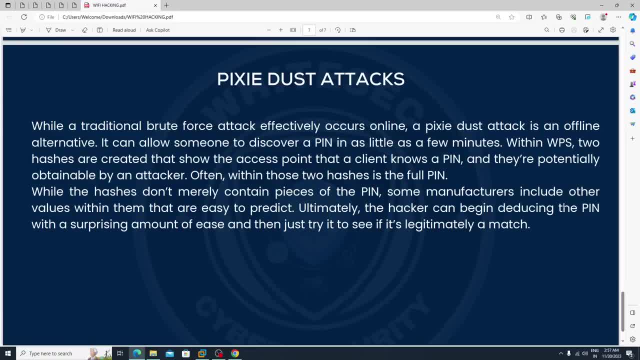 include other well values within them that are easy to predict. ultimately, the hacker can begin deducing the pin with a surprising amount of ace and then just try it to see if the legitimate mentally a match. okay. basically, it's a kind of also a brute force attack which is done by automation. 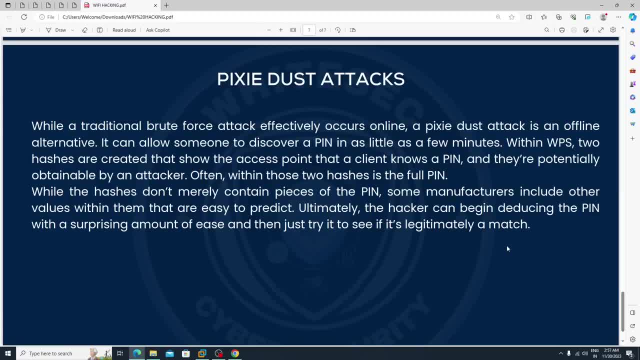 tools. if you use a wifi te, then you can able to do it. i'm gonna show you practically how to do it. okay, no need to worry here. so these are the attacks which uh which is in wps. now let's uh focus on practical things, then we will move to wps, okay. 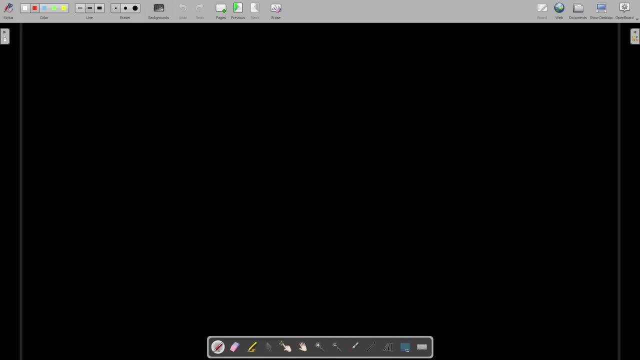 see, there are some conditions which you need to know before attacking the wpa wpa2 network. you can easily attack it, you can easily hack this wpa wpa2 network, but there are some conditions. okay, let's learn about that conditions. now, here there is a wi-fi network. 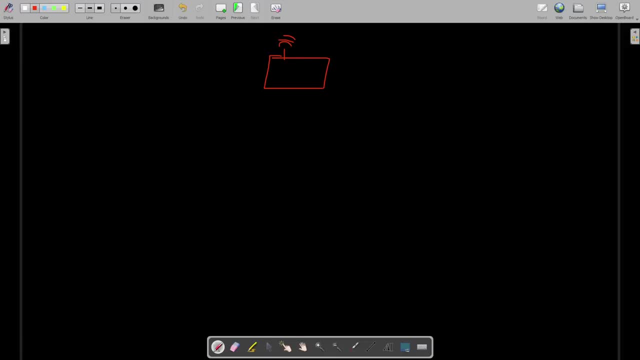 right now the assume that the just take any network, just the name of this network is test. okay, now with this network there are some devices. are there the clients? we can say it as a clients, like the user, who are connected with that network. okay, like there is a android device, computer. 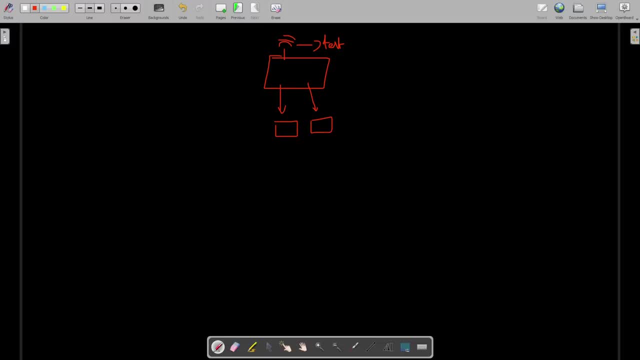 uh like windows laptop, any, any uh device, okay, or connected with this network. sorry guys, to hack now this router, this network is using the security of wpa, wpa2. by using the uh, this application, such as the wpa wps tester, we can't able to hack this, this type of uh routers. okay, assume that if 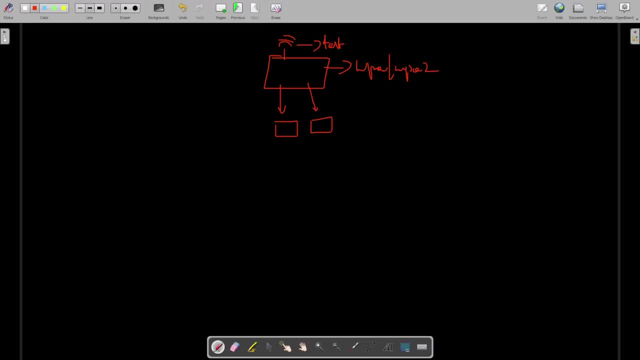 the router is if the wi-fi network is using the wpa2, at that time we can't able to hack it. so if you want to hack this wpa2, what you need to do see that for uh wpa. if you are hacking the wpa, the 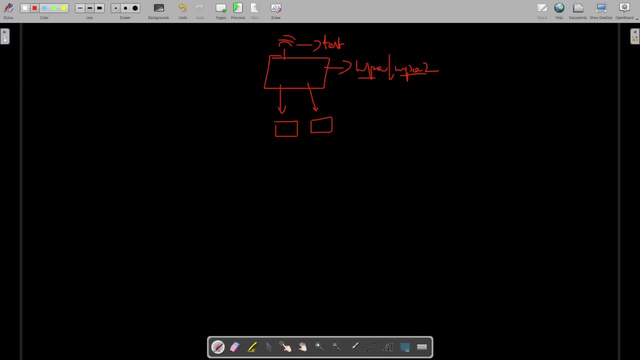 process is same for wpa, wpa2, you no need to worry. okay, now, if i want to hack this network, then what i need to do first of all, first condition, is the your target network. how clients? okay, assume that here. okay, no one is there in in this home. okay, simple, what they did means they just uh in this. 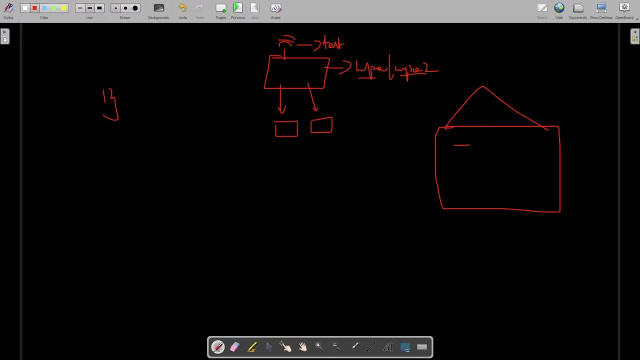 home there is a one wi-fi network, okay, which is turned on. okay, they, they, just the owner of this house has forgotten to turn off that wi-fi network and they, just simple, they are on vacation, okay, just assumed it. now, assumed that the this home wi-fi network is using wpa2. now that, what are 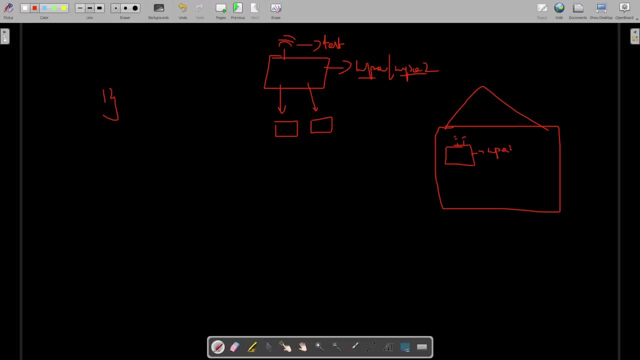 the requirements here simple: if you want to hack this kind of network, then the thing is, uh, they must need the clients, okay, the the people of this home, okay, who are connected. uh, who needs to connect with this network? okay, if no one is connected with this network, then you can't able. 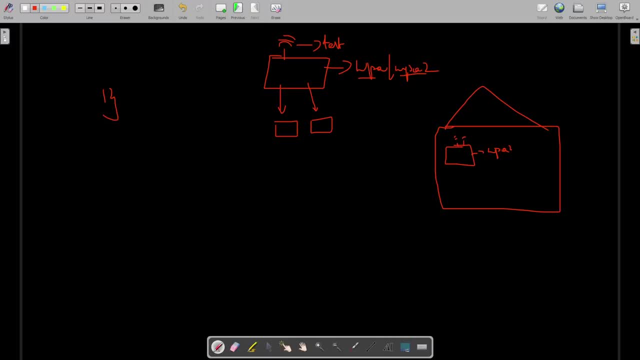 to hack it. this is the thing now. now, as a attacker, you just visited to that home location and you just started the attack. simple, after scanning that you didn't find any clients there. simple, the- the user who are connected with the router- is known as a client. okay, this is the thing. now, assume that there is a no one is connected with. 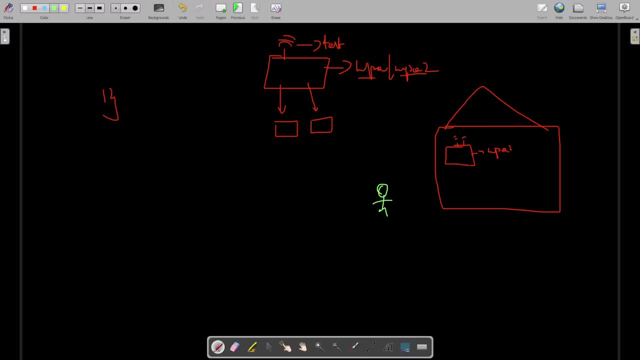 that network. at that time, you can't able to hack it. this is the thing. okay, the the condition is they must need to connect with this. uh, the clients must be connect with this network. okay, if the wi-fi router is using wpa2. these are the requirements. 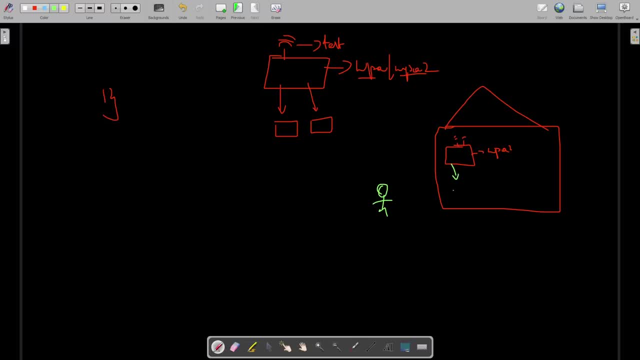 okay, you need to uh. assume that there is a one company. okay, in this company there is a wi-fi network. in this wi-fi, hundreds of people are connected with this network. assume that, okay, hundreds of network, uh, hundreds of people are connected with the, uh, with that network. okay. 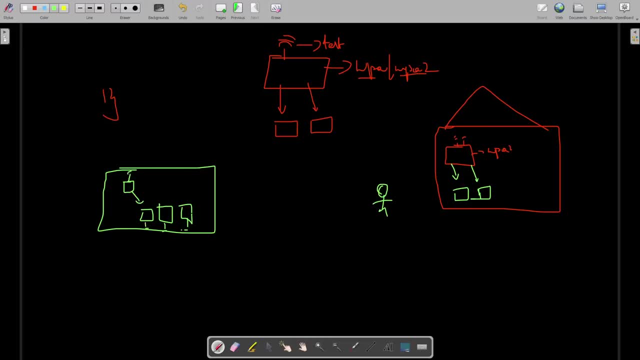 what is it people? people is nothing but the devices. okay, like we use the devices, like android device, this laptop computer, so these devices i am talking about, this is the thing. okay, so now they are connected with this network. now for us as a attacker point of view. i just visited to. 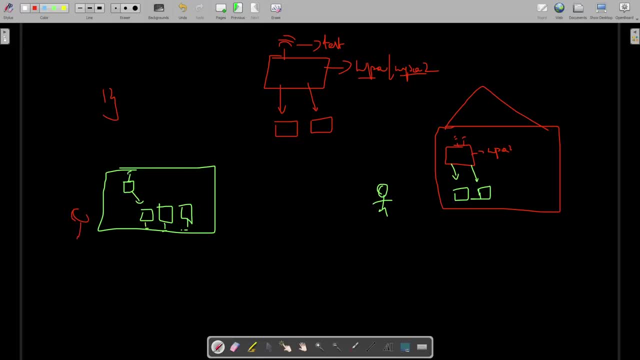 this company. i can easily hack this network because there are a lot of systems are there who are connected with this network. assume that no one is connected with this network. okay, this network is using the wpa2 security. if no one is connected with this network, at that time, what will? 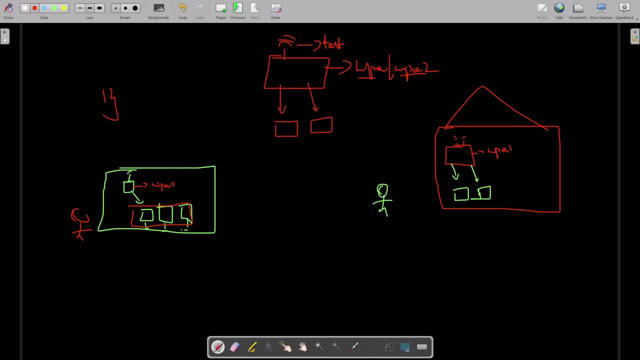 happen. we can't able to hack it. this is the thing. assume that they are using some other technology, such as wep. at that time there are chances, but in company they won't use wep. let me tell you this thing: mostly people who knows about wi-fi hacking, what they? they have some kind of doubts, okay. 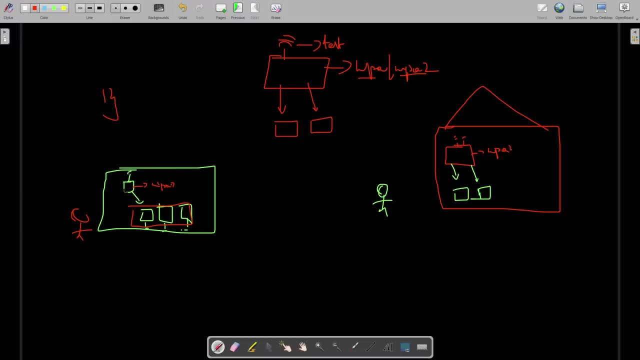 simple. we can also bypass these things. okay, like we can also use a fake card. there is a one uh uh feature by using this uh attack, sorry, attack. fake out is a one attack. okay, by using this we can able to bypass this one. okay, but it only work with wep. it won't work on wpa2. this is the thing which you need to remember. 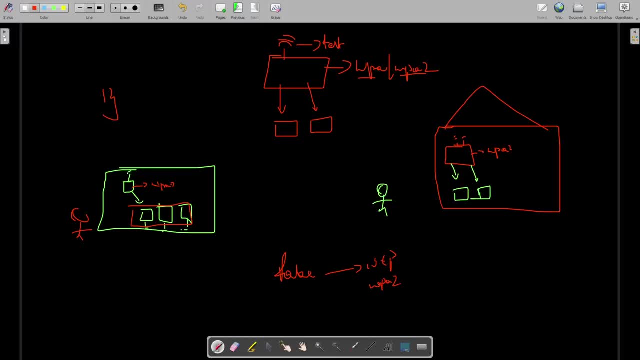 see wep. i'm sorry, guys, i am not covering about the wep, because hacking wpe- sorry, wep network- is very easy. no one is using this one. okay, in hundred percent. maybe five percent of people are using. okay, i'm not talking about everyone. okay, i'm talking about these things. okay, like, uh, the areas which 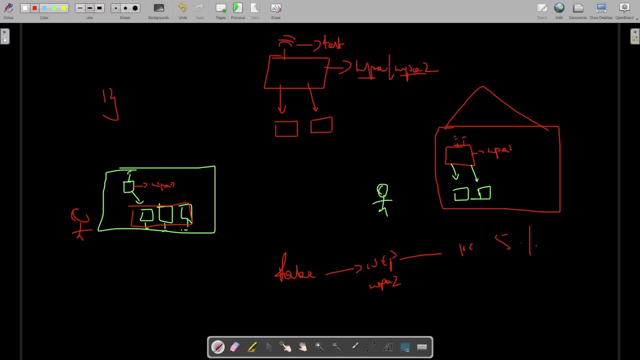 are popular, okay, like there there are. let's take an example of company only. okay, in companies, they won't use a wep. this is the thing, okay, so you need to remember this thing. uh, if you want to target wpa2, then the clients must uh need to connect with this network. okay, they need a user. 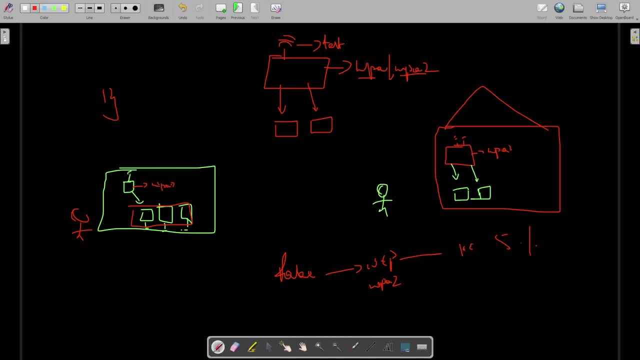 we need a users who are the legit users- okay, i'm talking about the legit users- who needs to connect with this network so we can able to capture the handshake? okay, we will learn about this. all steps, how to capture the handshake. it's not a big deal, it's a very easy steps. okay, you no need to worry. 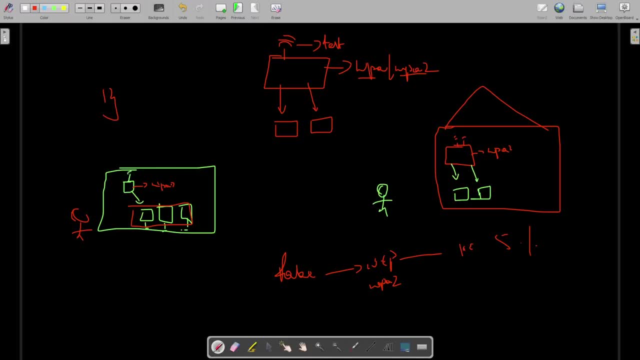 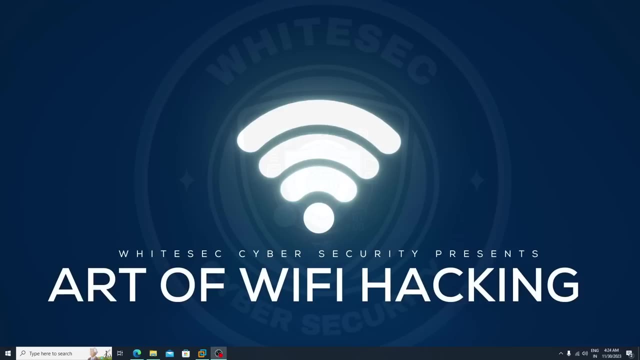 so this is how it's gonna work. these are the conditions, right? so now in this class, we are learning practical things. okay, how we can able to perform wi-fi pentesting or wi-fi hacking. now the thing is, first of all, a single tool. okay, by using one single script, you can able to perform whole, whole topics which we just covered in the 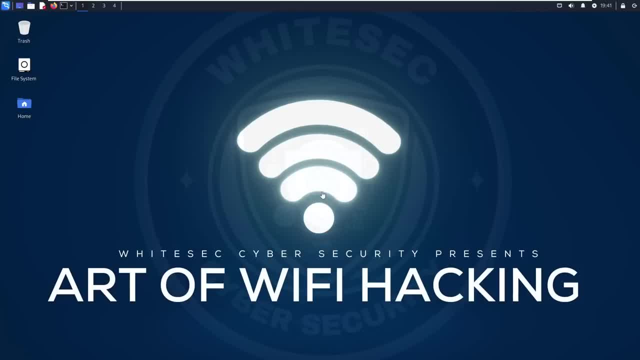 last classes. like you can able to hack wps network, wep network, wpa2 net. uh, this one as well, uh network as well. okay, now how to use this. i'm gonna teach you how to use this tool in a right way. okay, like, uh, if you learn this tool completely, then you guys can able to hack the wi-fi networks. okay, 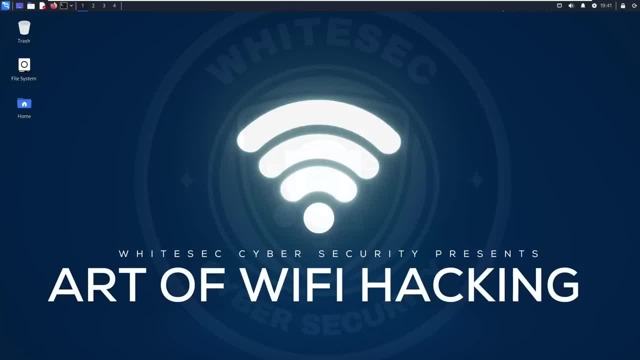 like i just told you, this course is for beginners. okay, like uh. if, if you don't want to, if you're having kind of fear- okay, like a majority of beginners having a fear of commands. okay, they can't able to remember the commands. okay, like uh, whenever they see the. 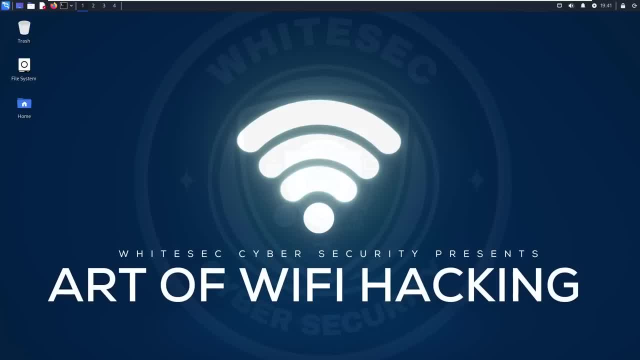 terminal. they. they think that, okay, it's a kind of hard thing. okay, for you guys, this thing is very difficult. okay, like, by using one single tool, you guys can able to perform whole wi-fi hacking. okay, like, just follow me. if you are not getting the things as well, just try to follow me. that's it. 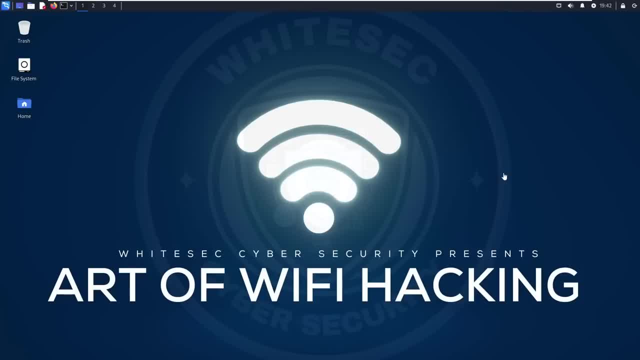 you can able to achieve your goal. okay, this is the thing now here. first of all, just open. once you open, the kali linux, don't go with this wallpaper. okay, what i did means i just change the wallpaper here. this is the thing now here. just click on the icon, which is a kali icon. okay, you can. 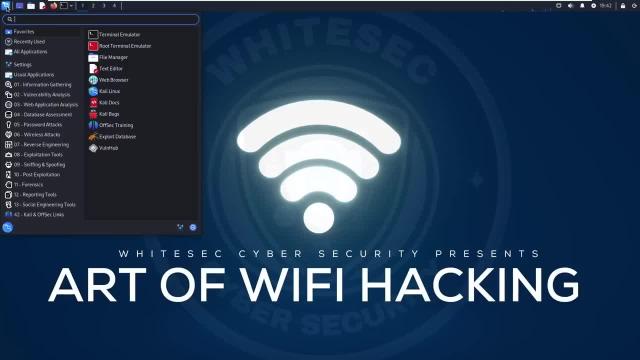 it as a menu now here you can able to see once you go in, wireless attacks. okay, there are wi-fi t. is there river? is there pixi? wps? is there kismet? is there? okay, farin, we will learn about farin okay. and wi-fi t. mostly by using this we can able to perform the whole wi-fi hacking like. 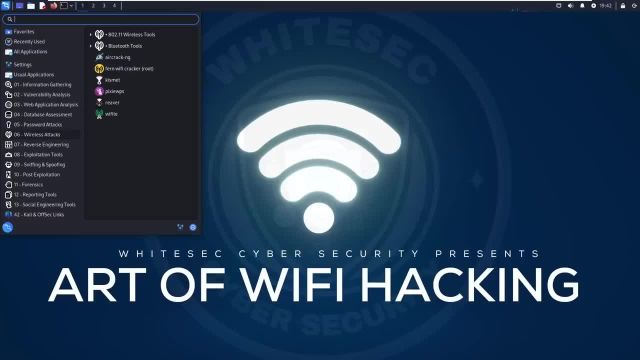 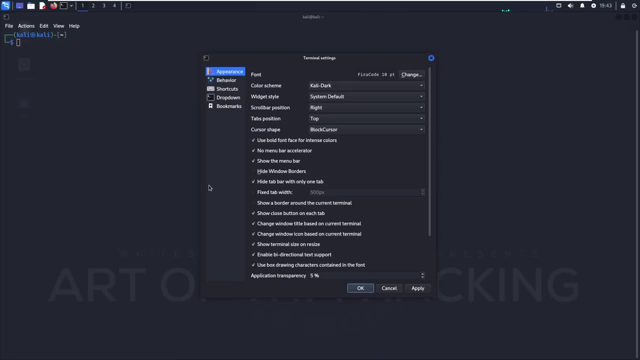 which we just which i just told you in the last classes. right now, if you want, first of all you need to know how to use this tool. okay now, first just open the terminal here. after opening the terminal, just click on preferences, simple right click on this terminal and click click on. 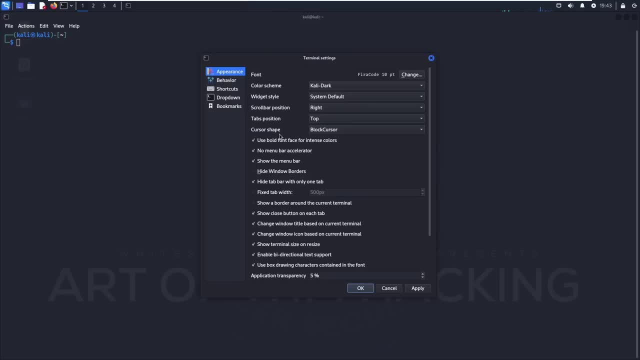 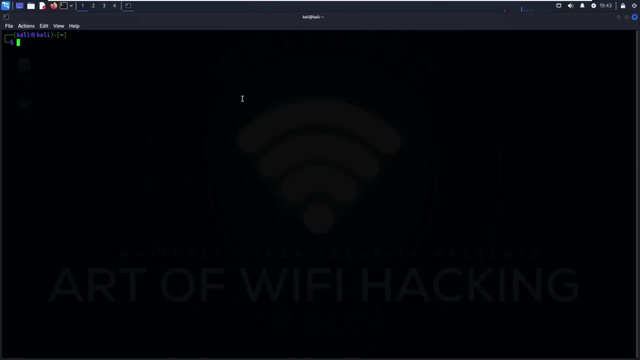 preferences and see there is a color schema now here. select black on green on black and click on apply because this one is good for you. okay, whenever you see any kind of errors during the this kind of pen testing, at that time the green color, okay, will play a very important role here. this is a 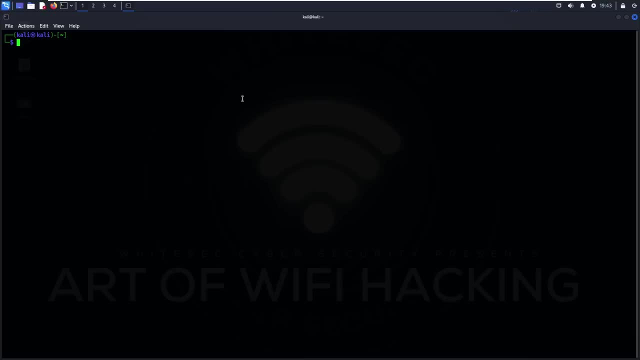 thing now. first of all, what you need to do means you need to execute this command: apt get update. this is a very important guys. now see here what it's saying: list directory- uh, it's required. it put. it's saying that, sorry, permission denied. okay, now simple execute as a sudo: sudo space: apt get. 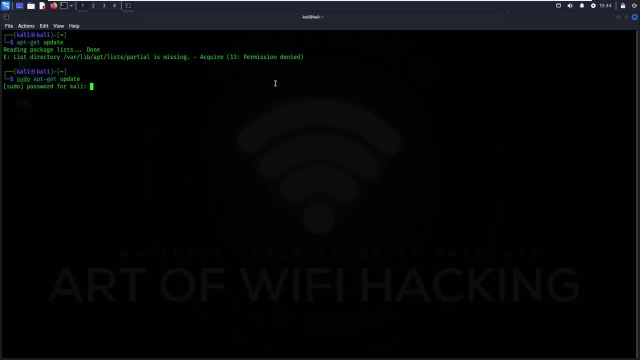 update now. just type the password of your kali machine, which is kali. now here, it is right, it's successfully done. clear this. just let me zoom it again now to run this Wi-Fi te, just type here: sudo its Video Calibration. run this kind of hacking tools. just try to run it as a sudo, these tools which are a system tools. 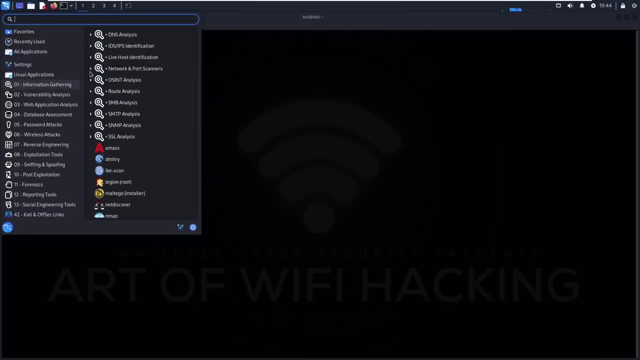 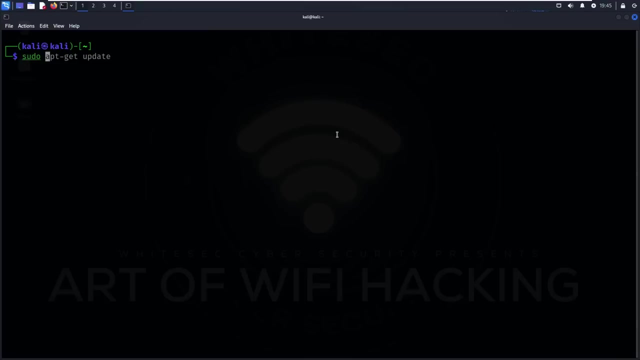 okay, by default, you guys are able to see the some tools in this system. right, so simple. the thing is: you want to run this tools as a sudo? okay, assume that if you want to run nmap, just try to run it as a sudo. okay, this is the thing now here. just type sudo and just type wi-fi te. okay, simple, no. 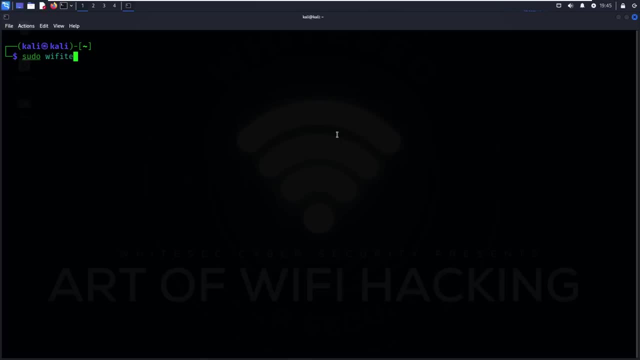 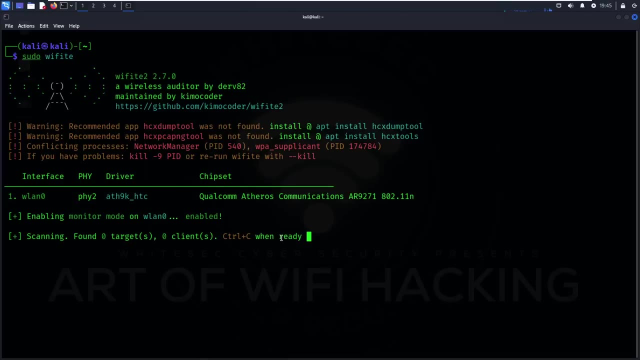 need to type anything, just enter: okay, here you guys can able to see. it will automatically detect your wireless adapter, right, and it will change your wi-fi adapter to monitor mode. just see enabling monitor mode on wlan: 0. if i go, if i open this terminal and if i type here: if config. 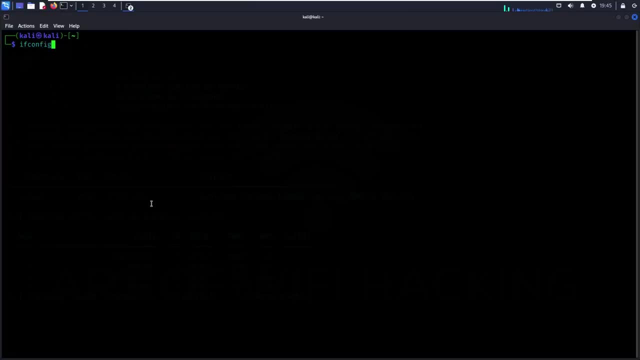 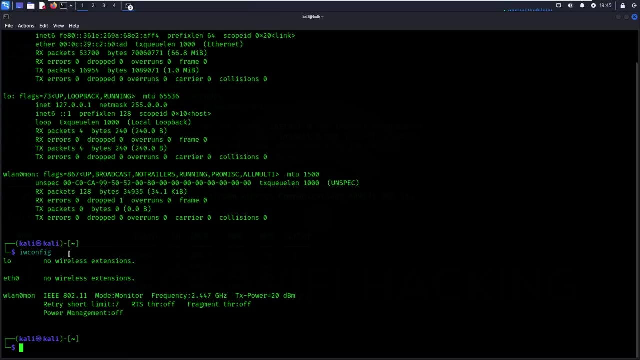 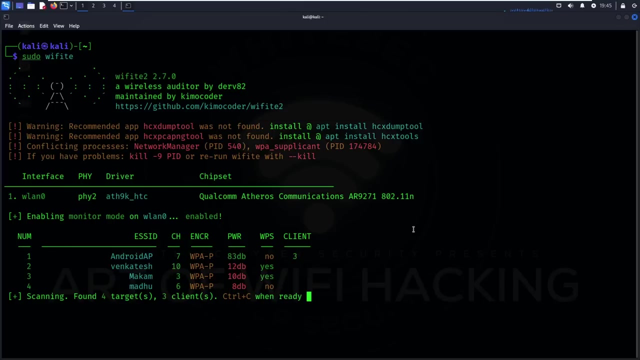 here you guys can able to see, the adapter is in monitor mode. if i type iw config as well, here you guys can able to see, mode is monitor. so the thing is here. you no need to execute the air moon ng start wlan 0 or something like that. it will automatically do the whole process okay. 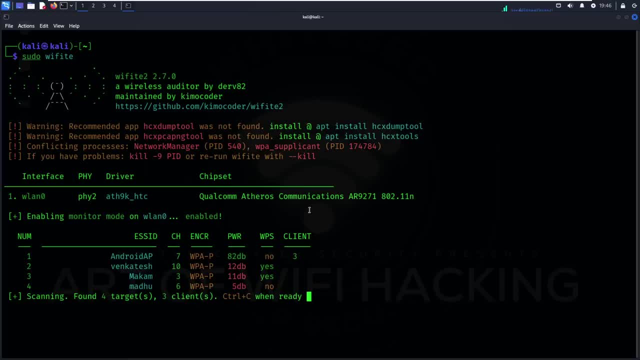 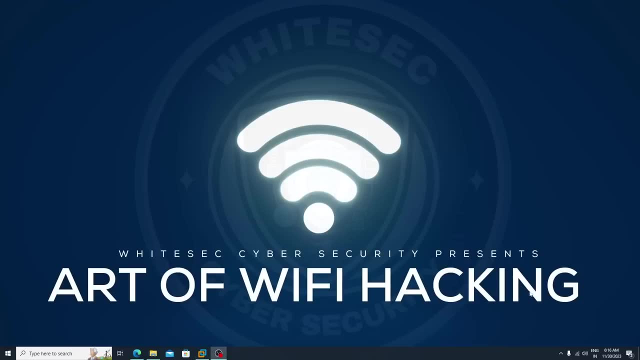 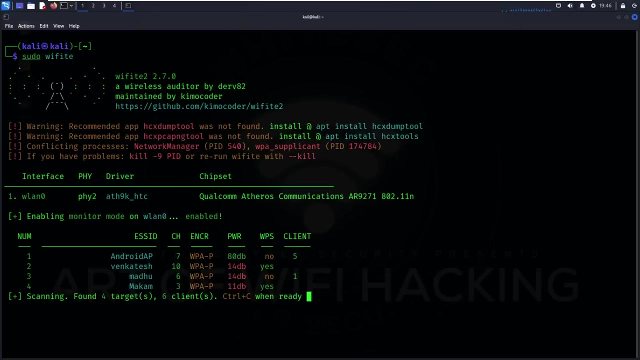 now. just remember here: okay, uh, right now, what is the time here? now time? uh, the time is 6 am. okay, it's around 6 am. now here what you need to do. let me explain you about this one scanning- still it's scanning and found four targets. right now it can able to detect. 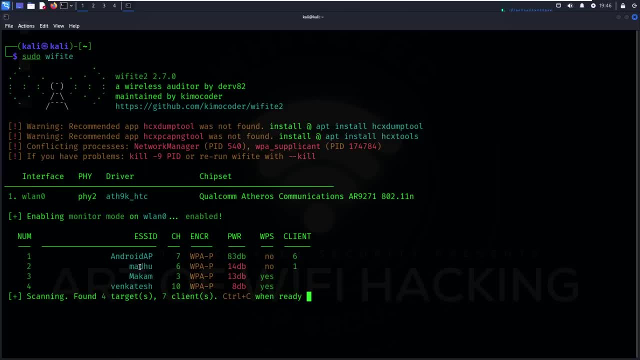 four wi-fi network. now the uh seven clients are there and uh control c. assume that if you want to target any of this uh network, uh, this network, then what you need to do, first of all you need to type ctrl c to stop the scanning. now see, the scanning has been stopped. now you need to choose your target. 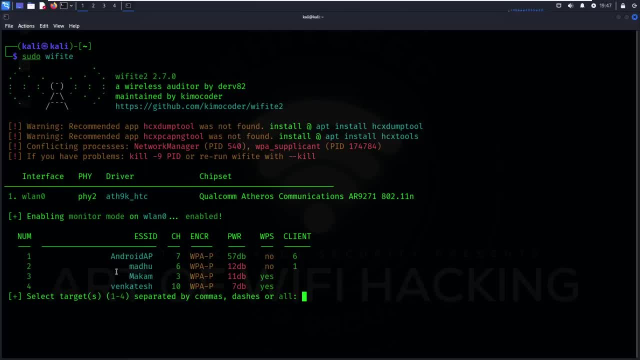 from here now for uh, doing this whole process before hacking the wi-fi network. let's learn about these things. okay, now see esser ess id there. sorry, let's start from here. there is a num, is there? what is this? it's a nothing, but it's a number. number play a very important role here in this script, because you 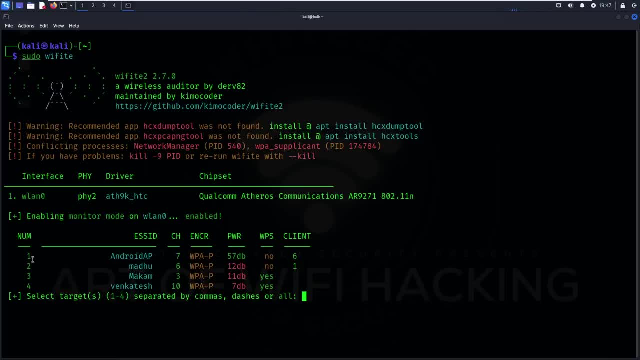 need to choose your target through number. okay, assume that i want to target android ap. then what i need to do? simple: i need to choose a number, i need to type one there so it will start attack on android ap. okay, this network. assume that i want to choose, uh, some multiple networks at the same. 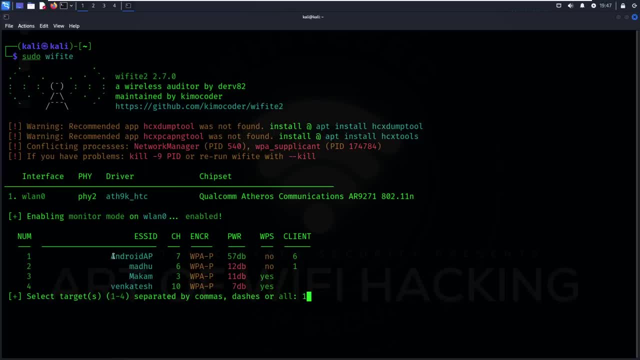 time. at that time, what i need to do? simple, uh. assume that i need to target android, ap or madhu. now, simple. what i need to do? simple, uh. i need to type the numbers here: one, then just add the comma and two, the, the target number. okay, this is a thing. assume that if you want to target all this, 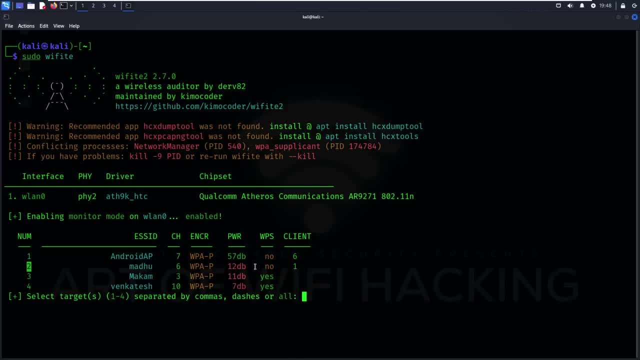 network at the same time. okay, this whole four networks at the same time. assume that in your case it might be more at that time simple: if you type all, then it will start to target that all networks. okay, this is the thing. it's a complete automation process. just you need to type some simple keywords. okay, that's it now. 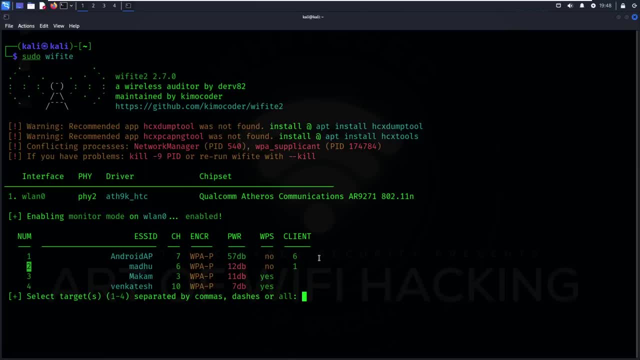 just see here the channel channel. if, uh, sometimes the channels are same, sometimes it may not. okay, this is the thing the you no need to worry about the channel function in failure if you're using, you know, 43CM. you would be satisfied with not making有关 spo allons. 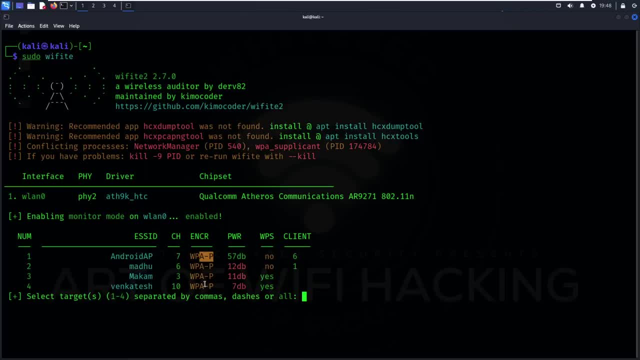 if it's using the web, the age in which should we use, for example, 1, 4 or 5 years if it's using a internet network? this is the channels. so right, this column, as you will see right now, the course, we'll see that you no need to do friendship. 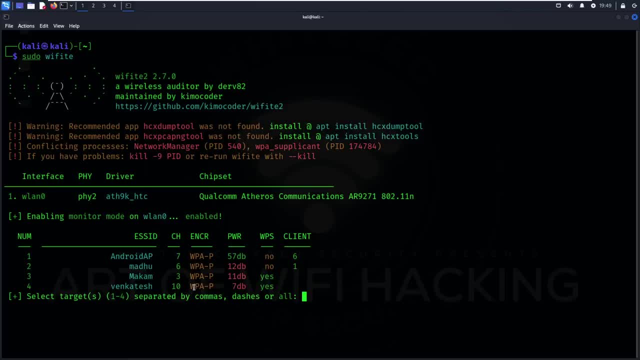 these are coming. this is not of hard work- nothing. if there is a w ep here, you won't see that. okay, mostly in bangalore you guys can able to see hell lot of w ep networks. okay, this is a thing, but uh, this is a once you join. 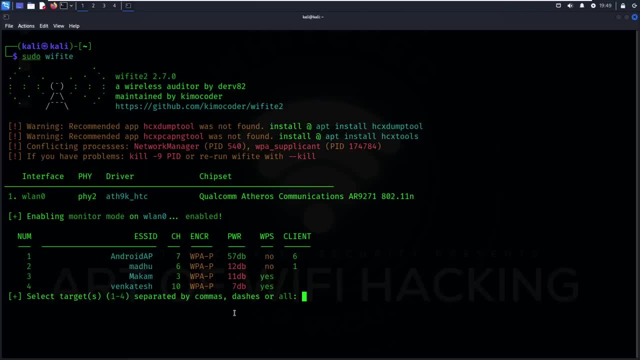 uh, go for any pentesting uh, if you want to, if you are providing pentesting services, then in organization, in companies you can't see w ep network. okay, this is a thing. now, here there is a power, is here. what is a power? power is a nothing. but see, here there is a green signal. 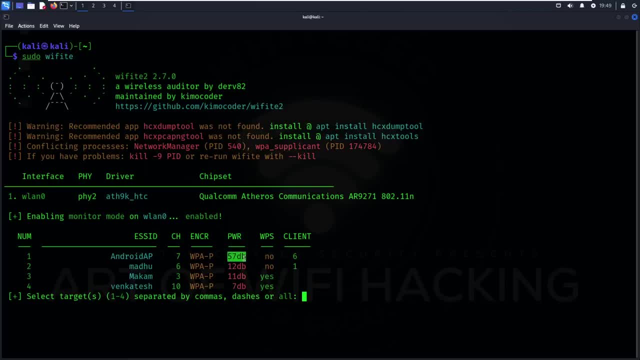 is here. green signal is a nothing, but this network is very close to me, okay, so i can easily uh like, hack it. okay, this is a thing. see, this power plays a very important role. let me tell you, if you are seeing red here, okay, at that time the, the, this network is very far okay. this, uh like it can't. 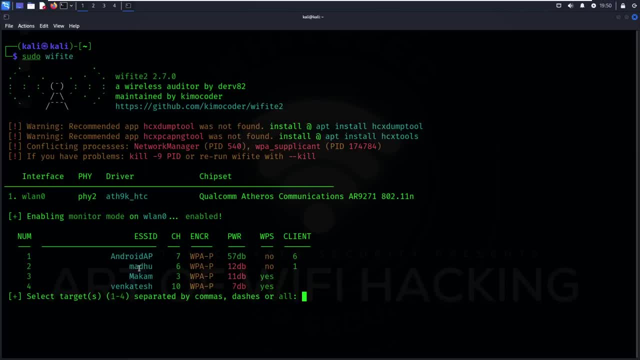 it can able to detect the network, but still the signals are weak there. okay, still you can able to hack. but let me tell you this kind of network: there is a venkatesh is there right? see, it's saying that 7 db. maybe i can't able to hack this one. now how to hack this? networks okay, this, uh, red networks okay. 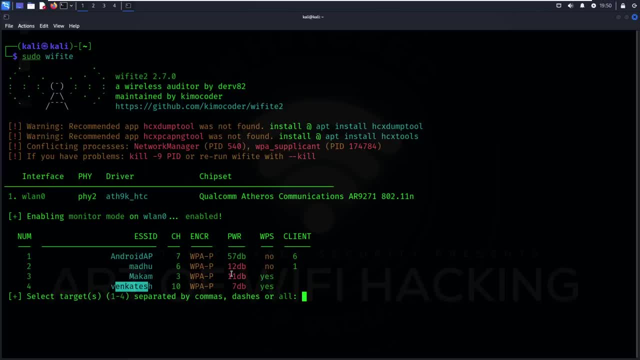 like how i can able to make my attack wide, in a wide range. what you need to do, miss, you need to use, uh, antennas. okay, this is a thing you need. uh, there are a lot of antennas. you need to purchase a lot of antennas. you need to purchase a lot of antennas. you need to. 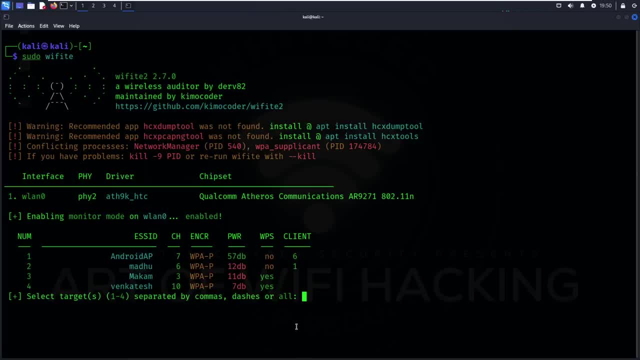 purchase a lot of antennas, spread it separately, then you need to use it okay for wide attacks, simply can able to detect it. okay, this is a thing now here, just see there is a wps. i just told you about the wps, right, the last classes in another class, before and after. 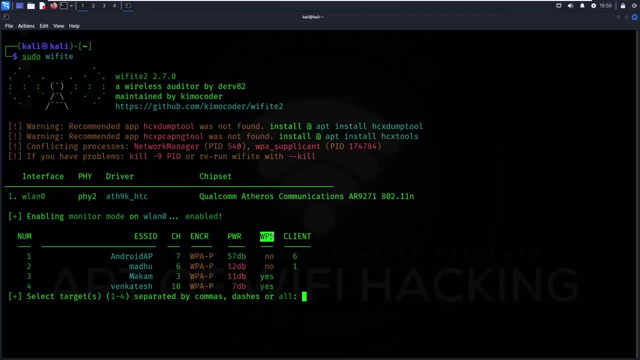 Jeff Wall процесс say github, here you can able to see in android ap. wps is no, that means wps is not there in this android ap in general. now in madhu see in madhu also the wps is not there, it is Samsung. smartphone at least. as for this password, central hafta case, after this, just apply yogurt, obviously, and tryMag writer better as soon as possible, and system smart phone 못 accep. then what can the yays but don't pass is a phace. Rom seja composing, which means the dioxide right in. 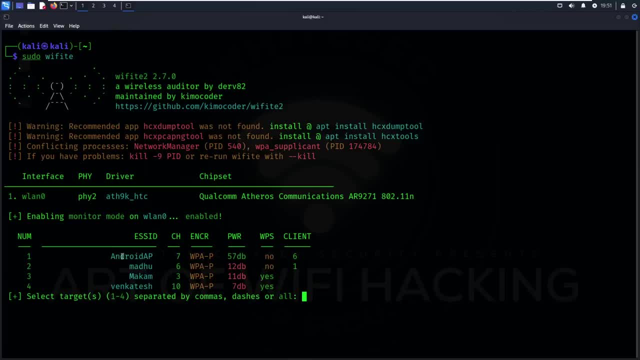 that connection. that's an alpha- and that to watch the application. basically the steps that i which th elderly network. okay, on this networks, like, there is a lot of attacks out there, such as wps, pin attack, push attack is there? okay, we can't able to perform on this network because these guys what they did, 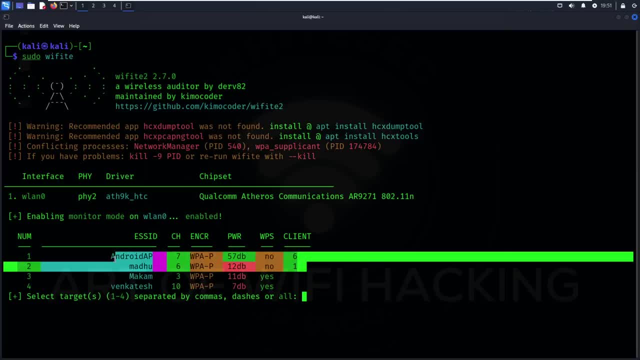 means they just disable the wps. uh, but this thing there, okay, the feature there in the router. so that's why we can't able to see that wps here now. just see on makam and venkatesh. see in makam what happened. means this guy having the wps enable? now just think that to hack this. 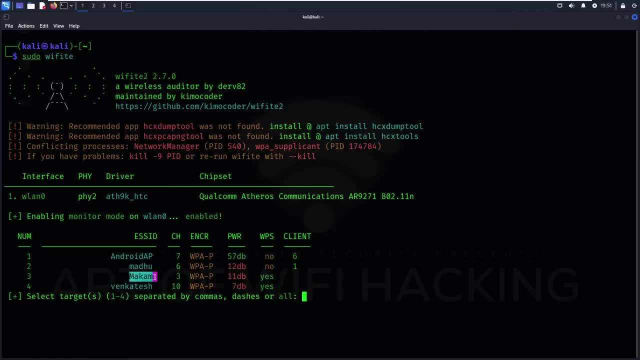 network. it is easy for me, okay. i can able to perform wps brute force attack there and i can able to perform the hacking. it's not a big deal for me, okay. now in same for the venkatesh. see here there is a. wps is unable. that means the push button is enabled and you can also perform the. 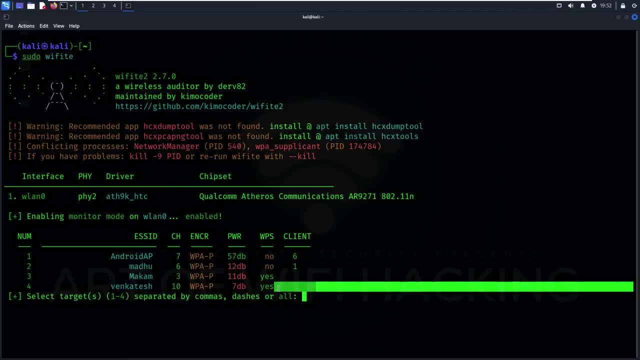 eight digit attack which we just learned in the last classes. right, you can also perform the eight digit attack which we just learned in the last classes, right, you can also perform the eight digit attack which we just learned in the last classes. right, so simple we can. sorry guys, we can able to perform those. all attacks on this networks, okay. 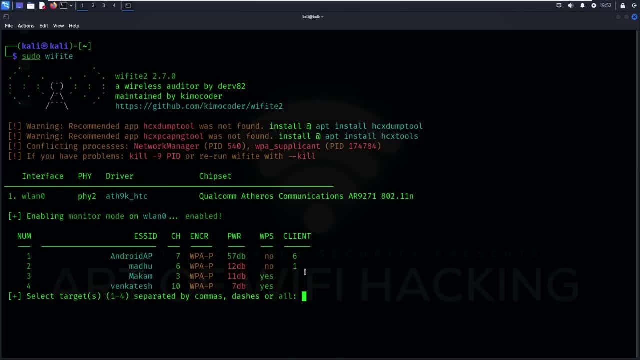 but in this network you can't able to perform it because wps is not enabled. this is the thing. okay, if you want to hack this networks, then what you need to do, you need to perform the deauthentication evil twin attack, something like that. okay, all right, like, first of all, you need to capture the 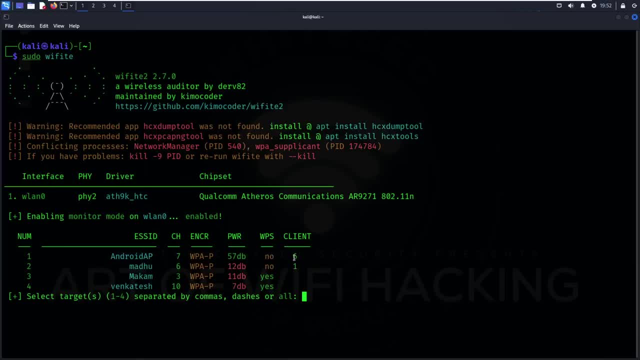 handshake, then you need to crack it. we will learn this all steps in this class, don't worry. and here just focus on the client. now see android ap having six clients. okay, madhu, having one client, that means only one guy is connected with that network. even it's a- uh, maybe it might be android, mobile, iphone. 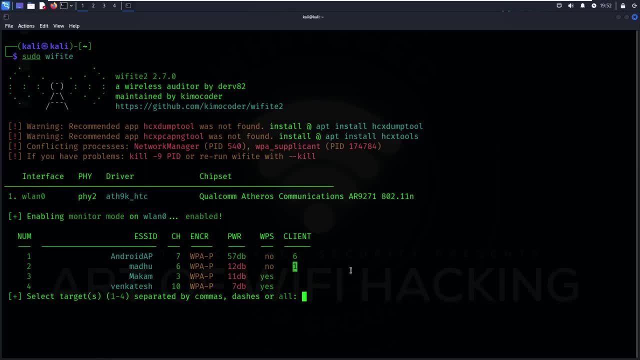 okay, laptop or something like that. we can't say that. okay, we can able- sorry guys, we can able- to detect it. okay, like which android? by using the mac or something like that. like, we can able to see the providers here. so we can able to see the providers here. so we can able to see the providers here. so 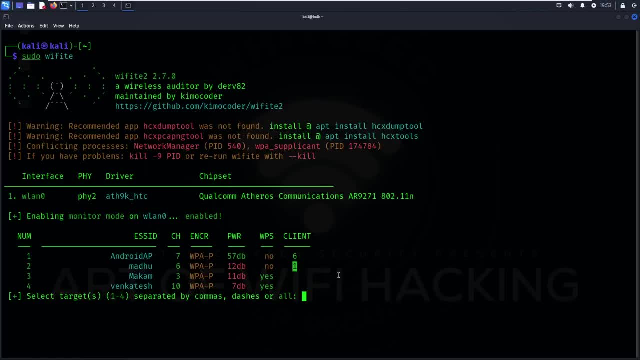 it's not a big deal for us. but the thing is, i just told you in the last class as well, you clients are very important. if the wps is not enabled and if the target network is using the wpa or wpa2, okay, at that time these things are very important. see, here it's using the wpa, but the wps is enabled. 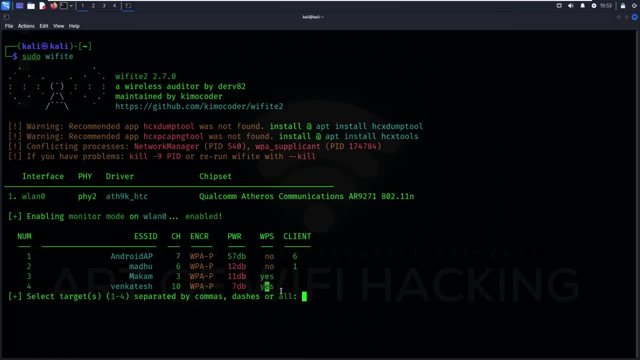 here. that means for us there are having two chances. okay, we can also perform the brute force attack if theous a right uh things okay, like if you perform the attack in the right way, then you guys can be able to hackit like uh. sometimes. if there is a uh, we will learn about the all subs in next class, don't worry. 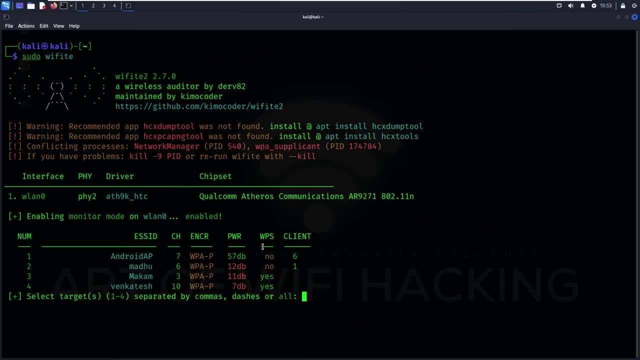 now here. the thing is, we have for this- what is this? networks? we have two chances. okay, like i can also perform the, the authenticatio attack or attack on it. okay, or i can also use, uh, perform the wps attack on it, like by using the wpa wps tester, i can able to. 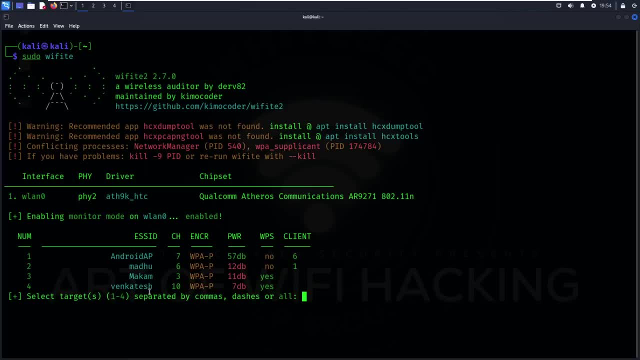 hack this network as well. okay, now, sometimes, what will happen? you can't able to exploit this wps. at that time, what will happen? this wi-fi te will automatically start attack on wpa. okay, we will see this. all things in the next class as well. okay, so this is the thing, guys. it's not a big deal. 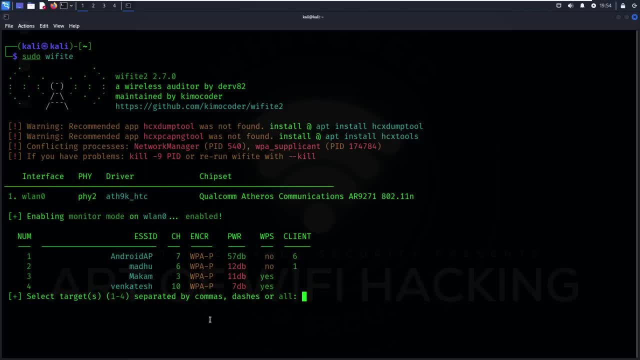 once you jump, uh, once you do this process on your own network, okay, just create one network, any hotspot or something like that. just try to test there. okay, you will see a lot of results and also you will learn a lot. okay, once you just do practical right here, just see, it's saying that. 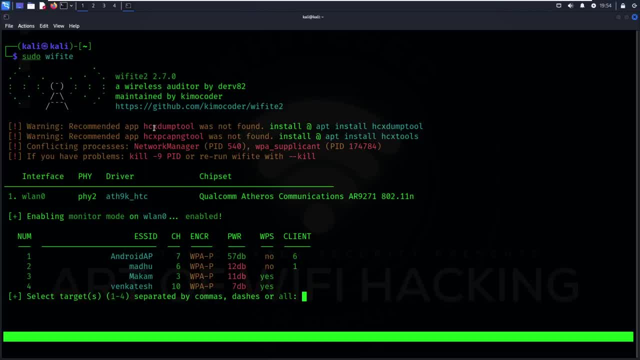 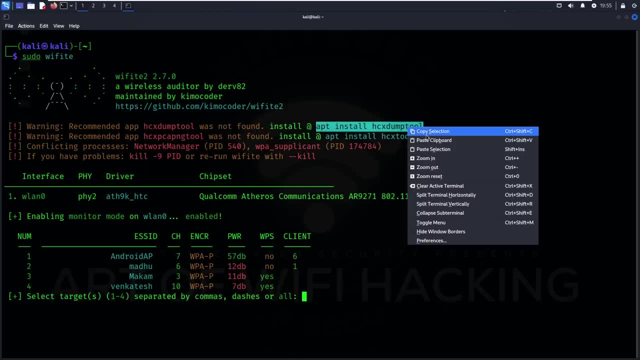 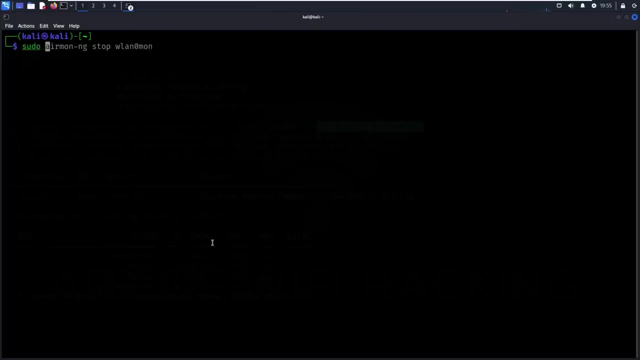 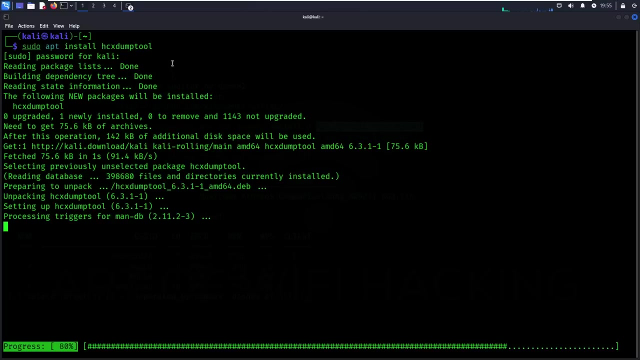 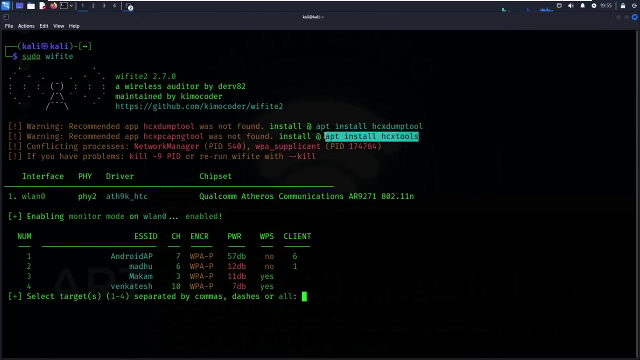 recommended app: scx dump tool. need to install. okay, how to install it? simple, copy this command. this is very important. tools. just type sudo and paste this one. now, here there is a scx tool is here. tools are there, just let me copy. just paste it here. 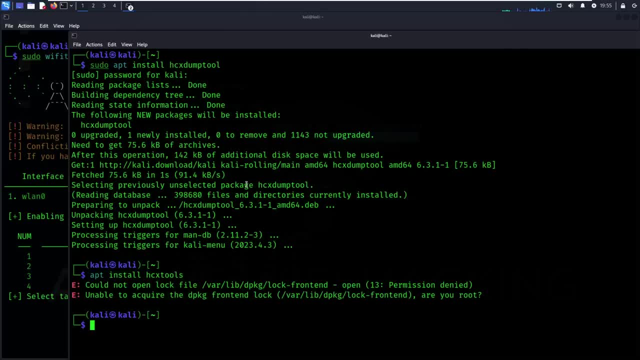 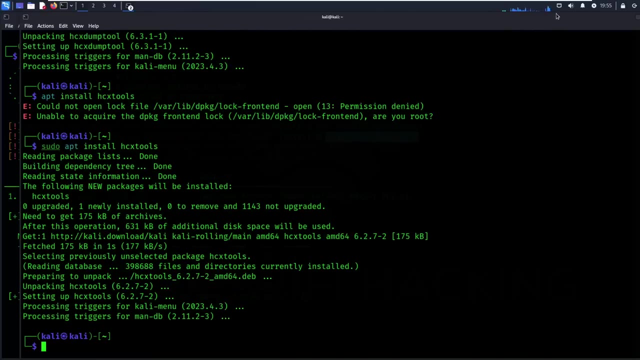 see, yeah, without uh typing sudo, i i didn't added the sudo there, so that's why, sorry guys, i got the error there. okay, sorry. the climate due to climate change: uh, there is some cough. okay, just just see, this is we successfully installed this one, so let's start the attack in the next class. 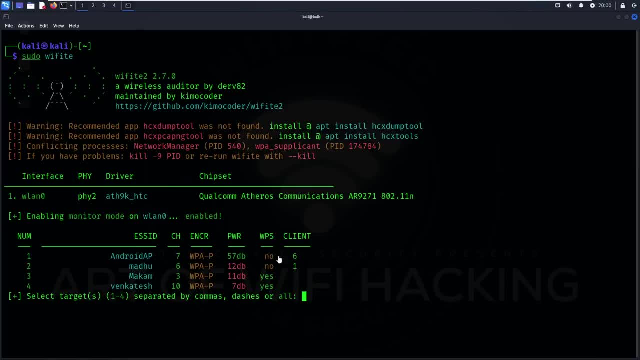 now just see here in android ap and in madhu there are clients, are there, okay, but wps is not available. so what i need to do? again, i am saying i need, uh, i'm gonna target this one, okay, uh, i'm gonna perform the deauthentication attack. i, uh, i'm gonna capture the handshake or something like that. but here 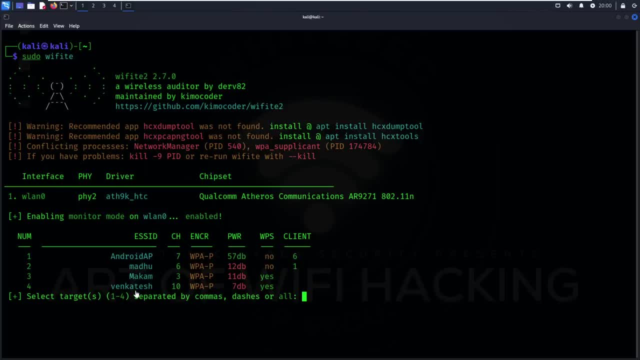 in makam and venkatesh. what happening means there is no clients. i just told in the last classes: if there is no clients, then we can't able to perform the attack on wpa network or wpa to wpa network. okay, this is the thing. at that time, what you need to do means you only perform the wps attacks on it. 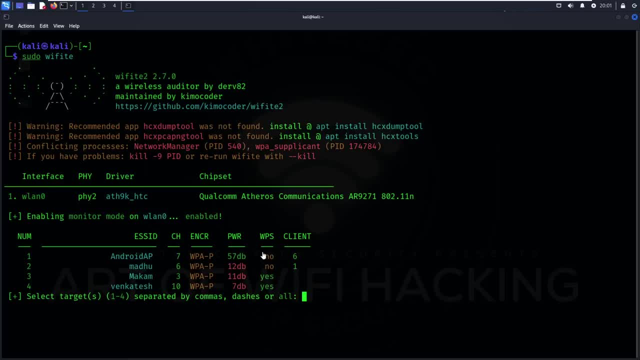 because the wps is enabled in this networks. okay, so this is the thing i. i just forgot to tell you this thing. okay, so you no need to worry, even if you don't know the attacks. simple, the single tool can able to help you. okay, it can help you. okay, just just focus on it, that's it. 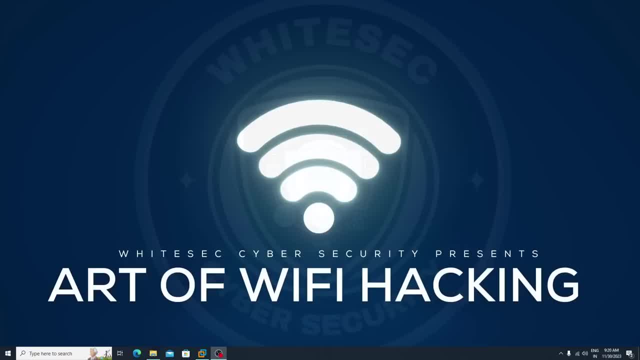 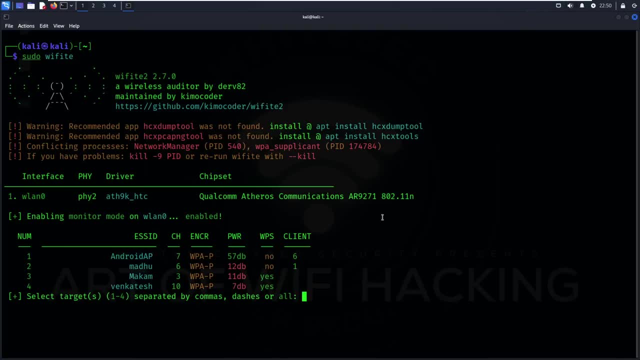 in this class we are learning about wash tool. see, wash is a tool. by using that, you guys can able to scan wps enabled network. so you can scan the wps enabled network. you can scan the wps enabled network. now, just see, we can also do the same process using wi-fi te. but just see when we just perform the. 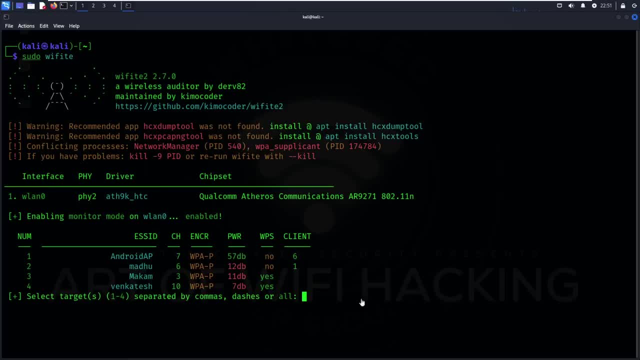 it will. uh, it will show all networks, okay, even the wps is enabled or not, it will show that. okay, but wash is a tool which only shows you wps enable networks. okay, you can also scan using wi-fi te as well. let me cover that one. uh, this one as well. okay, how you can able to scan the wps enabled network. 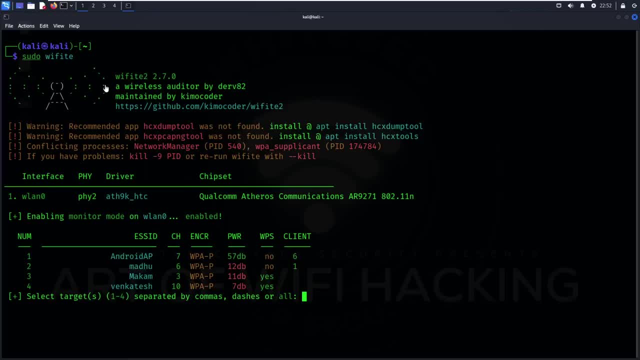 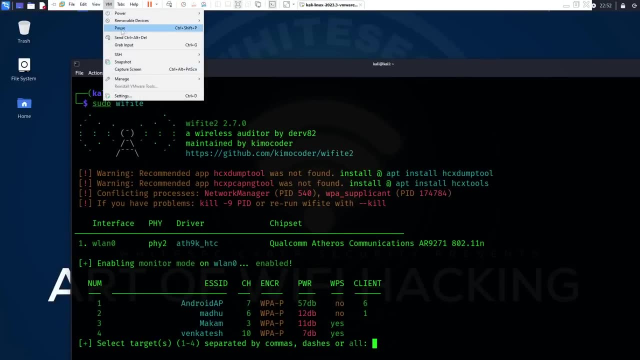 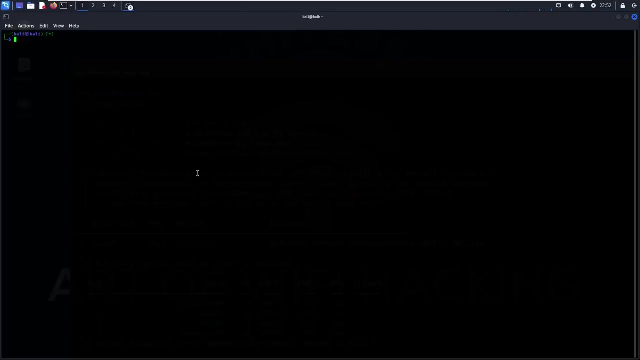 to scan only wps network by using wi-fi te. okay, now let me show you. let me tell you about wash. okay, just first of all, let me connect this wi-fi adapter. let me open the terminal here. let's start here. you just need to change your adapter to monitor mode. okay, sudo airmon. 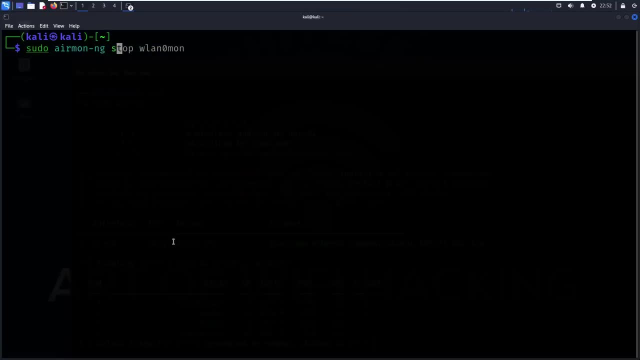 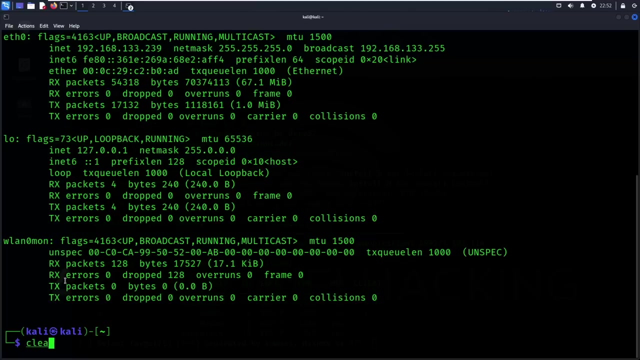 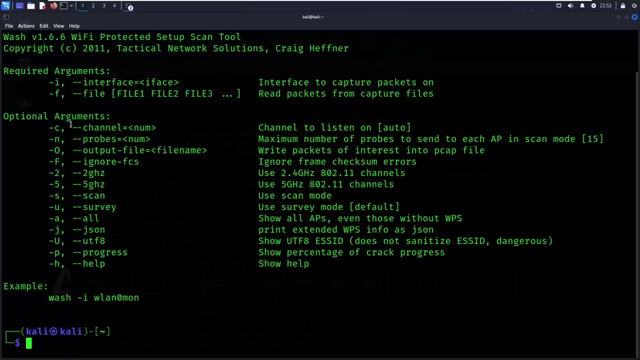 dash engine start wlan zero. right now my adapter is in monitor mode. okay, so let's use a wash here. if i type here wash, then you can able to see the optional arguments: requirement arguments- okay, sorry, required arguments. basically, it's a help, just see here there is a one argument which is dash a. what it's gonna do. it will show all aps even. 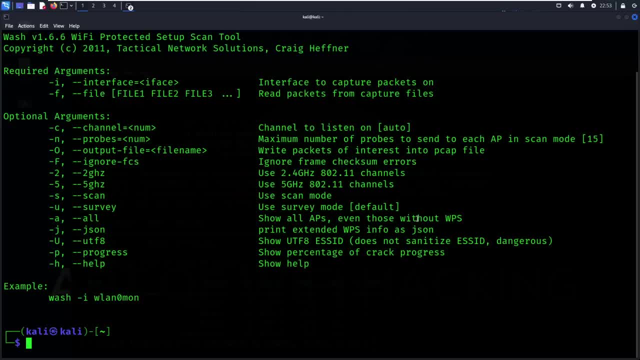 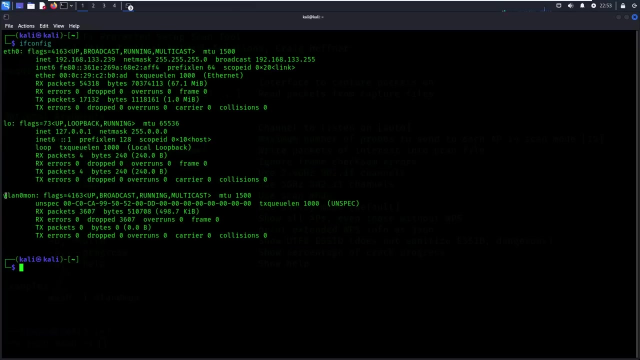 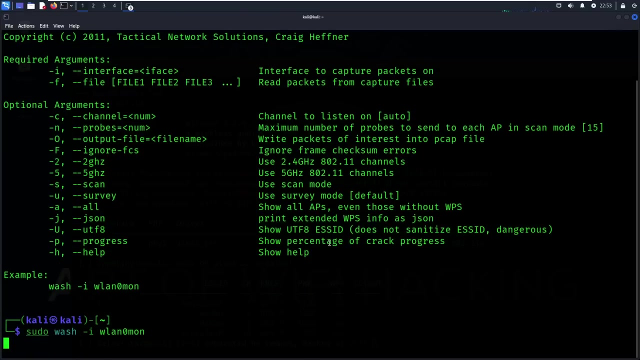 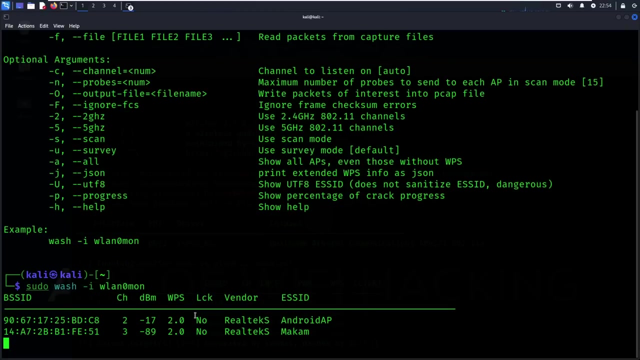 those without wps. now we no need to go deep in these things. okay, simple, just type: sudo wash dash i for what interface? okay, here it is. then just type your interface at this one. then just type your interface at this one: Run WLAN. disappoint, okayёл. 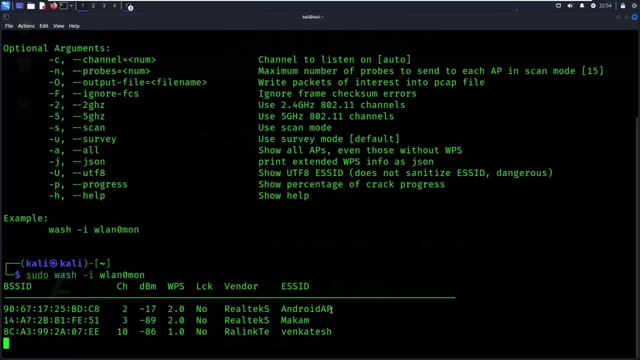 ok, ن ap having the wps. see it's using wps 2.0 is here lock lock is no, there is a no lock there. see, when you perform the brute force attack, then what will happen means, due to security the router, it will get lock. okay, by using this wash you can able to check that. 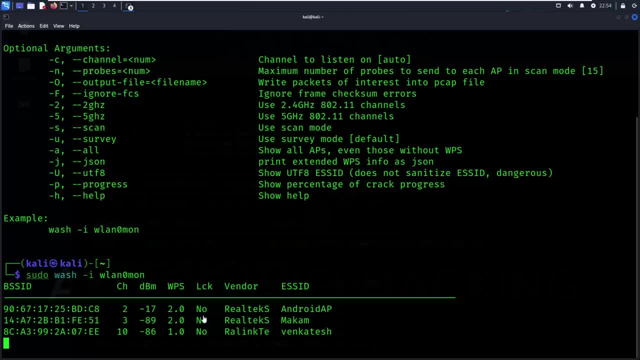 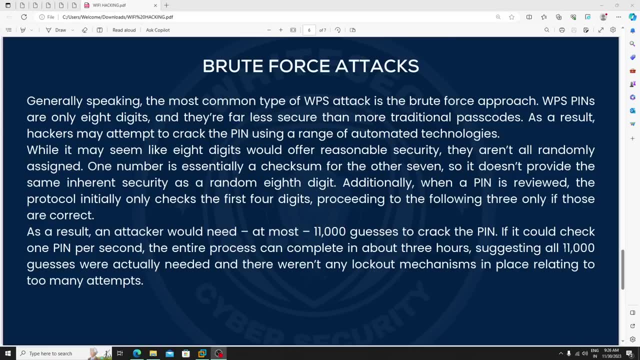 okay, the router is locked or not? okay. so this is the thing here. we just learned that. okay, just let me show you. see this point. guess where actually needed- and there were- there weren't any lockout mechanism in place relating to too many atoms. if it sometimes due to security, what will happen means. 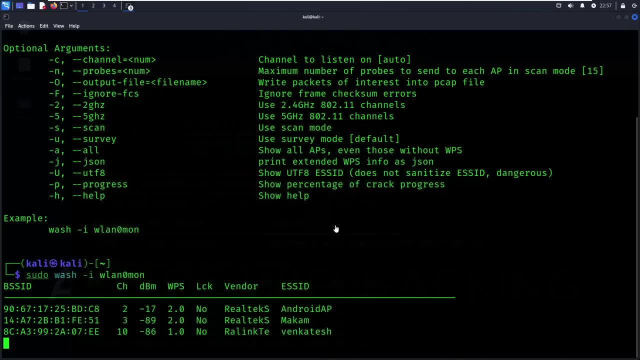 if this w the router is advanced, okay, sometimes there is a security in that router. once you perform the brute force attack on it, then what will happen means this will get locked for. by just typing wash, dash, a and interface here you guys can able to check that: uh, it's lock or not. 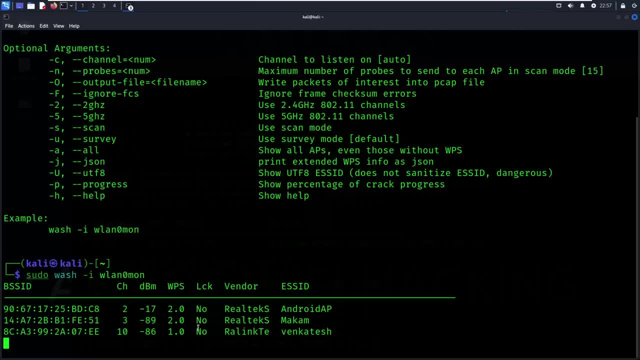 right now the wps is not locked. okay, see, here there is a no. once you perform the brute force attack. okay, after performing that brute force attack on the wps network here, if there is a security, then what will happen means here you can able to see: yes, that means the router has been. 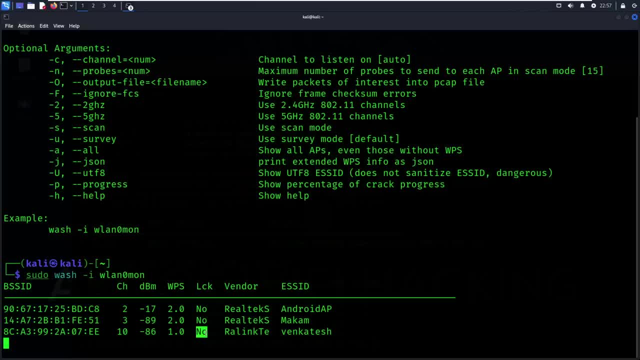 blocked. so this is the thing: simple: to unblock it. what you need to do to send the deauthentication packets on that network so everyone will disconnect. they think that, okay, something bad has been happened. let's restart the router- simple. after restarting the router, everything will be get normal there. okay, this is the thing. this is a kind of. 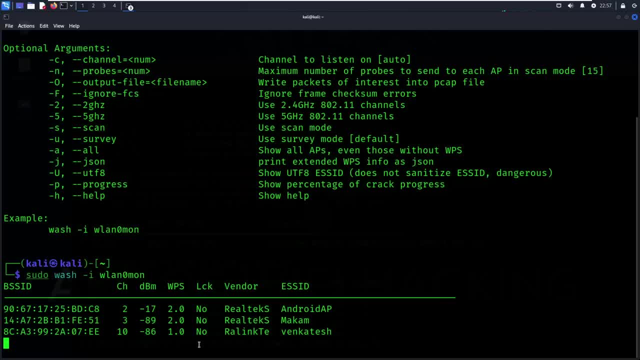 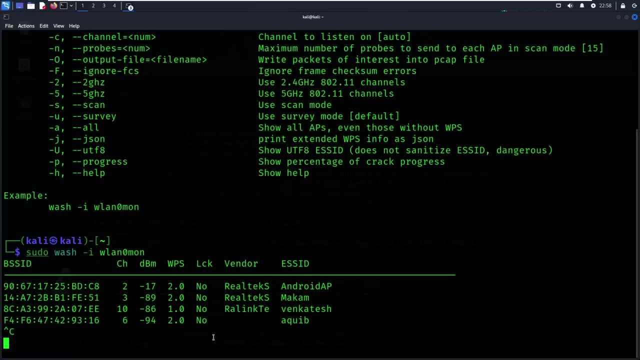 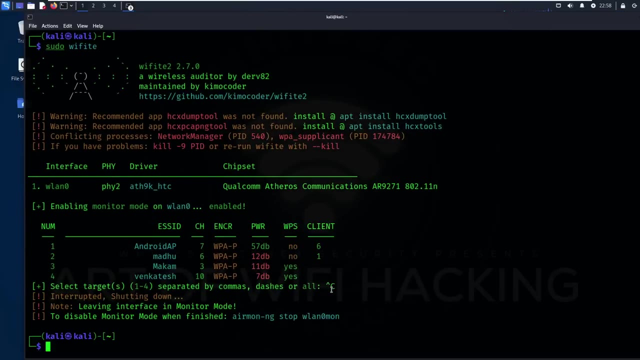 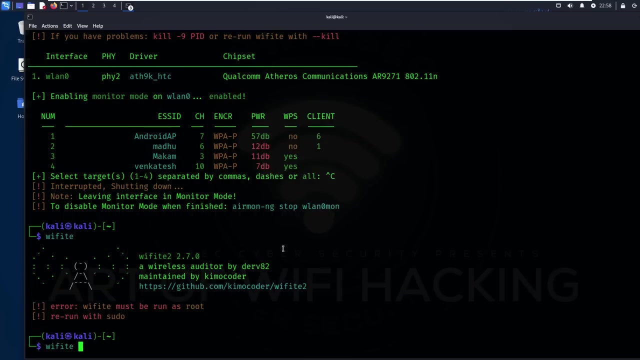 social engineering technique. okay, so here we got some other network which having the wps. now let's stop this one. let's do this same process using wi-fi ta. if you type here wi-fi te, this type, sorry, wi-fi t, dash h, here you can able to see the help. okay, the. 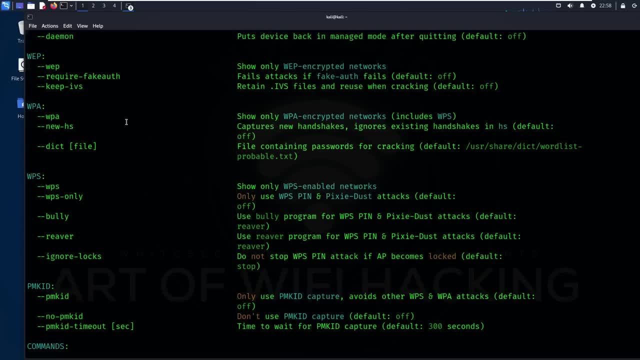 if you want to target wpa network, then what you need to do. sorry, if you only want to scan the wpa network, then you just need to type wi-fi, te, space, dash, wpa, then it will only scan for the wpa network. this is the thing. now see, let me scan only for the wps networks. right, to scan it. what you need. 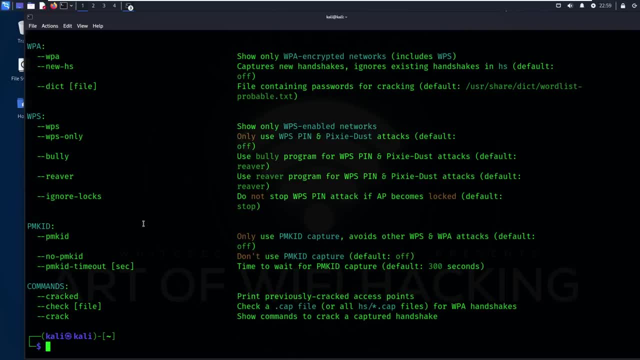 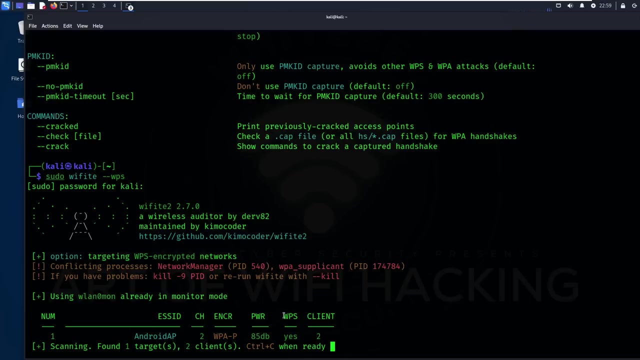 to do? just type here sudo instead of using wash. you can also use wi-fi te. i just told you wi-fi te is a very excellent tool. okay, now let me scan only wps networks. just type enter now it will only scan. see previously what is the result. okay, once i just 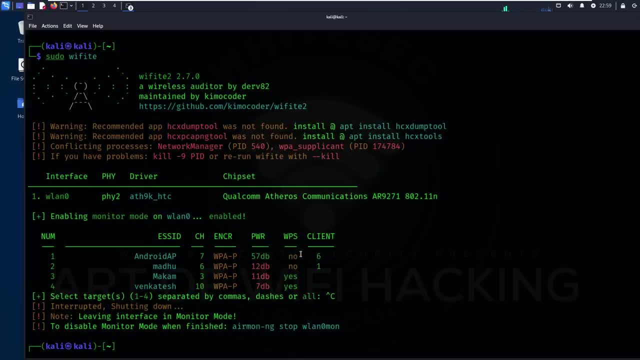 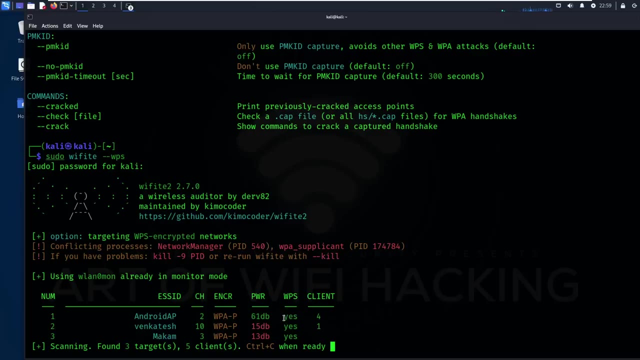 there is a wps is not available there. see, no, is here what i did in my router. i did some settings and i just enable the wps there. so that's why here i can able to see wps is enabled right. so in venkatesh also the wps is there. in makam also wps is there. so here the previous. 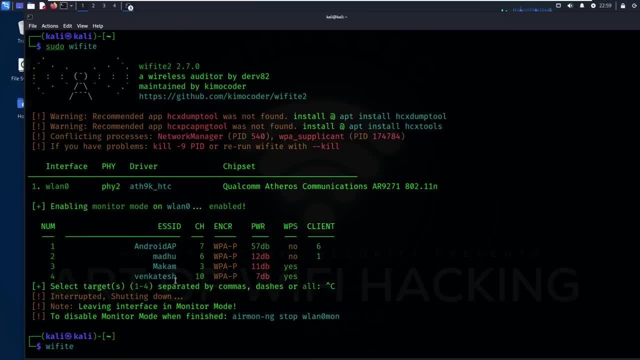 result is here so i can able to see wps is enabled. right, so in venkatesh also, the wps is there in results. just see the previous results. you can't able to see the venkatesh there. okay, venkatesh. sorry, madhu there. okay, because madhu doesn't have the wps in it. okay, this is the thing, so that's. 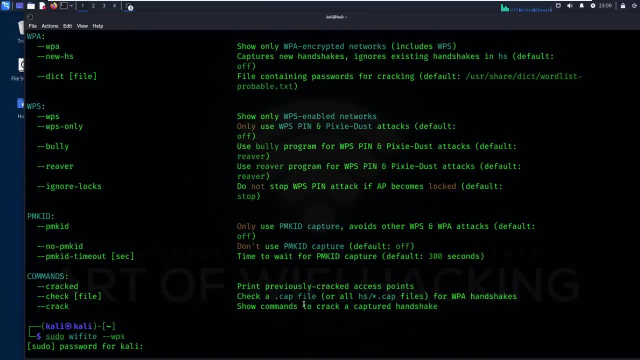 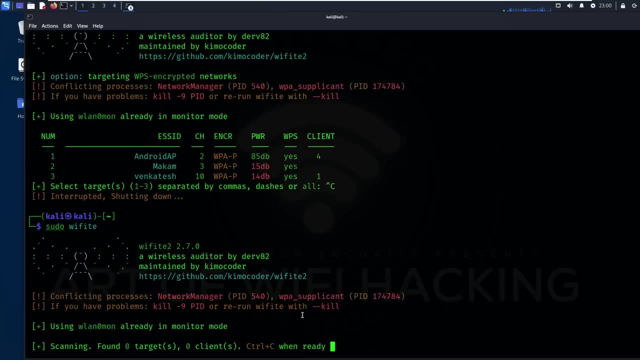 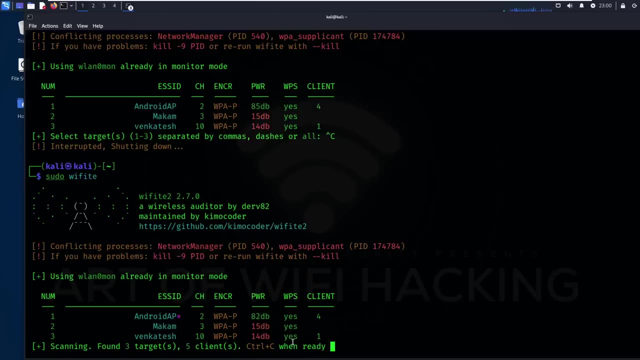 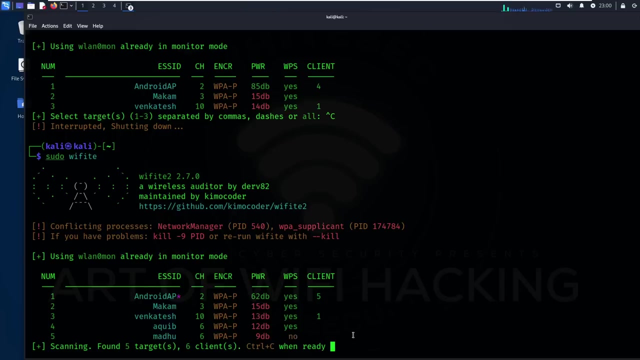 why i can't able to see the madhu network. okay, now, let me, let me stop this one. let me run this normally now see what will happen. see, now i can able to see the madhu network here. so this is how its gonna work. ok, now how to scan the wep network simple. 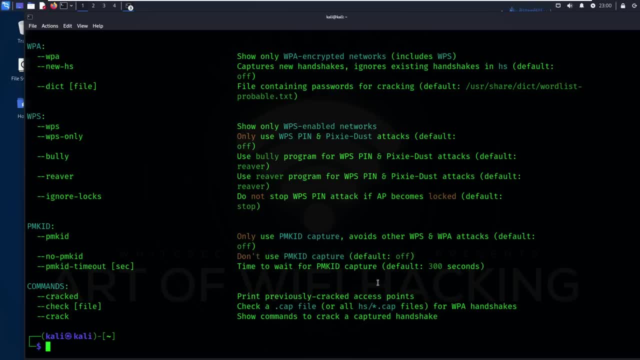 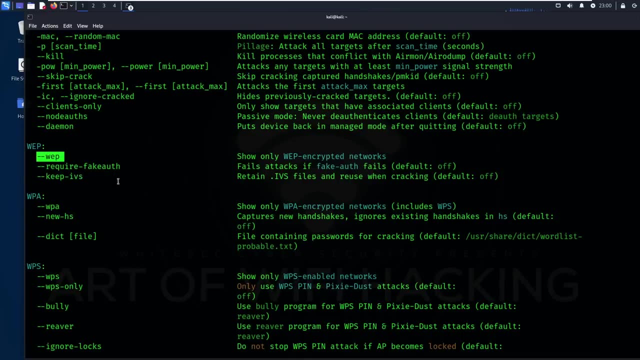 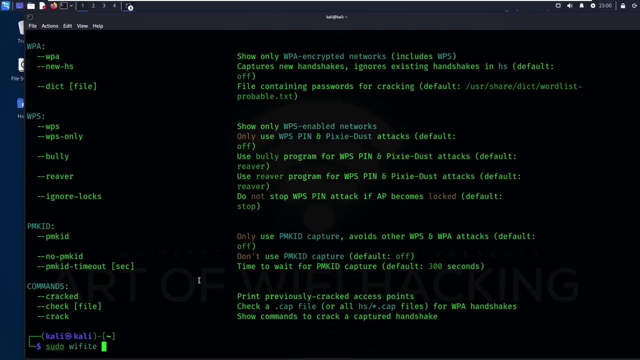 thing, the same thing. ok, see, there is a fake. it is not a big deal. ok, it is very easy to hack the wep network, the same methods you can able to apply on this wep. let me tell you, this is not that much necessary. ok, now, instead of wps, let me scan for wep networks. 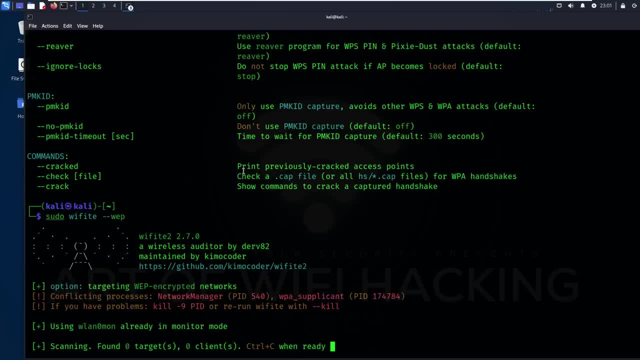 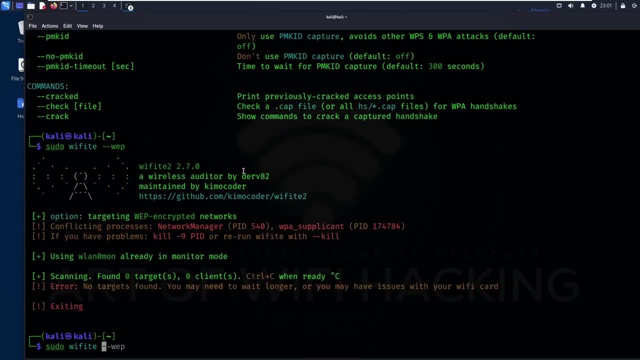 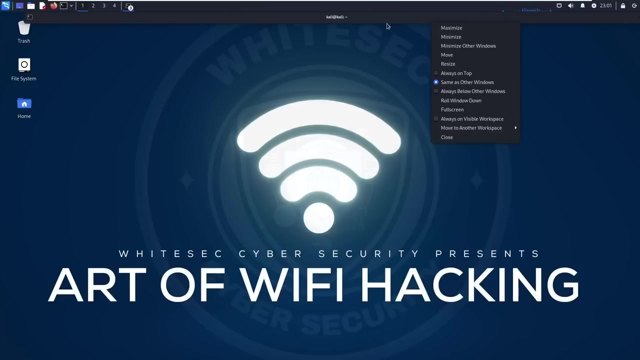 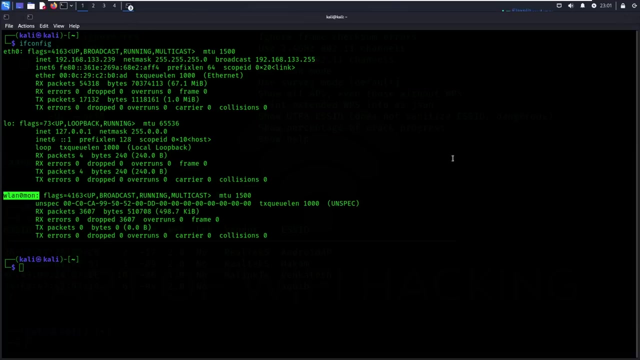 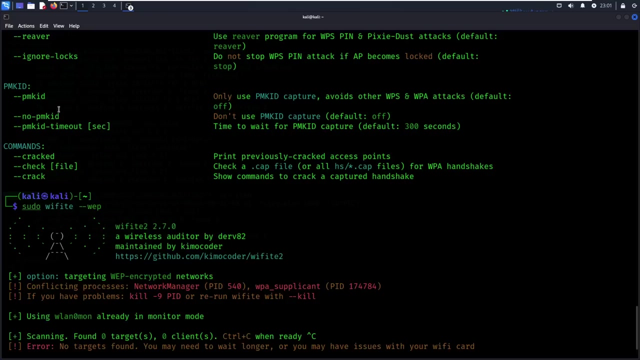 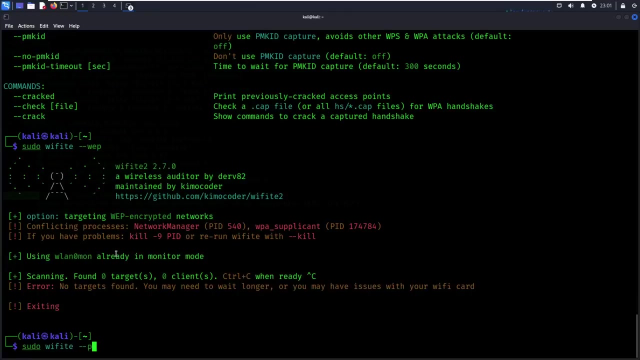 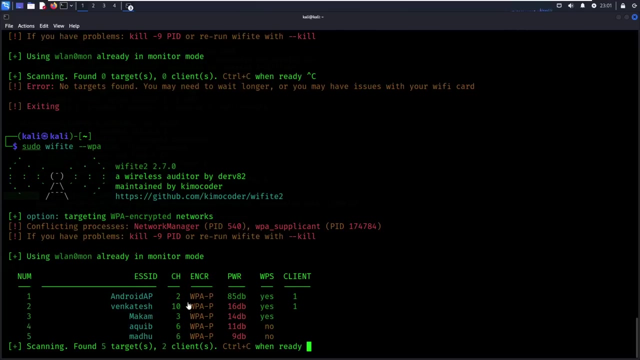 now you won't see any wep network. just see, there is no wep networks in my surroundings, right? so that's why i can't able to see it now. let's scan for now. let's scan for what wpa now see? now, here you can only see the wpa networks. just see the encryption it's talking about. 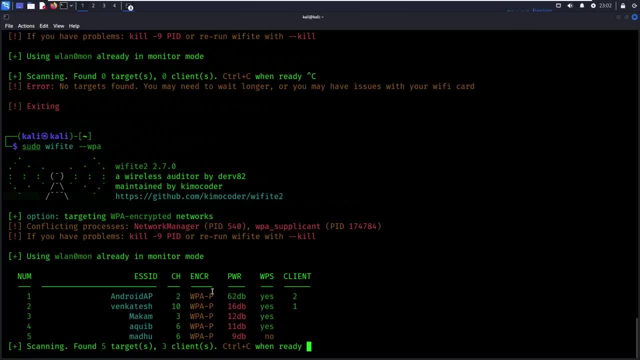 the encryption. once you scan for the wep networks, then what will happen? you can also see wps networks as well. ok, this is the thing. see, don't be confuse here. if you are using any router, then it's totally depend upon you. if you enable the wps, then you can able to see. 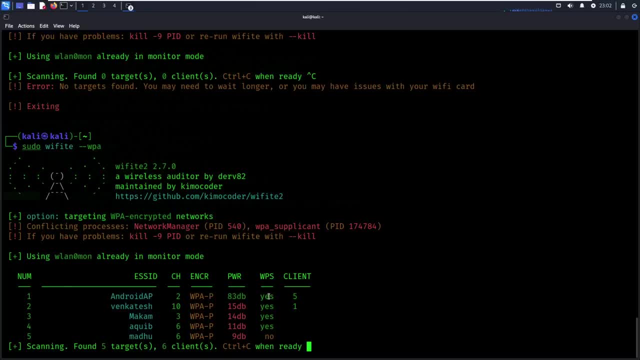 there. if you disable the wps, then you can able to see no there, but still your network will be this one. ok, wpa, this is also a security which we need to compromise. ok, this is the thing. so the thing is sorry, guys. what i am trying to say is, once the wps is there, that 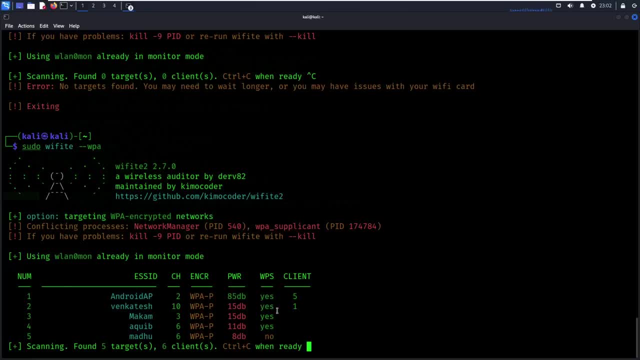 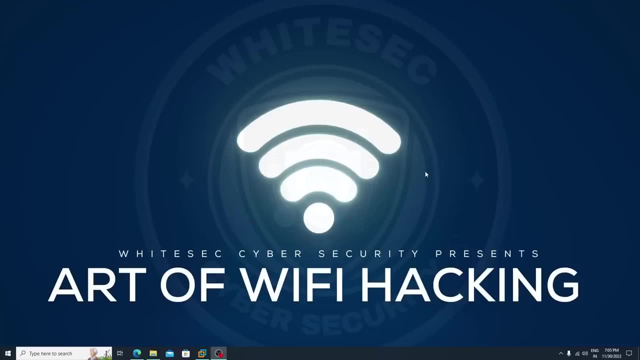 means our chances will increase to hack this network. ok, so in this class you will learn how you can able to hack wep, wps, wpa, wpa2 networks. ok, now the thing is, the attack is completely automation. you no need to worry here. but there are some limitations. 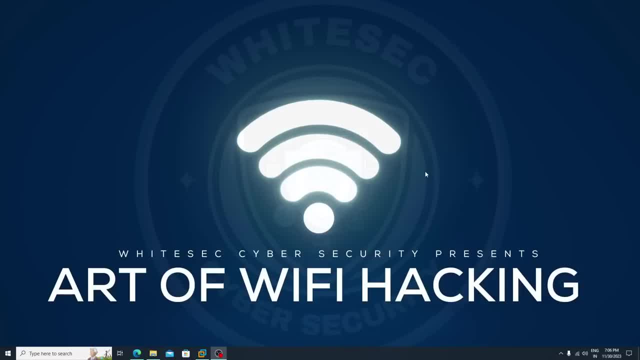 we will cover those limitation. how we can able to avoid those limitations, we gonna cover in the next classes. ok, now, here the thing is. just see for you guys what i did means i just created one testnet, ok. so here you can see that i have created one testnet, ok. 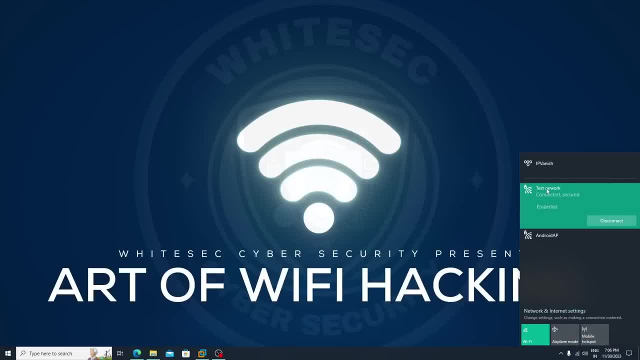 now here. the thing is just see for you guys, what i did means i just created one testnet for the security of this test network. is wpa2 right? it doesn't have any wps. even your target having the wps ok and wpa2 at the time, the attack is same. you no need to worry, even if 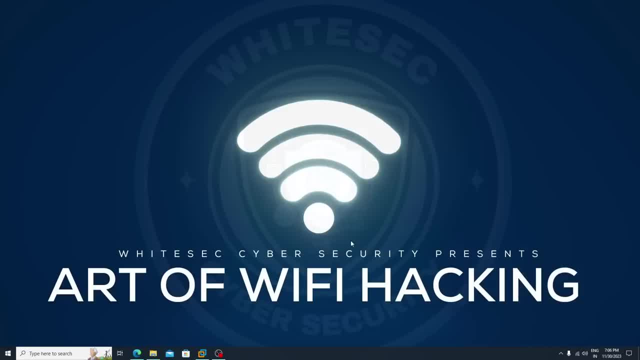 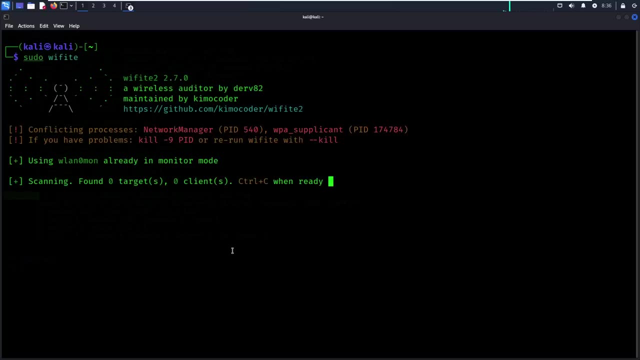 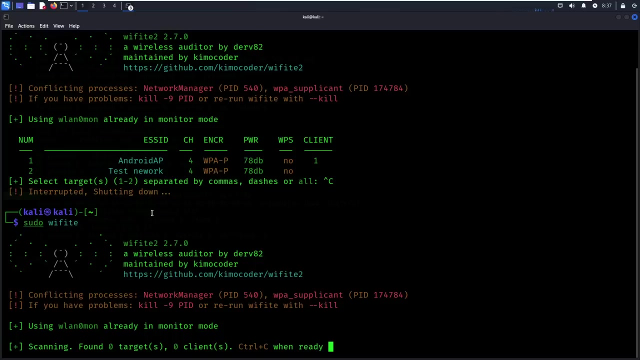 your target is using wep, wpa, wpa2. still, the attack will be same. you just need to run this tool, that's it. it gonna do your the whole work for you. ok now, simple, just execute sudo wifi te. so here i got my target network, which is testnet. ok, now let me scan again. see. 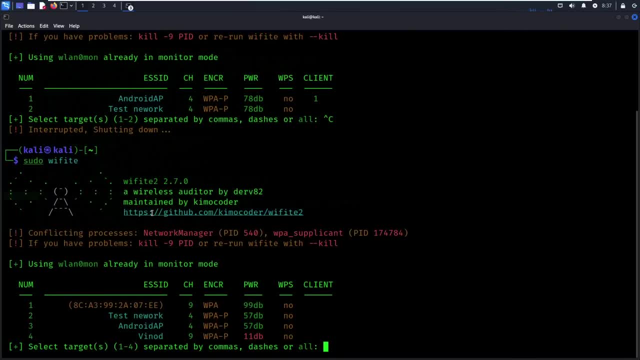 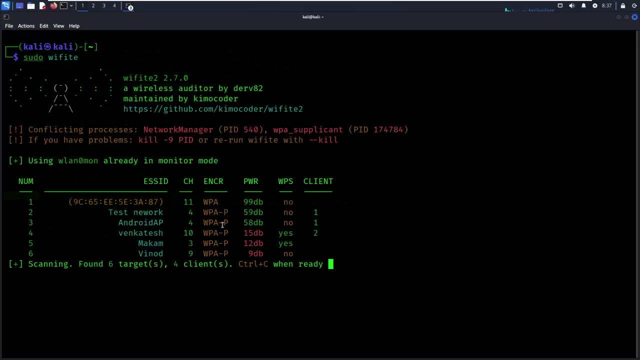 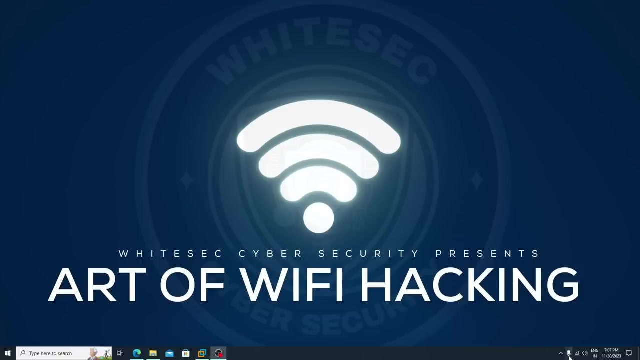 right now you can able to see there is a testnetwork, the client, the device. there is only one device is there which is connected with this testnetwork. let me stop it right. so the device is this one, this windows machine. see, my windows machine is connected with the testnetwork. assume that. 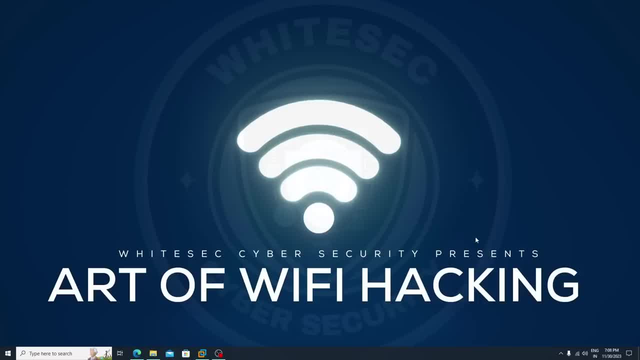 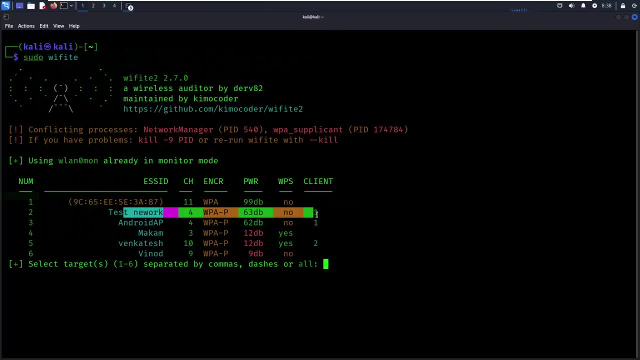 if my android device or my laptop or other devices will connect with this network, then the number will increased. ok, this is the thing. now here, let me target this testnetwork here, just type 2.. let me tell you again: if your target doesn't have wps, ok, and it's using wpa, wpa2 at the 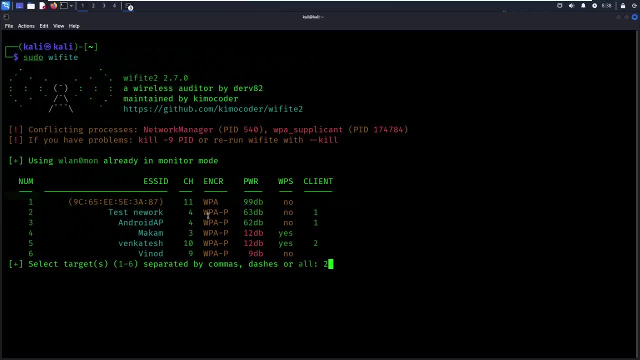 time, what you need to do at the time, what you need to see, just focus on the clients. if the clients are more there, then the attack will be excellent. ok, like you can able to can able to perform 80% of attack there? simple, you can. you just need to capture the handshake, that's it ok. 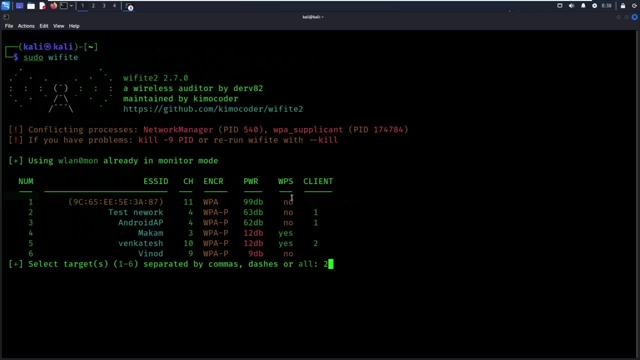 now here let's do one thing: the capturing the handshake. it's a complete automation here, but if you are using this tool, then the tool will do the complete work for you. it will capture the handshake, it will crack it for you, gonna do each and everything ok, so you no need to worry. simple, let me use this testnetwork. 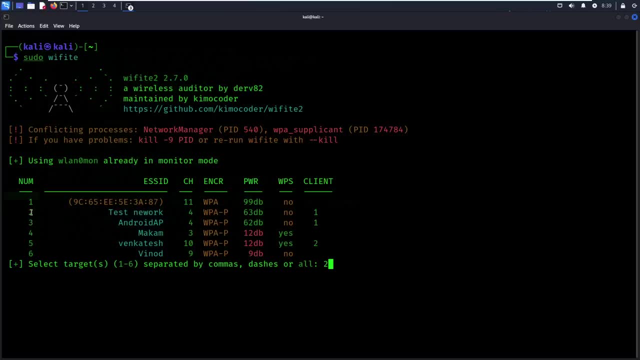 what is the number? number is 2 here? simple, just type 2 there. now the attack will start. see the pmkd. this attacks are basically work on this wps network. still, ok, see here the attack. this network doesn't have the wps. still the attack will gonna perform. uh, even the 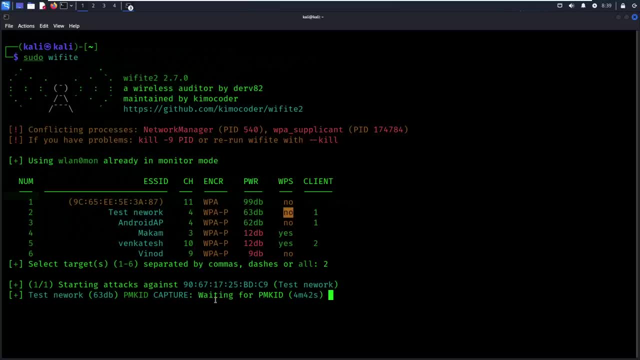 wps is not enabled, still, the attack will start. the wps attack. ok, you want to stop it? you can also stop this attack because see i no need to perform this pmkd attack. i, i want to stop it. ok, simple ctrl c to stop that attack. now here, do you want to continue attacking? just type here: 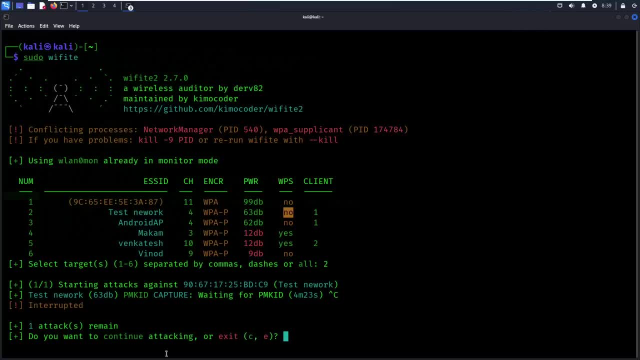 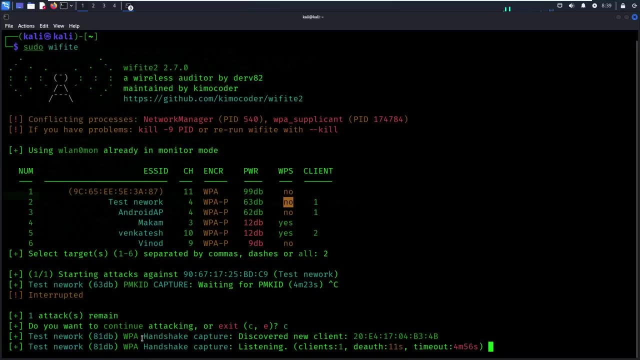 c. i want to continue the attack now from here. wpa handshake will start. ok, see, let me explain you, just wait now. first of all, it will discover the client. the client is here. ok, it does. uh, just discover the connected clients. ok, like connected devices right now. i just told you. 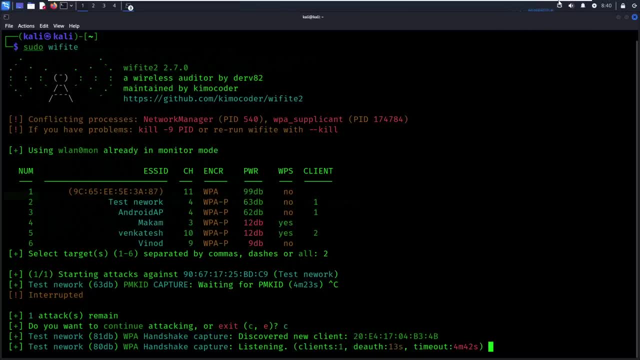 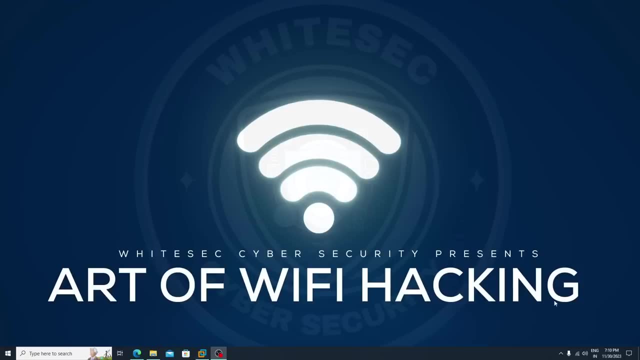 there is only one device which is connected with this network. now it's starting the de-authentication attack. the authentication attack is a nothing, but it will disconnect this system. see, it's successfully disconnected the system. sorry, the the device with the with that wi-fi network. okay, after disconnecting it, what will happen means it will. 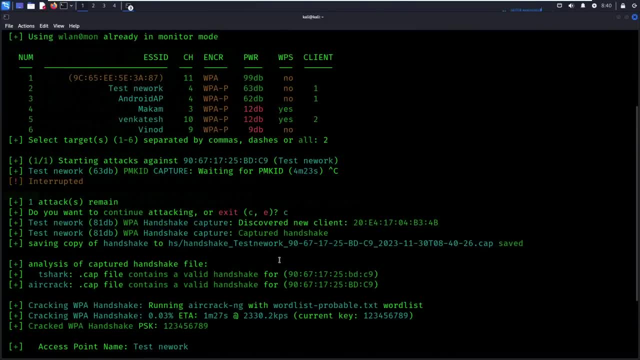 successfully capture the handshake here. okay, i'm gonna explain you the complete process how this gonna work, this capturing handshake, each and everything. so the simple thing is the. the attack is complete automation. okay, after reconnecting the network, what it's do means it: it gonna capture the. 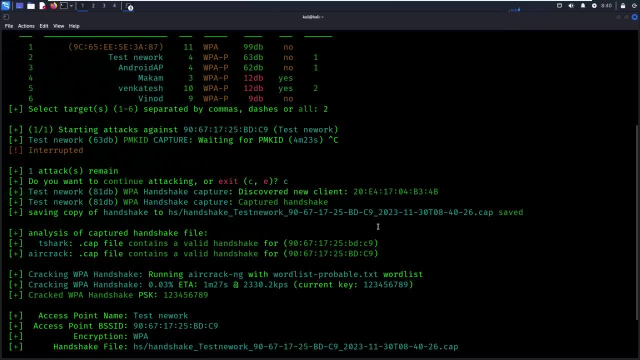 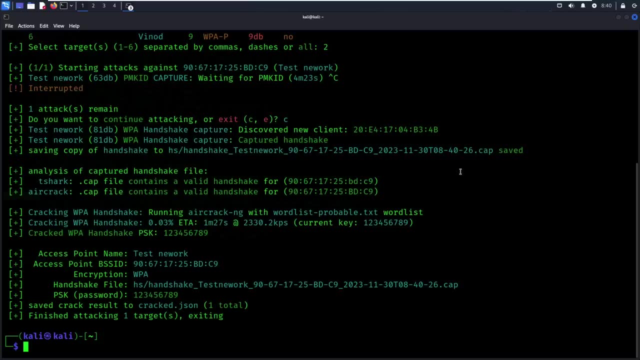 in this handshake there will be a password which is encrypted. you need to know that. now, to crack that encrypted password, what it gonna do? it will perform the brute force attack on it. okay, see, by using air crack ng simple the process. again, i am saying the process is complete. 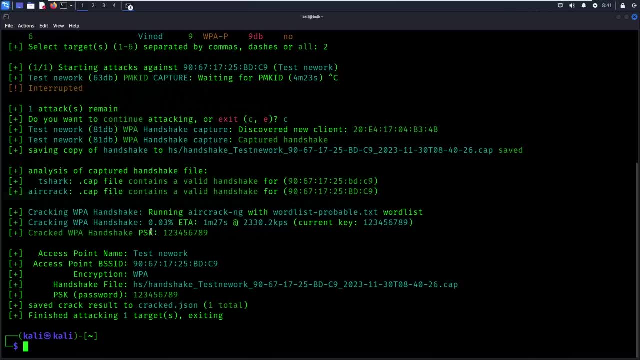 automation, it will crack the password. see the current key. is what here? the key is one, two, three, four, five, six, seven, eight, nine. this is my wi-fi password. okay, if you are. if you are target using complex password, at that time the things will become complicated like you need to use, uh, the. 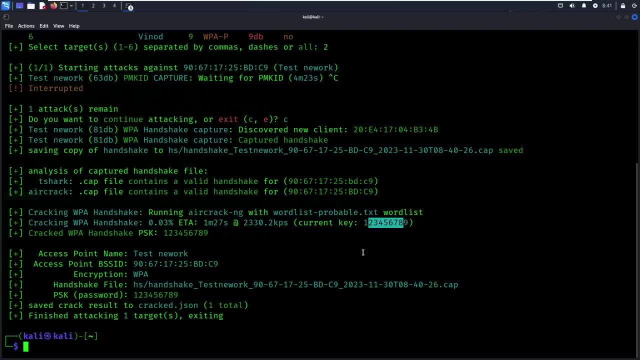 word list for it. okay, like, see, by default in wi-fi t there is a word list, it will use it. okay, but how to add your own word list here to perform this attack? okay, like, from where you need to download the word list? i'm gonna cover this whole process and later i'm gonna cover how this uh attack gonna. 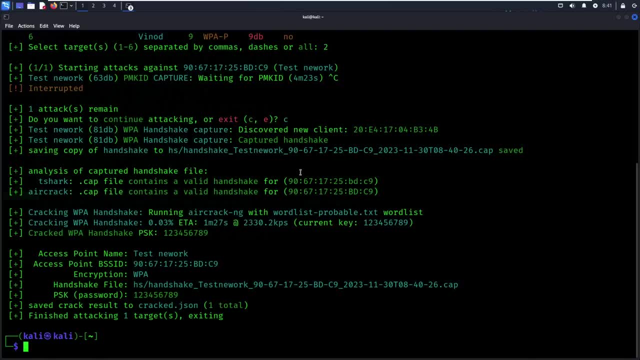 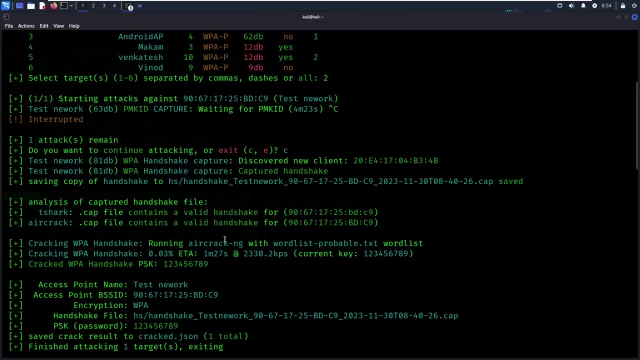 work like capturing handshake. what is this? each and everything i'm gonna cover in next classes. you're gonna learn how to do it, okay. so now let's learn about dictionary attack. see by default the wi-fi t. use the default world list. okay, which is this one which is useful to crack the handshake? see in. 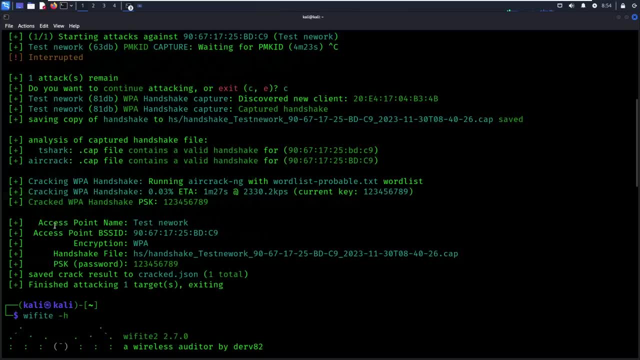 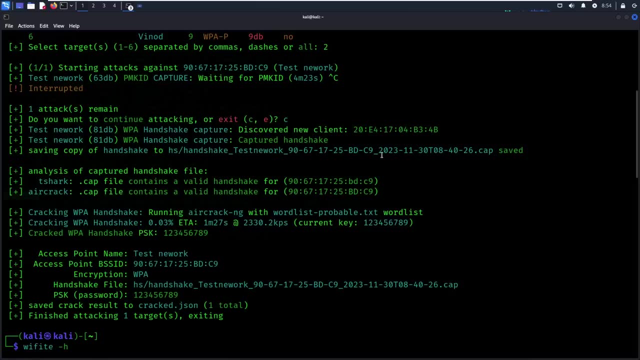 the last classes we cracked the handshake right. the simple thing is the handshake file is encrypted. you can't able to see. see in handshake file there is a password, right, you can't. if you open this handshake file, you can't able to see any password there. simply, we'll see. the network name security. 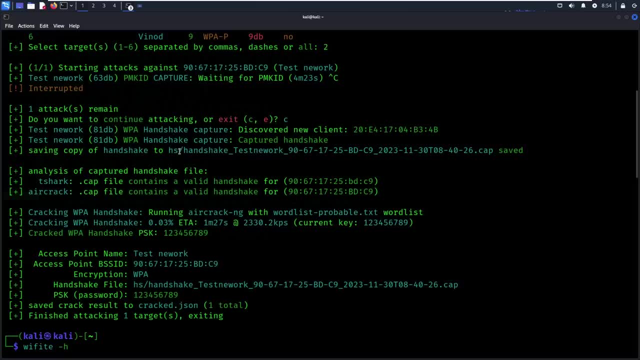 like that, but you can't able to see the password. password is present in this uh cap file. okay, this in the handshake file, but the password is encrypted, you can't able to see it or you can't able to read it, so you need to crack that this one. okay, this handshake file. after cracking that, what? 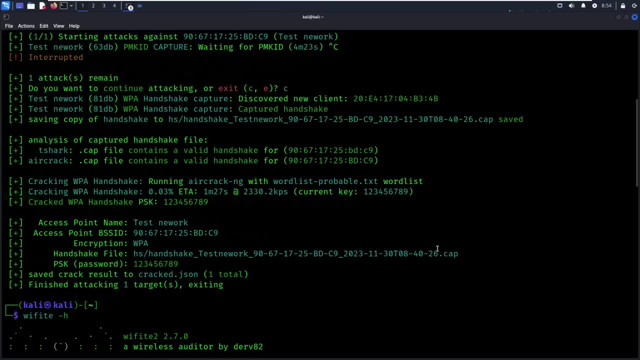 will happen means it will show you the clear password. okay, this is how it's gonna work. the simple thing is by using aircrack ng, the process will done. you no need to worry here. okay about, but the thing is here. yeah, in the real world you need to use excellent word list. okay, if you are. 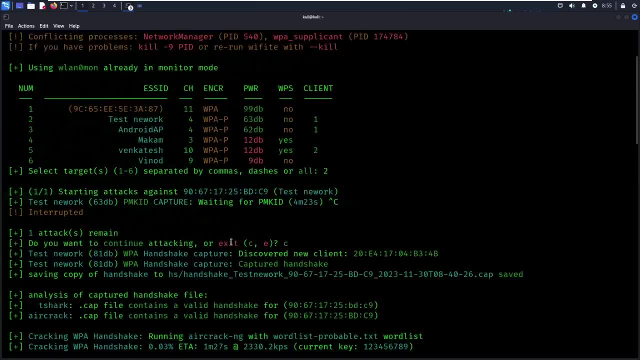 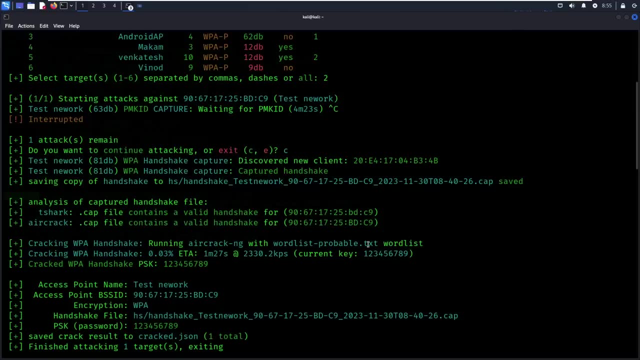 using the by default word list of wi-fi t, then it won't work. okay, this is the thing. mostly incorporate areas. what will happen means the password is uh, not uh that much secure. okay, simple, you can able to use a word list and you can able to crack it. 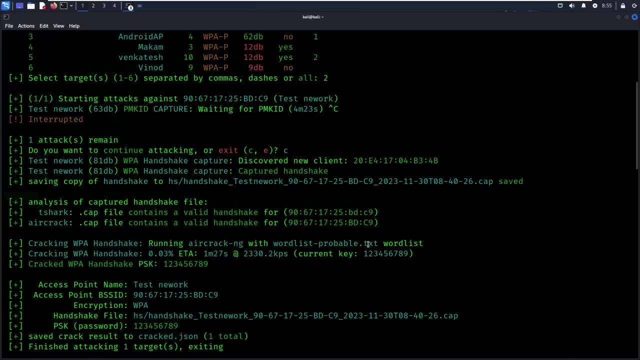 okay, but when you target the home network right at that time that things become complicated, because these guys in home network, what they do means they use their own names, phone numbers okay, uh, they use their birthday, something like that. so here the things will become complicated. at that time you need to create your own word list. okay, according to your target, but during targeting 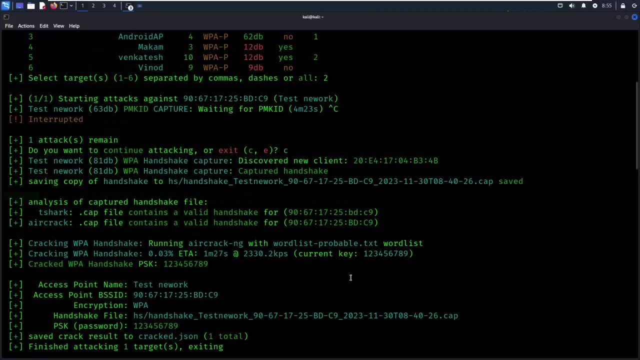 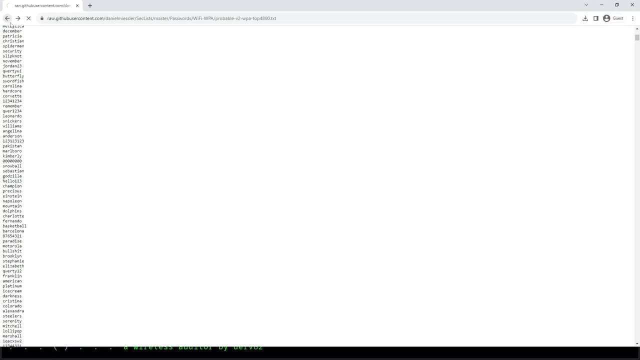 the corporate networks at the time. you can go with the word list, okay, or you can also generate your own word list according to the company as well, okay. but the thing is, let's go for the easy way, let's go for the checklist here. just search for checklist in google. uh, in google. just let me show you. 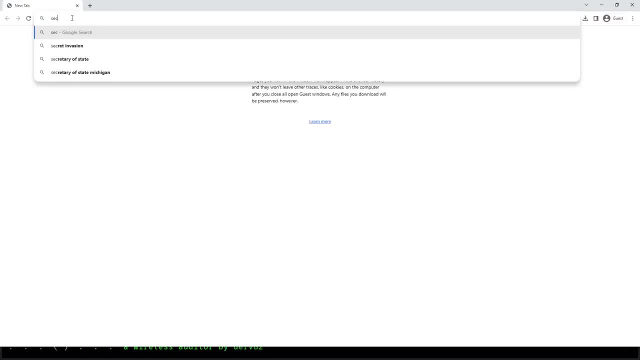 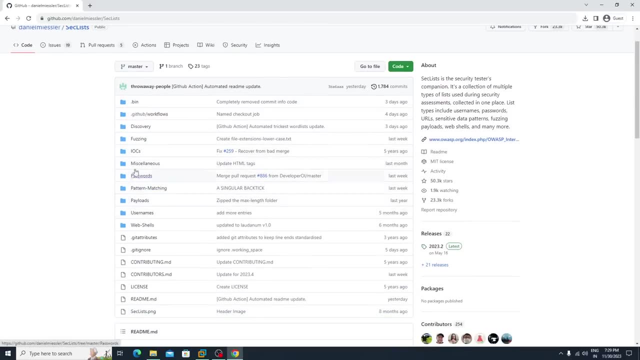 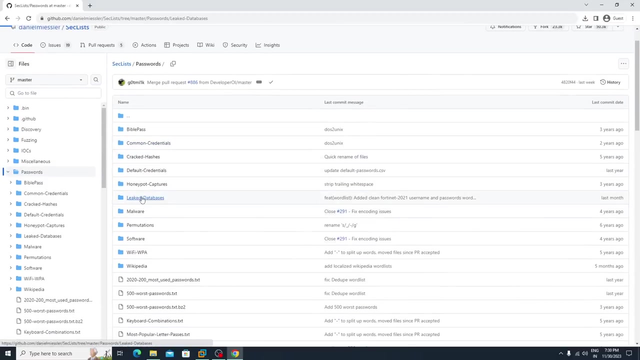 just type here checklist. this is a very now. simple go with the. there is a fuzzing, okay. simple go for passwords. see there is a leaked databases. this one is very useful for you. I feed thanks to assist pandas jing for one company at that time. this word list is very 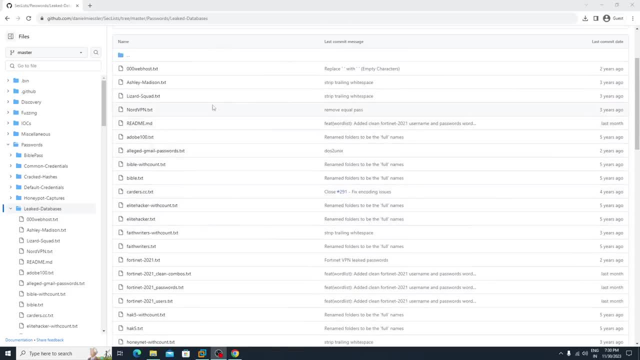 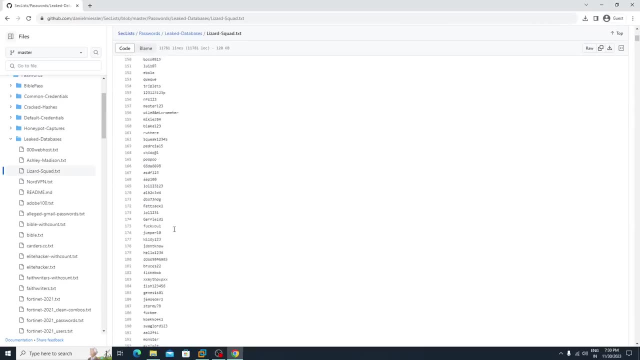 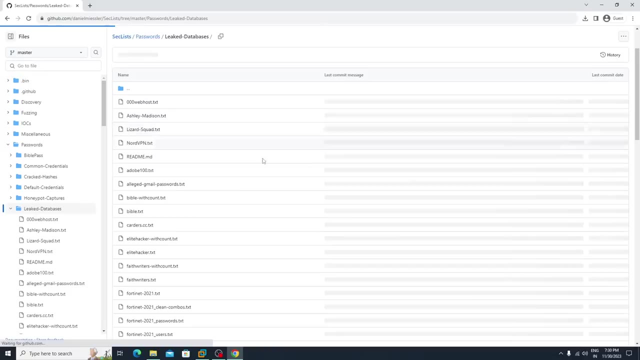 useful for you, because this are the leaked database- uh, leaked database from where they just founded the password. okay, so this are the passwords. will there? just dumped it? okay, after hacking that database, they just got this one. okay, this is the thing mostly during targeting this corporate network. 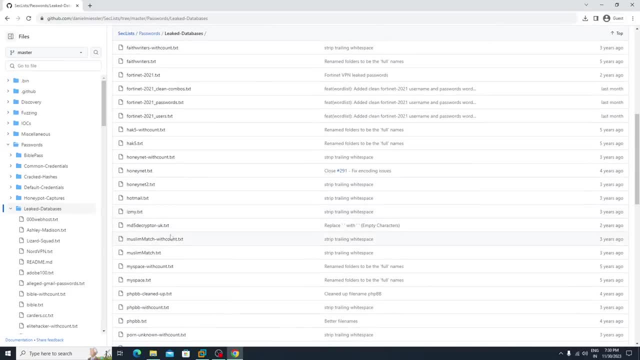 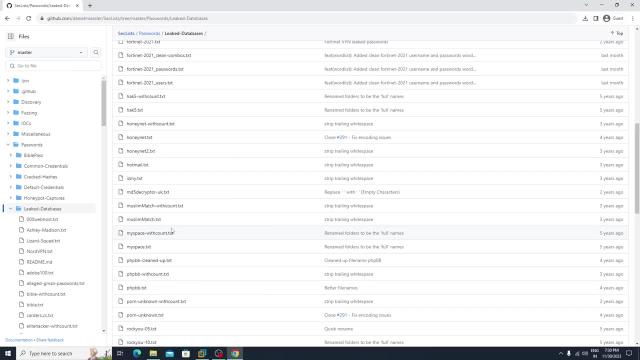 at that time this will again. I'm saying these three things are very useful for you. okay, If you are targeting your family network and friends still get leaked, uh, the things are very kind of uh hard, okay, because the home network use their own name. 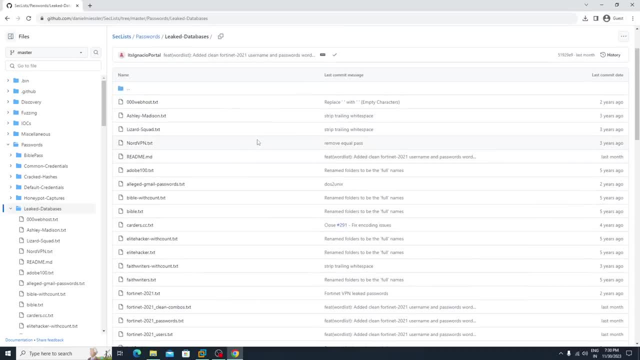 sometimes they use their phone numbers, they use their car. uh, sometimes what they do means they use their car plate. there is a number, is there right? they use like that? okay, they use their birthday, uh, year or something like that. so the way you are targeting the home network you need. 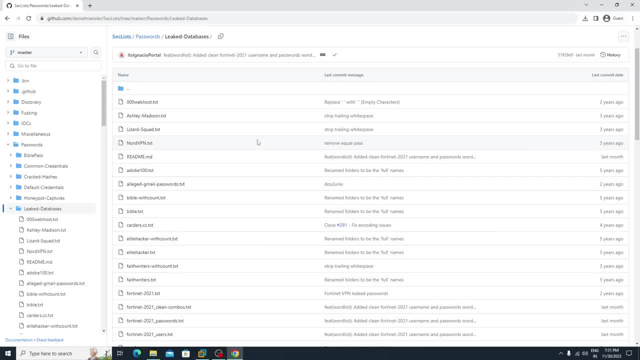 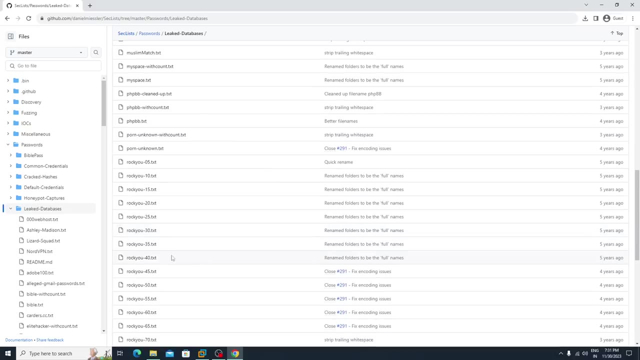 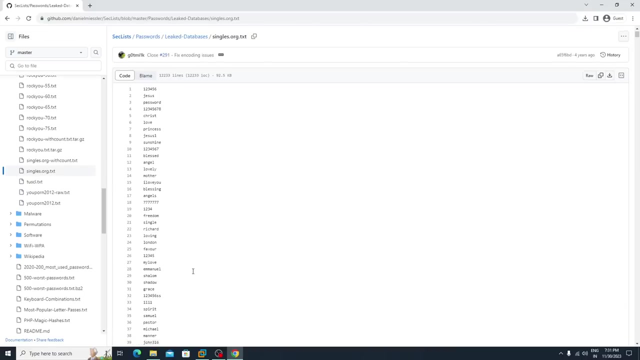 to create your own word list according to the target. okay, this is a thing. but uh, just right now, let's go with this. this word list only. okay, now, here there is. just just select any. uh, raw queue is here. okay, just select any of this word list. okay, let me select this one. if you click on raw, 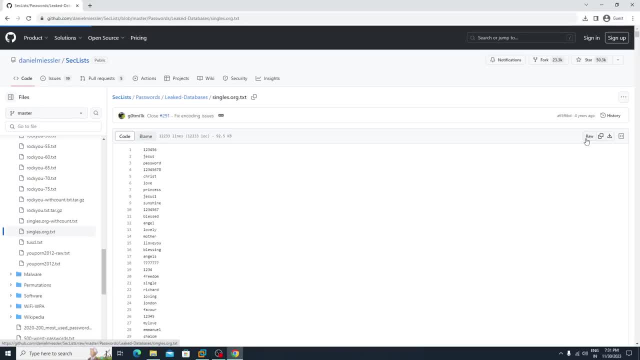 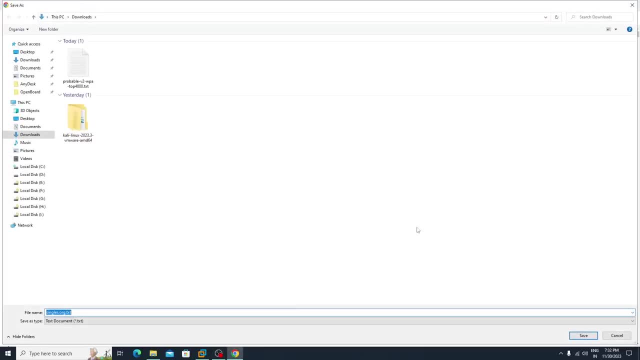 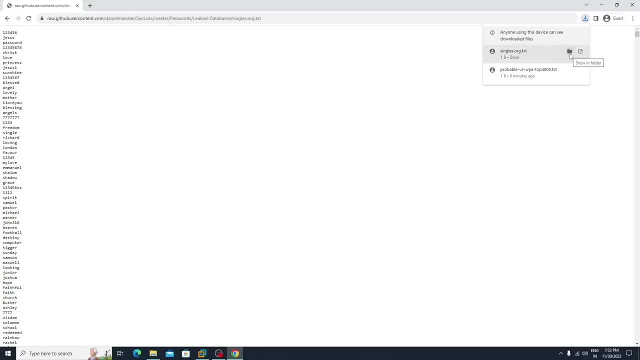 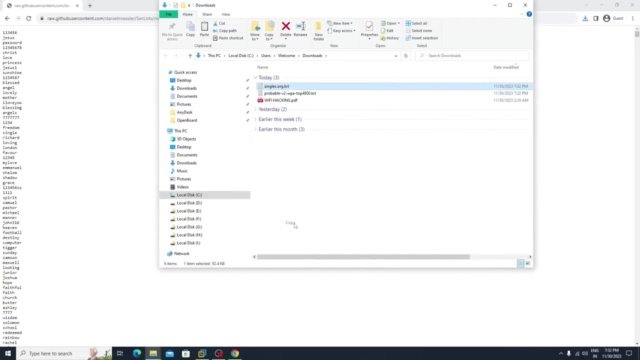 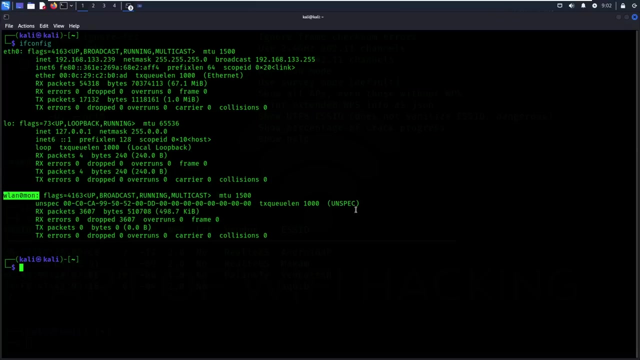 simple right click, save as and save the this text file. you can also open this url and download it on your linux machine as well. but for you guys, i am doing from here simple: let me copy and paste it in my linux machine. so let me paste here right now. the thing is, if you want to perform a dictionary attack at that time 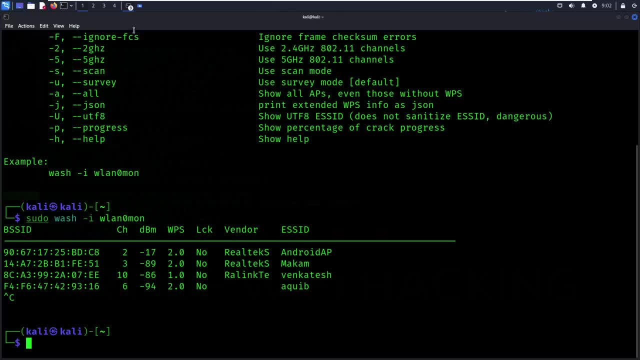 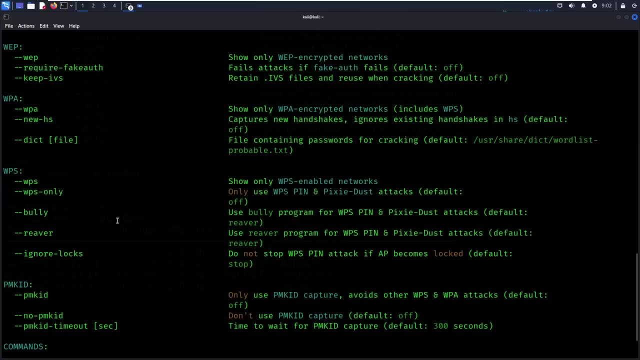 what you need to do? just type wi-fi dash h. here you can able to see dict. is here right file containing password for cracking. by default, it's use this one, okay, but we can also provide it okay our own word list. how to do it simple: you just need to type here: wi-fi te dash- what is it? the flag? 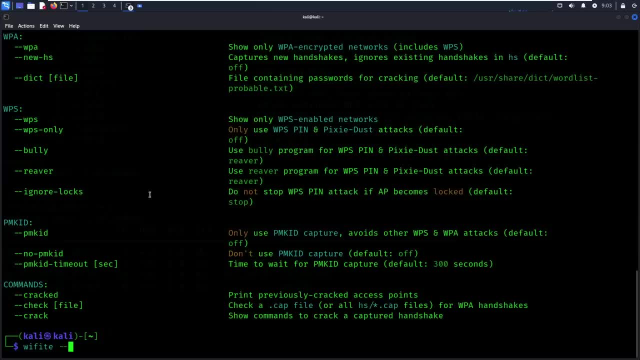 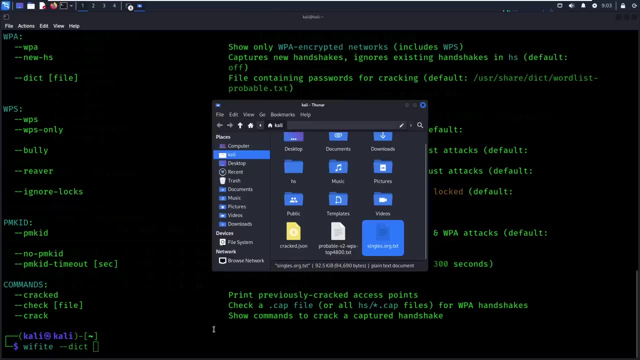 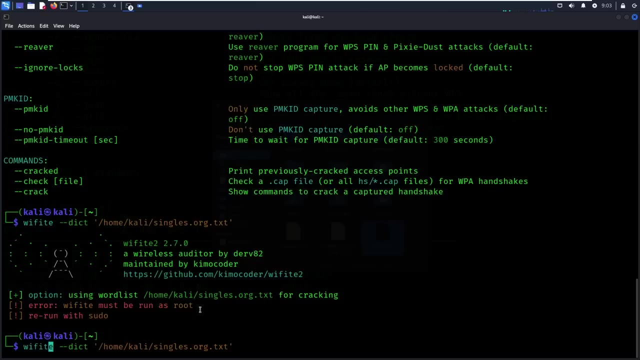 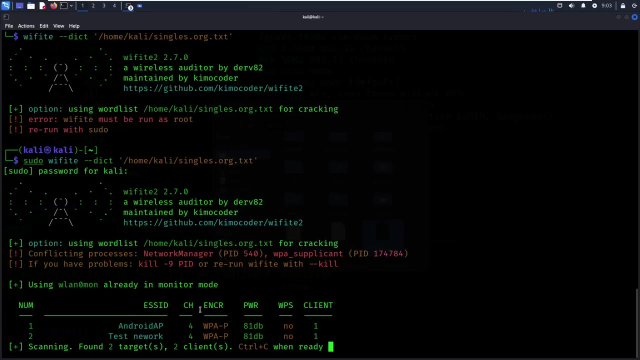 dash, dash, d-i-c-t. okay, then just drag and drop your word list okay, which you just downloaded from the internet, from checklist. see, you need to run it as a sudo. so here is my text network. just let me select that one. now i don't want to perform the pmk id capture because my wi-fi network is not. 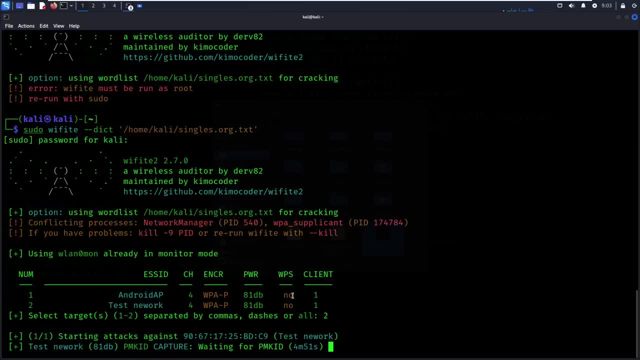 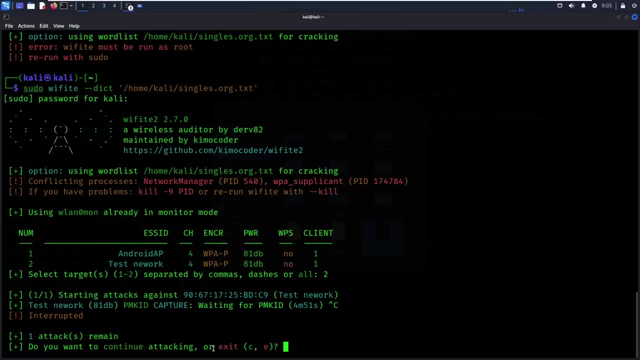 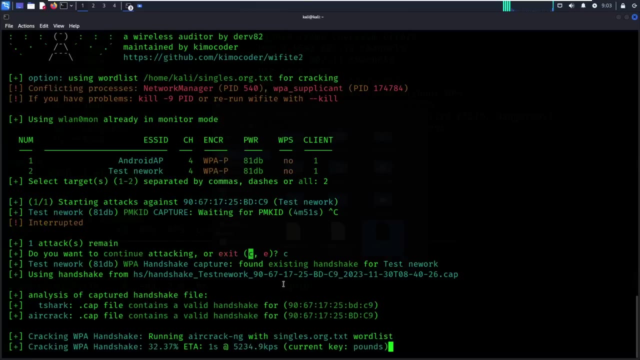 wps. simply let me stop it. now let my. my network is wpa, right, so let me do. do you want to continue? attack or exit? simple, let me continue. just type c there and control. now see it started to cracking the. it successfully captured the password. okay, after capturing the password. 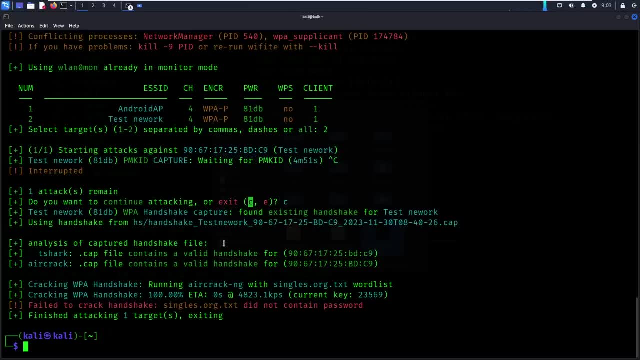 what it did means it's started to crack that password there. okay, now that hash simple what it's saying: fail to crack. handshake did did not contain password. this is the thing at the time. in real world, you will see a hell lot of these things at the time. you need to create your own. 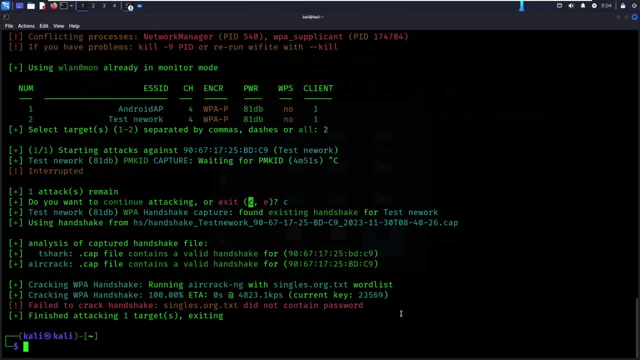 word list or simply download it from internet. mostly, just try to use the raw queue first. okay, the raw. uh, there is a raw queue. it's a huge gb. if you search it on internet then you can able to find it. okay, uh, it's just use the file which is related to six to eight gb. okay, if you are. 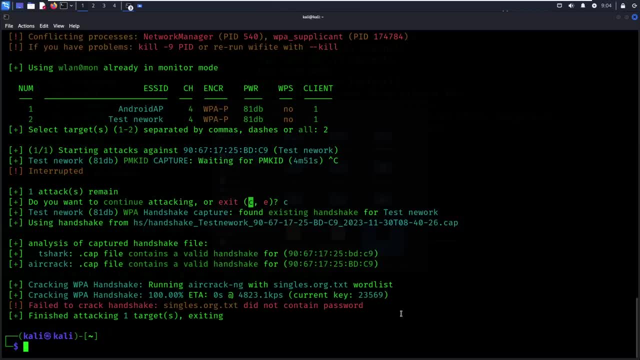 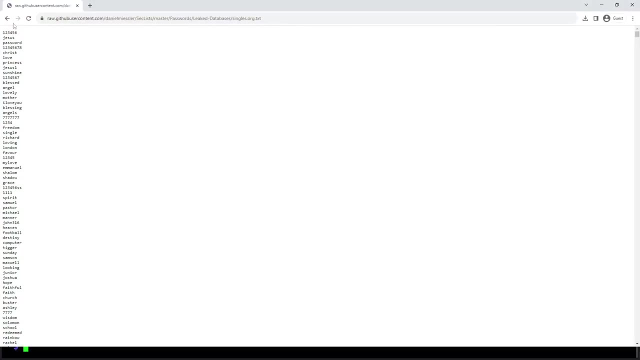 targeting the home network or something like that. at that time, just the file size must be six to eight gb. okay, this is the thing. maybe it may contain the passwords. now here, if you are targeting the corporate network, at the time, first of all just choose, choose this things. okay, from here, mostly you can able to crack it, but it will take a huge time. 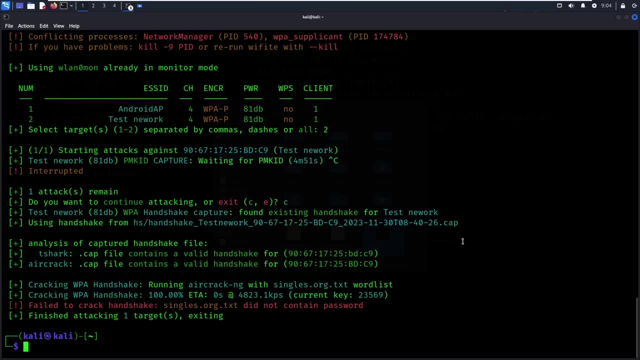 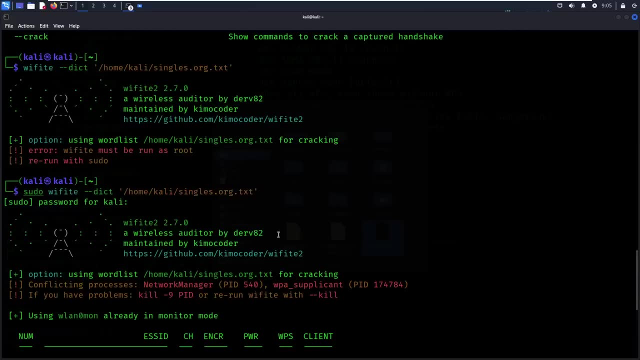 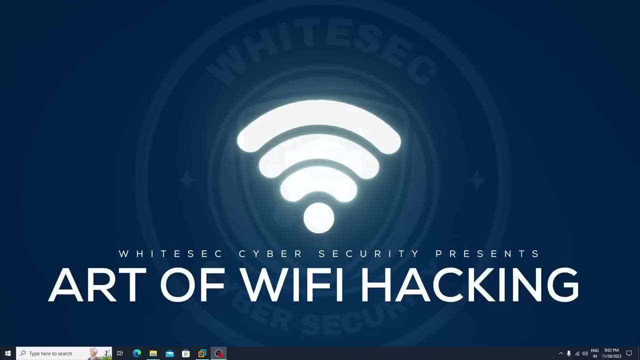 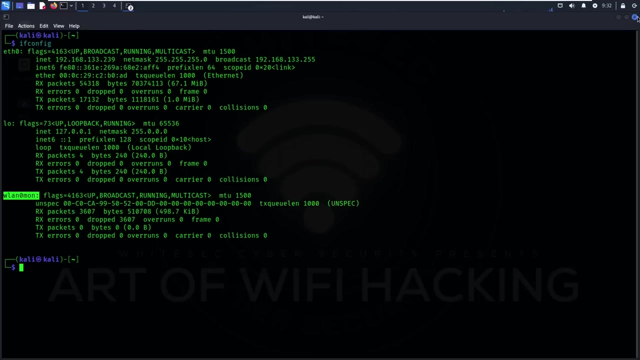 so hope you guys enjoy this classes. basically, here we just learn how we can able to perform this dictionary attack, how we can able to add our own. what is there to crack that handshake file? in this class we are learning how we can able to perform attack on wps, enable networks- okay, by using river. see here we are using river. okay. now. 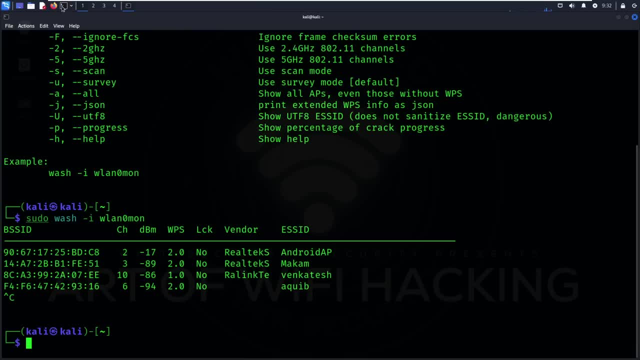 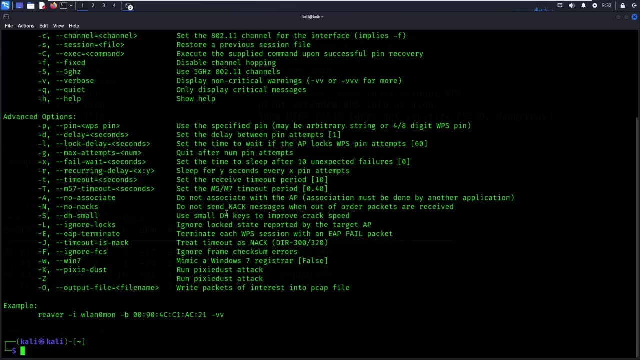 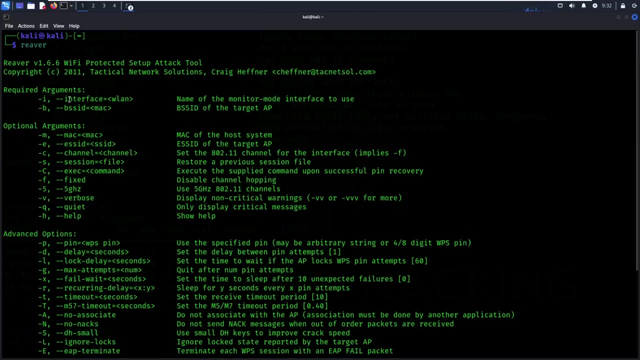 by you. no need to install the river here. simple, by default in your linux there is a river. simple, just type river, then here you can able to see the arguments. now dash i for the interface, your name of the monitor mode: interface. you must, first of all you must- be in monitor mode. 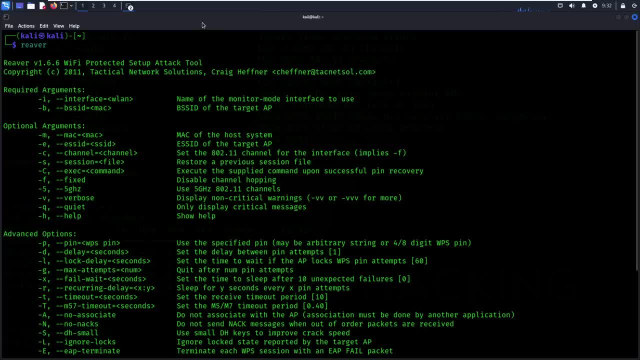 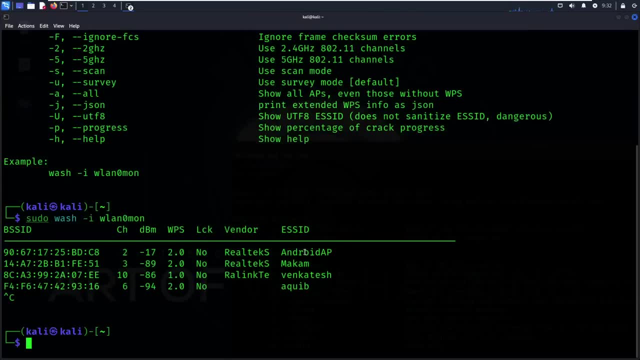 your adapter must be in monitor mode. after that there is a dash b bss id. bss id is a nothing but your target. right now, i'm targeting android ap, right, so you just need to specify your target bss id here. okay, this is a thing. after that there is a mac. is there e s s id? is there e s s id is a nothing but. 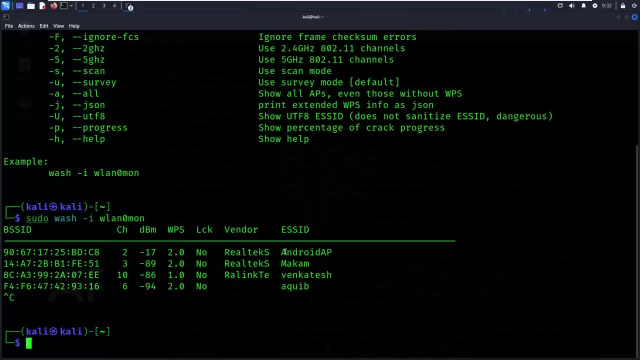 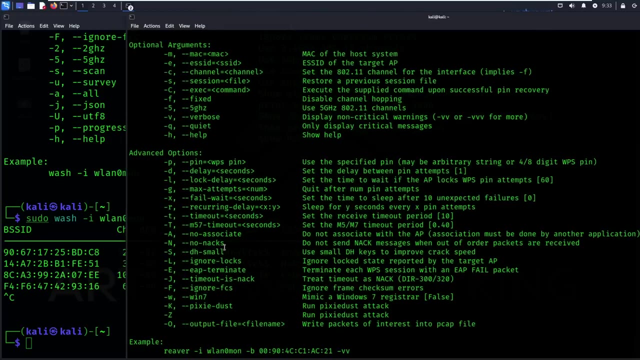 the name. okay, if you don't have, uh like, you can also provide the bss id or essid as well. okay, this is the bss id here, so you can just use the bss id to activate it, and here you. this is the thing. so there is also a pixie dust attack here. see, there is a dash k, dash k is. 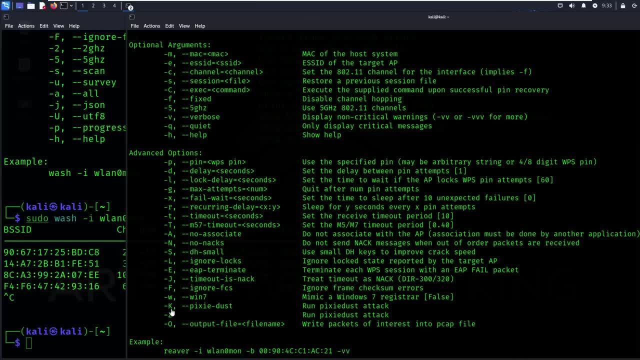 nothing. but if you want to perform the pixie dust attack, then you can able to do it. okay, the same, for if you type z as well, the capital z, it will start the pixie dust attack, sorry, dust attack. okay, now here how to run it. first of all, this attack will only work on those devices, those 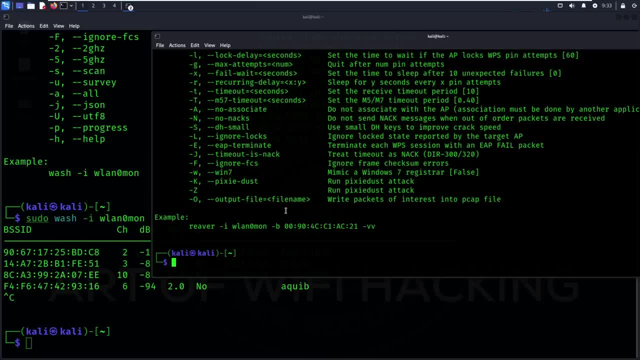 routers which enable, which have the monitor wps enabled. okay, now how to use it. the simple thing is just let me type from here, only just type: sudo a river, r-e-a-v-e-r, then first of all change your adapter to monitor mode. if i type ifconfig. 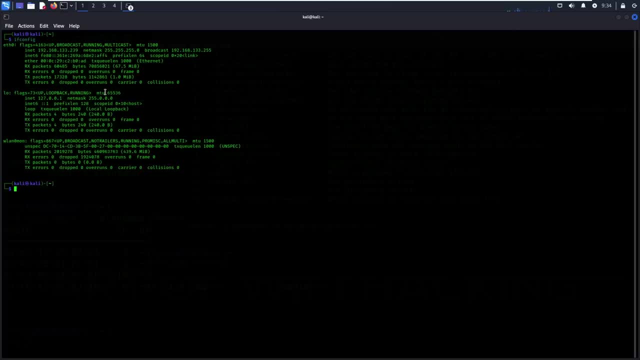 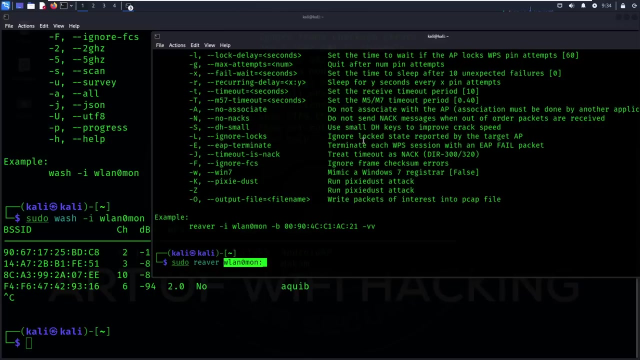 here you guys can able to see my adapter is in monitor mode. okay, if i just covered how you can able to change this to monitor mode, okay, your wi-fi adapter to monitor mode. simple copy the name there, we'll paste it here. in my case it is wlan 0 mode. now here you just need to add the. 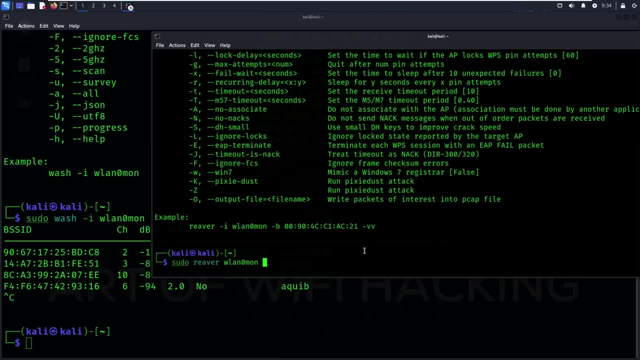 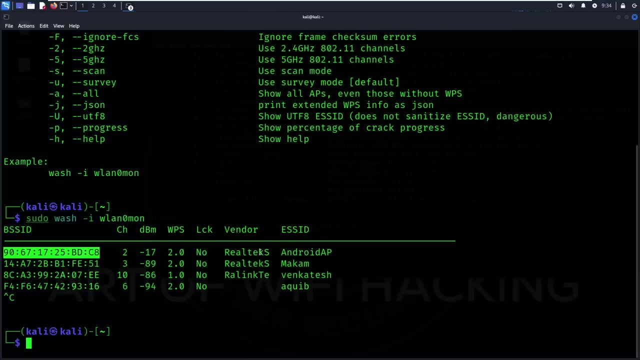 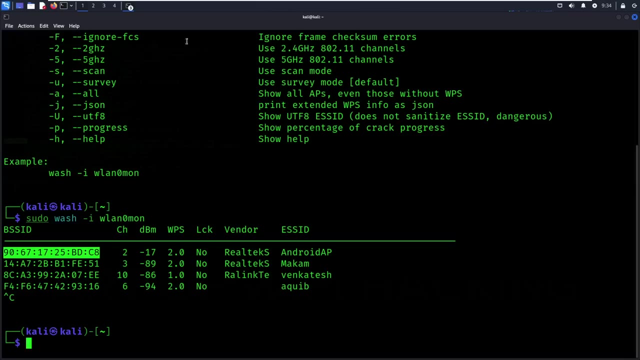 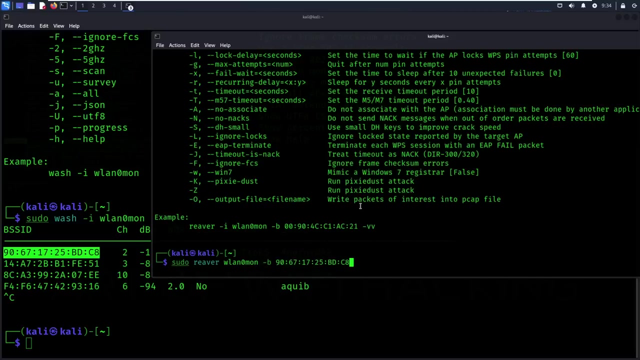 bss id. just type dash b and your target bss id, simple, just in my case the target is android ap, but still, let me cover that, okay, so you guys can able to implement this. it's a very easy, you no need to worry here. simple just type here your target bss id. then now i want to start. i want to use 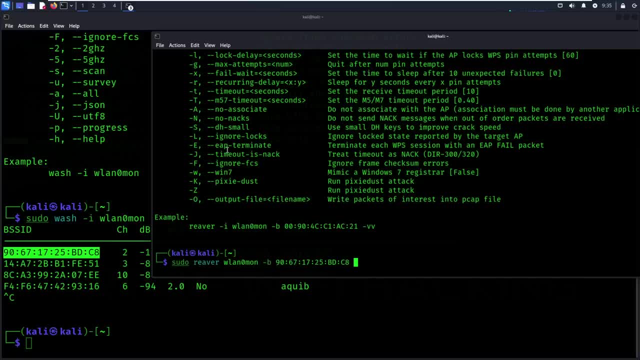 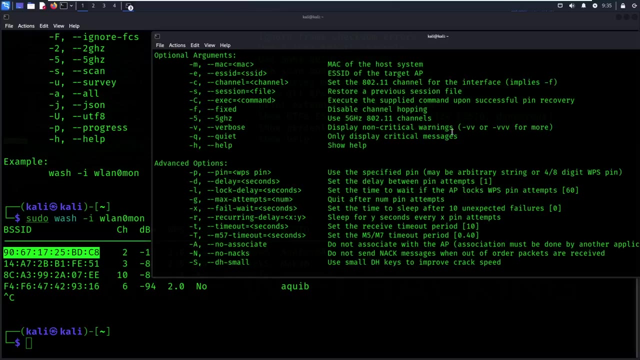 this one as well: pixie dust attack. okay, at that time, what you need to do, you can also say: if you want to see the output, okay, you can type here a verbose output. okay, you can type here a verbose: there display, non-critical warnings. simple, just just. first of all, let me use the pixie dash here. 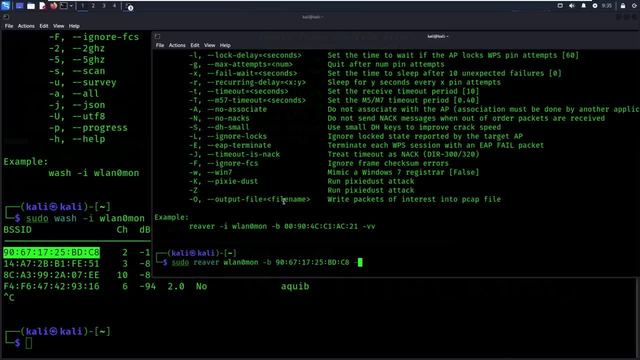 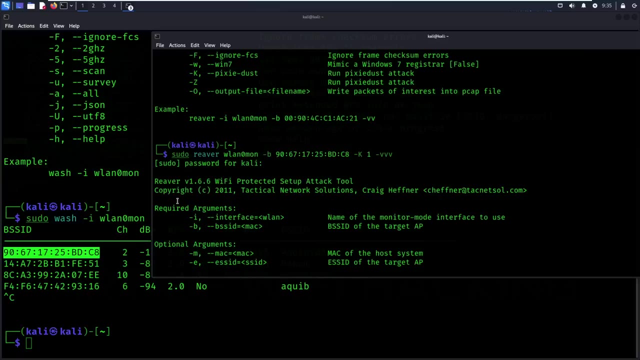 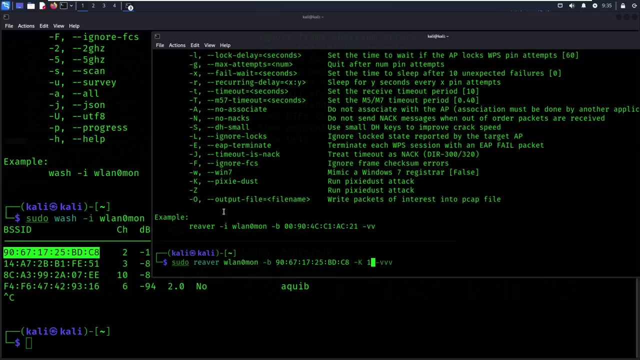 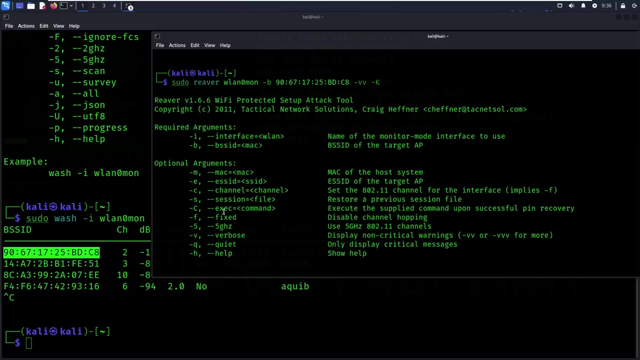 attack a dash k, just type one to use it. then just type here: verbose dash vb. just type enter. now the attack will be what happened here. so let's start it. okay, the thing is the wps, i think, is not enabled here. first of all, you need to run the wash. 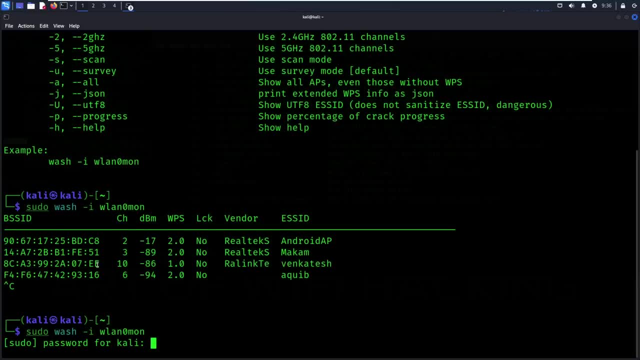 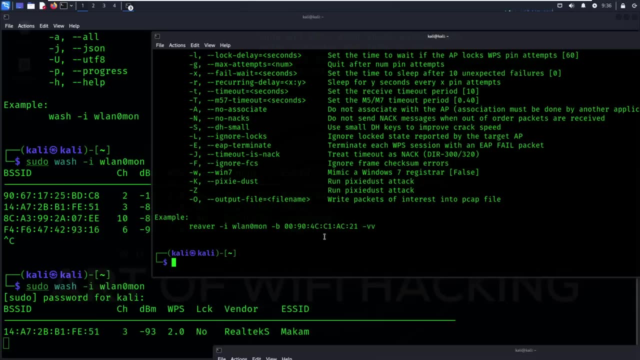 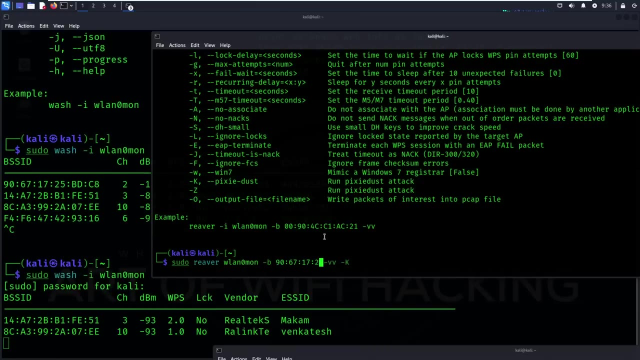 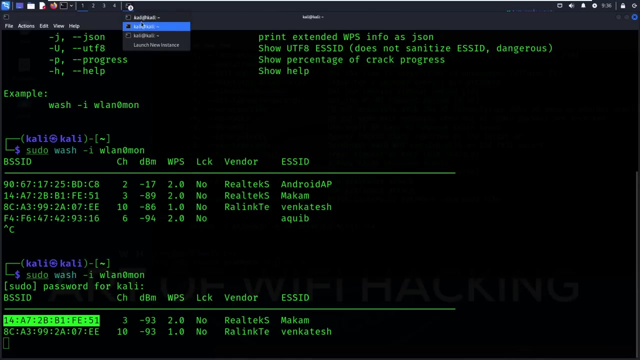 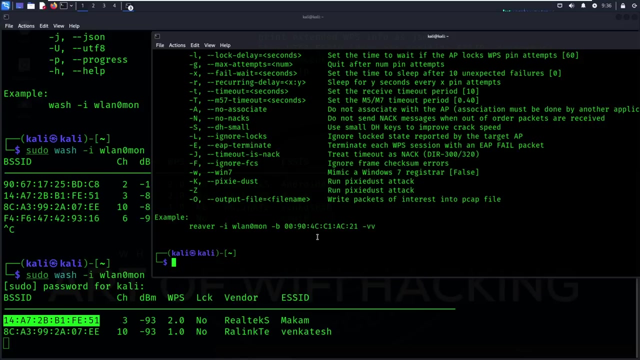 and then you need to start this one. the the network is not that simple. let me do one thing. let me use this one. okay, i'm not hacking it. simple, i am just testing it. okay, i'm gonna stop the attack. okay, you no need to worry, so simple, just type here. okay, let me type one here. the verbosity is not. 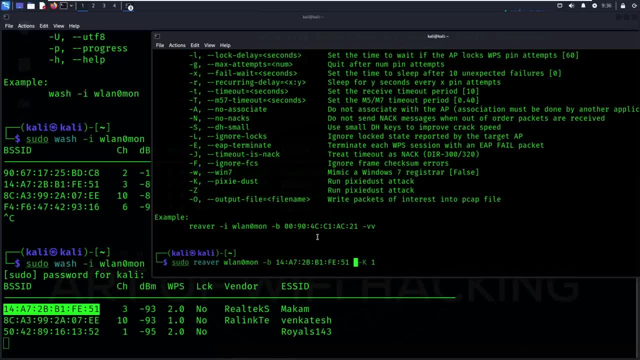 working, but i'm gonna stop the attack. okay, you no need to worry, so simple, just type here, type enter, or simple. let me type this command: pss id. okay, man, sorry for that, i just forget it to add the dash i there. okay, so this is the thing. 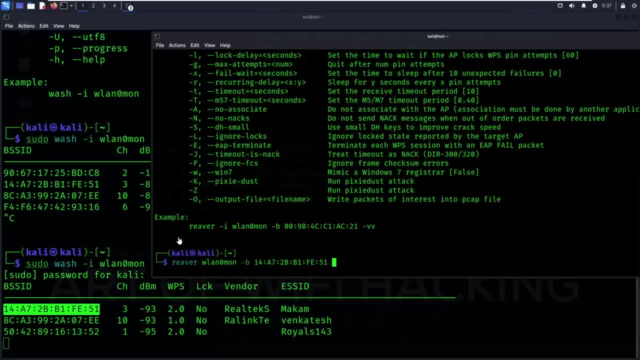 mostly i won't use a reverb. instead of using reverb, i use a wps wpa tester. sometimes what will happen means by using reverb you can't able to hack this wps enable network at the time. i use this one w. mostly i use wpa wps tester. when is there any kind of wi-fi router? 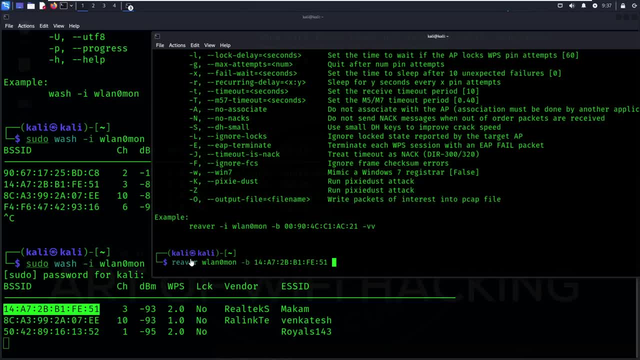 is there where the this thing is enabled? wps is enabled. at the time i use the wps wpa tester. it's excellent. okay, just type here: dash i. let me target my own network. okay, i know, or i'm not alive, let me look my network. ok. 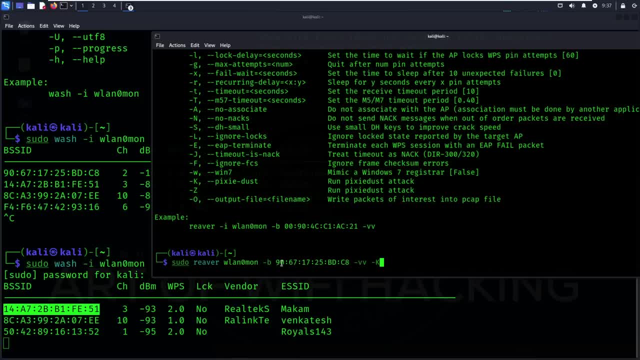 what is that, which is this one? right now in my network there is no wps enabled, but still i am doing it. sorry, see again, i need- i just forget it- to add the dashi here. this is a thing: if you forget to add the things, then it won't work. 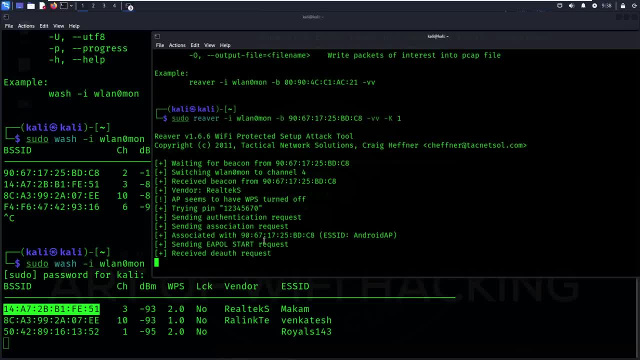 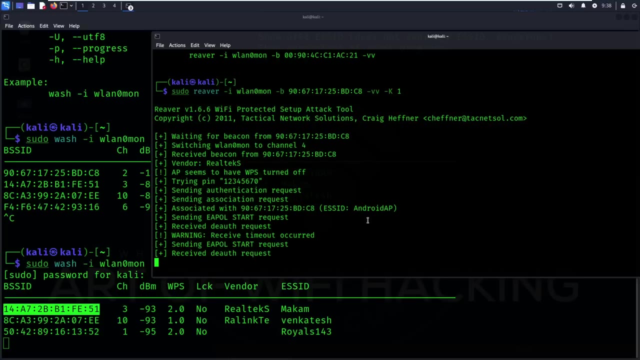 no, it will start the attack. okay, it will take some time, not sometime, it will. like we just learned right, it will take my might be hours. we uh, sometimes this things are hours, minutes, minutes, light, week and day, blah, blah, blah, but i don't die. weeks sometimes as well, not weeks. hours, okay, sometimes minutes, sometimes seconds as well. 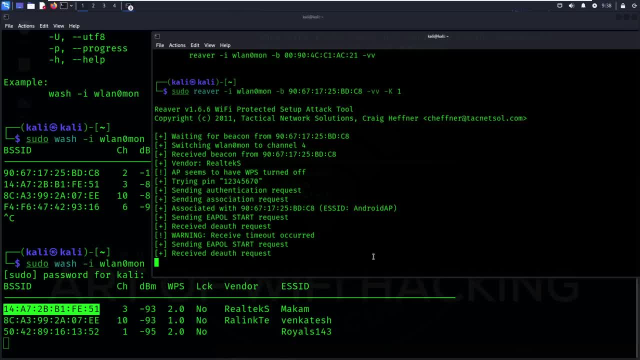 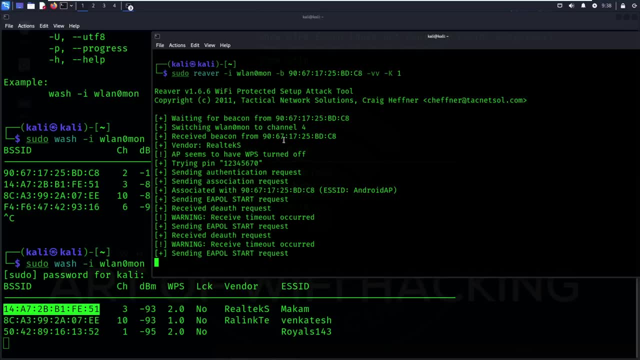 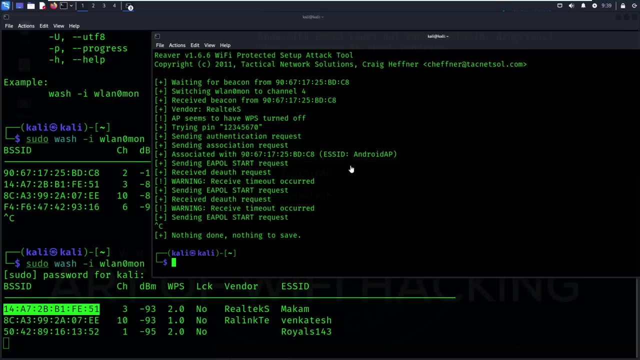 so this is a thing. see, let me tell you, the wps is not enabled in my network, so that's why let me stop it. okay, now here you need to remember something here. the thing is you must be close to your target network. if you are very far, then the attack won't work. this is a thing. 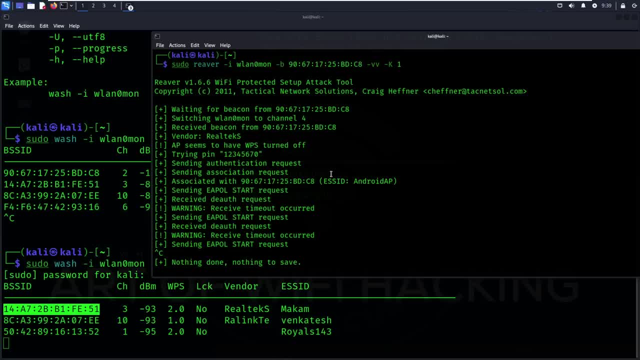 okay, the wps attack. if you want to perform the wps attack, or by using reaver or wi-fi t or wps enabled network, at that time what you need to do is you need to go close to that network. okay, this is a thing. if you are very far from the from it, then you can't able to do it, okay. 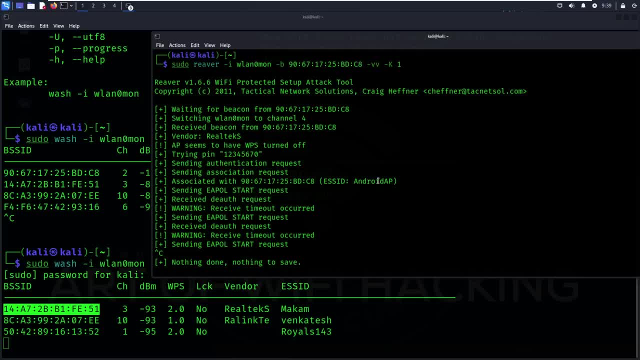 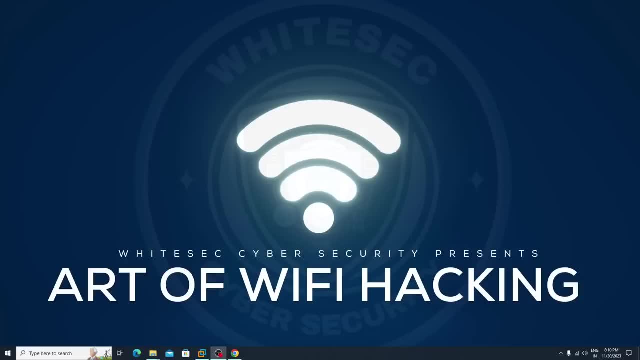 even it's vulnerable. sometimes even it's vulnerable, still you can't able to do it. so this is a thing in the last class i just told you. right, sometimes the reaver won't work, okay, okay at that time, if you are not getting any results from reaver at that time, just go with. 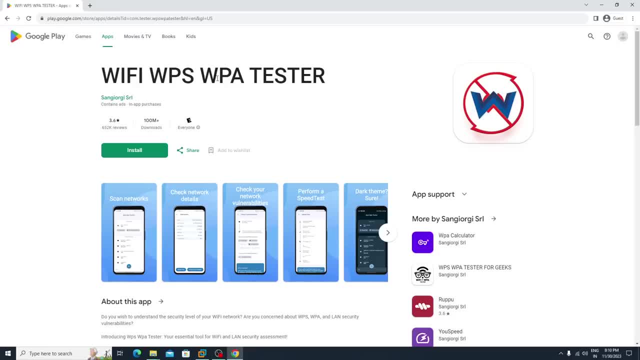 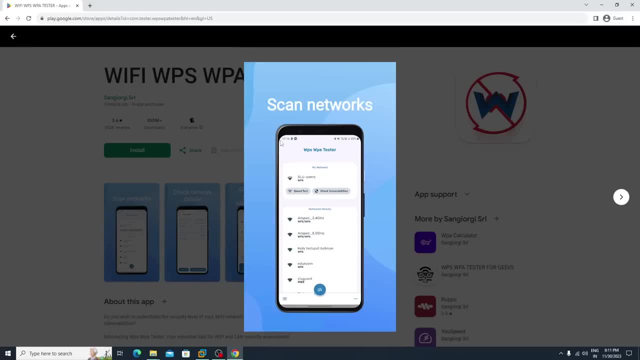 wi-fi wps wpa tester. it's very excellent. guys, if there is any kind of wps enable network. first, just try to perform pen testing using this application. okay, see, it's a. right now. it's a very updated. they are just added a lot of features in it, okay. 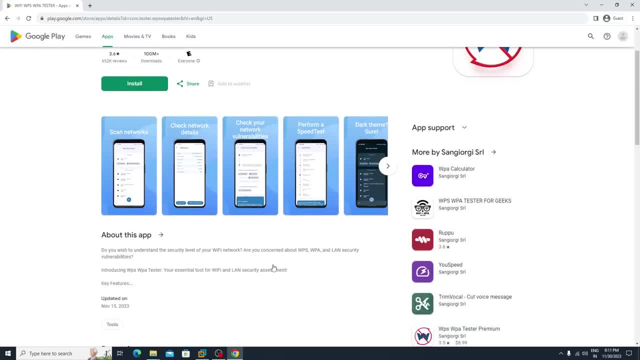 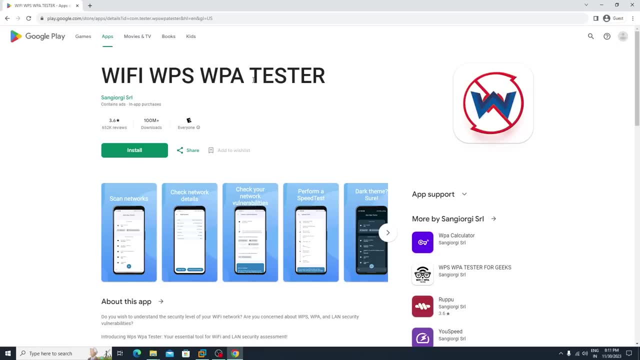 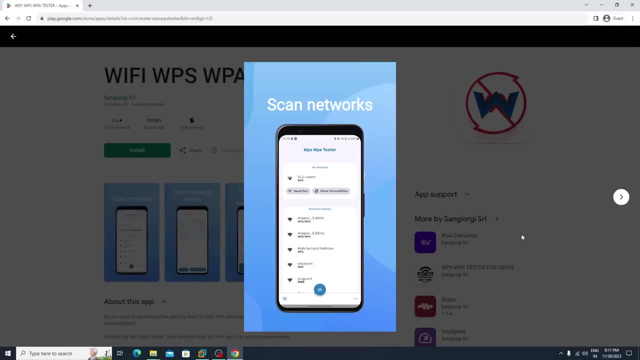 so just try to use this, uh, wi-fi, wps, wpa tester. if any network is enabled, it's a see to you. uh, if wps is enabled, see, it's not a big deal to use it. okay, it's very easy. it's a complete automation thing. okay, simple. you need to select the network, simply. first of all, you need 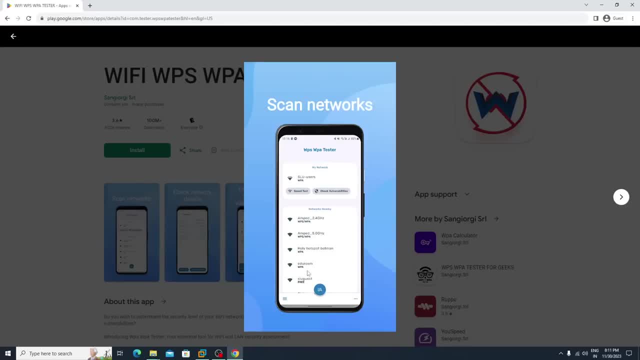 to scan it. after scanning it, you need to select your target network. from there you need to choose attack. see, there is a mostly go with this one, okay, which is: try all pins, simple, just leave it. it will try to crack it. okay, this is the thing. you can also add the custom pins. if you want to add your own pins there, you can also add it. 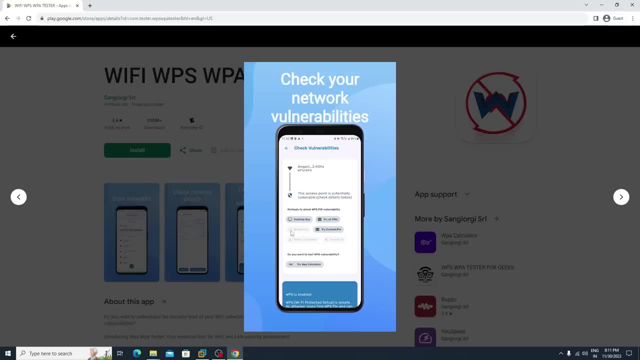 okay, there is a brute force is also. is there? see here, brute force. i just covered in the last classes. what is a brute force attack? simple, you can also use it. see, mostly the brute force attack will work. this is the thing. now pixie dust is also there here you no need to type any command, simple you. 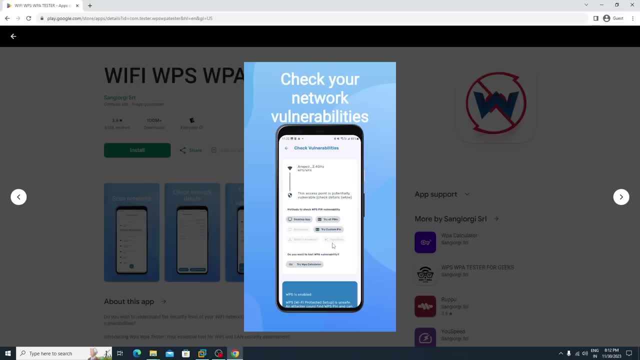 just need to select the options there and you need to perform the attack. this is the thing now. uh, from here you can able to see the things. okay, speed test it, say it's not in that much. okay, it's also having the dark theme. now the thing is: uh, maybe it's a premium in premium. 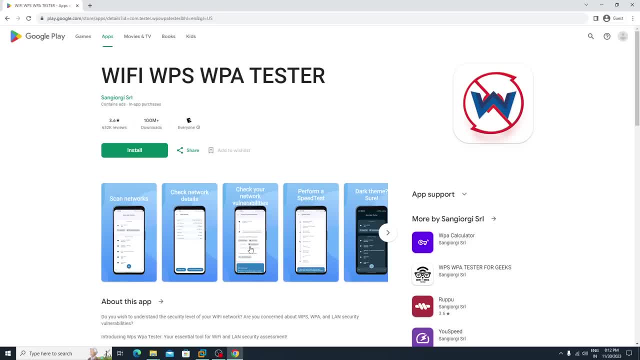 one. you will see these features, such as brute force, uh, or this pixie dust features. well at the time. what you need to do just search for the modes. okay, something like that. then you can go with it. so hope you guys enjoy this class. thank you, have a. 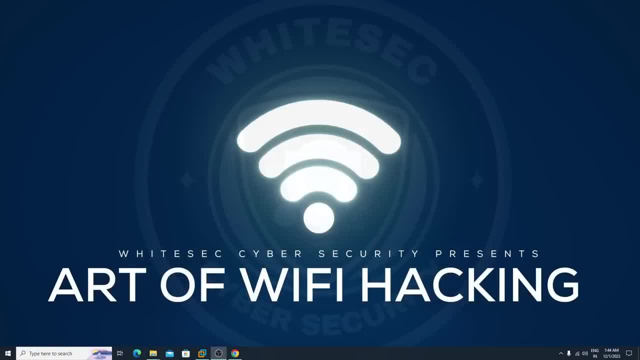 nice day. in this class we are learning how we can able to perform the authentication attack. see, in a simple words, the authentication attack is a nothing, but it's also kind of jamming. now assume that here. let me explain you. there is a wi-fi network, okay. 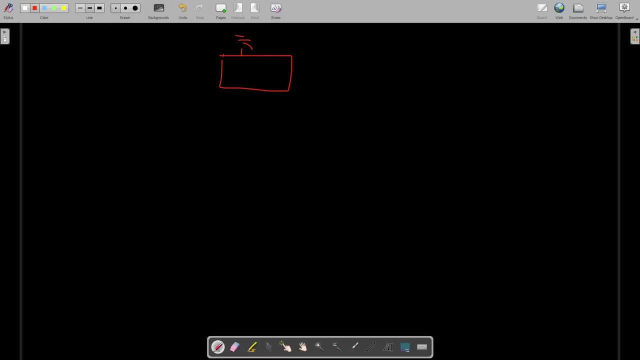 now there are the devices which are connected with this network. now, simple, as a hacker, as an attacker, what i do means i'm going to perform the deauthentication attack. for to perform this deauthentication attack, you no need to connect with this network or something like that. simply, you can able to perform deauthentication on any wi-fi network. this 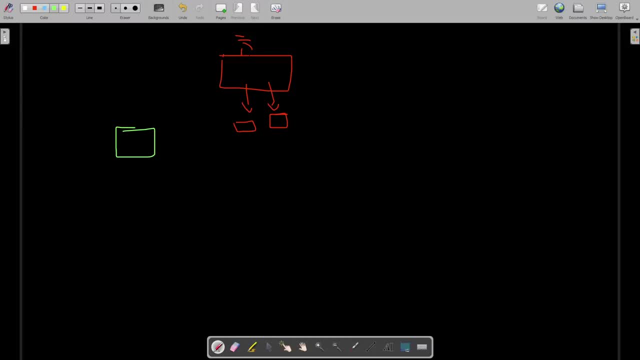 is the thing, okay, without connecting with that wi-fi network. okay, this is the thing now. here, what will happen means: if i send the deauthentication attack, then what will happen means here: assume that i just perform the deauthentication attack, then these devices, okay, which are connected with this wi-fi network will get disconnected. okay, 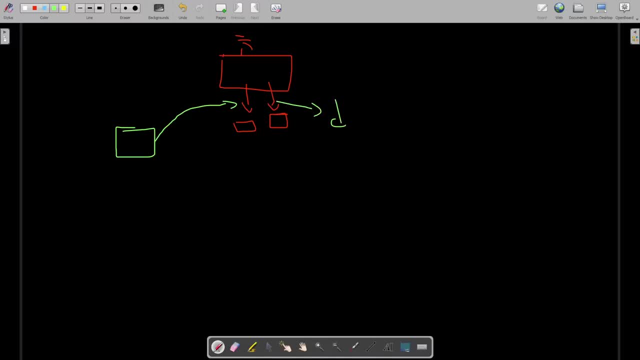 you'll get what disconnected. so it's a kind of jamming. now this is a first advantage. advantage to capture the handshake. okay, see, in wi-fi network there is one feature. just open your android device and simple go to the wi-fi option. okay, now simple run, hop that one, just turn off your wi-fi network. 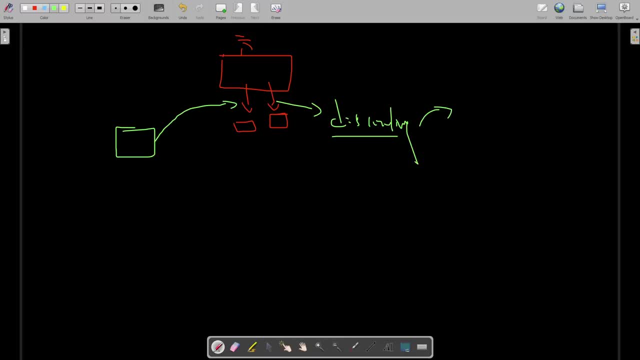 then turn it on again, then what will happen? automatically the wi-fi will connect with your network, your home network or your office network or something like that. this is a thing once see. after performing the deauthentication attack, the clients who are connected with this network will get disconnected. okay, after disconnected, then what will happen means the hacker will. stop this deauthentication attack. okay. yeah, he gonna perform this deauthentication for 70 seconds, 80 seconds or something like that. it is very easy attack. okay, after stopping that attack, these guys will add this clients. okay, the devices will automatically connect with that wi-fi network during this process. okay, during the connection process: reconnect. 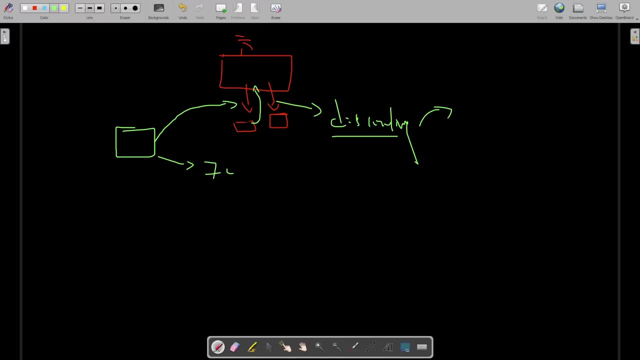 this process, reconnection, reconnecting process. at that time here what will happen means the attacker will steal the handshake. okay, which is the handshake which we just learned. this is a very simple explanation which i am saying. there is a four-way handshake, is there? uh, if you go for that, then maybe for beginners it is hard. 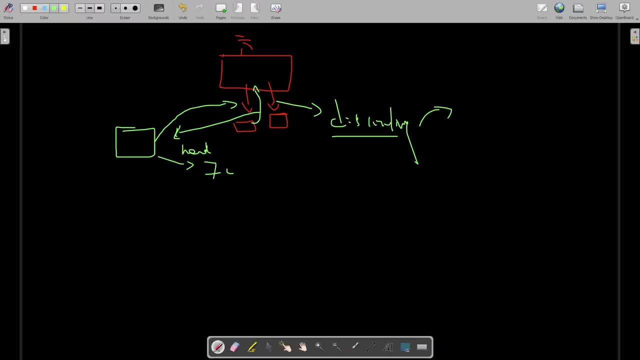 so that's why, in a very easy what i am saying these things now during this process: okay, we, the attacker, will capture the handshake. you no need to do that whole process simple. it's a complete automation process, uh, which is did by wi-fi te and also you can able to do it. 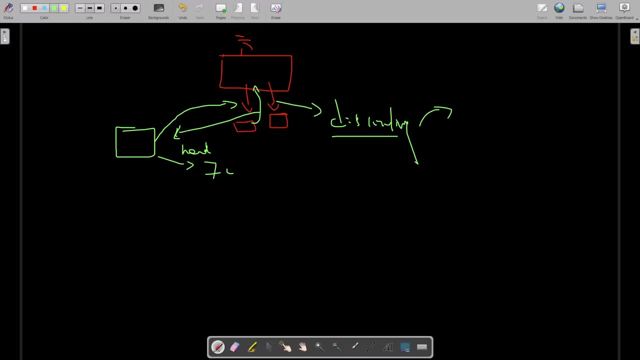 by using aerodrome or something like that. you will see this, all stuffs. and also the thing is here: if in that, in this wi-fi network, in this network is there is any kind of camera, okay, which is using the wi-fi, wi-fi for connectivity, at that time you can also join the cameras there. 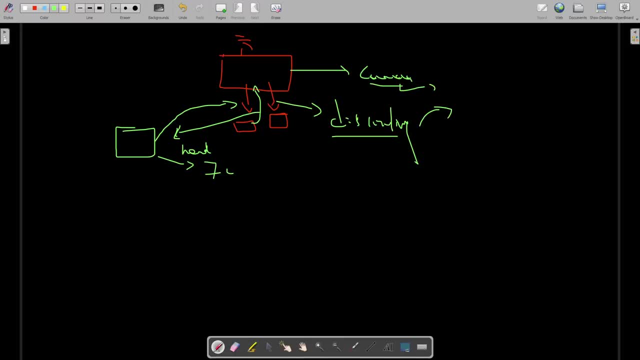 okay, this is the thing simple: see in camera, once you give the power. there are a lot of cameras out there. once you connect with uh, provide the power to it, it will give you one wi-fi. okay, the camera will generate one wi-fi network right now. to access that camera, you need to. 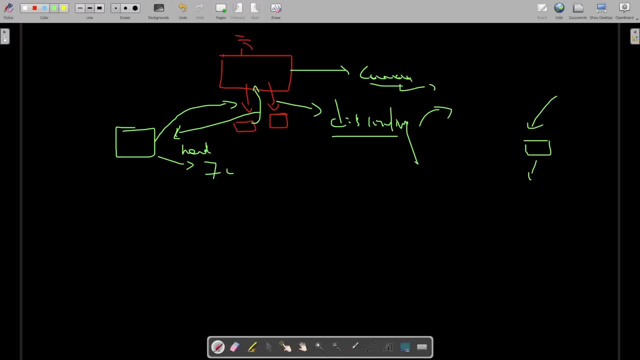 connect with that wi-fi network, then you need to go to the ip and you can able to see the camera there. this is also one kind of cameras right, so simple. the attacker, if the attacker send a de-authentication on that wi-fi network which is generated by camera. 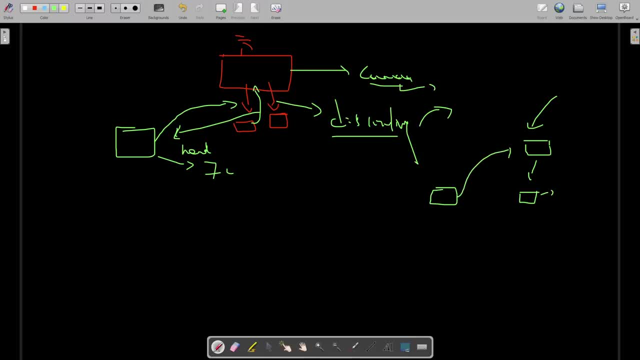 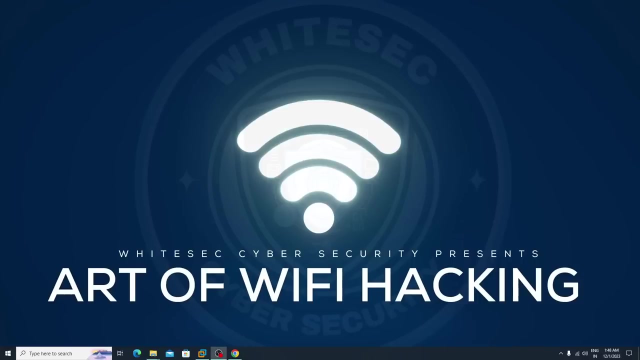 then what will happen? the guys- okay, they can't able to access that camera as well. okay, this is a thing. so wi-fi hacking is kind of easy thing, but you need to think a lot here now. in the next classes, we will learn how we can able to perform this jamming de-authentication. 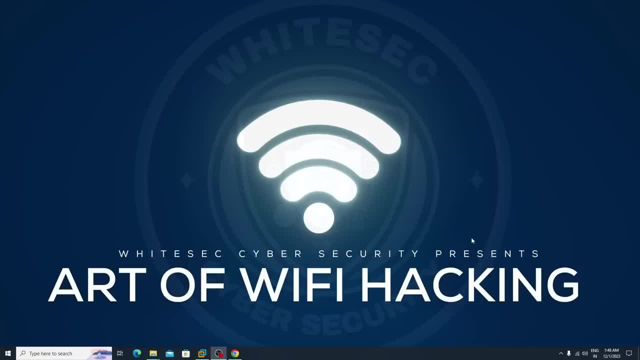 okay, right now, in this classes, we will learn how we can able to perform the authentication attack, how we can able to capture the handshake. okay, this all stops. it's a very easy class. now the thing is here you can able to perform the same thing by using wi-fi. okay, 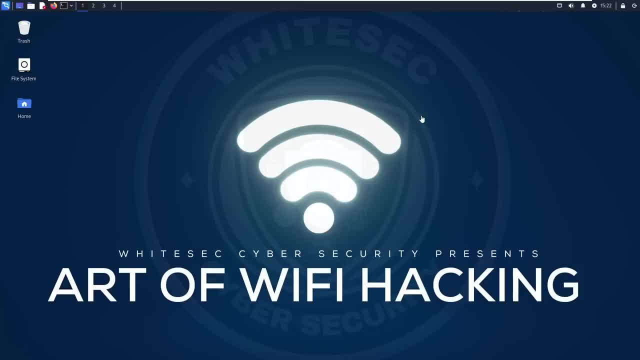 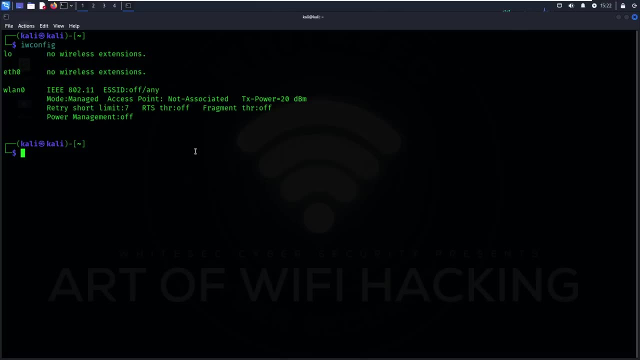 but here we are learning some kind of manual things. you need to execute some commands here. okay, now how to perform this attack. first of all, the thing is you need to change your adapter mode to monitor. now let's see. uh, just type iw config here you can able to see right now my monitor, my 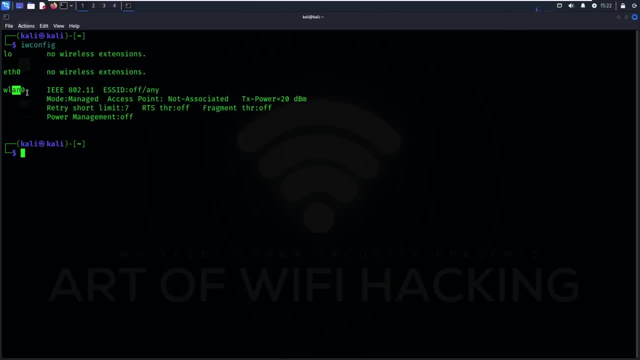 adapter is in management. now let's change it to monitor mode. to change to monitor mode what i need to do. i just told you- sorry, earmon-ng, start w launch zero your interface name right now. this is: my adapter is in monitor mode. okay, now then what you need to do. you need to scan for the wi-fi. 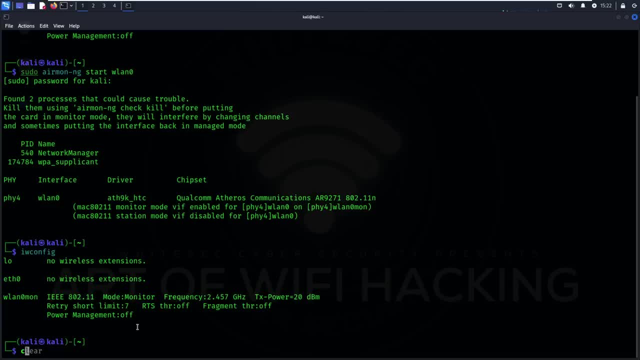 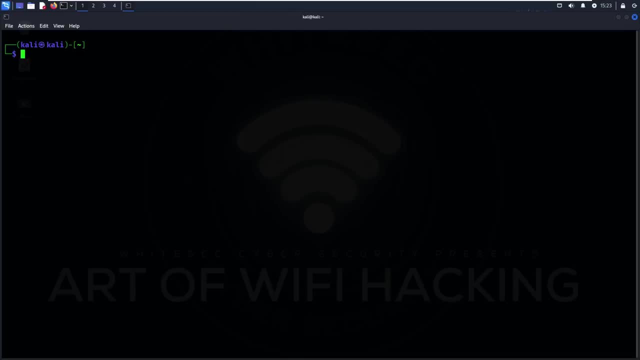 networks. you can also use wash or some other tools to scan the wi-fi network, but let me use mta control. so let me go back to my computer. arrow dump: okay, simple, just type sudo arrow dump. sorry guys, dash ng and just execute your. sorry. just type your interface name. okay, wlan0mon. 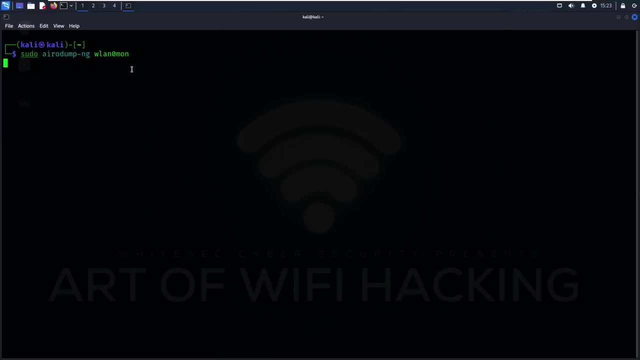 just type enter there and here i can able to see my target network, okay, which is test network, simple. let me stop it now from. by this you can able to scan, scan the wi-fi network and also you can able to see here in this section the clients who are connected with that networks. okay, 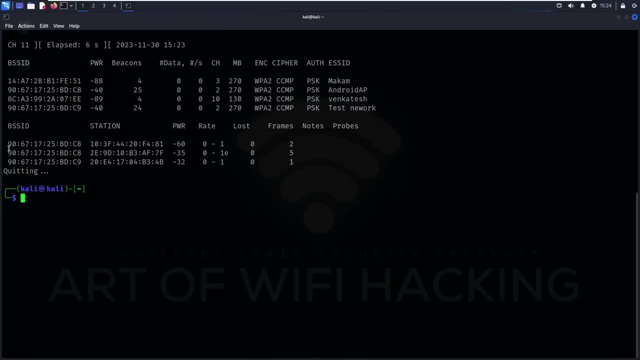 now here. just see, bss id is c8. now in android, this or the, this is a one client which are connected with android ap. just see the same bss id. see you, now there is c9. is there here? just focus: c9. now the test network. bss id is c9. basically, this is. 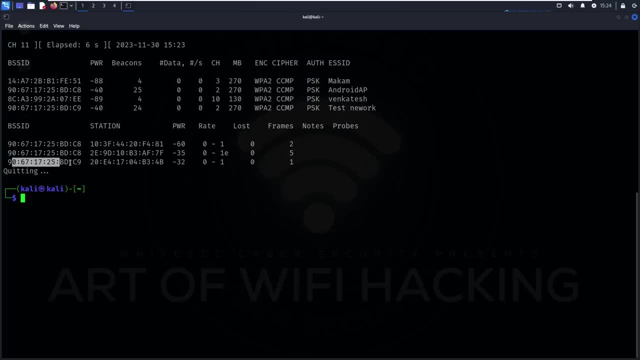 a client which are connected with this network. okay, with test network. okay, this is a station of that client. okay it. it is a help. the stations are very helpful. once you are jamming the one specific client. okay, let me show you that one as well. don't worry. now, here, let's start the. 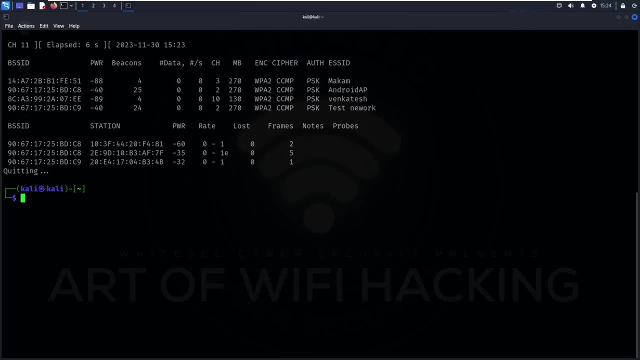 attack. now i want to perform attack on test network. what you need to type here? just type sudo er Kiev ruth mix. just type sudo erした hng. that's see what is our channel. see this one. i am talking about ch. is there right? it's known as a. 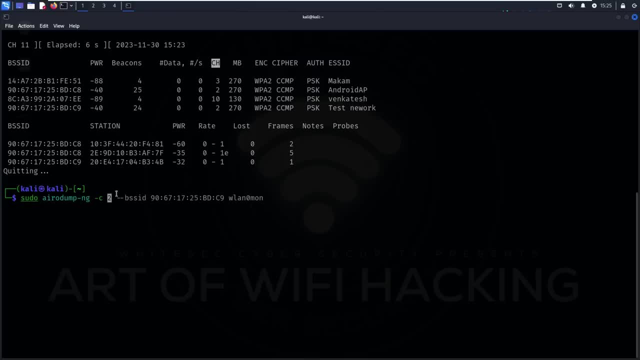 channel. you need to type here: dash c for a chanl. what is my target channel? target channel is to c. every network have, uh, some different channel? okay, this is a thing for venkatesh. there is 10 for android, ap2, macam, 3, something like that. you need to specify the channel, then you just need to type dash, dash bss. 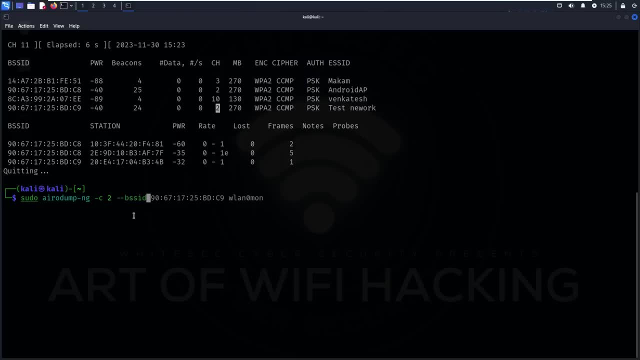 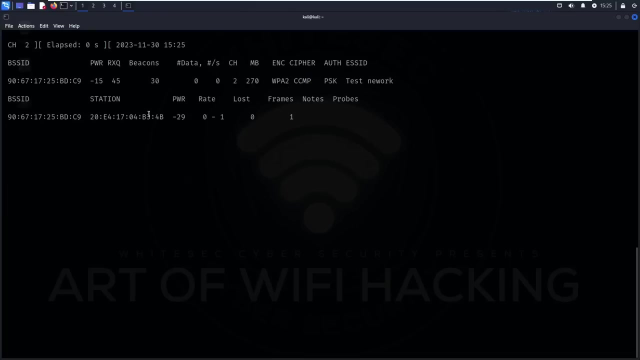 id. then just provide your target bss id here. this is my target network and this my target bss id is this one. okay, simple, just paste it here. then just type wlan, zero, moon your wi-fi adapter interface. then just execute it. now it will target on this one. now we. we just started the attack on. 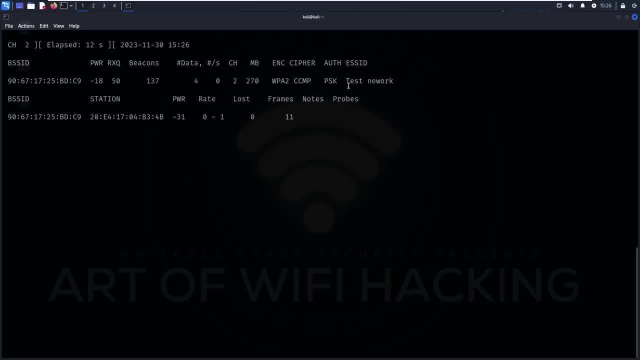 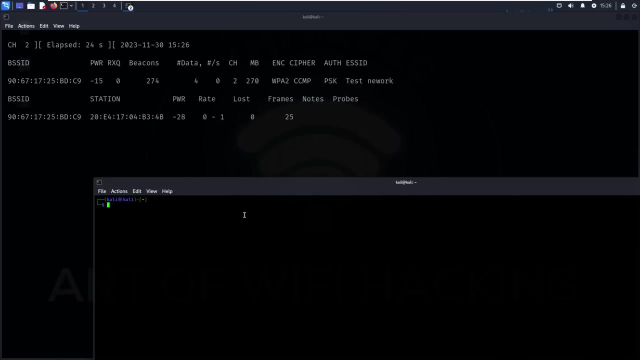 test network. okay, now we need to capture the handshake. how to capture the handshake? simple: you need to start the deauthentication attack here. to start deauthentication attack, what you need to do? simple: just open any other other terminal and then just type you pseudo: a replay, dash ng. now just add a flag of dash. that dr. 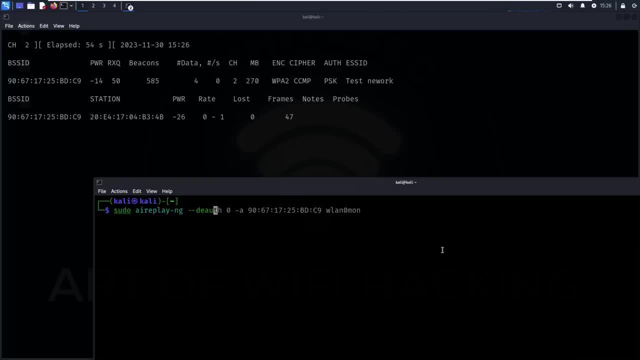 okay, and then see: here you can add 70 or 80 or something like that. now what happening is, if i add the 70, then it will perform the deauthentication attack for 70 seconds. this is a thing. then just type here: dash a. in the dash a you need to add your target bss id here. okay, in my case the target bss id. 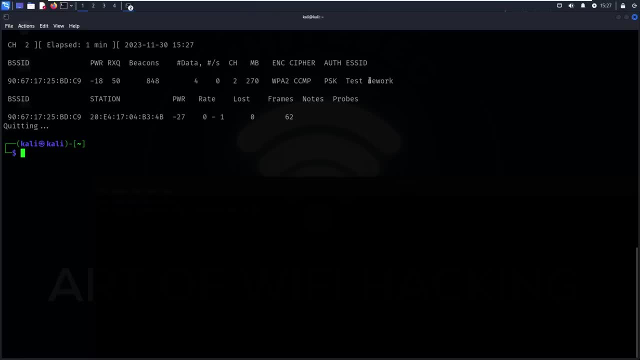 is bss. in my case, my target is test network. okay, the test network bss id is this one. simple copy this bss id here. then simple paste it here. okay, see, you need to don't stop this one, because once it started, i can't able to copy it, so that's why i just stopped this one. 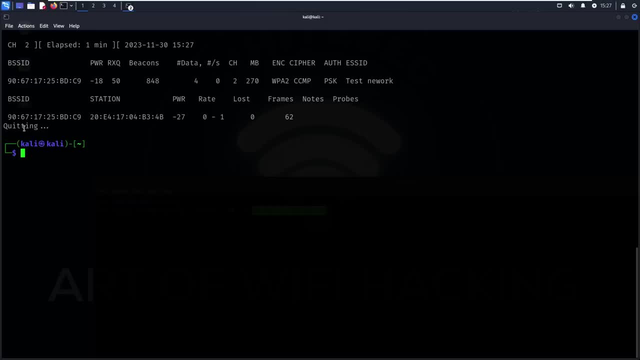 by just typing ctrl c: okay, before executing this command. okay, before executing this command, you need to run this one. okay, if you? if you are not running this one, then at that time you can't able to capture the handshake. this is the thing, simple, you are performing. 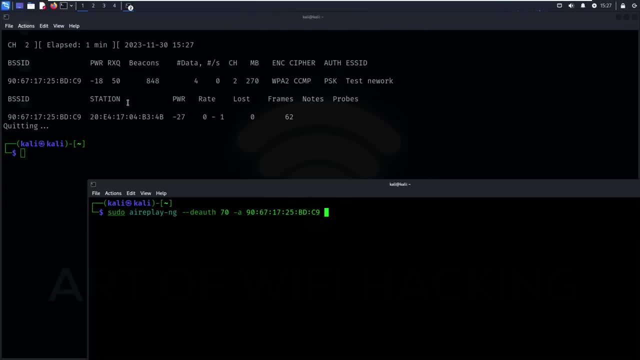 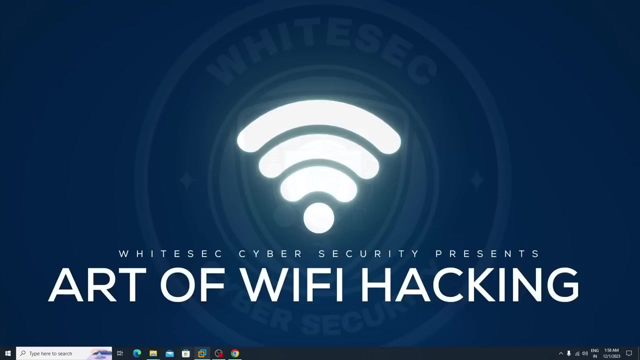 the deauthentication attack you are connecting. you are performing that like jamming attack there on this machine. okay, just see what will happen now. see, right now, this system, my computer system, is connected with a test network, right, okay, okay, once I start the attack here, let me target this machine. okay, like the station I just told. 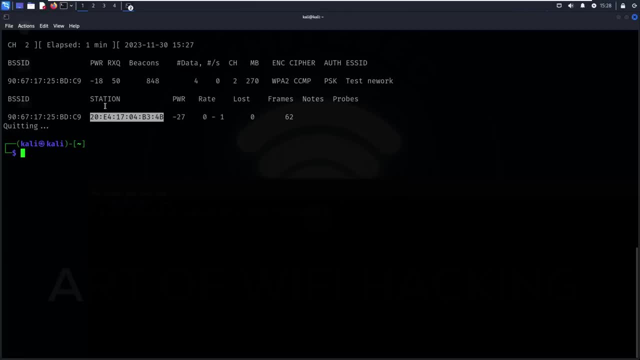 you station is nothing but the client who are connected with the, with your target network. okay, so simple. what you are doing means you are selecting one of the client. okay, in assumed in your system, sorry, in your target wi-fi network, there are hundreds of clients out there. 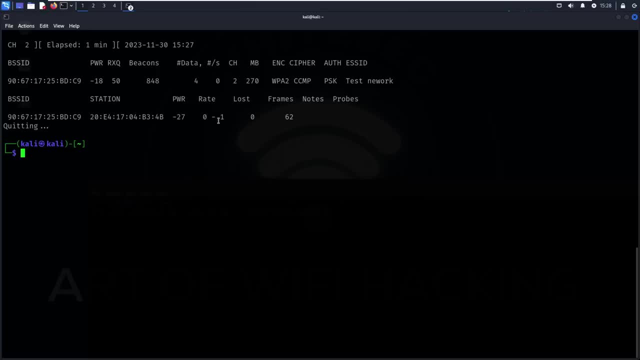 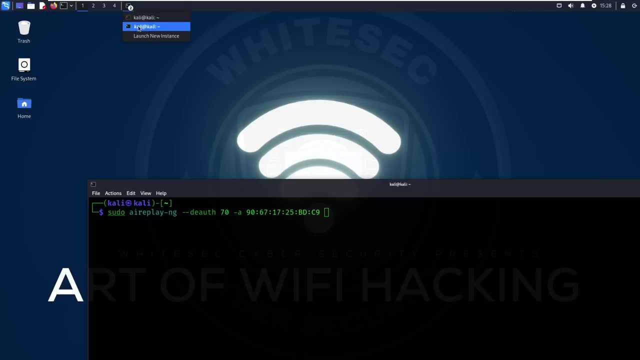 simple. you can able to select any client from that network and you can able to perform the deauthentication on attack on one specific client as well. if you don't want to perform deauthentication on specific client, you can also perform. just wait, man, just first of all let me show you, then I'm going to explain you these things. 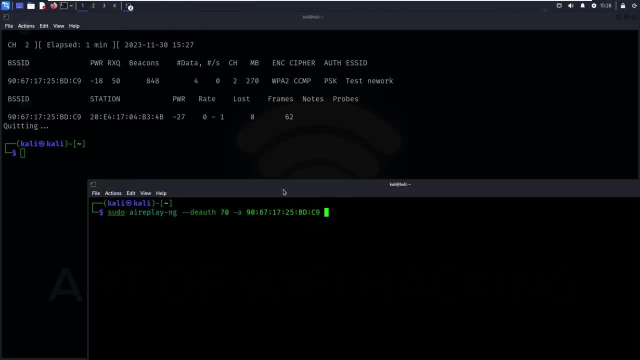 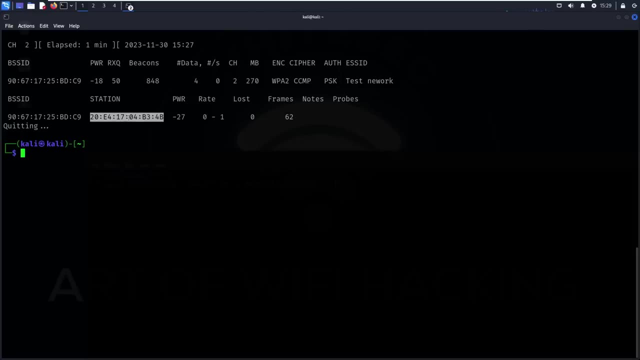 see here. just add: see, I'm going to perform the deauthentication attack right, check, check on this system, on this client. simple, just type c there, then add your interface name: wlan01. before executing this command, just execute this. then execute this one. now see what will happen. right now i can able to use a internet, right. 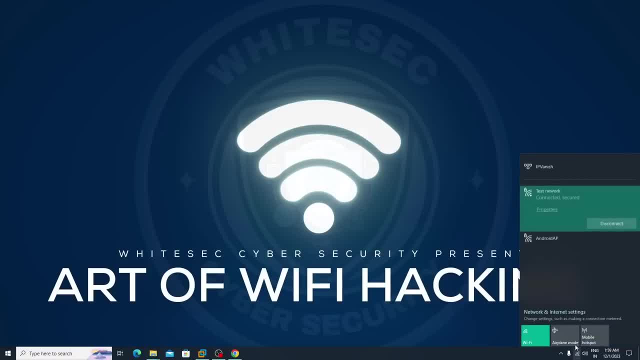 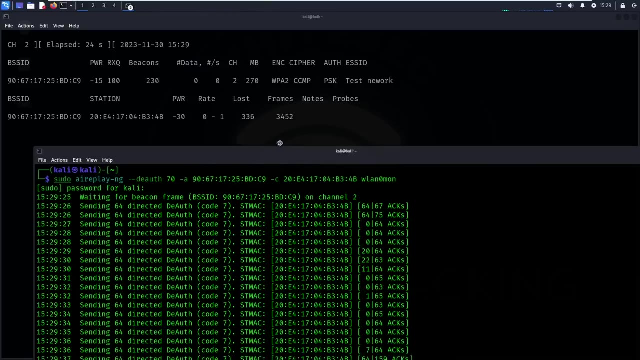 just see, now my internet will be disconnected from here. just wait, see, my internet has been disconnected for 70 seconds. until 70 seconds i can't able to connect with my internet. just see, if i click on connect, then i can't able to connect with that. 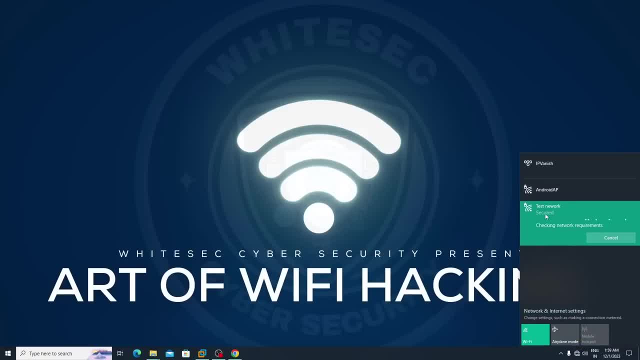 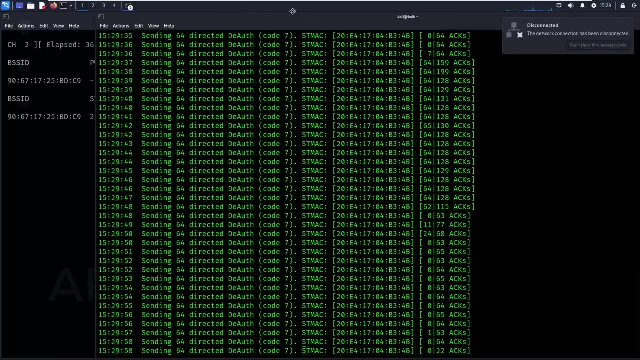 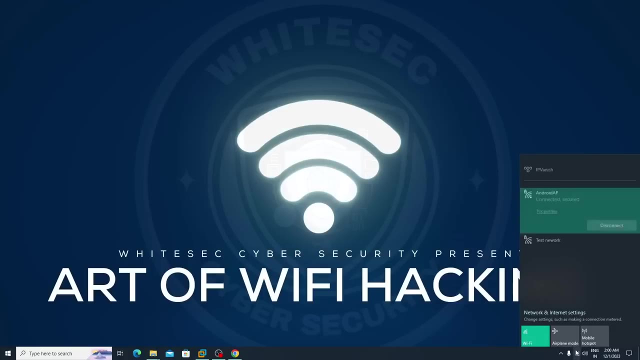 network, see, for 70 seconds. you can also stop it by just typing ctrl c. but let's see, okay, you can also stop it by just typing ctrl c. see, now i am connected with android ap, but still i can't able to connect with this network. so let me see now. 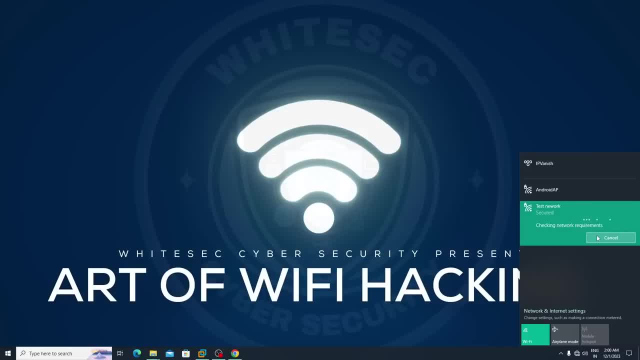 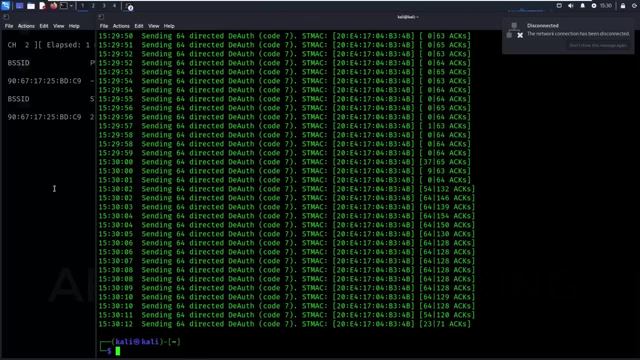 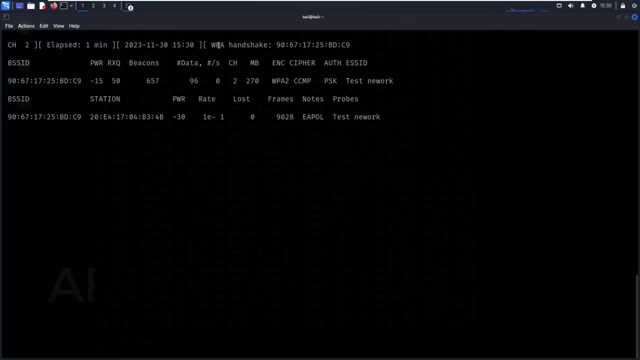 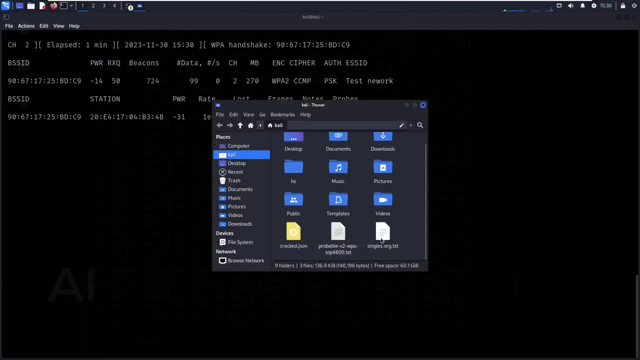 now. i connected because of 70 seconds i think completed. now see here we successfully capture the handshake. hope you guys can able to see now. you need to crack this handshake now. okay, where you can able to find this handshake simple, just open your file manager. here you can able to see it. okay, in hs folder, not in hs folder. 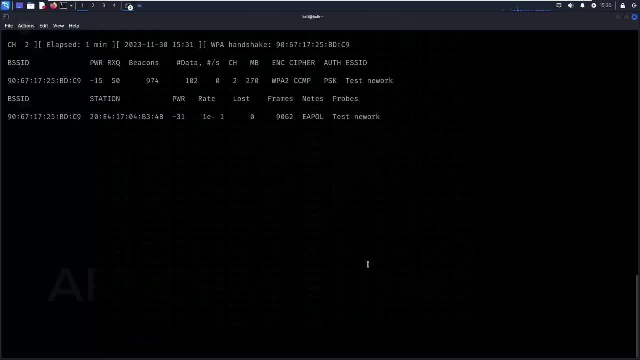 first of all, let me stop this one, because i got the handshake. i don't need any. i don't want to perform now, okay, this deauthentication attack or something like that. now the thing is, if you want to disconnect all clients at the same time, what you need to do. 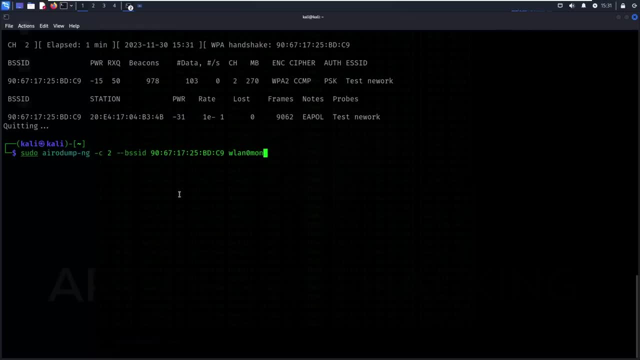 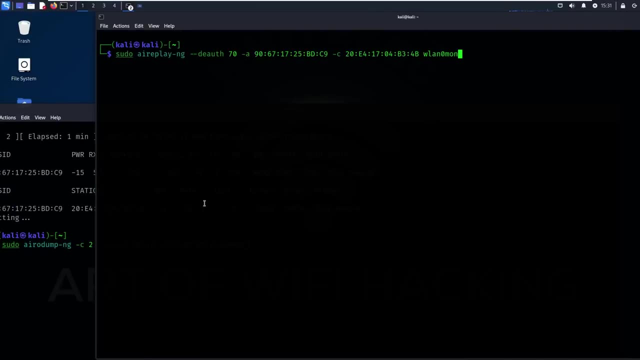 simple, just instead of adding. just let's go back here. let me clear it: instead of adding the client dash c here, simple, just remove this one. okay and simple, just execute like this. then what will happen means: if there is a hundreds of clients in your target network, they will get at the same time, they will get disconnected from that. 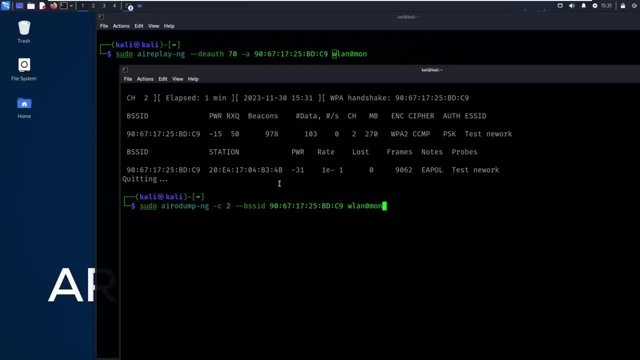 network. okay, this will happen, but in real world scenarios we won't do that thing. okay, you need to select one specific target. assume that if in one network there is a one camera, is there- okay, wireless camera. you can also select the that camera and you can able to jam that uh thing as. 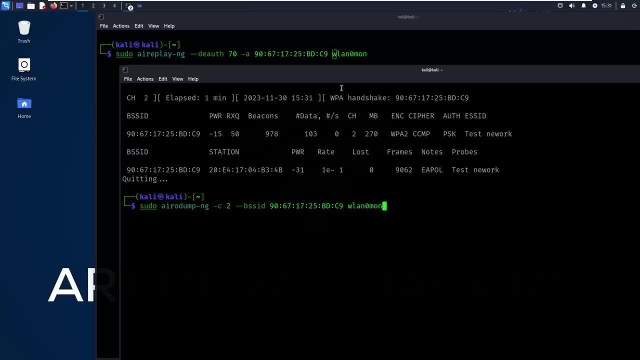 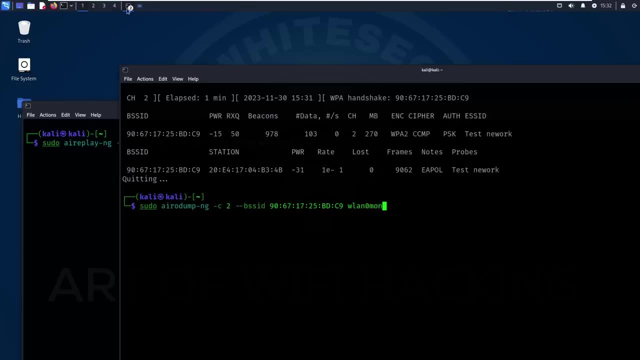 well, that camera. okay, it's not a big deal, it is very easy attack. hope you guys get it now. how to crack this handshake. simply, you guys can able to see the handshake file here only, but i don't know why, but i can't able to see it. okay, just wait. 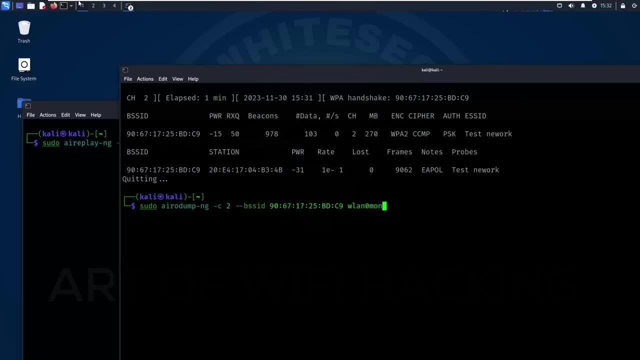 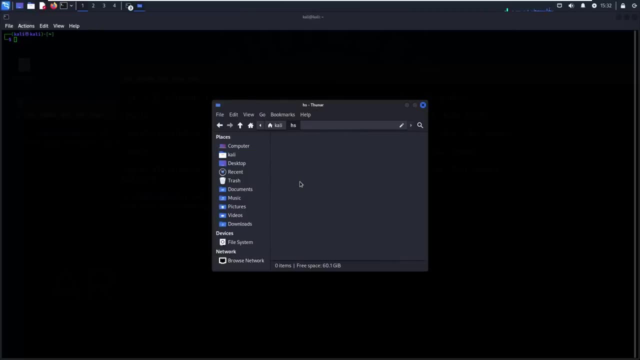 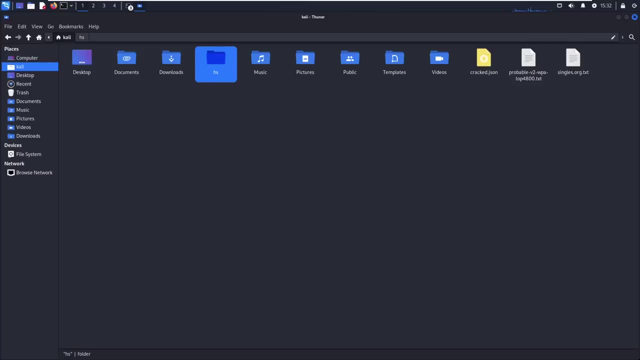 so you can able to see the handshake file in kali folder. but maybe due to some reasons i can't able to see it because i just deleted the previous one. so in the next classes we will learn how to crack it as well. sorry the thing, what you need to do means you just need to show this thing. okay, like just wait. 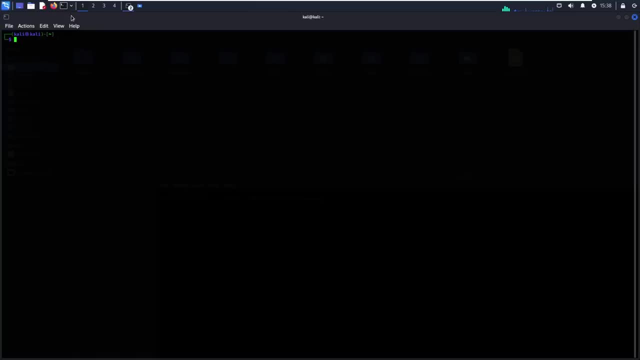 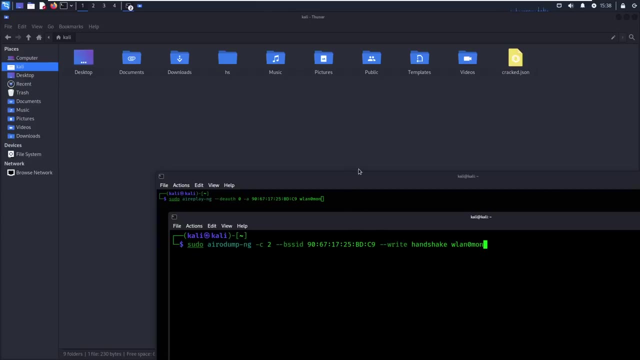 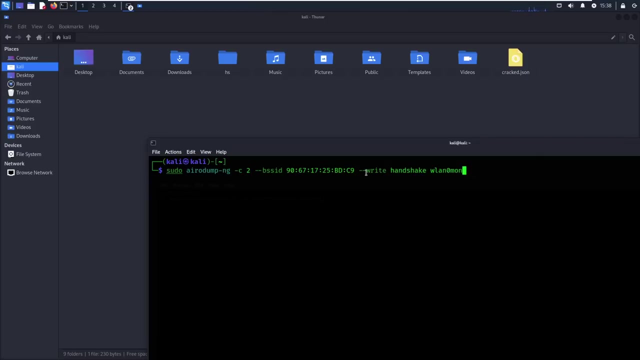 let me show you. see, after typing, you can able to see the handshake file in kali folder, but maybe, due to some reasons, i can't able to see ituren and provide any name. after capturing the handshake, it will save it with this name. okay, let me save this with the name of. 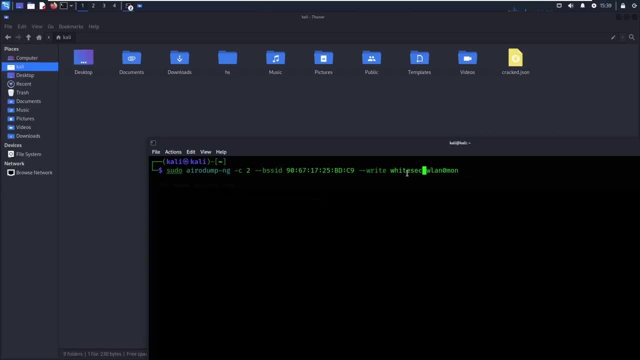 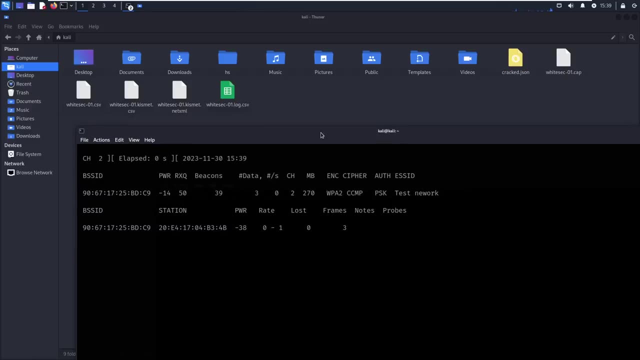 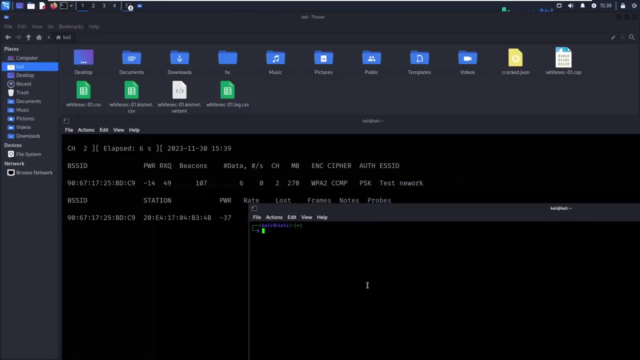 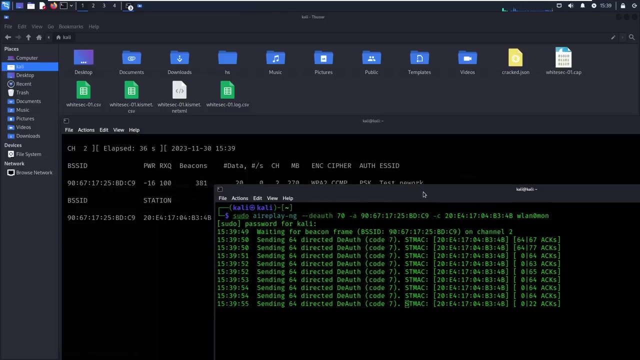 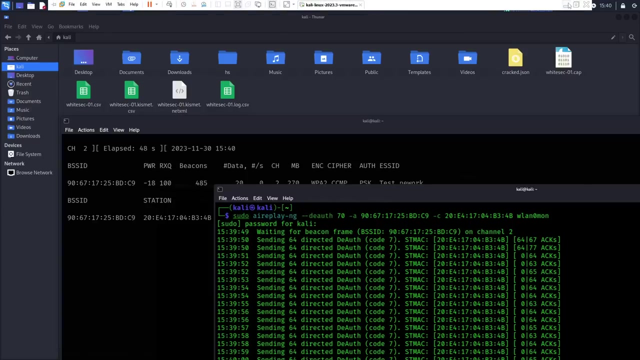 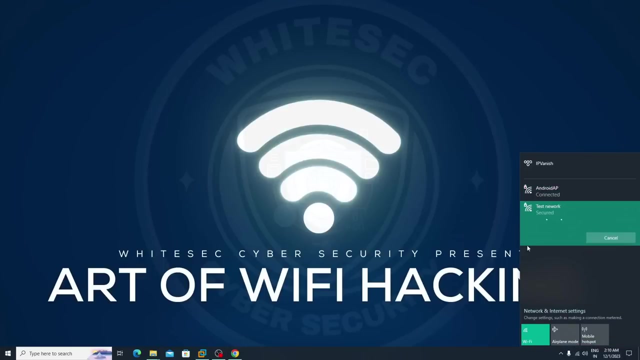 white sec. okay, just type enter now what will happen? it will. Now I need to perform the deauthentication attack which we did in the last classes. ok, So let's see what will happen. first of all, let's see: ok, it's connected with android ap, so that's why let's connect with this one. I'm doing this right now manually. 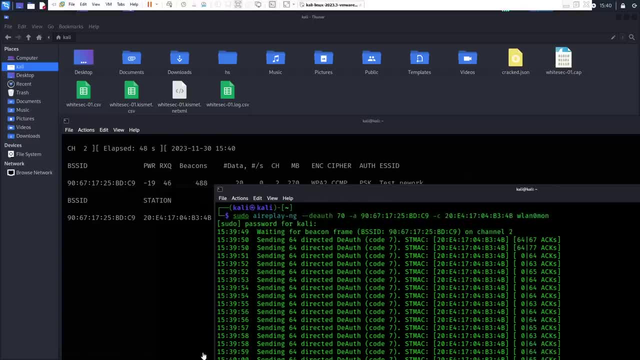 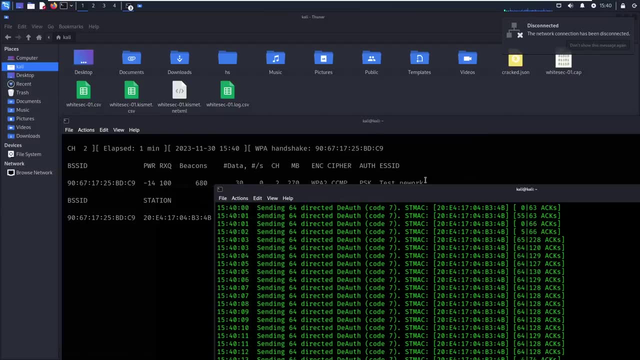 So, after doing this process, I can able to capture the handshake file. ok, where is? what is how to find the handshake file? simple, just see, the handshake file will be created with the extension of dat, dot cap. ok, this is your handshake file. this one, ok, with the same name which we just added there. 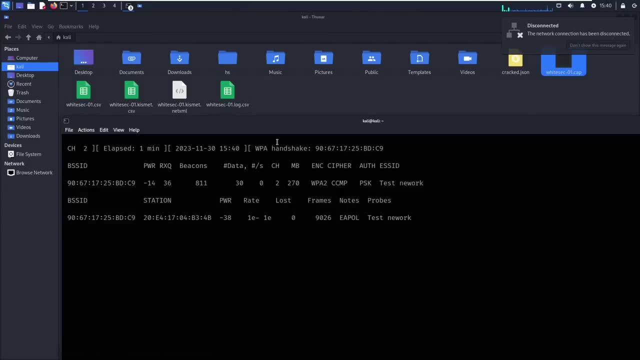 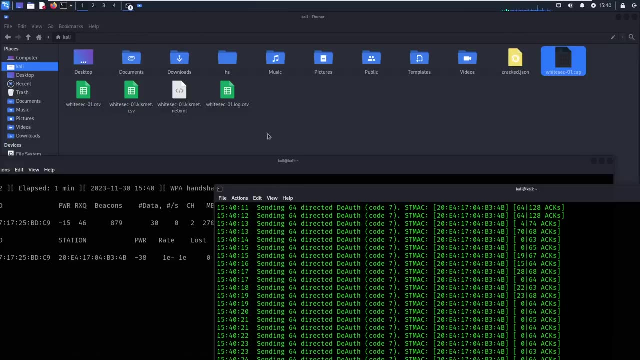 ok, like a white check or something like that. for simple, let's close this all steps because we got the handshake file. So if you won't add that right Right flag there, then what will happen? it won't save the handshake file. ok, this is a. 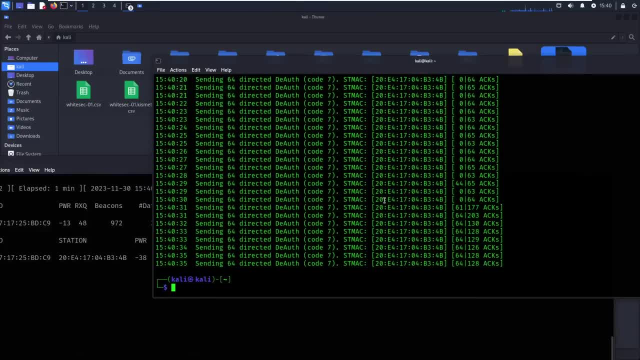 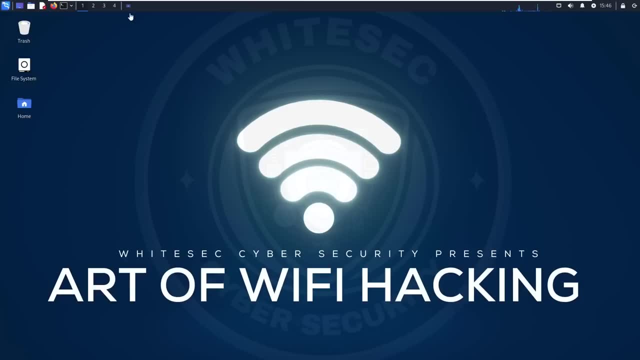 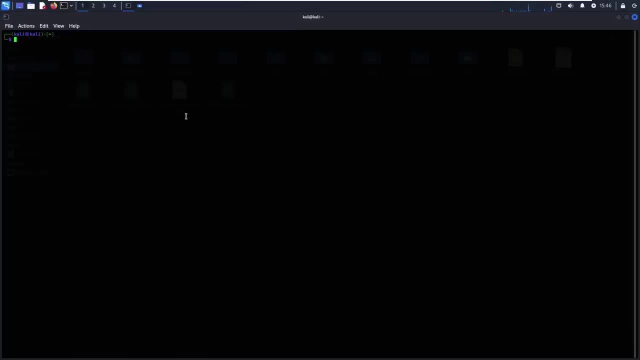 thing simple. let me close this: all steps in this class we will learn how we can able to crack this handshake file. ok, to crack it simple, we will use air crack wifi. de will perform this whole process in an automation way, but still manual process is also very important. 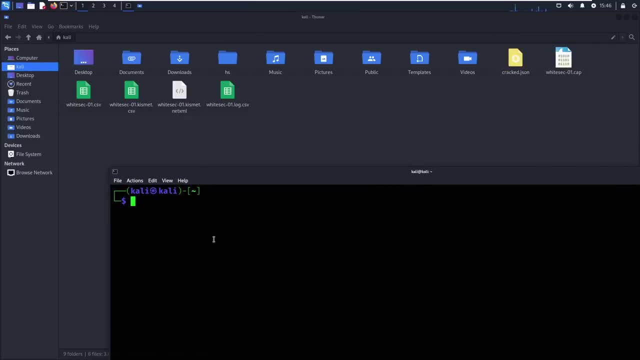 for you. Now the simple thing is just type: air crack dash ng. sorry, airy, not air. just execute as a sudo. sudo: air crack dash ng. just type here dash w. what is dash w here? dash w is a nothing, but it's a word list dictionary, ok, which we just downloaded from where. 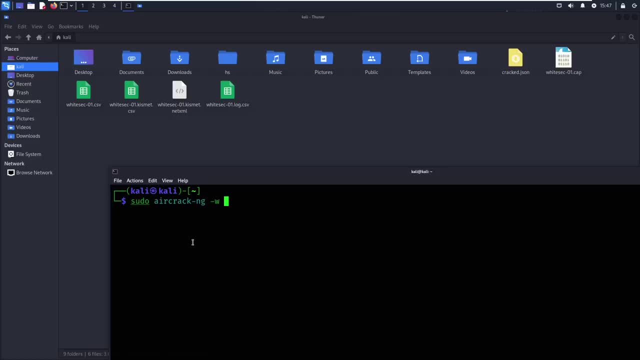 In the last classes. we just downloaded one dictionary right from second list simple those dictionaries you need to add here. the word list is simple. what you just need to add the word list here. ok, to add the word list simple. you can also download it from the internet or in kali linux machine by default there is a one word list if you click on user. 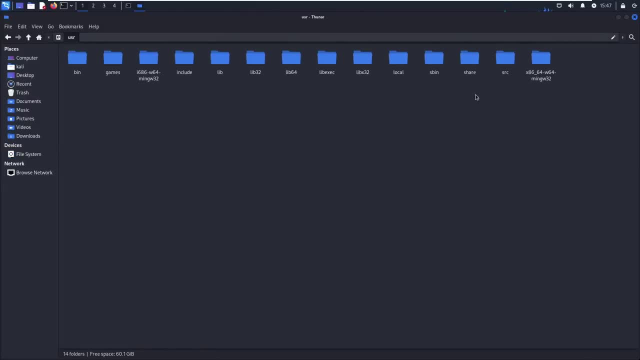 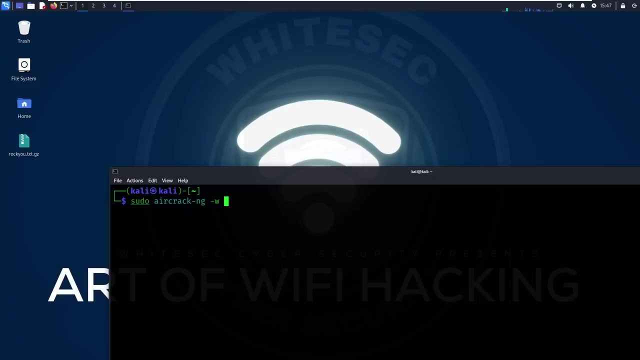 there is a share Here You can able to see. There is a A word list. ok, there is a raw queue dot txt. let me copy it. i just pasted that raw queue dot txt in my desktop. simple extract it. extract here. so here is a folder. ok, man, just just. 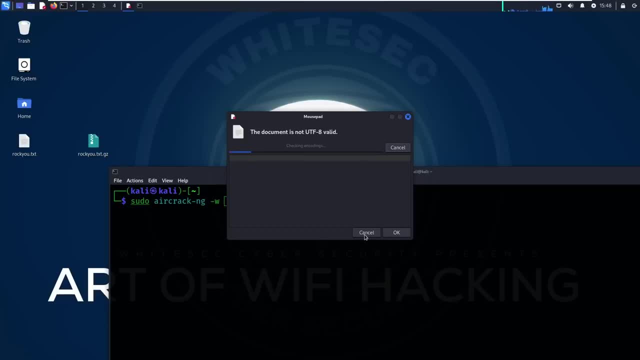 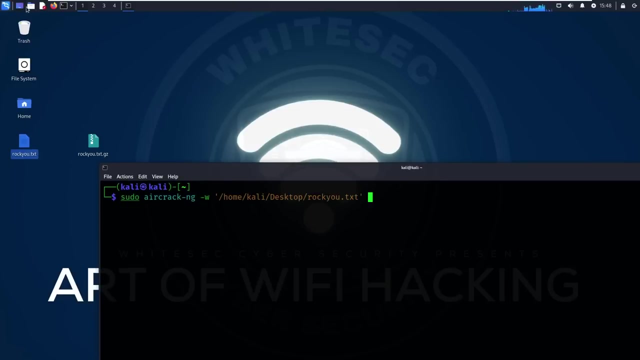 don't open it. ok, because it is around 139 mb, i think. so it will take some time to open this file, so that's why don't open it now. what you need to do simple: just drag and drop this word list here, then just go to your file manager in the last classes we just capture. 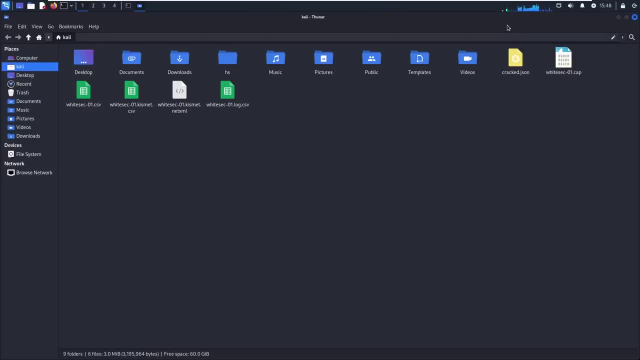 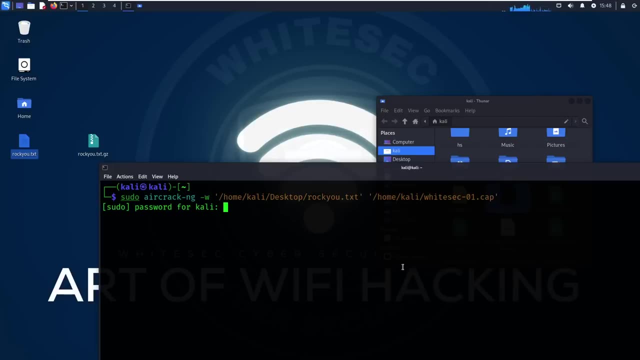 the handshake file. right, simple, just drag and drop this handshake file here. that's it. just type enter now no need to add any kind of interface, just type enter. it will start the cracking process. simple, just see, we got the key found. the key is one, two, three, four. 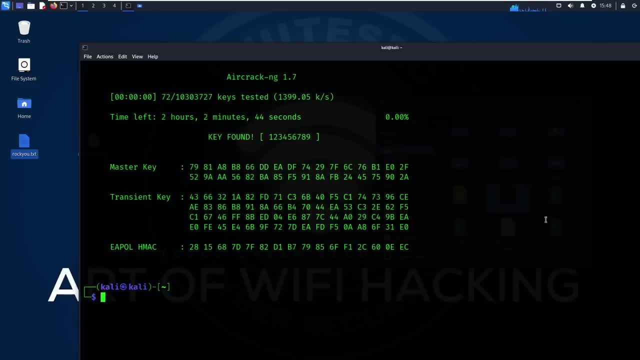 five, six, seven, eight, nine, Again. again, i am saying: in real world, the things are not this much simple. you can easily capture the handshake, but cracking this handshake file will take a time. ok, you can able to crack. it's not a big deal, but it will take a time, ok. so this is the thing which you need to. 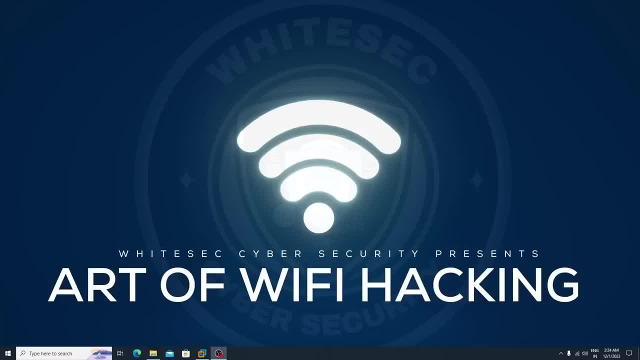 read. in this class we are learning how we can able to perform deauthentication attack using mdk3. basically, mdk3 is mostly we use this for the jamming purpose. ok, it's also same like This. I have this thing only areplay ng, but a mdk3 will generate a huge amount of noise there. 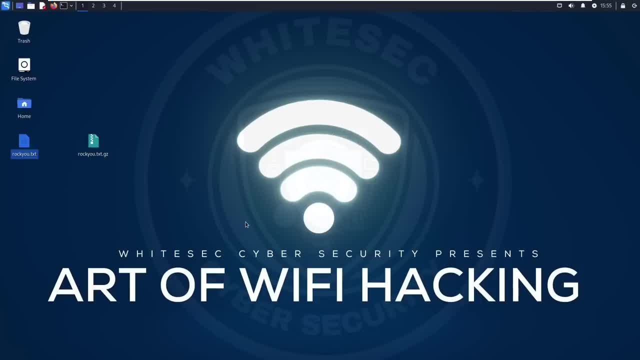 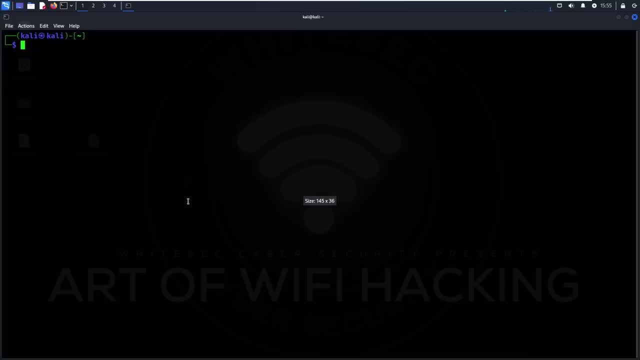 like it gonna effect on every channel. let me show you. first of all, let me open the terminal. just type sudo arodump-ng- wlan01. now the thing is right. now i have this much channels. now, sorry, the in my surrounding there is this wi-fi networks out there, okay. now the thing is. 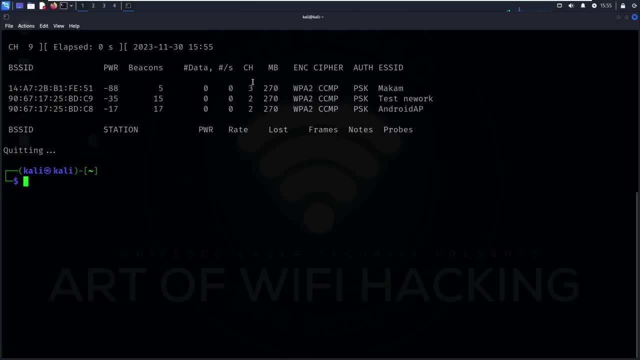 here, just see the channel. i just told you the channel. sometime the channel will be same. sometimes it might be different. now here, just just let me execute again. just wait. now here you can able to see the channels. right, there is a channel. two is there for test network: the channel is same, it's two. and android ap: the channel is same, two. 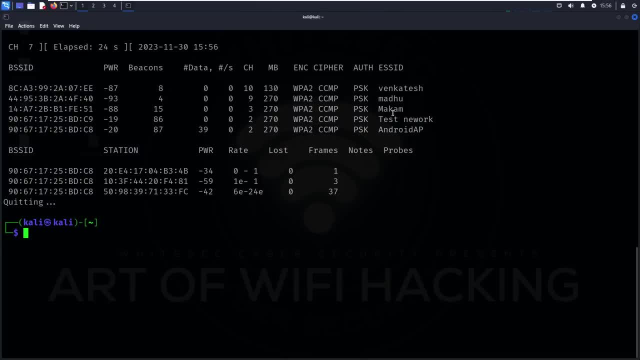 and for makam the channel is three and madhu the channel is nine and for venkatesh the channel is ten. here now, assumed that i am targeting the test network, the test network channel is two, okay, and assumed that, okay, i am just saying as for example purpose, okay. assumed that the madhu 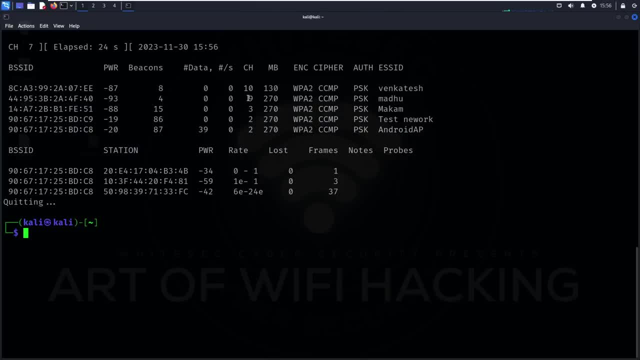 channel is also two. at that time, what will happen? this attack will affect on this thing. this thing will affect on this thing- and i am just saying as, for example, purpose, okay, on madhu network as well, and also in test network, which, which is our target, and also it will affect. 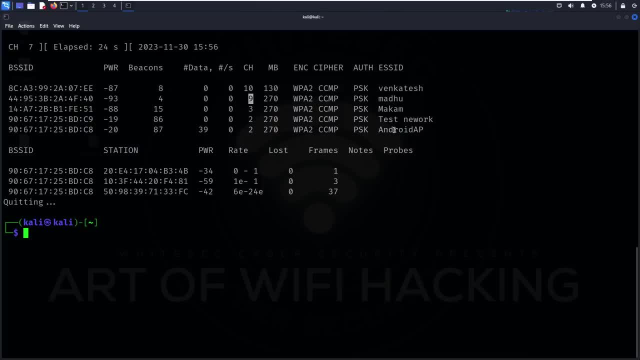 on android ap as well. this is the thing, okay. so how to use this? one simple just type here: mdk three. maybe mdk3 is there? no, it's not that simple. just install it, just type mdk3. or simple just type sudo apt. install mdk3. just type y there, or it will take some time. 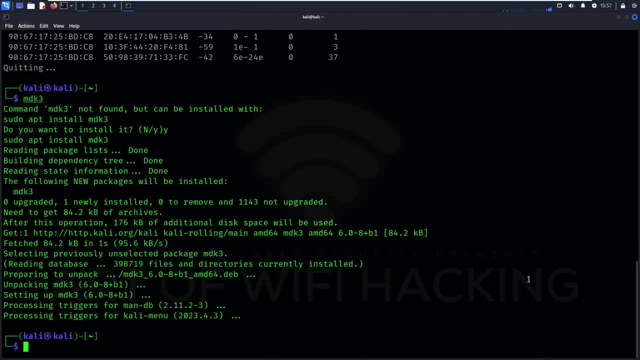 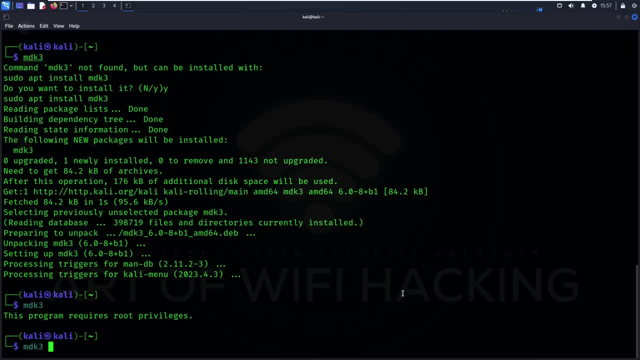 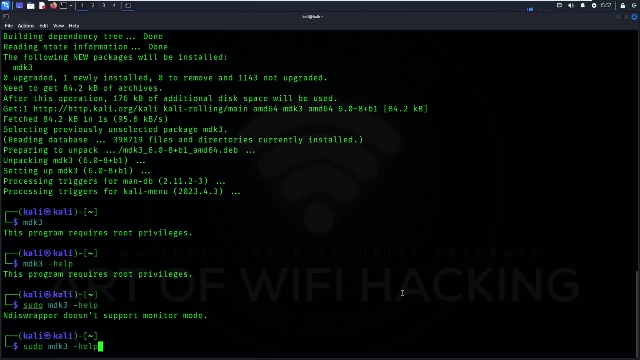 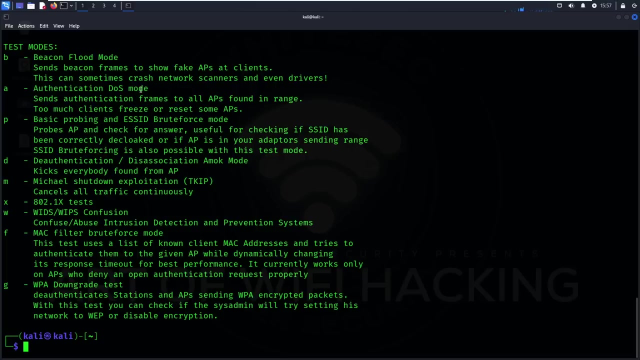 so here it is. see, running mdk3 is very easy. just first of all, just run mdk3. dash help. you just need to run it as a sudo. okay, here it is. you can also perform the beacon fold, authentication, dose attack, basic probing and essid brute force mode. there is a lot of stuff out there, but, simple, we are using the. 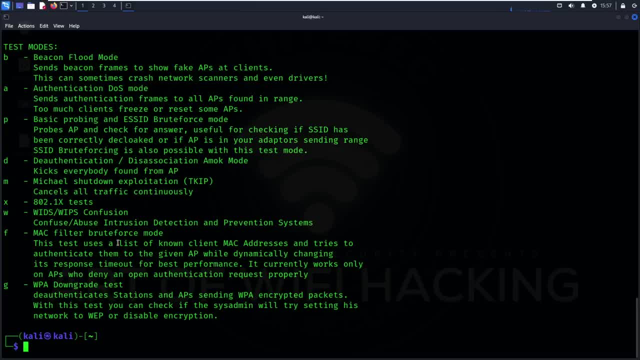 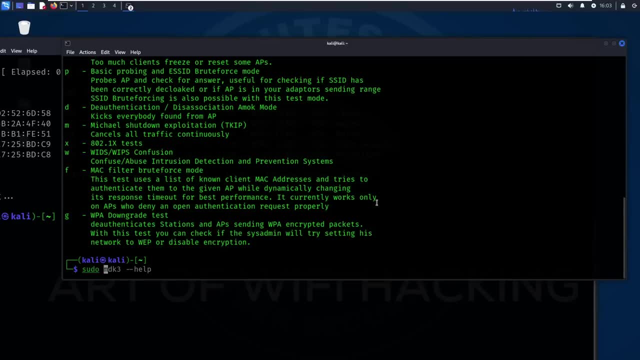 deauthentication attack here now simple. just type sudo mdk3. just type your interface name wlan0 moon. then here we are performing the deauthentication attack. just type d there, then dash c. you just need to add a channel here. what is a channel? your target? my target channel is two here again. 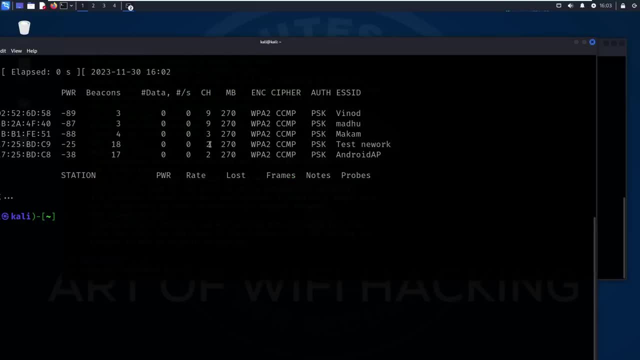 i am saying: you see, right now we know that madhu having the same channel, if i target madhu, the, we know the network will get affected as well. okay, madhu, network will also get affected. we know network also will get affected because the channel is same here. the mkd, mdk use this channel for the. 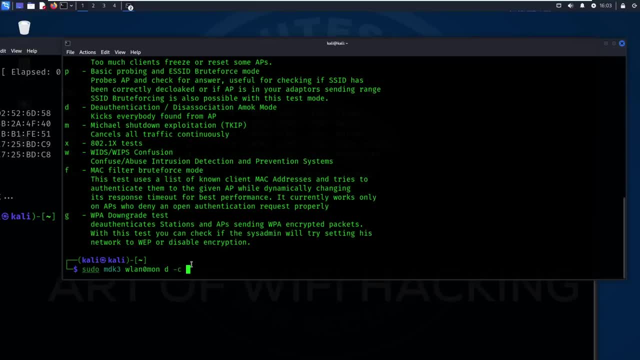 attack. okay, this is the thing i just told you. the channels will same. okay, sometimes the network- the your wifi, your or your target wifi network- the channels will same. so that's why this attack will generate a huge noise. a lot of clients will get disconnected. okay, so this? 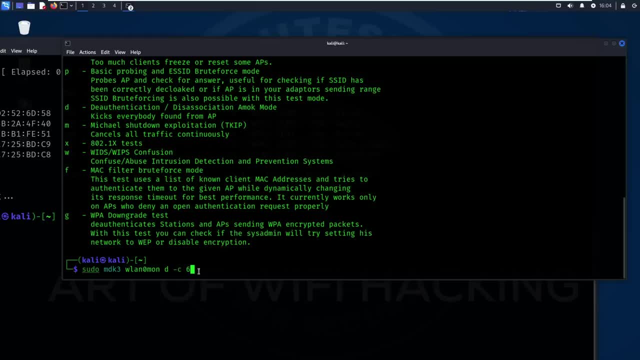 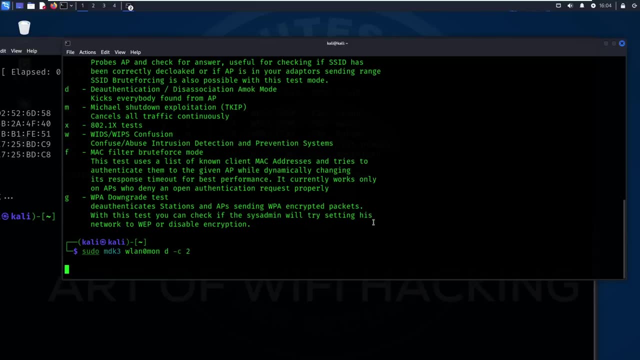 is the thing now simple? my target is what here? the channel 2, i think, just channel 2. let's type enter now it will perform the deauthentication attack. let me see, i can't even connect with this functioner when you just rock your mic just. sell it to your businessman. today anyone has a big fucking computer, maybe going phone. it's only in so many people égal me maybe, me see, i am going to buy and control it for you guys now, quick done. if i had told you that much space for this one right below here. i am just cigarettes Njanji. 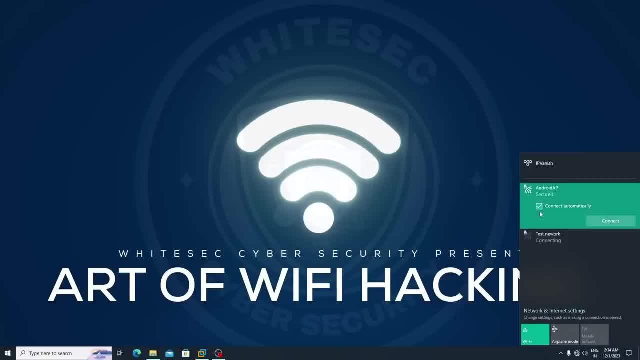 both network here, not not with this android ap. and see, i can't able to connect with android ap as well. i can't even connect with test network as well. see, if i click on connection, i can't able to connect with it. why? because the channel is same here, see, the channel is same. so that's why. 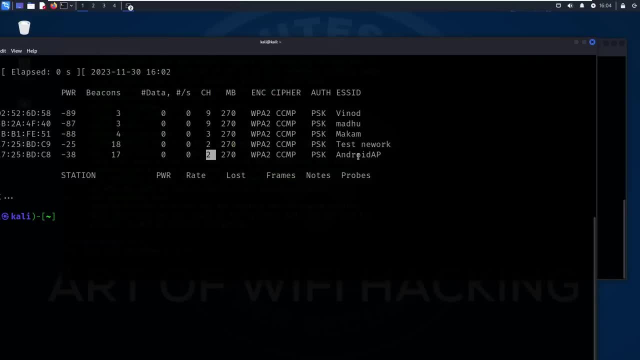 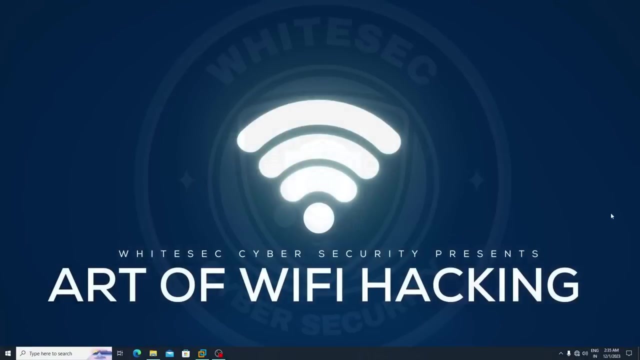 i can't able to connect, so this is one kind of disadvantage. okay so, but the attack is cool. okay, this is a thing. let's see. see. there is no internet connection. i can't able to connect with this wi-fi networks. until after stopping this attack, i can able to connect, see. 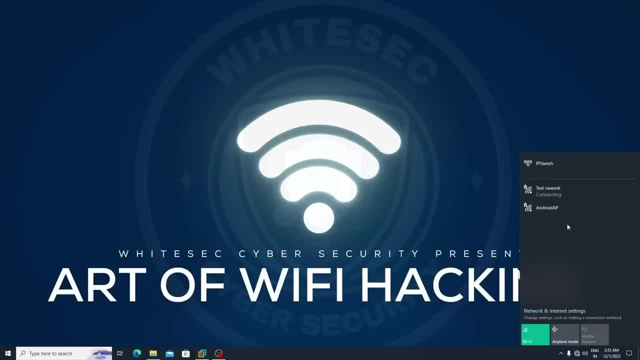 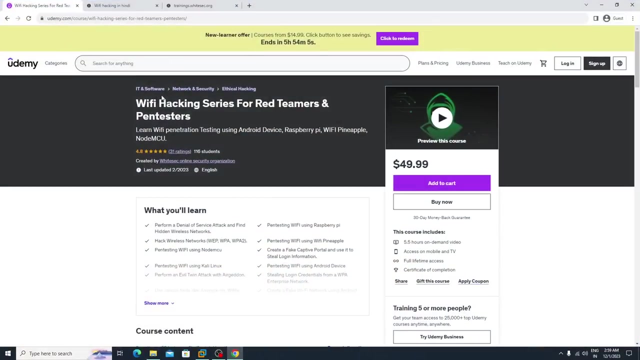 here you. it is okay, now i can able to connect it, connect with that network after stopping the attack, right. so hope you guys enjoy these classes. so if you want to learn more about wi-fi hacking, then you can also check out our wi-fi hacking series for red teamers and pinterest shirts on udmi see. 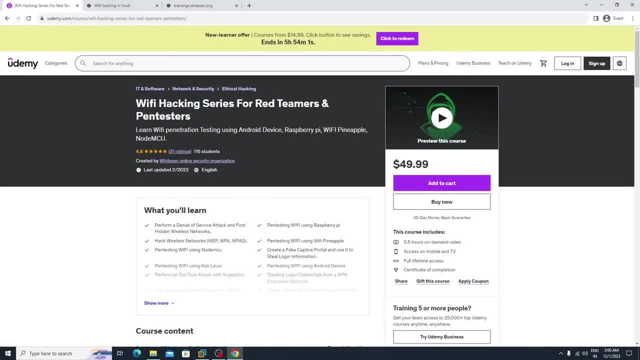 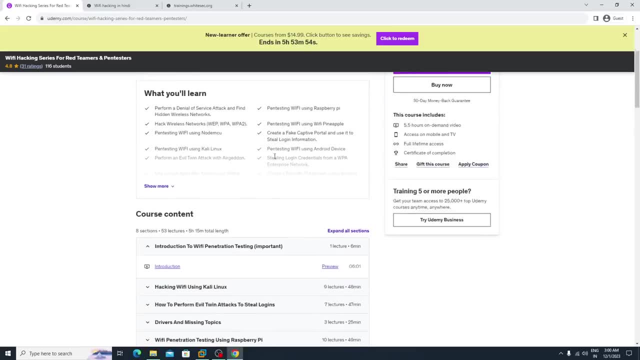 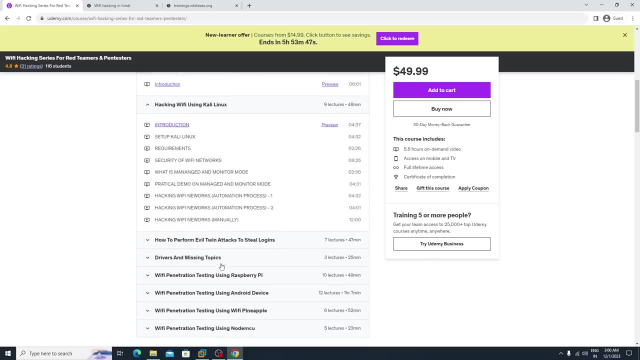 previously. what we did means we just added this course on our own platform. later, we just added this on udmi. okay, this is the thing you. you will learn here: how you can able to perform wi-fi hacking or wi-fi pentesting using different hardwares, such as we are using here: kali linux. okay, it's a complete uh. here also, we will go from. 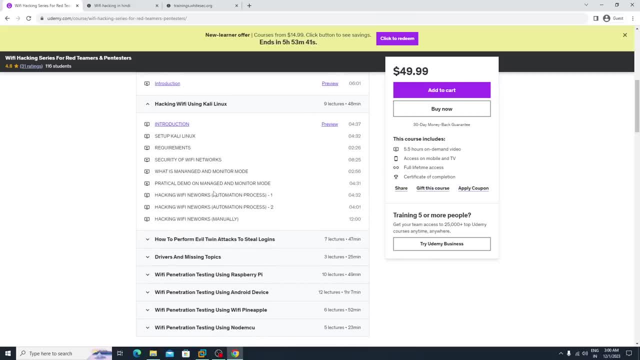 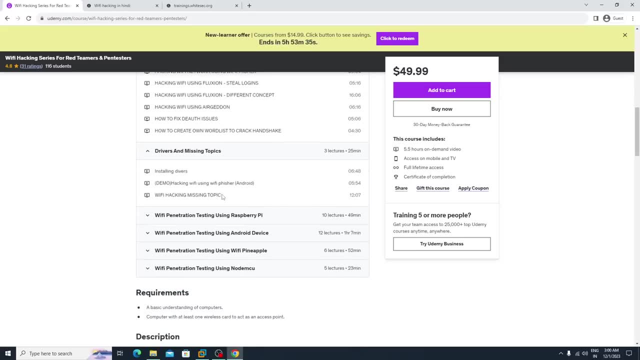 beginner to advanced. we will use, we will learn- evil twin attack. okay, if there is any kind of issues, we will try to fix it, okay, in this section. then there is a wi-fi penetration testing using raspberry pi. here we will learn about how we can able to use a raspberry pi for wi-fi hacking. 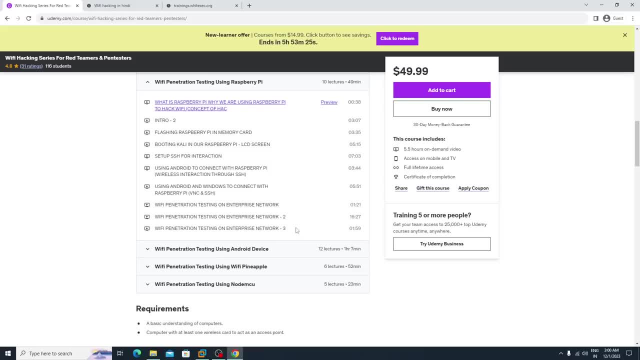 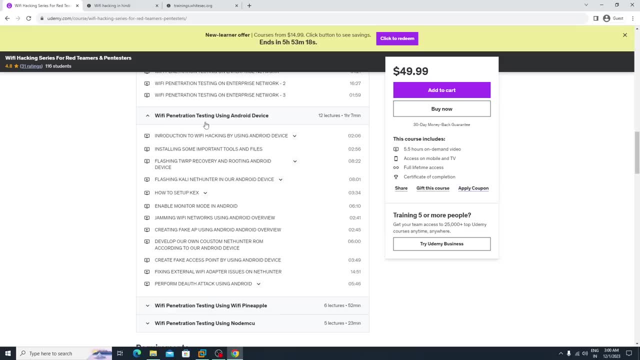 purpose. then we will learn how we can able to use the android device for wi-fi hacking. wi-fi hacking, wi-fi penetration testing using android. here you will learn, uh like by how you can able to hack wi-fi network using android. okay, later we will learn how we can able to hack wi-fi network using wi-fi. 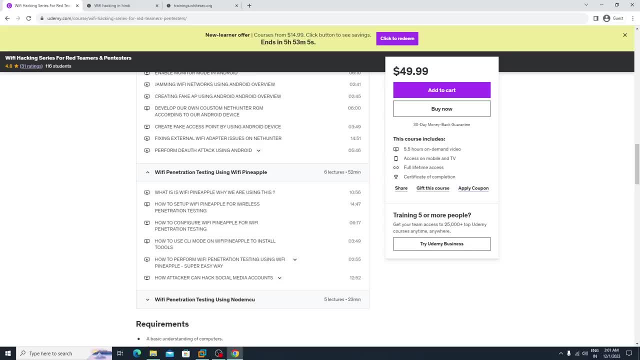 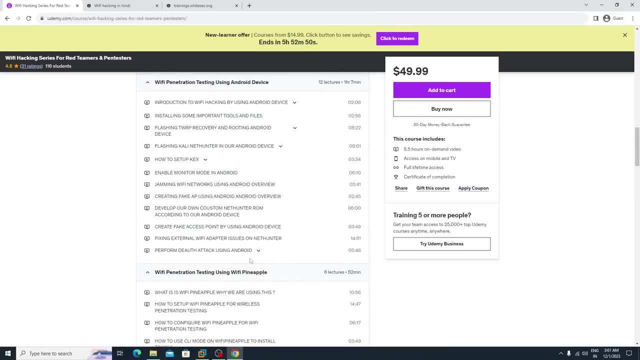 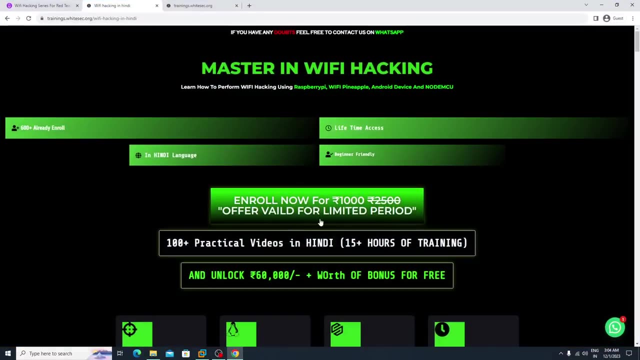 pineapple, then we will go for node mcu as well. so if you are inter interested, then you can also check out this one. so if you want to learn wi-fi hacking in hindi, then this is for you. master in wi-fi hacking- basically recently we just launched this training in hindi. okay, because 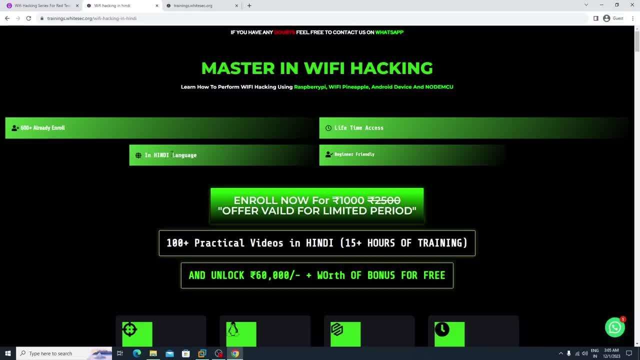 lot of students are from different countries. okay, now, uh, mostly the students are from bangladesh, india, pakistan, okay, some other countries where they speak hindi or urdu language. okay, uh, for they demand, they are demanding that, uh, they need a training in, in, in hindi or urdu. 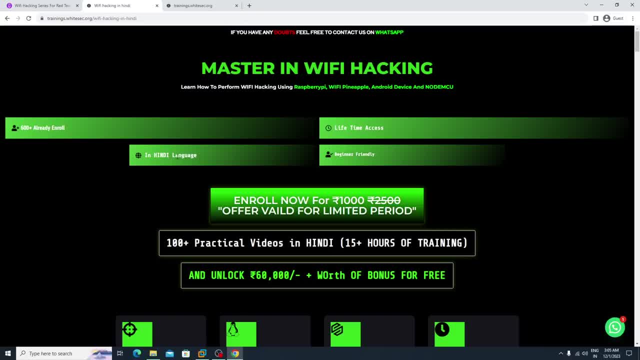 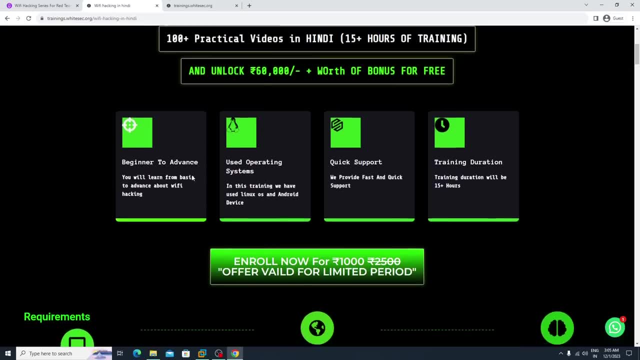 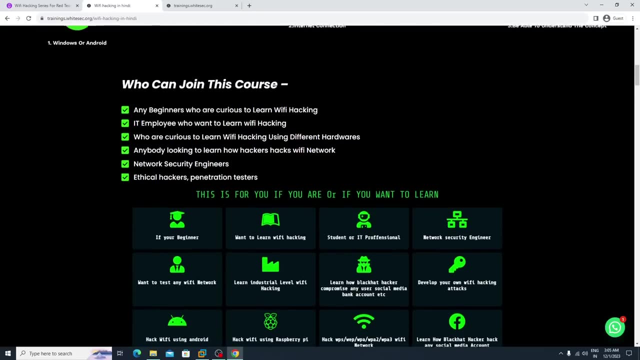 language. okay, so that's why we just launched this training, okay, uh, here we just added some more topics like: here you can able to see more. uh, just just wait here. these are the skills you will then just try to. uh, just visit this url and just try to read it. okay, the topics are. these are the topics. 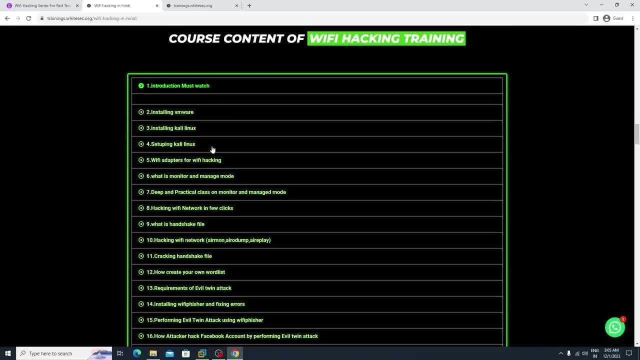 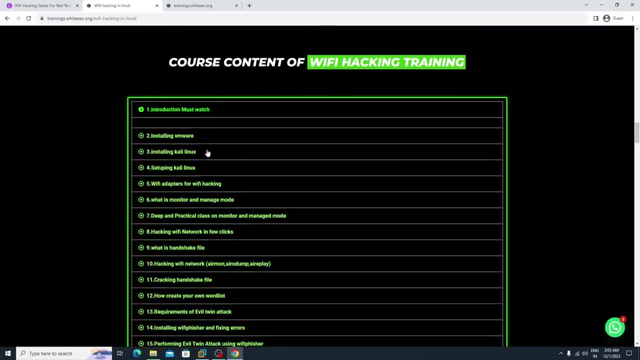 such as uh installing vmware, installing kali linux. this is also from beginner to advanced level. okay, it will cost you around 12 dollars, i think. okay, if you are convert this inr to usd, then it will cost your own to a dollar to a dollar. 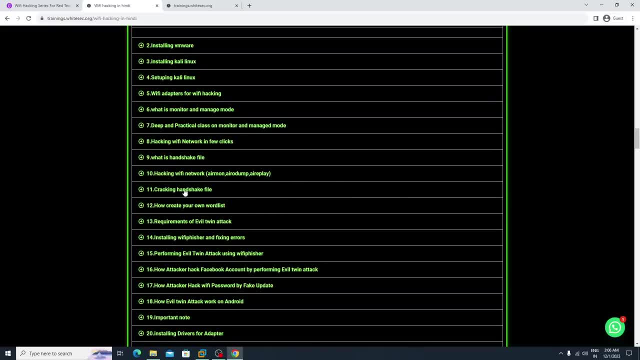 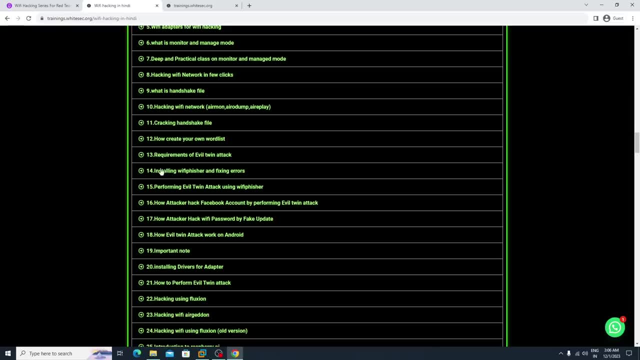 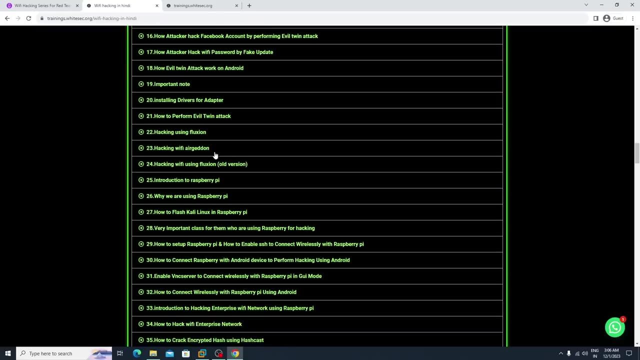 okay, right now here the same thing. okay, like what is handshake file? hacking wi-fi network, cracking handshake file, how to, uh, how to create your word list requirements of evil twin attack, installing wi-fi feature. here we just added some more topics related to how you can able. 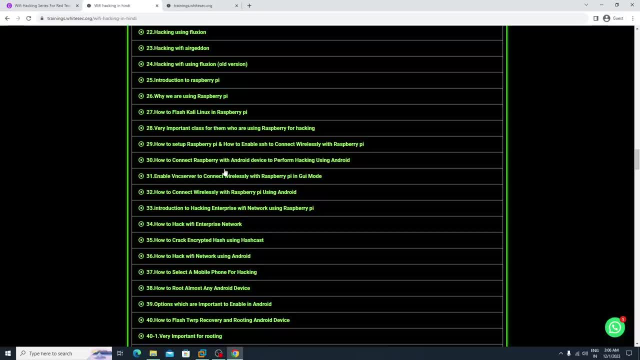 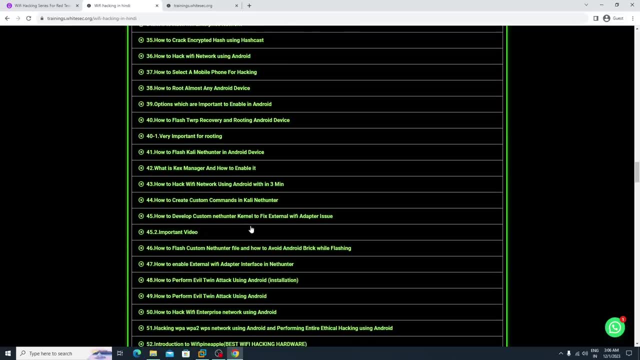 to develop your own wi-fi hacking hardwares as well. okay, we just added those topics as well. okay, we added a lot. we just also added uh evil twin attacker. okay, uh evil, sorry, not evil twin attack, it's a man in the middle attack. we also added a man in the middle. 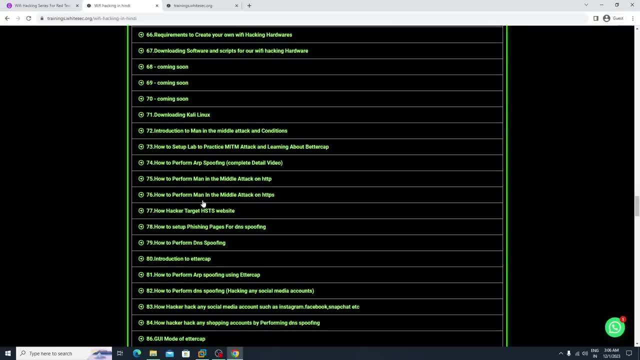 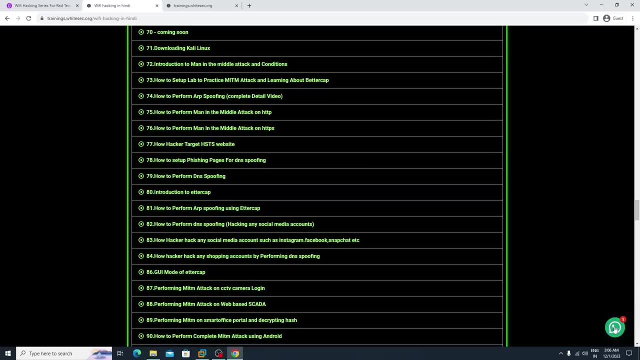 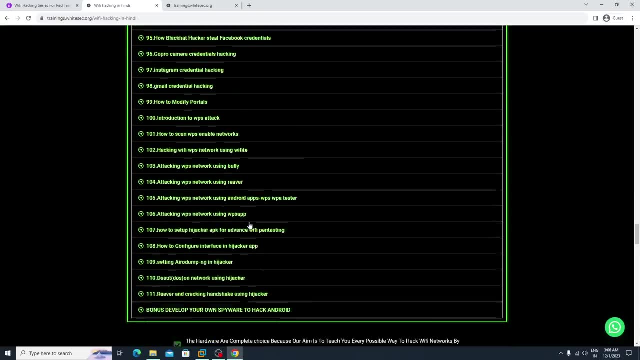 attack here. okay, so simple, if you want to enroll this training. simple contact our support team. here is the whatsapp. simply, if you click, then you guys can able to redirect to, uh, the whatsapp support. okay now, uh, here is the topics. just try to read it, okay, you, you will get a lot of bonuses. 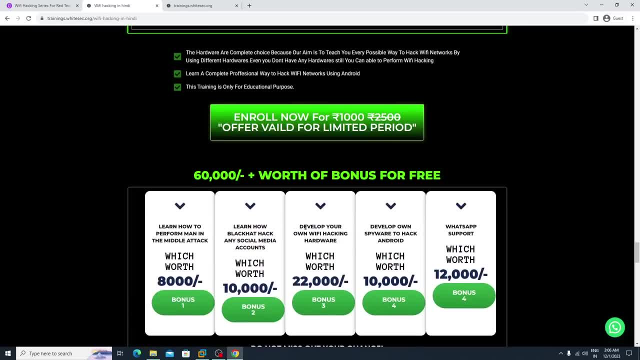 here like: develop your own spyware to hack android. develop your own wi-fi hacking adverts. learn how hackers hack any social media accounts. yeah, it comes under man in the middle attack by using- i'm sorry, by performing this- dns spoofing, we can able to steal the social media accounts as 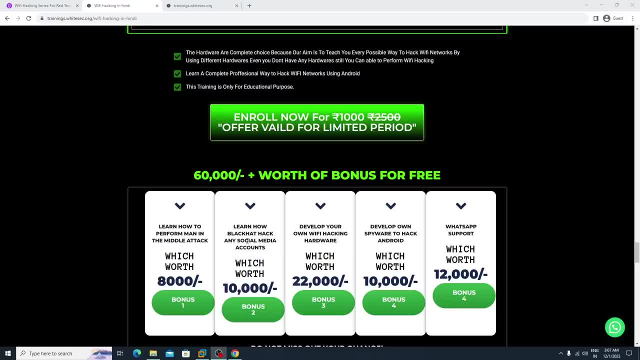 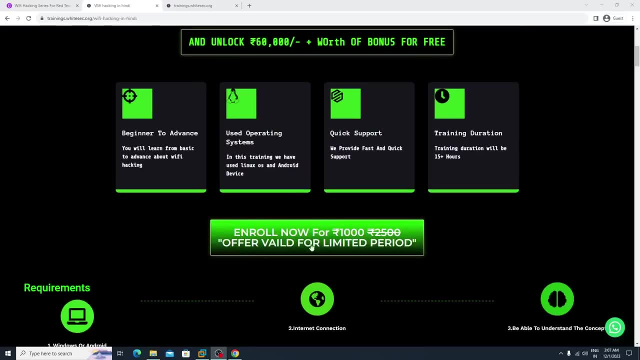 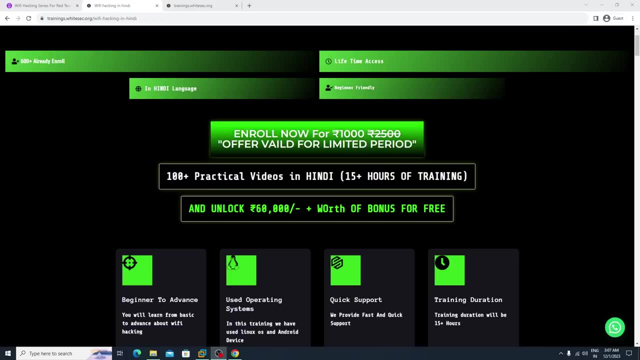 well, okay, so we just learn each and everything. practically, the training duration might be: just wait, it might be 15 hours. okay, that you uh, that the training duration is 15 hours. you will get panel assets. you just need to contact our support team. you need to provide your full name and email address. okay, with this proofs- payment proof then. 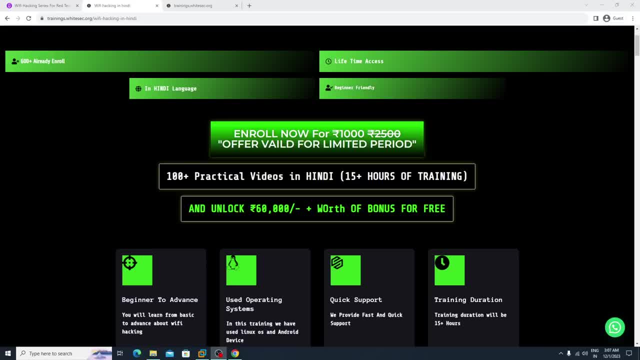 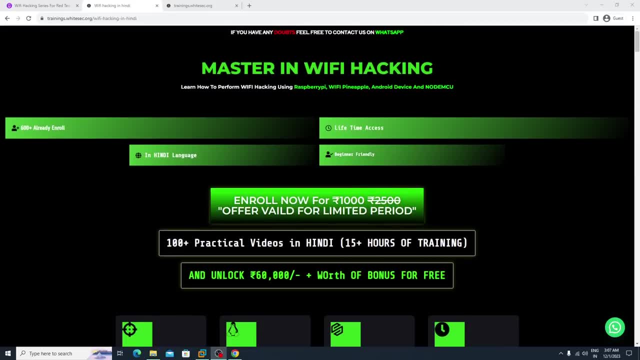 they will provide you the access on your email address. this is the thing, simple: just contact our support team if you are interested, uh, if you uh for this training right, want to learn how to perform red teaming, then this training is for you. in this training, you will learn how you can able. 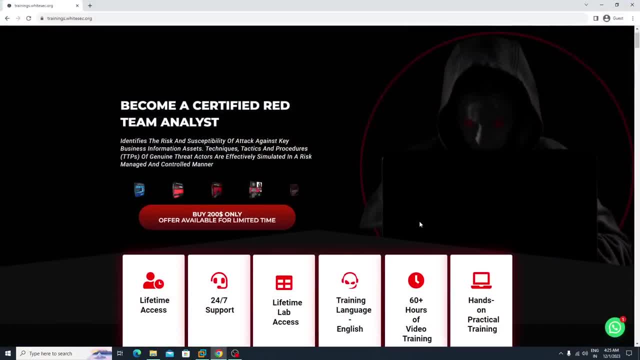 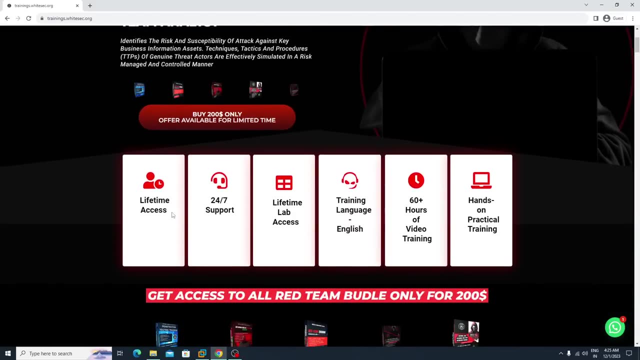 to perform red teaming, miter attack, active directory, pen testing, internal and external team operations, etc. now here, this is a pre-recorded training. you will get a panel, as is from where you can able to, as is from where you can able to watch this training. let 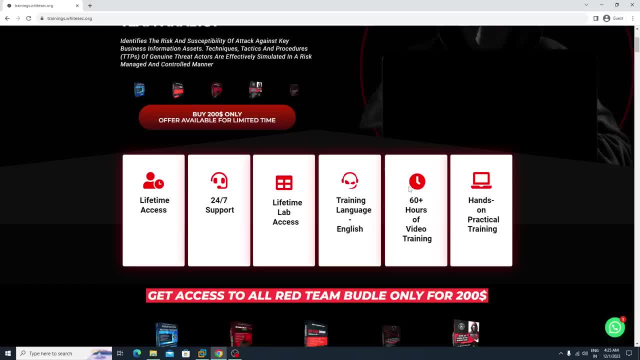 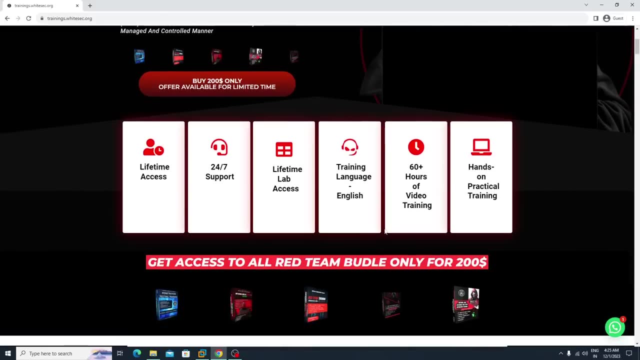 me tell you, you will get a lifetime access for panel and you will get 24 by 7 support lifetime lab houses. you will also get a download, downloadable labs, okay, and also the training languages in English: 60 players plus hours of video training. maybe we will try to update more. right now, the training duration is: 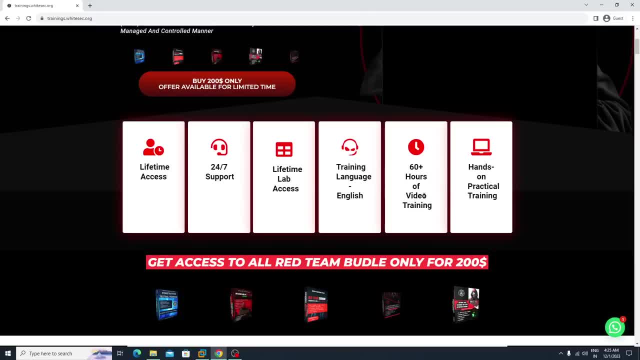 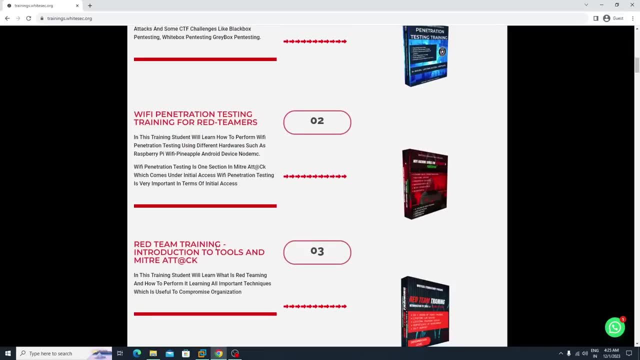 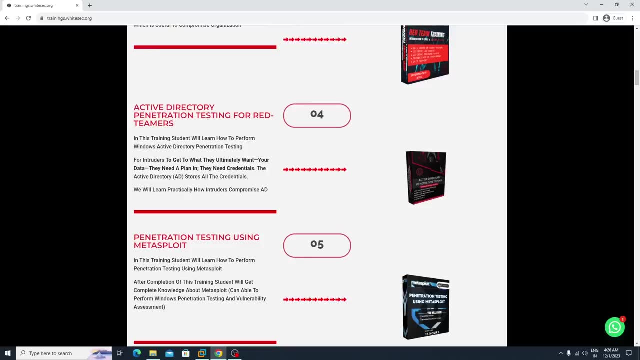 60 hours now. here you will learn pen testing, Wi-Fi penetration testing, red team training, introduction to tools and MITRE attacks. then you will learn active directory pen testing for red teamers. then you will learn about meta exploit, penetration testing using meta spread. it's a complete training for red. 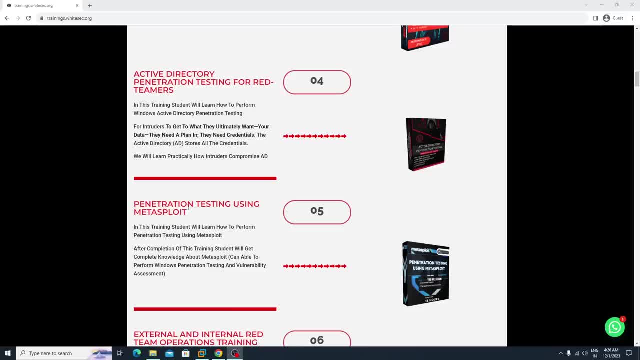 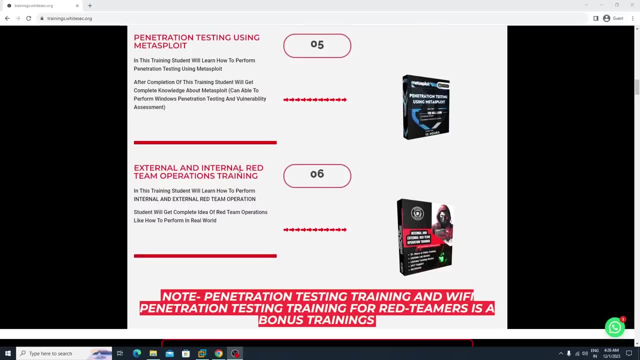 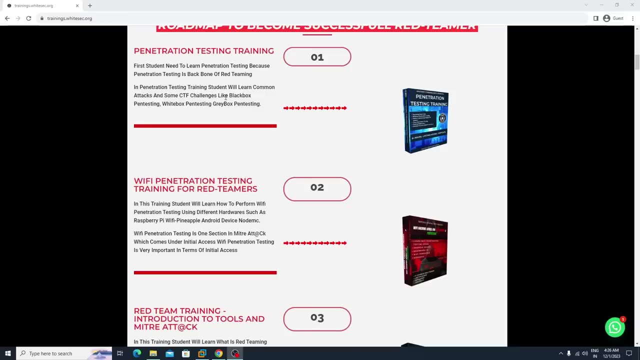 teamers how you can able to use a meta exploit okay, and also you will get asses to an external and internal Red Team operation. it's kind of good map. first you need to complete this, then you- first you need to complete it- you will learn a basic pen testing as well, if you don't know about penetration. 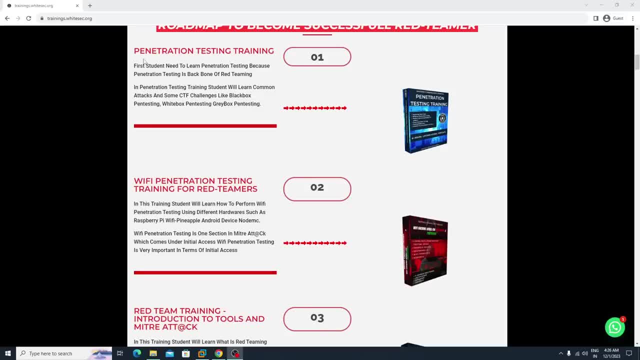 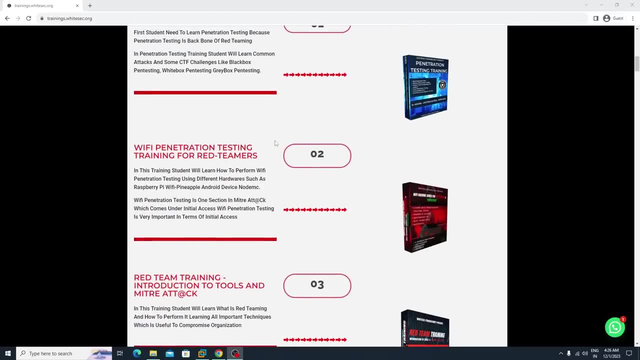 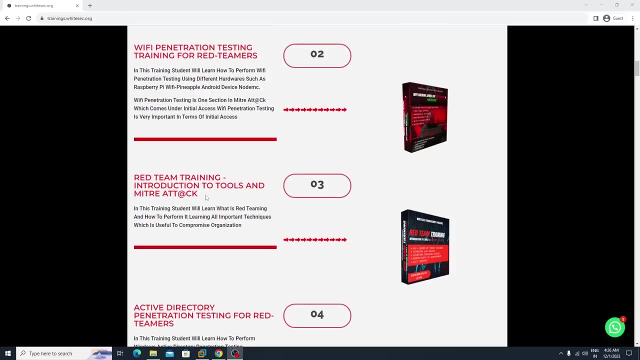 testing. then you will get asses for penetration testing course. then after that you need to watch the Wi-Fi pen testing course. it's a kind of roadmap, as I said: you roadmap to become a successful red teamer. then you will learn about red team MITRE attack. it's a good, very you. 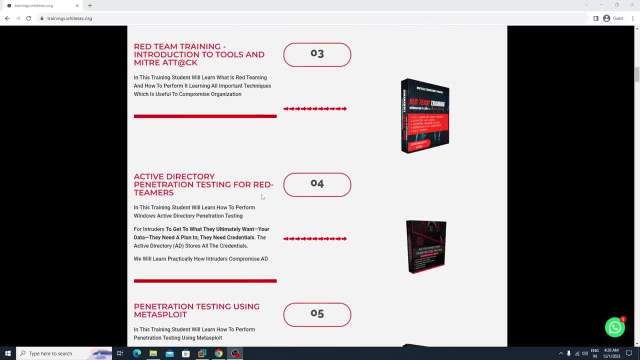 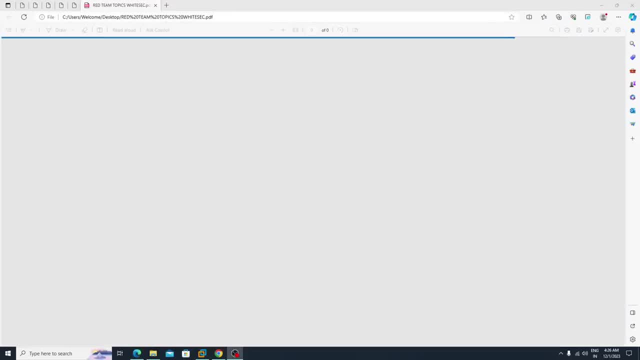 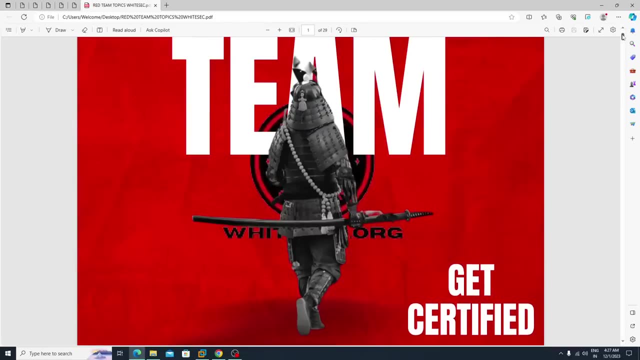 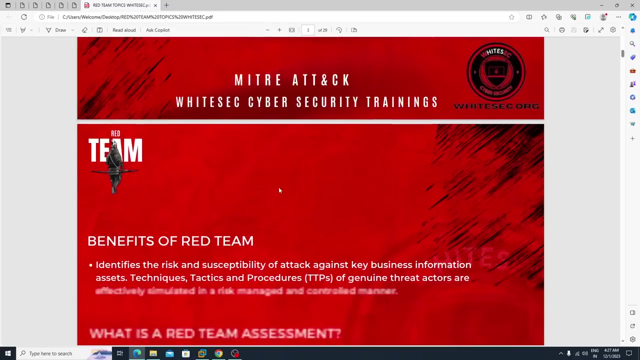 training. so here are the topics and let me explain you here what you will learn in this training. okay, what we are covering here. see, I'm gonna provide you the PDF as well here. from here, you can able to see what is red teaming, benefits of red teaming, what it read a red team. 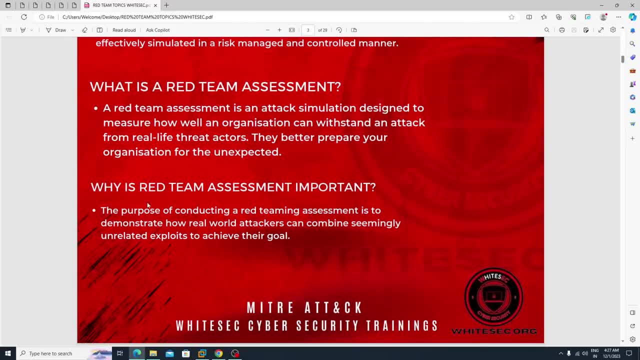 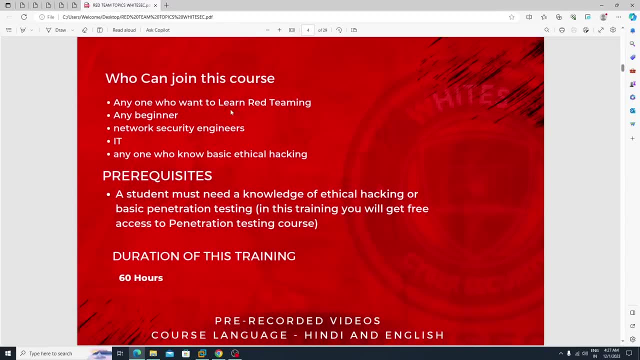 assessment. why is red team assessment important? who can join this training? it's for anyone. if you don't have knowledge about ethical hacking, just watch our training, which is available on YouTube, then you can also join this training. if you don't have ethical hacking knowledge as well, you can able. 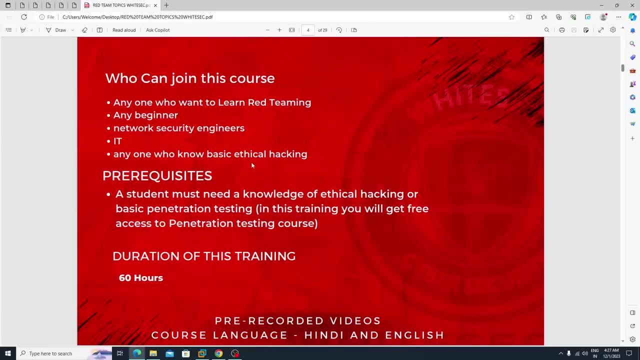 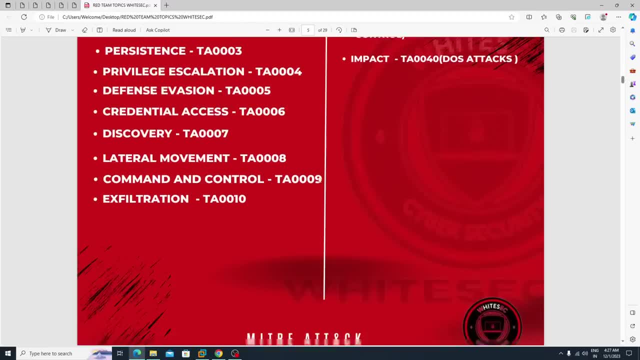 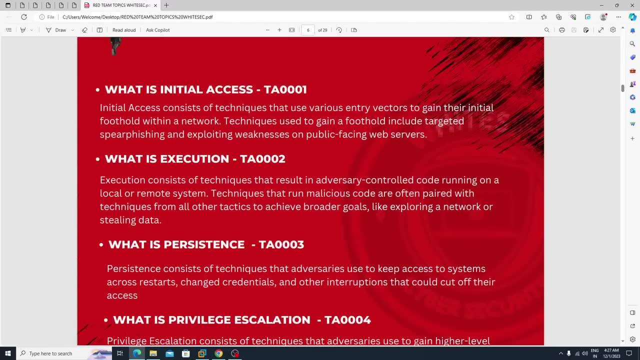 to join it, because this training is completely designed for the beginners. these are the tactics which we are covering here. it's a complete red team tactics like in: just let me show you you. from here, you can able to learn about what is initial asses, what is execution. 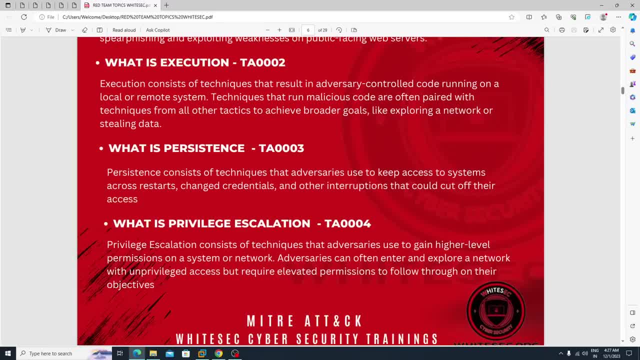 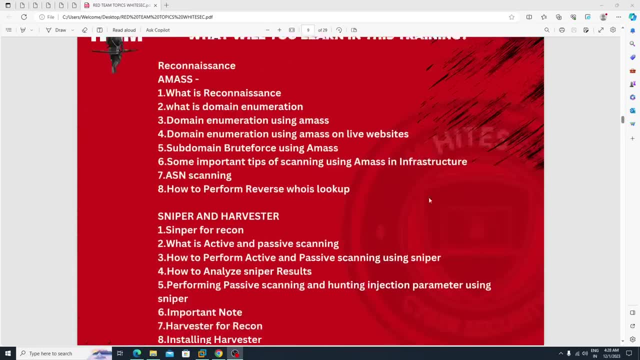 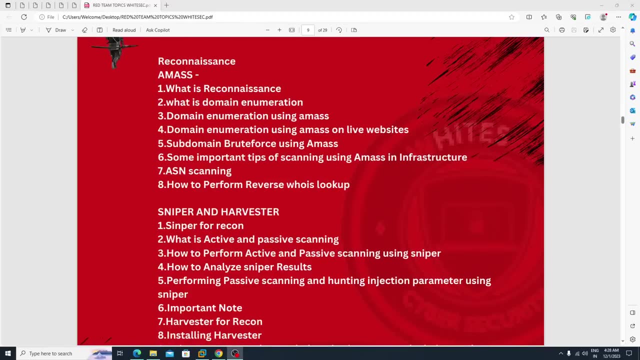 what is persistence, what is privilege escalation, this all stuffs. and just try to read it, then here are the topics which we are covering here in reconnaissance section. we will learn about a mass sniper and harvester. then we will learn about reconnaissance. these are the topics in reconnaissance we are 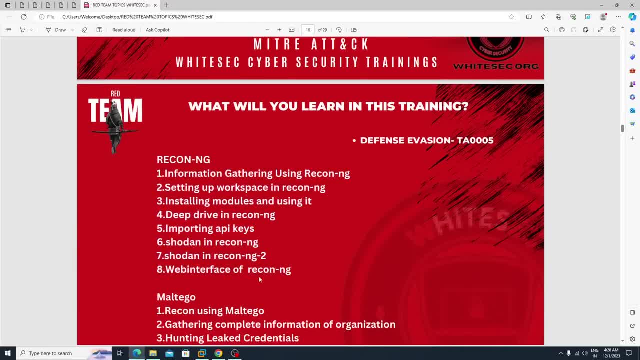 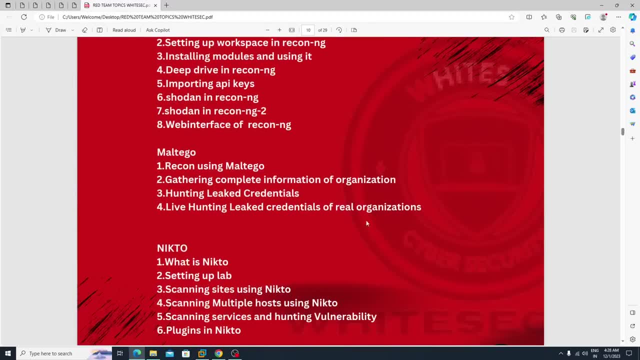 covering these things in sniper and harvesters, and then we will learn about harvesting or harvesting harvester. we are covering these topics. okay, in multi go. we are covering these things, and we are also using Nikto. we are covering these things as well. okay, showdown. we are learning about. 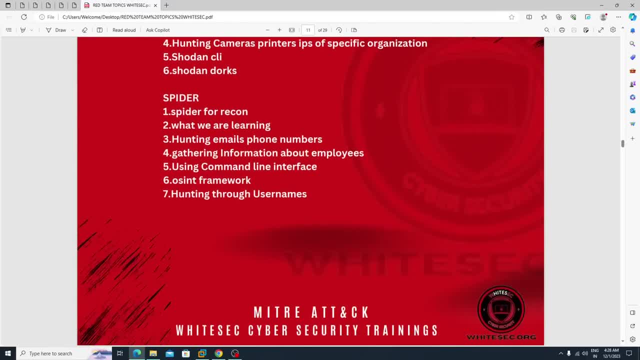 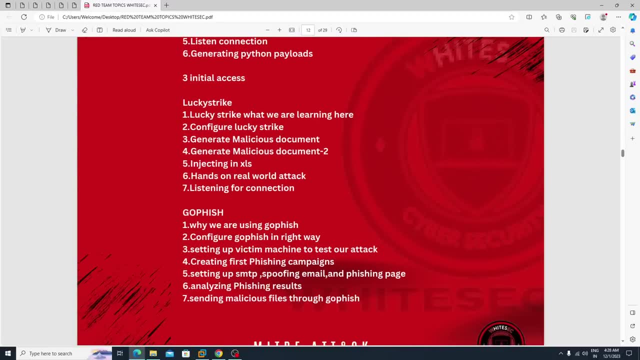 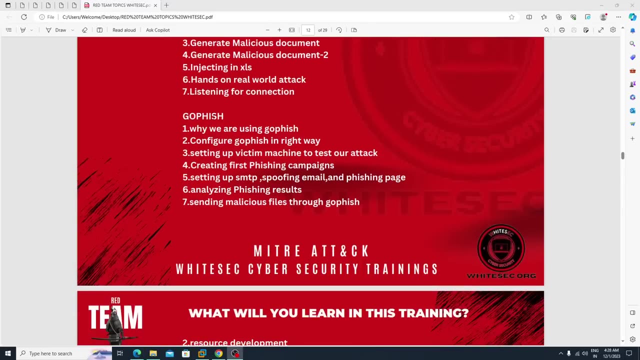 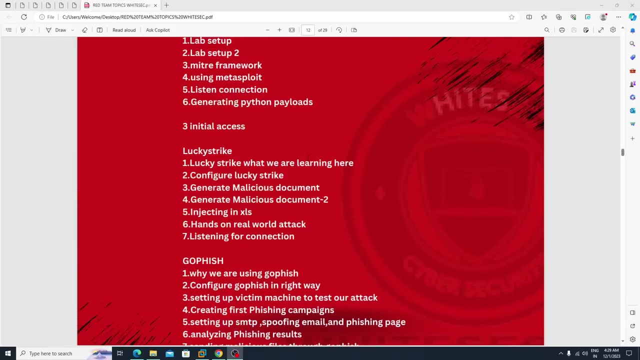 showdown spider. then we will go for the resource development. then we will learn about initial asses like generating a malicious document, injecting in XLS. let me tell you it's a very huge training. GoFish: we are learning how we can able to perform a fishing campaign organization. basically, here you will learn how you can able to perform this. attacks on real world. 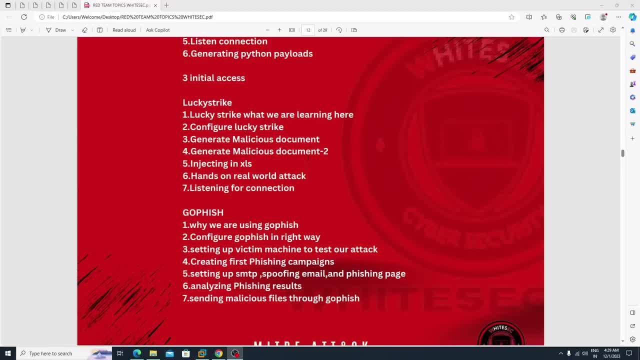 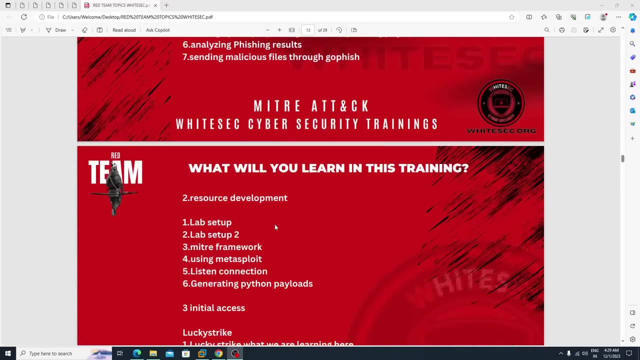 organization, like you are working as a pentester or any i. if you are in any it field, then this training is excellent for you. if you want to become a red teamer, okay, like here. we just covered each and everything which is necessary in one organization. okay, like if they want to conduct. 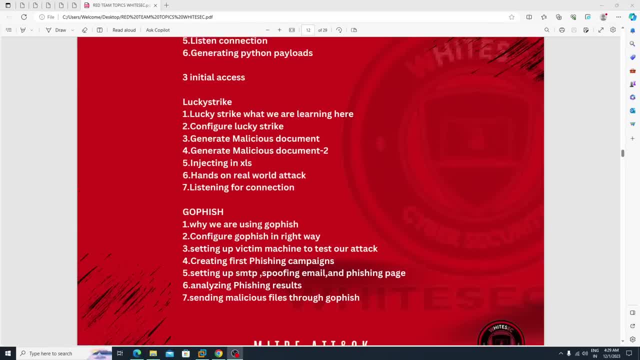 any kind of phishing campaigns. you guys will know that uh, time to time, a red teamer will conduct a phishing phishing campaign. okay, to check the their employees, uh knowledge, okay, like they are, they're having a correct knowledge about phishing or not. like these are the things which we are. 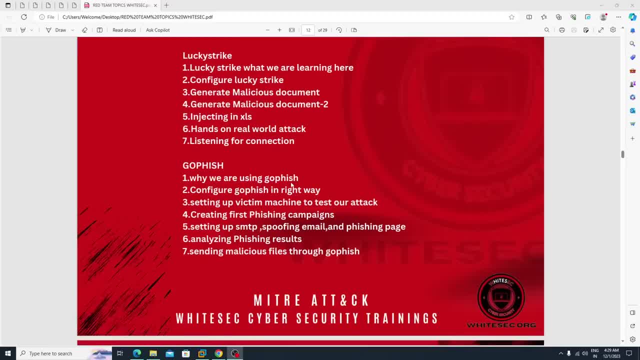 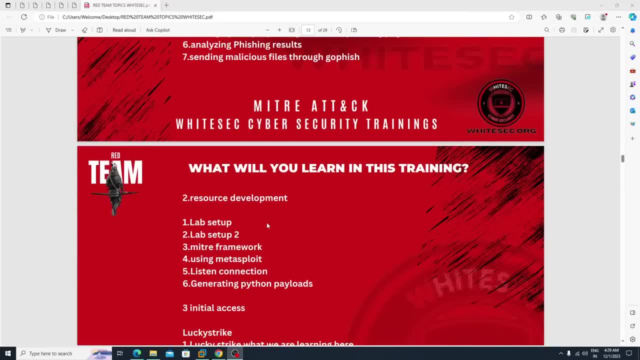 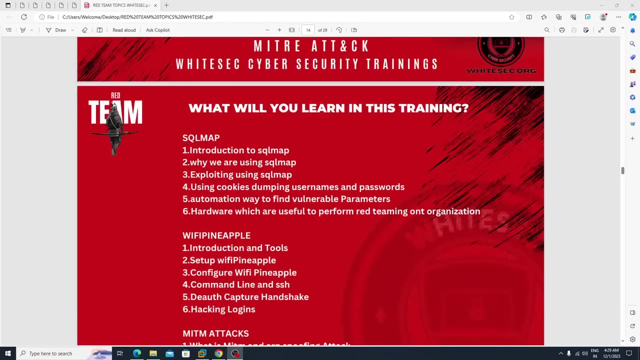 covering here. the simple thing is, we are learning complete, hands-on, practical okay, and we are covering how the attacks will work in real world. this is a thing now. here you will learn about initial you a sql map, wi-fi, pineapple, midm attacks. here also you will learn about midm attacks and then 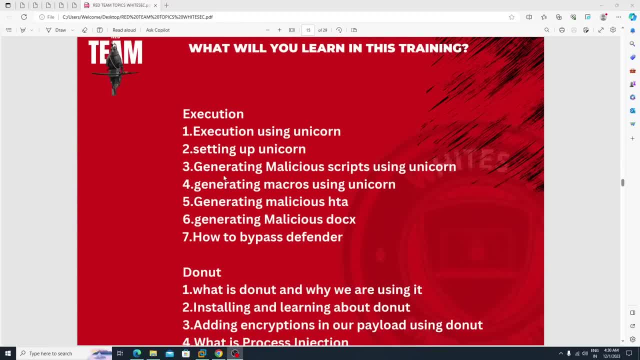 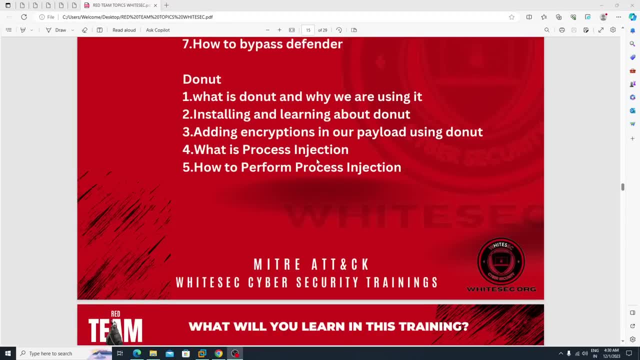 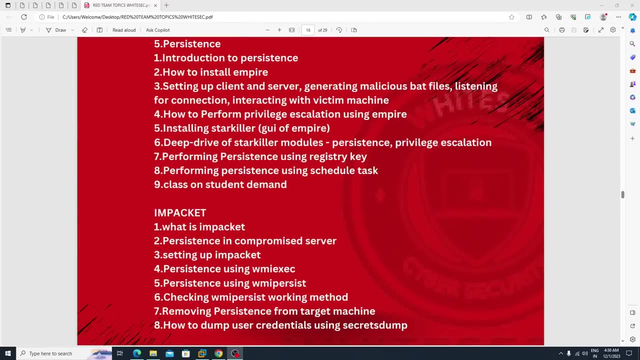 execution. we here, we are covering about donut, like how we can able to perform the process injection. what is process injection? this kind of stuff. then there is a persistence in persistence. we are learning this. all steps in lateral movement. we are covering this. all steps like pass the ticket. 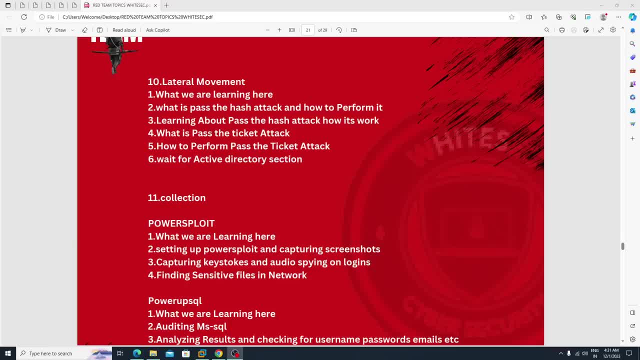 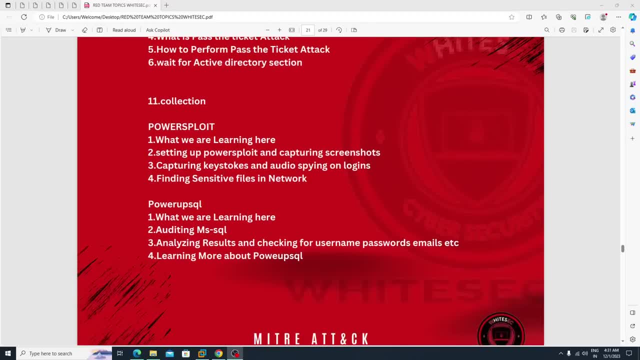 attack. pass the hash attack. what is the pass the ticket or pass the hash attack, how it's gonna work. here we are covering this: all shops. then we will move to collection. in collection we are learning about power of power up, sql's power exploit, and then we will move to commands and control. here we 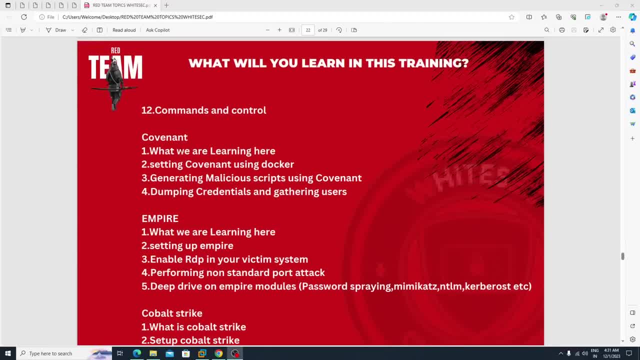 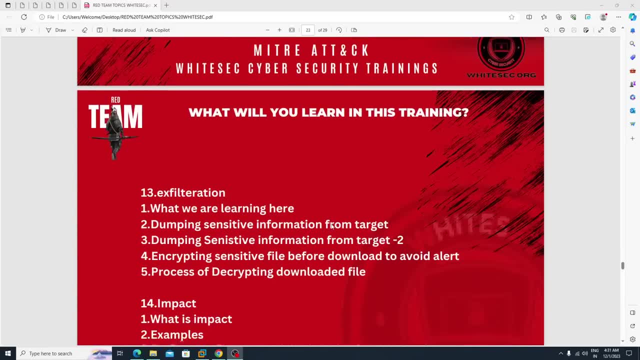 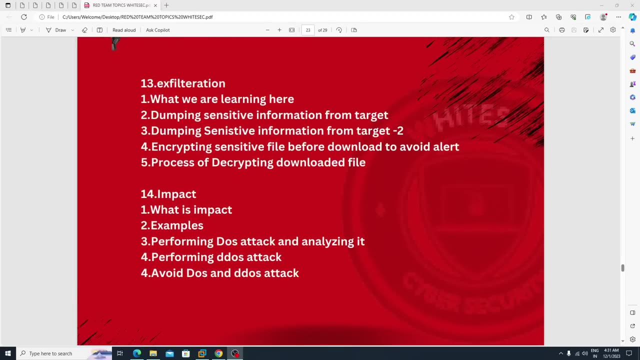 are learning about c2. okay, covenant is there, empire is that we are learning about cold cobalt strike, then we we will move to exfiltration, like dumping the sensitive information from the target, like a password, files or any private informations like. then we will go for the impact. 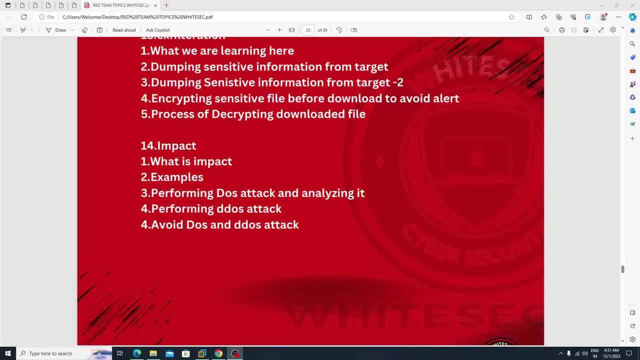 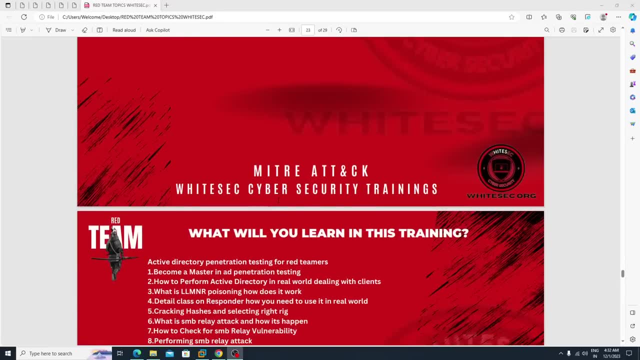 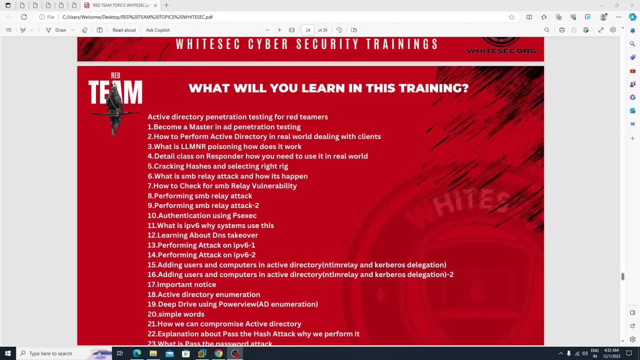 like: here we are covering about dos or ddos attacks, then here, after completing this whole section, then we will move to active directory pentesting here in active directory pentestings. uh, these are the topics which we are covering. okay, these are the. let me tell you, this is a very huge. again, i'm 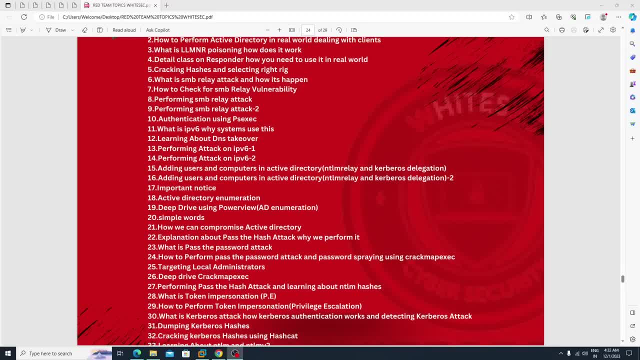 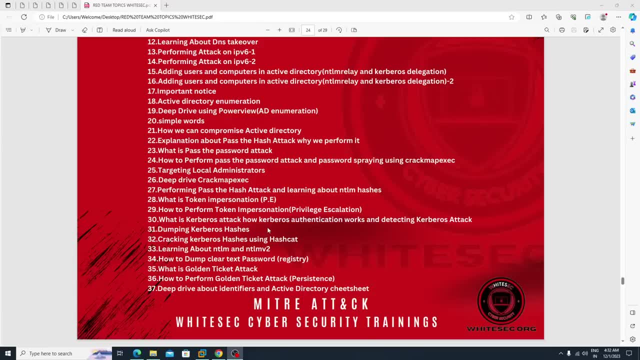 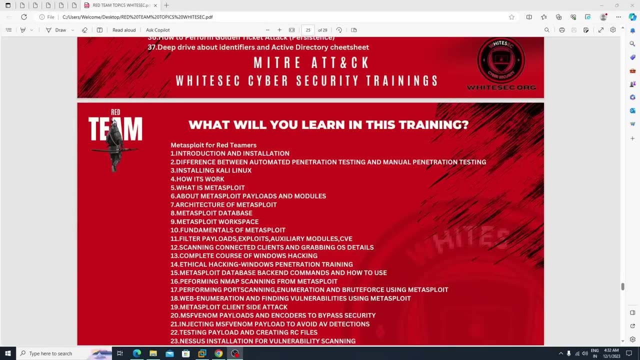 saying it's a huge training. okay, so here you will learn about Kerberos, how to perform the pass, the ticket attack, golden ticket attack, silver ticket attack. okay, like that. then we will move to metasploit for red teamers. then we will learn about how we can able to use this metasploit. 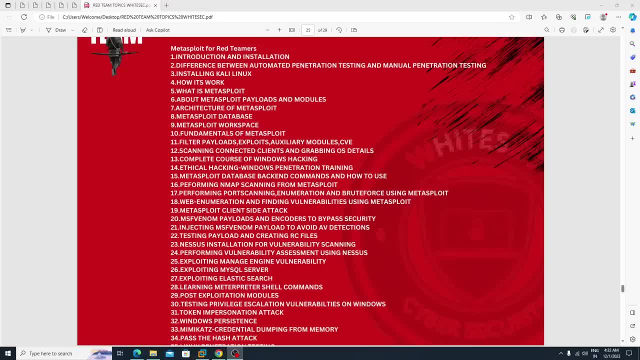 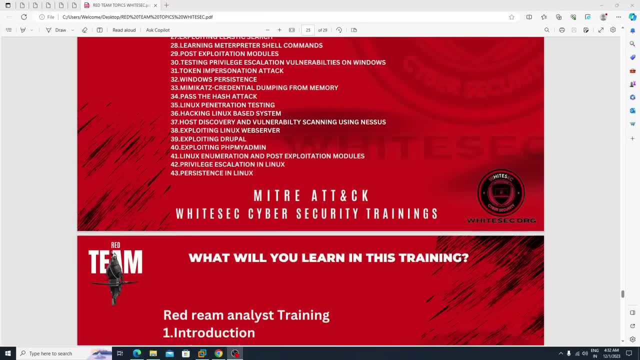 in a red teaming purpose. okay, like during red teaming assessment, like we will learn about this all stuffs. okay, then we will learn how we can use these all stuff. okay, then we will learn how we can able to perform this internal and external red team operations. this is a 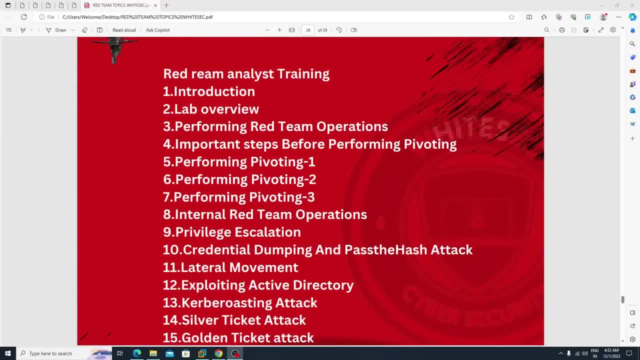 also one section where you will learn how you can able to perform this whole: attacks in real-world organization. okay, like once you jump in one company, then from where you need to start and how to perform the attack, is it okay? this is this, all the simple things which we are covering here. okay, like from maybe it's. 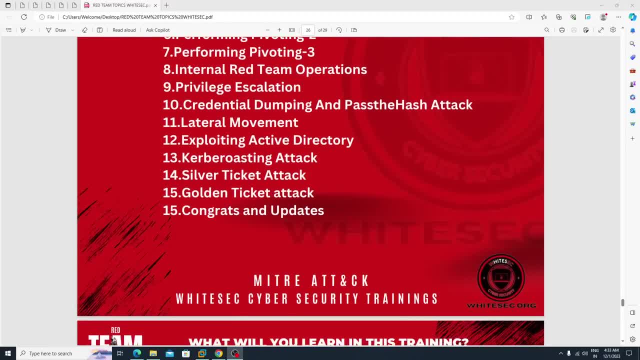 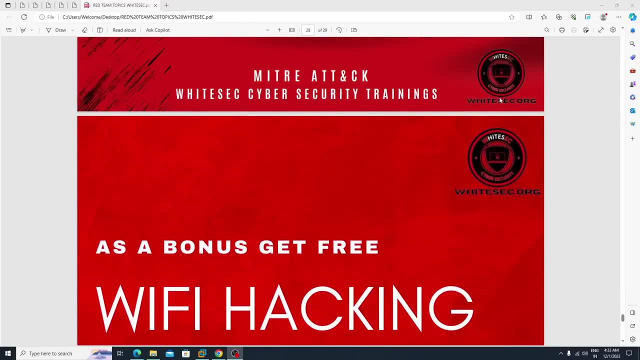 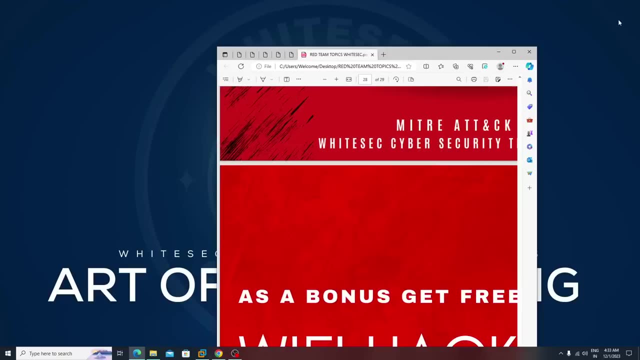 a 16 topics and we will try to cover more topics here, right? so if you are interested, simple contact our support team then they will provide you more information about this training. so hope you guys enjoy this training, this Wi-Fi hacking training. thank you have a nice day. so, guys, hope you are fine in this. 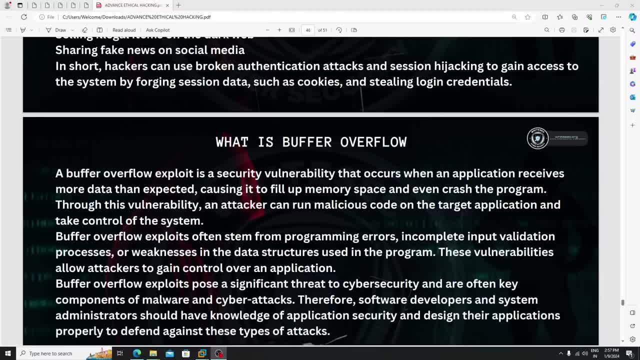 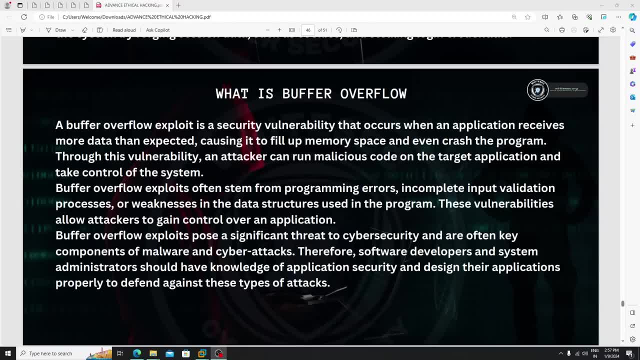 classes we are learning about. what is buffer overflow? the buffer overflow exploit is a security vulnerability that occurs when an application is installed in the buffer overflow and the buffer overflow is received more data than expected, causing it to fill up memory space and even crashed a program. through this vulnerability, an attacker can run. 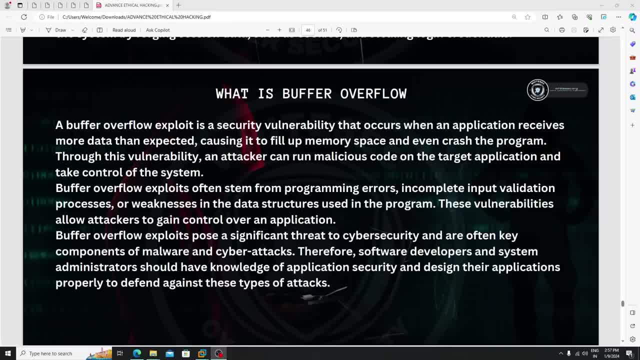 malicious code on the target application and take control of the system. buffer overflow exploits often steam from programming errors, incomplete input validation process or weaknesses in the data structure and used in the program is this ability's allows attacker to gain control over an application. basically, if there is kind of C exploit of just focus on this point which is a buffer. 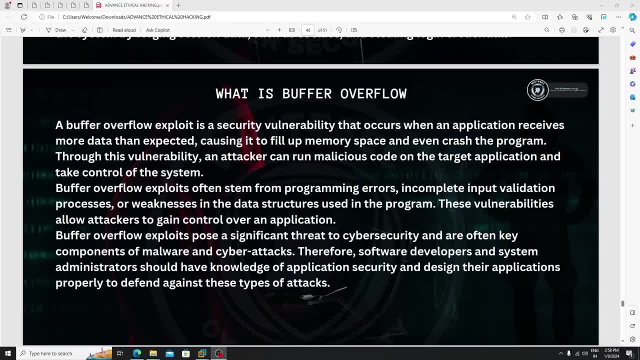 overflow. exploits often steam from programming errors, incomplete input, validation processes or weaknesses in that data structure using the program right. so these for remember, disputed attacker to gain control over what an application. this is the thing. basically, we are targeting the application here. okay, the application might be anything. okay, like. 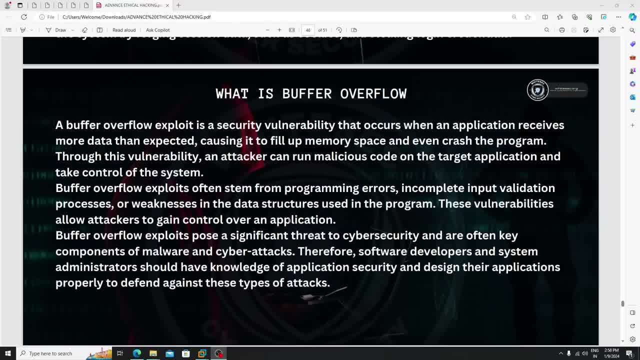 it might be a browser, it might be any exe file, right. so this is the thing. now, the main thing you need to focus is this one, which is, uh, you need, uh, just remember this point, okay, which is this one: a buffer overflow exploit is a security vulnerability. okay, this one from here, causing it. 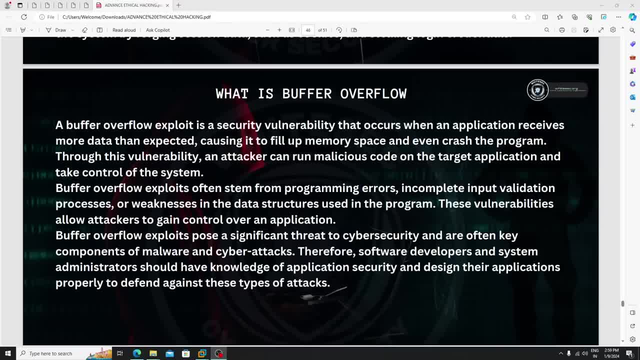 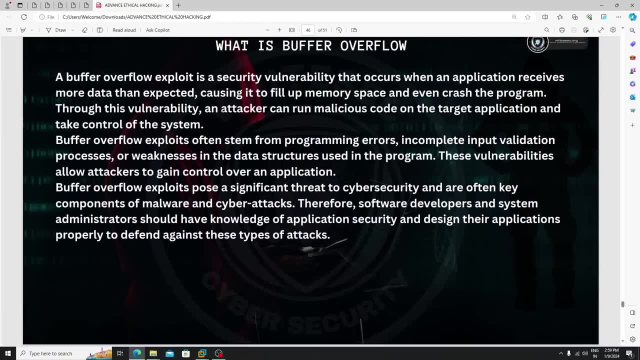 to fill up memory space and even crash the program. this is very important. okay, you need to remember this point. you will see why, uh, why i am saying this. remember this point. uh, in next classes you will see that. okay, why this point is important. now here. components of marvel and cyber. 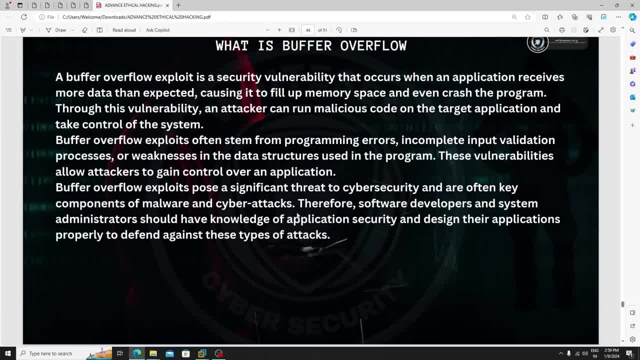 attacks. therefore, software developers and system administrators should have knowledge of application security and design their application properly to defend against these types of attacks. let me tell you here: assume that you, you are a developer. okay, if you don't have the application security knowledge, then these attacks might occur on your application. this is the thing. assume that there. 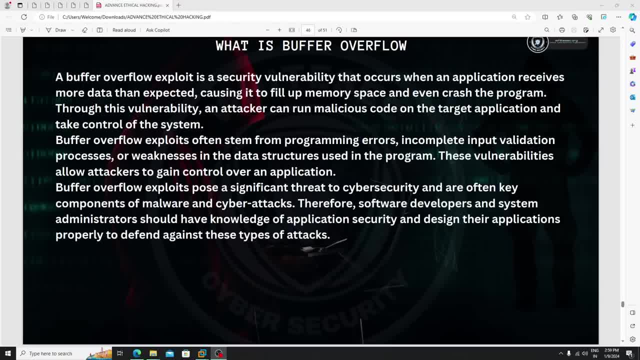 is a secure coding, is there? okay, this is also one topic which is known as a secure coding. basically, there, we covered, uh, this kind of stuff, such as how to secure the code to avoid this kind of attacks, right, so this is a kind of secure coding where the 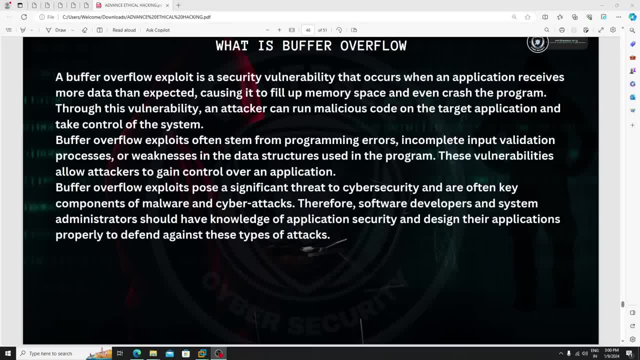 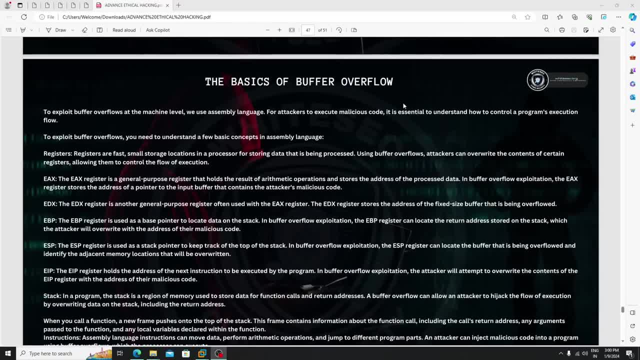 uh, programming, uh, this developers will learn that one. okay, this is the thing. now, here you will see the basics of buffer overflow. this is this pdf is very important guys. this page, the uh, to exploit buffer overflow at the machine level, we use assembly language. okay for attackers to execute. 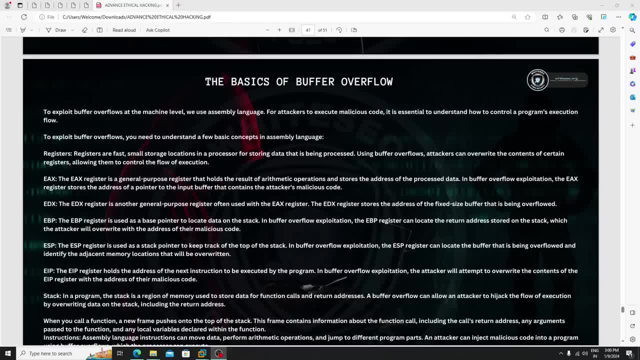 malicious code. it is essential to understand how to control a program execution flow to exploit buffer overflow. you need to understand a few basic concept in assembly language. let me tell you. if you don't know about some assembly language, you no need to worry. there are a lot of. 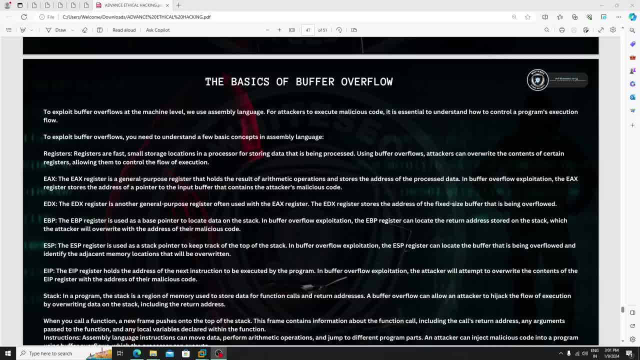 courses on there on youtube channel. just try to watch it. okay, it's not a big deal to learn assembly language, but it is hard by comparing to other languages, because it is a kind of confusing thing, right? so just you no need to uh do a lot there, but still you need to. 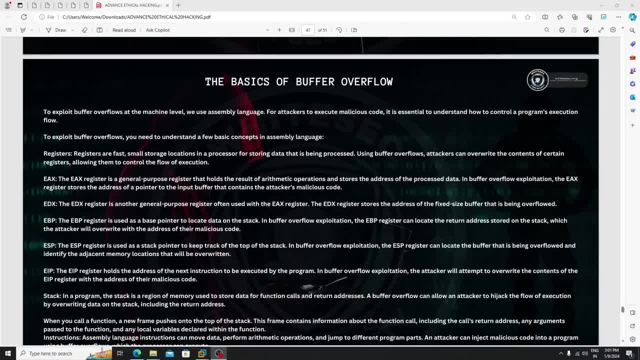 learn that stuff right. so just learn the basic knowledge about this. you will get the basic knowledge about the assembly language. if you want to, uh, learn more about this buffer, overflow or exploit development things, now here there are some. there is a registers or their ex is there: eds, edx is. 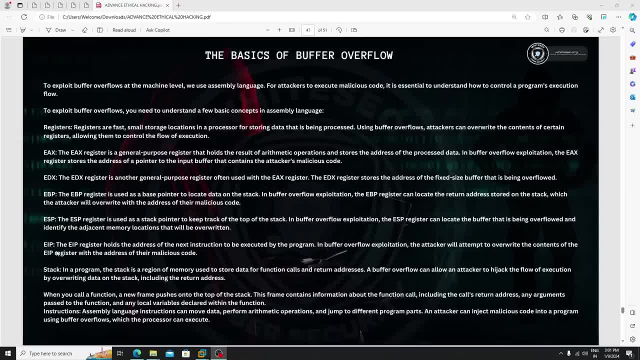 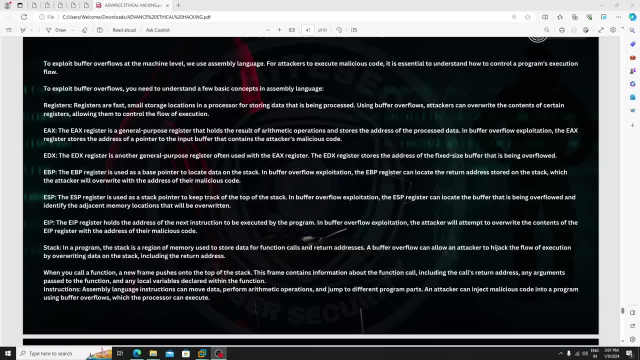 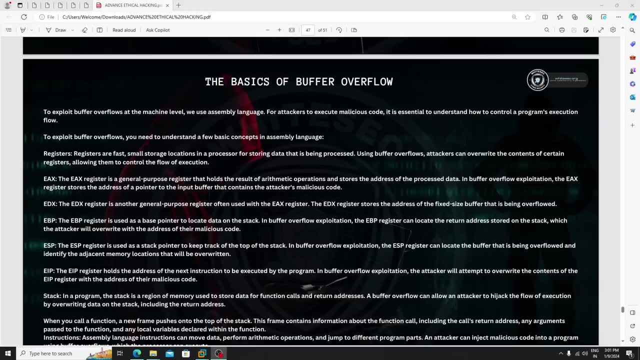 there evp? is there esp eip stack? see, let me tell you, uh tell you, eip plays a very important role during this uh offer overflow attack. okay, now uh registrars, registers are fast small storage location or bla bla resistance. yeah, these�로ay storage location in a processor for storing data that is being processed. 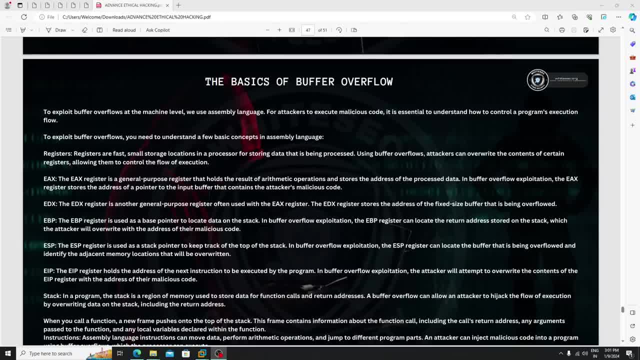 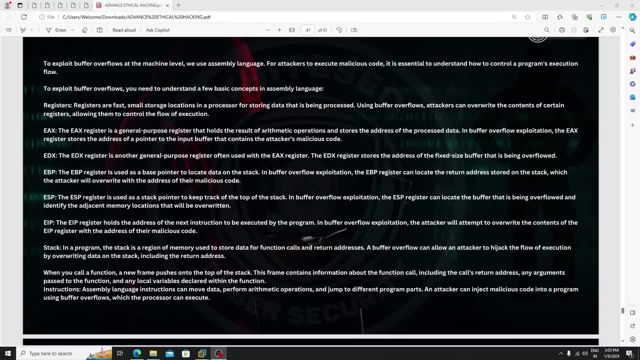 Using buffer overflow, attackers can override the content of certain registers, allowing them to control the flow of execution. EX. The EX register is a general purpose register that holds the results of automatic operations and stores the address of the processed data in buffer overflow exploitation. The EX register stores the address of a pointer to the input buffer that contains the attacker. 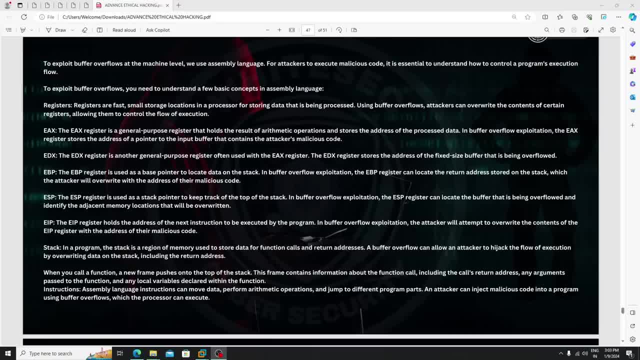 malicious code. In EX, the register stores the address of a pointer to the input buffer that contains the attacker malicious code. This is the thing. you don't worry about this, all stuff. Once we jump in practical, you will see what is EX where the what is EX is there, basically, 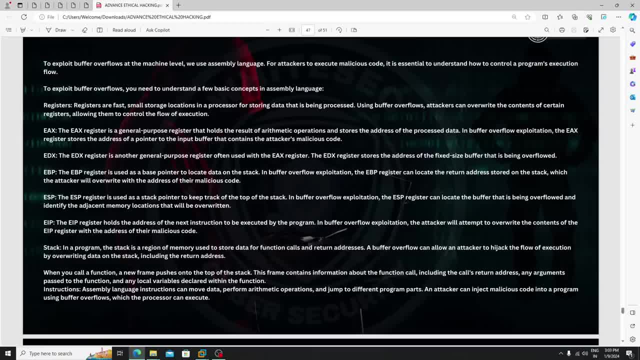 it's stored, it's addresses. This is the thing: EDX. The EDX register is Another general purpose register often used with the EX register. The EDX register stores the address of the fixed size buffer that is being overflowed And there is a EBP. 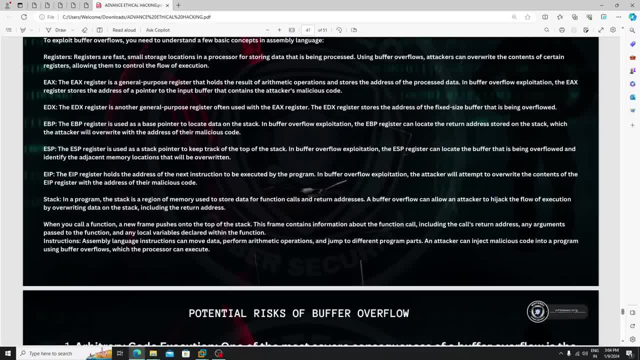 The EBP register is used as a base pointer to locate data on the stack In buffer overflow exploitation. the EBP register can locate the written address stored on the stack, which the attacker will override. with the address on the stack, The EBP register can locate the return address stored on the stack, which the attacker will. 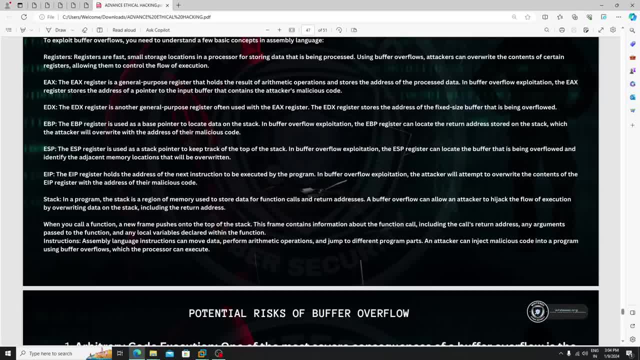 override with the address on the stack. This is the thing. you don't worry about, this all stuff. Let me just show you what the buffer overflow means. In the buffer overflow the EXP register is the OSP of the stack. The ESP register is used in the stack to locate the buffer itself. 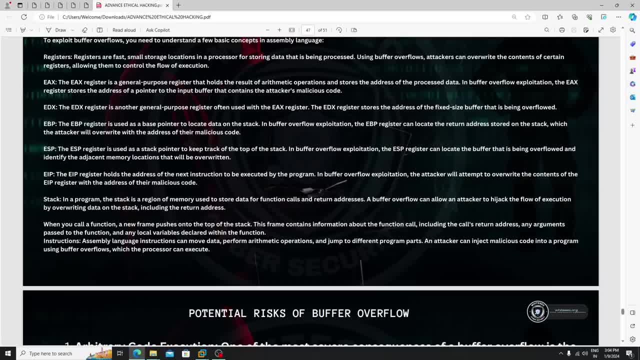 The ESP register is used to locate the buffer itself. The ESP register is a stack for the stack. There is an ESP, Now there is a ESP. ESP register is used as a stack pointer to keep track of the top of the stack In buffer overflow exploitation. the ESP register can locate the buffer that is being 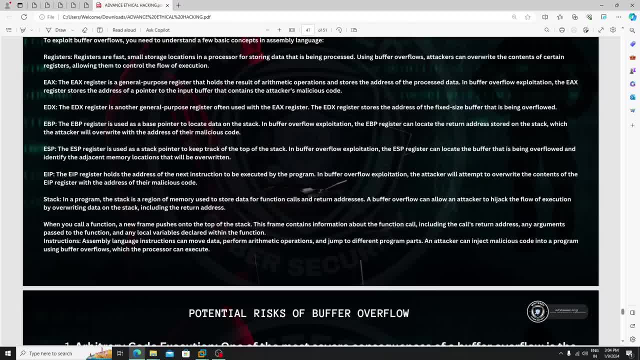 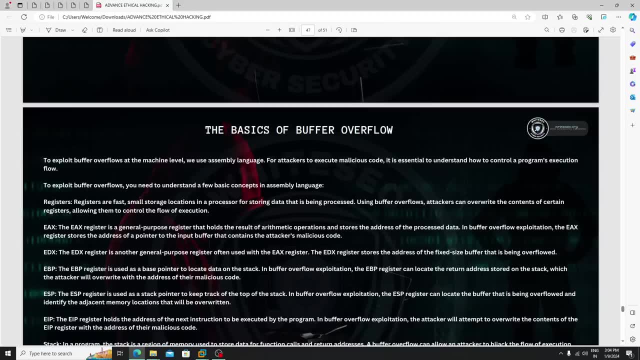 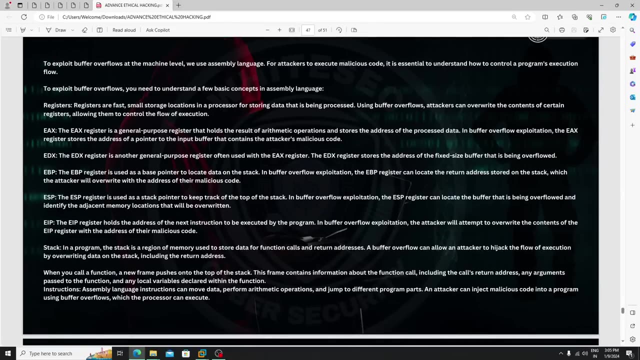 over flowed and identify the adjacent memory location that will be over return. See, let me tell you what. now, maybe you'll be confused. Okay, this buffer, what is this? what is this? each and everything, the simple thing, it's not a big deal. okay, now, see, assume that there is a one input. okay, like, let's take an example of. there is a. 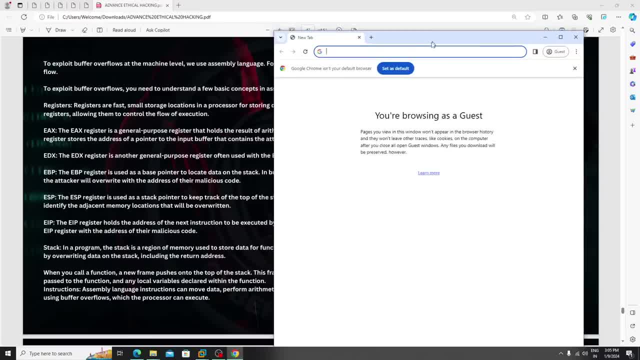 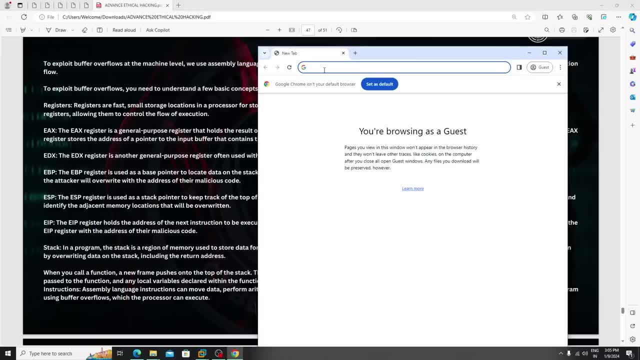 search bar. is that? just assume that this is application. okay, now, here you need to type something. okay, just, i will type something here now. uh, basically, what will happen? means: assume that if i type a huge data here, okay, if i type huge data, then what will happen? uh, it will, it will. 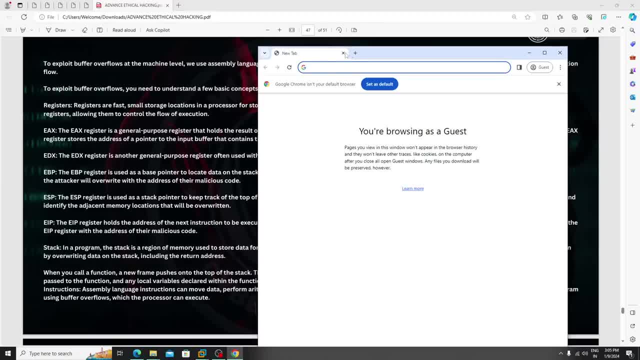 uh, this application will allow it. okay, you, i, if i search a hundreds of thousands of keyword, if i type keywords here, then what will happen? it will search it. it's not a big deal for uh, this application, but there are this kind of applications are there where assume that there is an application? 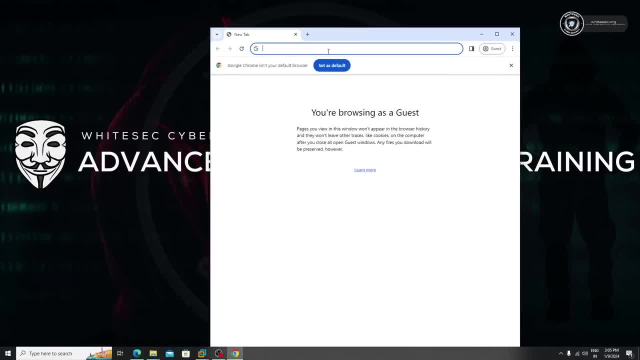 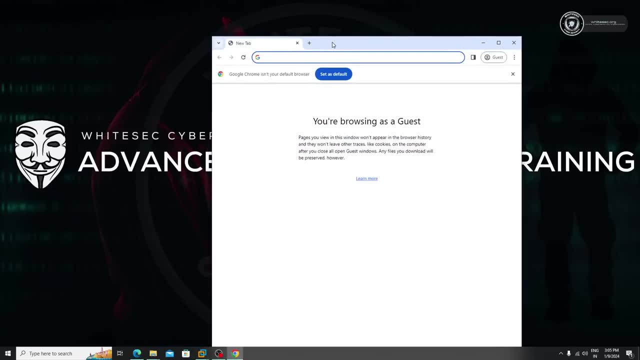 okay, if i type uh about thousand characters here, then what will happen means this one: the application will be get trashed. okay, this is a thing. basically it's known as what buffer overflow here. if the see assume that i am, i am only accepting eight characters. okay, i just coded. 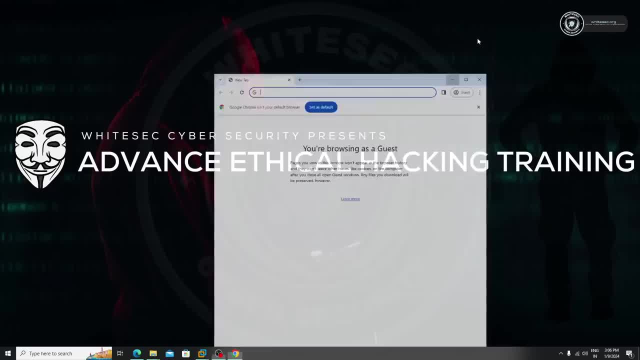 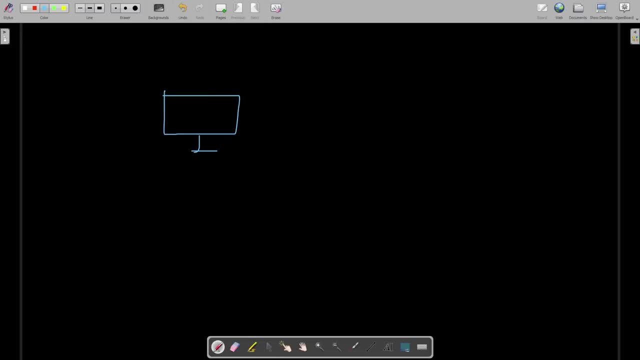 let me explain you here. i just coded one software. okay, now in the software, what will happen means: just assume that this is the sorry. assume that this is a software panel. now, here there is a something like a password field. assume that this is a password field is here here. uh, software is accepting only. 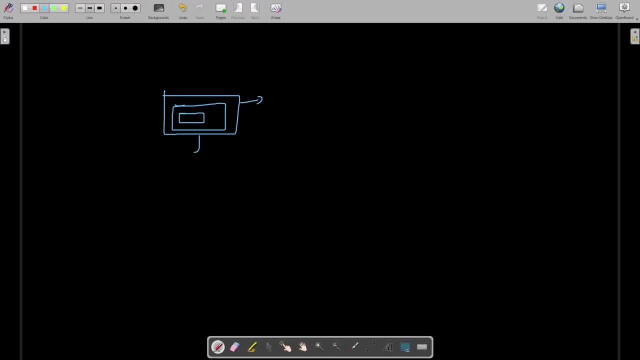 eight characters. just type eight characters here. if we type nine or something like that, it's not accepting that uh thing. okay here. assumed that i just type around thousand characters here. okay, thousand characters, then what will happen? it's not accepting even uh, more than eight here. if i type thousand, then what will happen? the application. 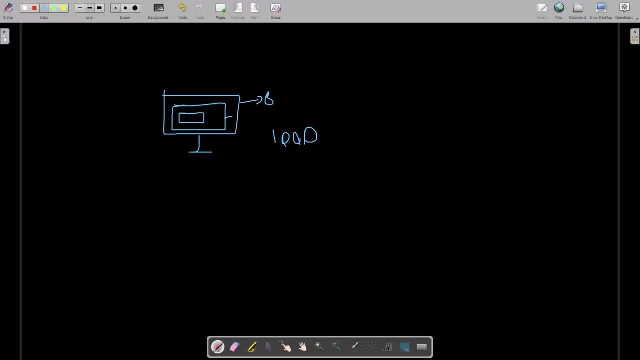 may get crashed. okay, just assume that. uh, let's take an example of if you, if you guys know about apk modding and this kind of stuff. uh, there is a apk. okay, just take any apks. uh, like, uh, any application, android application. see if you decompile that application and if you do any. 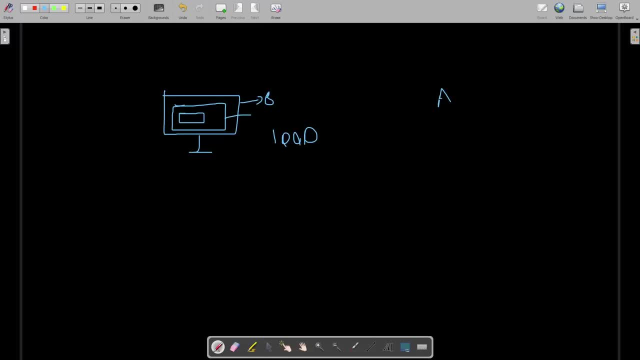 kind of changes, then what will happen? the application won't run there. okay, this is a thing. uh, it will throw some kind of errors, something like that. the same. just take the same scenario as this thing: if you do any changes, if you add a more data, okay, then what will happen? 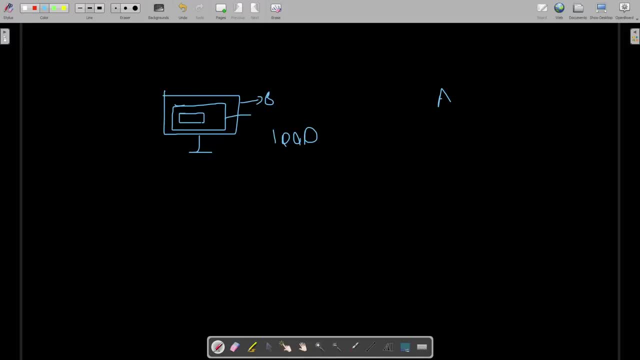 the software will get crashed there. okay, due to this, we can able to inject the malicious codes there. the first point here is: assume that the software is crashing and what? uh, then there is high chances. are there the buffer over of buffer overflow vulnerability? this is a thing. it's not a. 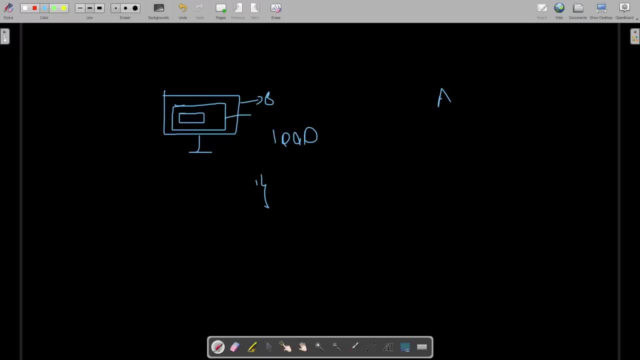 big topic. uh, it's not that much hard topic as well. basically, uh, let me tell you in previous, okay, in oscp, uh, there is a section is related to buffer overflow. okay, right now they just removed it and they added the active directory pentesting, but still lot of students just message these things, okay, like they want to learn exploit. 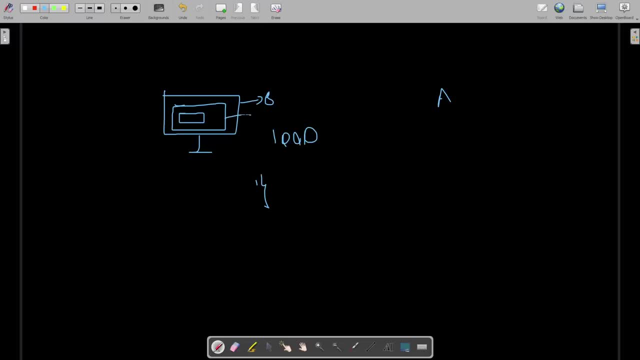 development, this kind of stuff. so that's why we are adding this topic. it's not a big deal because the things are right now. it's it's uh kind of limited. okay, even in companies also, they won't ask to do this kind of pen test here there. okay, this is a thing i am just telling you. reality. 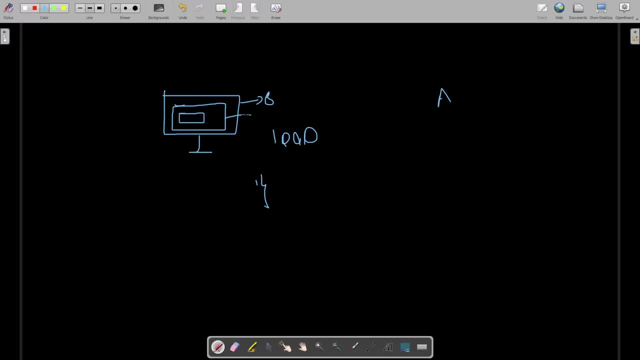 uh, i didn't see these things okay a lot like mostly we we work with active directory and initial assets like this kind of social advanced social engineering techniques like compromising employees, this kind of stuff. uh, shops, i do a lot okay once i uh, if any company hired 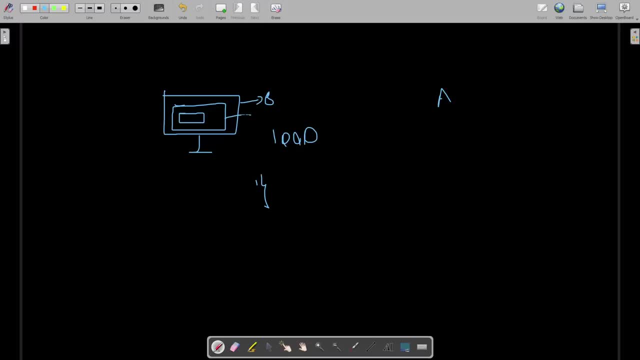 me at that time. my, my work is this thing: okay, like bypassing avs, like i i kind of play uh these things okay, but i didn't see a lot about buffer overflow and exploiting uh this kind of stuff. okay, this is also one thing, but it's important, like if you want to become a good 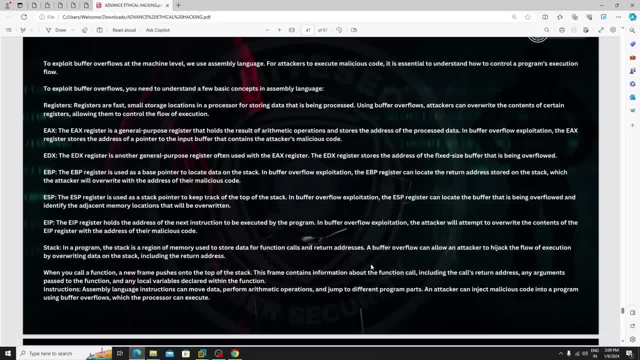 hacker, then you need to learn these things. now. there is a- uh- we just covered about esp, right, and let's uh. there is a eip. the eip register hold the address of next. next instruction to be executed. executed by the program in buffer overflow exploitation. the attacker will attempt to. 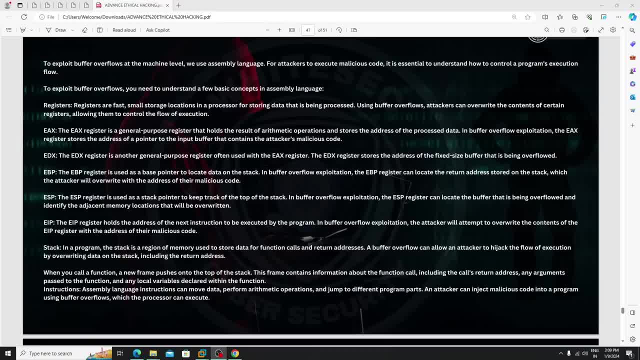 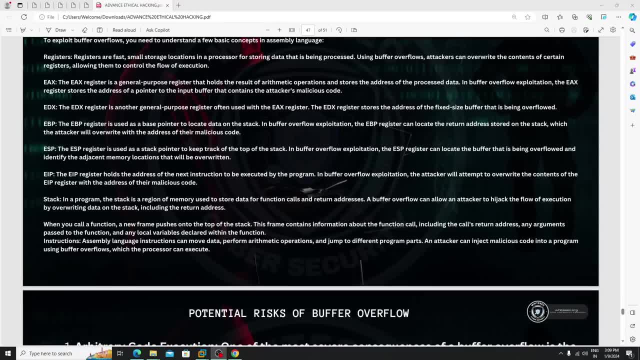 override the content of the eip register with the address of their malicious code. okay stack. in a program, the stack is a region of memory used to store data for function calls and return addresses. a buffer overflow can allow an attacker to hijack the flow of execution. 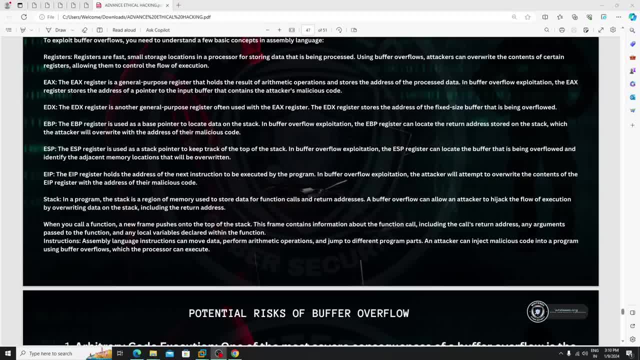 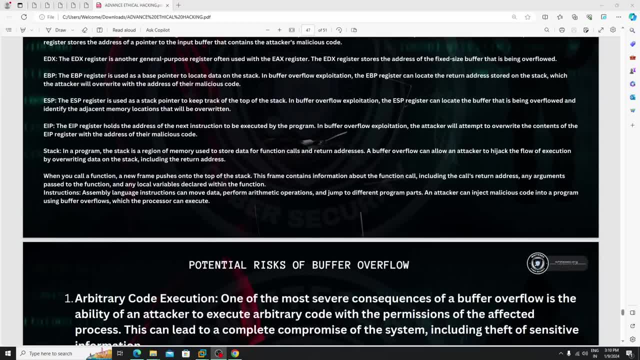 by overriding data on the stack, including the return address. when you call a function, a, a new a frame, a new frame pushes on the top of the stack. this frame contains information about the function cell- sorry function call, including the car return address, any argument passed to the function and any uh local variable declared with the declared within the. 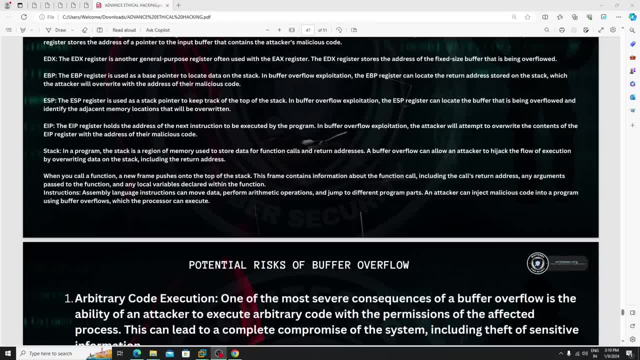 function instructions. assembly language instructions can move data, perform automatic operations and jump to different program parts. an attacker can malicious code into a program using buffer overflow. this is the thing with the which the process can be executed. the main aim of the buffer overflow is what here we are injecting. 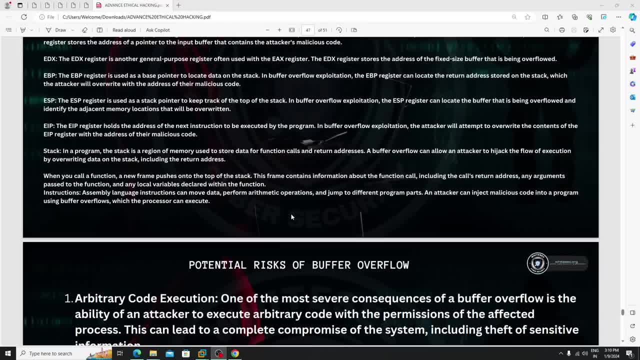 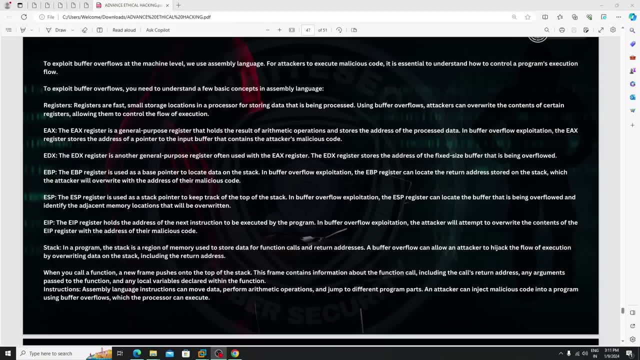 our malicious code in that software. okay, right in the next classes you will learn about potential risk of buffer overflow. see again, i am saying: don't worry about these things, these points, because once we uh open the immunity debugger, there you will see each and everything clearly. okay, it's not a big deal for you, just just try to read it. uh, you will get the pdf link, as i think. 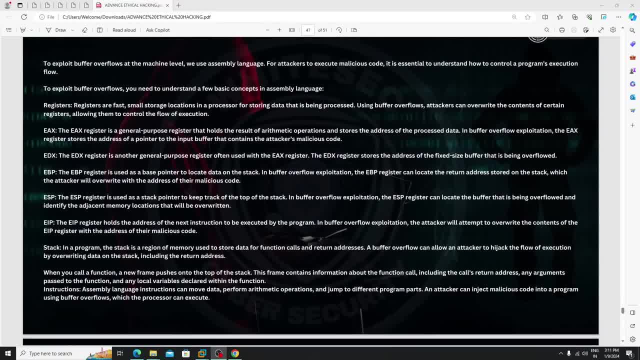 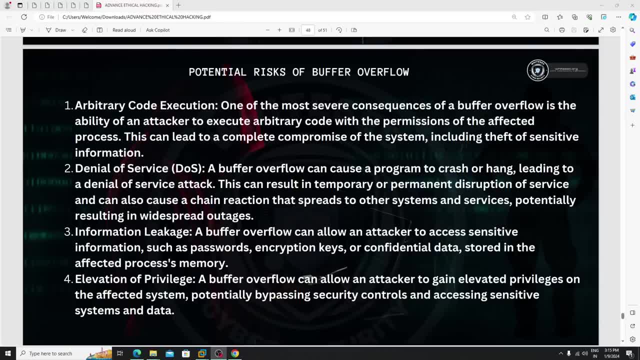 if you don't get the pdf link, just simple contact the support team. they will share the drive link, okay. potential risk of buffer overflow- arbitrary code execution. one of the most similar consequences of a buffer overflow is the ability of an attacker to execute arbitrary code with the 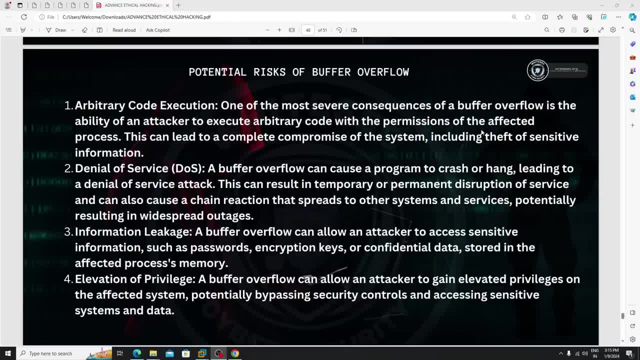 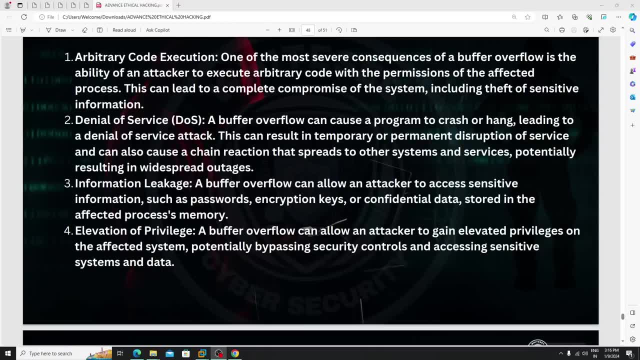 permission of the affected process. this can lead to complete compromise of the system, including theft of sensitive information. there is denial of service dose. a buffer overflow can cause a program to crash or hang- we just covered this thing as well- leading to a denial of service attack this. this can result in temporary or permanent disruption of service and can also 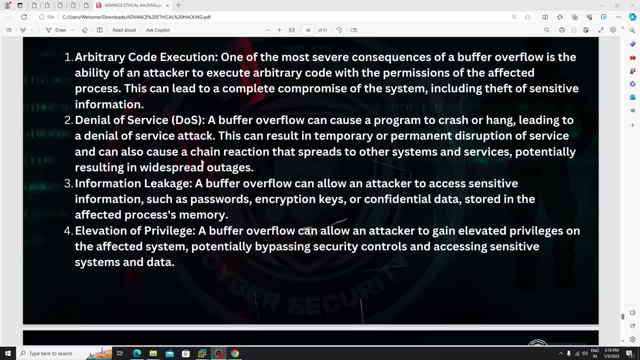 cause a chain reaction that spread spreads to other systems and services, potentially resulting in spread outages. now there is also information leakage. a buffer overflow can allow an attacker to access sensitive information such as password, encryption keys or confidential data. confidential data is a kind of data which is, uh, private. this is a thing like we can't able to share that data with. 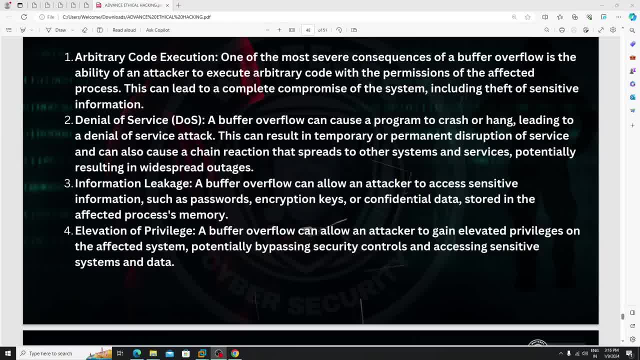 anyone. okay, it's a highly confidential, like there is a credit card information or a company database. like the users- there is a sales team, their leads, this is these things stored in sorry guys stored in the affected process memory. elevation of privileges: a buffer overflow can allow an attacker to gain elevated 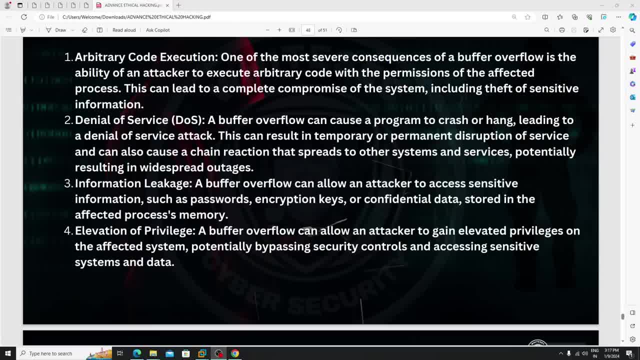 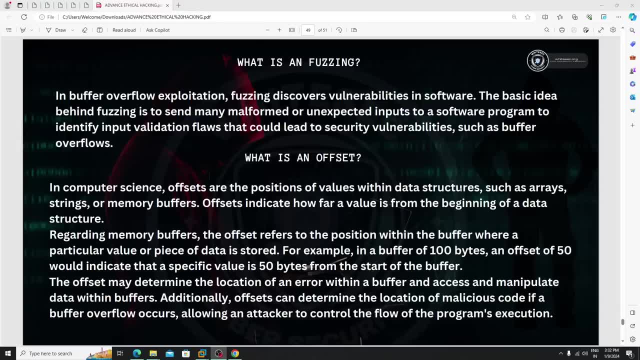 privileges on the affected system, potentially bypassing security controls and accessing accessing sensitive systems and data. so this is the risk of buffer overflow now in this classes we talked about fuzzing and offset in buffer overflow exploitation. fuzzing discovers vulnerability in software. the basic idea behind fuzzing is to send many malformed or unexpected in inputs to a. 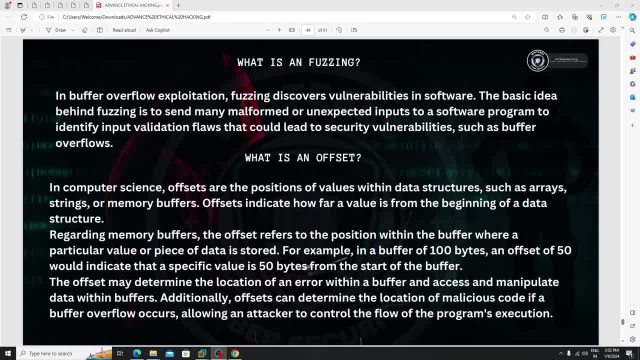 software program: software program to identify input validation flaws that could lead to security vulnerabilities, such as buffer overflow. now here the fuzzing. let me tell you in a very easy way what is this fuzzing? see, in fuzzing what will happen means we also don't know which value will work. 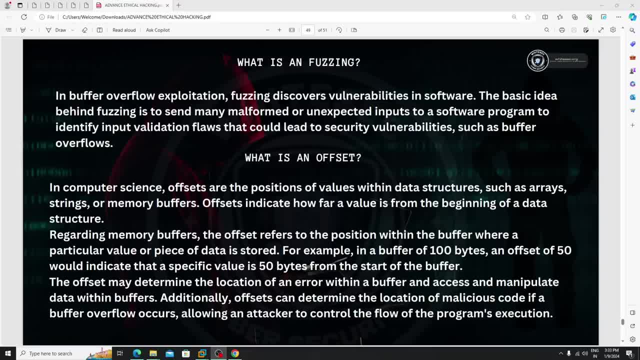 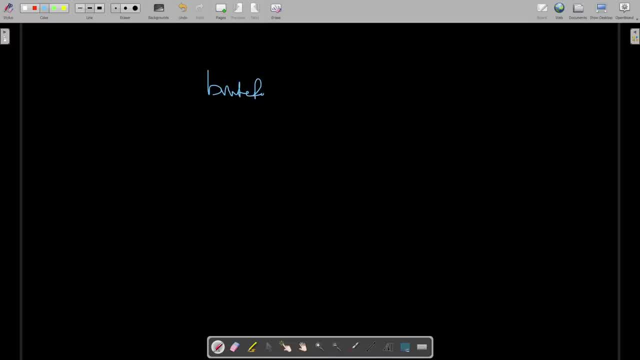 okay, just just take an example of brute force attack. okay, brute force attack. what we do? we just generate a word list. right, we generate the word list and we just perform the brute force attack on it. we don't know which one will work. okay, if it's work, then we will get the output. okay, this? 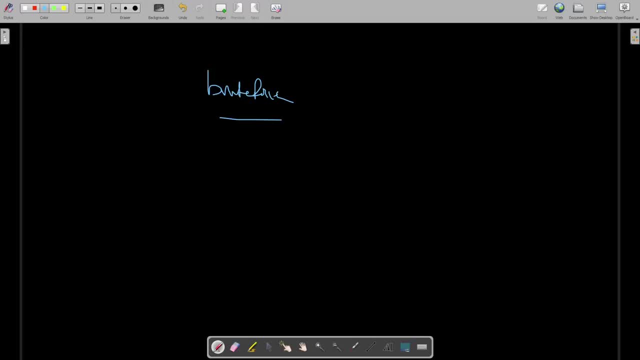 password is right for this username, like that. okay, basically, here in fuzzing, what we'll do means we continuously, uh, perform kind of brute force attack there. okay, we also don't know which one, uh, which one will work. okay, this is the thing. it's a nothing, it's a fuzzing. okay, in a simple, let's. 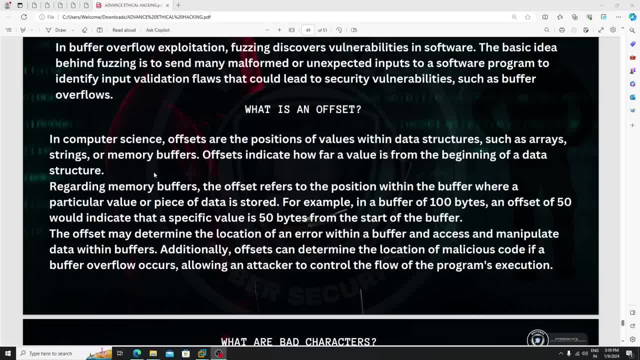 learn about offset. in computer science, offsets or the position of values within data structures such as arrays, strings or memory buffers. offsets indicate how far a value is from the beginning of a data structure. regarding memory buffers, the offset refers to the position within the buffer where a particular value of p 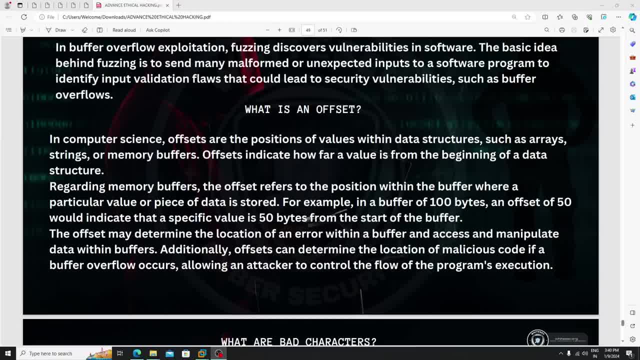 of data is stored, for example, in a buffer of 100 bytes, and offset of 50 would indicate that a specific value is 50 byte from the start of the buffer. the offset may determine the location of an error within a buffer and assist them. assist and manipulate data within. 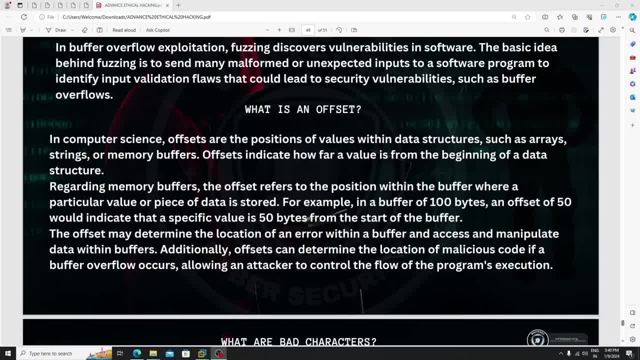 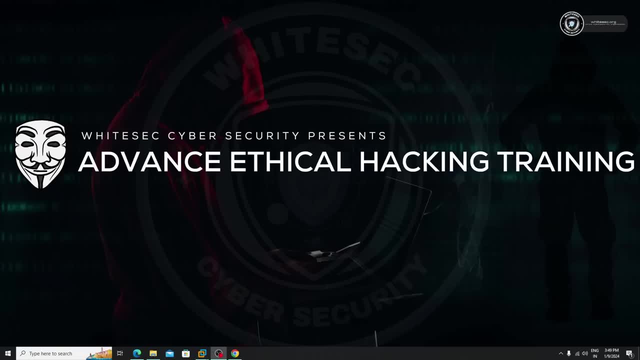 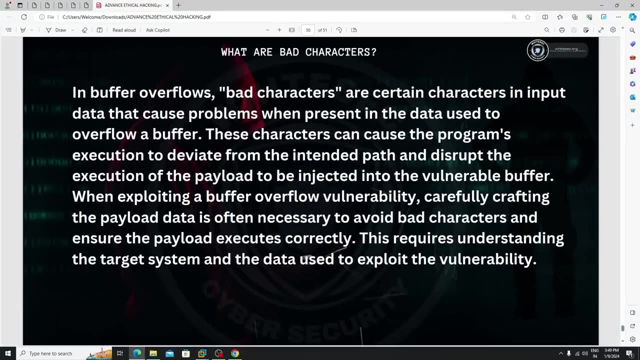 buffer. additionally, a offset can determine the location of malicious code if a buffer overflow occurs, allowing an attacker to control the flow of the program execution. so this is known as what offset. now in this class we are learning about bad characters. what are bad characters in buffer overflow? bad characters are certain characters in input data that cause problems. 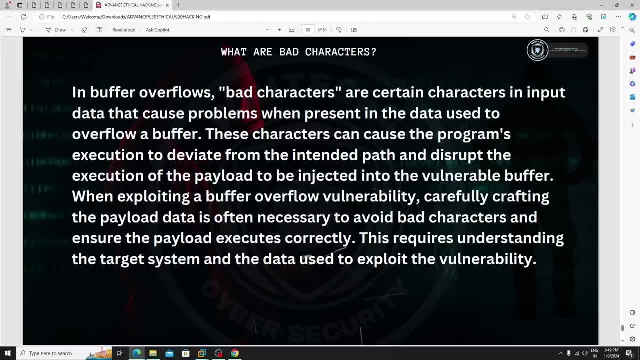 when present in the data used to overflow a buffer. these characters can cause the programs execution to deviate from the intended path and disrupt the execution of the payload to be injected into the vulnerable buffer. when exploiting a buffer overflow vulnerability, carefully crafting the payload data is often necessary to avoid bad 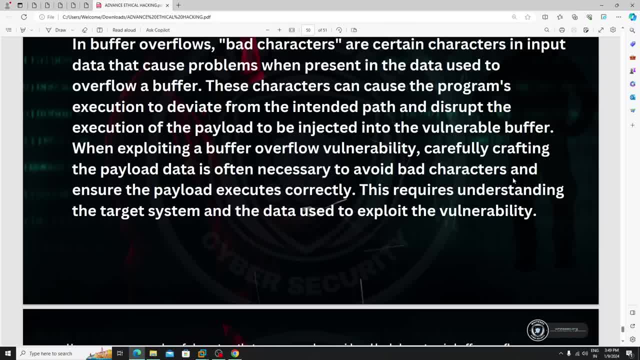 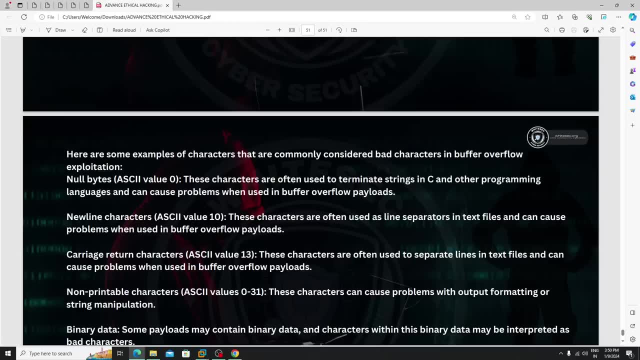 characters and ensure the payload execute correctly. this requires understanding the target system and the data used to exploit the vulnerability. now here are some examples of characters that are commonly considered bad characters in buffer overflow exploitatively. the first one is the Ethos formula, which is used to perform the execution of the pay load coherently. 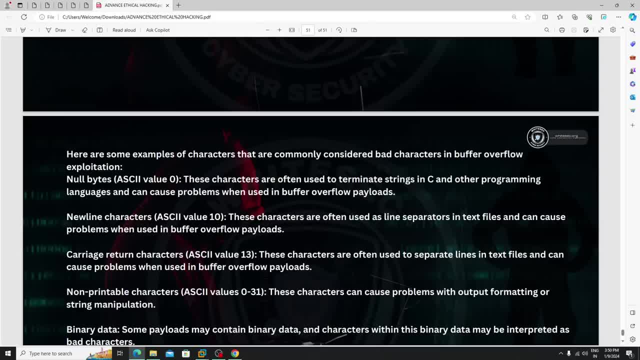 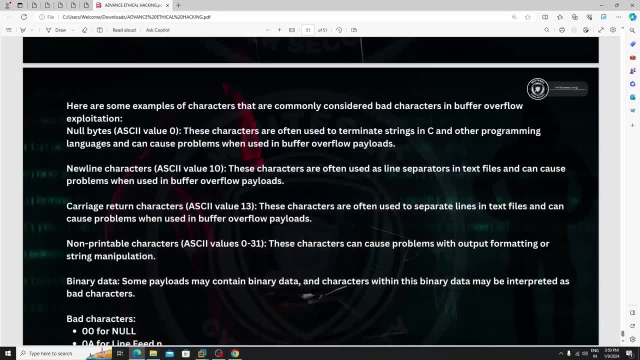 exploitation. now the thing is. just open this website. okay, let me show you again. here is a website. now just see null byte. ascii value 0. these character are often used to terminate string in C and other programming languages and can cause problem when used in buffer overflow payload. now, what is ascii value 0 here? what is ascii value 0? just see 0, just. 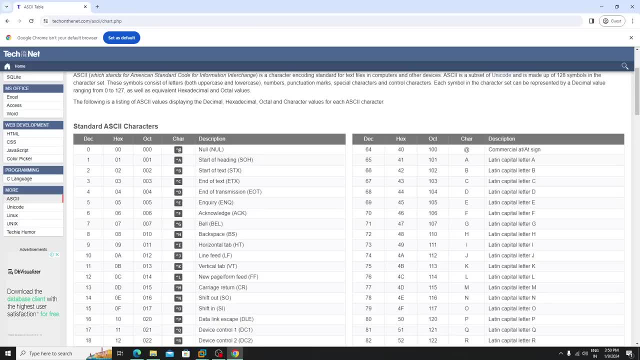 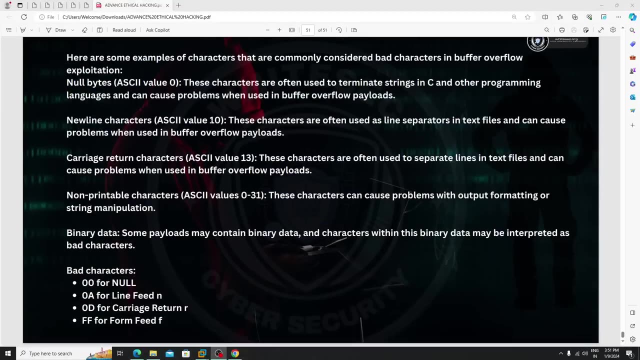 wait, man, it's null here. okay, 0 is what null here, which is comes under. you just need to take it as a hex. okay, which is 00, right, and new line characters: ascii value 10. now, what is ascii value 10 here? 10 is 0a. 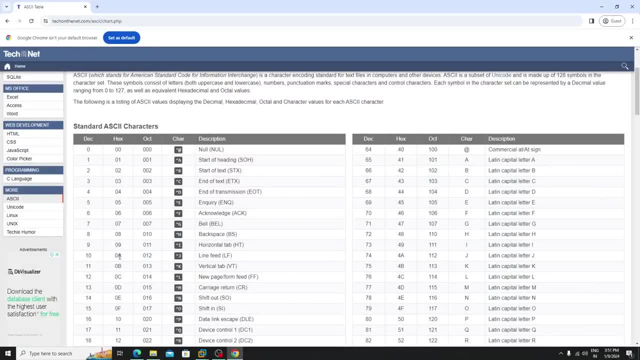 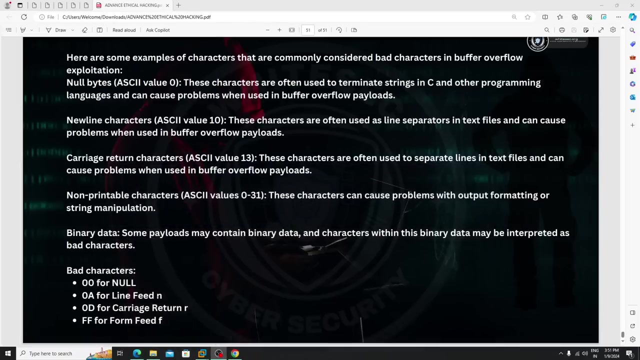 okay, 10 is what here? 0a you need to see in hexa format. okay, this is a thing. 0a, see 10 and 0a. which is what line feed lf? you also need to check the description here. also added 00 for null, 0a for line feed n. 0d for carriage return, return r. ff for the form feed, f something. 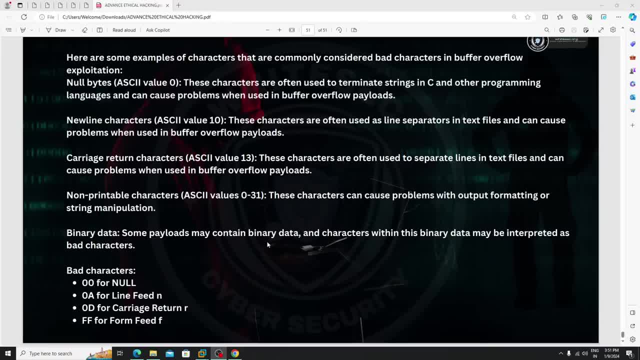 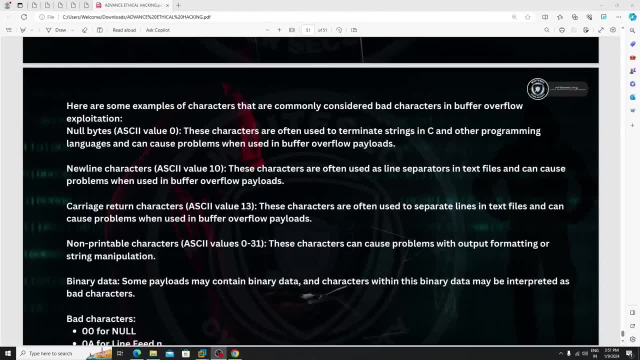 like that. okay, but still just use this chart as well. okay, which is easy to understand. now, new line character, which is ascii value 10. these character are often used as a line separator in text file and cause and can cause problem when used in buffer overflow. payload carriage return. 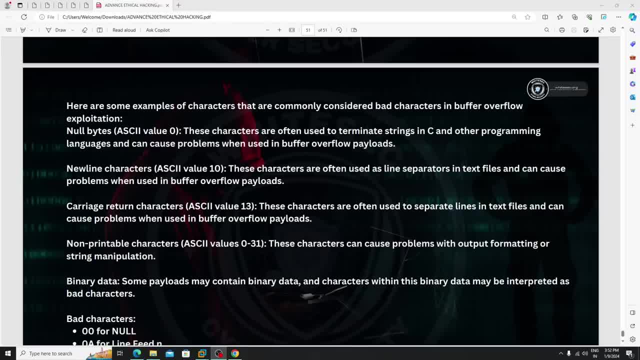 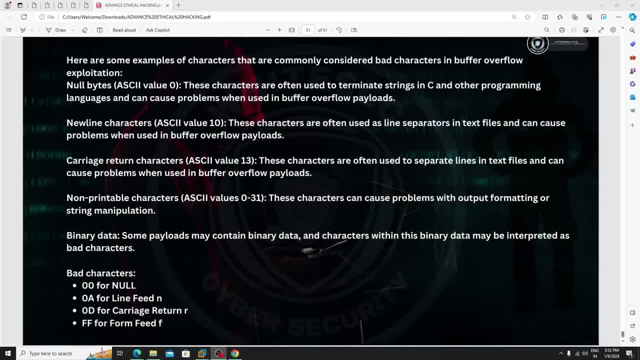 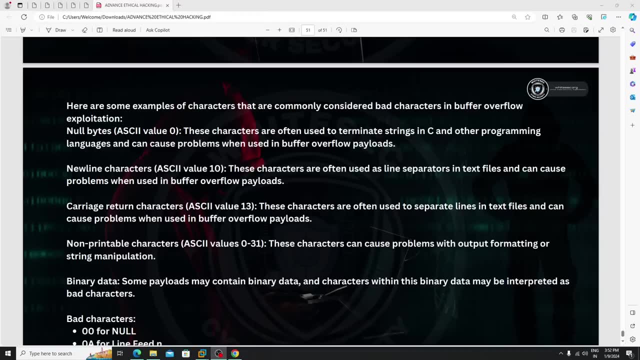 character ascii value 13. what is ascii value 13? here it says 0d. right, so here it is. it's a 0d for carriage return. this character are often used to separate lines in text file and can cause problems when used in buffer overflow payload. basically, the thing is just. 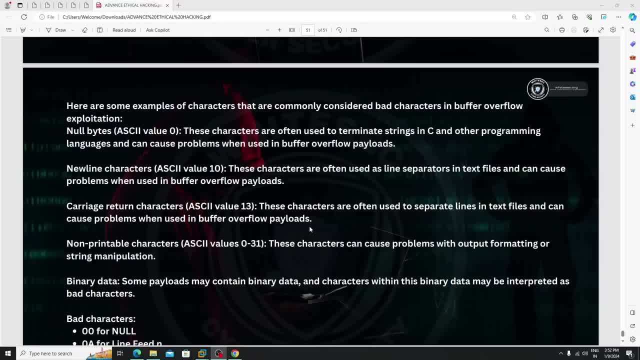 assume that in payload we are avoiding the spaces. okay, which is you can also say it as a space man- when you type the space bar, right the space. basically you are avoiding the space here. it's not a big deal. okay, now here. non printable characters. ascii value 0 to 31: okay. 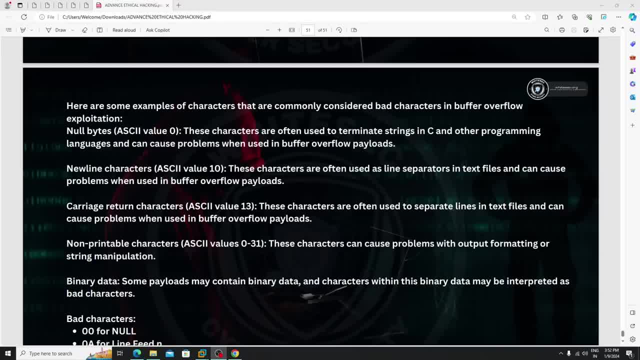 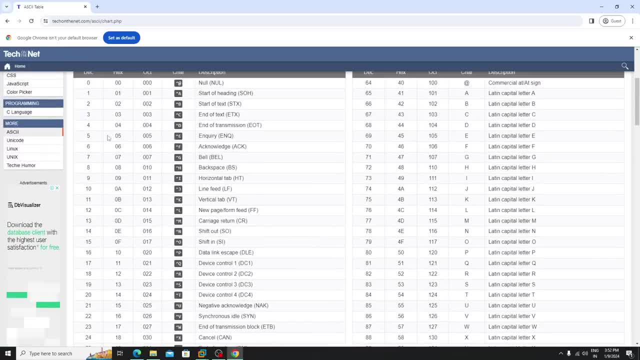 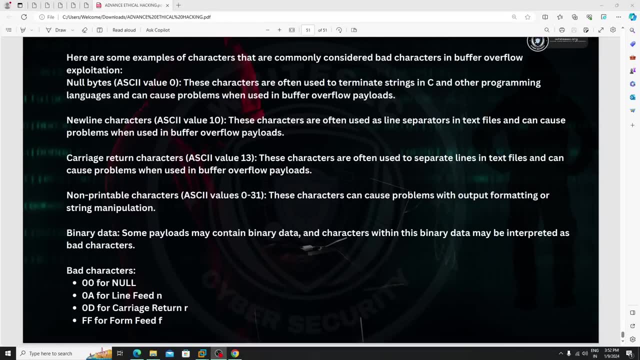 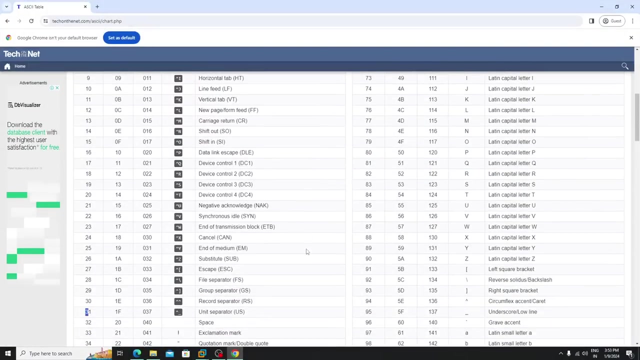 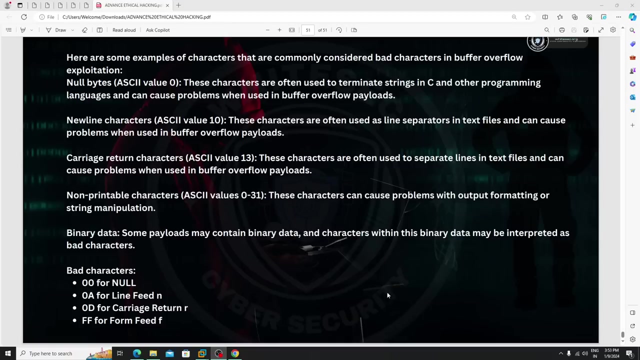 what is this? 0 to 31 here. just take from here to 31 here. okay, 1f from here to here. from 0 to 31. this character can cause problem with output formatting or string manipulation, or, here, binary data. some payloads may contain binary data and characters within the within. 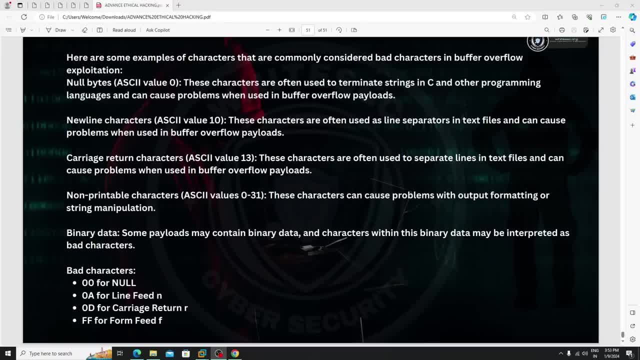 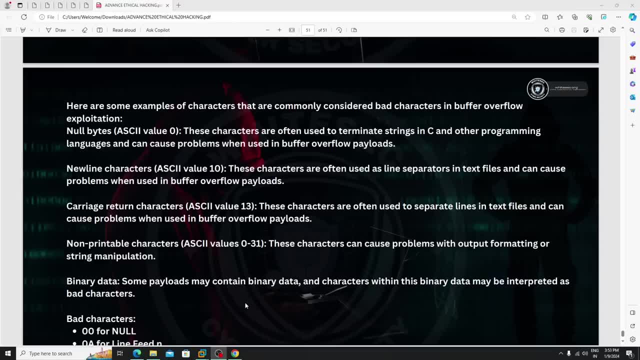 this binary data, maybe interpreted as bad characters. here you can see these things which we just covered, right? basically, you need to avoid zeros here. this is the thing. okay, if you see 0, 0 here: 0, 0, 0, no, no, no, this is the value that you are allowing and we are absolutely. 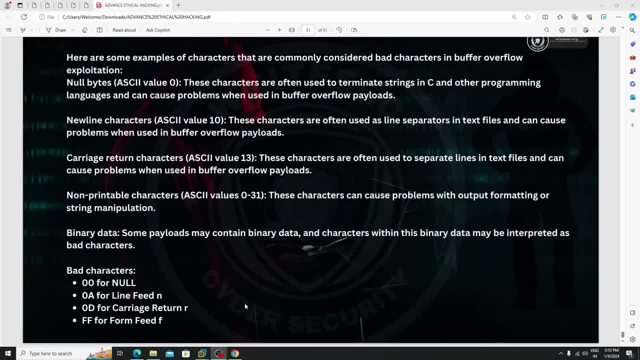 zero, then you need to craft it. this is the thing. so let me show you how we can able to do this practically. it's not a big deal. again, i am saying just the thing is, if you are not getting this class as well, you need to execute the same command, same things, which i am doing here. if you are not, 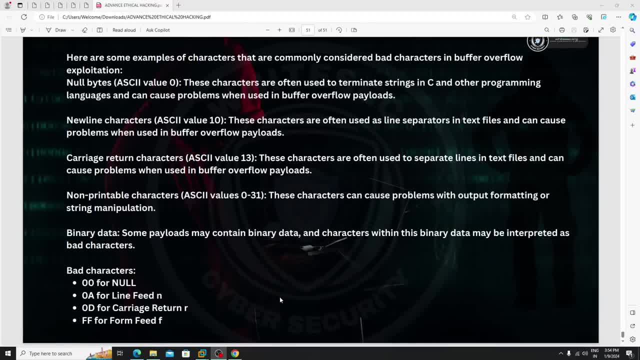 getting this as well. you need to practice it, just watch it and execute it. this is your work. okay, right. in the next classes we are starting the practical right: how we can able to do it right. okay, so, guys, hope you are fine. in this class we will learn how we can able to perform. 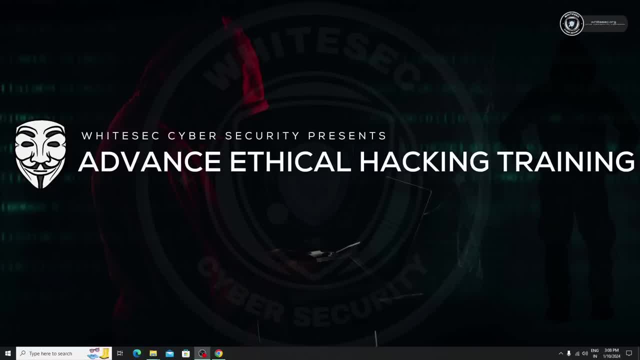 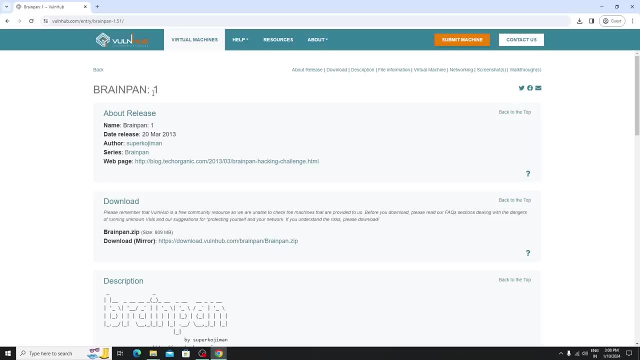 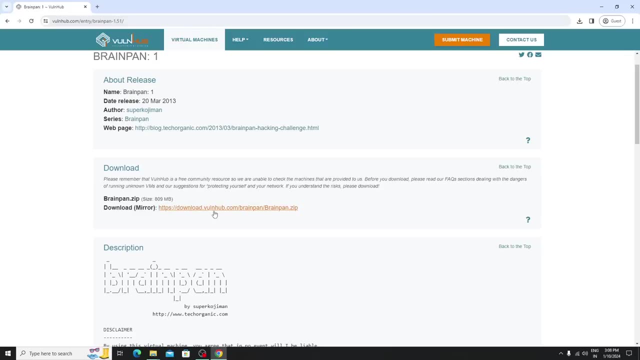 buffer overflow attack. whole thing is, first of all, you need to download a lab here. simple: just search brain pan one, and here you can able to see one hub url. just just visit this url and download this file, which is around 809 mb. see, i already downloaded this one, so let me show you. 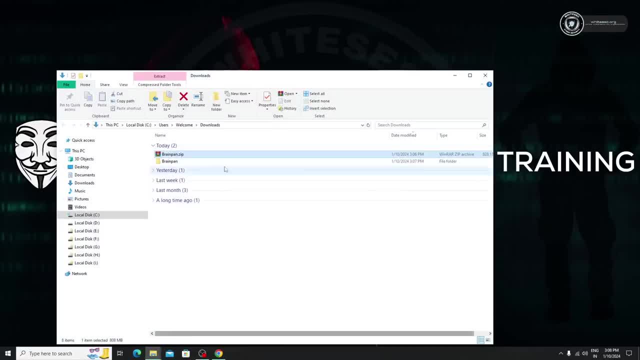 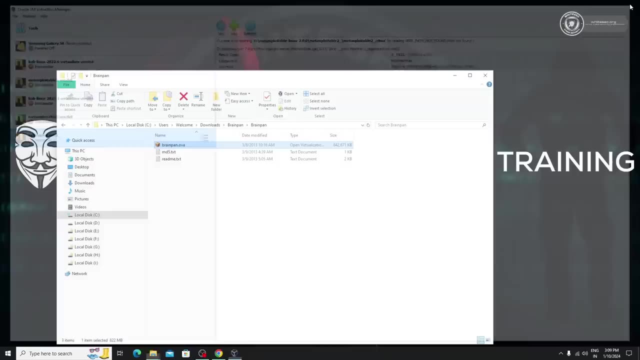 so here it is simple, extract it right. and here there is a brain pan, dot ova. simple double click it. so it's opening in a virtual box- simple. if you want to run this in vmware, simple just click on open with and just select vmware workstation here. 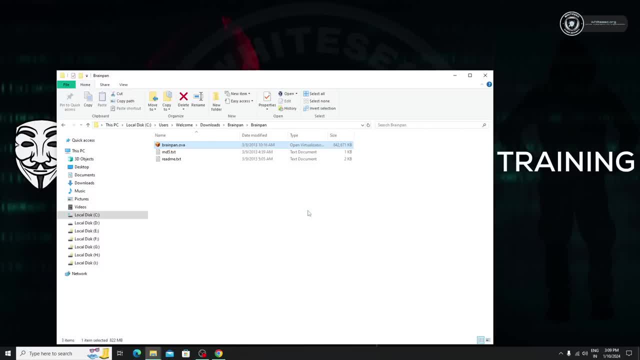 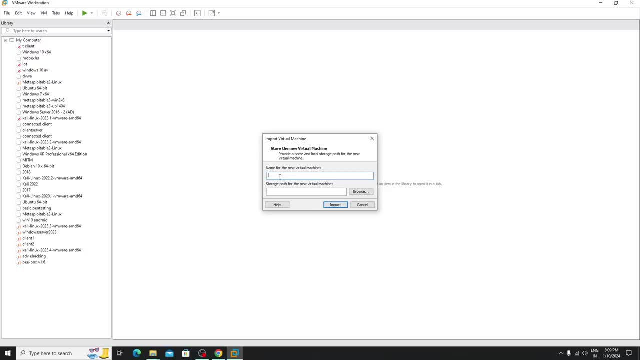 so just give the name. let me give the name as a buffer overflow storage path for the new virtual machine. let me select d drive here. simple click on import will take some time. just wait. now the thing is, guys, you just need to remember this words because once you watch this class it might be confusing for you. don't worry, just do and execute the same. 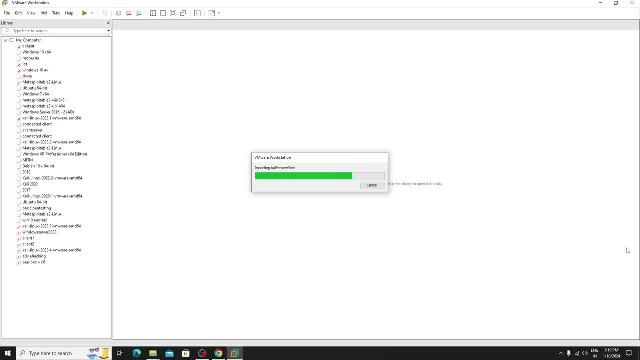 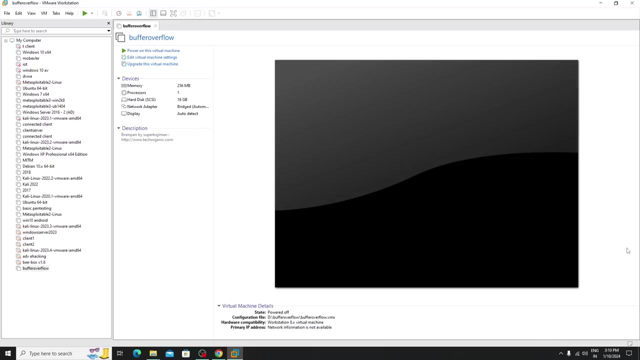 commands, which i am doing here: your system, setup the lab and practice it. if you are not getting it, uh, also just try to uh practice it, because buffer overflow and exploit development. these topics are little bit confusing. okay, not little bit. it's a huge confusing thing sometimes, okay, but you no need to worry here, because the 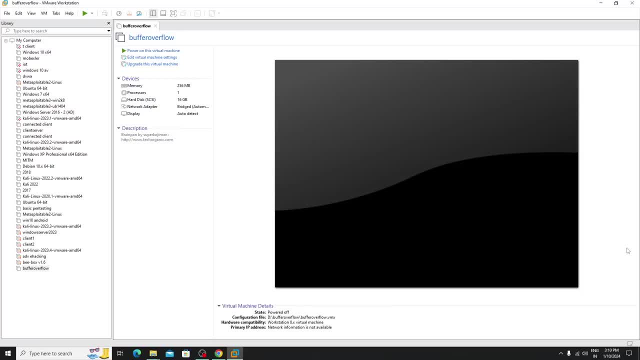 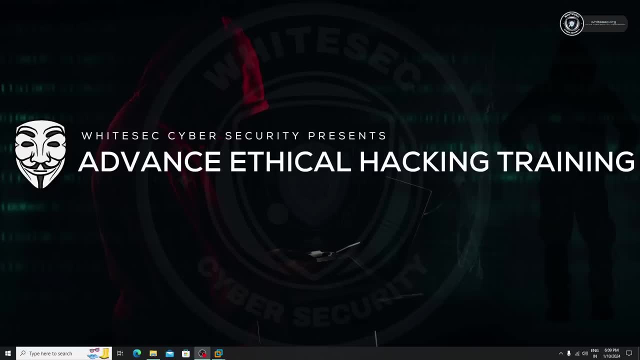 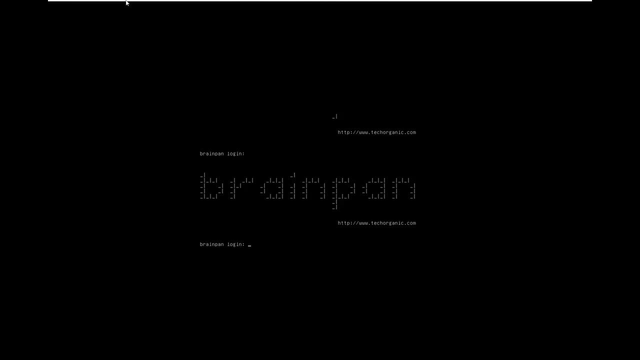 things are: once you jump practically, the things will become easy for you. okay, let's perform some practical attacks here. so this is our vulnerable machine, which we just downloaded in the last classes. right now, simple, just do this, this thing like click on vm and just click on settings. 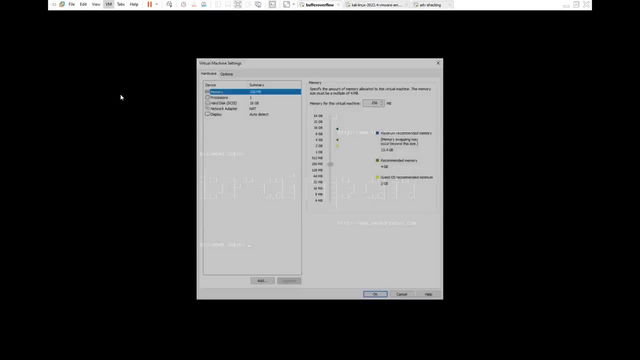 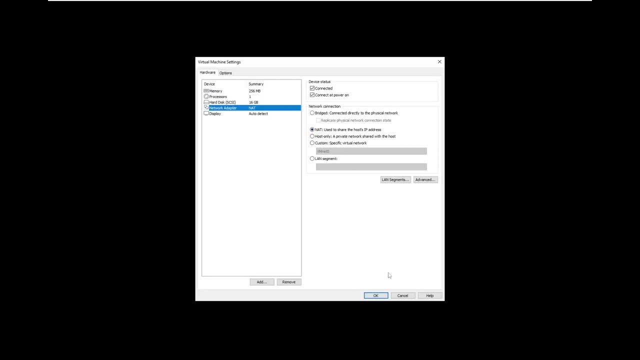 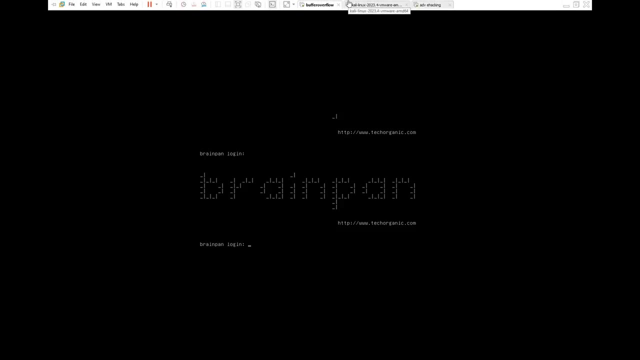 here and change the network adapter to not. maybe in your case it's it might be bridge. okay, just change it to not. if it is not in not network in this network, then what will happen? we can't able to scan it. okay, because the thing is, we are created the lab here, right, so everything comes. 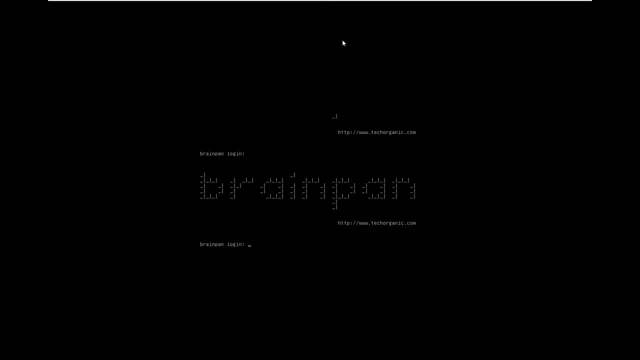 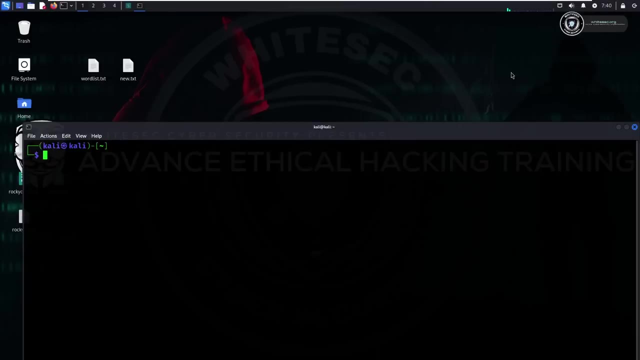 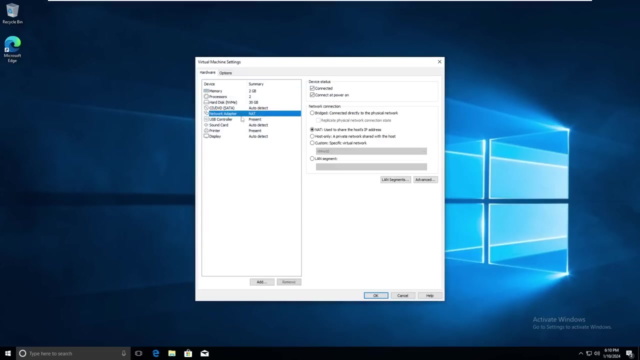 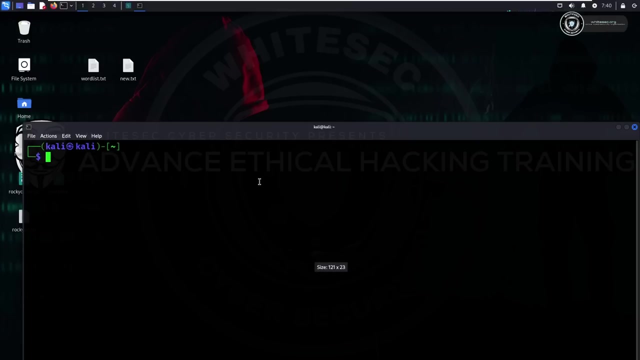 under in one our network. so that's why you need to set up this in a not network. okay, because our kali machine and our windows machine also running in not network. okay, just let me show you. so here it is. now the thing is, let's perform nmap scanning here. first of all, let me see my ip address, just 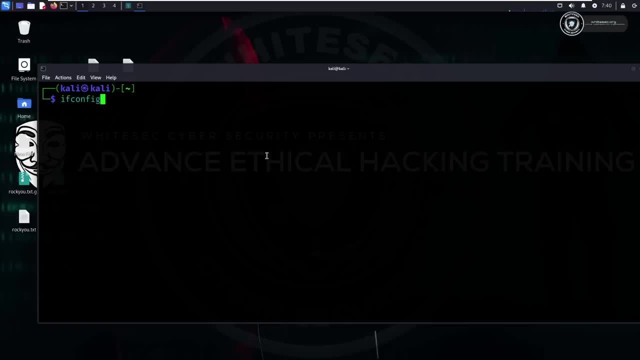 type here: ifconfig. this is my ip. okay, this kali machine ip. let me clear it and just run nmap scan here. nmap dash sn. so let me see how many devices are there in my network. okay, mostly students are getting kind of error in net discover. so instead of net discover you can also use nmap here. 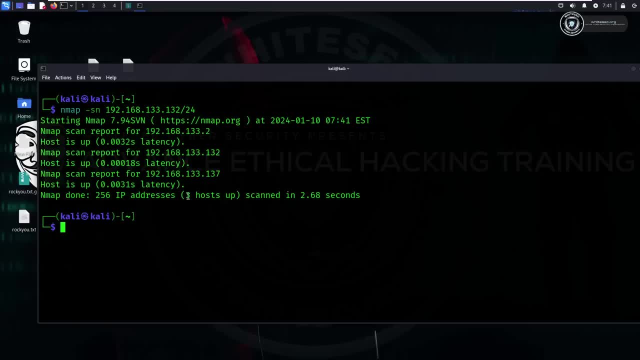 so here are the devices. this is the kali ip right and this is my router ip and this is the vulnerable machine ip address. i think so. let me perform os detection here in map and dash capital o ip address here. see: whenever you are performing the os detection, just run it as sudo there, because for os detection you need to. 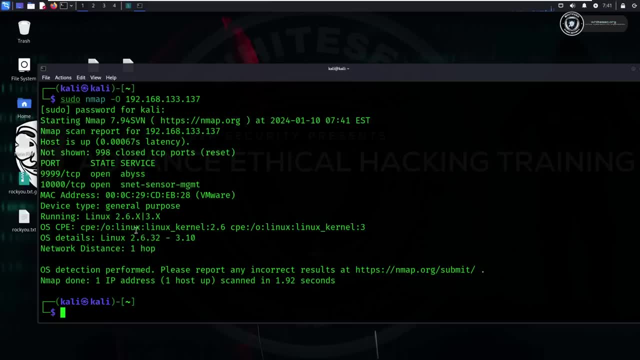 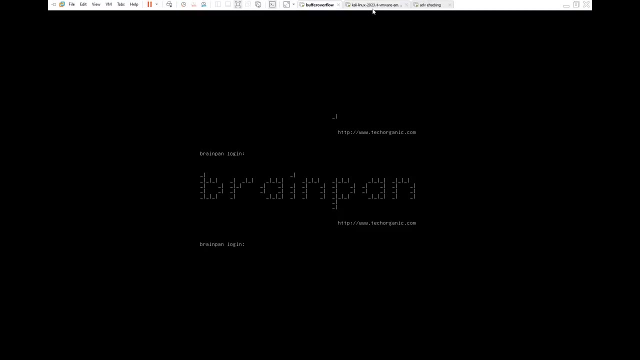 run it as a sudo. now the thing is it is a kali based machine. it's a sorry, it's a linux based machine. the version is this: okay, right now i got the complete idea that, okay, this is my target because this is a linux based machine. right? so this is the thing. and here, just see, there is a. 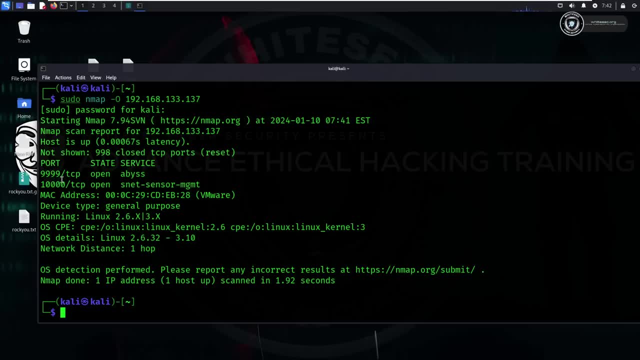 two ports over there, like one is uh, double nine, double nine and uh, and the second one is ten thousand. so basically, remember one thing, guys: here this software is running on a sudo, so this is the software you use, uh, set up this ports manually. they are not using the by default ports here. 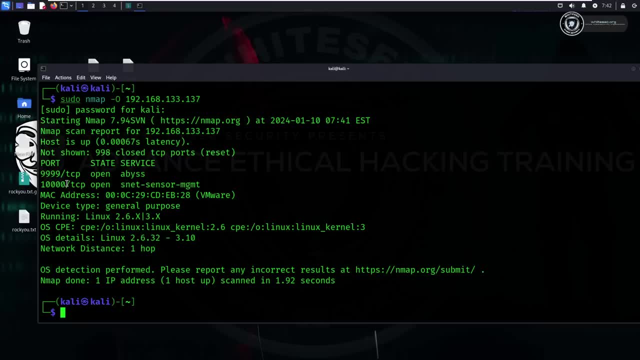 okay, this is the thing. yes, you can. whenever you are set up in any service, assume that you are set up in a sss service in your system. at that time you can also change the ssh port to any port. okay, like a by default ssh port. is what 22 right? so the simple thing is, you can also. 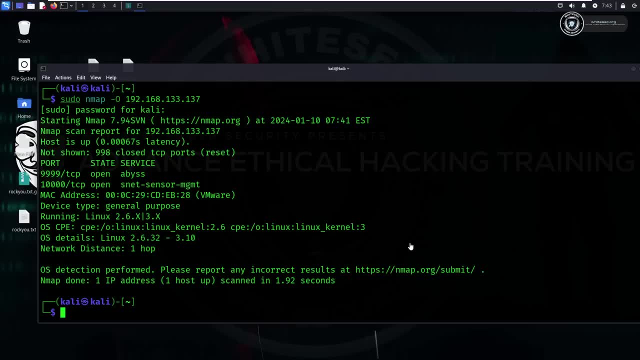 change it to your desired port. okay, this is the thing. now here, let me perform the service version detection as well and let me scan for all open tcp ports. so it will take some time, just wait. now here you can able to see the results. okay, the thing is. 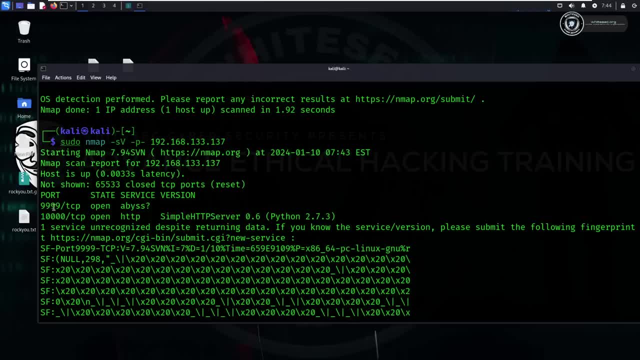 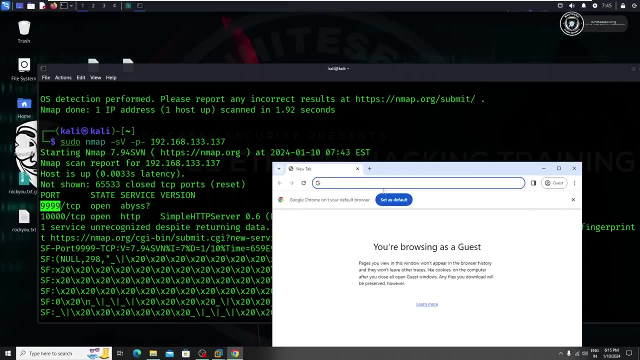 vote. 99 is using vs. basically it's nothing, but it's a web service. okay, now, simple, let me open this in browser. what is your target ip? 192.168 point, 192.168.1 point, oh sorry, 133.137. right now, simple, just add the port as well. what is the? 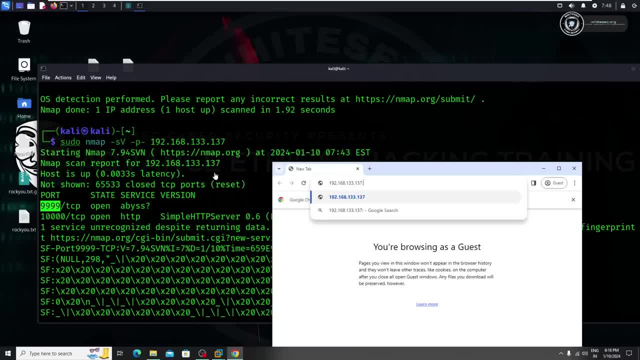 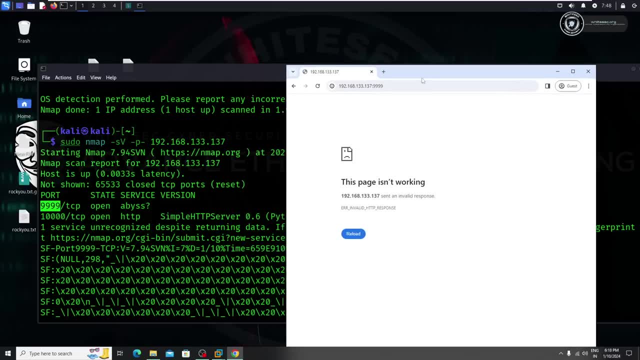 port: double line, double, uh, double line, right, so there is nothing here. you can open this in browser and open this in browser. open this in browser and open this in browser, right? so this is also a web server. let me tell you, okay, how you know that this is a web server. 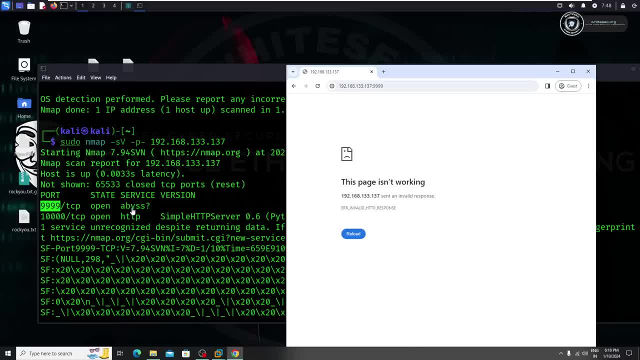 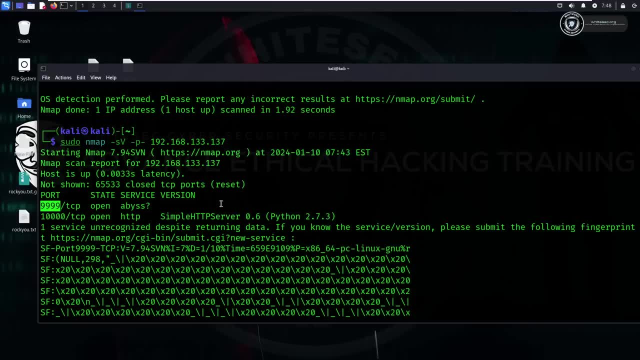 simple by seeing the service name. okay, now http is also web server. but here it doesn't show the version. this is the thing. but here, just see in http we got the simple http server 0.6. is there? okay now simple. let me search for uh thousand. here is there any server is running? 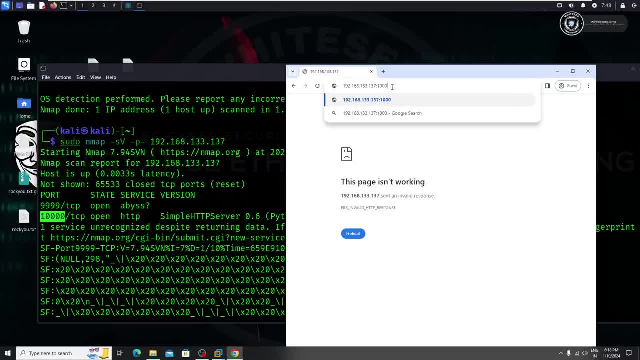 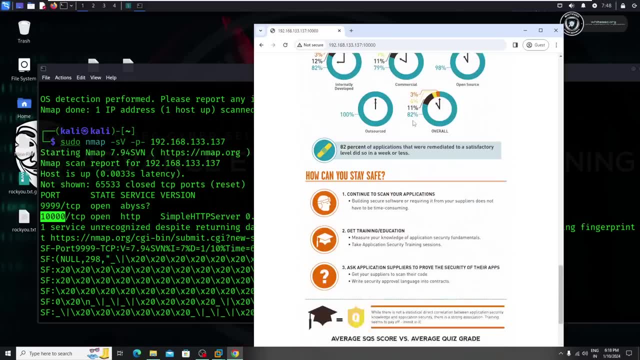 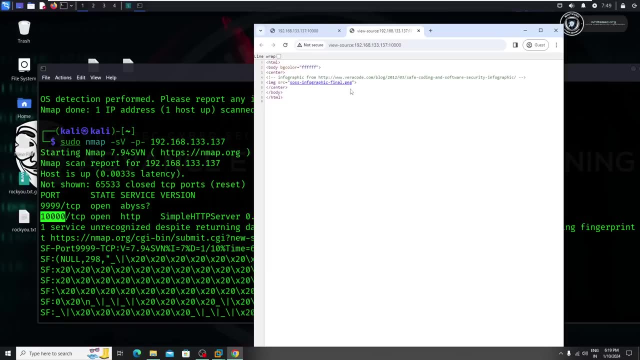 sorry, ten thousand. yes, there is a web server is running here, so this is the. basically, this is a web page. okay, now the simple thing is what you need to do: click on view phase source and just check this. okay, there is nothing right, there is nothing, man. so simple now. if you didn't find, 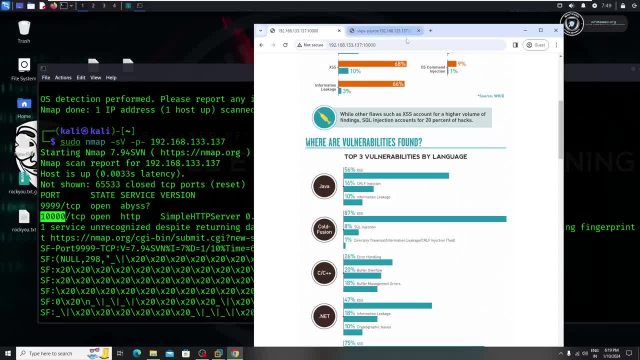 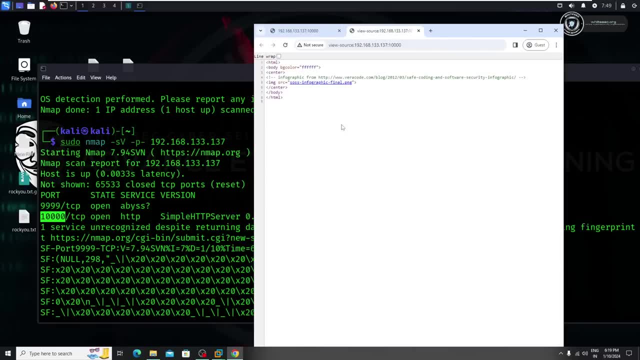 anything in the source code at the time. what you need to do? simple: you need to start the fuzzing here. what kind of fuzzing? like directory brute force attack? now how to do it. so, basically, this is now how to do it, simple thing. just type here: okay, this is a one excellent tool which i 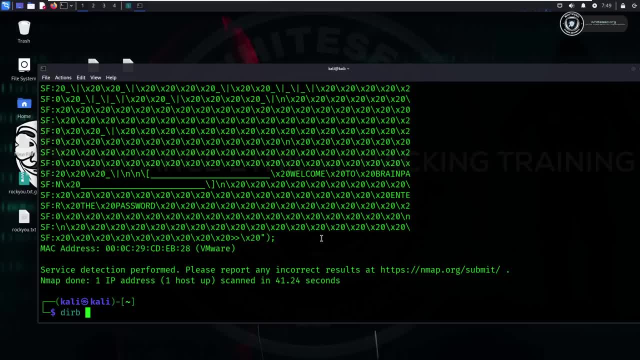 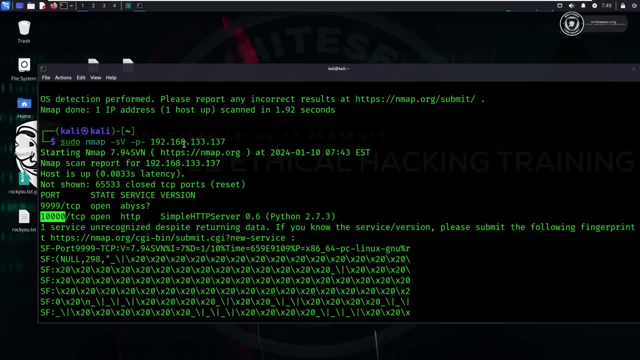 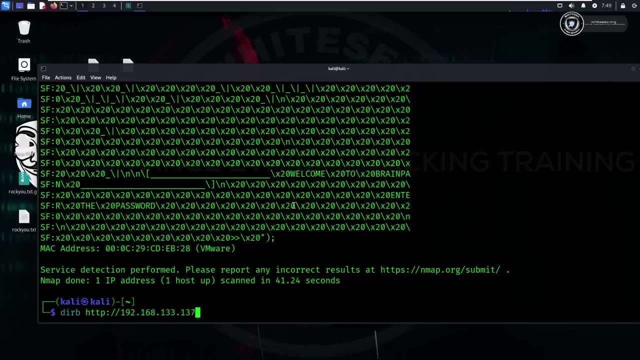 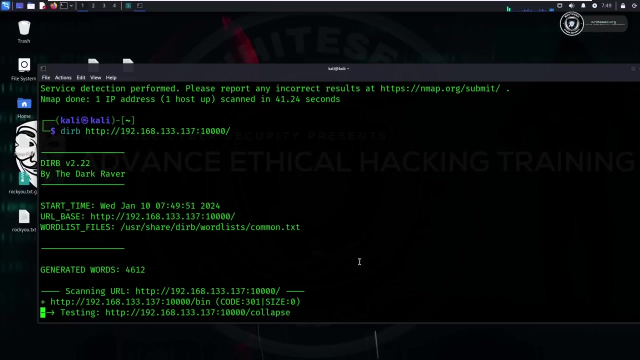 use a lot. okay now, simple: just type here the url, http, your target ip. just paste it here now. just type here the port number: is what ten thousand? right? just type: enter now let's see. so here i can able to see there is a bin and there is a indexhtml, basically. 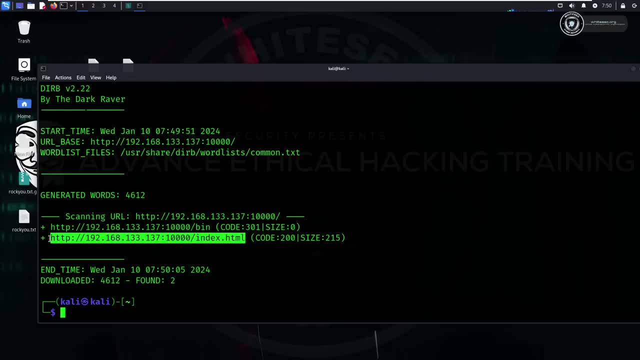 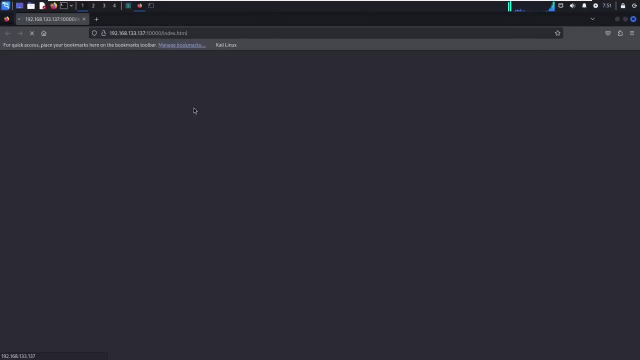 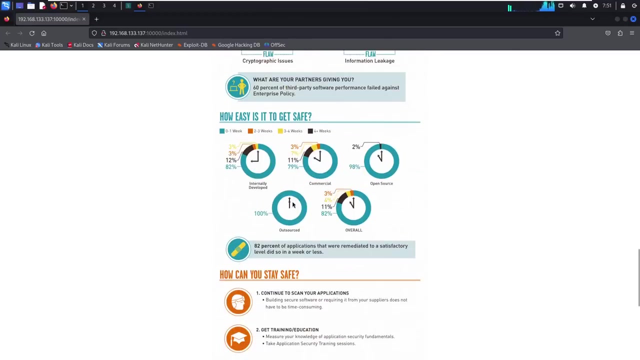 indexhtml is a nothing, but it's a normal one. okay, just let me show you. okay, i can't able to paste it here, let me open this browser only. so it's a normal index page, the same thing which we just saw there, right, and what is a bin? here? i got one another one which is bin. 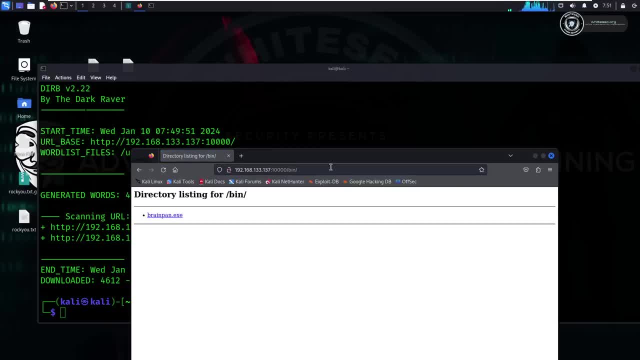 so here i can able to see bin brainpanexe in bin page. the simple thing is: this is a exe, so i need to run this in windows system. this is the thing here, right? so basically the thing here is we need to exploit this exe file. we need to find the 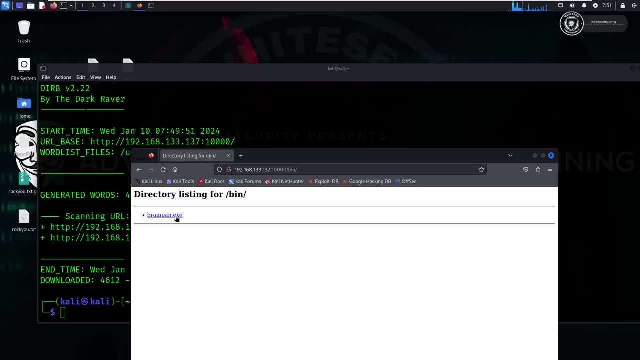 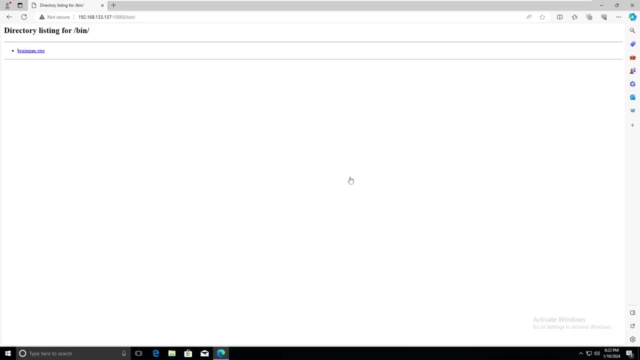 vulnerability in it and we need to exploit this. this is a complete challenge here, so the simple thing is: let me download this one in my windows machine. so let me open the microsoft here. so simple. what i did means i just open that url in this windows machine and let me download this brainpanexe. 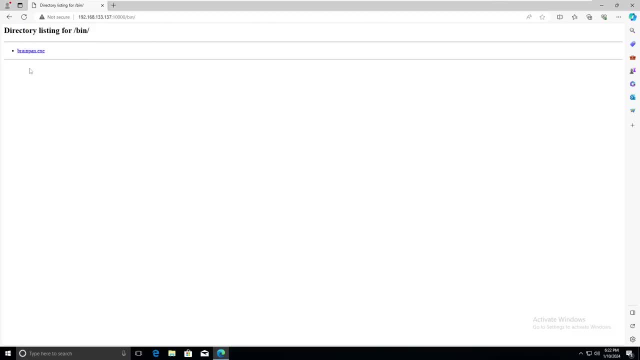 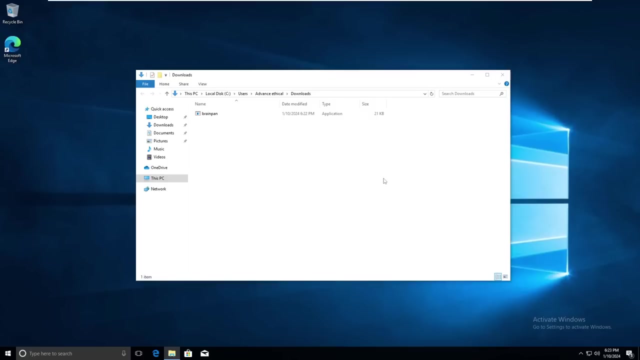 here. so here it is in pandexe, right, this is in download folder, so now we need to install the debugger here, community debugger. the simple thing is: let's see how we can able to install it, and also we will install monapy as well, which is a very excellent tutorial for us. so we need to install monapy and 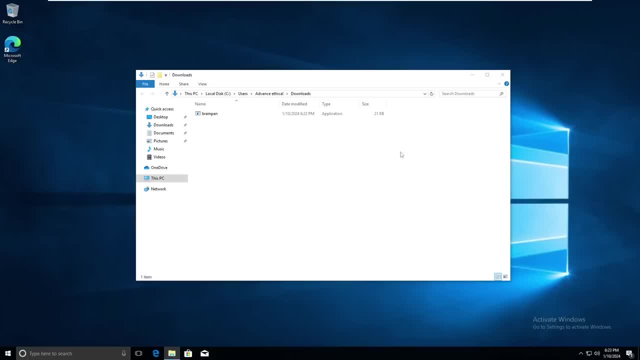 also, we will install my macbook as well, which is a very excellent and very useful plugin for us. so we need to install monapy as well, which is a very excellent plugin for us. so we will install monapy- excellent script, which is very useful for us. ok, so let's see it. now let's download the. 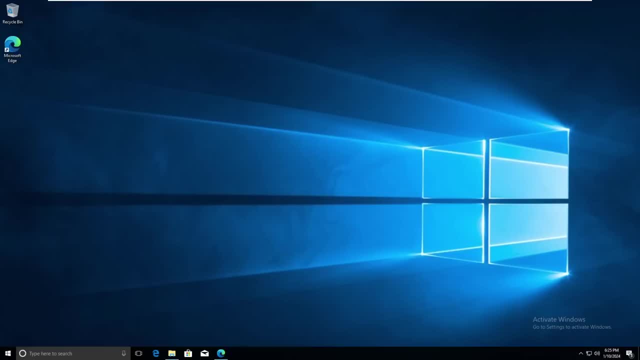 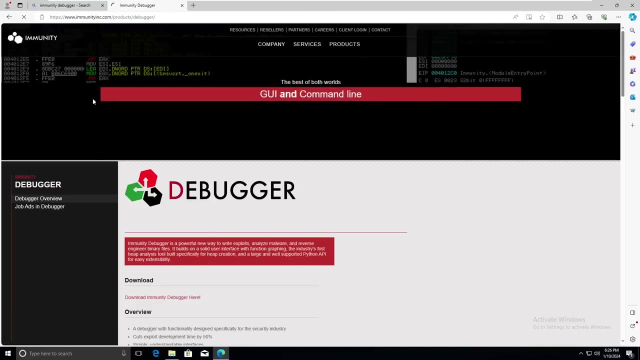 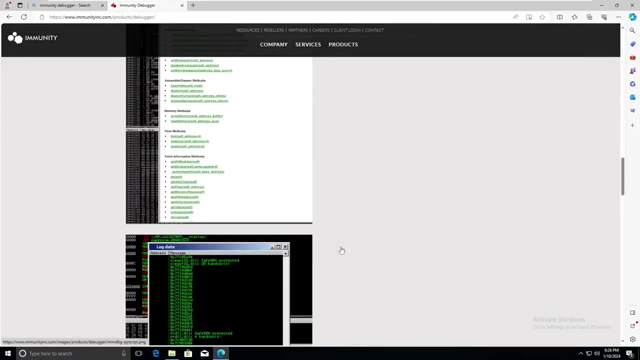 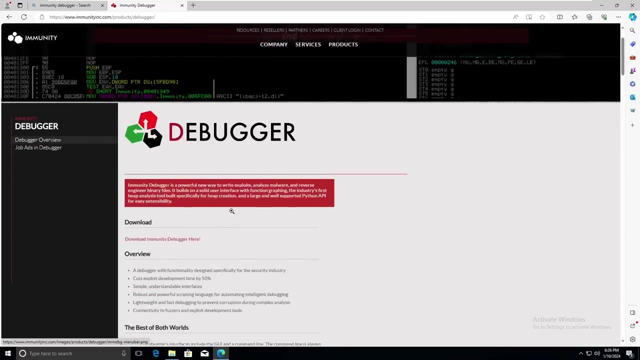 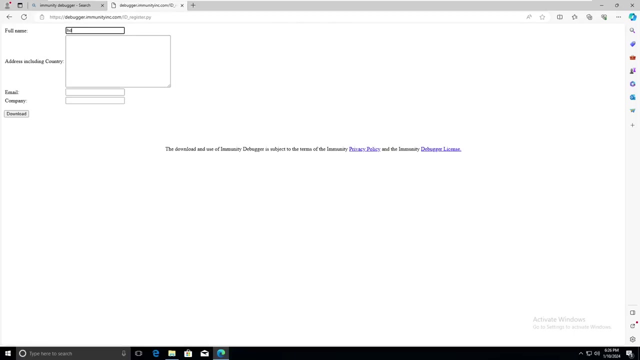 immunity debugger: simple: just search for immunity debugger, right. so here, simple click the first link and from here you need to download it. ok, just go down. ok, sorry, here it is. now you can type here anything. ok, now you can type here anything. ok, ok, ok, ok, ok. 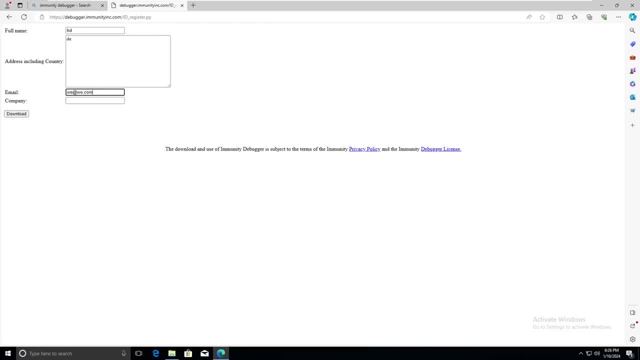 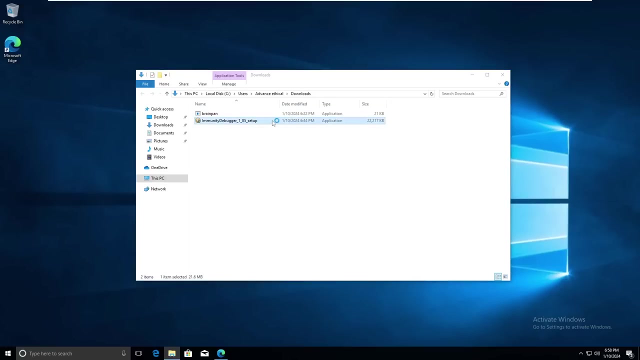 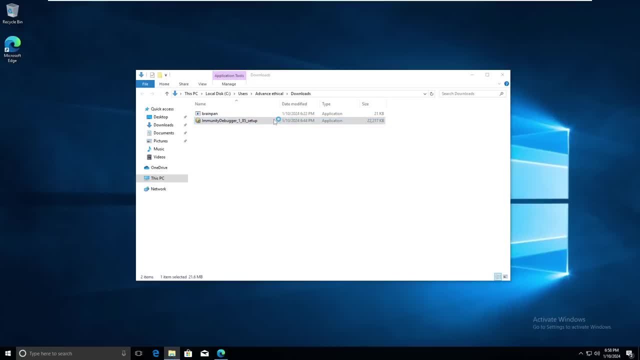 ok. so the thing is it's taking some time. so simple here. click on s see python is not there. simple, let me install it from from here. only you guys can able to install it. okay, just simple. just type yes, there, i accept. next install. okay. immunity debugger is there. simple, close and install successfully launching. 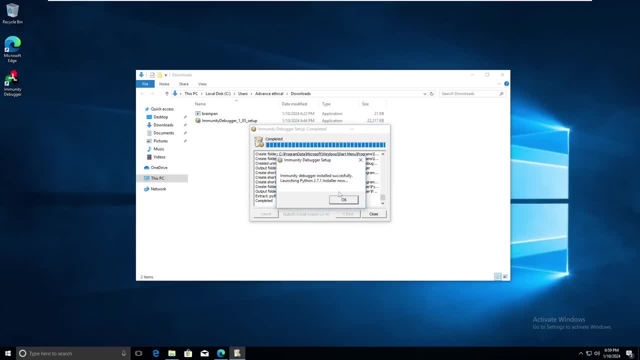 python 2.7. okay, let me install it as well. install for all users. next see, there is a test suite is here. simple, entire features will be installed on local hard drive is simple, click that one and next. so we successfully install the python right. simple click on finish. now click on this pc, click on local hard, local disk and here there. 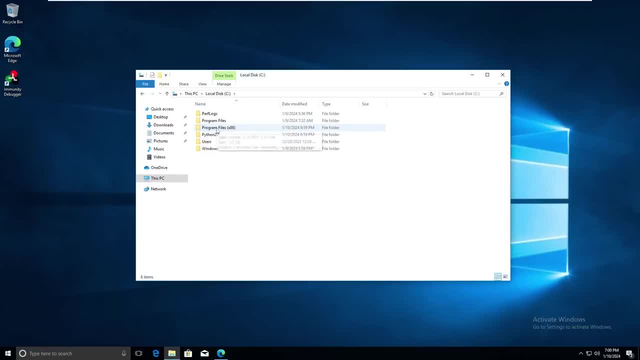 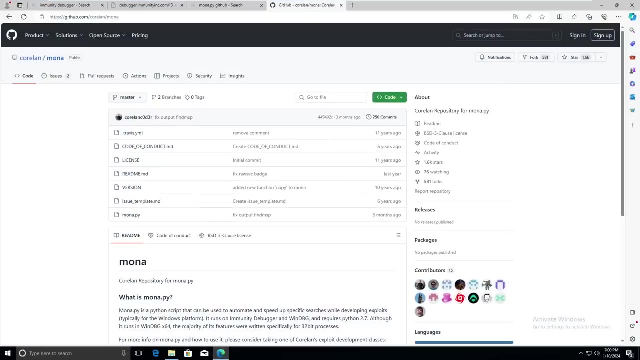 is a program files you can able to see immunity inc. simple double click it and just open this immunity debugger folder. and here there is a py commands. simple open this folder. and here what you need to do is there is a one script with the name of monarpy. what you need to do is you need 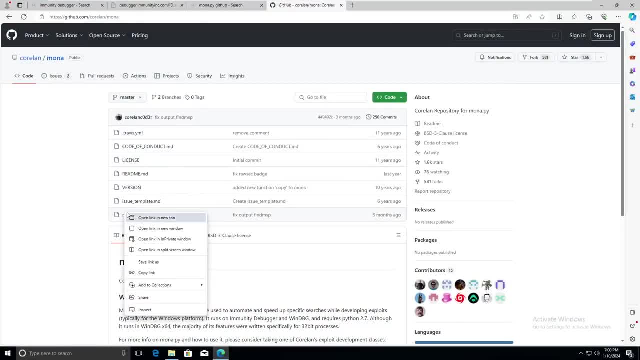 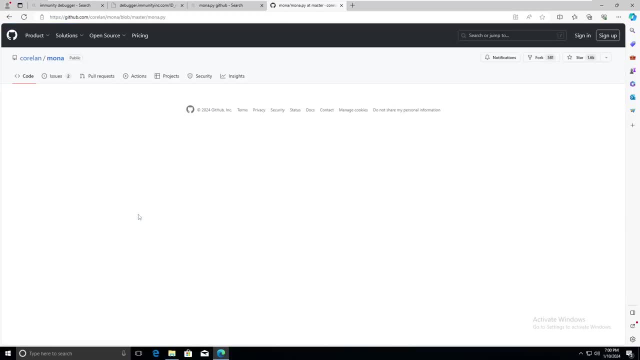 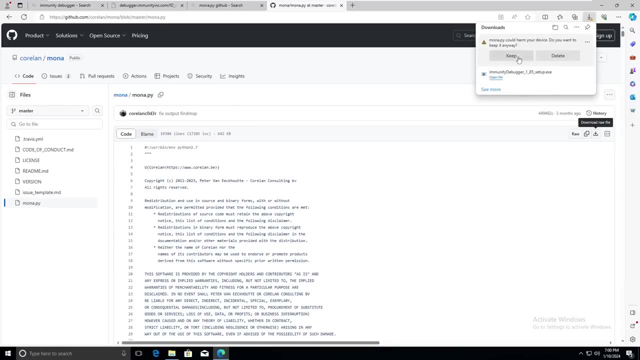 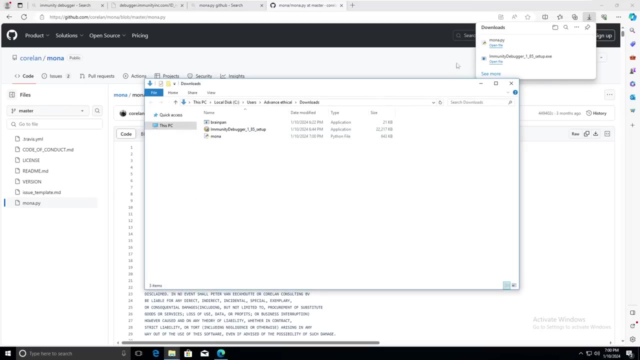 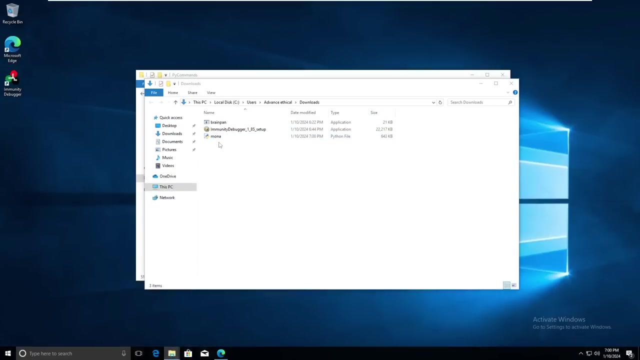 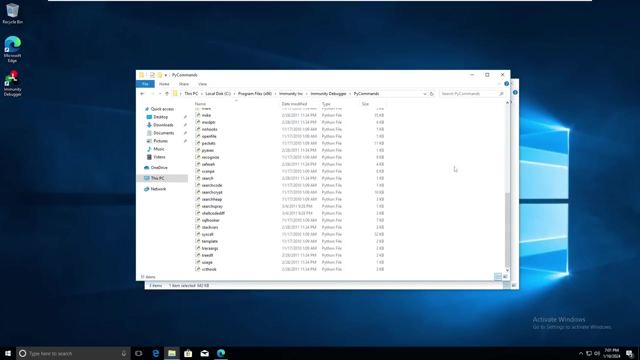 to download this script here: simple click here and download this. this one. download raw file. click on keep, just open file. let me open it here. so here is a python file, right, so simple. let me copy this and paste this in py commands folder. simple paste it here. continue. so we successfully pasted mona there. ok, now in the next classes. 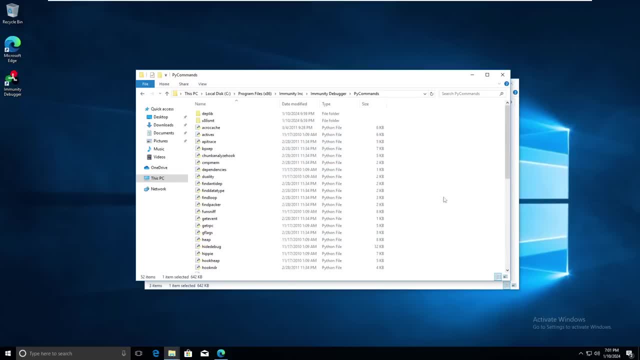 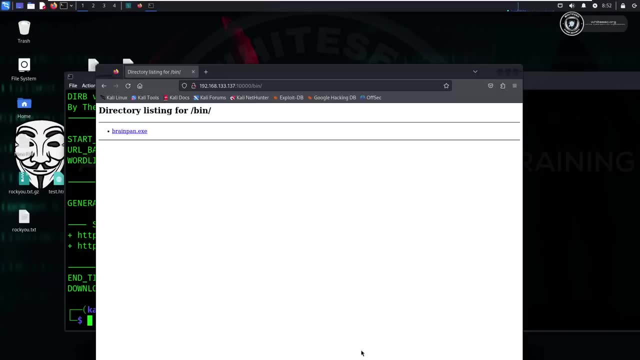 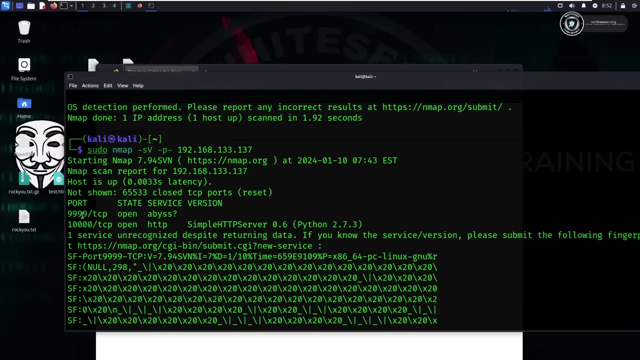 we will start attacks now. here is the thing right. so basically, we can, as can able to see, there are two ports out there, one is 9999 and one is 10000. ok, what is 10000 here? so 10000 is a simple http server and 999 is what? also a kind of server. ok, so let me do. 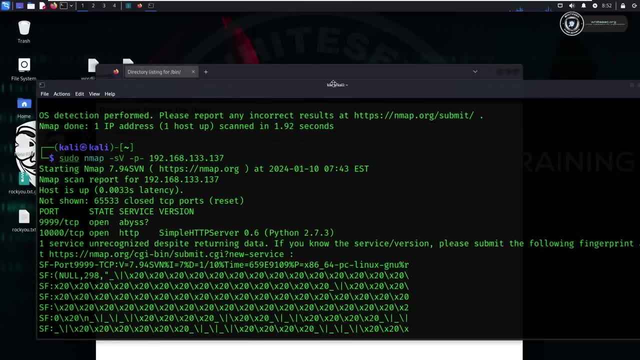 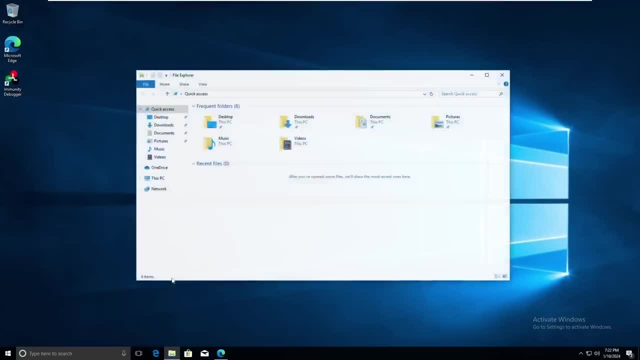 one thing: go back to my windows machine and here you can able to see there is a brianpanexe, is there? ok, now let's see how we can able to perform a crash here. ok, how can we able to perform a software crashing like we can able. 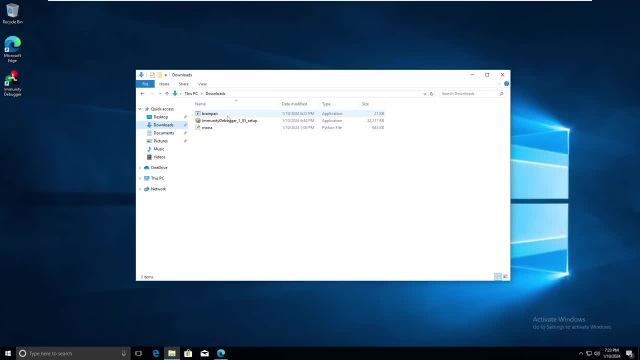 to solve. stop the software here. basically we can able to crash it. assume that i just told you past classes as well. you see a software which is crash. then there is a vulnerability, is there? ok, basically, let me show you practically right. so it might be any software, ok, not only. 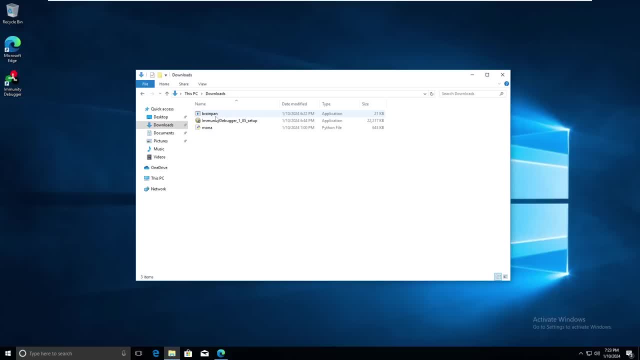 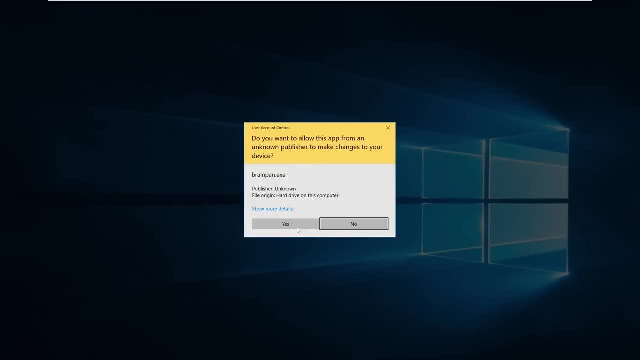 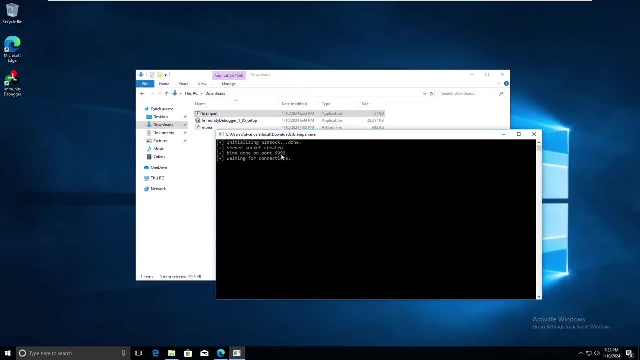 brianpan, it may be any service. ok, So let me run this service as administrator. allow this one. basically, this software: use port 999, 9999,. this is the thing. now see what will happen. what is the aim here? the? 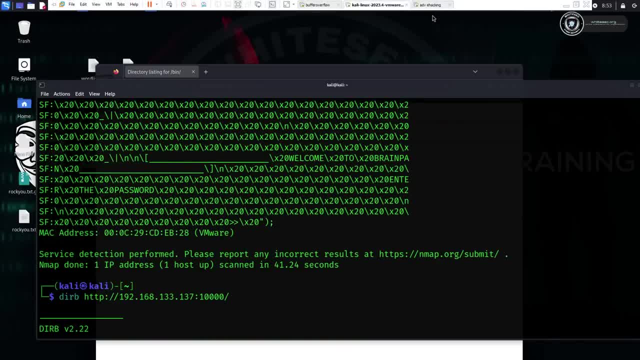 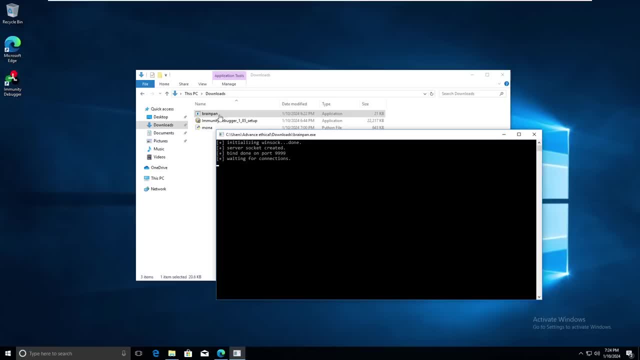 simple. let me tell you the simple thing. see what we are doing means we are exploiting this software. after exploiting this software, what we can able to do? simple: we can able to control this windows system. we can able to hack this windows system. here this is. 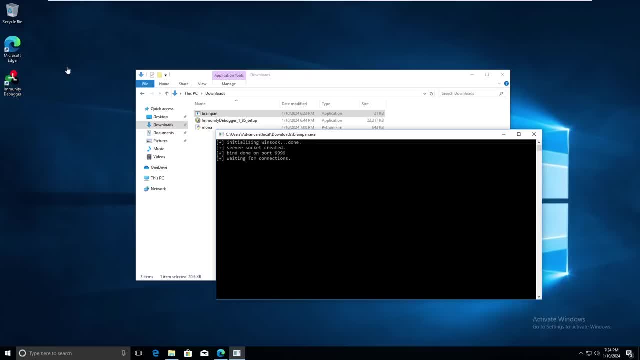 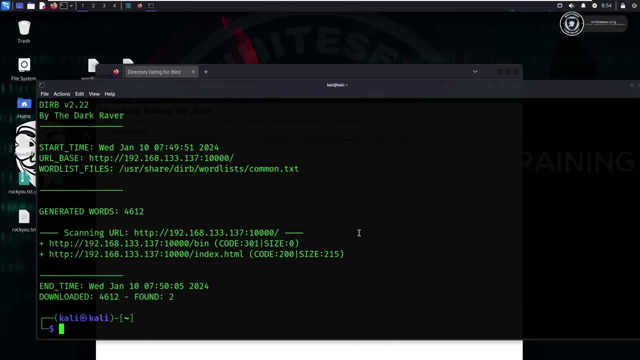 the thing. ok, same like eternal blue vulnerability. by exploiting that service, we can able to take control on that system. right, this is the thing now. let's go back here. now. let me do one thing first of all. for this attack, what we need to do means we need a target. 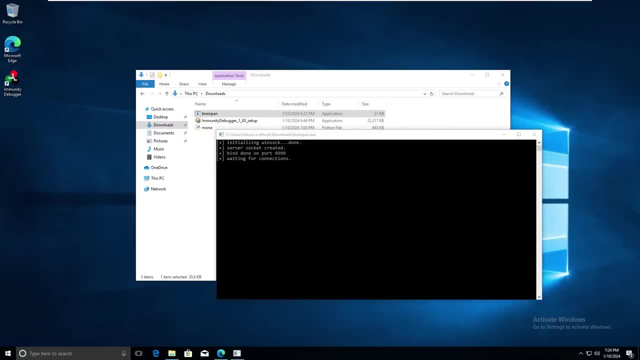 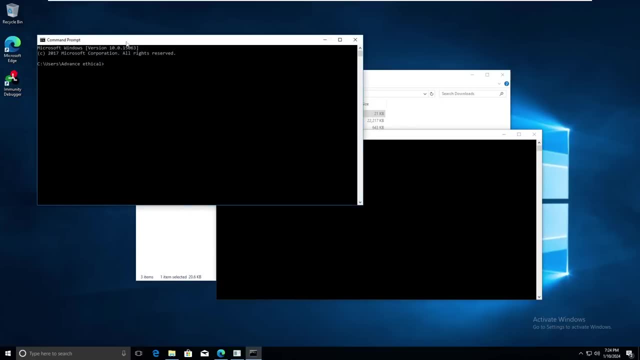 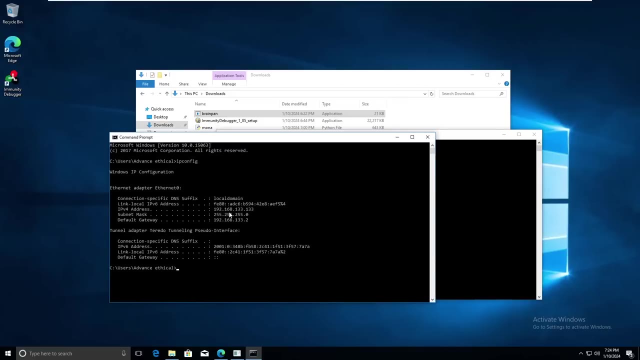 IP address, The windows IP here, because this software is running in this windows system, right? so that's why we need the sorry guys, the IP address. it might be any server, anything, might be any domain as well. so this is the windows IP address, which is 133.133, ok. 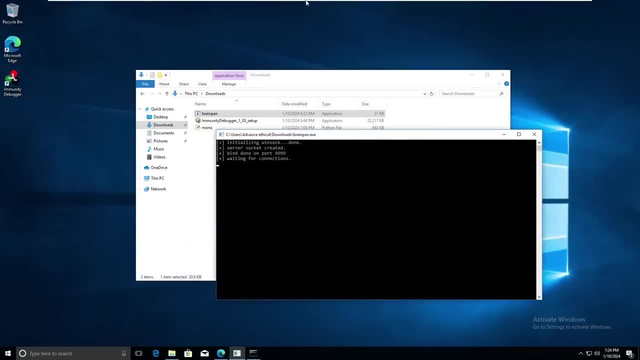 now let's perform the scanning on this windows system. why we are performing the scanning on this windows system? because the service is running here. ok, this service, brain pan- is a service here. ok, it's not a kind of EXE or something. 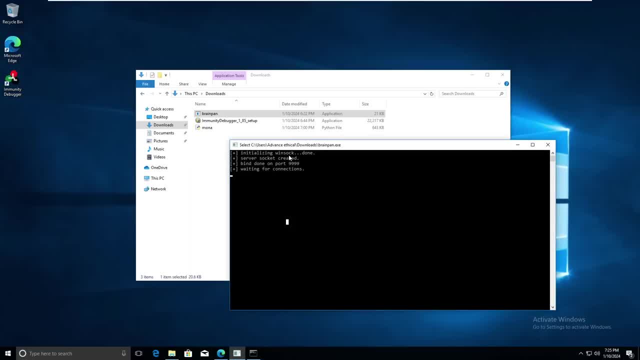 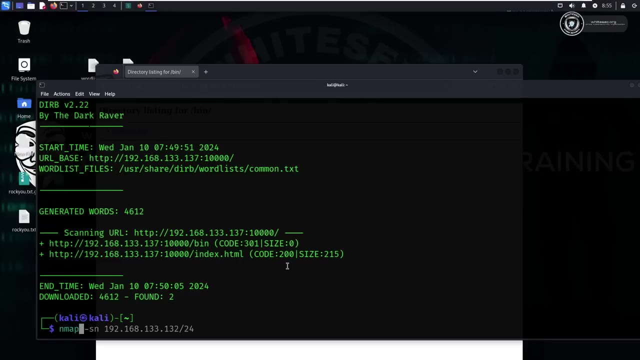 like, not any a normal application. basically, it's a service right which is using the port 999, right, so simple. let's do one thing. let me perform a basic nmap scanning here. just type here nmap. let me perform something like a service version detection here. ok, 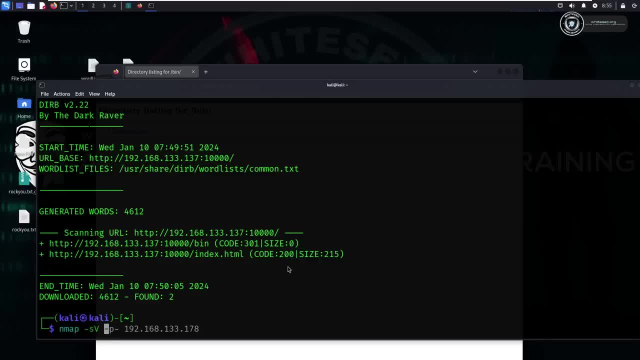 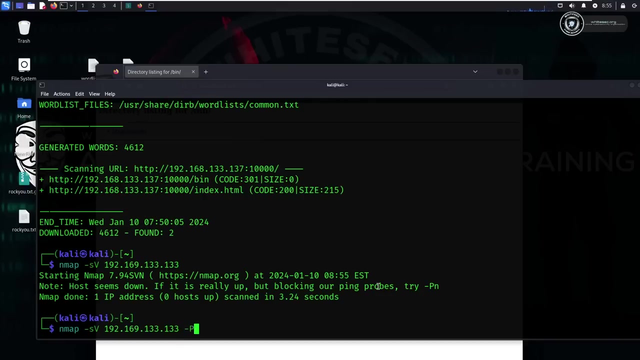 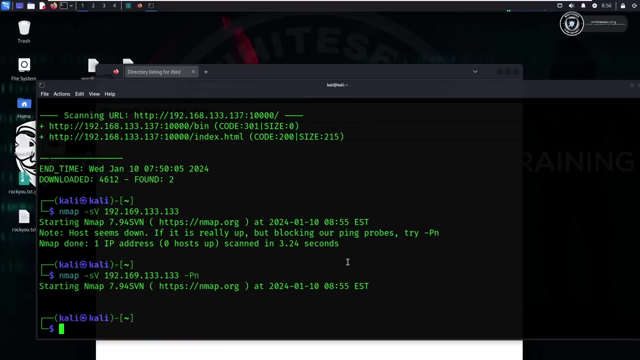 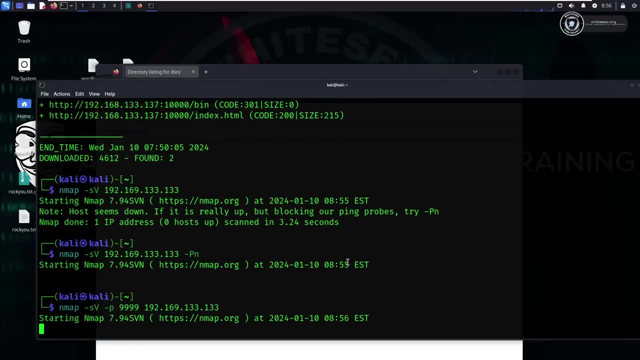 on this IP, which is 192.168.133.133. just wait, instead of giving this much, let me scan for specific port here, which is 99999. just type here dash P for port and just add the port 99999 here and now it will. it won't take that much time here to add this flag: dash P. 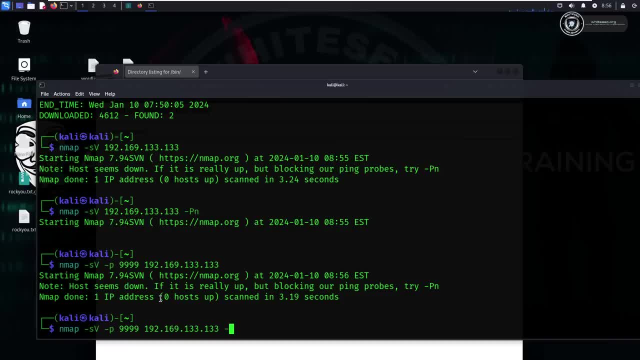 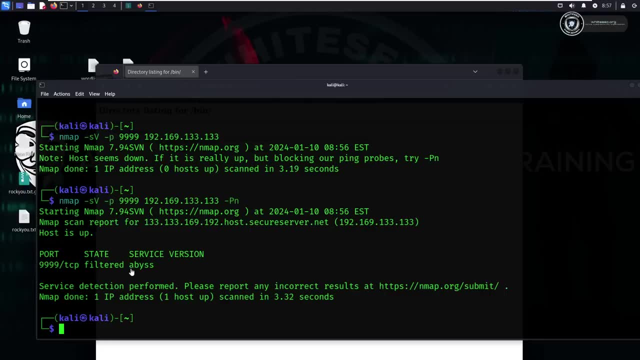 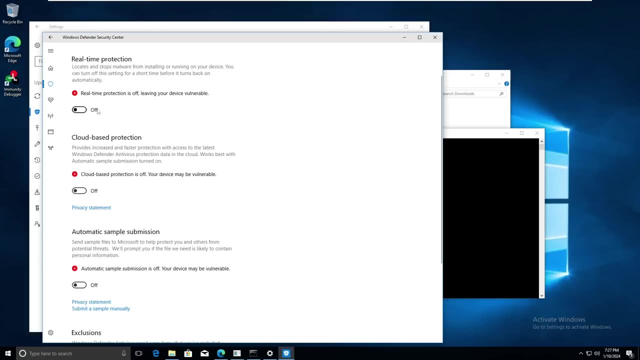 capital P, small n here. oh, I can able to see filter here. that means the fire, the firewall, is enabled there. what you need to do, I need to disable it. okay, let's disable the real time protection here. there are a lot of ways out there to bypass these things. 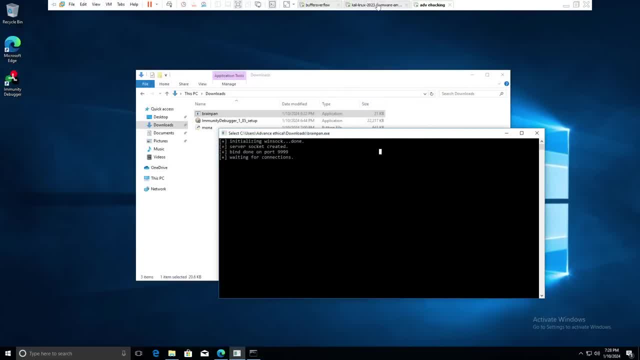 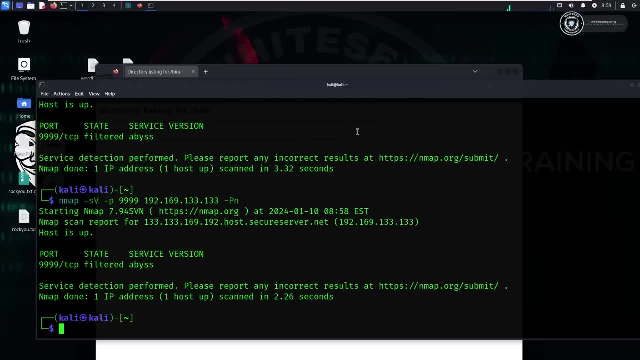 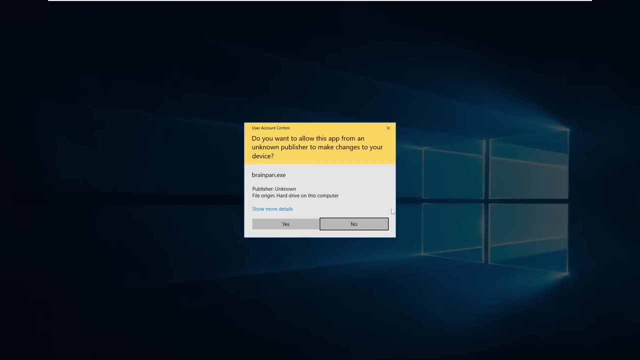 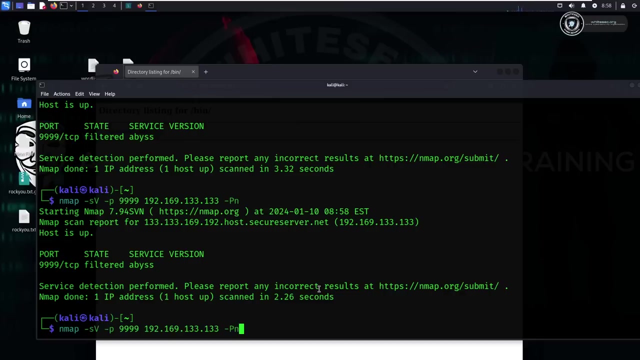 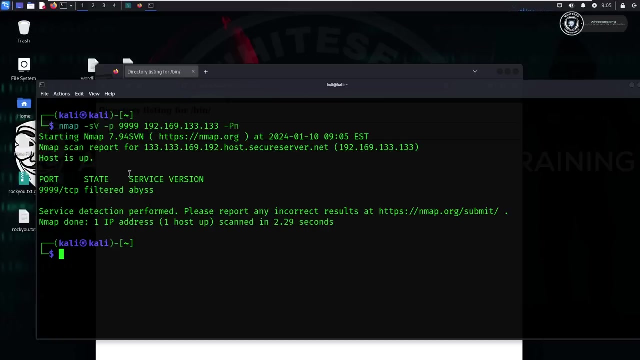 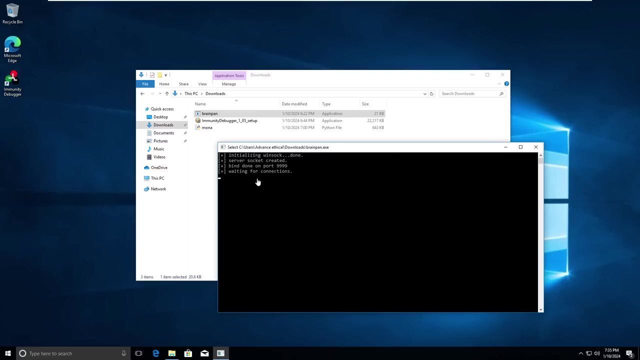 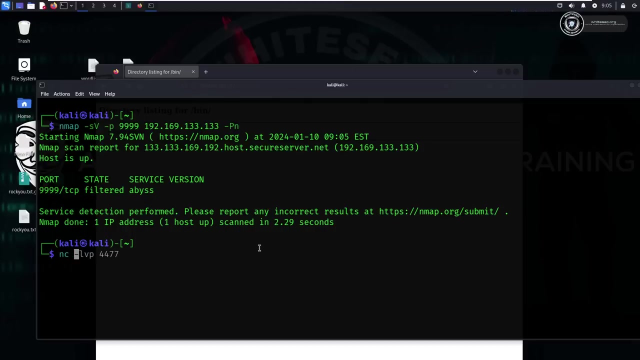 just try to watch Windows penetration testing training, you will get complete ID had. how simple. let me do it again. hey, hey, and it again. user a go here I can able to sell its filter, no problem. the one thing. basically, it's using the band shallow, right, but what? 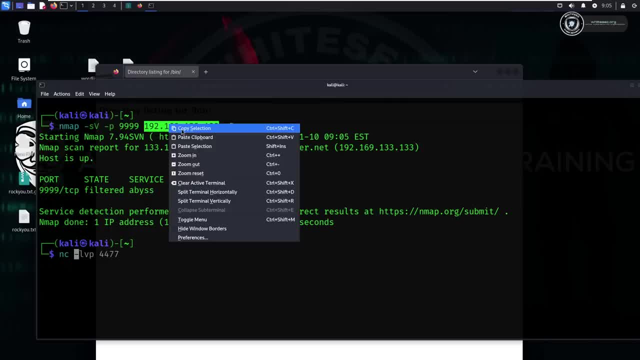 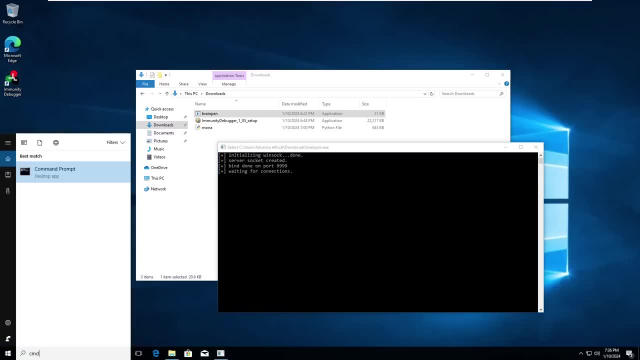 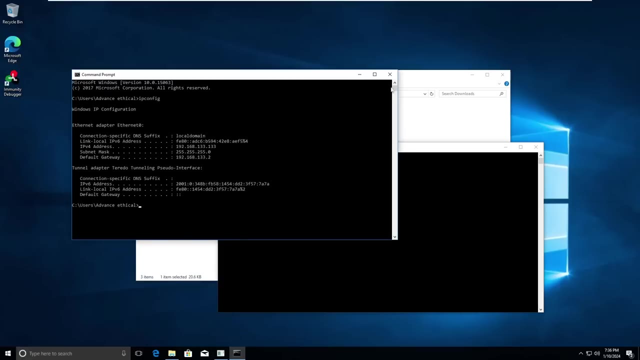 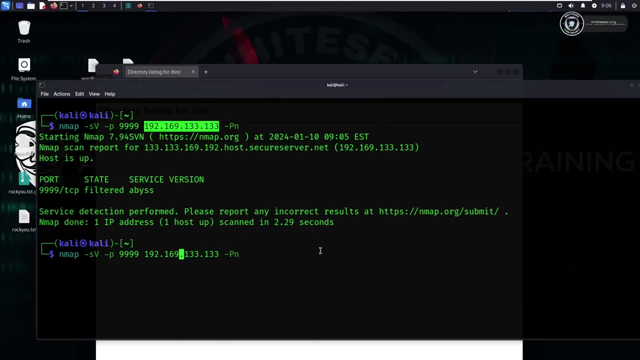 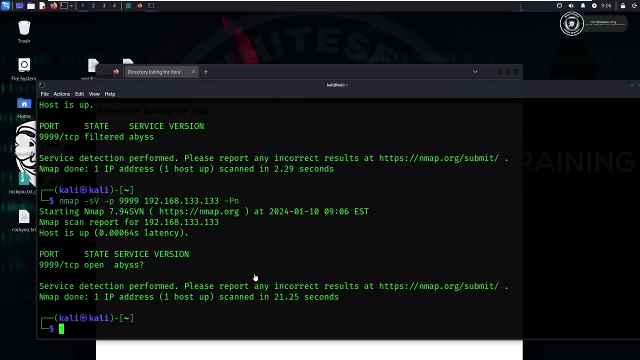 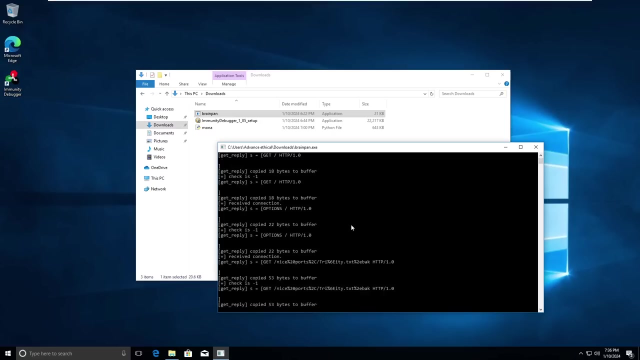 ip address: 192.168. ok, ok, ok, just use the wrong ip there: 192.168. so here you guys can able to see there is a date is open. if i go back here you will see the output. ok, like, i just perform the scanning, right? so that's why i can able to see the output here, right? so this: 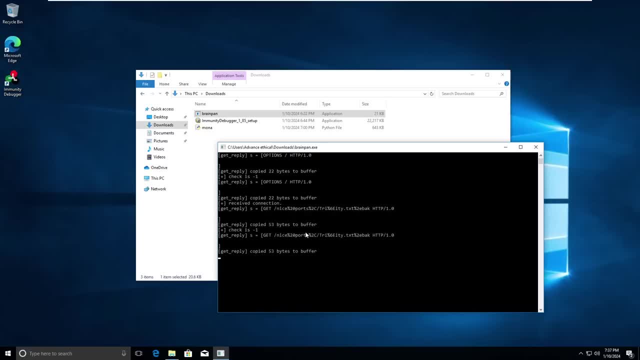 is the thing. see, let me tell you, is there any kind of ftp? there are any kind of services running on any server. at that time, you can also do the same stuff here. instead of giving the ip address of the computer system, you can also give the ip of domain. this is the 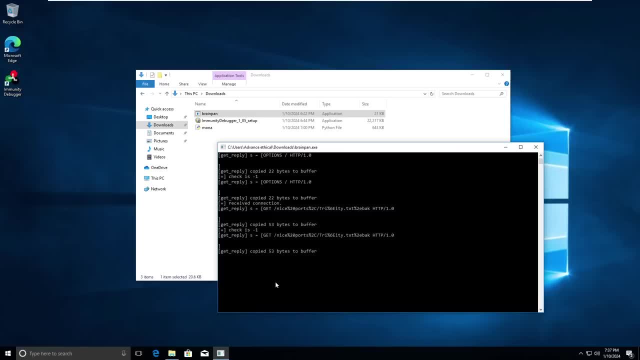 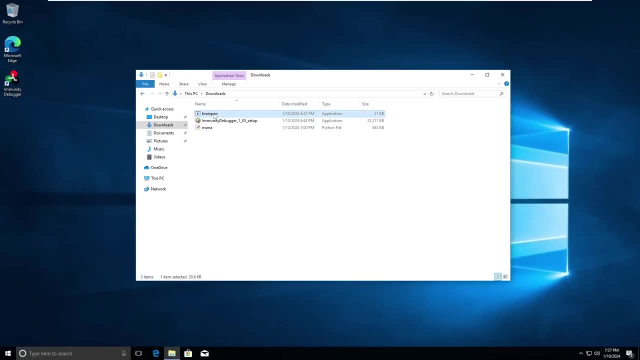 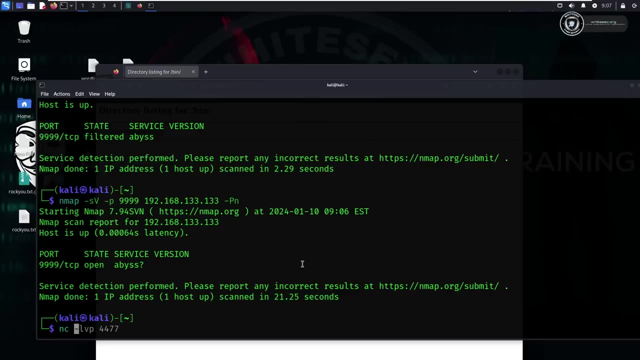 thing right. see in bind shell what will happen means: let me let me show you about the bind shell as well. let me run it as a administrator here again, see in bind shell what will happen means: let me use netcat here. just type nc, ok and your target ip address. simple, i am. 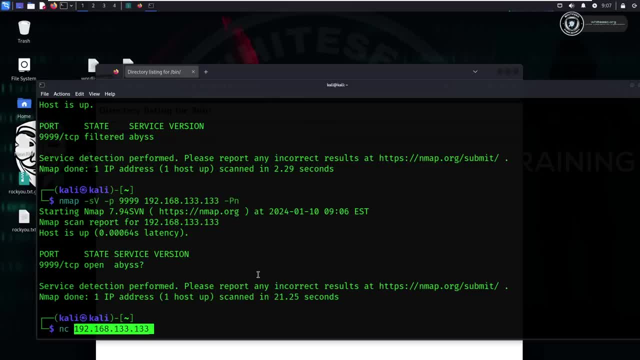 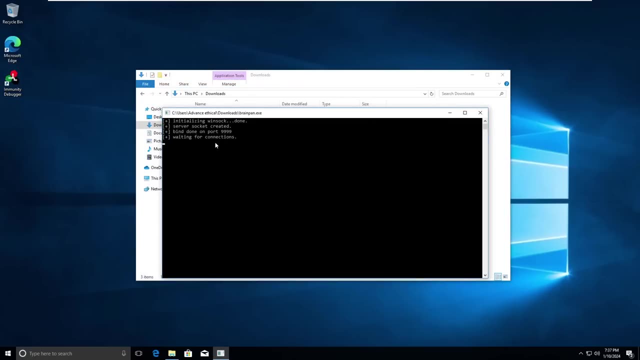 connecting with the machine using netcat here. ok, netcat, you no need to perform a reverse shell or something like that. simple, if you, if service, is using bind shell here, then what will happen? simple, you just need to add the ip address of your target and the port which service is using here. ok, the service is using 9999. 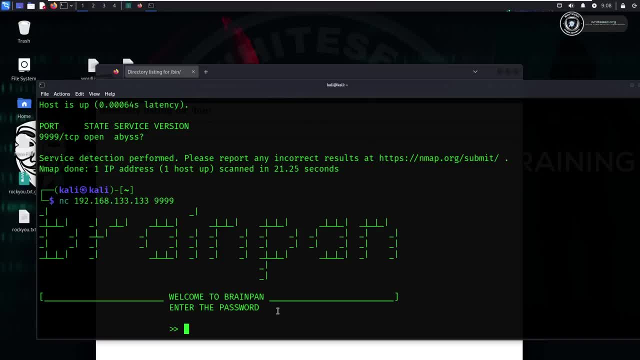 ok, so here i can able to see the output. simple. if you are not getting this one, then just try to watch. open ports, penetration testing, training there. we just covered these things now here let me do one thing, see mostly, if you know buffer overflow or exploit development during. 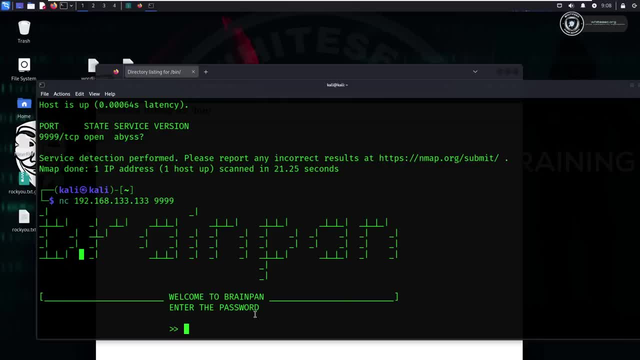 this process, what we do. we use the a characters here, why we use it. the simple thing is: see, it's a it it is easy to detect. ok, this is a first thing, because a use a value of four one. ok, let me tell you. maybe in next class i am gonna explain you about this thing here. 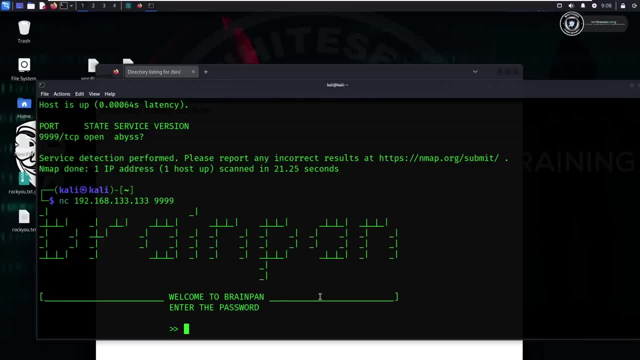 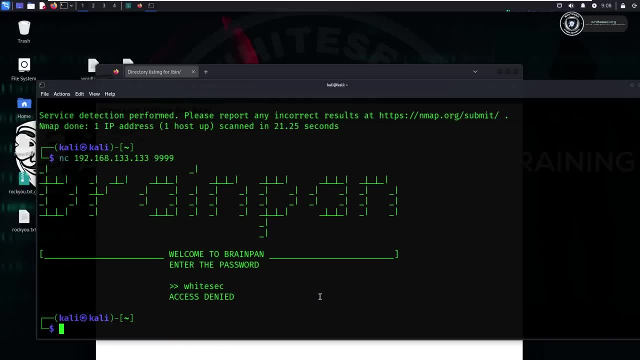 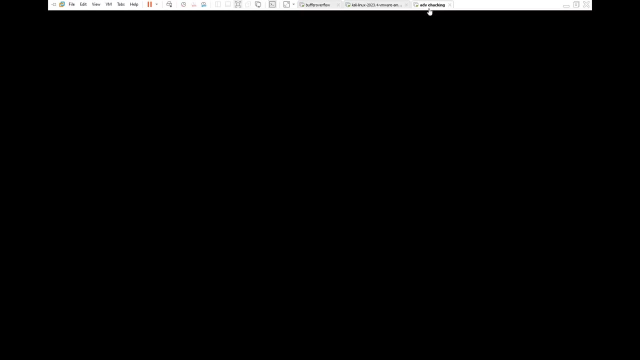 you can type any value. ok, just type here: whiteset. let me type enter here. now, after typing the input, it saying that adds is denied. ok, let's go back here and let me see: ok, whiteset. i just type the the input there as a whiteset, here again able to see ok. 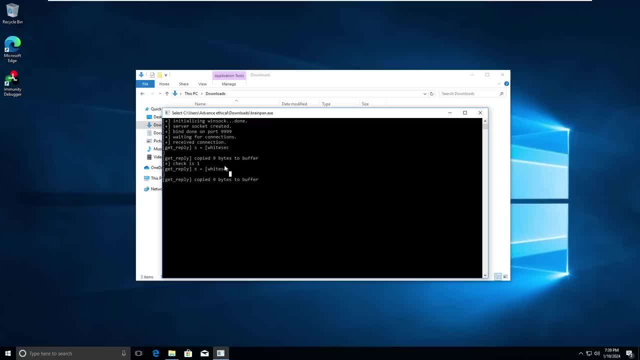 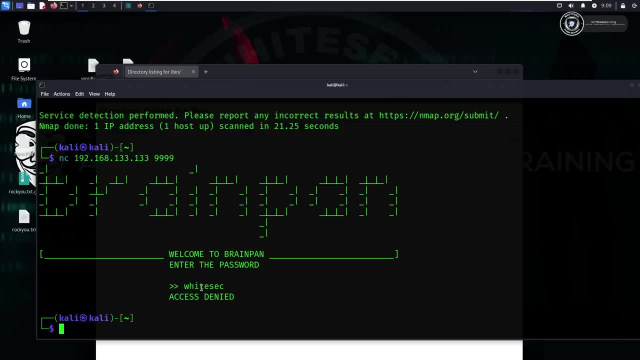 now this character. ok, by typing this simple, this much characters, it's not affecting the software here. ok, the service. here. i just told in the last classes, i just given one example- assume that if the software is asking any kind of, is there any kind of form it's accepting only. 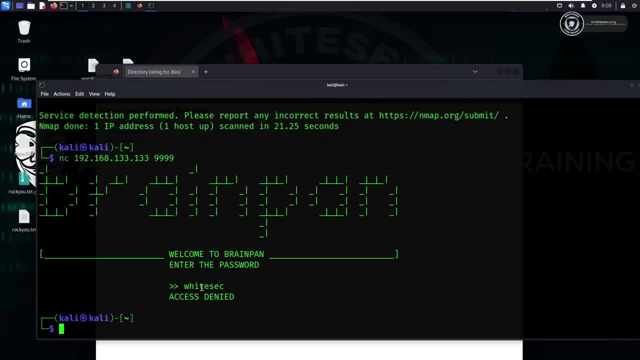 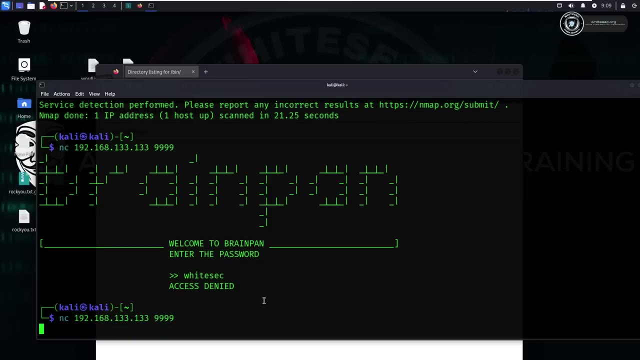 eight characters there to type more than eight characters, and what will happen? the the software might be crashed. it won't accept. i just told you that example. right, so simple. the same thing which we are doing here. okay, now see, let me do it again using netcat. 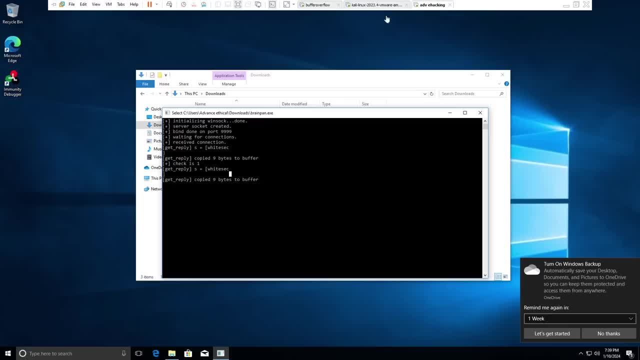 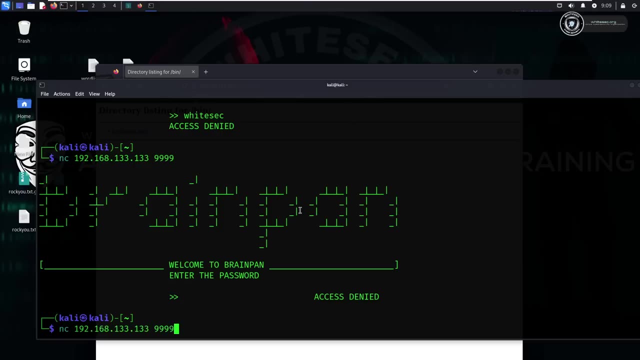 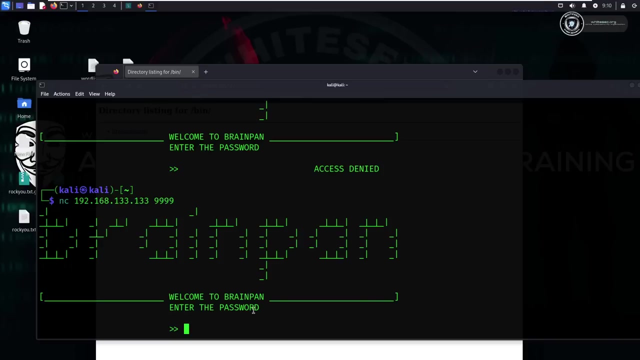 simple thing is: let me close it and let me run it as administrator again. let me use netcat instead of typing a small character characters like a eight or four. instead of doing that, let me type a huge here, okay, such as: let me type a number of ace here. 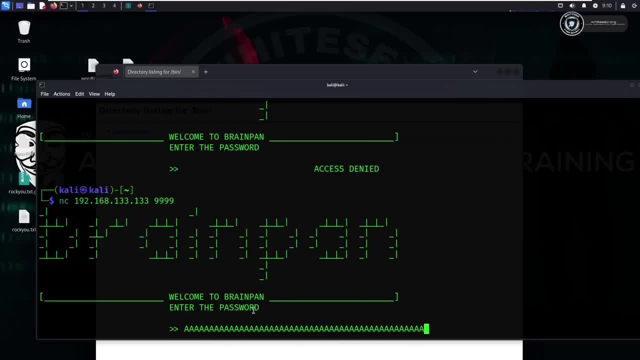 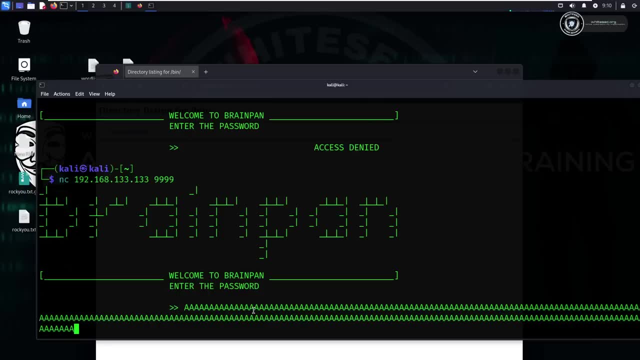 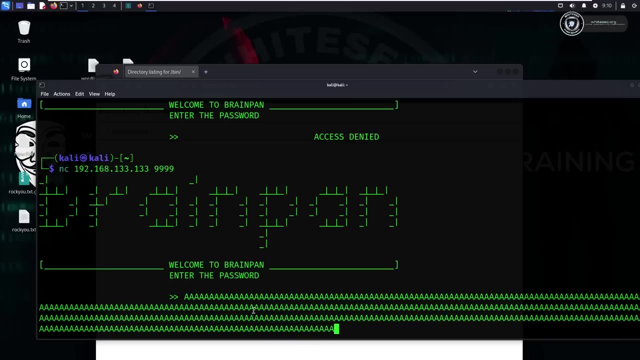 right. so let me see if it is accepting that these characters or not. see, basically all these characters go in buffer, okay, which we just learn in the next classes. if i, if this hit in eip, then what will happen will get crashed, okay. so this is the thing, if i try after. 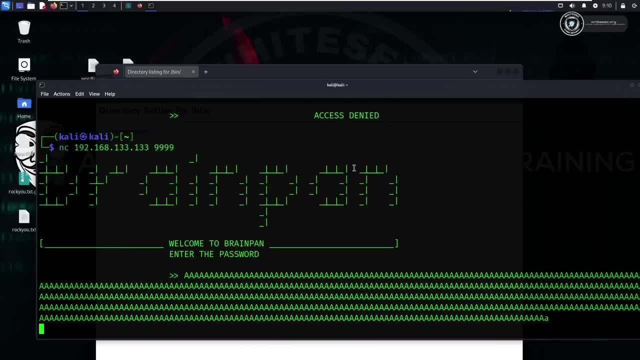 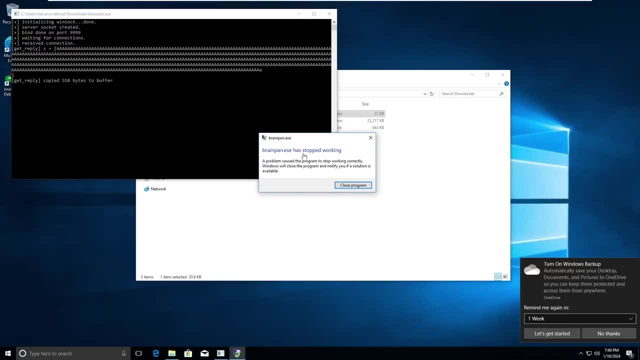 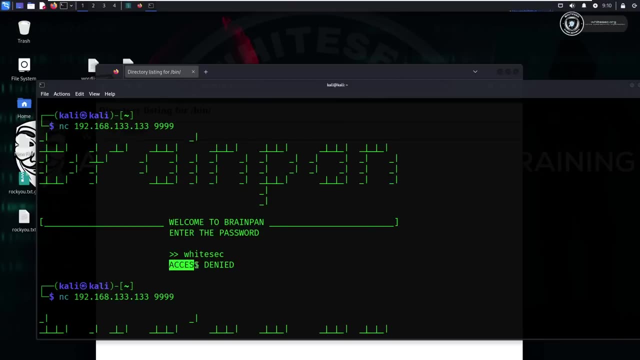 typing this much is what will happen. the software has been crashed. so this is the thing. so, uh, brainpanexe has been stopped working. now see before, uh, before typing this much characters, what happened. it showed the output as as is in it. now just see it's not showing any kind of output. nothing now, just assume. now you need to. 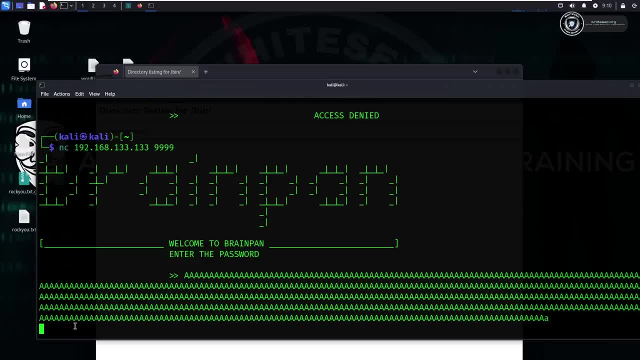 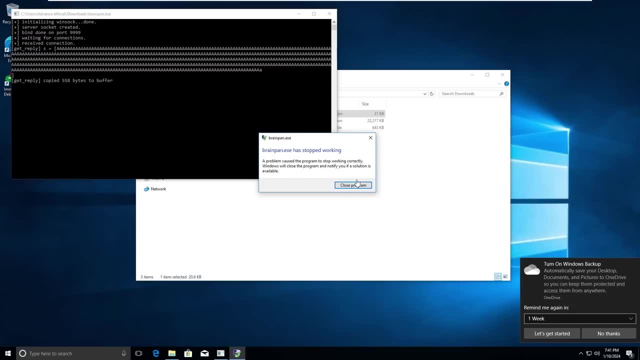 think that the software has been crashed. in real world, you won't see these things, okay. you can't see the back end here. real world, you need to identify like this, only okay. this is the thing before doing applying the process in real world. first, you need to set up a lab. 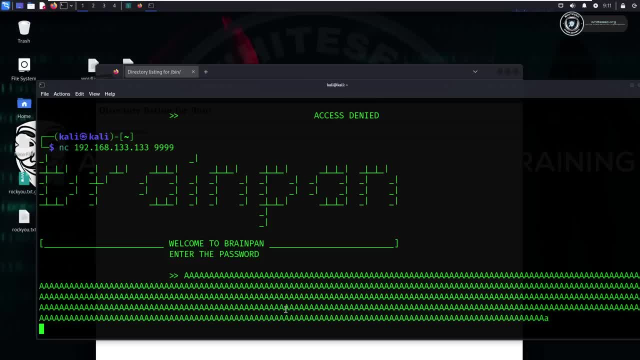 there you need to install your target. assume that your target is using some kind of services like. assume that your target is using ftp. okay, at that time you need to set up the same version of ftp in your lab. then you need to perform this testing there. okay, if it successfully work, then you can. 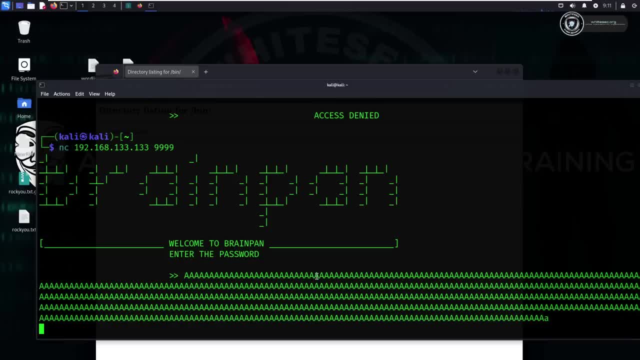 able to apply that thing in real world. this is the thing. this is the complete approach here. okay, uh, it's not that much hard, but it's hard. okay, this is the thing. like, uh, how it is hard. the simple thing is, if you don't practice it, then it is hard. man, this is the thing. 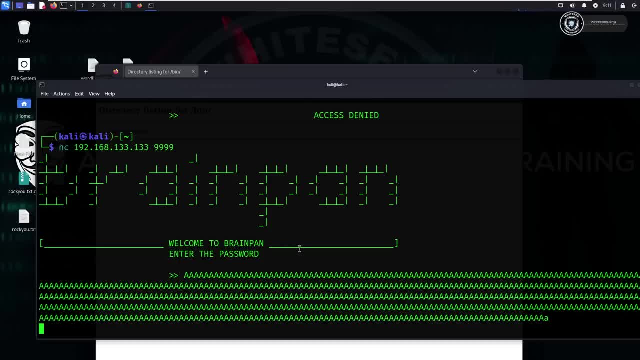 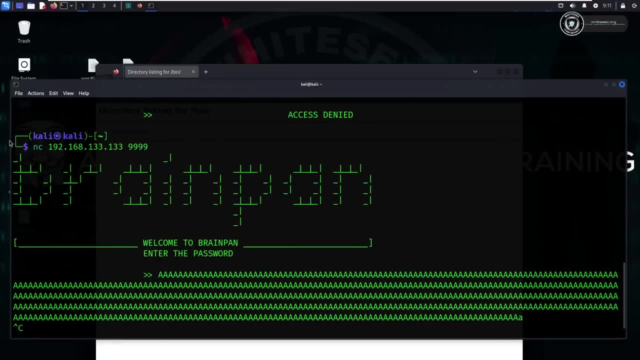 now, soon i'm gonna create a complete course on exploit development. see, i just told in the first class as well. mostly i don't go for exploit development. okay, uh, because i have, i do, a lot of shops like scada automobile wireless attacks this, this kind of shops. okay, so, uh, mostly i don't. 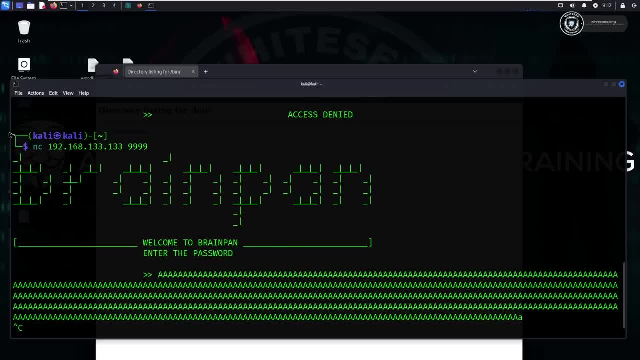 go with this one. but if i got any kind of project related to this, or if i have, if i got any kind of client- uh, if you're developing any kind of software, and he just called me to test that software, at that time maybe i'm gonna create a. 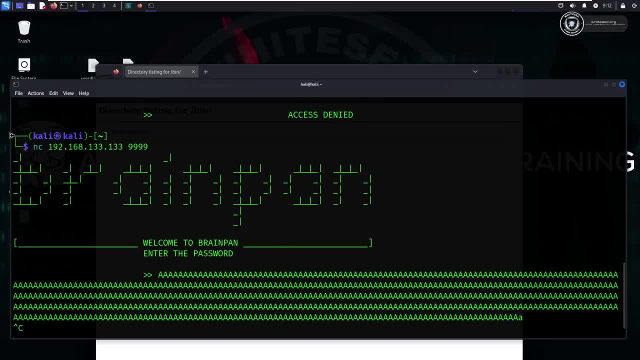 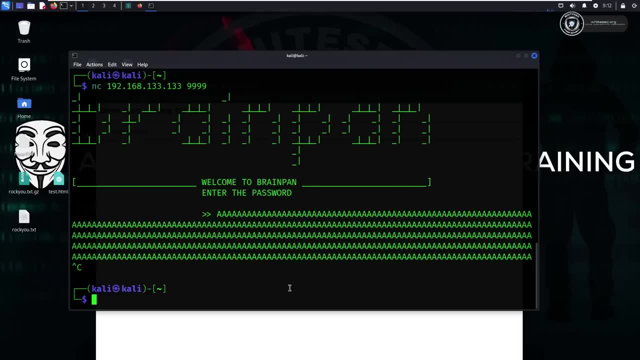 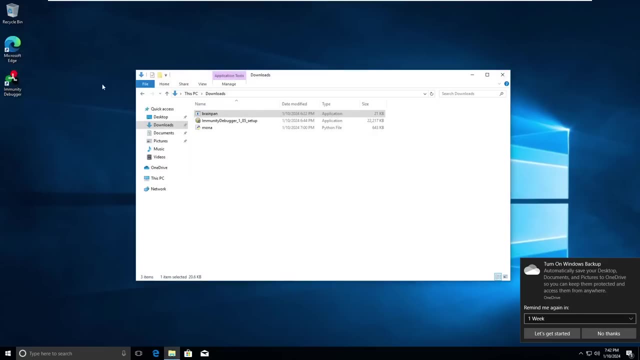 complete training on it. okay, this is the thing now. so this is the thing. we successfully crashed the software here. now in the next class, let's learn about immunity debugger. here is a one of the excellent tool. right by using that, you guys can able to see a complete backend of the software. 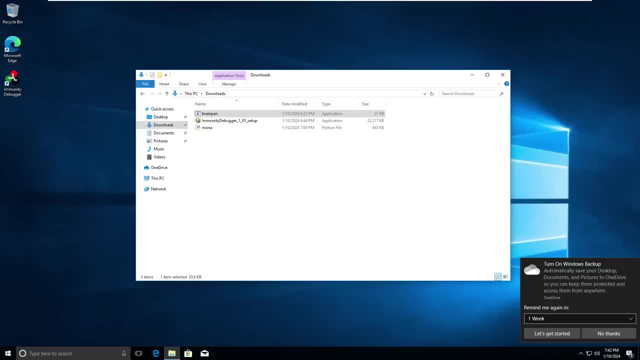 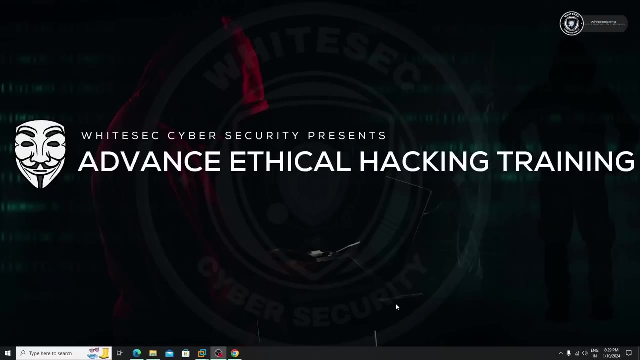 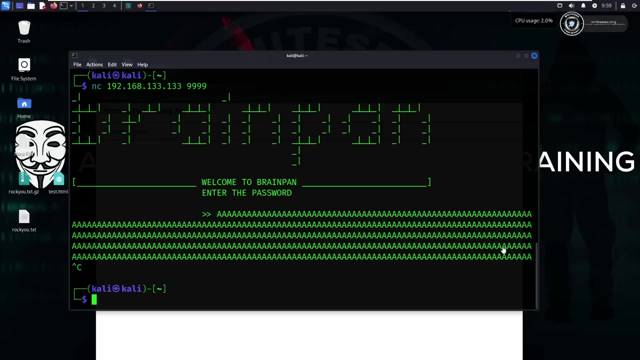 right how it's working. like we just learn about eip kind of shops, right simple. we will see those stuffs, uh, in immunity debugger app. okay, just wait. let me now see, basically in last classes, what we did. we just send it here, is there? okay, the software has been crashed. now let's see how it's affecting backend. 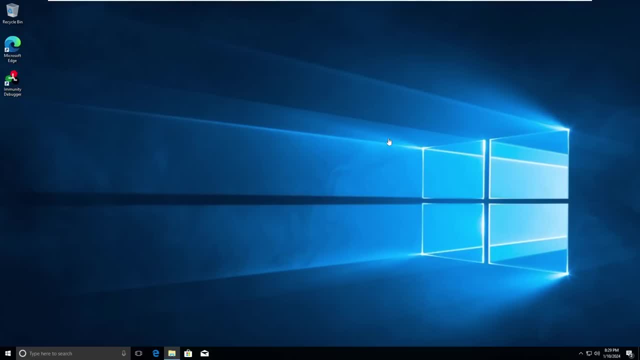 you just saw here: okay, the, the software here, the brain pan, is stopped working like it's crashed right. so what i am trying to say means: let's see the backend, that's it. we are not doing anything here, we are just seeing the backend, how it's affecting it. okay, now, first of all, what you need to do, simple. 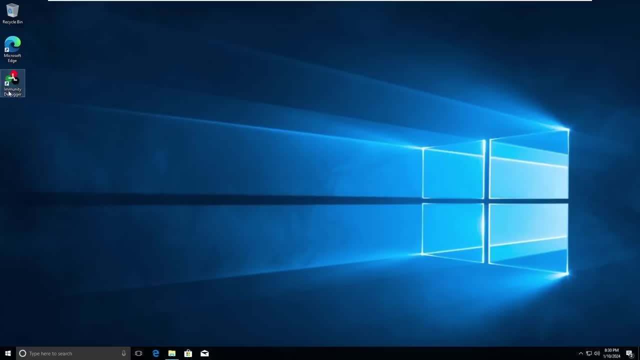 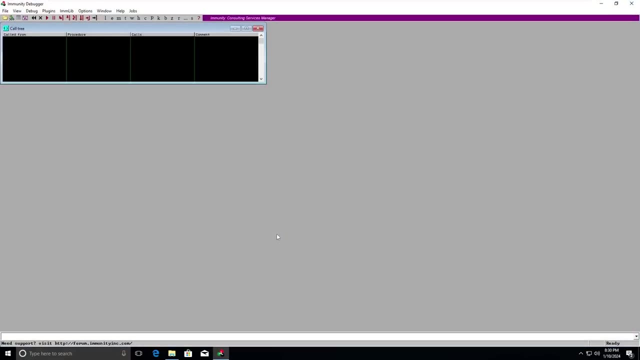 let me open the immunity debugger here. let me run it as an administrator, because we are running the service as an administrator, so that's why you need to run this as an administrator. this is a thing. okay. now here you will see the file here. okay, simple click on file. click on open select. 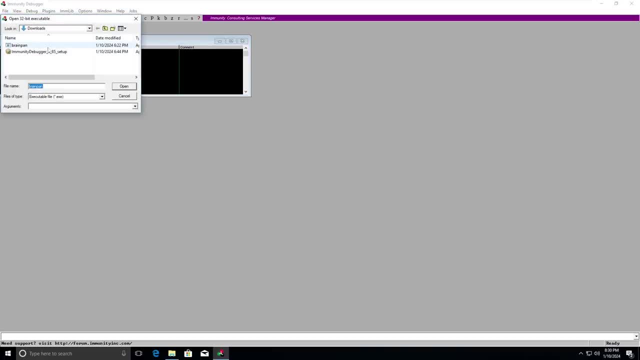 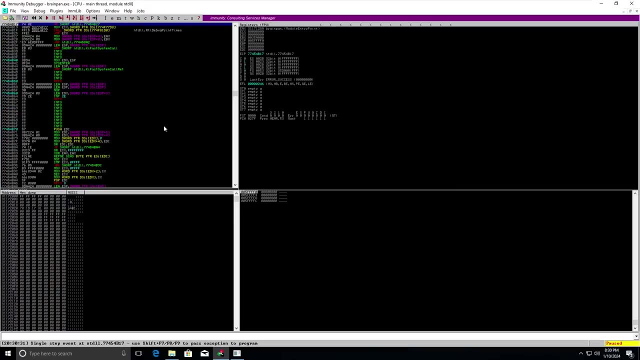 your brain pan dot exe selected, so here you can able to see the tab, right? basically, you will see four things here, four tabs. first one is disassembler. a second one is a register. this is a registers. here we just learn this things. okay, what is a register? see here we. 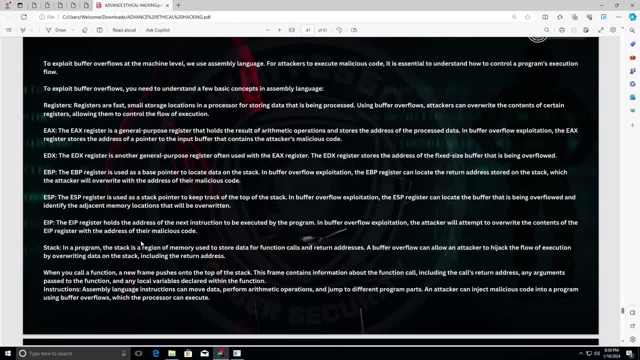 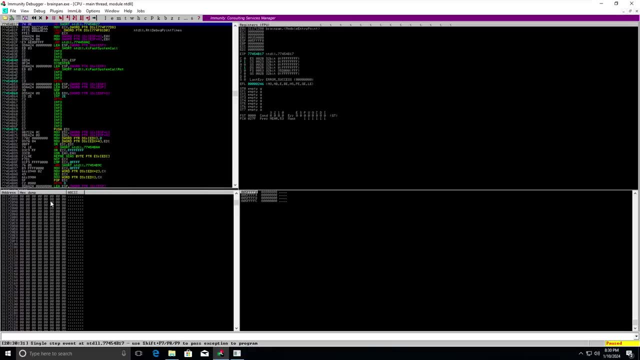 just covered it. or the fast small storage location in a processor or storing data that is being processed. okay, just try to read it. and here, this is a dump. okay, basically we tell it as a dump here. okay, and this thing is what stack? this is a stack, right, so let's load a software. basically we just loaded a. 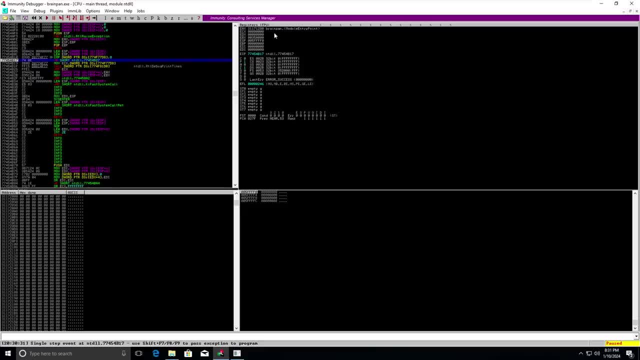 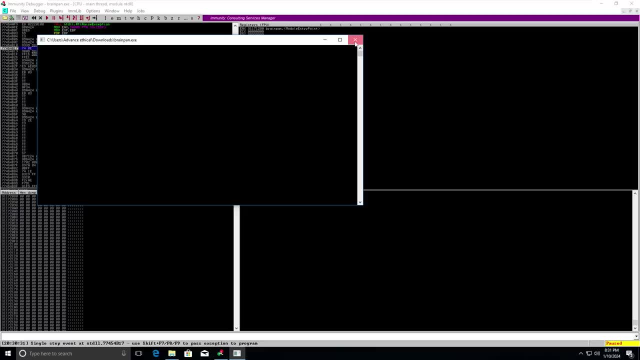 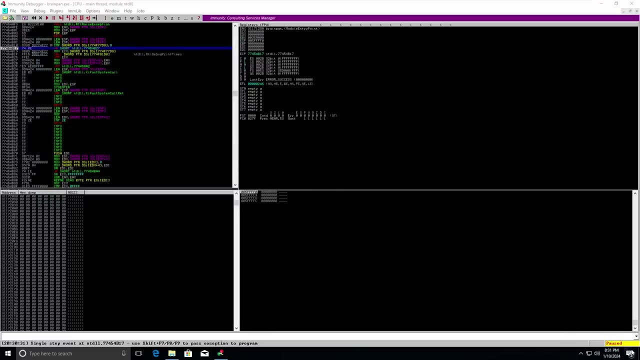 brain pan here. now let me do one thing, see. also, let me close this one. see, once you open the software, any exe file using immunity debugger, then what will happen means it will get passed. okay, this is the thing, right. so if i play this one, if i want to run it, see, the program is. 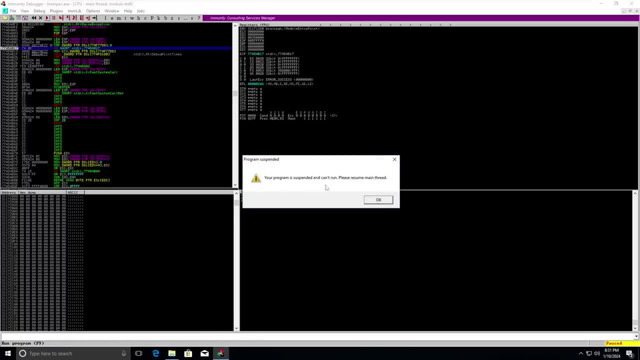 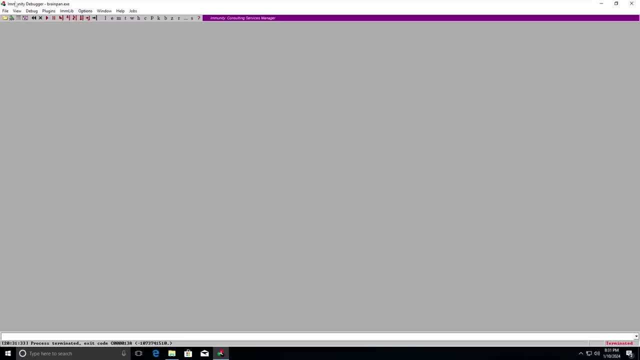 suspended and can't run because i just removed from here. let me open it again. okay, we'll click on it. click on file. now you can able to attach it because we what we did, we just open it for first time. you need to open any software. then you can able to use attach here, a simple attach, if you. 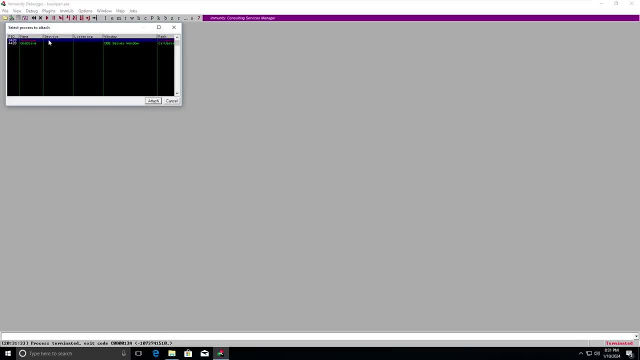 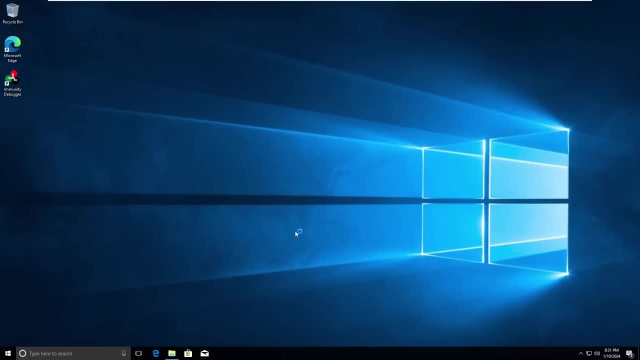 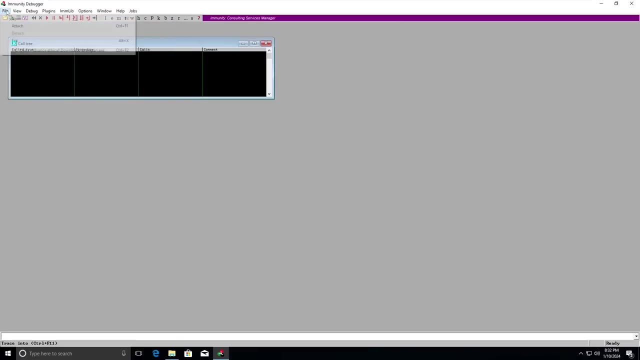 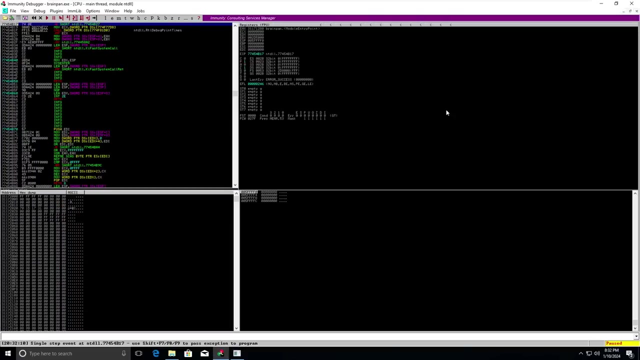 click on this thing, then it will get attached. let me reopen it. okay, so good for you guys as well. okay, here let me attach select brain pan. and here it is right. so here is a software, right here. i just told you, once you open the exe using immunity debugger, then it will get passed. 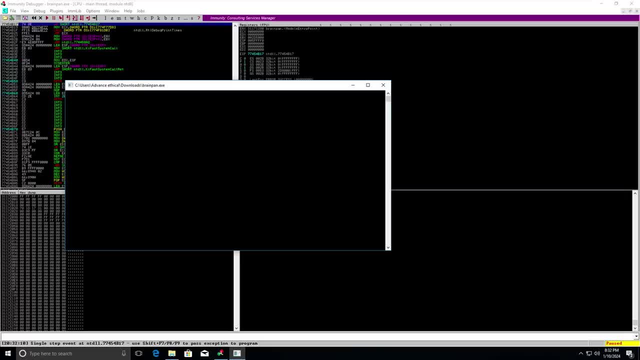 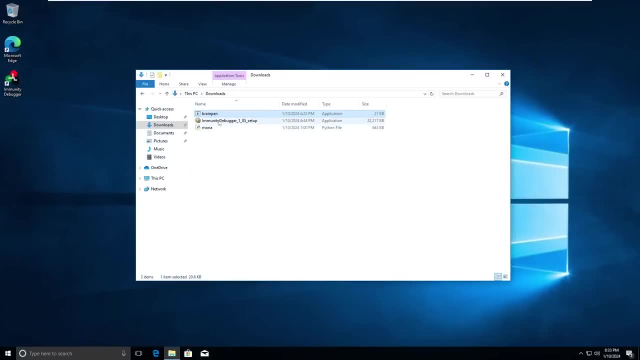 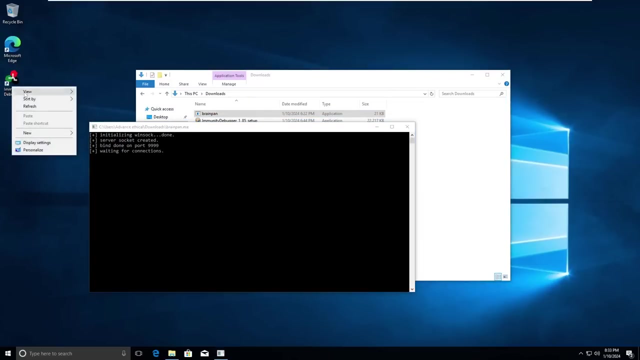 this is the thing. now let's see how it's effects. right again, let me first let me run this brainpan dot exe as administrator. right, it's running as administrator. now let me open the imminent debugger as well. see, i am doing again, again, again and again, because you guys will get it. 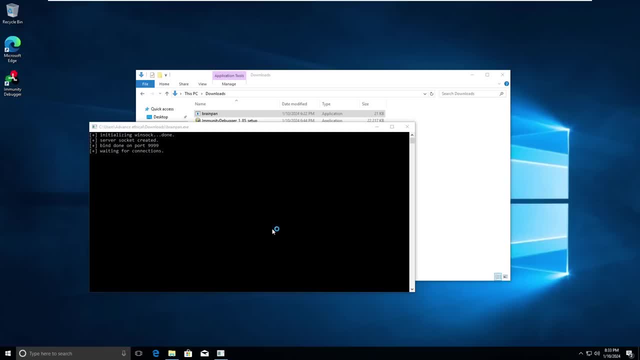 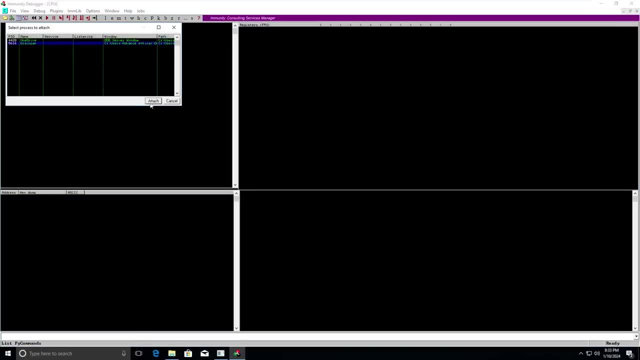 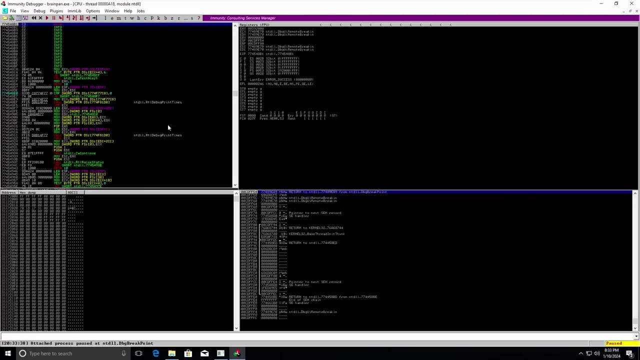 so click on file, click on attach- now i can able to see the brain pan here will select it. click on attach. okay, i successfully attach this one. i just told you what this is. a. this tab is a disassembler. this tab is registered. this tab is done. this tab is what stack. 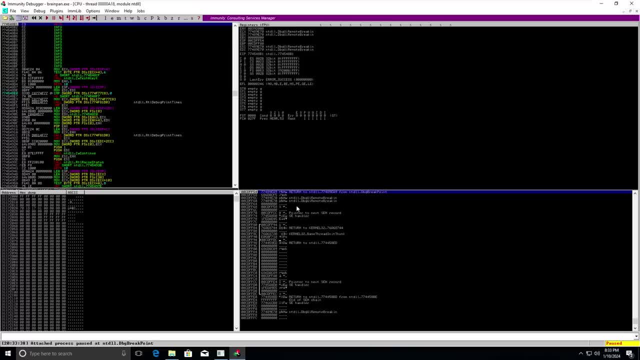 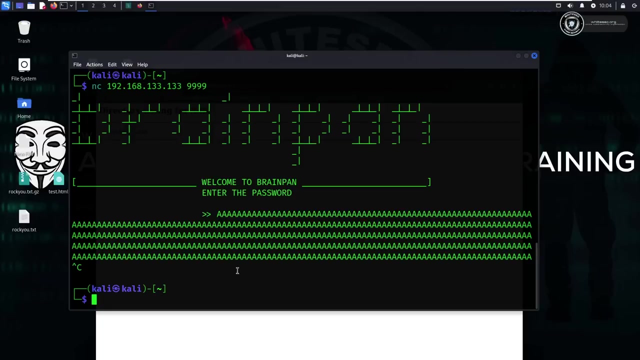 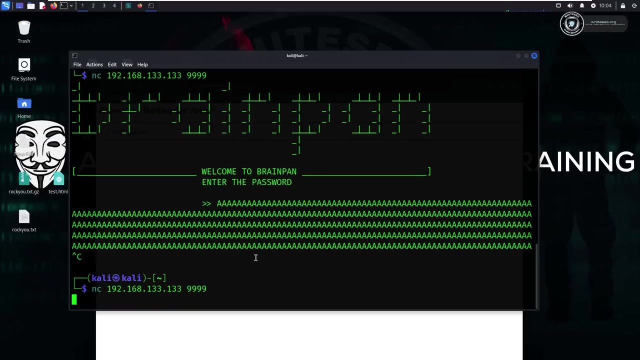 this is known as stack here. please just try to zoom the video here. i can't able to zoom now here let me do one thing, let me execute the same thing here. just type netcat table line, the double line, double line port and click on play here. 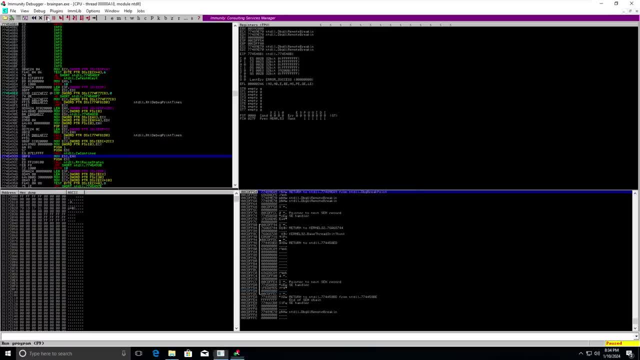 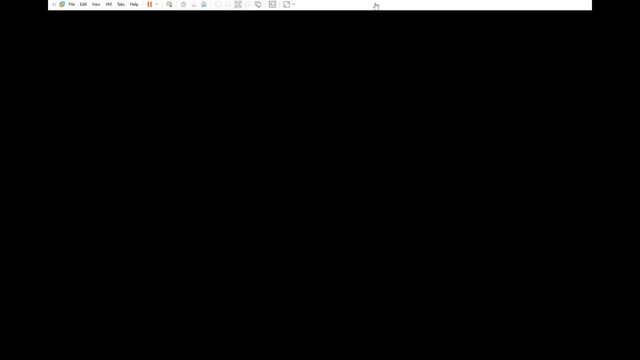 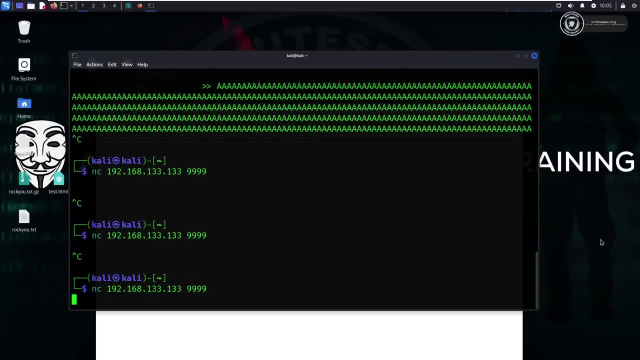 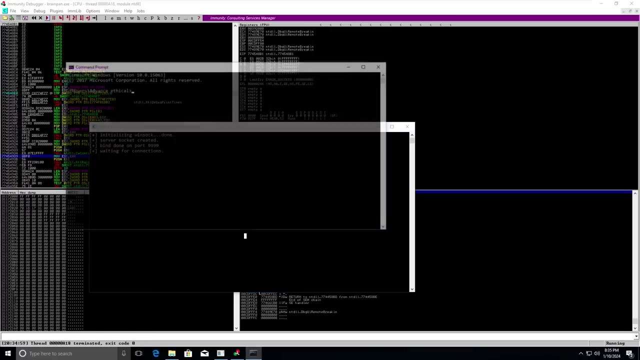 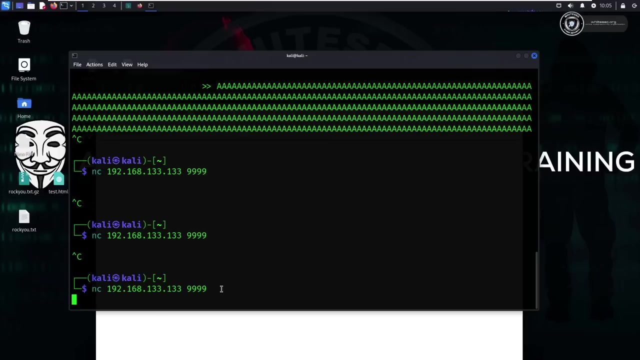 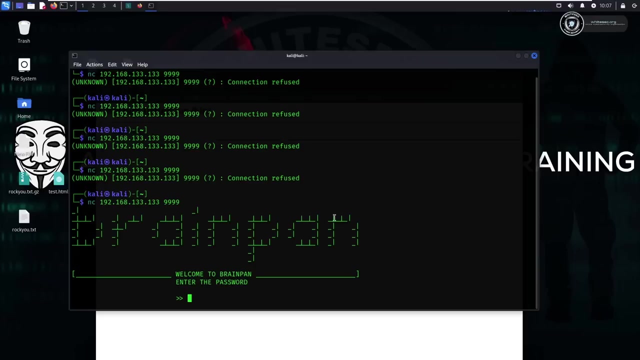 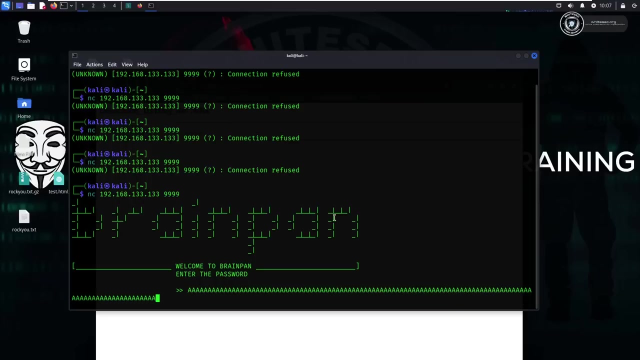 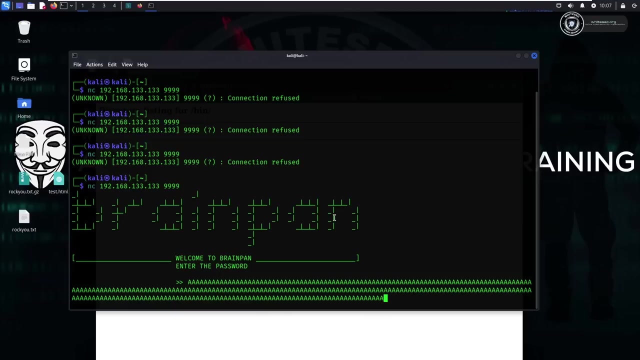 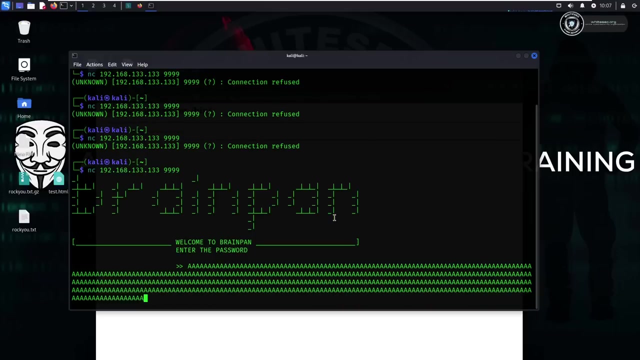 see, software is now running. go back here. let me ctrl c and let me type enter again. type here, verse here. so here it is now. let me send yes here. okay, see now what will happen. okay, let me send it as it's denied. i need to send more here. let me do it again. 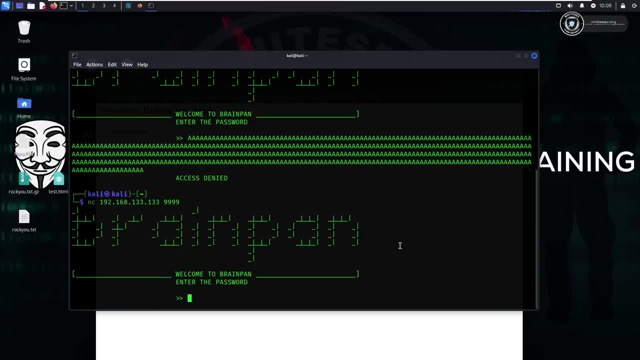 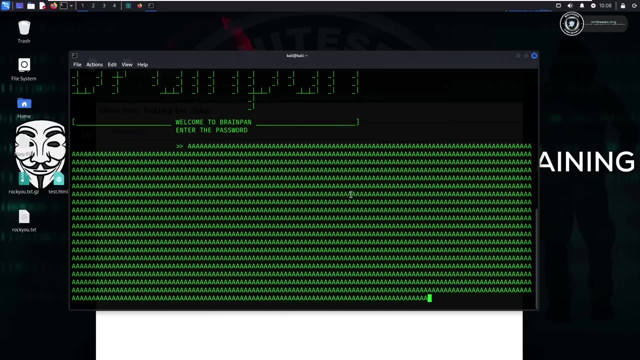 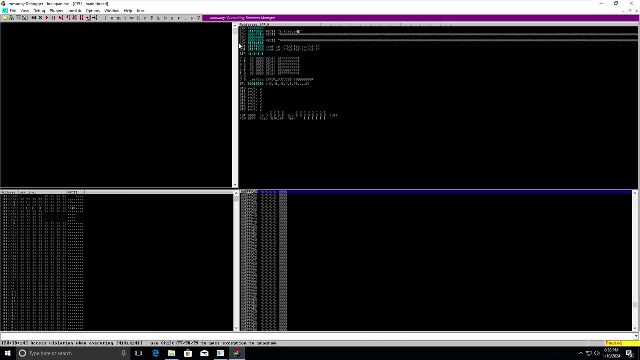 copy type: enter. now it's what happened. the software has been crashed. just see here in. i gonna load all of these, copy and paste what you want. okay, press anything that is damaged. okay, i will just slow down some bit and just select all of these all team. 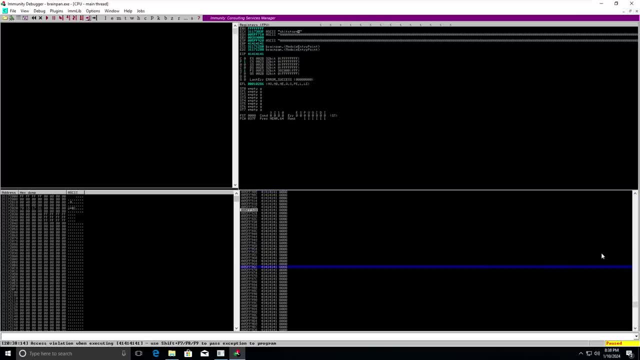 and guys, what you will see now is when i am putting a stack block in here. i want a rows folder. what is this? MountainOS manager? you just seek here and that is a block. now look at that all here and that vector here read 것을 view. there is a, edX is filled with what is here and here is what is esp. also filled with a here and also seen stack also. you have also, you see, in stack here in hearing is also filled with a and the value you see, the total figure is just the value here. value is what: 441414 1, what is for one. basically, let me specify, let me see that here your no theypot, almost here we will you. 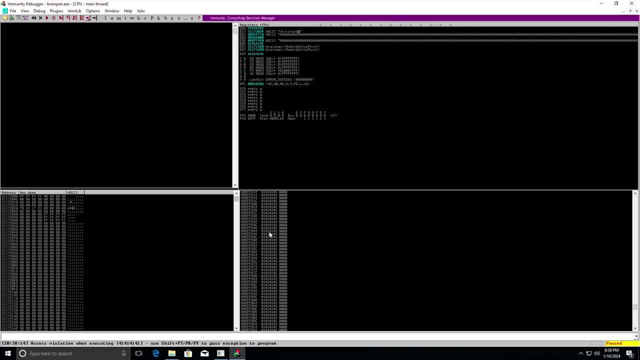 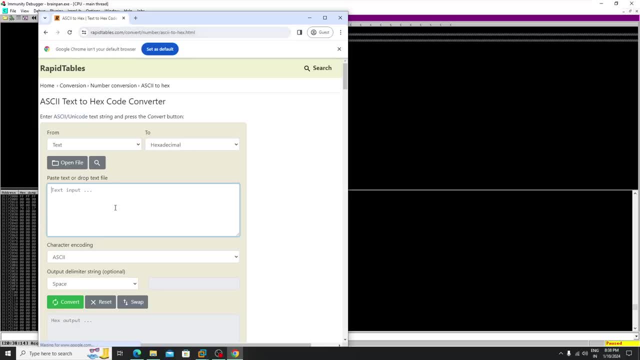 say, let me show you here, see, just visit this website, which is ascii to hex. okay, here, if i type capital a, then see the value here. if i convert this uh value, then what, what you can able to see? you can able to see 41 here. okay, this is a thing, right. if i type another a, then you can. 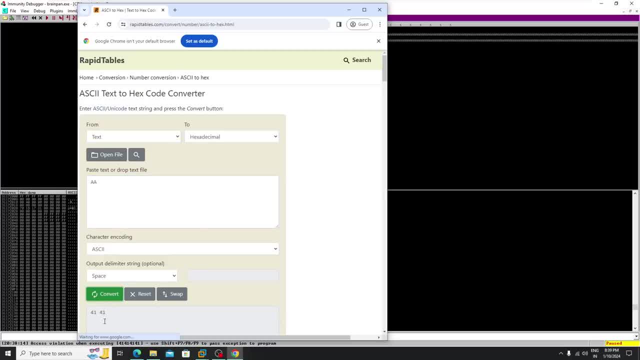 able to see 41 again. this is a thing. basically, if i type here b, then what you can able to see. sorry for type capital. i am using the capital for small- the value will be different. okay, see here, the value will be 61 for a small character. if i am using the capital one, then the value will be. 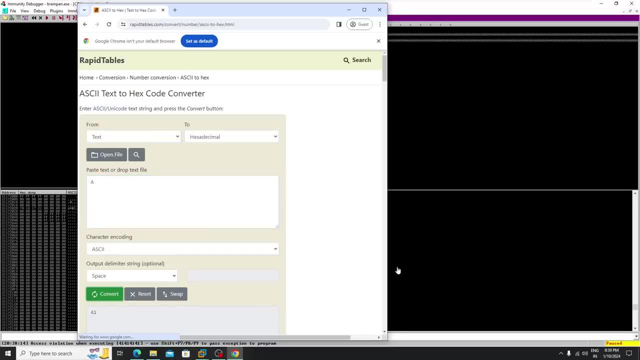 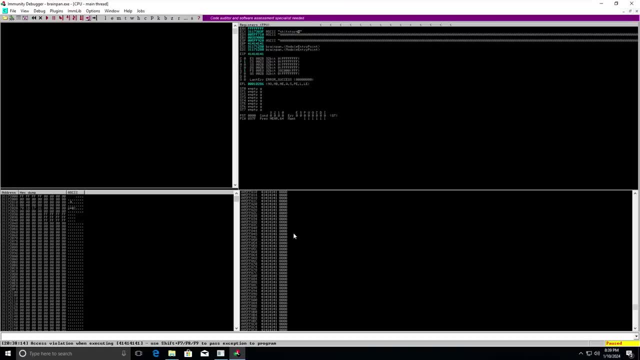 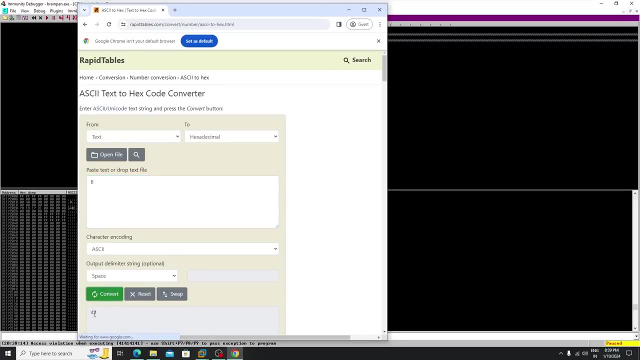 41. so that's why i can- uh, i am seeing here 41. this is a thing, don't be confused here, okay. so that's why i'm doing. just try to practice it. see, if i use a b, capital b, here, then what is the value? value is 42 here. this is a thing. if i use a small b, 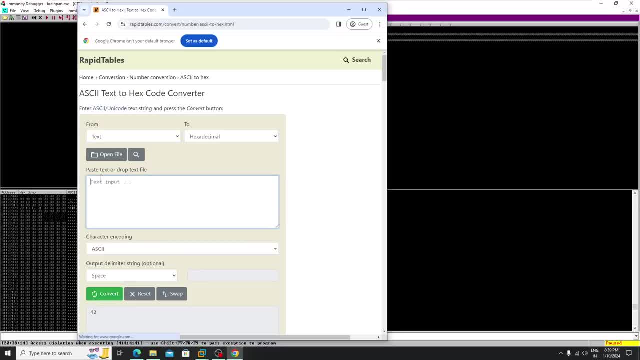 b, then the value will be 62 here. this is a thing, right, hope you guys get it. basically, we are converting ascii to hex. okay, right, just just remember this website. okay, this is very useful for you, right here. if i try to see, if i try to play this one, then what? what i can able to see? 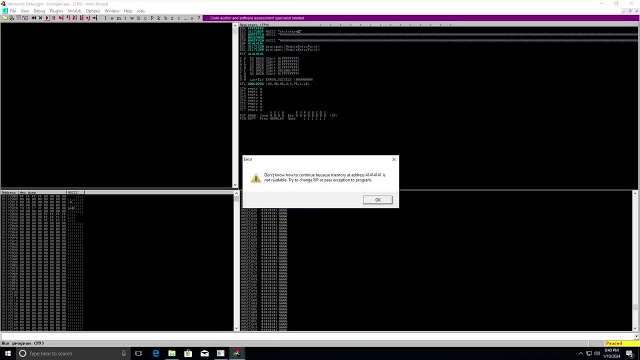 don't know how to continue because memory at address 41, 41, 41 like a, a, a is not readable. try to change eip or pass exception to program. see here i just showed you in the last classes as well. the eip, this one, the eip register, hold the address of the test instruction to be executed by. 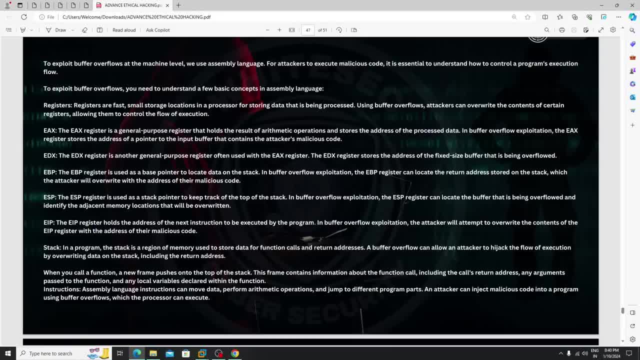 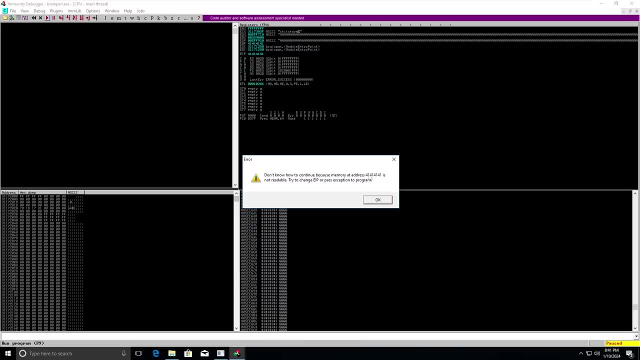 the program in buffer overflow exploitation, the attacker will attempt to overwrite the contents of the eip register with uh, with the address of their malicious code. basically, it will tell you to uh to tell that where to go next. okay, this is the thing here. so, basically, right now the eip is overwritten, uh written by: as here. this is the thing right. 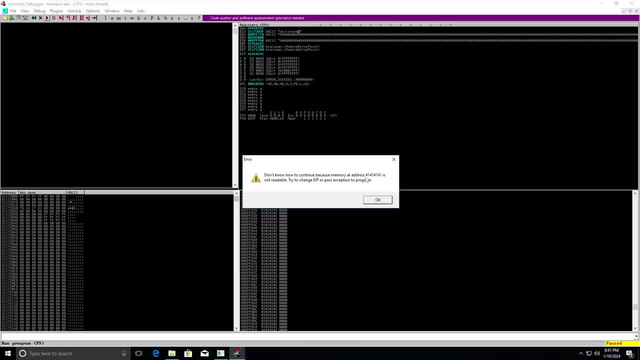 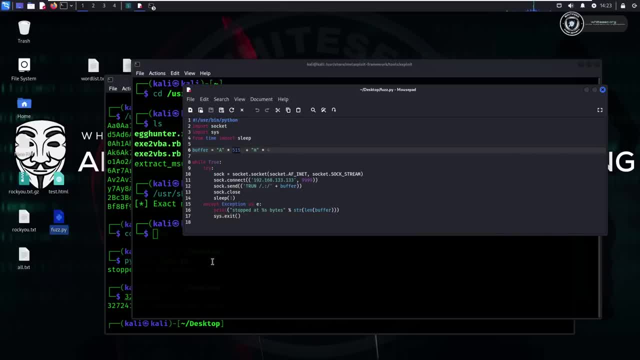 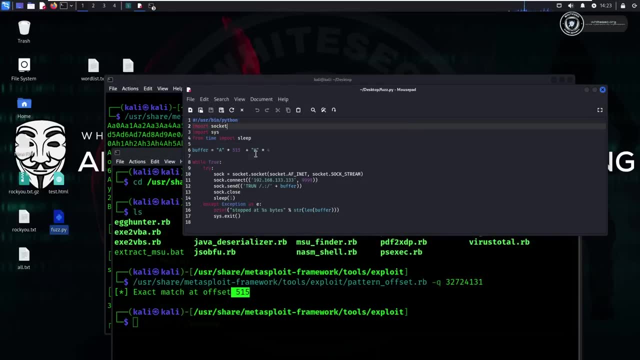 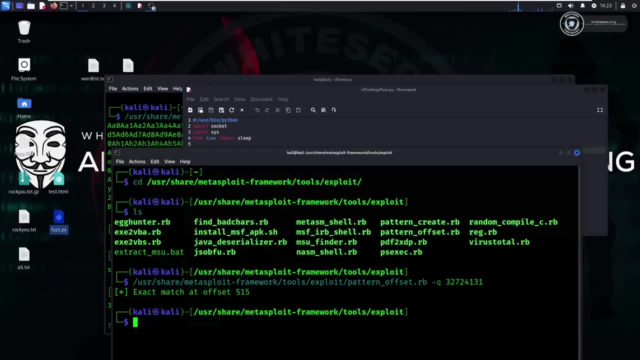 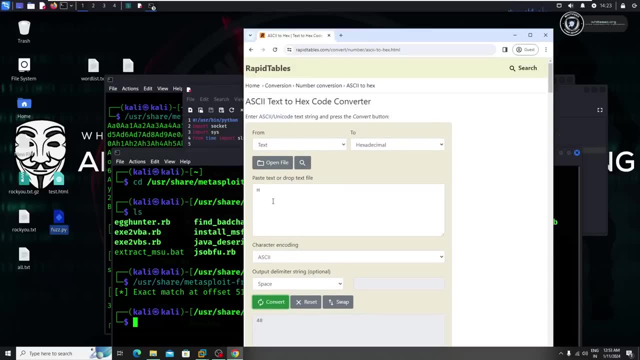 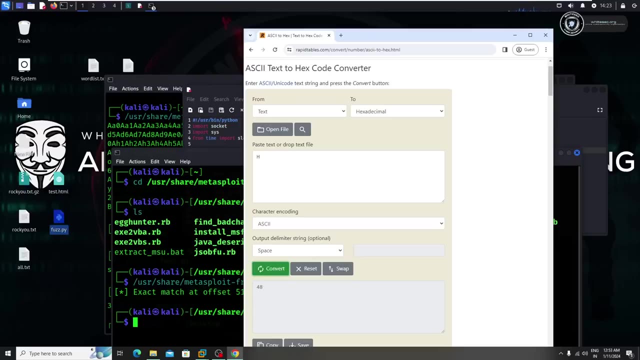 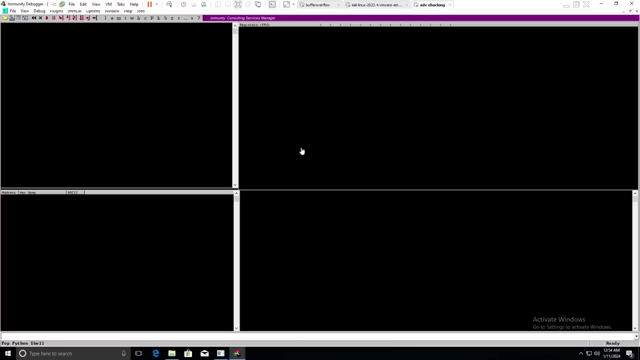 see in ascii. sorry guys, if here you guys can able to see the: the hex value is what? here it's a 48, right, so after executing this script the eip must be uh, 48 there, okay, 48, 48, 48, 48, 4, 48, 4 48. that means 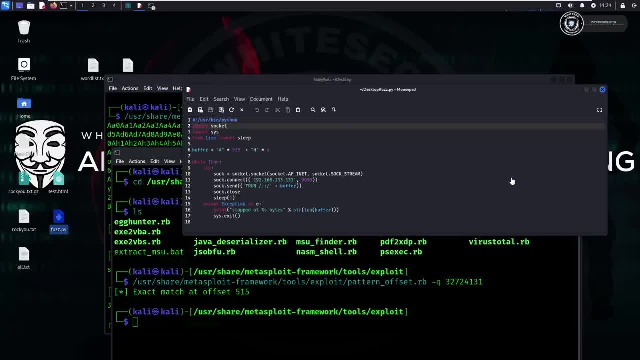 4h. okay, this is the thing now, simple. just remove this one as well. uh, in previous class, we just changed uh changes to half set, right? just uh, rename it to buffer there and also remove this one as well. uh, in previous class, we just changed uh changes to offset, right? just uh, rename it to buffer there and also remove the. 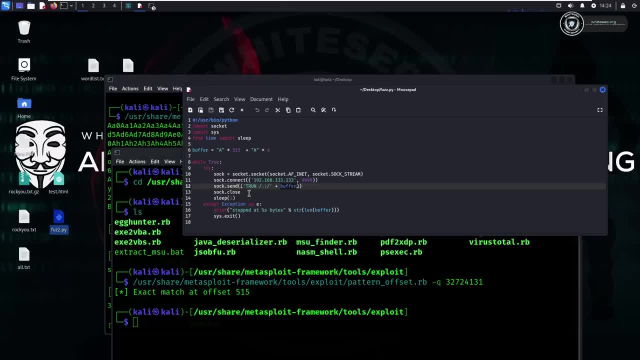 the line which is: uh, this one buffer is equal buffer. we just uh, there is one line, one line is there? just, uh, just remove that line. okay, that's it, just save it. okay. see here, i just added only four, because i just told you, right after 515, the next four values will be the eap, the exact location. 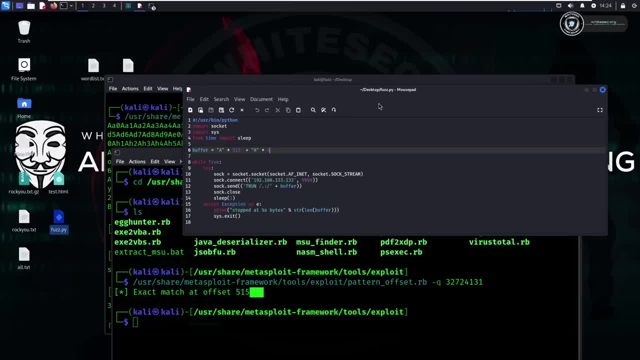 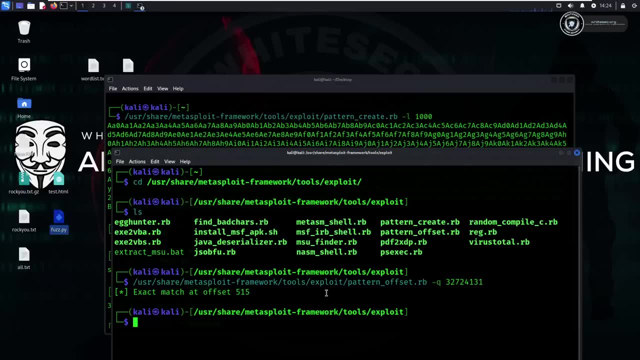 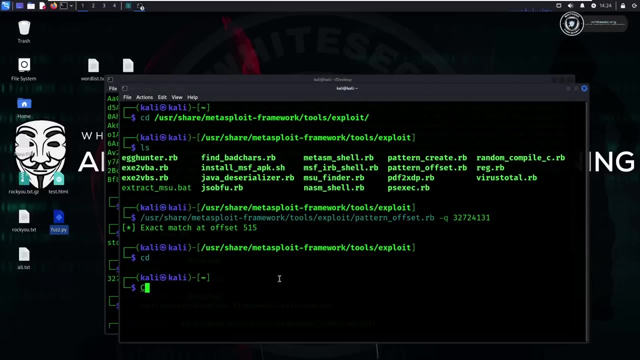 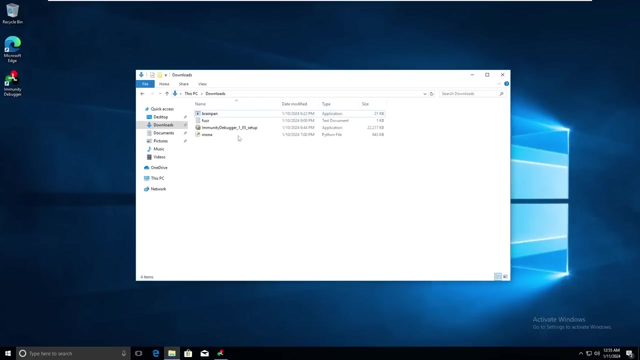 this is a thing. so here, what you need to do, simple: save it. after saving it, just let's go back here. this: let me type cd now. let me type here cd desktop. okay, now, before doing this process, let me do one thing here, do it again. so, first of all, let me run this brine pan as run, as administrator. 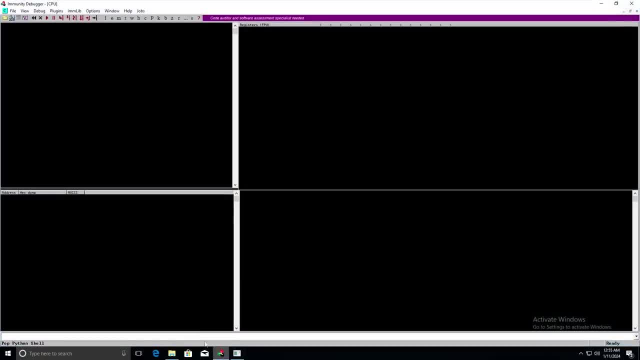 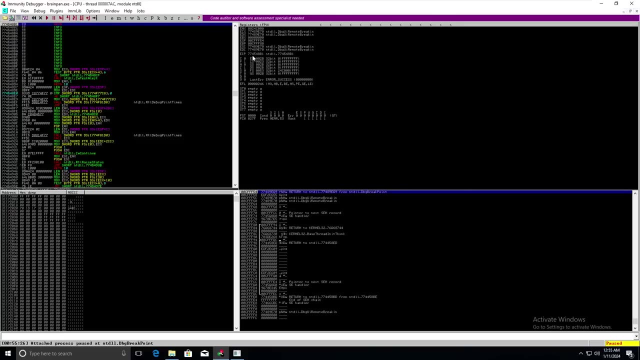 and here click on file, click on attach. let me select brain pan here. basically, we are taking control on eip here. right now the eip is what 77. previously, in the last classes, the eip is different. okay, because i just loaded it again, so that's why it has been changed. okay, now the simple thing is just see what will happen now. 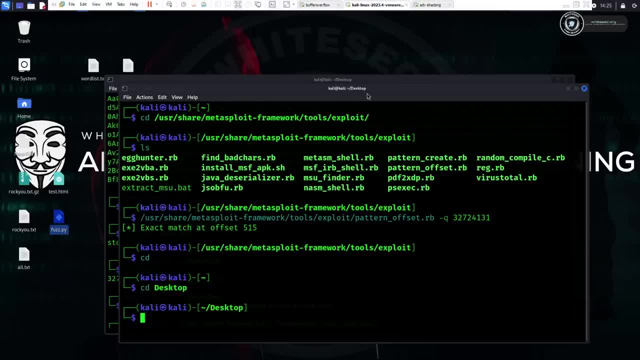 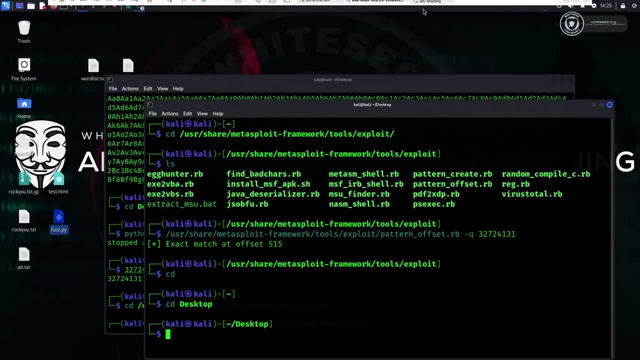 my aim is: i want to control the eip here. this is the thing: after controlling the eip, what will happen? okay, assume that i successfully right now, if i successfully control the eip, and what will happen? i can able to execute the malaysian codes here. okay, now see in ascii: what is the value here? 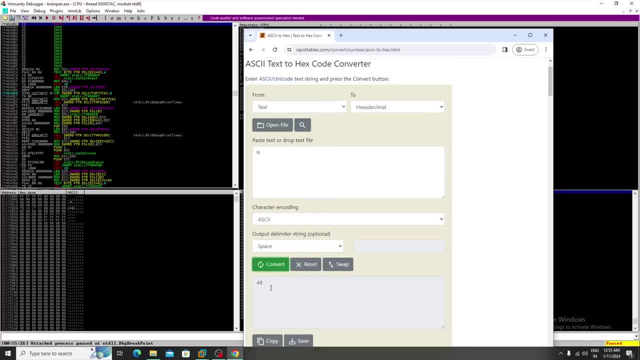 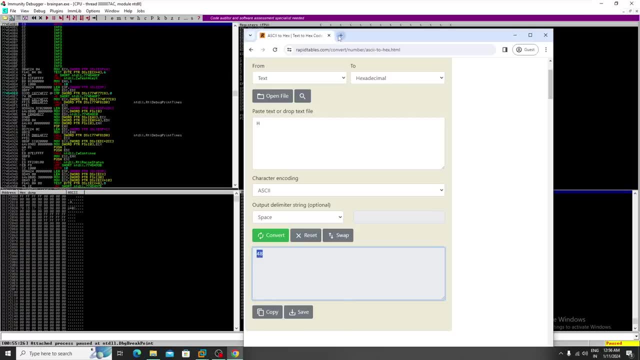 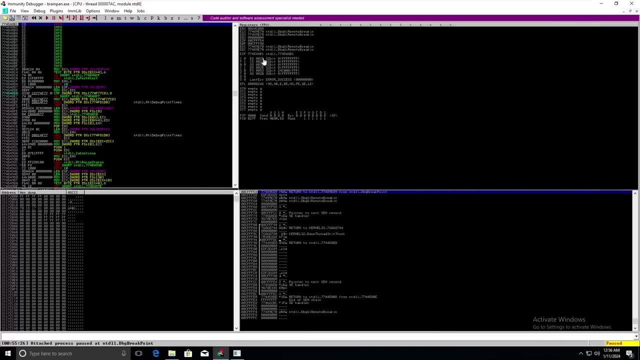 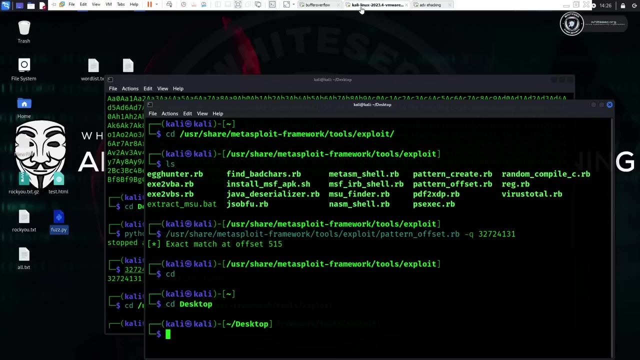 the hex value 48. okay, now i want to see something like this in eip, like this one, like this: 48484848 448. okay, so if i see 448s here, then that means i successfully take control on this eip. okay, so let's go back and let me execute. uh, this one, the first dot py after. 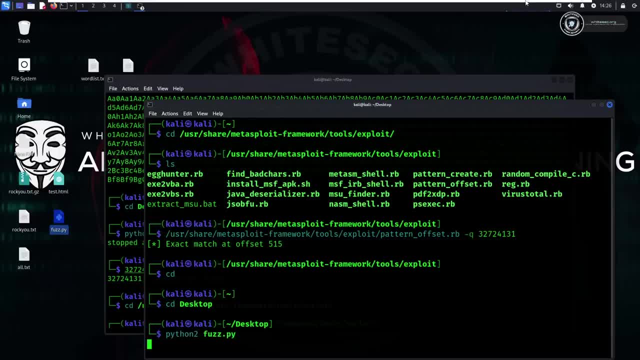 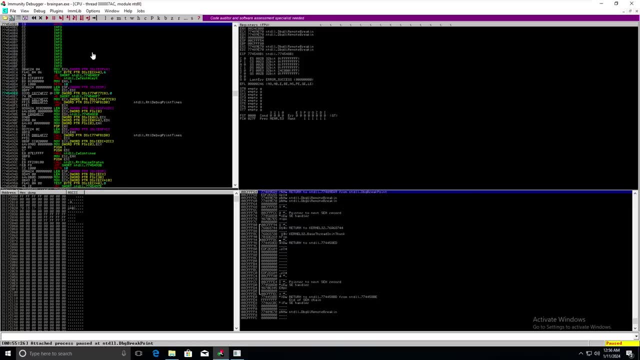 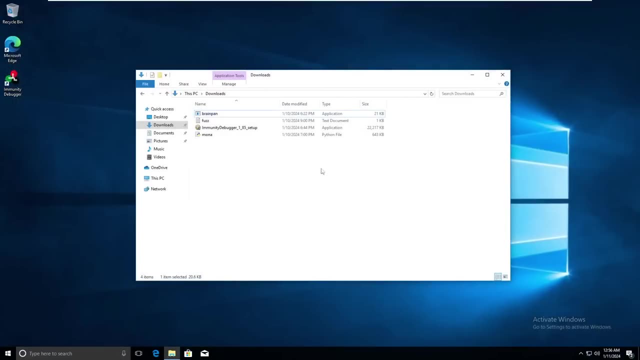 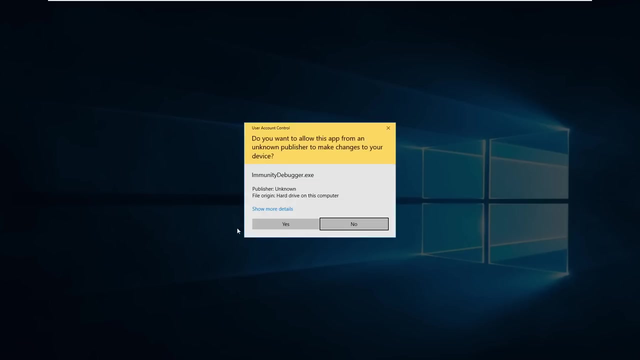 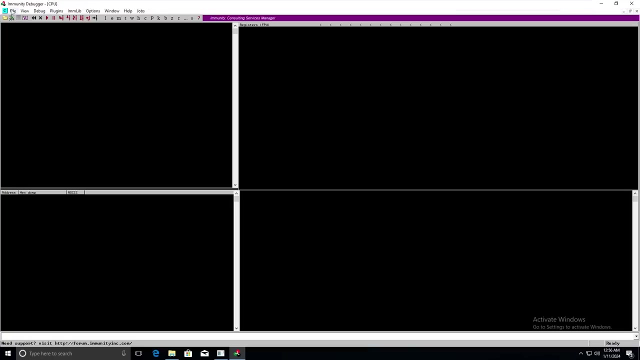 executing it. now i can uh: sorry, it's, it's passed, so i need to play it again. okay, sorry for that if i would close it. let me close it. okay, let me do it again because i need to run it. this is the thing: while dash like brain pan here, just click on run here. okay, play button. now it's running. 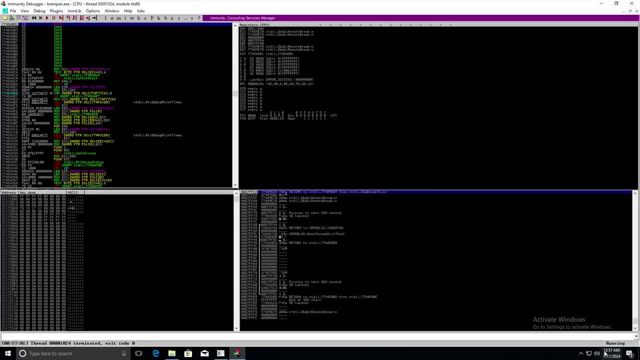 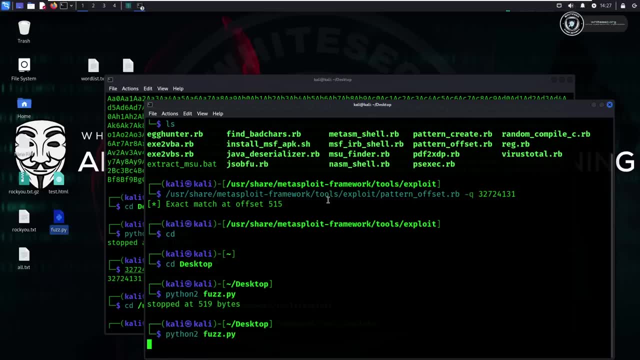 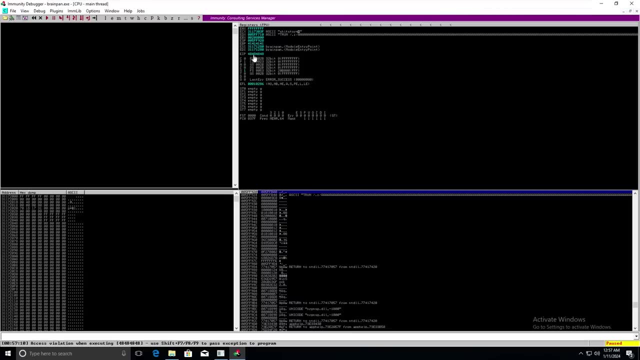 the last time what we did? it's a pass, so that's why we can't able to see it. so let me execute it now. see what will happen. let's go back. okay, see, the eip is what here. see, just focus on the eip. eip is 48484848, right, so i successfully. 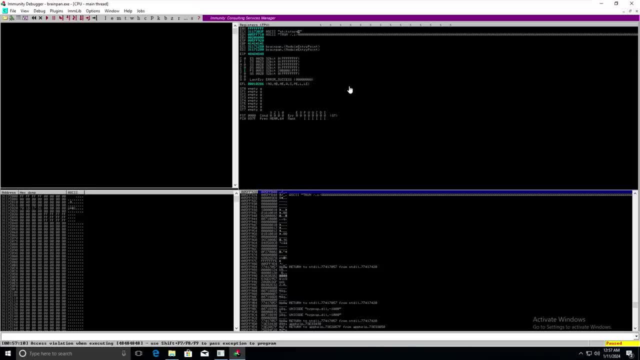 control the eip here, that means i can able to execute anything. okay, i don't want to send any kind of malicious scripts, nothing simple. this is a vulnerability here now, okay, this is the thing. see. again, i am saying, uh, if you are not getting the theory to do the practical, then it is more. 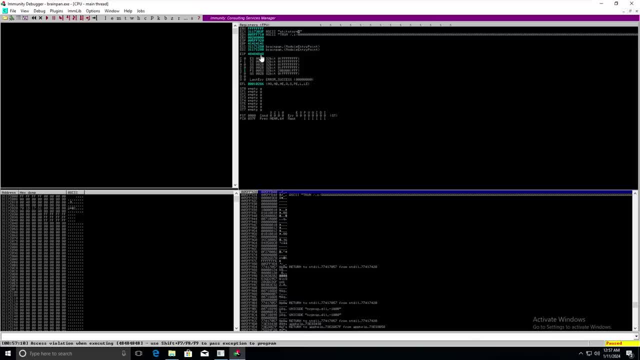 easier than theory. okay, this is the thing: just just execute the same things which i am doing here. okay, it's not a kind of rocket science. okay, easy man, that's it. okay, i successfully got the eip here again. i am saying i just told you what i need: this one: 484848, four times. see, i got 48484848. 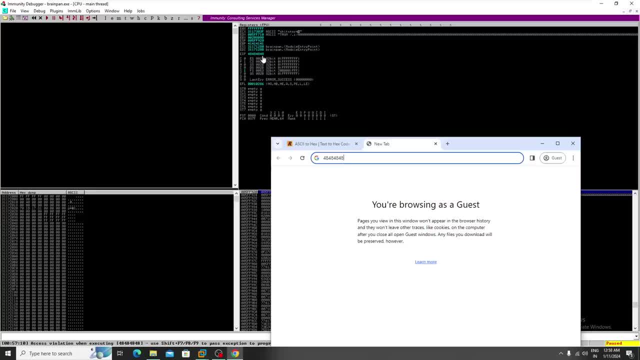 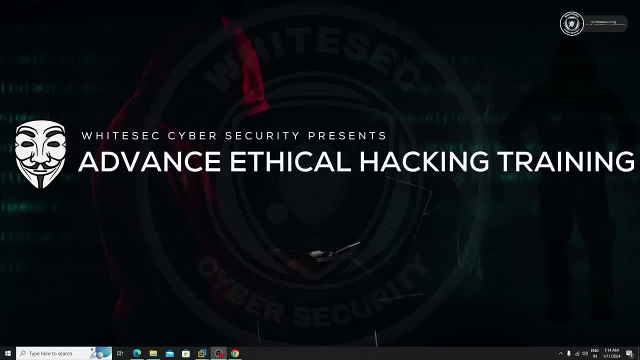 four times. this is the thing, so hope you guys get it in the next classes we learn more. hello guys, hope you're fine in class. we are learning about bad characters. here is a definition. just try to read it. what is bad characters? you are learning about bad characters. 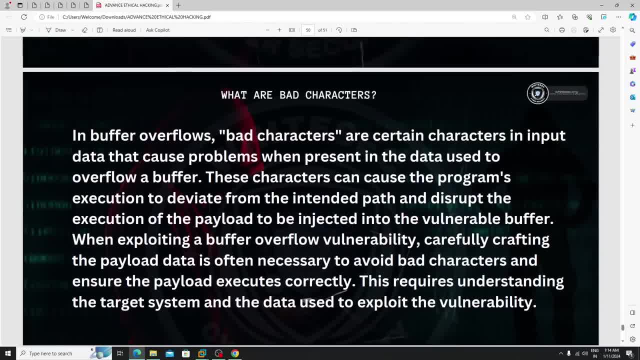 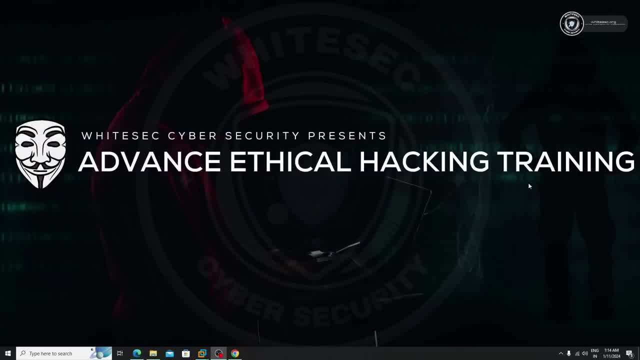 characters. okay, and here you can also see the examples. okay, for every application, the bad characters are different. okay, this is the thing. now let me explain you and let me show you, uh, how you guys can able to figure out the bad characters and how you can able to remove them. 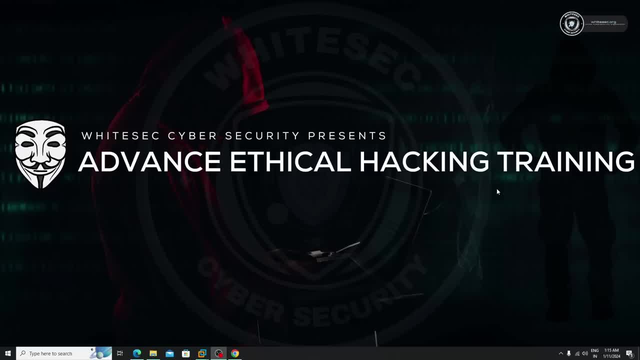 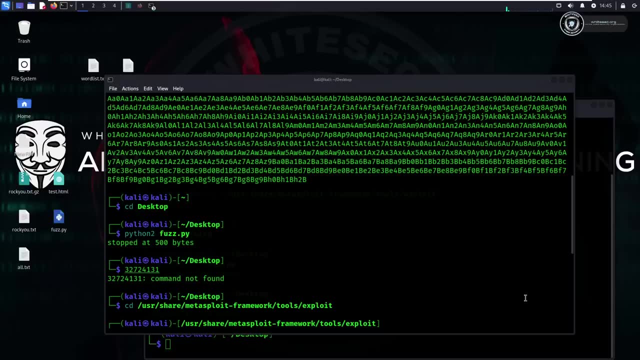 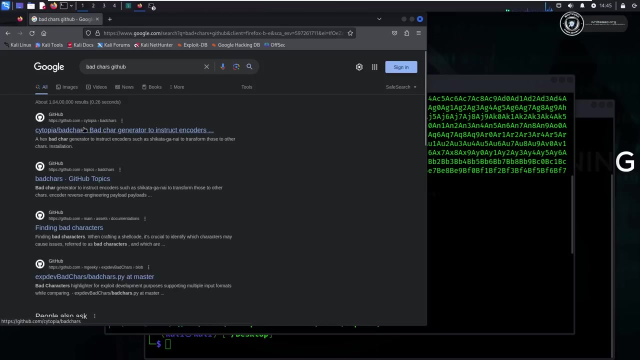 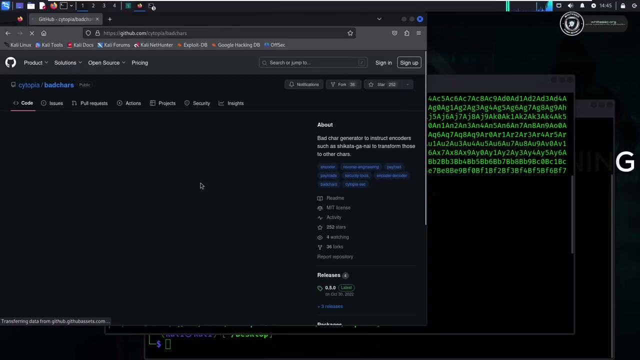 each and everything now here. what you need to do is, it's passed simple- open google, sorry, and search for bad characters. github, first of all. you will see first link here of github page. here you can able to see the bad characters. no need to download the script here. simple, this is enough for you guys. 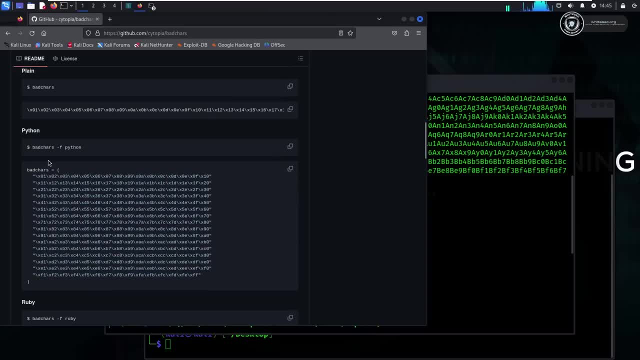 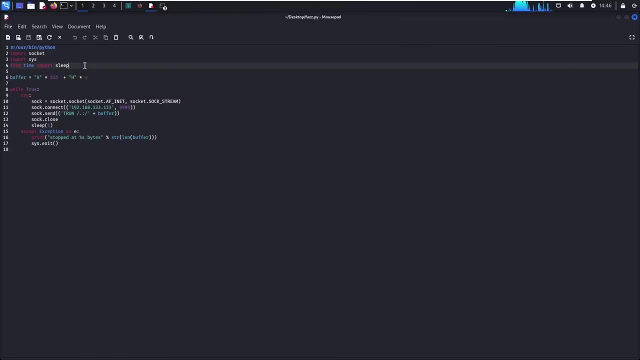 this is for uh python, right, so simple, let me copy it. just open first dot py here. just let me paste those bad characters, okay, and let me add this: give space and add characters, the same variable name like this. now, the simple thing is: paste it now, save it. 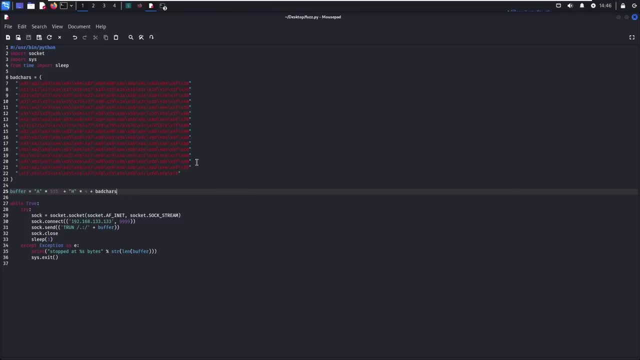 it's not a big deal again. i'm saying simply: you need to copy from here. just paste it, okay? see it's starting for from 0, 1, 0, 2, 0, 3, 0, 4, 5, 6, 7, 8. 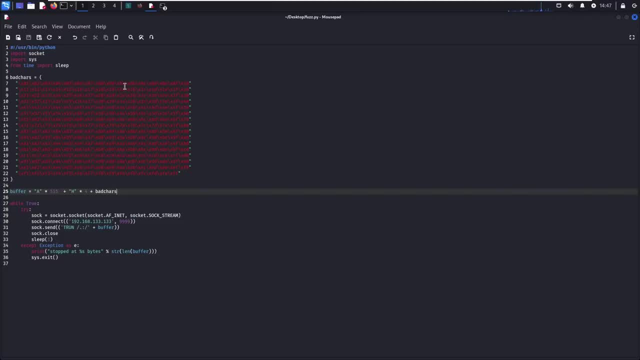 after 9: it will start with a 0, a 0, b 0, c, d, e, f, 10, 10. okay, then 11, 12, 13, 14, 15, 16, 17, 18, like the it's starting. okay, this is the thing. 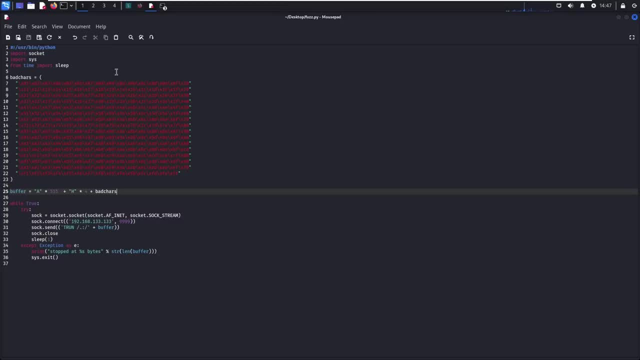 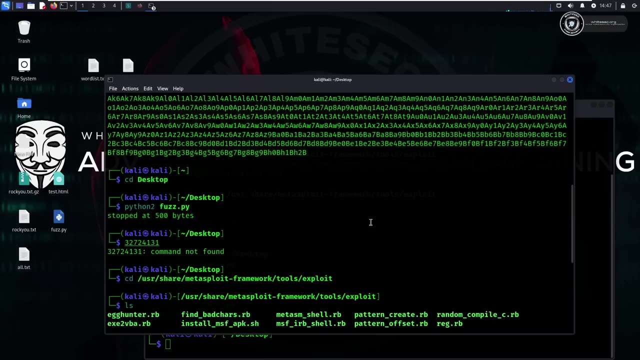 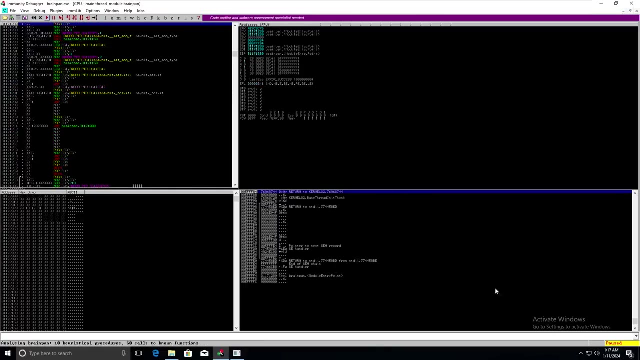 now see here, Just save it, close it and let's go back here and let's play this one. It's running Now. it's running. just see. Now let's go back here and let me execute this firstpy and see what will happen now. 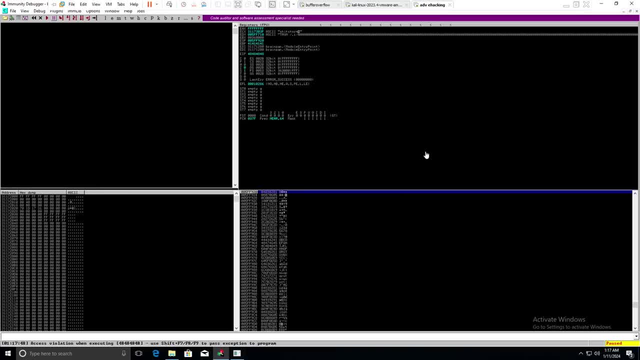 So simple. just see the ESP here. ESP. just see here. just try to zoom it and see it. okay, ESP. and here, just click the value and click on follow in dump. okay, So see what is ESP. just see. just read the definition again here. 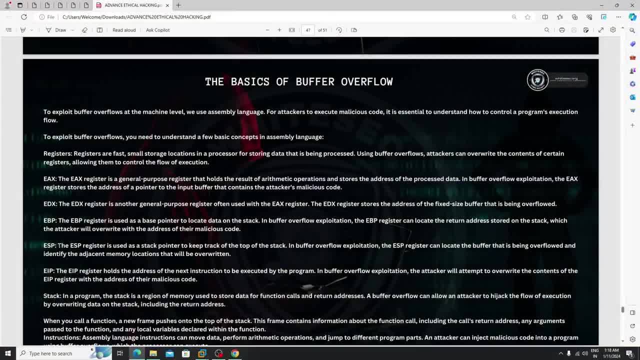 What is the ESP? The ESP register is used as a stack pointer to keep tracks track of the top of the stack in buffer overflow exploitation. The ESP register can locate the buffer that is being overflowed and identify the adjacent memory location that will be overwritten right. 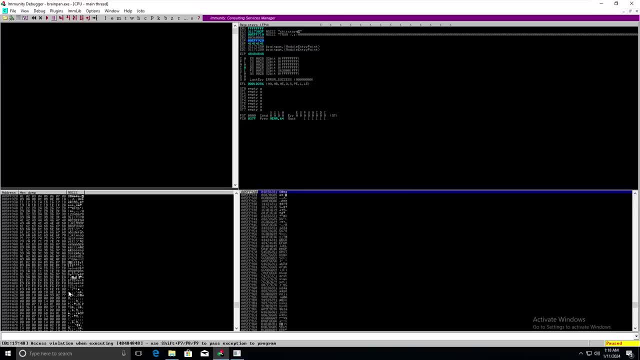 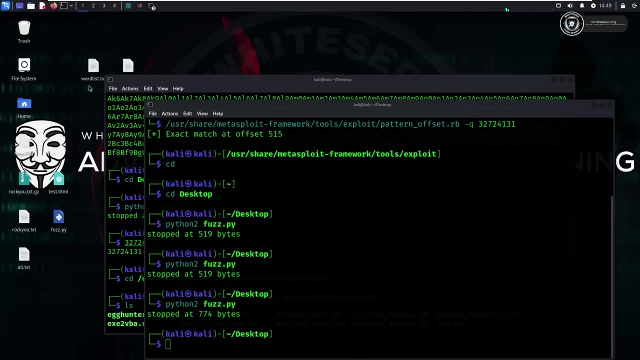 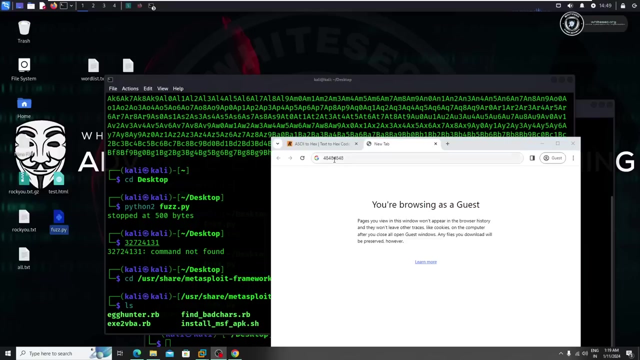 So here now, what you need to do basically means you need to compare this results. okay, Let me show you. You need to compare this. compare this results with this one, with this bad characters. okay, Just wait, let me Open here. right, so you need to compare this which one? we just take python, right, so just, 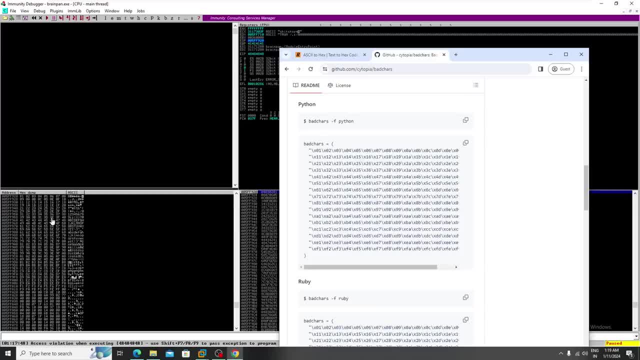 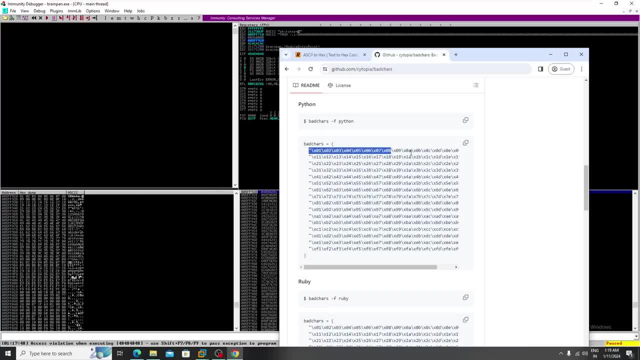 Then it's right. Then it's right. Then 0 a 0 b. Then it's not right. Then 0 a 0 b. Then it's not right. Then 0 a 0 b. Then 0 a 0 b. 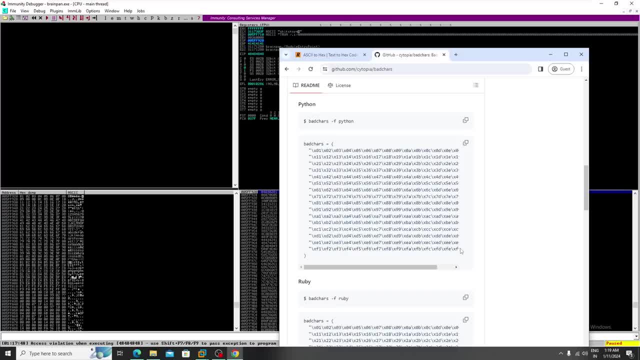 Then 0, a, 0, b. Just see these things. okay, you can see the x there. this is the thing. see the values. it must be same. assume that any value has been changed. see, assume that there is a x, 16 is 0. okay. 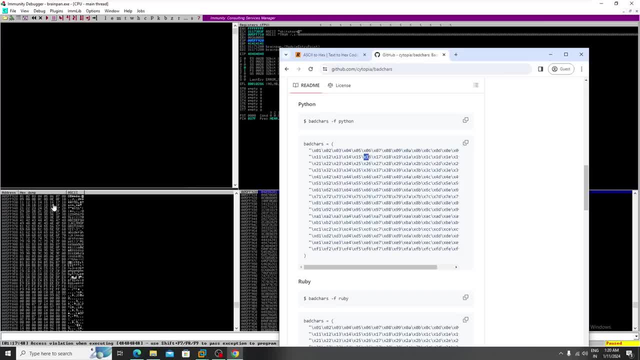 Let me see x 16. you can able to see the x 16 in dump, right, so just see the mouse pointer here. x section is there? okay, here it is assumed that after uh adding this, bad characters, what will happen means instead of section. you will see something like uh, uh 14, uh, sorry, instead of 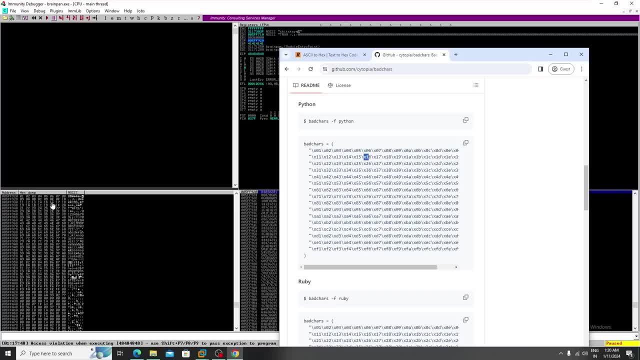 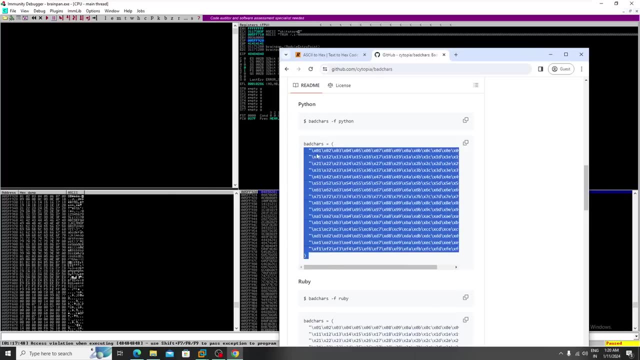 section, you guys will say you see some kind of such as 0, a, any kind of things. okay, instead of see, it must be follow this pattern here. okay, here also in dump, it must be follow this pattern. if it's not following this pattern, then, uh, there is a bad characters, are there? you need to check. 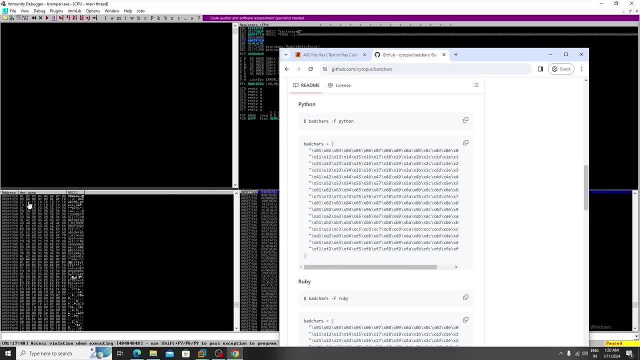 this manually. okay, this is a thing like each and everything must be same. like there is a 0 1, here also 0 1, is there 0 2, here also 0 2. like this: you need to check. assume that any value has been replaced in this dump. at that time it's a bad character. simple copy that value. 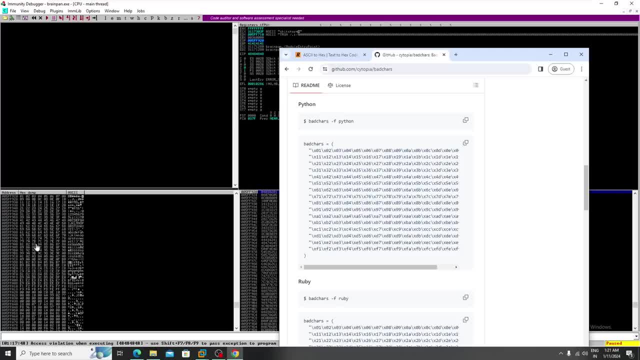 and paste somewhere. you need to uh modify it. okay, this is a thing, you, it's not a big deal. again, i am saying you need to focus this thing, okay, this bad characters sometimes: what will happen if you uh take other uh softwares or any other application at the time? 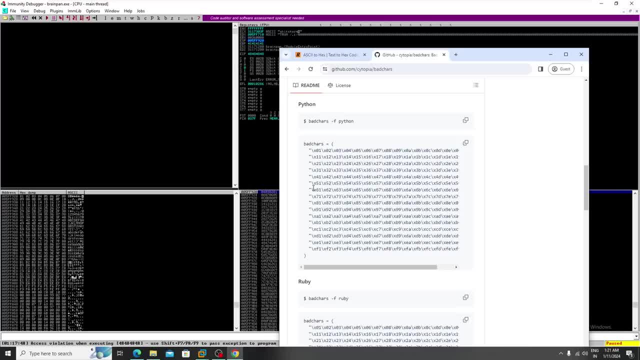 maybe the bad characters will. uh, it won't follow this complete thing here. okay, maybe in middle the values will be changed like there is a 67 instead of 60. uh, 67, it might be 41 or something like that. it comes under what this it needs to be. 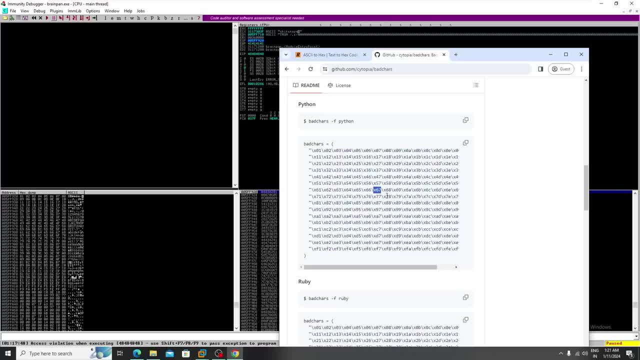 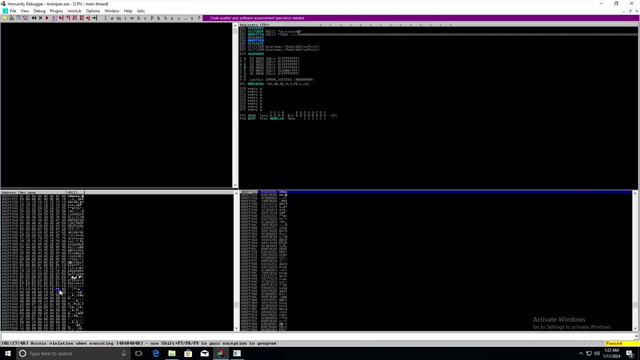 test this thing only. okay, it needs it. it need to follow the same thing which is here: right if its ending. faría till f if iff, right. so let's see, is there? see, here it is ff, right, here is ff, but successfully. uh, there is a nothing and uh, it successfully added. okay, this is a thing. 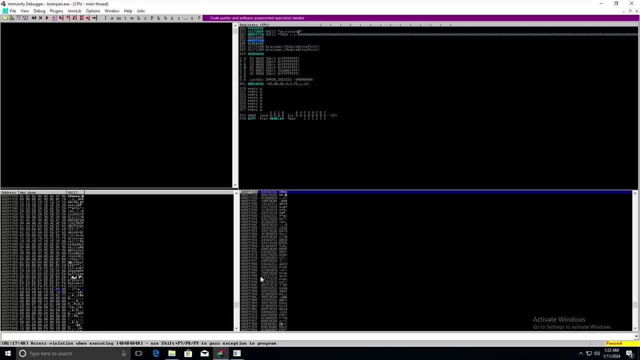 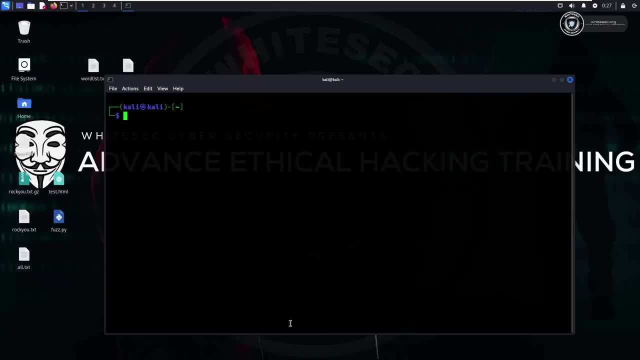 hello guys, hope you are fine. in this class we are learning how we can able to get a return address. last classes we learn how we can able to identify the bad characters, how we can able to take control on api as well. now, here the thing is, the challenge is we need to get. 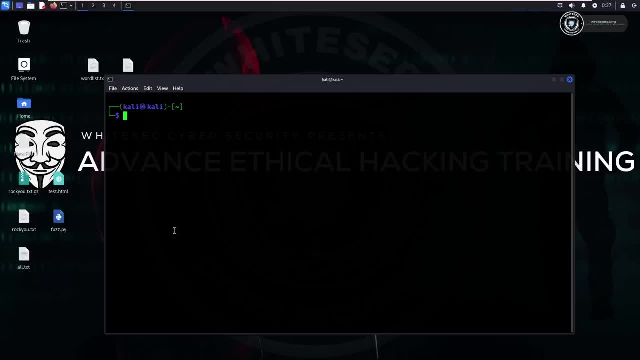 a return address here. how to get a return address? the simple thing is you need to use this script, which is nazam, underscore: fill dot rb, say ruby file, just type enter and just type this command: jmp, jmp is a nothing but jump. basically, here we are jumping to esp. 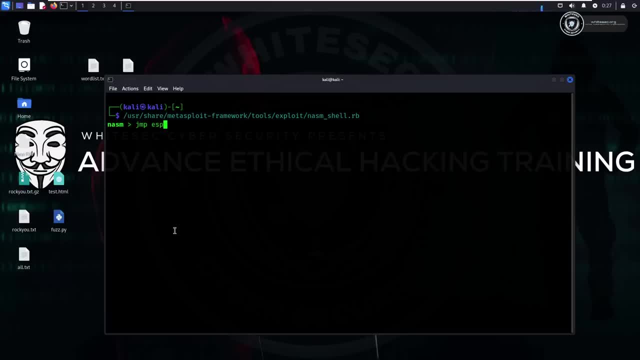 here. ok, here you will get the address, which is ffe4. now lets go back to windows machine. let me do one thing. ok, just try to restart it. see, you can also restart this. ok, so here you can see that we have got a return address and we can able to get a return. 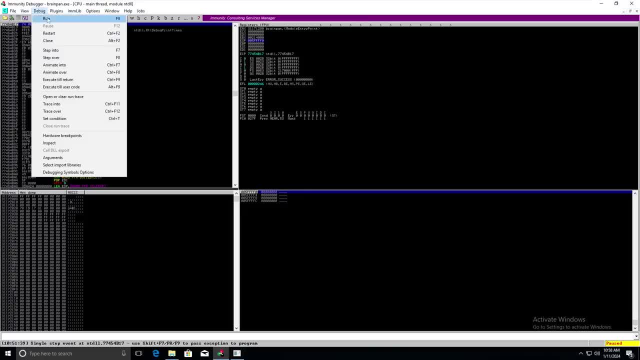 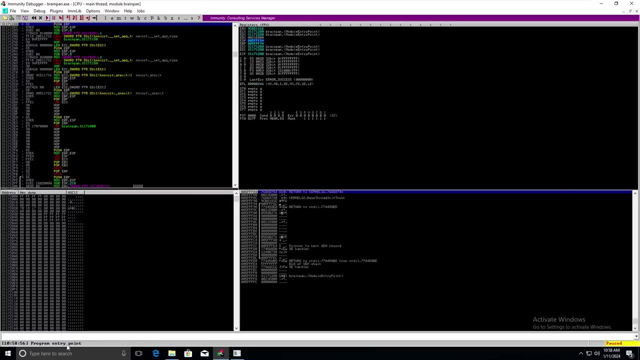 address. just simple click on debug and restart it right now. we successfully restarted this one now here. ok, this one now. there is a search bar. basically, here just type cban, mona modules, you type this one and if you hit enter here, then you will see that you will get a return. 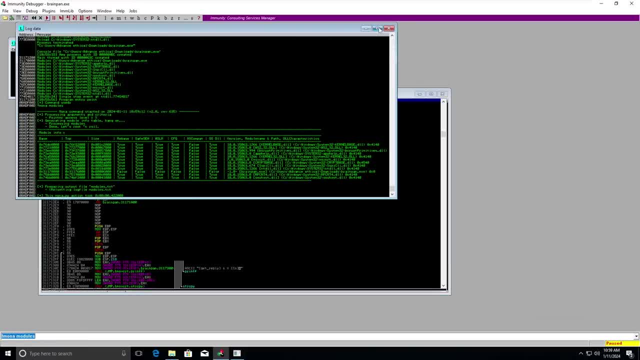 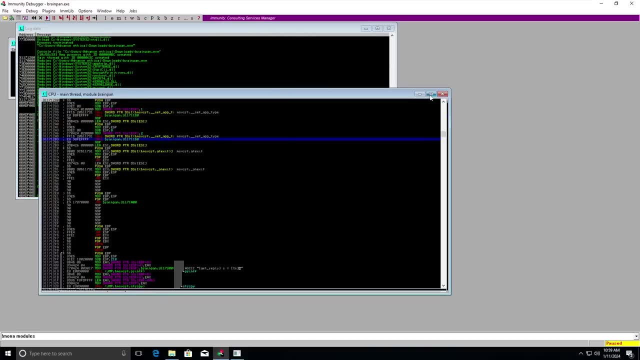 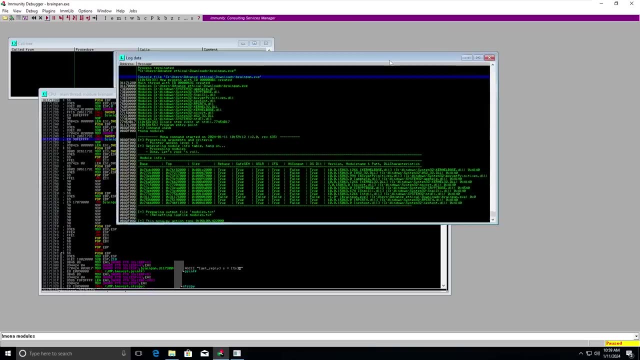 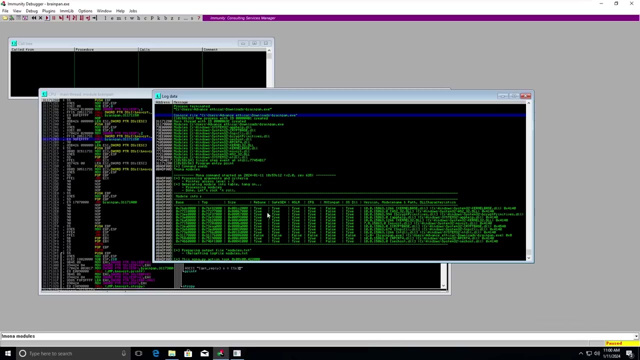 adress, which is rmb. this is where the return address is actually come from. let me just write the return address we want to hand over. yes, now we got our return address. don't worry, this is our release, the release part of. we have been forced to do this. how to, to to? 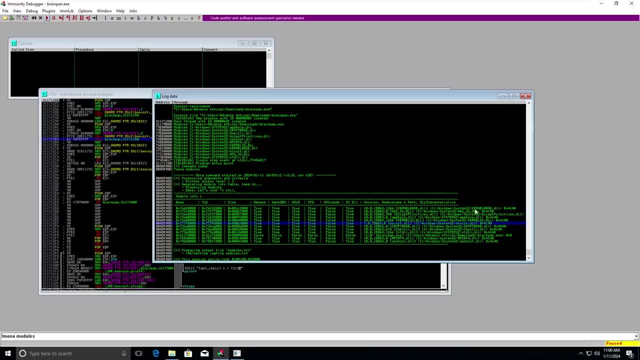 shift our data. basically we will need to to move this after know to the default Ultraselect file. use the things we can people at kakao output console. we can also do para time this us on this one, like: see there is a uh rebase, is there safe? seh is there. asl aslr is there. 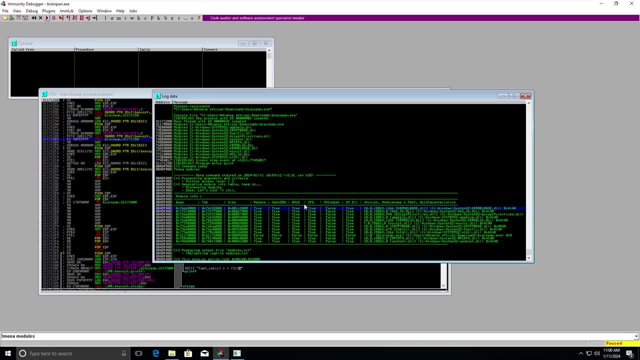 basically, if aslr, if these things are true, then it is hard to perform buffer overflow- okay, because uh may be huge confusing. if it's a kind of security here, okay, not kind it's a security basically right, by following some uh steps you can also bypass this aslr as well. 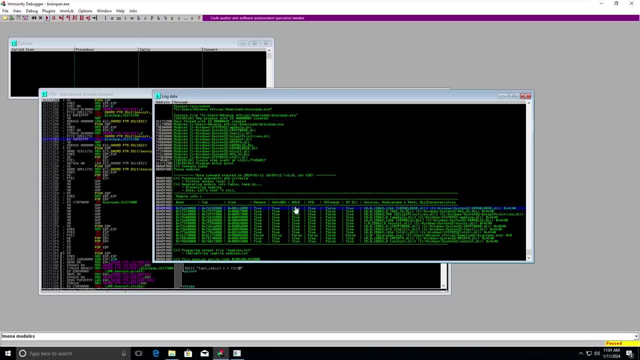 but the thing is here we are just covering the basic things. see, you need to select those which having the false, see in rebase, this is a false and any, any application. okay, from here you can select any file which having the everything must be false here, like here, rebase is false. 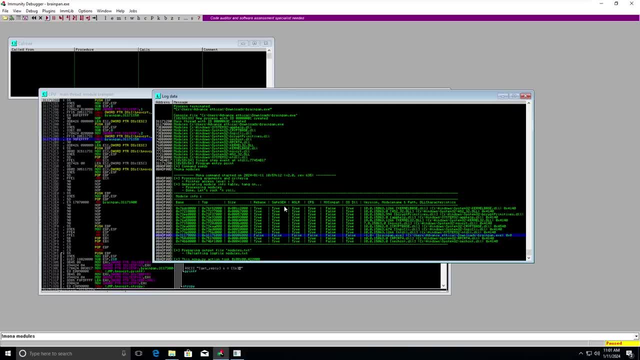 safe. seh is a false. aslr is false, okay. cfg is false, okay. you need to select, not a single one. just select everything which is having the false okay. now what's the next step? is that it's a brainpanexe? maybe, if you are targeting other applications, at that time, the 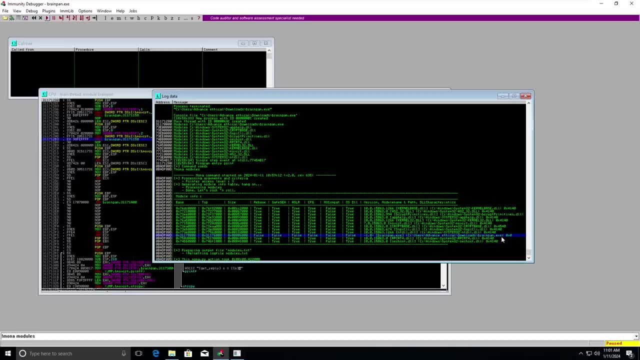 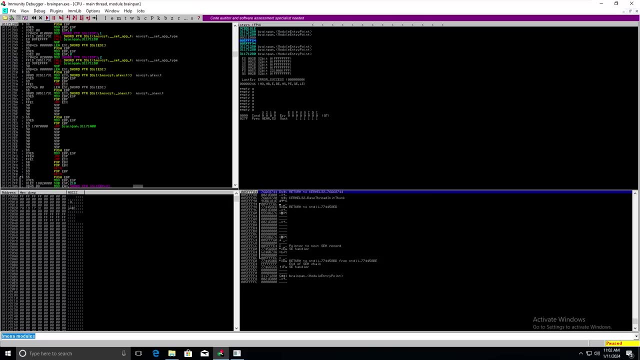 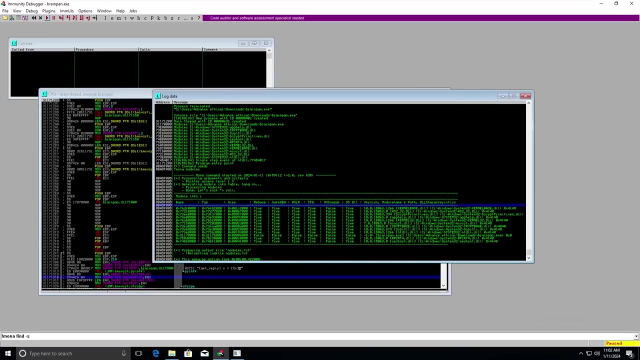 it might be a dll files as well. simple, you need to select it. okay, just select it. select that one. after selecting it, let's go back here and just type in this search bar, such as mona find, dash s, and see here. just selected it and just type mona find. 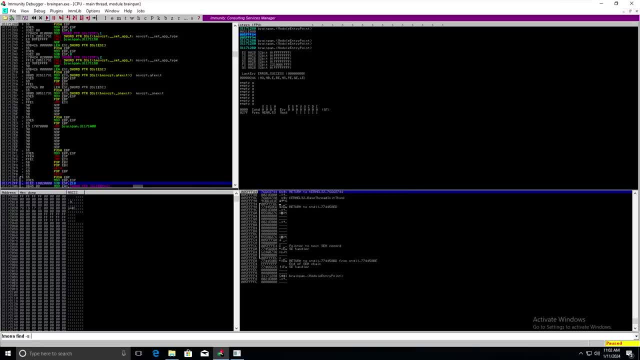 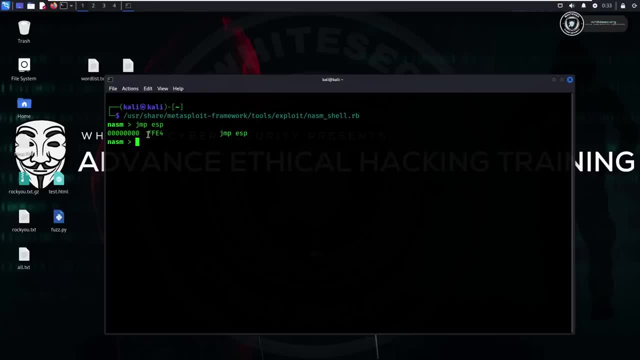 space dot uh, space dot, uh. dash s. go back to your kali machine, and here it is a address. okay, ffe4. now you need to change to hex value. this one like simple. you just need to add x in front of this. values such as: let me show you how to do it. 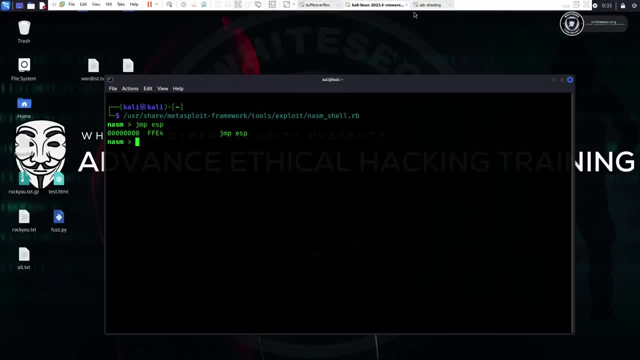 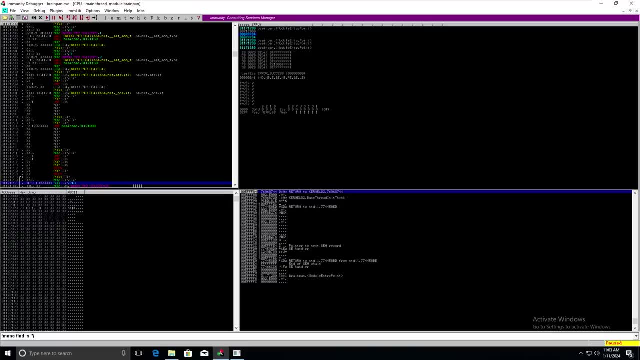 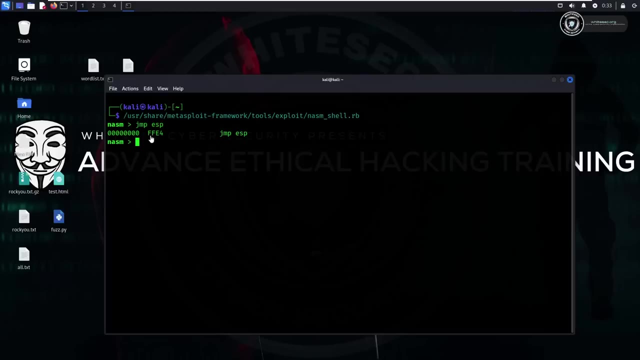 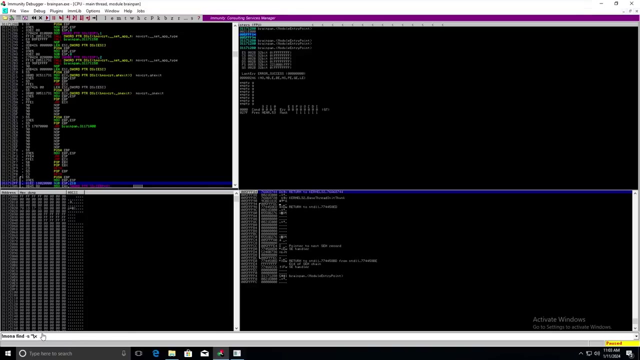 just add here: double good, just add backward. here the start x, here the value is what if? if it is a capital, OK, then ff, then back slash, and then what is the? uh, what is the? it's a value of e4. right, it's a e4. now, simple, just add x, then small e, capital 4. 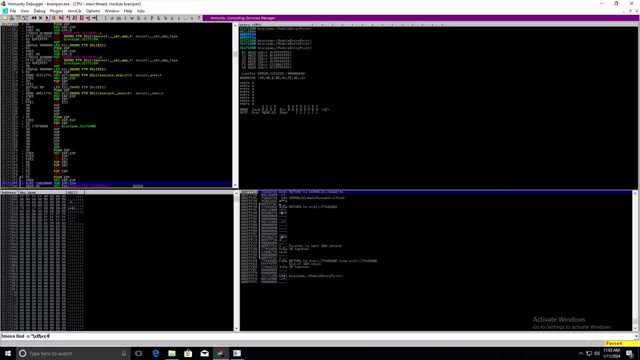 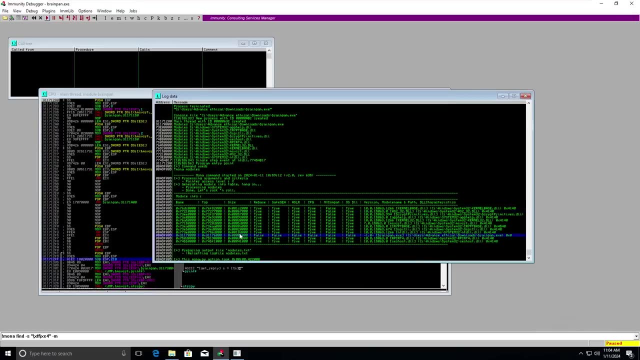 and just close with double quote here. then just type here: dash m. okay, dash m is nothing, but what here? basically, we are specifying this one here. right, you need to give the name. what is the name of that file? basically, we are giving the module there, the. what is the name here? the name is just. 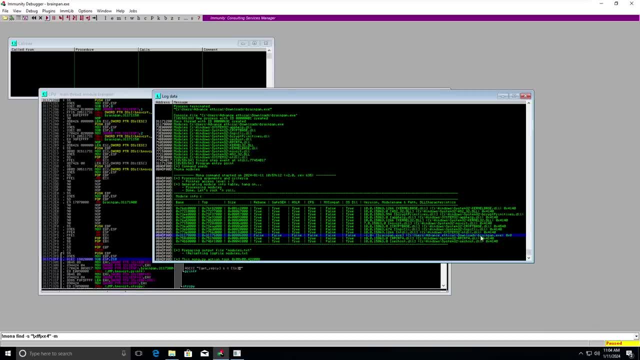 see, at last it's a brain pan dot exe. okay, again, i am saying it might be anything in your case. okay, you need to select the that files which having the false right, everything must be false there. you need to select that and you it might be anything like. it might be a dll file, it might. 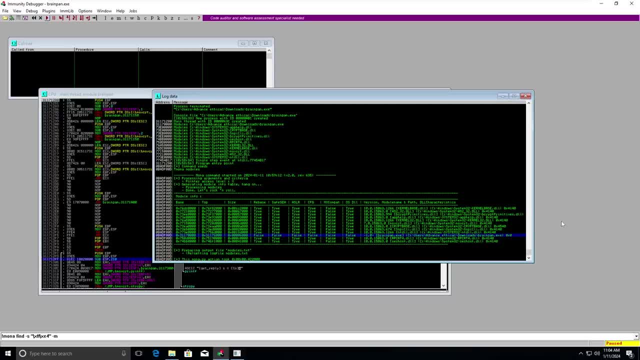 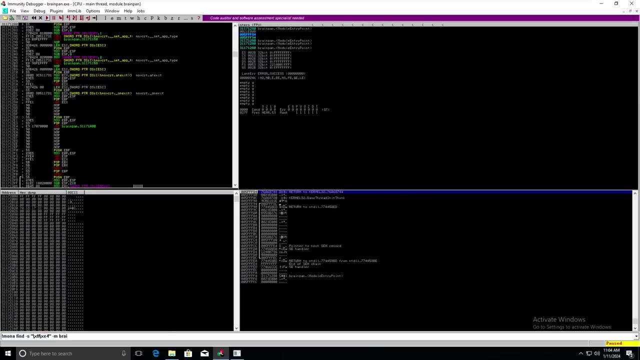 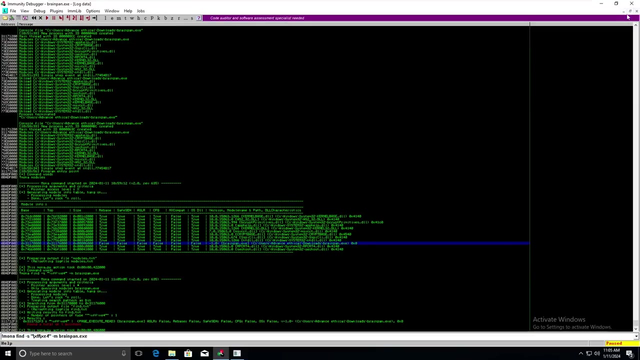 be a exe file. okay, you now simple. what is the name? it's the name is brain pan dot exe. type the name there: brain pan dot exe. now, just simple. just hit enter here. now, here you can able to see. okay, size is kind of small here. okay, now here you can able to see. 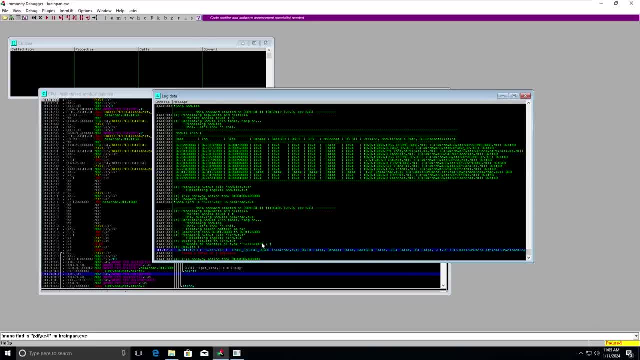 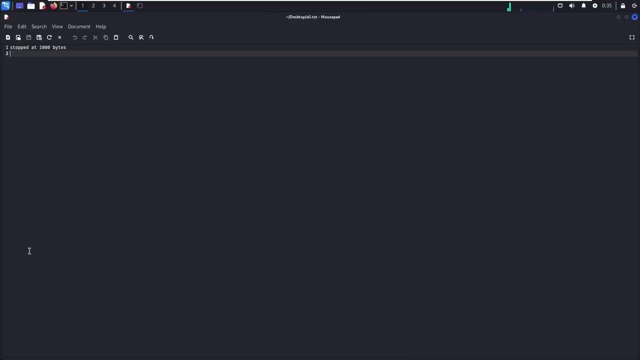 here there is a founder total of one pointer. now, here you got the. what a written address. okay, the thing. what is a written address here? hero: x31171 to a if3. okay, so let me write here right: result: zero x x, double one. zero x, zero x. 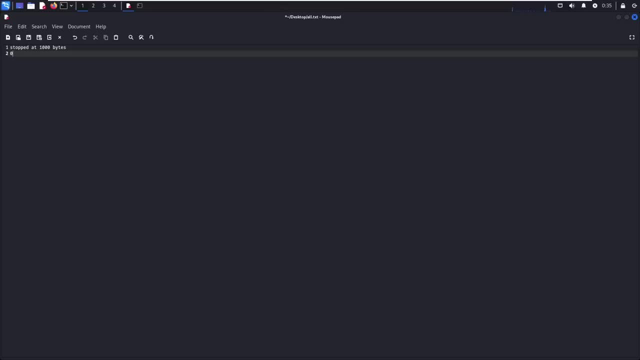 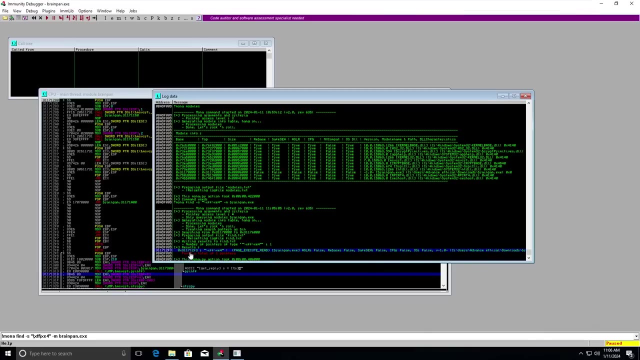 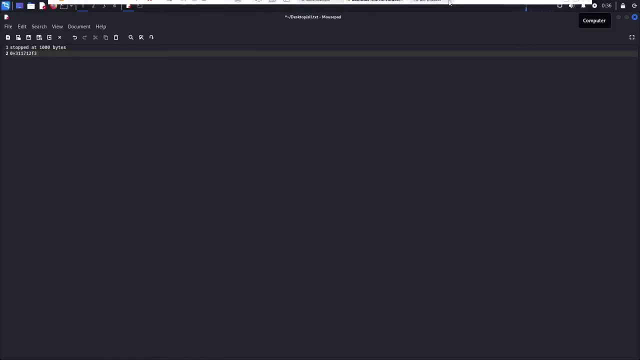 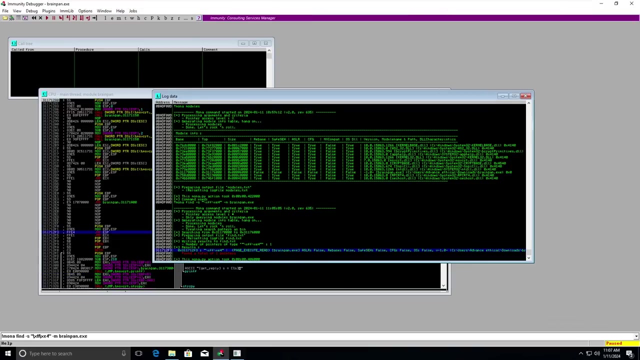 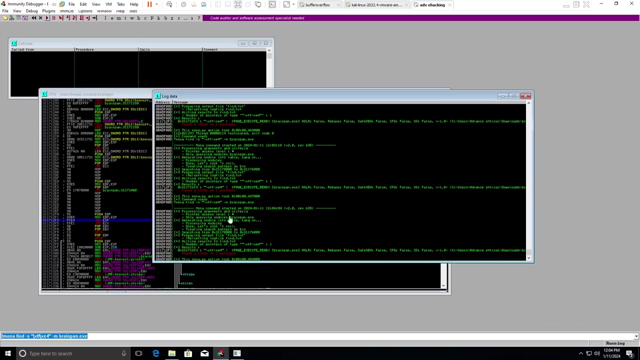 one, seven, one, two, five, three zero x 712. right, this address is very important. right here. we got this value right. 3117 1 f3 from here. they just see here. from here we got this value. simple thing is: let's see from where we we are getting this value. simple, just select this one, this line. 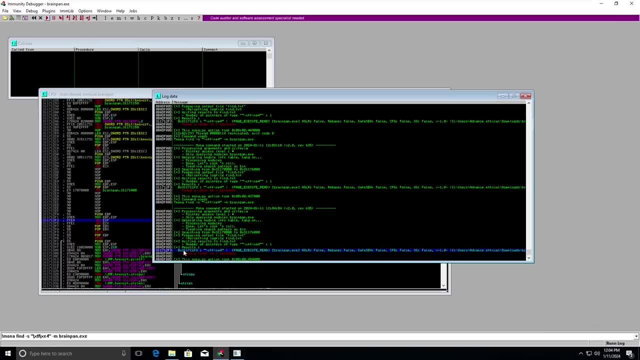 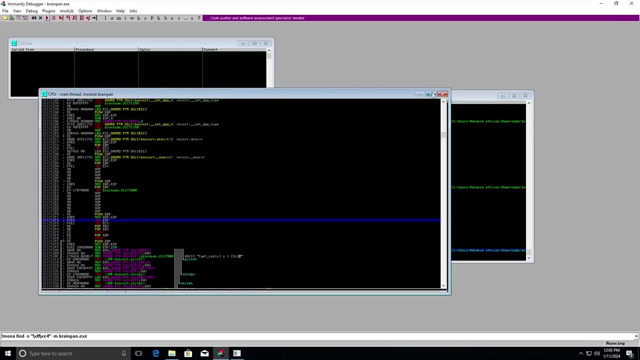 and right click and click on copy to clipboard and select address here. basically, I am copying the address here. you can also double click it and it will redirect to here. okay, but simple, just copy it. okay, it's a not a big deal, a full screen, this one. now here you can able to see this one, which is a enter. 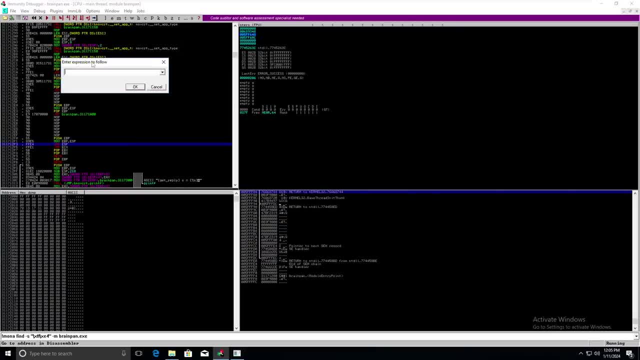 expression to follow, which is in blue color: simple: just paste that value there- okay, this value. and click OK there. here you can able to see the value, which is 3 1 1, 7, 1 2 f3. I can able to see it here, which is: jump ESP, right, oh, if you are not getting it, no. 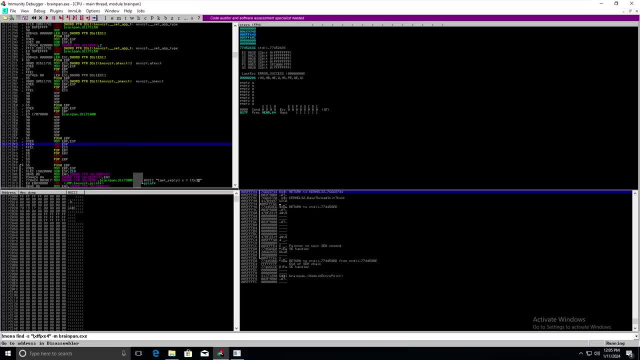 need to worry, just follow me. that's it. basically, the thing is I this video. the challenge is: I need to add this address to EIP. is the thing? see what is that address? it's 3 1, 1, 7, 1, 2, f3. 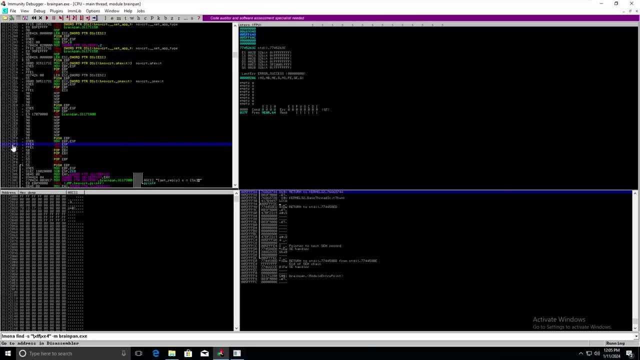 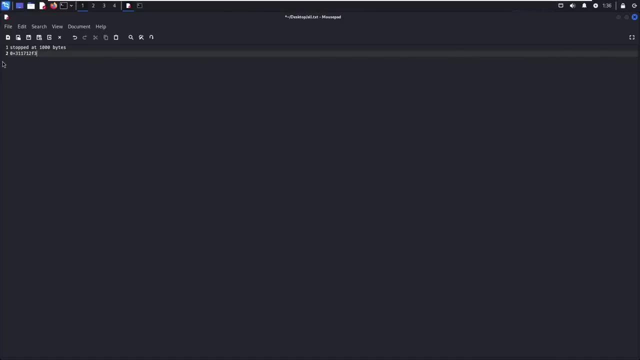 you need. the aim is in this video. I need to see this address in EIP here, okay. so to do that, we need to modify the exploit here. okay, which is first dot P, why I can't able to paste it from here to here. let me see. 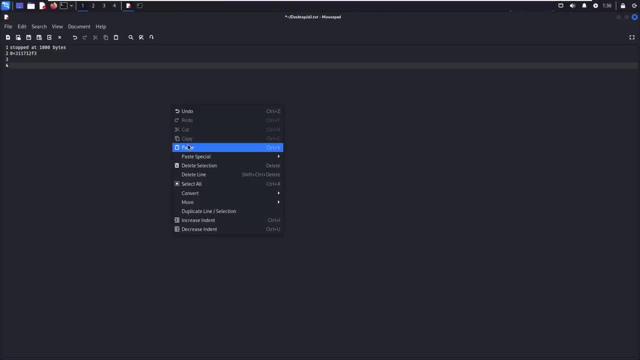 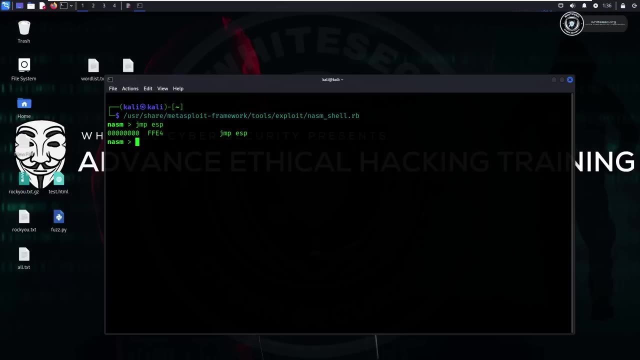 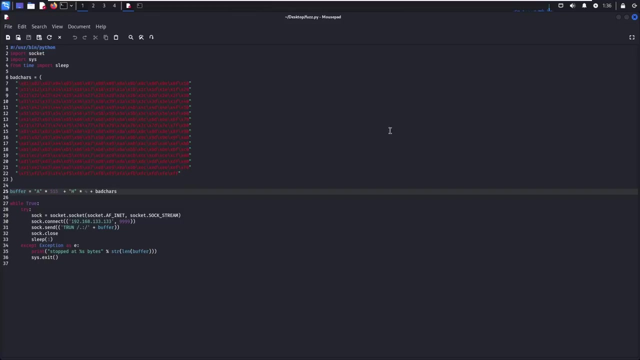 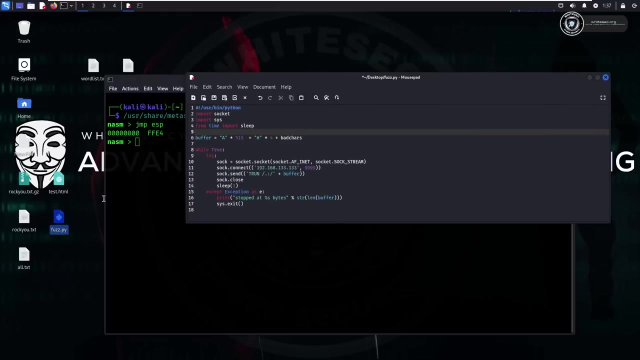 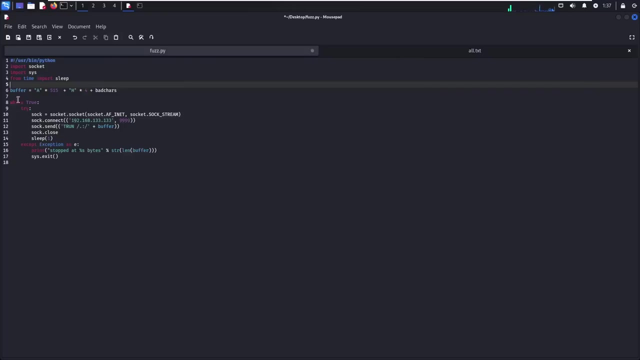 I can. it is a value. you me this. this one is first dot, P, Y. basically it's exploit. okay, just do one thing: just remove this bad characters from here. in no need bad characters now. also add this values in reverse order: this one, copy it, I paste it here. I can able to explain how we can. we can able to do it. okay now just 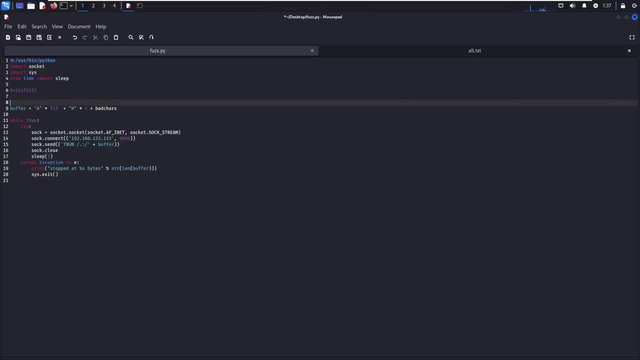 do any variable name here? let me do: reverse is equal now. see, just add double quotes. see, just add this one here. backward slashes. basically we are writing in hex format, right, so just just type a X and here unit it is a F, is all letter. okay, simple, you just need to. 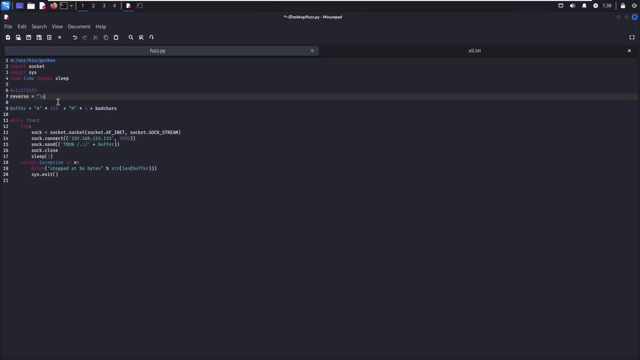 write it as a capital F, then just type here three and basically we are going to reverse here. just see the value, how it's look like. okay, the Shard again bad X here. and what is the next value is to work. just add here 1, 2, then again backward slash, it'll be 2, 222.. 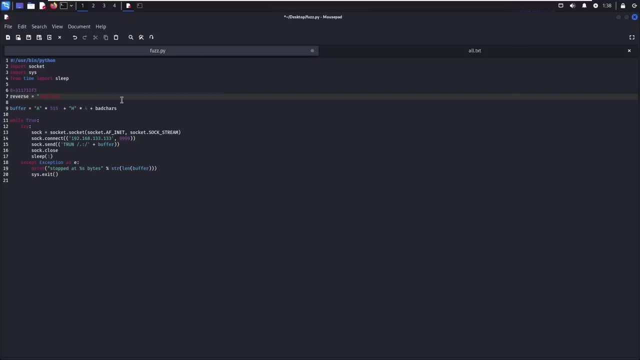 and what is the next value? it's too well, just add here 1, 2. then again backward slash: it'll be 2, 223.. then again backward slash: it'll be 2, 222.. x. what is the another value? it's a 17. now just type here 17. now again backward slash. 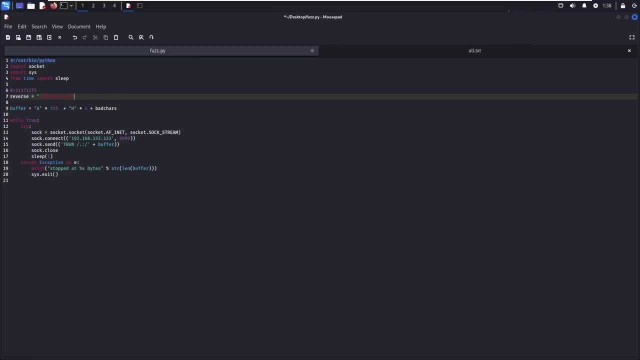 and sorry guys, it's a 31. just type here x 31, right and double click put it and close this one. okay, also, let me remove this bad characters as well from here, because we just removed that one and instead of this, just remove this h. just add the reverse here. we are using variable here, reverse, right. 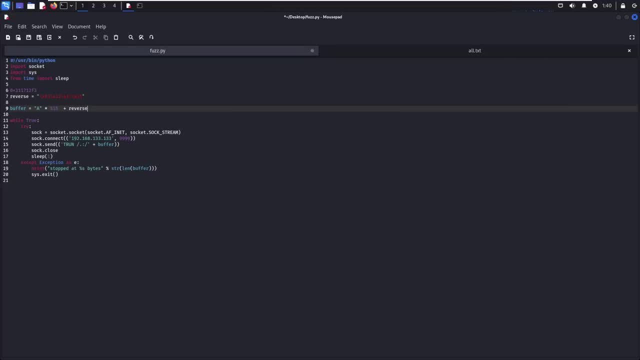 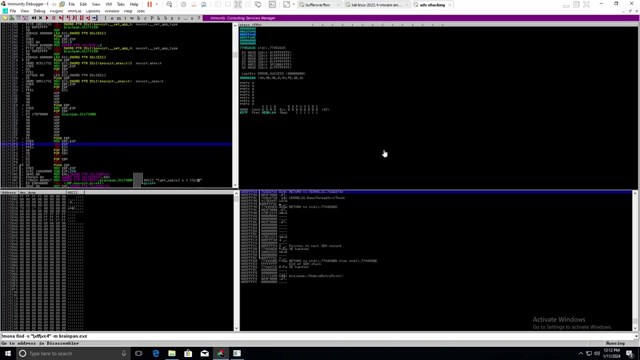 like this: close it back here. so basically, we need to add a breakpoint here. let's do the process again simple: click on one and just paste the address there and click ok. here you can able to see the value right, which jump e sp, simple. let's add a breakpoint here. 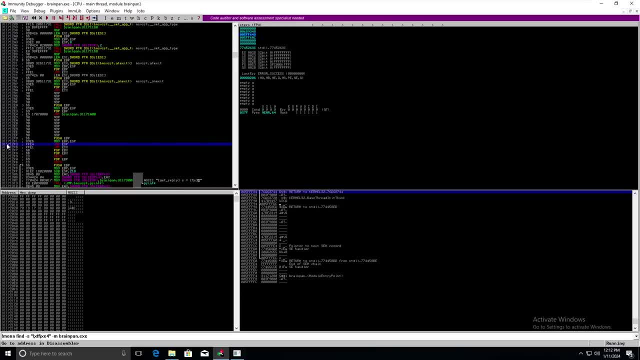 you can also, let's say, type F2 there, right, simple, here there is a breakpoint and toggle type here and it successfully. we just added the breakpoint, right. that means whenever this value will trigger. at that time what will happen means the software will get. so here we just added the breakpoint, right. 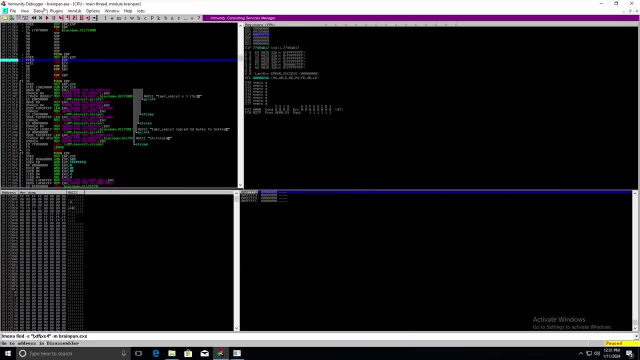 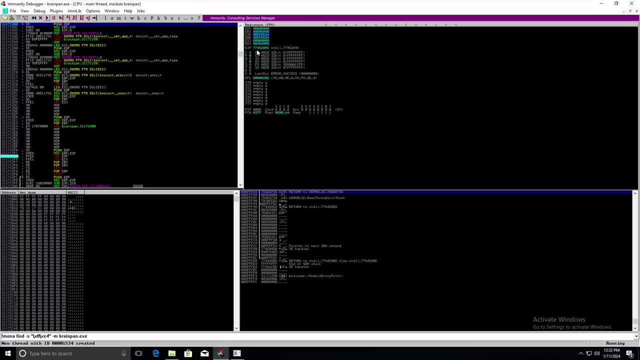 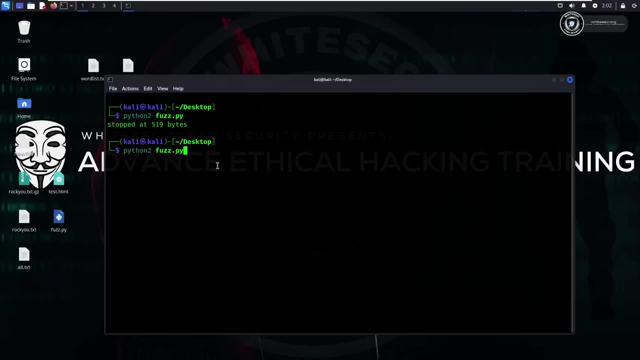 play this one. now the software is running. here you can able to see the EAP is 7745289C. basically, now we let me run this one. okay, python2 first, dot py now. here you can able to see: now the EAP is pointing to which address that jump ESP address, just see. 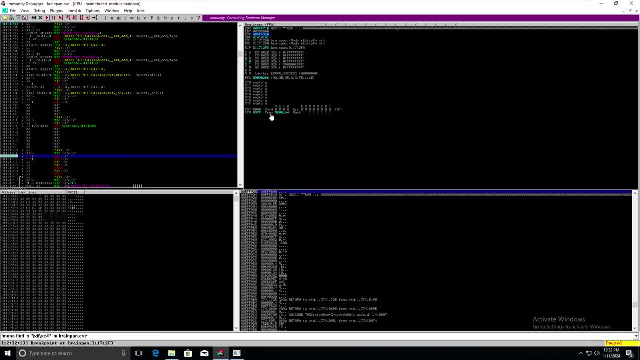 see the EAP. now it's changed to that address. okay, we just given the breakpoint, right. so this is the thing. basically it's pointing to that given address here. so hope you guys get it. it is a very easy process, just try to practice it. that's it because why it's giving the EAP here? because in this first 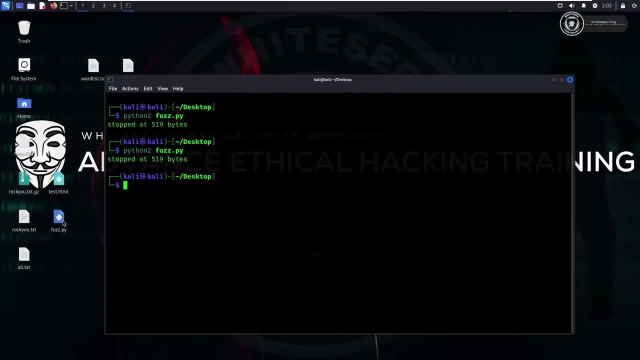 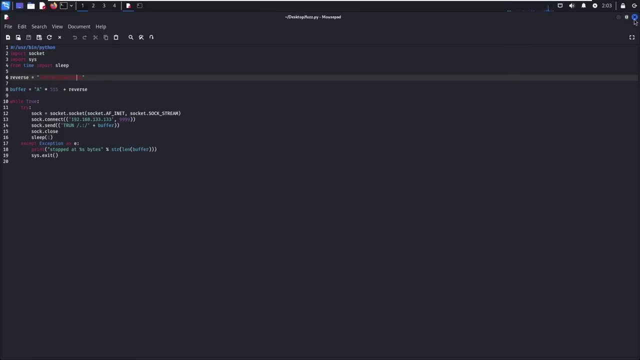 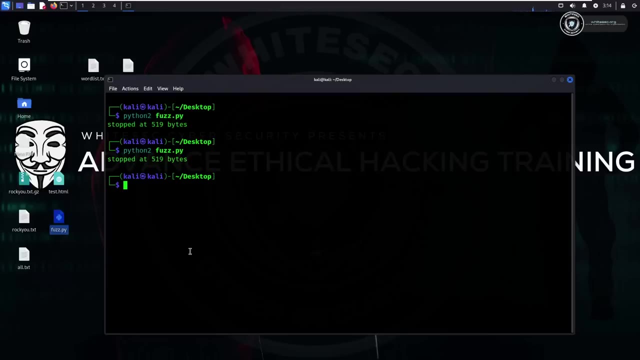 dot py, we given the value in hex format, right. so that's why this is the thing: let's generate a shell. so to generate a shell, we will use msf, enum, dash, p, close shell. let's go reverse. let's go reverse for post Kali IP. 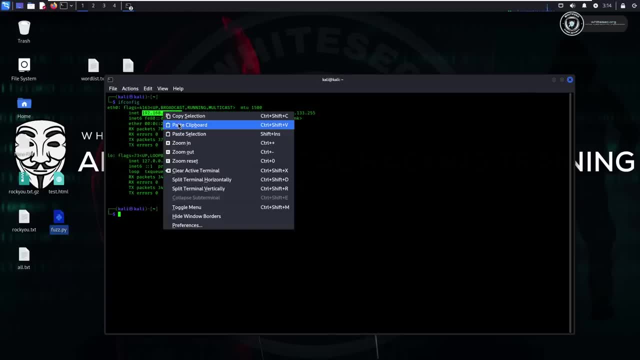 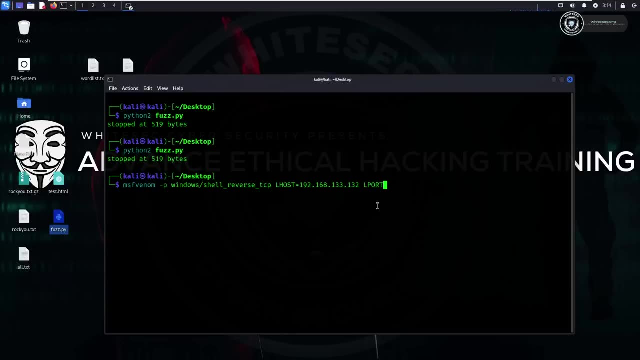 use the l-port as 0.455 file and let me just type the x to try and get it there. generate this format of c language and let me use the architecture you can also, uh, my windows system totally depend upon. let me use architecture of x86. see, i just uh, if you watch the windows. 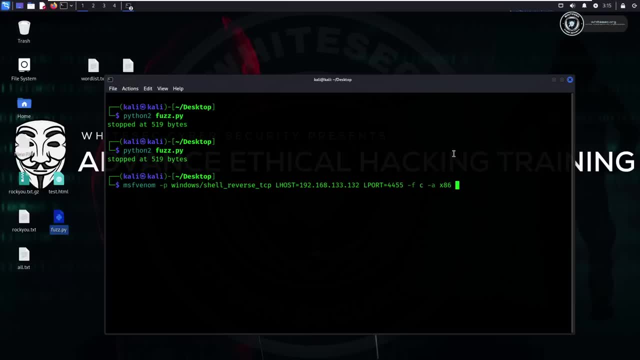 penetration, testing planning, then you will get it. what is a x86 and what is the use of the x86? okay, if we generate the payload in x86, then what are the advantages there? okay, there are that one advantages, right? so here you want to add bad characters here? you can just type here dash b, okay, and just add the bad characters here. 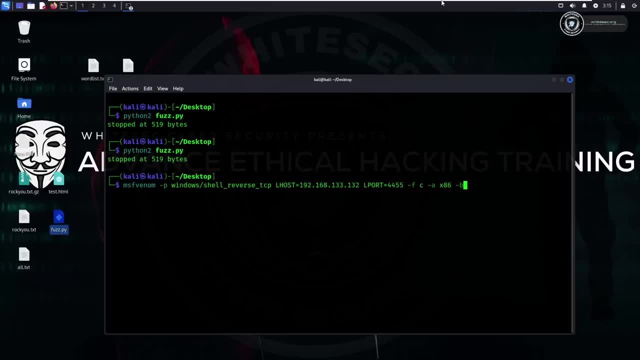 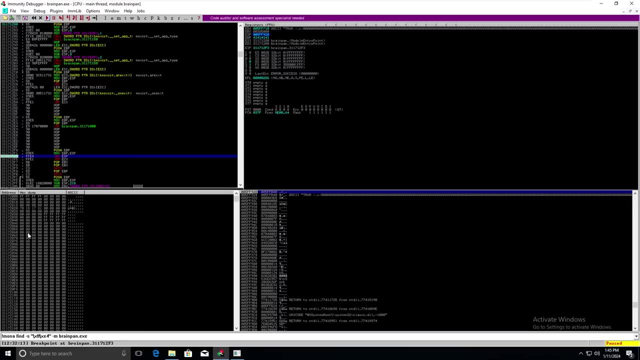 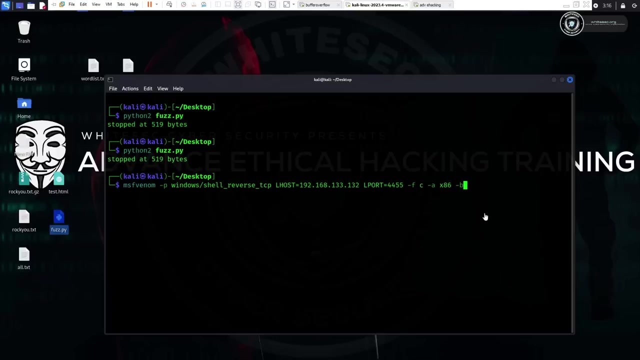 simple see how you can able to add the bad characters here. simple in the last is: uh, that bad characters are not matching here at that time. select that characters and simple add it here. okay, this is the thing. simple, just add double quote. see what is the universal bad. 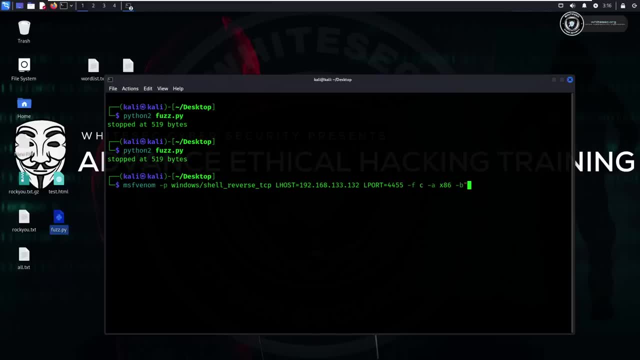 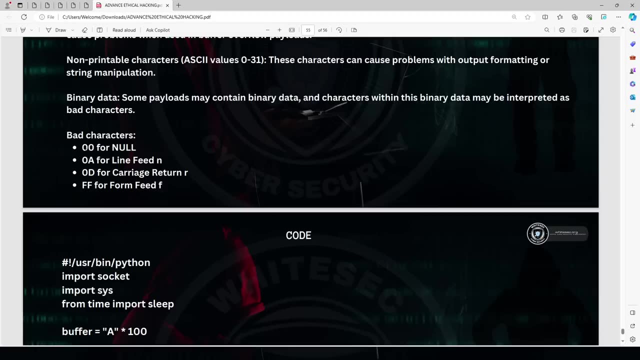 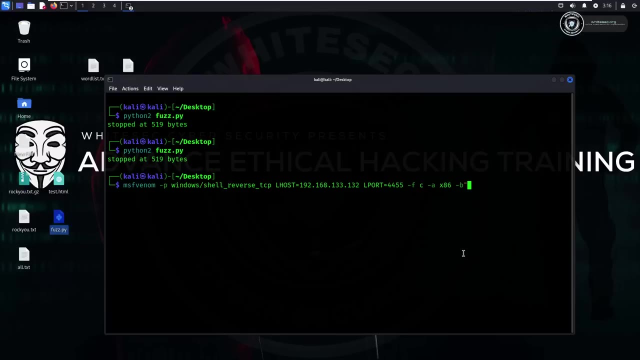 character here. you can also say it as a null zero. zero is the universal bad character. okay, v, v, 0 a. 0, 0, 0 a 0, d. okay, what these things are? universal bad character. simple, you see these characters there in your program at the time. uh, if you see those characters here at the time, what will have? 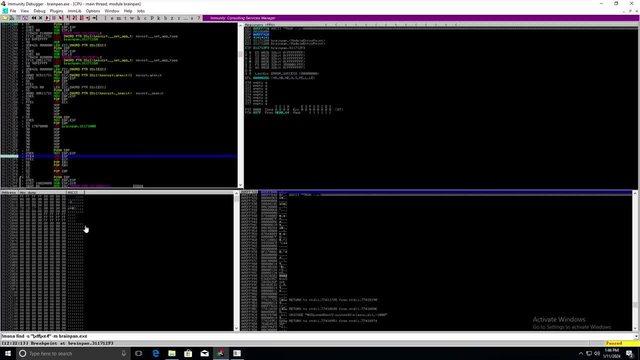 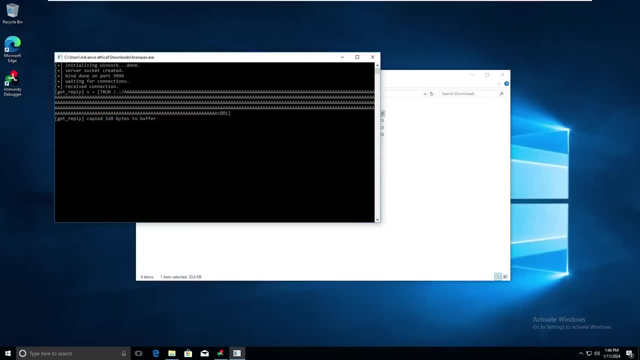 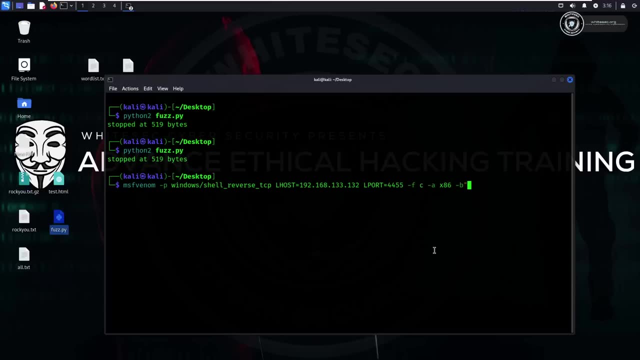 in dump. okay, this, see here. then just, it's a bad characters. okay, remember this thing. now let me use 0- 0 here. you need to use something like this thing: x 0, 0 double code. let me save the name of shell so it's generated. 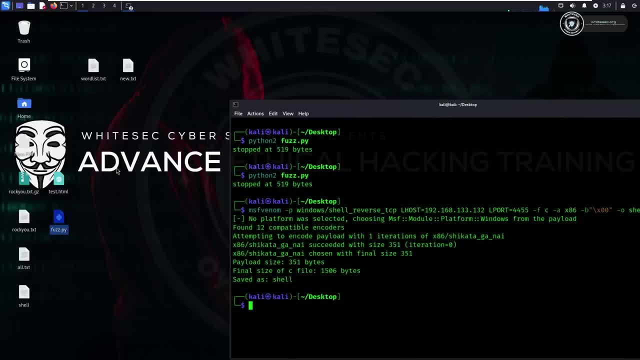 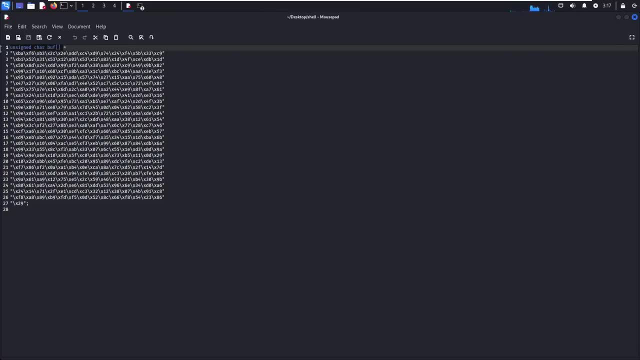 stop here. it is hope you guys can able, right, do one thing: just remove of unsigned characters buffer. just remove it. also remove this. see well, here, right, also remove the semicolon from here. just close with double brackets here. just start with packet and just add this in packet. okay, 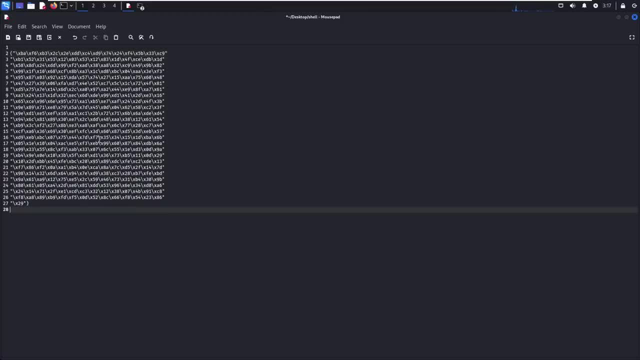 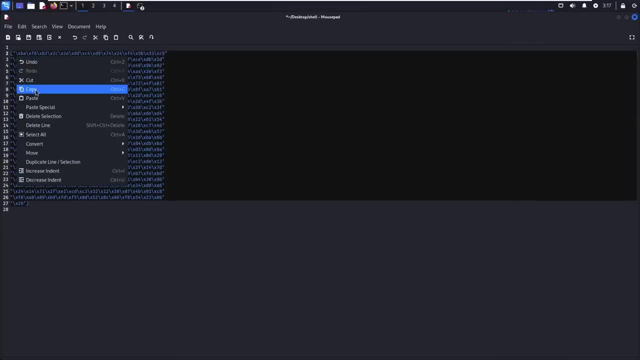 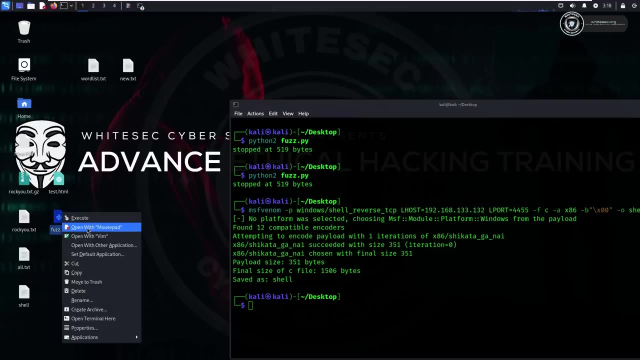 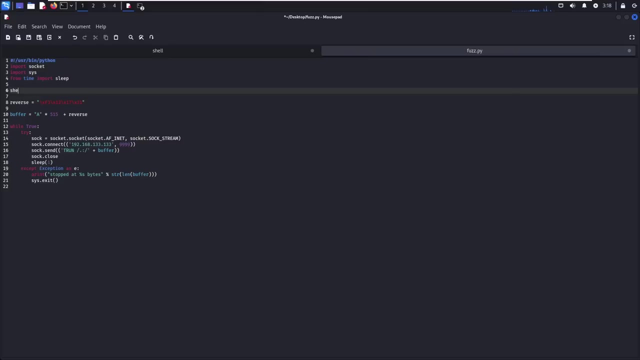 so it's look like: copy this. see, instead of using the bad characters, what we are using there: simple the shell here. now do one thing: just create one variable here, just add: let me create the variable with the name of shell- just type is equal here- and paste that how. 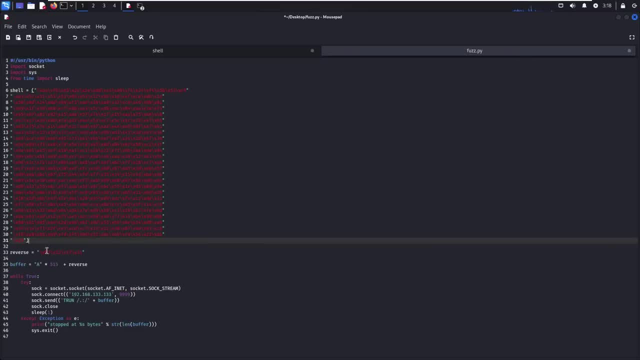 it's look like: see, here there is a reverse. we just added like this: now simple, just add plus and add this one as well, this variable shell. let me tell you here you can, you need to add the space as well between this thing, in between shell and reverse and shell. you. 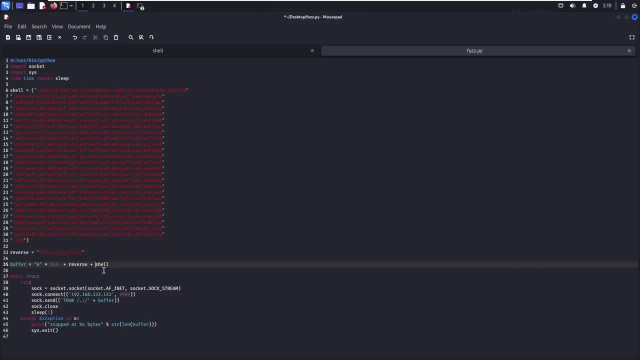 need to give some spaces. how you can able to give it simple: just do one thing, add here something like this: okay, double quote: just add x 90, close it. now let me generate. it's a kind of enter. okay, like see, assume that here you enter. right, how it's gonna work you. 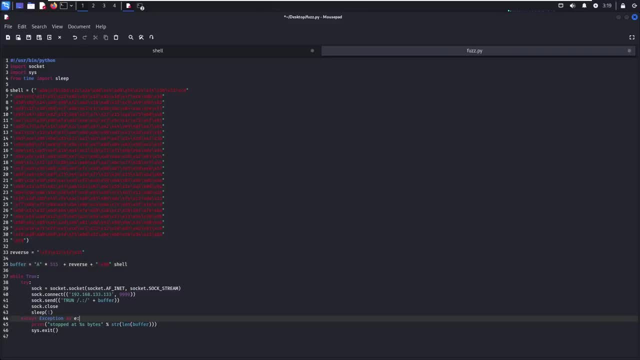 will see it. just wait, let me generate this spaces, like. generate 16 spaces here. double quote: just add 16 spaces here. you can explain. you don't worry this. add plus here because I am generating in between of reverse and shell. what is the reverse here? reverse is: 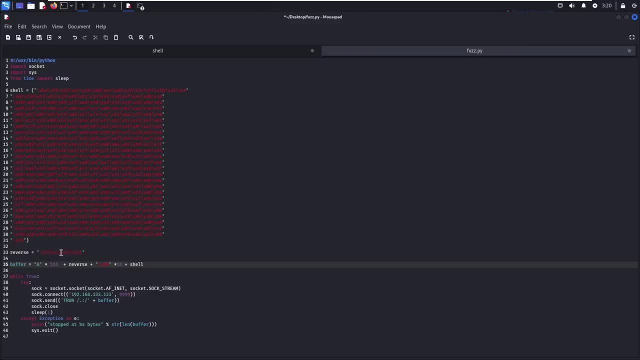 our this one, this value which we just got from jump esp right, and in this is a shell in between these values. what we are doing we are adding some spaces here, like 16, kind of spaces like this. man see, here it will work like this. we will add kind of spaces here like enters, like 16 times, okay, and then it. 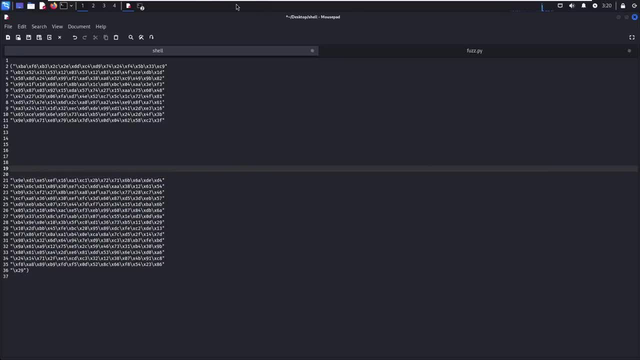 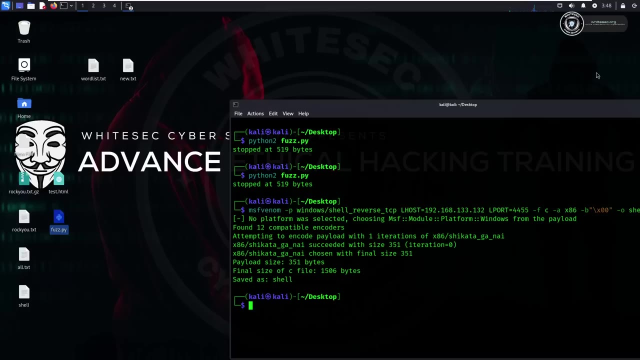 will execute the payload there. the thing: it's not a big deal, right, you need to worry about this. just do practice, you will get here. we successfully developed the exploit. the thing is here, let's exploit it. okay, let's exploit this windows 10 machine. then we will exploit the this machine as well. brain pan. now let me remove. 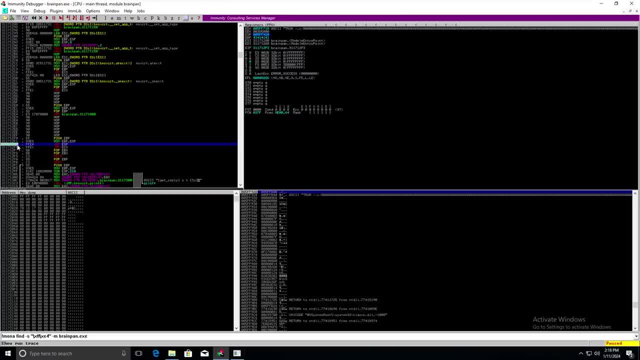 this breakpoint from here, because in real world you can't able to do it right. so basically what we did here, we just assume that first of all, let me exploit it, then I am gonna explain you about the real world scenarios as well, like what we can able to achieve this by using: 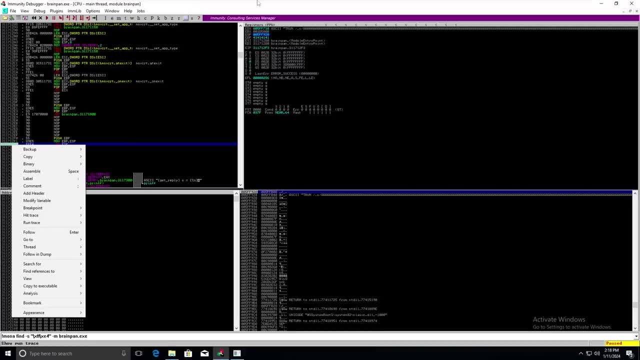 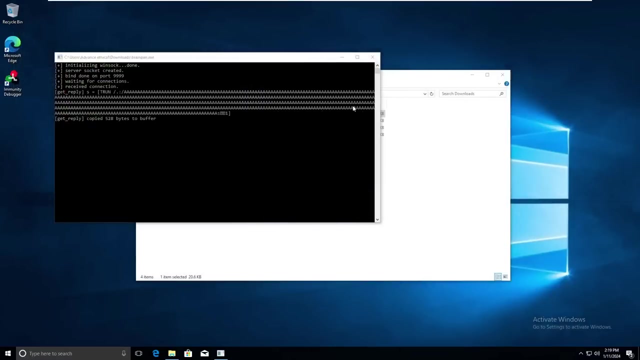 this exploit. okay, now, if you type here the brain pan the break or type here f2 breakpoint will be removed. okay, I just removed the breakpoint from here from jump esp. right now, let me do one thing: let me close this immunity debugger as well. yeah, now assume that in this machine the brain pan is running, this ex is running here and 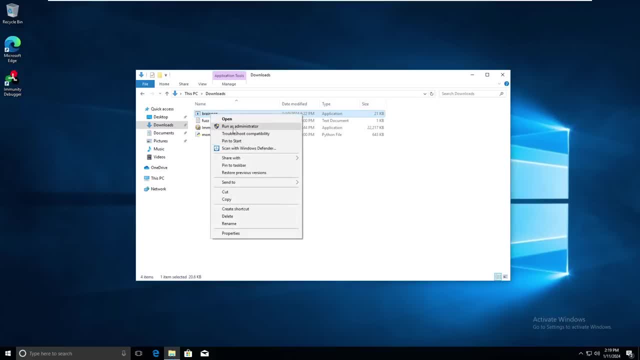 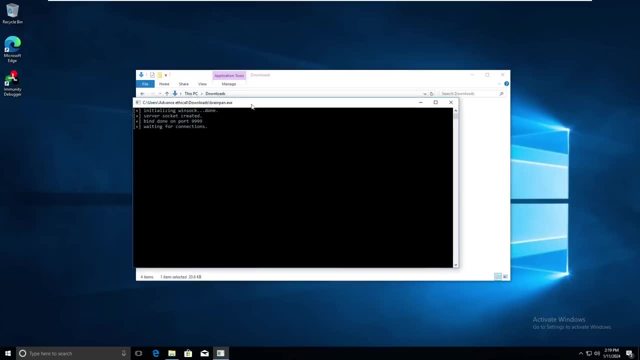 I can easily use this exploit on this main path. okay, just assume that this is a service like a FTP or something like that, a service which is running in server right now. here, let's go back in our attacker machine. what we will do is: here. we won't send any kind. 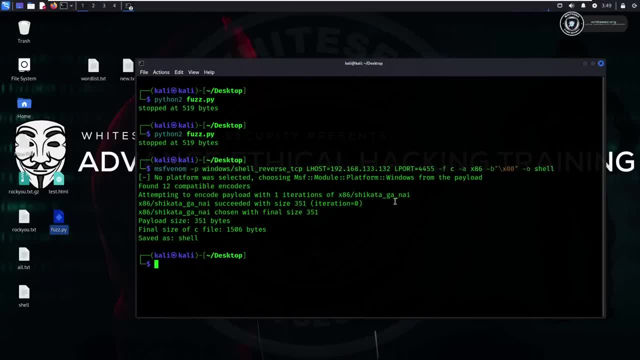 of shell simple. we will use this exploit, like what I am trying to say, means I no need to send any kind of phishing email, something like that simple. by having that my target IP, I can able to hack in. this is the thing. again, I'm saying it's not a big deal okay. 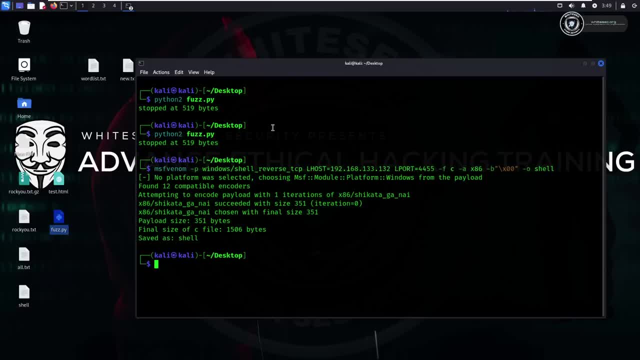 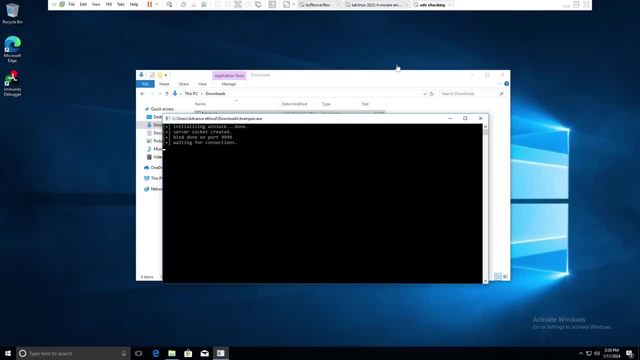 let's go back in our attacker machine and what we will do is here. we won't send any. and again i am saying i no need to send any kind of attachment or something like that simple in in this case, what we need, we just need our target ip address. that's it. okay, the same. 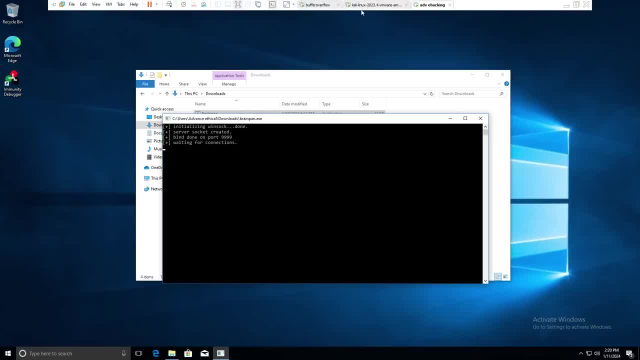 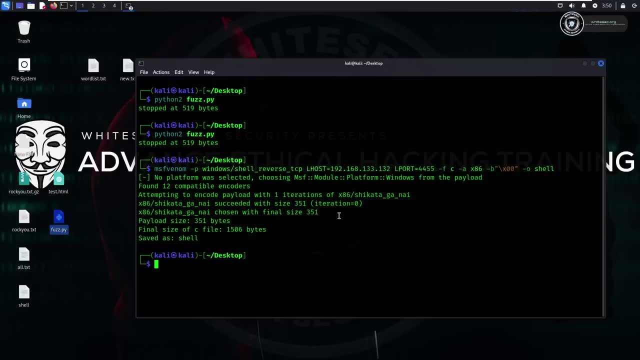 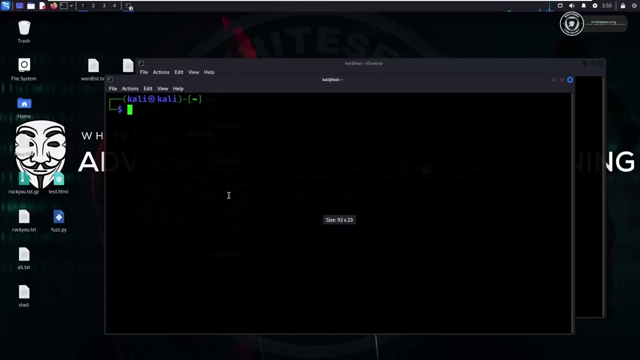 like it, eternal blue vulnerability. okay, in eternal blue also, what we need? we simply we need the target ip there, that's it. okay, now here, just remember the port. here, the port which we are using is double four, double five. let me you open one new terminal. let me use netcat here to listen for the connection. just type here: netcat. 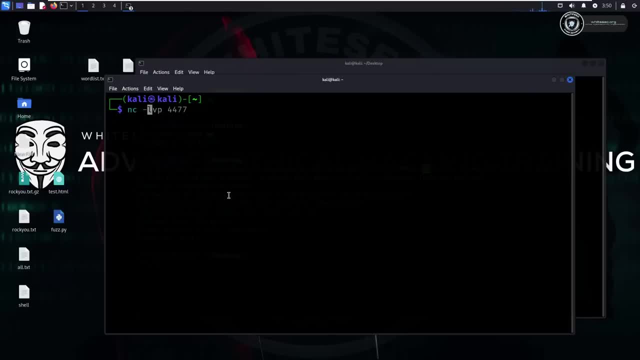 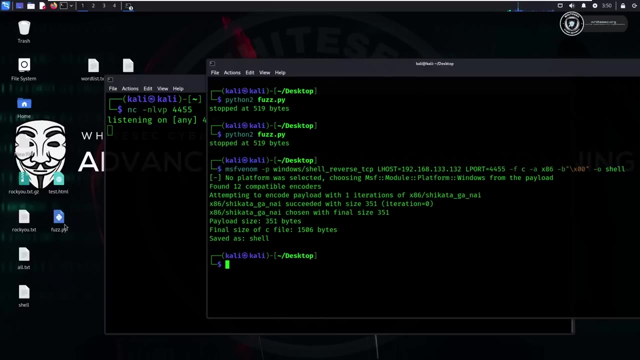 dash nlvp and what is the port? let me listen on port. double four, double five. okay, now simple. just type enter. right now, let's uh run this first dot py here. just type here dot forward. sorry, this is a exploit. simple. let me run python 2 first, dot py. see, i got the shell here, right this? 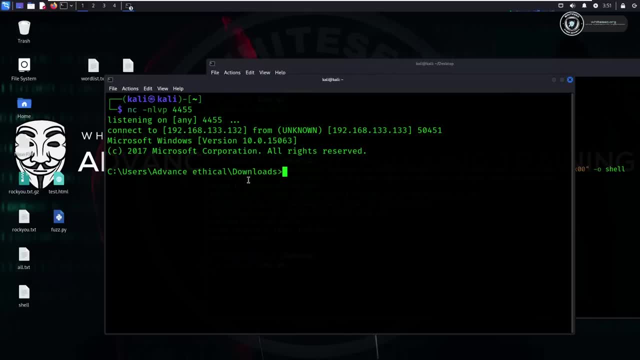 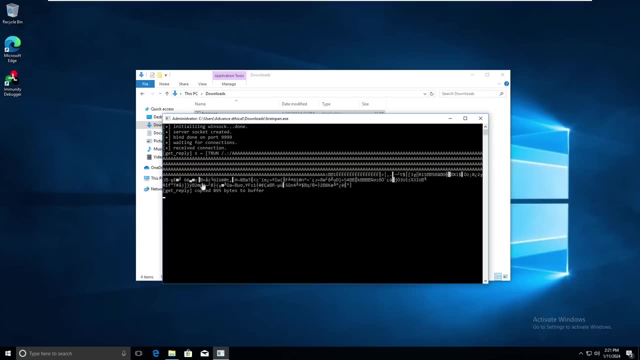 is the thing. i didn't send any kind of payload, nothing, simple by exploiting the vulnerability in this service. basically, i got the shell there. now just assume if any system run this brainpanexe in their computer system, like in windows, linux, then what will happen? i can able to exploit it. 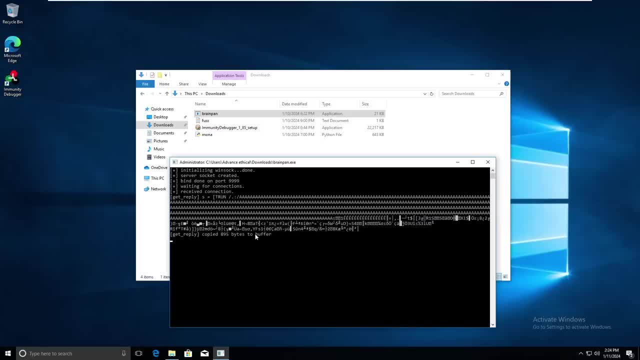 okay, i can able to exploit those systems without sending any kind of attachments. like i don't need to perform any kind of social engineering there. simple, i just need those guys ip address right. simple, i can use this exploit here which i just developed. simple, i'm gonna run it and. 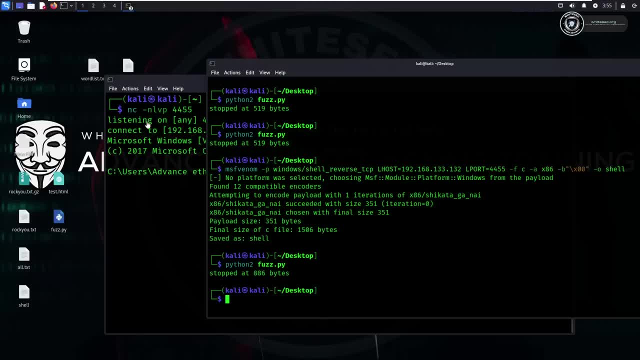 i'm gonna listen for the port simple. i will get the connection there. that's it, a simple thing, okay. again, i am saying this section is basic. okay, there is a lot. okay, you can't even image that i can imagine. okay, how excellent this uh field is, this exploit development field, but you will get a huge 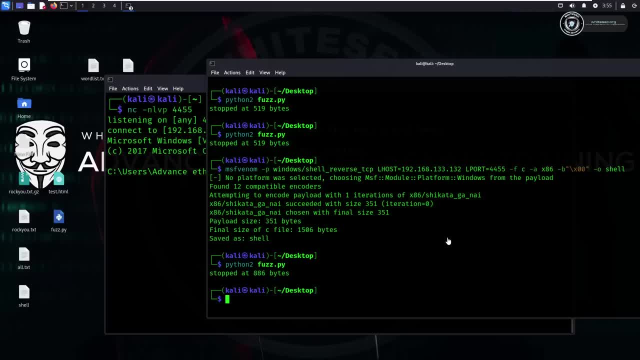 amount of headache. just i am. i'm telling each and everything, okay, like i don't want to hide. simply, you will get a huge amount of headache here and also you will- uh, if you learn this- exploit development, then you will earn a huge money. okay, legally as well. okay, 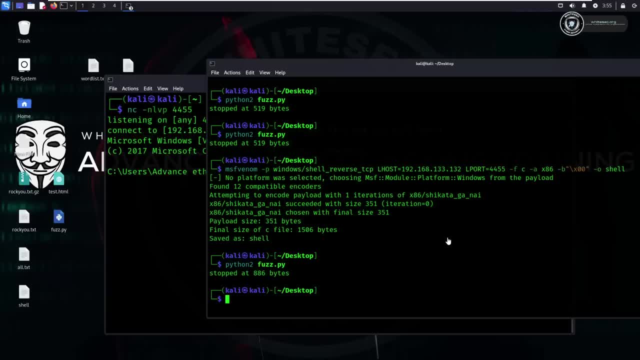 we are talking legally, right. okay. now what is illegal here? so just let me tell you about zero-day exploits. okay, what will happen in zero-day exploit? it's a six day split. try that. write here: cheers, not that much thing. okay, basically in whole world. okay, just assume that there is a ssh, is there? 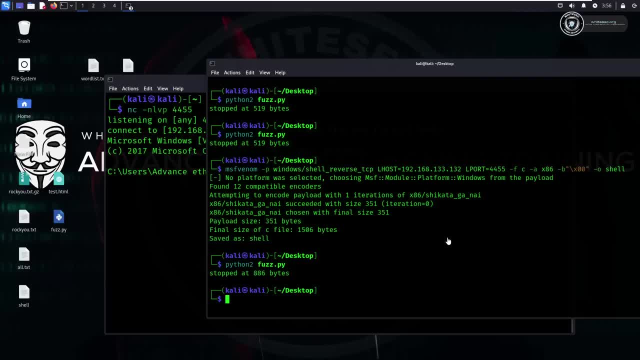 every system- mostly every system- use the ssh service there. okay, assume that i just found the vulnerability in that ssh service at that time. what will happen? if any system run that ssh service, i can able to exploit it. okay, without sending any kind of payload, i just need the ip. 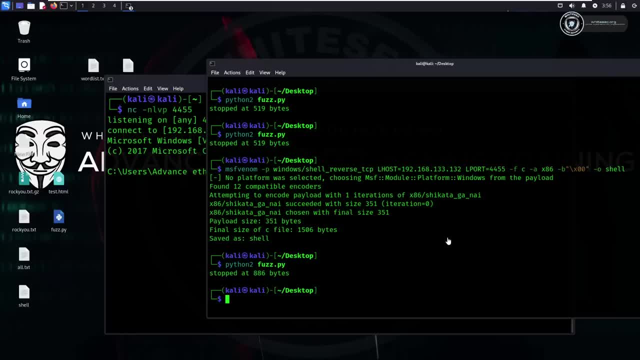 address of that system, i can able to exploit it. okay, this is the thing now in the whole world. okay, no one knows, know about that. uh, vulnerability, you are the only guy who just found it and you are using, and you are using it okay, and due to some reasons you just shared with someone and 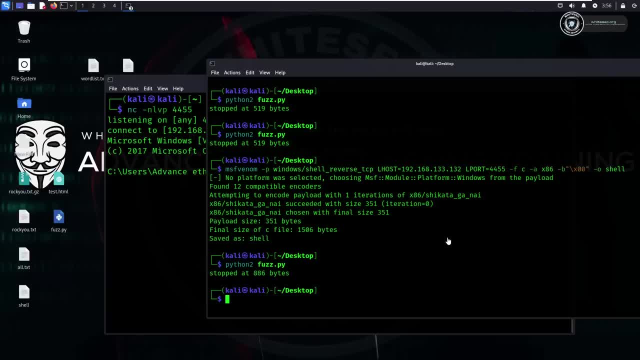 you just sold it okay, then what will happen? it will known as a zero day. okay. again, i am saying: no one knows. in whole world, no one knows that, uh, there is a kind of vulnerability, is there? if you leak that vulnerability or the hackers will sold it okay, like in dark web, they, they just 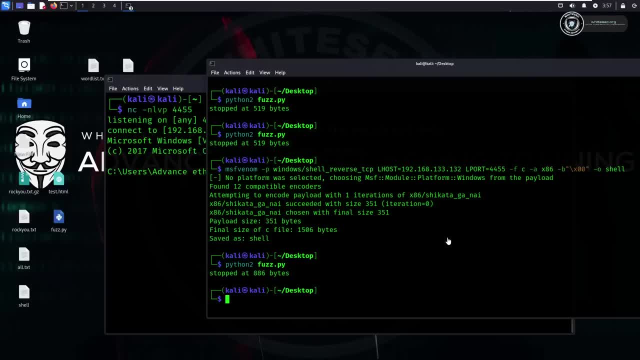 you will see a lot of things like zero day has been leaked. zero day is there, okay something? we will see that in daily news- yes, okay, uh. zero day is there for ssh or ftp or something like that. simple, this is the things. if they leak, then it's known as a zero day. this is the thing, right, hope you guys. 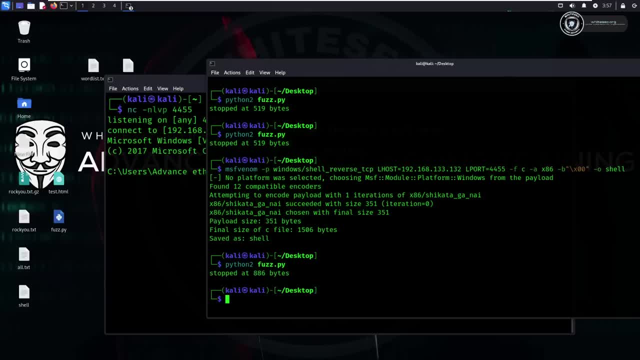 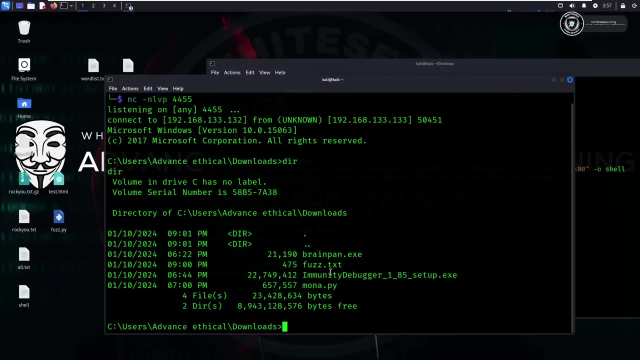 get it again. i am saying it's just a basic thing. okay, don't think that you just learn a lot here it's a basic. again i am saying now, here i got the shell, here i got the shell, here i got the shell. you can see theseactualitv folder. here again, this is the 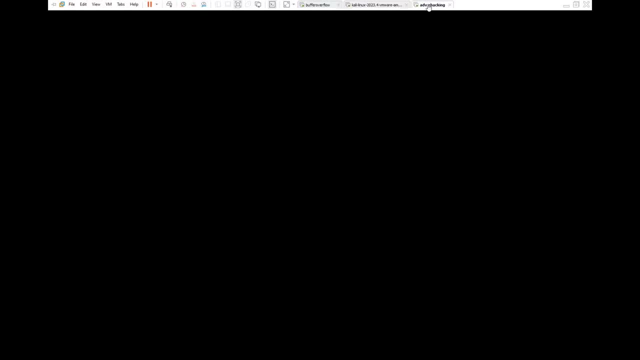 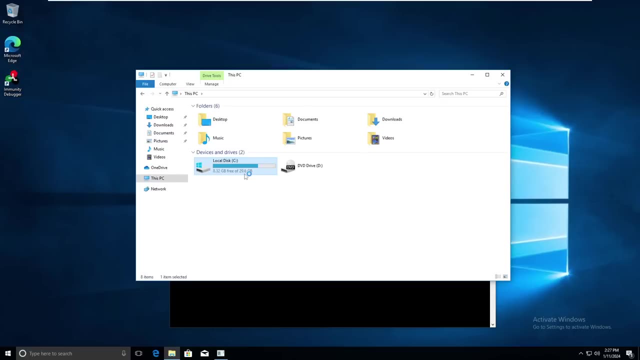 ändernmentрав if i type here d i r then i can able to see brand band dot e x e each and everything if i type here c caused trans � USA 唔 work because this is a windows system see if i type ls herebels won't work because this is a windows system 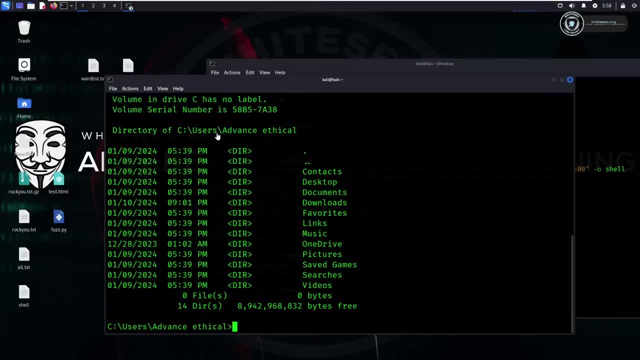 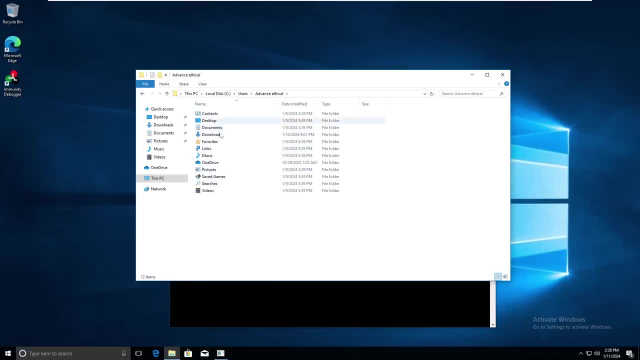 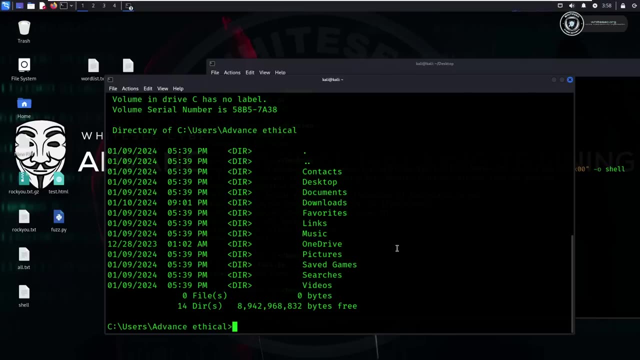 see, here there is a Hom Fehler D friends download system at eye type: ls users advanced- ethical is advanced folder. see, i can able to do these things. okay, see, windows defender has been detected it. so the simple thing is: you, you need to be uh secured systems. okay, like uh, assume that you are using some outdated versions at that. 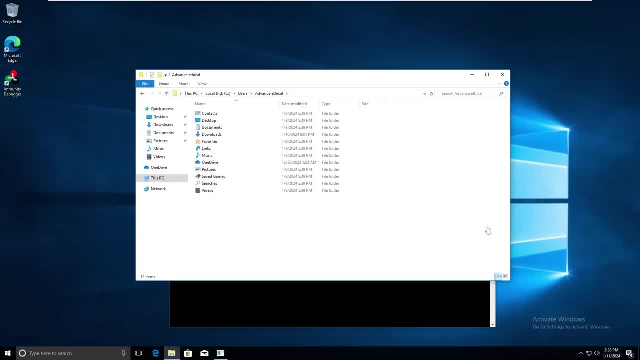 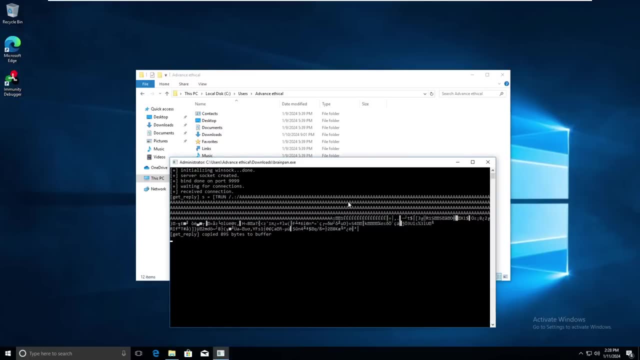 time, what will happen? the attackers can able to get. uh. assume that the, the outdated version is vulnerable. with this attacks. at the time, what will happen? the attacker can able to take control on your system, right, so that's uh. that's why what you need to do, you need to use a excellent antiviruses. 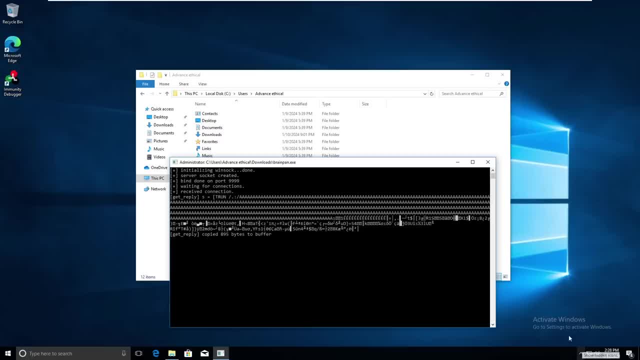 it is easy to bypass windows defender. okay, by by doing some techniques you guys can able to bypass it. but there are such antiviruses, are there? by using that you? uh, it is hard for us to buy. now. let's exploit this brain pan machine here. to exploit it. what? 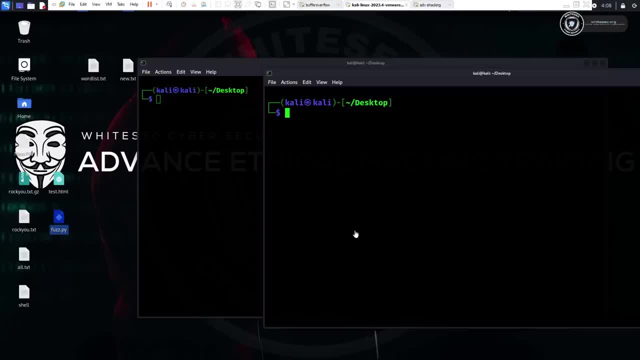 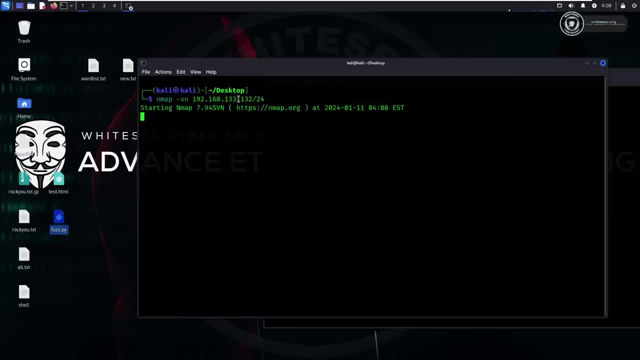 machine and forward slash 24 and from here you can able to see the ip address of your target machine. right, simple you need. what you need to do means just copy uh, your target we. we know that this is a brain pan ip because in the last classes also we did. 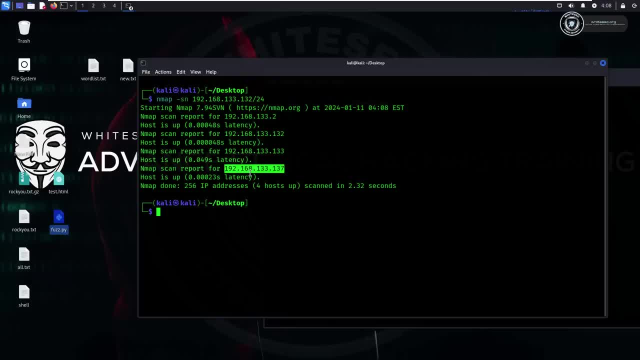 this all right by using dub. we just downloaded the brainpanexe, so that's why we have the idea. so this is the thing. if you don't have the idea, what you need to do, simple: just type here: nmap, dashes, capital v, and just see the open ports there and just perform the os detection as well. 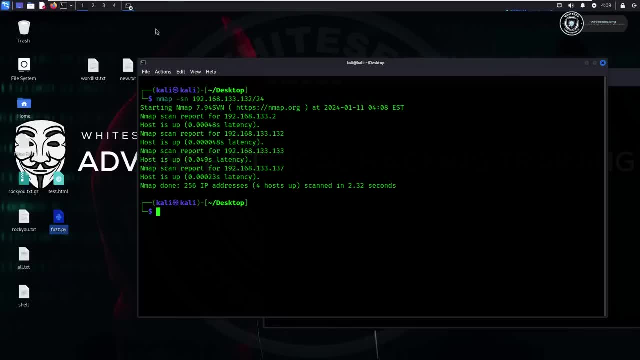 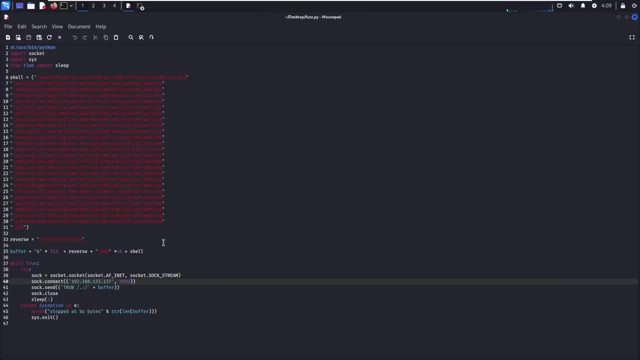 now here. let me copy this ip address. just focus here. see there is a first dot. py is here right. so in the last classes what we did means we just added here our windows ip address. okay, instead of adding the windows ip address now you need to add your brain pan ip address, because this is our. 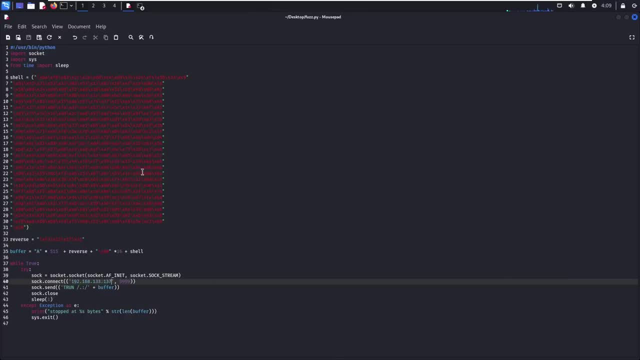 target, assume that this is a system which is vulnerable. at that time, what we need to do? we need, uh, we need- to add that system ip address here and save it. no need to change the port anything, because the service is using the port double nine, double nine there, okay, you no need.